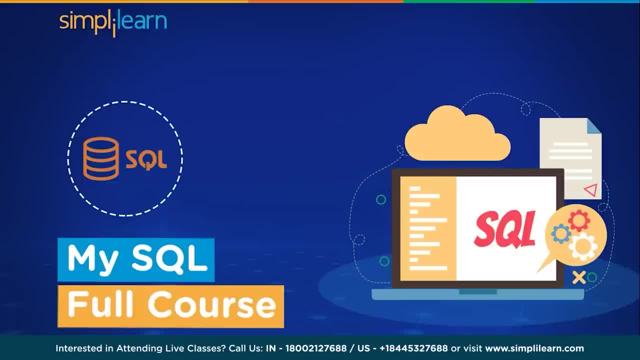 users. As more businesses move to the cloud, there is likely to be a greater demand for cloud-based MySQL deployment. This includes both MySQL as a service and running on cloud-based virtual machines, So learning MySQL can add great value to your array of skills. Now this MySQL full course. 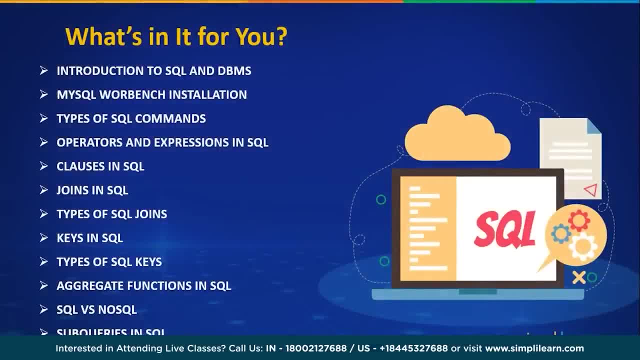 is designed to provide a comprehensive overview of MySQL database, covering everything from the basics of installation and understanding what is SQL and using various types of commands, operators, clauses, joins, to advanced topics like serverless storage procedures and triggers. So, whether you are new to MySQL or an experienced developer, 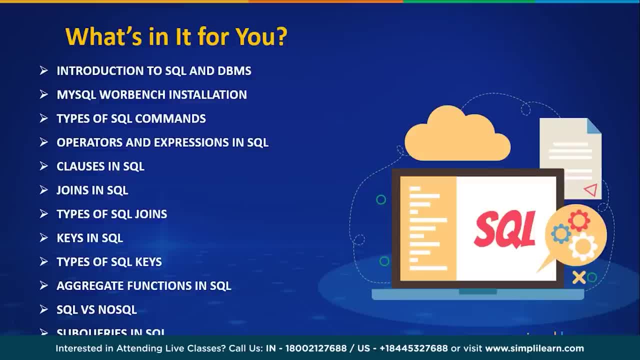 looking to expand your knowledge. this course will provide you with the foundational knowledge and practical skills that is needed to work with MySQL effectively. Throughout this course, you will learn how to create and manage MySQL databases, how to query and manipulate data using SQL statements, and how to optimize performance using indexes and other techniques. So, without any further ado, let's. 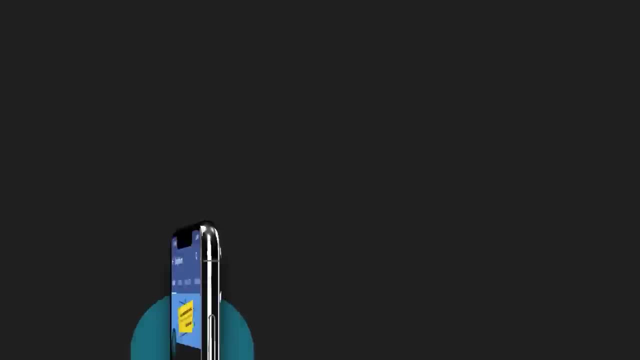 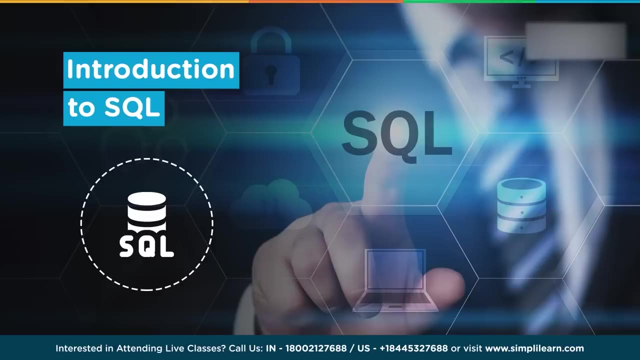 get started With today's session over to our training experts and I welcome you all to this interesting session, or introduction to SQL. Learning SQL isn't an uphill task because, unlike other programming languages, SQL is quite simple and uses common English words in its usage. 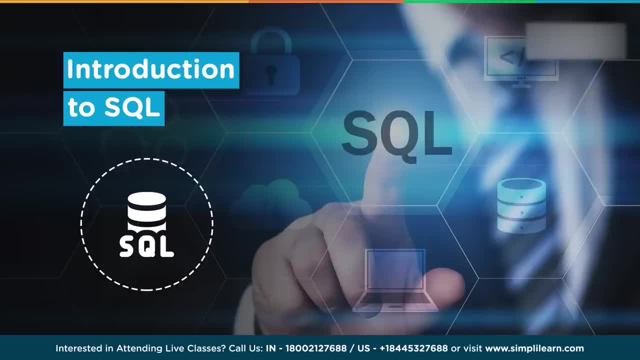 Even a non-technical professional with no prior experience in programming can easily learn and understand it. According to a survey by stackoverflow in 2020, SQL ranked as the 3rd most used programming language. Also, every 9 out of 10 companies in the world uses SQL. 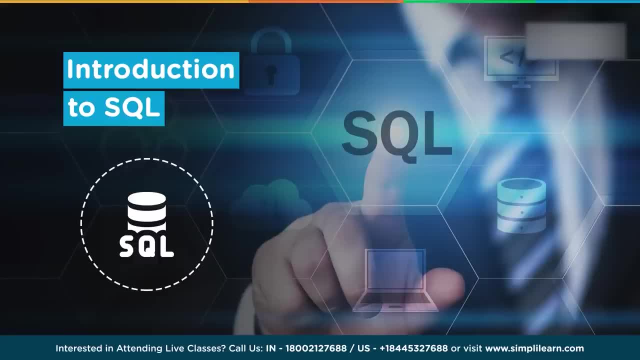 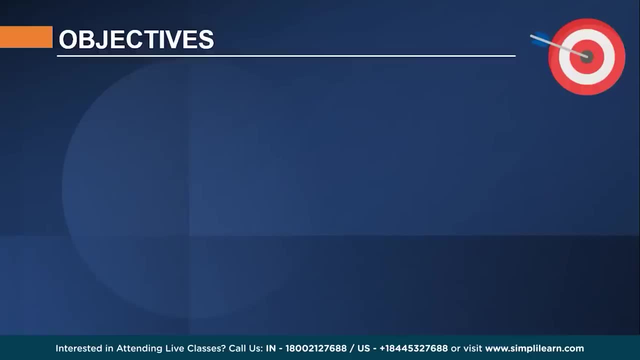 So, without any further ado, let us dive straight into today's topic on introduction to SQL. Firstly, let us discuss the agenda for today's session. We will start this tutorial by understanding what a database is and look at some popular databases to understand the need for databases. 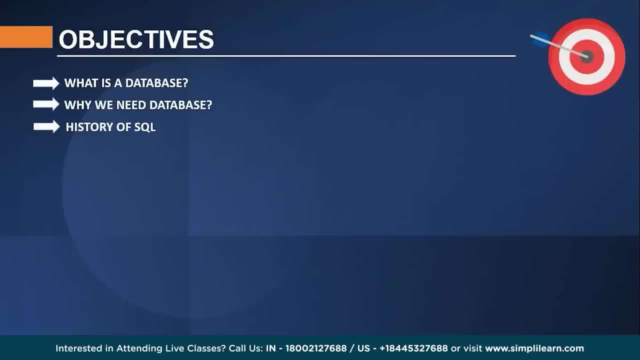 Next we will understand the need for databases. After that we'll look at the evolution of SQL and how it grew over the years. Then we'll discuss what exactly is SQL, followed by some of its unique features. Next we'll go through the working of SQL, types of SQL commands. 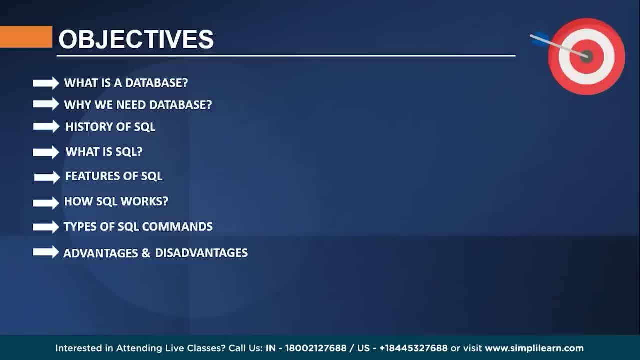 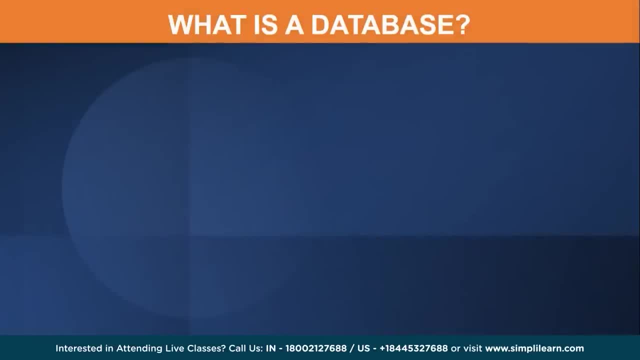 Towards the end. we'll discuss the advantages and disadvantages of SQL And, finally, we'll see some applications of SQL in real life. What is a database? Data in today's world plays a vital role in our everyday lives, be it your work-related. 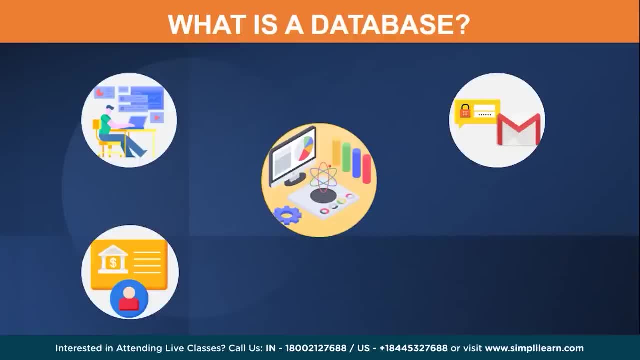 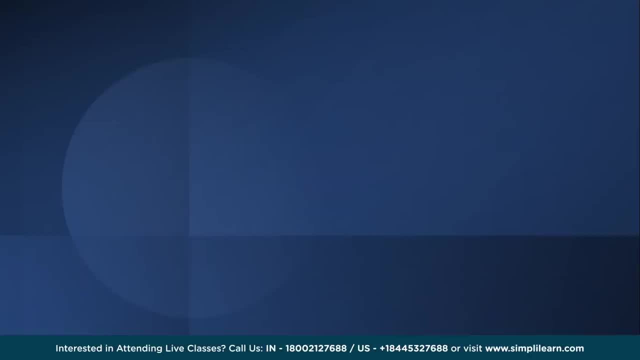 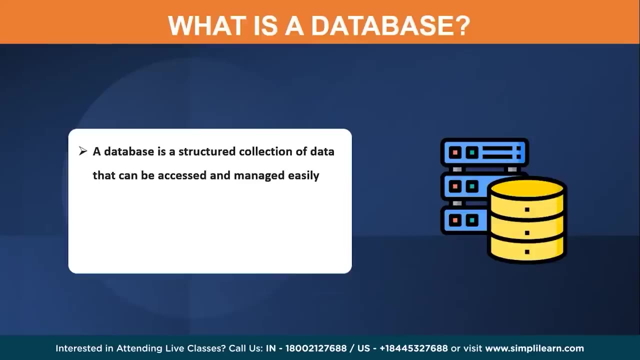 data in your laptop, your bank account details or even your Gmail password, So it's necessary to store this data safely and in an organized way. That's where database comes into picture, which holds and manages the data. A database can be defined as a collection of information or processed data that can 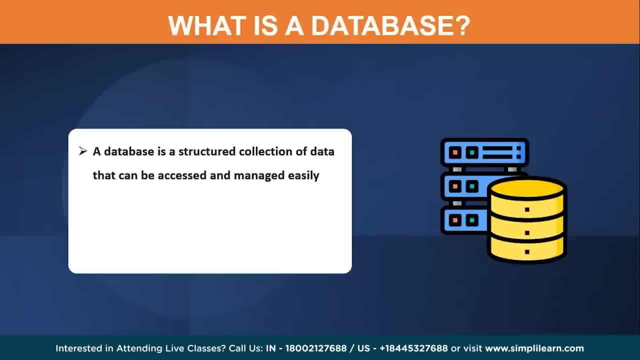 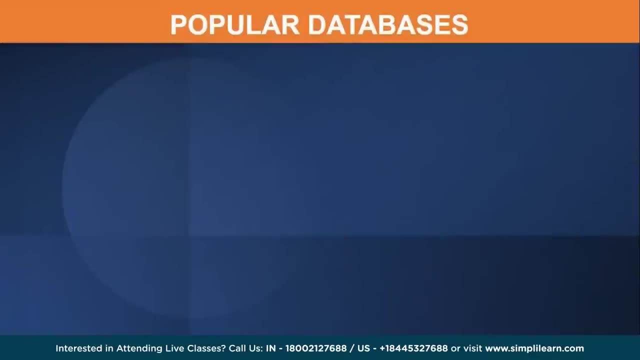 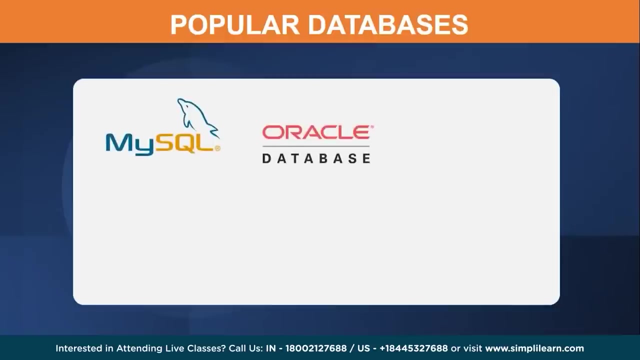 be stored and accessed whenever needed. For example, We can use a database to store the complete details of an employee working in an organization. The primary goal of a database is to store and retrieve information efficiently. Popular databases: Some popular open-source and commercially available databases are MySQL, Oracle Database, Microsoft SQL Server, MongoDB and PostgreSQL. 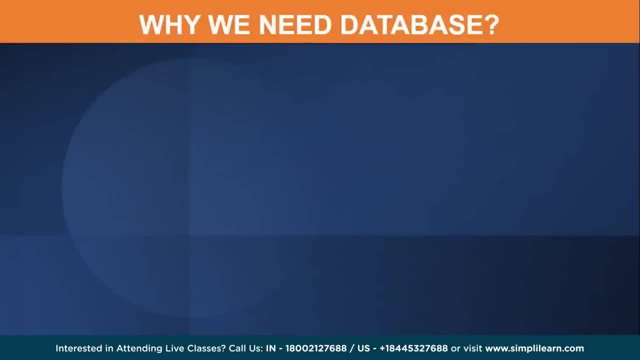 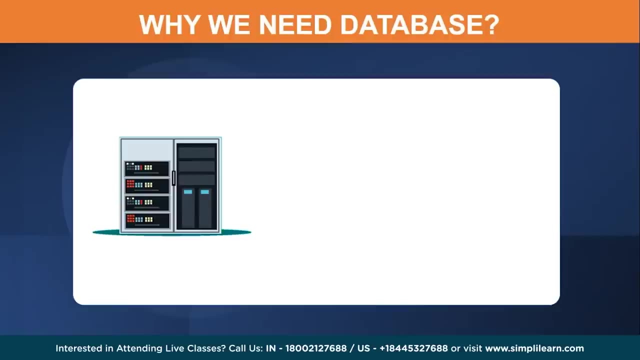 Why we need a database. Now that we've understood what a database is, let's understand the use of a database and the need for it. Database came into existence in the early 1970s, But all the data was stored in computer files before that. 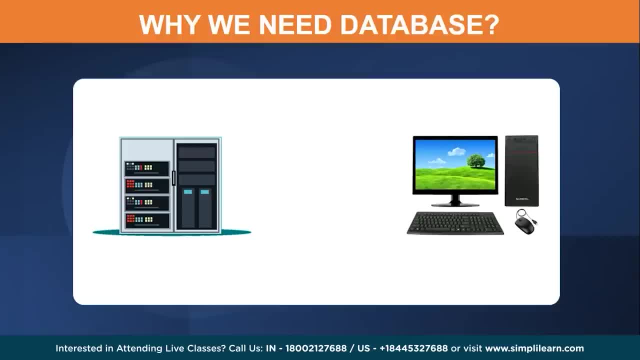 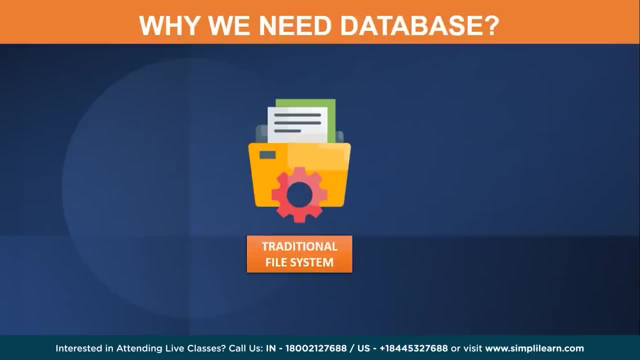 As the technology kept advancing, it became difficult for computers to handle. when the number of files increased and the volume of data grew, The so-called traditional file system was no longer able to store and retrieve data efficiently. Let us now see some of the limitations and disadvantages of a database. 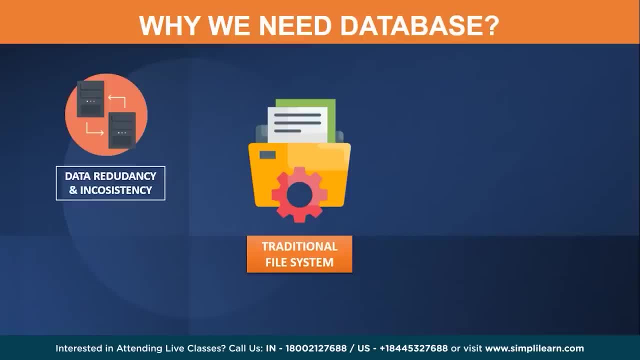 Data Redundancy and Inconsistency. Redundancy means when the same data is getting duplicated and repeated in different locations. This leads to excess and unwanted storage, which eventually results in inconsistency, where the data in separate files do not match with each other. 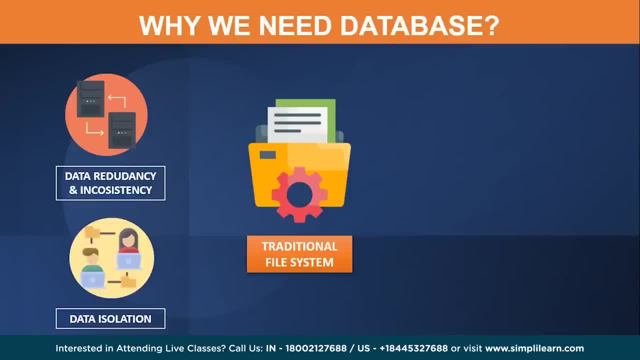 Data Isolation. Data is isolated because it is scattered in various files in different locations, And the files may be in different formats as well. At any point, writing the application programs to retrieve the appropriate data becomes difficult as the files are separated from each other. 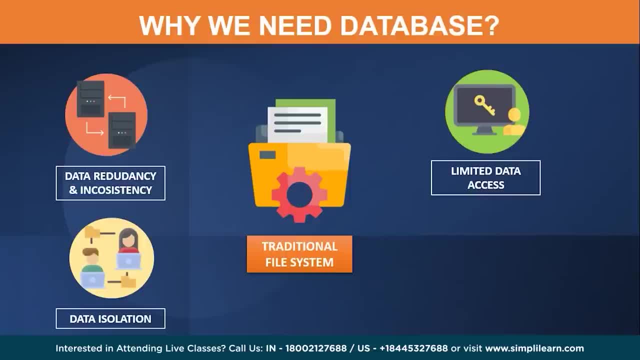 Limited Data Access. File storage systems usually do not have access for multiple users. This means multiple users at different places cannot access the data simultaneously. It becomes difficult to access important data if multiple users are searching at the same time. Data Stored in files can easily be accessed and tampered. 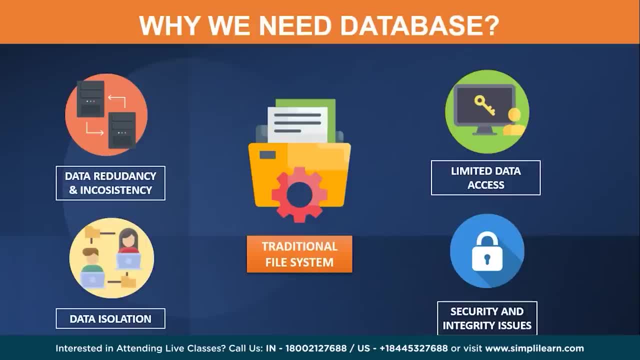 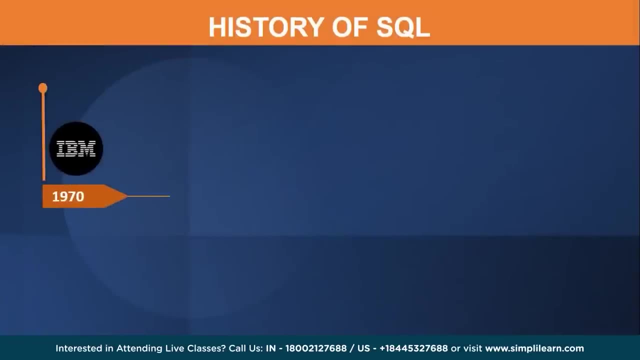 So it's essential to prevent unauthorized users' access, to hold the data's integrity. In order to eliminate all these drawbacks, we use a database that is controlled by a database management system. Let us now look at the history of SQL. SQL was developed by IBM in the year 1970.. 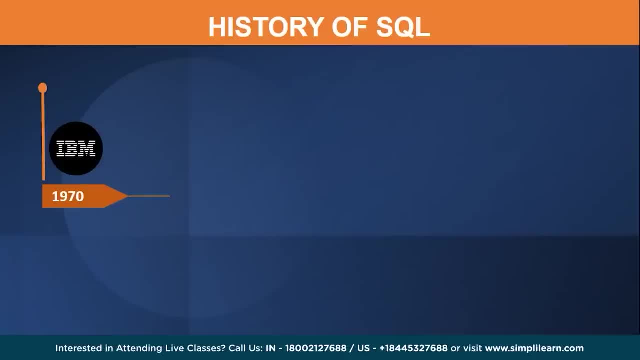 Dr Codboys and Donald Chamberlain proposed a paper on usage of relational database management. They came up with SQL, which can be used to perform operations on data stored in the databases. SQL was made publicly available and was accepted for the use of relational database in the 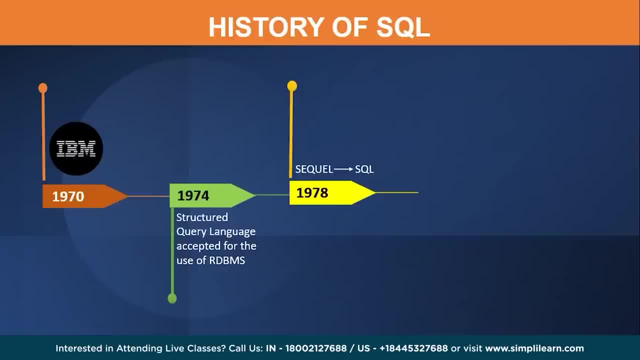 year 1974.. Initially the language was known as Structured English Query Language, pronounced as SQL, which was later changed into SQL in the year 1978.. The American National Standard Institute, ANSI and other international organizations have standardized SQL as a language for database communication in the year 1986. 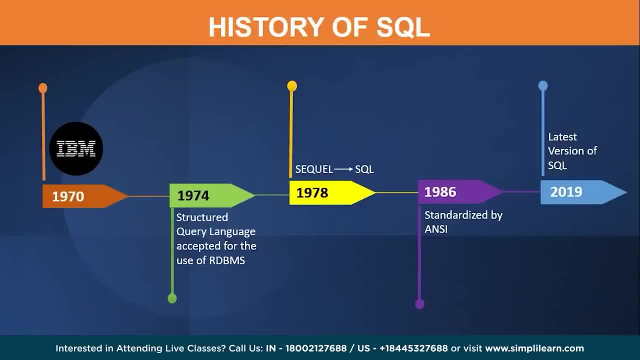 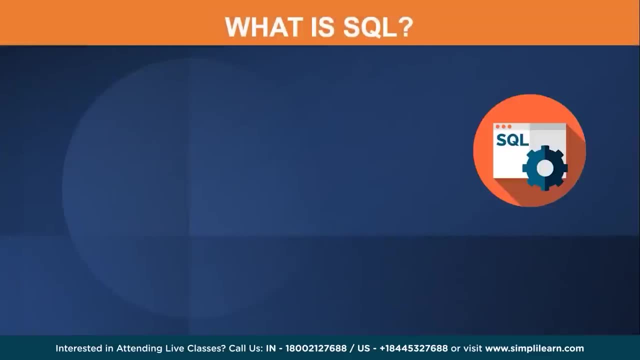 Though companies use a different version of SQL nowadays, the latest version of it was released in 2019 by Microsoft. What is SQL? SQL is defined as Structured Query Languages. It allows the user to manage and manipulate the data. SQL is defined as Structured Query Languages. 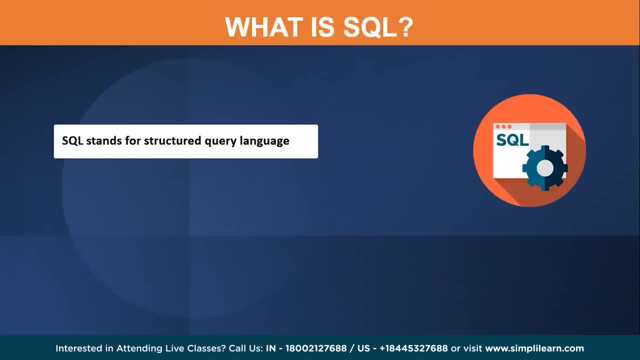 It allows the user to manage and manipulate the data from the database. So you might have got a doubt in your head that we have discussed databases earlier and why we are discussing SQL now. Well, you got it right: Both database and SQL are interconnected to each other. 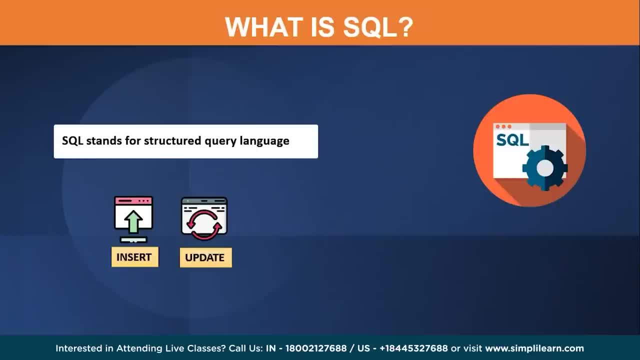 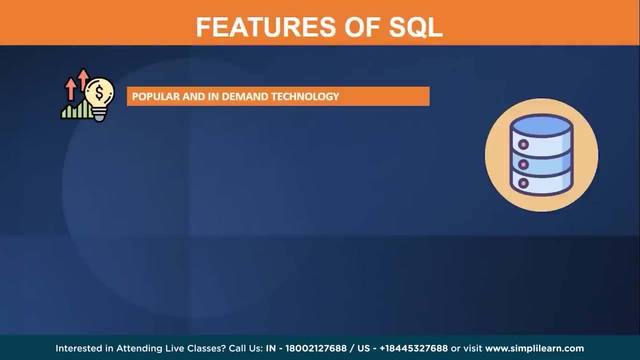 SQL allows you to perform operations like insert, update, modify and delete in the database. SQL is used to communicate with the database systems to retrieve the information Features of SQL. SQL is one of the most demanding skills. nowadays, With the ever-increasing amount of data, SQL serves as a powerful tool to provide insights. 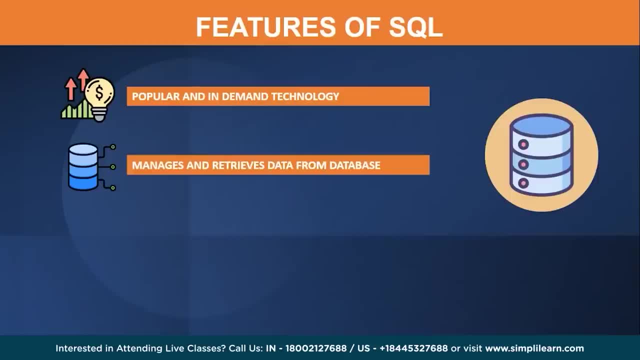 to businesses. while handling databases, SQL is used to define the overall schema, that is, the complete structure of the database, by managing and manipulating the data accordingly and retrieving the information whenever required by the user. SQL also allows flexibility, as it uses simple English words in its queries, like create. 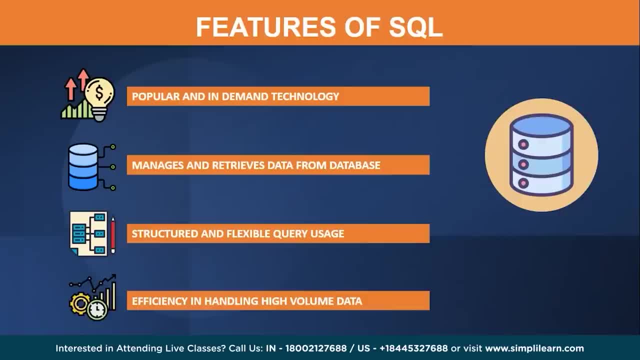 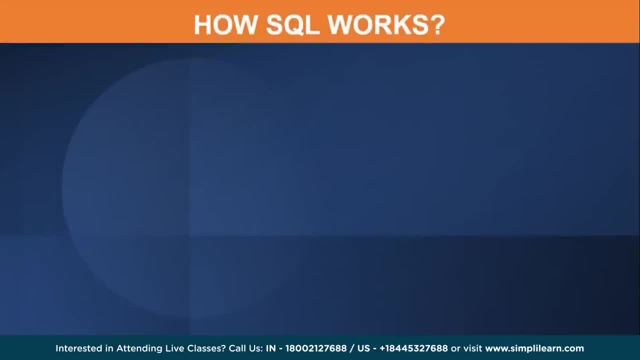 delete, etc. SQL can handle large amounts of records stored in databases with utmost efficiency. Let us now see how SQL works. A typical SQL database engine includes a storage engine, which is a database server, and a query processor within the SQL engine. To understand it simply, 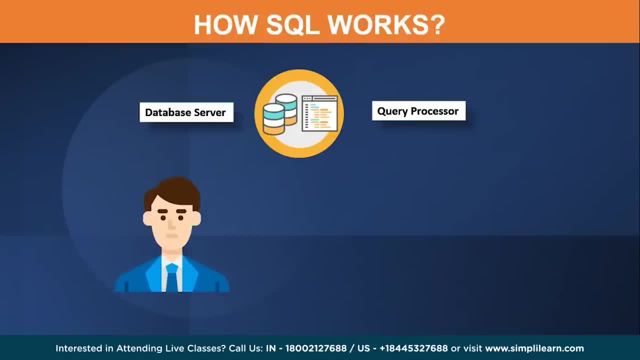 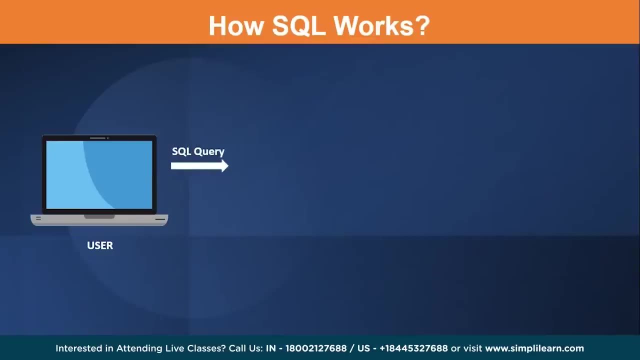 Let us take an example. Suppose John is an HR manager working in an organization. He wants the information of all the employees who have joined last year. John writes an SQL query in his laptop to retrieve the data. In order to execute the query, it must interact with relational database management system. 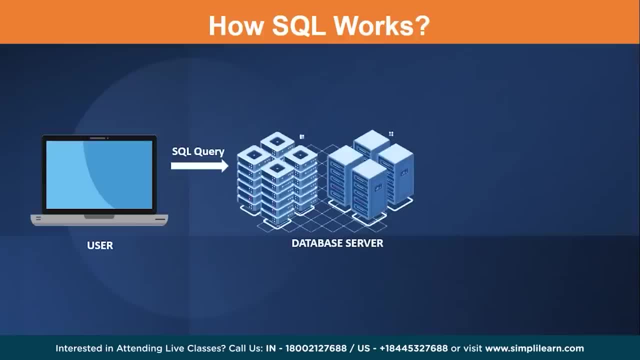 within the database server And the request should be a valid query before the SQL engine can process it. The SQL engine then writes to and retrieves data. The database server and SQL engine work hand in hand to process the required data. The system process the SQL request and sends it to the web server to access the information. 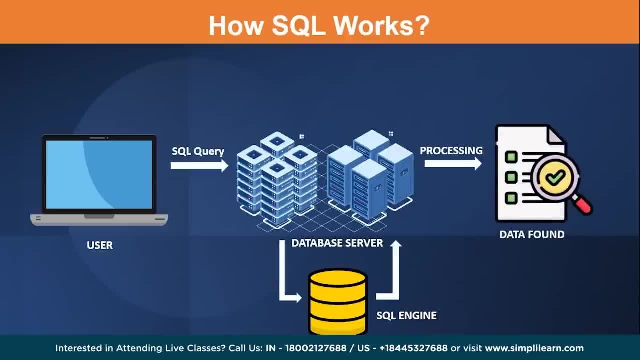 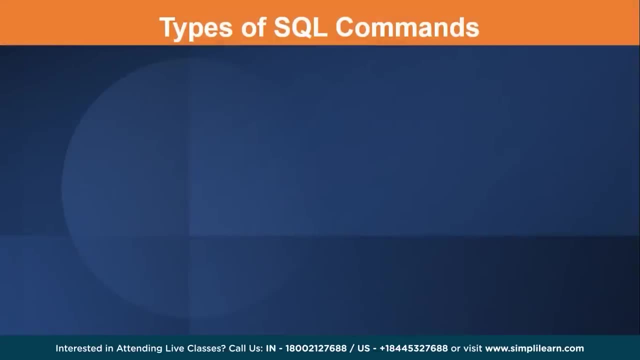 via SQL database And if the information is found in the tables, the database server sends the information back to the user. In this way, John can retrieve the information from the database using SQL Types of SQL commands. SQL commands give instructions to the database to perform specific actions to retrieve the data. 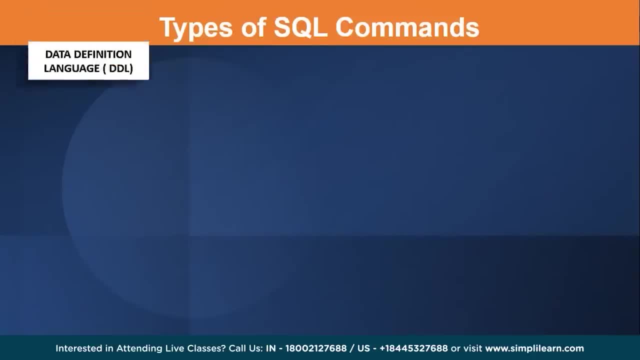 SQL commands are broadly classified into four types. The first one is Data Definition Language, or DDL. DDL allows the user to define the table and change its overall structure. Commands that are used in DDL are: it is used to create a new table. 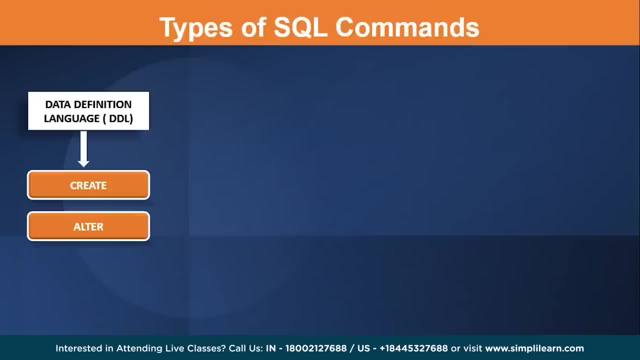 it is used to modify the existing table by adding unique attributes. it is used to delete the whole table and the data stored in it. it is used to delete the rows in a table. The next one is Data Manipulation Language, or DML. 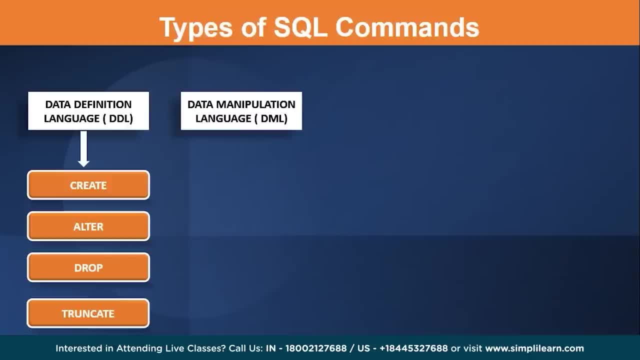 DML is used to access and manipulate data in tables. Commands that are used in DML are: it is used to extract data from the tables. it is used to update a value in the existing table. Unlike the drop command, the delete command is used to delete a specific row in the table. 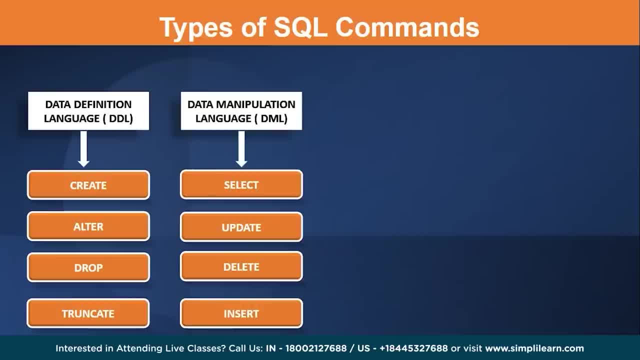 It is used to insert a new value into the table. The next one is Data Control Language, or DCL. DCL is responsible for maintaining the security which gives control, access and permissions to the database Commands that come under DCL are. It is used to grant permission to the user to access the database. 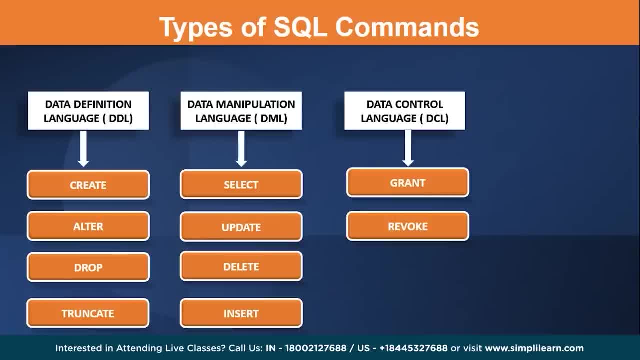 It is used to cancel or take back the earlier granted permission. The last one is Transaction Control Language, or TCL. TCL has three commands, namely: It is used to permanently save the transaction. It is used to restore the transaction that is not saved. It is used to hold a transaction temporarily. 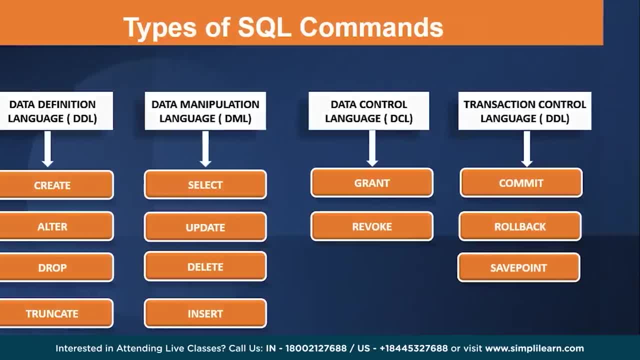 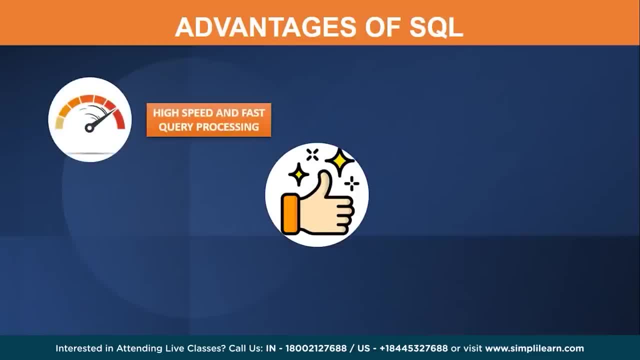 It can be rolled back to its previous state at any point. Let us now look at some of the advantages of SQL. One of the main advantages of SQL is that it provides access to data stored in database. with its high speed and faster query processing quickly and efficiently. 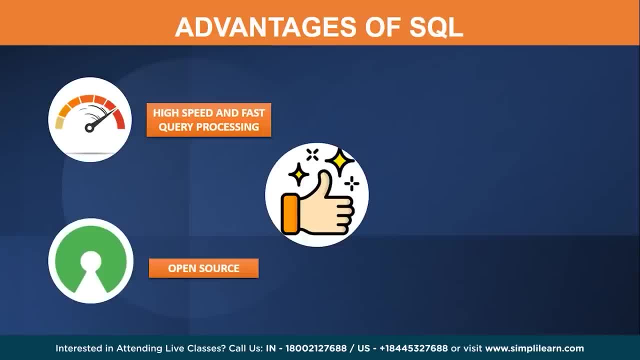 SQL is open source. That means it is publicly available and can be accessed from the internet. It is also straightforward to implement as well. SQL also provides the user to have multiple views of their content stored in the database. SQL is efficient in retrieving vast amount of data using simple queries. 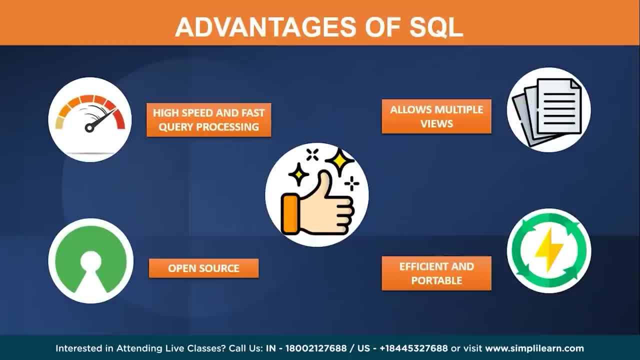 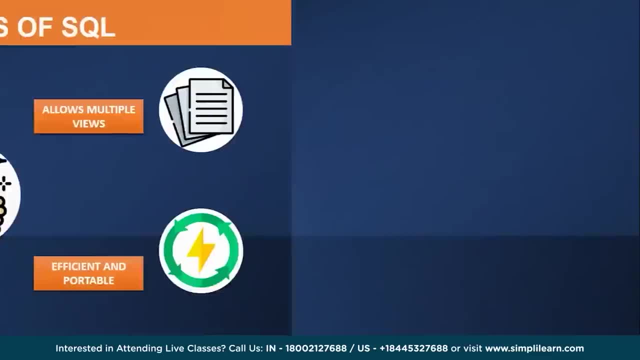 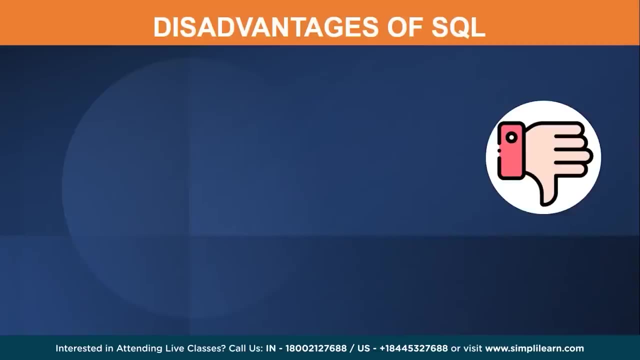 And also it is portable as well, Which means you can perform all these operations at your home or your workplace through your laptops and PCs. Disadvantages of SQL: There are two sides to every coin and similarly, SQL also has few advantages, which are not that significant. 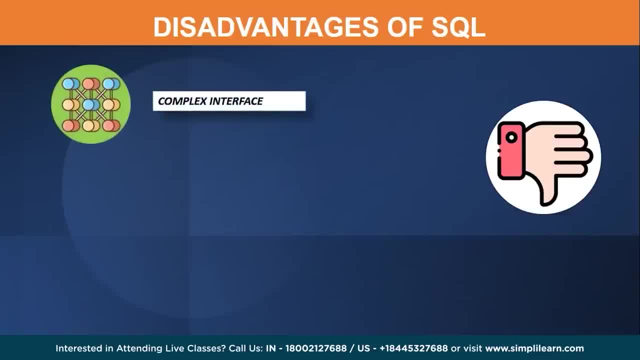 Initially one may find it challenging to work with SQL Due to its complex interface. Since it is a platform based language, most of the commercially available SQL servers costs are relatively higher. SQL is constantly working on these massive amounts of data stored in the databases. 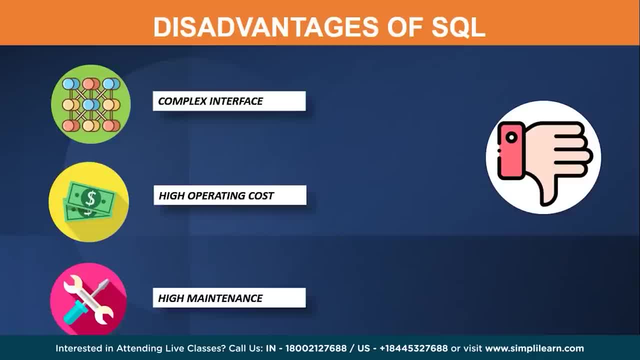 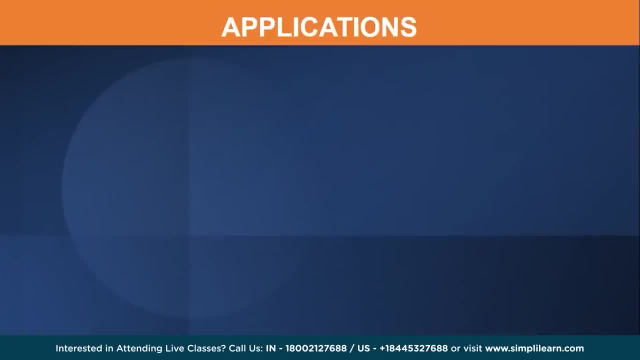 And hence maintenance costs are also high as well. Let us now look at some of the applications in real life of SQL. SQL is widely used in various sectors nowadays. Some of them are Education Schools and Universities use SQL and databases to store and retrieve information about their students, faculty and staff. 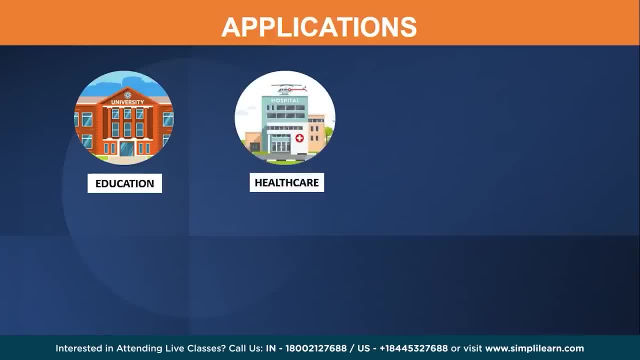 Healthcare, Hospitals and other medical centers use SQL to store the details of the patients without any hassle. It also helps in maintaining all their documents and bills as well. Retail and E-Commerce. With its vast presence in the market, Retail and E-Commerce is one of the most popular services in the market. 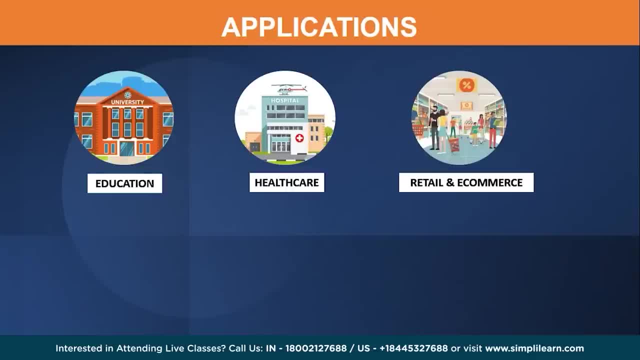 Retail and E-Commerce companies store their customers' data to improve their shopping experiences by providing special offers, which will, in turn, help their businesses to grow. Banking SQL is one of the significant components of the banking sector as well. Banks store the account details of customers and the transactions done on a day-to-day basis in the database. 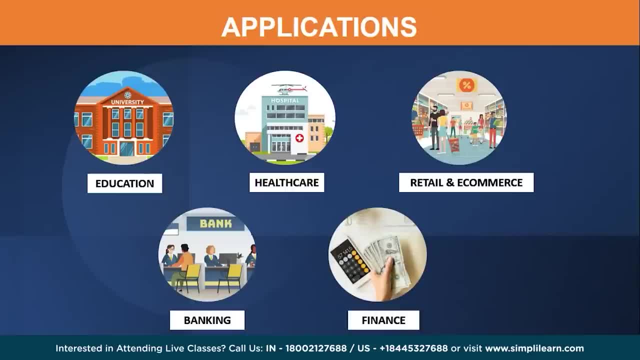 Finance. Finance is another massive area where SQL queries are used regularly in managing the assets, revenue details and transactions, Shares of the companies, etc. Faster execution and retrieval of data are key for all the businesses to make strategies and derive insights from it. Companies using SQL. 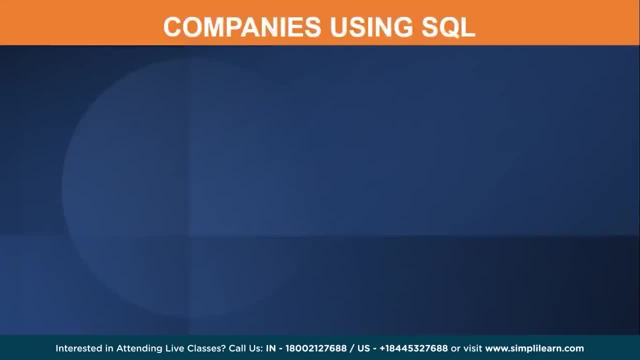 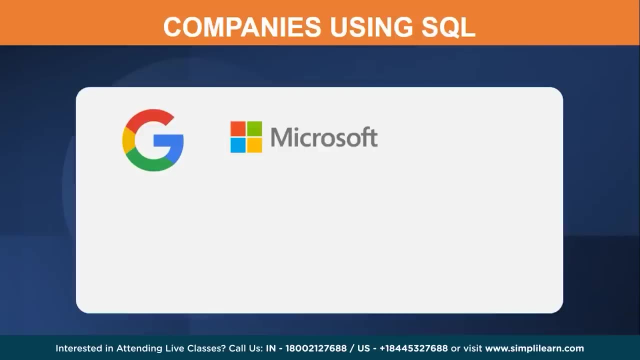 SQL is used extensively every day by some big tech giant companies like Google, Microsoft, Oracle, Amazon, Facebook, etc. Even small companies and start-ups heavily rely on SQL: Google, Microsoft, Oracle, Amazon, Facebook, etc. Even small companies and start-ups heavily rely on SQL. 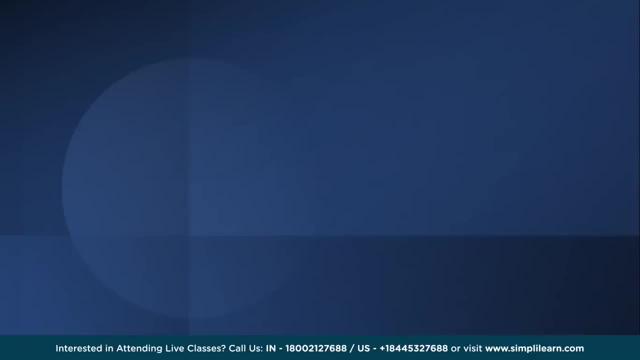 Google, Microsoft, Oracle, Amazon, Facebook, etc. Perfectlyf Doing다는 SQL With. We've come to the end of this session on introduction to SQL By Now. you must've got some idea of what SQL is. Over the years, SQL has evolved and is widely used nowadays worldwide. 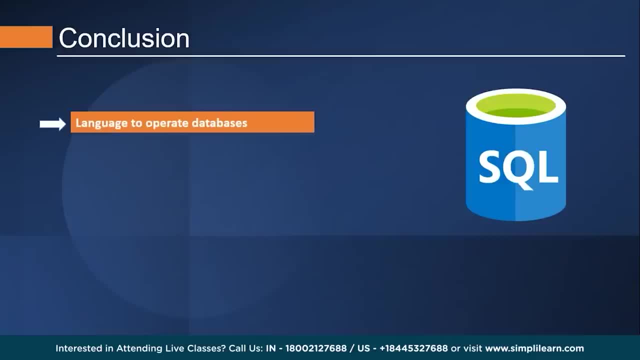 It is one of the most efficient database languages out there. It can perform various operations on the database to retrieve the data instantly. SQL is very simple to understand and easy to learn, as well as all the commands and queries are written using English words. Unlike other programming languages, SQL requires almost no coding. 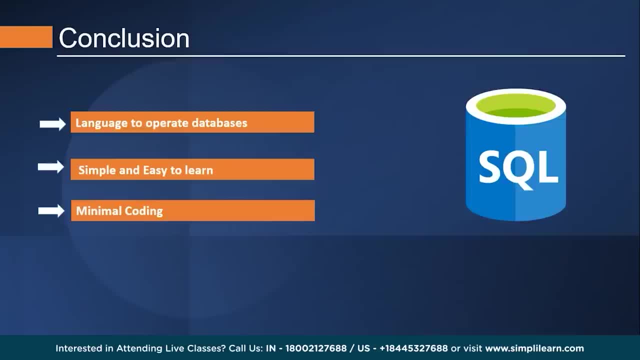 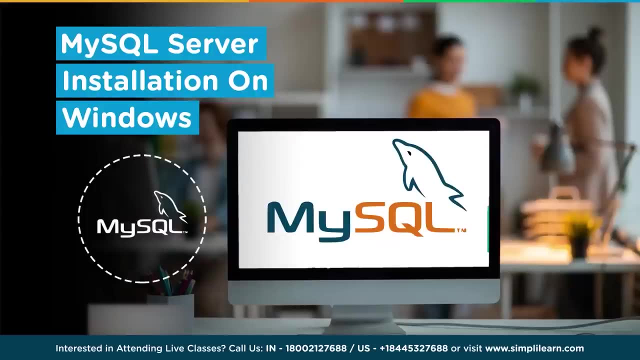 It does not require thousands of lines of code. The syntax is also user-friendly and easy to implement. Welcome to another interesting video tutorial on how to install MySQL server on your Windows system. So in this session we'll go to the complete installation process of MySQL Workbench, as well as MySQL Shell. 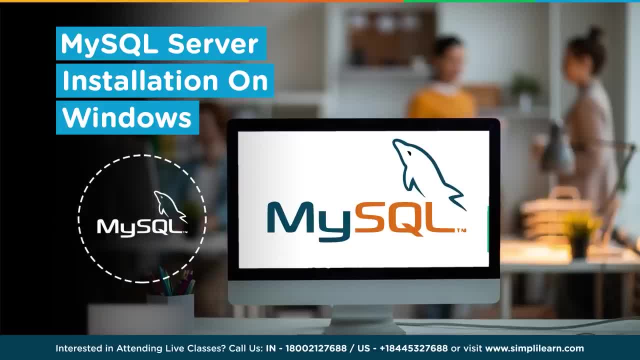 which is basically a command line used to create tables with the help of SQL language. So, without any further delay, let's get started. But before we begin, make sure you have a good internet connection so that at any point you won't find any issue or difficulty with the installation process. So let's go. 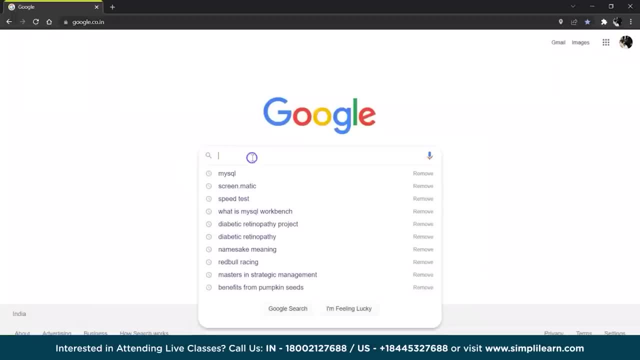 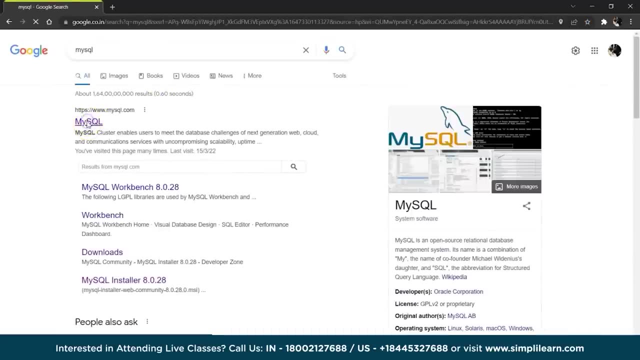 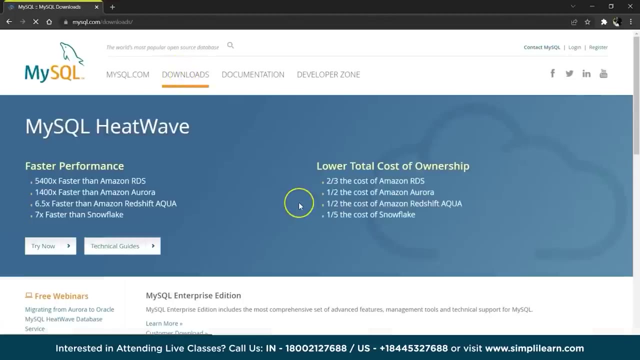 ahead and start with the installation. Firstly, go to Google and type MySQL. you'll find MySQL Server on your computer. Click on the official website page on the search result. Click on that. Once you reach their official website page, you'll find download section. Click on that Now. 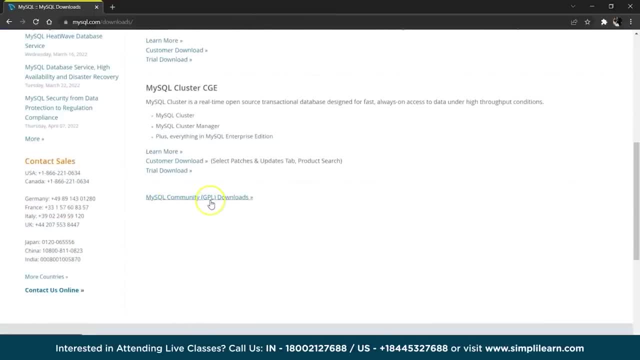 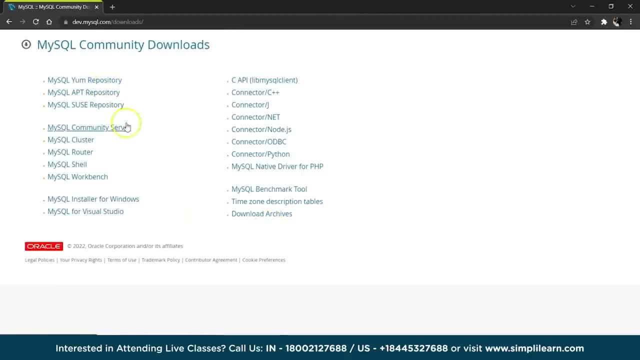 scroll down a bit and you'll find MySQL Community GPL downloads. Click on that link Now. you'll find various options for downloads, such as various repositories, MySQL Shell, MySQL Workbench, etc. But since we are installing it for the first time on our Windows system and we are 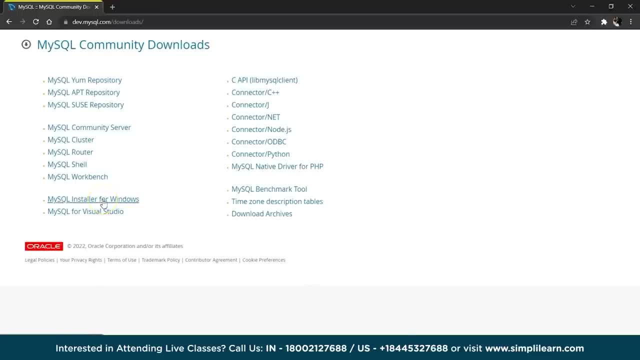 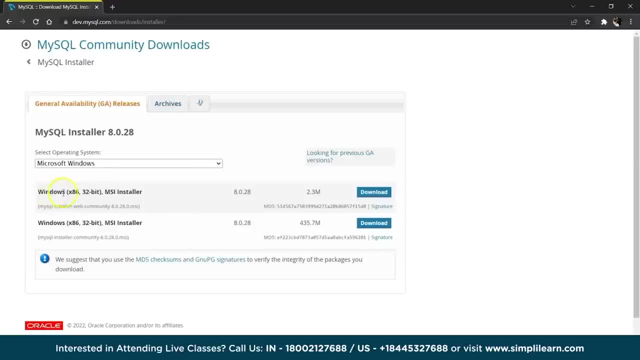 only concerned with the Windows system. we are going to install it on our Windows system. MySQL Workbench and Shell will go with MySQL Installer for Windows. Click on that link Now. you'll find two options for download. The first one is Windows 86. 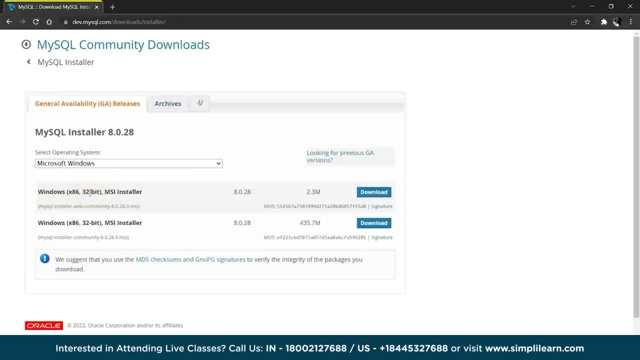 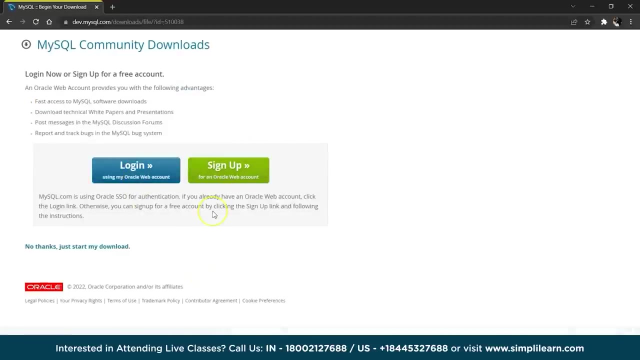 32-bit MSI installer. It is showing here 32-bit, but it will work for 62-bit systems as well, so don't worry, And you can choose either of the two, and I'm going with the first one. Click on download. Now you'll find this page where you'll have login and sign up for the Oracle account. 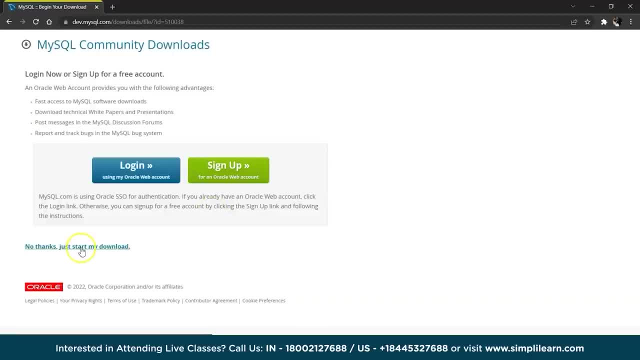 Now you'll find this page where you'll have login and sign up for the Oracle account. For time being, just ignore that and click on no thanks and start my download. For time being, just ignore that and click on no thanks and start my download. 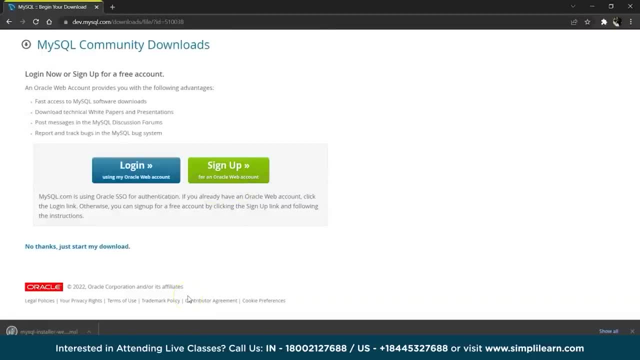 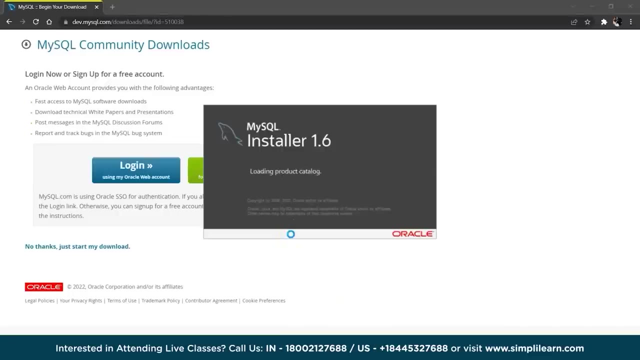 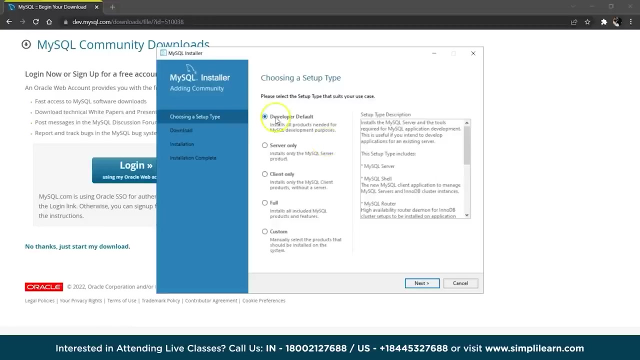 Save it on your system. Once it's downloaded, open the file, Give all the necessary permissions. Now you'll find a setup page where you'll have different options, such as developer server client, full and custom. We'll choose custom because we want MySQL Workbench and MySQL Shell. 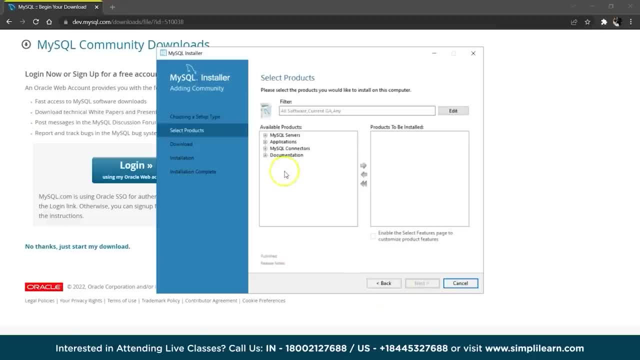 So click on next. Now we have to select the products which we want to install on our system. You can find MySQL Server. Click on that and expand it. You'll find MySQL Server 8.0.. Click on that. You'll find the latest version of it. Click on that and select the arrow, and. 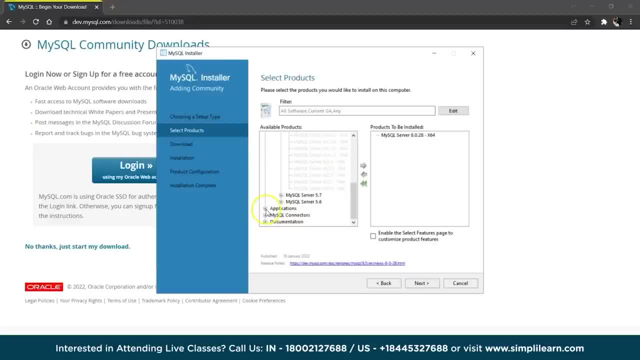 send it to the other side. Now. scroll down a bit and you'll find applications. Click on that. You can see MySQL Workbench. Expand it and you'll find the latest version of it as well. Click on that and click on the arrow and send it. 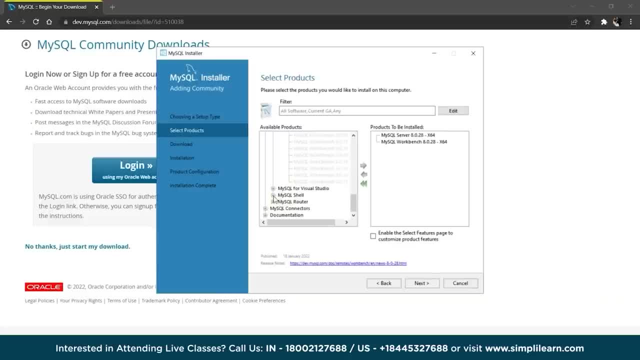 to the other side. Scroll down a bit and you'll find MySQL Shell as well. Click on that. Expand it, Select the latest version, Click the arrow and send it to the other side. Now we are good to go and click on next. 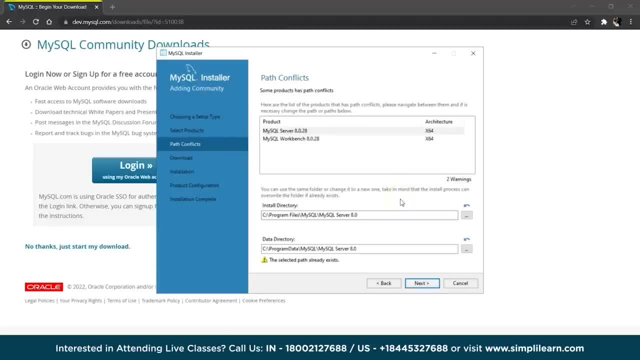 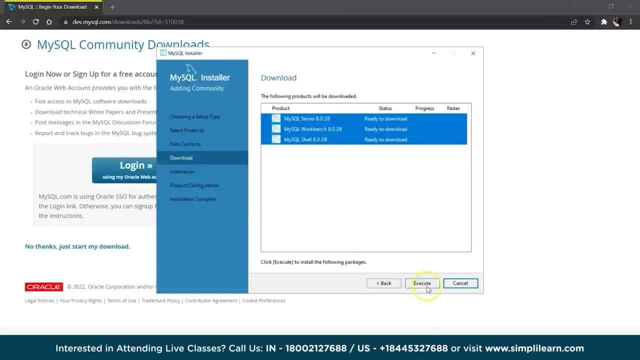 Now it will ask for the path where you want to install all these files. We are saving this on our C drive. Just check all the necessary paths and click on next. Now all the three products are ready to download. Click on execute Again now. depending upon your internet speed, this may take a while, So don't worry. Just 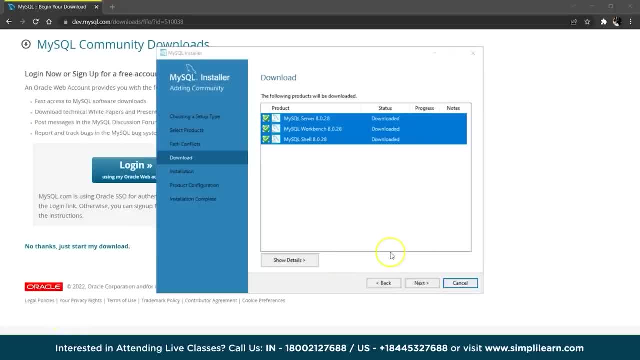 sit back and wait for it to get downloaded. You can see all the three products are ready to download. Click on execute. You can see they are successfully downloaded. Click on next. Now we need to install all the three products. Click on execute So you can do the installation. 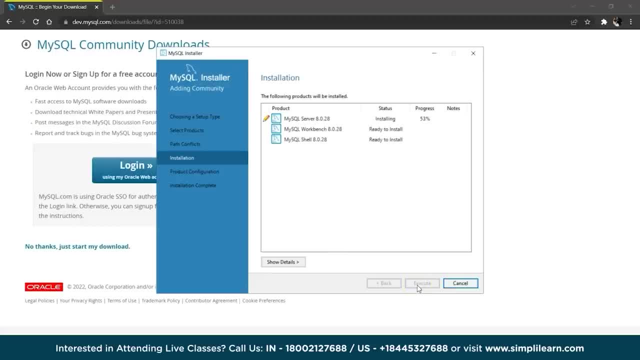 process simultaneously with me, or just take a note of it and perform it later as well on your PCs and laptop. This might take a while, so we'll wait for it to get installed. As you can see, all the three of them are successfully installed. Click on next. Click on next again. 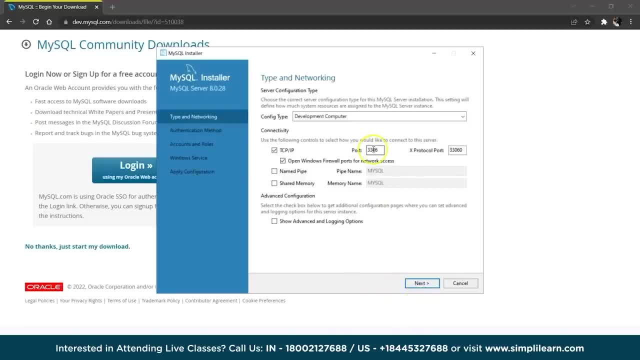 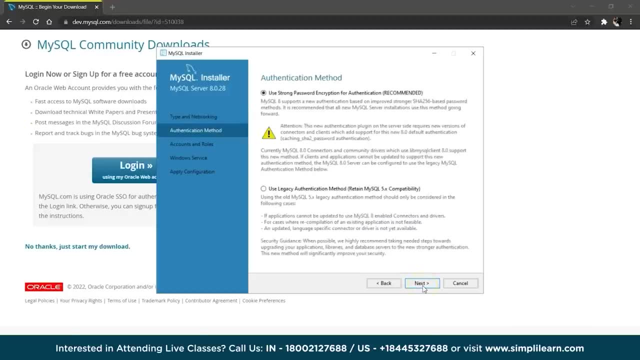 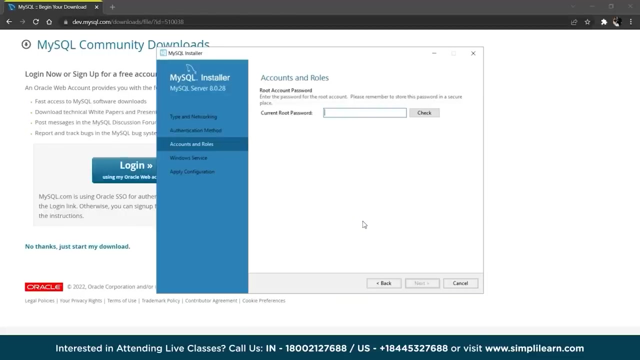 Now we have successfully installed all the three of us, We'll saved all of them. Click on next once again. Click on Next Now once again. This method is very simple: the files and programs. so enter a password of your own choice and make sure you take a note of it, because we'll have to use it at a later. 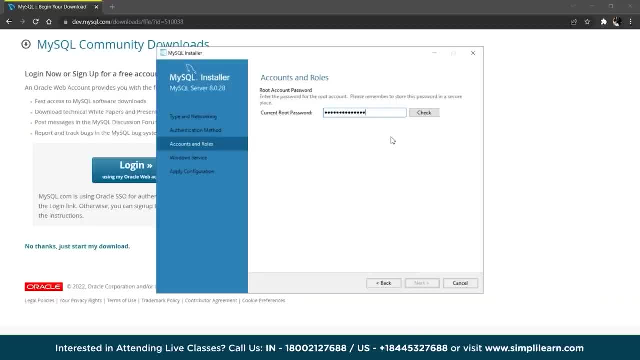 stage and also by logging into the mysql server. you will use the same password. so click on, check you so, as you can see, there's a blue tick mark which means it's verified. uh, so you can go ahead. click on next. now you'll find the windows service, which is: 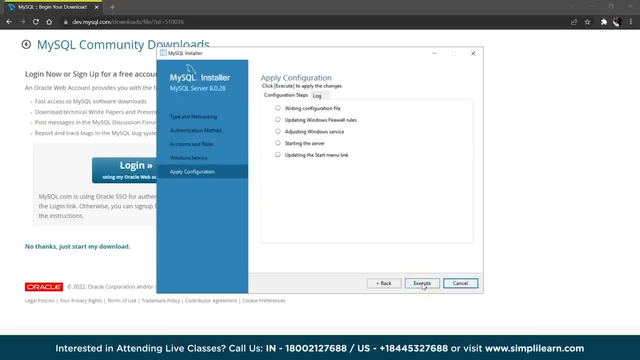 the standard system account. choose that and click next. now you have to apply all the configuration for the system files. for that, just click on execute and the system will automatically configure itself. so this might take a while, so we'll wait for it to complete. as you can see, the all the files are successfully configured. 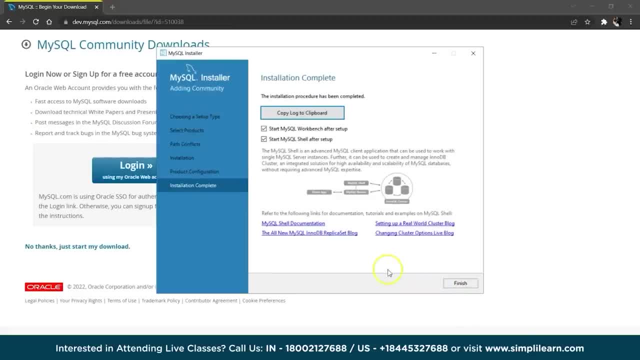 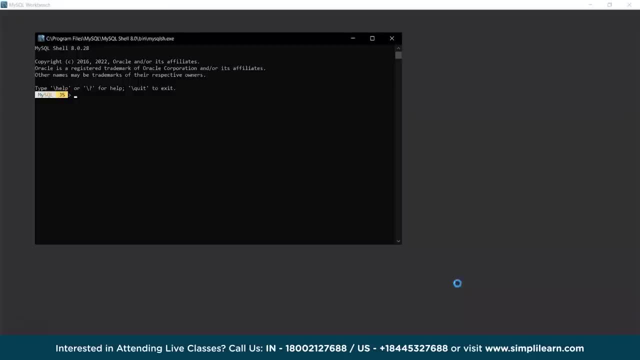 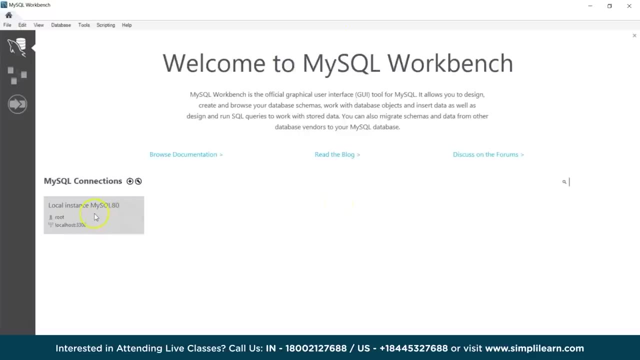 click on finish, click on next. so once you uh click on finish, uh, mysql workbench and mysql shell will automatically launch. so workbench and shell are started in the background. uh, as you can see, there's a local instant mysql 80. click on that now it will ask you to enter the password which you have set. 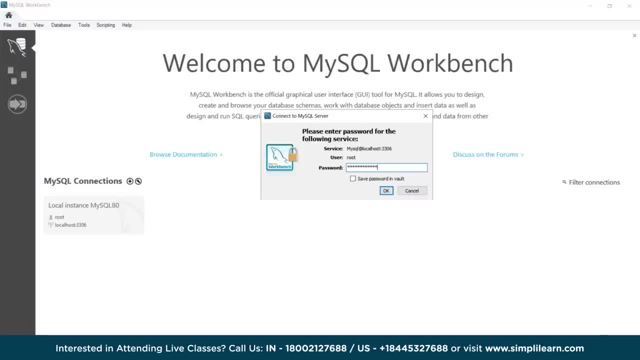 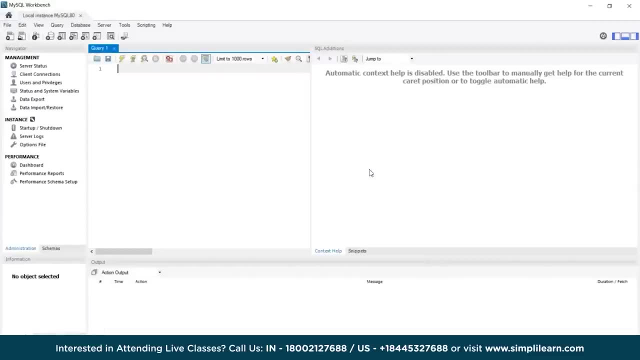 earlier. click on that. so that's it, guys. we have successfully installed mysql workbench on our system. but before you get started, there's another little process that we'll, with that we are left behind with. now you have to connect all the files and packages to the server before you start working on the tables. so for that, we need to locate really where the mysql files are stored. for that we'll go to file manager. since we have saved the files on local disk d, local disk c, uh, click on c drive. go to program files. click on mysql: open my skills over 8.0. 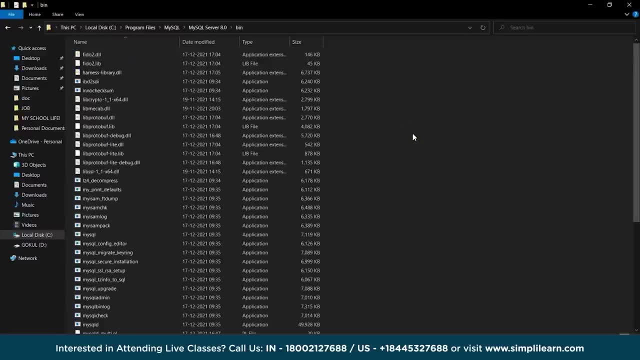 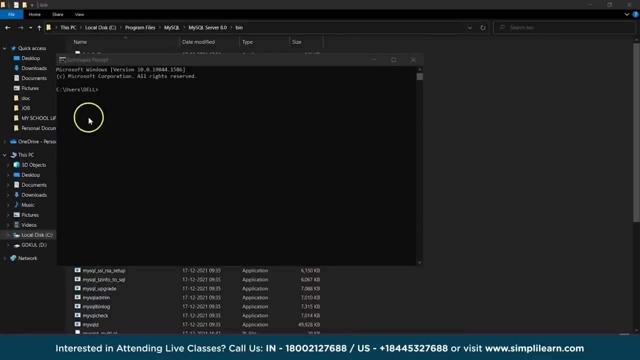 click on bin. now these are all the files and packages that you have to connect to the server. for that, double click on location path, copy the whole address and open command prompt. on the command prompt you will have to type cd- that is the current directory- and paste the address that you have copied earlier and click enter. now type mysql space myu root. 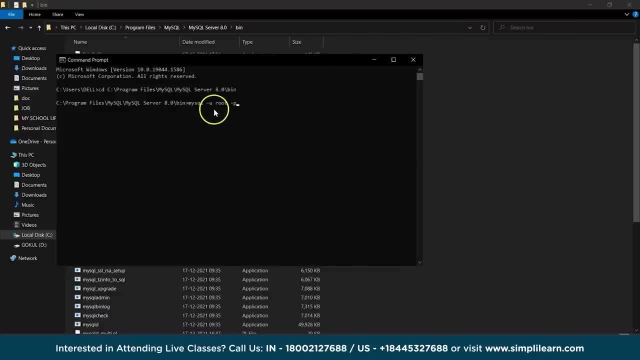 minus p here. minus u is the user, which is the root user which we have taken. minus p is the password. click on enter now it will ask you to enter the password and then you will have to enter the password that you have set earlier. type the same, so if you find what you're seeing, 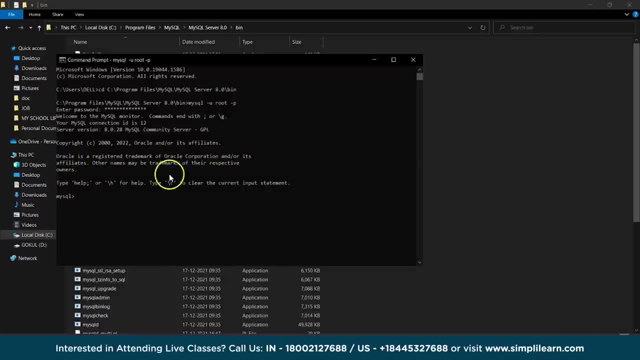 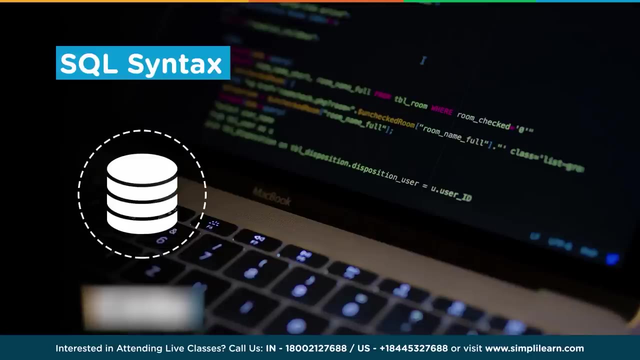 in my system, that is, oracle, is registered trademark of oracle cooperation and all this thing. that means you have successfully downloaded and installed all the files and packages into the mysql server and you are good to go and start working on your tables right away. learning a new programming language and its syntax can be quite difficult sometimes, whereas 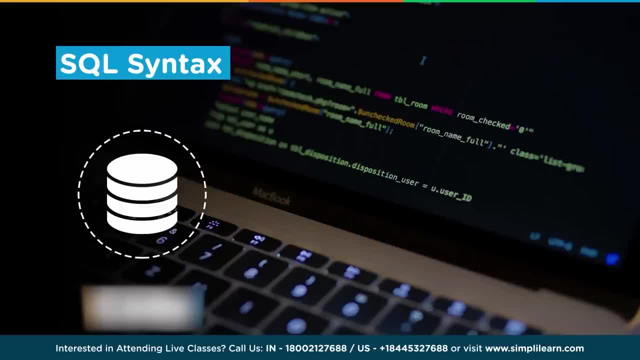 sql server is a very easy way to learn a new programming language, and its syntax can be quite difficult sometimes, whereas sql syntax is very simple to learn and easy to execute as well. more on that soon. so without any further delay, let's get started with today's topic. 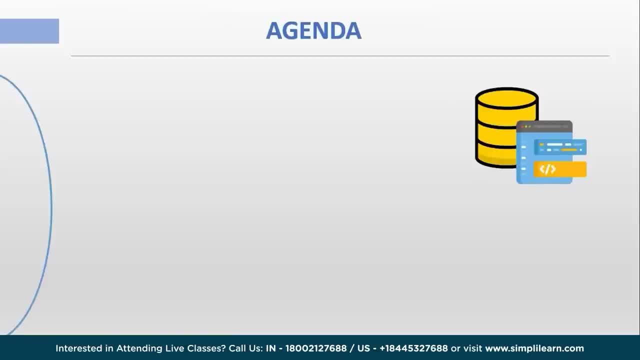 firstly, let us discuss the agenda for today's session. we'll start the tutorial by understanding what sql syntax is and why we use it. next we'll understand what are sql expressions and sql statements. then we'll discuss about sql data types, followed by sql operators. next we'll go through sql commands and its types. 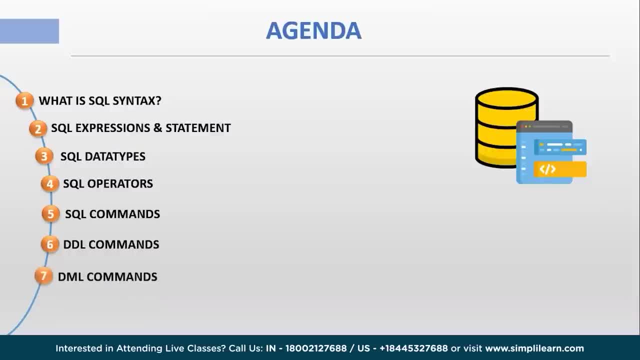 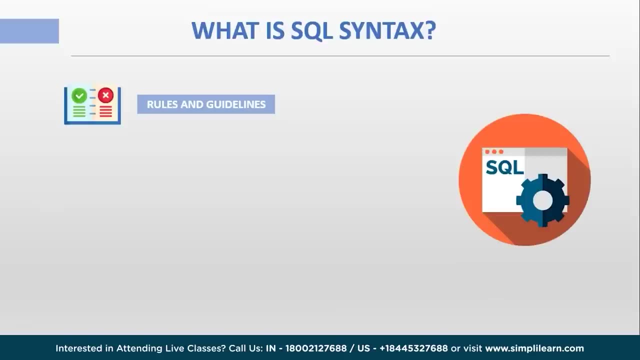 After that, we'll discuss the syntax of ddl commands, followed by DML commands, and finally we'll have a look at the syntax of DCL commands as well. what is sql syntax? just like other programming languages, sql follows a unique set of rules and guidelines called syntax. we use simple English words in the sql syntax in order to execute various 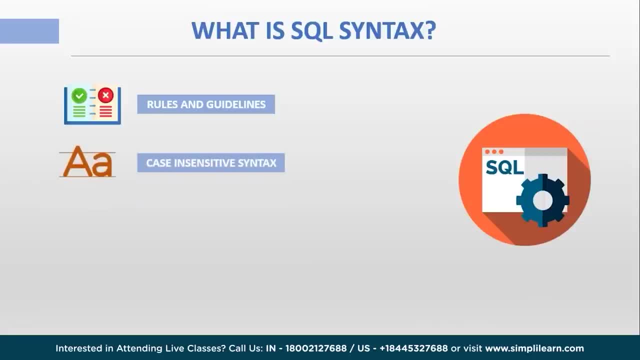 queries. sql syntax is, by default, case insensitive. that means the system is set up to Massachusetts consensus. we're investigating the key features of sql syntax and hope we find some useful. bye bye to and authorities- those important to our policy. The system allows the user to write the queries in both uppercase as well as lowercase. 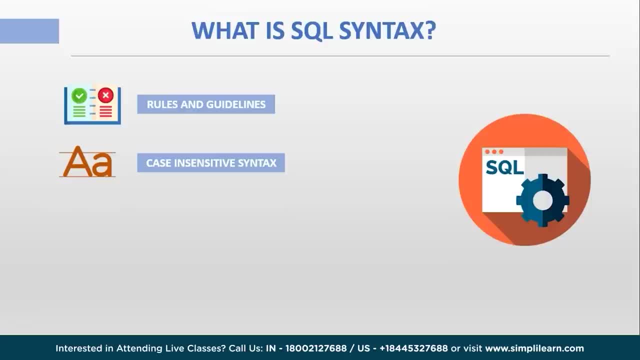 But if you are working with MySQL server, then you need to give table names exactly as they exist in the database. We know that RDBMS is the basis for all modern database systems, including SQL, which manages and performs various operations on the tables, like insert, update, modify and delete. 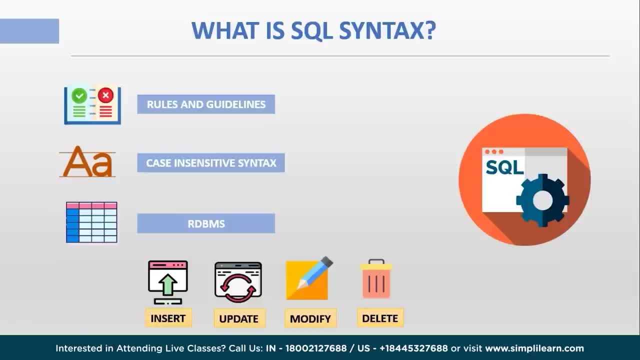 So in order to retrieve the data stored in the database, it is necessary to learn SQL syntax first Before we move ahead with the topic. if you want to learn more about the basics of DBMS and SQL, make sure you check out our previous playlist videos on introduction to DBMS and SQL on our channel. 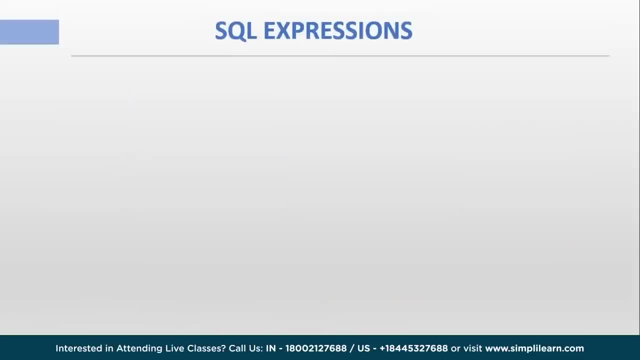 We'll leave the link in the description below: SQL Expressions. SQL expression is a combination of one or more keywords and values, operators, data types and other SQL functions. These SQL expressions are like a formula, which are similar to mathematical formulas which we generally use to solve a problem. 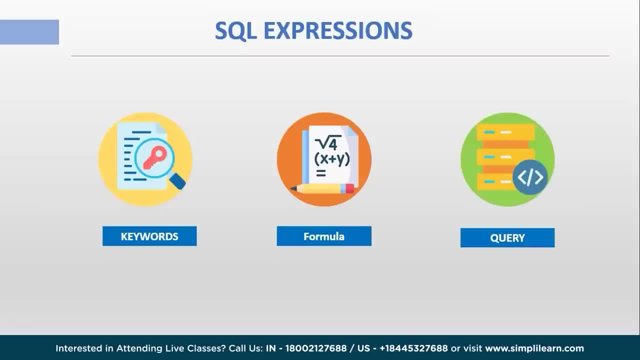 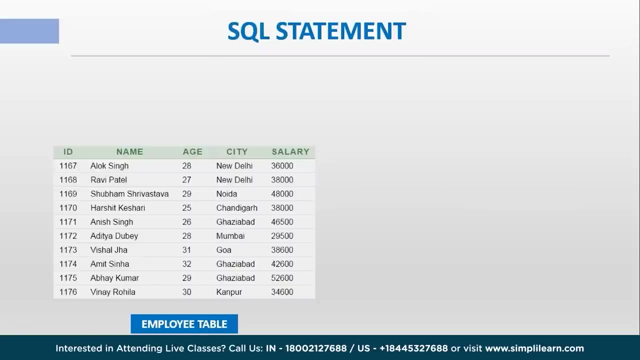 And in this case they are written in a query language using a proper syntax. SQL Statement. SQL statements are basically a collection of SQL expressions. For example, let us consider an employee table to understand it in a better way. The table is having attributes like employee ID name, age, city and salary. 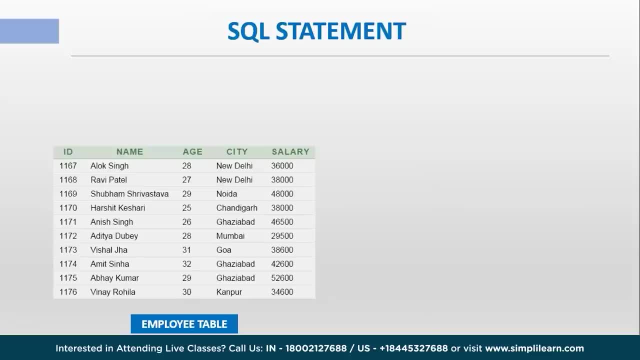 The table is having attributes like employee ID name, age, city and salary. Now if I want to fetch the record of all the employees and their IDs, I'll write a simple SQL query, That is, select ID name from employee. 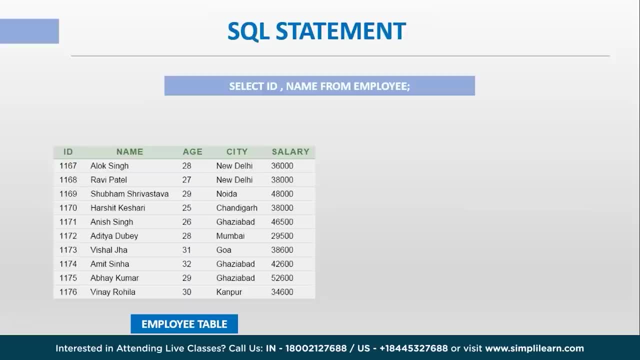 Here. select is the database object or the keyword that is used. ID and name are the columns from employee. Employee is the name of the table. When I execute this query, this will be the output. It will display the ID and name of the employee. 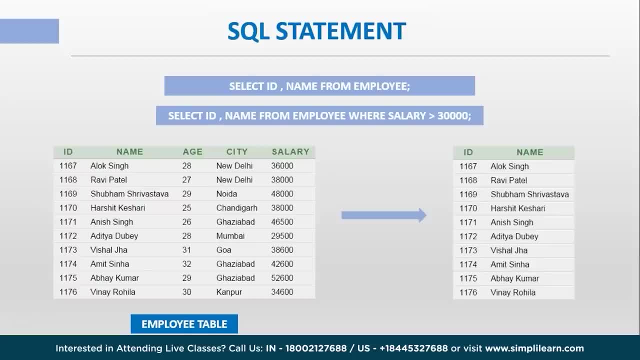 Let us look at another query: display the salary of employees having more than 30,000.. For that, I am using the query as select ID name from employee where salary is greater than 30,000.. Here, where is the conditional statement that I am using? or it is a SQL clause? Also, we are using greater than symbol, which is an. 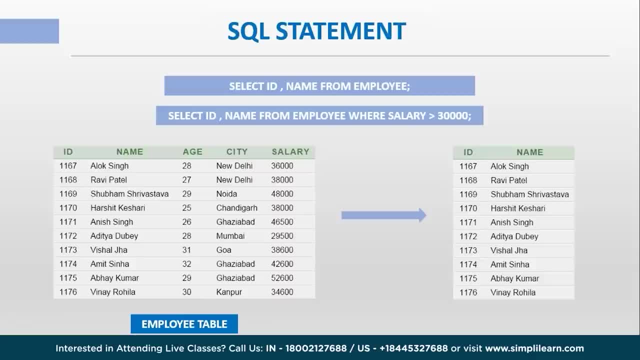 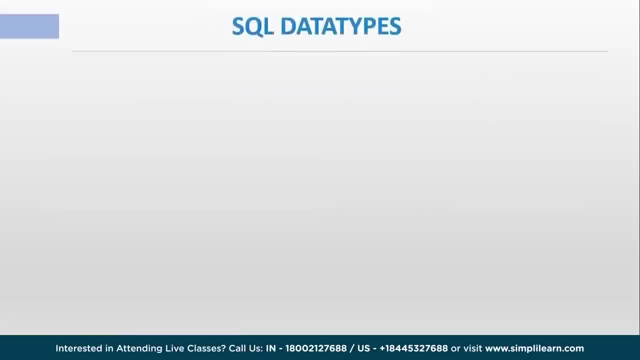 SQL operator. So, with the help of SQL statements, we can fetch the records of all the information from SQL tables. SQL data types. SQL data type specifies which type of values is stored in the database tables. SQL data types are mainly classified into three categories. The first one: 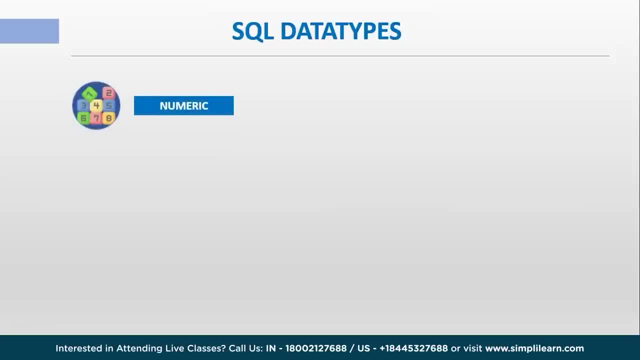 is numeric. Numerical data refers to the data that is in the form of numbers. In numerical data type we have different types as well. For example, int. Int holds values of integers and whole numbers without any decimal points. Int holds values of integers and whole numbers without any decimal. 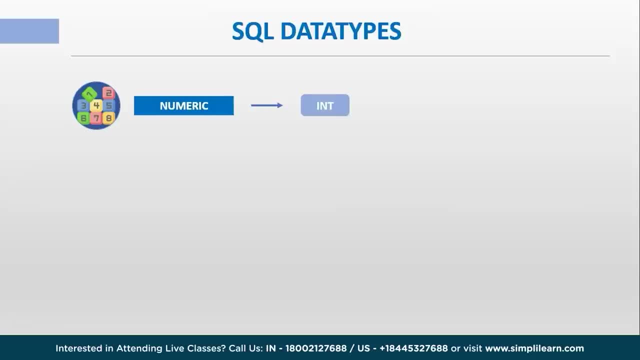 points Further. they are again divided into small int and big int. also, The difference between them is the size and range of the value they can store and operate. Bit Bit data type is an integer data type that can only take values of 0,, 1 or any null value. SQL optimizes storage of bit columns If a 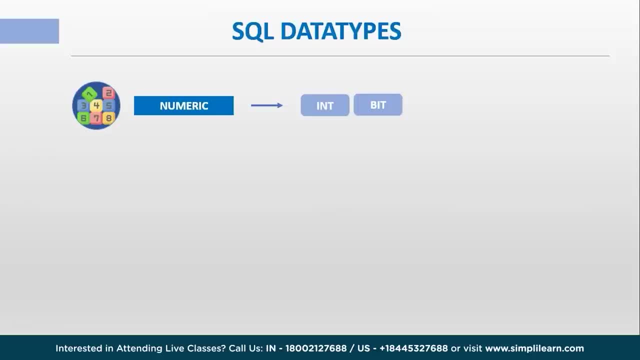 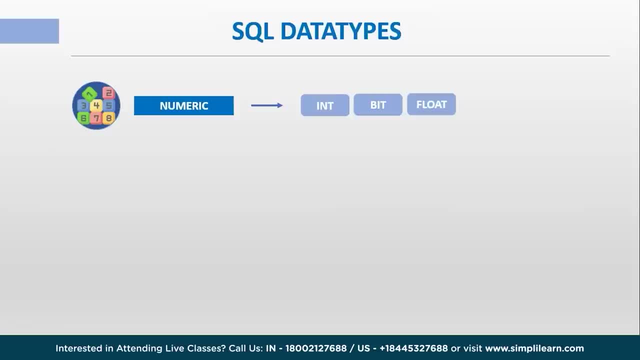 Float. Float stores the numbers having decimal values Depending upon the number of digits after the decimal point. SQL gives the size accordingly in its range Boolean. It is used to specify Boolean values, ie true and false. Zero is considered as false. 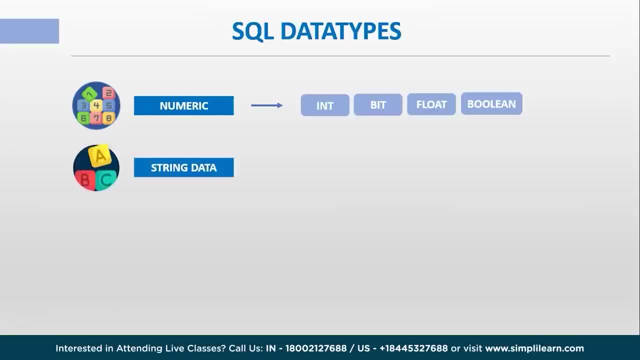 and non-zero values are considered as true String data type. String data type allows us to store fixed or variable character values. They are again further divided into various types. The first one is char. Char is used to specify a fixed length string that can contain numbers. 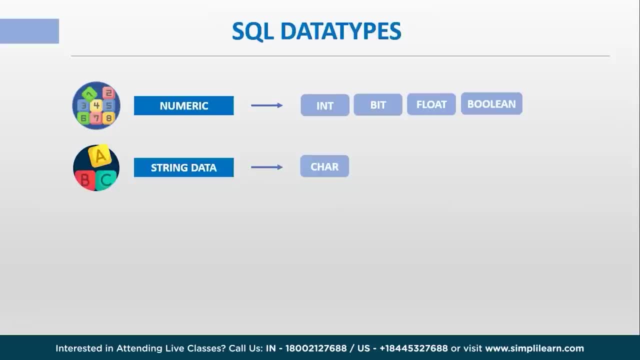 letters and special characters. Its size can be 0 to 255 characters. Var char- Var char is similar to char, but it stores variable length strings, and size of var char is also more than the char data type, with a range of 0 to almost 60,000 characters. So if 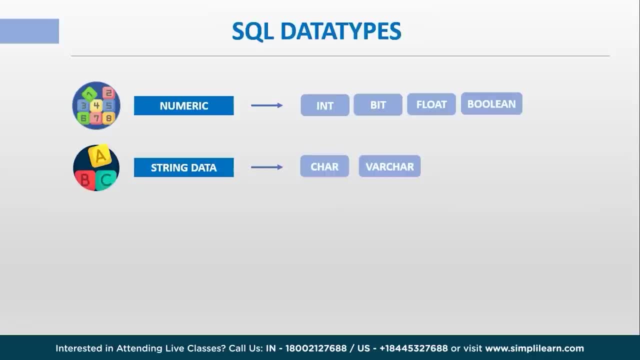 you're storing strings with a widely variable length, such as name, address, email id, then we have to use a var char. Text Text data type stores any kind of text data. It can hold string value that can contain maximum length of 255 characters. Date time In SQL: date time data. 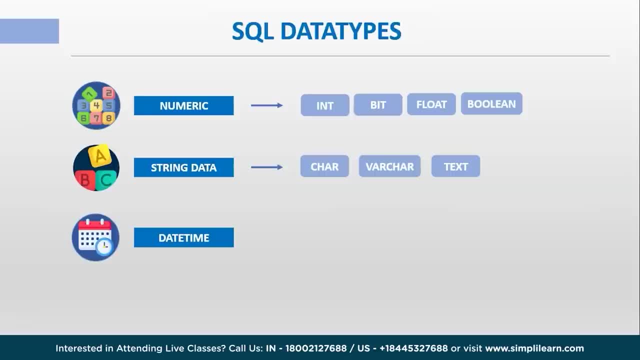 type is used for storing values that can contain both date as well as time. The first one is date. It is used to specify date format, ie year, month, date. In this data type, we can store only the value of date, And the next one is date- time- It is used to specify. 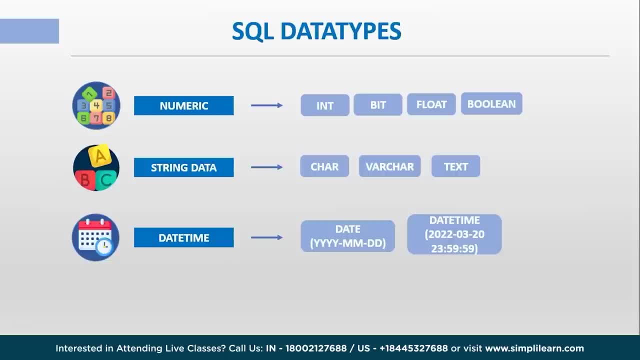 the combination of both date and time. The format is year, month, date, hours, minutes and seconds. For instance, I've taken the example as 2022.3. that is the month, 20 is the date, 23 hours, 59 is the minutes and 59 is the seconds Timestamp. It is also similar to date. 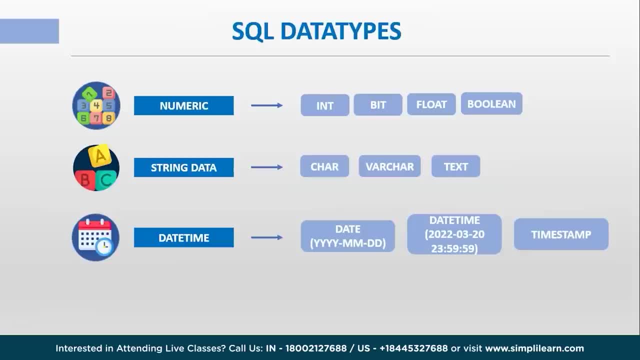 date time data type. The format specification is also the same as well. The only difference is it has less range of values to store. It is also used to convert current time into various time zones like UTC, GMT, etc. We also have XML and JSON data types, which are not that significant. 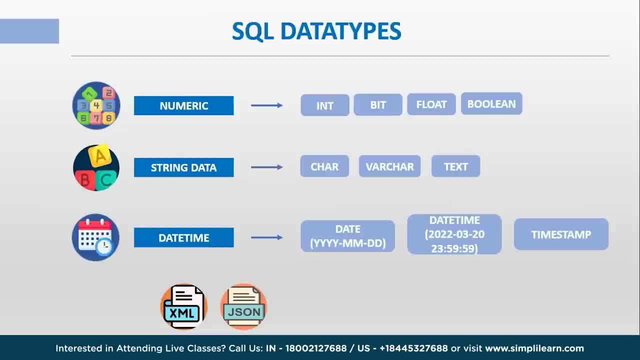 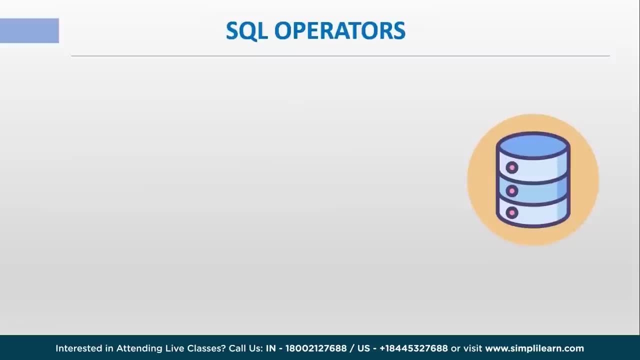 and we do not use as frequently as other data types in SQL SQL operators. SQL operators are used to specify certain conditions in a SQL statement. SQL operators are broadly classified into 5 categories. The first one is arithmetic. Arithmetic operators perform mathematical operations on numerical data. 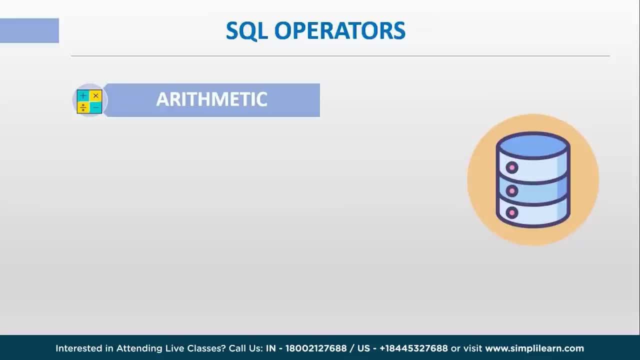 on the SQL tables. These operations perform addition, subtraction, multiplication and division operations on the numerical operands. The next one is logical. The logical operators in SQL perform Boolean operations, which gives two results, either true or false. These operators provide true value if both operands match the logical condition. 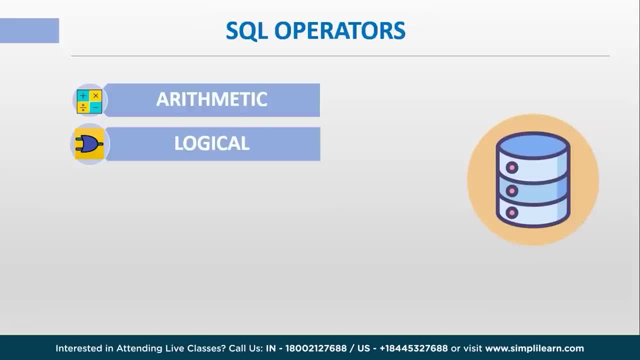 Some logical operators are: AND, NOT, OR, BETWEEN, etc. Comparison: The comparison operator in SQL compares two different data in the SQL tables and checks whether they are the same, greater or lesser. The SQL comparison operators are used with a conditional clause WHERE in the SQL queries. 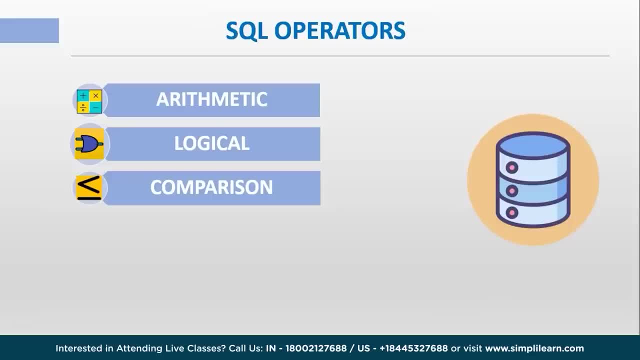 BIT-WISE. If the purple bar represents the same number of using variables of any specific integer in a SQL field, in that data alone the historical device belongs to a particular key type, it will may select the inbox by default. BITWISE Bitاس operator performs bit manipulations between two expressions of any integer data type: И, ans, �vl, FrSab��这, ys, Employer, c, Ys, reflexes, Bit, 봤 operators convert two integer values to binary bits and perform AND OR BUT OR operation on each bit which finally gives the required result. Final one is SET. The SET operators in SQL combine Ys and Entry Bits between the two data-type categories In Ys, company B. applaud llam a setも. 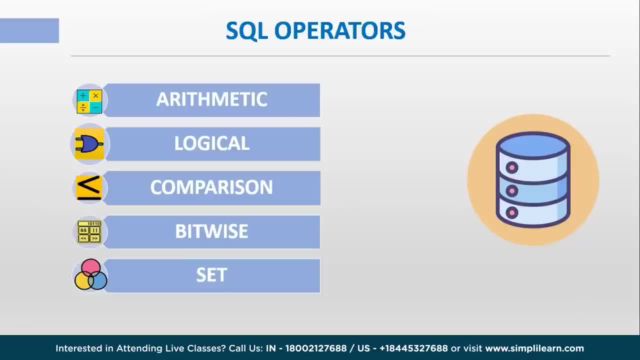 a similar type of data from two or more SQL database tables. Basically, it merges the result which is extracted from two or more SQL queries into a single result. SQL Union, Intersect and Minus operators are some of the examples of set operations. 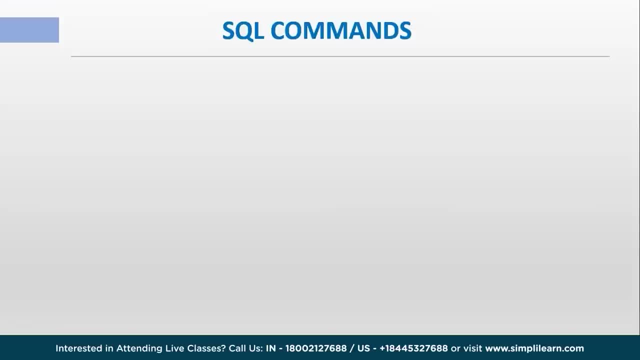 SQL Commands. We know that SQL commands are broadly classified into four types. The first one is Data Definition Language. DDL allows the user to define the table and make changes to its overall structure. Commands that are used in DDL are Create – It is used to create a new table. 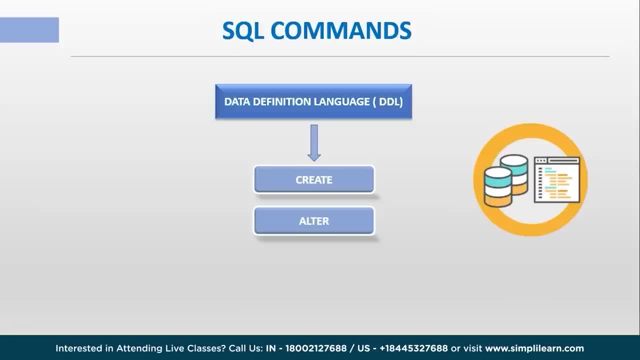 Alter – It is used to modify the existing table by adding new attributes. Drop – It is used to delete the whole table and the data stored in it. Truncate – It is used to delete the rows in a table. Now that we have gone through all the steps, let's move on to the next step. 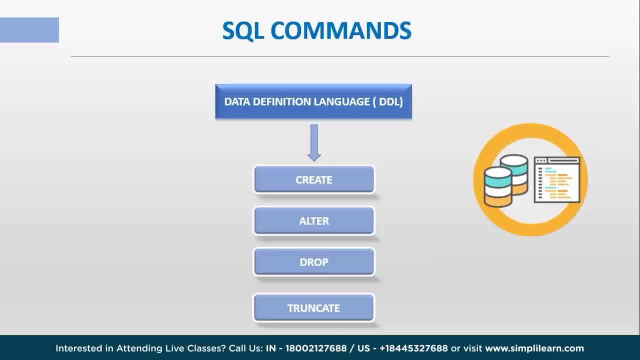 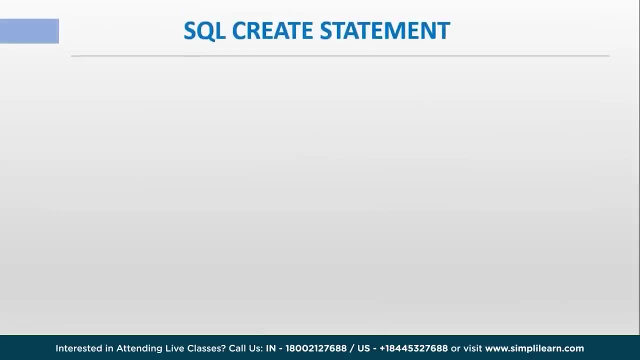 Now that we have got the idea and understanding of various operators, data types and commands, let us look at the syntax of all these commands. The first one is SQL CREATE statement, perhaps one of the most important and used SQL statement, Because if you want to create a table, you have to first name the table and then specify. 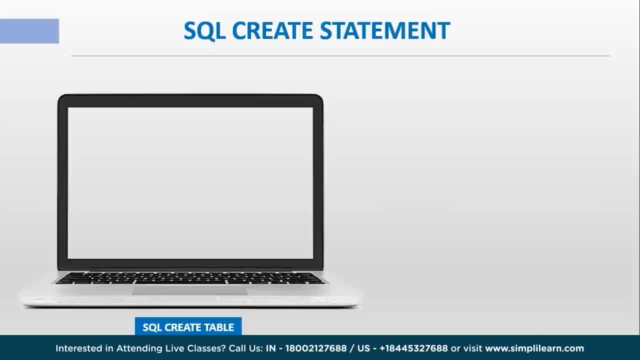 the columns and the column's data types. So let us look at the syntax of CREATE statements. The syntax is followed as CREATE table, which is the keyword that is used, followed by table name that you want to create, And within the parenthesis you have to mention the column, give space and add the data type. 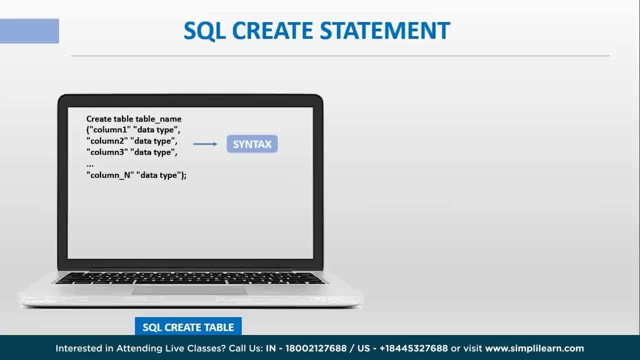 So in this way you can add n number of columns and mention the data types. But make sure, guys, you have to give the appropriate data type for the columns that you have taken, Because there might be an instance where you have given the column, such as age. 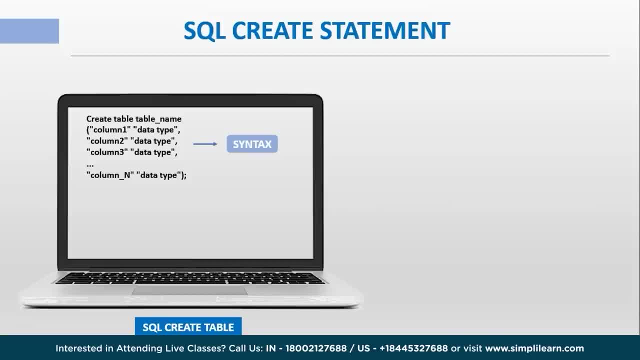 and you are mentioning data type as character char, which is basically a mismatch. The computer doesn't accept it because generally, age is basically a numerical value, but you are mentioning char. but it should ideally be int to store the data. So just keep an eye on it when you are creating your tables. 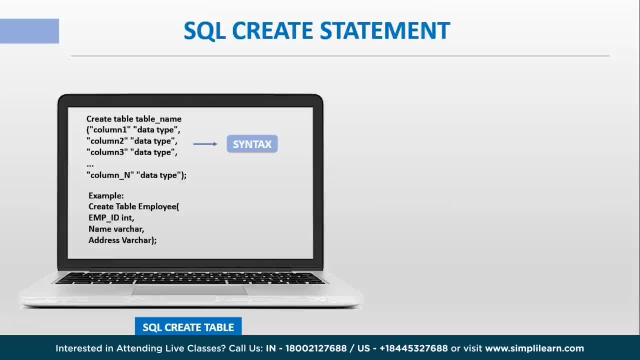 So let us now look at an example of CREATE statement. So I want to create a table named employee. for that I am writing as CREATE table space nth, And within the parenthesis I am mentioning employee ID as my first column. space int. 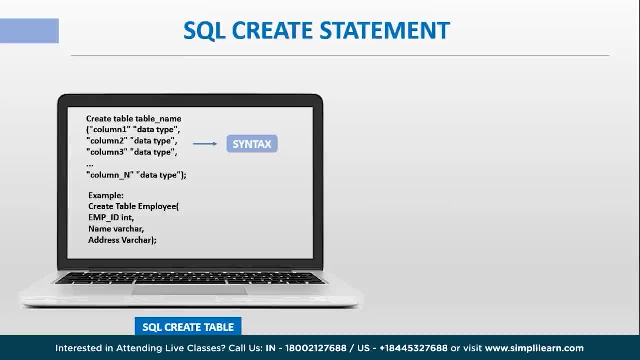 which is the data type and I am giving name varchar, address varchar. close the parenthesis and put a semicolon, And if you execute this statement, this will be the following result: It will display the table with different columns, with the first column as employee ID. 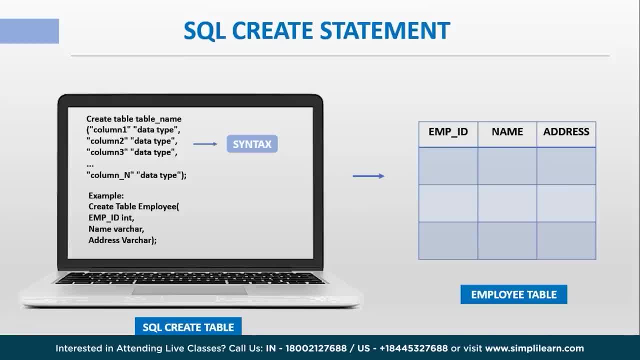 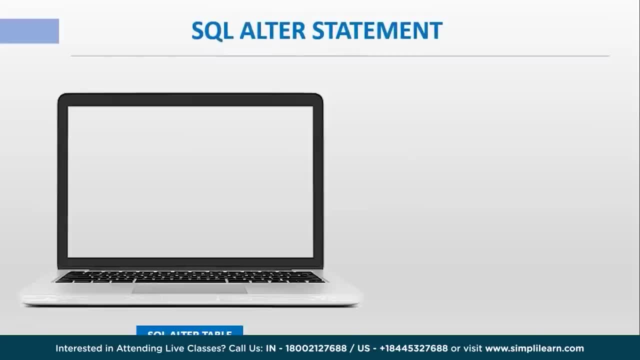 the second column as name and the third column as address. Easy right. The next one is SQL ALTER table. The SQL ALTER statement is basically used to add, modify or even delete certain columns from the existing table. Let us look at the syntax of SQL ALTER command. 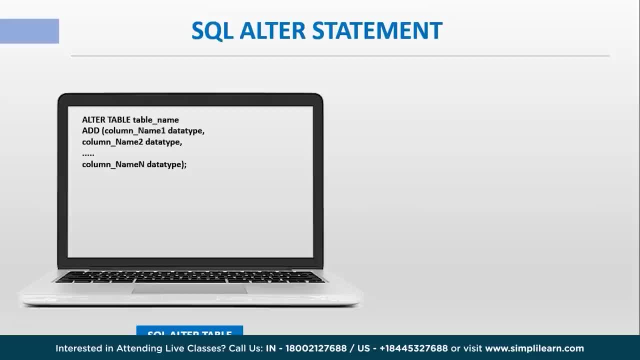 So the SQL ALTER command is ALTER table space, table name. that you have to mention add, and within the parenthesis you have to mention the column and the data type. Similarly, you can add a number of data types as per your requirement. 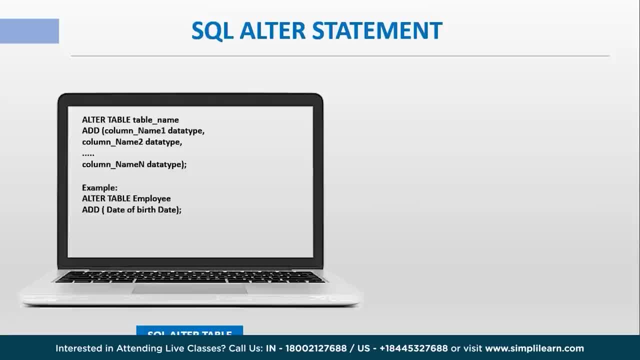 Let us now look at one of the example. Now I wanted to add the date of birth of the employee in a new column. For that I'll write as ALTER table employee add, and within the parenthesis, date of birth, And I'll mention the data type as well, which is the date. And if you execute this, 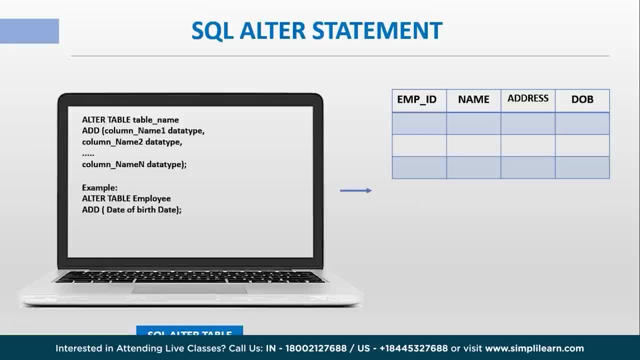 it will show the result like this: It will add another column- date of birth- in the already existing table. Now, due to certain reasons, if you want to drop or delete the date of birth column for that we have to write syntax as ALTER table. give the employee table name: drop. 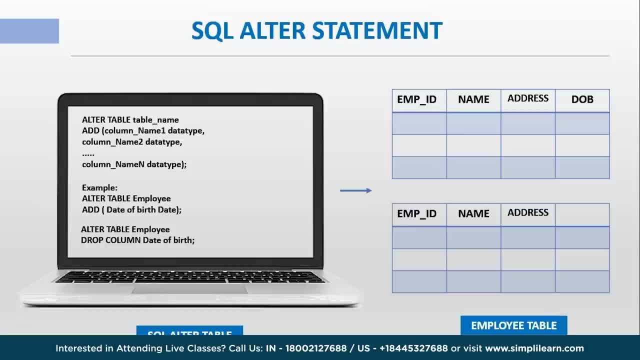 column, which is the keyword we use, and date of birth. So this will be the final output when you execute the query. It will completely drop the date of birth from the table. Next we'll look at SQL DROP statement. SQL DROP statement. 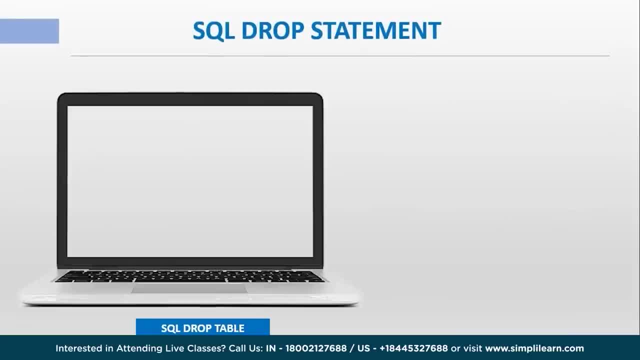 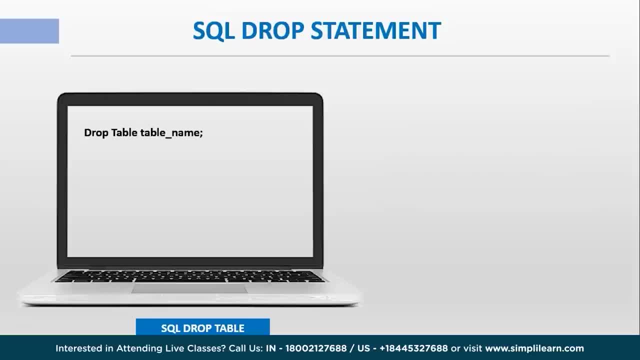 So let us look at the syntax. The syntax followed is a drop table followed by the table name that we want to create, And let us look one of the example. The syntax followed is a drop table employee And when I execute this, it will show an error stating that table name. 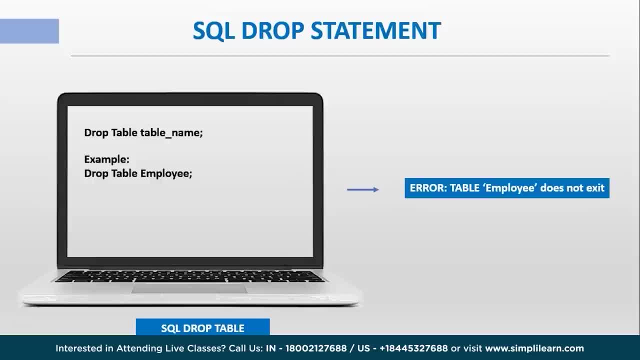 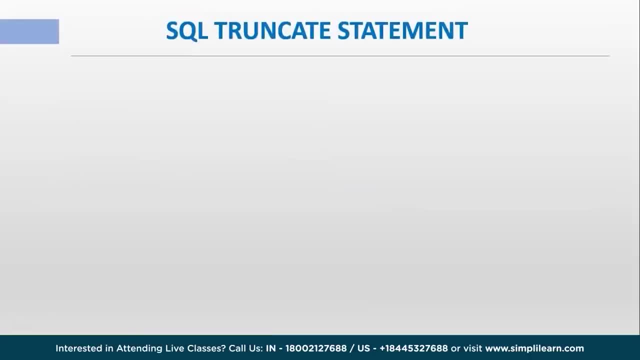 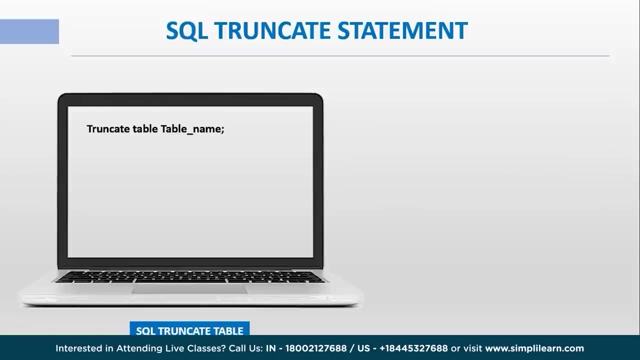 employee does not exist, which means you have completely deleted all the records from the employee table. SQL truncate statement. Let us look at the SQL truncate statement syntax. The syntax is truncate table, which is the keyword that is used, and we have to specify the table name. 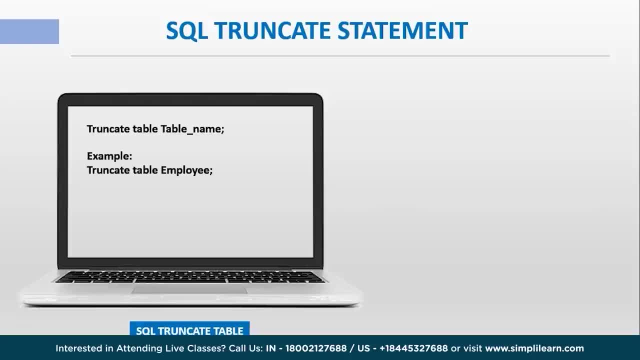 For example, if you want to truncate the values in employee table, we have to write truncate table- employee. So this will be the output where it shows null, that is, there are no values in the employee table, and you can further add values of your own choice. 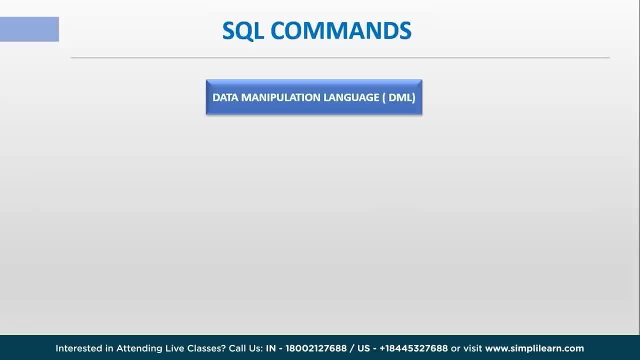 Let us now look at data manipulation language. Data manipulation language, or DML, is used to access and manipulate data tables. Commands that are used in DML are: insert- It is used to insert new values into the table. Select- It is used to extract data from the tables. 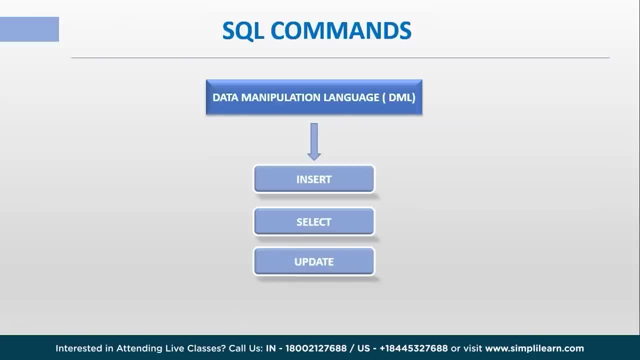 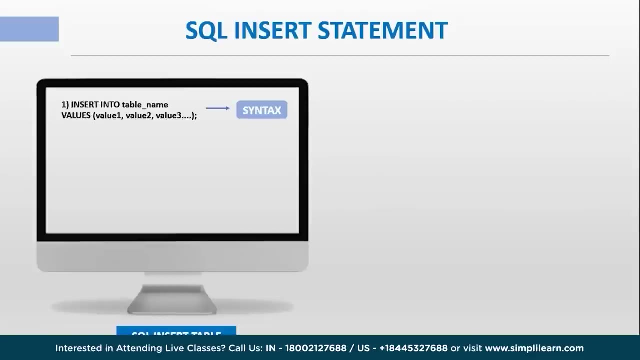 Update: It is used to update values in the already existing table. Delete: Unlike the drop command, delete command is used to delete a specific row or all the rows in the table. Let us first look at the SQL insert statement. The syntax followed in SQL insert statement is insert into: 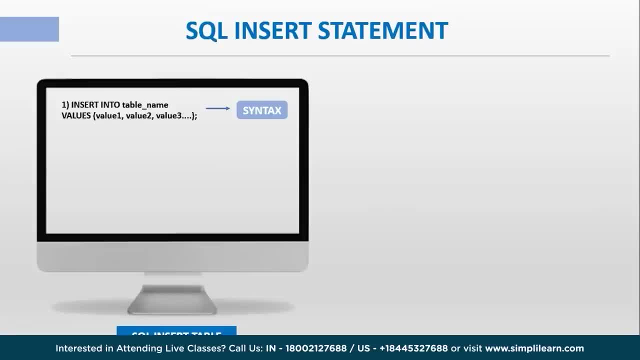 which is the keyword that we use. It is used to insert the table name, space, table name, that we have created values, and inside the parenthesis you have to mention the values. There is also another method to insert the values, where we specify the column name as well as the. 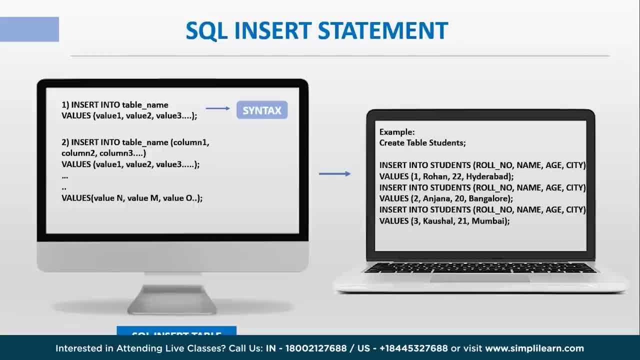 values. Now, if you execute this, So, but before executing will take an example. we are creating a table- student- and we are inserting values such as role number, name, age and city. So the role number is given as one, The name is given as Rohan. 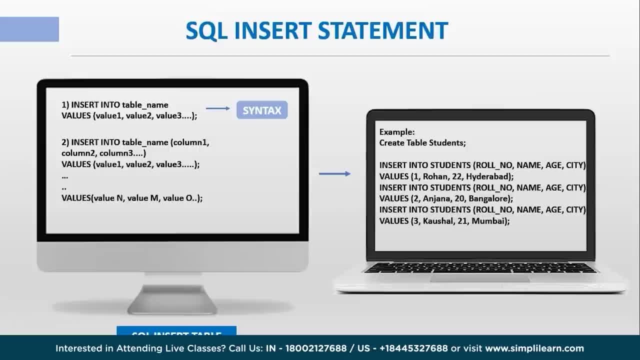 The age is given as 22 and the city is given as Hyderabad for the first row. Similarly, we'll do the same for the next two rows as well, and if you execute this query, this will be the final output, where you will have four different columns having. 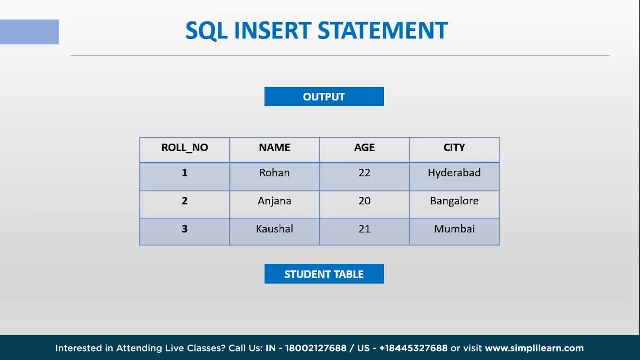 the first column as role number, The next one having name age, city, with the role numbers as one: Rohan, age and city. So we are giving Rohan, 22, Hyderabad, and the second row consists of the role number two, Anjana, age being 20 and the city Bangalore. 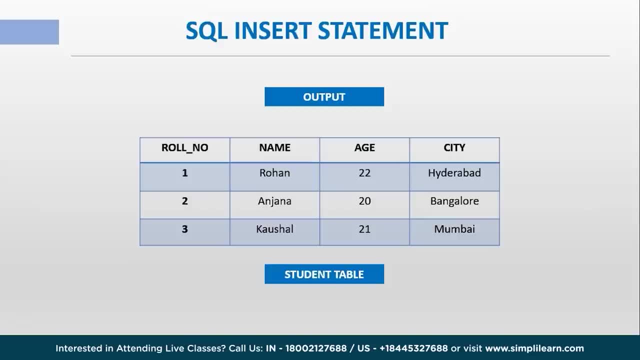 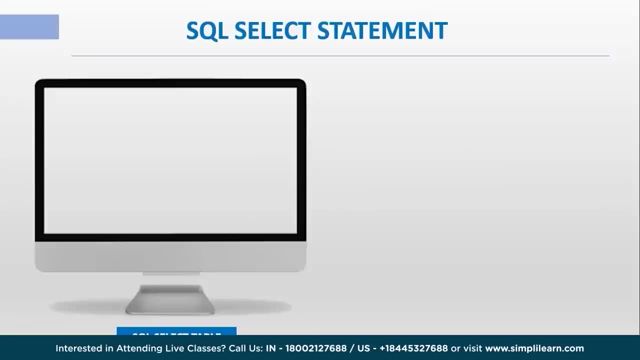 and the third one is role number three. The name is Kaushal, age 21, and the city is Mumbai. SQL SELECT statement. Let us now look at the syntax of SQL SELECT statement. The SQL is followed. The syntax is followed as: select column 1, column 2 and n number of columns. 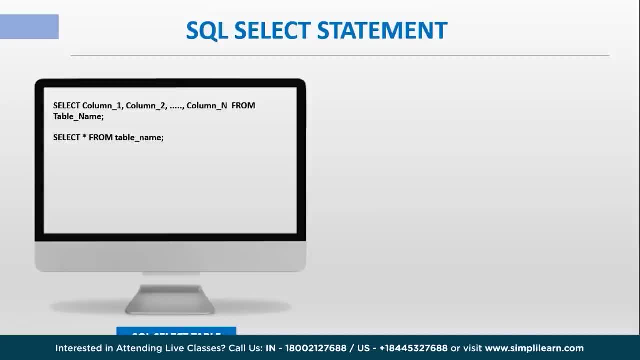 from the table name And if you want to display all the names from the table you have to use asterisk, that is, select star from table name. Let us look at the example. So I want to display the role, number, name, age from the student table. For that I'll write. 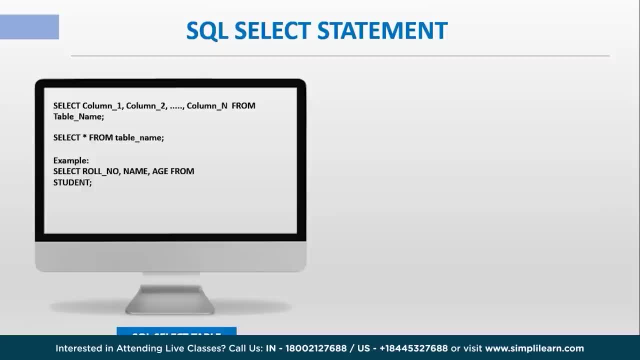 SELECT role number, comma, name, comma, age from the table that is student. and if I execute this, it will only display a role number, name, age of the students and it will not display the city of the students And, if you want to display, even the city to which they belong. 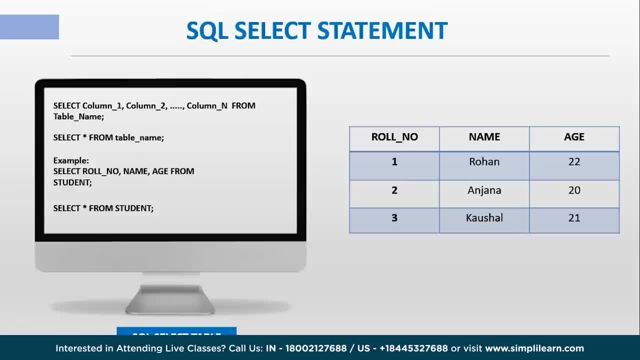 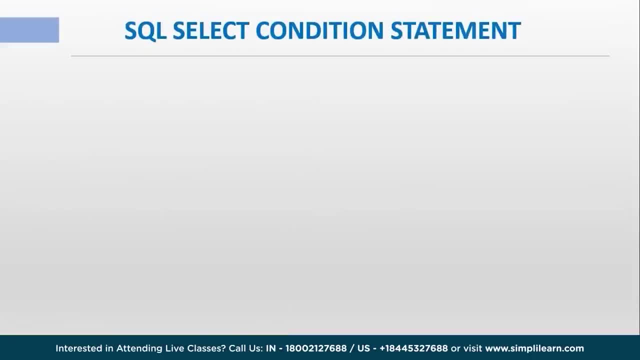 we have to write SELECT star from student, Then it will display even the city in the table. SQL SELECT condition statement. Consider the employed table with having ID, name, age, city and salary And if you want to specifically, you know, display. 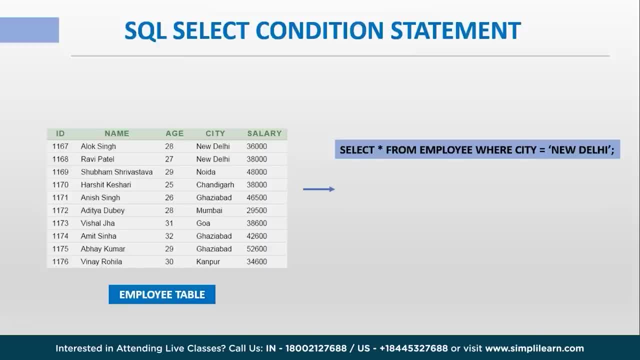 the, the name of the student and the age of the student. you have to write SELECT star from employee, where city is equal to New Delhi. Here we are applying a condition, that is, WHERE, which is a SQL clause, and we are using an operator as well, which is equal. 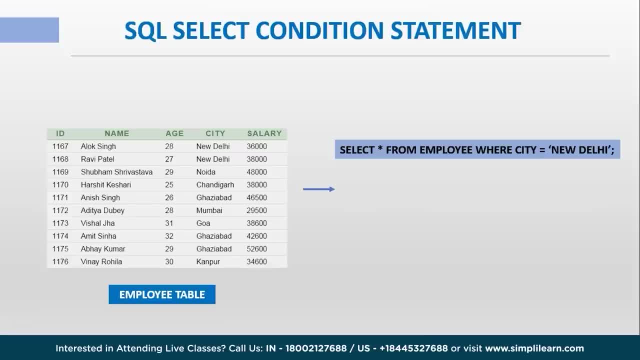 to: And. if you execute this statement, it will show this as output, where you will find the ID of Alok Singh Ravi Patel, who belonged to the city New Delhi. SQL SELECT statement. And if you execute this statement, it will show this as output where you will find the ID of Alok Singh Ravi Patel, who belonged to the city New Delhi. 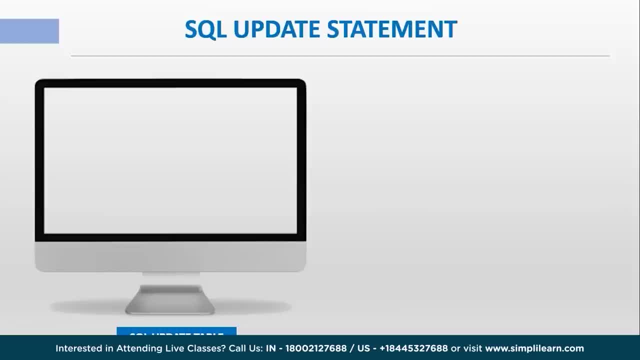 And again, this is our SQL update statement. It is used to update existing values in the statement. For example, if you consider the syntax, it is followed as: update space table Name that you have created. set column name equals to new. 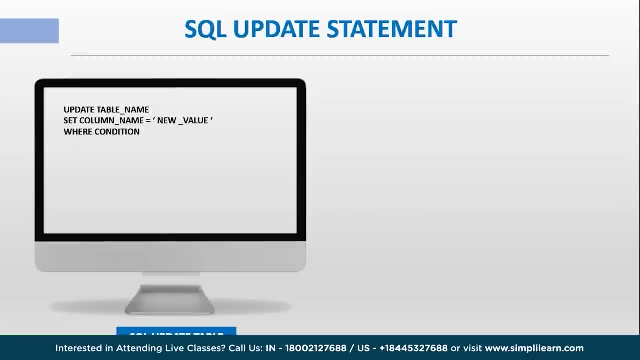 value. That is the updated value that you want to keep in to the new table- And you have two- can keep a condition as well. That is WHERE condition. let us look at example now. if you want to update the student table And if I want to insert 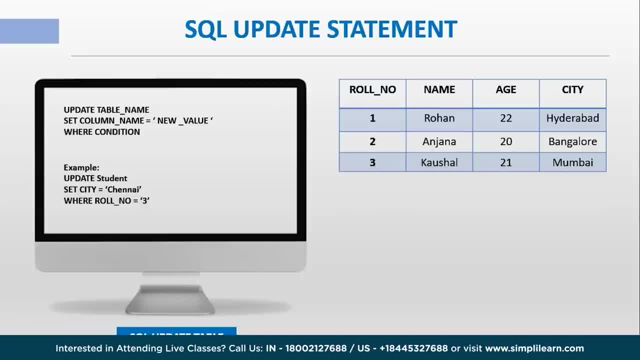 if I want to change the city of the role number 3, that is, Kaushal's city, I'll write as update: student set city equals to Chennai, where role number is equals to 3, and when you execute this it will show like this: so the city, which is Mumbai, has been changed into Chennai. 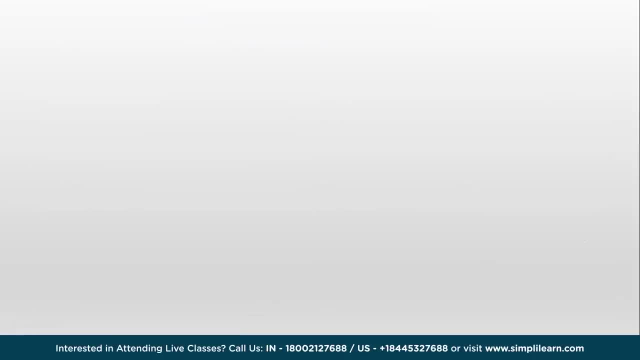 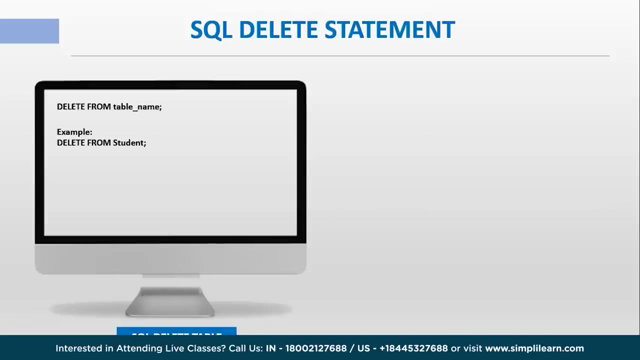 SQL delete statement. SQL delete statement is used to delete a specific row or even all the rows from the table. the syntax is delete from table name. for example, if you want to delete all the records from the student table, we'll write it as delete from student semicolon. so 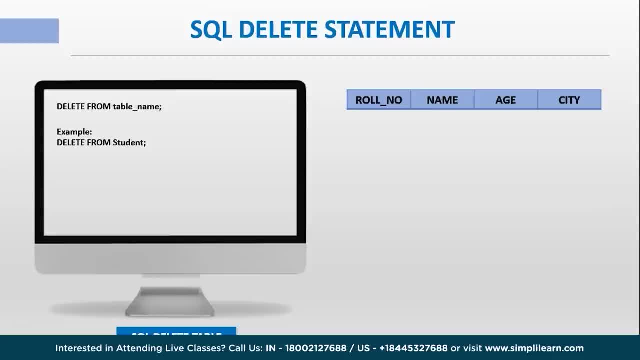 this will be the output. it will only display the column names and the data inside. it will be completely erased and if you want to delete only a certain number of rows, we have to use query as delete from student where role number is equals to 1 and. 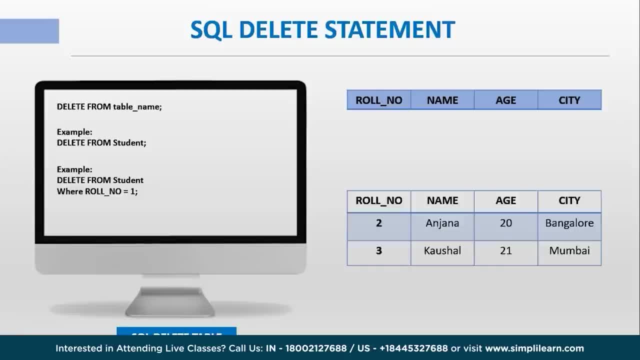 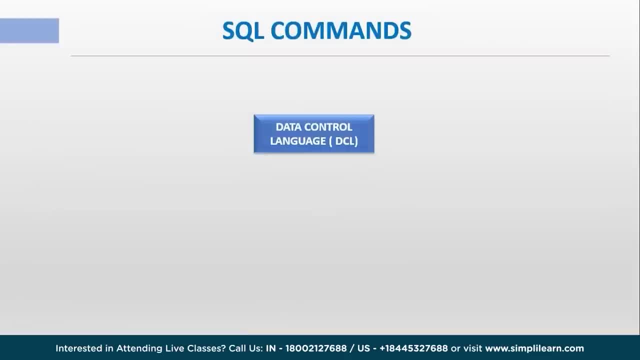 when you execute this query, it will show like this: it will completely erase the records of the role number 1, student. and the final one is data control language, or DCL. DCL is responsible for maintaining the data control language and the data control language is responsible for maintaining the data control language and the data control language is responsible. 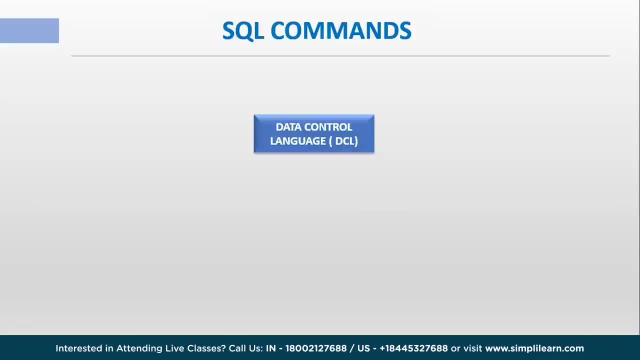 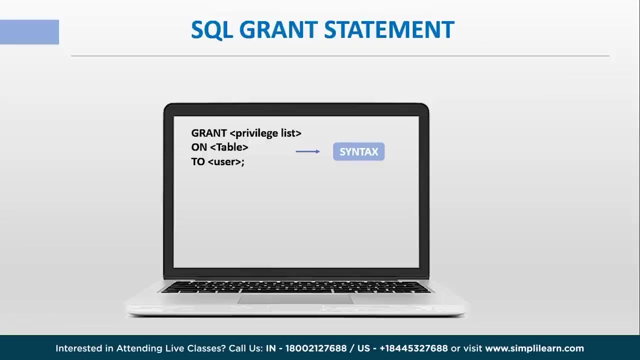 for maintaining the security which gives control, access and permissions of the database commands that come under DCLR. grant: it is used to grant the permission to user to access the database. revoke: it is used to cancel or take back the permissions that were earlier granted. let us now look at SQL grant statement. sometimes user is restricted from creating or making any changes. 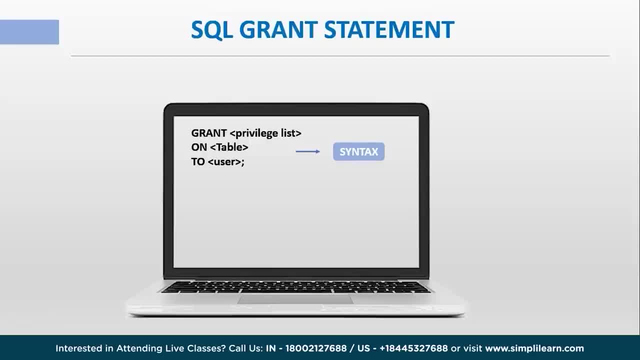 within the table, but with the help of grant statement we can give privilege to the user to create or modify the records in the table. let us now look at the syntax of SQL grant statement. it is followed as grant space privilege list. that is basically the set of commands that you are giving. 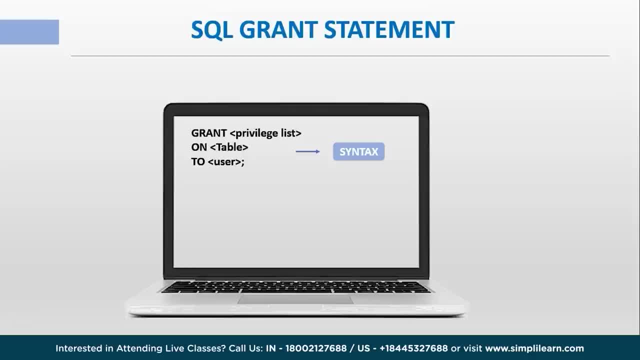 access of permission to the user to perform certain operations on the table that you have created to user. we have to mention the username. example: grant, insert, select on employee to Rahul. that means Rahul is able to access the employee to Rahul. that means Rahul is able to access the. 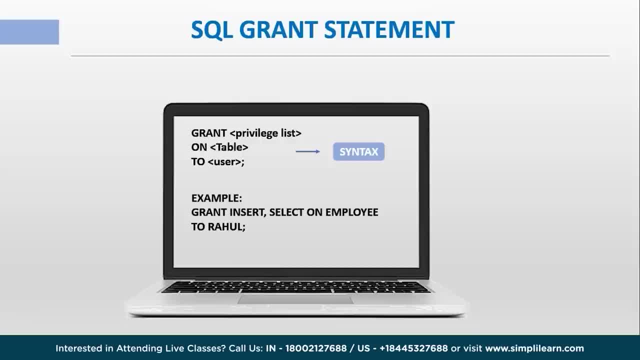 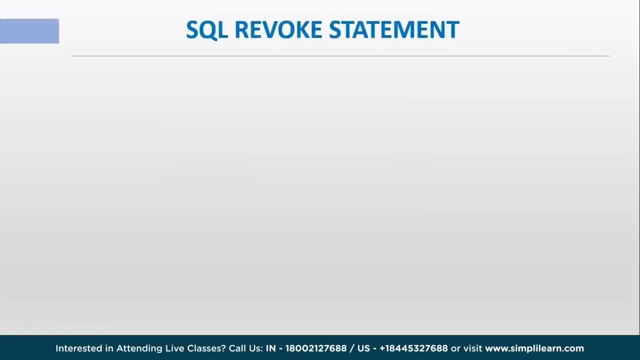 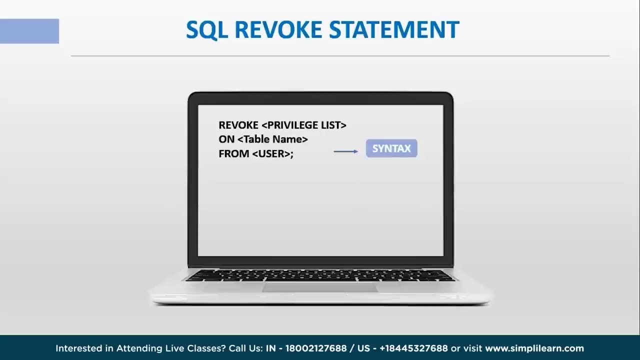 employee table and can perform commands such as insert and select SQL revoke statement. SQL revoke statement is basically the opposite of grant statement. it is used to take back the permissions that were earlier granted. the similar the syntax is also similar to the grant statement. instead of grant keyword, you have to replace it by revoke. let us look at the example: revoke insert on employee. 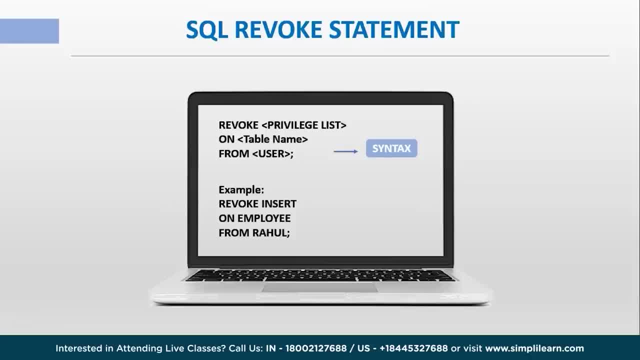 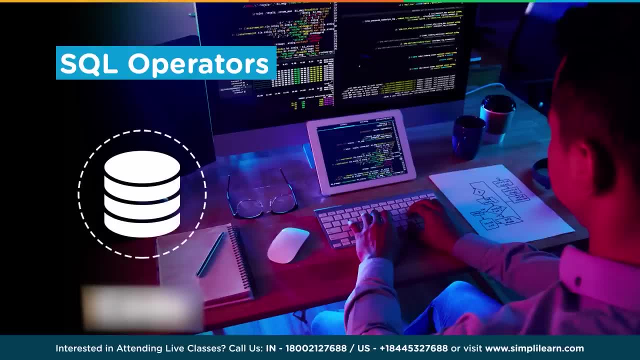 from Rahul. that means Rahul is able to access the employee to Rahul. that means Rahul is able to access the employee to Rahul. that means Rahul is no longer able to insert new values into the employee table. let us dive straight into today's topic on SQL operators. firstly, let us discuss the 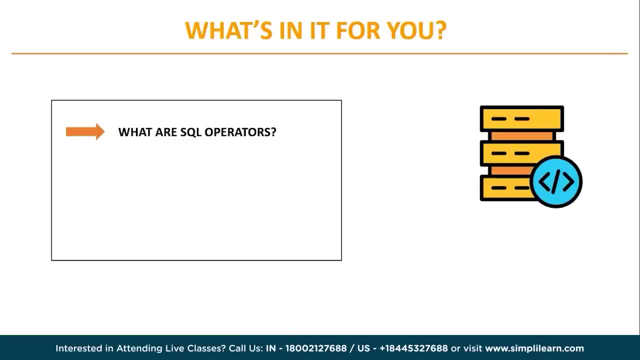 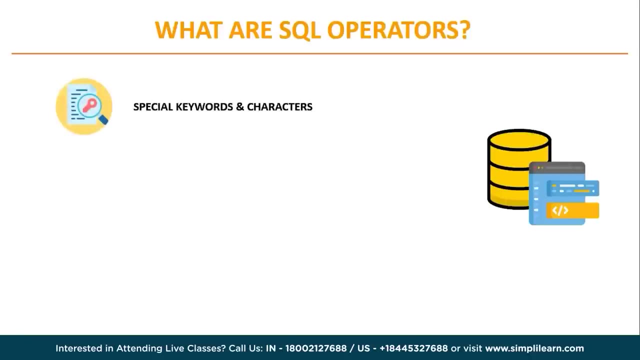 agenda for today's session. we'll start the tutorial by understanding what SQL operators are, then we'll go through different types of SQL operators and finally we'll look at the syntax of various operators and execute them in mysql workbench. what are SQL operators? SQL operators are basically. 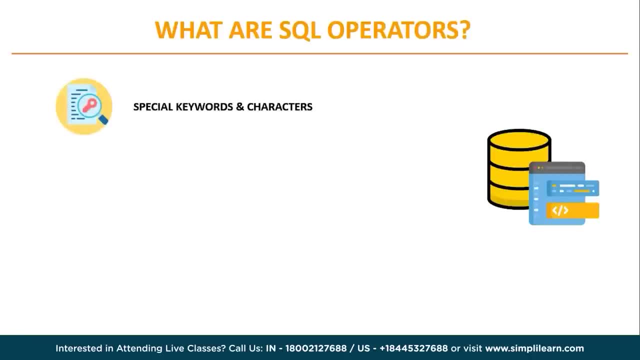 words or special characters that are used to query a database. SQL provides us with many such operators to ease the process of data manipulation. SQL operators are used to perform various tasks, including complex mathematical operations like arithmetic and binary. to query a database using operators, we use a var clause. operators are necessary to define a condition in SQL as they act. 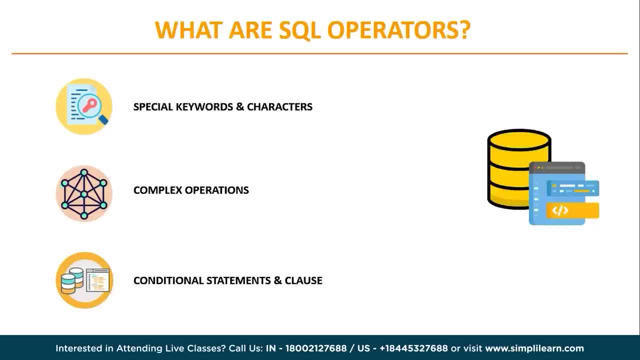 SQL operators are necessary to define a condition in SQL as they act as a connector between two or more SQL operators. as they act as a connector between two or more SQL operators, SQL statements Based on the operator functionality. it manipulates the data accordingly and gives. 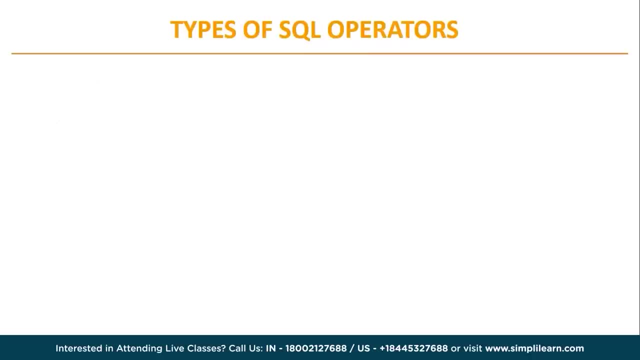 the result. Types of SQL Operators. SQL operators are mainly classified into three types. The first one is arithmetic operators. The arithmetic operators perform the mathematical operation on numerical data of SQL tables. They are further classified as addition operator. The addition operator is used to perform addition on numerical data. Using this, we can add: 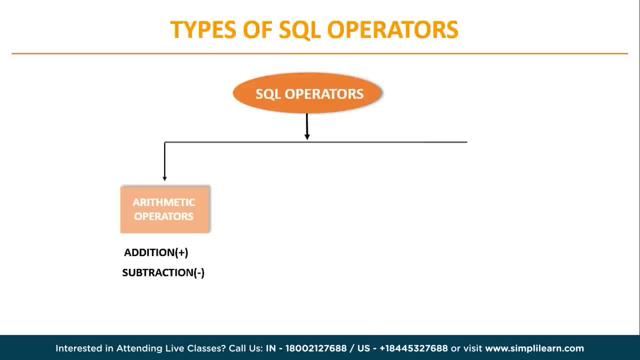 values of single or multiple columns in a table. Subtraction Operator. Subtraction Operator in SQL performs the subtraction on the numerical data of the database. table Multiplication Operator: Multiplication Operator in SQL performs multiplication on the data items. In SQL, we can easily multiply the numerical values of two or more columns. 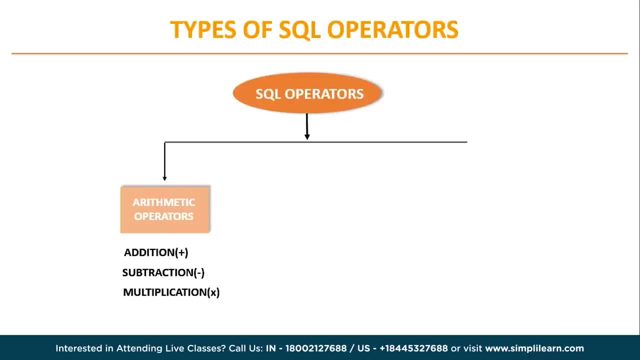 of the same table by specifying both North and Westということ column names as the first and second operand. And finally, division operator. Division operator in SQL divides the operand on the left side by the operand on the right side. We can also divide the numerical values of one column by another column of the same table. 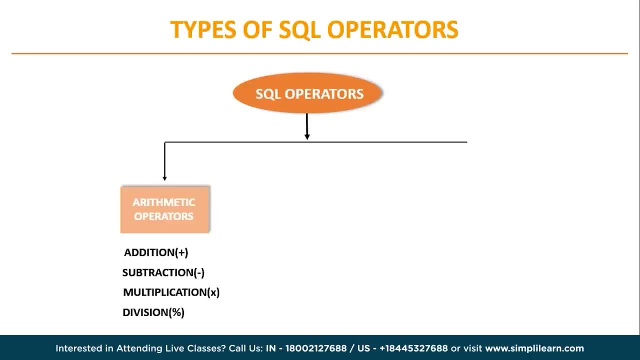 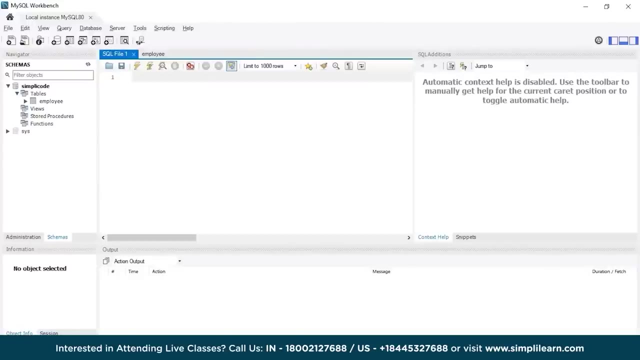 by specifying both column names as the first and second operand. Let us now look at the execution part of the arithmetic operations on MySQL Workbench. As you can see, Workbench has started, But before we proceed to the syntax of SQL operators, we have to first create a database. 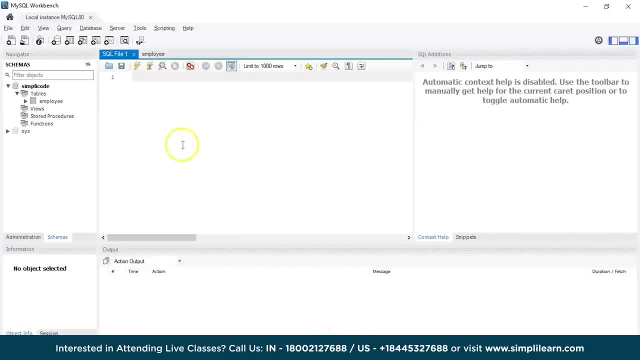 and then we have to create a table within the database. So for time being, I've already created a table named employee. So let us just briefly go through the syntax of create table. So the syntax is followed as create table space. Now we can declare the employee- that is the table name- in two ways. 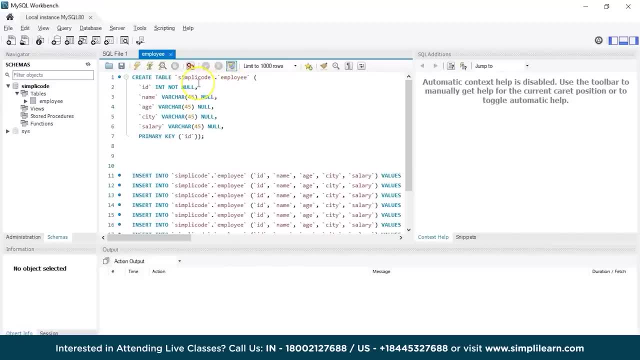 That is, you can directly mention the table name that is employee, Or else you can mention database dot table name that is employee And after that, in the parenthesis, you have to mention the column names followed by its appropriate data types. So as far as this table employee is concerned, I have taken column names as ID name. age: 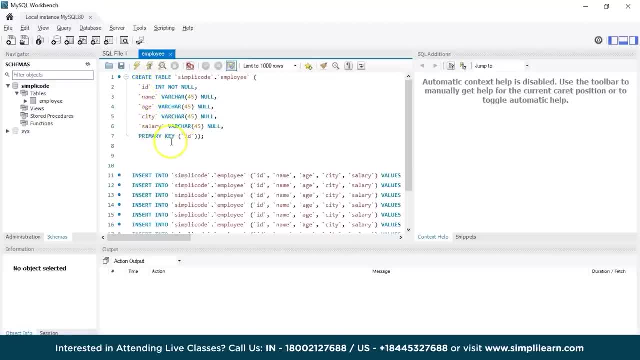 city and salary. And also I've chosen primary key as ID, as it uniquely identifies each and every record in the table. Close the parenthesis And put a semicolon. Now that you have created a table, you have to insert values into the table. 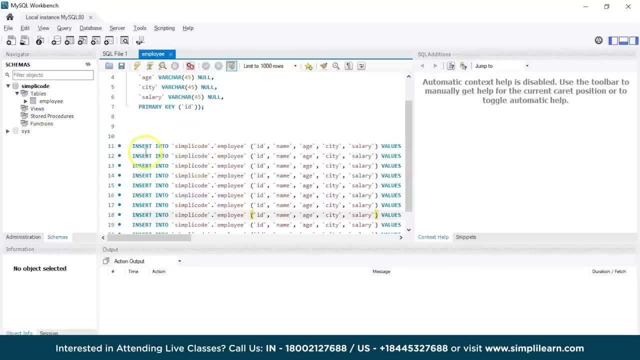 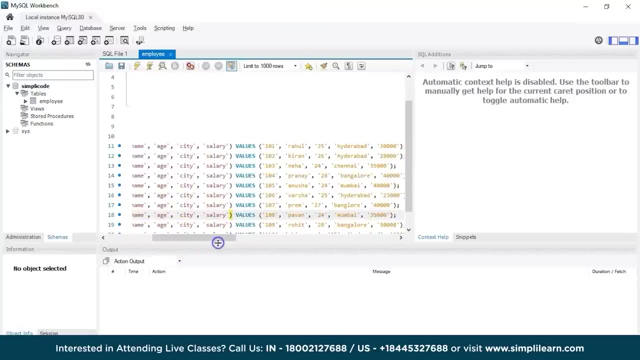 And for that we use insert command. So the syntax for insert command is: insert into space table name, that is, employee, And within the parenthesis you have to mention all the column names that you have taken in the single quotes. After that, close the parenthesis and you have to write values, which is the keyword. 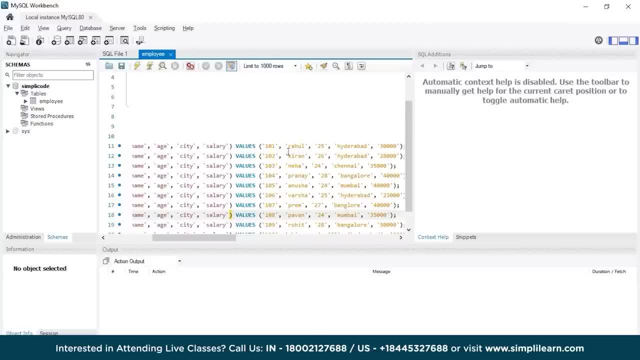 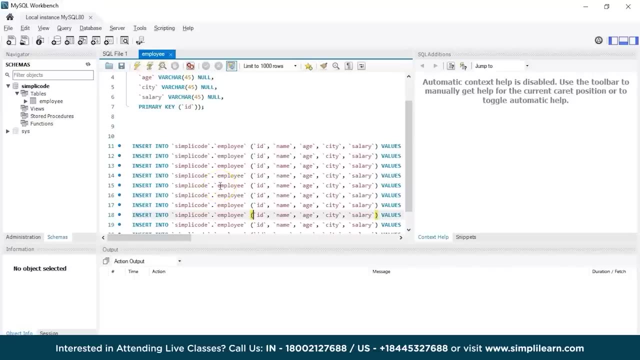 and mention. You have to write different values as per your choice. accordingly that you have taken into the columns. So in this way you can insert N number of records into the table using insert command. For this employee table I've taken values. total of 10 values. 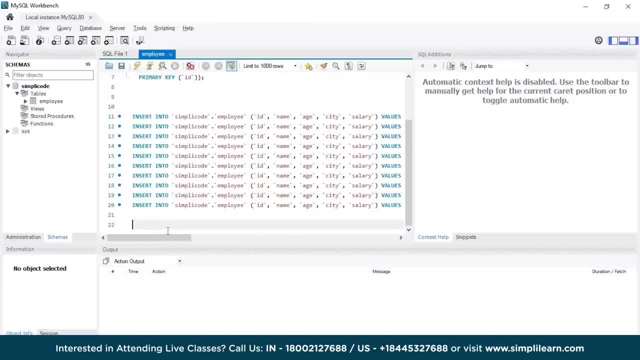 Now that you've created and inserted values into your table and if you want to display all the records of the employees You have to write, We have to have a set of records Here to select the query as select star from the table name, that is, employee and when. 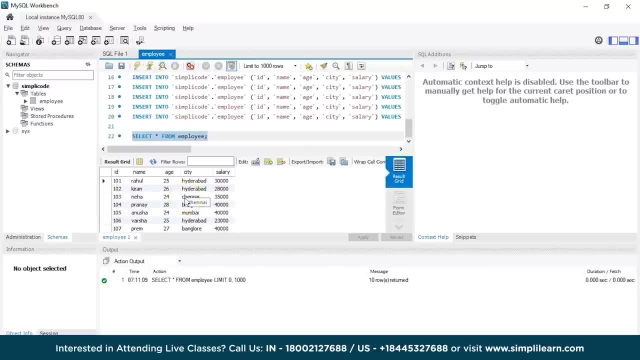 you execute this, it will show the records of all the employees that you have taken, that is, their ID, the name, age, city and salary. so we have taken total 10 values and it will be displayed. now that we have understood all these, let us proceed with the SQL operators. first, let us look at addition operator. let us understand this with the help of an example. suppose you want to add 10,000 to the salary of each employee specified in the table, then we have to write the query as select salary plus 10,000. as I am taking a new column, that is employee, new salary to. specify all these values into the column as employee: new salary from the table name that is employee. now, when you execute this, it will show the result like this, that is, it will add 10,000 to each and everyone's values. that is, 30,000 has been changed into 40,000. 28,000 has been. 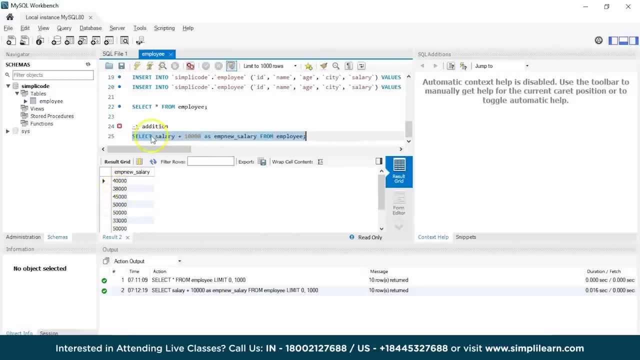 changed into 38,000 and so on. now, if I want to display their ID name, their previous salary and the final salary simultaneously, I'll write the query as select: ID comma space, name space. salary plus 10,000 as employee. new salary from employee. now, if I execute this, it will. 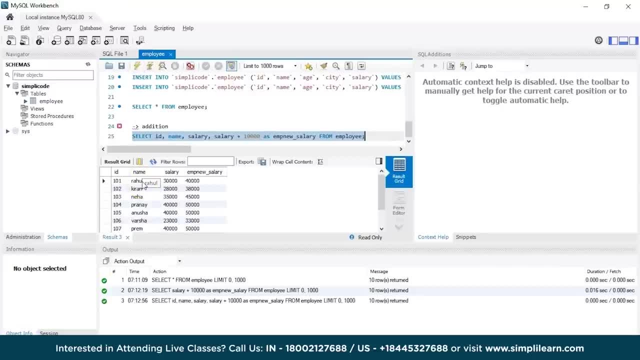 display like this, that is, it will mention the ID name, the previous salary and employee new salary simultaneously. so in this way you can add two or more columns in the same table using addition operator. let us now look at subtraction operator. subtraction operator is also similar to that of addition operator, the 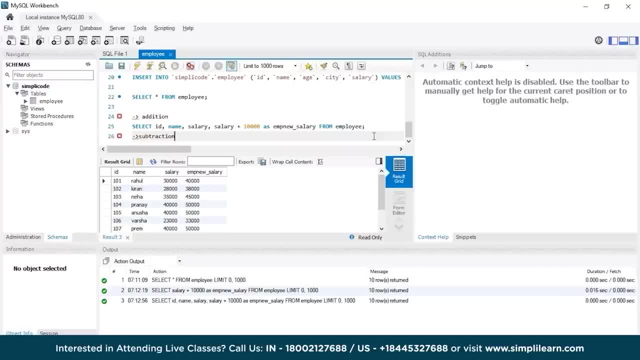 only difference between addition operator and subtraction operator is that it is you have to replace the plus sign with the minus sign. so again for this example, let us say if you want to subtract 2,000 from salary of each employee given in the employee table, then we have to write the query as select: ID, comma, space and. 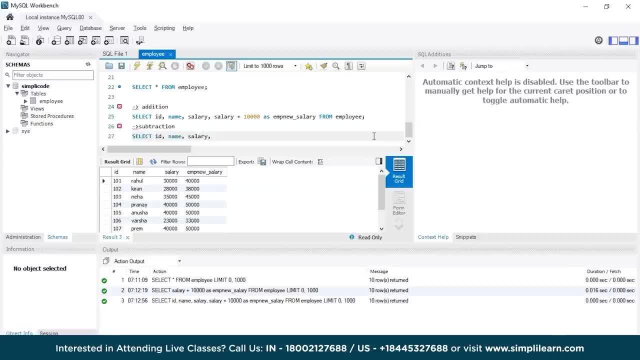 name: comma space salary: comma space salary minus 2,000 as employee: new salary from the table: that is employee. so let us execute this and it will show the new values. that is, 2,000 has been deducted from the salaries of each and every employee, as you can see. 30,000 has been reduced to. 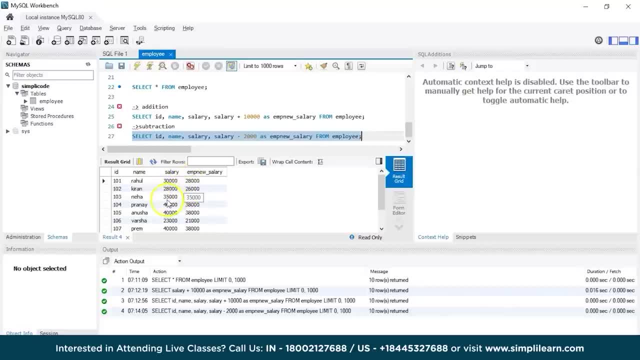 28,000, 28,000 has been reduced to 26,000, 35,000 and 35,000 are reduced to 36,000, 35000 has been reduced to 33000, and so on. so next let us look at the multiplication. 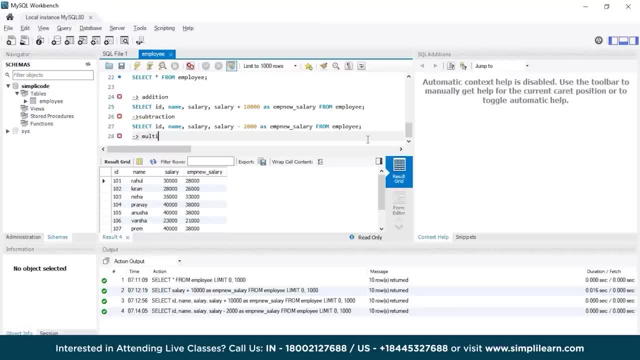 operator. again, let us take the same example. if you want to multiply the salary of each and every employee, then you have to write the query as select ID name- salary salary- into two. we are using hash asterisk operator as the multiplication sign here. as employee, new salary from the table name. 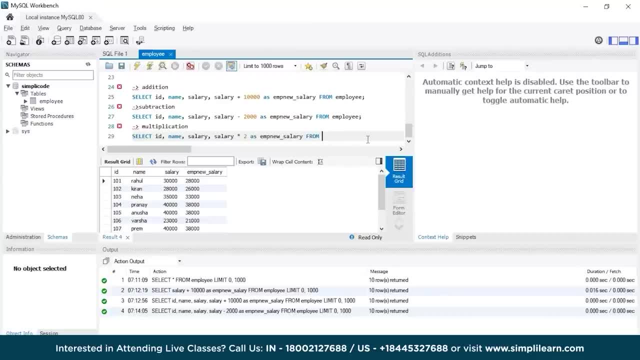 name. that is employee. now, if you execute this, it will show the values like in this way. that is, the salary has been doubled. as you can see, the employer Rahul's salary, 30000, has been multiplied and has changed into 60000. that is doubled. 28000 has been doubled to. 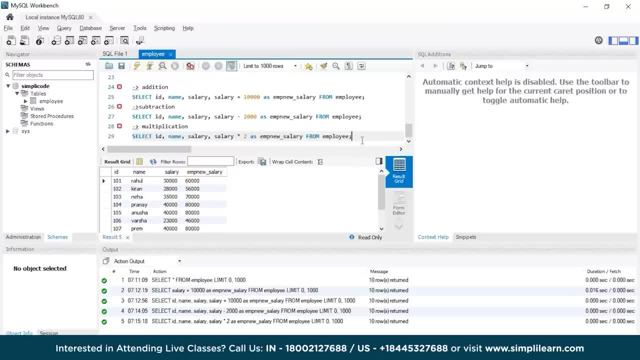 56000 and so on. So in this way you can Apply multiplication operator. and finally, let us look at division operator. let us take the same example, suppose. let's say, if you want to divide the salary of each and every employee, then you have to write the query as select ID name: salary. salary divided by. 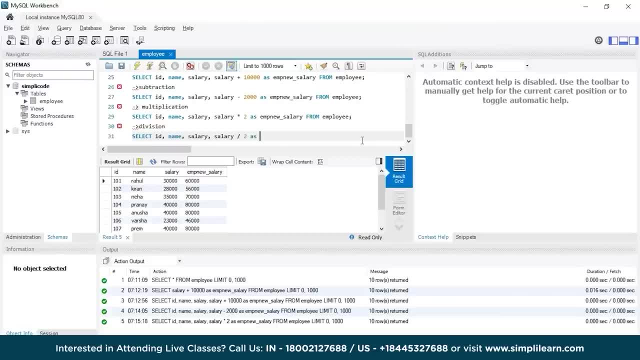 two As A D H C, H D H H, B D C, D A D H H D D C, H A C D C. 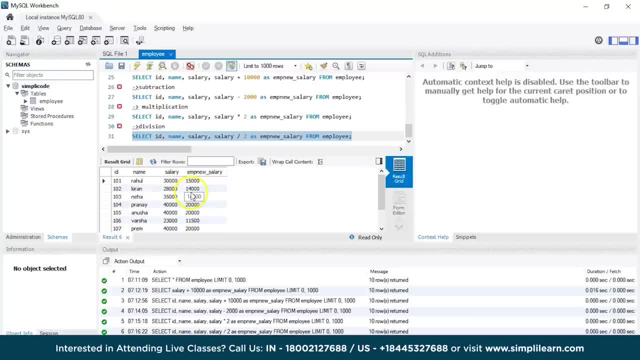 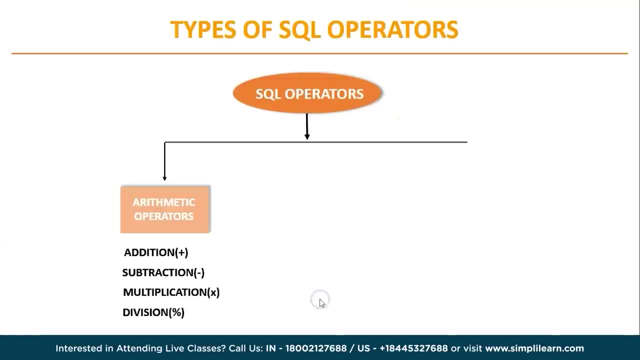 H D, C D D H H. use arithmetic operations to perform various operations on your table, ie: addition, subtraction, multiplication and division. The second type of SQL operators are comparison operators. The comparison operators in SQL compares two different data of SQL tables and check whether. 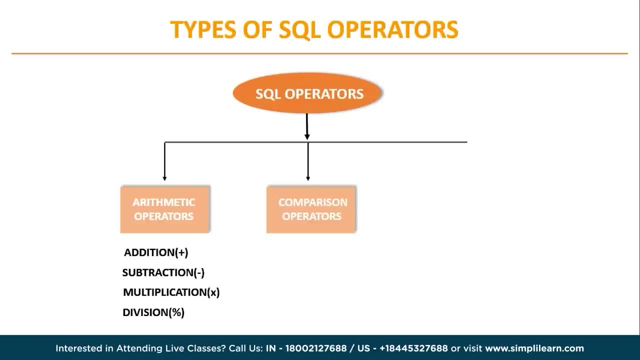 they are same, greater and lesser. The SQL comparison operators are used with the conditional clause var. in the SQL queries. They are again further divided into various types. The first one is equal to SQL. equal to operator is one of the popular and most frequently used operators in SQL. 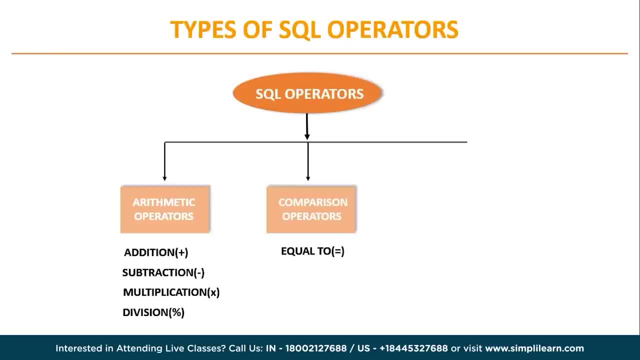 queries. It shows only that data which matches the specified value in the query. Less than The less than operator in SQL shows only those data from the database tables which are less than the value of the right hand side operand. Greater than The greater than operator in SQL shows only those data which are greater than the value. 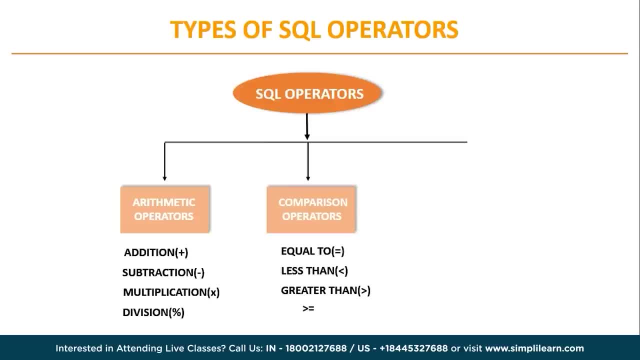 of the right hand operand. We also have less than equals to and greater than equals to operators as well, which basically shows the data in the tables which are less than and equals to, as well as greater than and equals to, the value of the right hand operands. 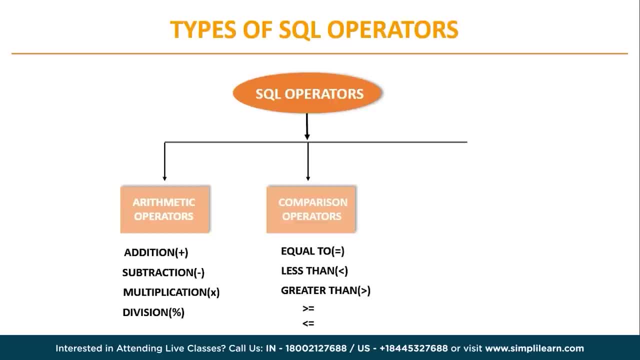 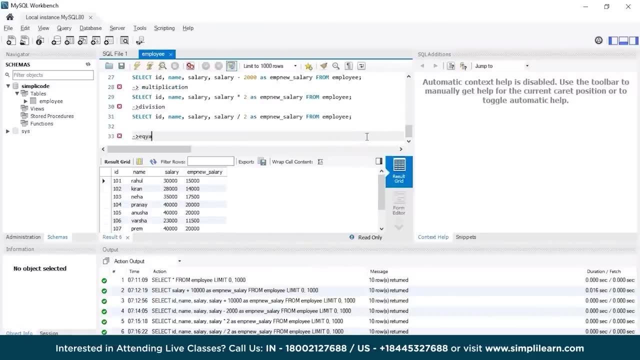 Let us look at the syntax and execute them in the workbench. Firstly, let us look at the equal to operator. Let's say, if you want to access the records of all those employees who are working on the workbench, You are having salary equals to 40,000.. 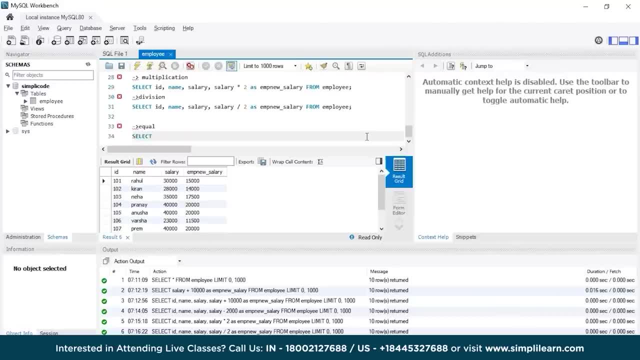 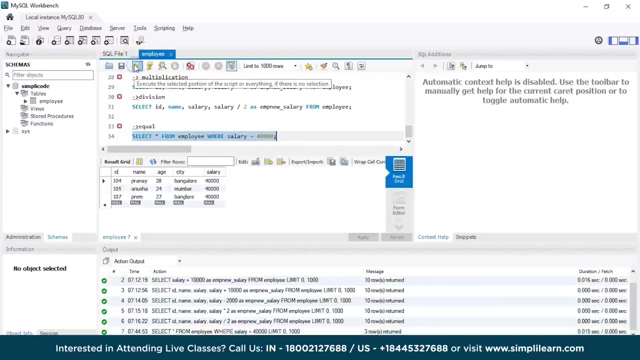 So for that we will write the query as SELECT star from the table that is employee. We have to use the conditional statement where salary is equals to 40,000 and put a semi colon. When you execute this, It will show the records of all those employees. 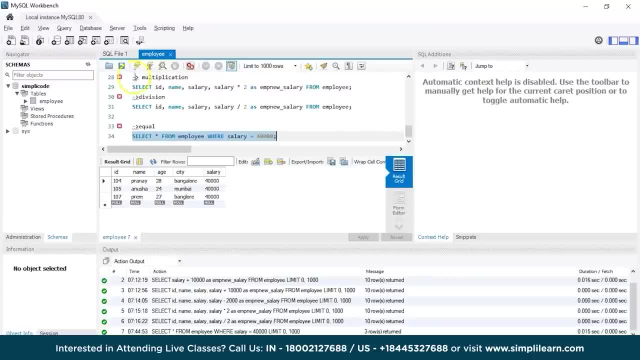 All those employees who are having salary equals to 40,000.. As you can see, it is showing three IDs: Pranay, Anusha and Prem, who are having salary as 40,000.. Next, let us look at not equals to: 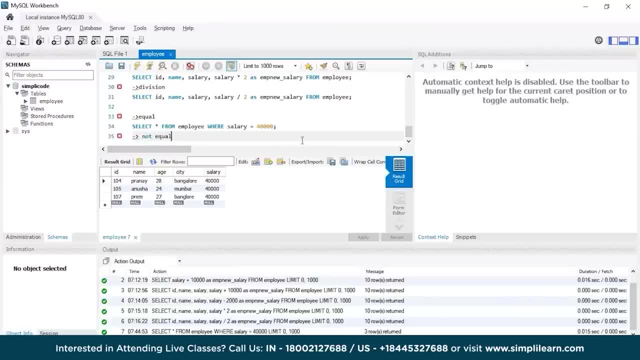 Not equals to is basically the opposite of equal to. and to understand this, let us take an example. Suppose if you want to access the records of all those employees whose salary is not equals to 35,000.. So for that We will write the query. 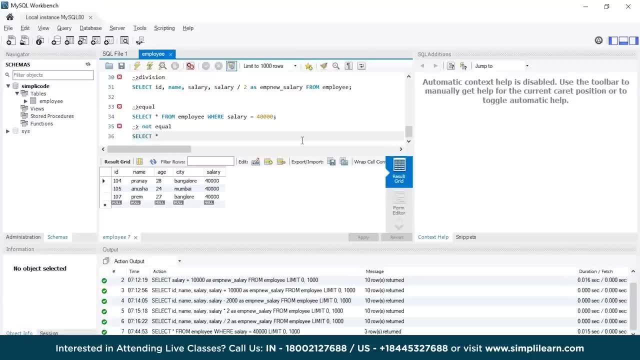 As SELECT star from the table, that is, employee, where let us put the keyword in the upper case where salary not equals to 35,000.. Let us execute this and let us see the output. So, as you can see, It will display the records of all those employees who are not having the salary 35,000. 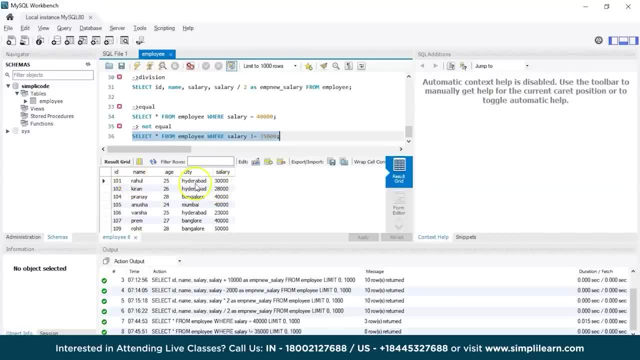 So it will display the records, such as Rahul Kiran, Pranay, Anusha Varsha, who are having salaries as 30,000, 28,000, 40,000, 23,000 and so on, which are basically not equals. 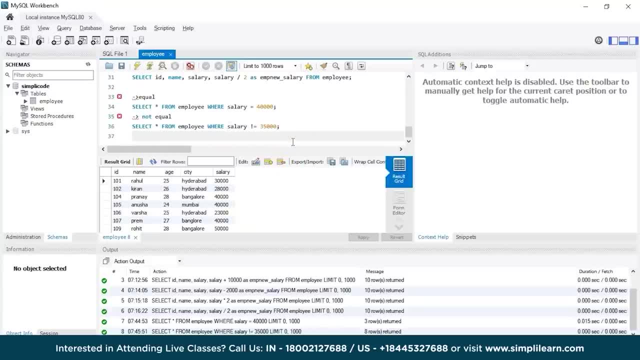 to 35,000.. Next, let us look at greater than operator. For this Let us take an example. for instance, if you want to access the records of all those employees from the employee table whose ID is greater than 104. So for that we will write the following query as SELECT star from the table that is employee. 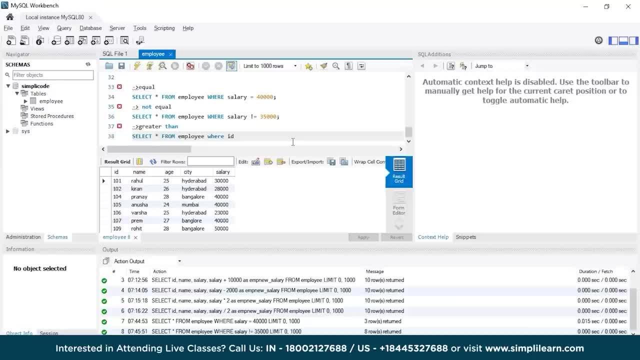 where ID greater than 104.. Put a second query, Put a semicolon and let us execute this So, as you can see, it will display the records of all those employees who are having ID greater than 104.. That is, it will display from 105 and up until 110.. 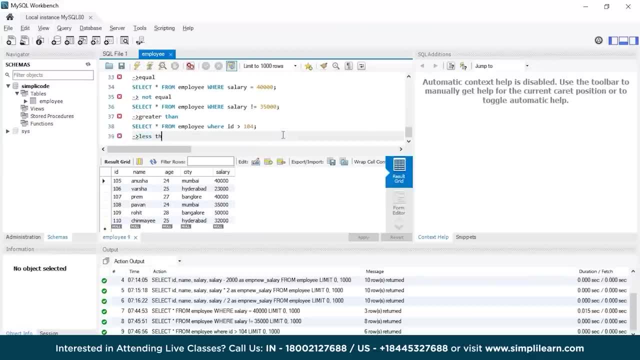 Similarly, we have the less than operator as well, which is basically the opposite of greater than operator. For that We will take an example. Let us take an example. Let us take an example Such as: if you want to display the records of all those employees who are having ID less, 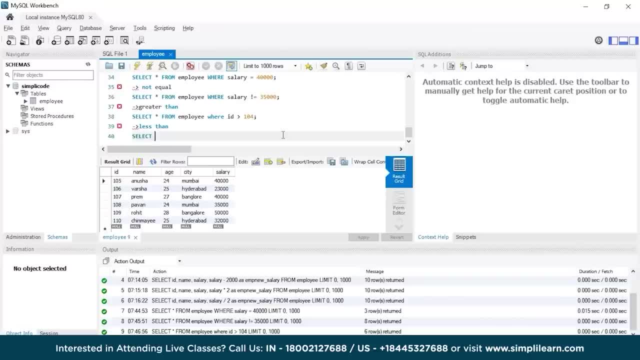 than 105.. So for that we will write the query as SELECT star from the table, that is, employee where ID is less than 105.. Let us execute this So, as you can see, it will display all those records of the employees who are having less. 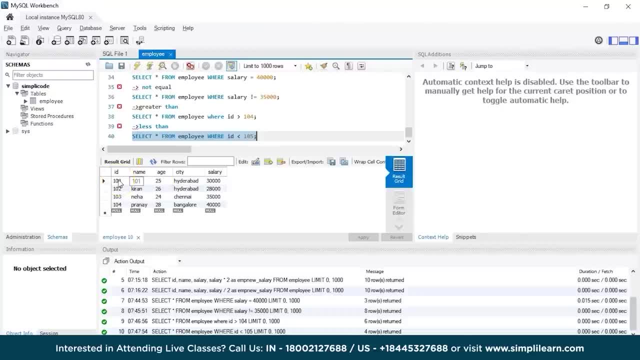 than 105. That is, it will display the records of the employees: 101,, 102,, 103 and 104 IDs. Next, let us look at a greater than equals to. Greater than equals to is what Is greater than equals to. 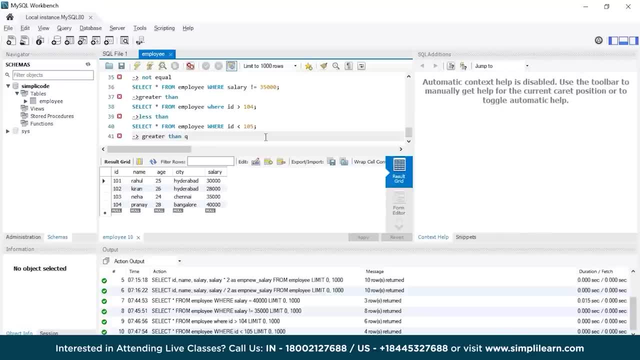 Is greater than equals to. The language of greater than equals to is what Is not equal to, or冑on, But it is more than or equal to. This is a, where g is less than, when the status field is less than and only equals to pluck. 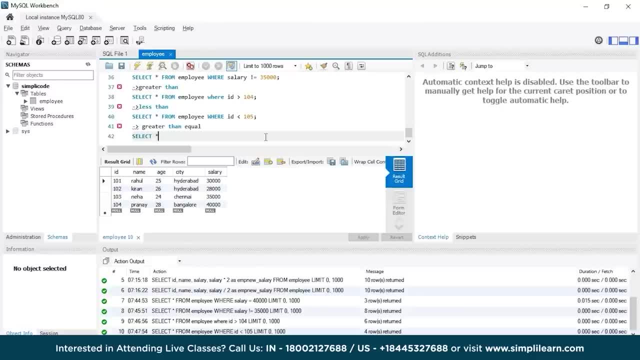 Thrice. In other words, we don't have to fetch this option, But it does exist. What I have shown is mentioning the r comma, and greater than equals operate as well salary greater than equals to 40,000.. Let us execute this and this will be the output. it will show the records of all those employees. 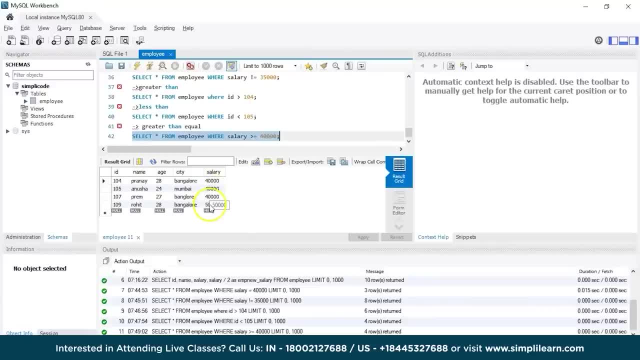 who are having salary greater than or equals to 40,000.. So in this case, it will display a total of four records of the employee table. Similarly, let us look at the less than- equals to operator as well, which basically uses less than and equal to operator. 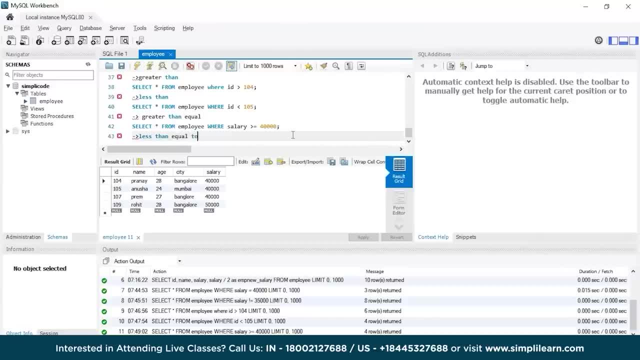 So suppose, if you want to access the records of all those employees from the employee table who's having salary, let's say, less than or equals to 30,000.. So for that we'll have to write the following query as select star: Okay, 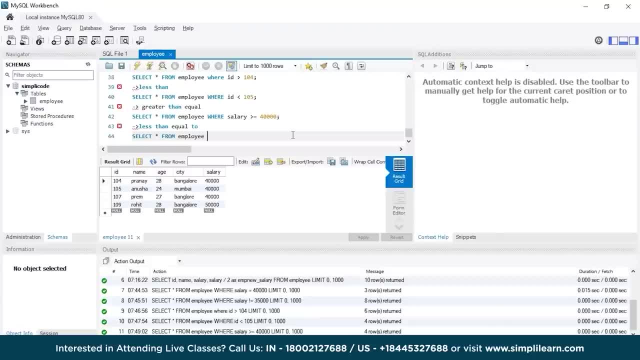 From employee where salary less than or equals to 30,000.. So let us execute this and the output will be like this, That is, it will display all the employer records who are having salary less than or equals to 30,000.. A total of three records. 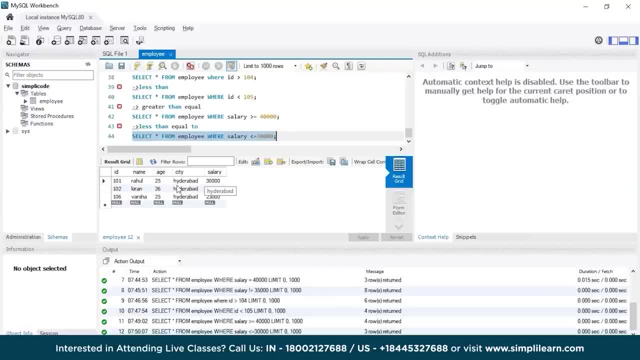 That is, Employee ID is 101, 102, 106 are being displayed because they're having salaries 30,000, 28,000, 23,000, which are basically less than or equals to 30,000.. So in this way, you can use comparison operator to perform various operations on your data. 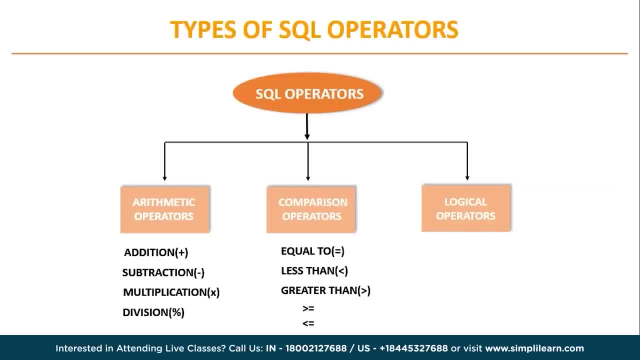 And finally we have logical operators. The logical operators in SQL perform Boolean operations which give two results, either true or false. These operators provide, true or false, The true value if both operands match the logical condition, and vice versa. Various logical operators in SQL are AND OR NOT, and BETWEEN. 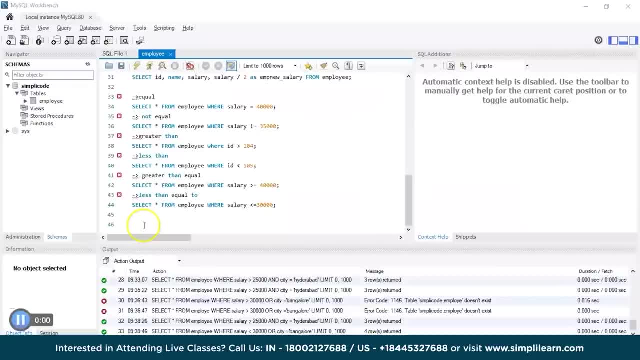 Let us understand the syntaxes and execute them in the workbench now. Firstly, let us discuss about the AND operator. AND operator in SQL will show the records from a database table if all the conditions separated by the AND operator is evaluated to be true. 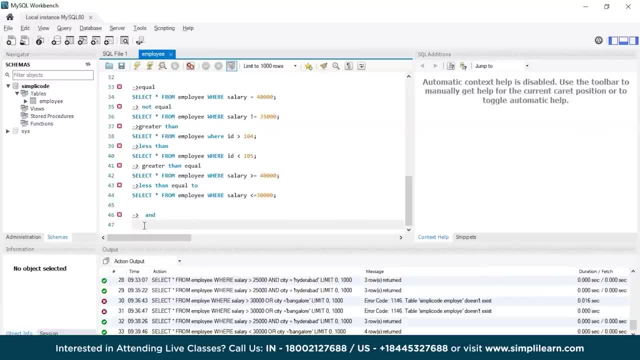 Let us understand with an example. Let's say, if you want to access the records of all those employees from the employee table whose salary is greater than 25,000 and the city that they belong to is Hyderabad, So for that we'll write the following query: as SELECT star FROM table name, that is employee. 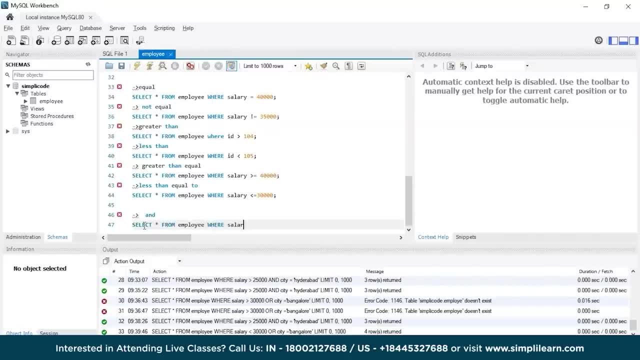 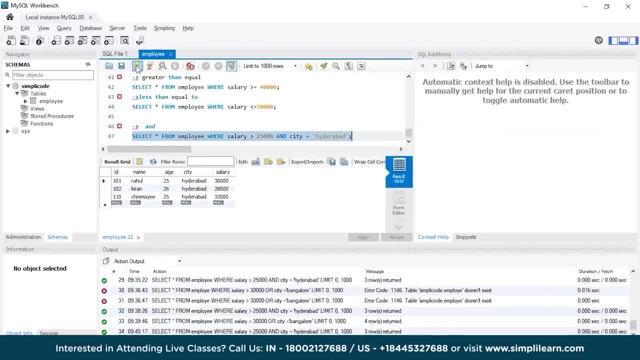 the total three records of the employees, that is, Rahul, Kiran and Chinmay, who are having salaries more than 25,000, and the city that they belong to is Hyderabad. So in this way, AND operator in SQL is used to compare data with multiple operators. 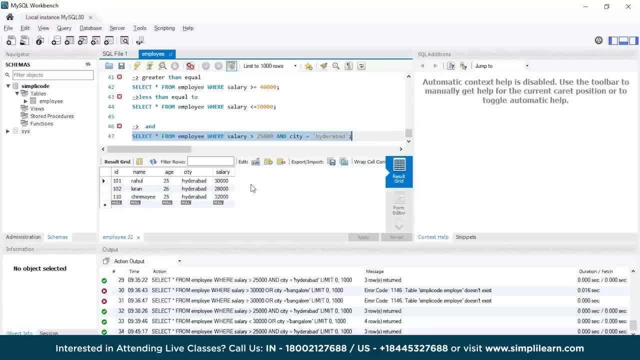 This is called the AND operator. The AND operator in SQL is used to compare data with multiple operators. In this way, the AND operator in SQL is used to compare data with multiple operators than one condition. if, and only if, all the conditions return true, then only it will display. 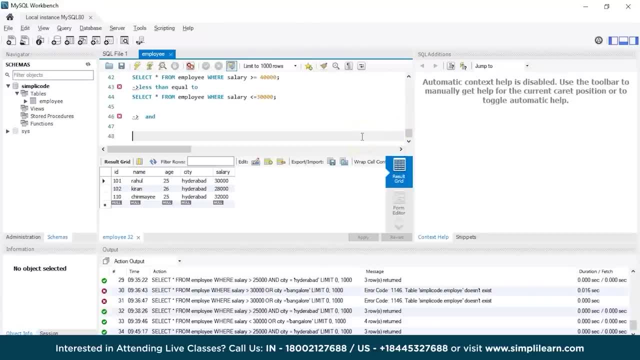 the records, otherwise it won't. next let us look at the or operator. or operator in sql shows the records from the table. if any of the conditions separated by the or operator evaluates to be true, let us understand with an example. for instance, if you want to display the records of employees, 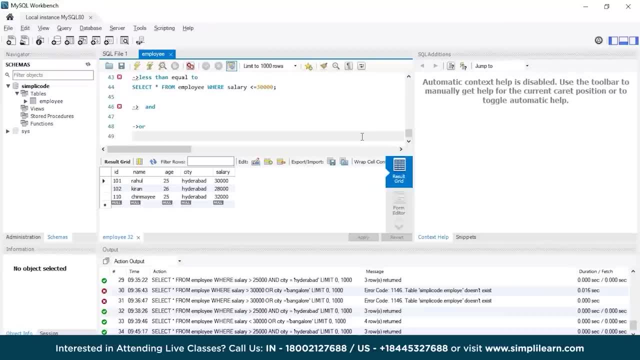 from the employee table who are whose salary is greater than 30 000 or the city that they belong to is bangalore. so the following query would be: select star from the table that is employee where salary is less than 30 000 or the city that they belong to is bangalore. 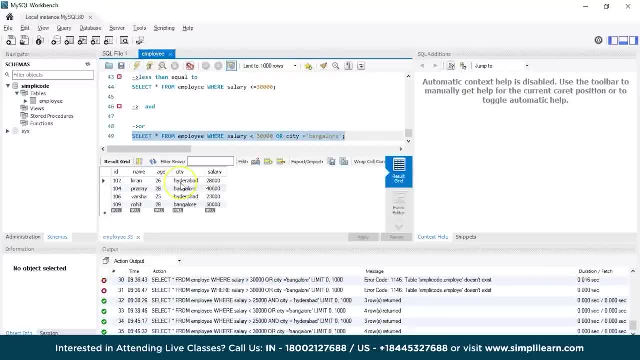 let us execute this statement now. so this will be the following output, where you can see a total of four records of the employees- uh, followed by kiran, pranay, varsha and roit- who are having salaries less than 30 000 or else they belong to the city bangalore. so in this way, we can use our operator, which 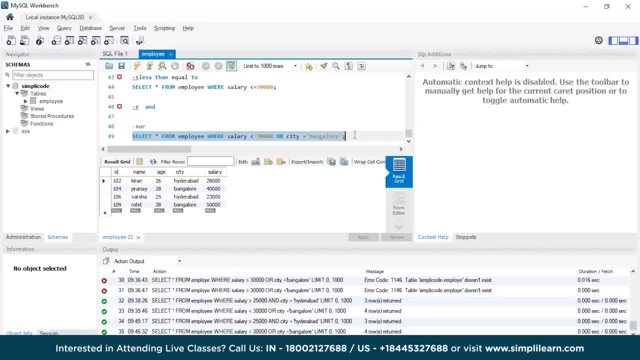 basically compares the data with more than one condition and unlike and operator. if either of the condition is true, it will return the data, otherwise it won't. next let us look at the operator. between operator in sql shows the record within a specified range mentioned in the sql query. 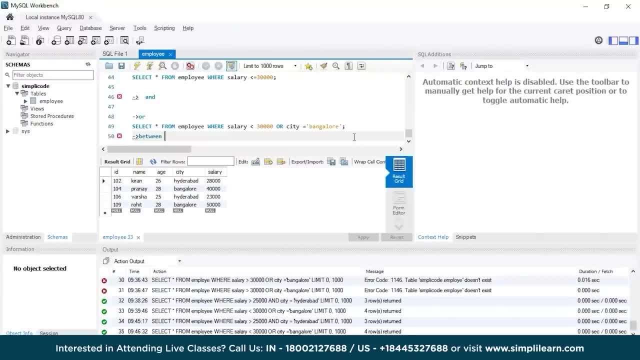 if there is no value in this given range, then this operator shows null value. suppose, if we want to access the information of all the employees from the employee table whose salary is in between 25 000 and 35 000, then we'll write the following query as select star. 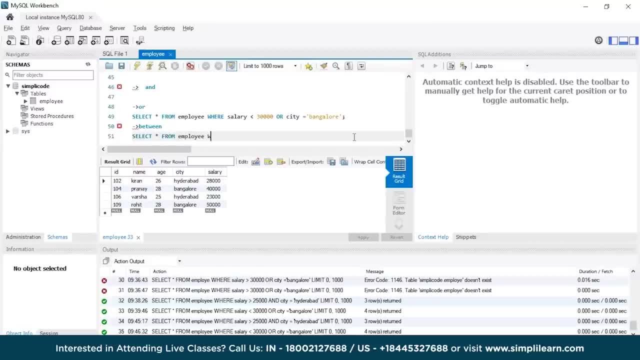 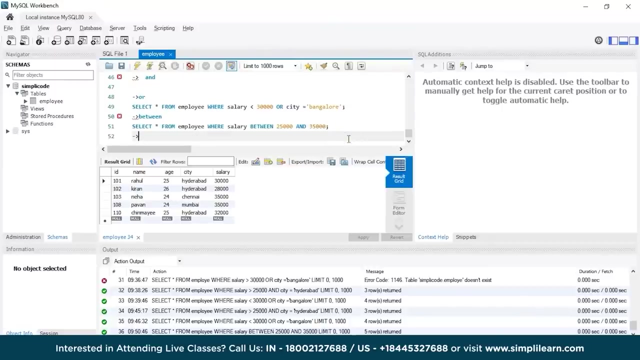 from table name, that is, employee where salary between 25 000 and 30- 35 000. let us execute this query now. so following is the output where it will display the records of all those employees who are having salaries in between 25 000 and 35 000. and finally, let us look. 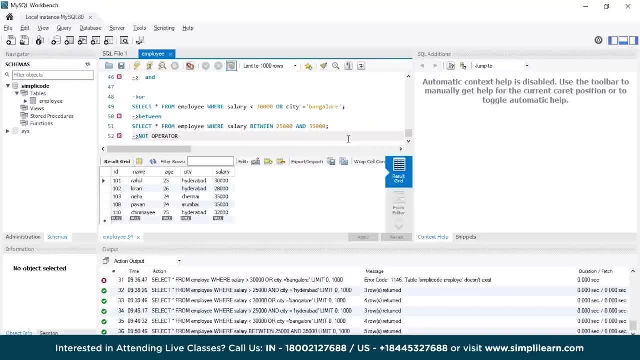 at the not operator. so, on, the Sqlاخase table not operator shows the record from the table. if the condition evaluates to be false, that means the not operator is also called as a negation or a negate operator, which shows data for the opposite of the conditions. 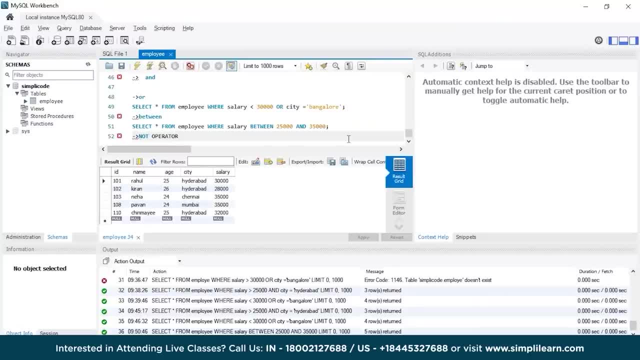 that we mention in the sql statement. let us understand this with the help of an example. let's say, if you want to access the information of all those employees from the table who are not having salary as 40 000 and 25 000 as ^^. 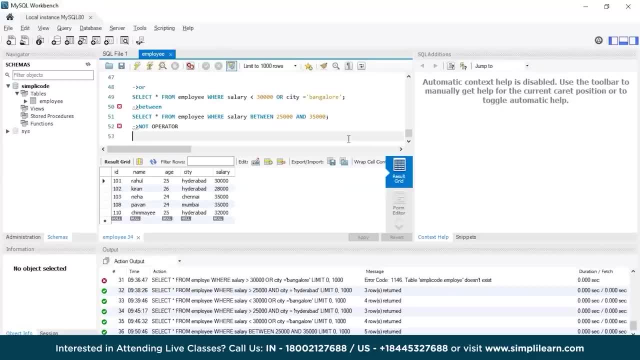 So for that we'll write the syntax as select star from table name. that is, employee where not salary equals to 40,000.. So let us execute this query now So, as you can see, it will display all the records of those employees who are not having. 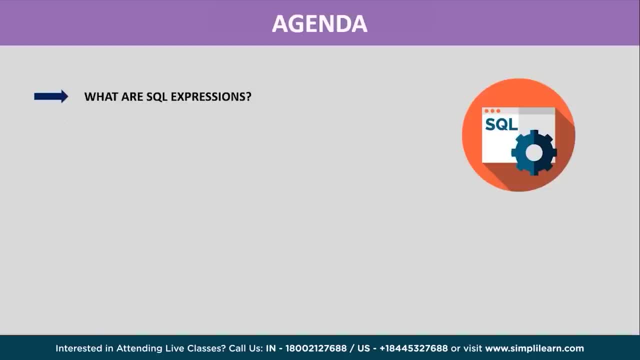 the salary as 40,000.. We'll start this tutorial by understanding what SQL expressions are, Then we'll go through different types of SQL expressions And finally we'll look at the syntax of various SQL expressions and execute them in MySQL Workbench, with examples. 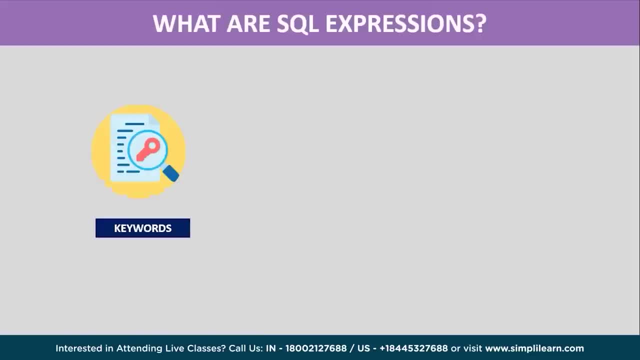 So what are SQL expressions? SQL expressions are composed of one or more keywords or values, such as operators, operands and various other functions that evaluate to a single value or a set of values for a given SQL statement. These SQL expressions are like a formula, which are similar to that of mathematical 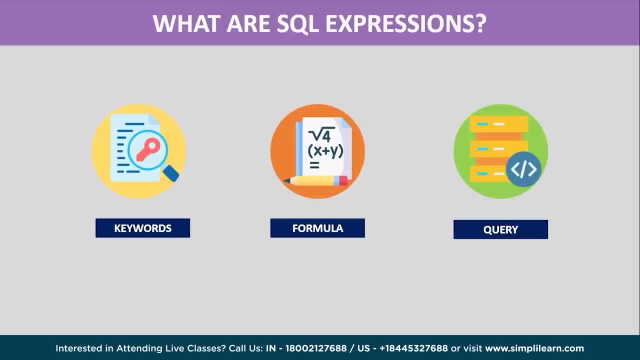 formulas we use to solve a problem And in this case they are written in a query language, using a proper syntax, to perform operations on the data we have stored in our database table. For example, consider the basic syntax of the SELECT statement. Here, expressions are used in many contexts, such as to retrieve any value from the table. 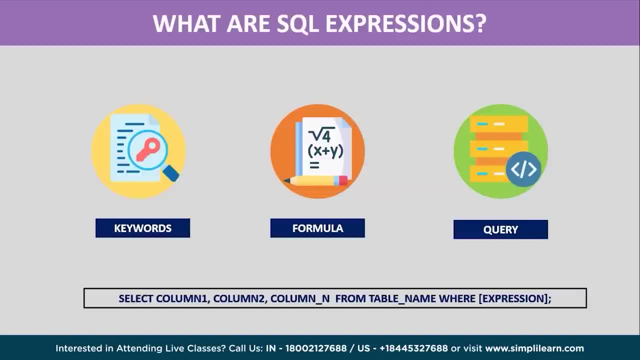 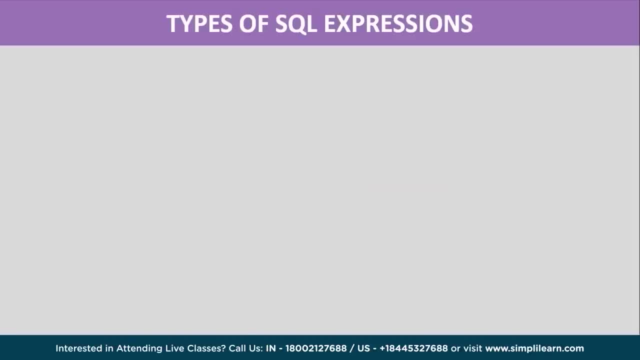 we use SELECT command and for comparison we use WHERE clause. So in this case, all these are SQL expressions, only Types of SQL Expressions. SQL expressions can be classified into following categories. The first one is Boolean expression. SQL Boolean expressions fetch data from the table. 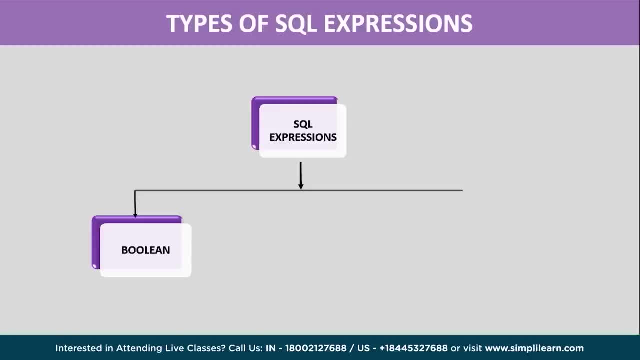 SQL Boolean expressions fetch data based on one-to-one matching. In other words, we can think of it as a query that fetches one result at a time. It will fetch the condition against the single value when the query is executed. The second one is Numeric expression. 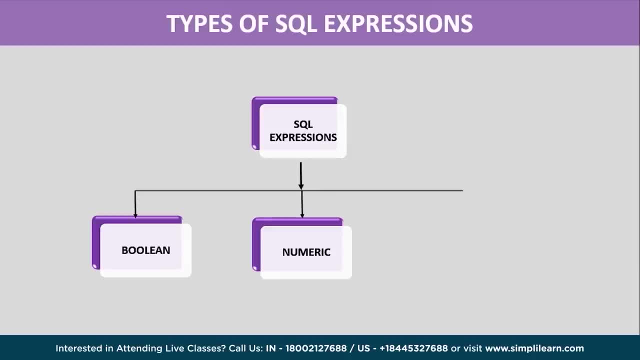 SQL Numeric expression is used for performing mathematical operations in a SQL query. Besides automatic operations, there are several built-in functions like AVERAGE, SUM, COUNT as well. DATE expression. SQL date expressions are used to compare and get date according to its various date. 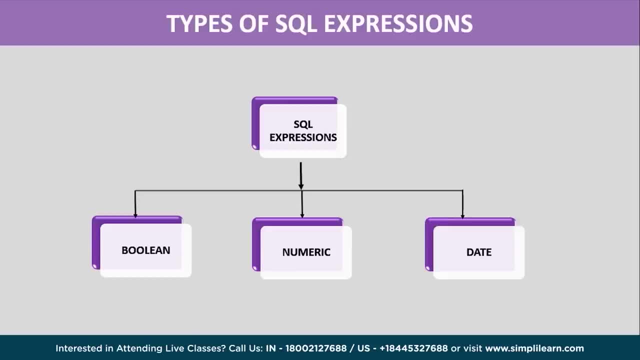 and time related query and conditions. They give date- time value as the output. It can also return current system date and time values. also, Now that we have understood what exactly SQL expressions are, let's execute them in MySQL Workbench with the help of examples. 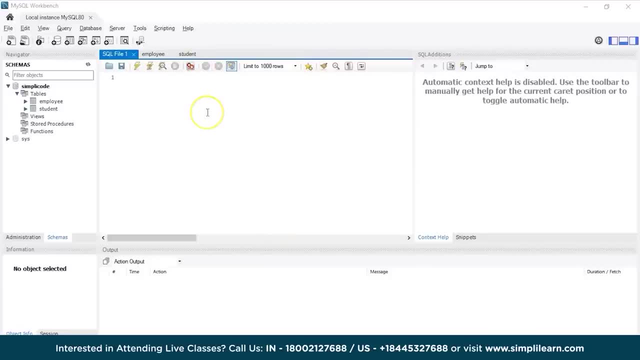 As you can see, SQL Workbench has started and before we get to the execution part of various SQL expressions, let's see how it works. First we have to create a table. So for that I have already created a table named student within the database SimpliQuote. 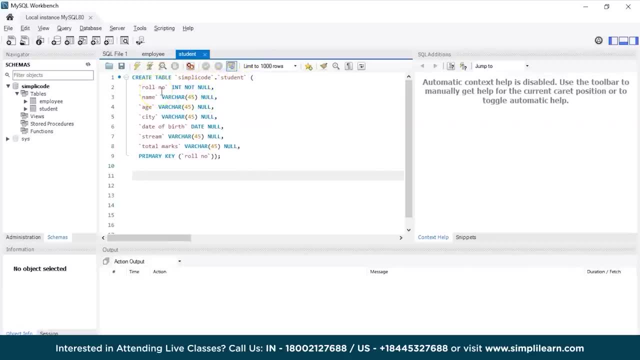 The student table consists of various columns, such as role number, name of the student, age, the city they belong to, date of birth, the stream that they have chosen and the total marks that they have scored in the final exam. And here the primary key is the role number, which basically uniquely identifies each and 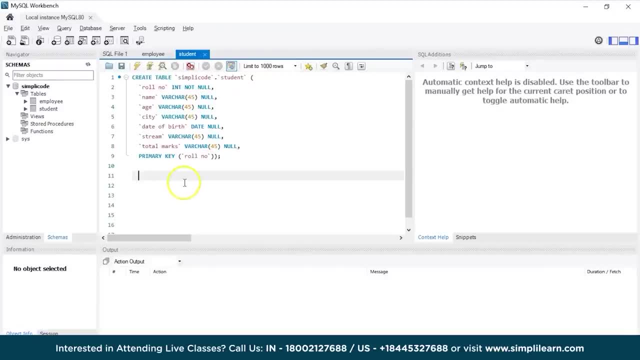 every record of the student. So now that we have created the table, if we want to retrieve the information of all the students, we will use SELECT command. So the following query would be: SELECT star from the table name, that is, student, and semicolon. 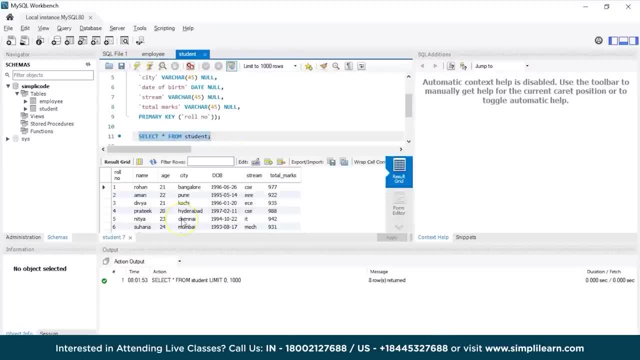 Let us execute this And, as you can see, all the records of the students are being displayed, that is, the name, their age, the city they belong to The stream and also the total marks that they have scored in the final exam. Now that we have created table and inserted values into the table, let us understand various 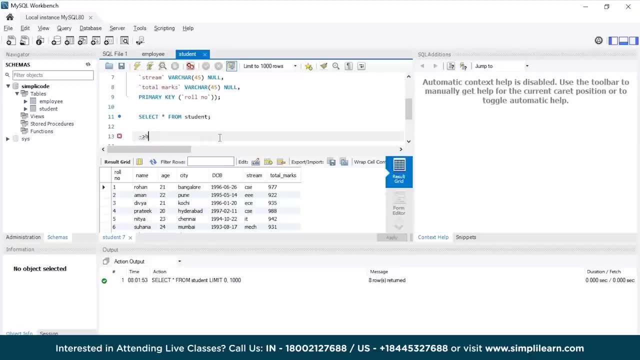 SQL expressions. Firstly let us discuss about Boolean expression. For that we'll take a simple example from the table itself. Suppose, let's say, you want to display the records of those students from the student table who belong to the city Kochi, For that. 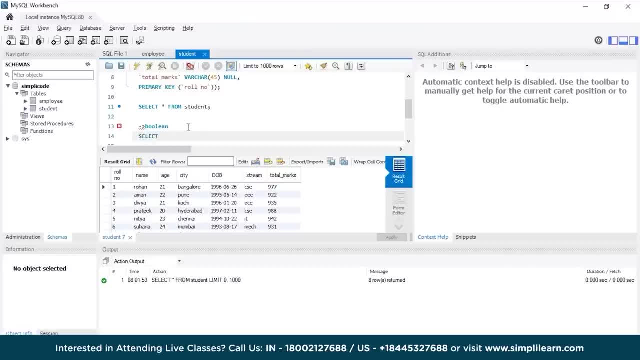 We'll write the SQL query as SELECT star from the table name, that is, student, where city equals to Kochi. Now let us execute this statement and see the output. So, as you can see, there's a student named Divya, whose age is 21, who belongs to the city. 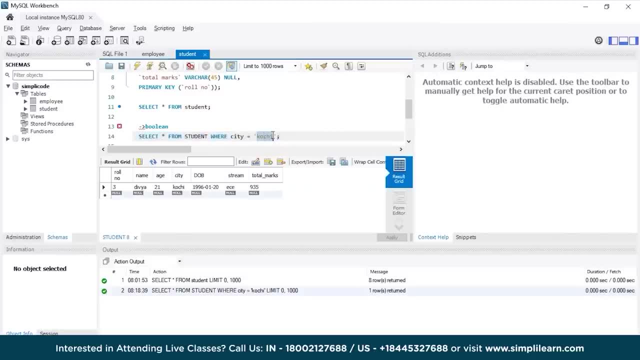 Kochi. Similarly you can find for other cities as well. So let us take for Pune and execute this query. So the output would be: it will show the records of two students named Aman and Indra, who's having age 22 and 25, who belong to the city Pune and having a stream says Tripoli and MBA. 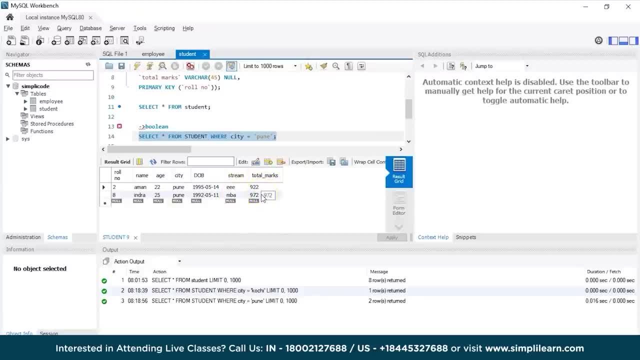 and the total marks is 922 and 972.. So the Boolean expression not only executes the values against the character values, which is in this case is Pune, but it can also take the values of numerical values as well. For example, let's say the university has got to know the highest marks scored by an. 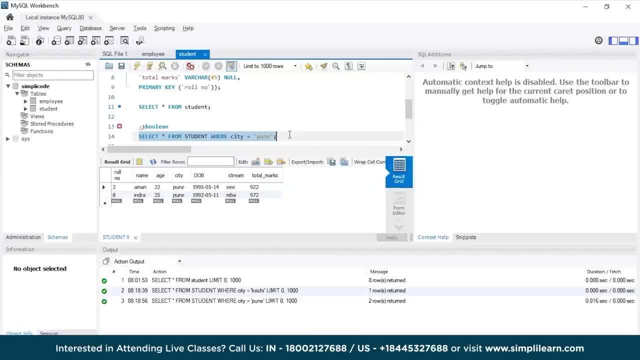 individual in the final exam is 988 and it wants to retrieve the details of that student. So for that, the following query would be: SELECT star from table name, that is, student where city Kochi, Where total marks is equals to 988.. Let us execute this query now. 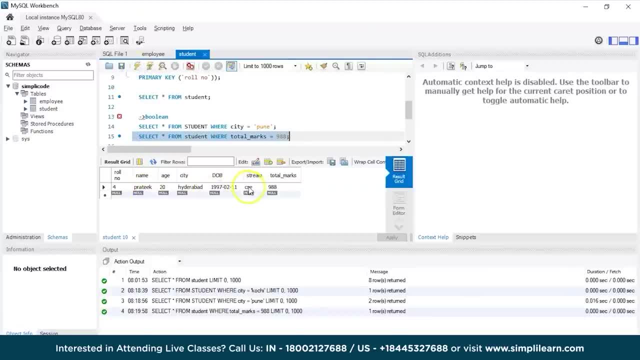 So, as you can see, a student named Pratik, who belongs to the stream CSE, has scored the highest marks: 988.. So, in this way, Boolean expressions are used to perform various operations, which basically evaluates a given condition to a particular value. 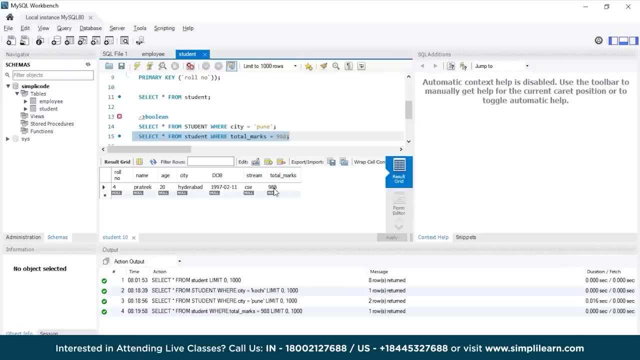 Or you can say a single value, And if the condition is true, it will return the output and display all those records. Otherwise it won't Up. next we have numeric expressions. numeric expressions, So numeric expressions, are basically used to perform various mathematical operations. 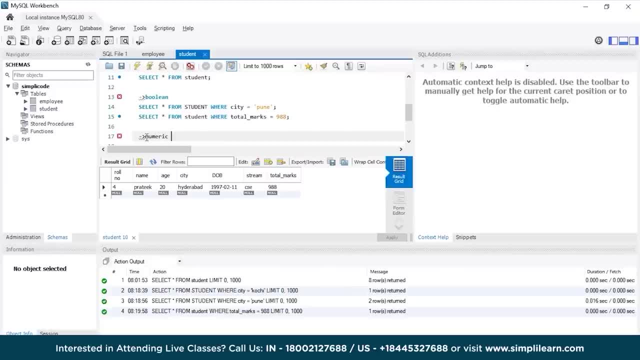 So let us understand this with an example. For instance, let's say the university has decided to change the total marks weightage from 1000 to 500. And I'll specify a condition where I'll take the total marks and divide them into half. 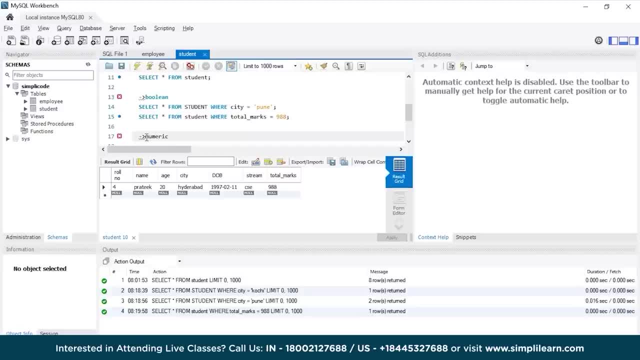 and check all those students who have scored more than 480 out of 500.. For that, the following query would be: SELECT star from the table, that is, student where total marks divided by 2 is greater than 480.. So that's the first query. 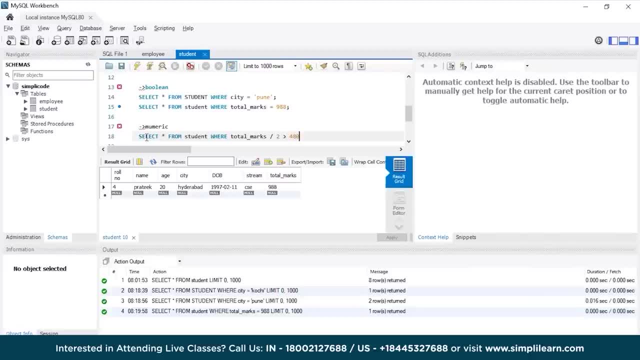 Let's see the next one. Let's see the next one. Let's see what happens when total marks divided by 2 is greater than 480.. Put a semicolon and let us execute this So, as you can see, there are total 4 students who have scored more than 480 when the total 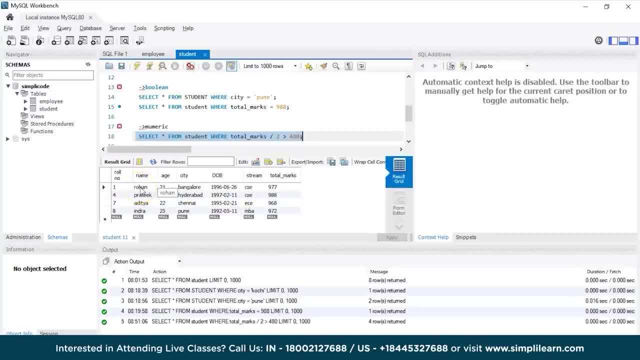 marks are divided into half. For instance, if you take the record of Rohan, who has scored, total marks 977, and if you divided it by two, that is approximately 488.5,, which is satisfying the condition, which is greater than 480. 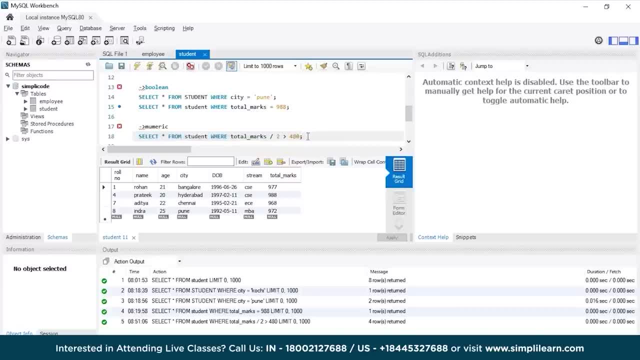 And if you look at this SQL statement carefully, there are a lot of SQL expressions here. Firstly, the student table name. that is the student itself, because it is used to retrieve the values from the columns. that is here. the total marks is the column, and we also have 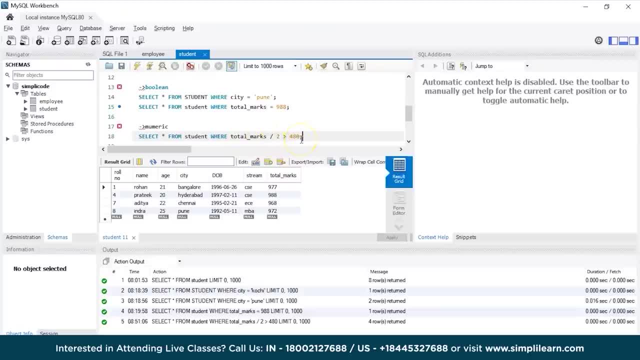 the operands, that is, total marks divided by two, and the right hand operand, that is 480, which can also be considered as an SQL expression here. Similarly, we have other inbuilt functions, as we discussed earlier, like some average, count, minimum and maximum. Let's say, if you want to calculate the average of total marks of each and every student scored. 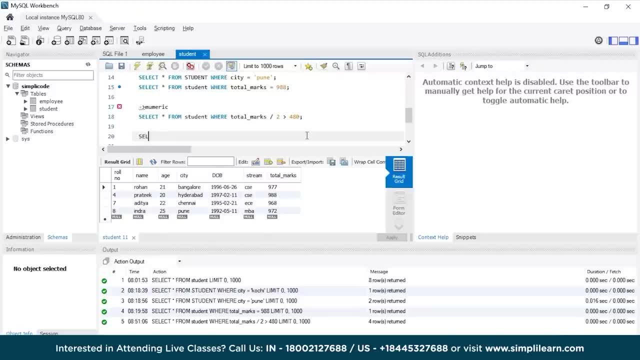 in the final exam. The following query would be select average, which is the SQL function, and within the parenthesis mentioned total marks: Total marks From the table. that is student. Let us execute this. As you can see, it is displaying the total average of total marks, that is, 954, 4.375. 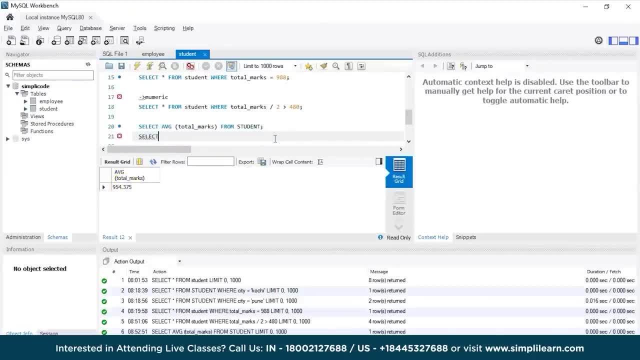 Similarly, you can calculate the sum of all the marks of the students as well, So the query would be: select sum Total marks- Total marks from the student table. Let us execute this, And this will be the following output. So there is a bit error in the code. 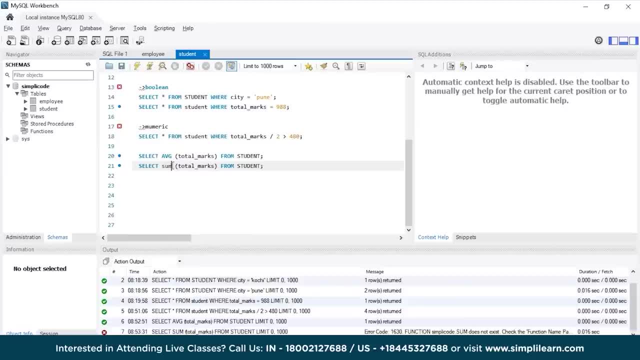 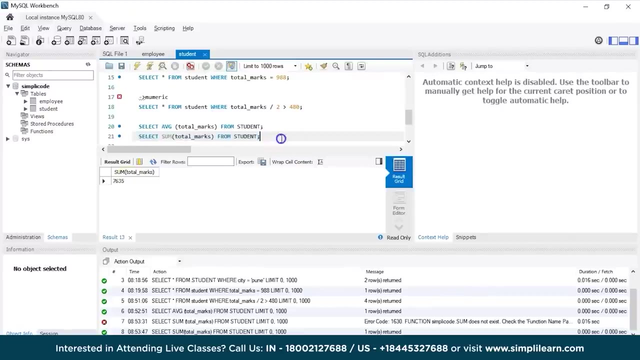 Let me check it once. So, as you can see, it is displaying the sum of total marks, that is, 7635.. So in this way, you can use numeric expressions to perform various operations on the SQL tables. And finally, we have date expression, which basically returns date and time values of: 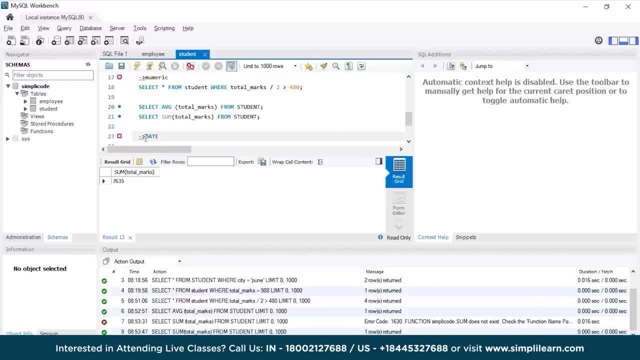 the table. So let us say, if you want to display the records of those students who are born after 1995 January, So for that the following query would be: select star from the table name, that is, student where date of birth is greater than 1995 January 1st. 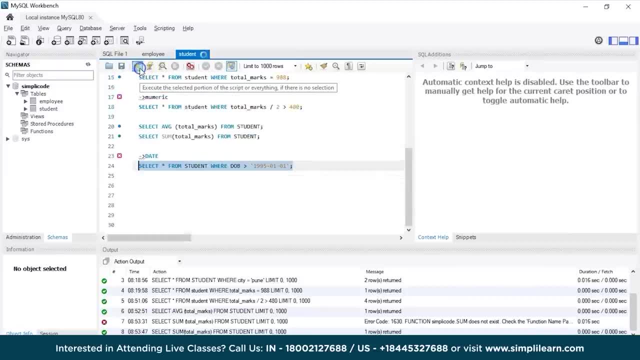 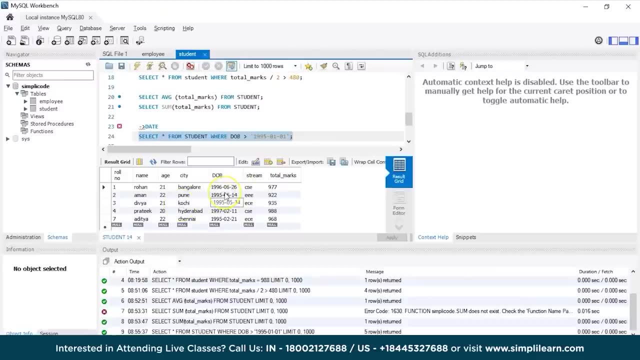 So let us execute this query and see the output. So let us execute this query and see the output. As you can see, there are total five records of the students who are born after January 1995.. Similarly, you can also display the current date and time as well using the current timestamp. 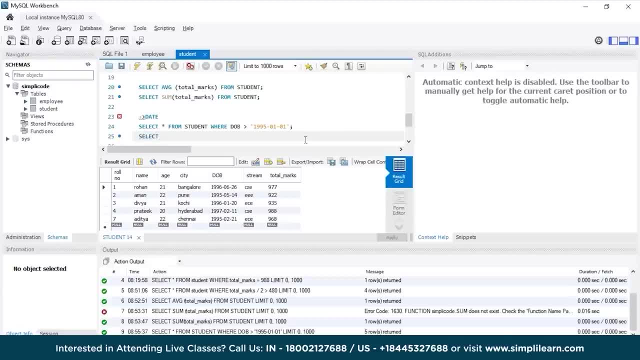 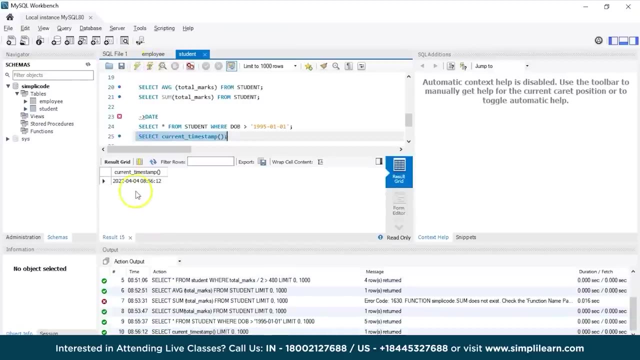 function, That is, select current timestamp, Current timestamp, Current timestamp, And let us execute this query. So, as you can see, it will display the current year, the date and the month format. Similarly, it is also displaying the time, which is in the format of hours, minutes and seconds. 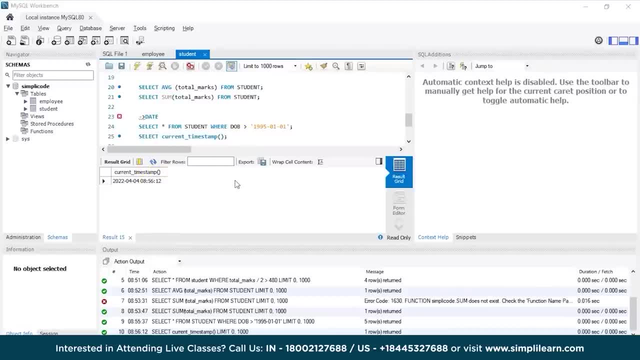 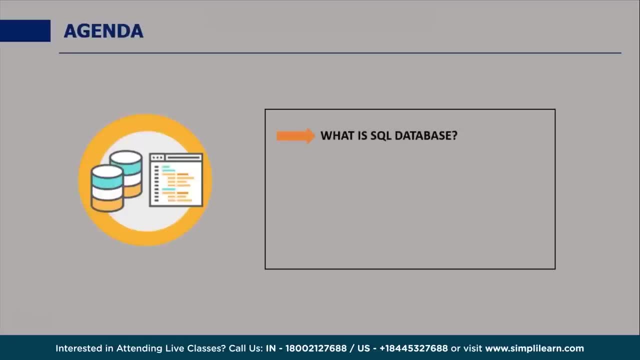 So in this way you can use various expressions to query the database for a specific set of data, to retrieve the information from the SQL table. Firstly let us discuss the agenda for today's session. We will start the tutorial on the SQL table. We will start the tutorial by understanding what SQL databases are and look at some popular. 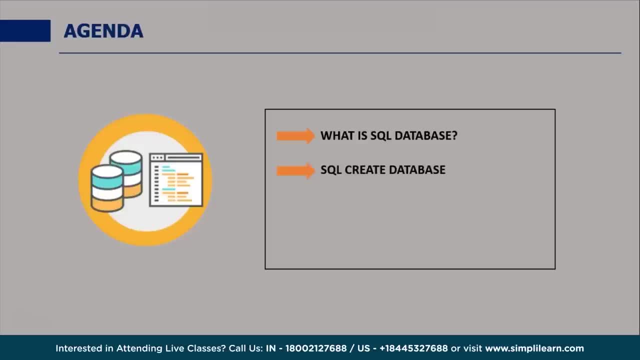 SQL databases. After that, we will discuss how to create an SQL database in MySQL workbench. Next we will see how to select the database in MySQL And finally, we will discuss how to delete the already created database as well. What is SQL database? 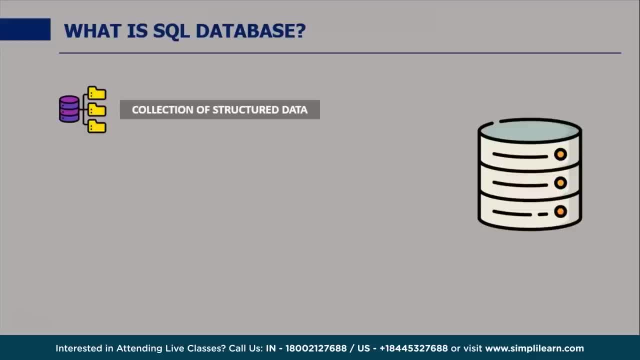 A database in general is a collection of organized data for easier access so that it can be managed and stored effectively. As far as SQL database is concerned, it is a collection of organized data for easier access. As far as SQL databases are concerned, a relational database is used to store and manage. 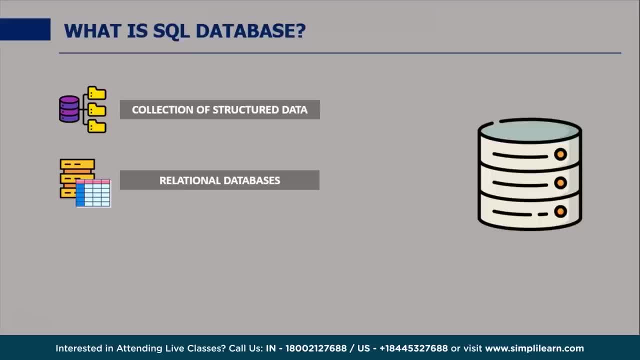 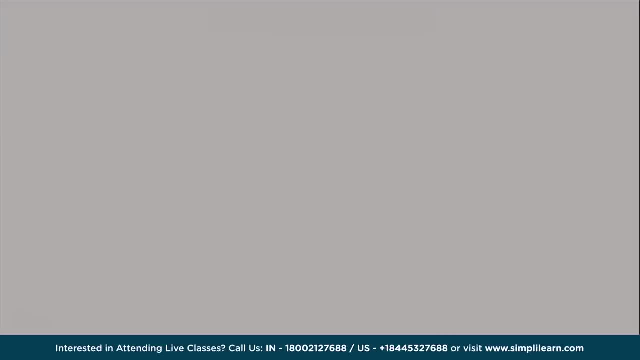 all the data in the form of tables. Simple SQL queries are returned to retrieve the data from these SQL database tables. In a nutshell, you can say that SQL is used to connect with the databases, as it directly interacts and communicates with the database to retrieve the information stored in tables. 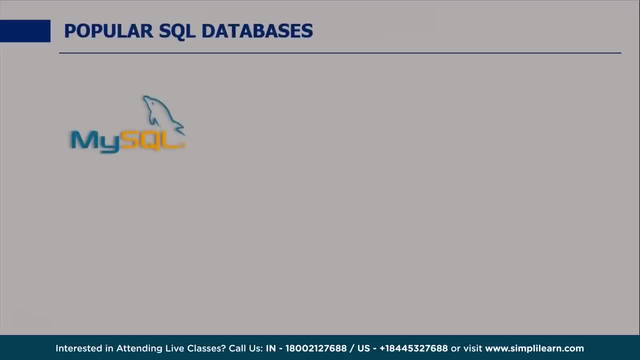 Popular SQL databases. Some popular SQL databases are MySQL, MicrosoftSQL, Serverless and Microsoft SQL. These are some databases that are being widely used nowadays by many companies. Each of them function in their own way and also the syntax of queries that are returned. 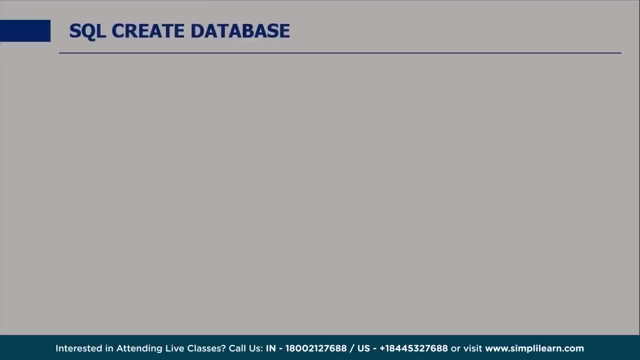 can also slightly vary from each other as well. Let us now discuss the first topic of today's session, that is, SQL create database. In SQL, creating a new database is the first and foremost step to store the data in the tables. SQL create database uses much use create database as a keyword in the syntax. 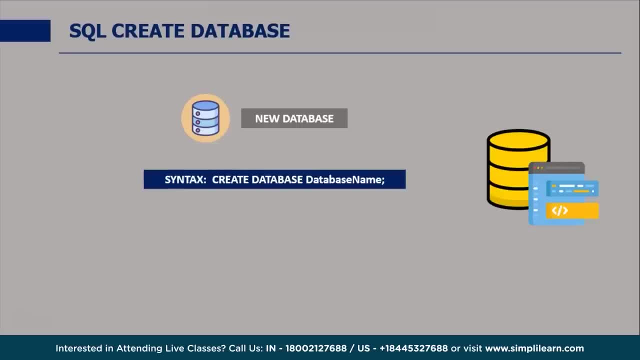 So the syntax is followed as: create database- that is the keyword that we are using here, followed by the name of the database name In the syntax, database name specifies the name of the database which you want to create in the system. Also, make sure that the database you are creating has a unique name and it does not. 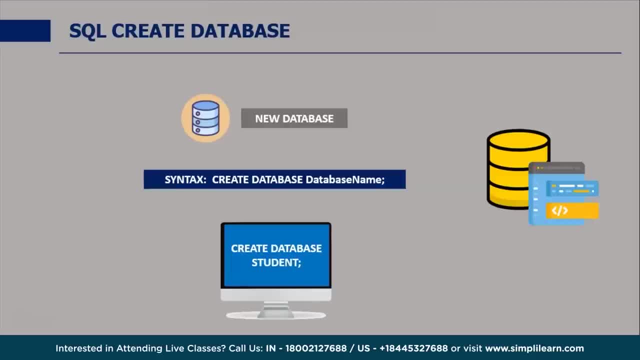 match with other databases as well. For example, if you look at the following example, I am creating a database named student, So the syntax would be create database, followed by the database name that is student. So let us now run this syntax on MySQL Workbench and see how it is executed in real time. 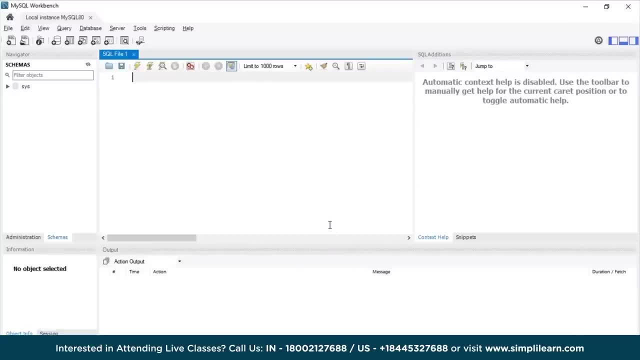 As you can see, MySQL has opened and if you look carefully at the interface of MySQL Workbench, on the left hand side, you will find schemas or the various databases that are available in the system. At the center You will find the SQL editor where the queries are written, and at the bottom you will find 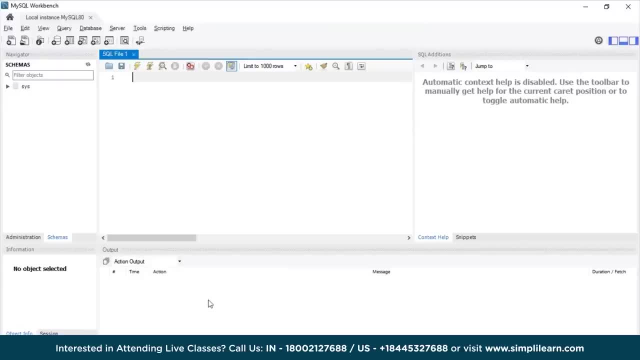 the console where you can see the status or the output of the query that has been executed. So firstly, let's go ahead and discuss the first topic, that is, how to create a database. Let's say, if you want to create a new database project, 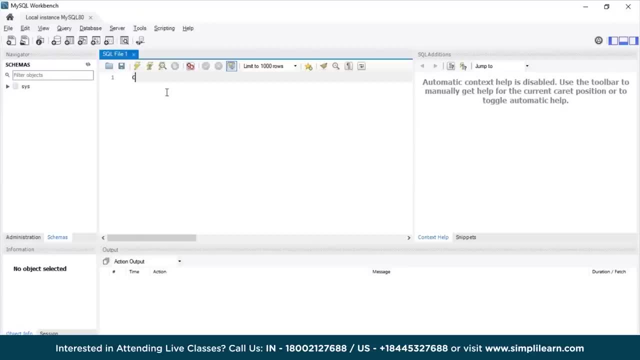 So the create database statement would be as followed: create database- that is the keyword that is used to create a new database. Followed by that, we have to specify the database name. that is, project. Put a semicolon and let us execute this. As you can see, our database project has been successfully executed. 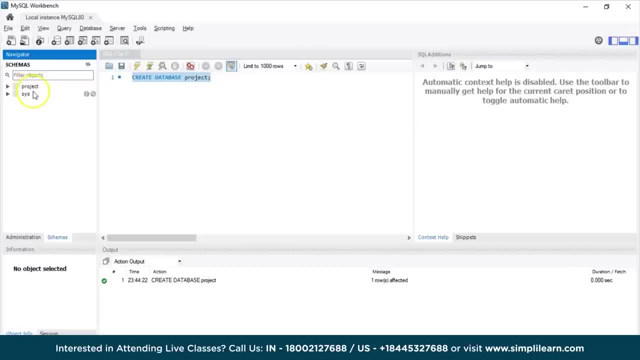 And if you refresh the schema you will find the database name as project. So in this way you can create a new project. And just for confirmation, if you want to check the databases created or not, you can check it in the list of databases. 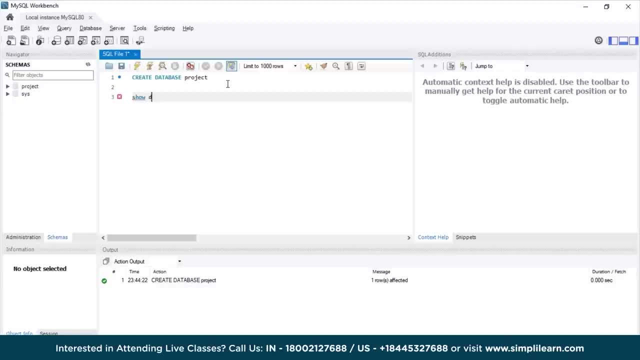 By using show databases keyword. So let us see and execute this. So, as you can see, these are the various databases that are available in the system, including our database project that we have created earlier. Let us now discuss our next topic, that is, how to select a database. 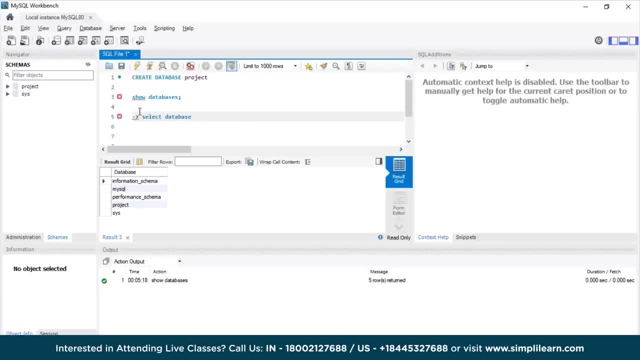 Now that you have created a database. now the user wants to perform some operations, like creating a new table and inserting values onto the existing database in SQL. For that, firstly, they have to select the database on which they want to run the database queries. 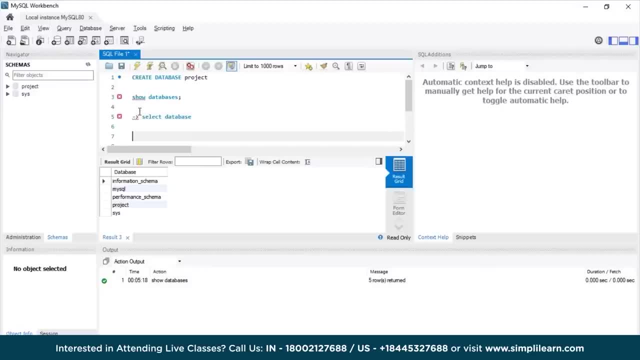 Without selecting the database, they cannot create a new table. For instance, if I want to create a new table, that is student and when I execute this query it will be a student, It will throw an error stating that no database selected. select the default database to be. 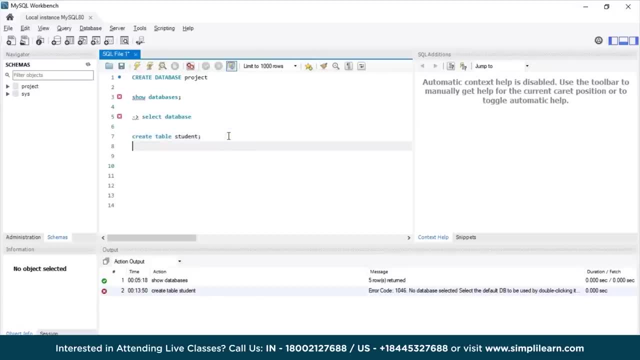 used. So in this way you won't be able to create a new table without selecting the database. Any database user can easily select the particular database from the current database server using the use keyword in the SQL statement. So the following syntax would be use, followed by the database name that you want to select: 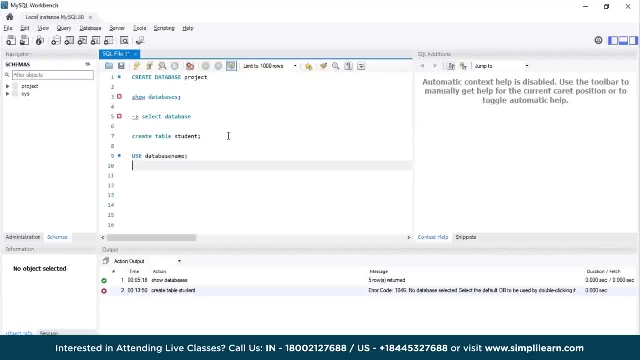 For example. Let us take, for instance, if I want to work on the database project, So the following query would be: use project, which is the database name here that has execute this. So, as you can see, the query has been successfully executed. 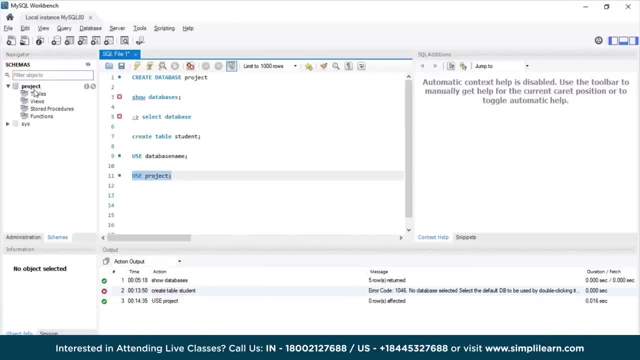 And also you can find the database name project is highlighted in bold. That means you have successfully selected the database And you can start creating your database. So the next thing you have to do is to create a new database. Let us take, for instance, if I want to work on the database project. 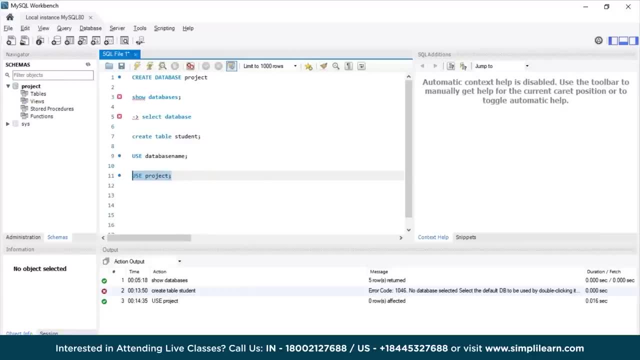 your new tables. So in this way, when you have multiple databases in your SQL schema, before starting your operations you have to select a database where all your operations would be performed. Also, keep in mind that the database that you are selecting should be unique. Finally, let us look at how to drop the. 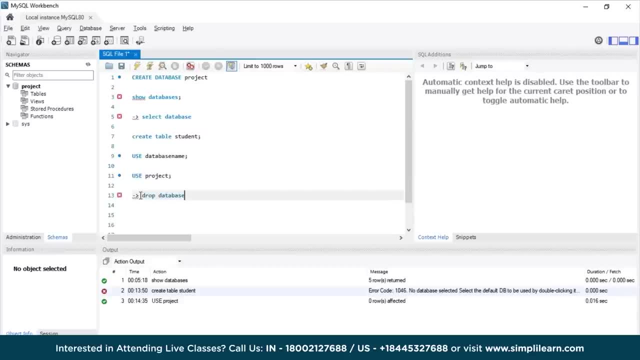 database. In other words, dropping a database is to delete a database. The SQL drop database statement deletes the existing database permanently from the database system. That means the statement deletes all this data and the tables that are stored in the database. So let us now look at the syntax of the drop. 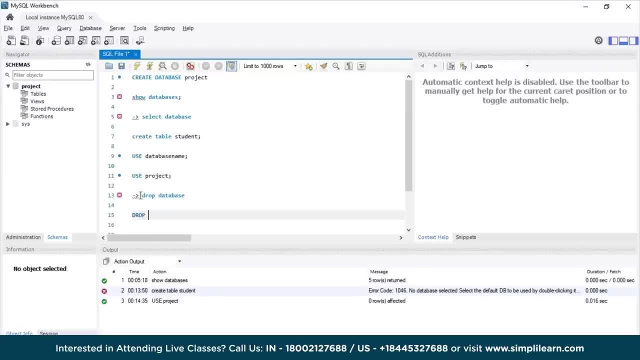 database. The syntax is followed as drop database, followed by the database name. that is project. Here in this SQL syntax we have specified the name of the database which we want to delete permanently, permanently from the database system, after the drop database keyword, And let us execute this and see the output. 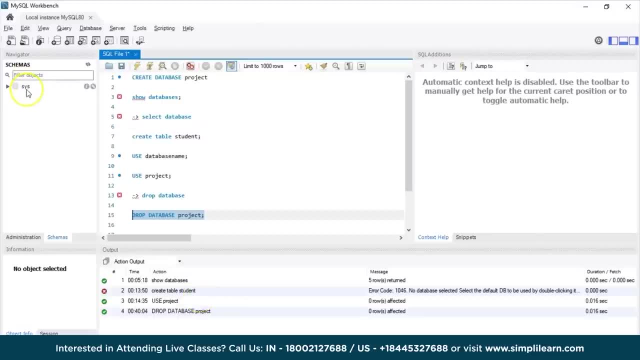 As you can see, the database has been dropped and even at the left hand side, if you look at the schemas, database project has been deleted successfully. So in this way you can delete database using drop database statement. but be careful before using this operation because by 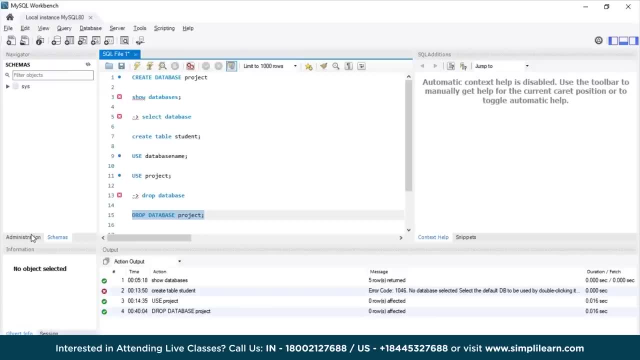 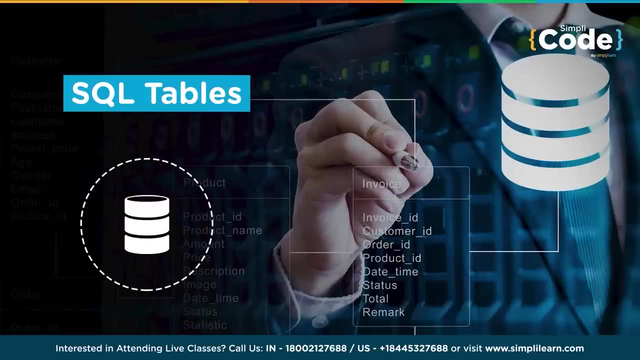 deleting an existing database, it would result in complete loss of information stored in the database. We'll understand how data is stored in the form of tables in SQL and also discuss some basic SQL queries related to these tables. Firstly, let us discuss the agenda for today's session. We'll start the 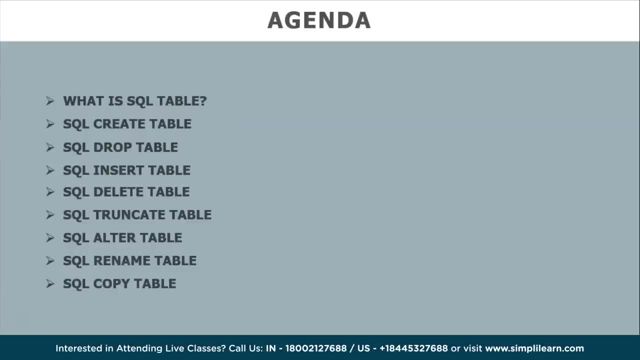 tutorial by understanding what is SQL table, and then we'll look at how to create a table. After that, we'll see how to drop a table, Followed by that we'll see how to insert a new value into the table, And then we'll look how to delete a table. After that, we'll 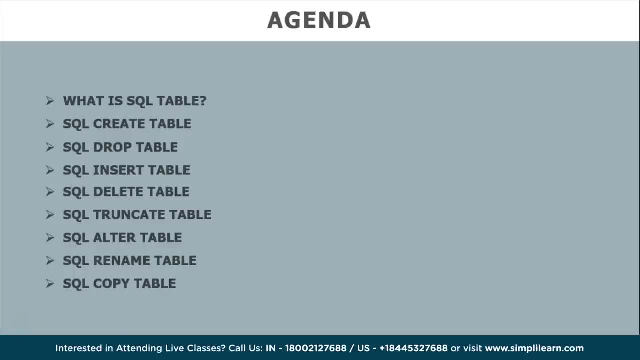 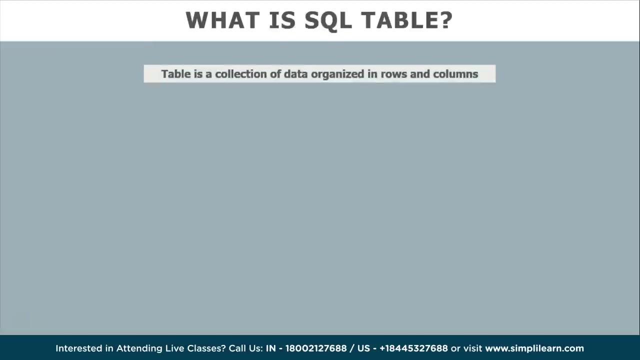 see how to truncate a particular table, and then we'll discuss how to alter an existing table. After that, we'll see how to rename an existing table. Finally, we'll look at how to copy a new table. What is SQL? table Tables are the essential elements of a database. 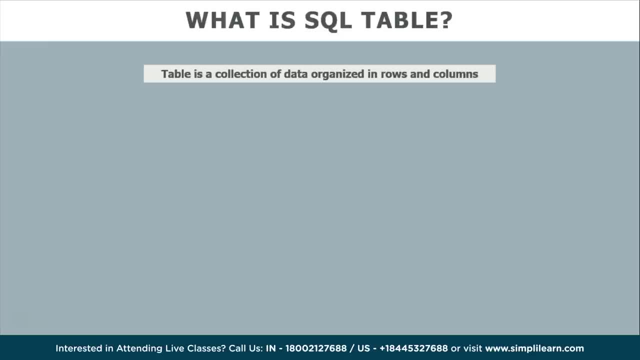 and, in particular, for relational databases, as it is one of the most used data models to store and retrieve data from tables. Tables are basically an organized collection of data that consists of rows and columns. Another point to be noted is that a table has a specified number of columns, but can have any number. 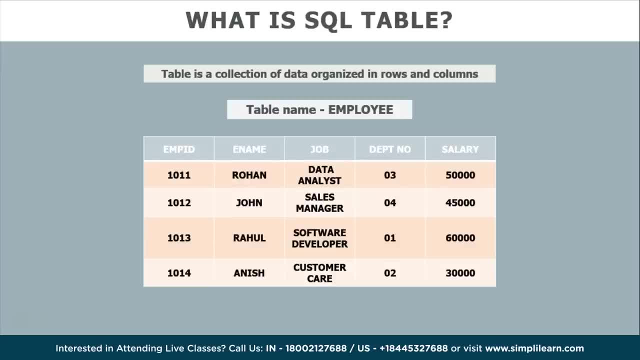 of rows. Let us understand this with an example. Here the name of the table is taken as an employee and in SQL, naming a table is very important because before performing any operation, you have to specify the name. Also, the name of the table should be: 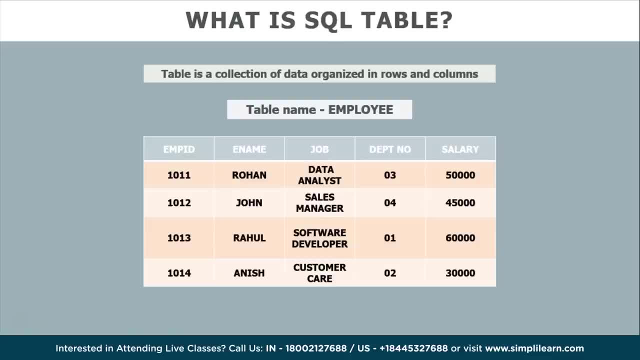 unique and it should not match with other tables in the database. The horizontal values represented in the tables are called as rows or tuples, and each row represents a unique record. Similarly, the vertical values represent columns or the attributes of that particular table, and each column represents a unique field in the 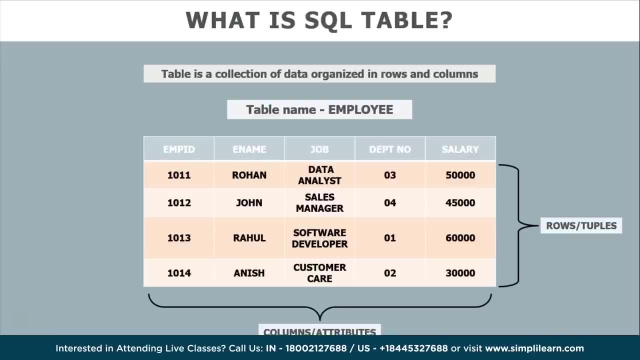 record, As we can see in the table: employee ID. employee name, job department number, salary. are the various fields or the column names. The data in this multiple columns are called rows or tuples, and these multiple columns, such as the employee name Rohan, who's? 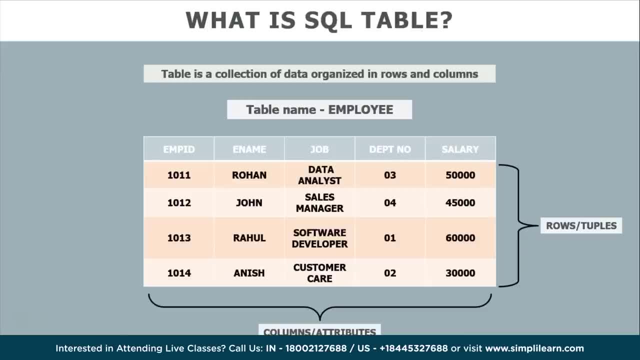 having employee ID 1011, who's working as a data analyst, belong to the department 3 and having salary 50,000 is stored in the form of rows. I hope you've understood what is an SQL table now, So let us now discuss some basic SQL queries that are performed on. 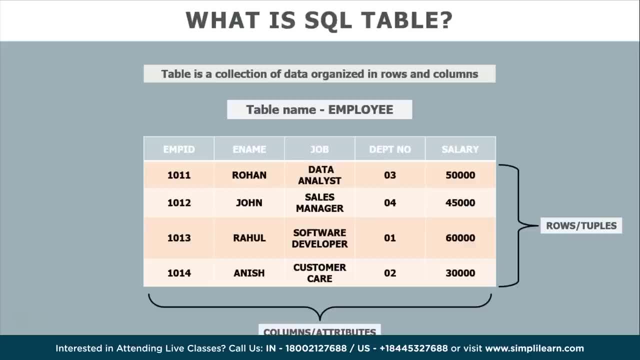 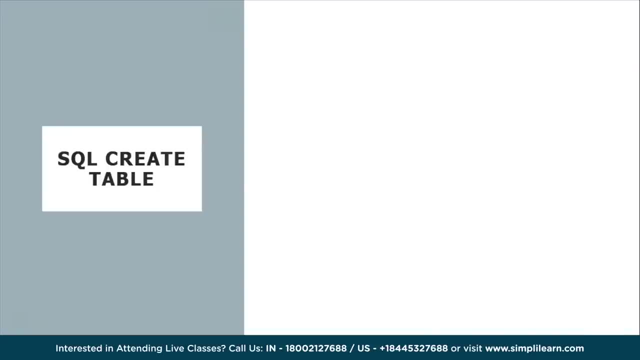 these tables and execute them in MySQL workbench as well. SQL create table. SQL create table is a basic SQL table that is used for creating a table. If you want to create a table, you should name the table and define its columns and each column's data type. 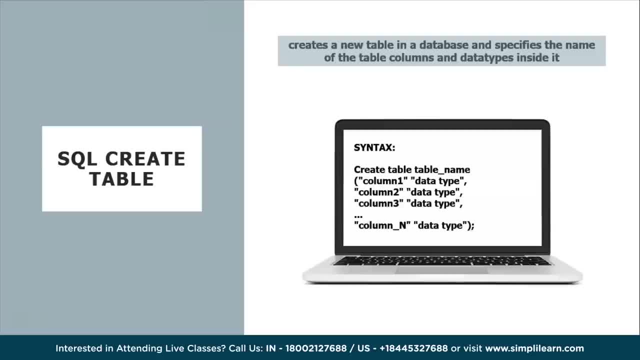 Let us now look at the syntax of create table. The syntax is followed as create table, which is the keyword used here. followed by that we have to mention the table name and, within the parenthesis, you have to mention the column names, followed by that you have to mention the data type. 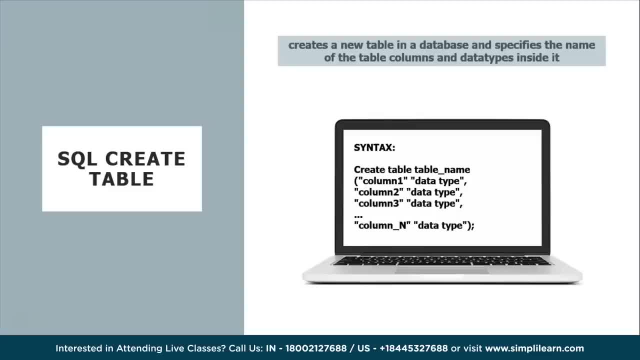 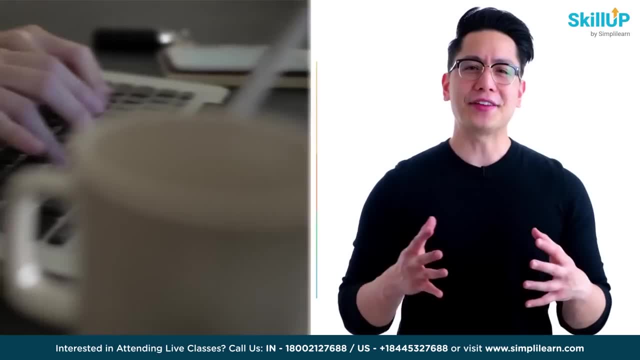 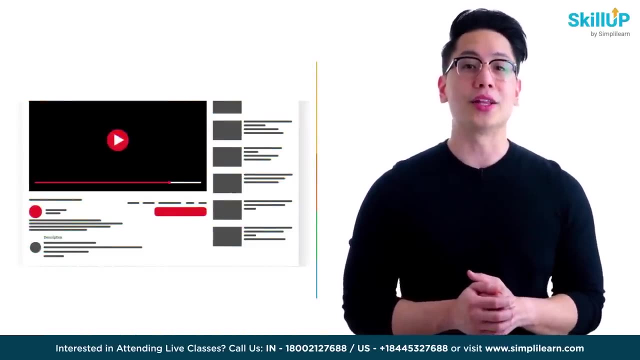 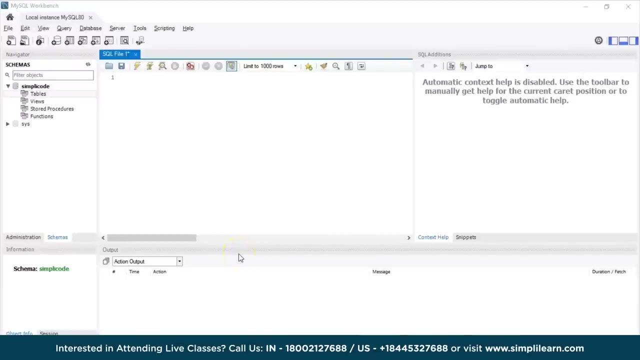 In this way, you can add a number of columns as per your choice. Now that we have understood the syntax, let's move on to the next one. Let's jump into MySQL workbench and execute this. As you can see, MySQL workbench has started and on the left side, 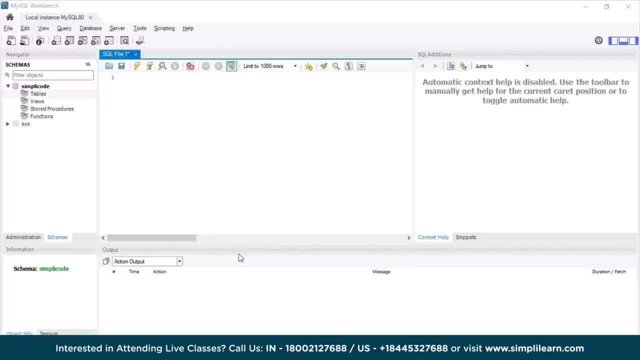 you can see that SimpliCode is the database which we are working on and in that database we are going to create a new table. So let us now look at the syntax of create table table. So syntax is followed as create table, which is the keyword we are using, followed by that we 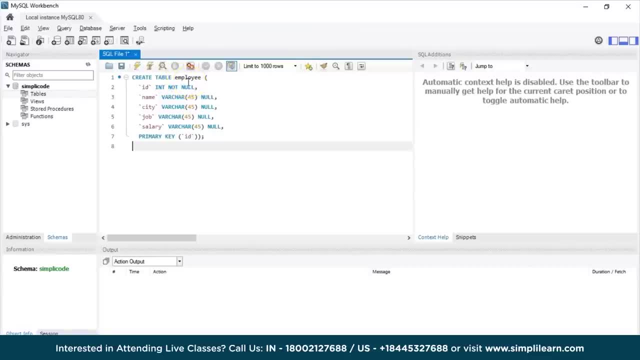 have to specify the table name, that is, we have taken employee in this case, and within the brackets or the parenthesis, we have to mention the column names, followed by that you have to mention the data types. Here I have taken column names as id name, city, job and salary and finally I have 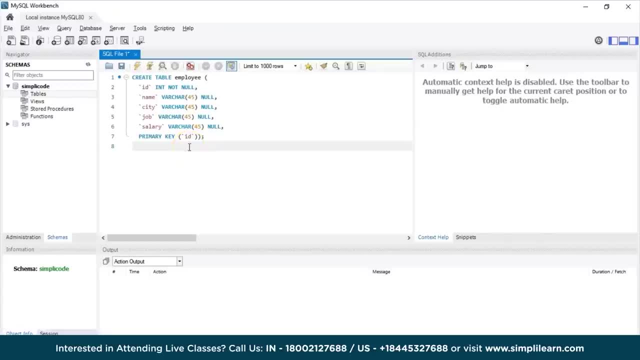 chosen the primary key as id, because it uniquely identifies each and every record in the table. In the end, you have to close the brackets and mention semicolon. Let us now execute this query and see the output. As you can see, our table is successfully created. so, in order to display the 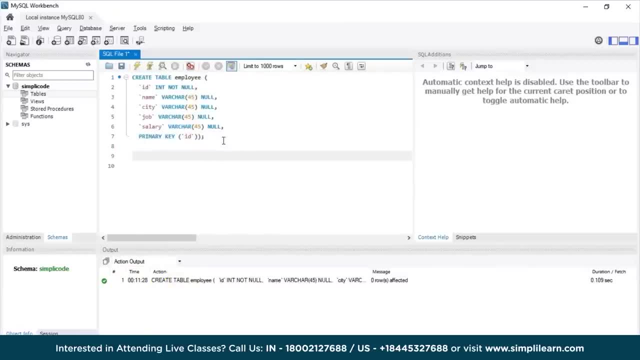 values or whether or not our table is created or not. we have. we have the query as select star from the table name, that is employee. Let us execute this and see the output. As you can see, the table is created and it is showing the column name. says id name, city, job and salary. 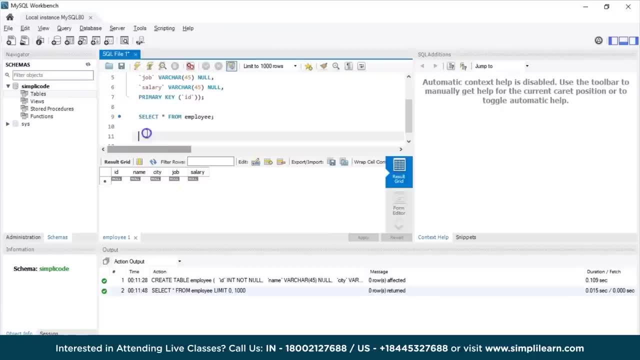 in this way, you can create a new table. Next, let us discuss about drop table. Drop table, in other words. in other words, it basically is to delete a table. The SQL drop scribble statement is used to remove the table definition and the overall structure of the existing table. 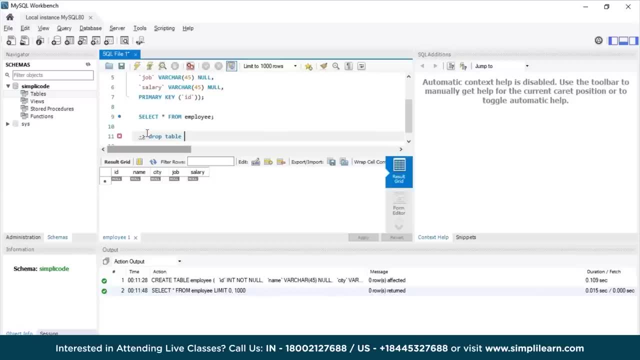 Be careful that while using the drop table command- because once a table is deleted, then all the information available in the data will also be lost forever- the syntax for the drop table is drop table and then you have to mention the table name. so let us now look at the example. now, for some reasons, if i want to delete the employee, 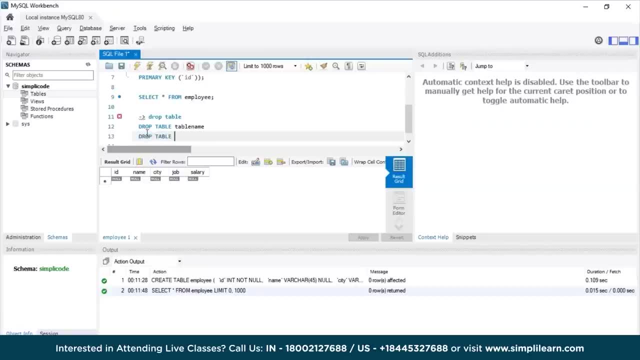 table. so the syntax would be drop table, followed by that the name of the table that is employed. let us execute this. as you can see, our table is completely dropped and let us now see if it is actually deleted or not. for that we'll use select statement, select star from the table name, that is. 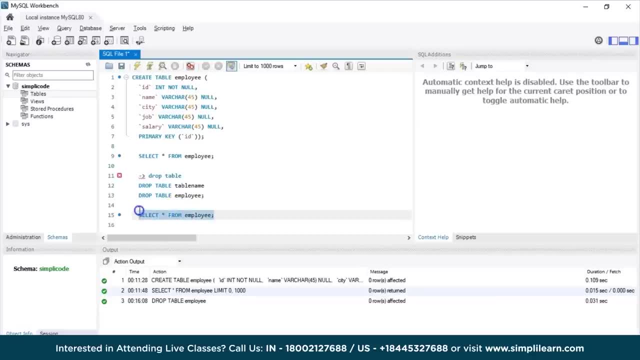 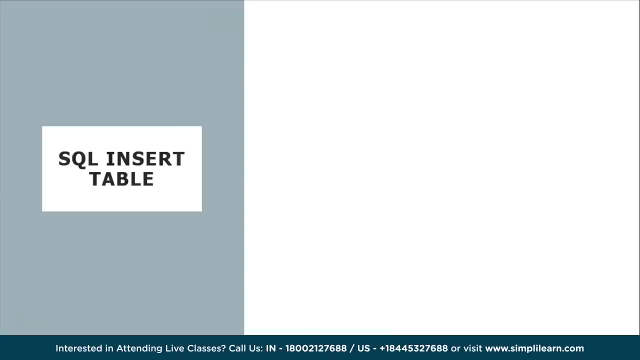 employee. let me execute this query. as you can see, it is throwing an error stating that table- simply code dot employee- does not exist. this means you've successfully deleted the existing table employee. let us now discuss the next topic, that is, sql insert table. sql insert statement is used. 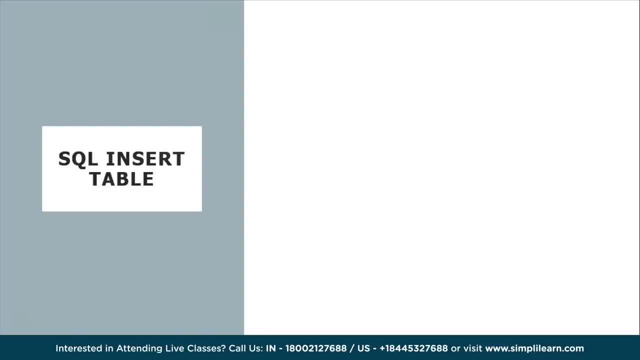 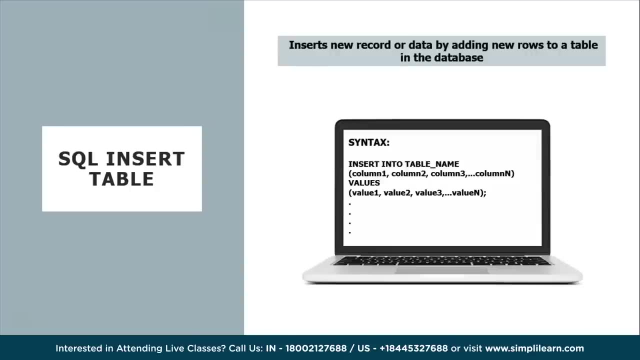 to add new rows of data into a table. this can be a single or multiple records into the database. the syntax for the insert table is: insert into, which is the keyword, followed by that table name, and within the parenthesis you have to mention the column names, values and again within the 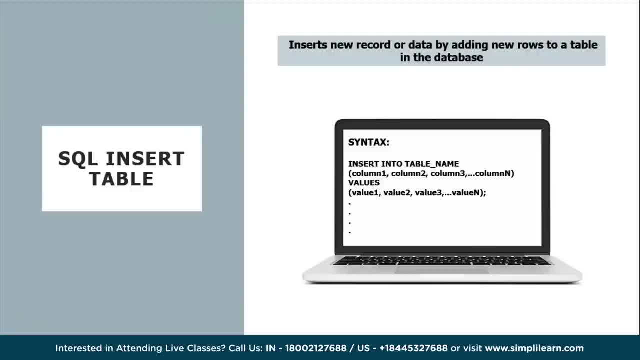 parenthesis, you have to mention the values. so here the column one, column two, column three and n number of columns are the names of the columns in which the table you want to insert the data into. you may not need to specify the column names in the sql query if. 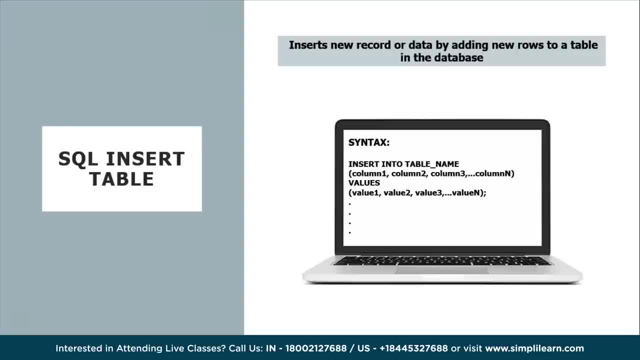 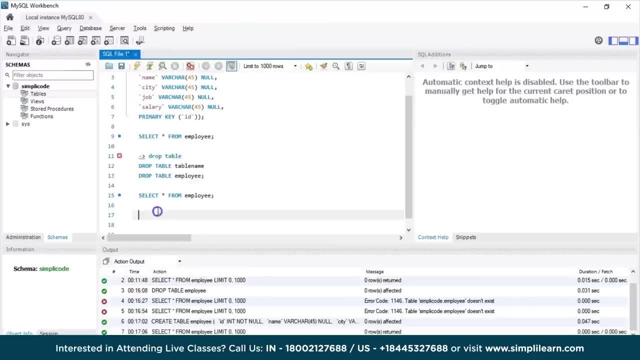 you are adding values for all the columns of the table, but make sure the order of the values is in the same order as the column in the table. let us jump into the execution part. now. i'm taking the same name, that is, employee table- to insert the new values. so the syntax for: 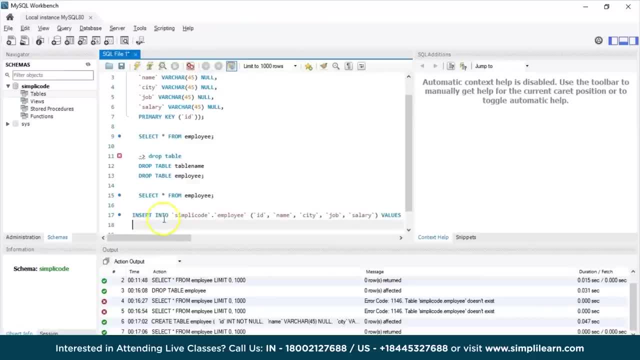 inserting new values into the table is followed as insert into table. name. that is employee, and within the brackets we have to mention the columns that we have taken earlier, that is, id name, city, job and salary. after that we have to mention the values using the values keyword. so within the 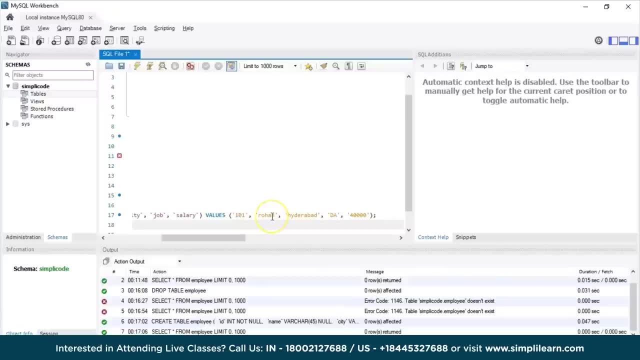 brackets. i'm mentioning the id name as 101, name as rohan. the city that he belongs to is hyderabad and the job that he does is da that data analyst, and the salary that he earns is 40,000.. So let me execute this query and see the output. 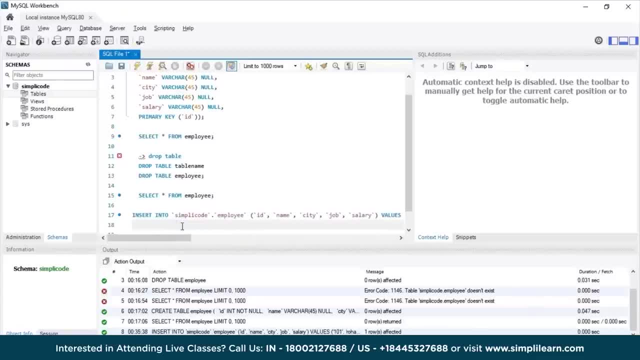 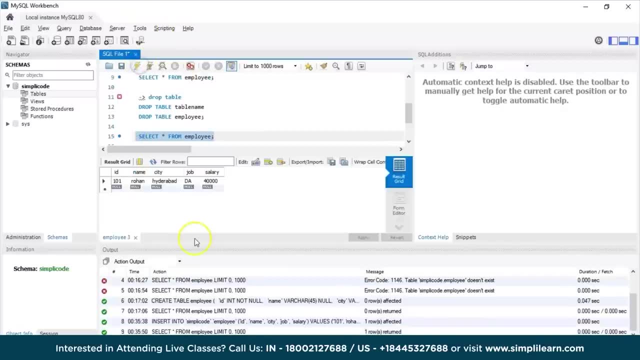 So, as you can see, our query has been successfully implemented. Now let us display the results by using select query. again, Let me select this whole query and execute this, As you can see, the details of employee name, that is, Rohan, whose ID is 101, and the city. 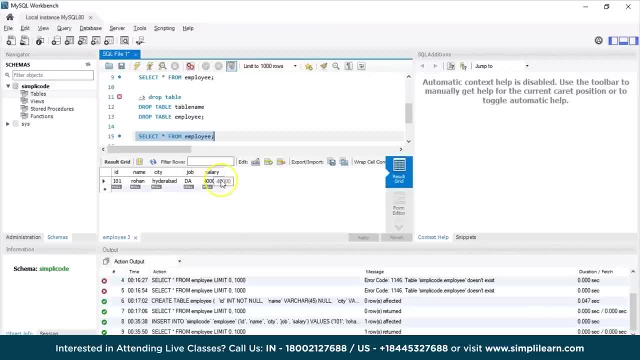 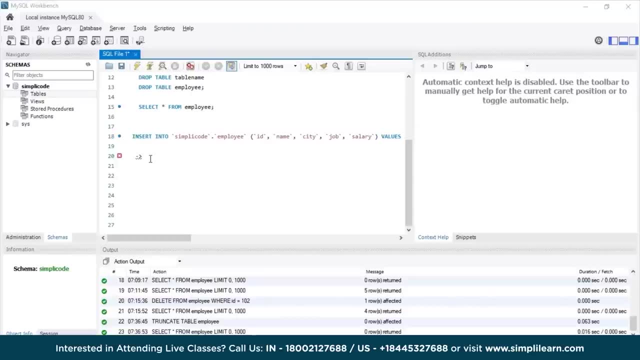 he belongs to Hyderabad. his job data analyst- his salary- 40,000- is being successfully displayed, So in this way you can insert new values into the table Up. next, let us discuss about delete table in SQL. Delete table in SQL is used to remove rows from a table. 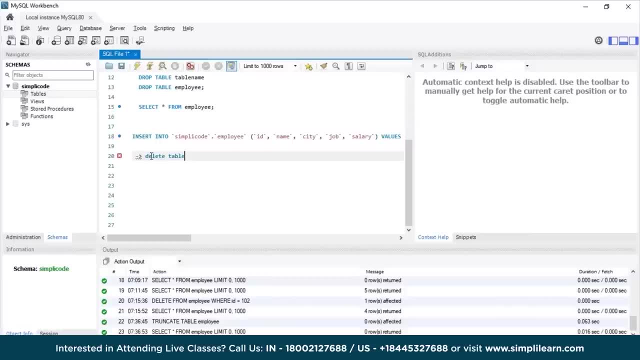 This can be a complete row from an existing table or a specific row. If you want to remove a specific row from a table, you should use var condition. But if you do not specify the var condition, Then here it will remove all the rows from the table. 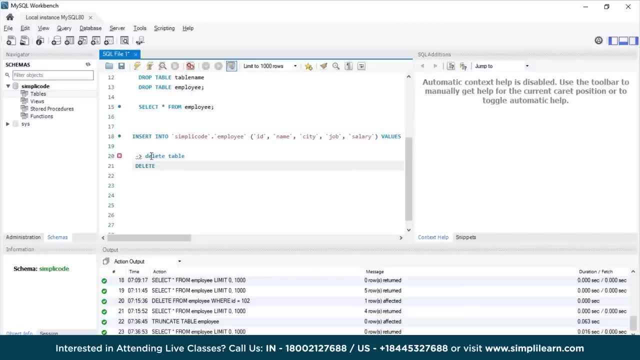 The syntax for delete statement is delete from the table name. So let us take an example now. Suppose if I want to delete the records of the employee who's having employee ID as 102 in the table employee. So the following query would be: delete from table name. that is, employee, specify the var. 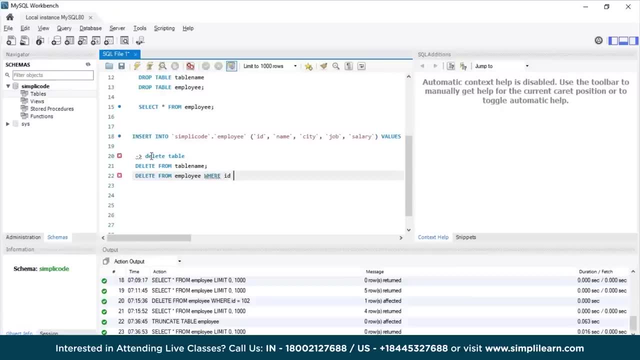 keyword, that is, var ID, is equals to 102.. Let us execute this statement now. As you can see, our statement has been successfully executed. Now I'll display the records by using select statement. As you can see, the employee ID who is having 102 has his employee ID has been successfully. 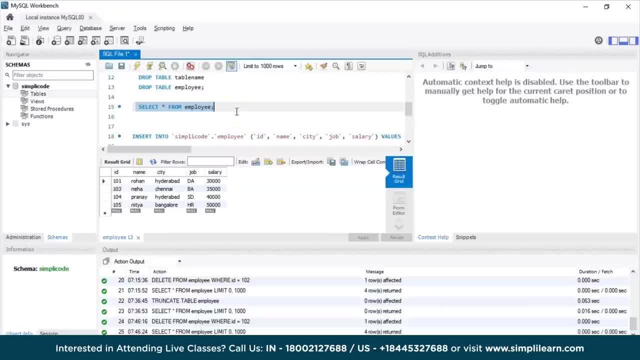 deleted from the table. So in this way, you can use delete statement to delete a particular record from the table. Let us now discuss about truncate table. in SQL, Truncate table statement is used to remove all the rows from the table. That means it deletes the complete data from an existing table. 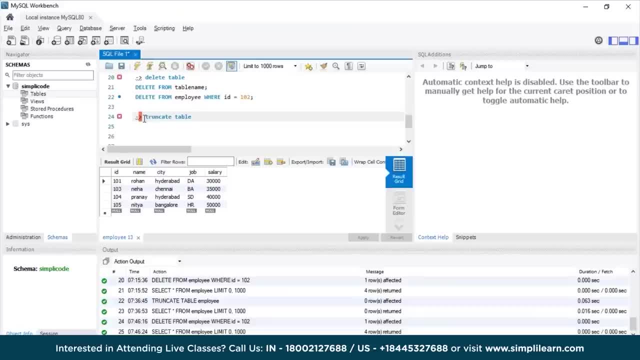 It is similar to that of delete statement, but here we do not use the var clause. Truncate table is faster and uses lesser resources than the delete table command as it deletes the records at a single time. Lock table command can also be used to delete the complete data, but it also deletes the 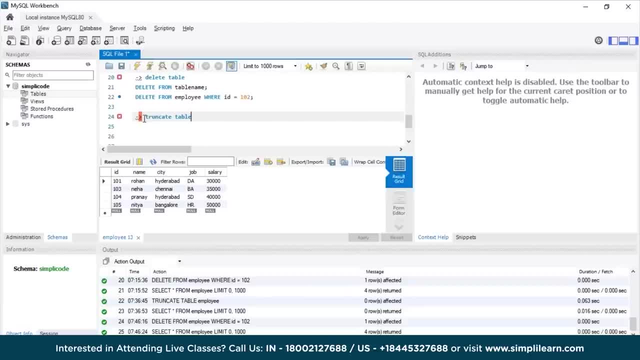 structure of the table as well. Truncate table does not delete the structure of the data. So the syntax for truncate table is truncate table and after that you have to mention the table name. So if I want to delete all the records from the employee table, the following query would: 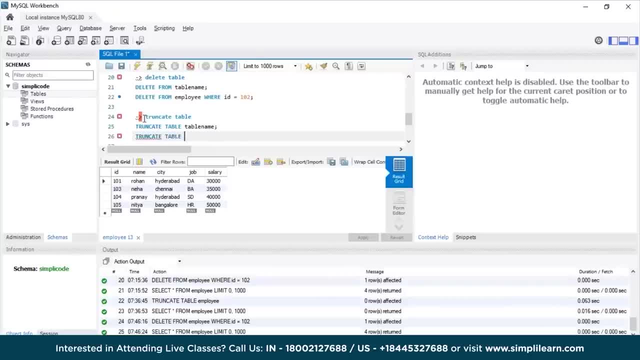 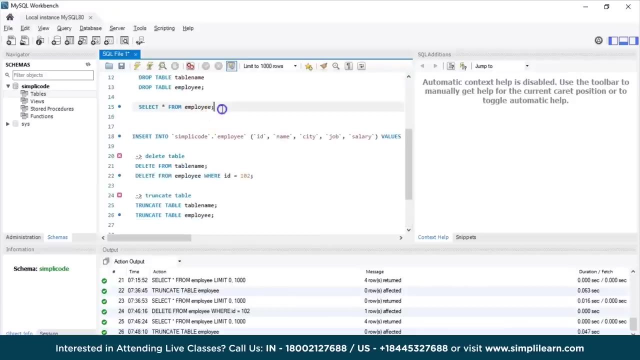 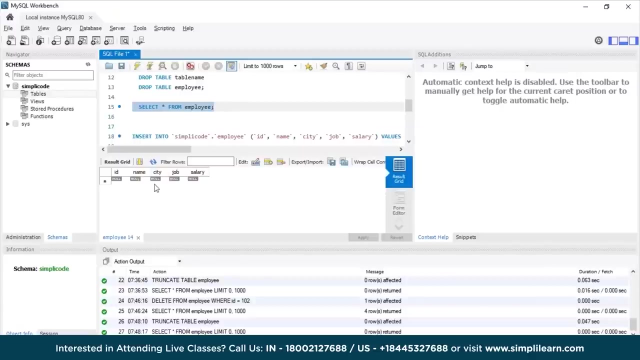 be truncate table, followed by that. Let us execute this and see the output. So the query has been successfully executed. So let me use the SELECT statement to display the records. As you can see, all the information of the employee has been successfully deleted from. 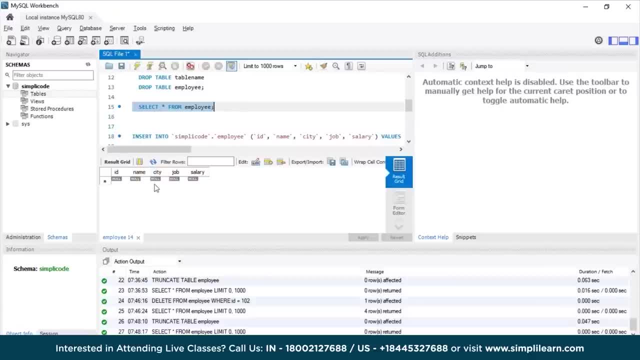 the table. But if you look at the output closely, the structure hasn't been deleted. here The column names of the table, that is, id name, city, job etc. are not deleted, But only the values in the table have been deleted. 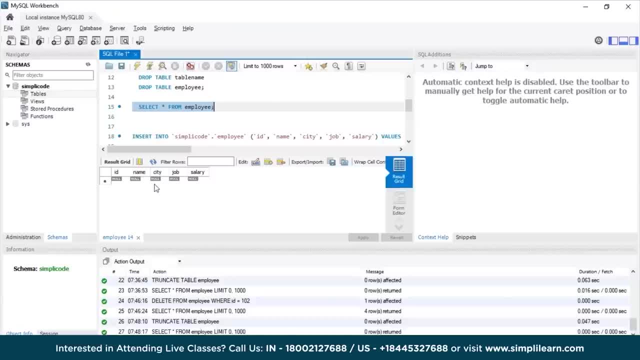 So in this way you can use truncate statement to delete all the records from the table at a single time. Make sure that you use this statement carefully, because the rollback process is not possible after using truncate table statement. That means if the data is once deleted, it is completely deleted permanently. 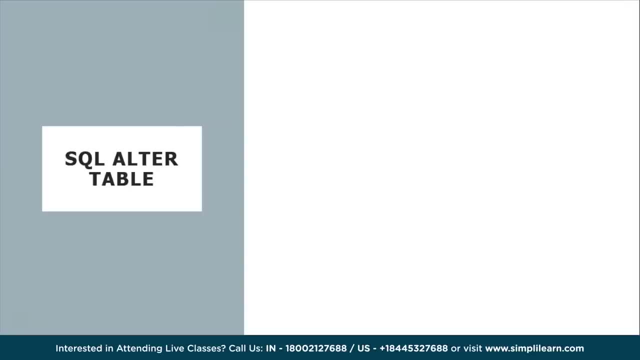 Next, let us see how to use truncate statement. Next, let us discuss about SQL ALTER TABLE. The ALTER TABLE in SQL is used to add, modify and delete columns of an existing table. In many situations you may require to add columns in the existing table. 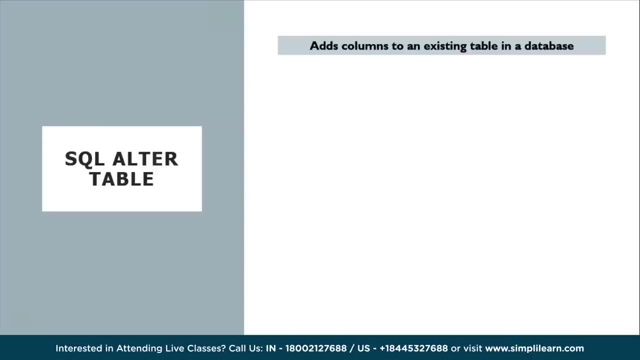 So, instead of creating a whole table again and again, you can easily add single or multiple columns using ALTER TABLE statement with the help of a keyword add. Let us now look at the syntax of ALTER TABLE. The syntax is followed as ALTER TABLE. So here: ALTER TABLE, tableName, add, and within the parenthesis you have to mention the. 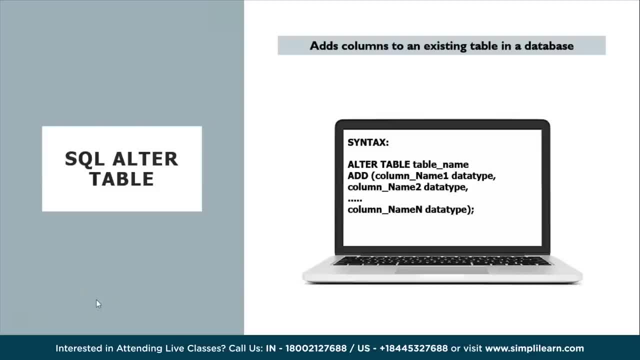 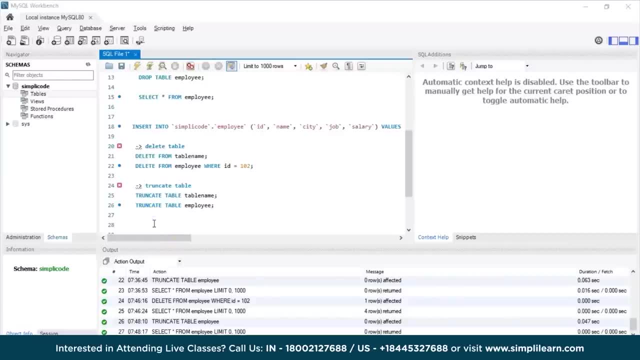 new column and the data type. So let us now jump into the execution part. Consider the same table employee again. Suppose if you want to add a new column that is date of birth of the employee in the above table. For this you have to type the following query as ALTER TABLE, mention the table name that 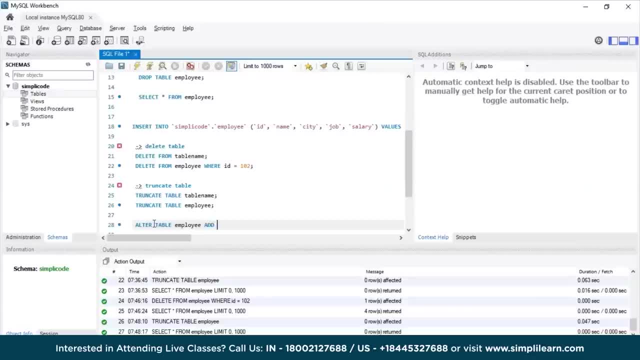 is employee. After that, mention the keyword add and, within the brackets, mention the new column name. that is date of birth and the data type of the date of birth is date. so I'll be mentioning the date data type. Close the brackets and put the semicolon. 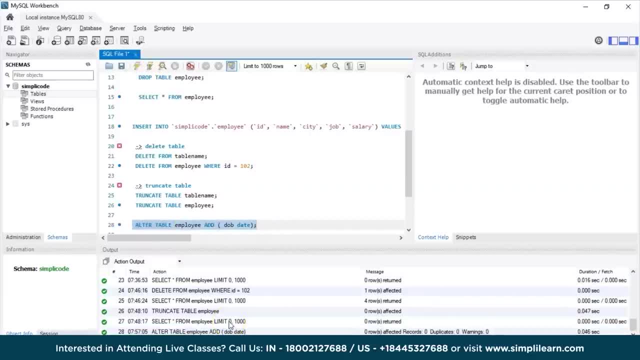 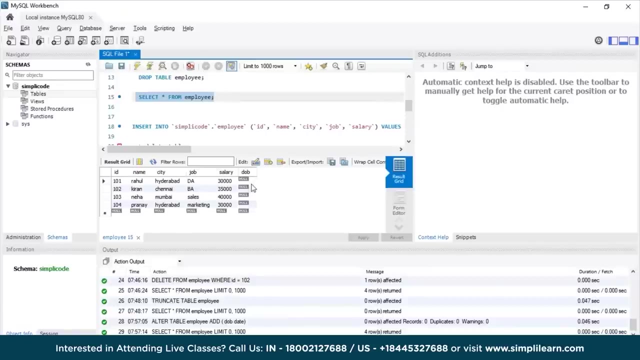 Let us execute this statement now. As you can see, our statement has been successfully implemented and I'll use the select statement to display the new records. As you can see, there's a new column named date of birth has been successfully added to our existing table employee. 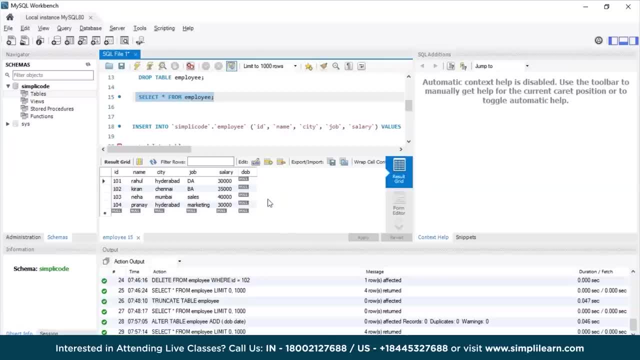 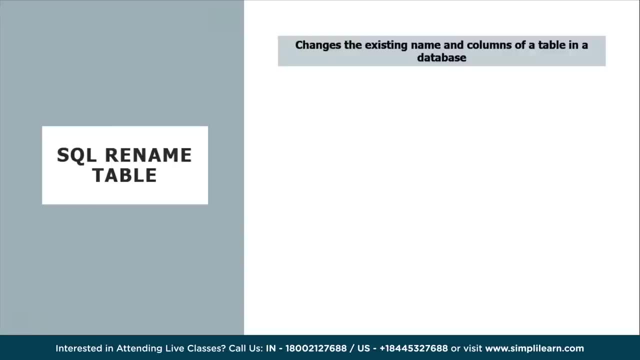 In this way you can use alter table to add or delete the columns from the table. Let us now discuss about SQL rename table. SQL rename table is used in SQL to change the name of the table, So in some situations the database user might want to. 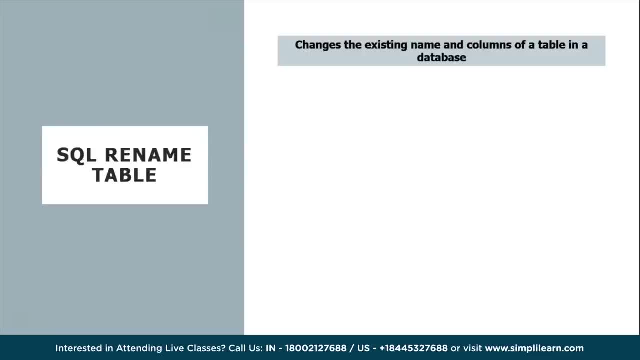 change the name of the table. So in some situations the database user might want to change the name of the table. So in some situations the database user might want to change the name of the table So that they want to give a more relevant name or the updated name to the table. 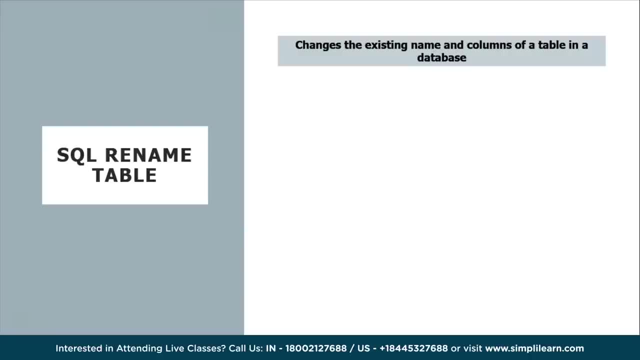 Any database user can easily change the name of the table by using rename table and alter table statement in SQL. Let us look at the syntax now. The syntax is followed as: alter table, current table name, rename to new table name. Let us now execute this in MySQL workbench. Consider the same table employee again. Suppose if you want to change the name of the above table employee into, let's say, employee new, for this you have to type the following query: that is, alter table old table name. that is employee rename to is the keyword that you have to use here and mention the new table. 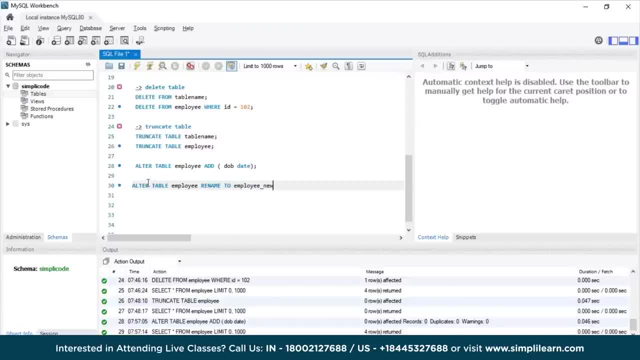 name. We are taking employee new as our new table name, So let us execute this and see the output. As you can see, our statement has been successfully executed, So let let us update the schema here and see whether or not the name of the table is changed. 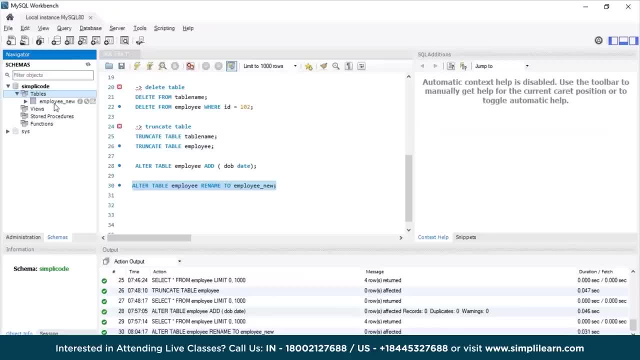 So, as you can see, our table employee, which we had previously, has been changed into employee new. In this way, you can use rename statement to give a new name to your existing table. Finally, let us now look at SQL copy table statement. Let us now look at SQL copy table statement. 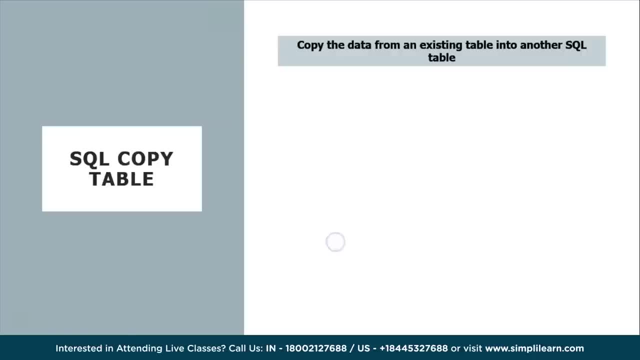 If you want to copy the data of one SQL table into another SQL table in the same SQL database, then it is possible by using the SELECT INTO statement in SQL. The SELECT INTO statement in SQL copies the content from an existing table into a new table. 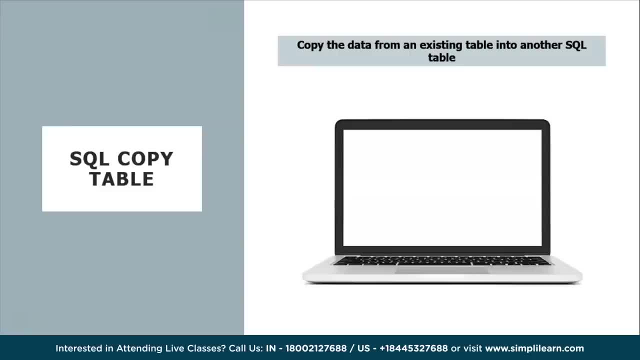 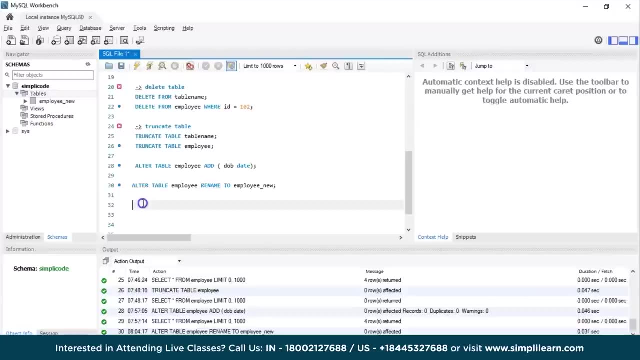 SQL creates the new table by using the structure of the existing table. The syntax is followed as: SELECT star INTO new table name FROM the old table name. Let us now execute this in MySQL Workbench and see the output. Consider the same employee table again and suppose you want to copy the content of the 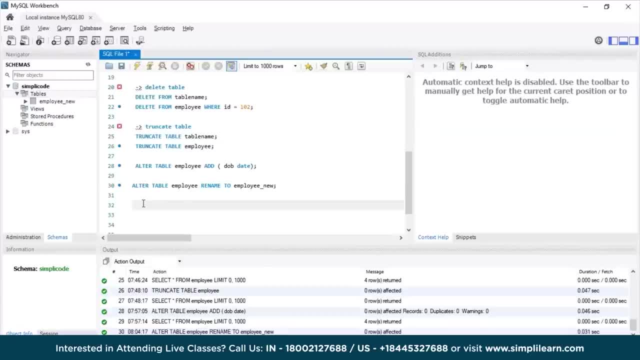 employee table into a new table, let's say employee details. Now, as far as MySQL Workbench is concerned, there is a slight change in the query. Now the syntax that we've discussed earlier is applicable to some other SQL databases like Microsoft SQL Server and Oracle Database. 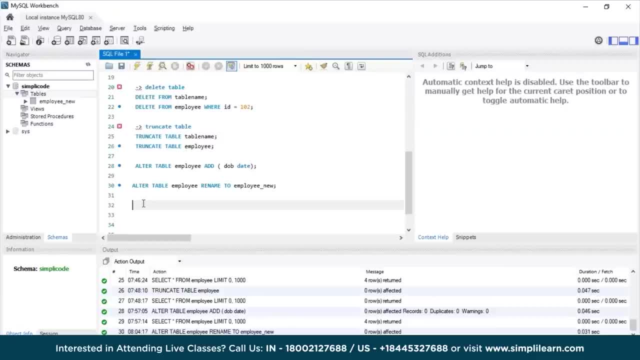 But for MySQL Workbench there is a different syntax to copy a new table. So the syntax is followed as: CREATE TABLE: mention the new table name, that is employee details. Now SELECT star FROM the old table name, That is employee. Let us now execute this and see the output. 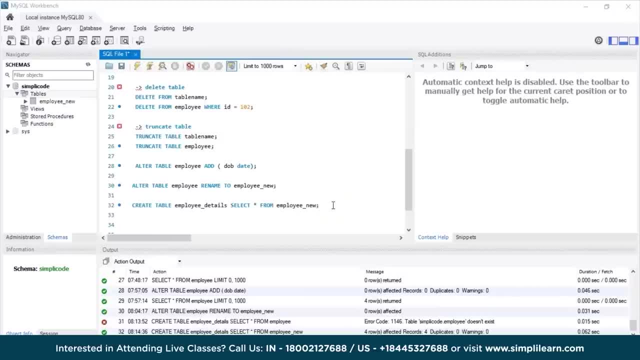 Now it will throw an error, stating that the employee table doesn't exist. That's because we have renamed our previous employee name table into employee new. So instead of employee, change it to employee new and let us execute this statement now. So, in order to display if the employee table is created successfully or not in the database, 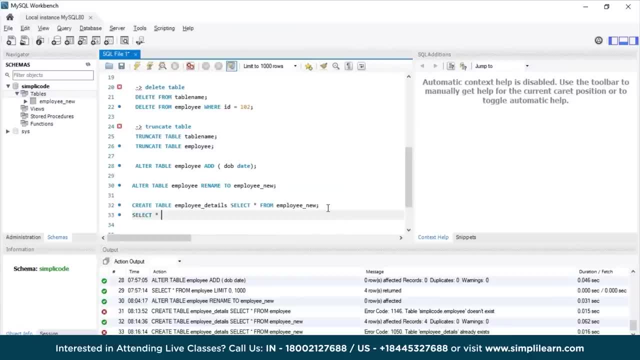 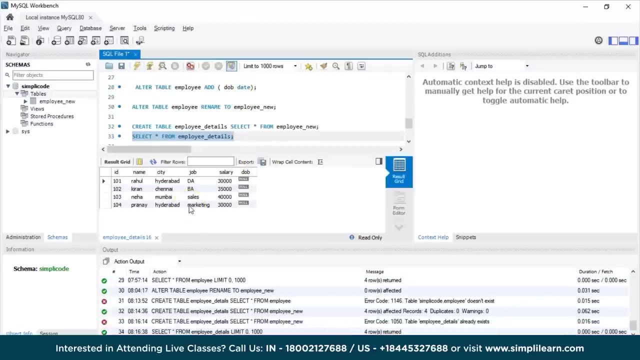 let us use SELECT statement to display the records. SELECT star FROM the table name, which is the new table name, that is, employee details. Let us execute this now. As you can see, the details that we had earlier in our employee new table Has been copied into another table, that is employee details. 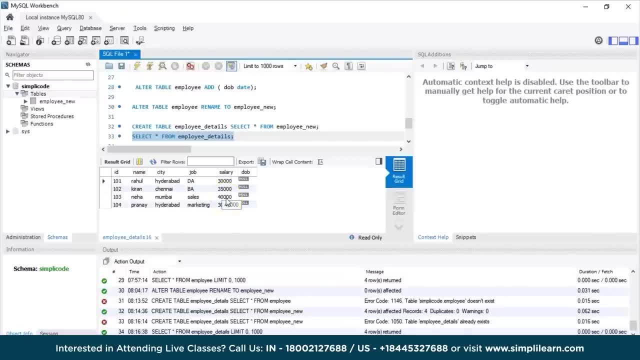 In this way, you can copy the content from one existing table from another new table by using copy statement in SQL, And with that we have come to end of today's session. These were some of the queries that were related to SQL tables. If you want to learn more about SQL, make sure to check out our previous playlist in our 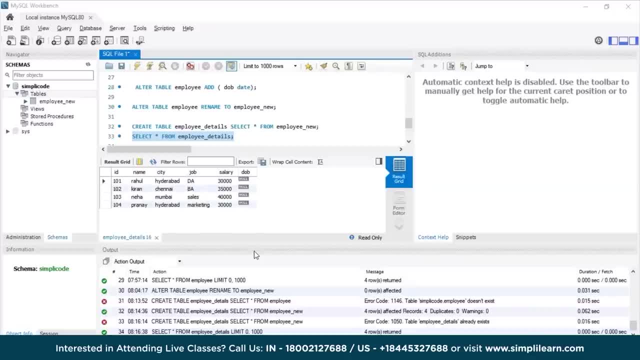 channel. Also, we have a dedicated video SQL full course 2022 for beginners. If you want to learn more about SQL, make sure to check out our previous playlist in our channel. Also, we have a dedicated video SQL full course 2022 for beginners. 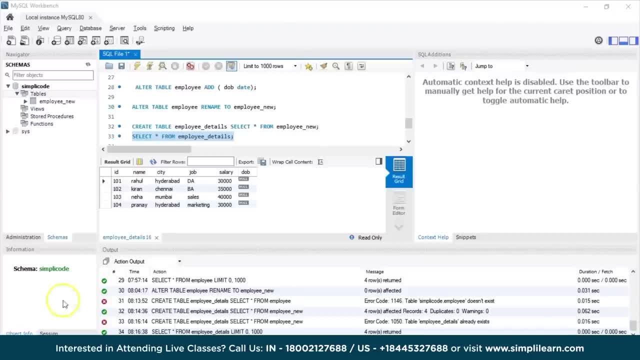 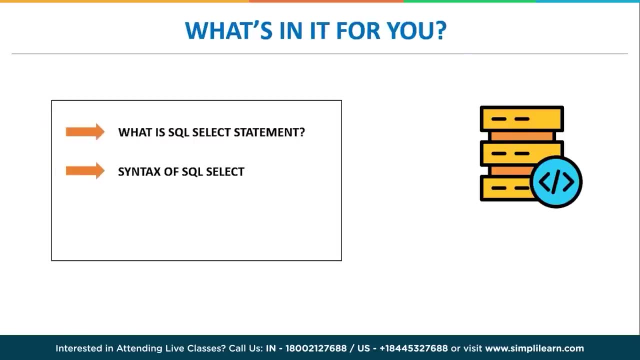 Where in we have discussed SQL and various concepts from the scratch. Firstly, let us discuss the agenda for today's session. We will start the tutorial by understanding what is SQL SELECT statement, And then we will discuss the syntax of SQL SELECT statement And finally we will go through some different functions in SQL SELECT statement. 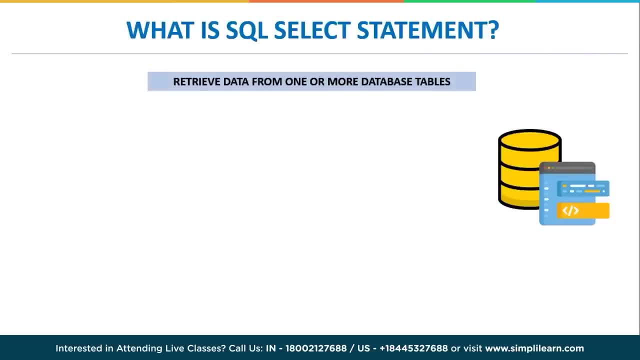 What is SQL SELECT statement? SQL SELECT statement is used to fetch the data from a database table, which returns the data in the form of a resultant table. In simple words, we can say that it is used to access the information from one or more database tables within the database. 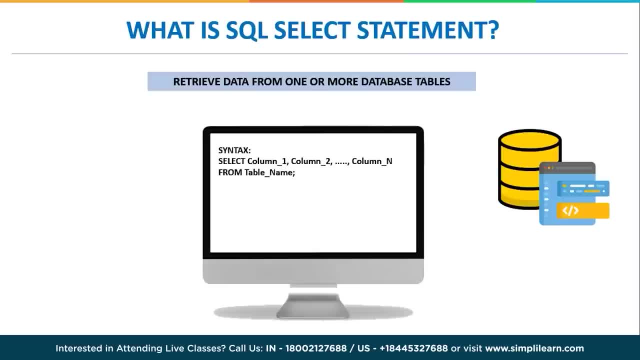 Let us look at the syntax of SQL SELECT statement. The syntax is followed as: SELECT column FROM table name. In the SELECT syntax you can see column name 1, column name 2 and n. number of columns are the name of those columns in the table whose data you wanted to read. 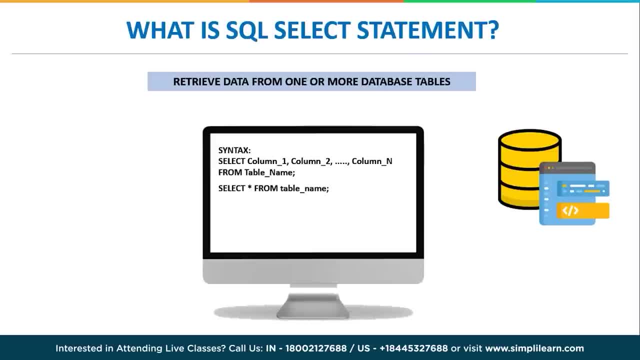 And if you want to access all the rows from all the fields of the table, you can use the SELECT star operator in the database by using SELECT star FROM table name command. Let us look at an example. If you want to retrieve the information of the student who is having role number, name. 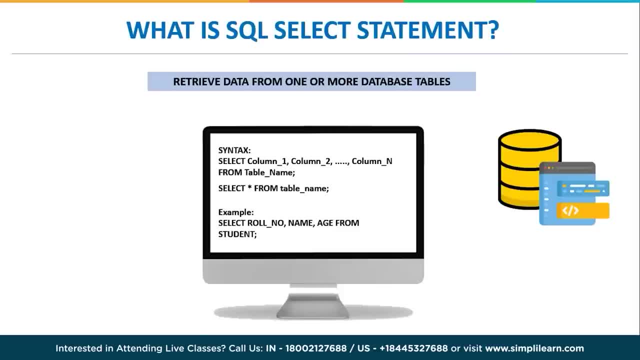 and age. we can write a simple query as SELECT: role, number, name, age FROM student. In this way, we can display the details of the student. Let us see how to do this. Let us see how to do this SQL SELECT condition. 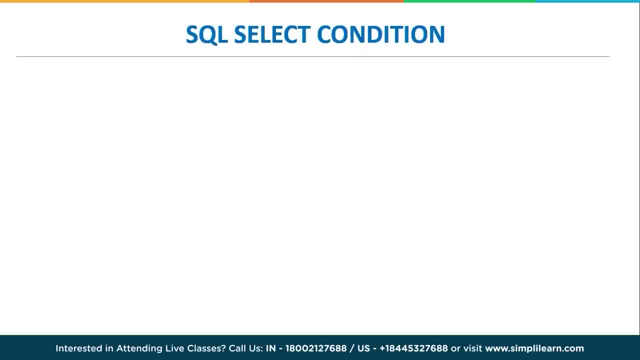 SELECT statement is used with various clauses as well. That means it also retrieves the selected data that follows a particular condition with the help of a WHERE clause. By using this command, we can access a particular record from a particular column of the table. Let's understand this with an example. 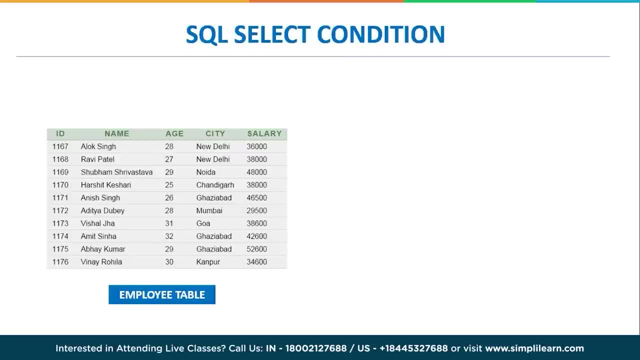 Consider the employee table here, which is having ID, name, age, city and salary as its column in the table. Let's say, if you want to access the information of those employees who is having age as 29.. For that we will write a simple query as: SELECT star FROM employee WHERE age is equals. 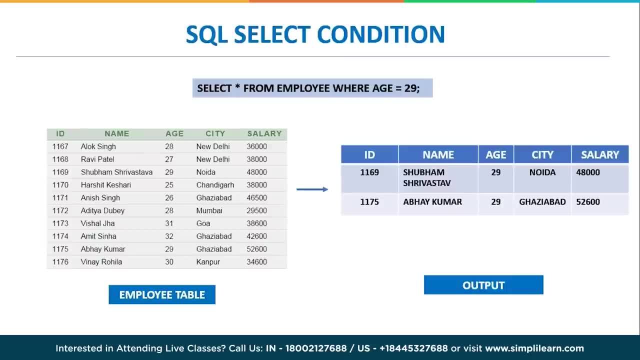 to 29.. And if we execute this, this will be the following output, which shows the information of those employees whose age is 29.. So in this way, you can use SQL SELECT condition by specifying a WHERE statement, which is used to filter the data in a particular table. 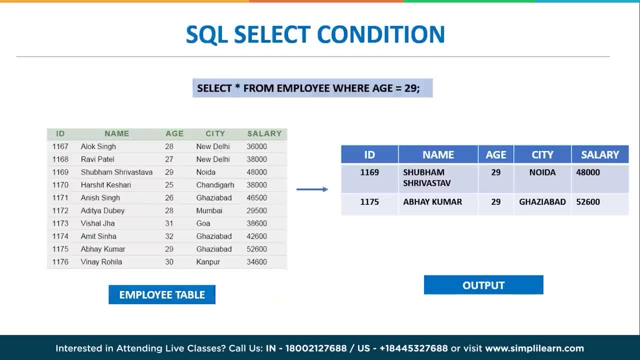 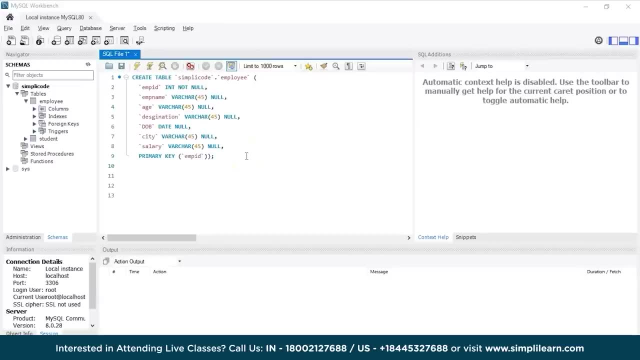 Now that we have understood the basics of SQL SELECT statement, Let us move on to the next step. Let's now jump into MySQL workbench and execute this and understand it in a more better way. As you can see, MySQL workbench has started and, for time being, I have already created. 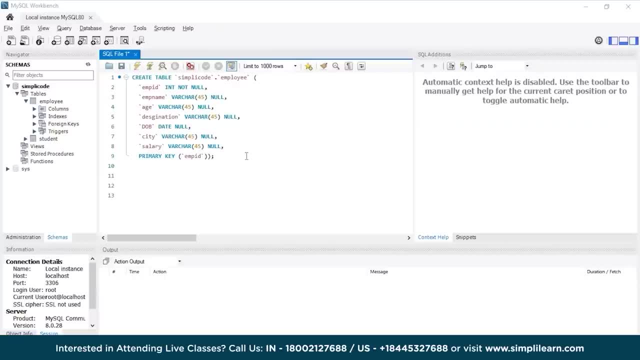 a table employee which is having column names as employee ID: employee name, age, designation, date of birth, city that they belong to and salary. And I have chosen primary key as employee ID because it uniquely identifies each and every record in the table. 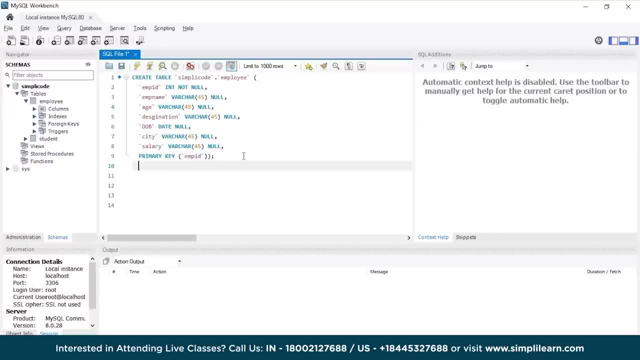 Now that We have created a table, in order to display all these records, we have to use this SELECT statement. ultimately, So to display all the values from each column of the table, that is, the employee table, we have to write the following query as SELECT star FROM table name, that is employee. 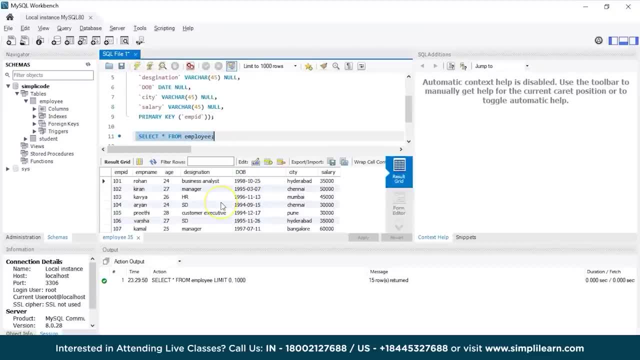 Let us execute this and see the output. As you can see, it will display all the values of the employees: their employee ID, employee name, age, designation, date of birth, the city and their respective salaries. So if you want to display a particular column, so for that you have to write the query as: 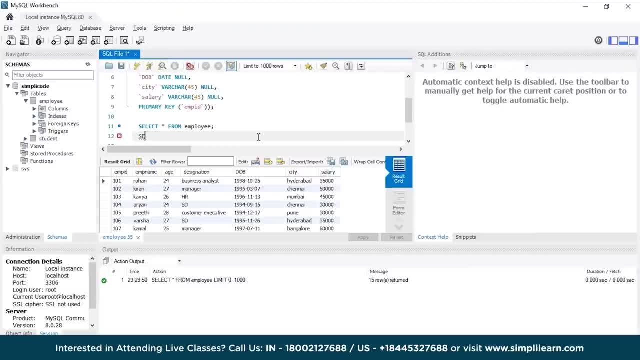 let's say, if I want to select employee ID, employee name and the city of the employees, So for that I will write SELECT employee ID comma. employee name comma. let's say I want to display the salary, So I am taking a salary from table name. that is employee. 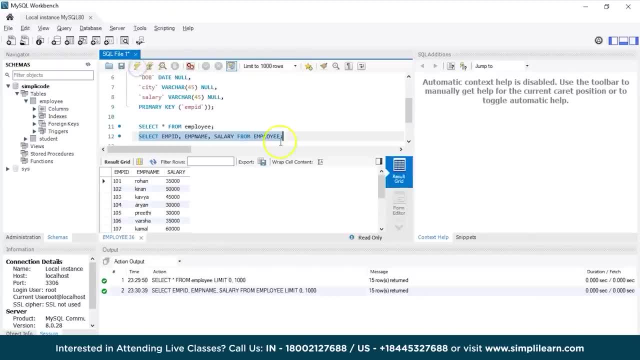 Let us execute this now. So, as you can see, only the employee ID, employee name and the salary of the employees in the table are being shown here, because we have only specified a particular column in this case. Now, similarly, we can use WHERE clause also. 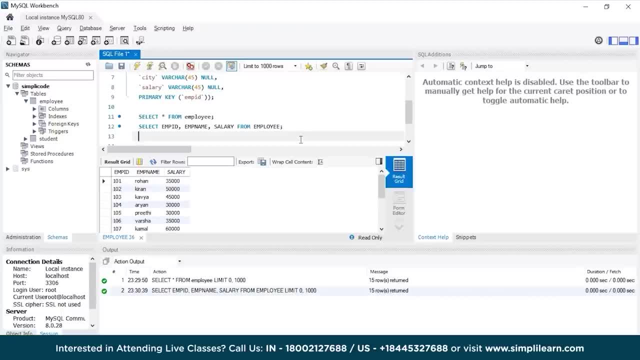 The WHERE clause is used with SELECT- SELECT statement to return only those rows from the table which satisfy the specified condition in the query, For example, if I want to show the salary of the employee who is having more than 30,000.. So for that I will write the query as SELECT star from employee WHERE salary is greater. 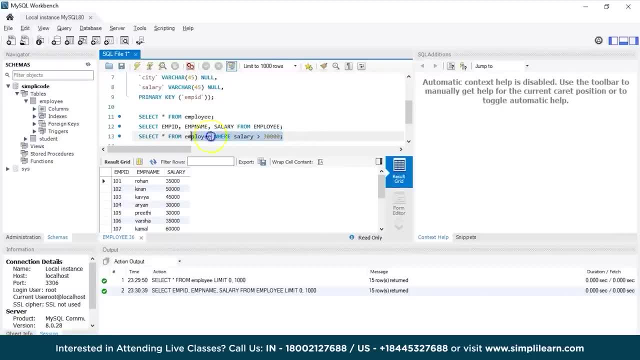 than 30,000.. So let us execute this statement and see the output. So, as you can see, it will display the records of all those employees who is having salary more than 30,000.. Similarly, you can see, you can also check whether the city that they belong to is Mumbai. 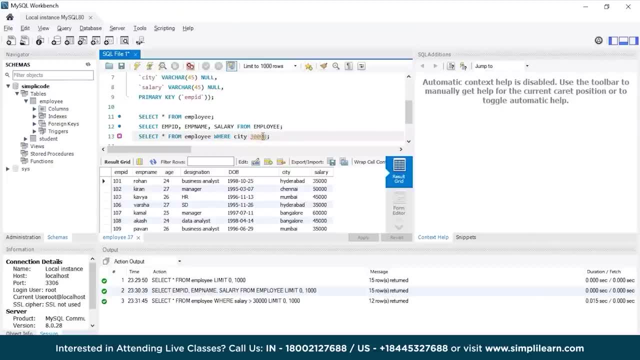 So for that we have to take the SQL query as SELECT star from employee WHERE city is equals to. suppose I want to display the employee who belongs to the city Mumbai, So for that I will take the city as SELECT star from employee WHERE city equals to Mumbai. 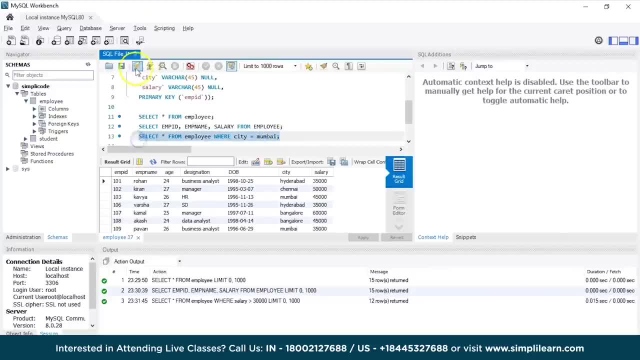 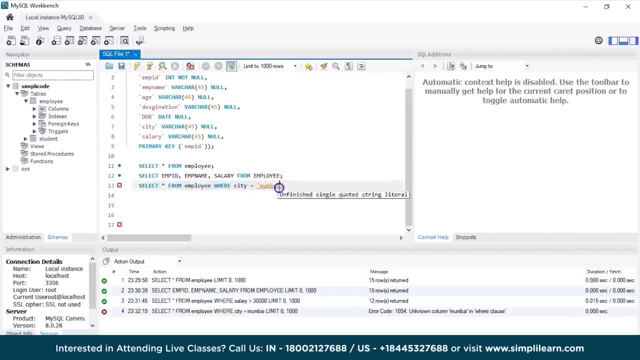 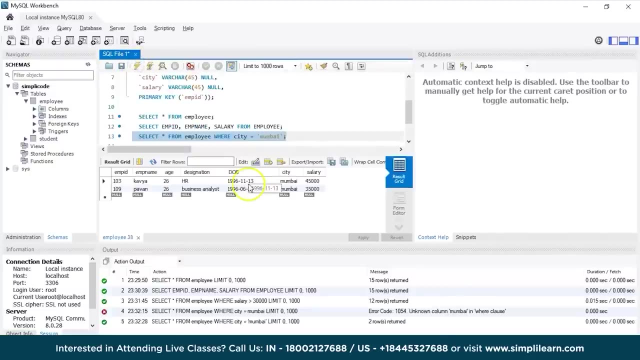 So for that, I will take the city as SELECT star from employee WHERE city is equals to Mumbai and execute the statement. Okay, you have to mention Mumbai in single quotes, So that is the reason it is showing error here. So let us now execute this and see the output. 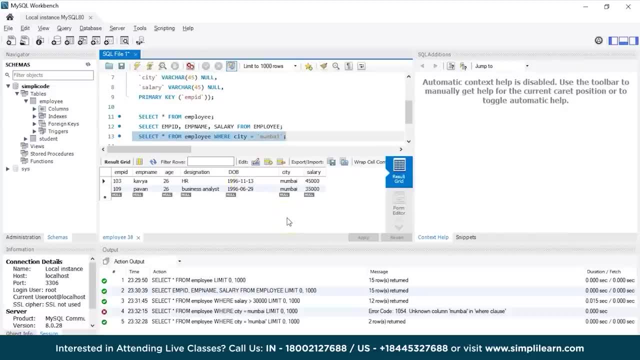 So, as you can see, there are only two employees who belong to this city, that is, the employee Kavya and Pawan, who is a having the employee ID 103 and 109.. So in this way, you can use select statement ah to display a particular record by using var clause. 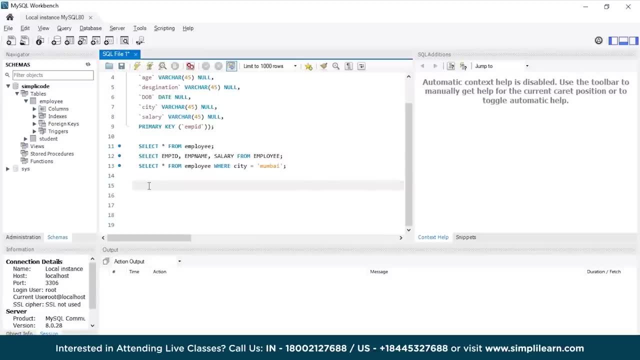 Now that we've got an idea on how SQL SELECT statement works, let us now discuss some SELECT statement functions. The first one is SELECT distinct. The SELECT distinct in SQL is used to fetch identical or distinct column values from existing table without any duplicate values. Now suppose in a particular table there might 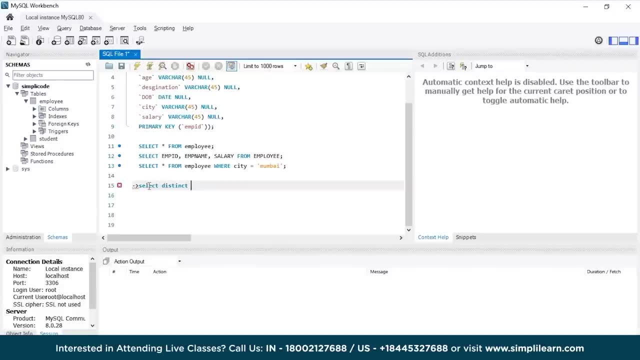 be a higher chance that there exists a duplicate value and if you want to retrieve only unique values in such scenario you use a SQL SELECT distinct statement. I know it might be a bit confusing, so let me make it clear to you guys. Consider the same employee table again here. 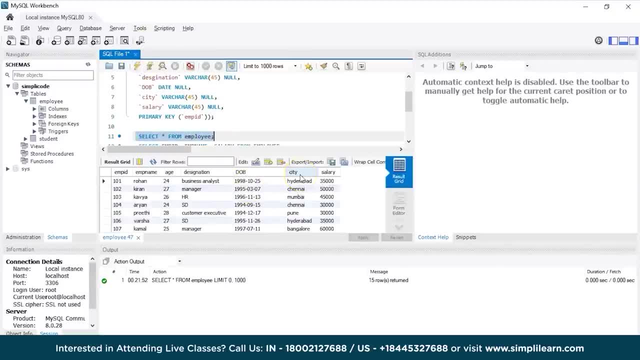 and if you look at the table, the values in the column city, the Hydra table and the SQL SELECT table are the same. Hyderabad has been repeated more than once here, and not just Hyderabad: Chennai has also been repeated twice. So in this case in a broader sense, 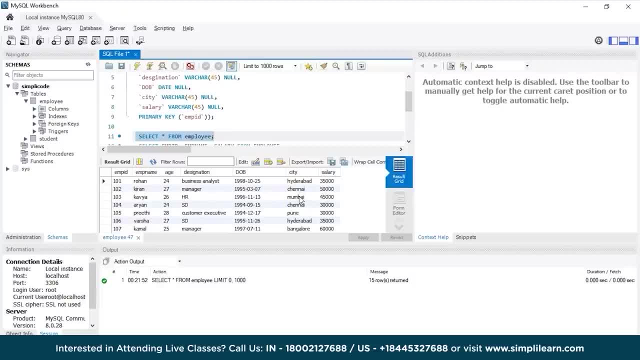 if I just wanted to know from which city the employee is from, I'll just use the distinct SELECT statement. So, using this, instead of multiple values that are being displayed, the SQL SELECT distinct statement makes sure that the value is retrieved only once and there is no room for any repeated or distinct value. So let us 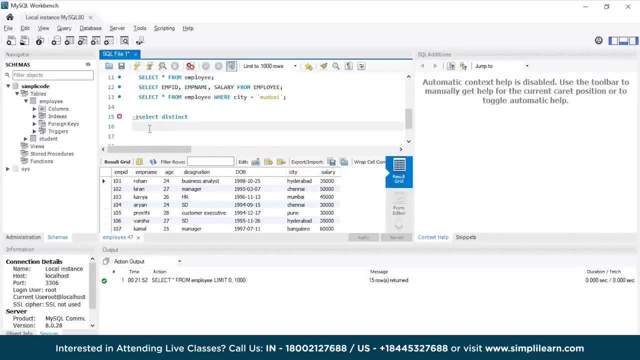 now understand this syntax with an example. The syntax is followed as SELECT distinct. Now let's say, if I want to fetch a distinct designation of all the employees of the company, so for that I'm specifying the column name here as designation from the table that is employed. Let us now execute this. 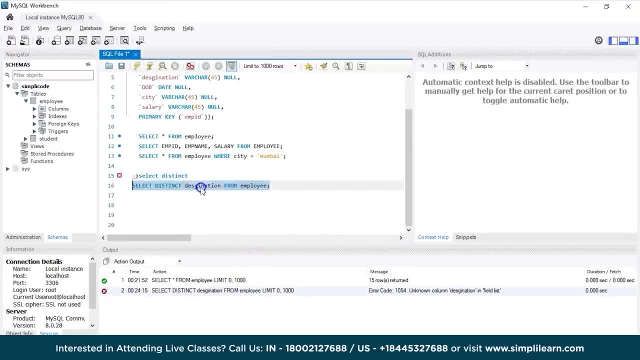 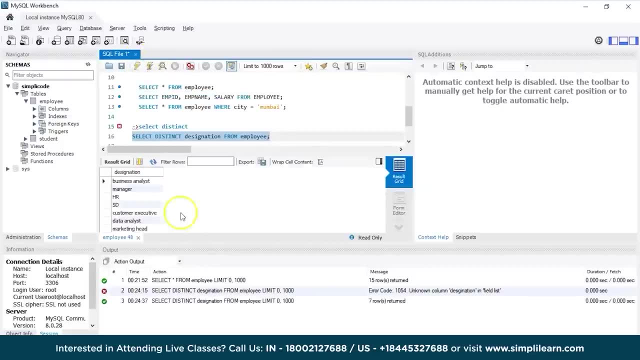 There is a bit error in the code. Let me just check it. So let us execute the query now and see the output. So, as you can see, this is the output that is being displayed, where the unique values of the designation of all the employees are being displayed. That is, business analyst manager. 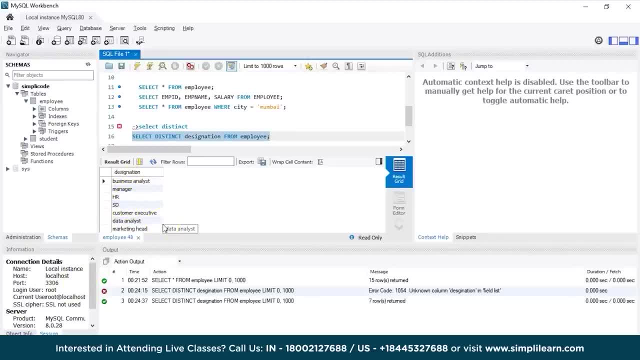 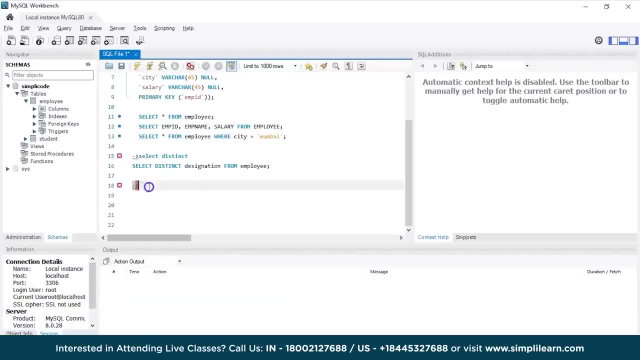 HR, SD and so on. So in this way, by using SQL SELECT distinct statement, we can fetch distinct values from the existing table. Let us now discuss about select count statement. in SQL, The SELECT count is used to get the total number of rows from a table. 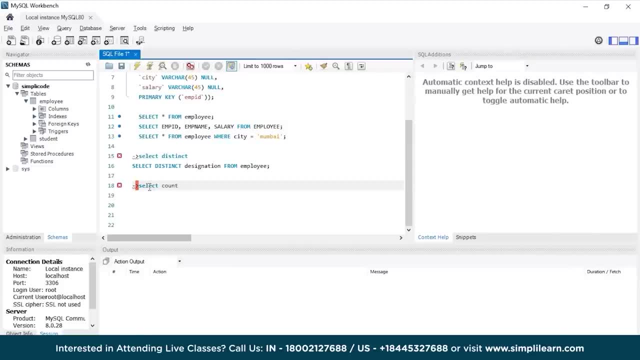 Basically, it returns the total number of records present in the database table. Let's take a simple example. Consider the same employee table Now, if you have a record in the table and if you want to count the total number of records in the table, 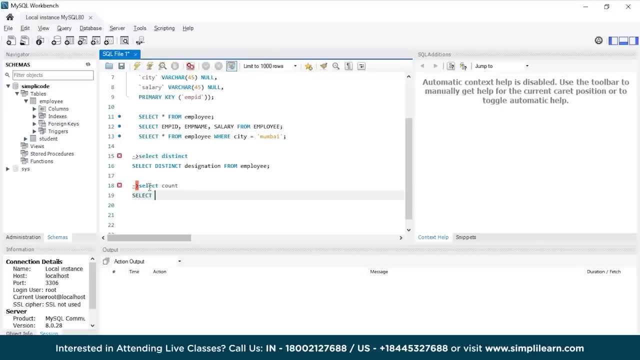 for that, the following query would be: SELECT count from the table, while SELECT number of records still present in the database table. select count star from the table name, that is, employee. let us execute this and see the output now. so, as you can see, there are total 15 records present in. 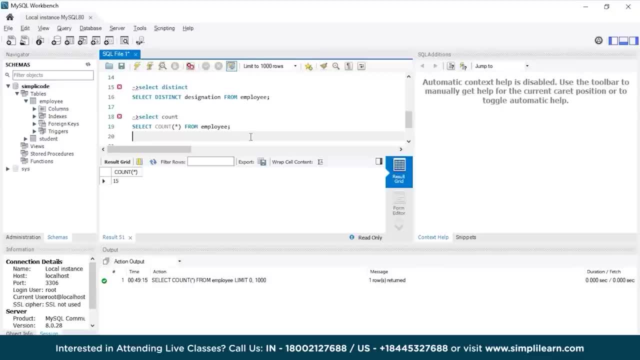 the employee table. similarly, you can use the where condition as well if you want to get the total number of rows of the employees who are having salary equals to 50,000 in the employee table. so for that the following query would be: select count asterisk from employee. specify the condition here now where salary is. 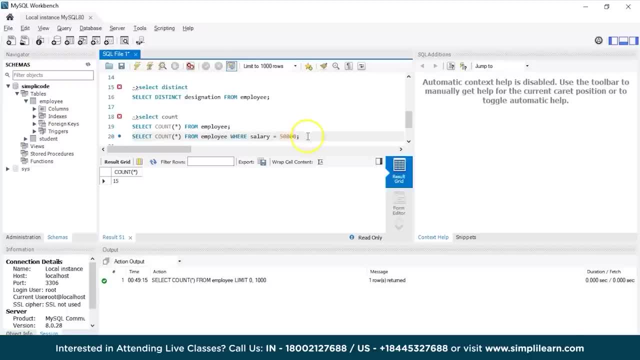 equals to 50,000. let us execute this statement now, so, as you can see, there are total three employees who are having salary equals to 50,000. similarly, you can get the total number of rows in a table by using the distinct statement as well. let's say, if you want to retrieve a unique count of the city. 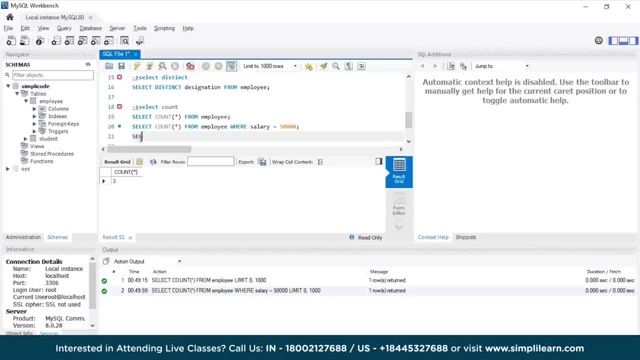 of the employees from the table. the following query would be: select count, which is the keyword that we are using, and inside the bracket, mention distinct keyword followed by the column name. that is city. from the table, that is employee. now let us execute this statement and see the 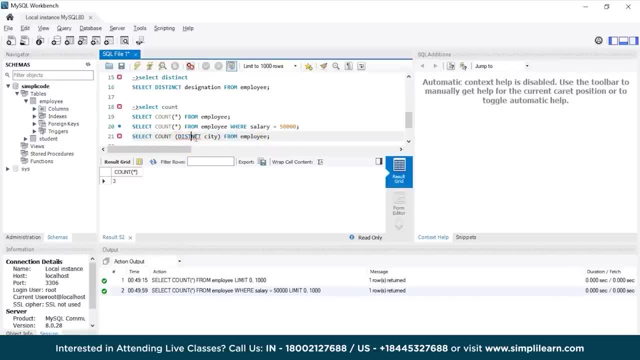 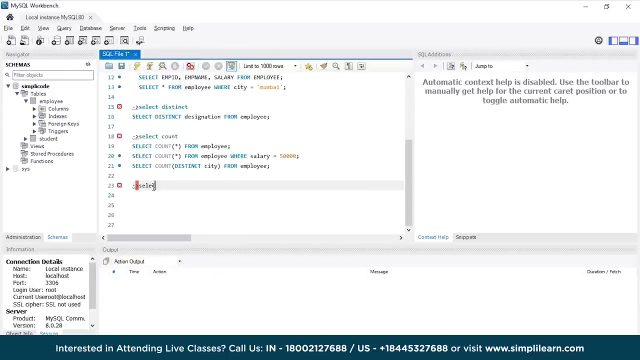 output. so, as you can see, there are total eight employees who are belong to different cities. so in this way you can use a select count statement to retrieve various number of records in the particular table. next let us discuss about select top or limit statement in SQL. the select top statement in SQL shows the limited number of records. 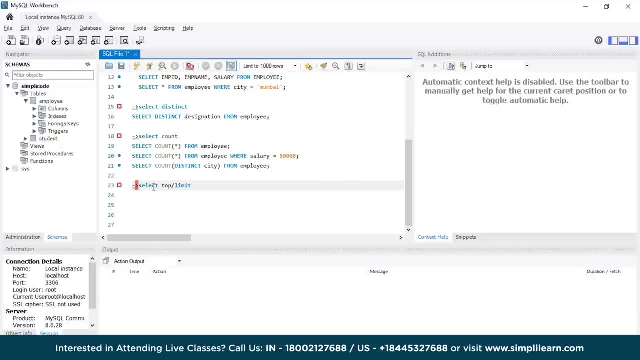 or rows from the database table. the top clause in the statement specifies how many rows we want to display from our table. this clause is used when there are thousands of records in the database table. now all database systems do not support top keyword. now as far as mysql. 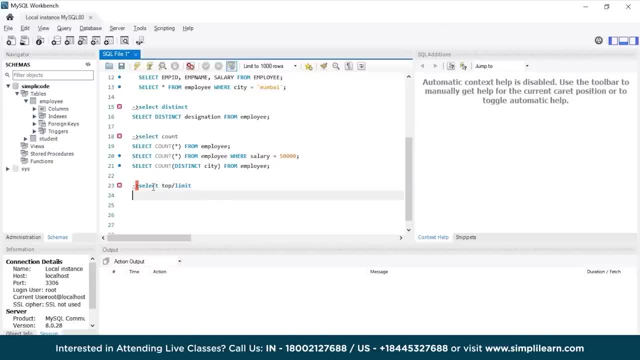 is concerned, it supports the limit keyword. so let us now look at the syntax of select limit statement. the syntax is followed as select star from employee table limit is the keyword that we have to use, and I will show you the definition of the keyword, if you are. 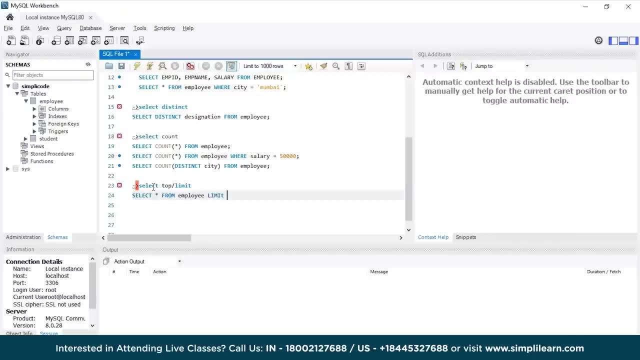 looking for the best way to find a key. So if you are looking for a keyword that you are using in the database and you want to see where you want to get that key, in the database you can see the citizen name or the, And I want to display the first three records of the employees, so I'm specifying three here. 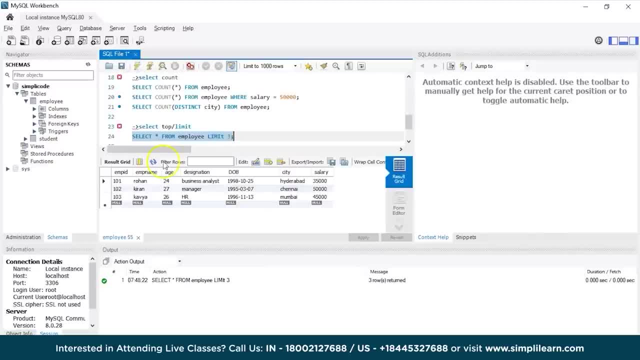 So let us execute this statement. So, as you can see, the first three records of the employees who are having employee ID as 101, 102,, 103 are being displayed. Let us consider another scenario here, If you want to fix the first three employees who got. 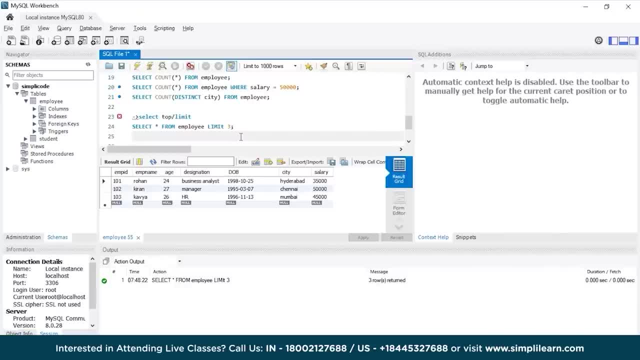 highest salaries from the employee table. then the following query would be: SELECT star FROM the table name that is, EMPLOYEE ORDER BY is the condition that I am using to display the employee details: SALARY DESC. that means descending. Now I want to display the records in the descending order. 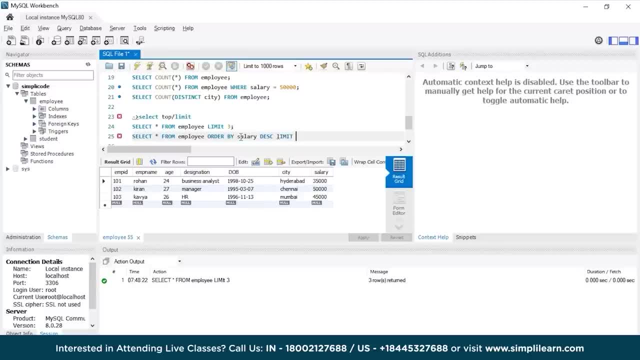 I am limiting the value up to 2.. So let us execute the statement now. As you can see, it will display a total of three records: who got the highest salary, in the descending order, That is, Kamal, who got the salary as 60,000, Sindhu having 50,000, and Kiran, who is 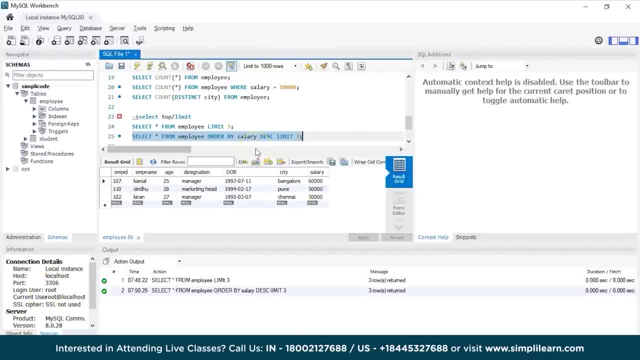 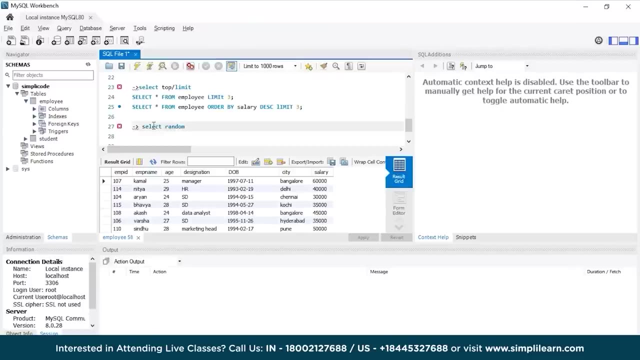 having 50,000.. So in this way you can use LIMIT statement to display the value of the employee. It is not necessary to display the specified rows, that is, the top rows in the table. Next, let us discuss about SELECT RANDOM statement in SQL. As the name suggests, 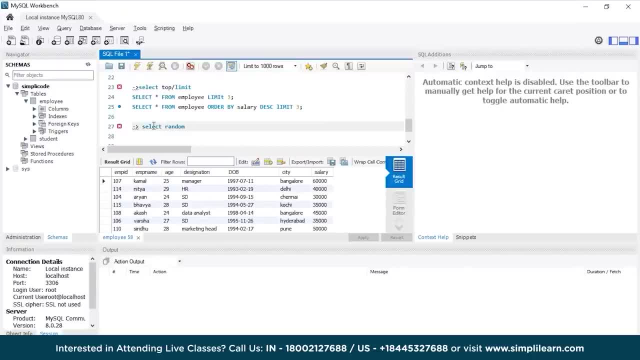 SQL SELECT. RANDOM statement is used to return a random row from a table present in the database. It has many real-life applications. For example, if a HR manager wants to send 10 random mails to his employees, then he can use RANDOM function in SQL. 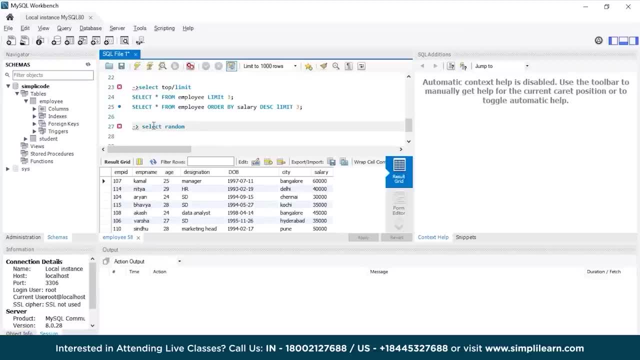 to send the email. It is also used to display random questions during an online exams for students, So the syntax for SELECT RANDOM is followed as SELECT column name. Now I want to display the records of all the employees, So I am choosing star operator from the table, that is. 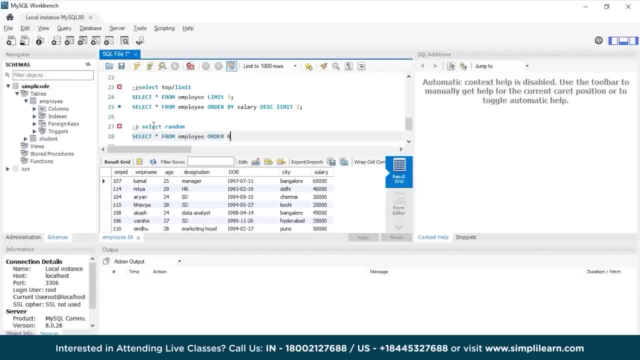 employee ORDER BY is the conditional clause we have to use, Followed by that, we have to mention RAND. Let us execute this statement. So, as you can see, the details of the employees are being displayed in a mixed manner, That is, they are displayed in a random way. As you can see the employee details of employee. 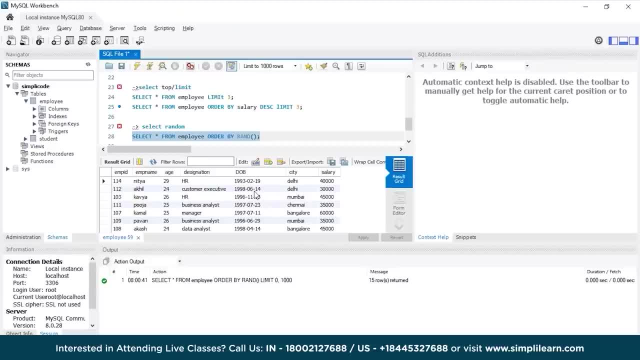 who is having ID 114 is being displayed here first, and then 112 and then 103.. So in this way you can display the values randomly using RANDOM function in SQLS. Similarly, you can also limit the values of employees If you want to. 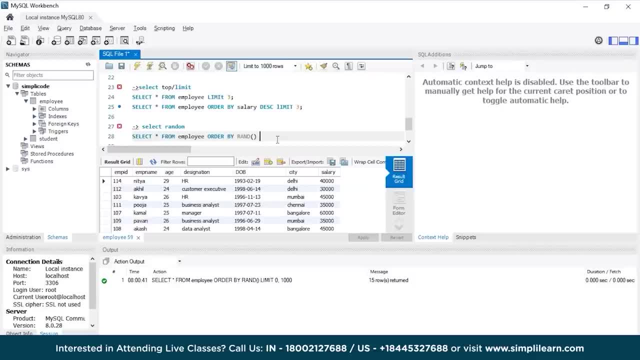 show the top 3 random values of the employees. you can serve an LIMIT statement here, So if I want to display the first 4 records of the employees, So I am choosing 4.. Let us execute the sticker statement. It will serve the details of all the employees. 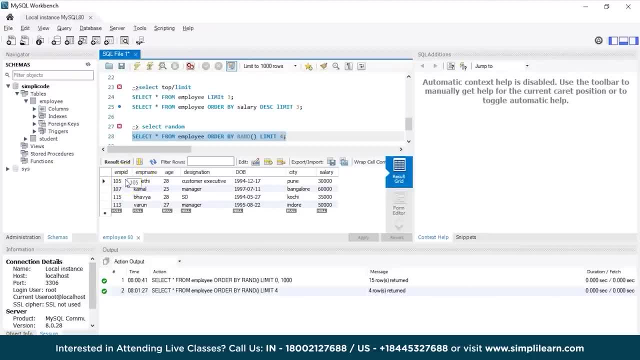 and the está listens randomly up to 4.. Now let us execute the statement That is the top four details of the employees. So in this way you can use a random statement to display random values within a database table. Next let us discuss about SELECT IN statement in SQL. 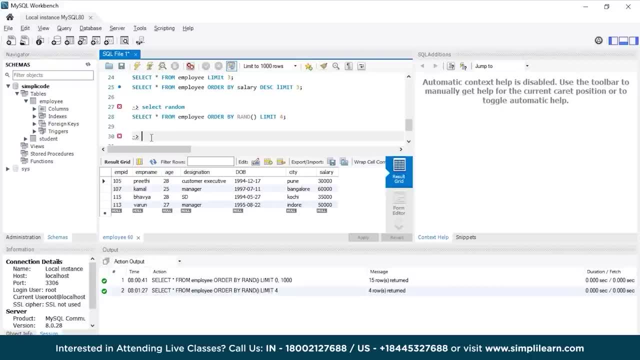 The SELECT IN function is used to fetch specific rows or values from an existing table with multiple conditions. The conditions are specified with IN clause. The operation of SELECT IN is same as OR operation. SELECT IN is used to reduce the multiple OR operators in SELECT statement. 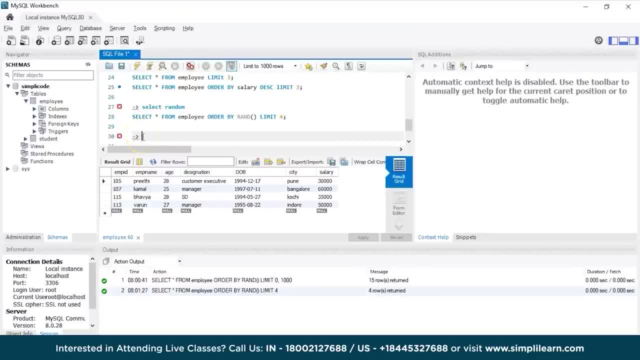 Let us understand this with an example. So if I want to fetch the details of employees who are having employee ID, as let's say, 102 or 104 or 107, from the employee table, then the following query would be: SELECT star from the table, that is. 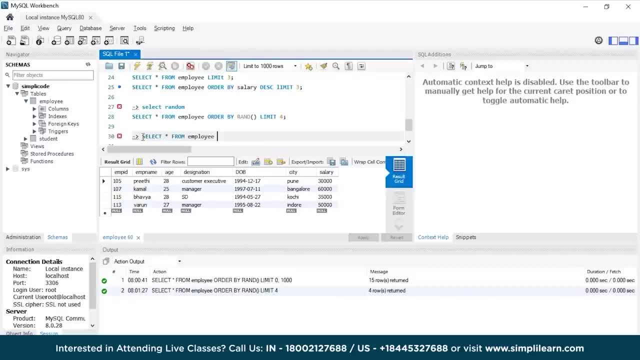 employee where employee ID. Now we have to mention the IN keyword here and within the brackets, mention the IDs. So I am taking 102, 104 and 107. So let us execute the statement and see the output. So, as you can see, it is displaying the values of the employees who are having ID either 102 or 104 or 107. 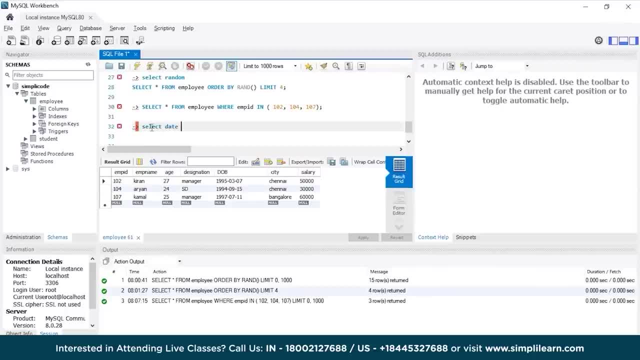 Next, let us discuss about SELECT DATE statement in SQL. SQL SELECT DATE is used to retrieve the values of date from a database. If you want to find a particular date from a database, you can use this statement. So let us understand with an example. 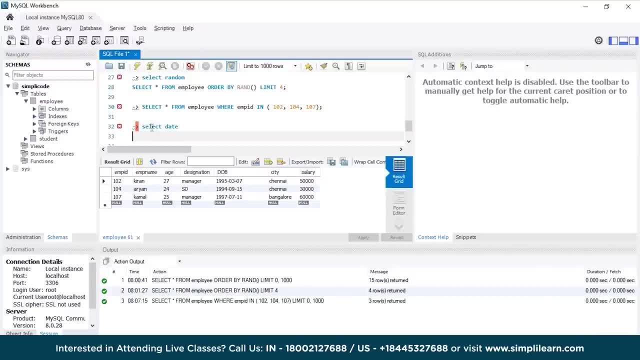 Let's say, if you want to Display the records of all those employees who are born before 1995 Jan 1st, So the following query would be: select star From the table that is employee Where date of birth is Less than 1995 Jan 1st. 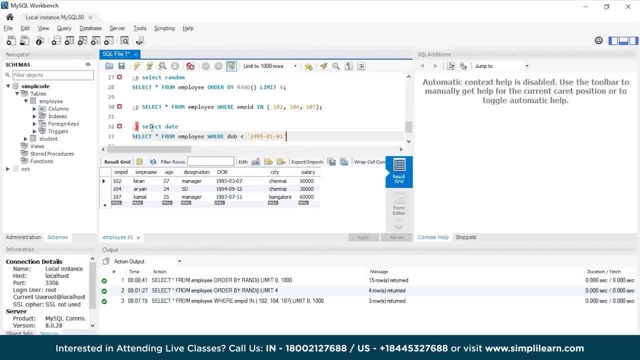 Make sure you incorporate the date in the single quotes, Otherwise it will throw an error. So let me execute this statement. So, as you can see, it is displaying the records of all those employees who are born before 1995 Jan 1st. similarly, you can use a. 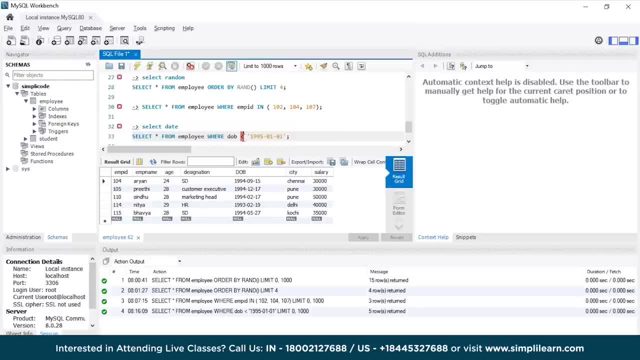 Greater than operator as well, to show the employees were born after 1995. similarly, if you want to fetch the employees who have born between a particular date, let's say who are born between 1996 and 1998, then the following query would be: select star from employee where date of birth. 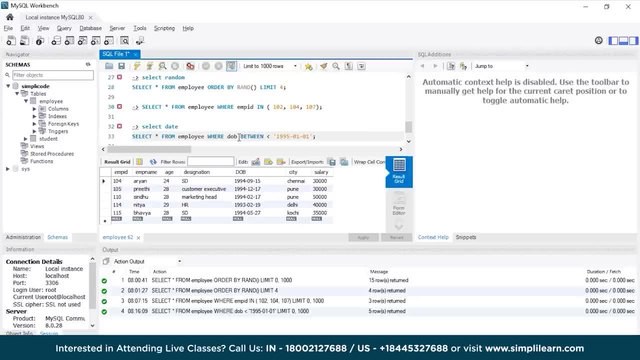 Between is the keyword we have to use. Between, let's say I'm using 1996 Jan 1st and 1998 and 1998 Jan 1st. so let me execute the statement and see the output. so, As you can see, it is displaying the records of all those employees who are born in between. 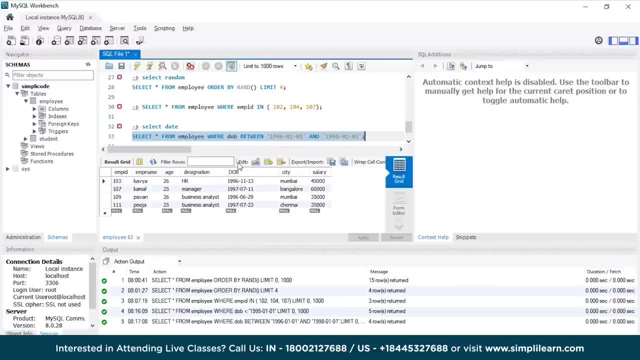 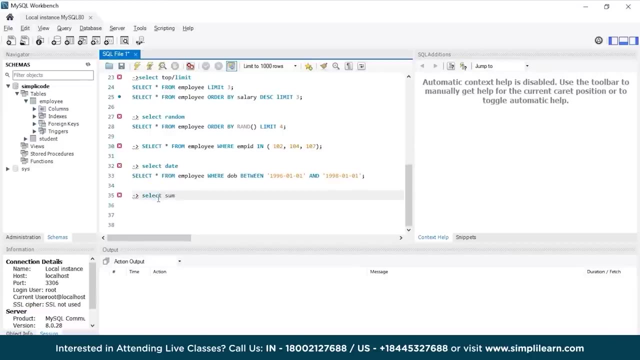 The particular date that we have given, that is, in between 1996 and 1998. So in this way you can use the select date statement to retrieve the date values in the database. Next let us about select some statement in SQL. select some is used to return the sum of. 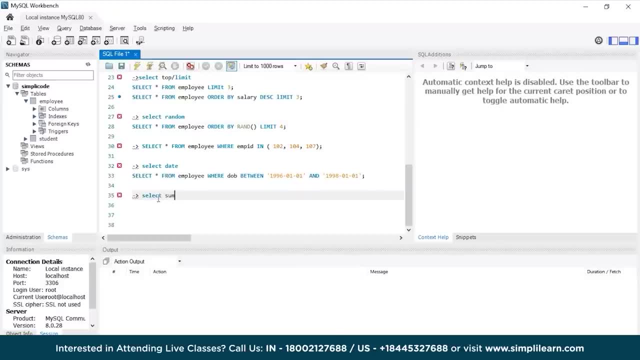 all the values in a specified column. now you have to make a note here that some some function is applied only on numeric or numeric related fields. let us consider the same employee table again, and if you want to get the sum of all the employee salaries in the employee table, then the following query would be: 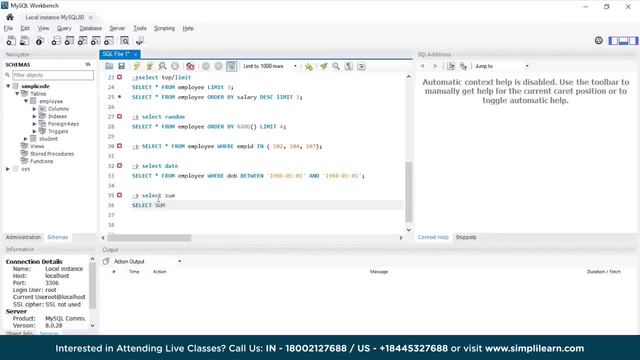 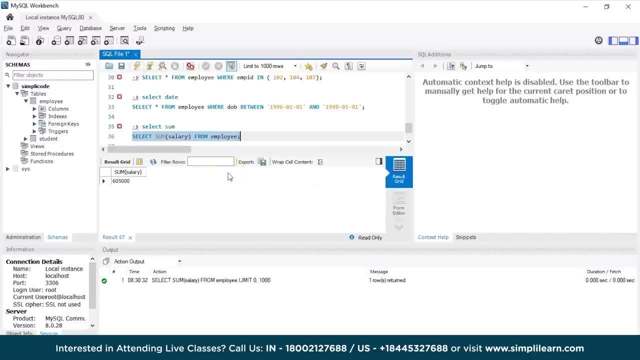 select some is the keyword, and within the brackets mention the salary column from the table, that is employee. let us execute the statement and see the output. so, as you can see, it is showing the sum of the salaries of all the employees here. that is, six lakh five thousand is the total value of the combined salary. 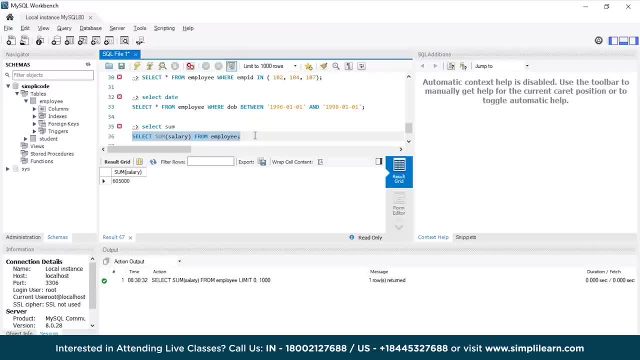 of all the employees. similarly you can use the where condition here as well to get the sum of the salaries of employee by specifying a condition. let's say, if I want to get the total salary of all those employees who belong to the city Mumbai, so for that I am writing the. 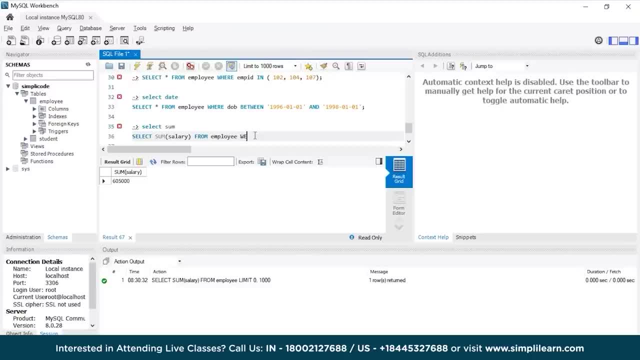 query as: select some salary from employee. where is the conditional clause? city equals to Mumbai. make sure Mumbai is in single quotes, otherwise it will throw an error. let us execute the statement now and see the output. so, as you can see, it is displaying the sum of all the salaries of those employees belonging to Mumbai. 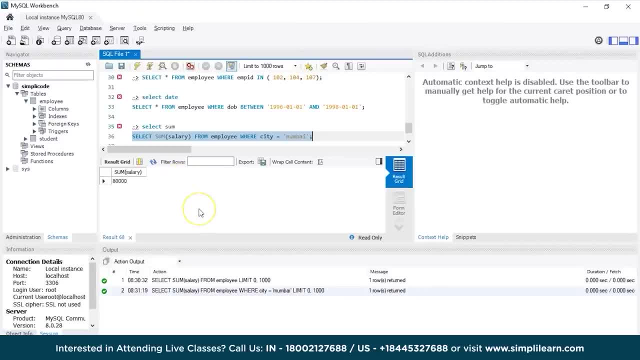 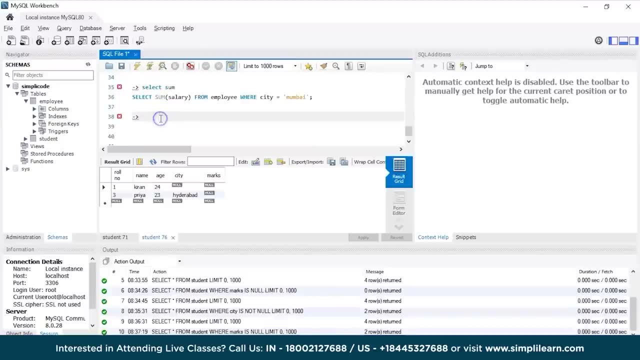 as 80,000. so in this way, you can use the some- select some statement in SQL to display the sum of values in a particular column. and finally, i let us now look at the select null statement in SQL. null in a table represents that the field has no value. 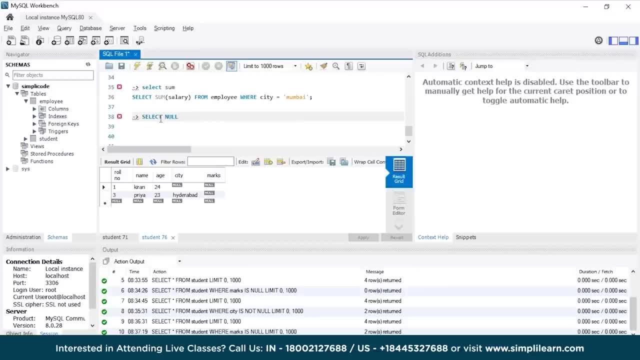 these Null values are used to represent the missing data in a particular table. Now, a null value is different from a zero value. That means a field with a null value is the one that has been left blank during the record creation. Now, to verify the column value is null or not, we can use the keyword isNull or isNotNull. 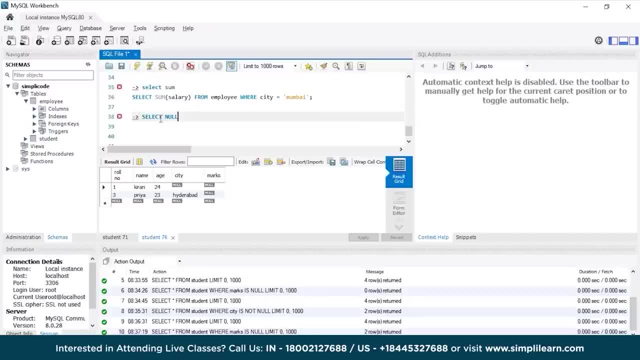 Now we should make a note here that null value can't compare with operators like equals to, greater than or less than. So let us take an example to understand the syntax. Now, if you want to fix the details of the students whose marks are null, that means: 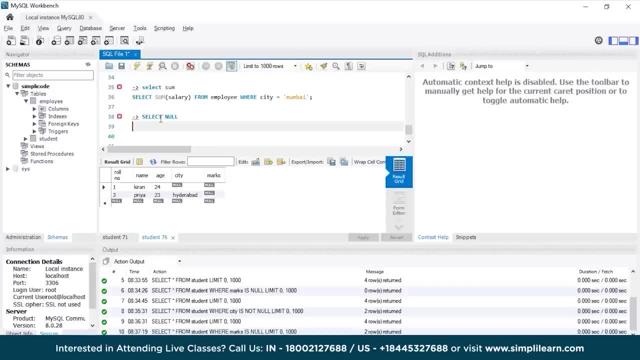 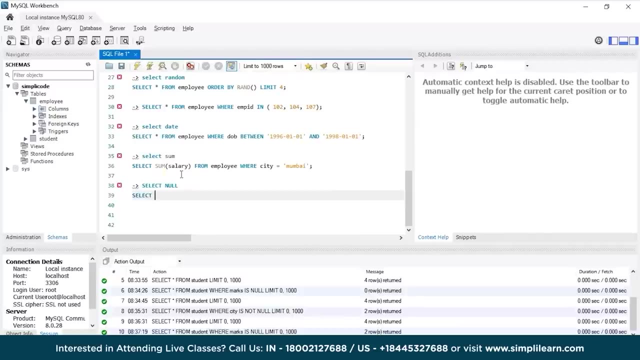 the marks that they have scored in the final exam are yet to be assigned to the students. So for that, the following query would be: Select, Select star From the table. that is student. where is the condition? marks is null, which is the keyword we are using. 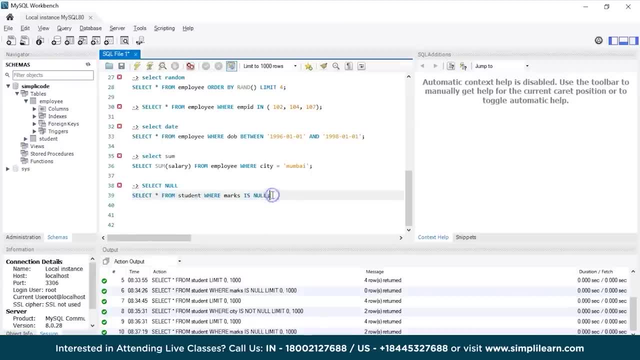 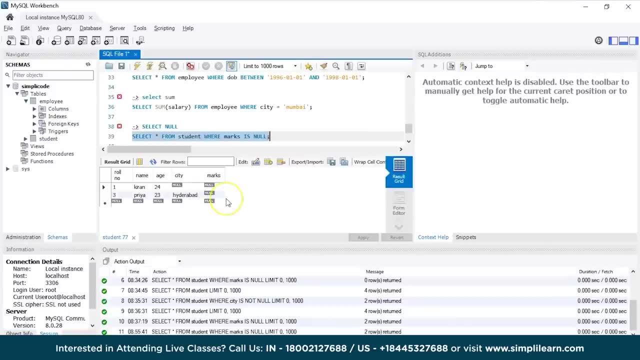 So let us execute this statement and see the output. So, as you can see, there are two students whose marks are yet to be updated, and it also means that their marks are not equals to zero. it's simply that their marks have been left out. 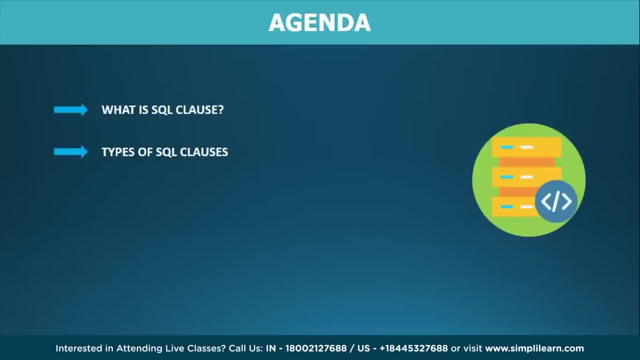 So the answer is null. Start the tutorial by understanding what SQL clause is. Next we'll go through different types of SQL clauses And finally we'll discuss about SQL where clause and execute MySQL Workbench. What is SQL clause? SQL clause are basically inbuilt SQL functions that use a certain conditional expression. 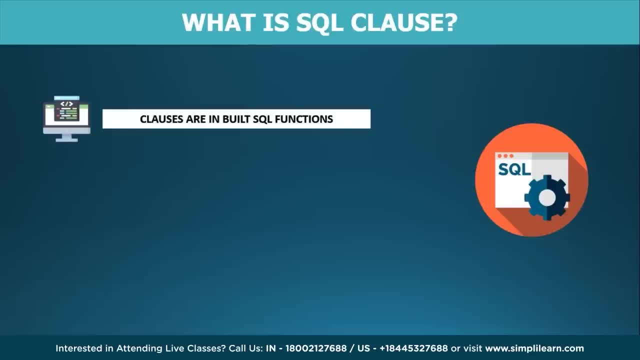 which helps to access a particular set of records from the database table. Clauses help us to restrict and manage the data, using valid constraints on the data in our database. Now, since we have large amounts of data stored in the database, we use clauses to query the. 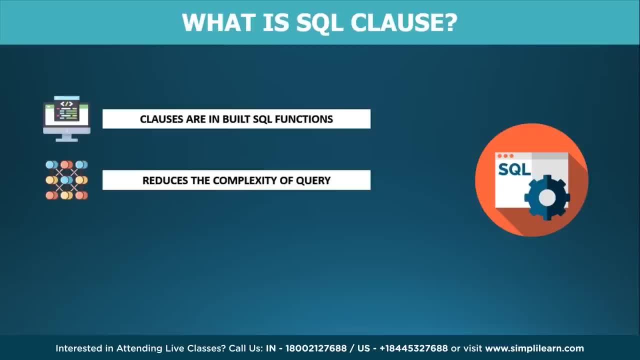 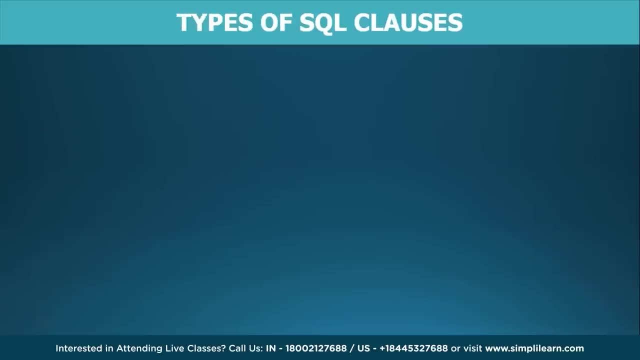 table to get the desired data only, So the complexity is reduced when a condition is applied to an SQL statement. SQL clauses use filters and analyzes the data quickly, because it is used to extract only those records that fulfill the specified condition. Types of SQL clauses. 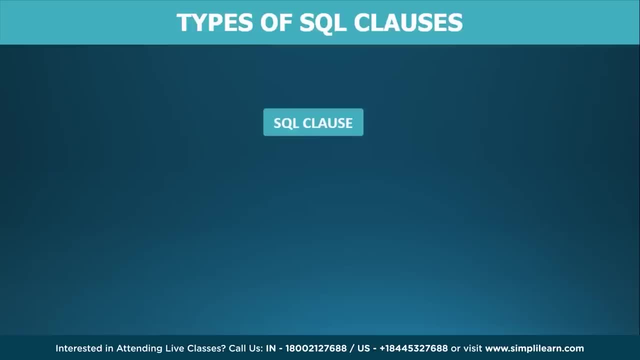 SQL clauses are divided into three types. The first one is the basic SQL clause. The second one is the standard SQL clause. The third one is the standard SQL clause. The fourth one is the basic SQL clause which uses a condition. The second one is the order by which is used to sort the data in tables, in either ascending. 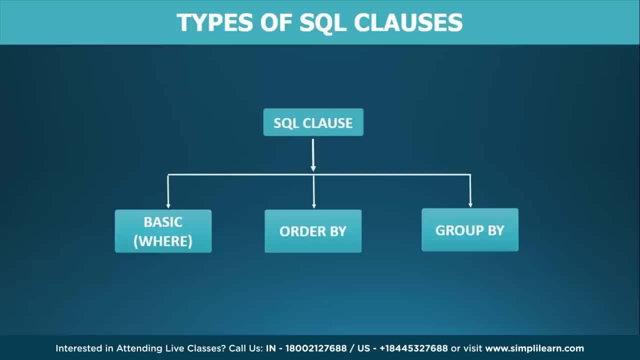 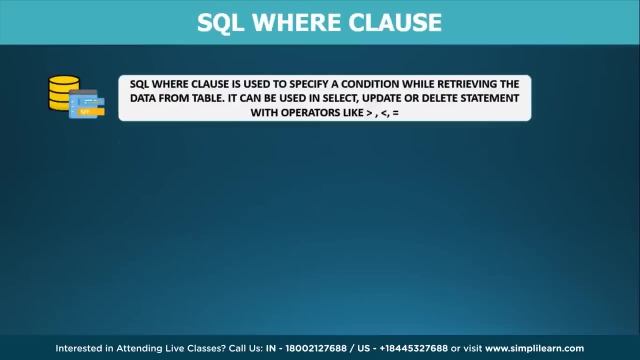 or descending order, And the last one is the group by which is used for organizing similar data into groups. SQL where clause. SQL where clause is the most used and integral part of any query- to specify a condition in the SQL statement which retrieves only those records which satisfy the given condition. 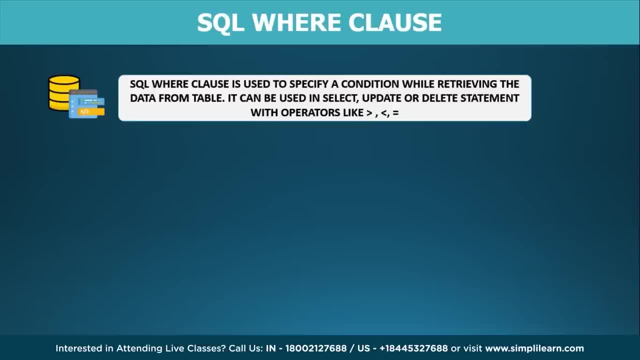 The where clause is not only used to sort the data in tables, but also to sort the data in the SQL statement. The where clause is used to sort the data in the SQL statement. The where clause is not only used in the SELECT statement, but it is also used in the UPDATE. 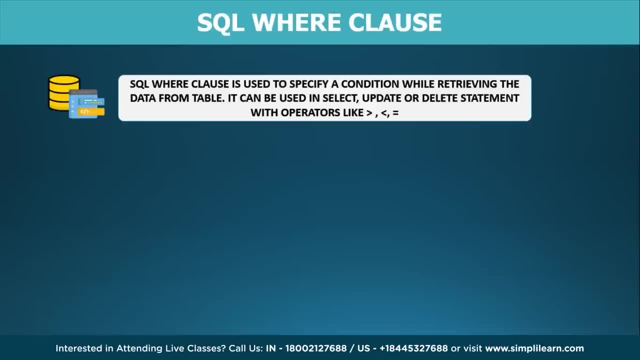 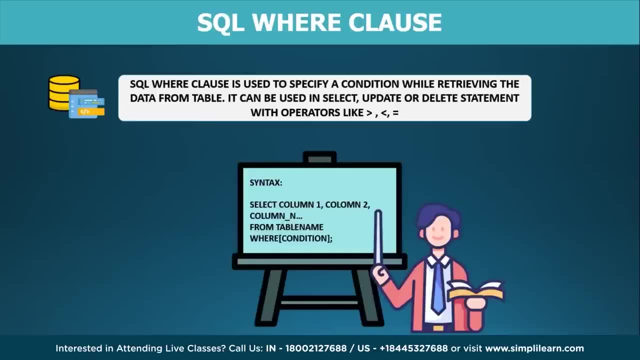 DELETE, statement, etc. using logical and comparison operators like greater than, less than and equal to operators. Let us now look at the syntax of where clause. The syntax is followed as: select column 1, column 2 and up to n number of columns from. 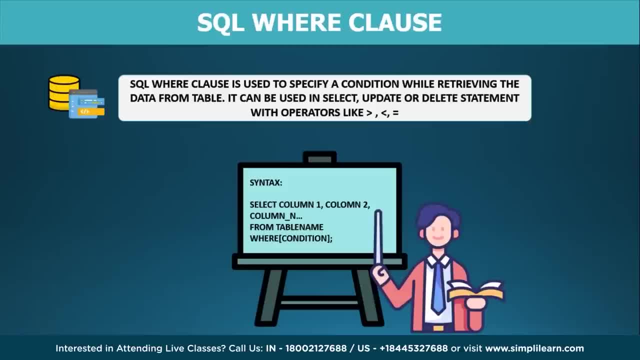 table name, where condition Here column 1 and column 2 represents the columns which we want to fetch the data from the table And the condition here represents the required condition And the condition here represents the required condition. This condition is used to fetch rows based on the requirement. 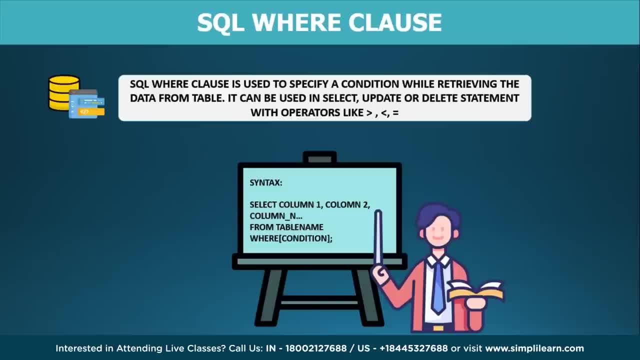 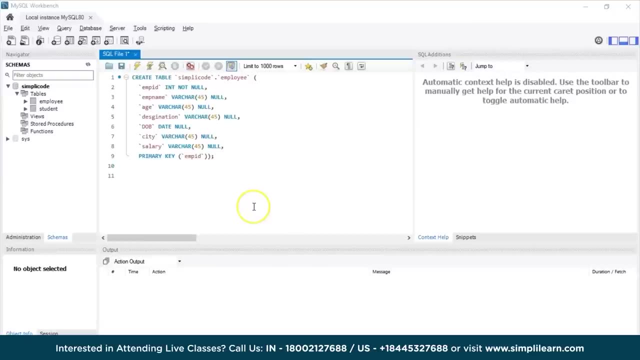 It contains column name, operator, user defined value, Comparison and logical operators are also used in this condition, So in this way we can use where clause. Let us now execute some statement which uses where clause in MySQL workbench. As you can see, the MySQL workbench has started and before we write queries using a where. 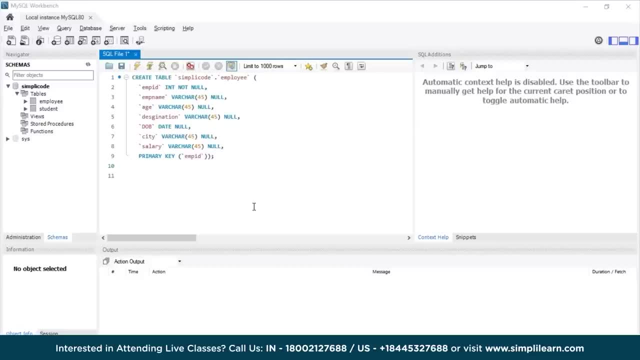 clause, we have to first create a table. so i have created a table here- employee- which has columns employee id, employee name, age, destination, date of birth, the city they belong to and their salary. and i've taken primary key here as employee id because it uniquely identifies each and every record in the table. now that we've created the 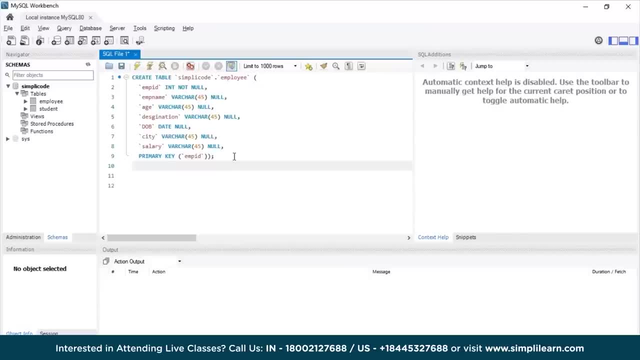 table. let us now look at the simple and basic query using the where clause. now, let's say, if i want to display the details of all those employees who belong to the city mumbai, so for that the following query would be: select star from the table that is employee. now we have to 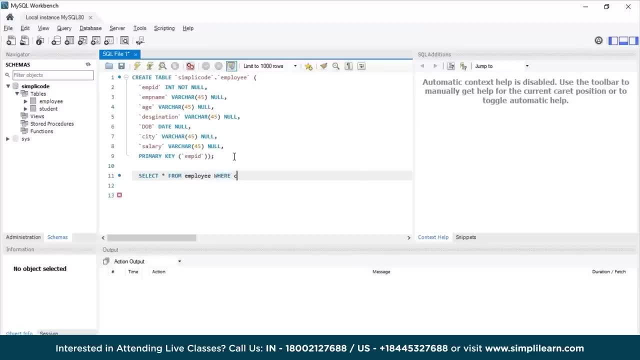 mention the condition, that is, the where clause, where city is equals to mumbai. mention mumbai in single quotes, otherwise it will show an error. so let us now execute the statement and see the output. now, when we execute the statement, it will show me the output of two employees who belong to. 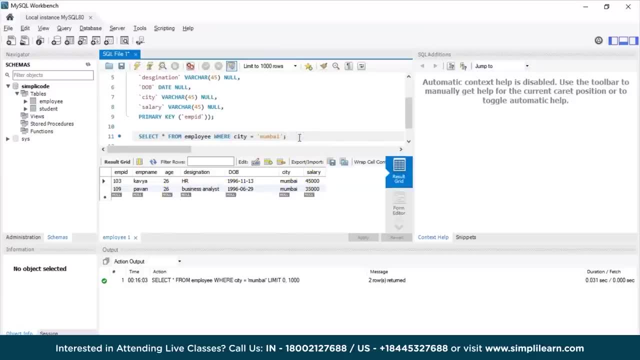 the city. so let us now take another example, a example. now we'll use the greater than operator, using the where clause. now, let's say, if i want to uh display the details of all those employees whose salary is greater than 30 000, so for that. 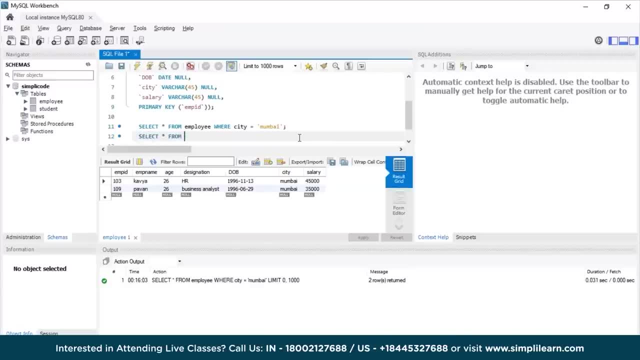 the following query would be: select star from table, that is, employee where salary is greater than 30 000. so let us execute the statement now. when we execute the statement, it will show me the records of all those employees who are in the city, who belong to the city, and this is the 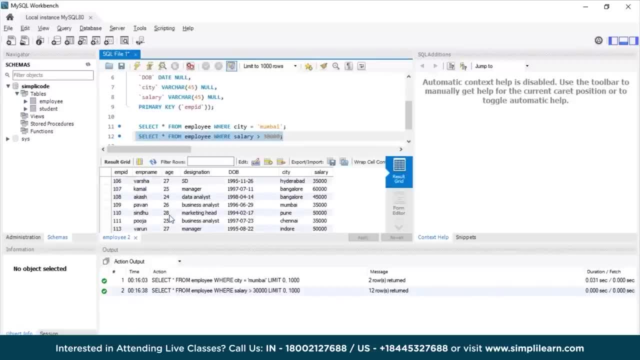 having salary more than 30,000. now I think here we have around 15. since we have 15 records in the table, we have a total of 8 employees whose salary is more than 30,000. so in this way you can use a greater than operator similarly. 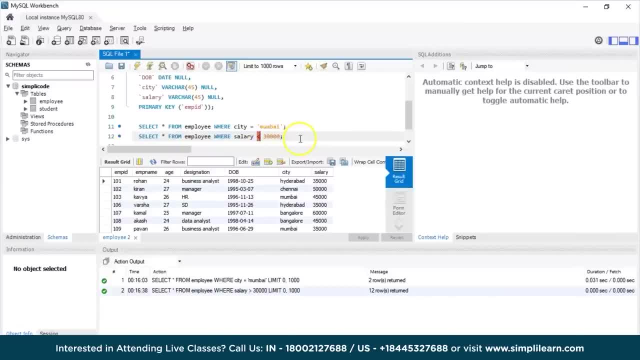 you can use the less than operator as well. and let us see the output. whose salary is less than 35,000 will take 35,000 here and now see the output. so there are total three employees who are having the salary less than 35,000. that 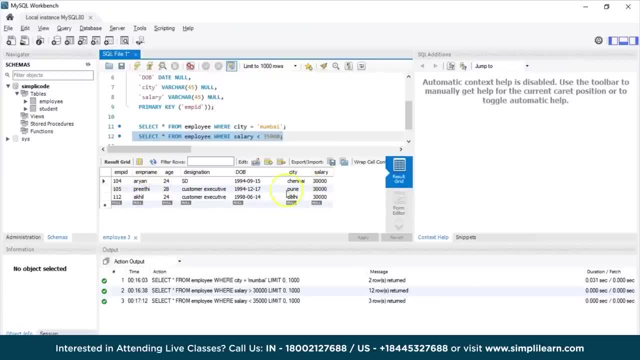 is Aryan Preeti Akhil, who are having salary as 30,000. so in this way you can use less than operator as well. now let us take another scenario. now, if I want to mention a range of salaries, of how much they earn, let's say if I want to. 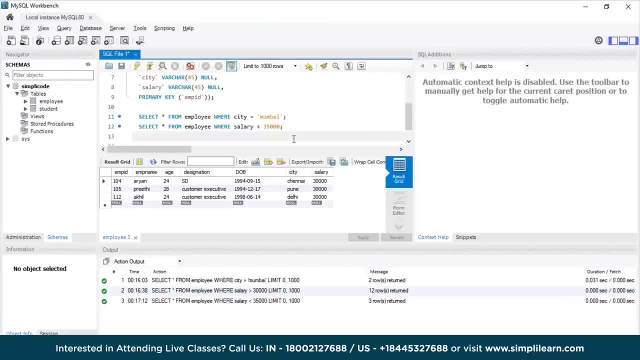 display the records of all those employees who are earning salary in between 35,000 and 50,000. so for that, the following query would be: select the star from the table that is employee, where salary between is the keyword we have to use here: 35,000 and 50,000. let us now execute this statement and see the 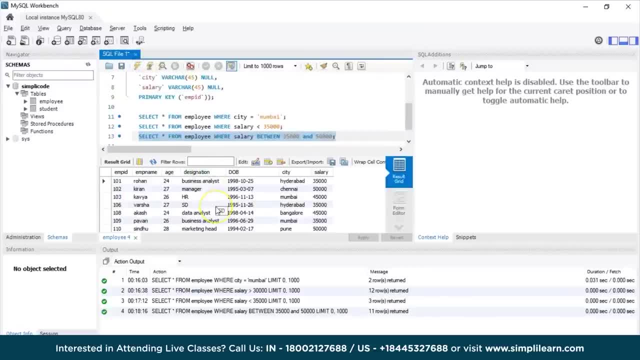 output. so now these are all the records of the employees who are having salary in between 35,000 and 15,000. so in this way you can use various comparison operators to perform queries using where clause. similarly, you can also update the values in the table as well using the update command. let's say if you want to update. 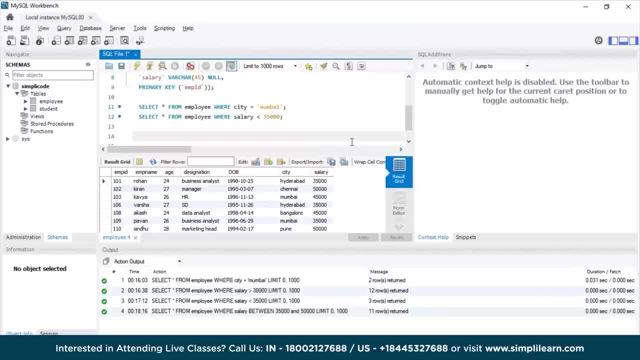 the salary of employee whose employee ID is 104. so for that, the following query would be: update salary of employee whose employee ID is 104. so for that, the following query would be: update table name. that is, employee set is the keyword we have to use here. salary now. 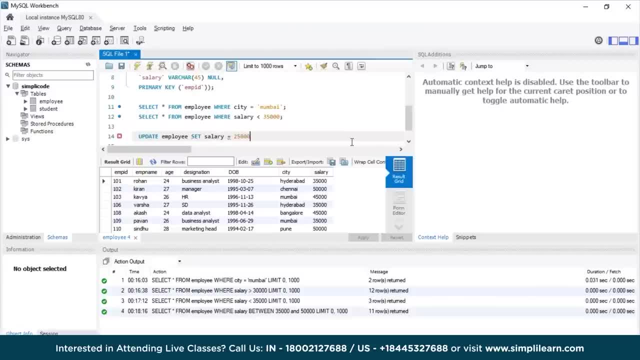 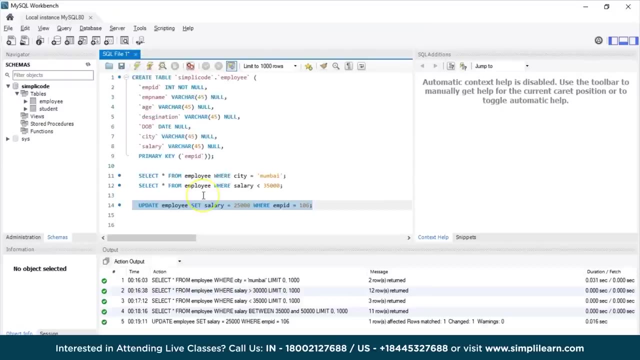 I want to change the salary as 25,000, so I am choosing 25,000. specify the condition where employee ID is equals to 106. so let us execute this statement and see the output, so as you can see our query successfully implemented and the employee who ID 106 who's having salary. 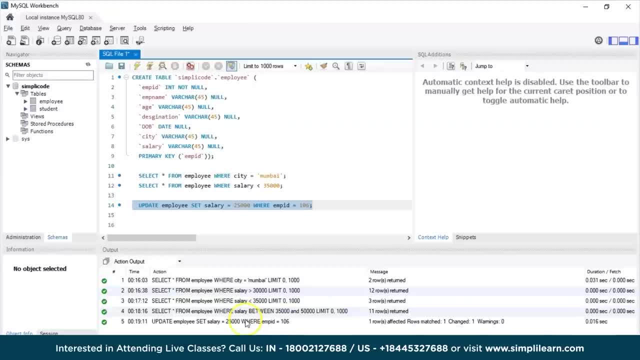 like before, he used to have some salary. now his salary is changed into 25,000, so let us see whether it is changed or not. we'll use the select command again to display the details of all the employees, so for that the query would be select star from the table that is employed. let us now execute the 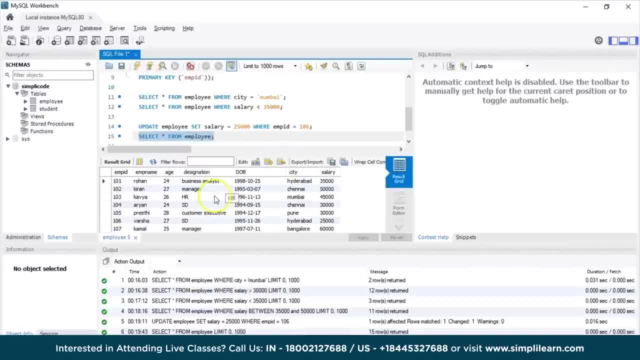 statement. so one, not six, employee name is Varsha, who is working as a software developer, and salary has been changed to 25,000. so in this way, you can use, where class, to perform various operations, using certain conditions. if getting your learning started is half the battle, what if you could do that for free? 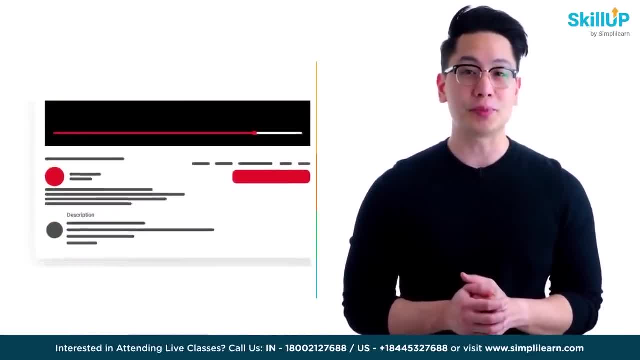 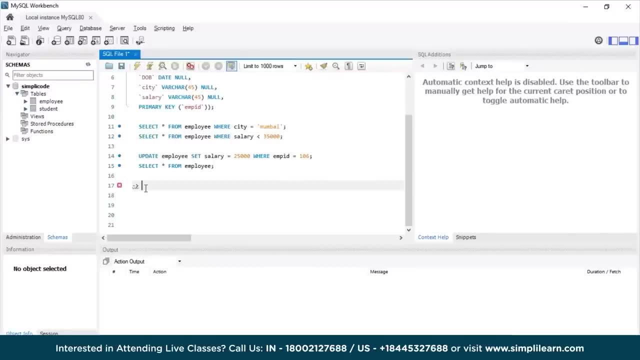 visit. scale up by simply learn. click on the link in the description to know more. now that we have understood how to to write a query using the where condition, let us now look at some other conditional statements which uses where clause. First, let us discuss about SQL and condition. SQL and condition is: 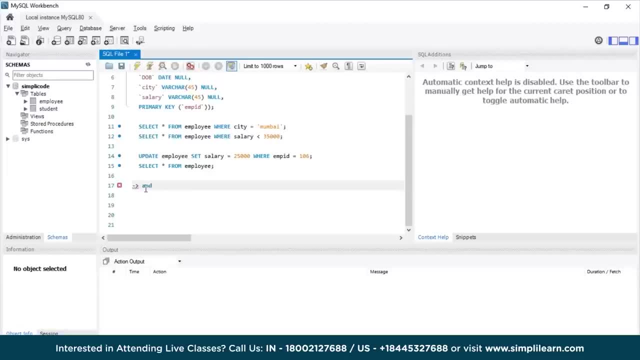 used to specify multiple condition in where clause and condition basically returns the rows or those values. that satisfies both the conditions that are written after the where clause. In simple terms, we can say that it will only return those values when both the conditions are met. Let us now 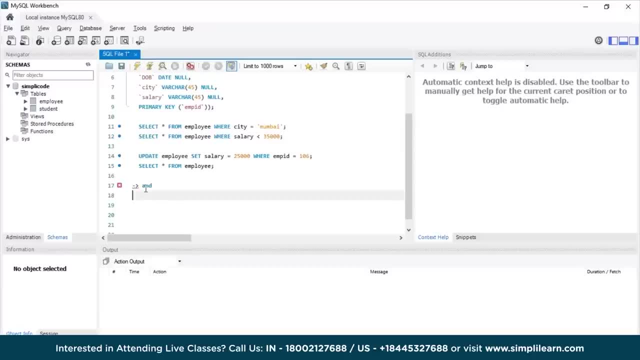 understand this with an example. Let us say if I want to access the records of all those employees whose designation is business analyst and their salary is 35,000.. For that, the following query would be: select star from the table that is employee where I am specifying the condition here. 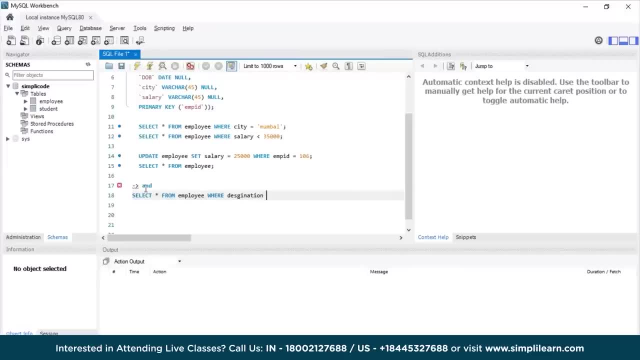 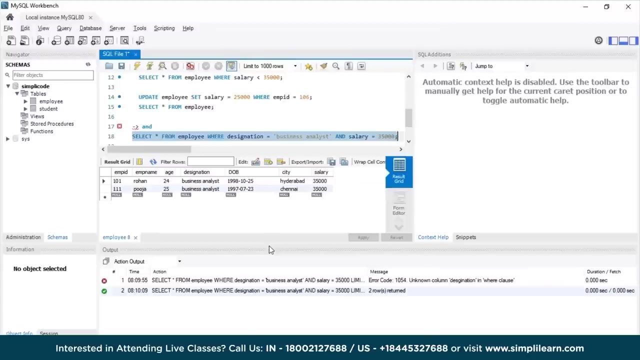 designation is equals to business analyst and is the keyword that we have to specify here. Salary is equals to 35,000 and let us execute the statement now. So, as you can see, it is displaying the records of two employees whose designation is business analyst and their salary is 35,000.. But if you look at the employee table cap, 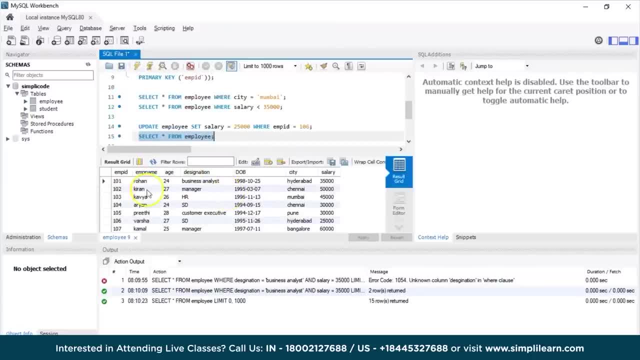 let me just display the values. There is the employee ID 101, who belongs to the designation business analyst, and similarly we have another employee whose employee ID is 109 and whose employee ID is 111.. Here we have three records, but instead it is displaying only two records. 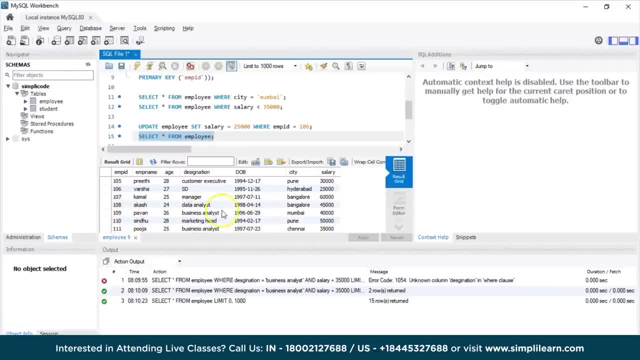 That's because there's an employee ID 109 who belongs to the designation business analyst, but his employee ID is 40,000.. So in this case he is not meeting the other condition. That is why it is being displayed only two values. So in this way you can use AND statement to filter the records from the table. 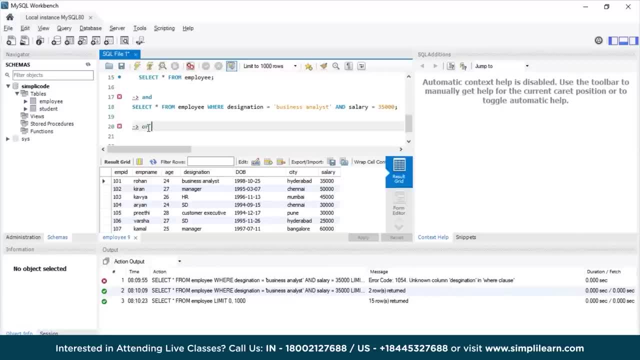 Let us now look at the next statement, that is, OR SQL, OR condition is used to specify again the same multiple conditions in WHERE clause, which is used to fetch the rows or values which satisfy any of the condition. Now, unlike the AND statement, if any of the condition that is provided is true, then it will return all those. 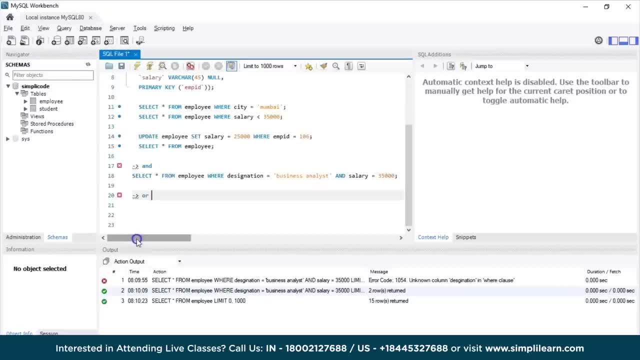 values. So let me just execute this with an example. Let's say, if I want to access the records of all those employees whose designation is manager and the city that they belong to is Chennai, So for that I'll write the query as SELECT star from the table that is employee WHERE. 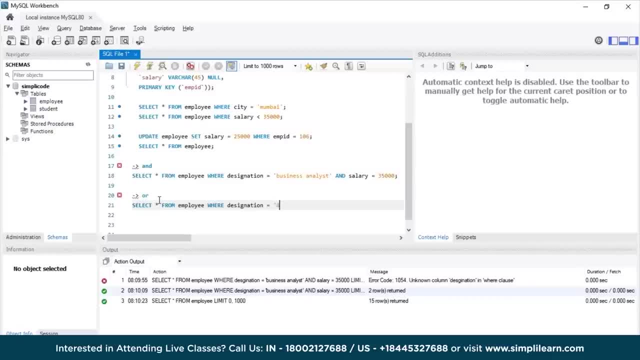 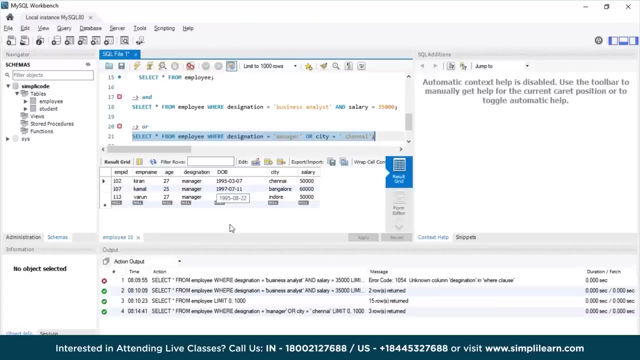 designation is equals to manager or the city that they belong to is Chennai. So let me just execute this statement and see the output. So when execute this statement, it will show a total of three records of all those employees whose designation is either manager or the city that they belong to is Chennai. Now we have 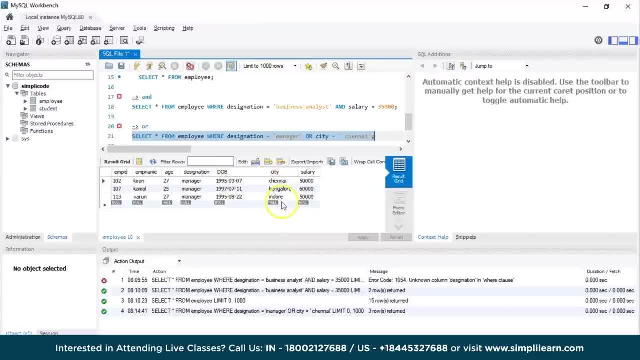 the records of employee who belongs to city Bangalore, Indore as well, but it is showing here because the designation is manager. that is here. it is satisfying either one of the condition, that is, either the designation that is manager or the city that they belong to is Chennai. So in this way you can use 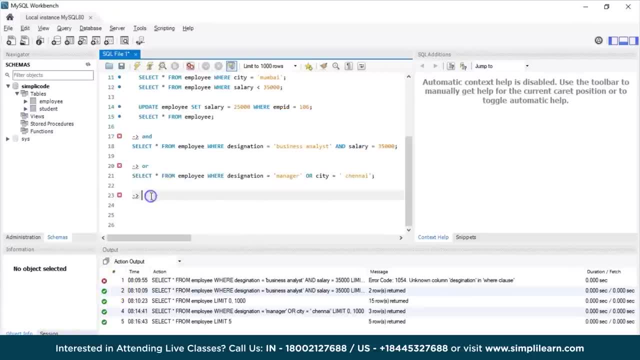 OR statement to filter the records. Next, let us discuss about the limit condition. in SQL, The limit condition is used to fetch those records that have only limited number of values. let say, if i want to access the records of first five employees from the table, then I'll write the Lonline query. 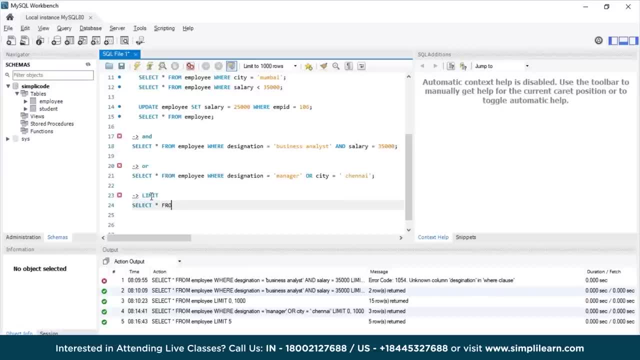 as SELECT star FROM TABLE. that is employee. Now you have mention the keyword limit. I want to access the records of first 5 employees, so i am specifying five as the condition here. let me execute this statement so it will display the first 5 records of the employees from employee limit. 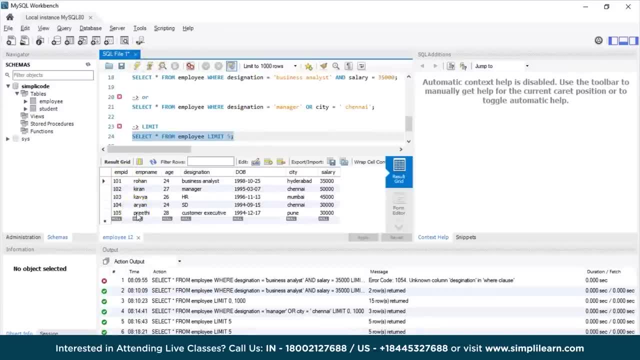 THE END, so it will display the first five records of the employees from the employee as solution. So i will write ver info: VлWOR main employee table. now this limit condition is used, like when you have thousands of records in a table, and if you want to access the first 100 records of the employees, then you can use the limit. 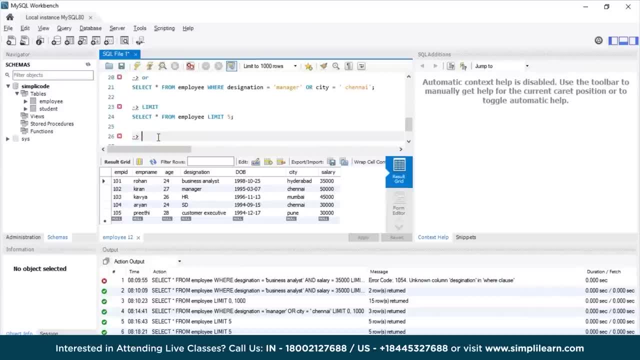 condition here with the example. next let us discuss about sql as condition statement. now sql as condition is used to rename a column temporarily in a given table. now in simple words, we can say that sql as keyword is used to give an alias name to the table or column name in the query. 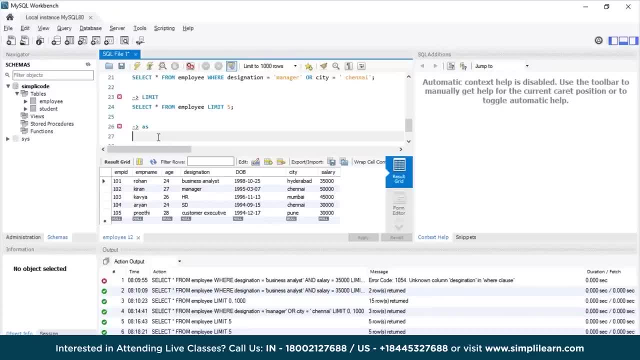 and in this way we can increase the readability and understandability of the query and call and also the column headings in the table. so let us understand with an example. let's say, if i want to change the column name of salary to the total salary, then i would write the following query as: 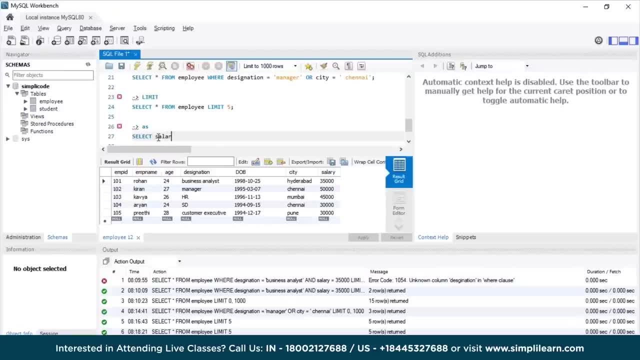 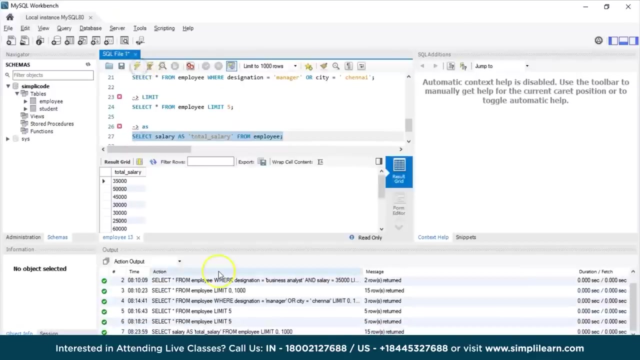 select salary as, within the single quotes, mention the new column name, that is, total salary, from the table that is employed. so let us execute this statement and see the output. so, as you can see, salary has been changed into a total salary in this way you can use. 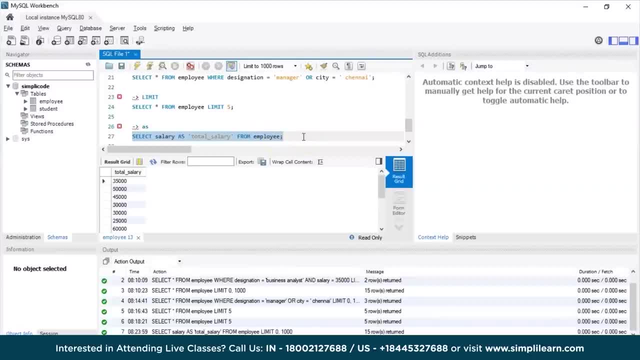 the and condition statement to change the column of the table temporarily. and finally, let's us discuss the like statement in sql. the like condition statement is used to fetch matching rows or values from the table that satisfies the wildcard operator. now, the wildcard operator in sql, uh, basically have two types. the first one is percentage sign. the percentage sign represents 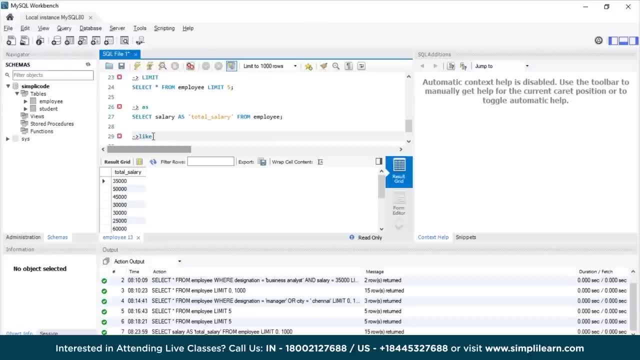 a single or multiple character, and the second one is underscore. underscore represents a single number or character. now you might be a bit confused here, so let me just explain with an example. let's say, if you want to access the records of all those employees whose name starts with k, 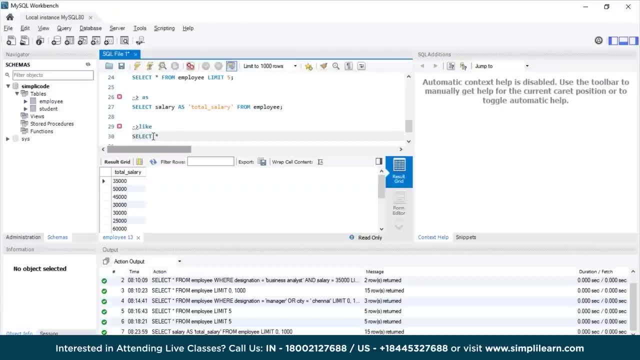 so for that i will write the query as select star from the table. that is employee. now specify the condition where employee name like, is the keyword we have to use here and within the single quotes. now we are displaying the records of employees whose name starts with k. right, so i am taking k. 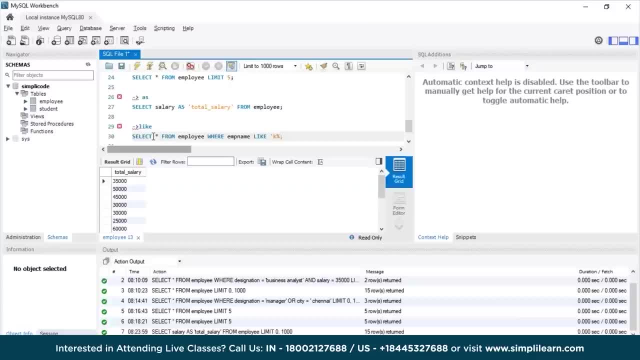 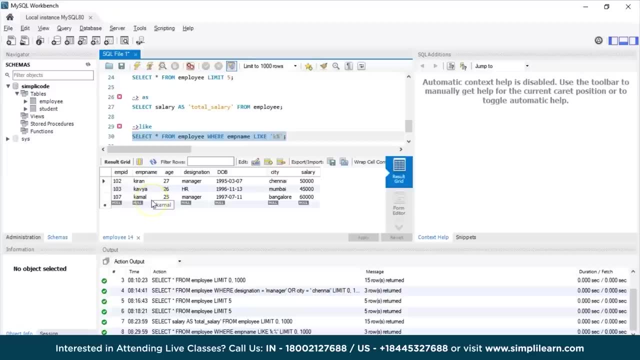 and mention the percentage symbol. so let us execute this statement and see the output. so it will display the details of all those employees whose name starts with k. so there are total uh three employees in the table whose name starts with k here. similarly, if you want to display the records of those employees whose 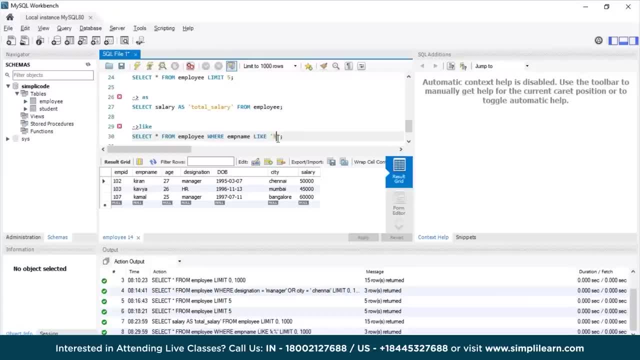 name ends with a, so for that we have to mention percentage a. so let me just execute this statement and see the output, so it will display the values of all those employees whose name is ending with the letter a. so there are total uh five employees in the table whose name is ending with a, so in 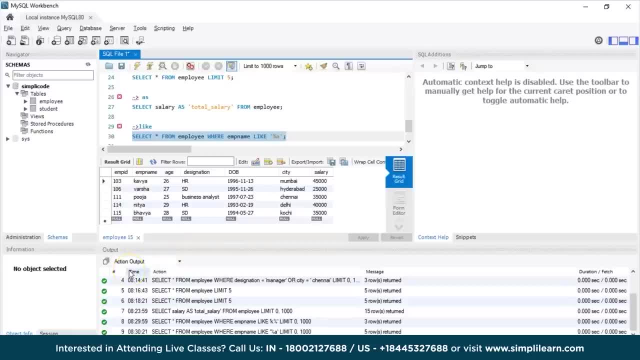 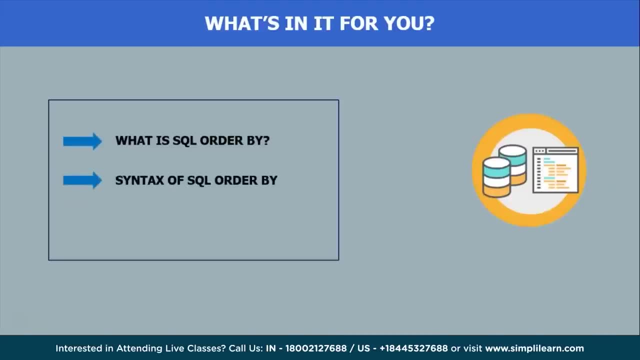 this way you can use the like operator, which also uses the where clause. we'll start the tutorial by understanding what is sql order by, and then we'll discuss the syntax of sql order by, and finally we look at some order by statements and execute them in the next video. so thank you for watching this video. 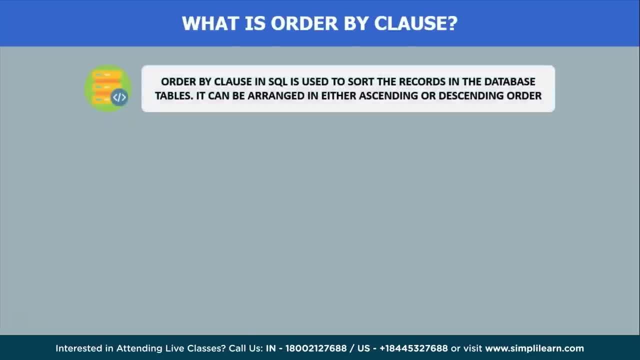 in mysql workbench. so what is order by clause? the sql order by clause allows you to sort the results of a query based on a specific column or group of columns. that means it helps you to reorder the data that is present in the tables in one or more columns. now this sorting can be either ascending. 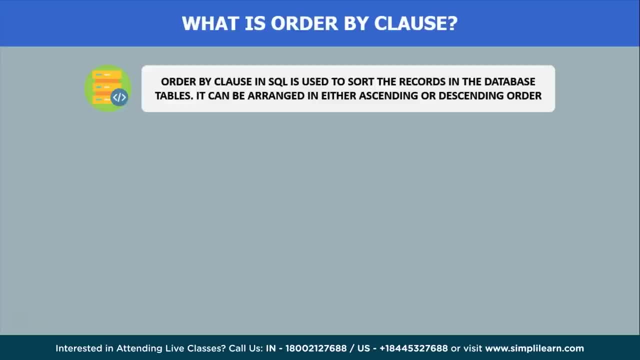 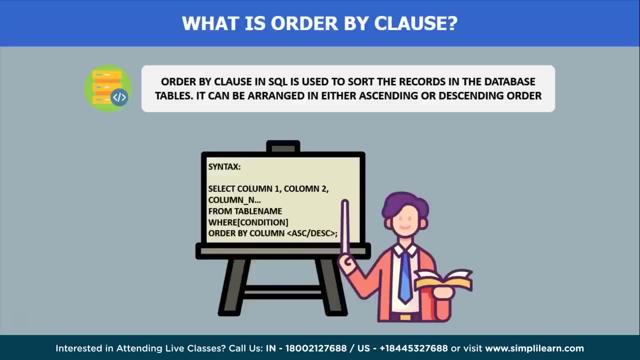 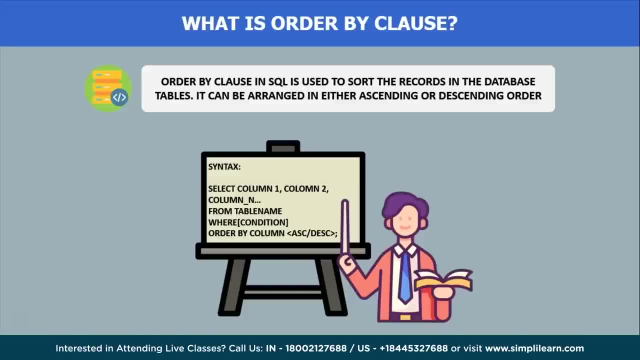 ordered by column asc or dsc. so let me just explain the syntax. the column specified after the order by keyword specifies the name of the columns that are used to sort data, and after that we use two keywords. that is asc, to represent the data in ascending manner, or 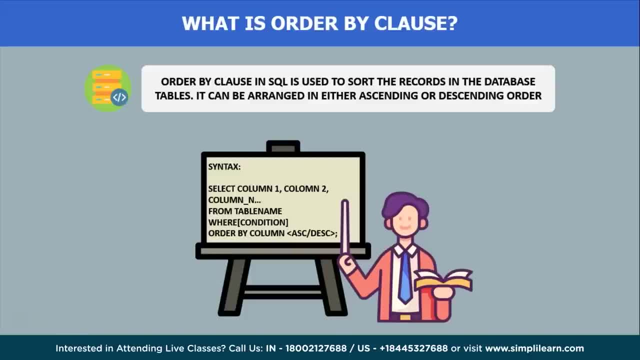 representing the data in descending order. now, the reason for using the order by clause is that the order that the data shows in a database table is completely random, and sometimes this might not be the order in which you would like to see when we run our queries in the database. so for that. 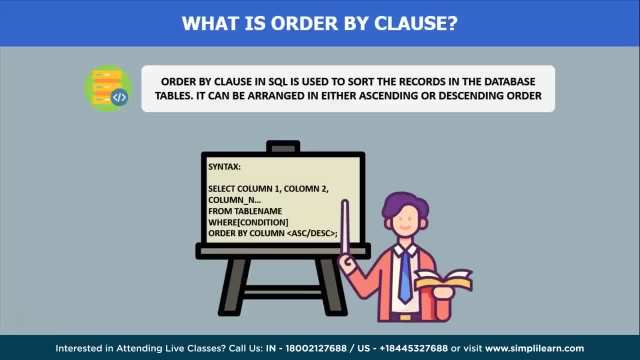 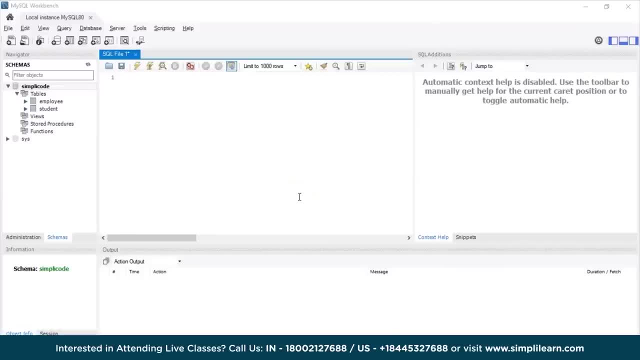 purpose we use order by clause. now that we've understood what the sql order by clause is, let us jump into the execution part. as you can see, mysql workbench has started and on the left side database, simply code which has two tables, that is, employee and student. we are going to work on the 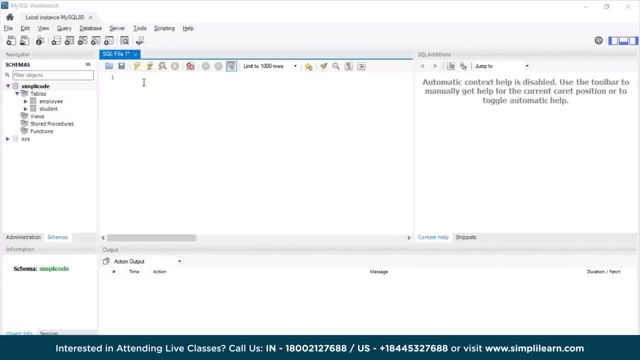 employee table now. so first let me display the records of all the employee details present in the employee table. for that i am going to use this select statement: select star from the table name, that is employee. let me just execute this statement so it will show me the results of. 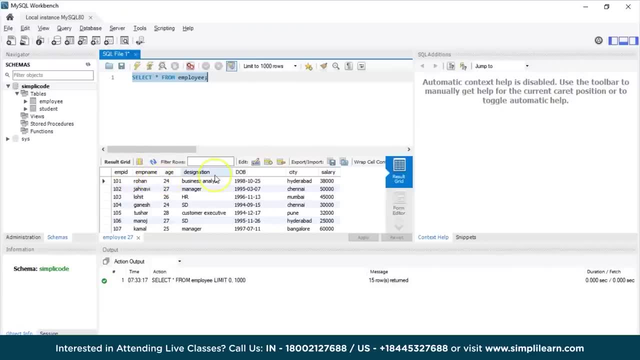 details of all the employees, with their employee id, employee name, age, destination, date of birth, city they belong to and the salary they have. so let us just understand the basic query of order by clause now. so the syntax is followed as select star from the table. that is employee order by salary. 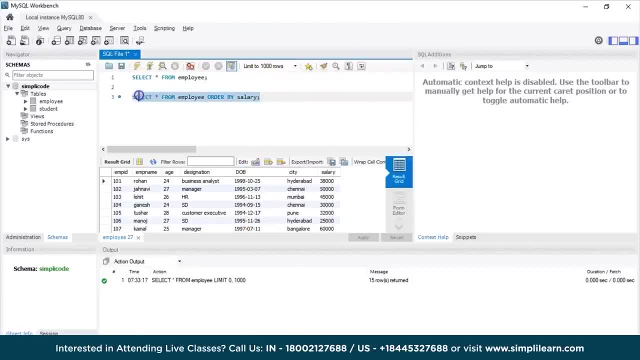 now, this is a basic statement related to order by and. let us execute this so it will display the output and in a particular order of the salary, and, if you look at carefully, it is displaying in the ascending order. now, if no keyword is specified after the column based on: 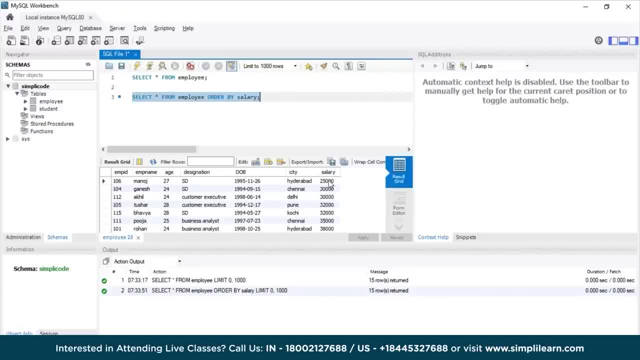 which we have sorted the records in a table. the sorting will be done by default in ascending order. so with that, uh, that brings us to the to our first order by statement, that is, order by ascending statement. now, the order by ascending statement is used to sort the data. 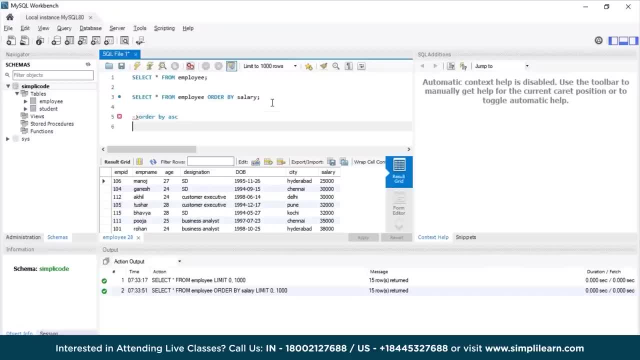 in ascending order. So let us consider another example here. Now, if we want to fetch the details of all the employees and their employee names in ascending order, for that the following query would be: select star from the table that is employee order by employee name and mention the keyword ASC. So let us 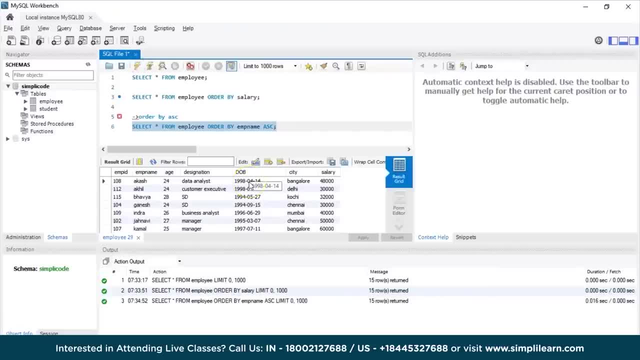 execute this statement and see the output. So it will display the results, the employee names, in the ascending order, that is, in alphabetical order, starting from Akash, Akhil, Bhavya, Ganesh and up until V. So in this way, you can. 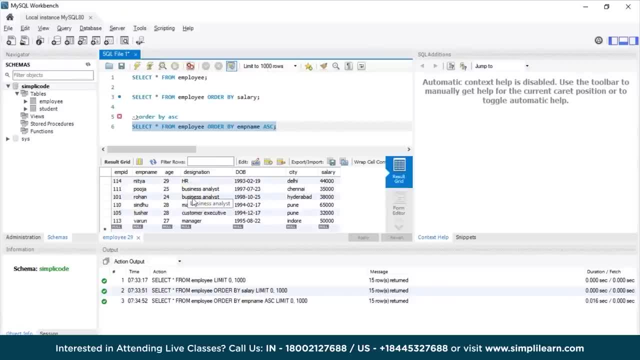 use the order by ascending statement to display all your records in ascending manner. Similarly, you can specify the where condition here as well. Let's say, if I want to fetch the details of all the employees from the employee table in ascending order of their employee name whose age is greater. 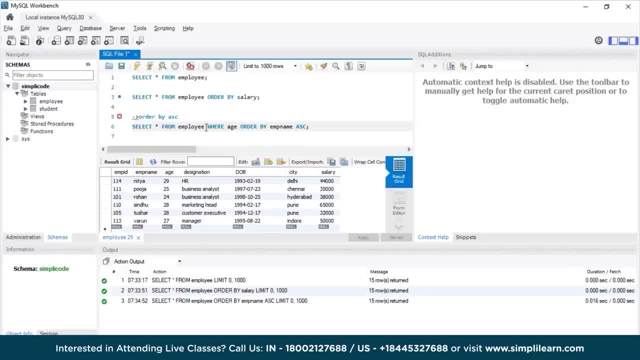 than 26.. So for that, the following query would be: select star from employee where age greater than 26. order by employee name: ASC. So let me execute this statement So it will display the records, all those employees whose age is more than 26, and it will sort that. 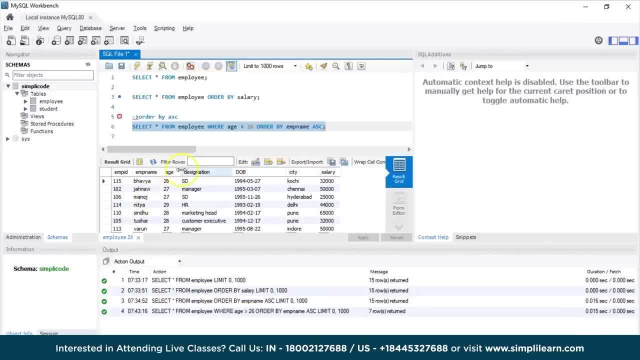 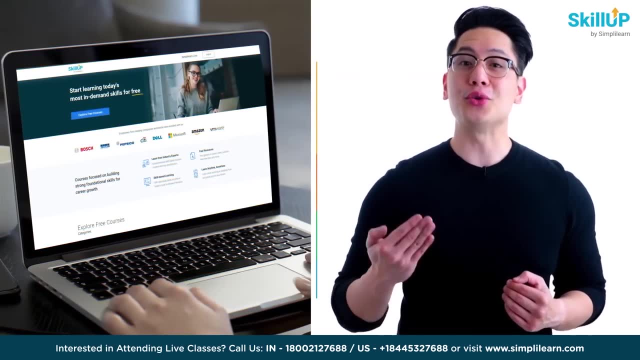 this data of employee names in ascending order. so in this way you can use the order by ascending. if getting your learning started is half the battle, what if you could do that for free? visit scale up by simply learn. click on the link in the description to know more. 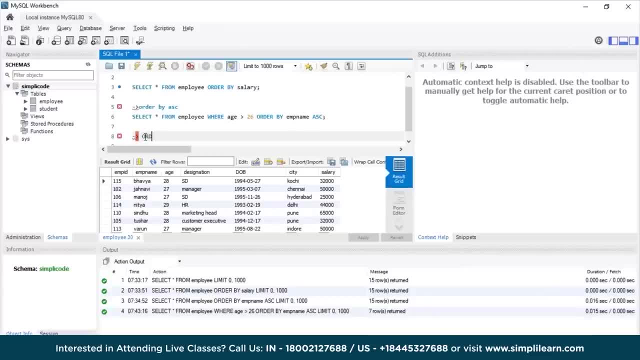 now let us discuss about order by descending statement. the order by descending statement is used to sort the data in the descending order. let us understand this with an example. let's say, if i want to display the details of all the employees from the employee table in descending order of their salaries, for that, the following query would be: select star. 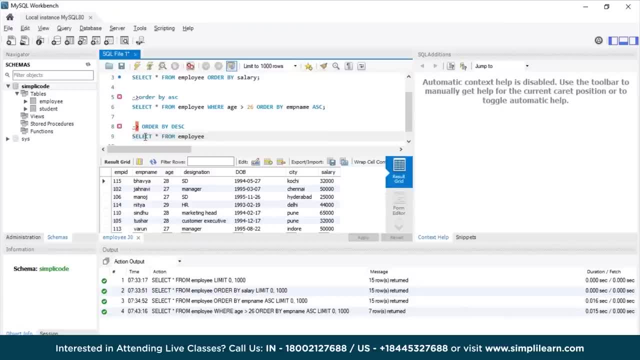 from the table, that is, employee order by salary, and mention the keyword des. so let us execute this statement and see the outcome. so this will be the following output, wherein it will show the salaries of all the employees in the descending order, that is, from highest to lowest, in this case, the first employee. 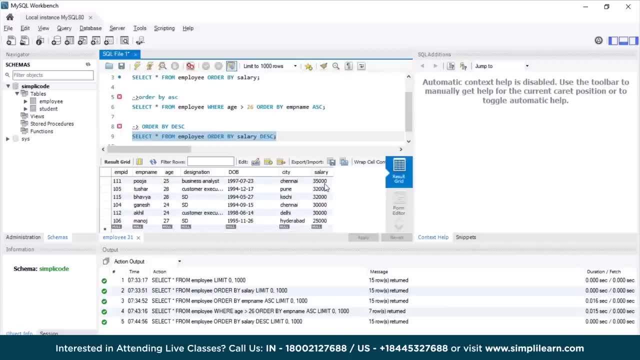 who is having the highest salary is 65000 and up until the lowest salary 25000. also, similarly, you can specify the where condition here also. so if you want to display the details of employees whose employee id is greater than, let's say, 106 and want to sort their salaries in descending order, for that i'll use the query as select. 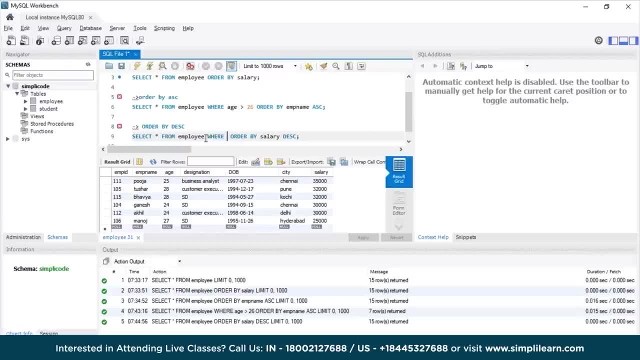 star from employee mention the keyword where employee id greater than 106. so let us execute this statement and see the output. so it will display the records of all those employees who's having employee id more than 106 and it will sort the data of their salaries in. 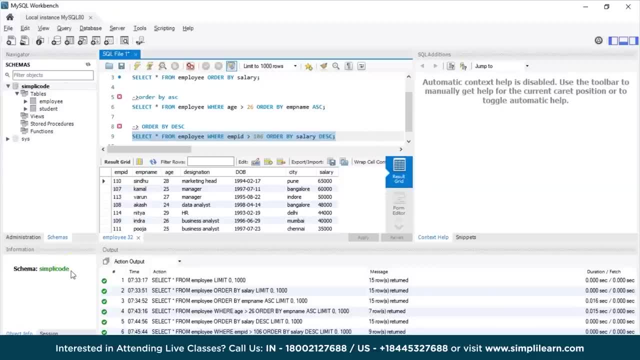 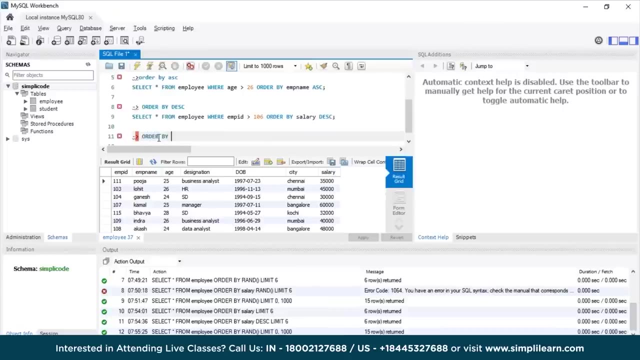 descending order from highest to lowest again. so in this way you can use the order by descending statement to display all the records present in the table in an ascending manner. let us now discuss the next order by statement, that is, sql order by random and as well as. 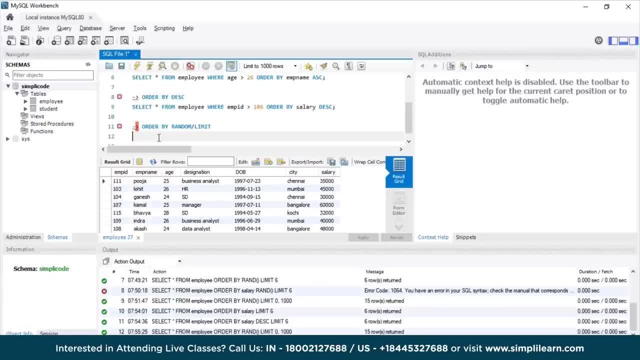 limit statements. the order by random statement is used to display the records present in the table randomly and the syntax for the order by random is select star from the table. that is, employee order by mention. the keyword random is the function we are using here. so we have to mention r a n d and let us execute the statement now. 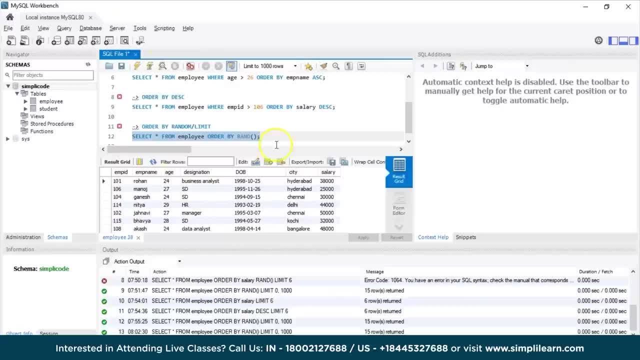 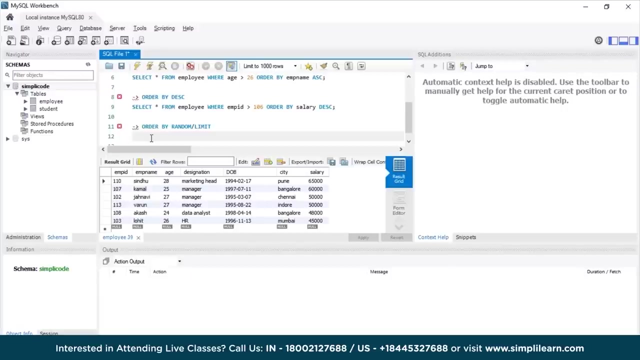 so it will display the records present in the table in an in a random order. similarly, we also have a limit statement, which is used to display only a specific number of columns in the database table. so let us now look at the syntax of order by limit. now, let's say, if we want to fix the first six employee details from the table in descending 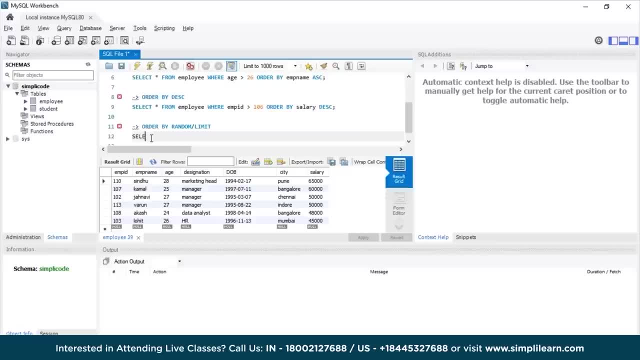 order of their salaries. so the following query would be: select star from employee order by limit value, bar, and this order by limit statement will be: select star from employee order by limit and then, if we want to, by salary. I want to display the salaries and descending order, so I'm specifying. 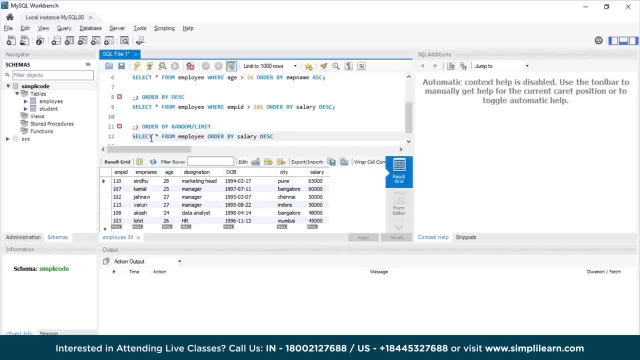 the DESC keyword and I'm limit. I'm using the limit function here, so let us display the output of this query. so it will show me the random six details of the employees in order of their salaries from highest to lowest, that is, in a descending order. so in this way you can also use order by random and limit. 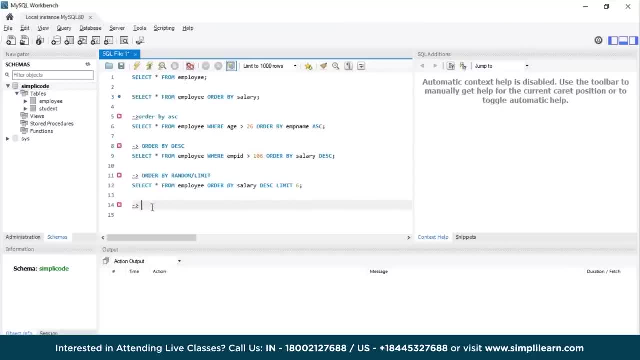 statement in your SQL queries. and finally, let us now discuss about the order by multiple statement in SQL. till now, we have discussed only how to fetch the records from only a single table and sort them out, but you can fetch the rows by sorting multiple rows in either ascending or descending order, using 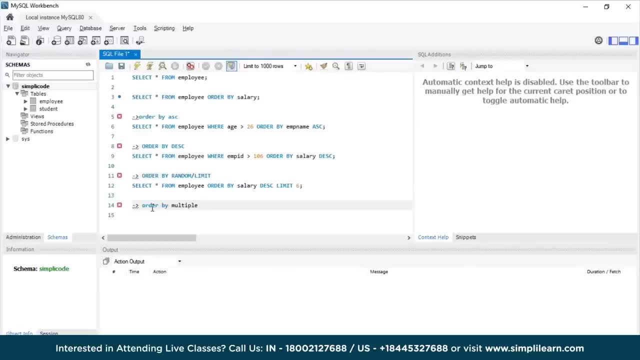 order by multiple statement. so let us understand this one. okay, so let us start with the order by multiple statement, and then we can also example. let's say, if you want to fetch the details of all the employees from the table in ascending order of the designation as well as descending order, 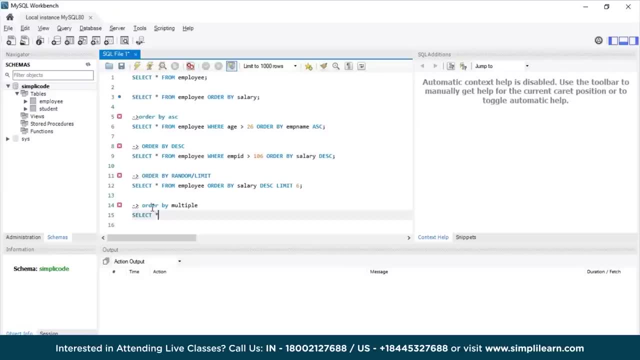 of their salary. then the following query would be: select star from employee order by: so we're taking the designation as ascending order, so designation, and then we can also mention the keyword ASC comma and their salary in descending manner. so let us display the statement so, as you can see, it will display the 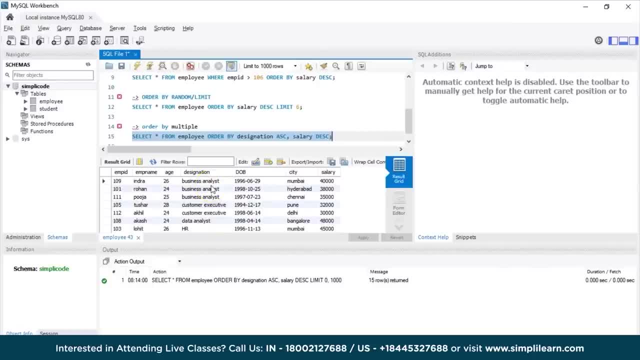 designation in ascending order, that is, business analyst and then customer care, data analyst, HR and so on, and their respective salaries in descending order form. so in this way, you can fetch the data from multiple rows using the multiple statement in SQL. lastly, we'll start the tutorial by understanding what 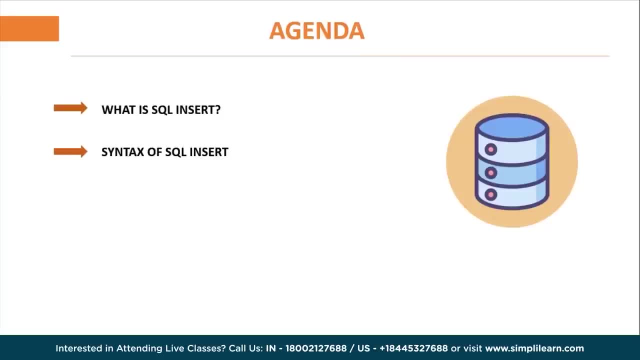 is SQL insert, and then we'll understand the syntax of SQL insert statement and finally we'll go through some of the SQL insert statements and execute them in MySQL workbench. so what is SQL insert statement? SQL insert statement is wide, widely used command in SQL which is a part of data manipulation language DML. 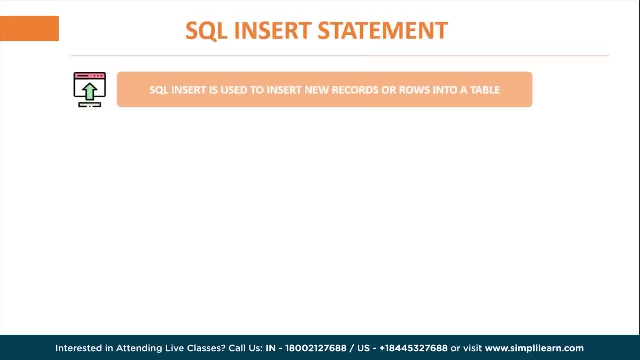 used by various relational databases. the insert command is used for inserting one or more rows into a database table with specified table column values. let us now understand the syntax for insert statement. now we have two types of syntaxes. the first method is insert into table name values. 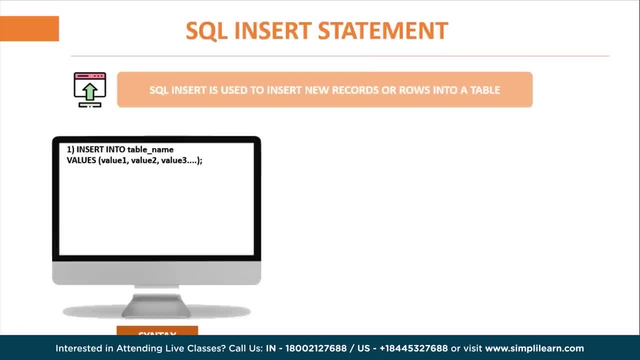 And within the brackets, you have to mention the values. In this first method, there is no need to specify the column names where the data will be inserted. You need to only insert their values. The second method specifies both the column name and the values which you want to insert. 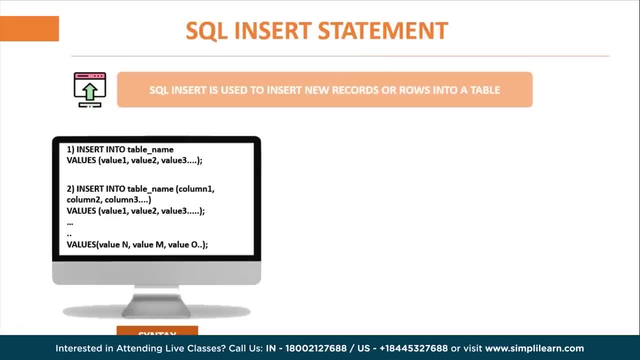 And the syntax is insertInto, which is the keyword we are using. After that, we have to mention the table name and within the brackets, we have to mention the columns, and then values: Values1,, values2,, values3 and so on, up to our requirement. 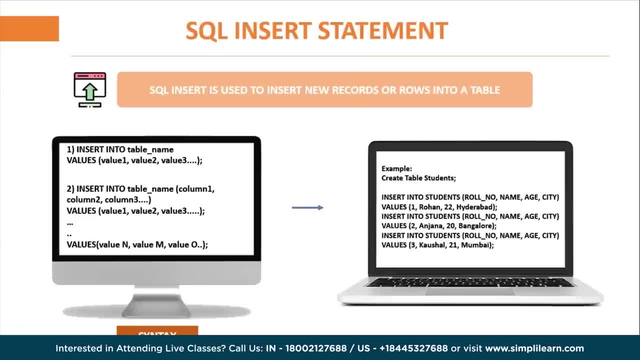 So this was the syntax. Let us take an example Now. let's say I've created a table, students, and I want to insert values into it. So the syntax for inserting the values is insertInto tableName. I'm taking here it as students and I'm mentioning the columns: roleNumber, name, age, city. 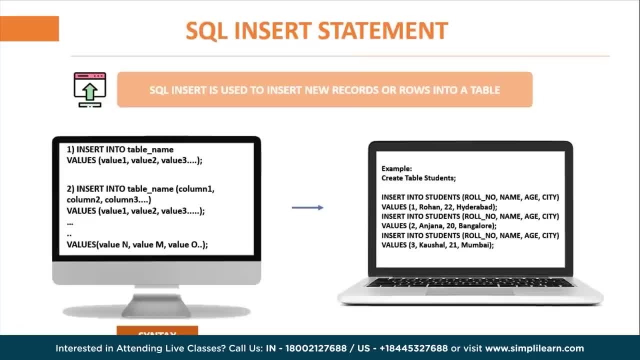 And I'm inserting the values as roleNumber, roleNumber as 1, name as Rohan, age as 22 and city as Hyderabad. So in this way you can insert values up to n number of rows into your table. So now that we've understood and got an idea of what SQL insert statement is. 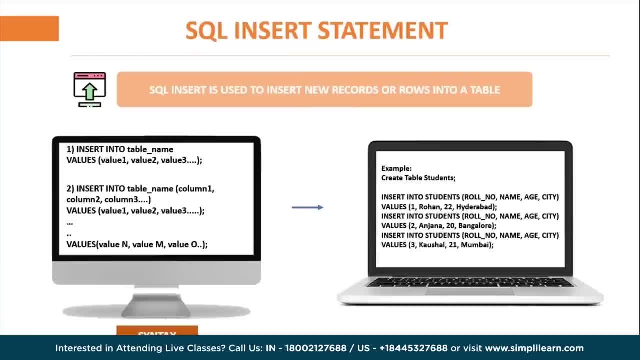 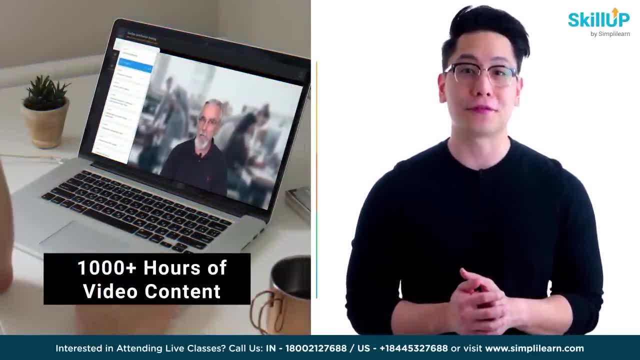 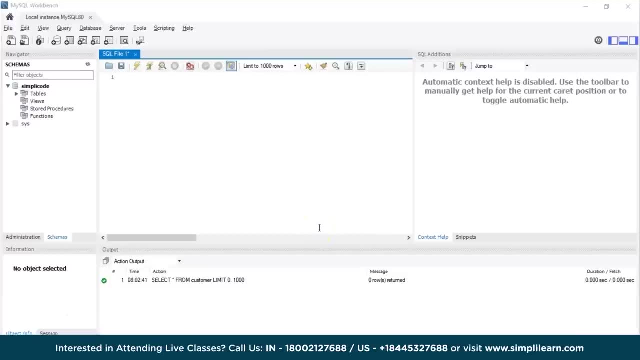 let us jump into MySQL Workbench and do the execution part. Click on the link in the description to know more. As you can see, MySQL Workbench has started and in order to insert the values into the table, we have to first create a table. 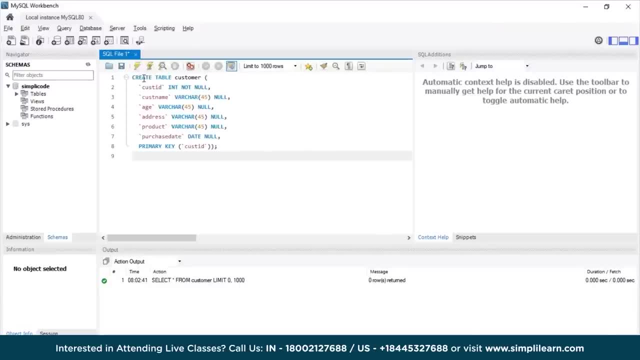 So let us first create a table, and the syntax is followed as createTable, which is the keyword that we use, And I'm creating a new table that is customer and which has column names as customerId, customerName, their age, address, the product they have purchased and the purchase date of the product. 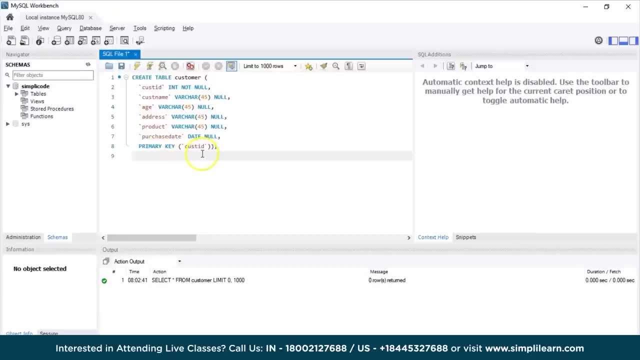 And I'm taking primary key here as customerId, because it uniquely identifies each and every record. So let me just use the SELECT statement to display whether the table is created or not. SELECT star from the table that is customer. So, as you can see, our table is successfully created with the column names that we have specified. 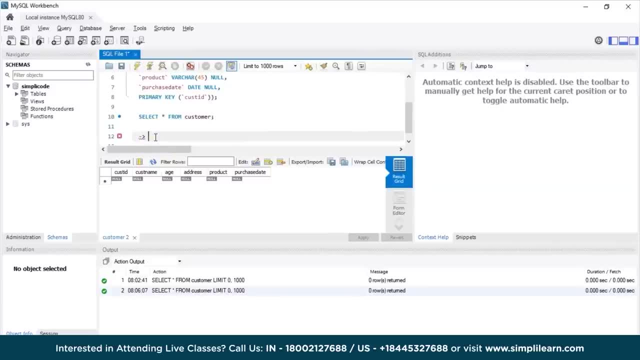 Now that we've created a table, let us see how to insert the values into it. For that, first let us discuss the INSERT INTO VALUE statement. The INSERT INTO VALUE statement is used to insert either all the column values or a specified number of column values in the table. 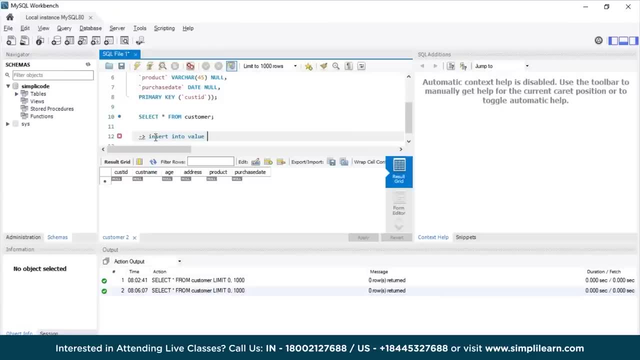 Inserting only specified column data in the row requires the column name should be specified in the INSERT statement. So let's say, if I want to insert all the columns into the customer table, the following query would be: INSERT INTO tableName, which is the customer. 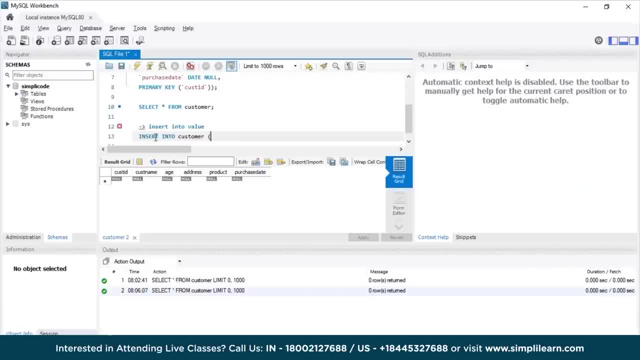 Now, within the brackets, we have to mention the column names. So the columns that we have taken are customerId, customerName, their age, address, product that they've purchased and the purchase date. Close the brackets. Now mention the VALUES keyword. 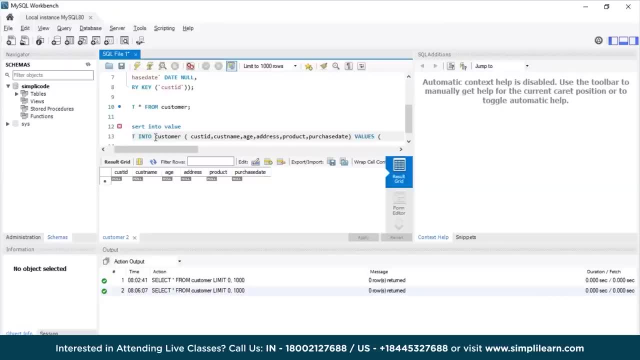 And again, within the brackets, specify the values for each of the columns. So I'm taking customerId, as let's say 1011, customerName, let's say Rahul. Now make sure you mention the character values inside the single quotes And for integer values. 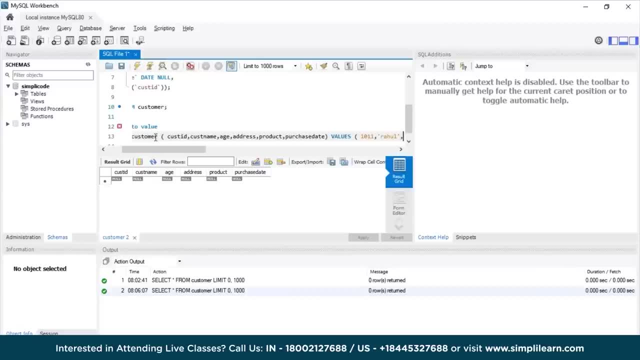 you need not mention the single quotes. Next, their age, let's say 25, address, Let's say the city they belong to is the address, So I'm taking it as Hyderabad. Next, the product that they have purchased. Let's say Rahul has purchased a phone as the product. 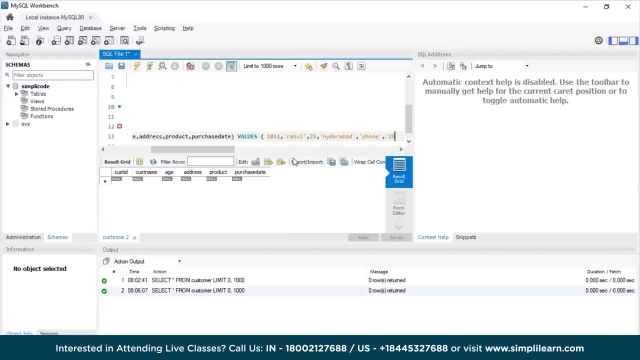 And finally, purchase date. Let's say 2022, March, And let's take date as 25.. So close the brackets and put the semicolon. So let us execute this statement and see. So, as you can see, our query has been successfully executed. 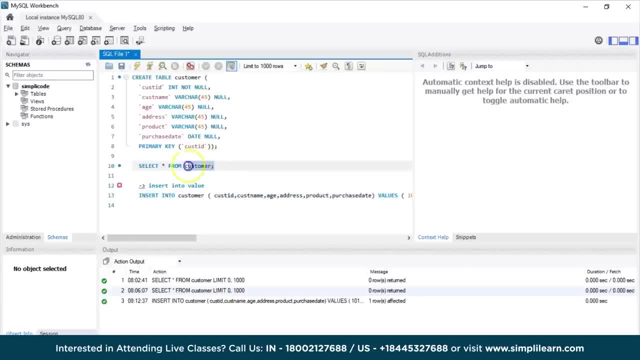 Now to display the values, I'll use the set command again, So let us execute the statement. So, as you can see, the values have been successfully inserted into our table with respect to their columns as customerId, customerName, age, address, product and the purchase date. 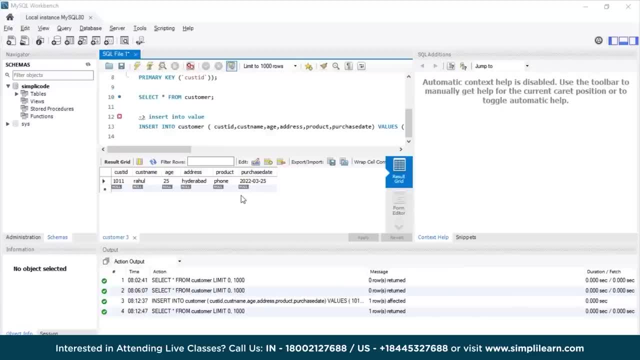 So here we've inserted a row with all the column values using the insert statement. Similarly, you can insert a row with only specified column values as well. Let's say, if you want to insert data for only the columns customerId, customerName and the product they've purchased. 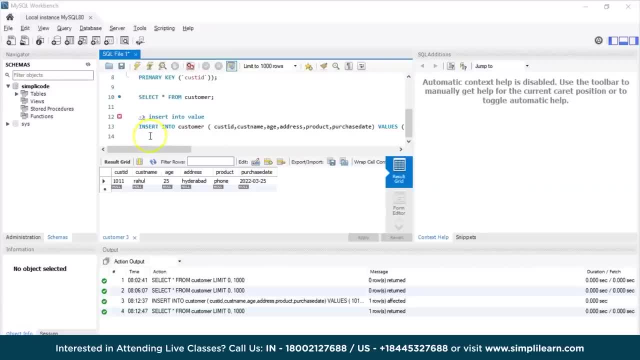 and leaving the rest of the columns as such. the following query would be: insert into tableName: mention the table name that is customer and within the brackets mention the columns that you want to enter the values. So I'm only entering the values for customerId- customerName. 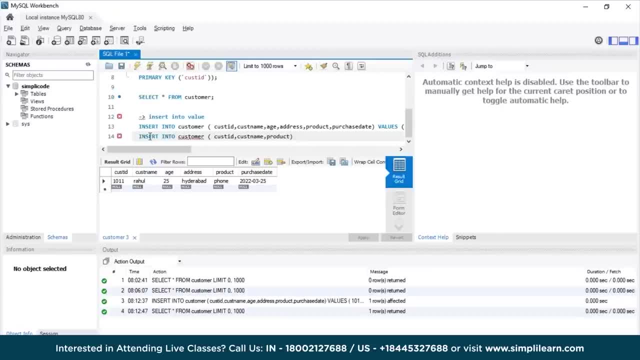 and the product that they've purchased And mention the keyword values, Open the brackets and specify the values accordingly. So I'm taking customerId as 1012, customerName- let's say Kavya- And the product that they've purchased is, let's say as AC. 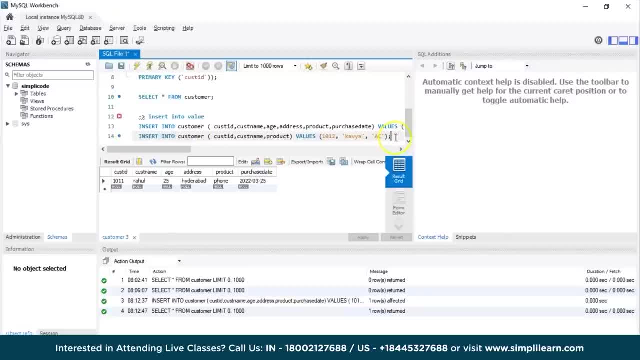 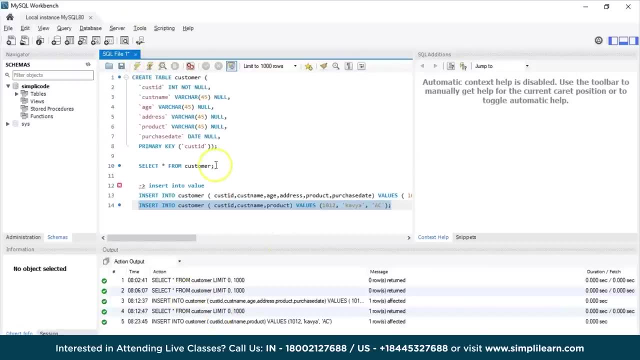 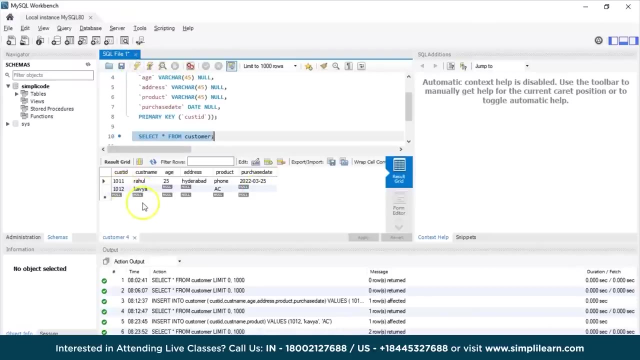 Close the brackets, Open the semicolon and let us execute the statement So as you can see our query successfully executed. So let me display the values and I'll use the set statement to display the values So as you can see only the customerId, customerName and the product that they've purchased. 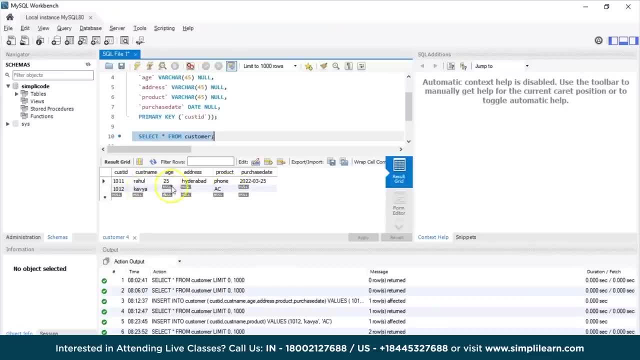 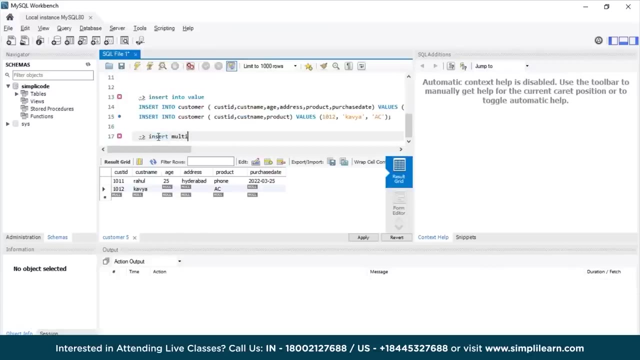 is being displayed here and leaving the rest of the columns- that is, age, address and the purchase date, as null values. So in this way, you can also insert values into only the specified columns of the table. Next, let us discuss about insertMultipleRows statement. 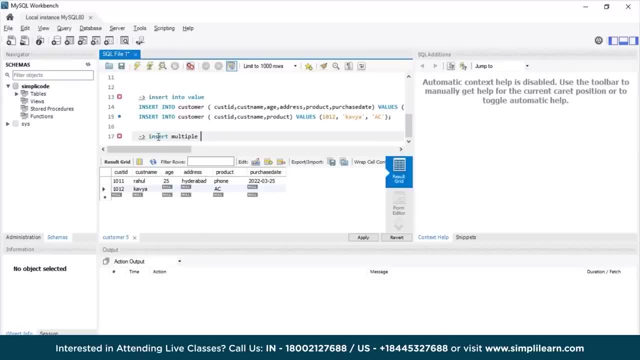 We can insert multiple rows in a single insert statement at a time. We can insert multiple row values by grouping row values with open and close brackets and separating each row with a comma. Now, if you want to insert, let's say, hundreds of records and insert values into it, 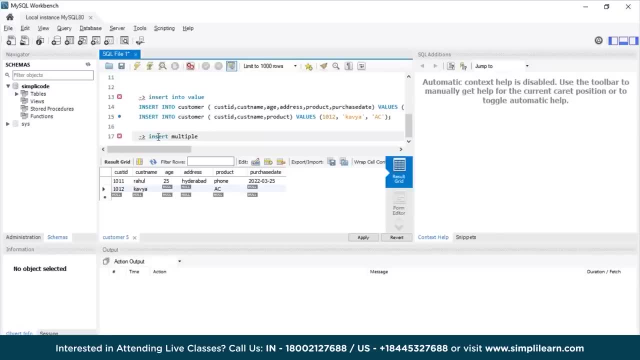 it will take a lot of time and at the same time it will become hectic if you specify the column names each and every time. So in order to reduce that and insert the values quickly, we use this multiple statement. So let's say, if I want to insert new values, 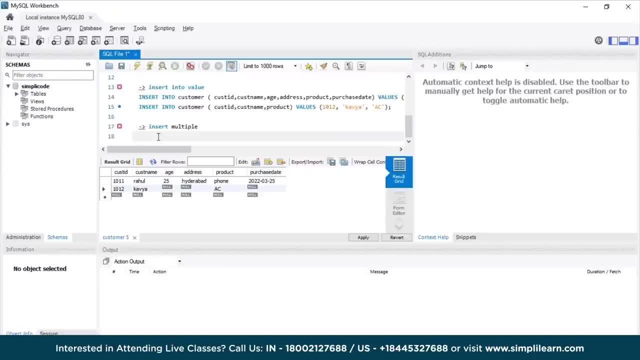 insert two rows of employeeId: 1013 and 1014.. So the following query would be: insert into customer, that is the table name and within the brackets. So before entering the values, you have to mention the keyword values And you can directly enter the values now without mentioning the column names. 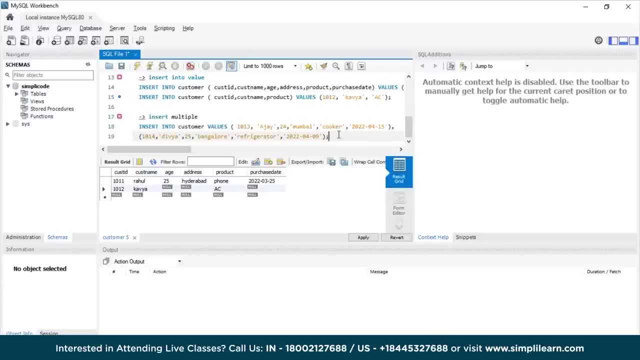 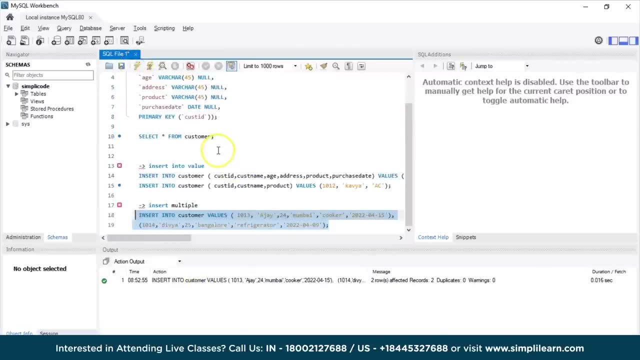 So, as you can see, I've inserted two rows and the data into the table, So let me just execute the statement and let us see the output. So I said, our query has been successfully executed. Let me use the select statement to display the new values. 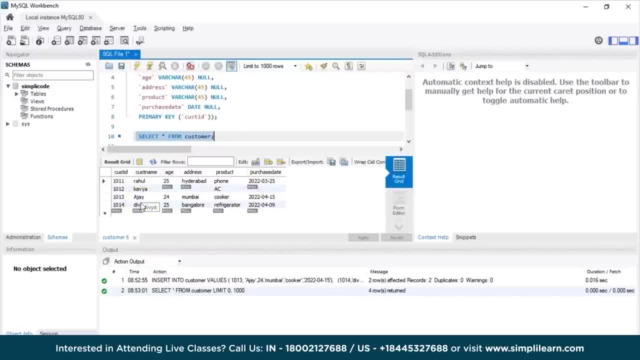 So, as you can see, the customerId 1013 and 1014 details has been displayed. So in this way you can use the insert multiple statement to insert multiple rows into the table. So just keep a note that make sure you insert the values accordingly. 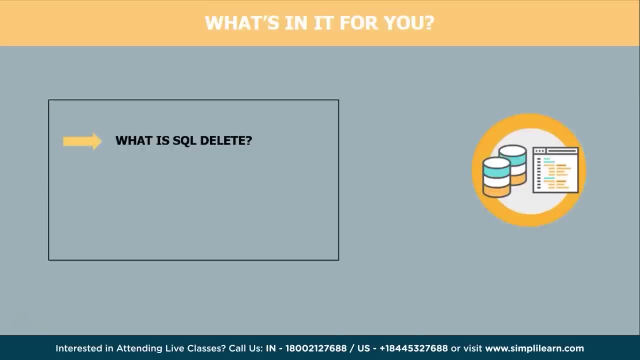 in the order of the columns that you have taken in the table. Let's start the tutorial by understanding what SQL DELETE statement is, And then we'll understand the syntax of SQL DELETE statement, And finally we'll look at some SQL DELETE statements and execute them in MySQL Workbench. 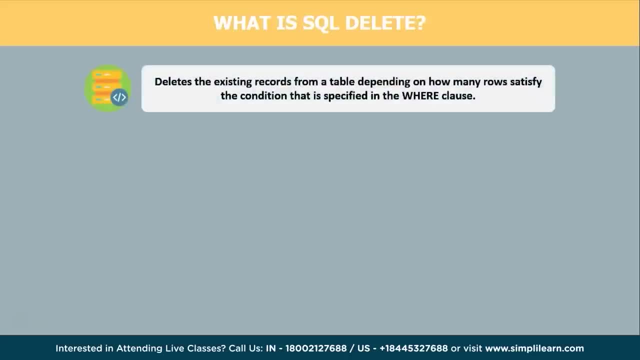 So what is SQL DELETE statement? SQL DELETE statement is one of the data manipulation command, DML, that is used to remove rows from a table. That means you will able to delete the existing records from the table. Now you can either delete a single row, multiple rows or values from the existing table. 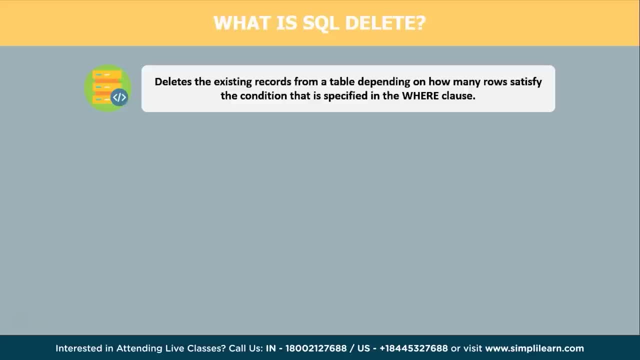 depending on the condition that is specified. That means DELETE statement with WHERE condition is used to delete the rows that satisfies the condition with WHERE clause and the remaining rows are not changed. Also, DELETE statement without WHERE condition is used to delete all the rows from the table. 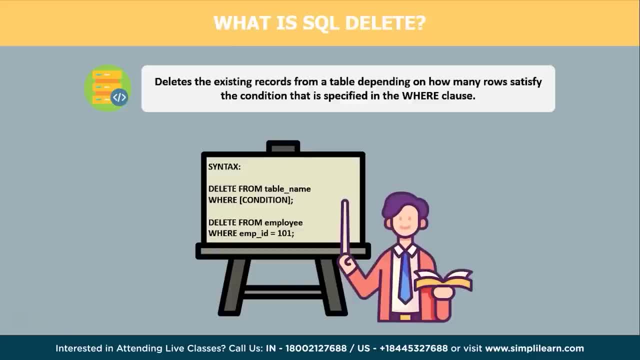 Let us now understand the syntax of SQL DELETE statement. The syntax is followed as: DELETE FROM TABLE NAME WHERE CONDITION- Here WHERE condition is optional. That means you can either use it or you cannot use it. So let us take an example. 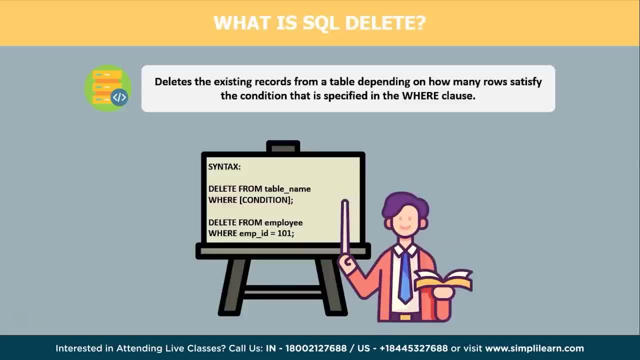 Let's say, if I want to delete the details of the employee from the employee table whose employee ID is 101. So for that the following syntax would be: DELETE FROM EMPLOYEE WHERE EMPLOYEE ID equals to 101.. Now, if you execute this query, 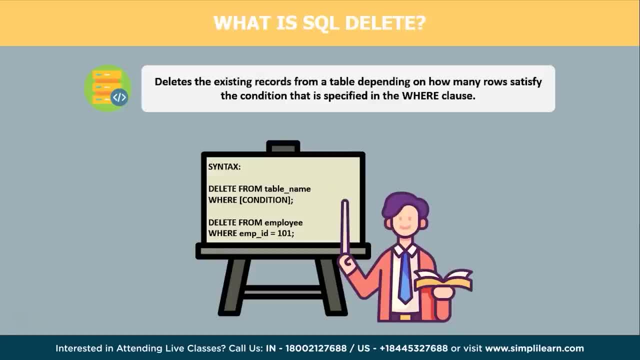 it will delete the details of that employee, whose having employee ID is 101.. In this way, you can use DELETE statement to delete one or more rows from the existing table. Now that we've got an idea on what SQL DELETE is, let us jump directly into the MySQL Workbench and get into the execution part. 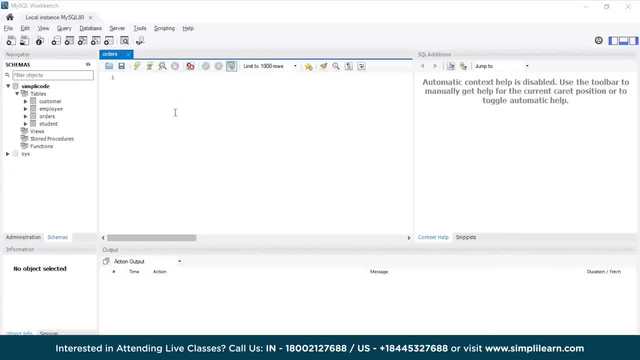 As you can see, MySQL Workbench has started and on the left side you can view the various tables that are present in our database. Simply Code. So let us consider employee table first as an example table to frame SQL queries to perform various operations using the DELETE statement. 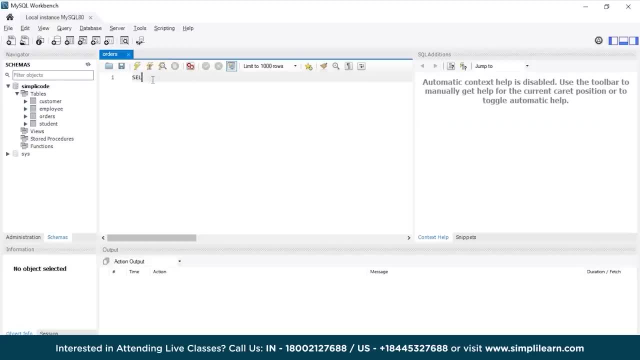 Firstly, let me display the values that are present in the employee table. For that I'm using the SELECT statement, SELECT star from the table that is employee. So let me just execute this statement So it will display the records of all the employees, their employee ID. 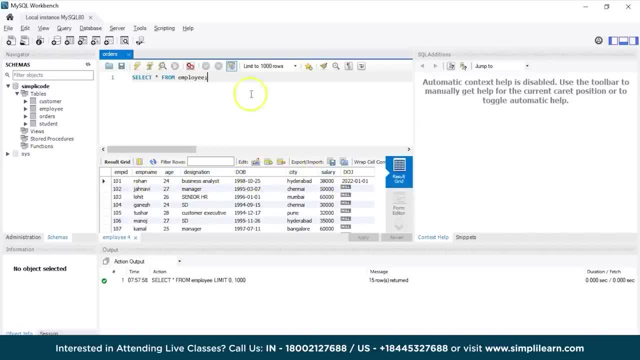 their name, age, destination, date of birth, city and salary. So firstly, let us see how to delete a single row from the given existing table. For that let me take an example. Let's say, if I want to delete one of the employee details from the employee table, 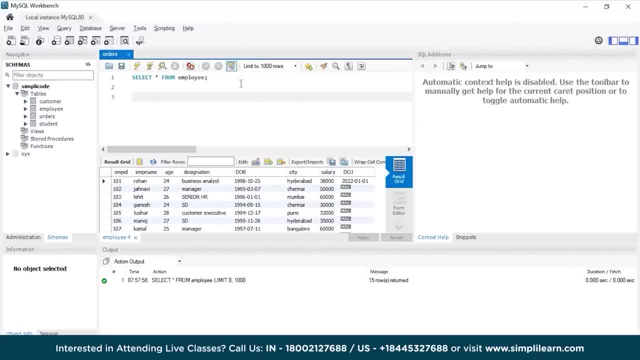 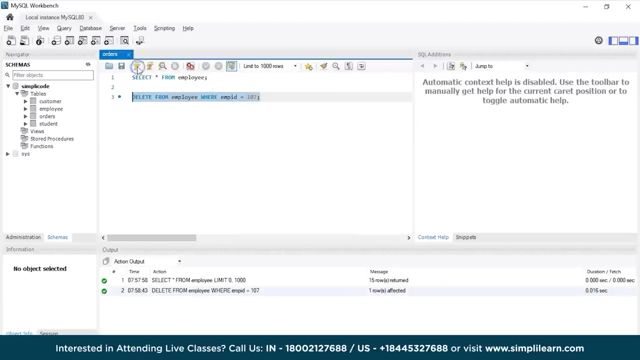 whose employee ID is, let's say, 108.. For that, the following query would be DELETE from table name: that is, employee, where specify the condition: employee ID equals to 107.. So let us execute the statement and see the output. So our query has been successfully executed. 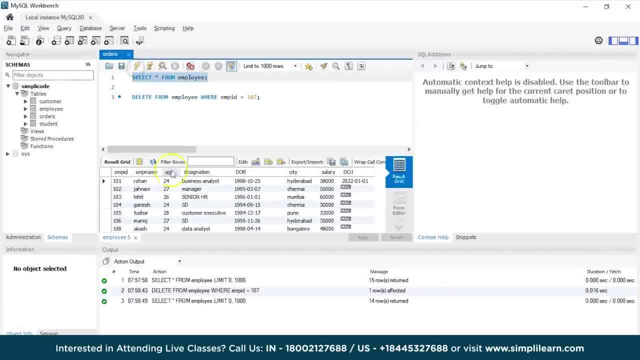 Let me use the SELECT statement to display the records and see whether or not our record is deleted or not. So, as you can clearly see, 107 record of the employee is missing from the table. That means we have successfully deleted the record of that employee. 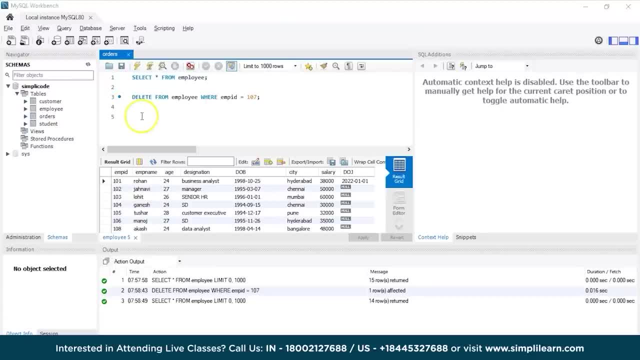 who is having employee ID 107.. Let us now understand how to delete multiple rows from the existing table. Before that, let me display the total number of records present in the table, so that we will have a clear idea on how many records have been deleted. 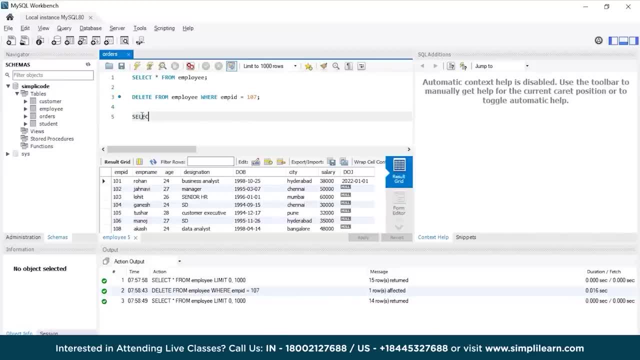 after executing the query. For that I am using a COUNT statement: SELECT COUNT. Use the star operator From the table, that is, employee, SELECT COUNT. We have total 14 records in the table. Let us now execute this statement. For that we will take an example. 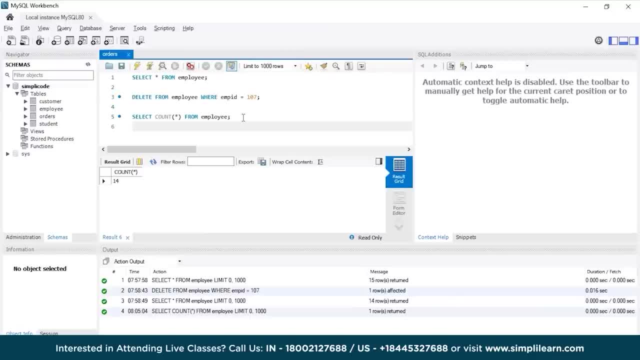 Let's say, if I want to delete multiple employee details from the employee table who's designation is business analyst, For that the following query would be: DELETE FROM table That is employee where designation equals to business analyst. So let us execute the statement and see the output. 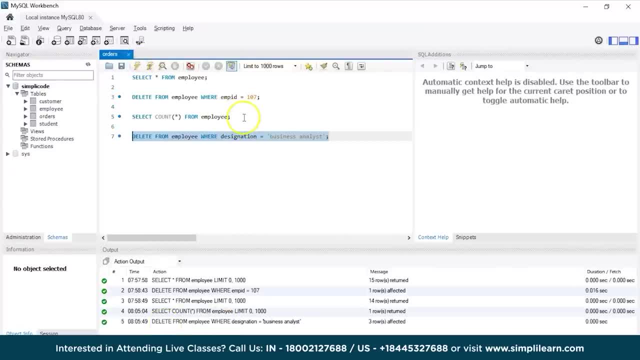 So, as you can see, our query has been successfully executed. Let us again use the count statement to see the values that are deleted. So, as you can see, the total count of the employees in the table has been changed to 11.. That means there are a total of three employees whose designation is business analyst. 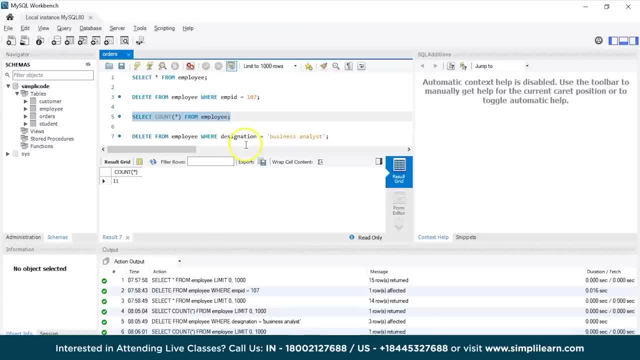 And since we have specified the condition where we want to delete only those records from the table whose designation is business analyst, So in this way, you can delete multiple rows By using the where condition statement. Now, similarly, you can delete multiple records from the table using multiple conditions, as. 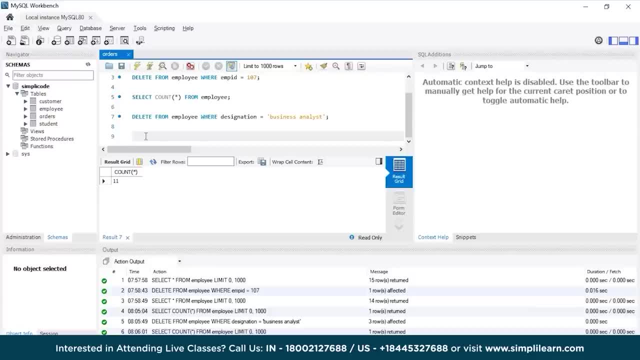 well, This can be done using various operators like AND, OR, BETWEEN, etc. So let us take an example for that Suppose. let's say, if I want to delete the employee details from the employee table whose designation is, let's say, data analyst, and their salary is less than 30,000.. 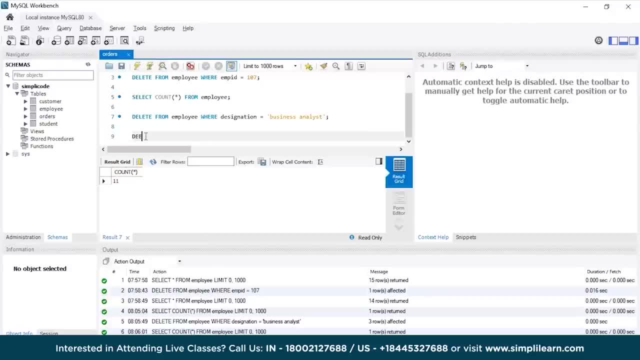 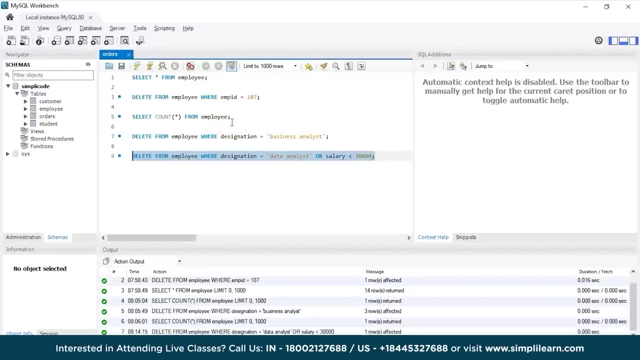 By using OR operator. for that, the following query would be: delete from table. that is: employee specify the condition where designation equals to data analyst or their salary is less than 30,000.. So let us execute this statement now. So our query has been successfully executed and let us see the output. 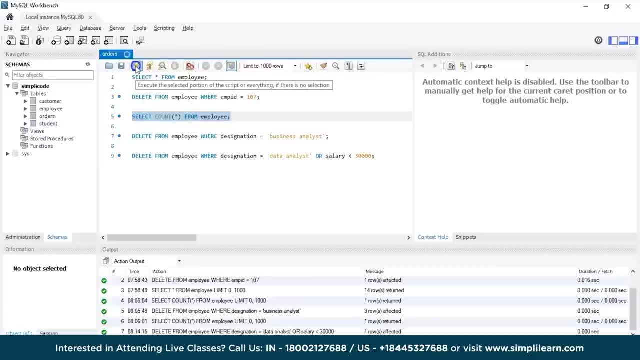 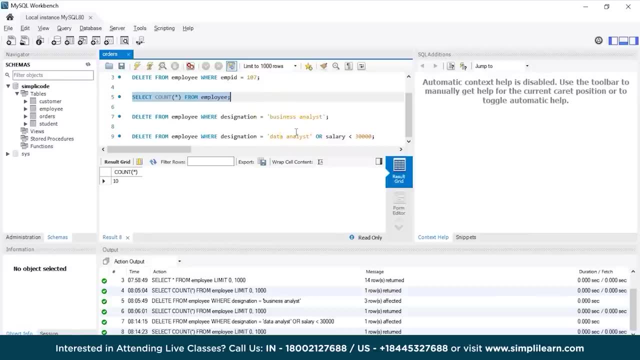 For that I am using the SELECT COUNT statement as well again. So, as you can see, only one record has been deleted from the table. That means there is only a record of the employee whose designation is either data analyst or their salary is less than 30,000.. 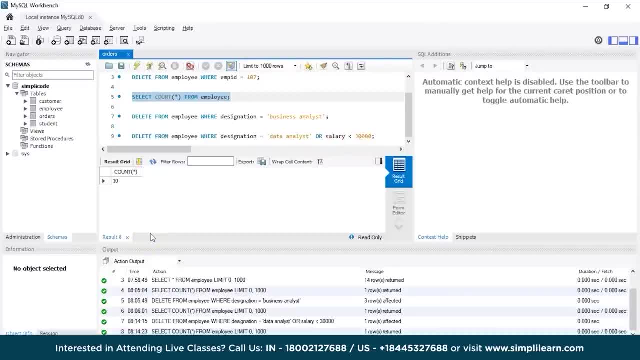 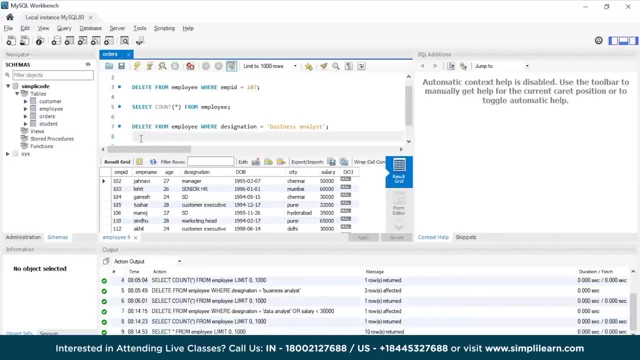 So in this way you can use multiple conditions to delete the records from table as well. Let us now take another scenario. let's say, if I want to delete multiple employee details from the employee table Whose salary is in between, let's say, 30,000 and 45,000, for that I'll use the BETWEEN operator. 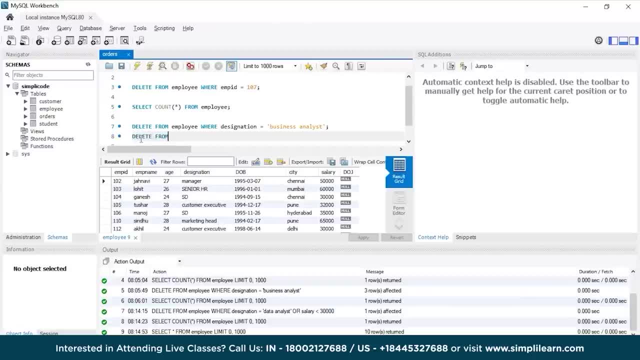 and the following query would be: delete from the table employee where salary BETWEEN is the operator that we have to use: 30,000 and 45,000.. So let us see. So let us execute this statement and see the output. So our query has been successfully executed. 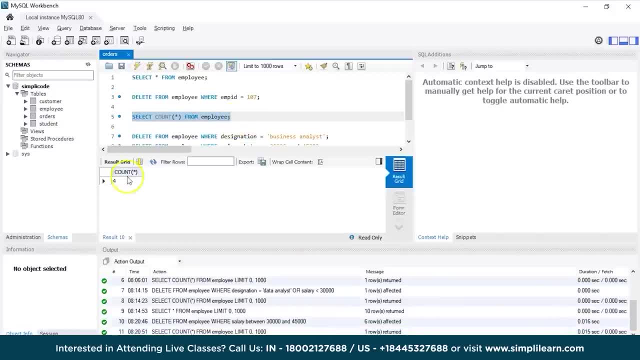 Let me use the COUNT statement to display the number of records now. So, as you can see, previously we had 10 records in the table. now it has been changed to 4.. That means a total of 6 records has been deleted from the table, wherein the salary of the employees. 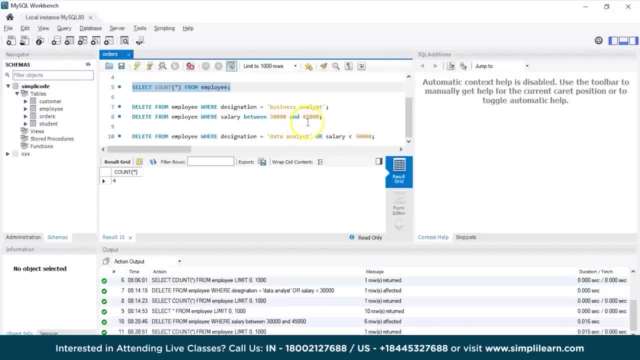 are ranging between 30,000 and 45,000.. So let's see how this works. Let's see So: in this way, you can use the DELETE statement to delete multiple records from the table by specifying the multiple conditions. Now we have seen how to delete a single record or multiple records, or even multiple records. 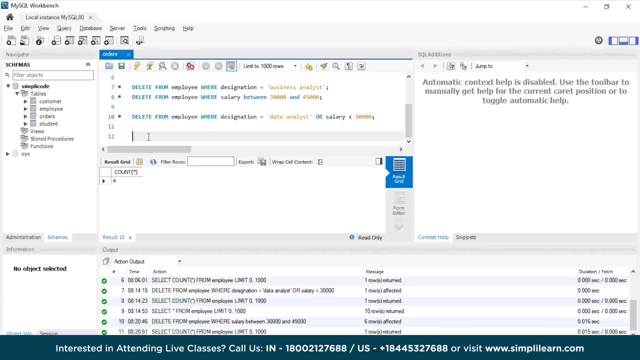 using multiple conditions in the existing table. Sometimes there might be a requirement to delete the entire table data to free up the memory or to allocate new data into the table. So in this case we use the DELETE statement to delete the whole record from the table. 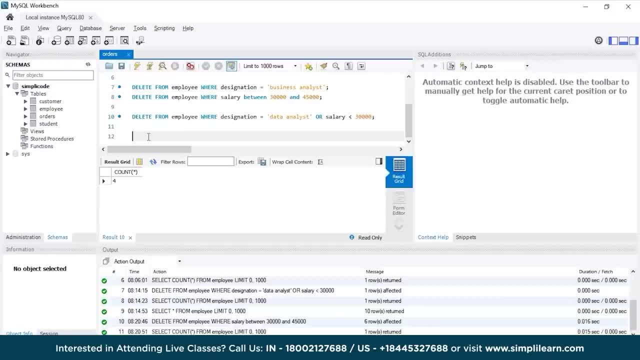 as well, For that executing DELETE statement without the WHERE clause deletes the entire table data. So make sure you are careful while using the DELETE statement, because you will end up deleting the whole table if you are using a without WHERE clause. Let's say, if I want to delete the remaining records of the table from the employee table. 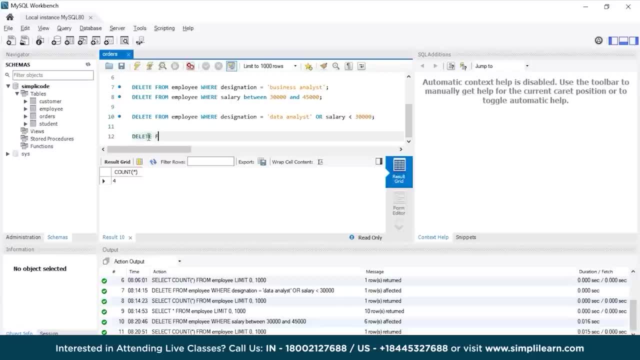 I'll simply write the query as DELETE FROM TABLE. So let's say I want to delete the remaining records of the table from the employee table. I'll simply write the query as DELETE FROM TABLE. So let's see how this works. Let's say I want to delete the remaining records of the table from the employee table. 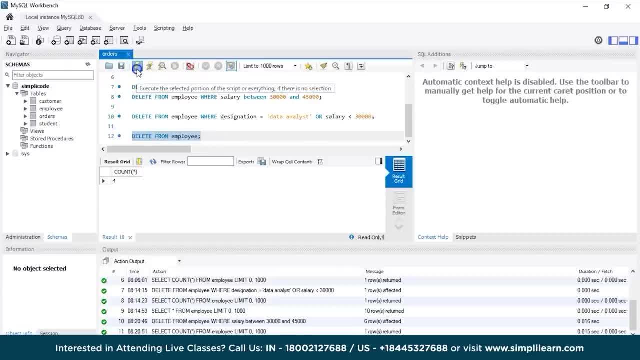 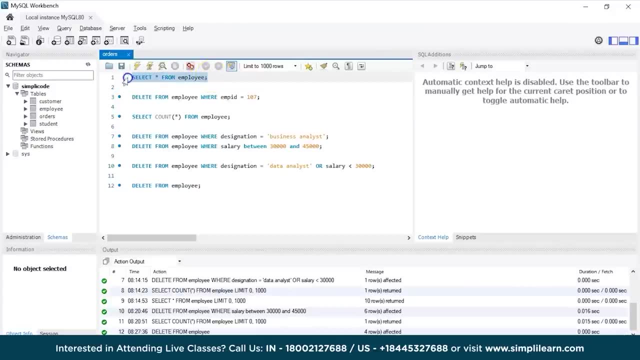 So let's say I want to delete the remaining records of the table from the employee table. Let's see how this works, So let me execute this statement and see the output. Our query has been successfully executed, So let me just display the records in the table. for that I'll use the SELECT statement. 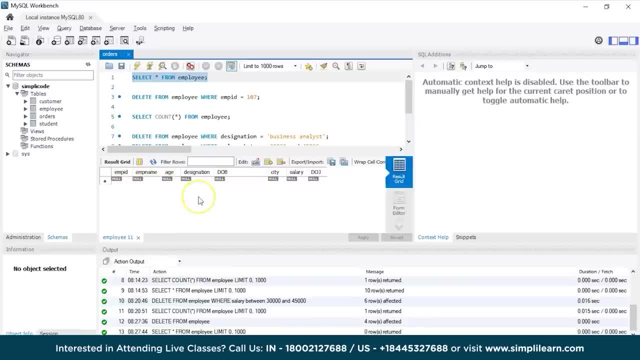 So, as you can see, only the columns have been present, but the records that were present in these columns have been completely deleted using the DELETE statement. So in this way, you can delete all the records from the table without specifying the conditions, trying the condition using the WHERE clause. 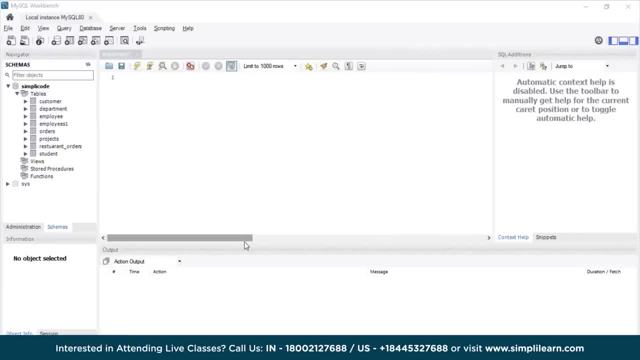 The column operations play an important role because for even for data analysis, or even if you're performing queries on your database table, it is quite essential Because, let's say, for instance, you have created a table as per your requirement, with a set of different columns. 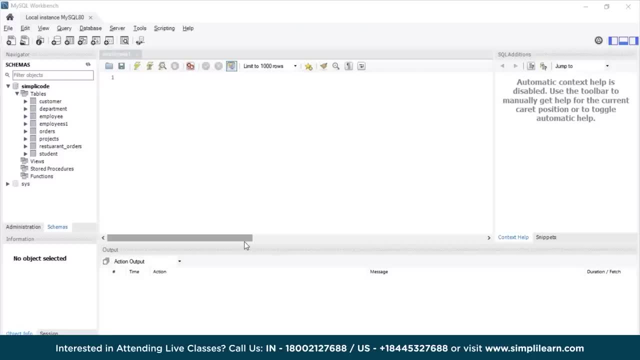 Now later, at a different stage, you might need to add some additional requirements where the table might need to have some additional columns, or even some columns might require to be deleted or some column names need to be changed into a new columns within that existing table. 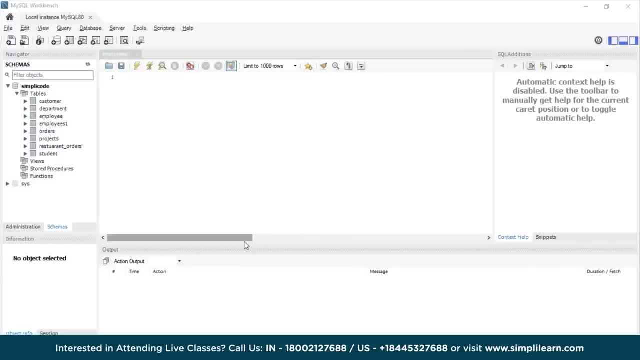 Now there are mainly two different ways to satisfy this condition. First is you have to delete the table and recreate a new table as per your new requirement. Now, this is possible and advised only when the table is empty. right Now, if the table is not empty, you have to copy the data and then delete the table create. 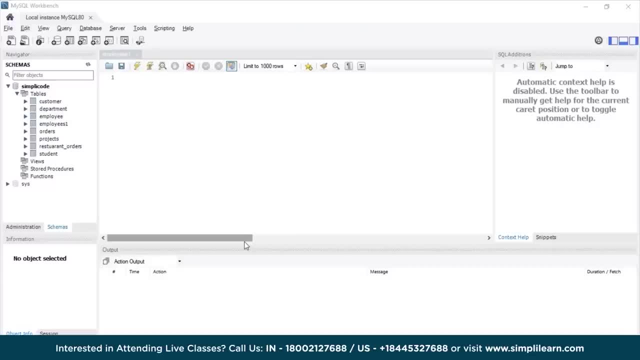 another table and then copy or load the data into the new table. Now, this is time consuming and also not advisable. The other way is to add, delete or modify the columns and the data present in it to the current table, without touching the existing columns and its corresponding data. 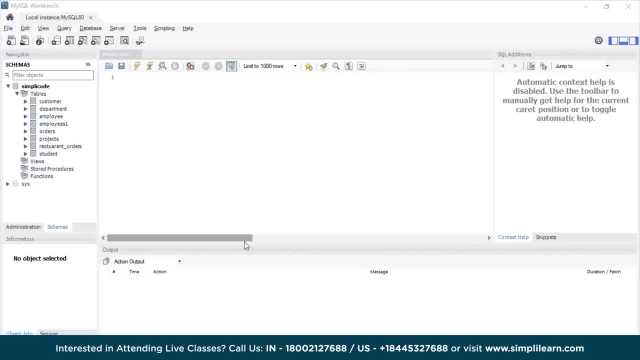 Now this is done by using the ALTER TABLE statement, which fulfills the requirement of adding new data within the existing columns. Now the ALTER TABLE statement is used to add new data within the existing columns. Now, the ALTER TABLE statement is used to add new data within the existing columns. 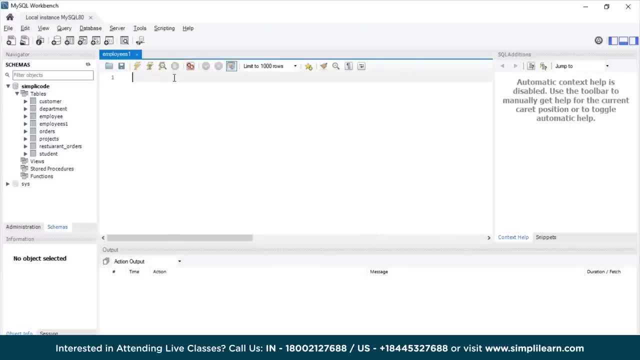 Now the ALTER TABLE statement is used to add new data within the existing columns. Now the ALTER TABLE statement is used to change the structure of the existing table by adding, deleting or modifying the columns, without modifying the data in it. So let us discuss what are the different operations that are performed in SQL. 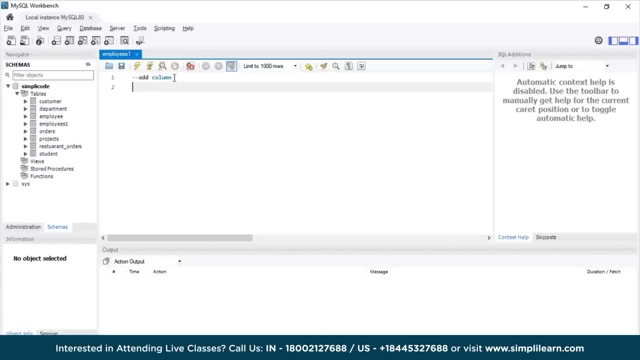 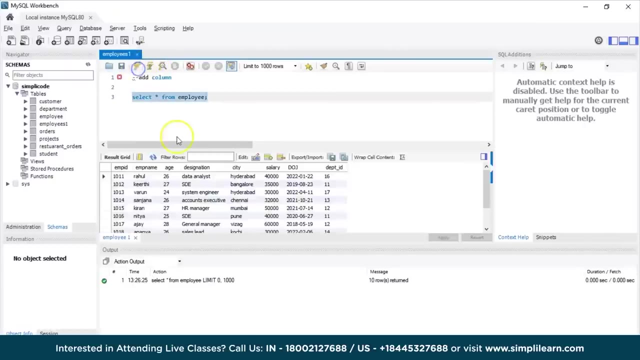 Firstly, let us discuss the add column operation in SQL. For that, let me consider the employee table. So let me just display the values in it. Select star from employee. So, as you can see, the employee table has various columns like employee ID, employee. 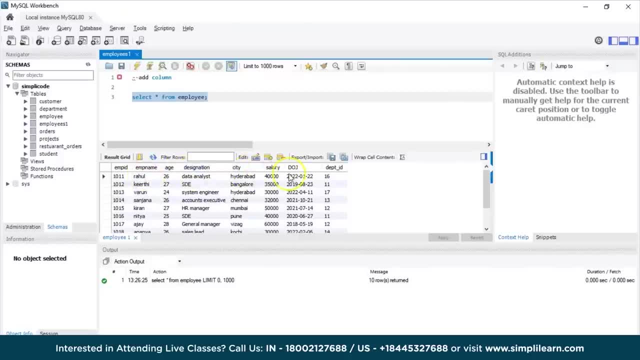 name, age, designation, city, salary, date of joining department ID. Now let's say I have an additional requirement where I want to add another column. Let's say, if I want to add the other number details of the employees, For that I'll use the alter statement and the query is: alter table employee, add column. 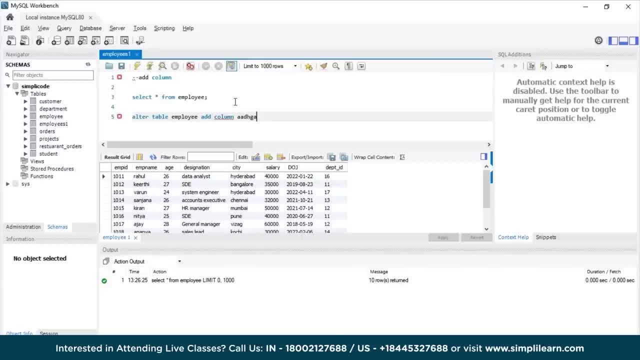 other number and mention the column data type. I'm taking varchar and we'll specify not null as our constraint. That means it must have a other number for every employee in the table. So let me just execute the statement. So, as you can see, our query has been successfully executed. 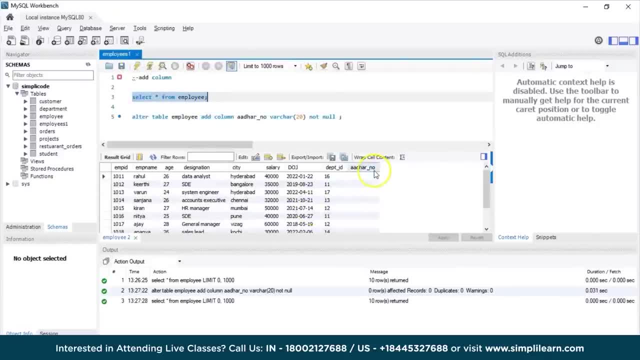 So let me just display the values. So, as you can see, there is a new column, other number that has been created in our existing table without disrupting any columns and its values in the employee table. Now, similarly, you can add multiple columns to your existing table as well. 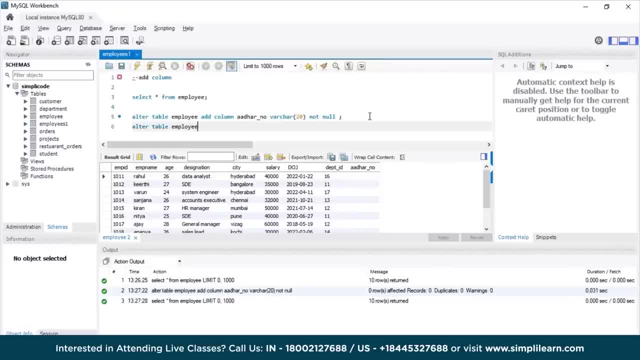 And the query is not null. The query is: alter table employee, add column and, within the brackets, mention the different column names. Now let's say, if I want to add the par number as well as the UAN, that is, the universal account number of the employees. 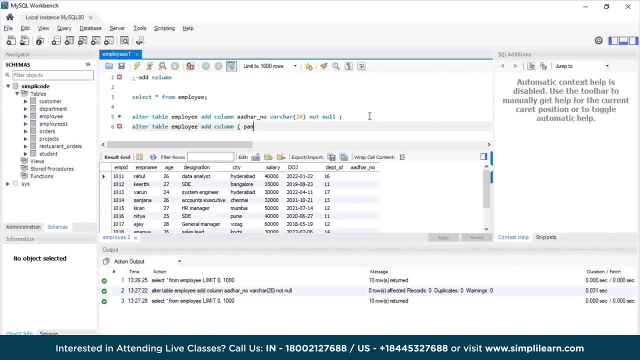 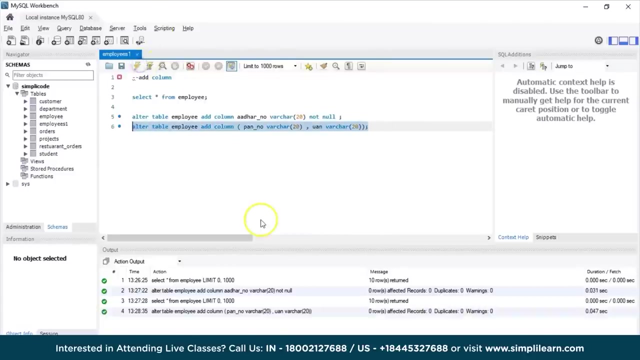 So the query will be: add column par number. mention the column data type. I'm taking varchar again. The next row: gamma UAN number. mention the data type as varchar. Let us execute the statement and see the output. So our query has been executed successfully. 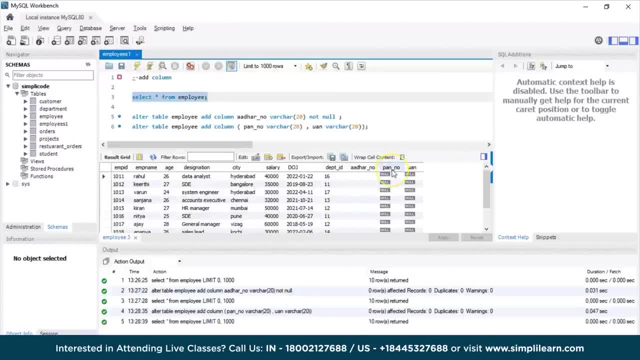 Let us see the output now. So, as you can see, we have two other columns par number and UAN number In our request. So let's see what is this. Let's see what is this employee table. since we have not mentioned, mention any constraints here as null or not null, so it by. 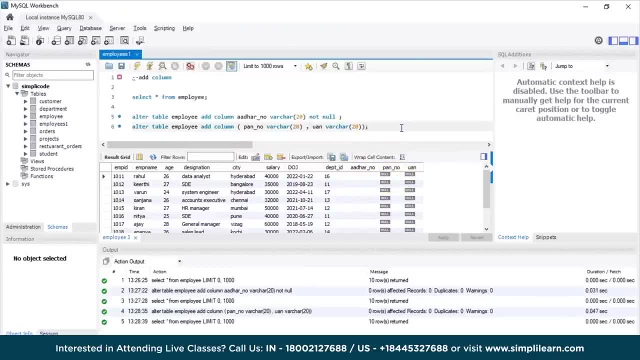 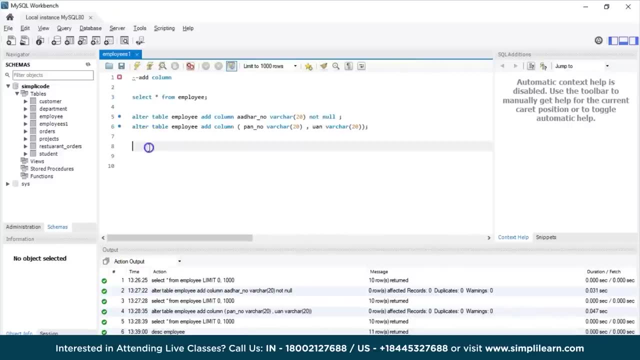 default it is taking here as null values. so in this way you can use the alter table command to add multiple columns in your table as well. now, similarly, you can even modify or update the column values as well. let's say, if i want to update the existing column name into a new name, now for that. 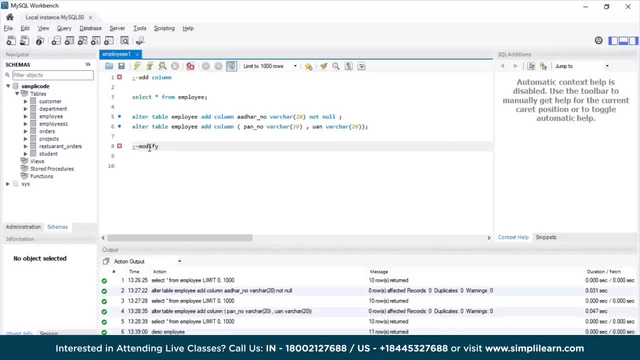 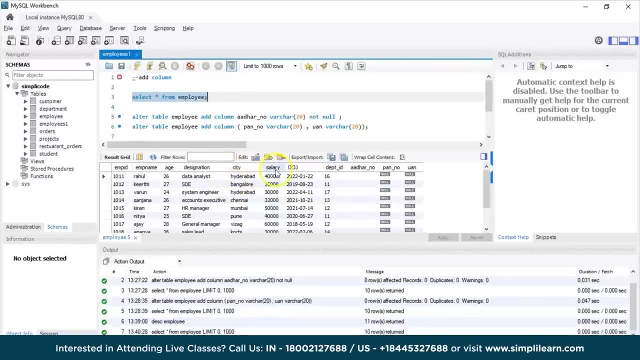 i'll use the alter table statement again now. consider the employee table again. so let me just display the values. now. if i want to change the salary column name into total salary, so for that the following query would be: alter table. employee change column is the keyword we use in mysql, so 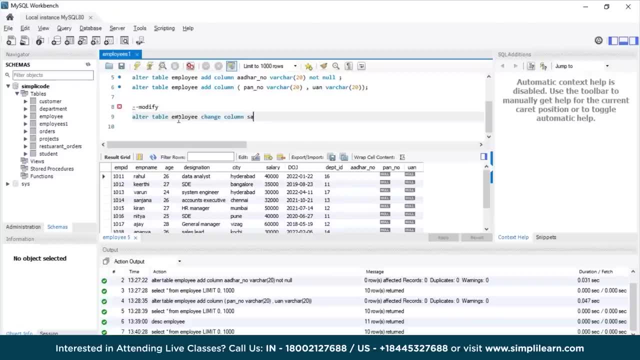 mention the keyword change column, so we want to change the salary column into total salary and also mention the data type as well. so let us execute the query and see the output. so our query has been successfully executed. so let me just display the records again, so as you 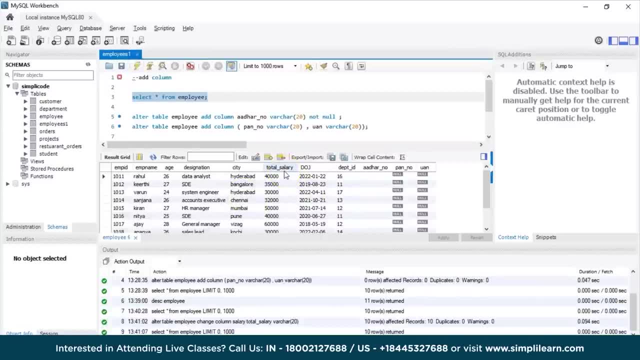 can see a salary name of the column. salary has been changed into the total salary here, so in this way you can update the column values as well now. similarly, you can also modify the existing uh column type in the table as well. for that, the following query would be: alter table. 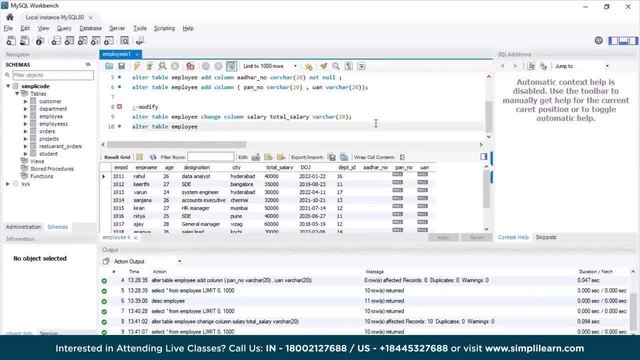 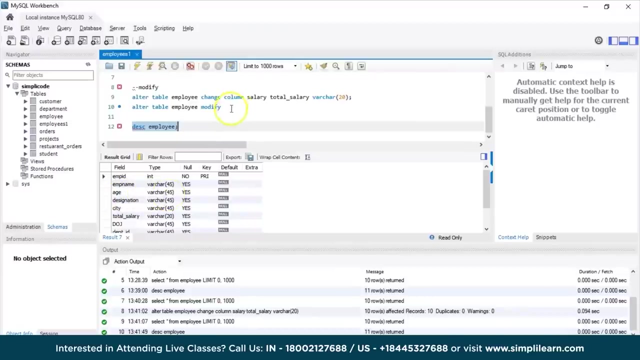 employee modify is the keyword now. let's say, if i want to change the age data type, so let's see what the initial or the previous data type version for age, so i'll use the describe employee query here. so we basically have varchar as our data type for the age. now if i want to change into int, so i'll just basically: 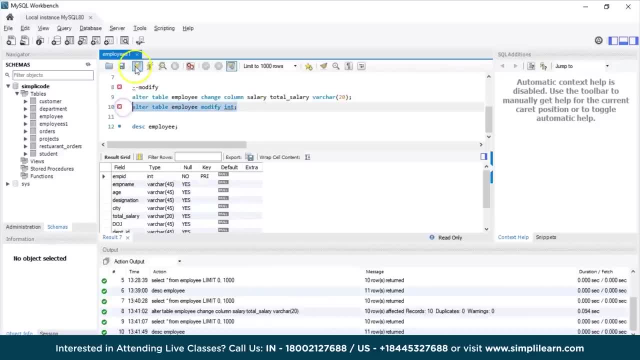 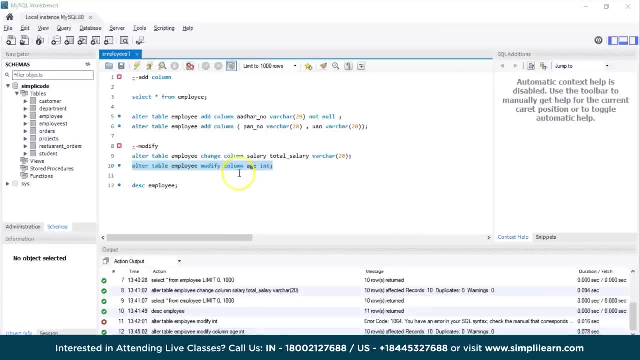 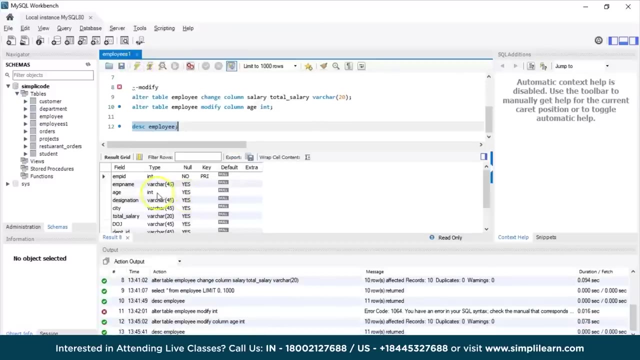 mention the int keyword here. so let us execute this statement and see the output. so there was a bit error. i forgot to mention the column keyword here, so that's how it is showing an error. so let me just again, uh, describe the table employee so as you can see the 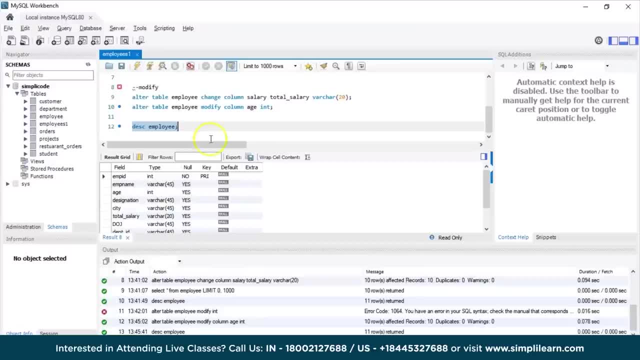 data type of the age column has been changed from varchar to int, so in this way, you can use the uh alter table to modify the column data type as well. now, similarly, we can also uh modify a new column or an existing column with a default value as well. uh, let's say, i want to take a new column. 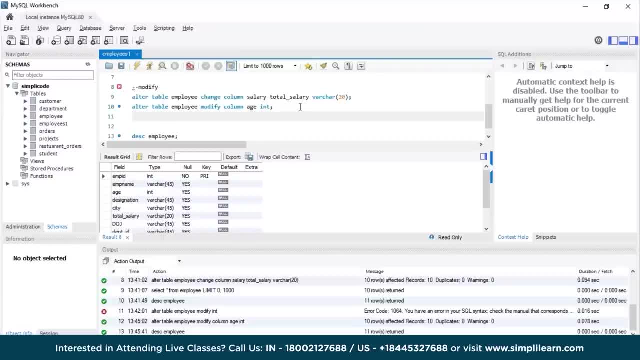 uh, bonus, that is the bonus salary for all the employees. so for that, the following query would be: alter table employee, alter column is the keyword we use here. bonus is the column that i'm creating, set default is the keyword and i'm keeping the bonus salary default as, uh, let's say, 15 000.. so let us execute the query and see the output. so i forgot to add. 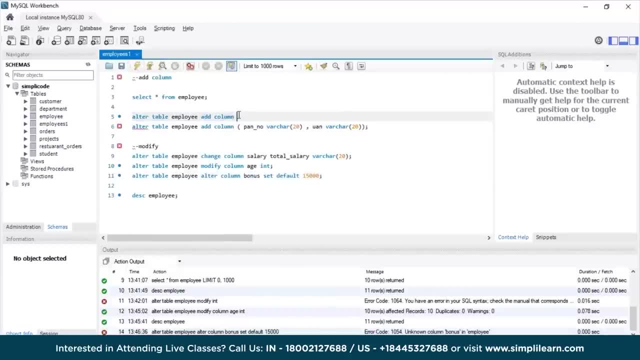 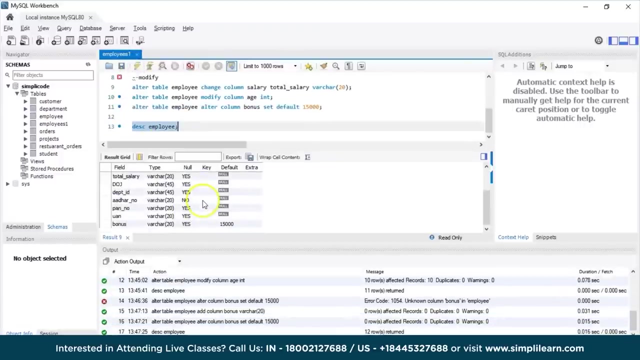 the column of the bonus. so let me just first add the column. so alter table employee, add column bonus: varchar 20. so our bonus column has been successfully created here. so now we can see our query will be successful here as well. so let me just describe the table again now. if you scroll down. 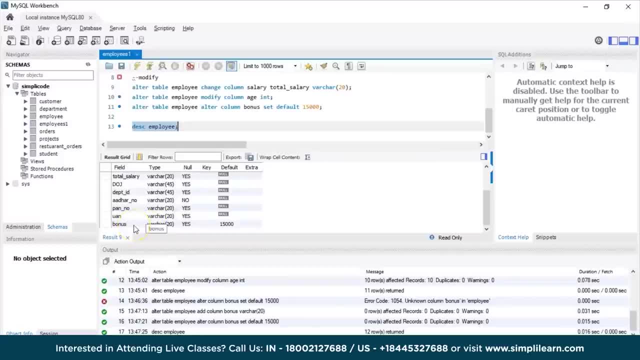 you can see the uh bonus column, uh, the field which it has the default salary as 15 000.. so in this way, you can add the default value to your existing columns or uh to your new columns as well. and finally, you can see that the default salary is 15 000.. so in this way, you can add the uh default value to your existing columns or uh to your new columns as well. 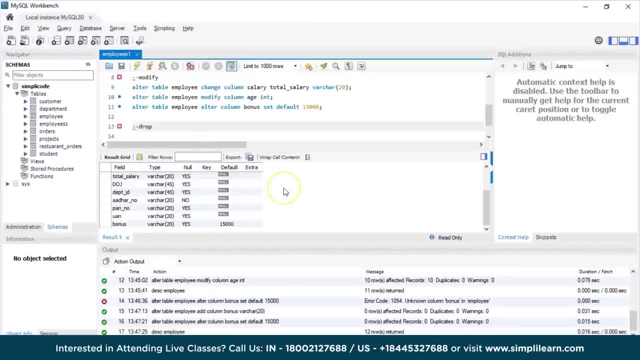 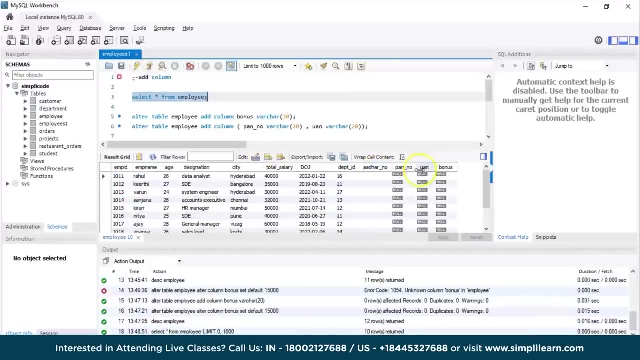 and finally, we can also drop the columns uh. the drop column is basically is used to delete the unnecessary or unwanted columns in our database. so let's say, if i want to delete the crea already created uh column, such as other pan, uan and bonus, so i'll use the drop statement here to delete the columns that were created earlier. so drop. 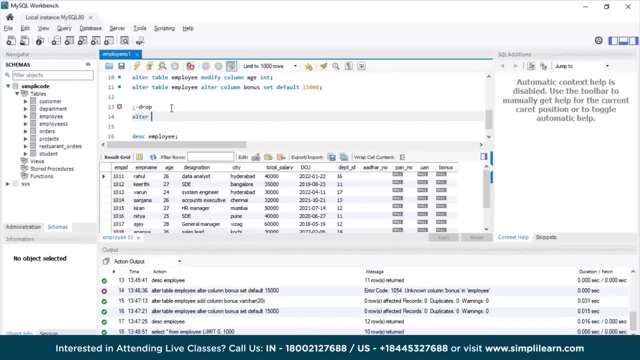 into drop statement. select the summary. click on the summary column. select another query. select a table, E table, employee. drop column. now first let us delete a single column here. so let's say, if I want to delete the other number column, so I'll use the other number. 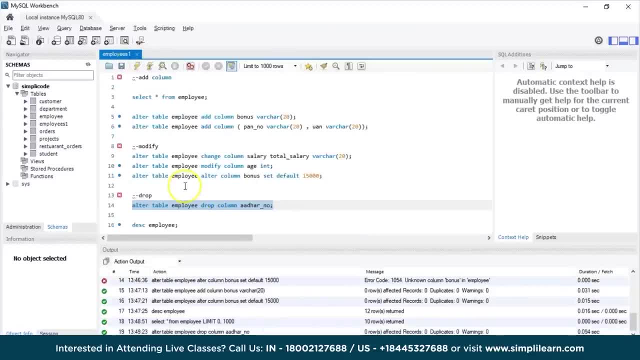 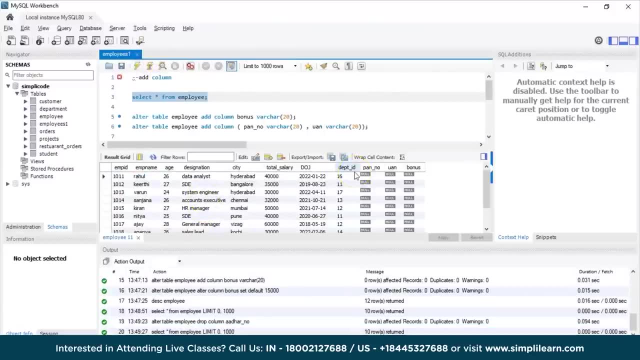 column here. so let us see the output. our query has been successfully executed. let me just select the records so, as you can see, other number column has been successfully deleted and similarly you can also delete multiple columns as well. all you have to do is just write the same query and put a comma and write. 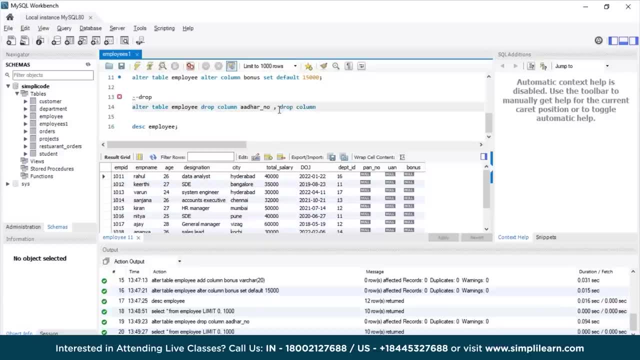 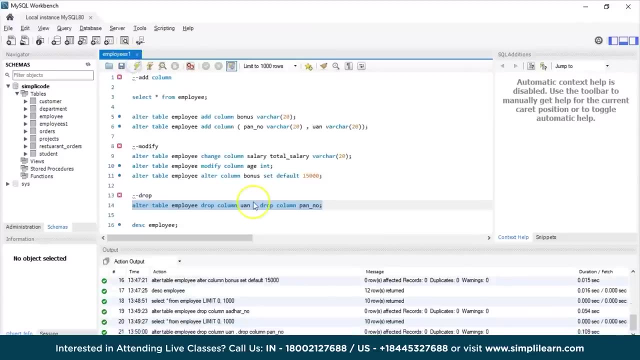 again the column drop, column keyword here. and let's say, if I want to delete the pan number as well, so pan number as well as the UN number here now, so I can use this query here. so let me just execute this and see the output. so our 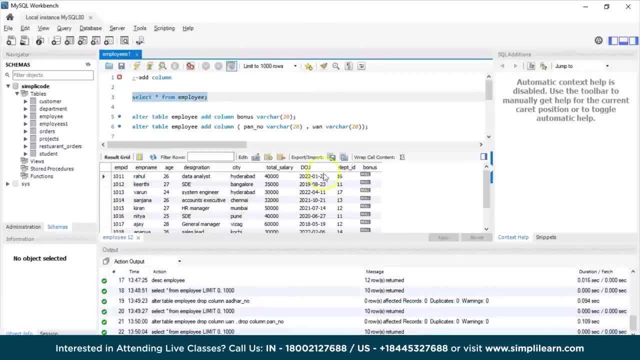 query has been executed. let me just display the records so as you can see. the UN number, as well as the pan number, has been successfully deleted from the employee table as well, and similarly the altered statement table. statement is also used to add and drop various constraints on an existing table, like 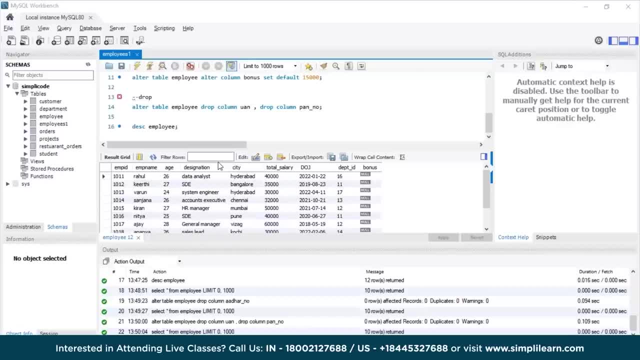 which we have discussed earlier. if you want your column a null value, then you can mention the null as the constraint there, and if you don't want any null values for your columns, then you can use the not null keyword in your alter table statements. so in this way you can use the 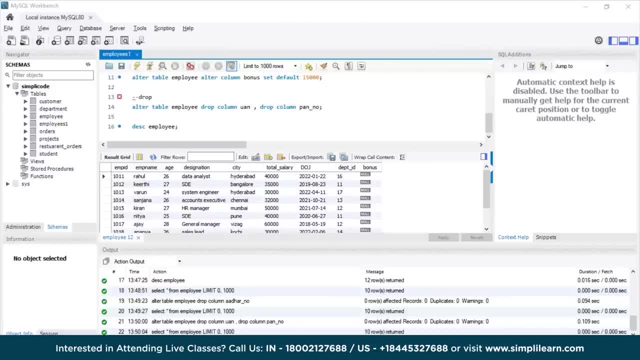 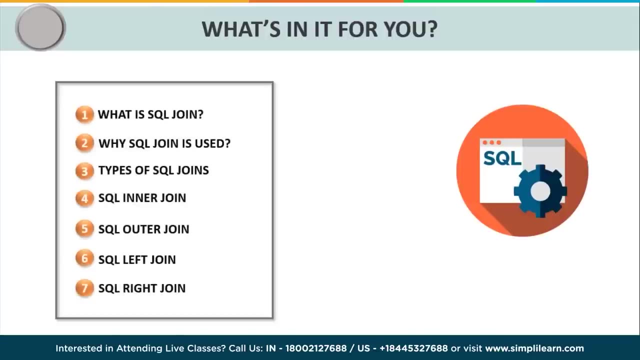 alter table statement to perform various column operations in SQL. so that was all about the SQL column operations, guys, where we have discussed about how to add, how to tell it and how to update or modify the existing columns in the database. start the tutorial by understanding what is SQL, join, and then 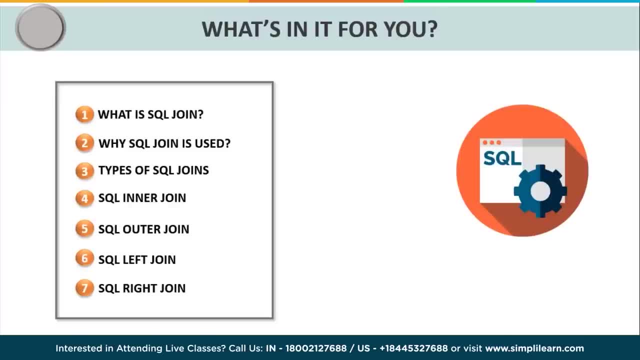 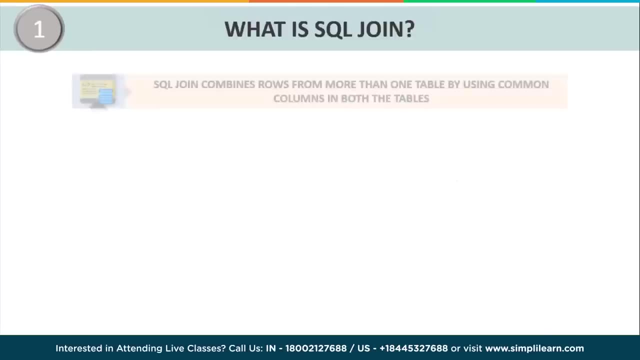 we'll discuss why we use SQL join and then we'll go through different types of SQL joins, such as SQL inner join, SQL outer join, SQL left join and final join and finally, SQL right join. so, without any further delay, let us dive straight into today's topic. so what is SQL join in relational databases? the information. 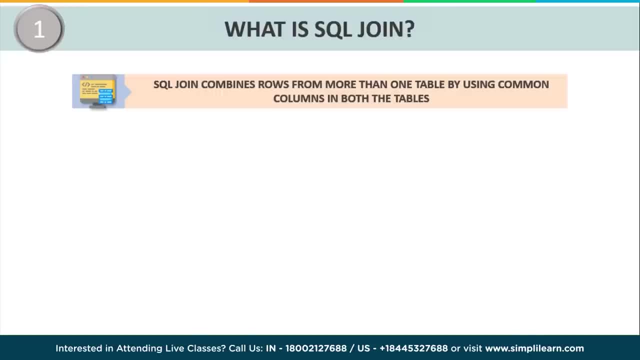 you want to retrieve is often stored in various different tables. in such scenarios, you'll need to join these tables to view data in a much better way. this is where SQL join comes into picture. SQL joins is widely used clause in SQL, essentially to combine and retrieve data from two or more tables. 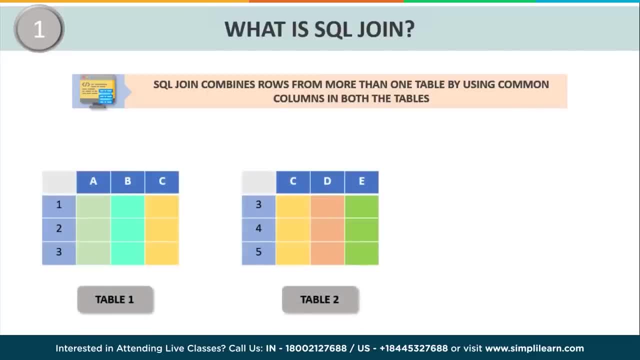 based on related columns or you can say common fields between them. now consider two tables here. table one has three columns, ABC and three records. let's say, for reference we will take them as 1, 2, 3. similarly, table 2 also has three columns, BCD and three. 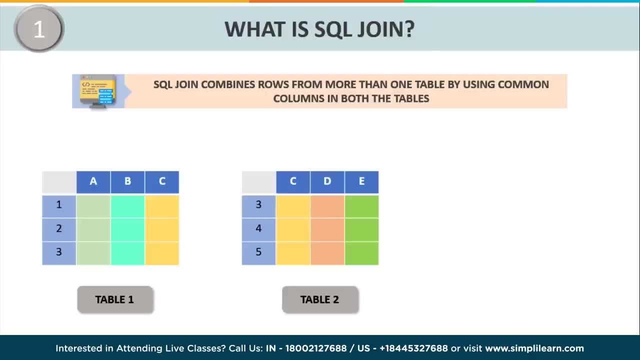 records 3, 4, 5. here I have taken a different color combination to represent values that are present in various columns. now, instead of querying each table every time to retrieve data, I'll simply join these two tables to view it. so we have D and Z rows and this will be the following resultant table: 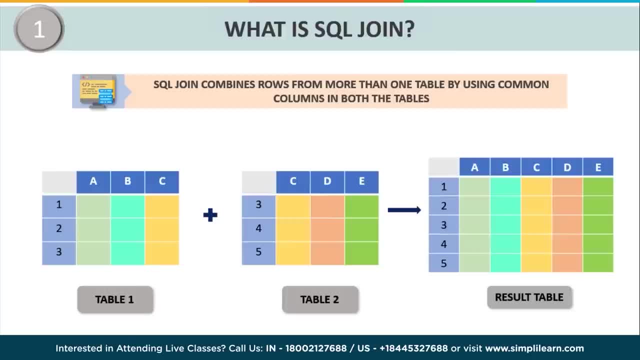 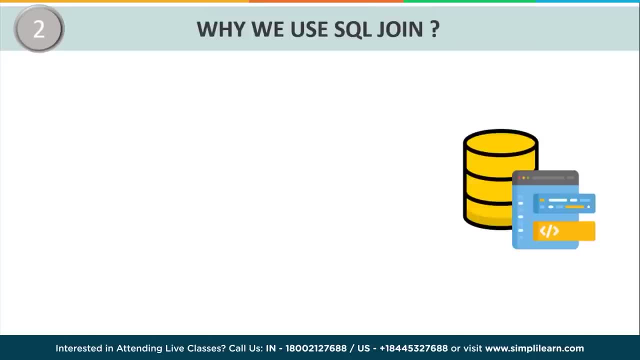 also make sure when you are joining two tables it should compulsarily have a common column. here, C is the common field which forms the basis to join these two tables here. why we use SQL join: flexibility: SQL join allows the user to access and manage records from more than one table easily. let us understand with: 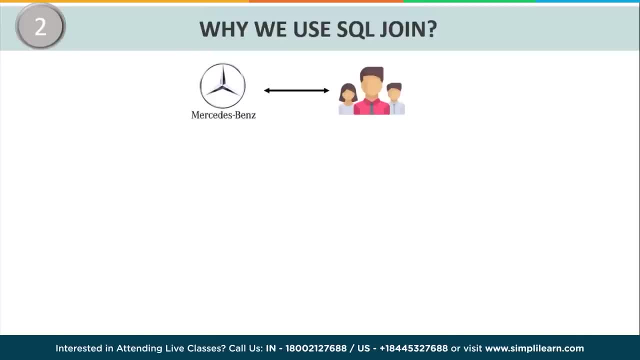 is one of the leading car manufacturers in the world and, let's say, they want to access the records of the customers from the database. Now, in the database, let us take, they have various different kinds of tables, such as customer table, order table, vehicle table. 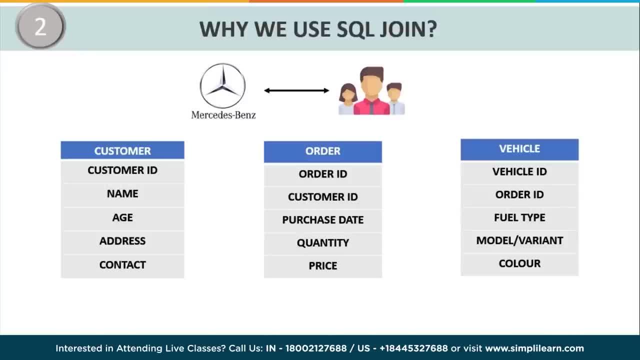 Now, if they want to get the vehicle details of so and so customer XYZ, for that they have to first query the customer table to get the customer ID. Now, if, once, if they get the customer ID, they have to query the order table to get the order. 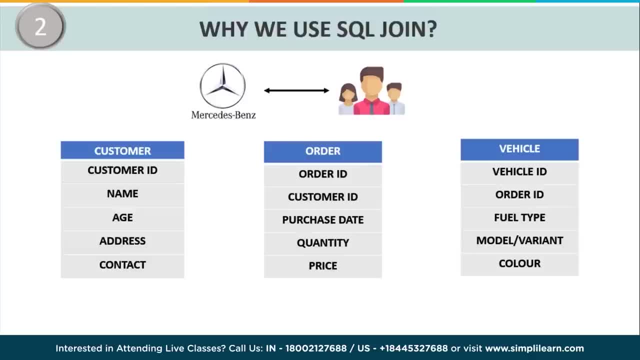 ID And, finally, with the help of order ID, they can get the vehicle details. Now, as you can see, this is a time taking, process and hectic at the same time. Now, instead of that, I'll just simply join these tables, which will allow the users to. 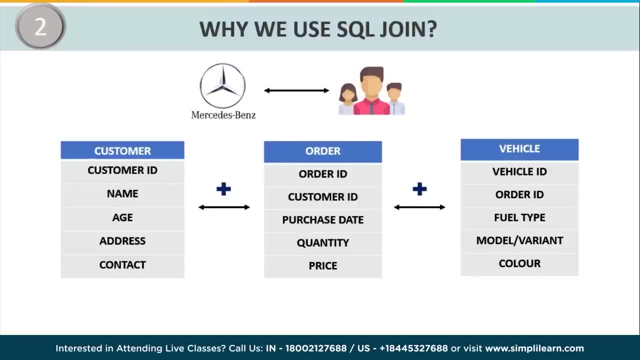 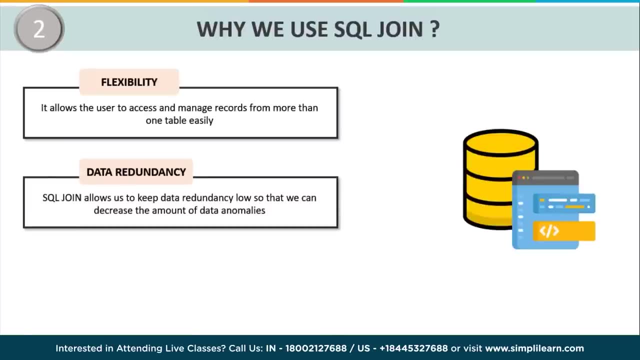 combine rows from two or more tables based on different types of conditions. In this way, you can access and manage your records easily. Data redundancy- SQL join allows the user to maintain data redundancy As much as low as possible, so that we can maintain the amount of data anomalies that. 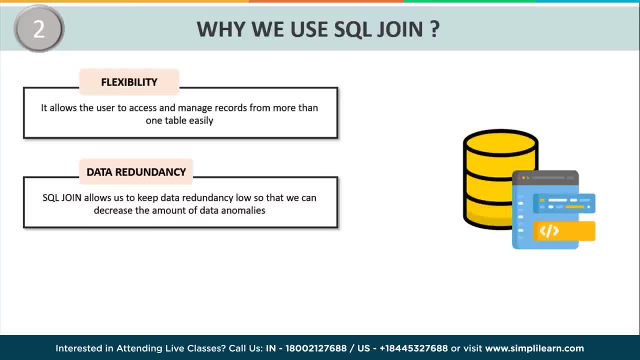 is the duplicate values that are repeated in various tables in the database. Finally, efficiency: SQL join executes the query faster and shows the result much more quickly because, instead of using various sub queries for each and every table individually, we can just simply join two tables using a simple single query. 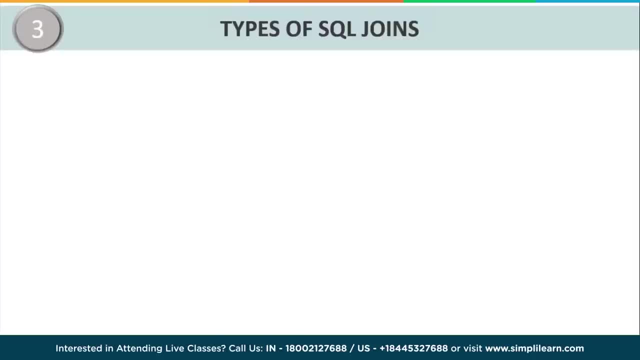 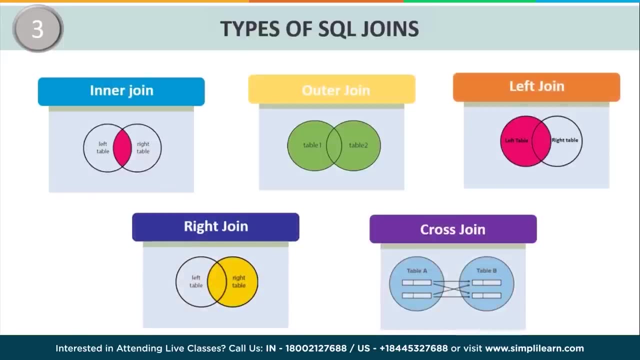 Types of SQL joins. SQL joins are broadly classified into four types. They are inner join, outer join, left join, right join and additionally we also have cross join, which is not that significant in its usage because most of the times we use the first four joins. 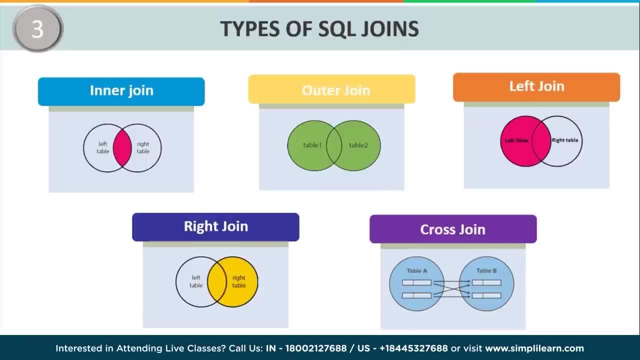 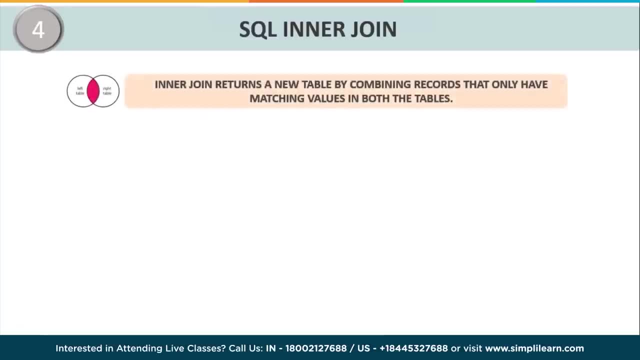 Now that we have gone through different types of SQL joins, let us discuss each of them in detail. Firstly, let us discuss about SQL inner join. SQL inner join joins two tables. It is based on a common column and selects records that have matching values in these. 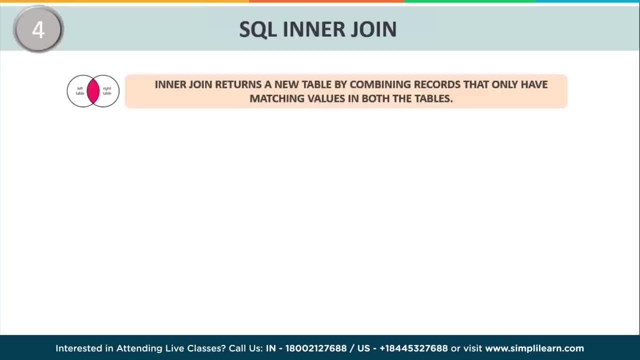 columns. Now, when the condition is applied for these columns, the query checks all the rows of table 1 and table 2.. Only the rows that satisfy the join predicate are included in the resultant table. Let us now understand the syntax of the SQL inner join. 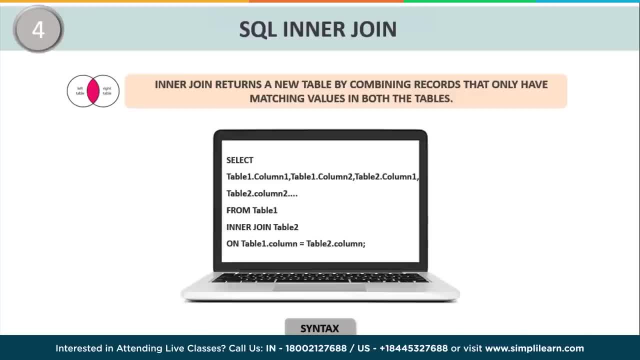 The syntax is followed as: select table 1 dot column 1, table 1 dot column 2, table 2 dot column 1 and so on from table 1 inner join table 2 on. table 1 dot column equals to table 2 dot column. 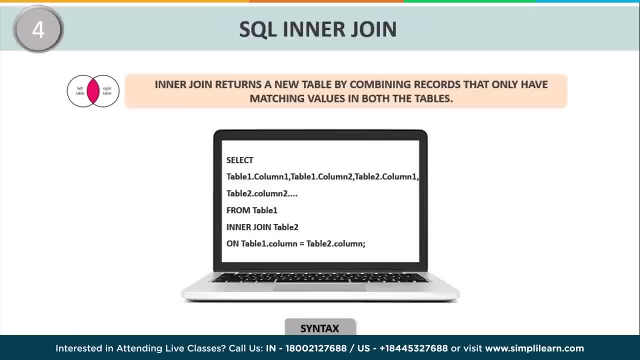 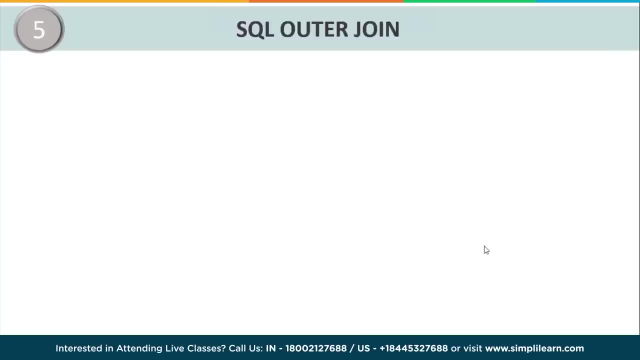 Now inner join syntax basically compares rows of table 1 with table 2 to check if anything matches, based on the condition provided in the on clause, and when the condition is met it returns matched rows in both tables with the selected columns in the select clause. 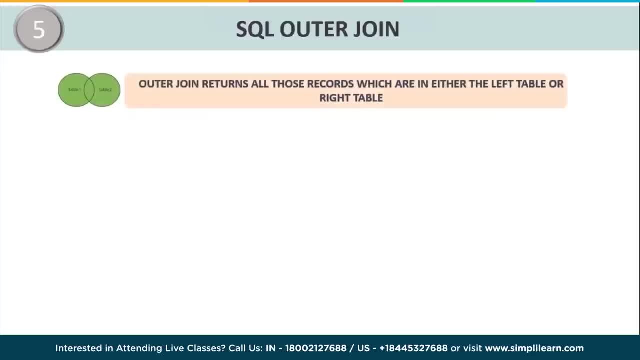 Let us now discuss about the SQL outer join. SQL outer join, Or else it is called as SQL full join or full outer join, is used to get all the rows which are present in both the tables. That means it will return all the records which are present in either left table that. 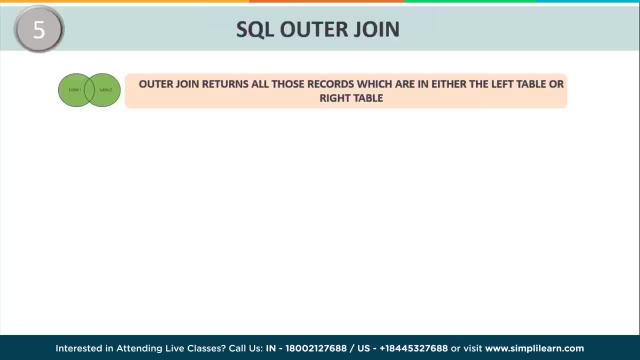 is the table 1 or the right table, that is, table 2, even if there are no matching records present in both the tables. Let us now understand the syntax. The syntax remains same, that is, select table 1, dot column 1, table 1, dot column 2, and so. 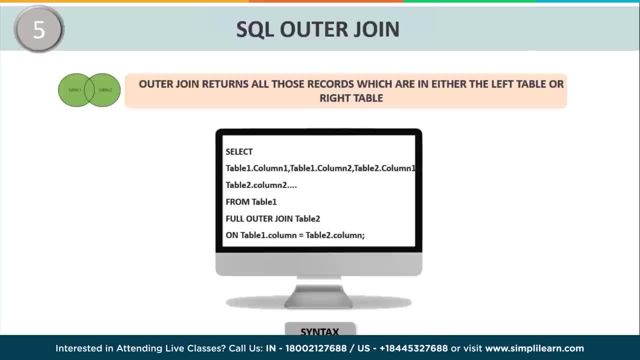 on up to table 2 dot column 2.. On table 1: full outer join is the keyword that we use here. table 2 on table 1 dot column equals to table 2 dot column. Now here you have to mention the same or the similar column name in the after the on predicate: 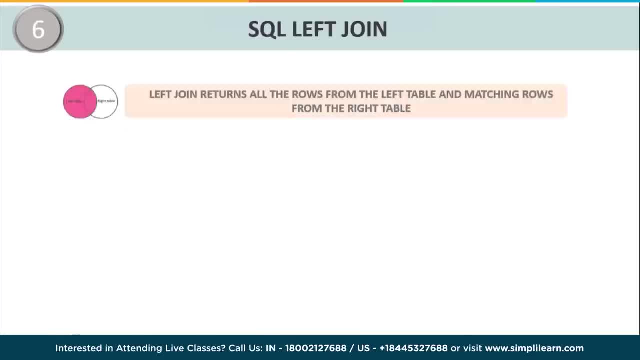 statement. Next we have SQL left join. Left outer join, also known as left join, results in a table containing all the rows from the table on the left side of the join- that is the first table- and only the rows that satisfy the join condition. from the table on the right side of the join- that is the second table. 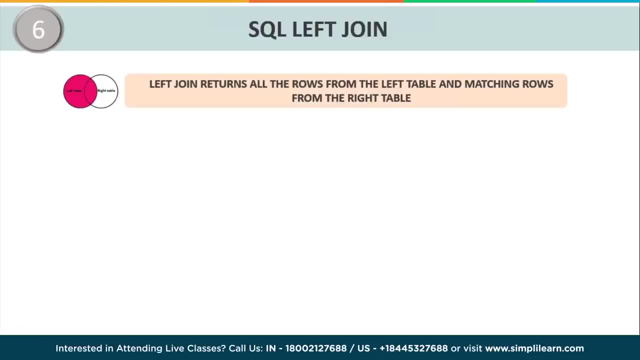 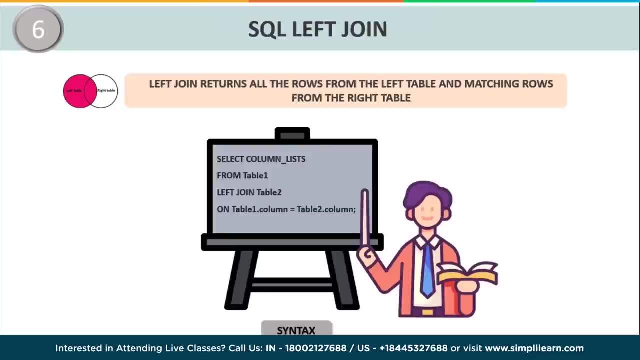 Any missing values for the rows from the right table in the result of the join tables are represented by null values. Let us look at the syntax. The syntax is followed as select column list. that is the column that you want to display in your table. 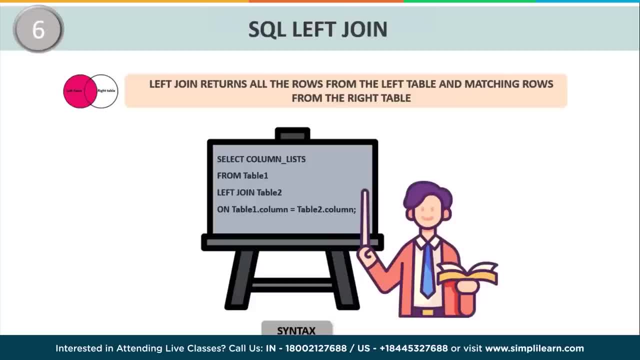 Now make sure you maintain the syntax of the column list, that is, the table name, dot column name. Otherwise you will throw an error. So let me just repeat the syntax. The syntax is: select column list from table 1. the keyword that we use here is: left join. 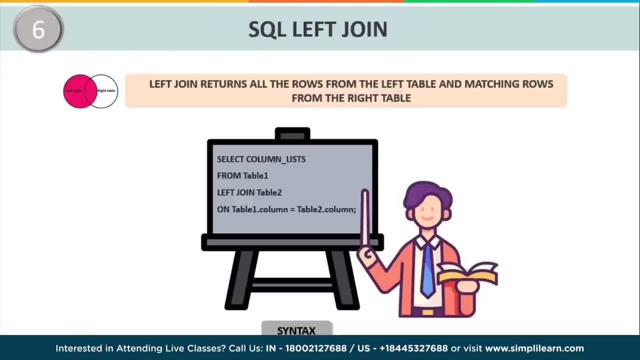 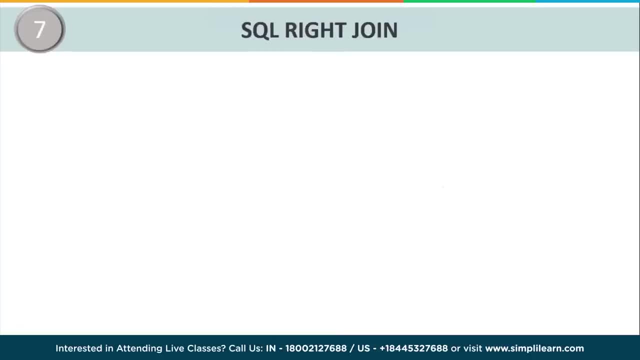 table 2 on table 1 dot column equals to table 2 dot column, So in this way you can use the left join to display the records. Next, finally, we have the SQL right join. Now right join or right outer join is opposite to that of the left outer join. 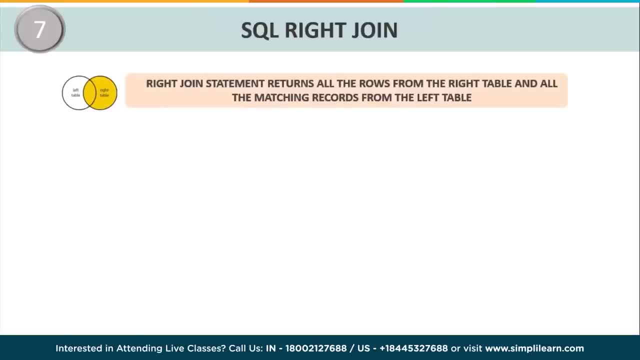 Now it follows the same rules as the left outer join. Now it follows the same rules as the left outer join, And the only difference is that all the rows from the right table, and only the conditions satisfying the rows from the left table, are present in the resultant table. 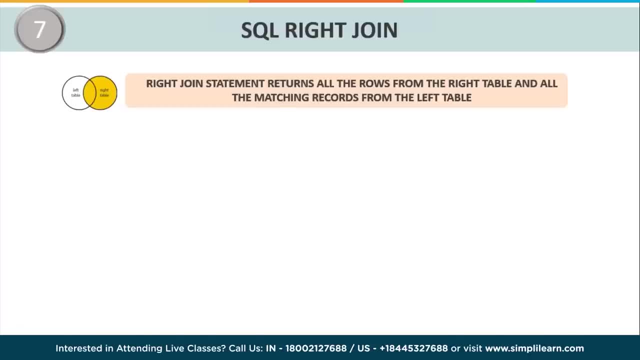 That means it will return all the rows from the right table and all the matching records that are present in the left table. The syntax remains the same, that is, select column list that you want to display in your table from table 1, right join is the keyword we use. table 2: on table 1: dot column equals. 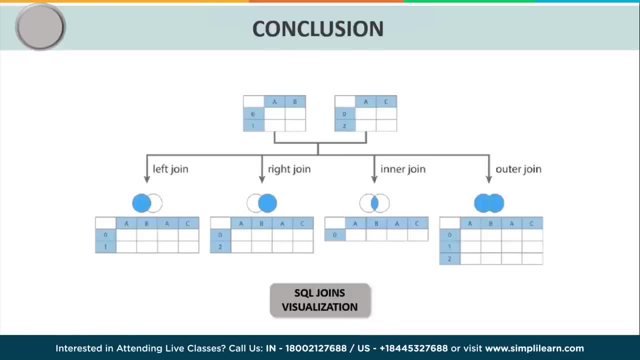 to table 2, dot column. Now to sum up all these different SQL joins and how they work. I've taken a graphical representation of two different tables here which will help us visualize the real time working of SQL joins. Now consider table 1 here, which is columns A and B and records two different records. 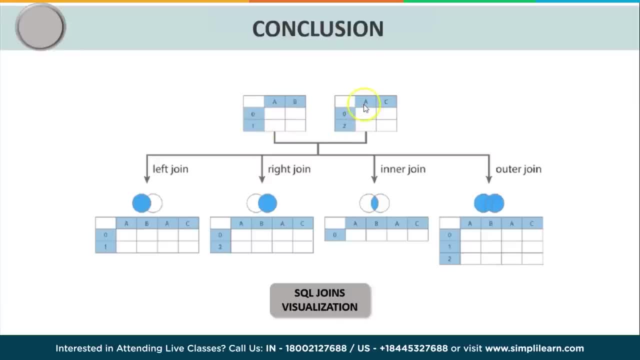 let's say record 0, record 1, and similarly we have table 2 which have columns A and C and two records, that is, record 0 and record 2. now if you apply left join and by the definition of left join, It will only return those values which are present in the left table and the matching 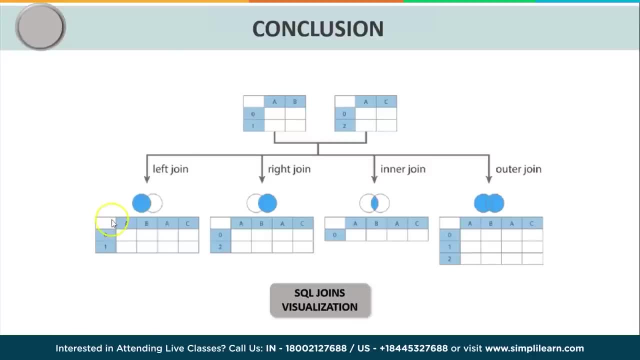 records that are present in the right table. Now, here the matching value that are present in both the tables is 0 and the record values that are present in the left table is 1, and if you consider the right join, it will match the records from both the tables and it will display the only the values from the right. 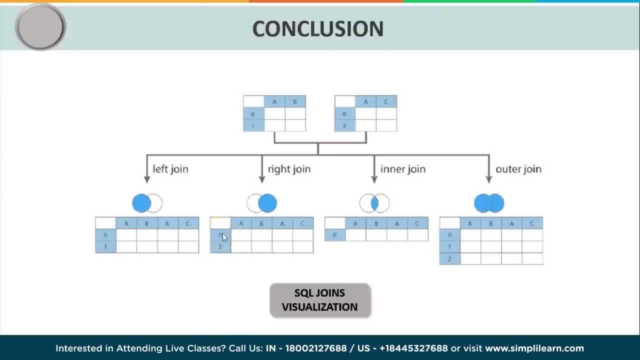 table- That is the reason it is being displayed- the record 0 and the record 2.. And if you look at the inner join, it will match the values from both the tables. Now, the common value that is present in both the tables is record 0, and if you finally, 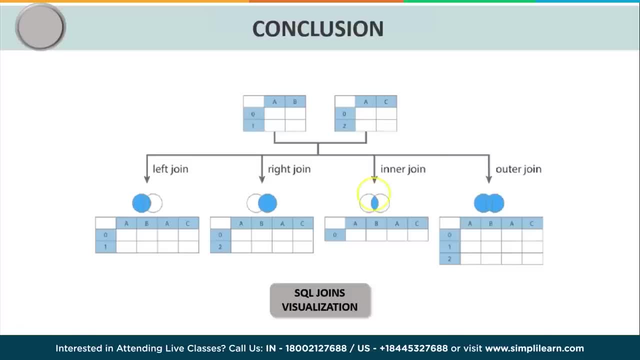 look at the outer join. it will return all the values from both the tables, irrespective if they are matching or not. that is the reason all the records, that is, record 0, record 1 and record 2, are being displayed, and with that we have come to the end of today's session. 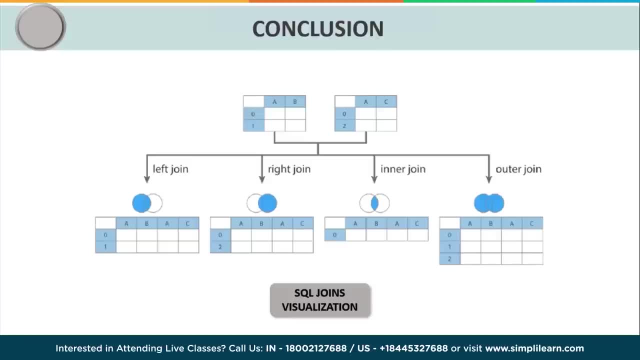 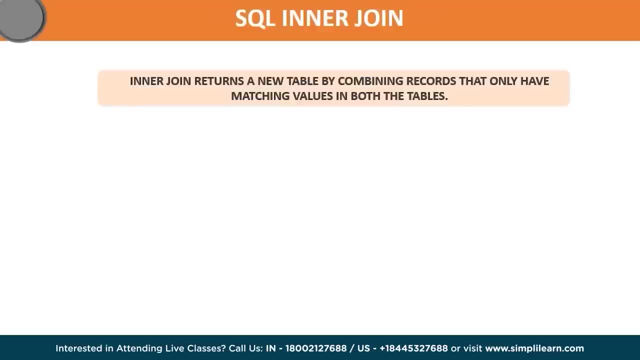 that was all about SQL joins. Stay tuned for more upcoming videos wherein we will execute all these types of joins in mysql workbench using various examples. So what is SQL inner join? Using the inner join, the tables are combined on the basis of a condition also known as. 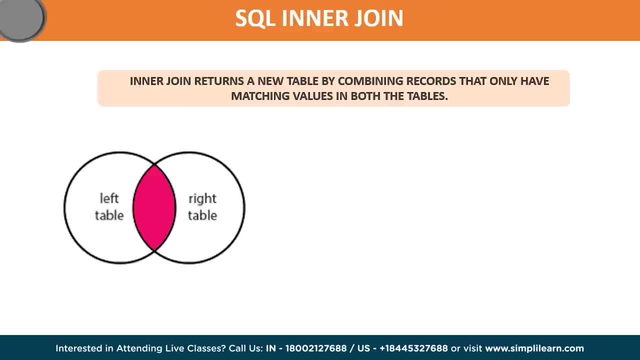 the join predicate. This condition is applied on the columns of both the tables on either side of the join clause. The query checks all the rows of table 1 and table 2.. Now it will display only those values that satisfy the join predicate. 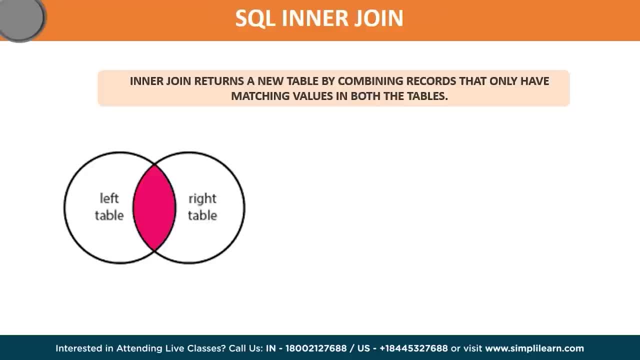 In the resultant table. that means it finds the matching values or the matching records that are found in both the tables. For example, I have a table A which has records 1, 2, 3, 4, and in table B I have records 3, 4. 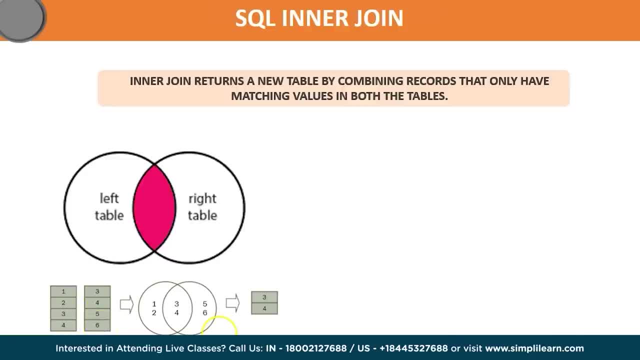 5, 6.. Now, if you join these two tables now, the resultant output will be 3 and 4, because these are only two records that are present in both the tables. that is, the table is matching the common values that are present in both the tables. 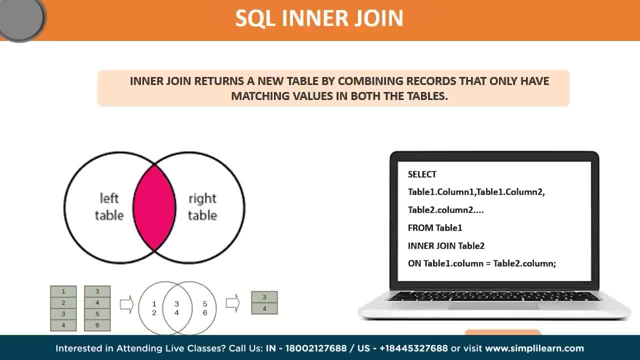 Let us now understand the syntax of SQL inner join. The syntax is followed as: select table1.col1, table1.col2, table2.col2 and so on from table1. inner join is the keyword we have to use. table2 on table1.colum equals to table2.colum. 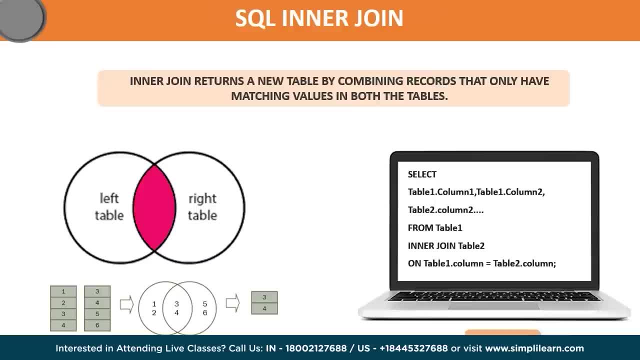 Here, after the join expression, we are mentioning the columns from which we want to match the both the tables. Now that we have understood what is SQL inner join, Let us now understand the syntax of SQL inner join join. let us jump into mysql workbench and execute it with the help of an example. 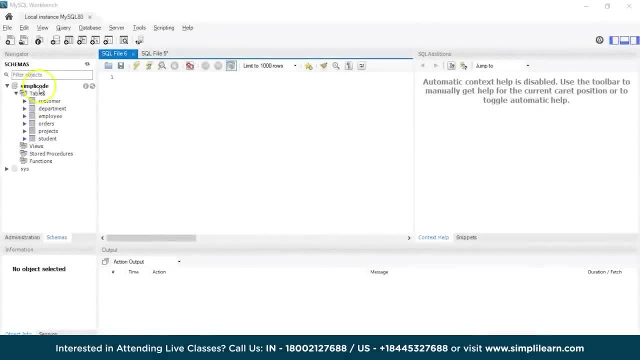 as you can see, mysql workbench has started and on the left side you can see the database. that is simply code and the various tables that are present in our database- simply code. like we have customer table, department table, employee table, order table, etc. now to perform the sql inner join operations we'll use the employee table department table. 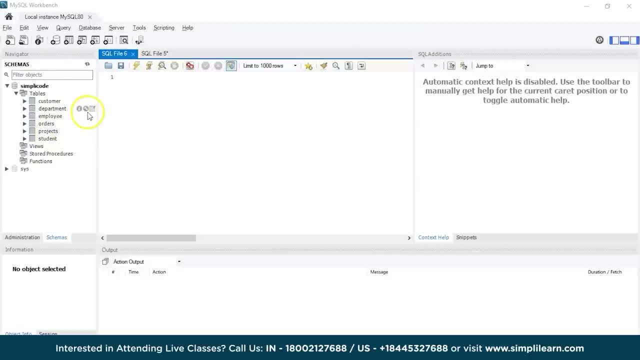 and the projects table. now let us display the values that are present in the table. for that we have to use the select statement or you can directly click on this table icon here. so first let us display the values present in the employee table. the employee table has the: 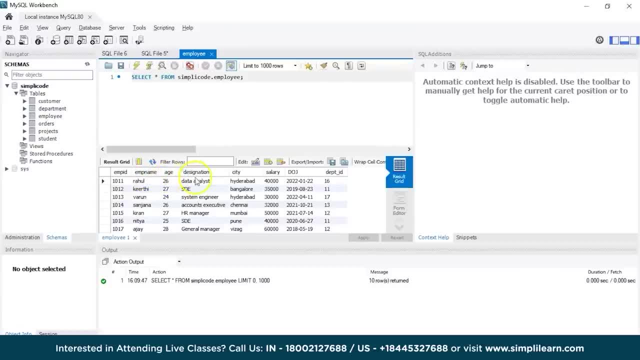 following fields, such as employee id, employee name, age designation, the city they belong to, salary, date of joining and their department id. next, let us display the values that are present in the department table. the department table has two fields, that is, department id and department name. and finally, let us display the values present in the projects table. the projects table has 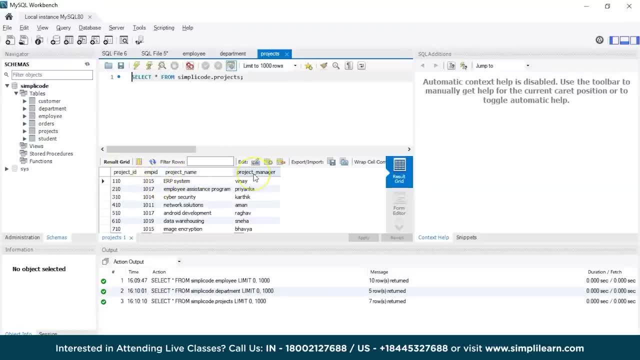 the project id, employee id, the project name and the project manager. now, let's say we have a query here which says to retrieve the employee details and the department they are working in. now, before we write a query we have to check, uh, for all those tables in which these informations are present in. 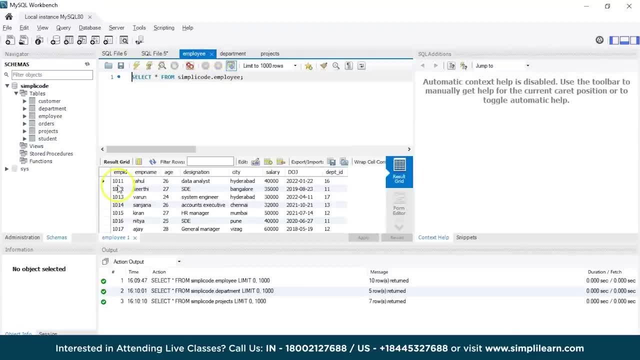 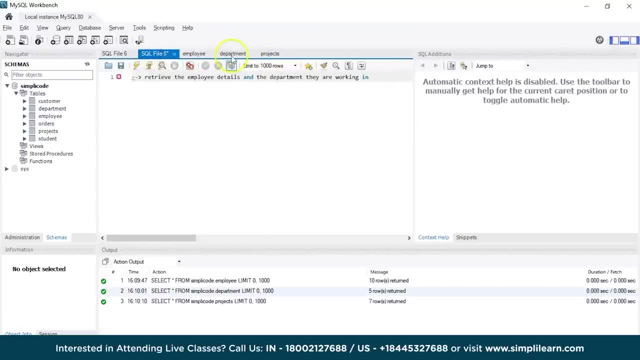 for example, i can get the employee details from the employee table, such as their employee id, employee name, the designation, such salary and so on, and also i can get the department details from the department table. now the expected uh query or the resultant table is based on these two tables. now, in order to 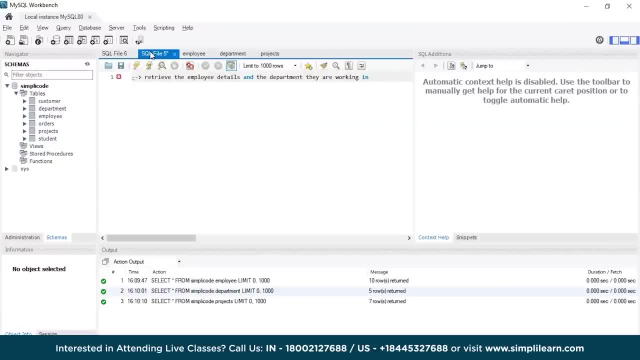 retrieve the records from these two different tables. i need to uh connect them. in other words, we have to join these two tables. this is where the inner join comes into picture. with the help of inner join, we can connect these uh two tables and we can retrieve all those matching records from those tables. now the following: 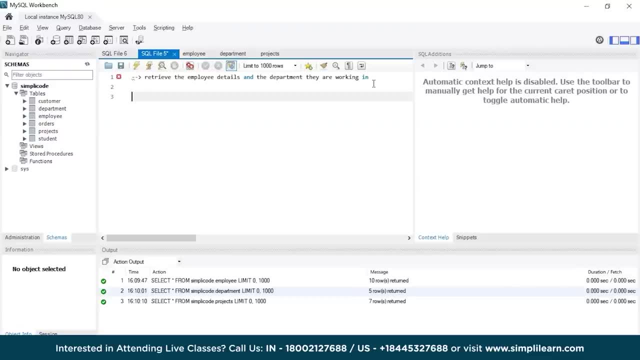 query uh would be for the inner join is select mention the column names that you want to display. now i want i'll display the employee id, so employee dot. employee id. i'll also display the employee name. so employee dot. employee name. i'll also display the employee designation. 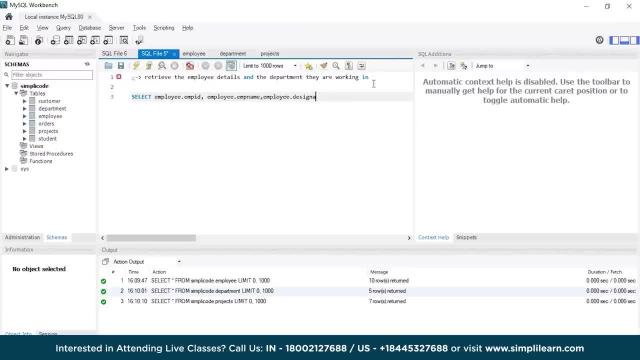 so i am taking employee dot designation now. i'll also retrieve the information from the department, so i'll have to mention the department table here as well. so department dot, department id. right now the query is continued as from the table table one that is employee. i'll just write in the next cent, uh, next sentence from employee. 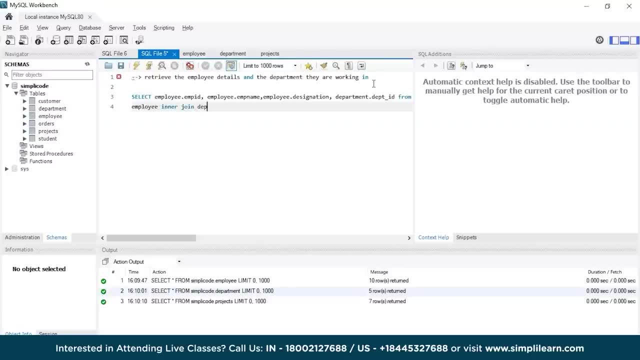 inner join is the keyword we have to use here, and mention the second table, that is, department on, which is the keyword, and mention the condition on the basis of which you are connecting these two tables. now i'm connecting the employee and the department table with the with the help of the department id, so i'll mention employee dot. 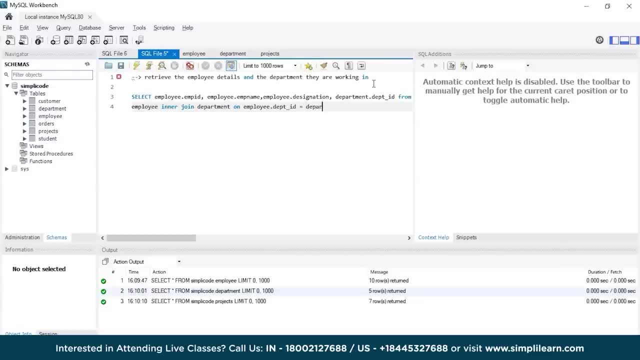 department id equals to department uh dot department id. so let us now execute the statement and see the output. so, as you can clearly see, it is displaying the values of employee id, employee name, the designation and the department id as well. now as you clear clearly, you can see that the join condition is specified in the inner join clause. 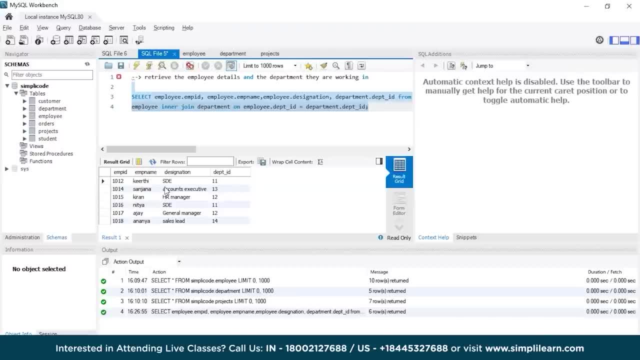 after the on keyword uh as the expression. now, for each row in the pr uh in the employee table, the, the query finds a corresponding row in the department table that has the same matching values, based on which we have mentioned here. that is the department id. now, if there is, 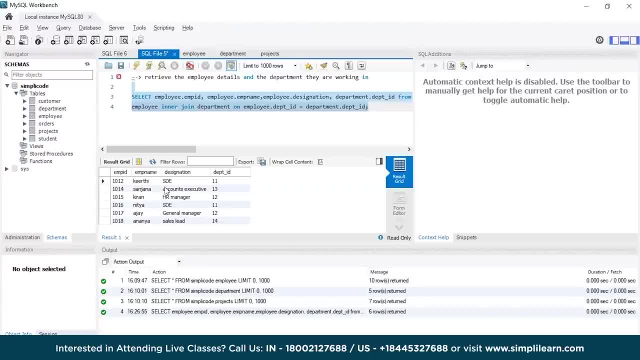 a match between two rows in both the tables. it returns all those rows that contains columns that we have specified. for example, we have specified employee id name, designation and the department that they belong to. so in this way you can use the inner join to get the records from both the tables. also, you can get the department name as well by mentioning 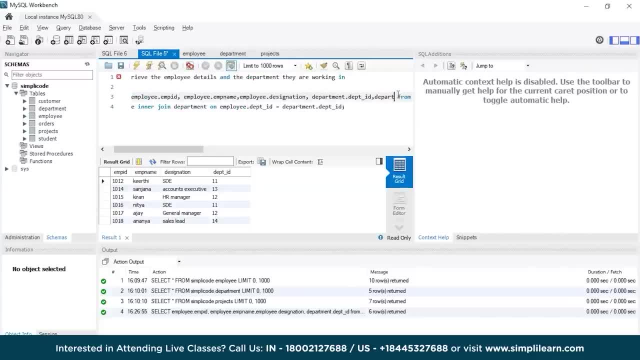 the department names in the query. the department name, department dot, department name- now this will display are the records of the department name that are present in the department table as well. so, as you can see, there are total of six records: the employee details and their department names that they are working in, and also if 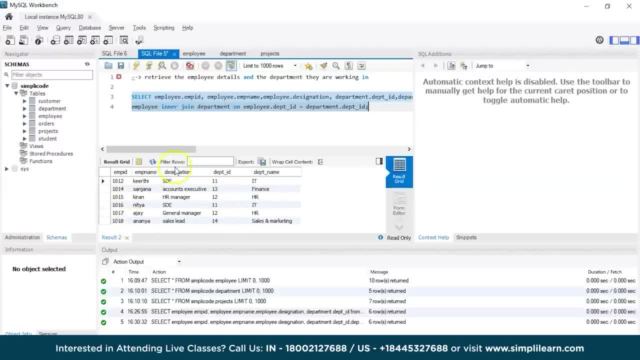 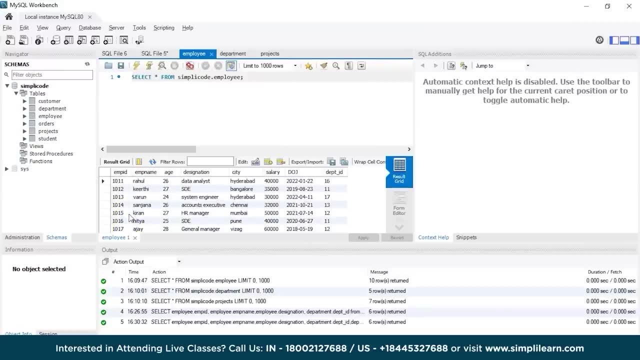 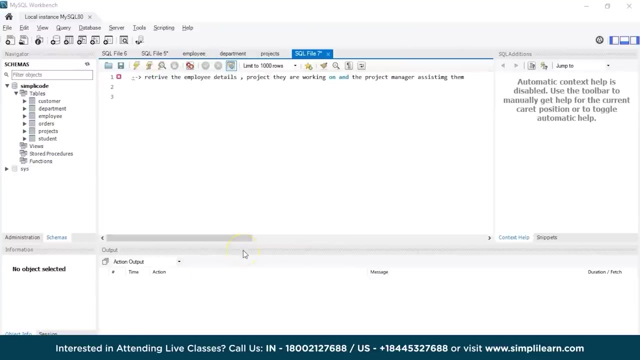 you notice, there are only six records that are present in our resultant table, when we have a total of 20 records that are present in the employee table. that's because the inner join only matches those records from those columns that are having matching values from both the tables and also the condition that we have specified in our inner join statement. 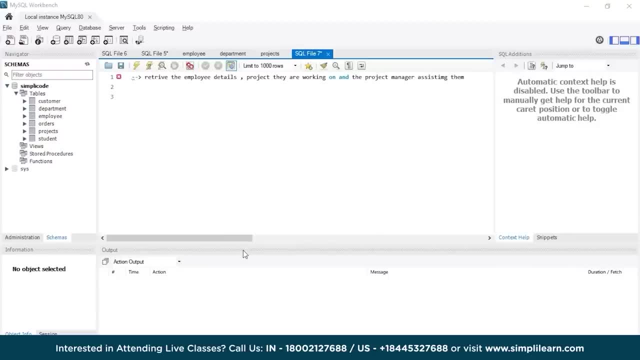 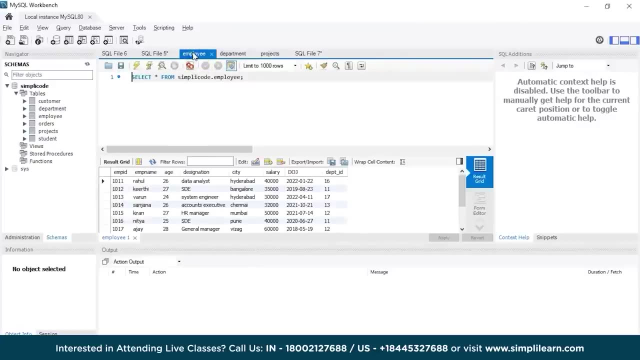 Finally, let us look at another query, which is to retrieve the employee details project they are working on and the project manager assisting them. Now for this, to get the employee details again, I'll again use the employee table. and to get the details of the project name and the project manager's name, I'll use the project table. 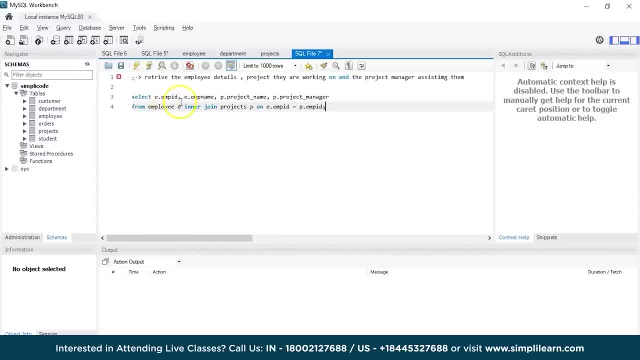 So the following query would be: select E, dot employee ID. Now here I have taken the alias name for the tables, that is, you can mention a temporary name for the tables that you have chosen. So for employee table, I'm taking as E and for projects, I'm taking as P. 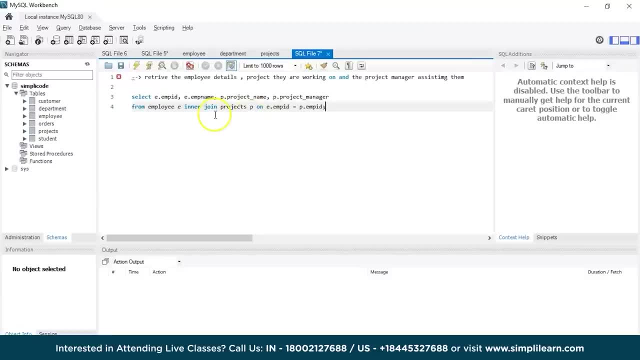 In order to save time, we'll write in this way, so the query is followed as: select E dot employee ID. E dot employee name. P dot project name. P dot project manager. from the first table, that is, employee E inner join projects. we have taken the name as P on E dot employee. 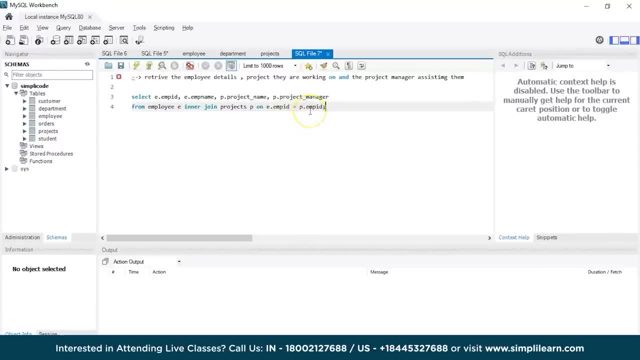 ID is equals to P dot employee ID, which is the common column from which the employee name is being entered. we get the matching values from both the tables. let us now execute uh the statement and see the output. so, as you can see, we can, uh we are able to retrieve the employee id. employee name project. 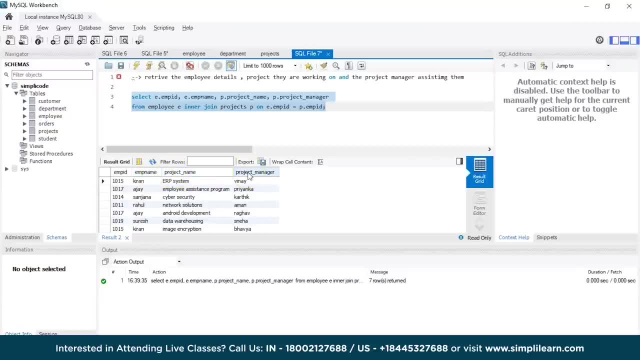 name that the employee is working on and the project manager that uh have been assigned to these employees. and if you notice uh carefully here, like some of the employees who are having employee id like 1000 and 12, 1013, 1008, 16, there have no project names assigned to their uh to their. 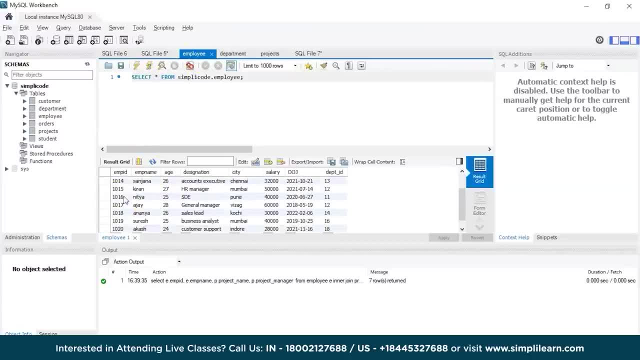 names that this is because, even though we have all the details of employees, uh, in the employee table, we do not have the data that that is being stored in the projects table. that is the reason. uh, only a limited number of records are being shown and, as per the definition of inner join, it will. 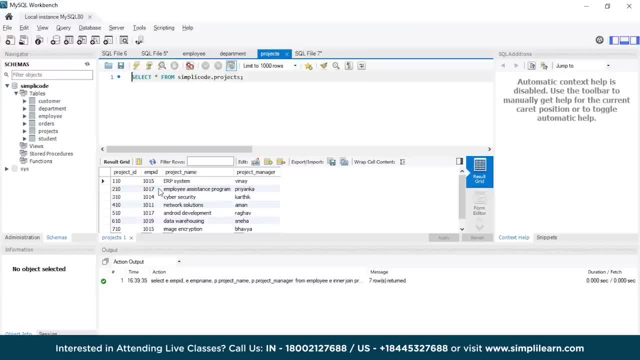 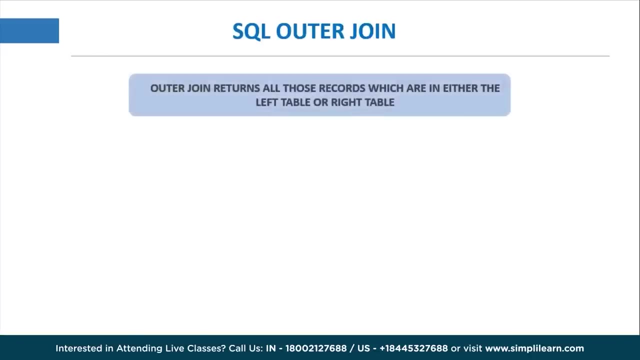 fetch only those records, records which have matching values from both the tables. so in this way you can join two or more tables using the inner join statement, and with that we have come to the end of today's session. that was all about into the execution part. let us just quickly discuss what is sql outer join. 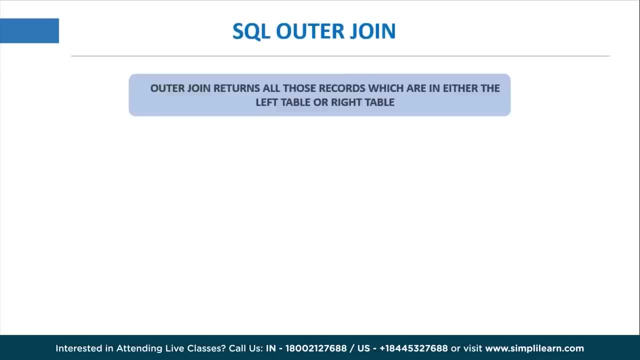 the outer join statement returns all those records which are present in either the left table or the right table. now, for example, if you consider the table here a, which has records 1, 2, 3, 4, and the table b, which has records 3, 4, 5, 6, now if you apply the full outer join to these two tables, it will 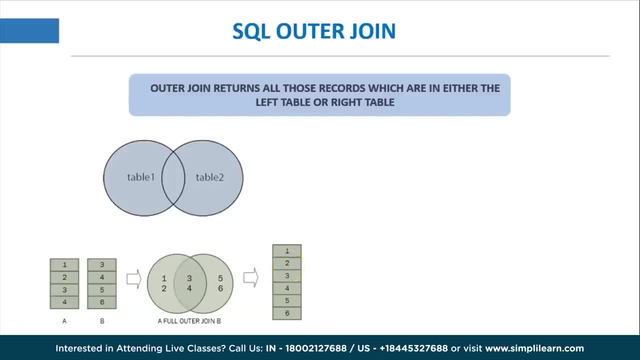 display all the records, that is, 1, 2, 3 and up to 6. now let us discuss the syntax of sql outer join. the syntax is followed as: select table: 1.column 1, table 1.column 2, table 2.column 1 and so on. 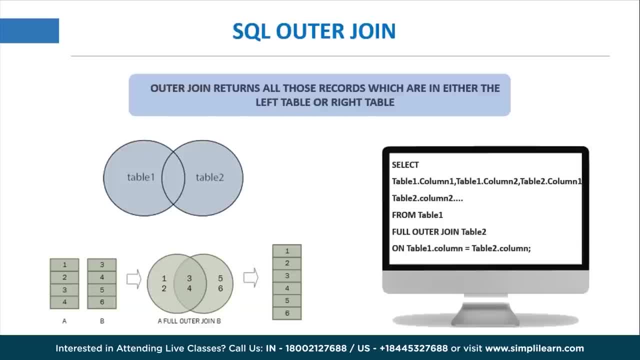 these are basically the columns that you want to display in your resultant table from table 1, full outer join table 2 on table 1.column equals to table 2.column. now, as far as mysql is concerned, this syntax is not applicable now if you are working on other databases like postv sql and microsoft sql server, 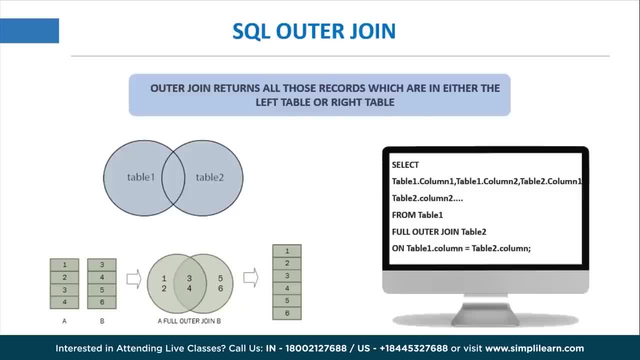 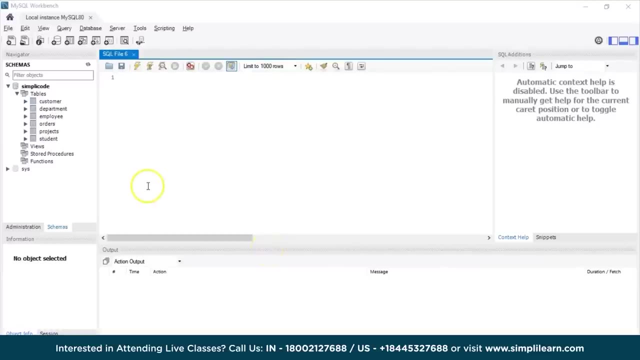 you can apply this syntax, but if you are working on mysql workbench, there is a different syntax, which i'll be discussing in a while. so now that we've understood what is sql outer join, let us jump into mysql workbench for the execution part. as you can see, mysql workbench has started and on the home page on the left side you. 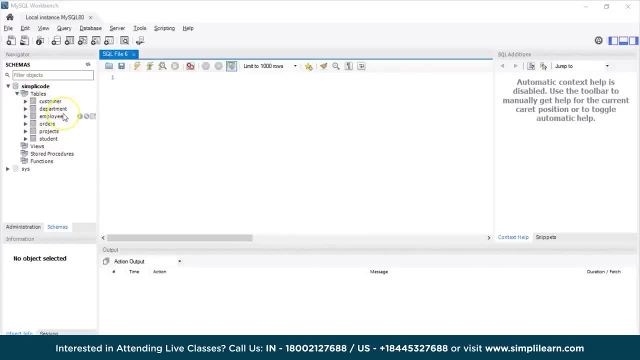 can view the databases and tables now. i've created a certain tables time for time being, so let me just display the values that are present in these tables. now, in order to execute the mysql outer join, we'll consider the employee table as well as the project tables, so let me just display the. 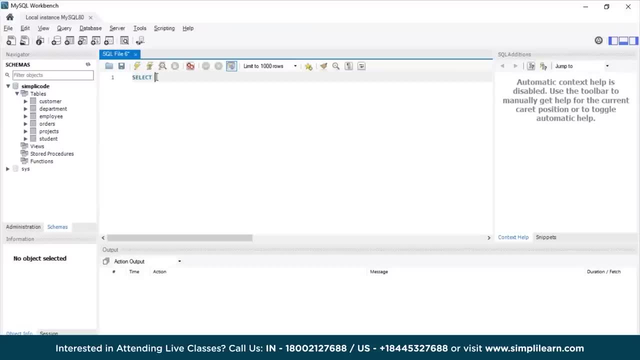 values present in the table, and i'll be doing that in a while, so let me just display the values present in the employee table. i'll use the select operator to display those values. select star from employee, so it will display the records of all those employees having 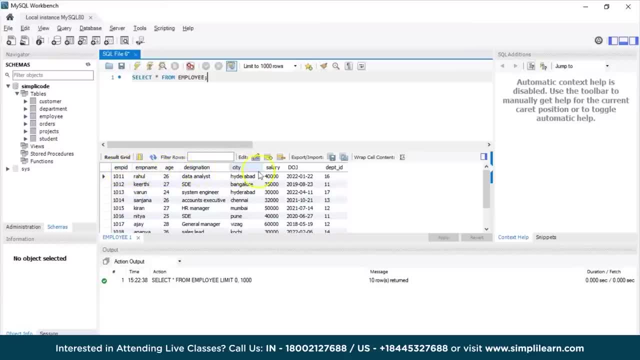 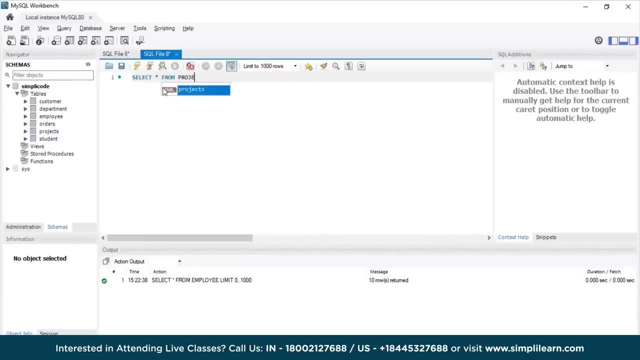 employee id: employee name, age, their designation, city, salary, date of joining and their department id. now, similarly, i'll display the records of projects. let me just take another tab. i'll use again the select statement to display the records star from projects. now, if you execute this statement, it will display the uh project id. 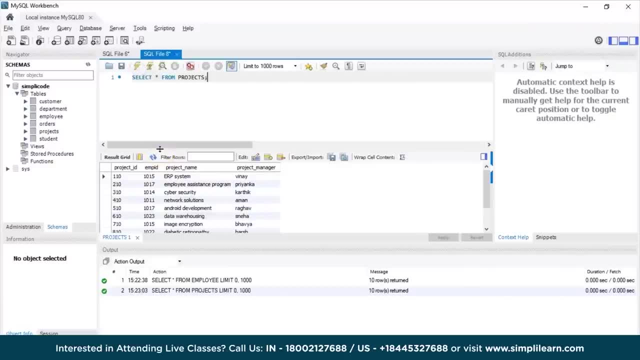 employee id, project name and the project manager details. now, let's say, if I want to fetch the details of all the employees from the employee table and the project details they are working on from the projects table, i'll have to use the full join to retrieve information from both the tables. now, as discussed earlier, the full outer join keyword is not applicable to mysql workbench. 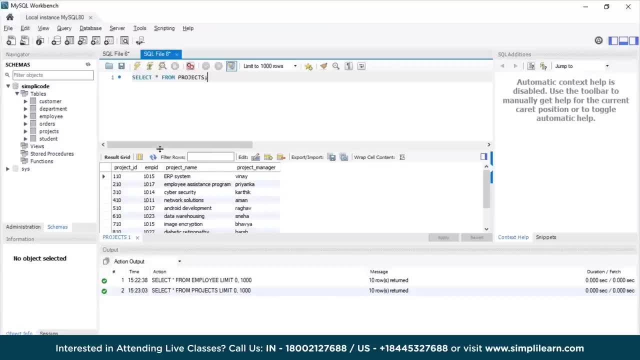 to MySQL database, So I'll have to implement a new logic here, which is quite simple. As you know, the full outer join is the result of combining the left and right table, So we'll first use the left join, then we'll use the right join and finally we'll use the. 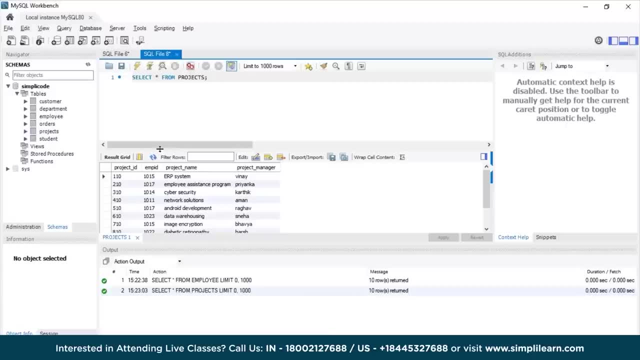 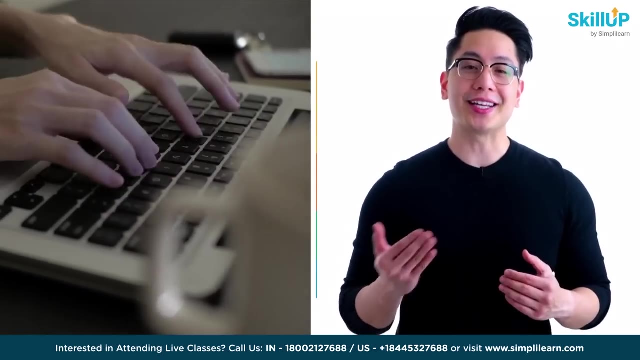 union operator, which is used to combine the resultant set of two or more select statements and execute it in a single statement. By the way, we haven't executed left and right join yet, so stay tuned for the upcoming videos on both these joints as well. If getting your learning started is half the battle, what if you could do that for free? 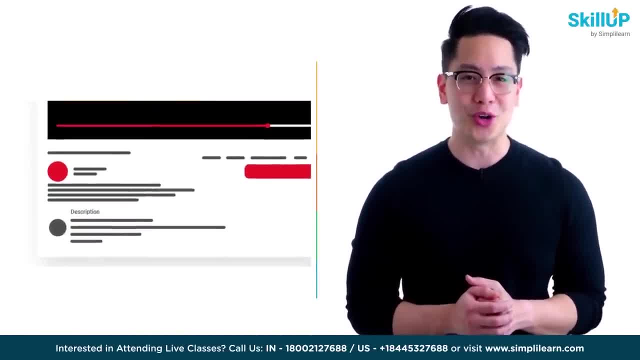 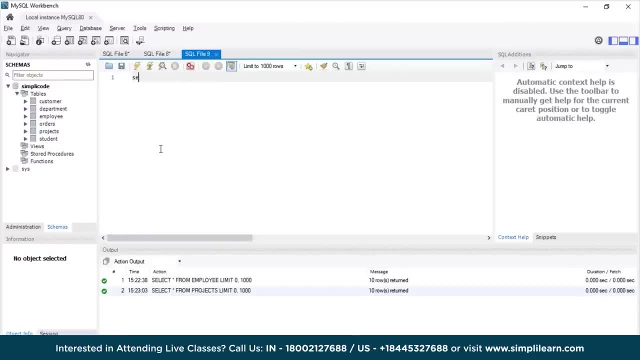 Visit Skillup by SimplyLearn. Click on the link in the description to know more. So the following query would be: let me just take another tab again. So the following query would be: select, now mention all those column details that you want to display in your resultant table. 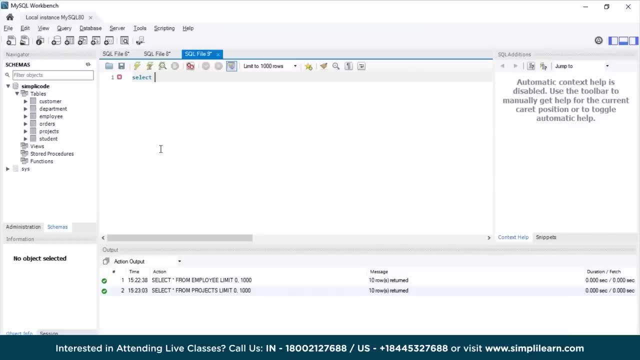 So I want to display the employee ID- employee name, project name and the project name Managers name as well. So you have to mention the column names in the format of table name dot column name. So I'm taking the alias name for the employee table as E. 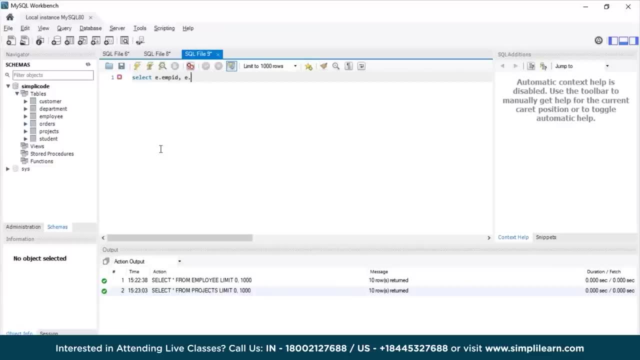 So E dot employee ID. comma E dot employee name. Now for the projects table. I'm taking the alias name as E So P dot project name: E dot project name: E dot project name. Comma P dot project manager's name From the table that is project tables. sorry, the first table is employee right. 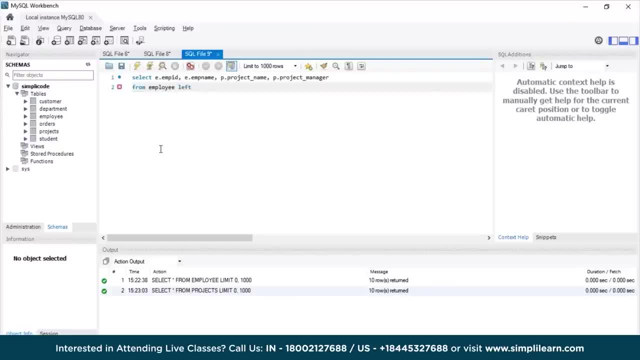 So we'll mention the employee. Now use the left join keyword, Left join on projects On. now you have to mention the condition On On the basis of which you are connecting these two tables. Now, if you look at the two tables, we have the employee ID that is present in both the 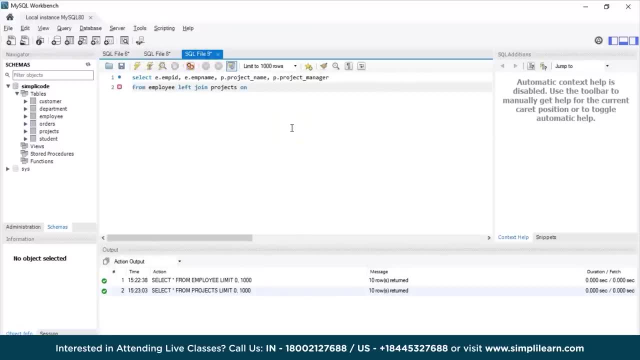 tables. So that will be the common attribute to specify this condition here. So E dot employee ID equals to P dot employee ID. Now I'll just copy paste this same statement. Okay, And instead of using the left join, I'll use the right join keyword. 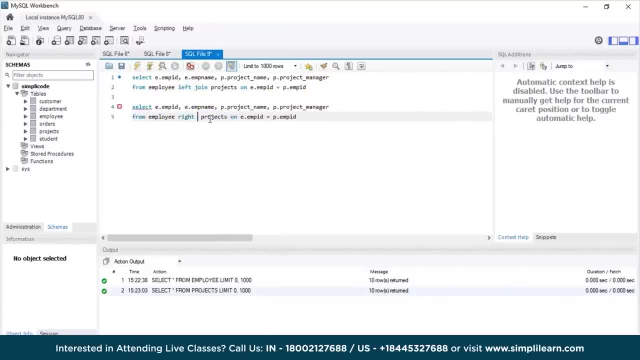 So let's just replace the left join keyword with the right join And I'll mention the union operator keyword to join these two tables. So that's it, guys. This is how you can use the full outer join in MySQL Workbench. Now let us just execute this statement and see the output. 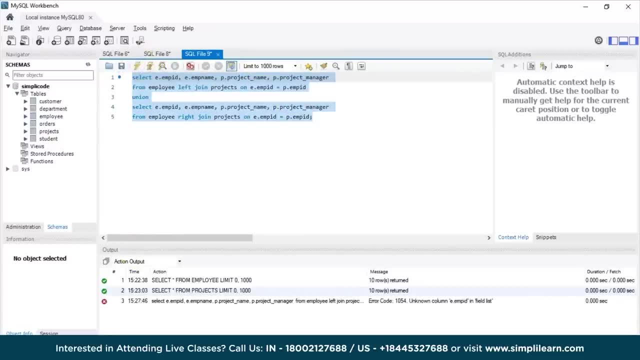 So there's a bit of error. So there's a bit of error. So there's a bit of error. Let me just check it once. So I forgot to mention the alias name here for both the tables, So that is why it is throwing an error. 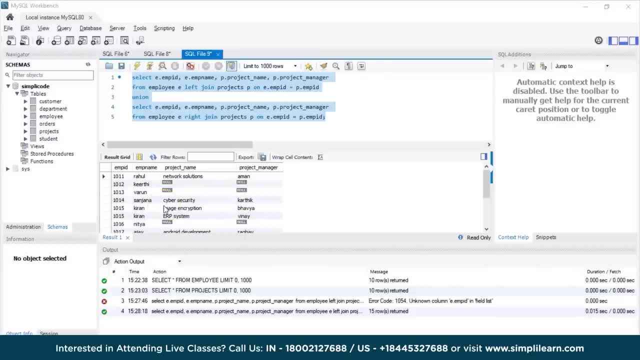 So, as you can see, this is our output and you can clearly see that the record from both the tables, that is, the left table, which is employee, and the right table, which is projects, are being displayed here Now, unlike the inner join which only fetches those records which have matching values in. 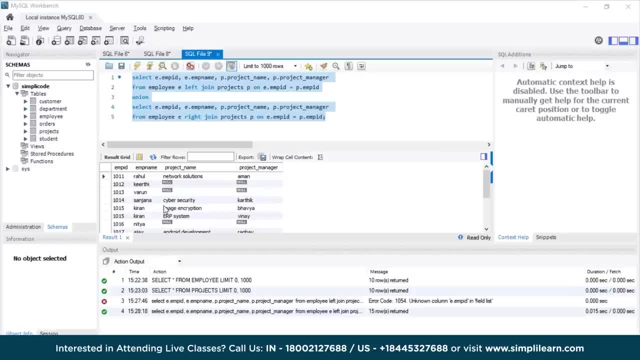 both the tables full outer join retrieves all the values, irrespective of whether they are matching or not. For instance, if you look at the employees having employee IDs here- 1012,, 1013,, 1016 and as well as 1018,, we have their information present in table 1, that is the employee table. 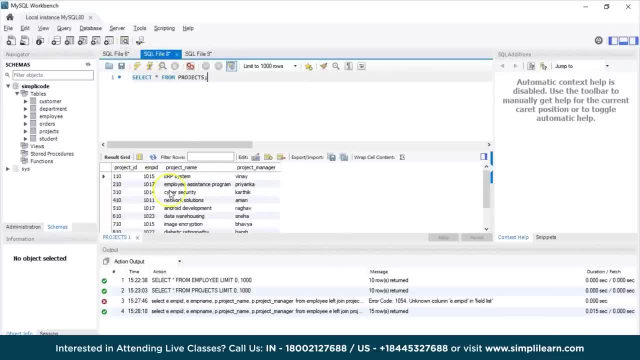 here, But we do not have their information in the projects table here. And similarly, employees having employee IDs like 1022, 1023 and 1024, their information is present in the projects table But it is not present in the first table. that is employee. 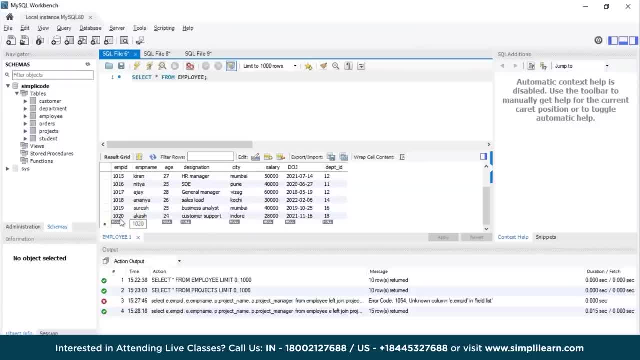 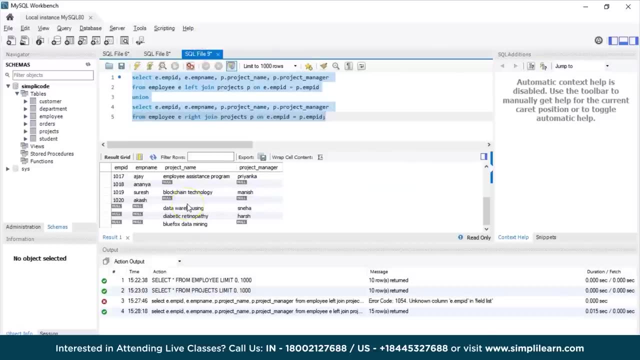 You can see only the employee details having their employees ID up to 1020 are being displayed in the employee table. Also, if you notice the resultant table here, guys, some of the employees like Kirti, Varun and Nitya have no projects assigned to their name. 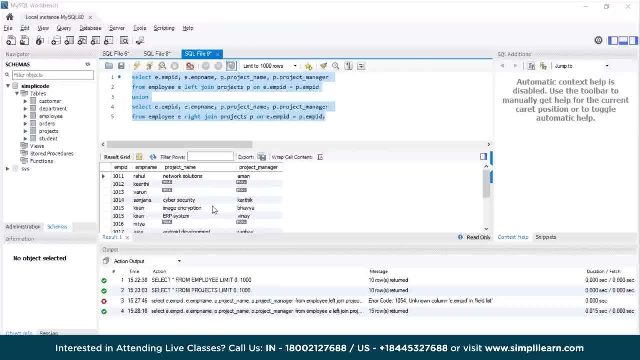 That's why we have null values in the project name column. That's because Their records are present in the employees table but their employees IDs are not present in the project table. That means all these employees are yet to be assigned a new project. 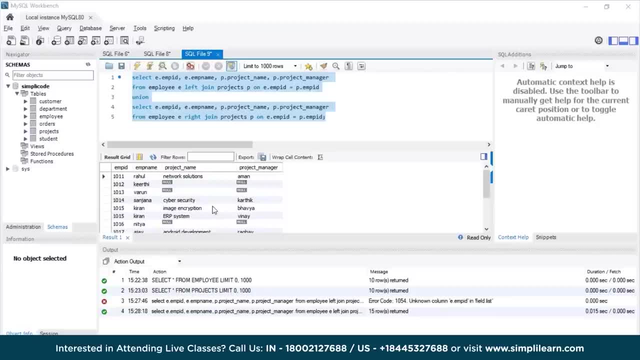 So if the values present in both the tables that does not match, it will simply just return null values. Similarly, we can see the other three projects that are present in the table, but there is no sign of employee details here, be it their employee ID or employee name, and it will. 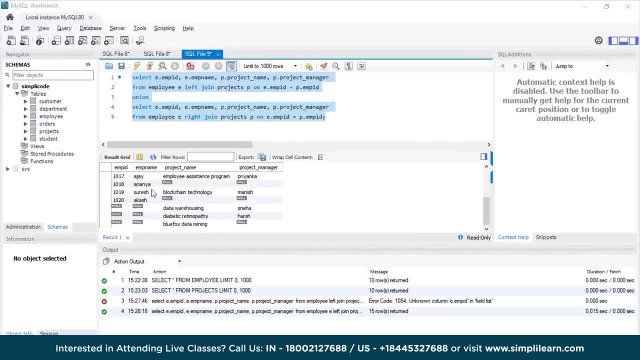 just simply return the null values again here, Because The employee information in the first table employee, even though their IDs are mentioned in the project table and hence it will only return null values. Now suppose this is just a demo table having around 20 or 25 records, but if you consider 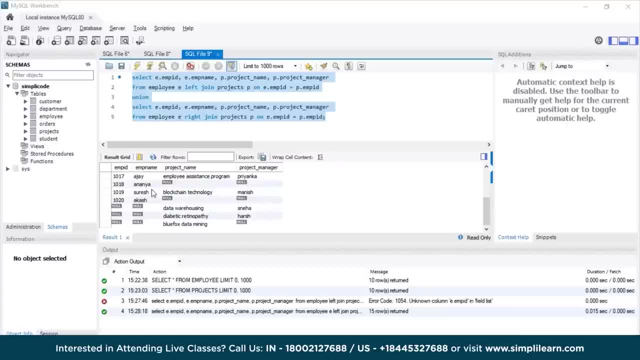 a company's database. in real life, it will have thousands of records. in order to access and manage various database tables and fetch information from those tables all together, It becomes quite difficult, right? So this is why we use full join to connect The tables and retrieve each and every information from them. 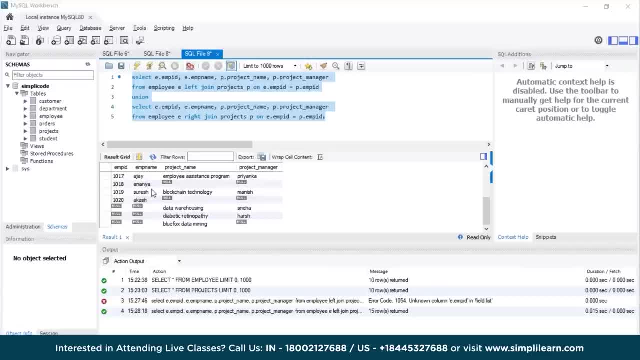 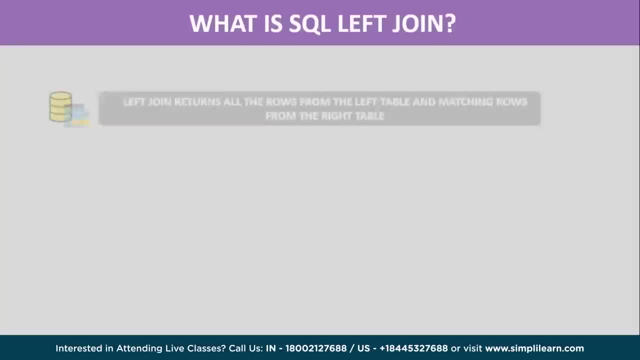 And if any column has null values, they can just simply update those rows or even delete them as per the required. Let's just have a quick recap on what is SQL left join, So SQL left outer join, also known as left join, results in a table containing all the 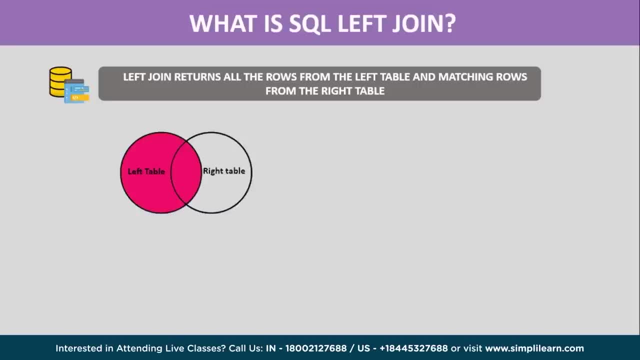 rows from the table on the left side of the join, That is the first table, and only the rows that satisfy the join condition from the table on the right side of the join, That is the second table. The missing values for the rows from the right table in the resultant table of the join are: 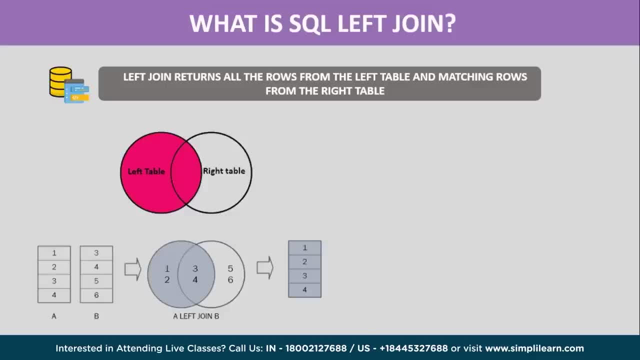 represented by null values. For example, if you consider here two tables, that is, table A and table B, which has values 1,, 2,, 3,, 4 in table A and 3,, 4,, 5,, 6 in table B, 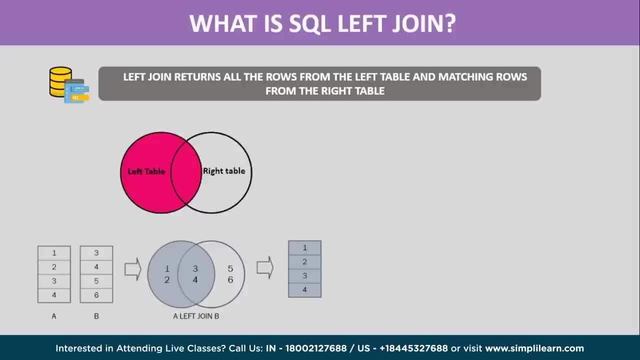 Now, if you apply left join for both these tables, it will display only the values from the left table, that is, 1,, 2, and the matching values from the right table, that is 3, 4.. So the resultant table will be 1,, 2,, 3, 4.. 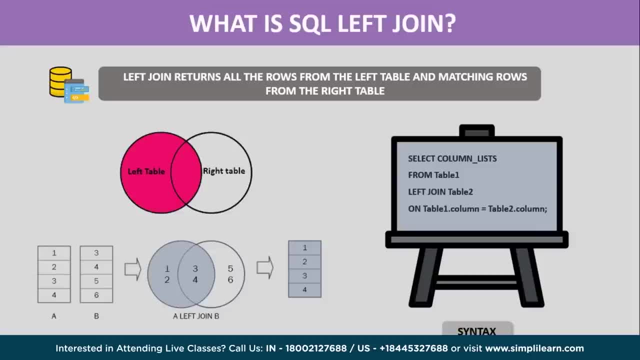 Let us now understand the syntax of the SQL left join statement. The syntax is followed as select column lists. these are basically the columns that you want to display in your resultant table from table 1, left join, which is the keyword we are using. 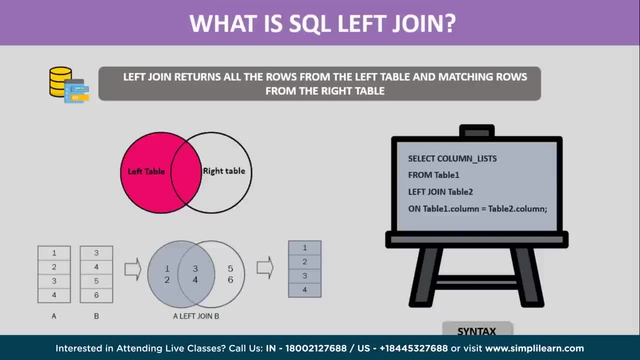 here, table 2 on table1.column equals to table2.column. Now here you have to mention a common attribute on the basis of which you are joining these two tables. As we have already understood about left join, let us know. jump into mysql workbench to execute. 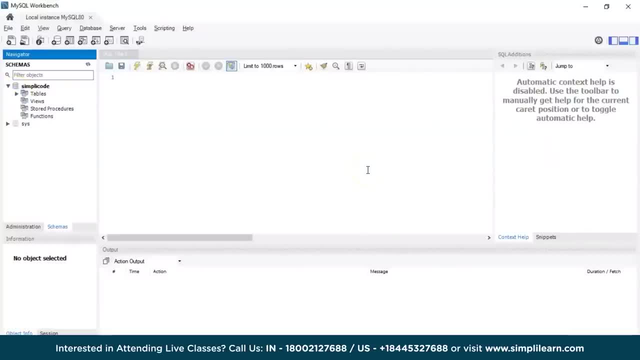 this using various examples. As you can see, mysql workbench has started and on the homepage on the left side, in the schema section, you can view the databases and tables that are present. So in this case we have the database, simply code, and various tables in that, such as customer. 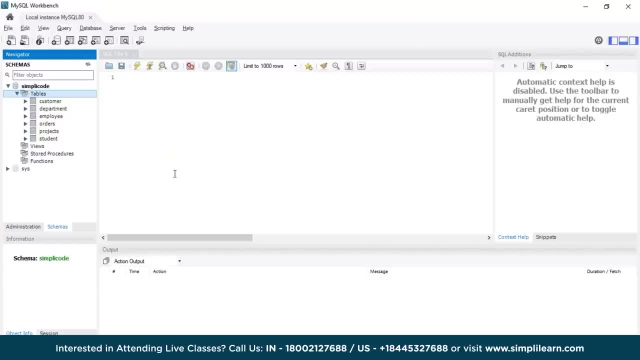 department table, employee orders and etc. Now, in order to execute this, left join statement to use customer and the orders table statement tables. so let me just display the values from both these tables. for that i'll use the select clause, select star from customer, which is the 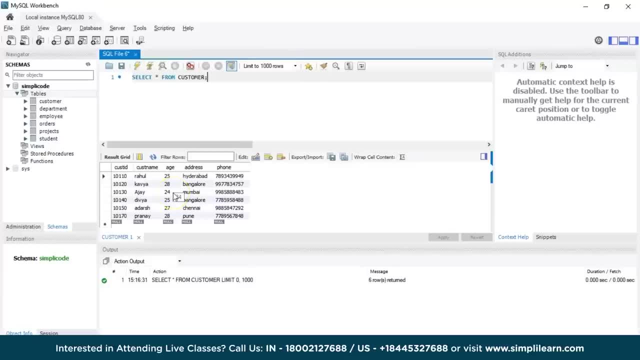 table name. so let us just execute. so as you can see, the customer table has various fields, such as customer id, customer name, age, address and their phone numbers. similarly, let us go to another tab and display the values that are present in orders table. select star from the table that is orders. 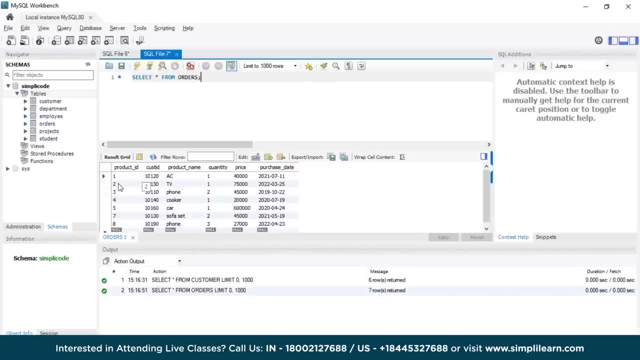 so let us execute the statement. so, as you can see in the output, the orders table has various fields, such as product id, customer id, product name- that is, the product that purchased- quantity, the price of the product and the purchase date. now let's say, if i want to fix the details of all the customers and the product details, that 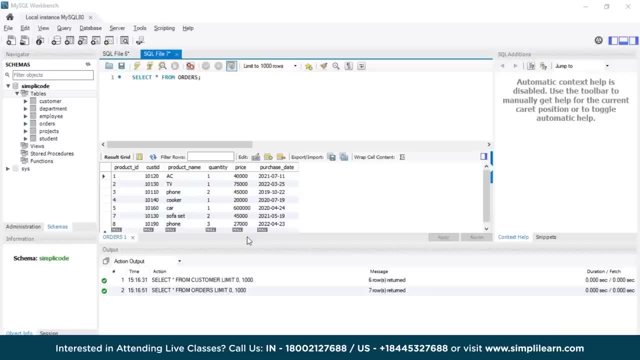 they've purchased. i'll have to connect these two tables, that is, customer and the orders table, to get the resultant table now, for that i'll use the left join statement. so let me just take another tab and execute the statement. so the following query would be: select, mention the column names that you want to fetch in your 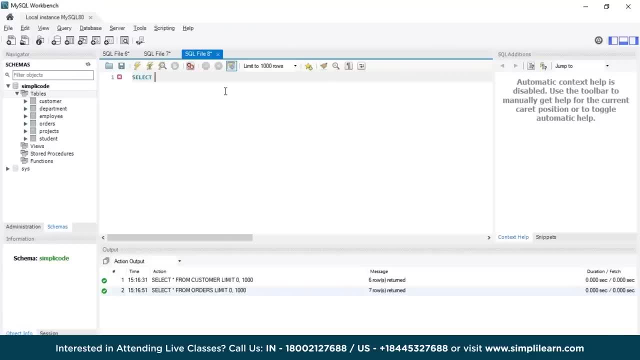 resultant table. so i'm going to take here alia's name, for both the customer and the orders table, as c and o. that's because, instead of writing the full name of the tables each and every time, you can just simply use an alias table to get the resultant table. so let's take the left join statement. so let's. 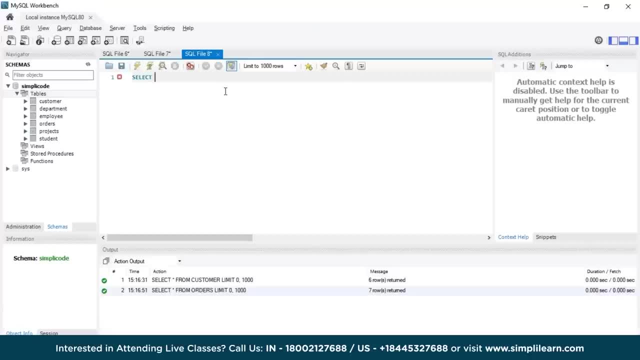 say alias name, which is a temporary name, which will save time as well. so for customer uh table, i'm taking a c so i want to display the customer id, so c dot customer id. i want to display the customer name, customers address, so c dot address. now from the orders table i want to uh mention: 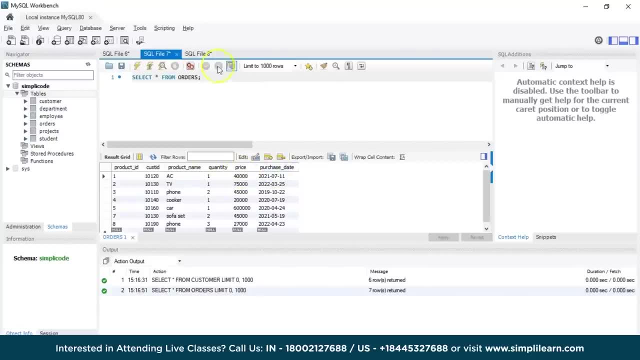 the product's name that they purchased, the quantity, price and purchase date. so we have taken o as the alias name for our table, so o dot purchase name- sorry, product name that they have purchased. i also want to display the quantity, so o dot quantity, it's price as well. o dot price and the purchase date: o dot. 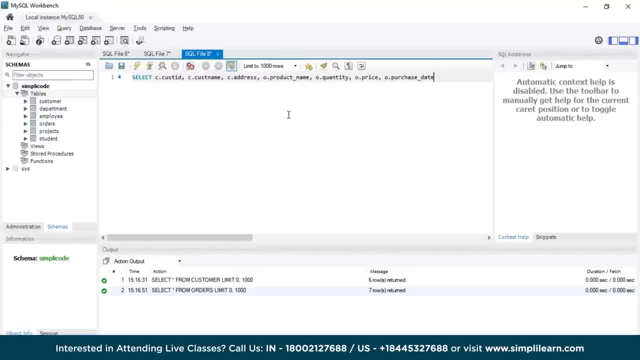 purchase date. from the table first table, that is, customer mention, the alias name c, left join, which is the keyword. on the second table, that is orders o on mention the condition on which you are joining these two tables. so, as you can see, we can find the customer id and. 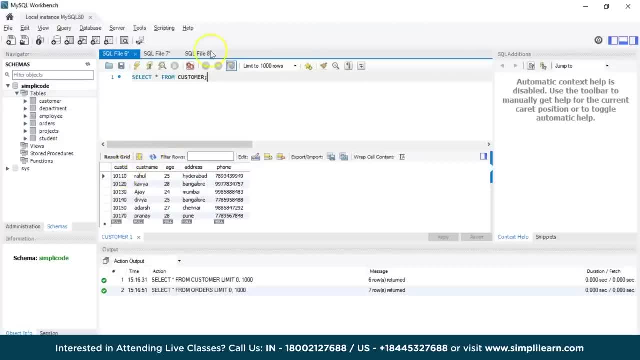 the customer id in both the our customer and your orders tables. so we'll mention the customer id as the column common attribute here. so c dot customer id equals to C dot customer id equals to o dot customer id. so let us just execute the statement and see the output. 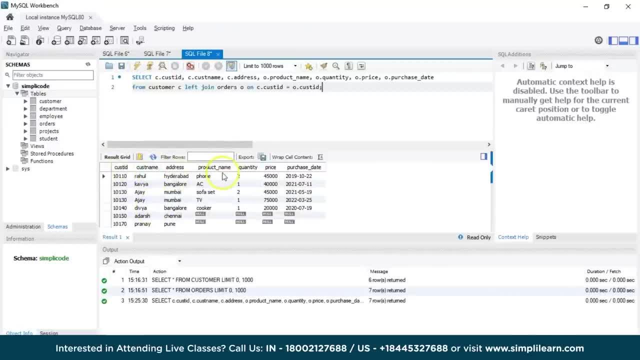 so, as you can see, it will display the customer id, customer name, address, product name, quantity, price and purchase date of the customers in a resultant table. now let us understand what the exactly the left join statement is doing here. firstly, the database checks each and every row of the table and looks for a match in the right table based on the related columns. now, if a match, 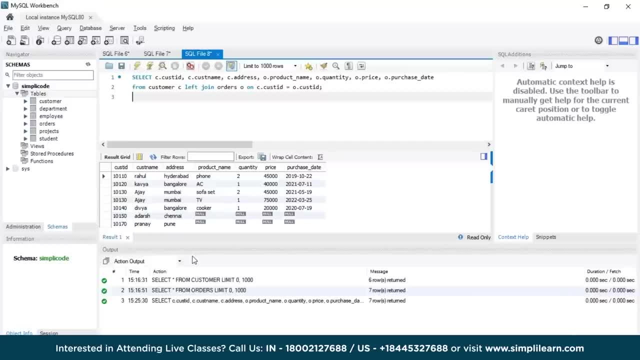 is found, the data from the right table is added to the corresponding row of the left table. now you can see uh customers having customer id 10110, 10120, 10130 and 1013- 140. we have the details present in the first table as well as the second table, that is orders, so it will display all those. 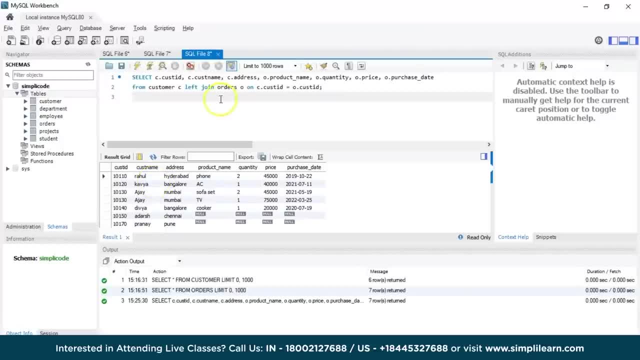 records and then if there are multiple matches- now, in this case, we can see a customer name ajay is having two different records, who has bought sofa set and a tv. so the rows in the left table are duplicated here, that is, the records are repeated in the resultant table in order to 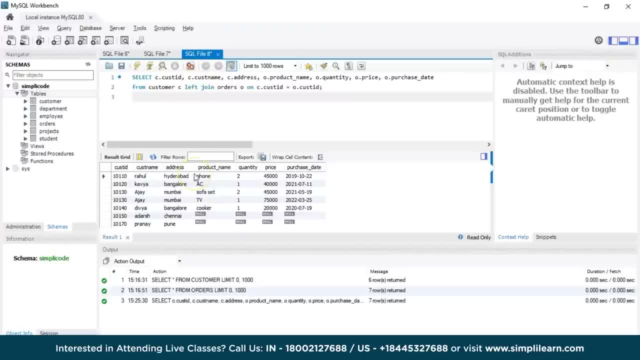 include all the records from the right table. you so now, for all the columns that you have fetched from the right table, that is, orders, which is not satisfying the join conditions, then the values present in the columns will be resultant as null. that means if there is no matching value found from the right table, it will simply retain the. 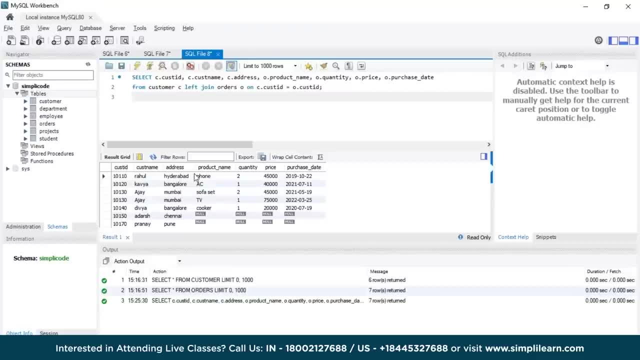 row from the left table and inserts null into the corresponding columns of the right table. now let me just explain this now. if you see here the customer- uh, customers like adarsh and pranay who are having details in the first table, that is a customer table, but they do not have their details in the prod orders. 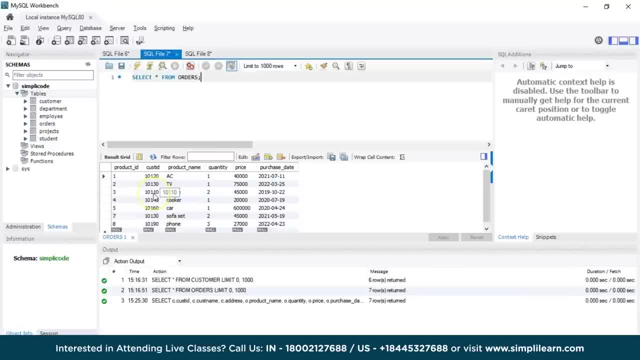 table. so there is no sign of uh any their customer id in the order table. that's why we do not have their uh details present in the uh resultant table, so it will just show the null values here. so basically, left join is a combination of inner join. we can say because: it just checks the matching values from both the tables first and then a fixed valueван is going to get, which is five, in addition to this seniors value as well. that's why we get less and less needs from each other while we do not have any more customer matches. so basically, left joint is a combination of inner join, we can say, because it just checks the matching values from both the now table, which will lively. right can say because it just checks the matching values from both the tables first and, yes, there are the negative freuements data from this resultant table, so that organic jewelry for a product, الخ, and organic shareholders, which are the adj, your winner or gender. 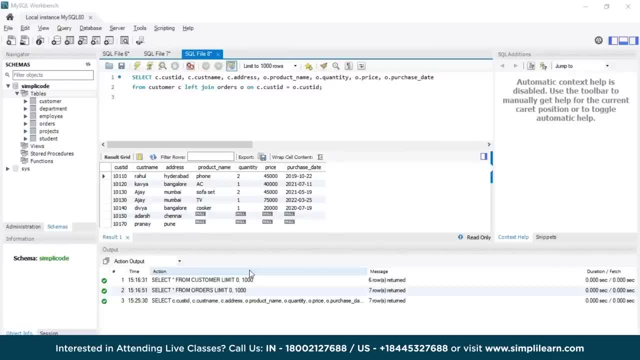 the tables first and then it will check for any additional or extra values that are left out from the left table, that is the table one. now you might have a question that when to use and why to use the left join like there are times when you want to keep rows from the first table that don't have 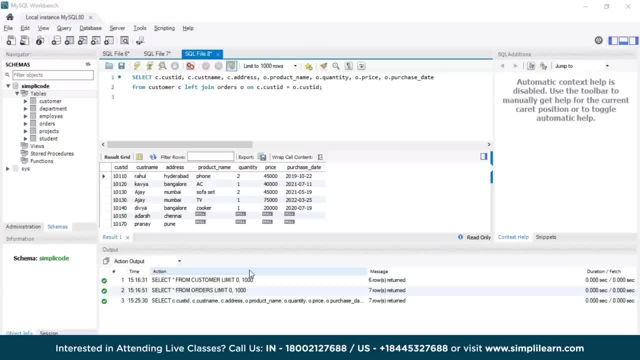 any corresponding records in the second table. now, if you, in this case, if you consider our example, we might want to see information about all the customers in our resultant table, even if they didn't place any orders. so in that case, we'll use the left join, which will be used to combine. 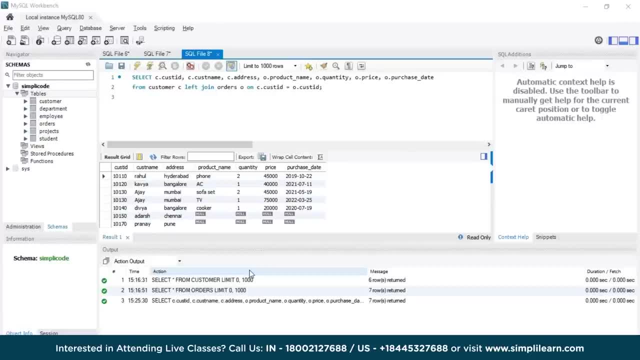 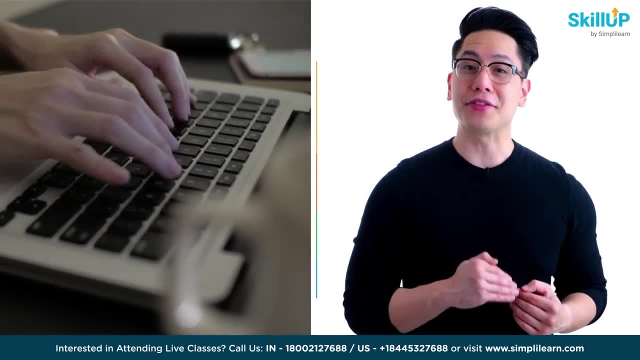 data from two tables so that all the rows from the left table are included in the resultant set, even if there is no matching value from the right table. if getting your learning started is half the battle, what if you could do that for free? visit skillup by simply learn. click on the link in the description. 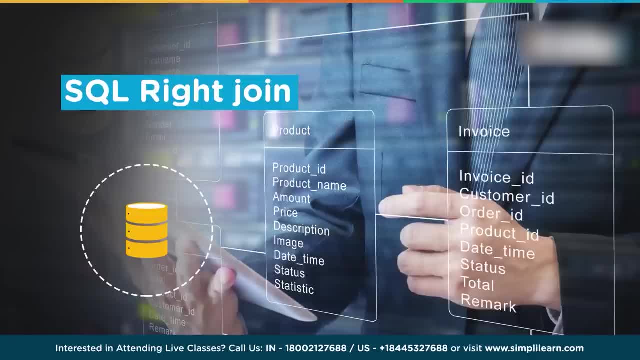 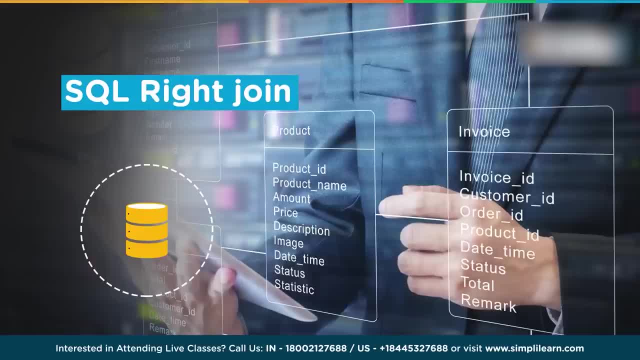 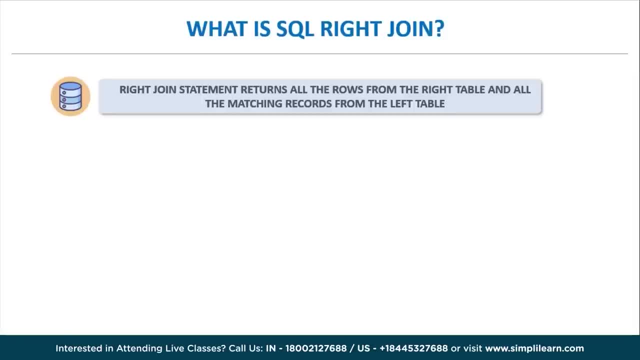 the right table and only the condition satisfying rows from the left table are present in the resultant table. So basically, the right join returns all the records from the right table and only the matching records from the left table are satisfying the condition. For example, let's: 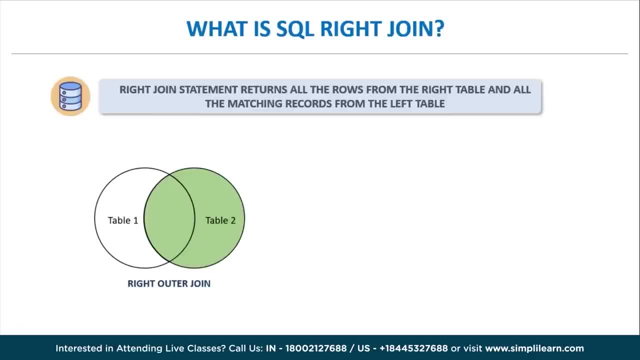 say, we have two tables, table A and table B, and when the left right join is applied to the two tables, it would give all the records from the table B and only the matching records from the table A, that is, table 1.. Let us now look at the syntax of SQL right join. The syntax is same. 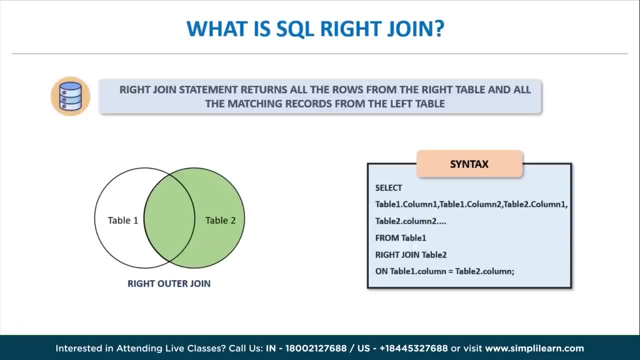 and it is followed as select: table1.column1,, table1.column2,, table2.column1, and so on. These are basically the columns that you want to display in your resultant table, From table1.column1 to table2.column1, table2.column1 to table2.column1 to table2.column1 to table2.column1. 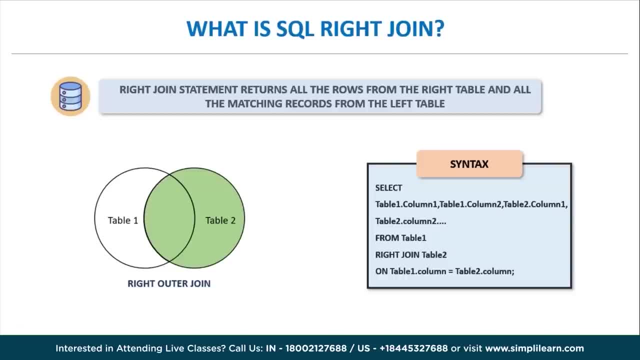 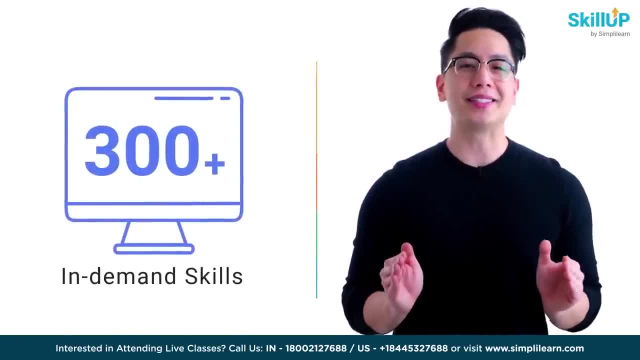 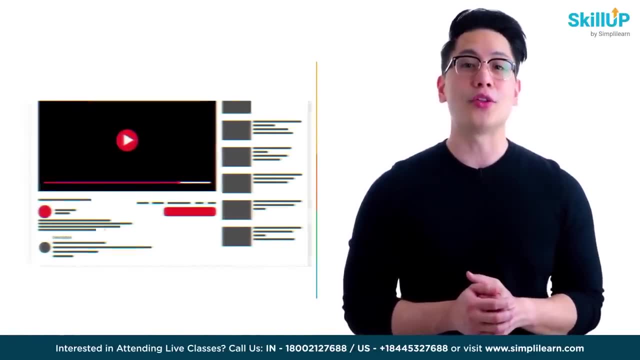 execution. Choose from over 300 in demand skills and get access to 1000 plus hours of video content for free. Visit skillup by simply learn. Click on the link in the description to know more. So mysql workbench has started and on the left side you can view the database. 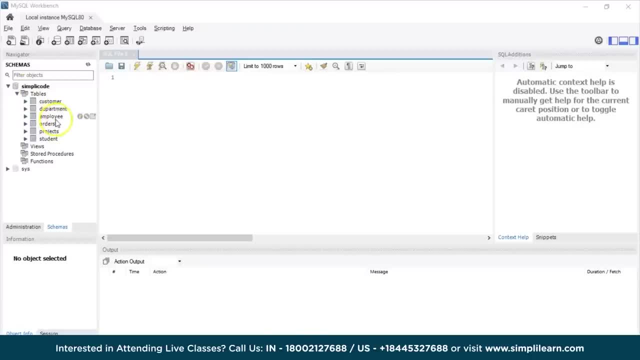 SimpliCode, which has various tables, such as Customer Department, Employee Orders. Now, for time being, I've already created and inserted values into all these tables and in order to execute the SQL write join, we are going to use the Customer table and the Orders table. So let me just display the values that 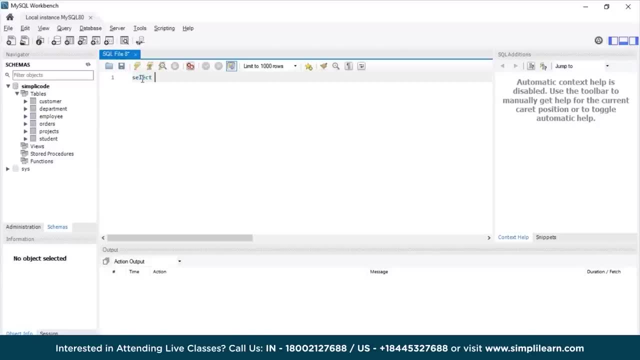 are present in these tables. For that I'm going to use this SELECT statement, SELECT star from the Customer table. So, as you can see, the Customer table has various fields such as Customer ID, Customer Name, their age, their address and the phone number. Similarly, let us just retrieve the records from the 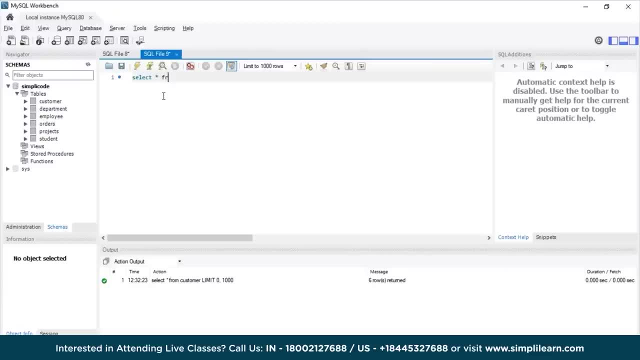 Orders table as well. SELECT star from Orders table. So the Orders table has various columns, such as Product ID, Customer ID, Product Name that they have purchased, Quantity, Price of the product and the Purchase Date. Now, if I want to join the SQL, I can do that by clicking on the button on the right side of the screen. Now, if I want to join the SQL, I can do that by clicking on the button on the right side of the screen. Now, if I want to join, 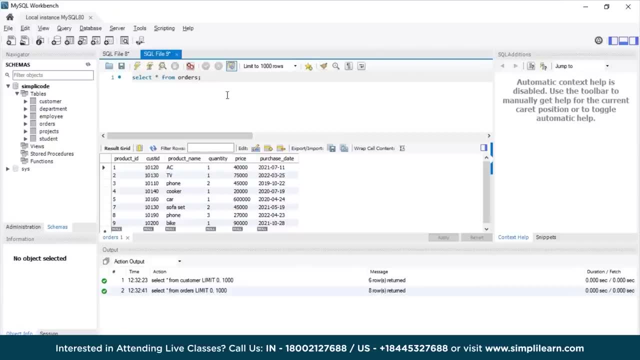 these two tables I am going to use the write join statement, So the following query would be SELECT: Now I'm going to use a alias name for both these tables: For Customer table, I'm going to take as C, and for Orders table, I'm going to take 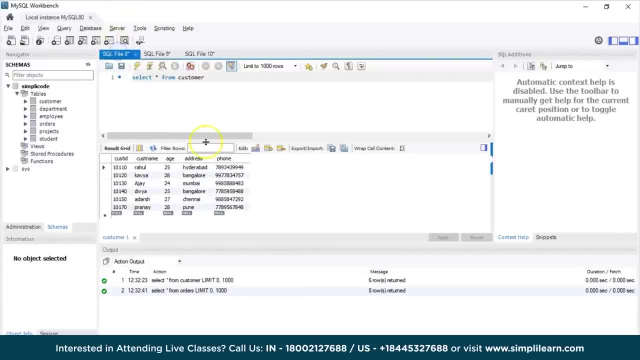 as O. Now I want to display the columns from the Customer table only. So the columns are Customer Name. I want to display their address as well. So mention the column name. Customer Name- CAddress. Now, from Orders table, I'm going to display the. 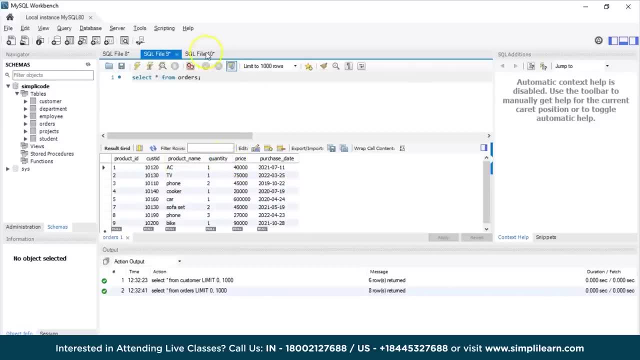 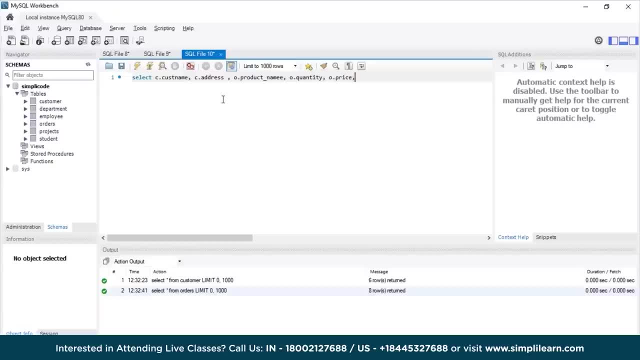 And finally, OPurchaseDate. From the table one that is Customer, mention, the keyword, write, join Mention. the second table name, that is, Orders ON Mention, the condition on which you are joining these two tables now. Now, as you can see, we have Customer. 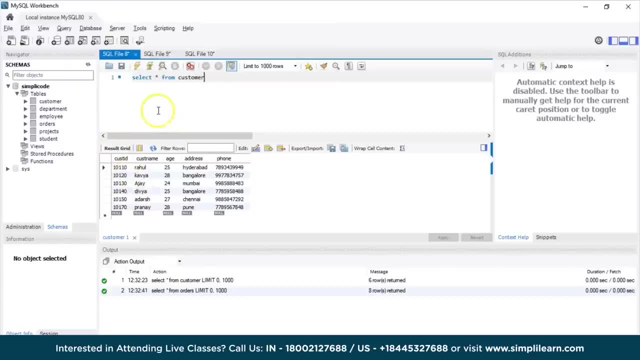 ID as well as the Customer ID present in both the tables: Customers and Orders. So we'll be taking the Customer ID here, as the common column On CCustomerID equals to OCustomerID. Let us now execute the statement and see the output. So there is just an error. Let me 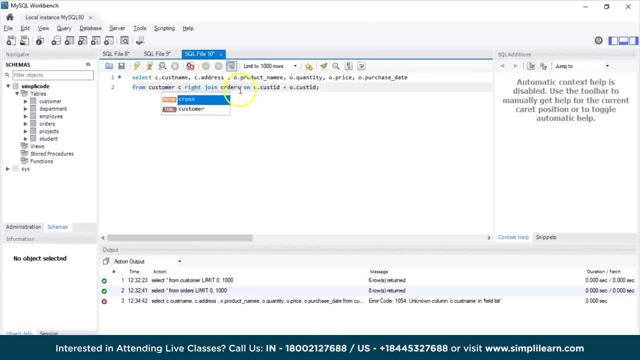 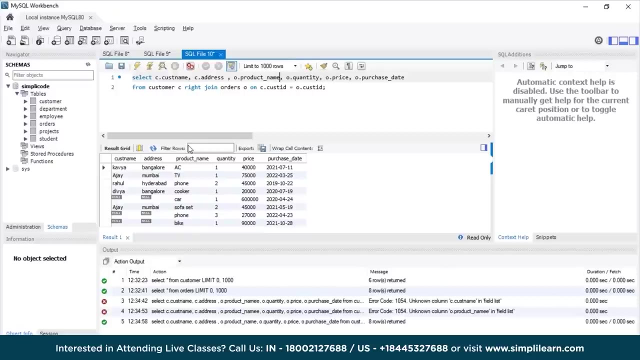 check. Okay, I didn't mention the alias name here, So mention the alias name for both the tables. I guess it will display now. So, as you can see, this is our resultant table, which basically displays the various columns: Customer Name, Their Address, Product Name, Quantity, Price and purchase date. Let us 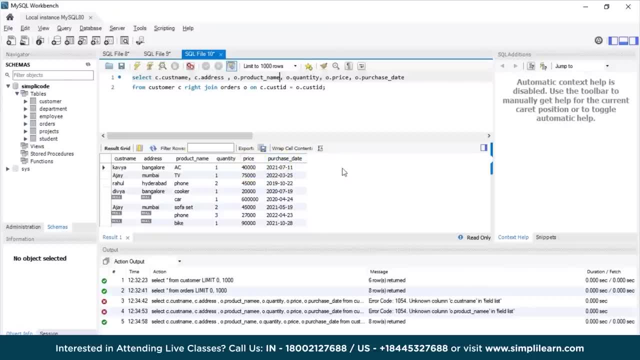 now understand what exactly the write join is performing here. Now, basically, the write join clause starts selecting the data from the right table and matches it with the rows from the left table. The write join returns a resultant table that includes all the rows in the right table, whether or not they're having matching rows from the left table. 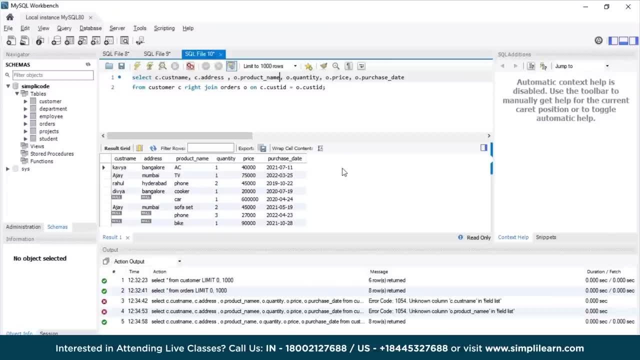 Now, if a row in the right table does not have any matching rows from the left table, the columns of the left table in the resultant set will have null values. Now, clearly, the SQL statement would return all the rows from the orders table. here, As you can see, we have all the details, like AC, TV, phone, cooker, car, sofa set and phone. 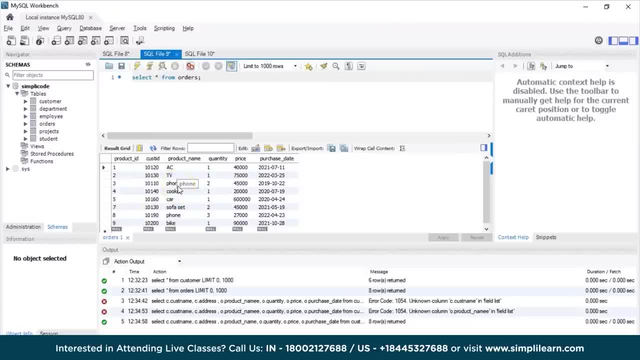 bike, etc. in our orders table. So it is basically retrieving all the data from the right table and only those rows from the customer table where the join condition is being satisfied. Now it will only display the matching values here, because, can you? as you can see, we have. 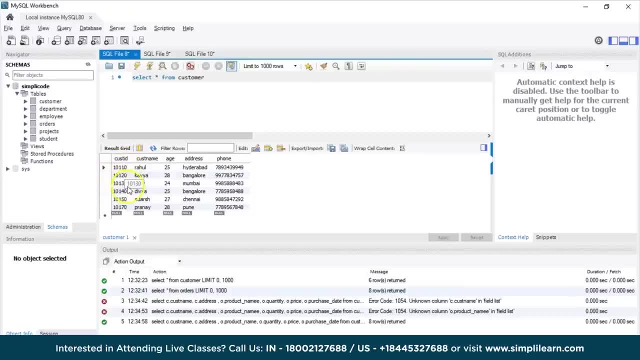 customer ID 10110, 10120, 10130.. So, basically, we have one total six records and we have them in the resultant table as well. Now, if you consider the resultant table here, it is showing null values. So we have to check for some of the customer names and address because, though we have the 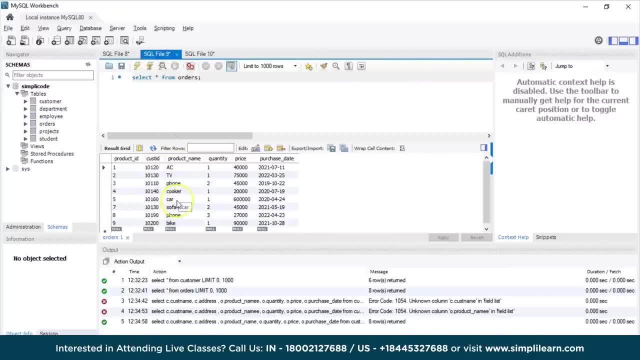 product names mentioned in the orders table. here, for example, the product name- car, sofa, set, bike- and the customer IDs are 10140, 10160 and 10190.. But we do not have their details present in the customer table and that is the reason. 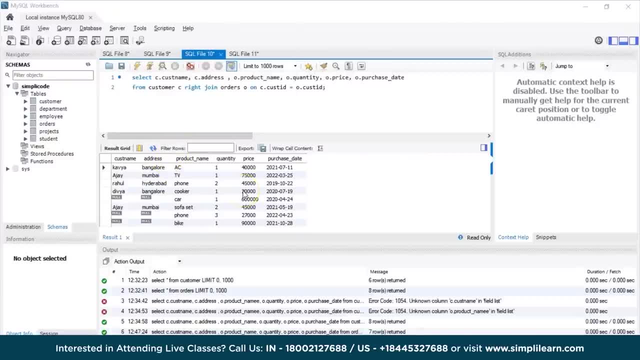 we that it is showing as null here. So in this way you can use the SQL write join condition. Now you might have a doubt that when to use and why to use the write join statement. Again, it will depend on your own requirement. For instance, if you want to keep the records from the second table that do not have any 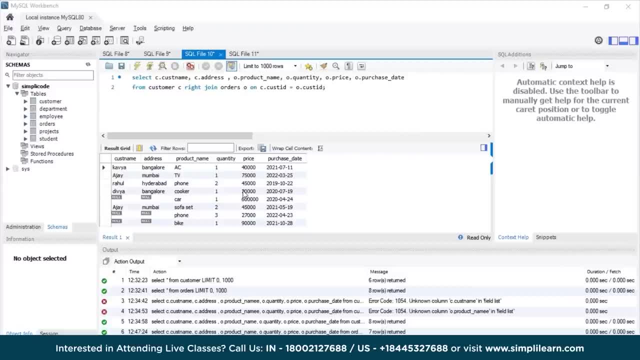 corresponding records from the first table. In that case we will use the write join. Also, another point to be noted here that the table that you have mentioned to the right side of the write join keyword, that is, we have taken here orders right. So it will give the highest priority to this table and it will display all the records. 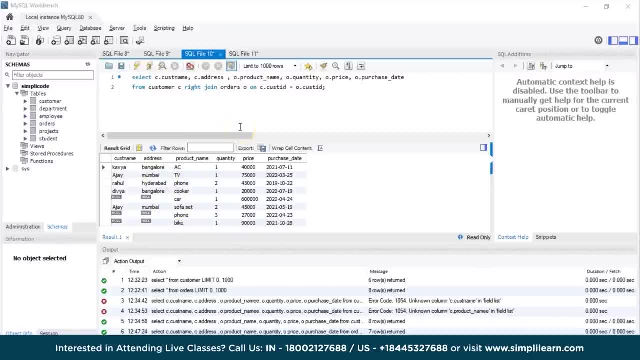 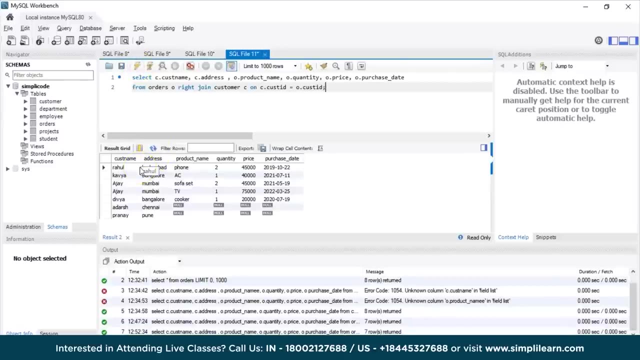 From the orders table here, even if they do not have any matching values. Similarly, just take another scenario here and just interchanging the tables here, like the first table I am taking as orders and the second table I am taking as customers. So when we execute the statement it will display the records from all the records from the. 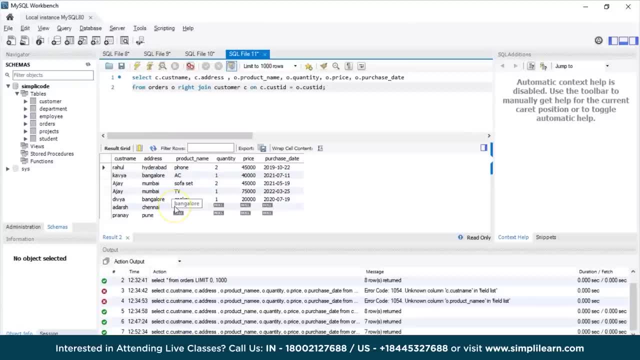 customer table. that is the first table, and even if they do not have the matching values, it will just display the null values here. That's because now, if you consider Adarsh and Pranay, we have their details present in the customer table, but we do not have their information present in the orders table. 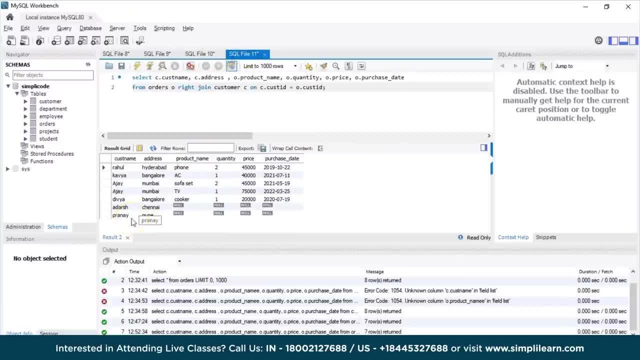 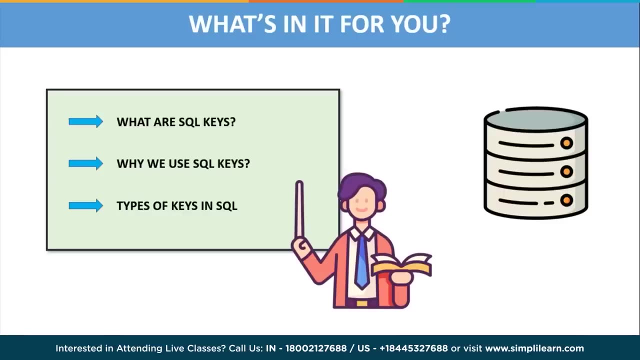 And that's the reason we can see that only their details are present, but they do not have the orders details that we have present here. So in this way you can use the write SQL join statement as well. So with that we have come to the end of session. guys, that was all about the SQL understanding. 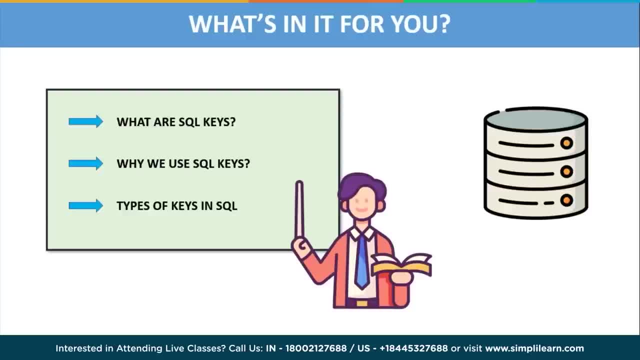 what exactly are SQL keys, And then we will understand why we use SQL keys, And finally, we will go through some different types of keys that are used in SQL. So, without any further ado, let's dive straight into today's topic on SQL keys. 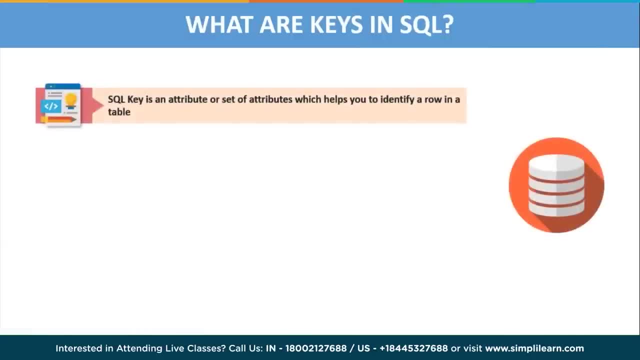 So what are keys in SQL? SQL keys plays an important role in relational databases. It is used for identifying unique rows from table. A key is a subset of columns in a table that allows a row to be uniquely identified, So a key can be more than just a column. 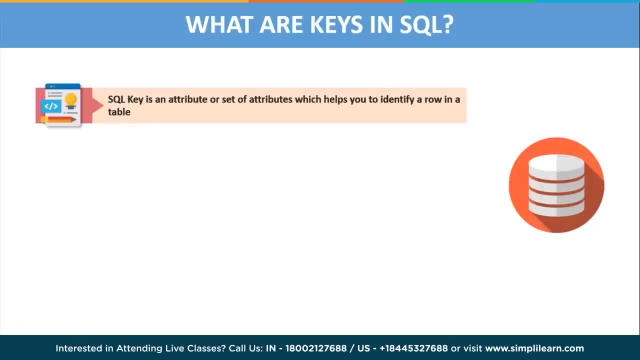 And every row in the table will be a column And every row in the table will have a unique value for the key, or a unique combination of values if the key consists of more than just one column. Now, as you know, databases are used to store massive amounts of information, which is stored 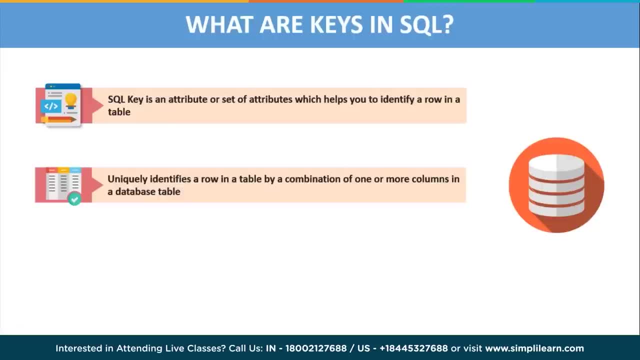 across multiple tables. Now, each table might be having more than thousands of records or rows. Now, needless to say, there will be many duplicate rows with redundant information. So how do we deal with that? Now? how do we manage these records that are storing only unique data? 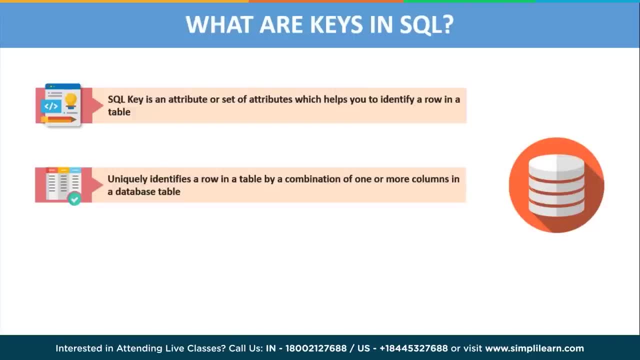 Now for that we might need a combination of one or more columns in a database table to uniquely identify a row in a database. So in that case we use the SQL keys. Now, SQL keys creates constraints that can be used to enforce data integrity in SQL. 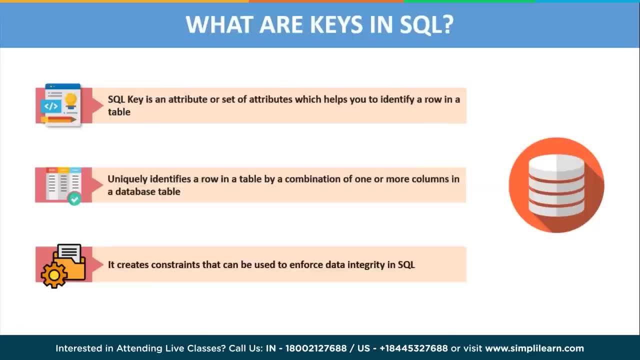 Now, as you know, a database must adhere to certain properties to maintain integrity and quality of the data that it is storing. Keys and constraints are rules that define what data values are allowed in certain data. Now, the key is a key. Now, what is a key? 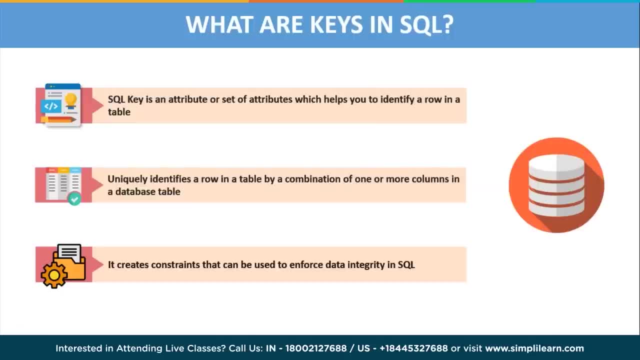 Key is a key data columns. They are an important database concept, as well as for SQL, and are part of database schema definition. Defining keys and constraints is part of database design process and ensures that data within a database is reliable and maintains its integrity. 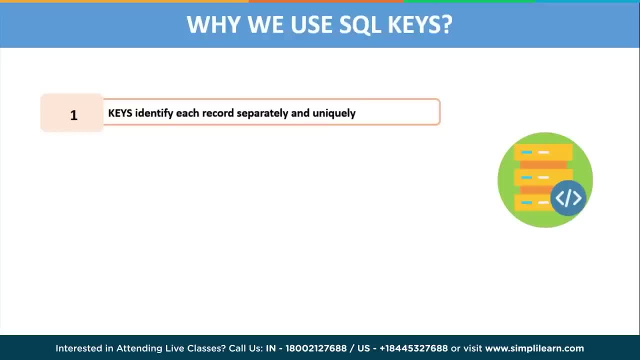 Let us now understand why we use SQL keys. SQL keys identify each record separately and uniquely. Now a key is used in the definition of various kinds of integrity constraints, and a table in a database represents a collection of records or events for a particular relation. 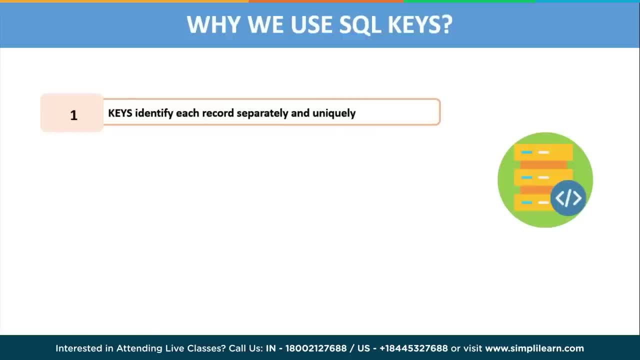 Now, since there are thousands and thousands of such records, some of which may be duplicated. Now, in order to identify these records uniquely and separately, we need SQL keys. SQL keys allows user to establish and identify a relationship between the tables as well. and finally, SQL keys access or manages the stored data quickly and smoothly. 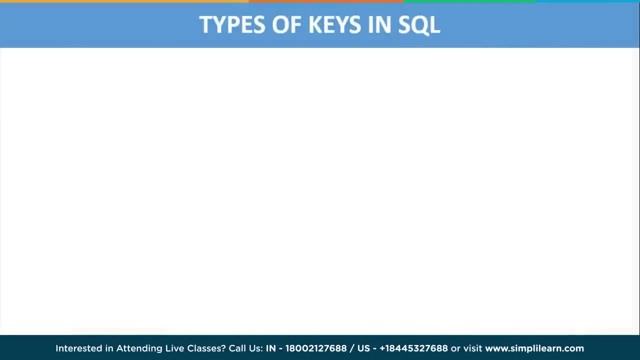 Now that we have understood what SQL keys are and why we use them, let us now discuss some of the various types of keys in SQL. SQL keys are broadly classified into various types, such as primary key, super key, candidate key, alternate key, composite key, foreign key. Now let us discuss each and every. 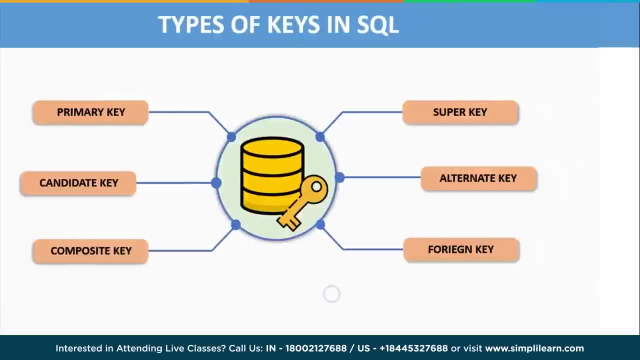 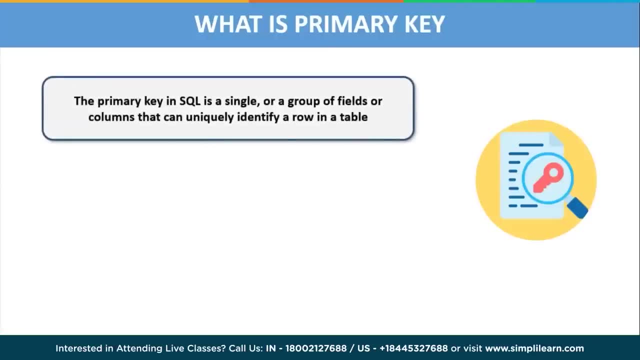 type of key in detail with an example. Firstly, let us look at what exactly is primary key. The primary key is one of the most important and commonly used SQL keys In the databases. the primary key in SQL is a single or a group of fields or columns that can. 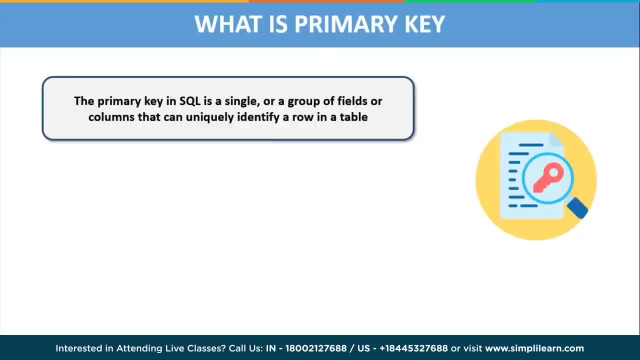 uniquely identify a row in a table. Putting it simply, it is a column that accepts unique values for each row. Therefore, whenever you use the insert into command to insert new values in a table, the value for a primary key column or columns need to be unique. Now, primary key advantages is mainly it. 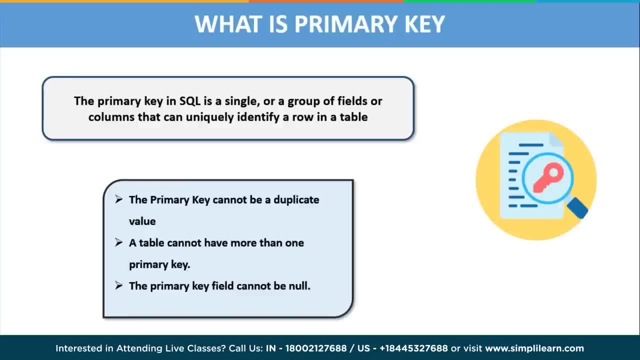 uniquely identifies each row of a table. Now let us look at the advantages of primary key. Primary key can take only one primary key for a table. Also, it gets a unique index for each primary key column. that helps with faster access. Now there are properties which are helpful. 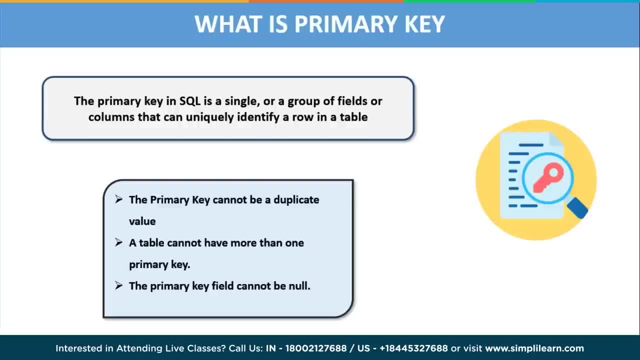 of SQL primary key. They are. it enforces uniqueness by not accepting any duplicate values, and a primary key also uniquely identifies each field and can take only one primary key for a table. Now, a primary key column cannot accept null values as well. Let us consider an example. 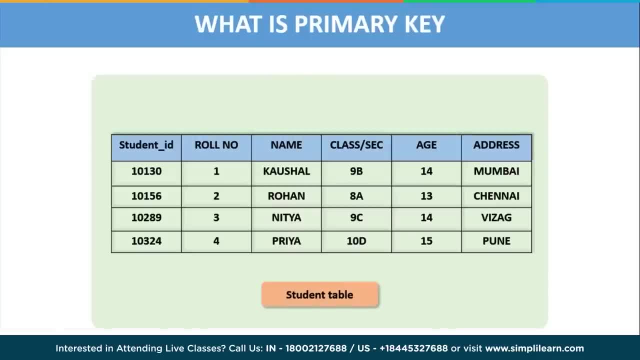 Consider a student table which is having a various fields such as student id, role number, name, class, section, age and address. Now, if you look at the table clearly, student id can be taken as a primary key here. Also, you can take the role number. but since we are taking the records of all the 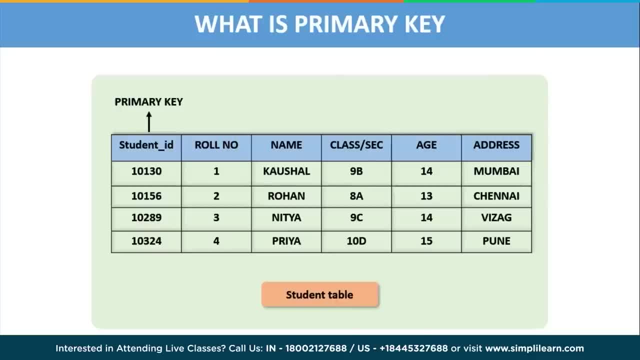 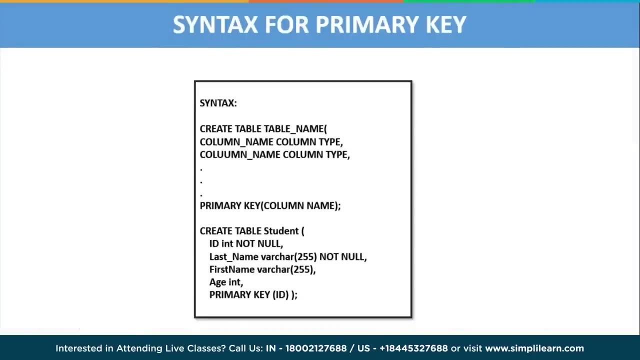 students in a school. that's why we are taking the student id as the primary key. Now, if you take the records of the students for a particular class, then you can take the role number as a primary key as well. Let us now understand the syntax of primary key. Now to create a new table with a. 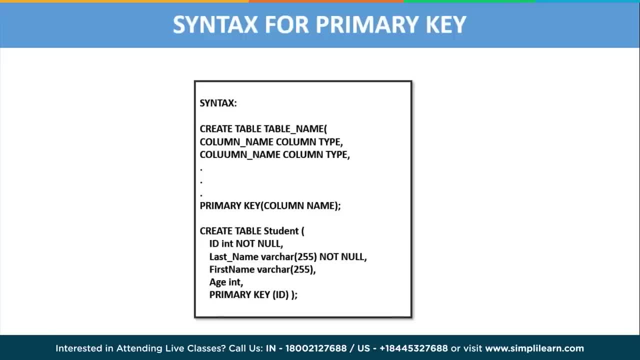 column defined as a primary key, you can use the keyword primary key at the end of the definition of that column and the syntax is create table, table name and within the parenthesis, mention the column names and its column types and finally mention the primary key inside the brackets. 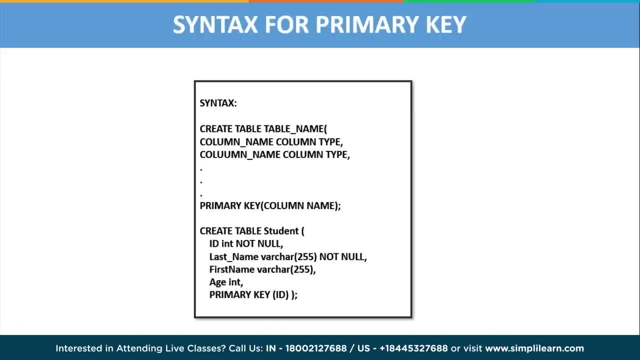 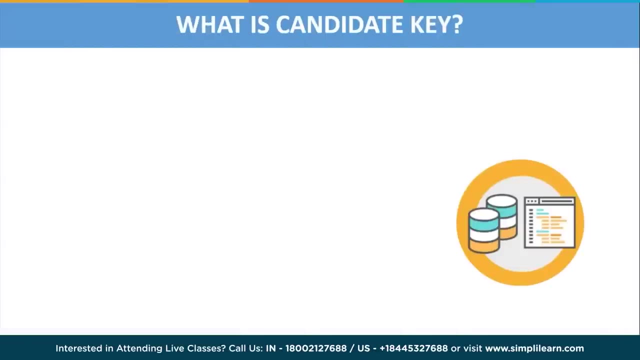 So, for example, if I want to create a table which is having id- last name, first name and age- in that I am going to use the primary key here as id. So in this way you can use the primary key in SQL. Next, let us discuss about the candidate key. A candidate key is defined as set of one or more. 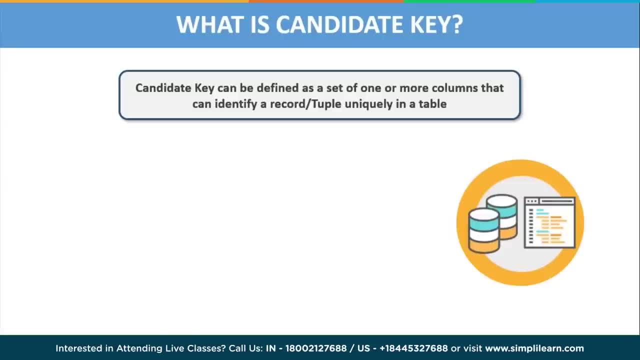 columns that can identify a record uniquely in a table. So basically, candidate key is a super key with no repeated attributes. By the way, we will discuss about the super key in a while. The primary key should be selected from all the candidate keys and every table must have at least a single. 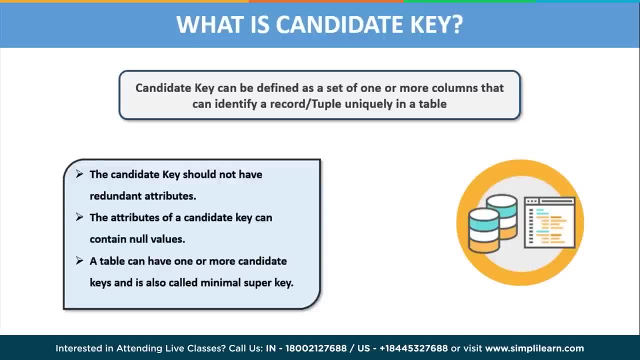 candidate key and a table can have multiple candidate keys, but only a single primary key. Now, candidate key shouldn't have redundant attributes. that means it should not have any duplicate values in the table. Now, unlike primary key, the attributes of candidate key can contain null values and, as discussed, a table can have more than one candidate keys, and it is also called as: 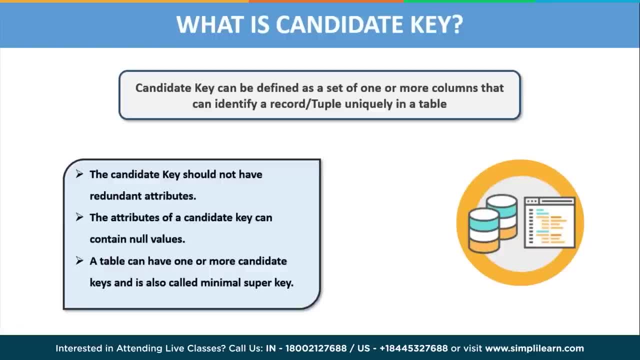 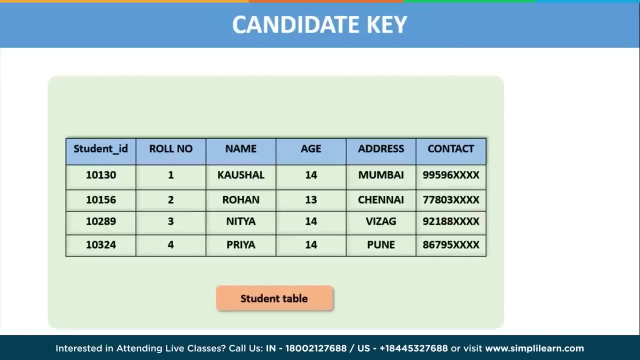 the minimal super key guys. We select a candidate key from a set of super keys such that the selected candidate key is the minimum attribute required to uniquely identify the rows in a table. So let us understand this with an example. Consider the students table here, which is having various columns, such as student id. 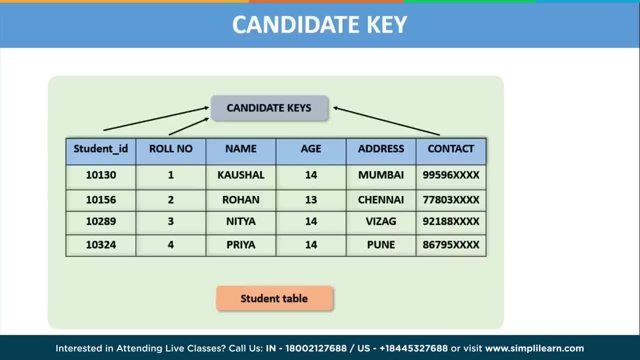 roll number, name, age, address and contact. Now, as you know, we can take the student id as the primary key and with that we can take the roll number as well as the contact of the students as the candidate key here, because all these three columns alone can uniquely satisfy the condition of 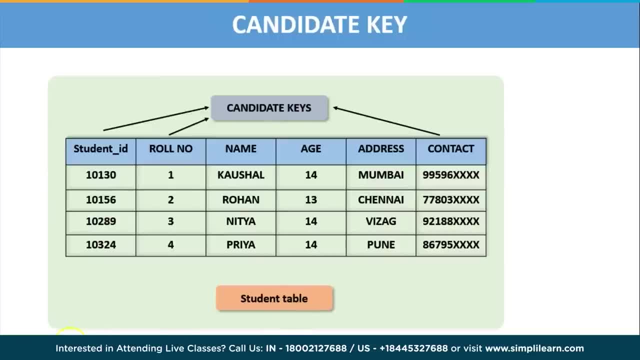 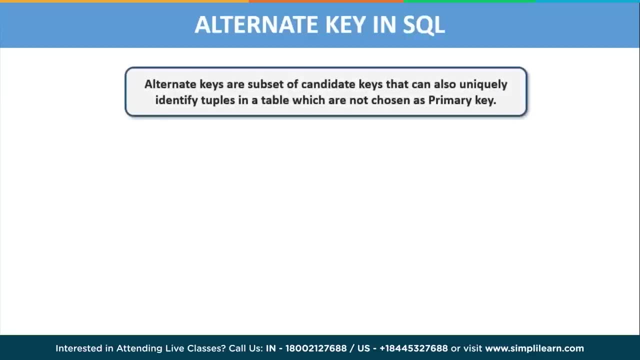 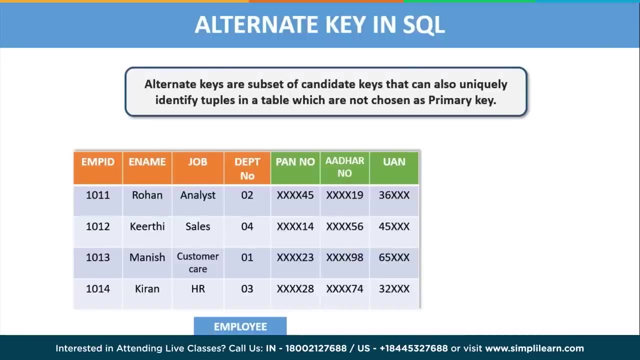 the candidate key here. So in this way we can use the candidate keys in SQL. Next, let us discuss about alternate key in SQL. Alternate key are subset of candidate keys that can also uniquely identify tuples in a table which are not chosen as primary key. 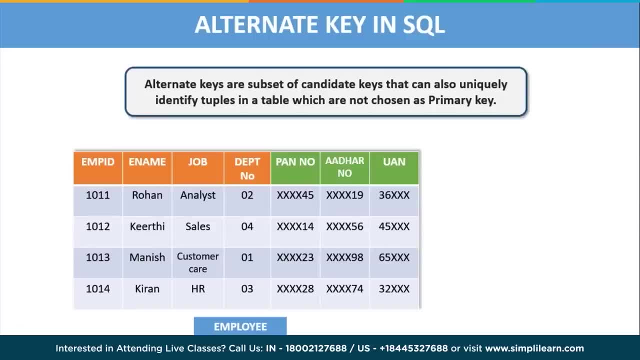 For example, consider the employee table here, which has columns: employee id, employee name name, job department number, PAN number, Aadhaar number and UAN. Now, if you look at the table, the columns that can uniquely identify each and every record are basically employee ID, PAN number, Aadhaar number and UAN number. 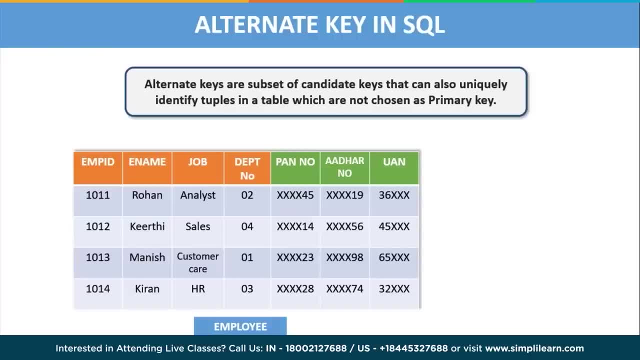 Now, since we have taken the employee ID as a primary key and the rest of all the columns that are not chosen as a primary key are considered to be alternate keys. So in this case we can take the PAN number, Aadhaar number, UAN number as our alternate. 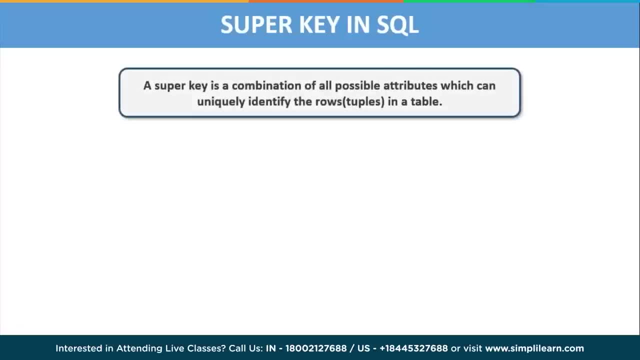 keys. Next, let us discuss about the super key in SQL. Super key is another important key that is used day-to-day usage in SQL databases. A super key or a simple key is a combination of all possible attributes which can uniquely identify the row or tuples in a table. 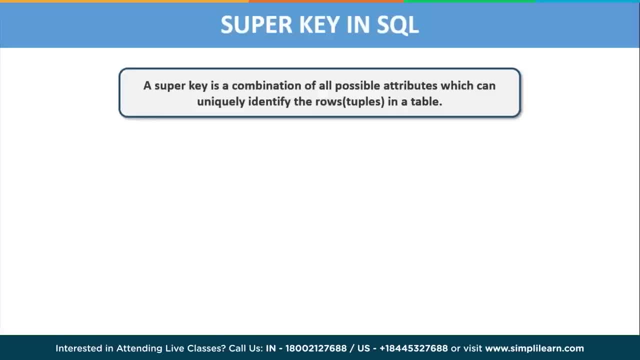 That means that a super key may have some extra attributes which isn't necessary for uniquely identifying the row or tuples in a table. That means that a super key may have some extra attributes which isn't necessary for uniquely identifying the row or tuples in a table. 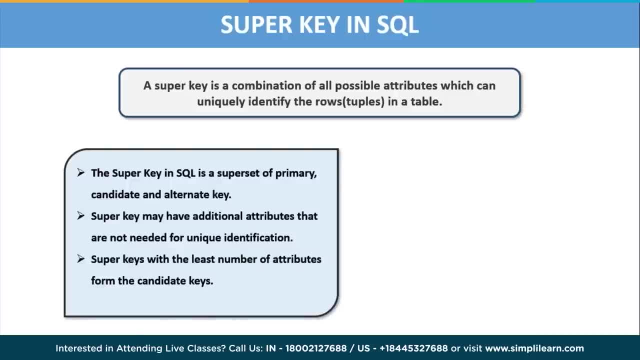 A super key in SQL is a superset of primary key, candidate key and alternate key. A super key is a superset of primary key, candidate key and alternate key. That means basically it is a combination of all the keys, such as primary, candidate and 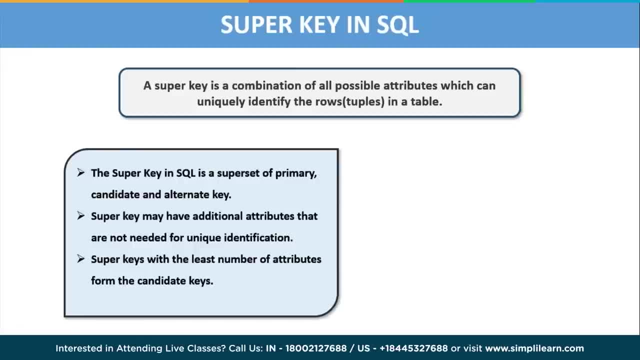 alternate keys. As discussed, a super key will have additional attributes that are not needed for any unique identification And finally, a super key with least number of attributes form the candidate keys. So let us take an example again. Consider the employee table here. 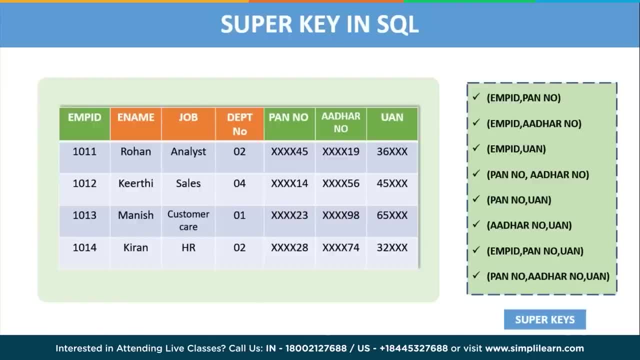 and if you look at the possible keys that will be for super keys are: Employee ID- PAN number, Employee ID- Aadhar number, Employee ID- UAN. PAN number, Aadhar number, PAN number, UAN. Aadhar number- UAN. Employee ID, PAN number, as well as UAN. 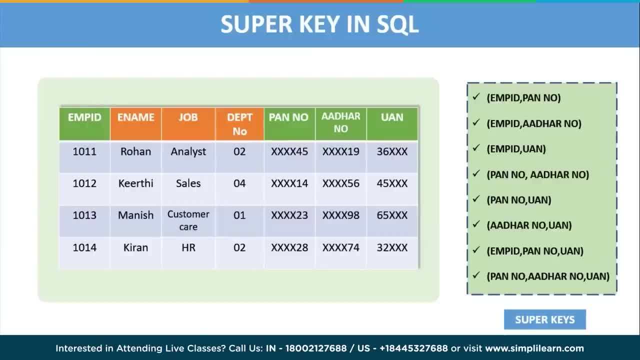 and finally, PAN number, Aadhar number and UAN. Now all the above keys are able to uniquely identify each row, So each of these keys is a super key. Now, again, in this example, we have like more than six super keys, but all of them cannot become a candidate key here. 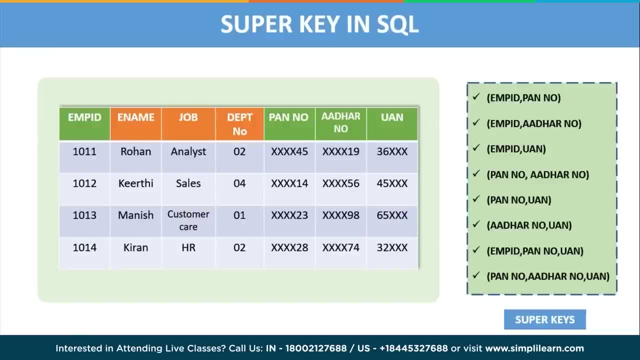 Only those super keys would become a candidate key which have no redundant attribute. For example, if you take Employee ID, PAN number, this key cannot be considered as a candidate key because when we take the subset of this key, we get two attributes, that is, Employee ID as well as the PAN number. 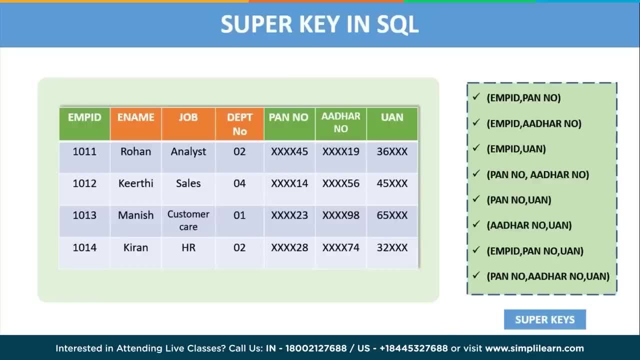 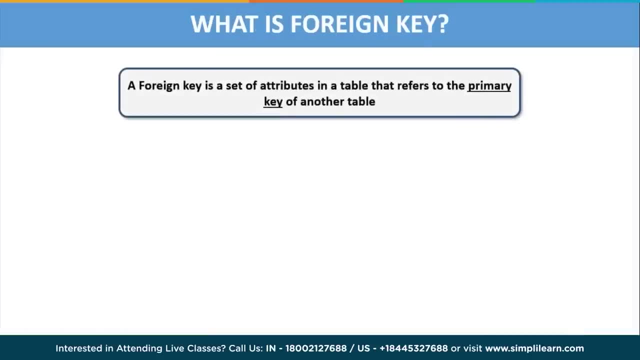 Now, each of these attributes is basically a candidate key, So it is a minimal super key, but hence this key is not a candidate key. And finally, let us discuss about the foreign key. in SQL, A foreign key is a column or combination of columns that is used to establish and force a link between the data in two tables. 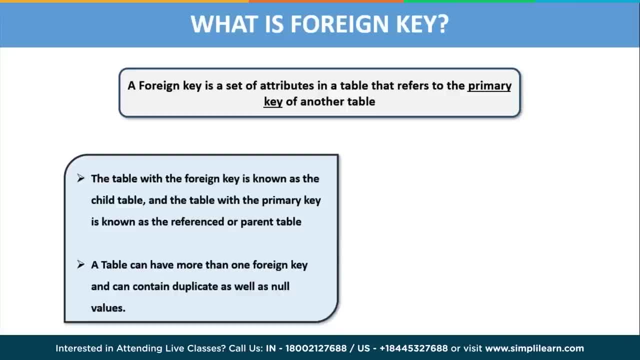 to control the data that can be stored in the foreign key table. In a foreign key reference, a link is created between two tables and the column or columns hold the primary key value for one table and the reference by the column or columns in other table. 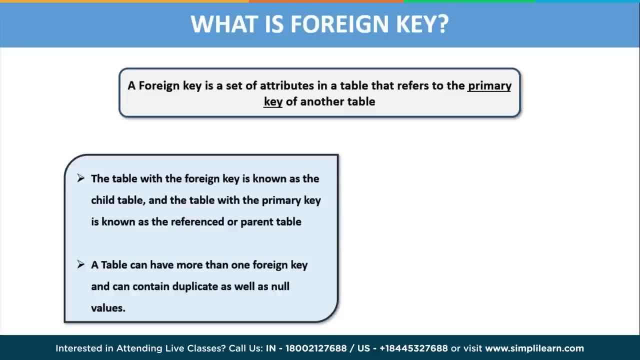 Now this column becomes a foreign key in the second table. the table with the foreign key is known as the child table and the table with the primary key is known as the referenced or parent table. now, as foreign key, has bought the referential integrity in sql, which means that it requires. 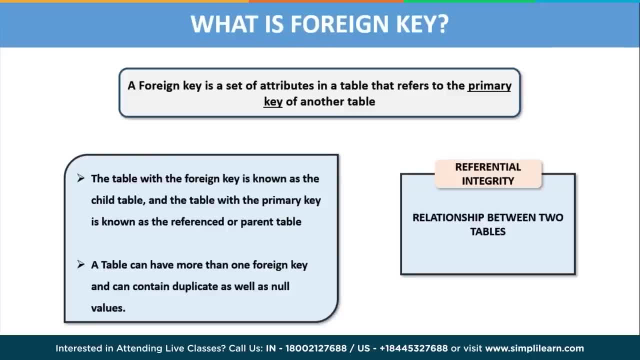 that a foreign key must have a matching primary key or it must be null. this constraint is specified between two tables, that is, parent and child, and it maintains the correspondence between the rows in these tables. it means that the reference from a row in one table to another. 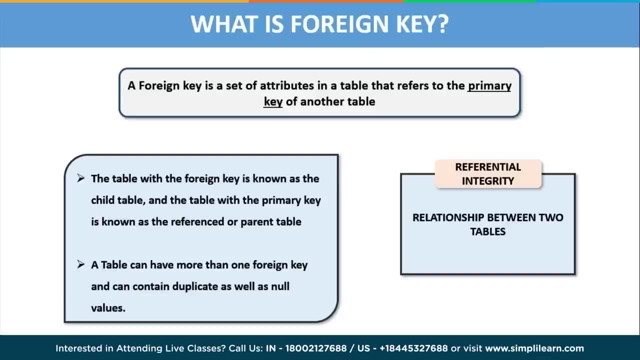 table must be valid now. the foreign key helps in maintaining the data integrity of the table and allows easy navigation between two instances or attributes. it is also used in sql to make the database data consistent, and it is also used for the prevention of any action that may result. 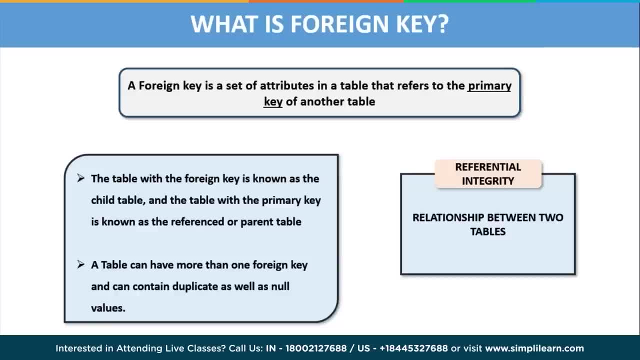 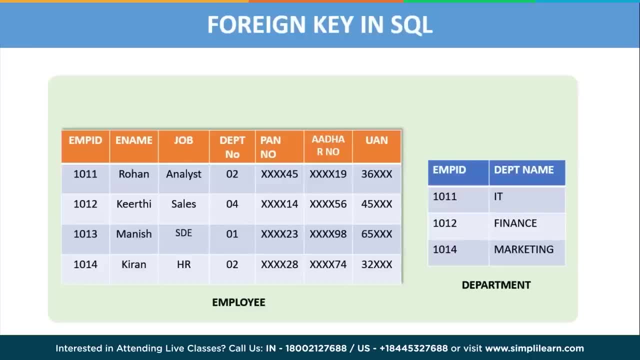 in destruction of relation between these two tables. let us understand this with an example. let us understand this with an example. now consider two tables here: employee and department. the employee table has employee id, employee name, job department number, pan number, other number and un number and the department. 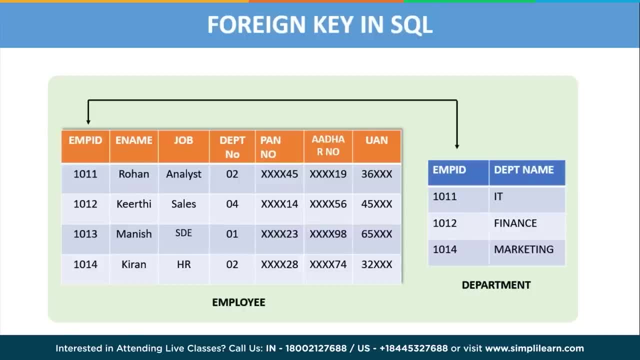 table has employee id and the department name. now, clearly, the employee id, which is the primary key in the first table- employee- is acting as a cross reference for the department table. that is, uh, the employee id acts as the foreign key here for the department table. so in this way you can use. 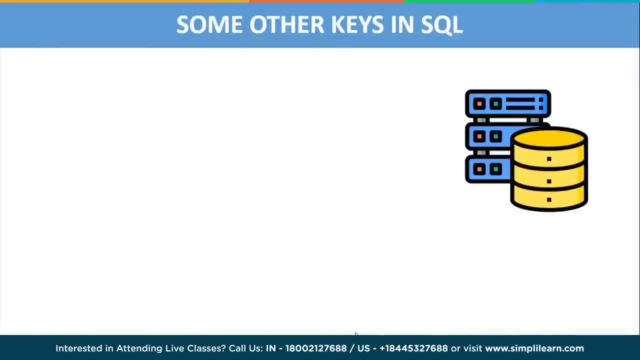 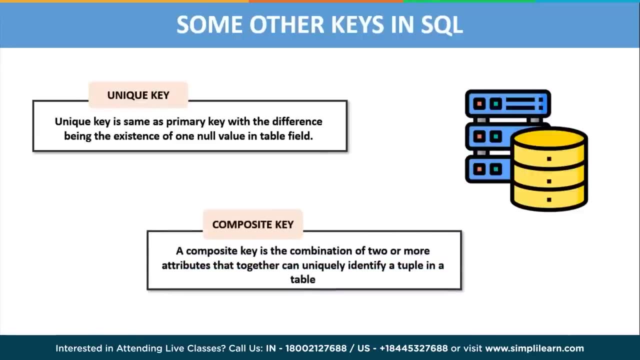 the foreign key in sql, and similarly, we have some other types of keys in sql which are not that significant in its usage, the first one being is unique key. a unique key, same as a primary key, with the difference being the existence of one null value in a table field or a row, for example. 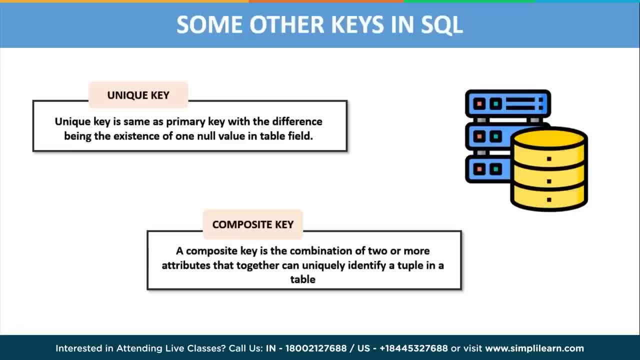 consider a student table having student id, roll number and its name. now, for some reasons, if the student is leaving the school, then his roll number might be deleted, although his student role number is not the same as the student's role number, then his role number might be deleted. 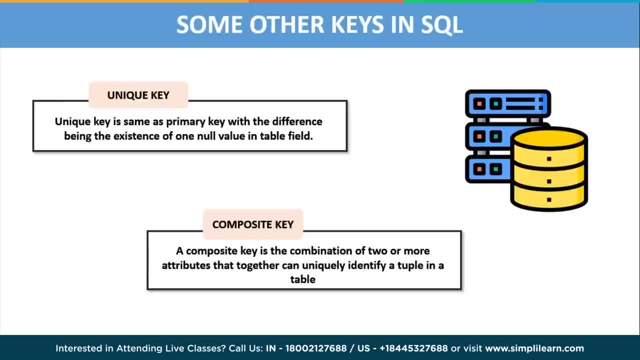 although his student role number is not the same as the student's role number, then his role number id will be preserved for further assistance. so since there is a null value in roll number, it can be considered as a unique key and student id can be considered as a primary key. similarly, we have 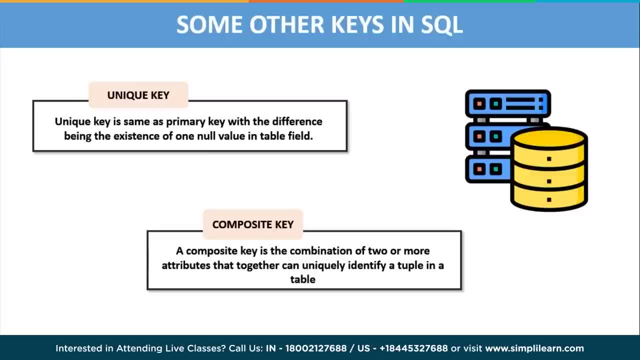 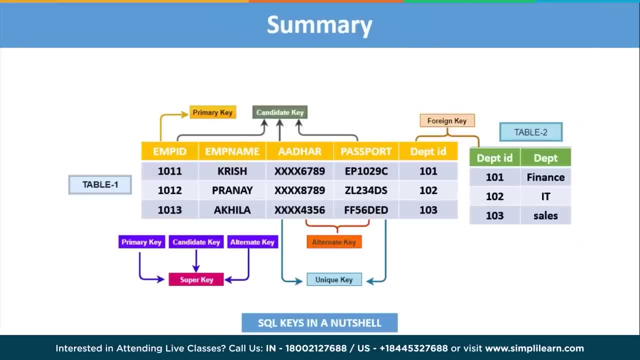 composite key. a composite key is a combination of two or more attributes that can together, uh can uniquely identify a tuple in a table. and that brings us to the end of today's session. uh, that was all about, uh, the sql keys. so let us just quickly recap what we have discussed, uh that, if 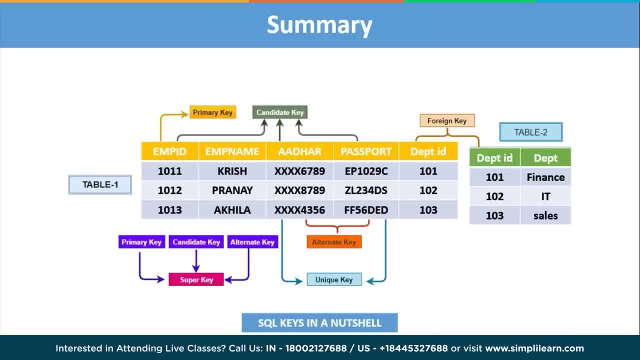 the sql keys were used right, then we would have identified the two key of the sql key for each of the sql keys and then, at the end of this session, we would have identified the two key of the sql key. so at the end of this session we are going to see how should we identify the two key. 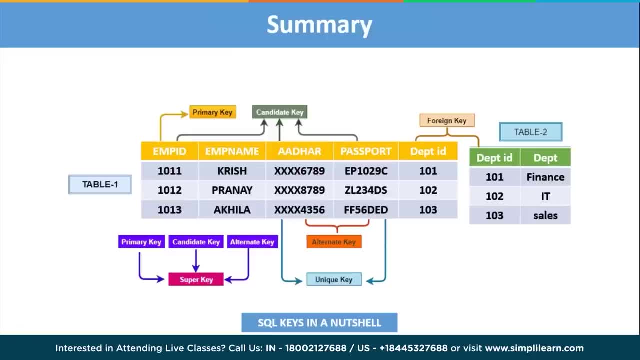 in the sql key. first we will discuss the sql key. the sql key is a key that is used as a powerpoint in a table to be used as a menu for a sql key. so let us first learn a little bit about sql series number and how we can use it to. 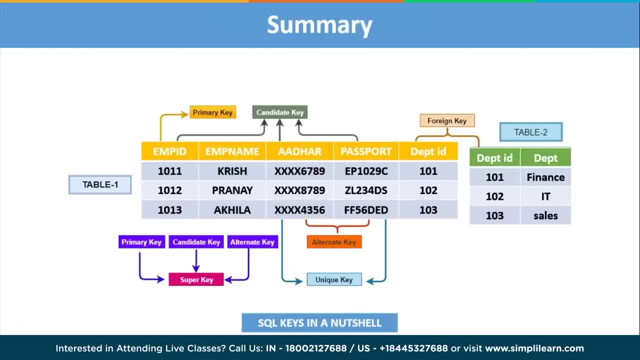 So they can be considered as the candidate key here Now, alternate keys which are other than the primary key, that is, employee ID. So I am taking Aadhar card and passport as the alternate keys here Now, the combination of all these keys such as primary key, candidate key, alternate key. 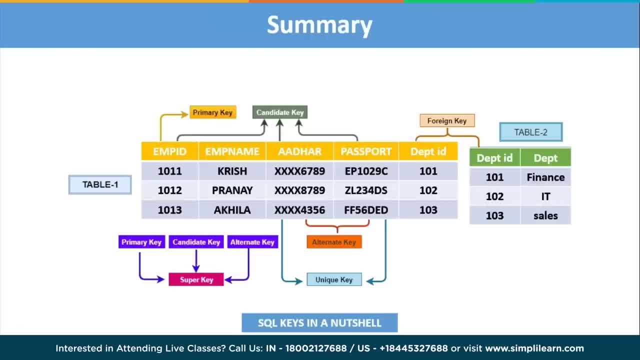 forms a super key. Now I am taking the passport as the unique key, since not everyone has a passport to their name, So I am taking the passport attribute here as the unique key. And finally, the foreign key is the department ID, as it points to the reference to the second. 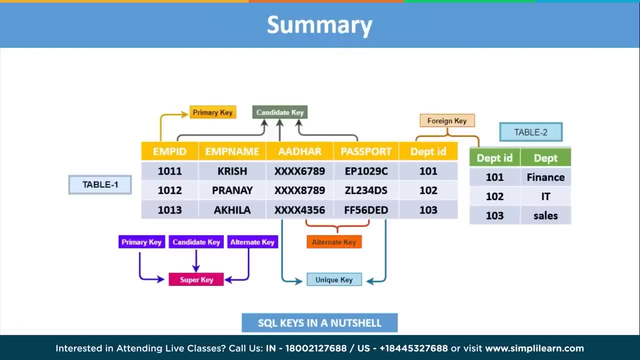 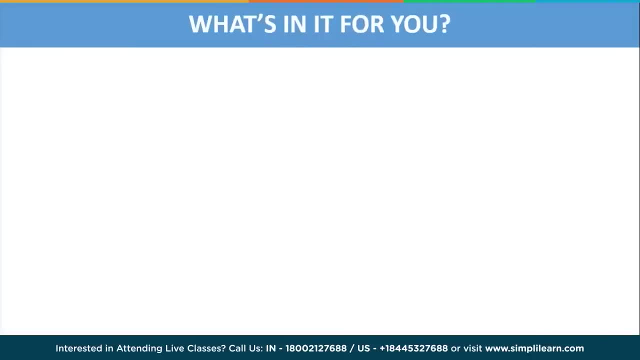 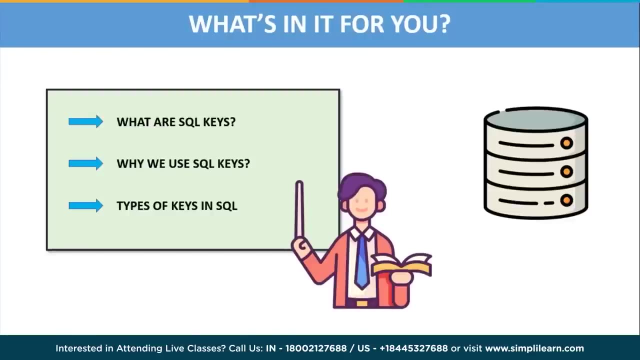 table, that is, department table. So in this way you can use the SQL keys accordingly. Before any further delay, let's get started with today's topic. Firstly, let us understand the agenda for today's session. We'll start the tutorial by understanding what exactly are SQL keys. 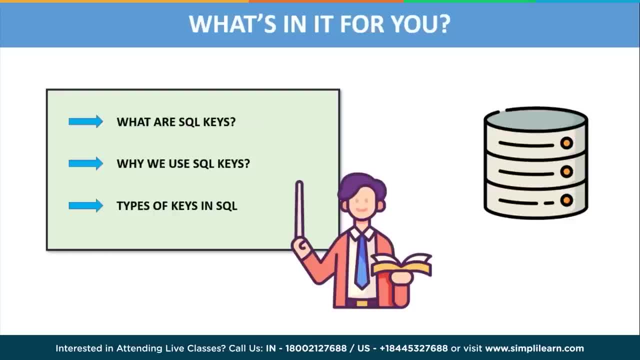 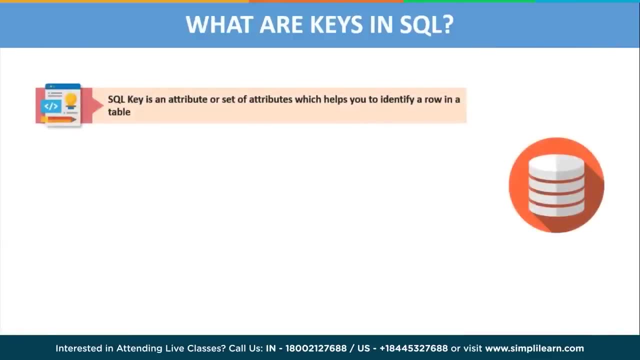 And then we'll understand why we use SQL keys And finally we'll go through some different types of SQL keys. So, without any further ado, let's dive straight into today's topic on SQL keys. So what are keys in SQL? SQL keys plays an important role in relational databases. 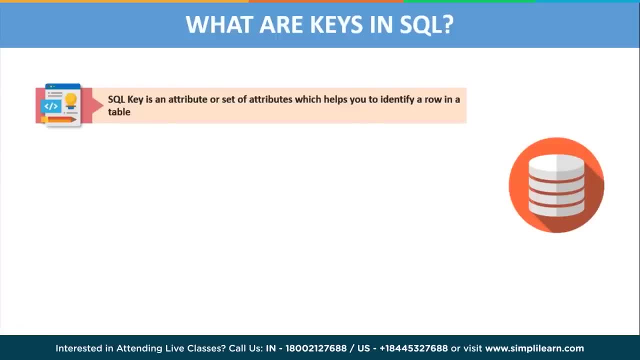 It is used for identifying unique rows from table. A key is a subset of columns in a table that allows a row to be uniquely identified. So a key can be more than just a column And every row in the table will have a unique value for the key. 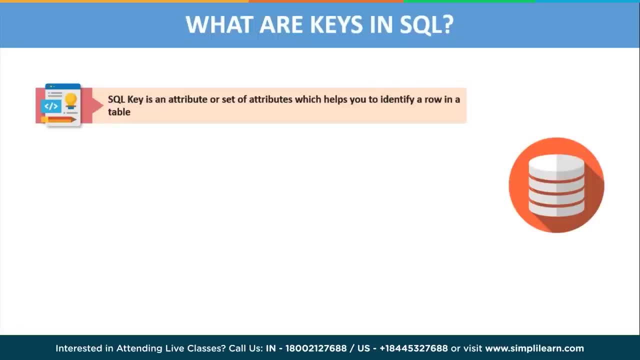 Or a unique component Or a combination of values if the key consists of more than just one column. Now, as you know, databases are used to store massive amounts of information, which is stored across multiple tables. Now, each table might be having more than thousands of records or rows. 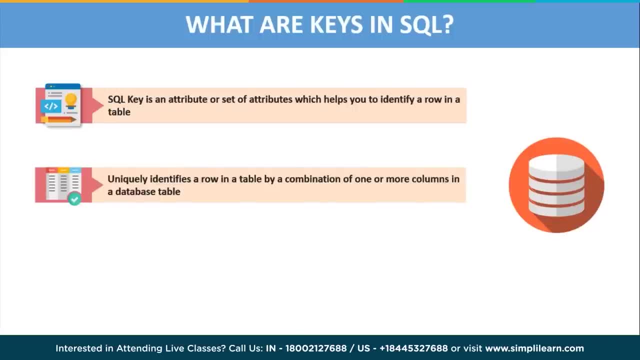 Now. needless to say, there will be many duplicate rows with redundant information. So how do we deal with that Now? how do we manage these records that are storing only unique data Now? for that, we might need a combination of one or more columns. 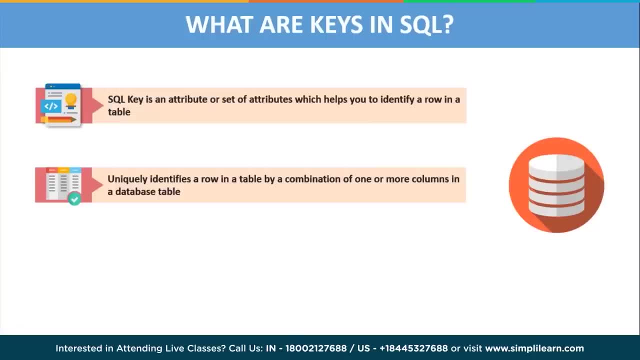 So how do we deal with that Now? let us first start with the SQL key. SQL key is a variable that can be used to store data that is stored in a database. A database is a set of columns in a database table to uniquely identify a row in a database. 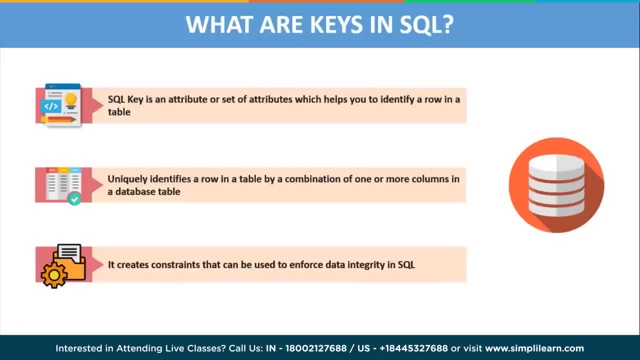 So in that case, we use the SQL keys. Now, SQL key creates constraints that can be used to enforce data integrity in SQL. Now, as you know, a database must adhere to certain properties to maintain integrity and quality of data that is stored. Keys and constraints are rules that define what data values are allowed in certain data. 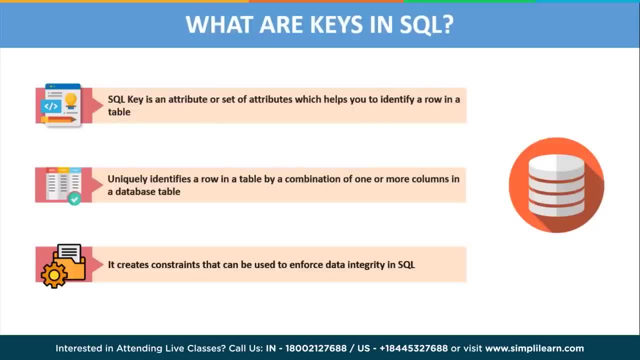 columns. They are an important database concept- I have a few examples here, well as for SQL- and are part of database schema definition. Defining keys and constraints is part of database design process and ensures that data within a database is reliable and maintains its. 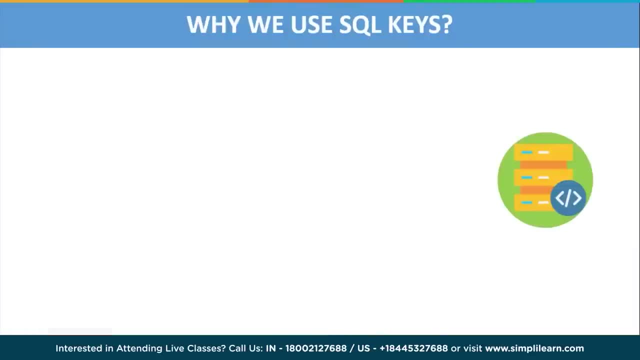 integrity. Let us now understand why we use SQL keys. SQL keys identify each record separately and uniquely. Now a key is used in the definition of various kinds of integrity constraints, and a table in a database represents a collection of records or events for a particular relation. 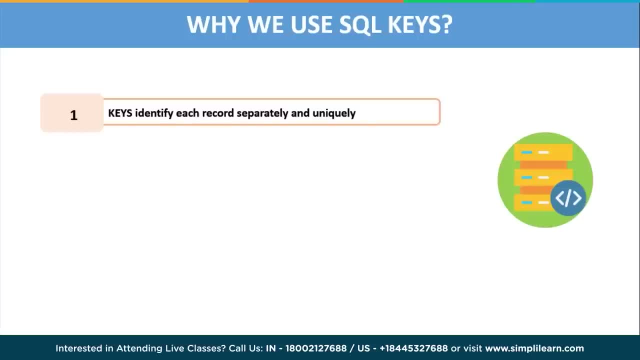 Now, since there are thousands and thousands of such records, some of which may be duplicated. Now, in order to identify these records uniquely and separately, we need SQL keys. SQL keys allows user to establish and identify a relationship between the tables as well. And finally, SQL keys access or manages the stored data quickly and smoothly. 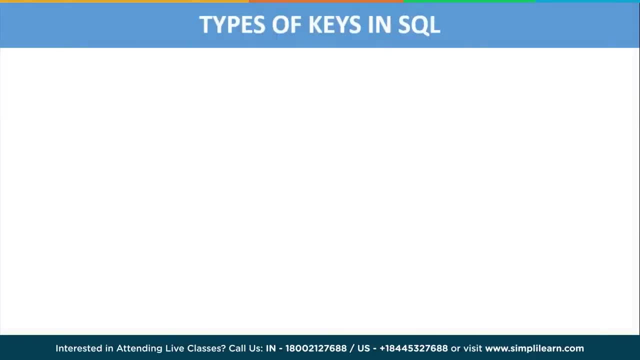 Now that we've understood what SQL keys are and why we use them, let us now discuss some of the various types of keys in SQL. SQL keys are broadly classified into various types, such as primary key, super key, candidate key, alternate key, composite key, foreign key. Now let us 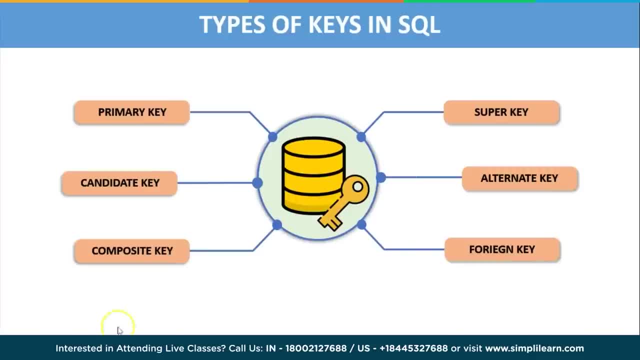 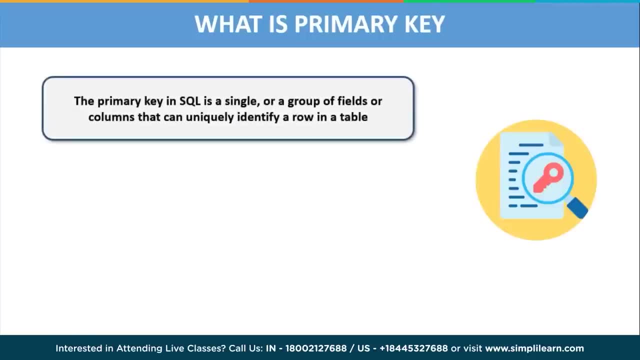 discuss each and every type of key in detail with an example. Firstly, let us look at what exactly is primary key. The primary key is one of the most important and commonly used SQL keys. The primary key in SQL is a single or a group of fields or columns that can. 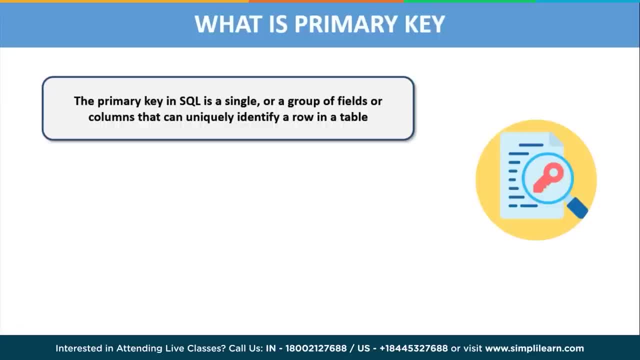 uniquely identify a row in a table. Putting it simply, it is a column that accepts unique values for each row. Therefore, whenever you use the insert into command to insert new values in a table, the value for a primary key column or columns need to be unique. 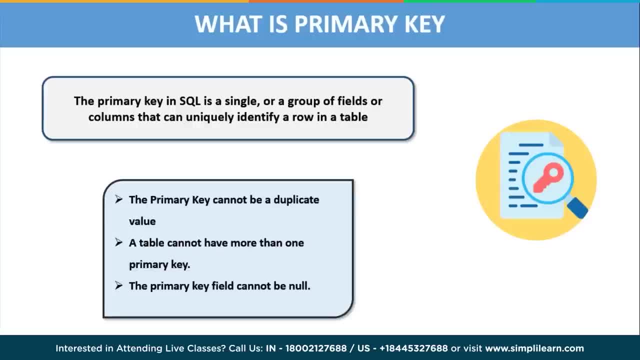 Now primary key advantages is mainly: it uniquely identifies each row of a table. Also, it gets a unique index for each primary key column. that helps with faster access. Now there are properties which are helpful of SQL primary key. They are: it enforces uniqueness by not accepting any duplicate values. 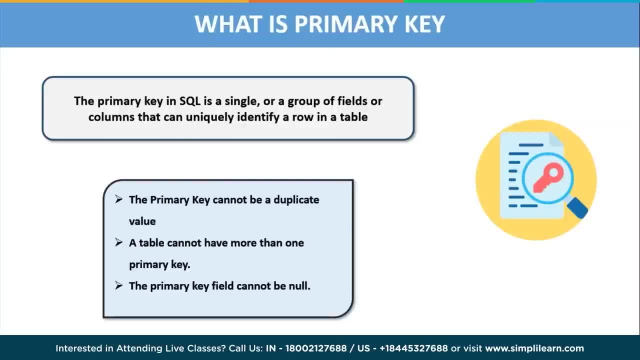 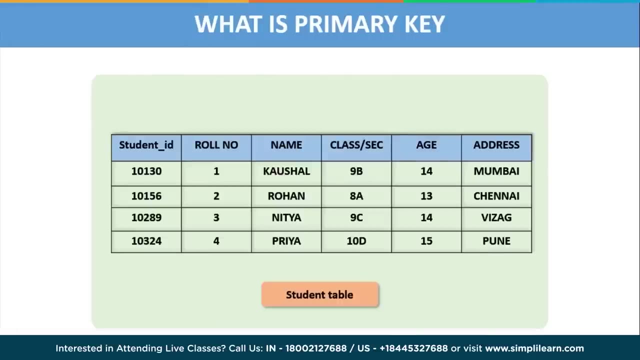 and a primary key also uniquely identifies each field and can take only one primary key for a table. Now, a primary key column cannot accept null values as well. Let us consider an example here: A student table which is having various fields, such as student id, role number, name. 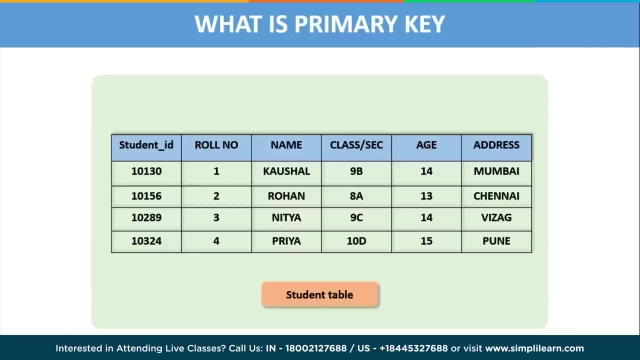 class section, age and address. Now, if you look at the table clearly, student id can be taken as a primary key. here. Also, you can take the role number, but since we are taking the records of all the students in a school, that's why we are taking the student id as the primary key. Now, if 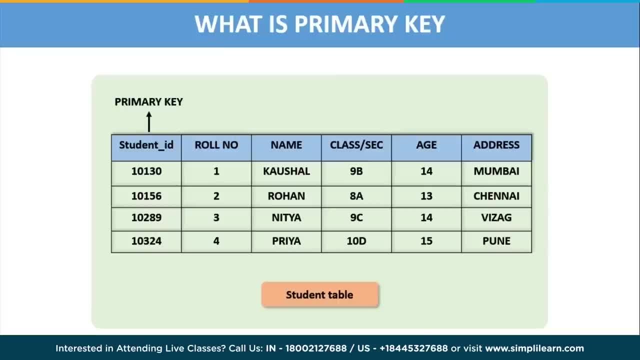 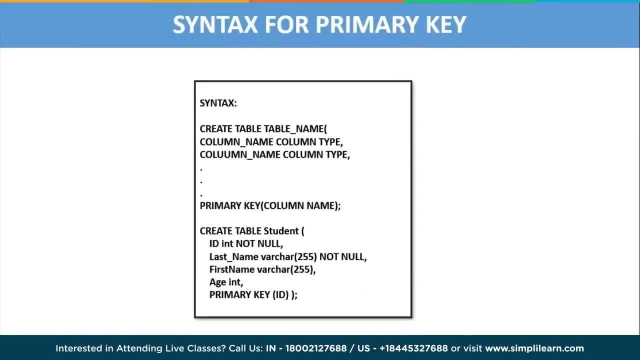 you take the records of the students for a particular class, then you can take the role number as a primary key as well. Let us now understand the syntax of primary key. Now, to create a new table with a column defined as a primary key, you can use the keyword primary key at the end of the definition of that column. 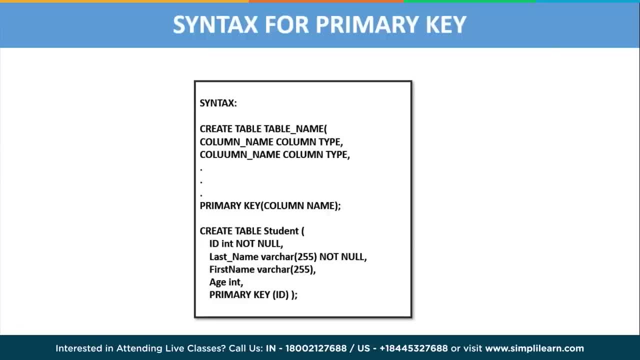 and the syntax is: create table, table name and, within the parenthesis, mention the column names and its column types and finally mention the primary key inside the brackets. So, for example, if I want to create a table which is having id, last name, first name and age in that, 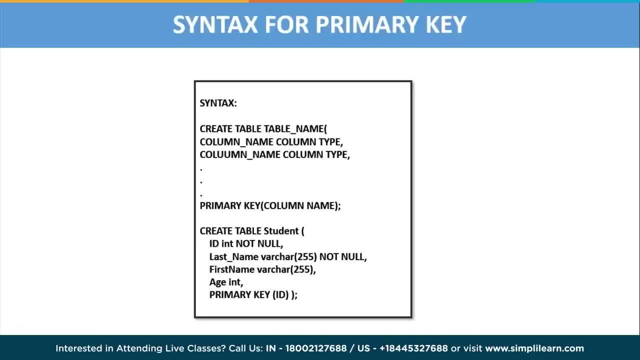 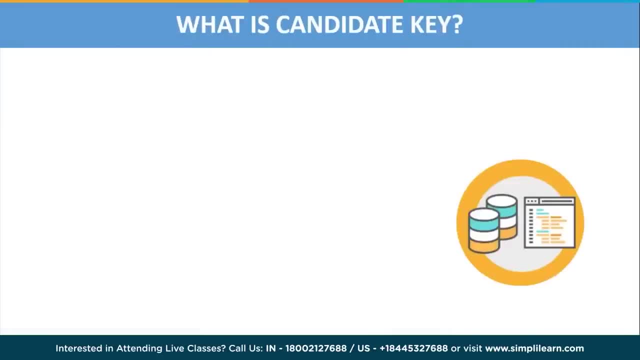 I am going to use the primary key here as id, So in this way you can use the primary key in SQL. Next let us discuss about the candidate key. A candidate key is defined as set of one or more columns that can identify a record uniquely in a table. So basically, candidate key is a super key. 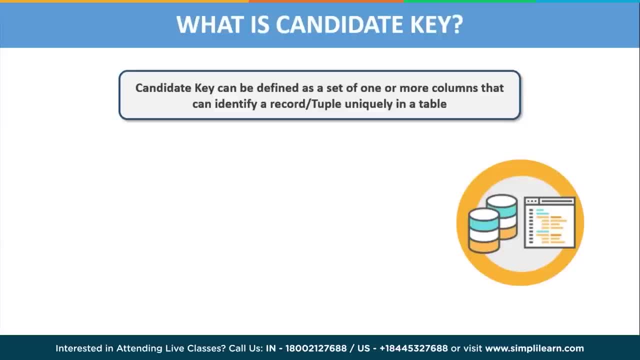 with no repeated attributes. By the way, we will discuss about the super key in a while. The primary key should be selected from the first row of the table and the second row of the table should be selected from all the candidate keys, and every table must have at least a single candidate key. 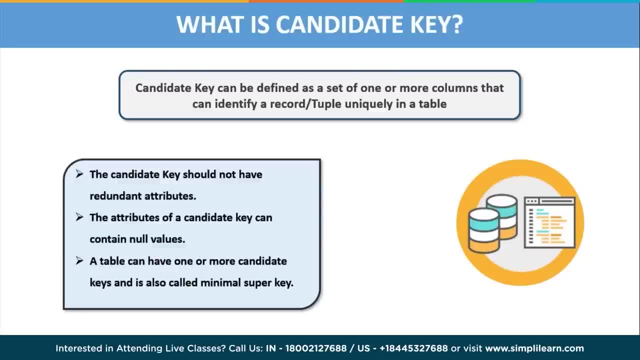 and a table can have multiple candidate keys, but only a single primary key. Now, candidate key shouldn't have redundant attributes. that means it should not have any duplicate values in the table. Now, unlike primary key, the attributes of candidate key can contain null values and, as discussed, a 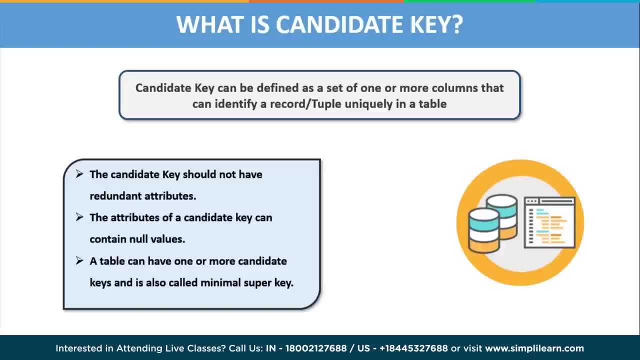 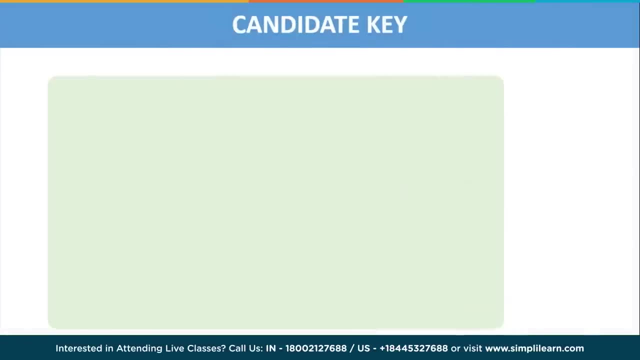 table can have more than one candidate keys, and it is also called as the minimal super key guys. That's because we select a candidate key from a set of super keys such that the selected candidate key is the minimum attribute required to uniquely identify the rows in a table. So let us understand this with. 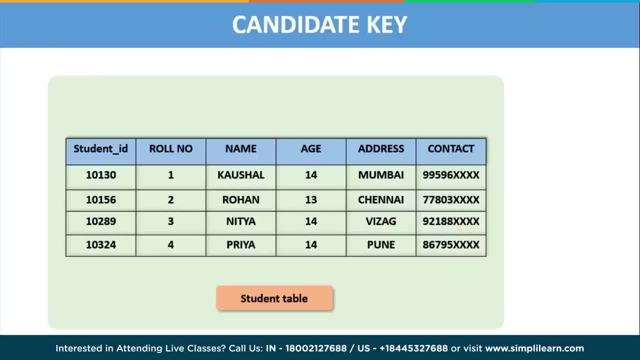 an example, Consider the students table here, which is having various columns such as student id, roll number, name, age, address and contact. Now, as you know, we can take the student id as the primary key and with that we can take the roll number as well as the contact of the students as the candidate key here. 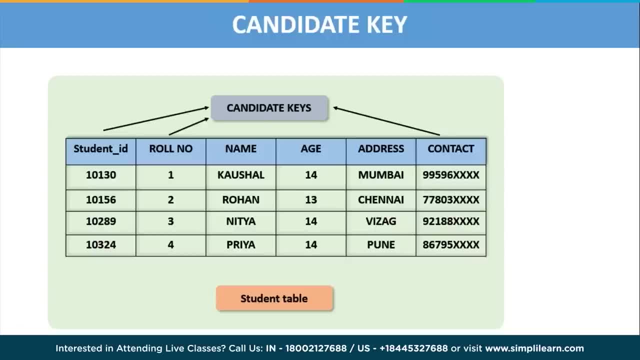 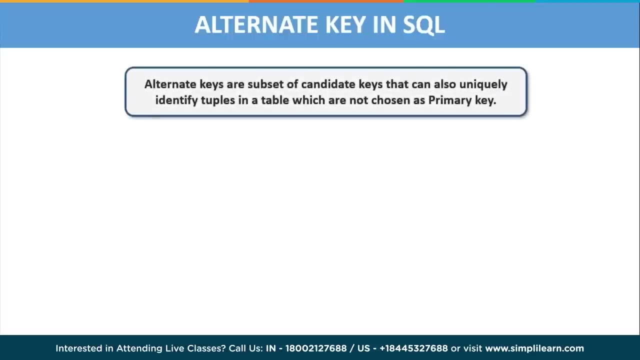 Because all these three columns alone can uniquely satisfy the condition of the candidate key here. So in this way we can use the candidate keys in sql. Next let us discuss about alternate key in SQL. Alternate key are subset of candidate keys that can also uniquely identify tuples in a. 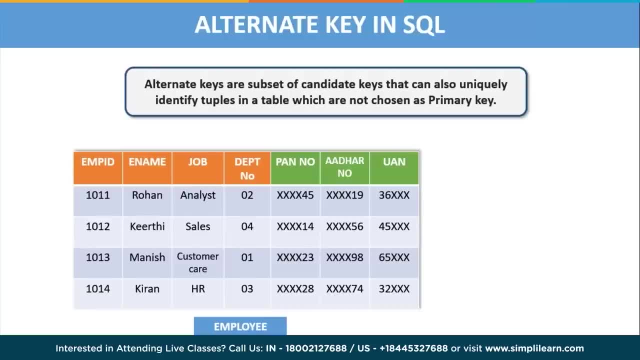 table which are not chosen as primary key. For example, consider the employ table here, which has columns employ id, employ name, job ect. We can decide whether the contact is pure or not pure. Thequell number is 12.. So we select sol dressing and here the flexible table. after that we choose Bl Painting. 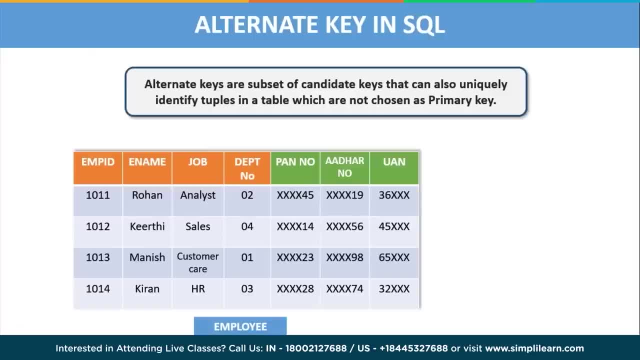 employee name, job department number, pan number, other number and uan. now, if you look at the table uh, that columns that can uniquely identify each and every record are basically employee id, pan number, other number and uan number. now, since we have taken the employee id as a primary key and 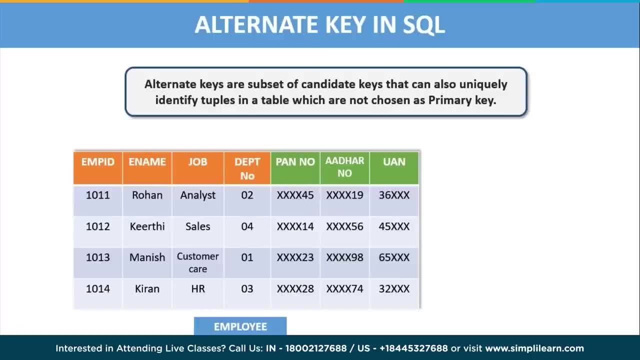 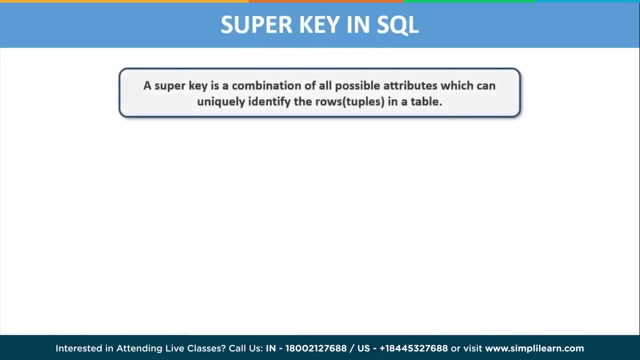 the rest of all the columns that are not chosen as a primary key are considered to be alternate keys. so in this case we can take the pan number, other number, uan number as our alternate keys. next let us discuss about the super key. in sql, super key is another important key that is used. 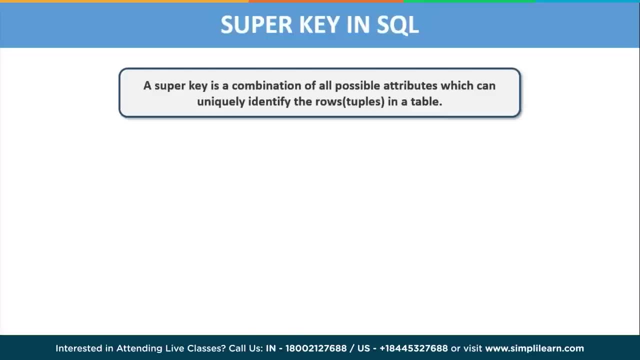 day-to-day usage in sql databases. a super key or a simple key is a combination of all possible attributes which can use uniquely identify the row or tuples in a table. that means that a super key may have some extra attributes which isn't necessary for the table. so we can take the pan number, other number and uan number as our alternate keys. 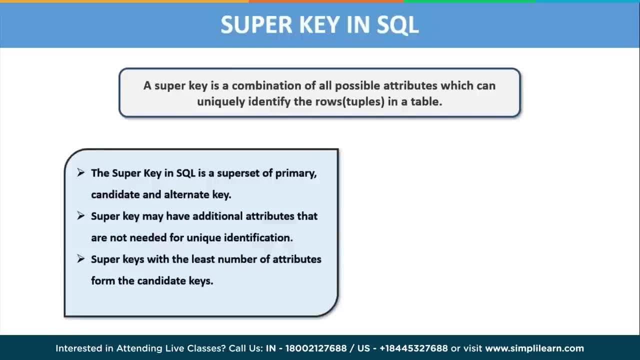 uniquely identifying the rows in the table. a super key is a. in sql is a superset of primary key, candidate key and alternate key. that means basically it is a combination of all the keys, such as primary, candidate and alternate keys. as discussed, super key will have additional attributes. 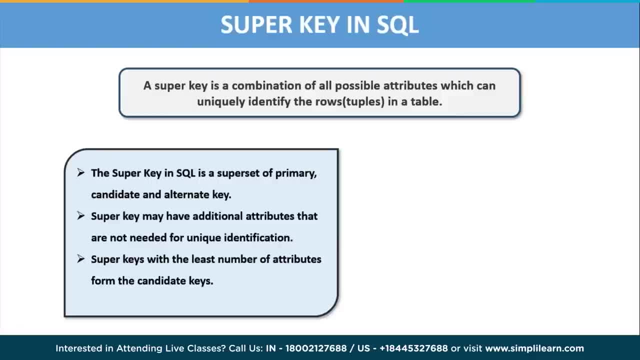 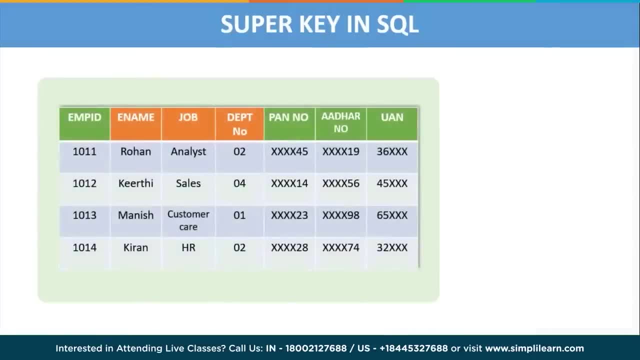 that are not needed for any unique identification and finally, super keys with the least number of attributes form the candidate keys. so let us take an example again. consider the employee table here and if you look at the possible keys that will be for super keys are employee id, pan. 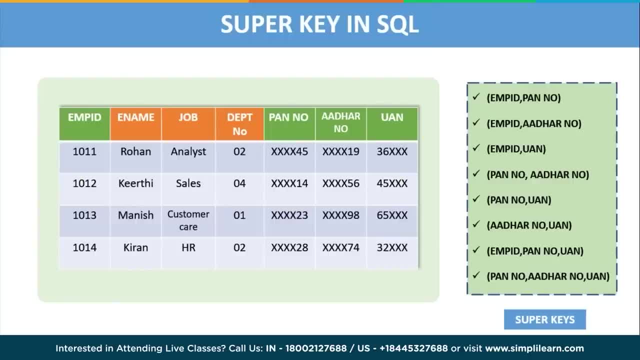 number- employee id- other number, employee id. uan. pan number- other number, pan number, uan. other number, uan. employee id, pan number, as well as un and finally, pan number, other number and uain. now, all the above keys are able to uniquely identify each row, so each of these keys is a super key. now, in this example we have like more than six super keys, but all of them cannot become a candidate key here. only those super keys would become a candidate key which have no redundant attribute. for example, if you take employee id, pan number, this key cannot be considered as a candidate key. 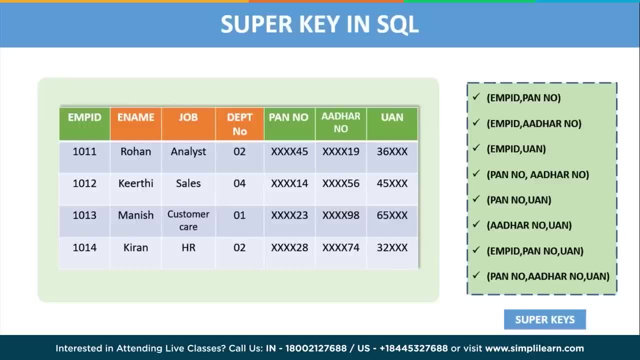 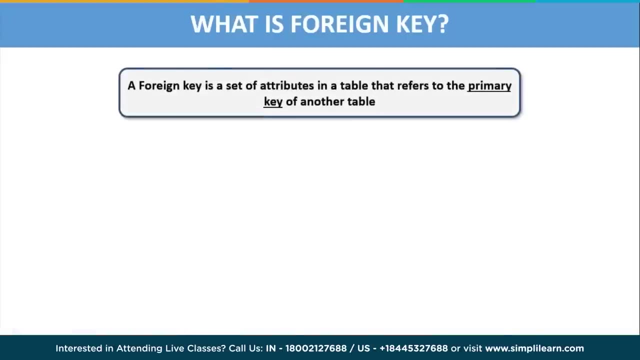 because when we take the subset of this key, we get two attributes, that is, employee id as well as the pan number. now, each of these attributes is basically a candidate key, so it is a minimal super key, but hence this key is not a candidate key. and finally, let us discuss about the foreign. 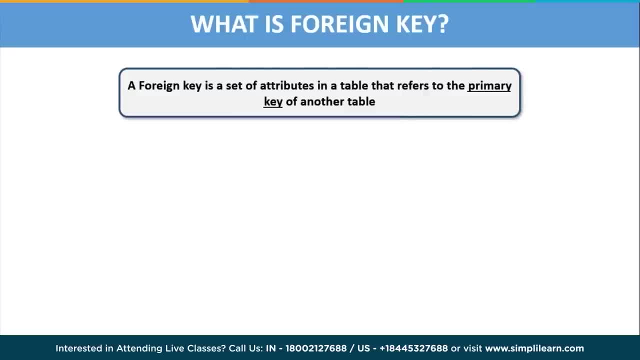 key in sql. a foreign key is a column or combination of columns that is used to establish and force a link between the data in two tables to control the data that can be stored in the foreign key table. in a foreign key reference, a link is created between two tables and the column or columns. 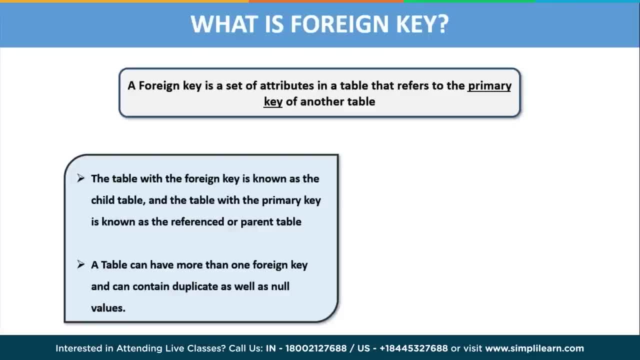 hold the primary key value for one table and are referenced by the column or columns in other table. you Now this column becomes a foreign key in the second table. The table with the foreign key is known as the child table and the table with the primary key is known as the referenced or parent table. 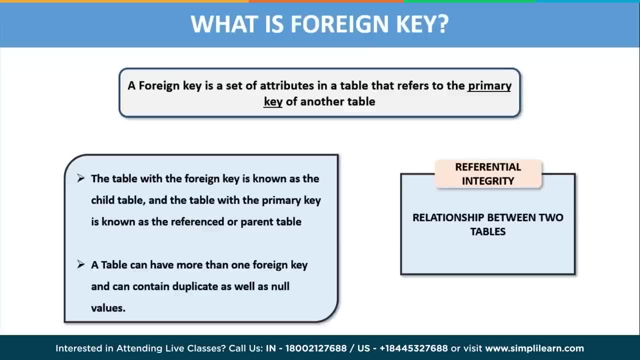 Now a foreign key has bought the referential integrity in SQL, which means that it requires that a foreign key must have a matching primary key or it must be null. This constraint is specified between two tables, ie parent and child, and it maintains the correspondence between the rows in these tables. 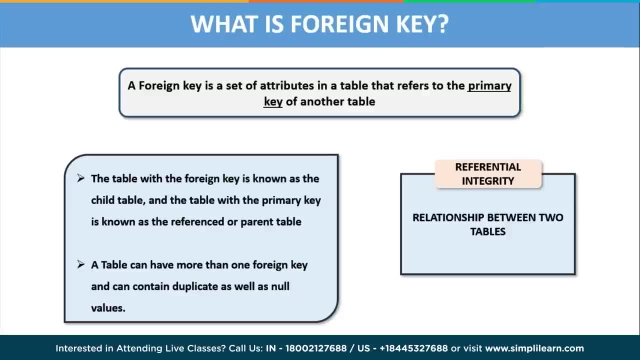 It means that the reference from a row in one table to another table must be valid. Now the foreign key helps in maintaining the data integrity of the table and allows easy navigation between two instances or attributes. It is also used in SQL to make the database data consistent, and it is also used for the prevention of any action that may result in disruptions. 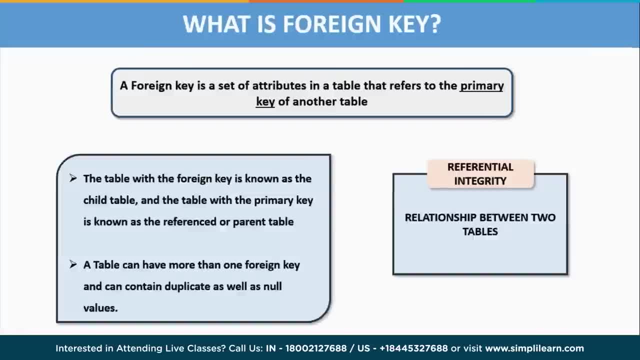 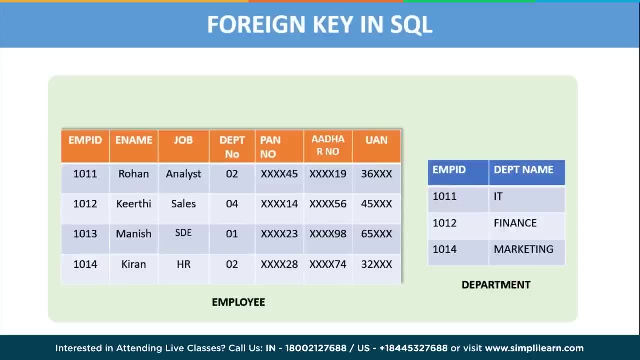 It is also used in SQL to make the database data consistent, and it is also used for the prevention of any action that may result in disruptions. Let us understand this with an example. Now consider two tables here: employee and department. The employee table has employee ID, employee name, job department number, PAN number, Aadhaar number and UN number. 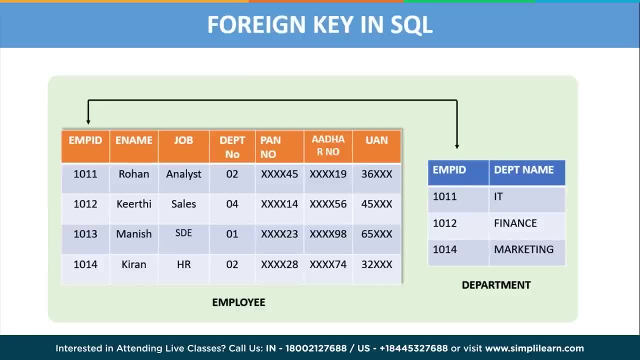 And the department table has employee ID and the department name. Now clearly the employee ID, which is the primary key in the first table- employee- is acting as a cross reference for the department table. That is, the employee ID acts as a cross reference for the department table. 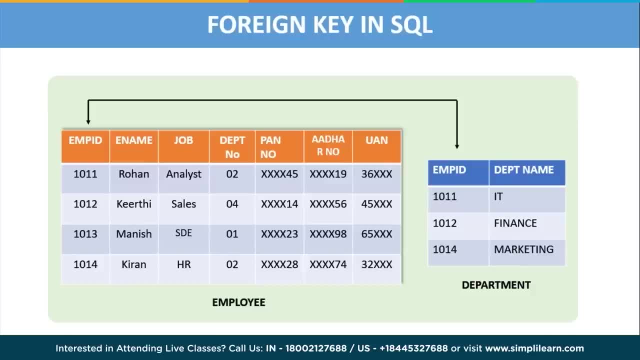 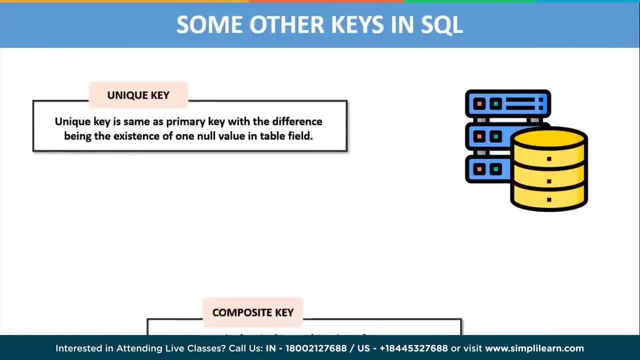 That is, the employee ID acts as the foreign key here for the department table. So in this way you can use the foreign key in SQL. And similarly we have some other types of keys in SQL which are not that significant in its usage, The first one being is unique key. 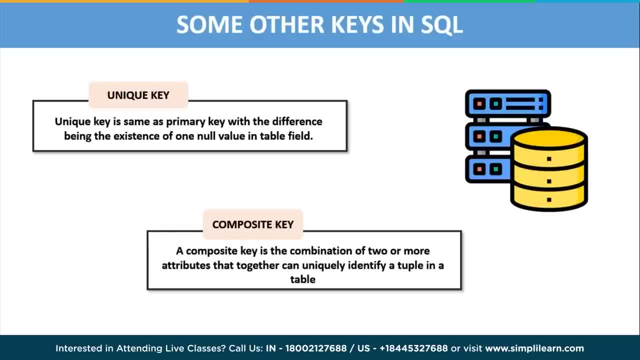 A unique key is same as a primary key, with the difference being the existence of one null value in a table field or a row. For example, consider a student table having student ID, roll number and its name. Now, for some reason, If the student is leaving the school, then his roll number might be deleted, although his student ID will be preserved for further assistance. 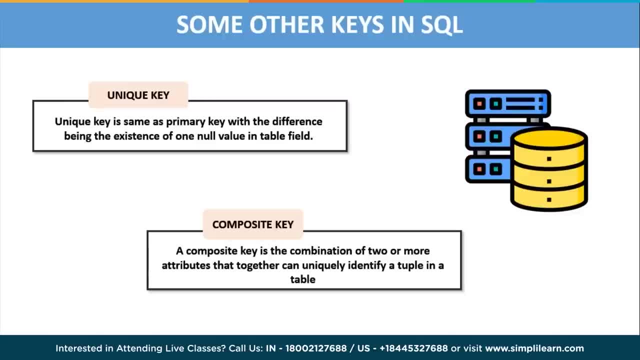 So, since there is a null value in roll number, it can be considered as a unique key and student ID can be considered as a primary key. Similarly, we have composite key. A composite key is a combination of two or more attributes that can together can uniquely identify a tuple in a table. 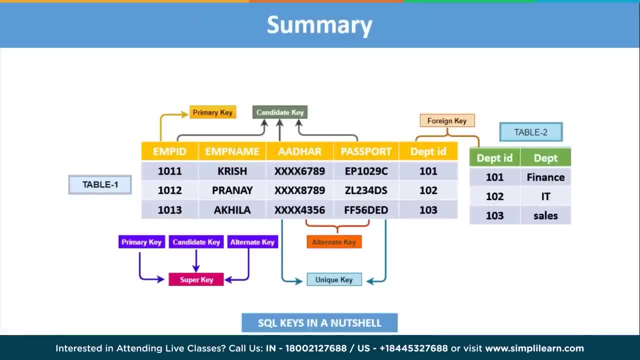 And that brings us to the end of today's session. That was all about The SQL keys, So let us just quickly recap what we have discussed: The different types of keys. So to summarize this, I have created a table here. Employee ID: Employee Name: Aadhar Passport, Department ID: 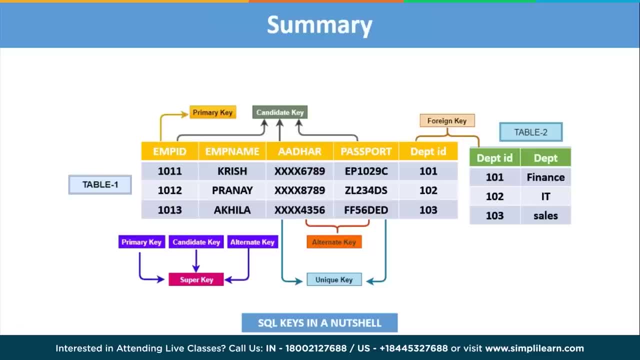 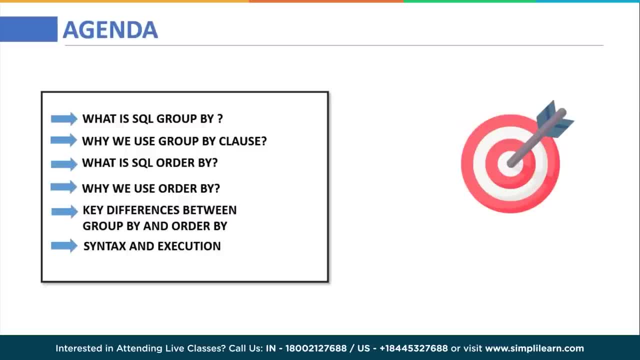 And Employee ID Aadhar Number Passport can be taken as a key And Employee ID Aadhar Number Passport can be taken as a key, And then we'll understand what is SQL order by statement and why we use order by clause. 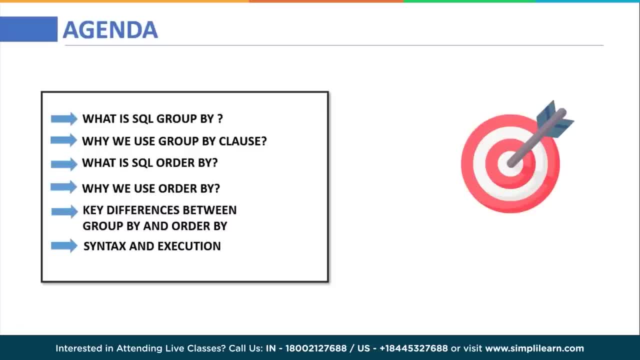 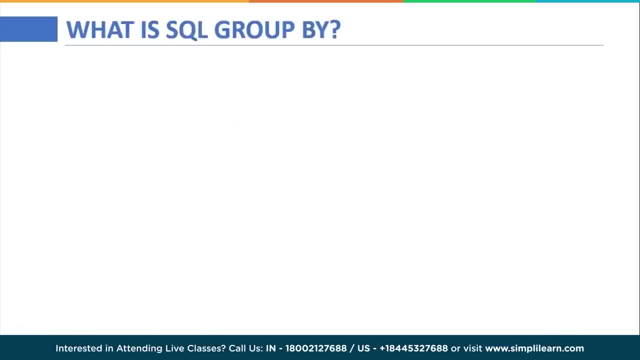 And next we'll see some key differences between these two statements. And finally we'll understand the syntax and look into the execution part in MySQL Workbench. So what is SQL Group Byte Now? SQL allows the user to store more than one type and up to almost 30 types of data types in as many columns as required. 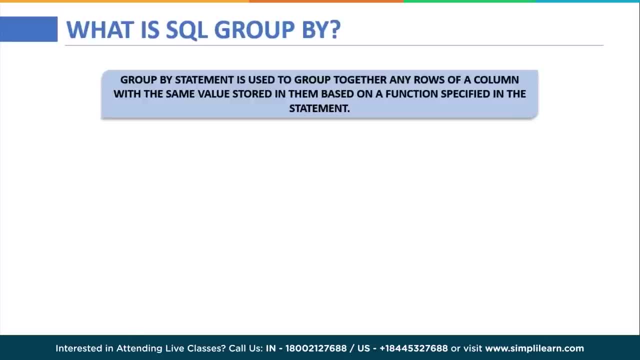 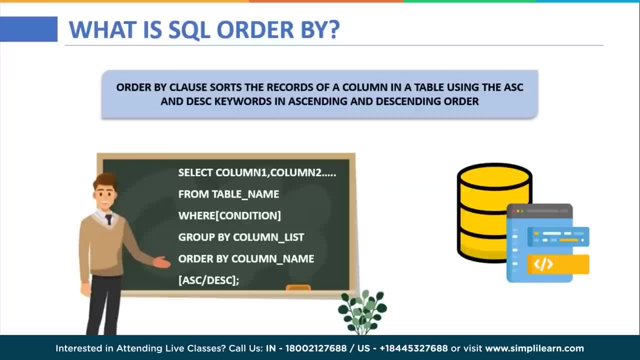 Now, another important thing to be noted here is that the order by statement always appear after the group by statement and is applied to the group of rows formed. Now let us look at the syntax. The syntax is followed as: select column 1, column 2 from table name, where condition, which is optional, as per your requirement. group by column list. order by column name and you can mention the ASC or DESC keyword as per your need. 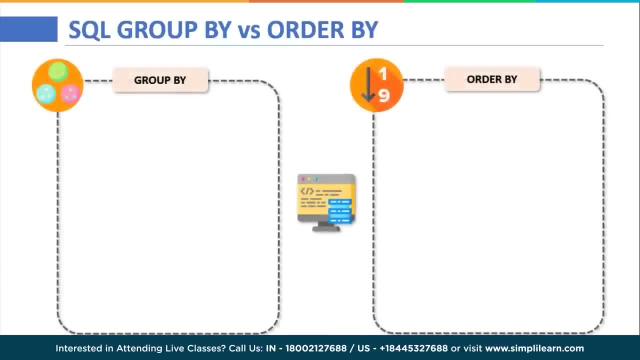 Now that we have understood about both of these statements, let us now understand the differences between group by and order by Now. group by statement is used to group the rows that have the same value, whereas the order by is used to arrange the data obtained in the resultant table of a query in sorted form. 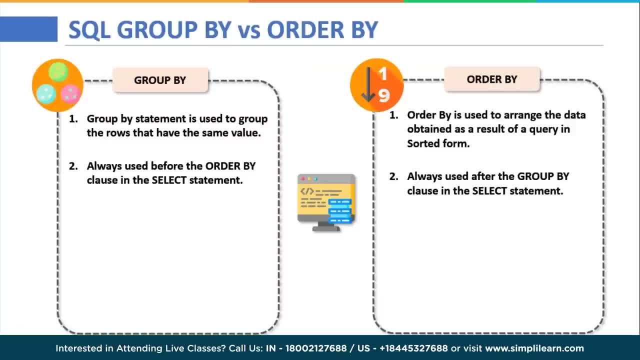 Now the group by is always used before the order by clause in the select statement, whereas the order by statement is used after the group by clause in the select statement. Now, in group by statement the attribute under the aggregate function cannot be in group by clause, whereas in order by, the attribute under aggregate function can be in order by clause. 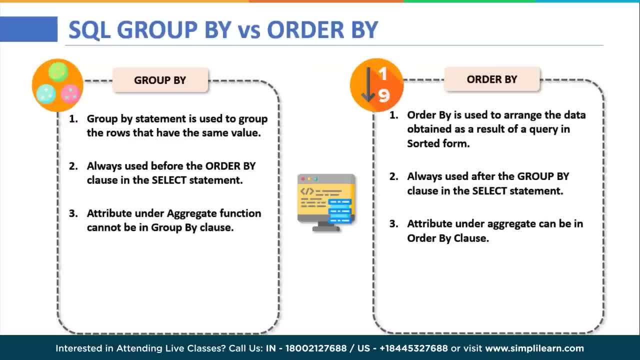 That means if the group by clause contains an attribute that is not under select clause, or if it is under select clause but under aggregate function, then the query becomes invalid and it throws an exception. Hence we can say: the group by clause is always used in collaboration with the select clause. 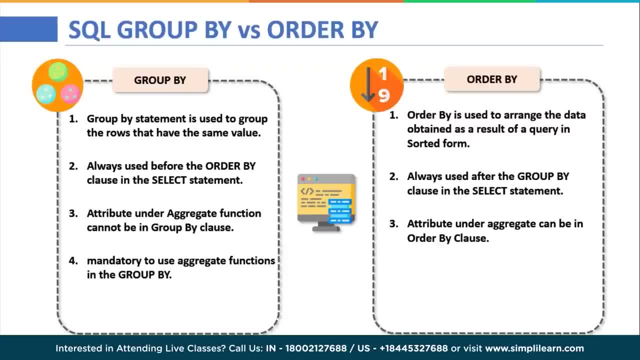 Now, in group by it is mandatory, It is mandatory to use one of the aggregate functions like count, sum, average, minimum, maximum, etc. Whereas in order by statement it is not compulsory and mandatory to use the aggregate functions. And finally, the group by clause controls the presentation of rows or tuples, whereas the order by statement controls the presentation of columns. 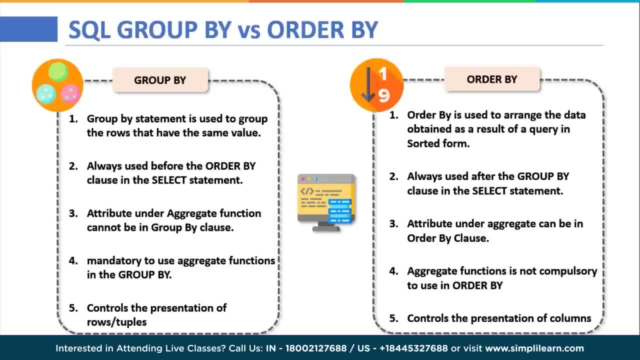 That means the group by is only concerned with the values of identical rows in the resultant set, Whereas the order by statement Basically arranges the data in the columns in either ascending or descending form. Now that we have understood about both these SQL statements, let us jump into MySQL Workbench for execution part. 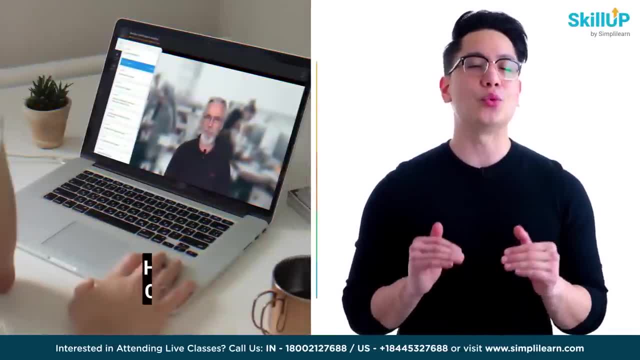 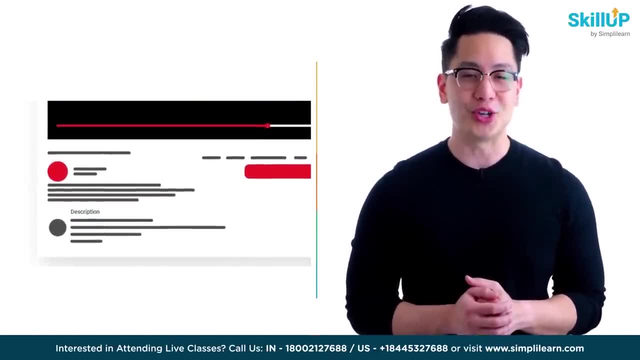 Choose from over 300 in-demand skills and get access to 1000 plus hours of video content for free. Visit SkillUp by SimplyLearn. Click on the link in the description to know more. So as you can see, MySQL Workbench has started. 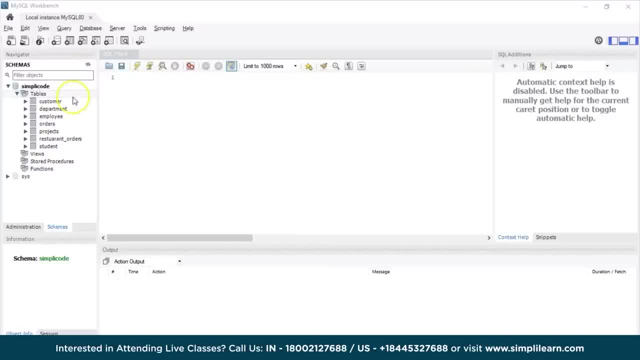 Now, in order to execute the group by and order by statement, We will consider the data set of an employee, which I have already downloaded from Google. So let me just import the data set into the MySQL Workbench. For that, all you have to do is just go to the tables tab and right click on it, and you will find table data import wizard. 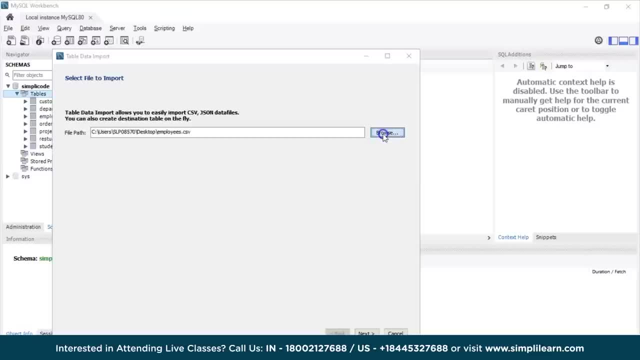 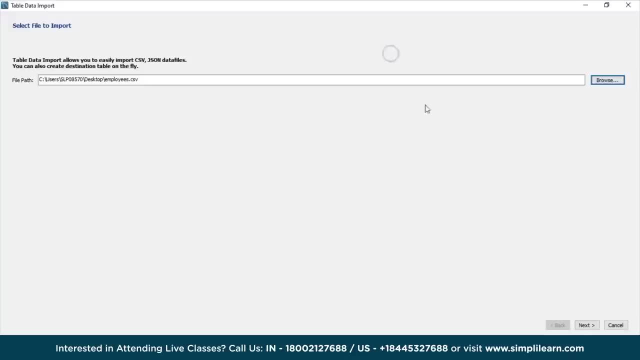 Click on that Now it will ask to import the location from where you have saved. So I have saved my file in desktop, So I am just selecting the file Now. once you have selected the file, click the next button here. Now it will ask if. 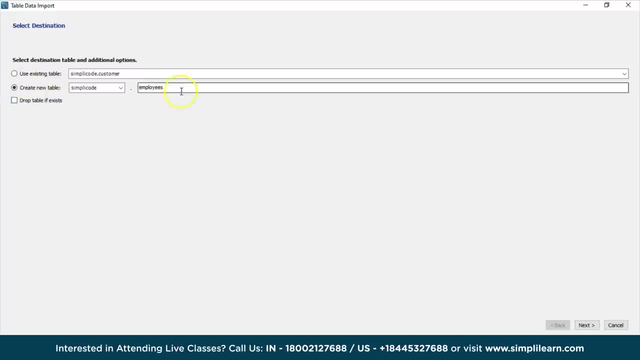 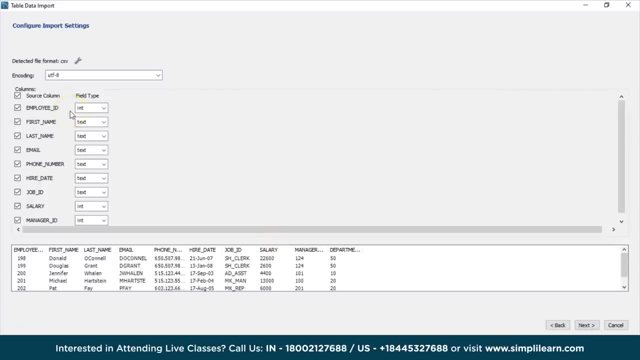 To name the table, whether to use existing table or to create a new table. So I am just taking a new table here, Employees 1.. And click on next. It will display all the columns that are present in that CSV file, So just click on next. 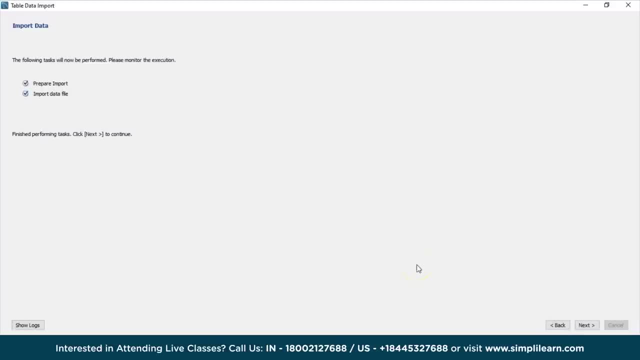 Click on next and it will start to prepare the import Now, depending upon the number of records present in the data set, it will take bit of time, So don't worry. Now, as you can see, our data set has been successfully imported, So we will click on next again. 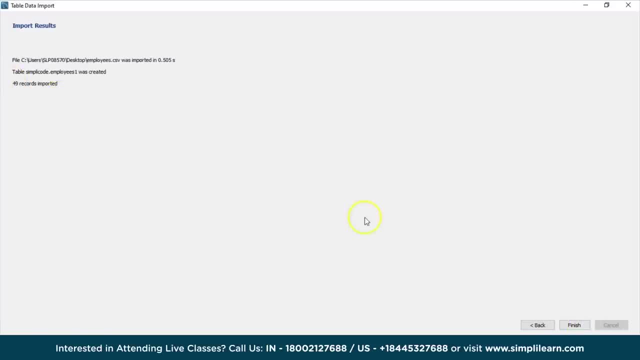 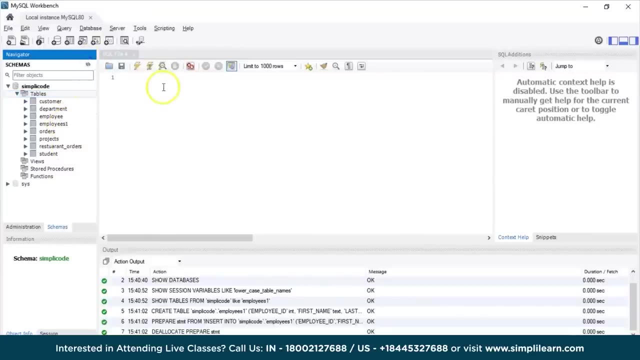 So it is showing that port name records have been imported successfully. So let me just refresh the schema here And, as you can see, employees 1 has been shown in the table section. So let me just display the records that are present in these tables. 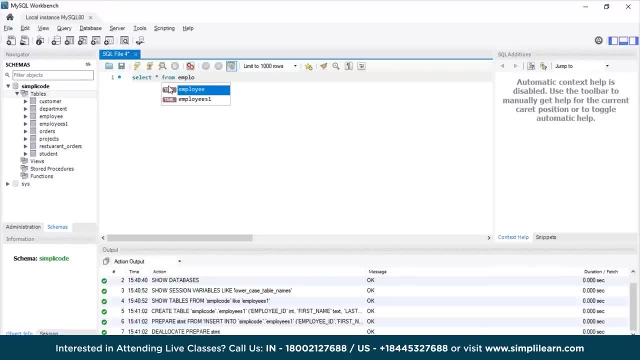 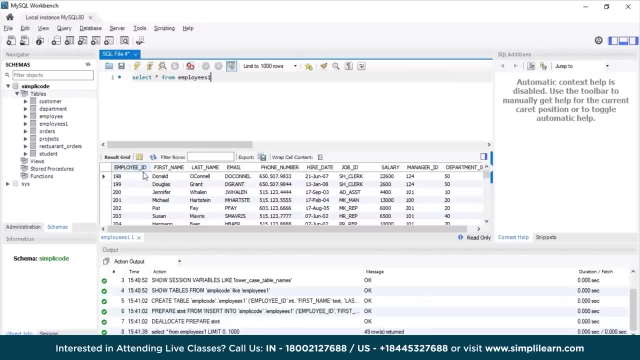 For that I am using this select statement: Select star from employees 1.. So, as you can see, our employees 1 table has been imported successfully. You can see our employees 1 table has employee id, first name, last name, email phone number, hiring date, job id, salary manager id and finally, department id. 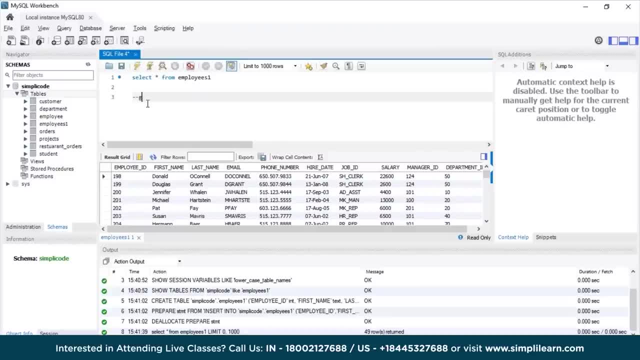 Now, firstly, let us discuss about the group by clause. Now let's say, if I want to fetch the total employees in all the departments from the employees 1 table, Then the following query would be Select: Now I can take the employee id to display the total number of employees. 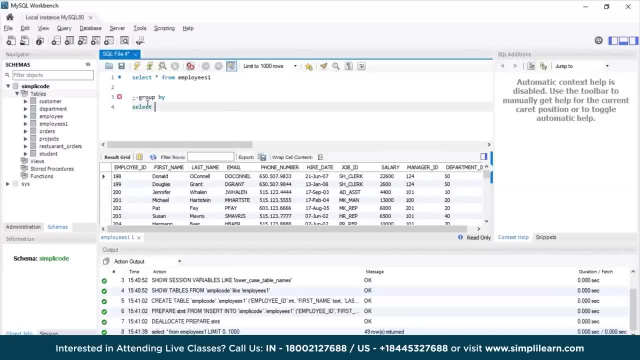 Because each and every employee has a different employee id to their name, So select count employee id as total comma. I want to display their department id as well, So I am taking department id From employees table. Employee 1. Group by. 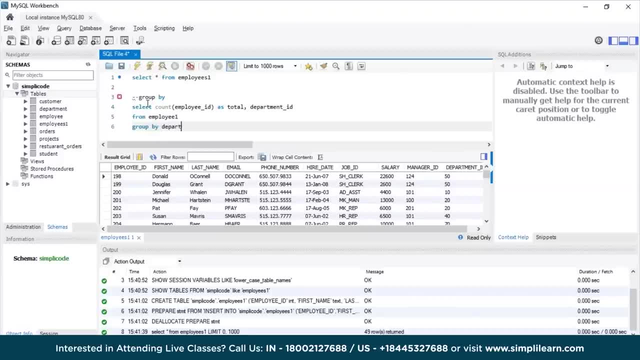 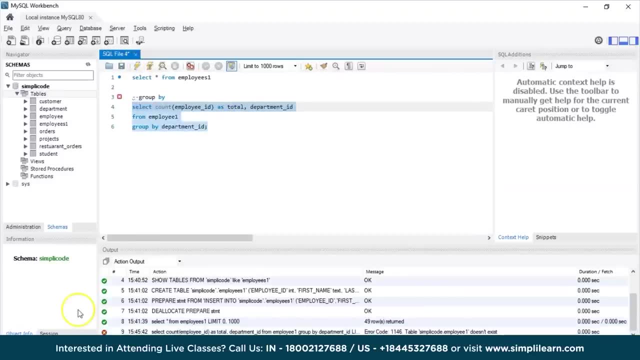 Now we want to group all their department id right, So I am taking department id, So let me just execute the statement and cd out. Okay, The table name is, So let me just correct it So, as you can see, it will display the total employees that are present in each and every department. 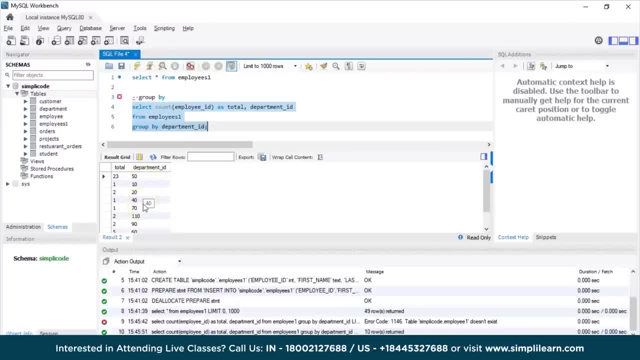 Now, if you look at the department id column, We have the values in a random way. Now, in order to display in a systematic and a proper way, This is where we use the order by statement, So we can sort the department id values in the ascending or descending manner as per a requirement. 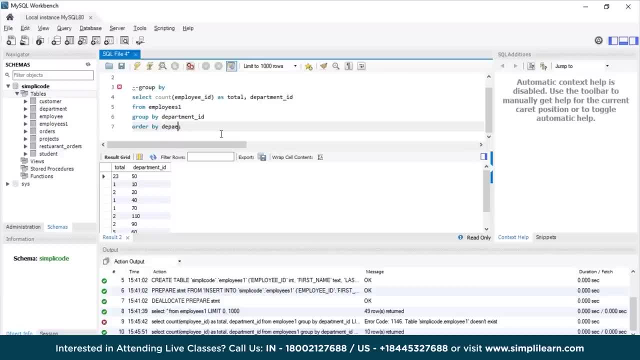 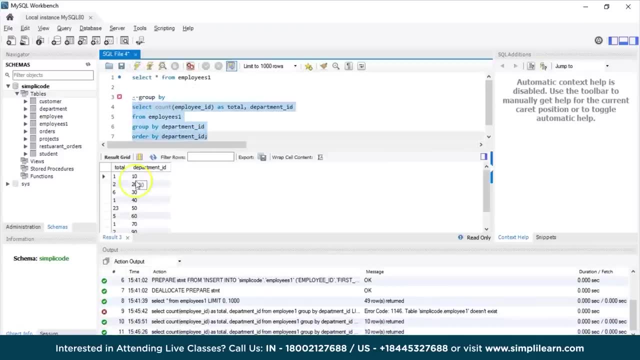 So I want to display an ascending order, So order by department id. Let us execute the statement and cd out. So, as you can now see that the department id are being displayed in the ascending manner, That is, 10, 20,, 30,, 40,, 50 and so on up to 110. 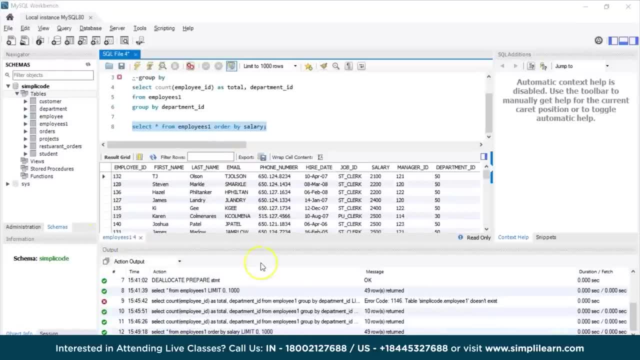 So in this way you can use the group by and order by statements. So that was all about the group by and order by statement. So this is just to give a quick Review on how these two statement works. Now, if you want to learn more about the order by statement, 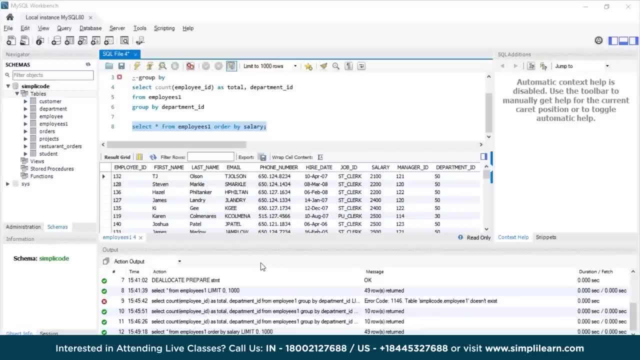 Make sure to check out our SQL order by video on our channel, Where we have discussed about it more in depth and with more examples as well, And also you might have a doubt that when to use group by and when to use the order by statement. 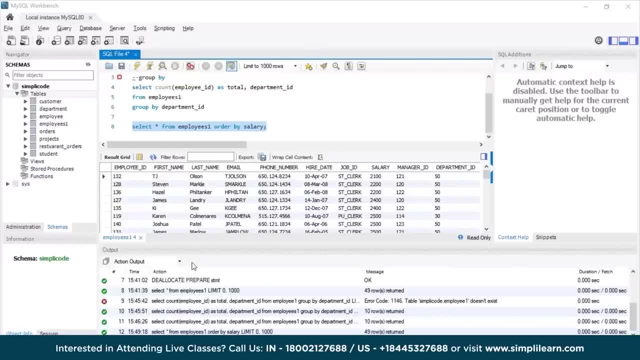 Now, if you want to form the group of the set of records or the identical columns having values in them, Then you must use group by clause. And in case you want to arrange the data of a single or a multiple column with variable, different conditions, 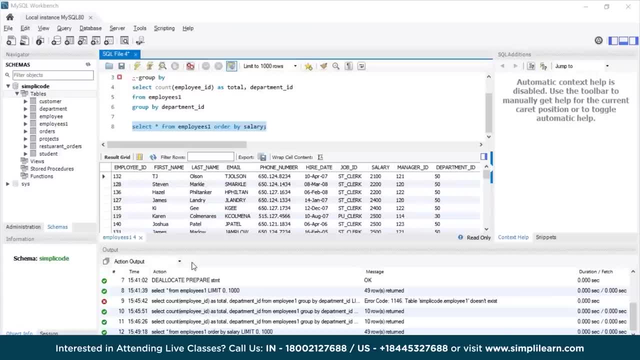 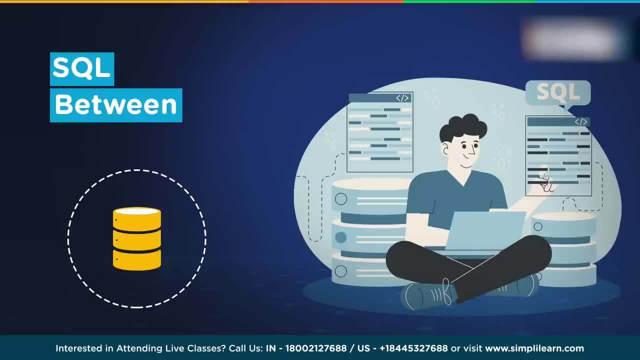 Or in that case, you have to use the order by to sort the data in ascending or descending order. In this session, we are going to learn about between operator and SQL. Now, SQL provides us with many such tools that help in retrieving useful information from all kinds of data. 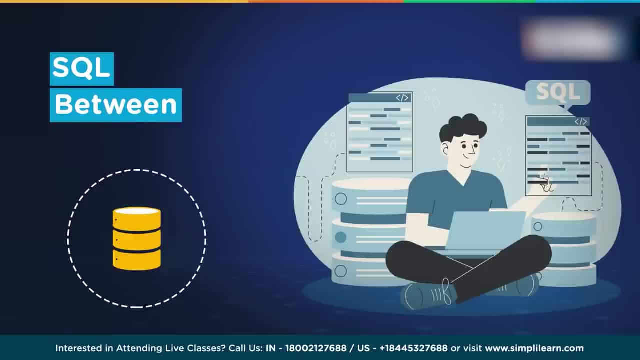 Sometimes we need to retrieve only a particular range of values from all the values of a tables column, For example, to retrieve the information about all the employees of a company born in a particular decade or year, Or let's say, to find the salaries of all those employees in a particular range. 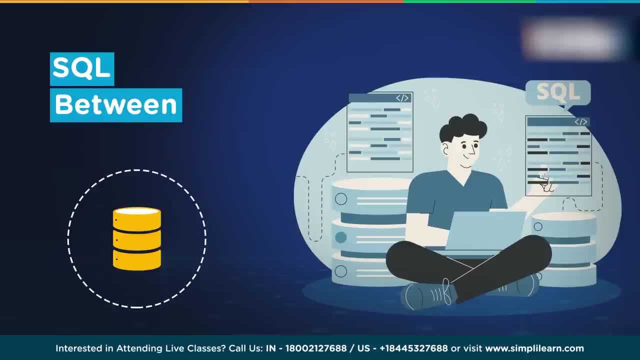 You need a tool for that Now. SQL between operator helps in performing these activities and is an integral part of this query language. So in today's session we are going to discuss about the between operator in detail, with its syntax and execution in MySQL Workbench. 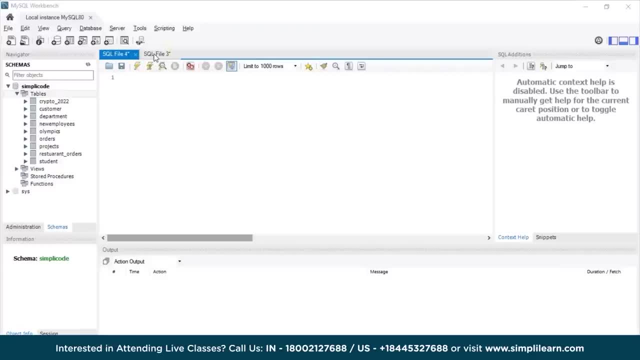 So, without any further ado, let's get started with today's topic. So, as you can see, MySQL Workbench has started and before getting into the execution, but let us just quickly understand what is between operator and SQL. Now, the SQL between operator is used to test whether an expression is within a range of values or not. 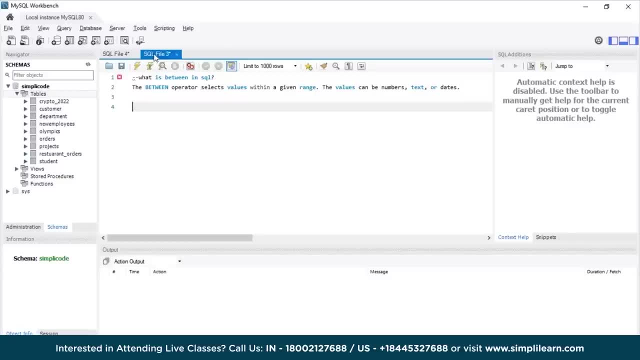 This operator is inclusive, so it includes only the start and end values of the range, And the values can be textual, numerical type or date type. Now between operator can be used with select, insert, update as well as the delete command. So to get a clear picture of how this operator works, Let us get into the syntax of it Now. the syntax is followed as select column names from table name where column name between range start and range ends. So the columns to be retrieved are specified after the select statement and the table columns are being retrieved from the specified is in the from statement. 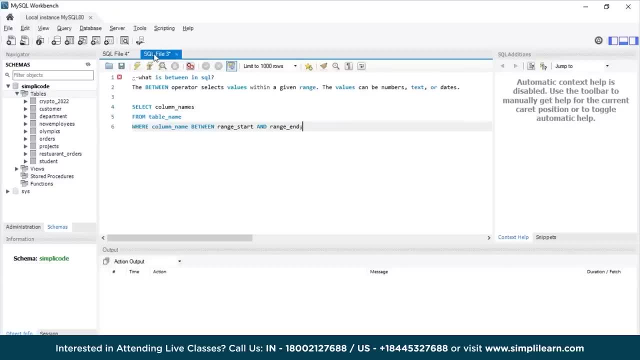 And then we have the between operator, which is used in the where clause. The column we want to apply the range condition on is specified with the column name parameter, And the starting value of the range of values is specified in the range start parameter and the ending value in the range end parameter. 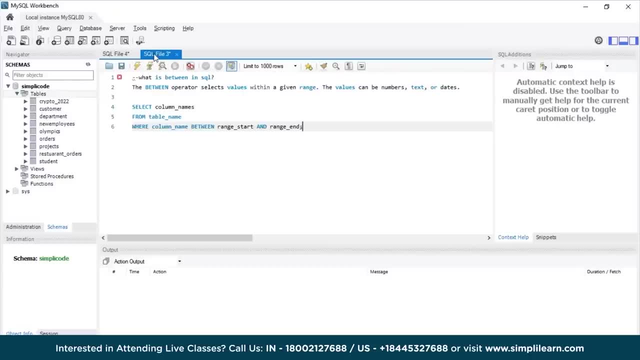 So now that we have understood how exactly the between operator works, Let us get into some examples and understand its execution part. So let us take an example to understand the SQL between operator. So I am taking the new employees as the example here, So let me just display the values. 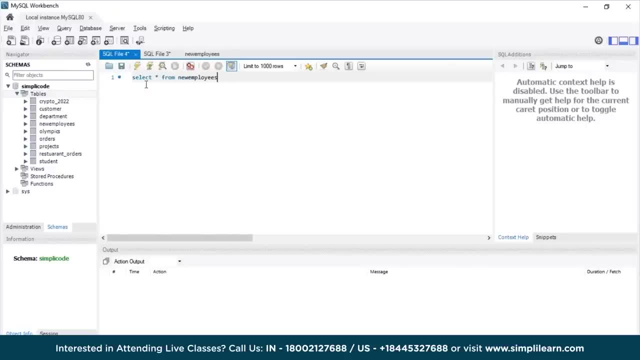 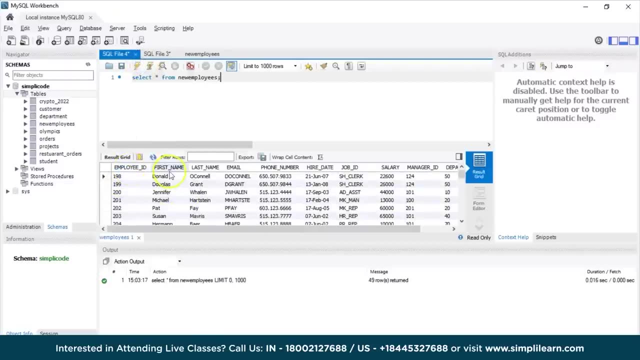 For that I am using the select operator, Select star from new employees. Let us execute the statement. So the new employees table has various columns such as employer id, first name, last name, email phone number, hiring date, job id, salary manager id, department id. 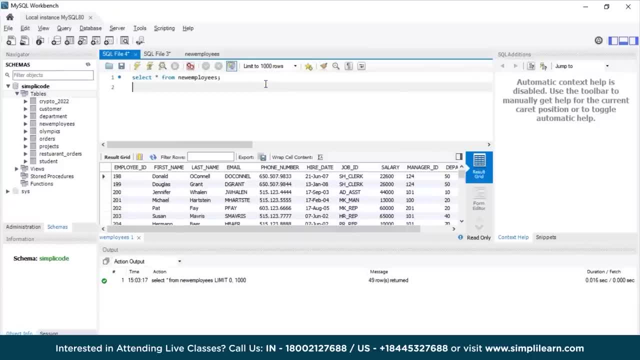 That's it. So now we will take a simple example to understand the between operator. So let us say, if you want to retrieve the id and name of the employees with ids in the range, Let us say, now we have ids up to range like 198,, 200,, 201.. 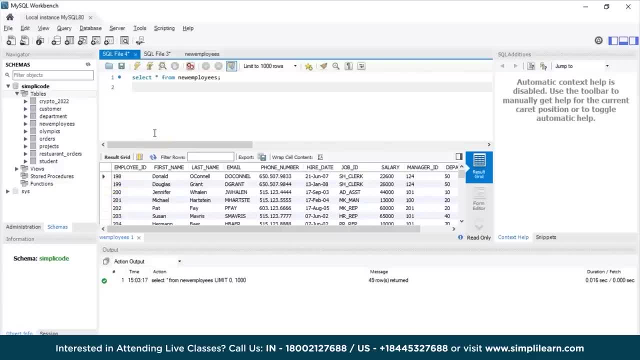 So let us take the range between 110 and, let's say, 170.. Then we will use the following query as select employee id first name from table. that is, new employees Use the where condition where employee id Between is the keyword 110 and 170. 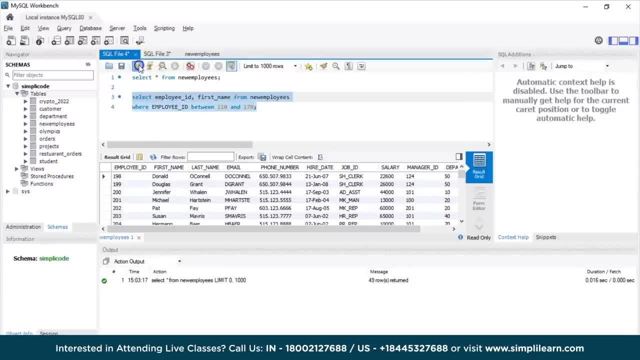 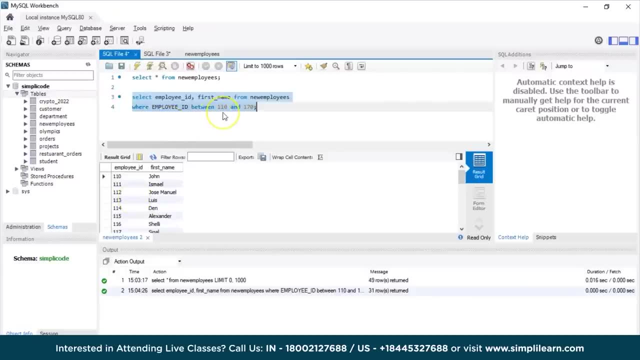 So let us execute this and we will see the output. So, as you can see, it will display the records of all those employees whose employee id lies between the range that is, 110 and 170.. Now, if any employee who is having their employee id as 110, even their values are also included in the resultant set. 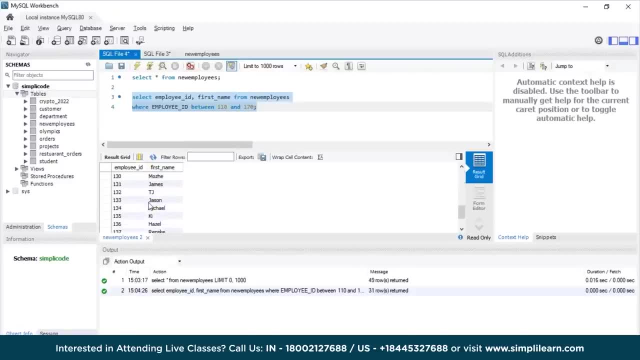 And similarly, if any employee has 170 in there as their resultant set, Even their data will be in the resultant set. Now in the table we do not have any employee who is having the employee id as 170. So we do not have the information now. 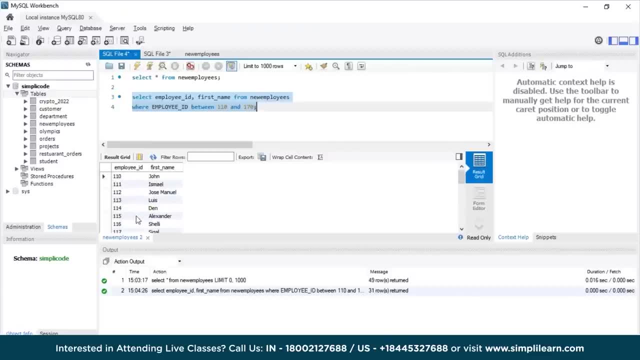 So in this case it will only display only the details of all those employees who is having the employee id range in 110 and 170.. Well, moving ahead, let us take next another example. Now we can use the order by statement also to sort the result based on some columns. 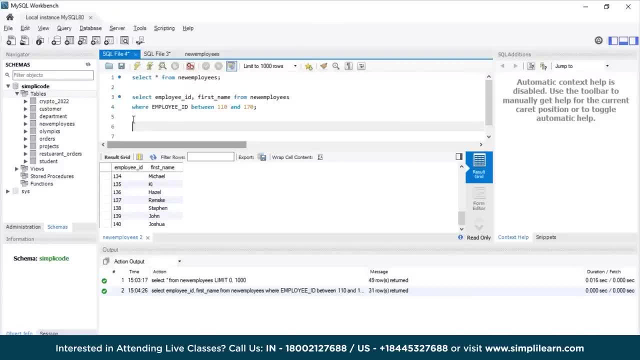 Now, let's say, if you Want to retrieve the details of all those employees with salary ranging from 35000 to, let's say, 75000. And in order to sort this result based on the salary, we will use the following query as Select: 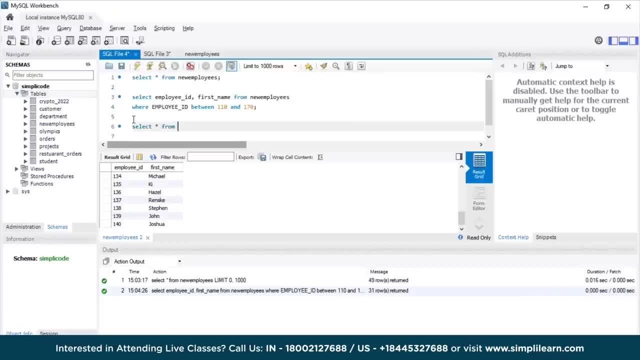 I want to display all the details, so I am using the star operator: Select star from new employee Where Salary Between 35000.. And Let us take, let's say, 55000.. Right, And I'll use the order by. 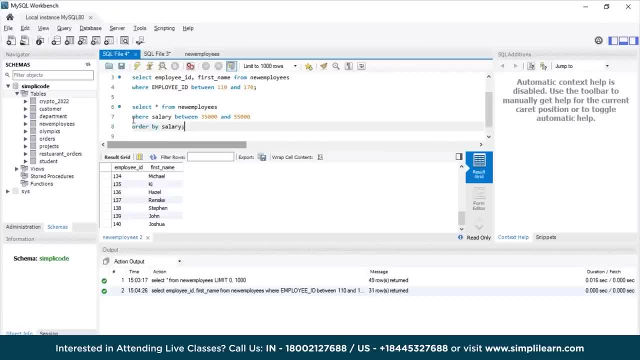 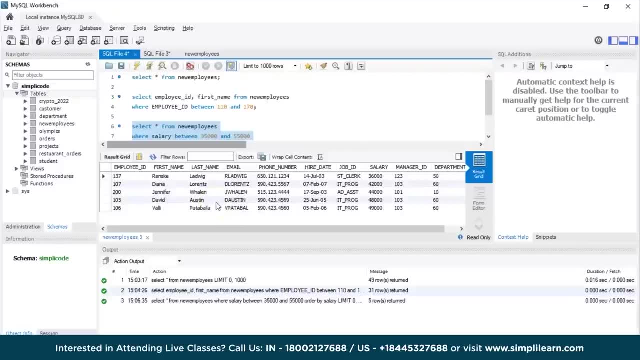 Salary So that it will display the values of all their salaries in the ascending order. So let us execute and we'll see the output. So, as you can see, there are only Five employees in our new employees table, For example, Renske Ladwig, who is working. 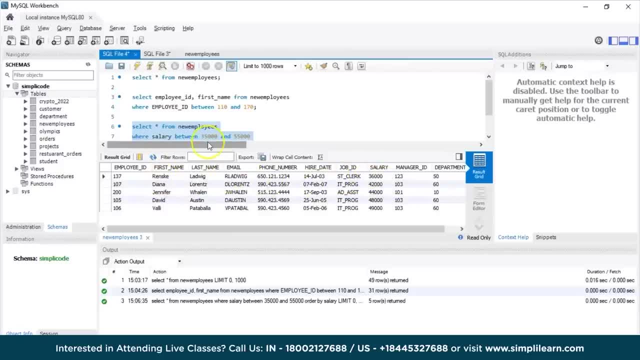 As a clerk, Is having salary 36000.. Which is in the bracket of 35000 and 55000.. Similarly, we have Diana Lawrence, whose salary is 42000.. Similarly, we have Jennifer Valen, whose salary is 44000.. And so on. 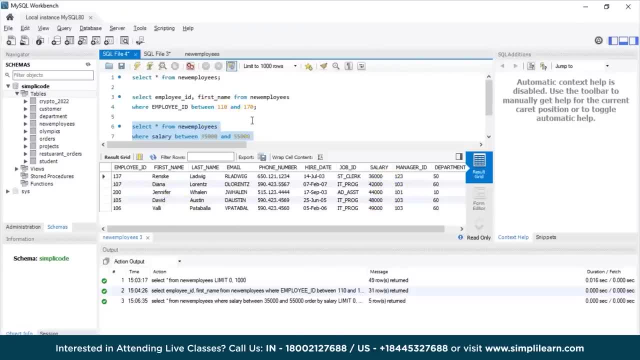 So in general we use the between operator to find the range of values, Like, for example, we are finding the salary range right. So in a similar way we can use the between operator To find the range between Two given values of a particular column. 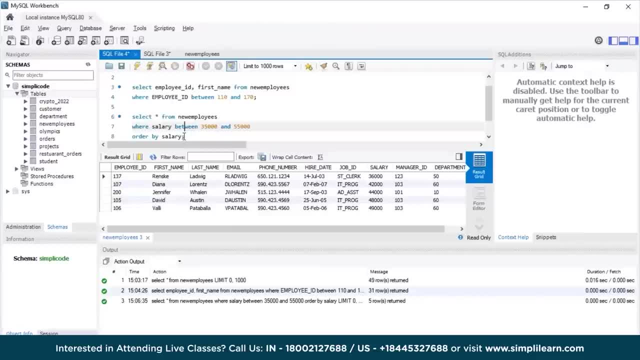 Now, similarly, we can use the not operator With between as well. Now we can also use the not operator with the between operator To select the values that do not belong to that specified range. Now, instead of using between, If I mention the not between keyword here. 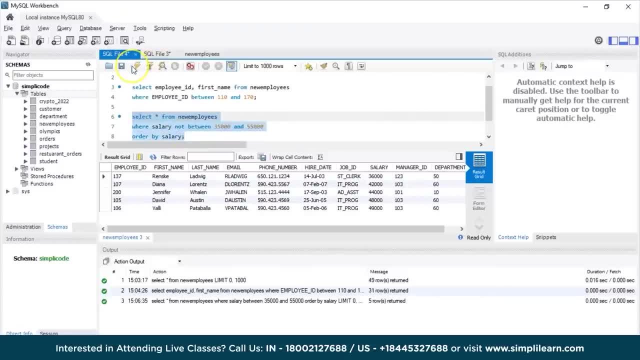 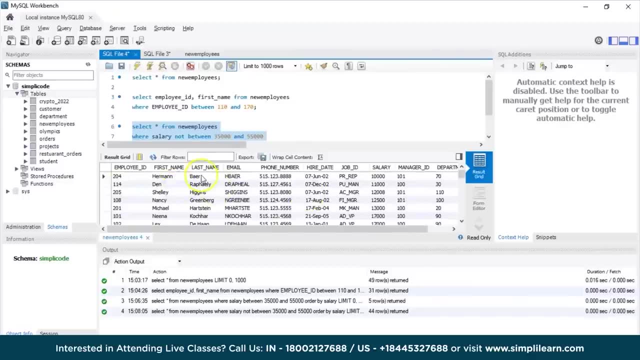 It will basically display all those records of employees Whose salary is not in the range of 35000 and 55000.. Now it will display the records of all those employees, Like if you take Herman Baer, Whose salary is 10000. 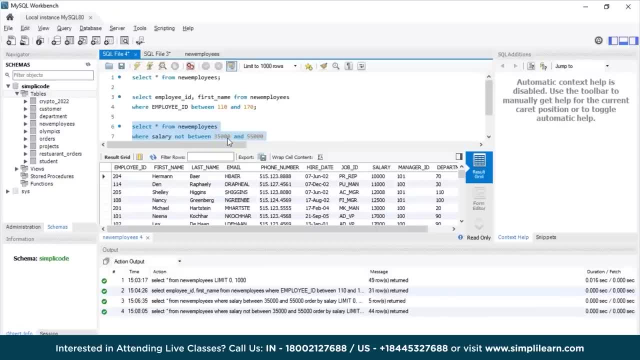 Which is not in the bracket or in the range of 35000 and 55000.. Similarly, it will display the records of all those employees Whose salary is not in between that range, Which is 35000 and 55000.. In this way, you can use the not between keyword as well. 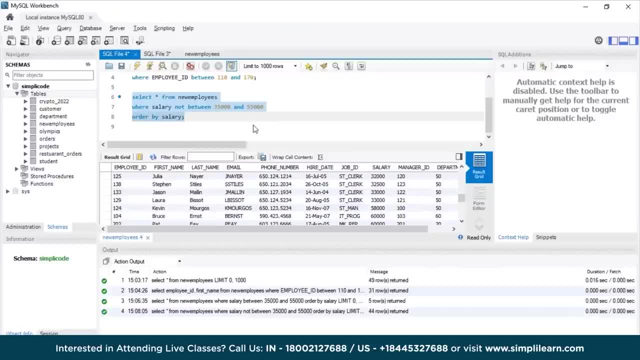 Which will exclude the results that are not in the given range. Now you can use the between operator with the date values as well. Now, when using the between with dates or the date time values, We need to remember to enclose the date in single inverted commas. 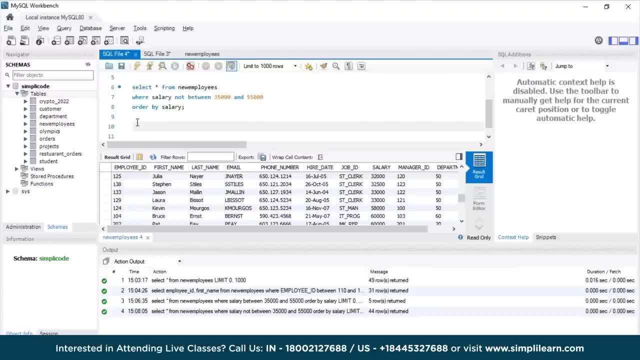 As otherwise the query will return a syntax error. So let us take an example here. Let's say, if I want to retrieve the details of all those employees Whose hiring date is in between, let's say, 2000 and 2007.. 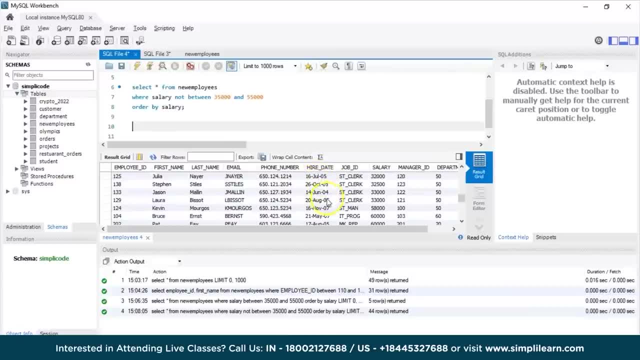 Now, as you can see, our hiring date is between like 2005,, 2004,, 2002 and similarly, etc. So in that case, I want to display all those employee details Whose hiring date was in between 2000 and 2007.. 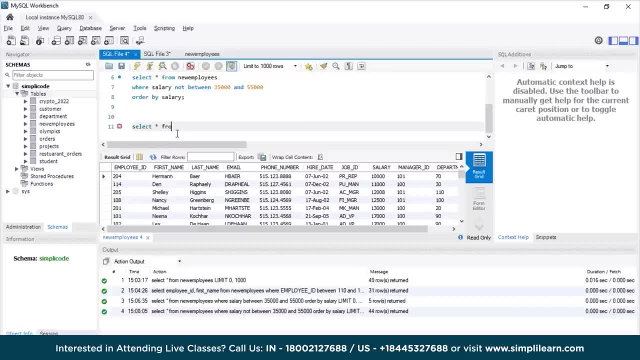 So in that case the following query would be: select Start from new employees again, Which will display all the records Where hire date between Mention the inverted commas. So I will take from 1st January 2000 and 31st December 2007.. 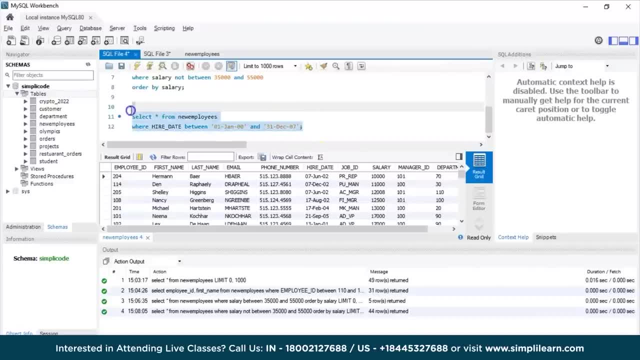 Right, So let us execute this statement and we will see the output. So it will display me the records of all those employees Who have their hiring date in between this range, Which is January 1st 2000 and 31st December 2007.. 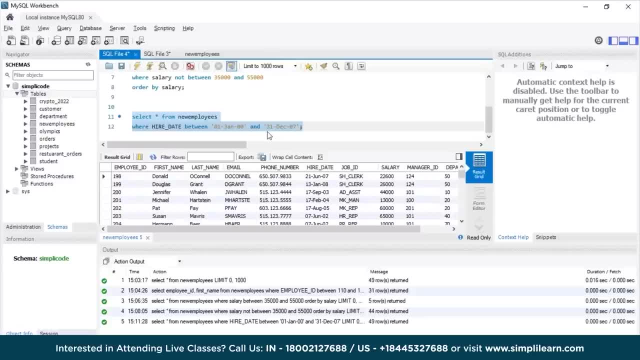 So in this way, you can use the between operator with the date values as well. Right Moving ahead, Now we can use the between operator with the text values as well. Between operator can also be used with the character data types, Like, for example, while using any text values. 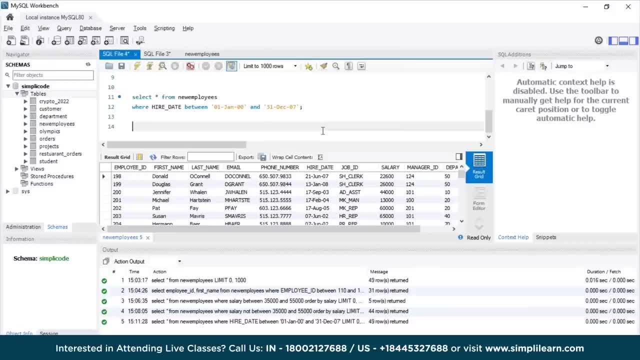 We need to remember to again enclose the data In single inverted commas, Otherwise it will return a syntax error. So let us take an example here. Let us say we want to retrieve all the employee details And along with their names, Belonging to a range from, let us say, alphabets A and J. 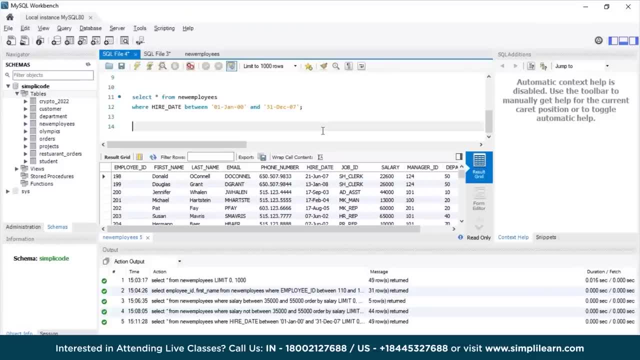 That means we want the details of all those employees Whose name is in between the first letter, that is, A, And the letter J. In that case, the following query would be: Select star From new employees Where I am taking first name. 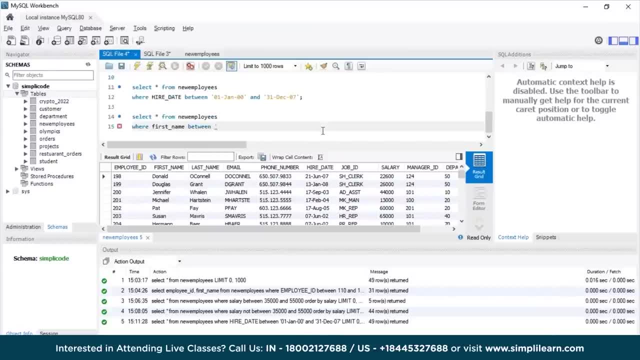 Right first name Between Letter A And letter J, Enclose them in the inverted commas And we will see the output now. So let us also order. We will use the order by statement so that we will have an ascending order. 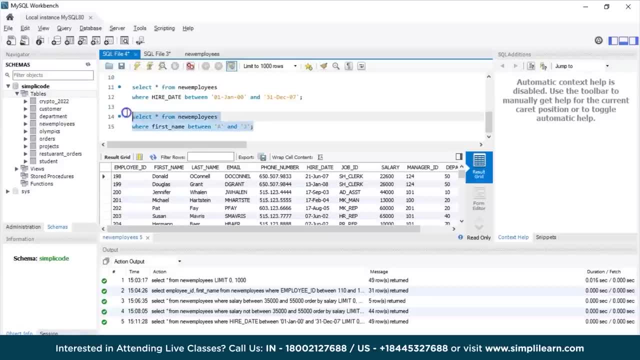 I think there is no need for that, So we will just directly Execute this. So, as you can see, It will display the records of all those employees Whose name is in the range With starting letter A And the starting letter J. 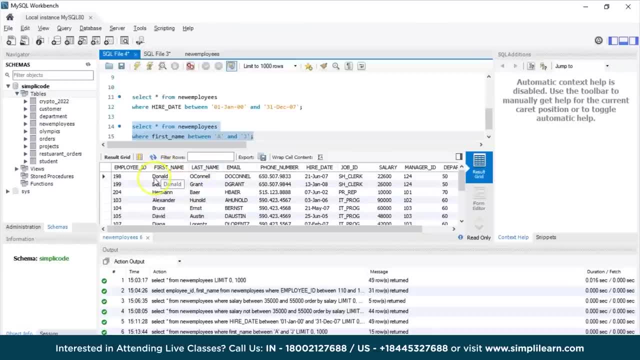 Now you can see Donald O'Connell, Whose first name starts with D Right. So it is in the range of A and J. It lies between A and J, And similarly we have Herman, We have Alexander And David Guy Hemero. 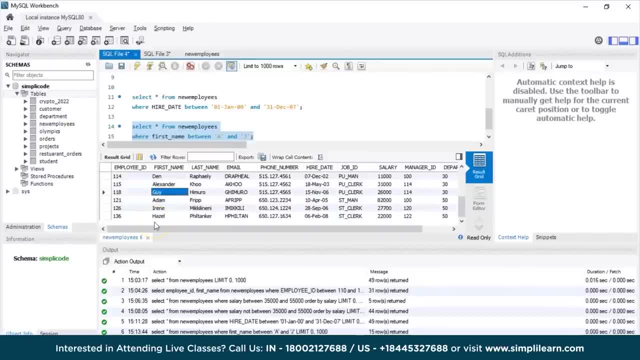 Etc. So in this way You can use The between operator To find the values In a particular range Which have only text Data types. And that brings us to the end of today's session. guys, That was a quick tutorial on how to use the between operator in SQL. 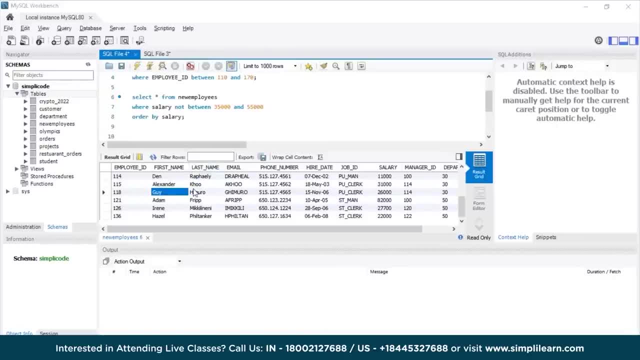 If you remember all the SQL between operator rules and syntaxes, You can easily customize your queries to retrieve the type of information that you want. This tool, along with other SQL tools, Enables us to write different kinds of essential queries. Now the between operator is generally used to find: 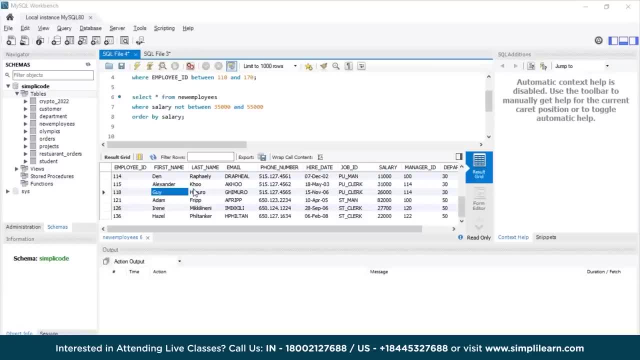 The values Of the data types And it is also used to write The values of the two words. So that means You can easily customize your queries By using the between operator And you can easily customize the values Of the two words. 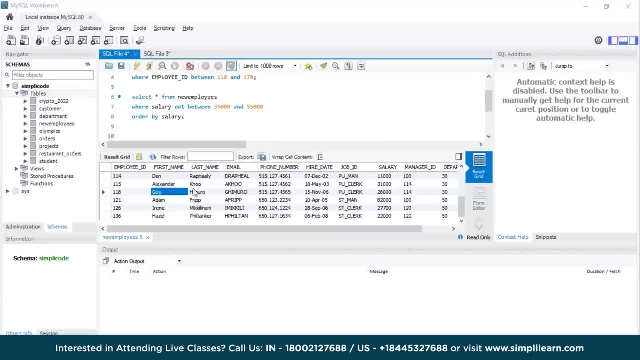 And you can easily customize your queries To retrieve the type of information that you want. enables us to write different kinds of essential queries. Now, this between operator is generally used to find the values within a certain range. For example, you can find the salaries of employees within a certain brackets. 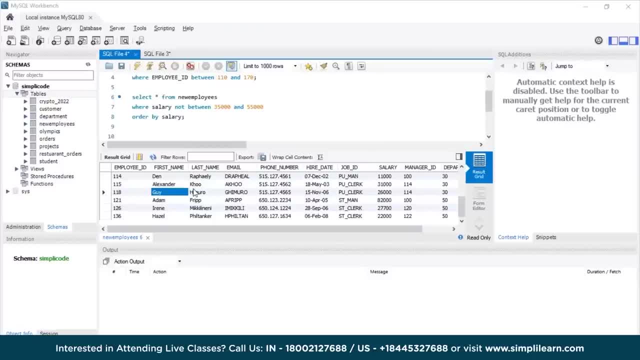 You can also find the marks of the students in a particular range And similarly, you can find the details of the products which lie in a certain range. So in all these cases, you can use the between operator as per your requirement. So now that you know about the between operator, 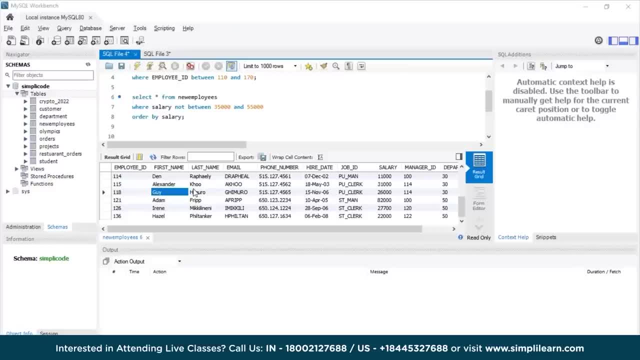 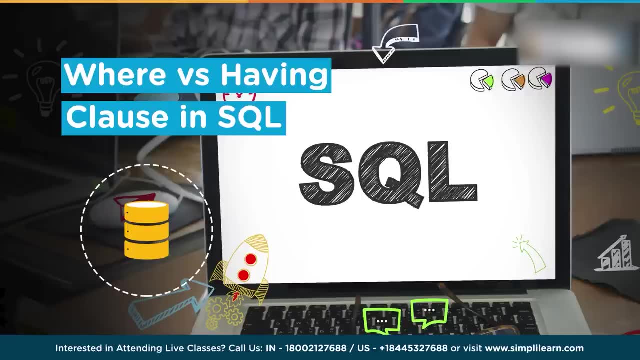 it is time for you to start using the between operator, along with other SQL commands, clauses and operators, to query your database tables. In today's session, we'll have a detailed comparison between the where and having clause. Now let's say you're navigating through a huge database. 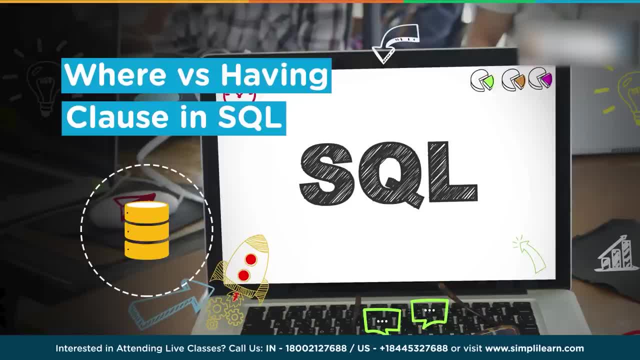 and you wish to display only certain records that satisfy a particular condition. Now, carrying this search process is extremely difficult and is also time taking. Now, in order to save time and make your search easier, we use the where and having clause, which is used to explicitly filter out only those records. 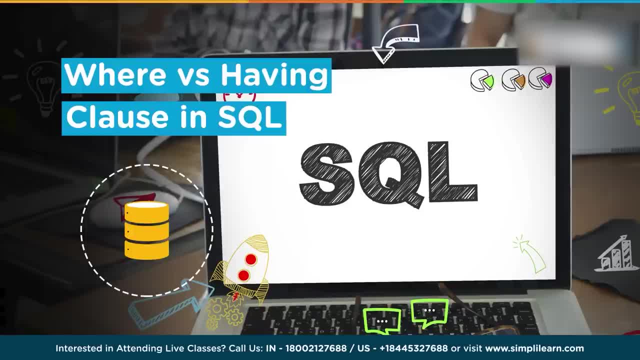 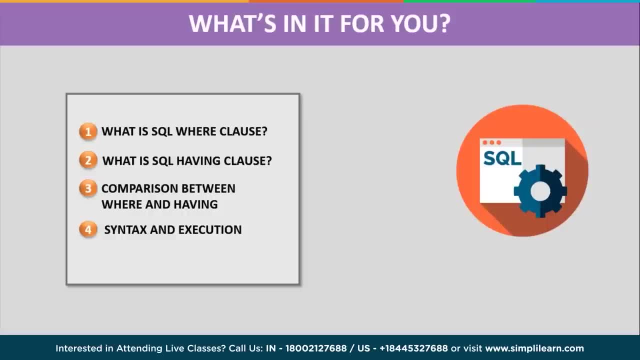 that meet the conditions specified by the user. More on that soon. Firstly, let us discuss the agenda for today's session. We'll start the tutorial by understanding what is SQL where clause and then we'll discuss what is SQL having clause and then we'll have a detailed in comparison between where and having clause. 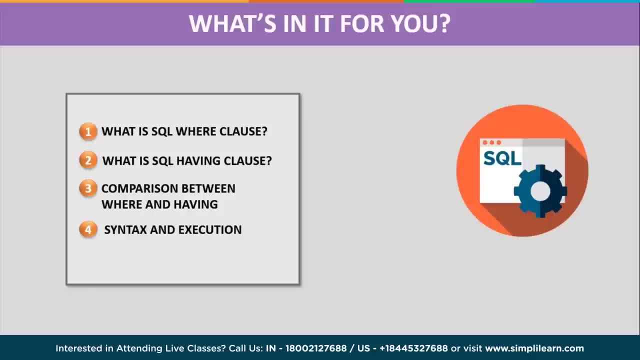 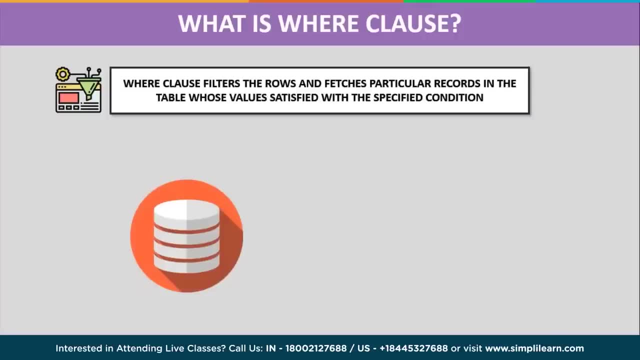 And finally we'll look at the syntax and implement the execution part in MySQL Workbench. So let us now dive into today's topic. So firstly we'll discuss what is where clause: The SQL where clause is used to specify a condition while fetching the data from more than one table. 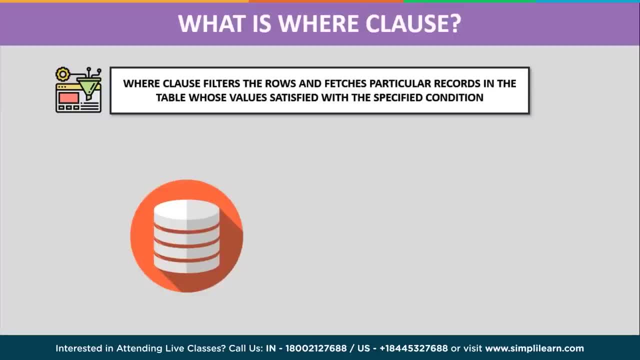 or by joining with multiple tables. If the given condition is satisfied, then only it returns a specific value from the table. Now we can use the where clause to filter the records and fetch only the necessary records from our database. The where clause is not only used in the SELECT statement. 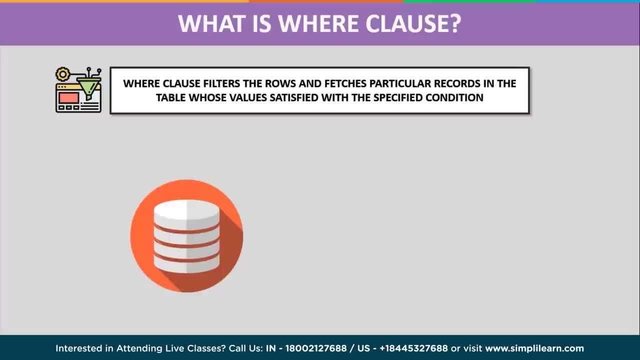 but it is also used in the update, DELETE, etc. Let us now understand the syntax. The syntax is simple and is followed as SELECT, column1,, column2, so on from table name where condition. Let us now understand with an example. 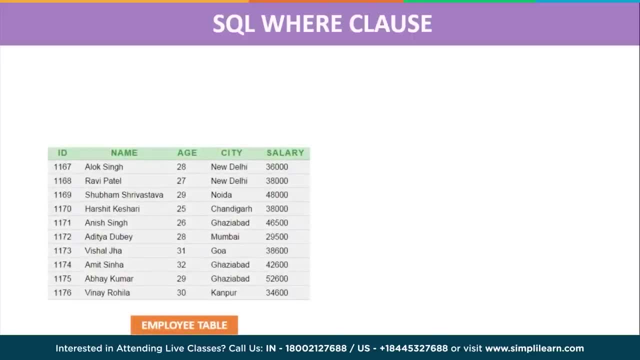 Consider the employee table here, which is having various columns such as ID, name, age, city and salary. Now, let's say, if I want to find the employee who is having the maximum salary in this table, And for that I'll, 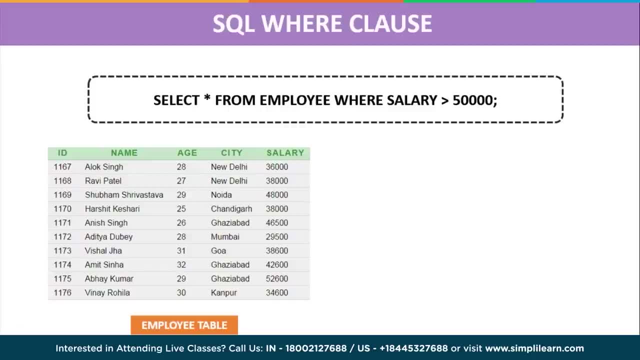 write a query stating SELECT star from employee where salary is greater than 50,000.. Now, if you implement this query, it will basically show those records, which is having salary more than 50,000.. Now, if you look into the table, Abhay Kumar, whose ID is 1175, is having 52,600, which is greater than 50,000.. 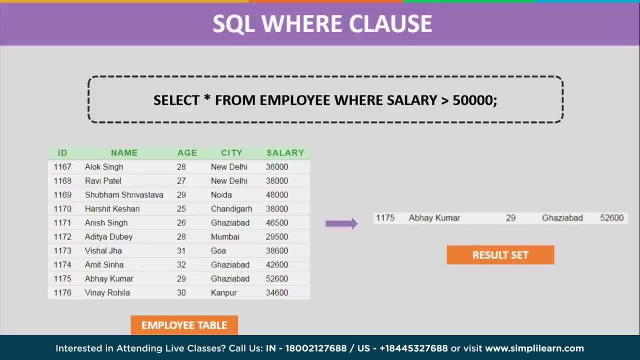 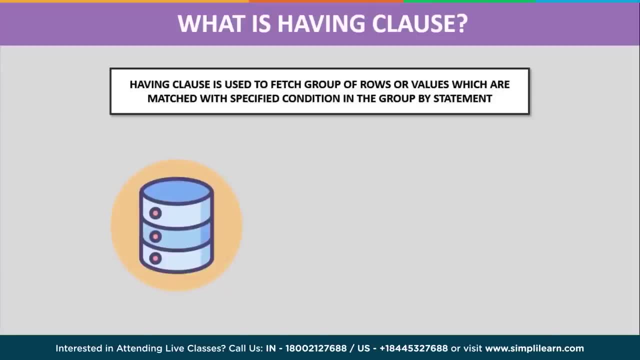 So, in this way, where basically meets the condition that is set by the user. Let us now understand what is having clause in it. What is having clause? in SQL, The having clause is generally used along with the group by clause, And having clause is used to filter the results obtained by the group by clause based on some specific condition. 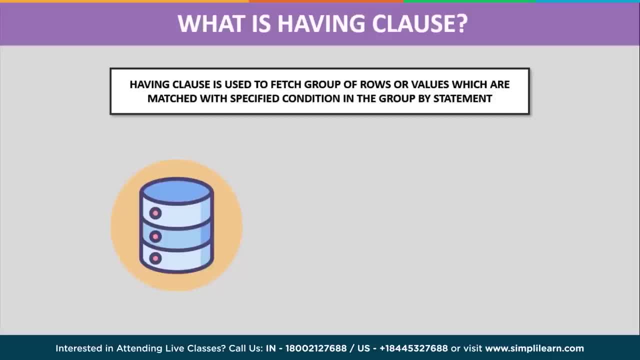 Having clause is quite similar to that of where clause, as both are used to filter records in SQL, But where clause cannot be used with the aggregate functions like COUNT, MAX, SUM and etc. Which is why having clause is needed and that is the reason we use the having clause. 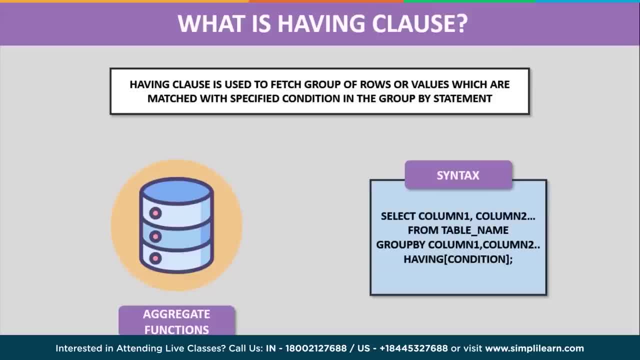 Let us now understand the syntax. The syntax is also similar. You have to mention the having keyword here instead of where, And the syntax is followed as: SELECT column 1, column 2 from table name group by column 1, column 2, so on having and mention the condition. 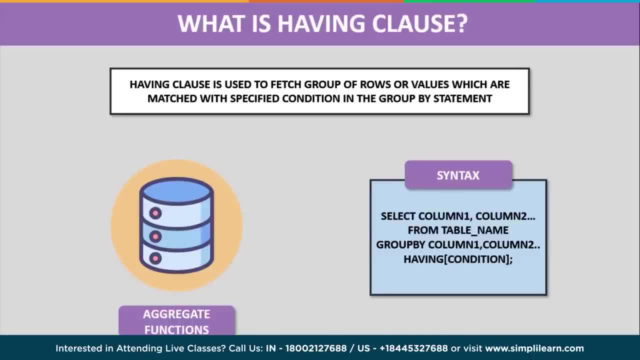 Now, group by clause is used to arrange the data into groups, and having clause is used in the column operations And it basically group all the identical data and gives you the condition that is specified by the you. Let us understand this with an example. 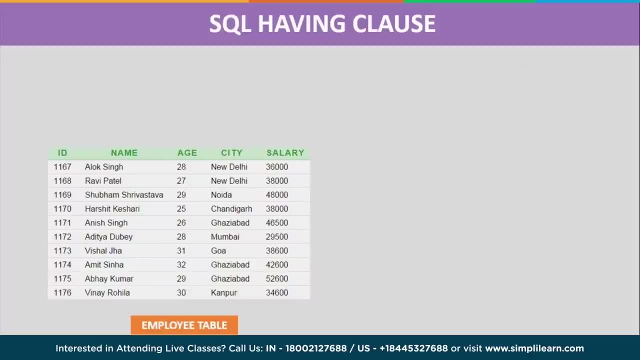 Again, consider the same employee table here, which is having ID name, age, city and salary. Now, as we know, we have to use aggregate functions, So I am using the average function here, And since the having clause also uses a group by, so that is the reason I am also using the group by. 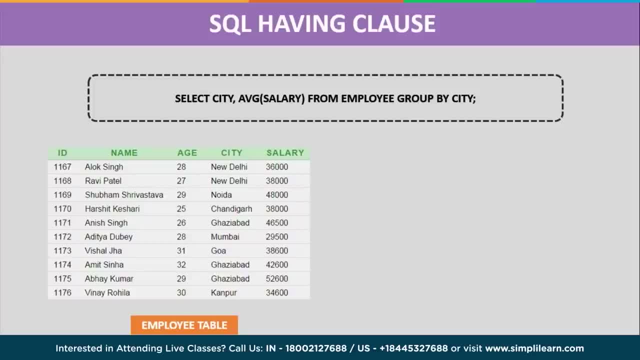 Now, let's say, if I want to find the average salary of all the employees from different cities, Then the following query would be: SELECT city average salary from employee group by city. Now, when I perform this query, this will be the following output, where it will show the resultant set of all the cities and their average salary. 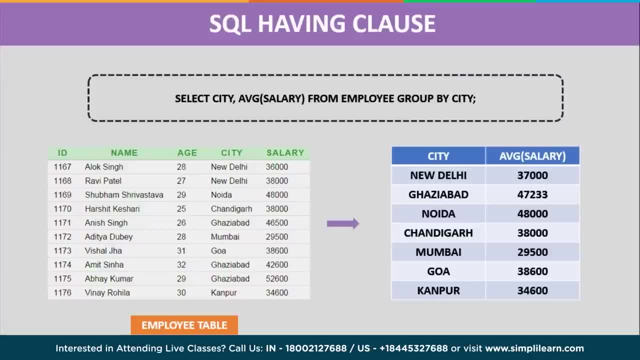 Now we have New Delhi- that is being repeated twice- which is 2 records, and we have Ghaziabad, which is 2 records. Now New Delhi has 2 records, which is having salary of 36,000 and 38,000. 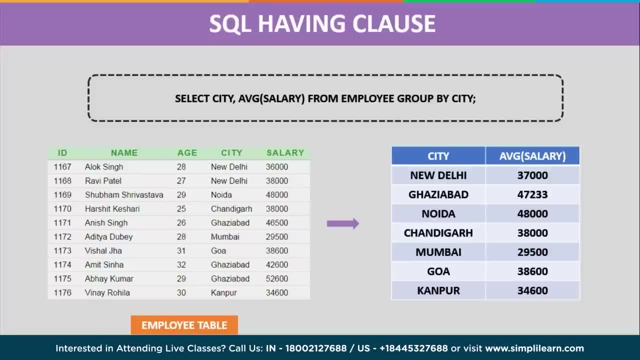 Now, if you consider the average, it is basically 37,000.. And similarly, for Ghaziabad, We have 3 records which have salaries 46,500, 2,600, 52,600.. Now, when you calculate the average, it is showing as 47,233. 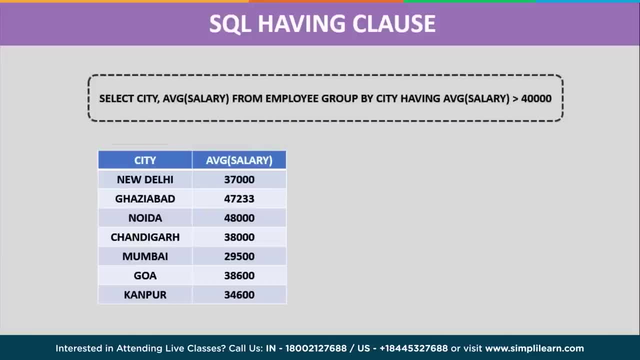 Now, now that you have applied this, Now, let us have the having condition here. Now let's say, if I want to find the average salary of all those employees from different cities, Who is having average salary greater than 40,000.. 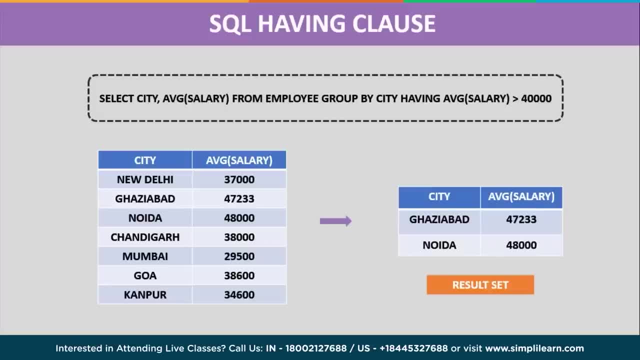 Now, in this case, if I implement this query, this will be the following output: As you can see, both Ghaziabad and Ghaziabad. As you can see, both Ghaziabad and Noida has the average salary more than 40,000.. 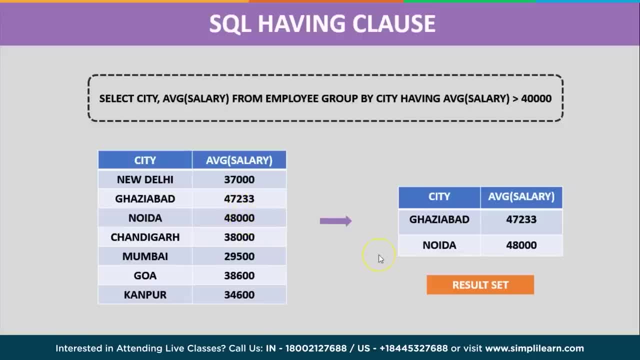 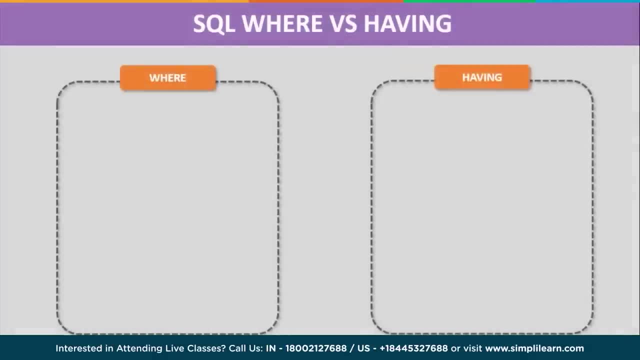 That is, 47,233 and 48,000.. So in this way, you can use the SQL HAVING clause as well. Let us now look at the differences between these 2 clauses, that is, SQL WHERE and HAVING clause. Now, SQL WHERE clause basically filters the individual rows in the table based on the specific condition. 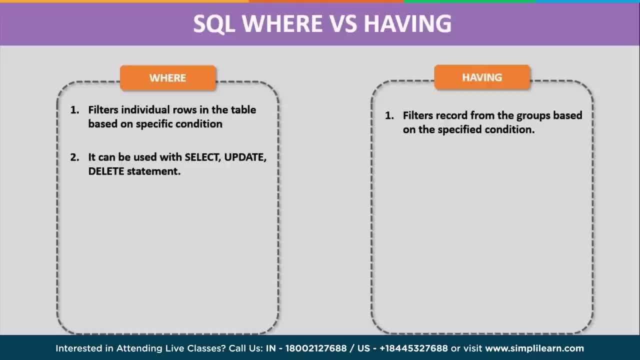 Whereas the HAVING clause filters groups instead of rows, Whereas the HAVING clause filters groups instead of rows. Now, as discussed earlier, WHERE clause can be used with SELECT, UPDATE, DELETE statement, Whereas the HAVING clause can be used only with the SELECT statement. 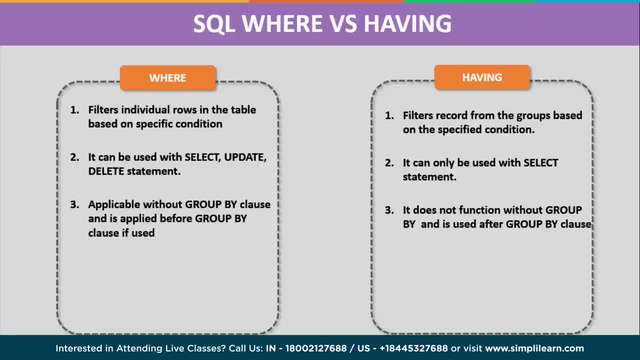 Now, WHERE comes before GROUP BY, which means that WHERE clause filters rows performing aggregate calculations, And HAVING comes after GROUP BY, which means the HAVING clause filters rows after performing aggregate calculations. So, consequently, HAVING is slower than WHERE in terms of complexity and efficiency as well. 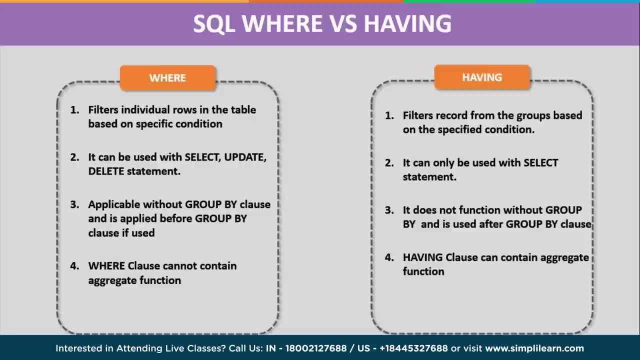 Now, as discussed earlier, WHERE clause cannot contain aggregate functions And HAVING clause can contain aggregate functions such as COUNT, SUM, AVERAGE, etc. Now SQL WHERE is considered as a pre-filter because it performs the row operations first And HAVING clause is considered as a post-filter because it performs the column operations after grouping the data. 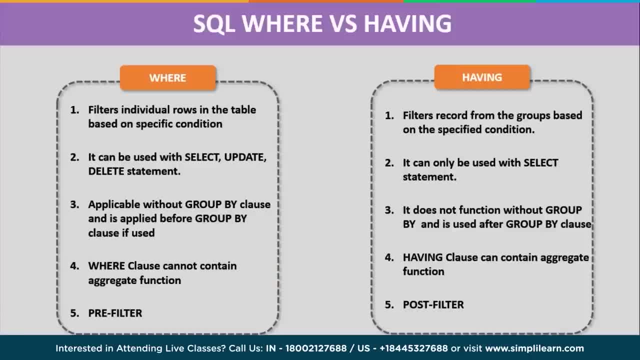 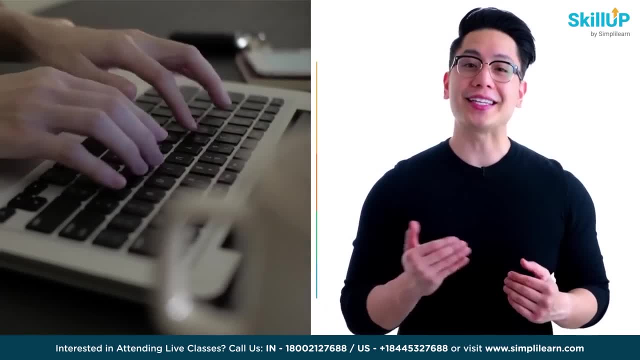 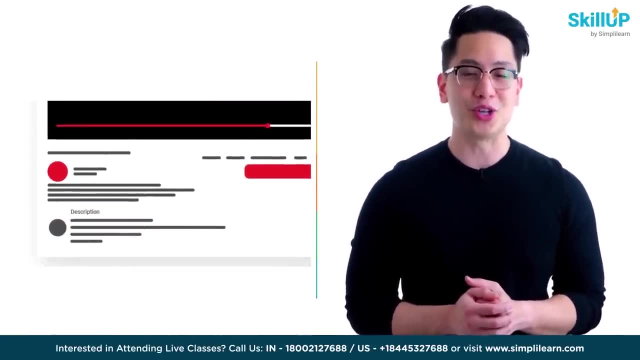 So now that we have understood about these both types of SQL clauses, let us jump into MySQL Workbench for the execution part. If getting your learning started is half the battle, what if you could do that for free? Visit SkillUp by SimplyLearn. Click on the link in the description to know more. 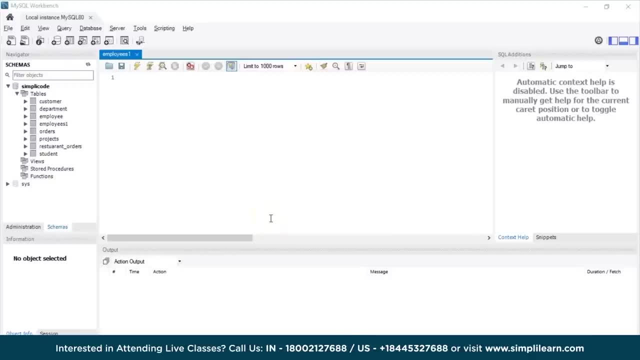 So, as you can see, MySQL Workbench has started And on the left side you can view the SimplyCode database, which is having different tables, such as CUSTOMER, DEPARTMENT, EMPLOYEE, EMPLOYEES1, and etc. So, as you can see, MySQL Workbench has started And on the left side you can view the SimplyCode database, which is having different tables, such as CUSTOMER, DEPARTMENT, EMPLOYEE, EMPLOYEES1, and etc. 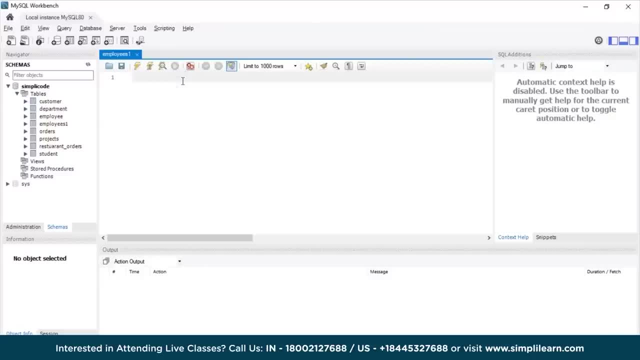 Now to perform the where and having clause statements, we will use the EMPLOYEES1 table. So let me just display the records present in that table. So I'll use the select operator. at the start and end of the day, Click on the executes button. 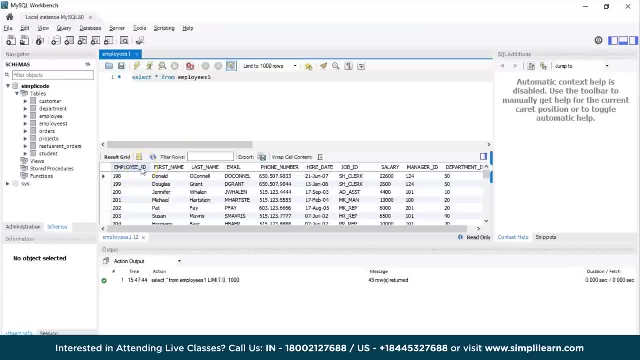 As you can see, the EMPLOYEES1 table has various columns, such as the employees ID, first name, last name of the employee, their email ID, phone numbers, hiring date, job ID and such more. salary, manager ID and department ID. 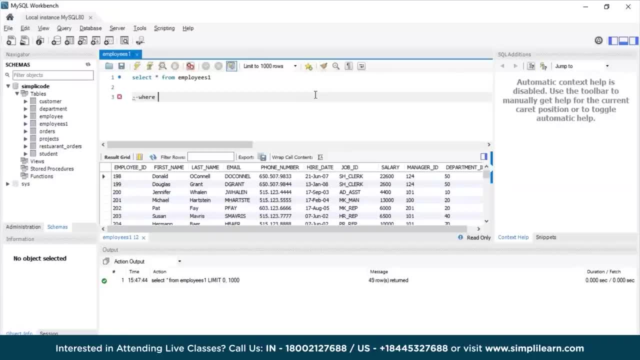 So firstly, let us discuss about the where clause or basically where condition. So let's say, if you want to fix the records of all those employees, from these employees one table whose salary is, let's say, less than 5000 and they belong to department 30.. 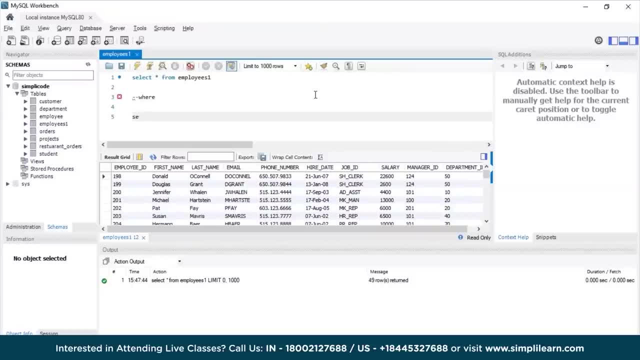 So in that case, the following query would be: select star from employees, table one where salary is less than 5000.. Now I'm using the and operator, which is basically a logical operator. So whenever you're performing the where condition, you can use the logical operators and comparison. 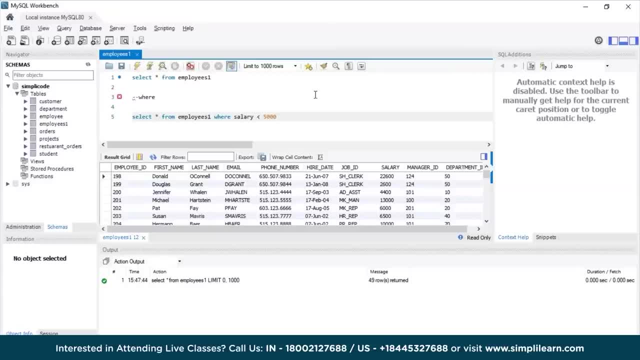 operators, of logical operators such as and, Okay, Or between, et cetera, and the comparison operators like less than equal to, less than greater than equals to, et cetera. So I'm using the and operator here, and department ID is equals to 30.. 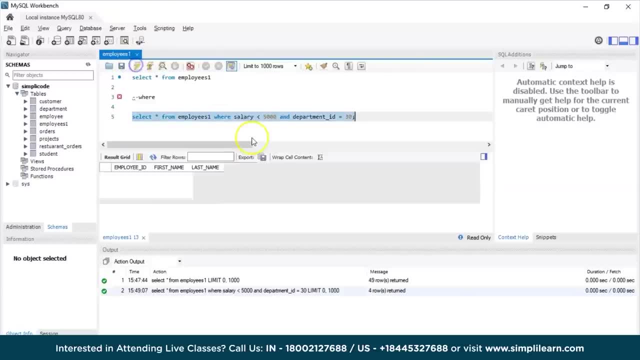 So let me execute the statement and see the output. So, as you can see, there are a total of four employees whose salary is less than 50000 and they belong to the department 30. Now you can also, as discussed earlier, you can also perform the update operations using 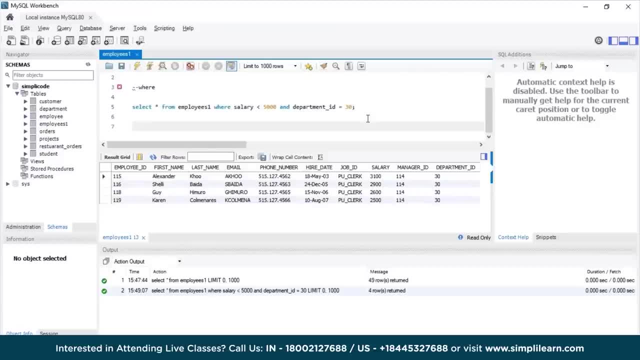 the where clause as well. Now let's say, if I want to update the salary of employee who's having employee ID 116, as let's say 10,000, then the query would be update table name. that is, employee one set salary equals to 10,000. 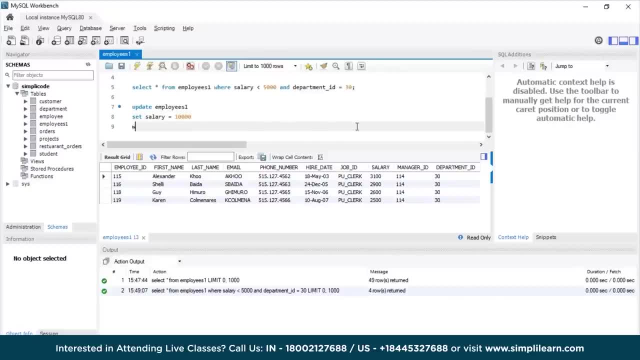 Okay, So I'm using the and operator, where employee ID is equals to, let's say, 116, and the employee name is Shelly Baida. So I'm just taking that example. So let me just execute this query. So, as you can see, our query has been successfully executed. 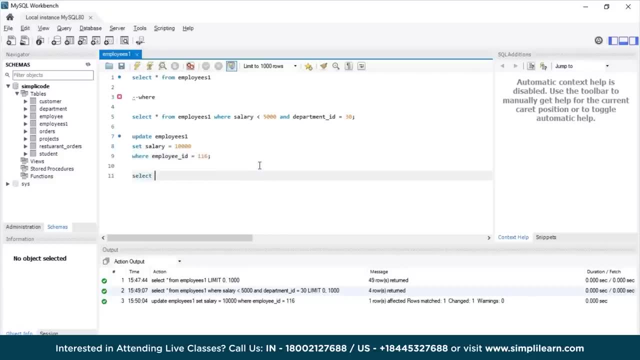 So let me just verify whether it is executed or not. So I'll use the select statement. Select star from employee ID: Okay, Employee one where employee ID equals to 116.. So let me run this query and we'll see the output. 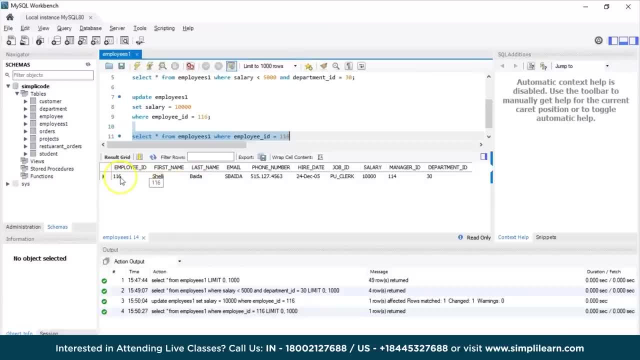 So, as you can see, the employee Shelly Baida, who's having employee ID 116 and their salary has been changed into 10,000 here successfully. So in this way you can use the where clause as well. You can also use the where clause for delete also. 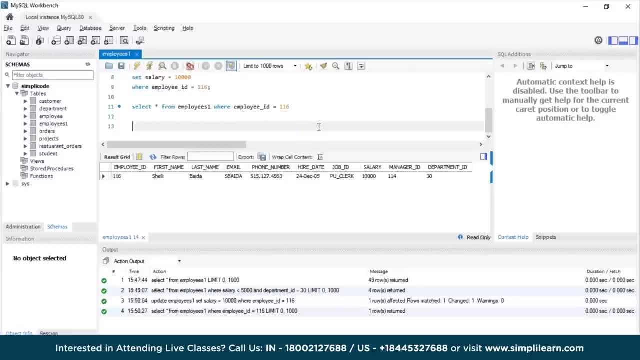 Now let's say, if I want to delete the details of the employee who's having employee ID as 120, let's say, then I'll use the delete statement: Delete from employee one where employee ID is equals to 127.. So let me just execute this query. 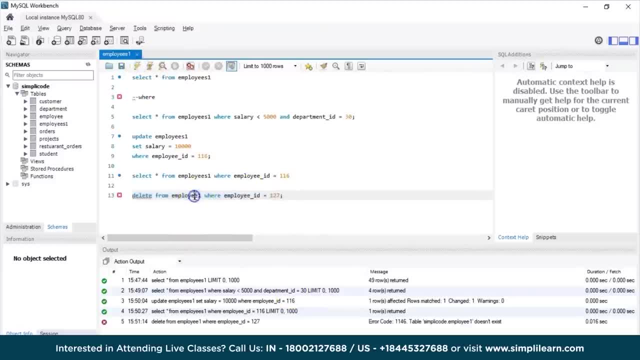 Okay, So, as you can see, our query has been successfully executed here and the details of the employee who's having employee ID as 127 has been deleted successfully. So in this way, you can use the where clause to perform various operations, such as select. 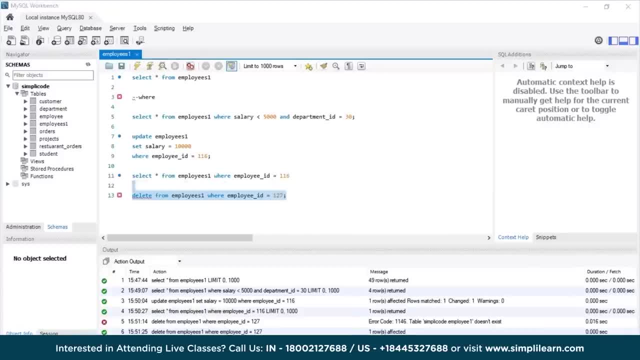 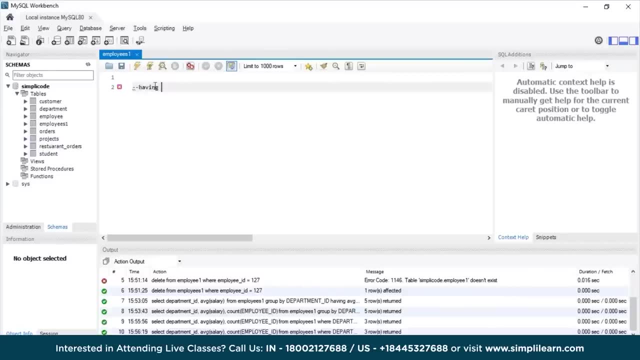 update, delete, etc. using comparison and logical operators. Let us now go to the next step. Let's now understand about the having clause For that. let me take an example. Let's say, if you want to display the records of all those employees present in different 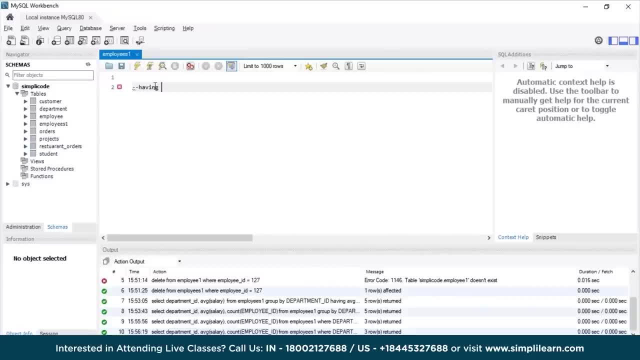 departments and whose average salary is greater than, let's say, 5,000.. So in that case, the following query would be: select. Now I want to display the department ID, so I'm taking the department ID column: average salary from employees. Okay, Okay. 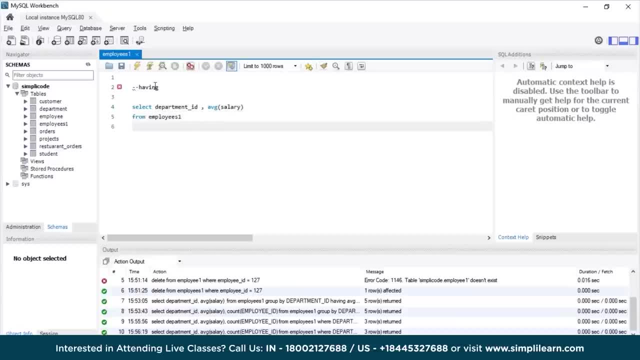 Okay, That's one. Now, as you know, while using the having clause, we have to use the group by statement as well. So I'll group by all the department IDs, since we have multiple department IDs present in the table. Department ID having average salary greater than. 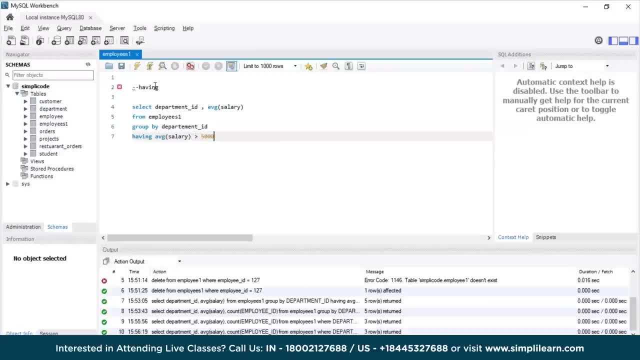 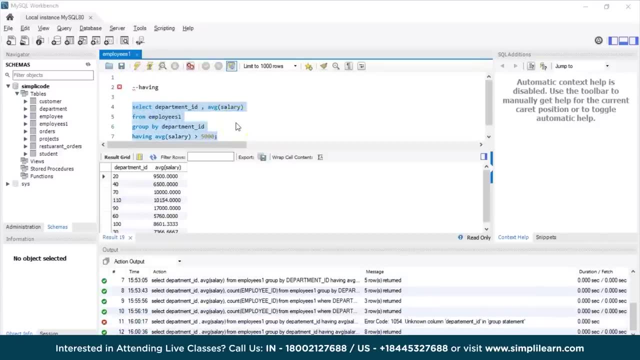 Okay, Okay, Okay, five thousand, five thousand dollars. okay, let me just display the output. so our query has been successfully executed and, as you can see here, it is displaying all the different departments and their average salaries as well here. now i can use different aggregate functions here as well. 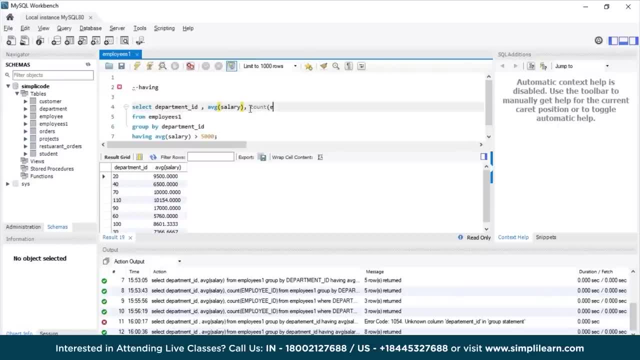 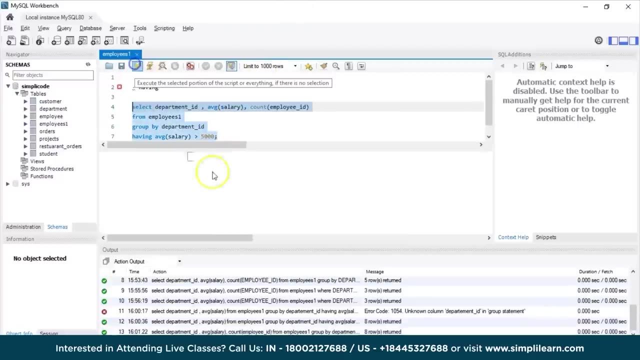 if i want to count the number of employees in each department, i can take the count function, so let me just use it- count employee id, which will basically count all the total employees in the different departments. so let me just execute this statement so, as you can see, it will display the count of all the employees that are present in different. 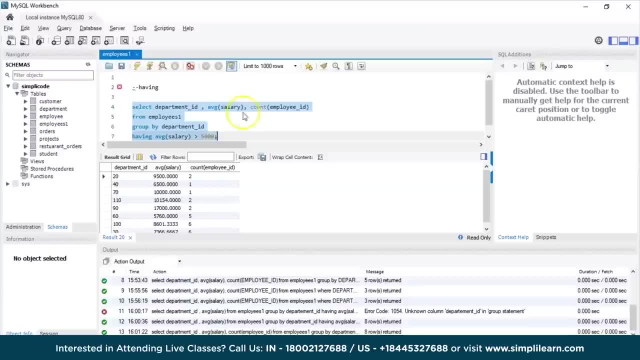 departments and having average salary more than fifty thousand. so in this way you can use the clause as well. now we can also combine both the where condition as well as the having condition condition as well. now we can combine the where and having plus together in a select query. in this case, the where clause is used first to filter individual. 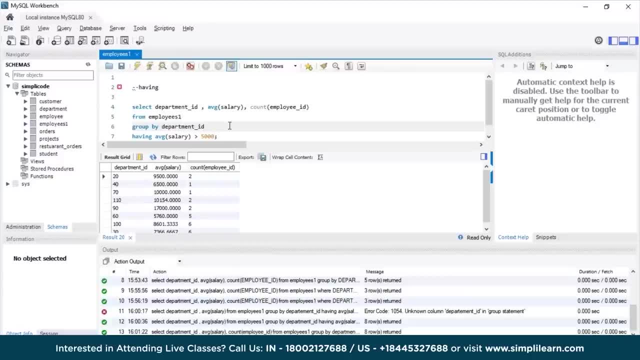 rows and then the rows are then grouped to perform the aggregate calculations and finally, the having clause is used to filter the grouped data, that is, the identical groups that are having the same values. now, as discussed earlier, we have to use the where condition before the group by, so I am just taking the. 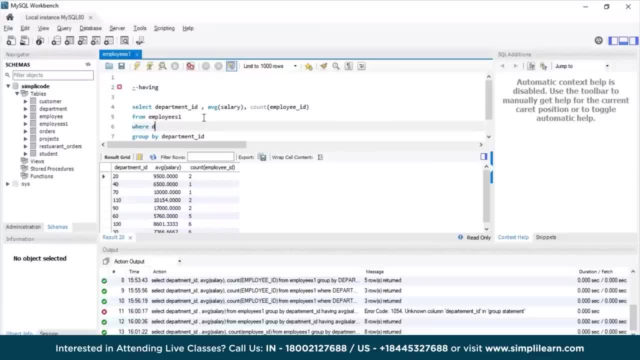 where clause before the group by. and let's say, if I want to display only those departments that are having more than 80 as the department ID, so department ID greater than 80, so let me just display, so, as you can see, it will display only those records where the department ID is more than 80, that is. 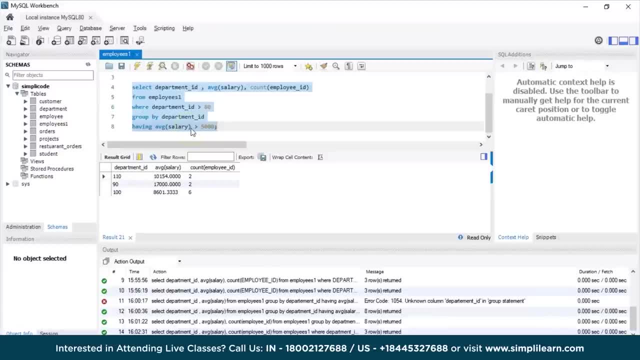 90 hundred and 110 and the details of all the employees whose average salary is more than 500. now i can also use the order by statement here in order to mention all these records in a systematic manner. that is an ascending or descending order. so order by department id. so let us execute this query. 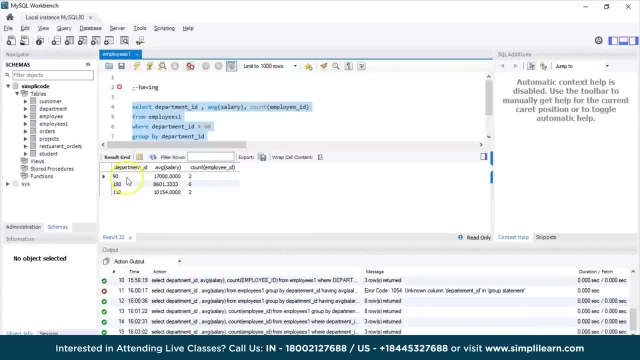 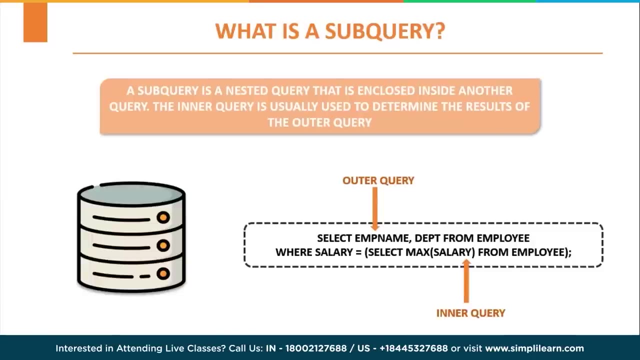 so, as you can see, it will showcase the department id values in the ascending order, that is, 90- 110. so in this way you can use the having clause as well in sql. so what is a subquery? an sql subquery is a query which is written inside another query. a subquery is usually added within the where clause. 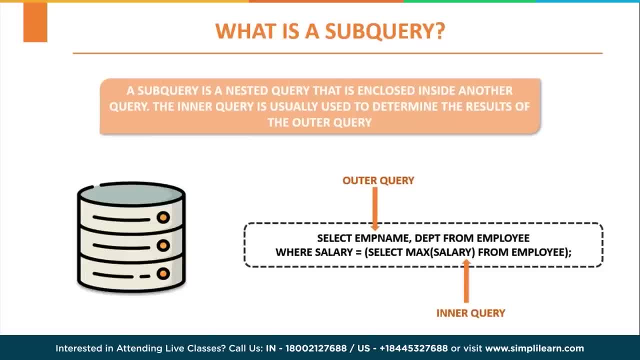 of another sql select statement in a subquery. the outer queries result is dependent on the result set of the inner query and that is the reason why subqueries are also called as the nested queries. a subquery is also called as an inner query or inner select, while the 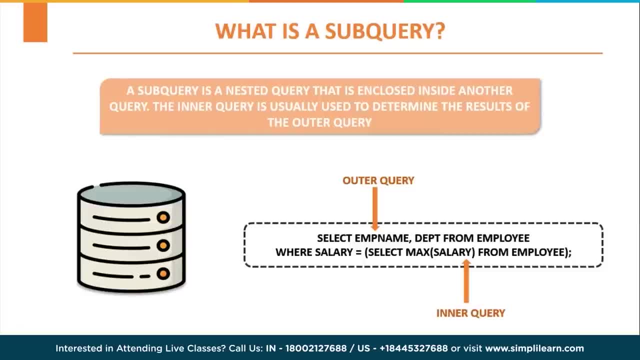 ô containing the main query or the parent query is called as the outer query or outer select query statement. Now the inner query executes first, before its parent query or the outer query, so that the results of an inner query can be passed to the outer query. Let us understand this with an example here Now. 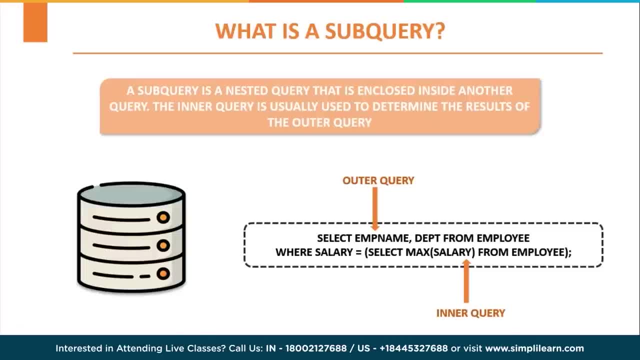 consider this syntax over here, which is followed as: select employee name department from employee where salary equals to select maximum salary from employee. Now, select employee name, department from employees. the outer query and the rest part is the inner query. Now, when the above query is applied, 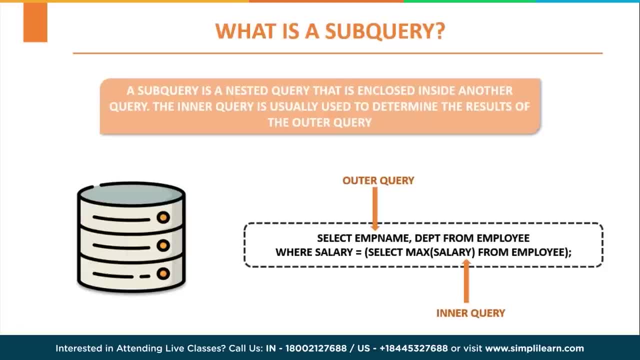 to the given employee table. here the sub query is executed first, which selects the maximum salary from the employee table. Then the resultant is the past onto the where clause of the outer query. Now this outer query is executed, which selects the rows- in this case the employee name and the department from. 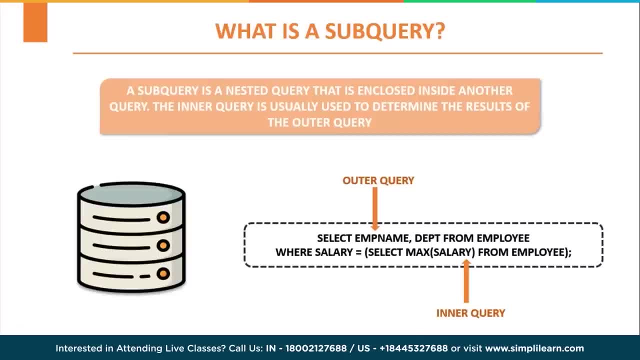 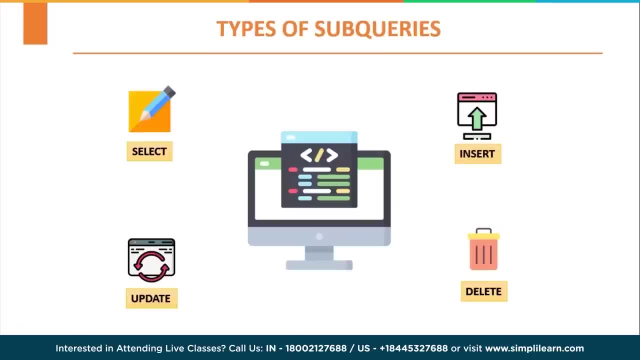 the employee table where the salary is equals to the resultant of the sub-query, which is the. it selects the maximum salary from the employee table, returns the final result. so let us now look at the types of sub queries that are used in sql. now, sub queries in sql are: 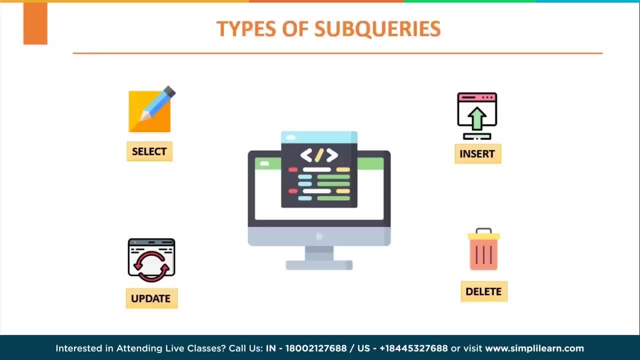 majorly used with insert, delete, select, update statement, along with the comparison operators like less than, equals to greater than or equals to between, in and etc. sub queries are used to execute a query dependent on the outcome of another query and it allows the user to fetch the results. 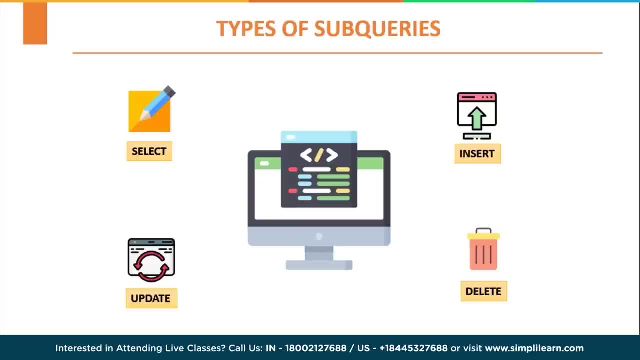 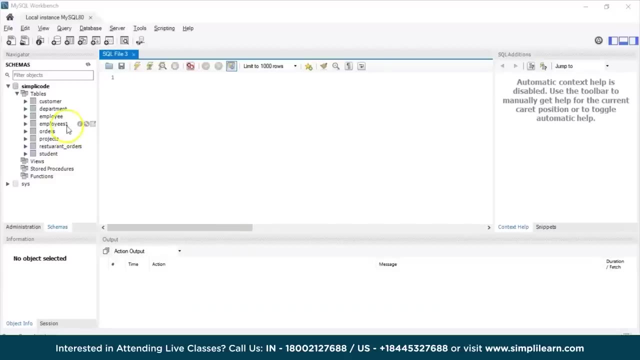 without writing two distinct queries, and it is time saving as well. so now that we have understood what is sub queries and at different types, let us jump into mysql workbench to execute the various sub queries that are used in sql. so, as you can see, mysql workbench has started and we have various 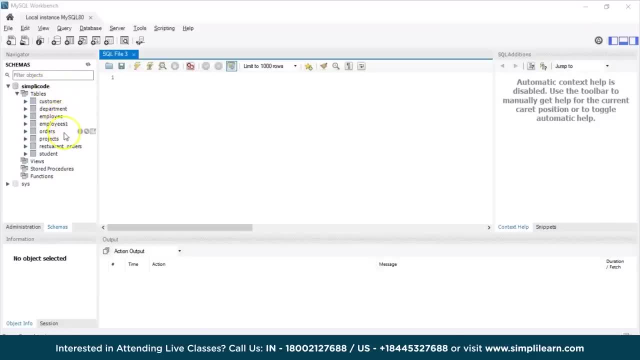 tables in our database, simply code, such as customer department, employee, employee one, and so on. firstly, let us discuss the sub queries using the select statement. now in sql, in most of the cases we use the select statement to perform the sub queries. so for that let us consider the table employees one here. so 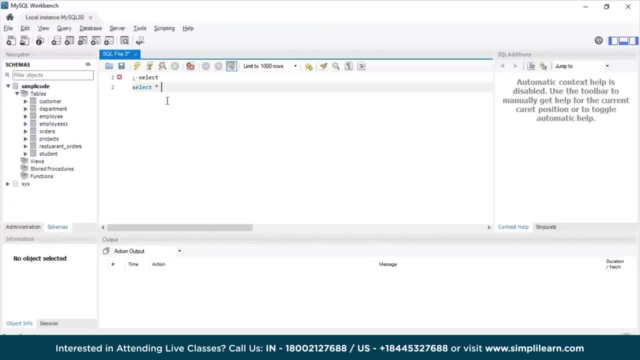 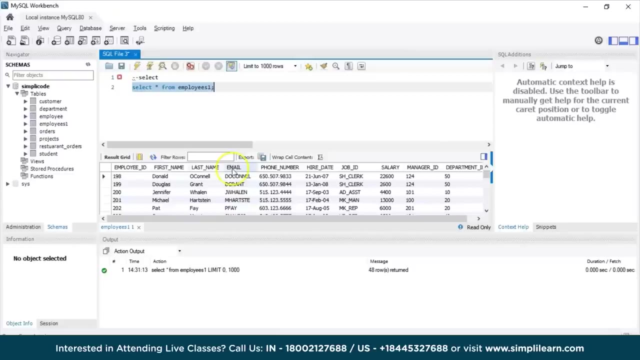 let me just display the records that are present in the table. for that i am using the select statement, select star from employee one. so let us run the query and see the records so as you can see the employees. one table has various columns, such as employee id, first name, first. 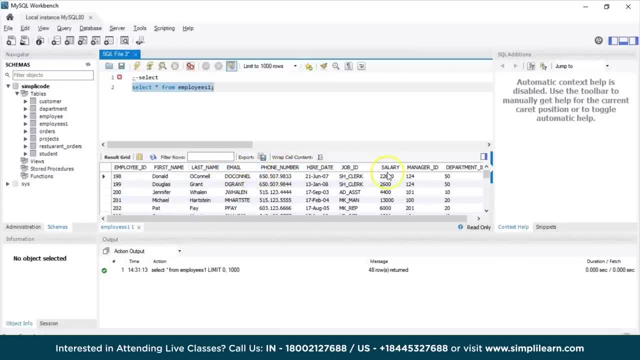 name, last name, email, their phone number hiding date, job id, salary, manager id and department id. now let us understand this concept with the help of an example for executing the select statement using the sub queries. now, let's say, if i want to find all those employees whose salary is less, 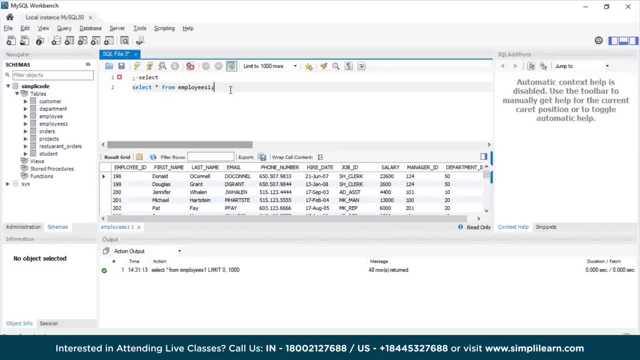 than the average salary of all the employees that is present in the employees one table. so in this scenario we'll use a sub query to get those employees whose salary is less than the average salary from the employee table. the following query would be select: now, since i want to display all the records, i'm using the. 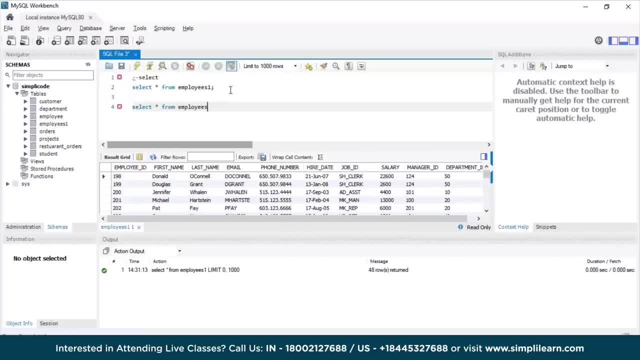 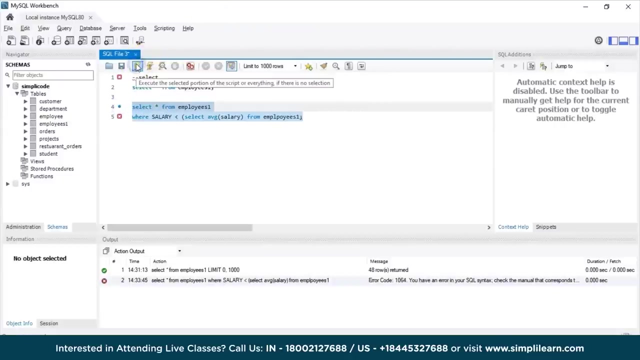 star operator from employees one where salary is less than- and within the parenthesis we have to mention the subquery that is select average salary from employees one table. so let us execute the statement and see the output. uh, there is a runner in the code, just let me check. so, yeah, i. 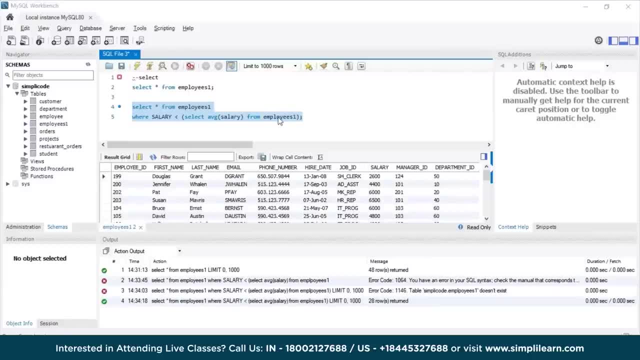 forgot to mention the parenthesis here. uh, make sure you uh write: the subquery is always within the parenthesis, otherwise it's not going to work. so i'm going to write the subquery in the parenthesis here. uh, make sure you uh write the subquery is always within the parenthesis, otherwise it's not. 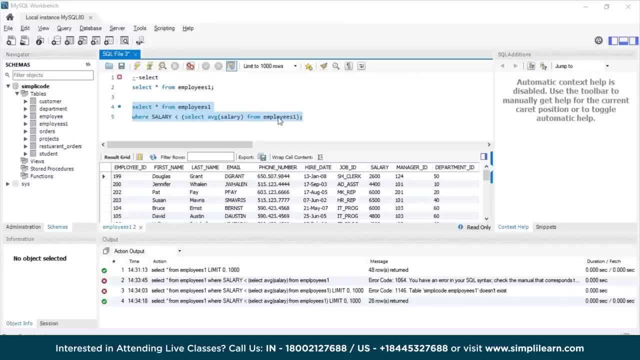 it will show an error here. so now let us understand this query and let us break this query statement to understand in a better way. now here the query to find out the average salary is the subquery here, that is the select average salary from the employee one table. so let me. 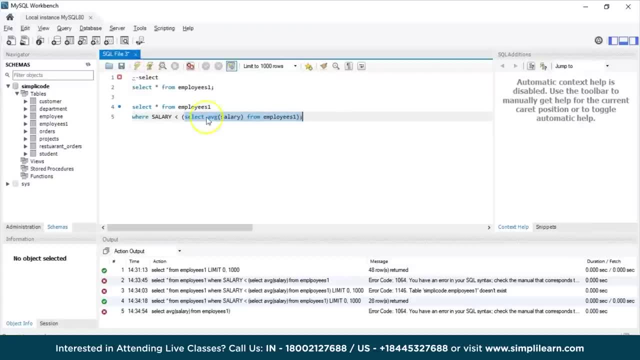 just execute this statement. so we have the average salary that is 6708.66. so now the outer query takes the result of this inner query, which is basically the subquery, and executes the remaining sql command based on the result. so the subquery first returns the average salary, that is 6708. 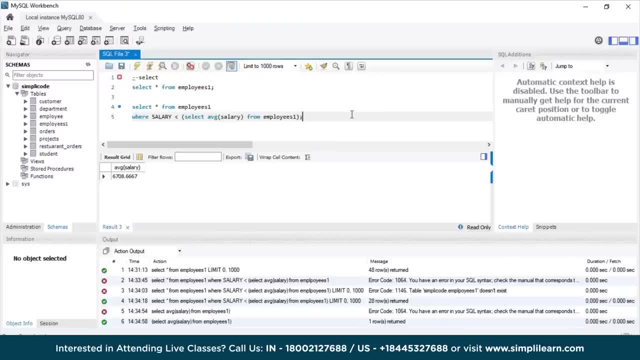 and this result is passed on to the outer query, which fetches the details of all those employees who's having salary less than the average salary, that is, 6708. so when i execute this statement, it will display the employees of all those records who's having salary less than 6708, that is. 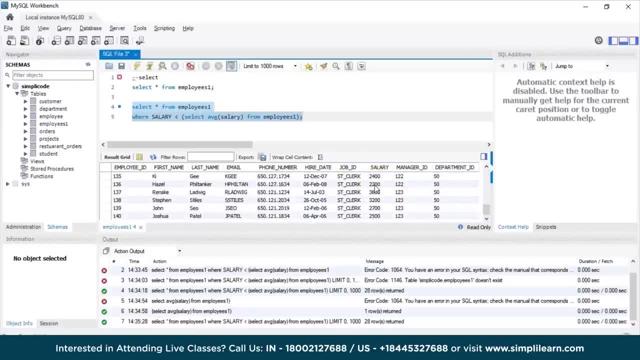 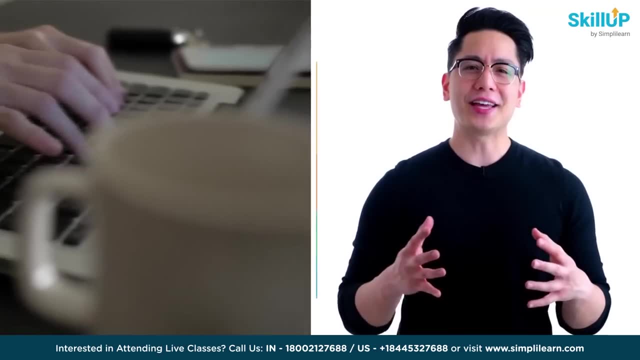 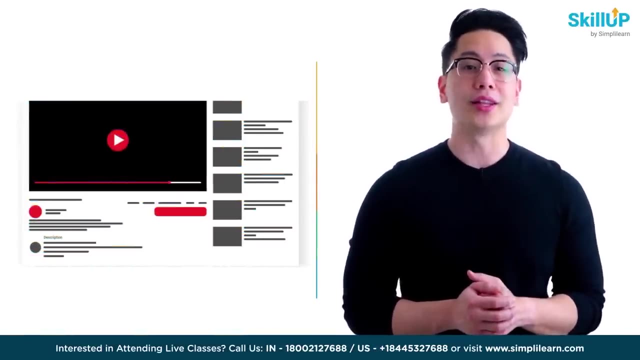 2600, 2400 and so on in this way. so in this way you can use the select statement to perform the sub queries in sql. if getting your learning started is half the battle, what if you could do that for free? visit: scale up by simply learn. click on the link in the description to know more. 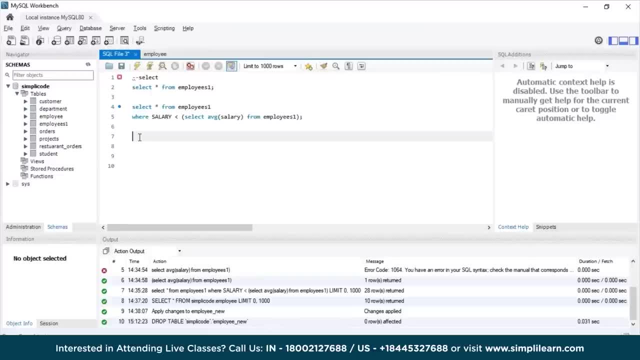 now, other than uh, the sql select statement, sql sub queries can also be used with the insert statement. in the insert statement, the data returned from the sub queries used to insert the data from one table, that is the existing table, into another new table. now let us consider the employee table here. so let me just display the records, select star from: 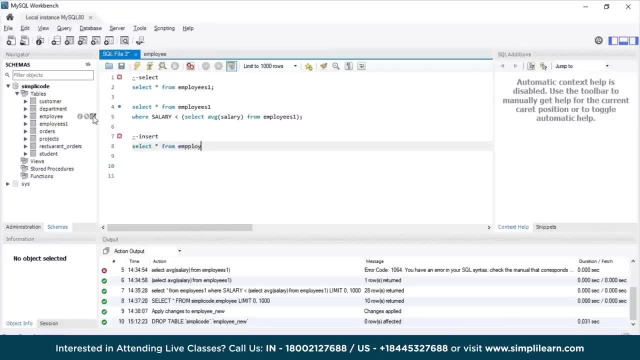 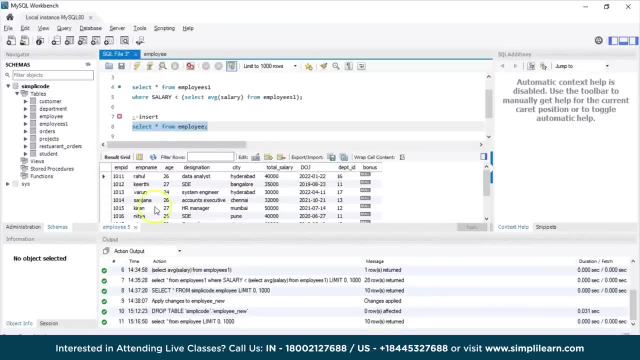 employee. uh, let me just display the records now. so the employee table has various fields such as employee id, employee name, age, designation, ct, total salary, date of joining department and bonus. now if I want to copy this data from the employee table into a new table- let's say employee, new table- so I'll have. I can use the sub queries with. 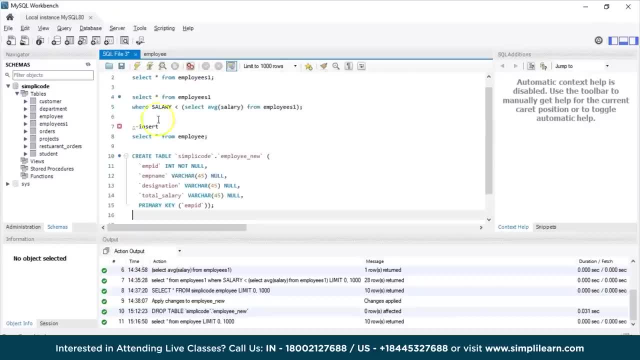 the insert statement here. so let me just create a new table here and the query is followed as: create table employee new. the employee new table has the employee ID: employee name designation. who does happy? that's it. so I'm taking primary key as employee ID as it uniquely identifies the each record in the table. 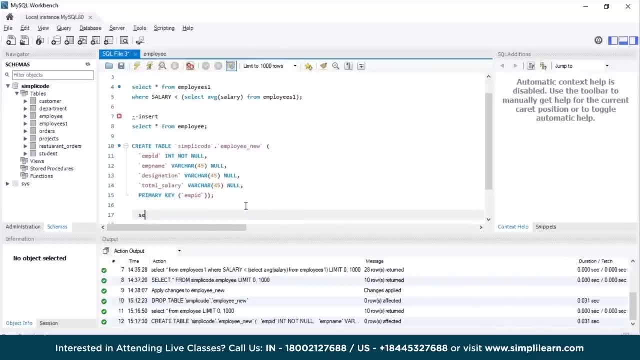 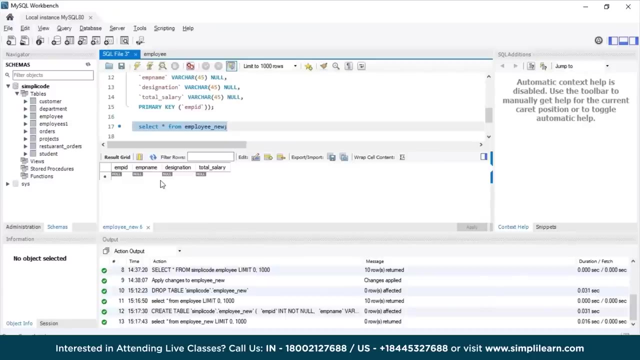 so let me just execute statement now. I'll use the select statement now. as you can see, the employee new table has various fields: employee ID, employee name, designation and total salary. but we do not have any values that are present in the employee new table, so we'll use the sub query using the insert statement to 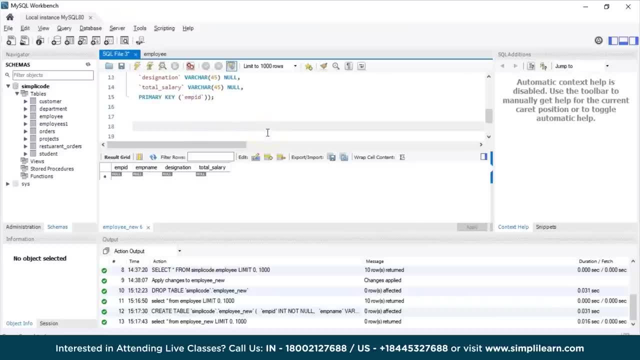 into insert value into it. now, let's say, if I want to insert the values from the employee table, that is, the existing table whose salary is greater than 30,000, so I want to fetch only those records from the employee table into the employee new table whose salary is greater than 40,000. so the following query would be: 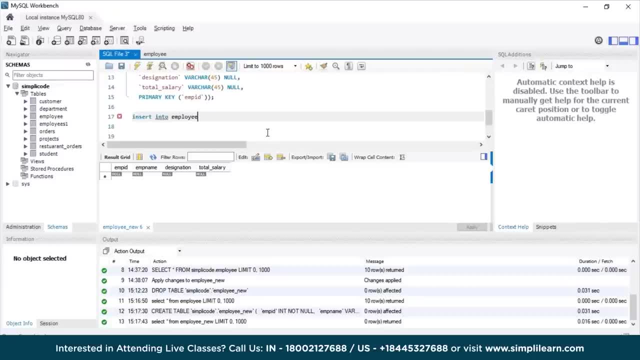 insert into the new table, that is employee new table whose salary is greater than 40,000. so let's say, employee new table is greater than 40,000, so this is going to be the employee new table whose salary is greater than 30,000. so we can use the total part as the employee new table and then from 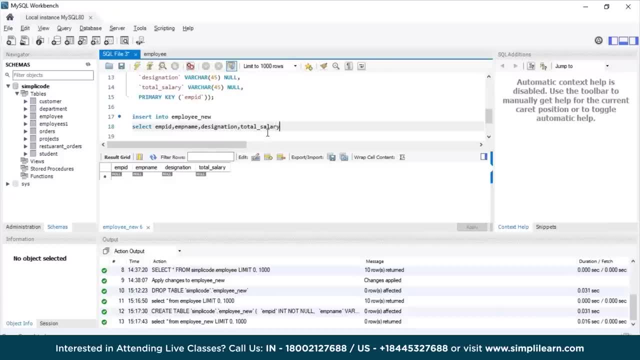 the employee new table: select. now, since we are only concerned with the employee ID, employee name designation and total salary, we'll mention only those columns where total salary. I'm using the in operator here and within the parenthesis I'll write the sub query, that is: select total salary from employee where total salary is greater than. 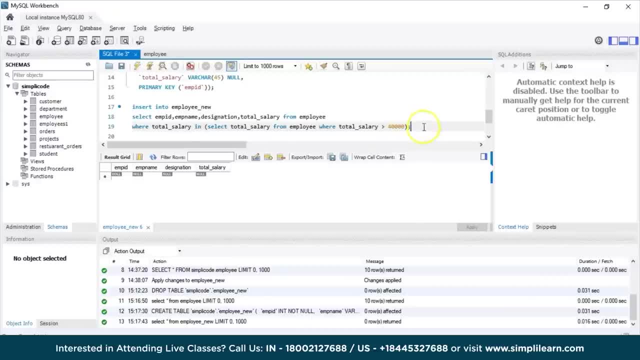 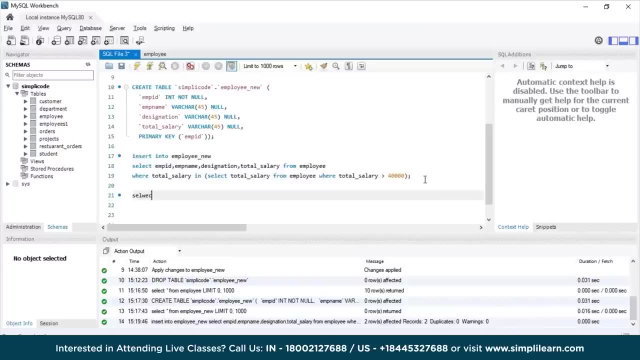 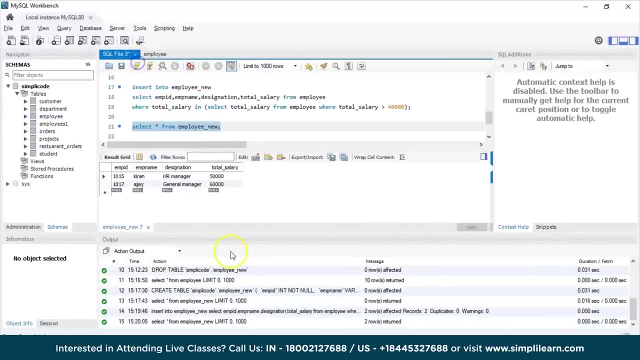 40,000. close the parenthesis and let us execute the statement. so our statement has been successfully executed. so let me just display the records again. select star from the table, employee new. so, as you can see, it will insert only those records. for all those employees, total salary is greater than 40,000. so we have only two employees. 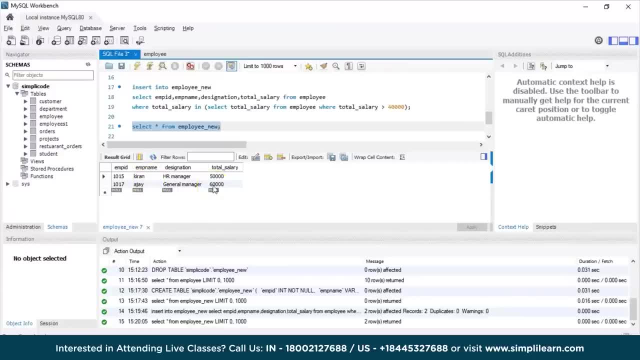 Kiran and Ajay, who is having salary as 50,000.. Now the insert statement basically specifies that new data is added to this table, that is, the employee new table, and as we are copying all the data from the employee table, which is our existing, 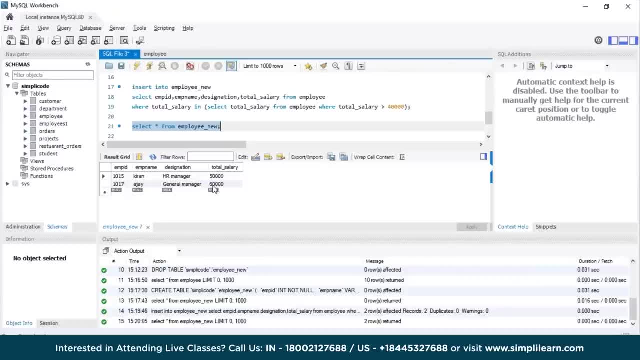 table to the new employee new table. there is no need to specify the column name in the insert statement. otherwise, you would need to mention the column name in which you want to add the data. the only thing that you have to keep in mind is that the table structure has to remain the same, even 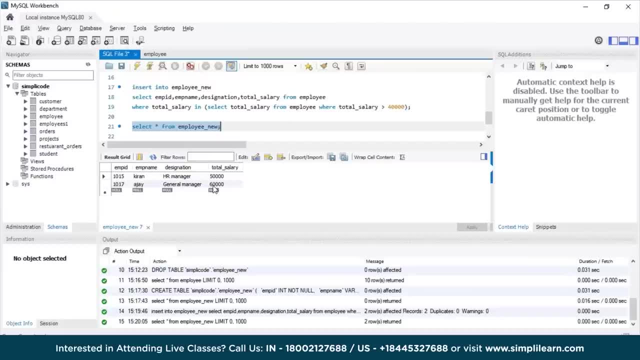 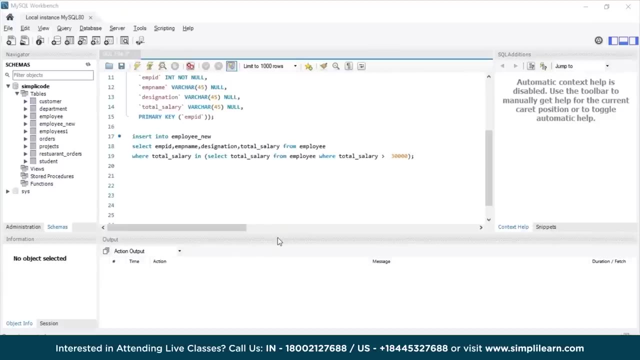 if the column names are a bit different, The column data types have must remain the same in order to insert the data using sub queries from one table to another table. So in this way, you can write sub queries using the insert statement as well. Also, in a similar way, you can use the update as well as the delete statement to modify the existing data that is present in the table. 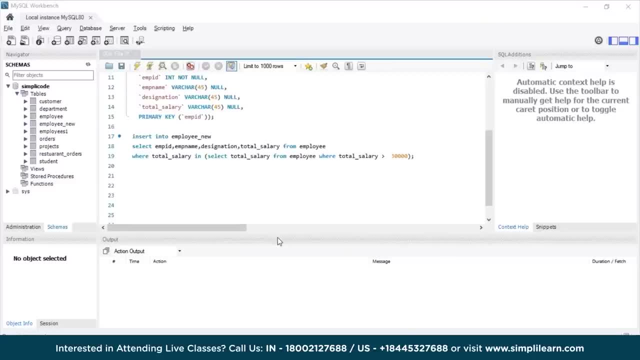 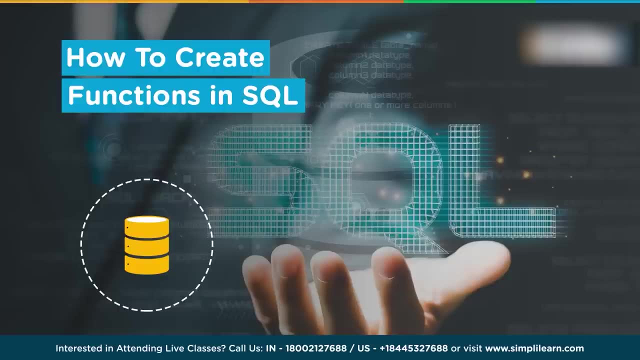 To know more about it. make sure to check out our SQL full course for beginners 2022 on our channel. So that brings us to the end of today's session. guys, that was all about sub queries in SQL To create and for the execution part of the functions. let us jump into mysql workbench. 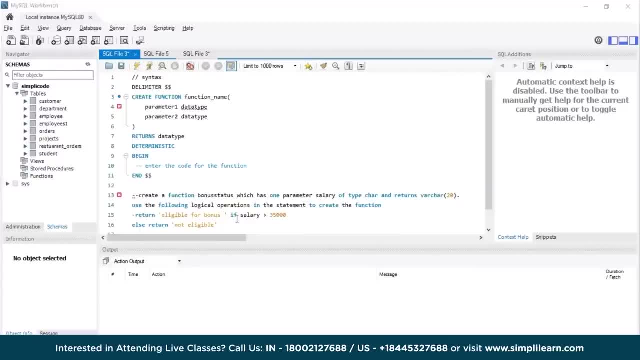 So, as you can see, mysql workbench has started, and before understanding the syntax of how to create a function, let us just understand what a function is actually is. Now, a function in SQL is basically a set of SQL statements that performs a specific task. Now, if you have to repeatedly write larger SQL queries to perform a task, you can simply create a function for that. 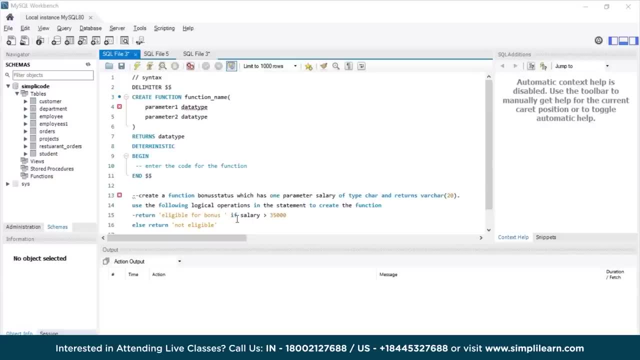 Now, next time, instead of rewriting the whole SQL query, You can just simply create a function for that. You can simply call that function to get the desired result. Now, these SQL functions are basically programs either developed by the user or already provided by the SQL system. 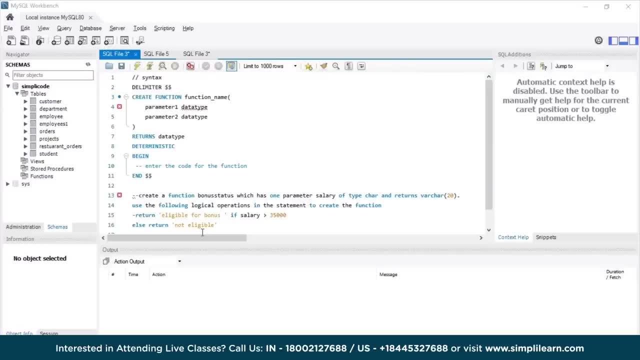 Now we have several inbuilt functions or the system defined functions like aggregate functions, string functions, date functions, etc. Now, other than that, we can create a user defined function as well. So firstly, let us go through the syntax on how to create a function. So the syntax is followed as delimiter, which I will explain in a while. 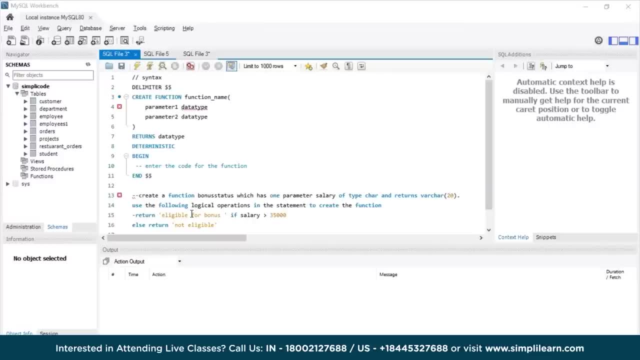 When we are creating the actual functions. so let us keep it aside for a while. Create function, function name and, inside the parenthesis, mention the parameters. Now you can create n number of parameters, as per your choice. The thing is, you have to mention the parameter name as well as its data type. 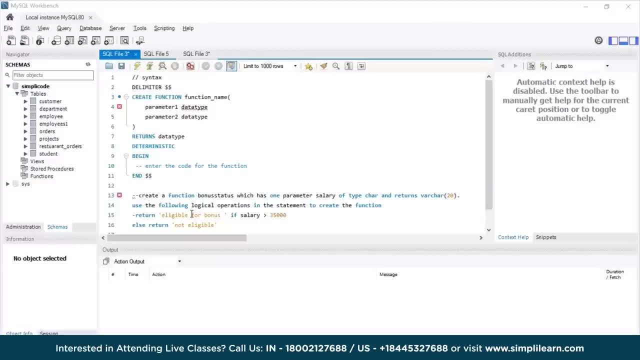 Returns data type: deterministic. begin, and inside that we have to write the code, that is, the actual code for the function, and use the end. So let me just explain how this syntax works. Firstly, we are specifying the name of the stored function That we want to create after the create function keyword. 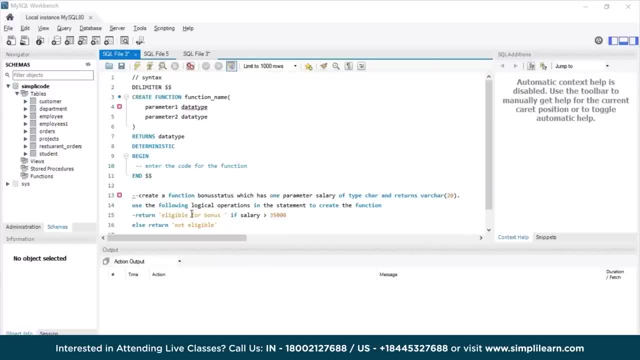 Next we have to list all the parameters of the stored function inside the parenthesis followed by the function name, And then we are specifying the data type of the return value in the return statement, Which can be valid using any data type here as well, like int, char, varchar, etc. 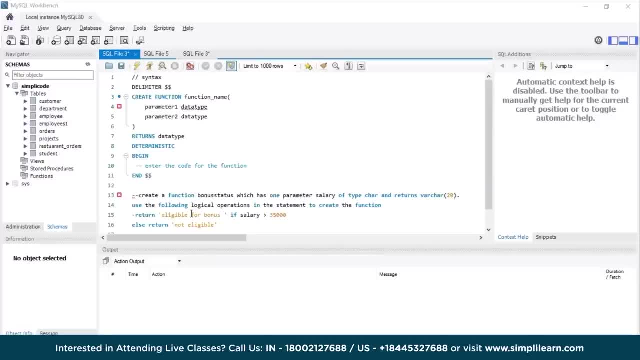 And then we are specifying if a function is deterministic or not. Now, a deterministic function always returns the same value for the same input value, Whereas a non deterministic function returns different results for the same input parameters. So let me just explain this with an example. 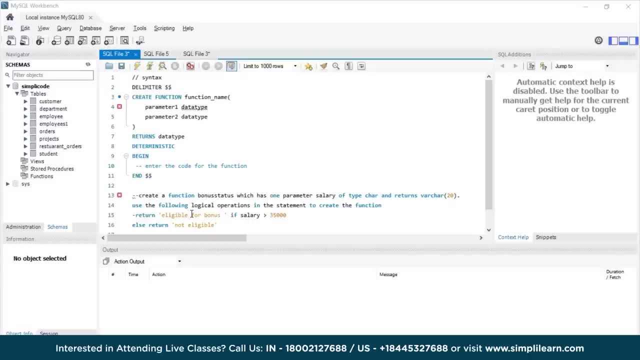 Now, if I take a function xyz, and I am specifying a parameter, let's say p function, So it will always result the same answer as long as its input, that is p, is the same. And finally, we will write the code in the body section after the begin keyword. 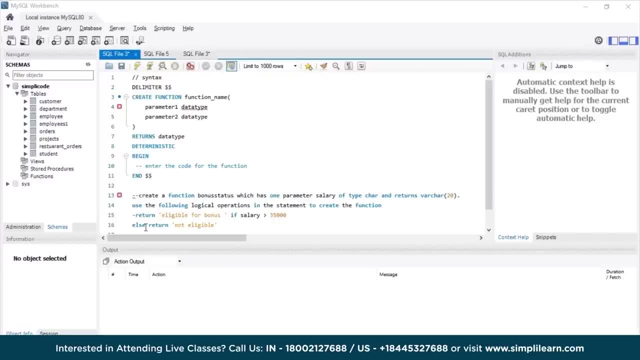 So this code will be returned in the body of the stored function In the begin end block. Now, inside the body section, you need to specify at least one return statement. This return statement basically returns a value to the calling program. Now, whenever the return statement is reached, this execution of this function is terminated automatically. 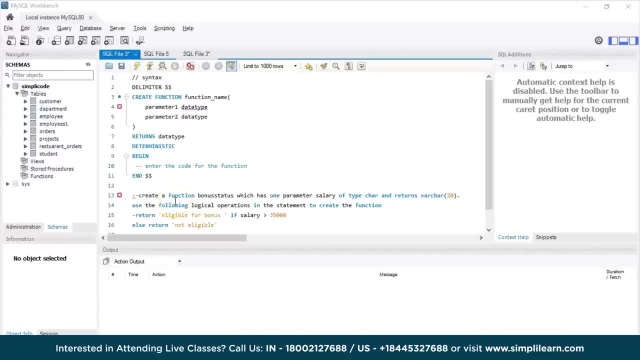 So let us now understand this with an example. We have a query here which says: like create a function- bonus status- which has one parameter- salary of type char And returns varchar of size 20.. Now we have to use the following operations in the statement to create this function. 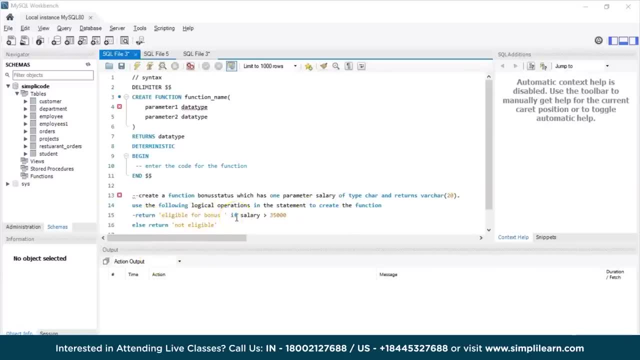 The first one is return eligible for bonus as the statement if salary is greater than 35000.. Else return not eligible. So let us now write the syntax for this. So let me just switch to another tab and we will write the query here. 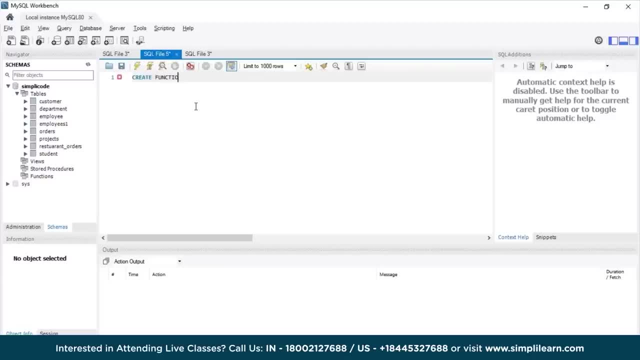 First write the keyword, that is create function. Now the function is bonus status. Inside the parenthesis mention the parameter. Now I am taking parameter as salary here, which is of character. I am giving size as 20.. Close the parenthesis. Now mention the return statement, that is, it returns varchar of size 20.. 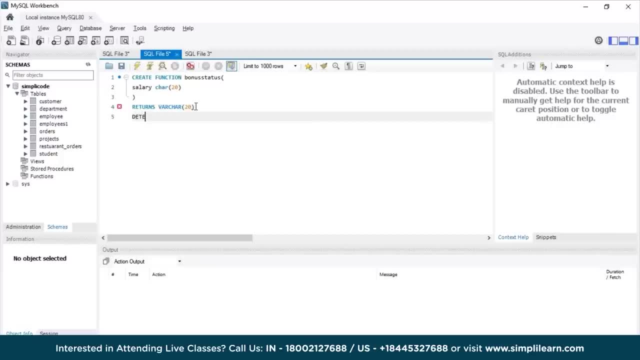 Deterministic Is the keyword that we are using here: Begin, And inside this we have to write our main query. Now, the query that we have earlier discussed is that if salary is greater than 35000. Then Return Eligible for bonus. 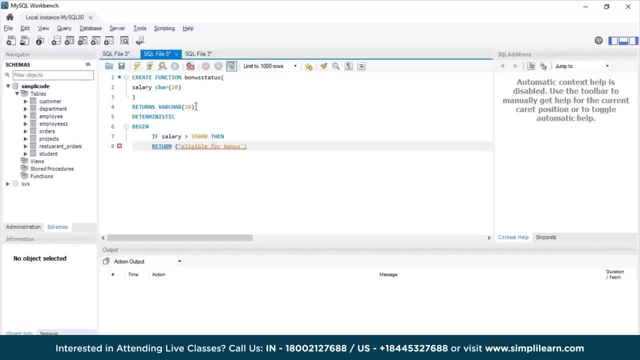 Eligible for bonus And close the parenthesis Else Return- Else return Inside the parenthesis Not eligible, Not eligible. Mention the double quotes and close the parenthesis And put a semicolon. Now that is it. That is the end of our body. 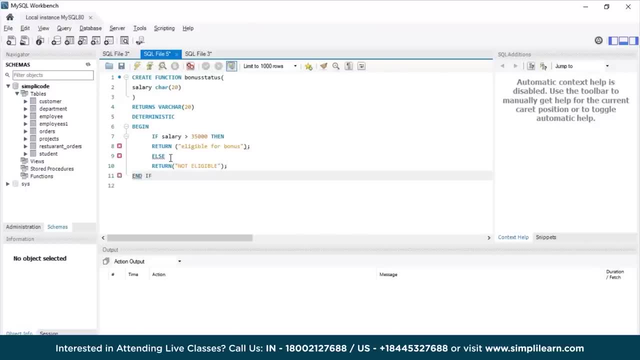 So now I will use the endif statement, Which will basically close the body of our function, And then I will use the end Operator, here With the dollar sign. And that is it. This is basically our code to create a function. So let us now execute the statement and see the output. 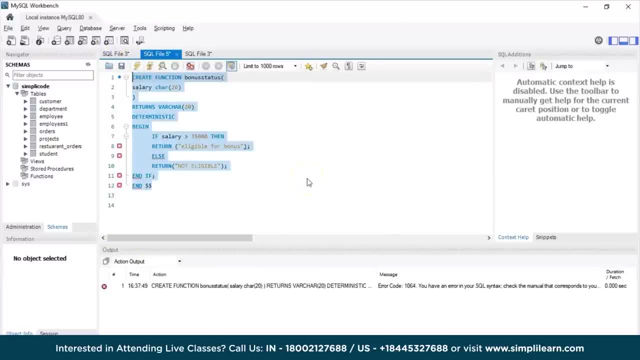 Now, while I execute the statement, it will throw an error, And this is where we will use the SQL delimiter. Now, as you know, when we write an SQL statement, You use the semicolon after the SQL statement, Like if you write a two separate statement. 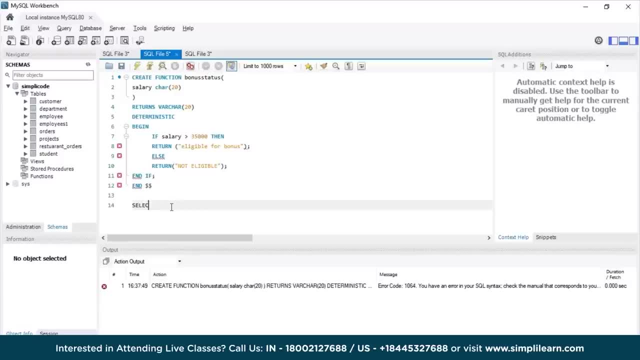 For example, If I say Select Star from, I am taking an example as employee And I am taking another example as select star From orders. Now, when I execute this query, it will throw an output Because I haven't selected which query I want to execute. 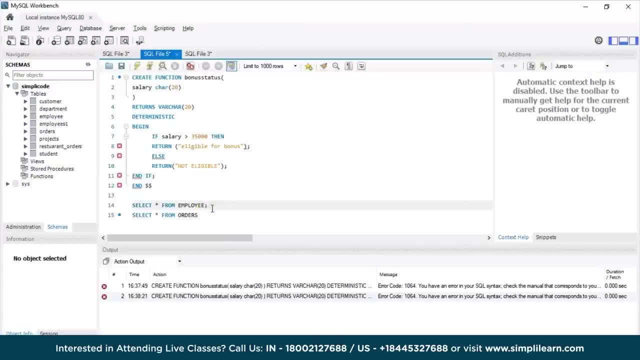 Now for that. we will place an individual semicolon at the end of our statement. So, in a similar way, MySQL uses the delimiter function to separate statement And executes each statement separately. Now, however, a function consists of a multiple statement separated by a semicolon. 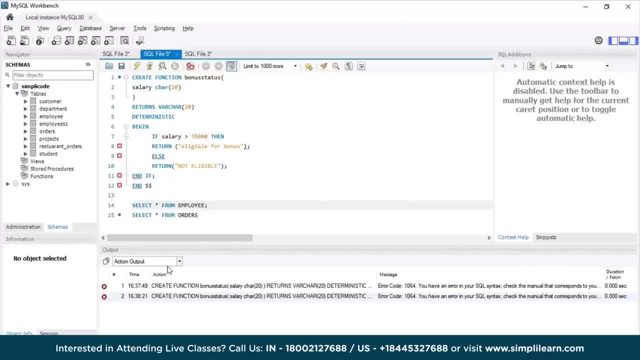 So if you used to define a function that contains semicolon characters, Then it will not treat the whole function as a single statement, But many statements. Therefore, you must redefine the delimiter temporarily So that you can pass the whole function as a single statement. 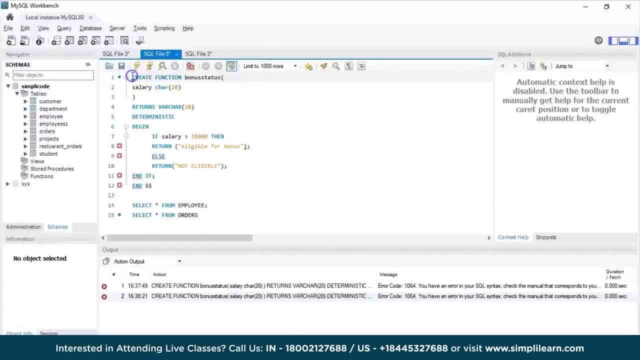 So for that we will use the delimiter here. So let me just incorporate the delimiter here You have to use delimiter with the help of double slash or double dollar sign. here You have to specify at the beginning as well as the end Delimiter. 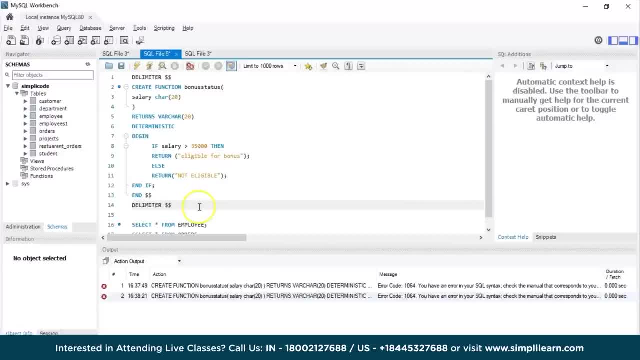 And I will mention two double. So that's it. Now our code is complete And let us execute the statement now. So our query has been successfully executed. Now to see whether our function is created or not, Let us just refresh the schema here. 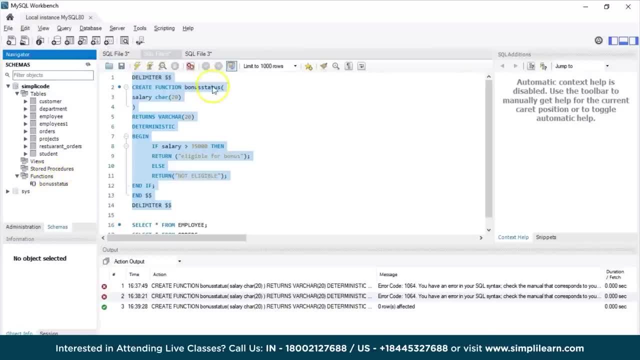 And, as you can see in function section, You can see bonus status, Which is the function we have created earlier- Has been created successfully. So let us now just verify whether our function is working or not. So I will just write a simple query as select bonus status. 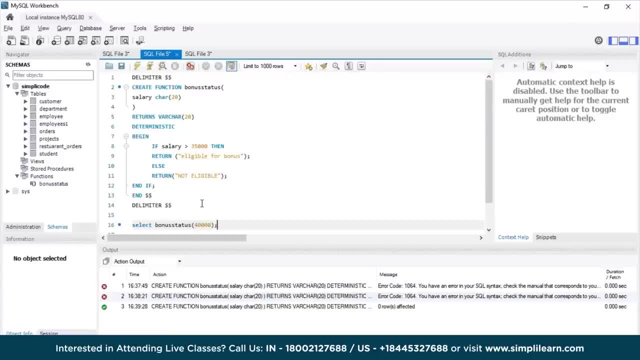 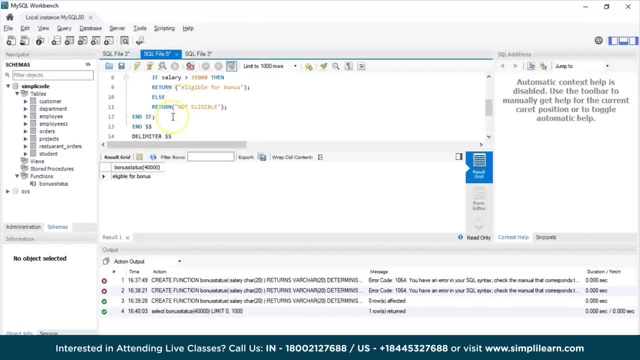 Let us take 40000 as our example. So let me just execute this statement And we will see the output. So, as you can see, The condition which was specified is If the salary is greater than 35000.. Then the employee is eligible for bonus. 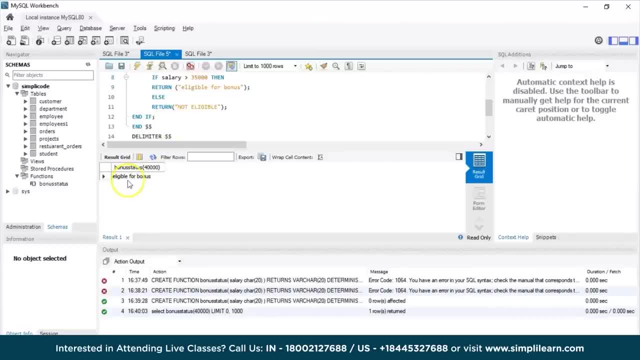 Now, since we have taken the salary as 40000. It is showing as eligible for bonus. Now, similarly, let us say, if I take 20000. And if I execute this statement, It will definitely show me not eligible. So, as you can see, it will show not eligible for bonus. 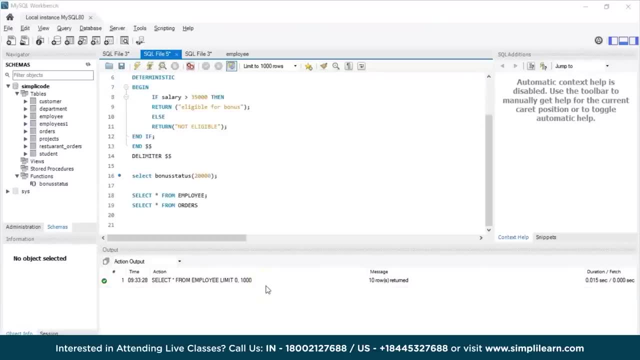 So in this way you can create and use a different function By passing certain parameters To get the desired result of your choice. So now that you have created a function, You can query an already existing table By calling that function in an SQL statement. 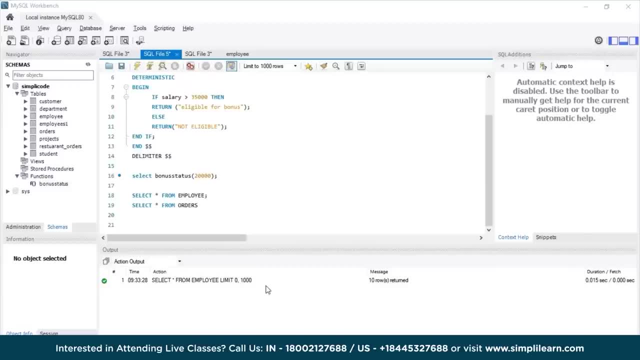 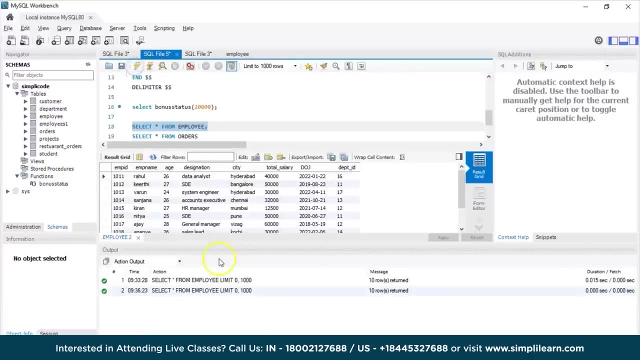 By passing certain parameters into that function. Let us understand this with an example. Consider the employee table here. So let me just display the records in that employee table. So, as you can see, the employee table has various columns, Such as employee id, employee name, age, designation, city, total salary. 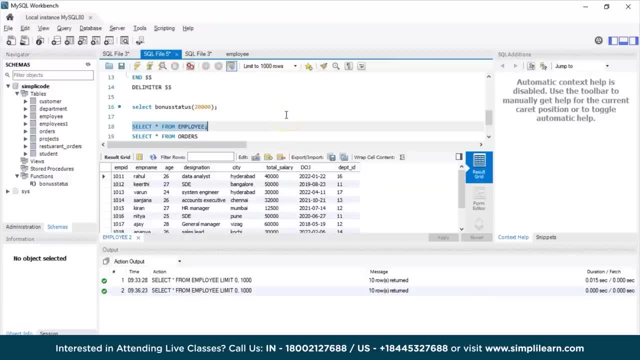 Date of joining and department id. Now, using this already created function, Let us say, if I want to know whether the employee is eligible for the bonus or not, Using the total salary, I will use the function And to achieve that, I will simply use the select statement to display the records. 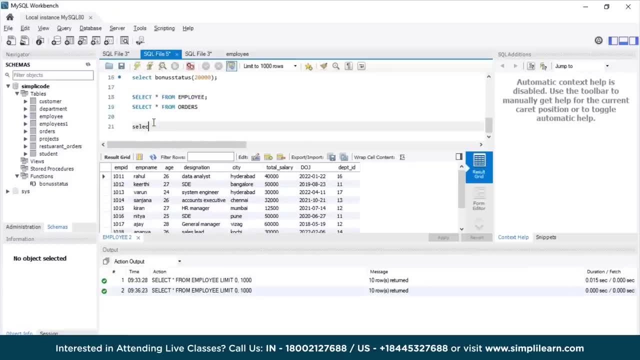 So let me just write the query here: Select. I want to fetch the employee id, employee name, the total salary. So I am mentioning the columns Employee id, employee name, the total salary. Now I will call the function here. 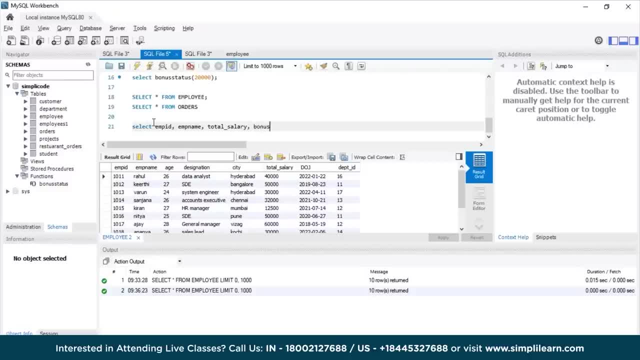 That is our bonus status And inside the function I am going to pass the parameter, which is the total salary, On which we will know whether the employee is eligible for the bonus or not. So I am taking as total salary from the table. that is employee. 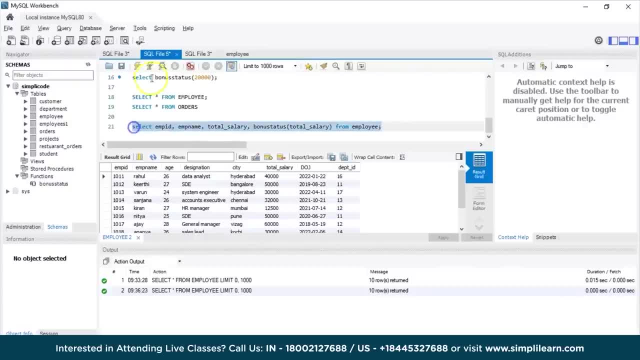 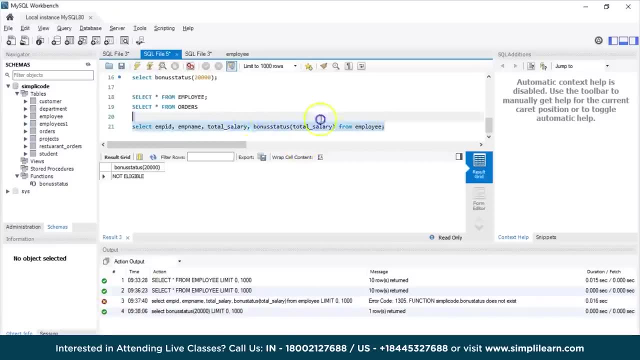 So let us execute the statement and see the output. So there was a mistake in the function name, So let us execute the statement now and we will see the output. So, as you can see, based on the total salary and the function that we have created earlier, 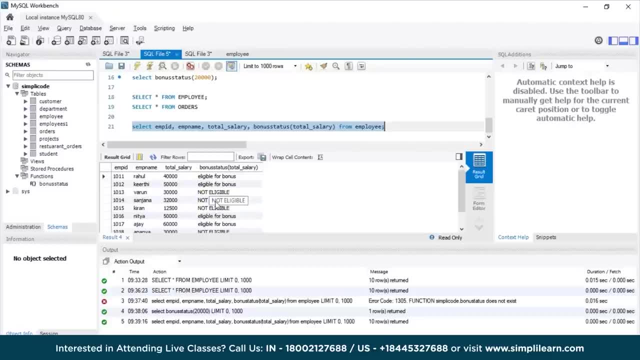 It will result whether or not the employee is eligible for the bonus or not. Now you can see the employee, Rahul, who is having salary 40,000, which is above 35,000.. So in this case it is showing as eligible for bonus. 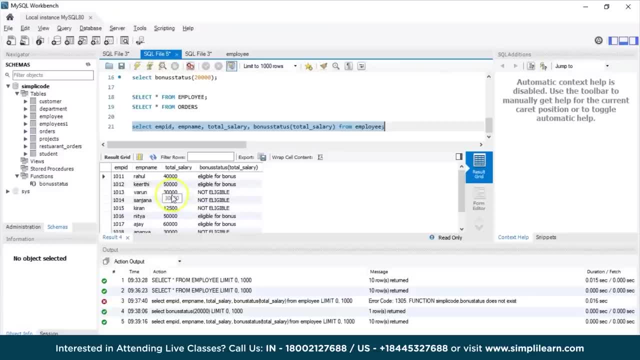 Now, if you consider another employee, Varun, whose salary is 30,000, which is less than 35,000.. So that is why it is showing as not eligible In this way, and for the rest of the employees also, it will show the same, as per the condition that we have specified in our function. 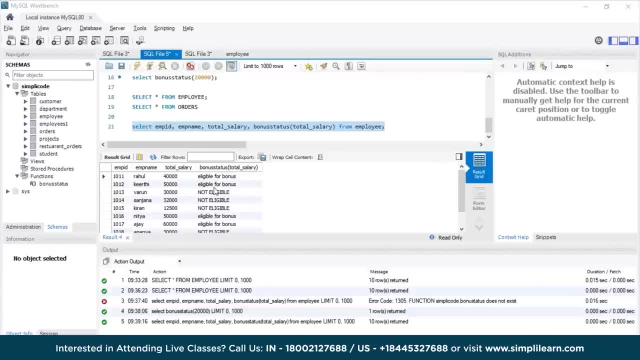 That is, The salary should be greater than 35,000.. So in this way, you can simply call a function using its name and provide the parameter and get the required output. Now the other important thing to notice here is that we have used a function as a column, as a parameter in our select query. 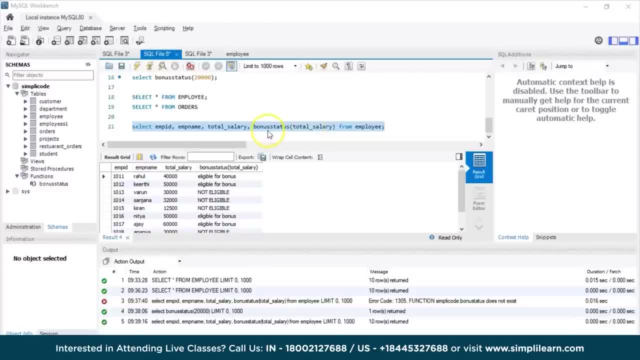 Now we have passed the parameter that is total salary into our function, That is, bonus status, and the function returned a result of this calculation. Now, in this way, SQL function can be very useful, As we have avoided writing complex calculations in a select query. 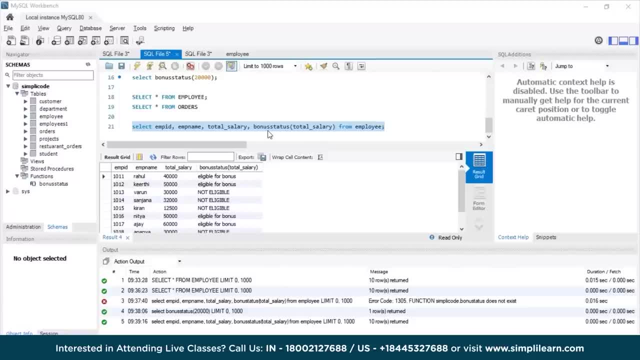 And also we can reuse this function later in any other queries as well. And that brings us to the end of today's session. guys, I hope you understood how to create a user defined function, And in today's session we are going to talk about another important function, that is, conversion functions in SQL. 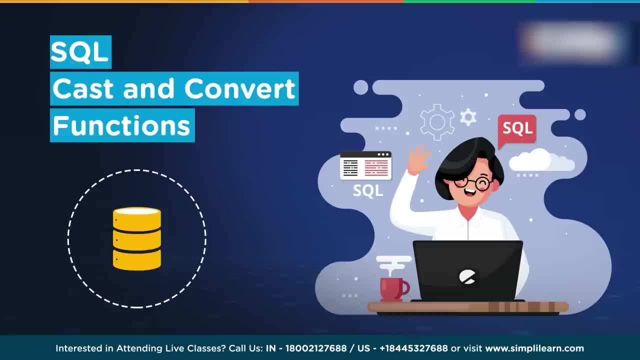 In this tutorial we are going to cover about the cast and conversion which are most commonly used conversion functions in SQL. More on that soon. But before we get started, if you are new to the channel and haven't subscribed already, Consider getting subscribed to our channel. simply quote to stay updated with all the latest tech content. 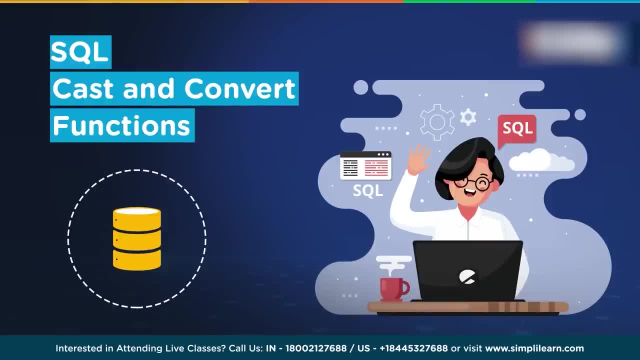 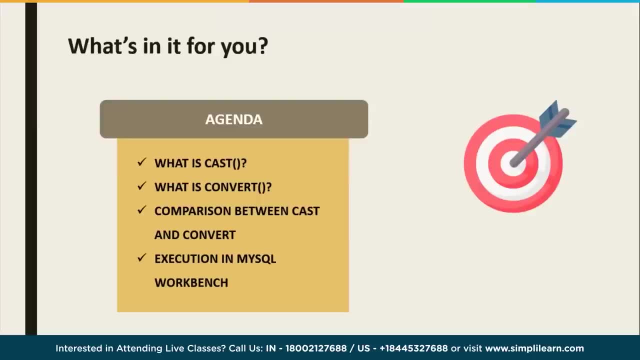 And hit that bell icon to never miss an update from us. So, without any further ado, let's get started with today's topic. Firstly, let us discuss the agenda for today's session. We will start the tutorial by understanding what is cast function, And then we will discuss what is convert function. 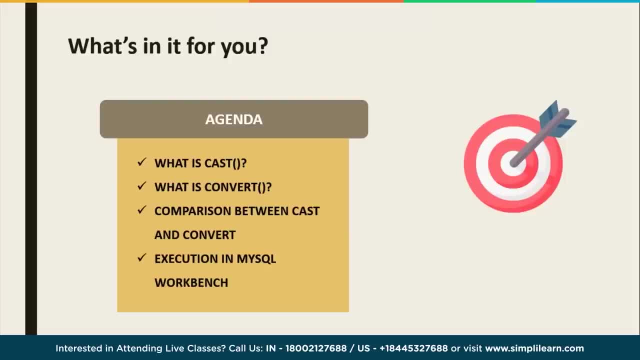 And next we will have a detailed tutorial Comparison between the cast and convert function and see how they are different from each other. And finally we will execute these two functions in MySQL workbench using various examples. So let us get started with today's topic. 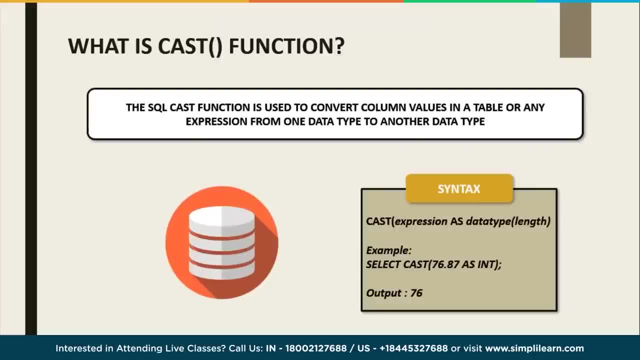 So, firstly, what is cast function? The cast function in SQL is one of the most commonly used conversion function which allows the user to convert from one data type to another. It is very useful for concatenating results from various data types. Now, this conversion can be either a single expression or the values from the columns in the SQL tables. 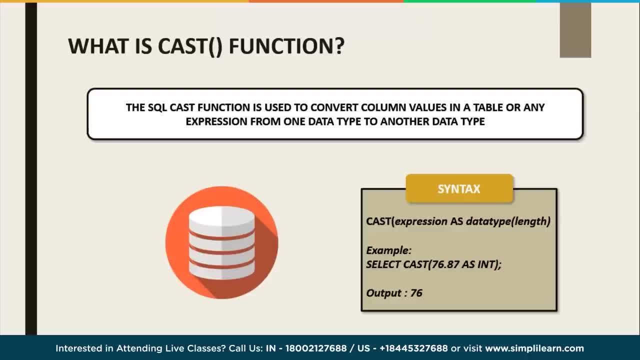 It also allows the user to perform calculations on two different data types as well. Now, using cast, it does not change the data complete in the database. This conversion of data from one data type to another is only valid while the query is running and is not permanent. 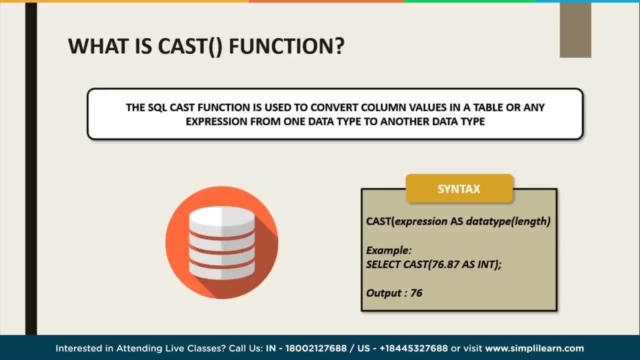 That is, the changes to the query, is only done on a temporary basis. However, it is possible to convert and insert into a new column or table as well. Let us now understand the syntax of cast function. The syntax is followed as cast expression as data type length. 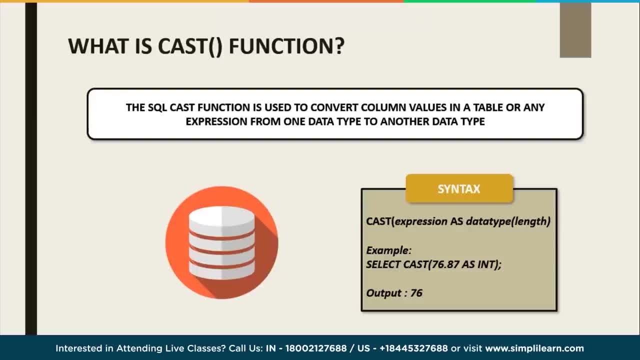 Expression here represents the data which we want to convert And the data type specifies the data type which we want to convert. the value And, finally, the length of the data, which is optional. You can give it a name. You can also give it as per your requirement for only certain data types, such as ncar or varcar. 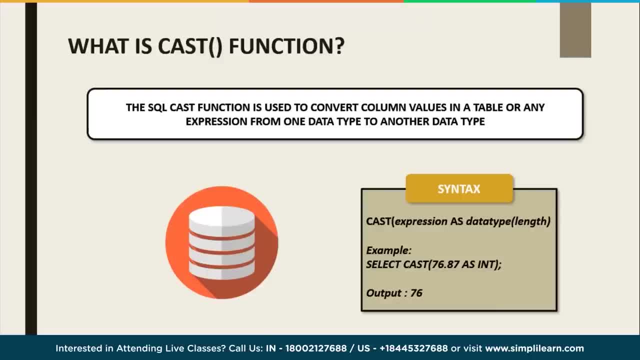 Now let us consider an example here which says: select cast 76.87 as int. Here I am taking a string value which is 76.87 and I am converting this data type into the int value. Now the output is as expected, that is, 76, which is an integer value. 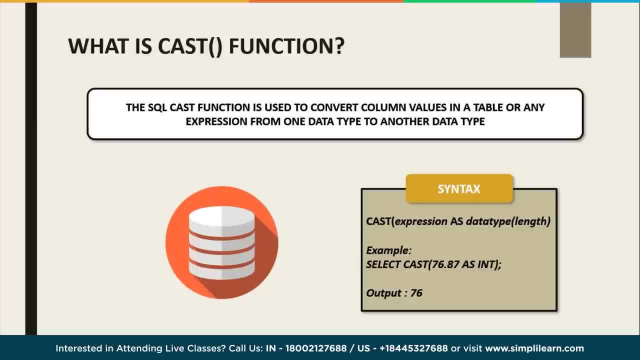 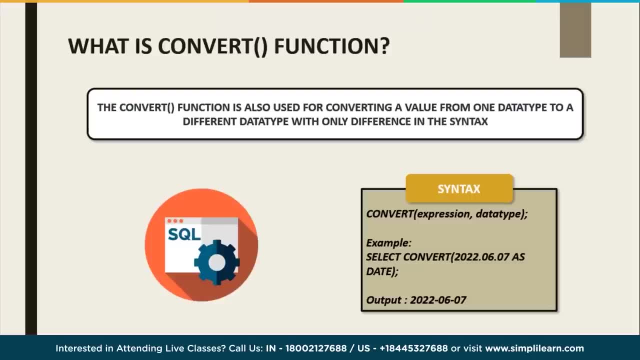 In this way, you can use the cast function to change the value. You can also use the cast function to change one data type to another data type in real time. Next, let us discuss about what is convert function. The convert function converts an expression in one data type to corresponding value in other data type. 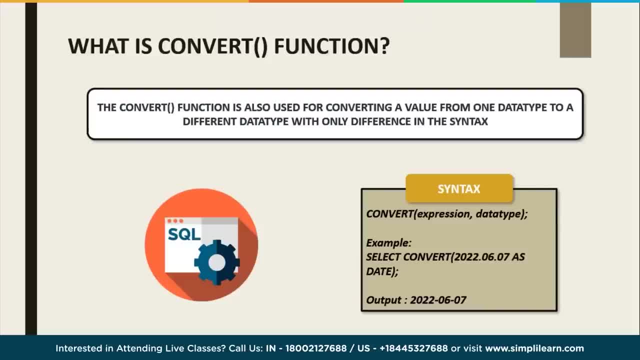 Now you might be confused that the convert is different from the cast function. Convert is similar to that of cast function as well. While the functionality of both these conversion functions is same, The only main difference is the syntax and the usage, So you can specify the format to convert as well as the data type in the convert function. 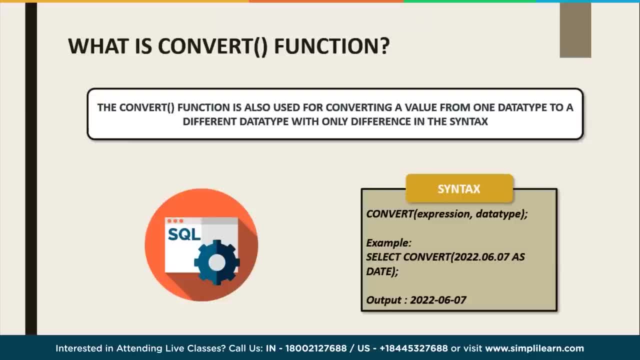 And it is a very useful function, especially for converting the strings to date formats, And the syntax is followed as: convert expression comma data type. Now again, the data type parameter defines the target data which is to be converted Now, and the data type parameter can take data types as an input. 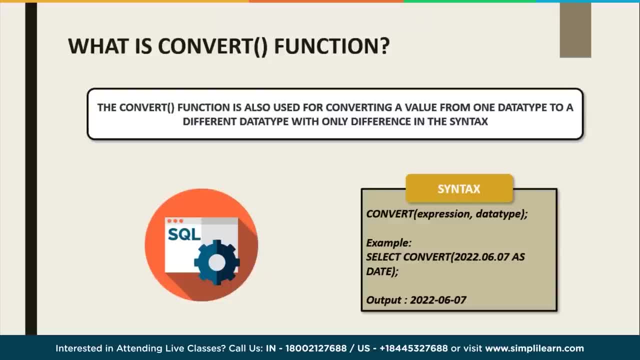 Such as big int, small int, decimal numeric values, float values, character values, variable characters in char, etc. And the length is optional parameter which specifies the target data type length And the default of this parameter is around 10 or 20.. 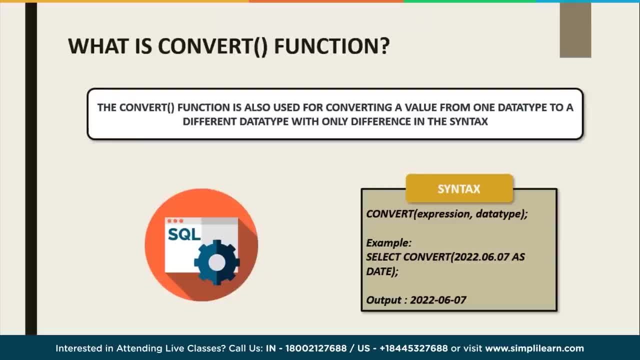 Now we also have the expression. This parameter specifies the value in which we want to convert to another data type. So let us consider an example here, Which is: select convert 2022.06.07 as date. Now, this is basically a string value, or you can say a part of a decimal value. 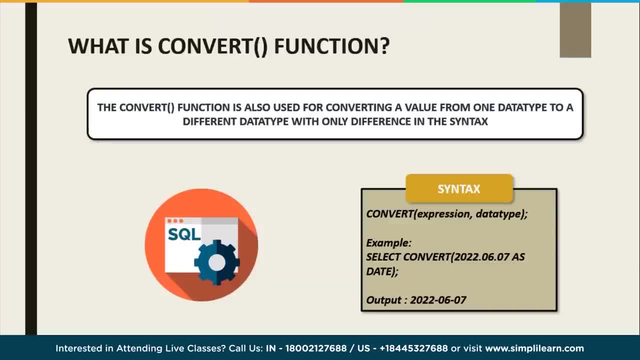 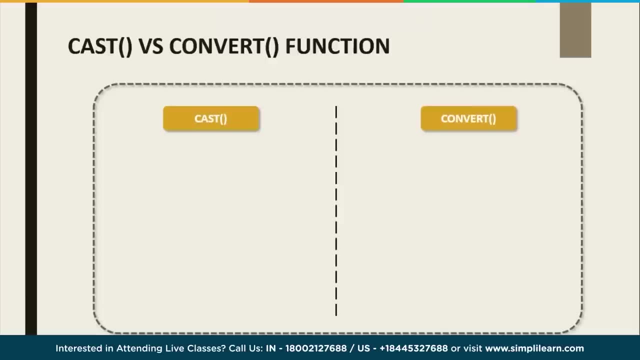 And I am changing this string or character into date format, Which is 2022-06-07, which is converted into date format. So in this way, you can use the convert function as well. Let us now understand the difference between the cast and convert function. 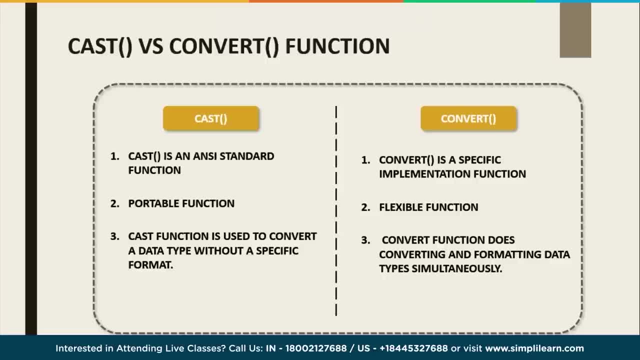 In SQL. Now, both these SQL conversion functions are row functions which are capable of typecasting column values Or an expression from one data type to another, And the functionality of both of the functions are almost similar, But there are some major differences in them as well. 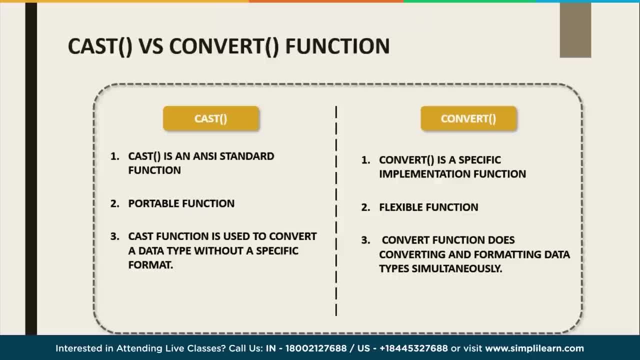 Now, both the cast and convert functions are obviously used to convert one data type to another data type, And one of the main differences is the syntax. The syntax of cast is very simple. It includes the value to convert and the type of resulting data type. 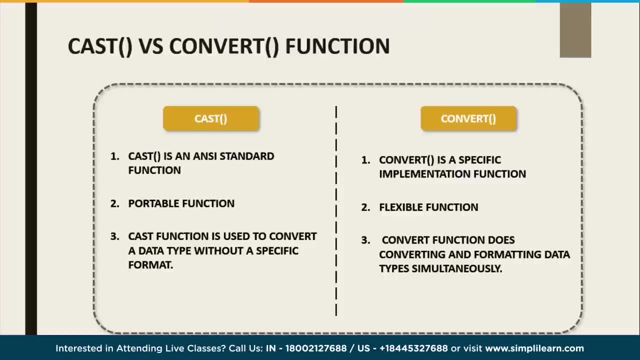 It has as as a keyword to separate the data type from the value, And there is an option to express the length, Which is the integer that specifies the length of the target data type, And, on the other hand, the convert syntax mentions the resulting data type first. 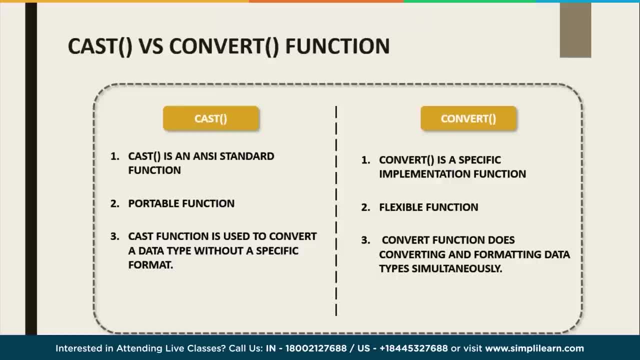 Along with the optional length, There is another expression and another optional parameter called style in the convert function, Which is only specific to the object SQL Server Database. Now this style allows formatting the data type And specifies how the convert function should translate or format the data type. 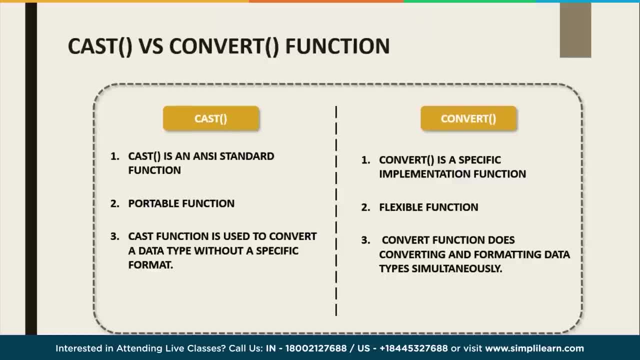 Now, apart from these, there are some certain differences as well. The cast is an ANSI standard function, That is, cast is considered as the American National Standard Institute's standard function. That means it is applicable to most of the SQL databases out there, Like PostViewSQL, MySQL. 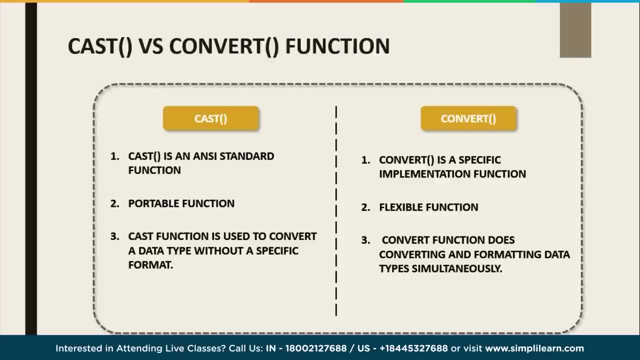 MariaDB, MongoDB, etc. On the other hand, conversion function is a specific function That is only restricted to mainly Microsoft SQL Server. Cast function is also more portable function of these two. It means that the cast function can be used by many databases out there. 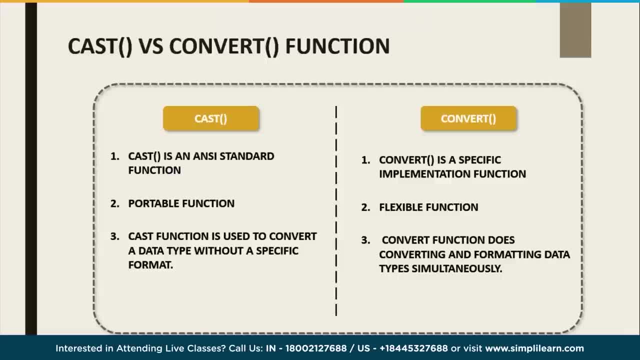 And also cast is considered less powerful and less flexible than the convert function And, on the other hand, the convert function is generally considered as a flexible function Which allows more flexibility and is mostly preferred to use for datetime values, etc. Convert is also useful in formatting the data's format as well. 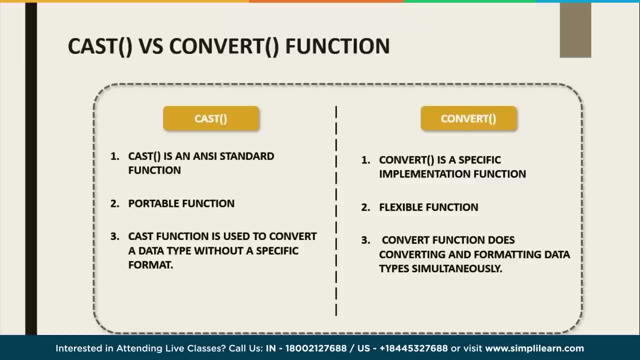 And finally, cast function is used to convert a data type without a specific format, Whereas the convert function does converting and formatting data types simultaneously. Now, for example, cast cannot convert a datetime to specific format, Whereas the convert function can do that. So these were some major differences between the cast and convert function. 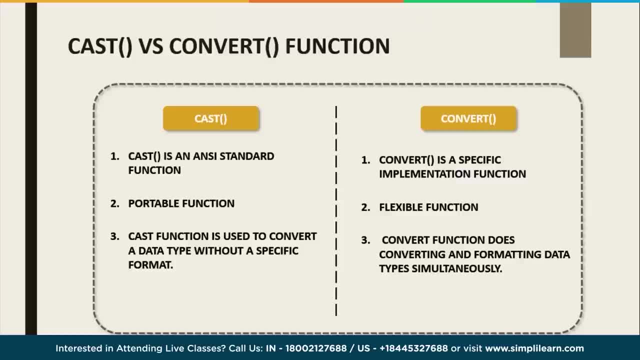 I know you might be confusing at first, Because there isn't much difference between these two functions, And also there is no difference in the performance of these two functions as well. So it's just a matter of preference to choose which function to use. 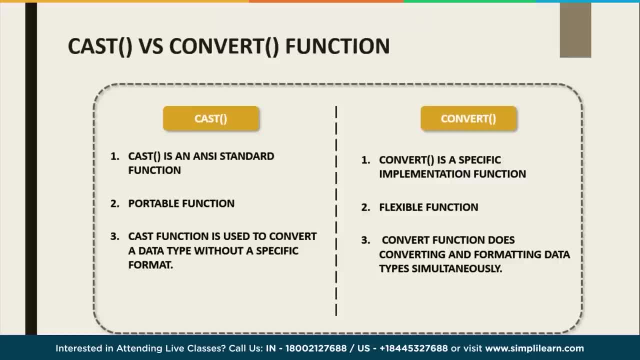 You can choose to use cast when you work with multiple relational databases, And the syntaxes are pretty standardized, Easy to remember And since it is an ANSI standard function, You can use it in any database as well. On the other hand, if you need to specify the output styling. 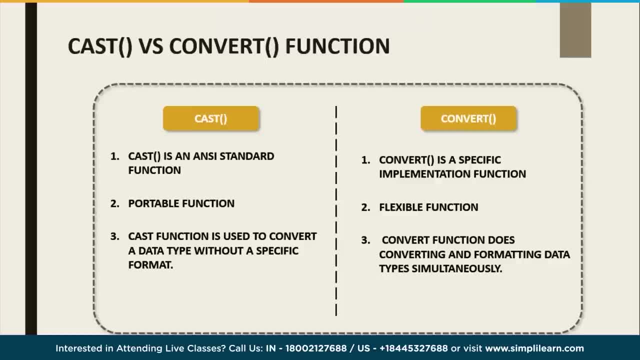 We can use the convert function for that, And even though the style is optional and is limited to certain databases like SQL server, The cast function is often used to preserve decimal values and places While converting between decimal numeric values, Whereas the convert function cannot do this. 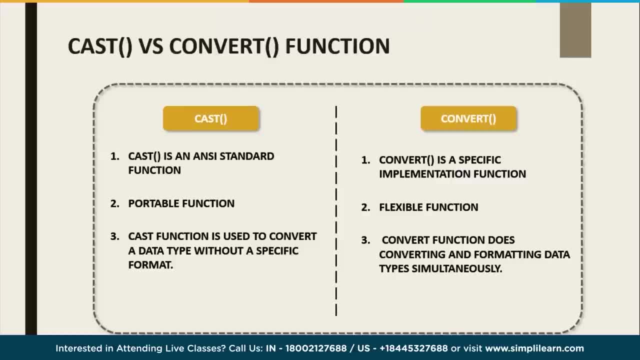 So it is a matter of requirement when to use both these functions, And it is up to the user to choose between these both conversion functions. So now that we have understood about these two functions, Let us jump into MySQL workbench for execution part. 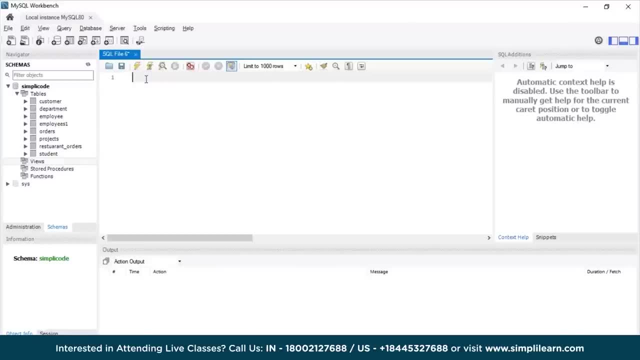 As you can see, MySQL workbench has started And we can now work on our conversion functions. Firstly, Let us discuss about the cast function in SQL. So let us take an example for this. Let's say, if I want to convert a string value into an integer data type, 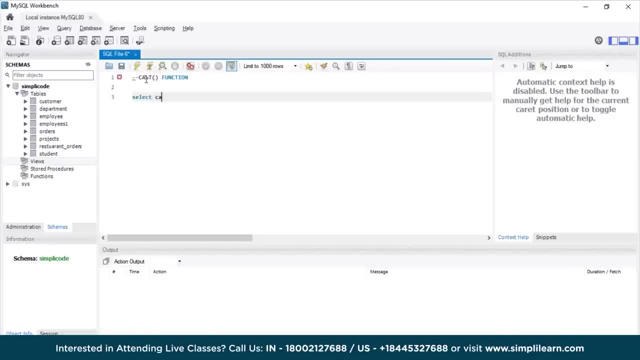 Then the following query would be: SELECT, cast. And within the parenthesis, Let's say, I have a string value which is 45.68.. And I want to change this into int data type, So I will mention int as int, Which is the keyword. 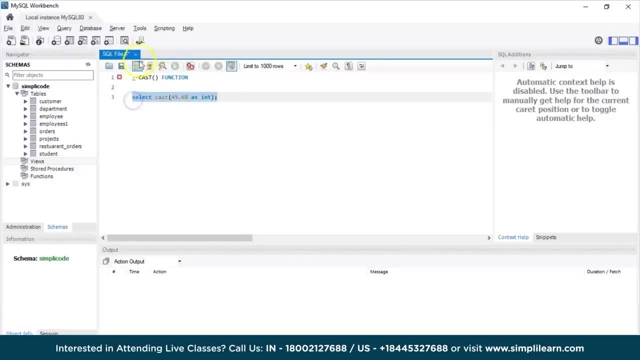 We use in the cast function. So let us now execute this statement and see the output. Now it will show me an error. That's because the int data type is not supported in MySQL workbench, If you are working on cast function. So instead of int you can take the signed function. 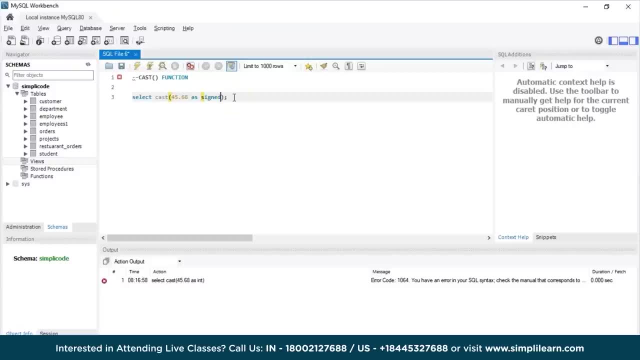 Which is basically a sister group of the int data type, So you can take the signed integer as well. So let us now display this value. So, as you can see, it will return me the 46. Which will round off the decimal value. 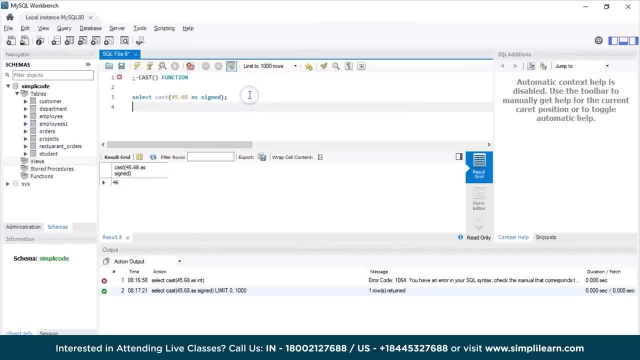 Which is 45.68 to 46.. Now let us take another example. Let's say I have a string value. I want to change it into date format. So then the following query would be: SELECT cast. So let me just take some string values. 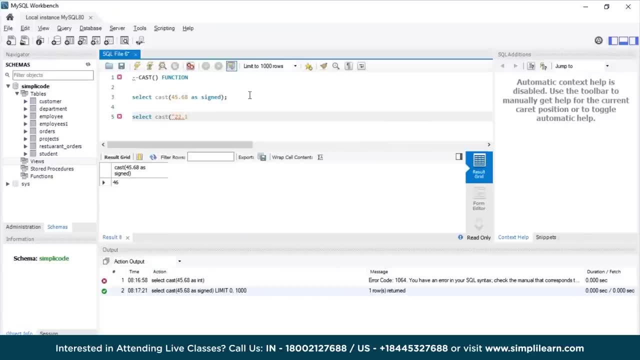 Like 22,, 9, 24.. As DATE: So let us execute this statement And we will see the output, So as you can see The string value that we have taken here, Such as 22,, 9, 24.. 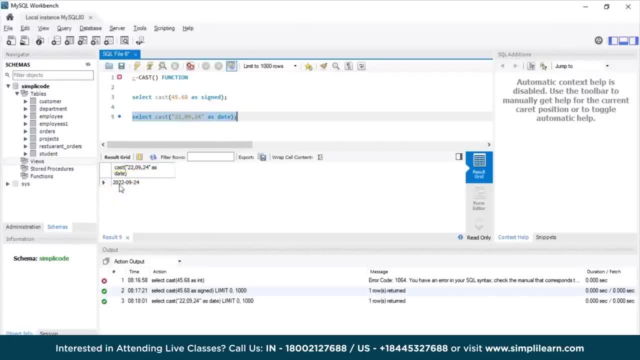 Has been changed into date format, Which is 2022., Which is the year. 9 is the month And 24 is the date, Which is in the format of year, month and date. Now, if you pass the values here, 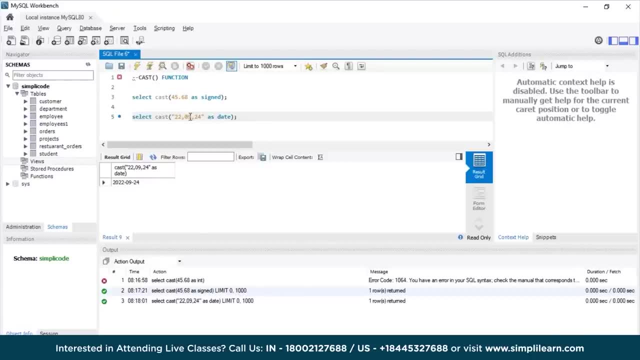 Which is not in the range of the function Of the data type that you have specified In this function, For example, Instead of 9.. If I take 14. And let's say, if I want to pass this function, Then it will show me a null value. That's because The value 14 is not in the range of the date value, That is 14.. There are only like 12 months, So the values it can take is only from 1 to 12.. Now if you pass other than this range, 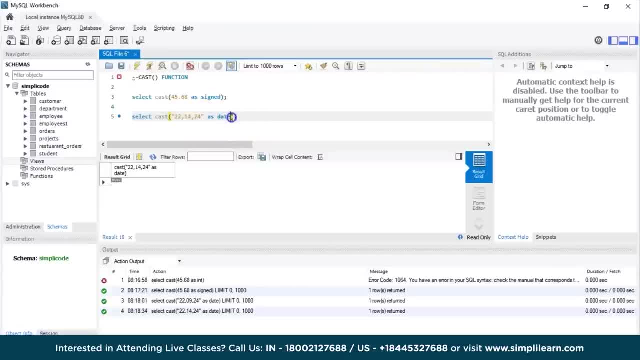 Then it will show an error Now. similarly, If I want to specify this value into date time function, Then I can simply mention the date time function data type as well. So let us see the output. So it will show me the output in the form of date. 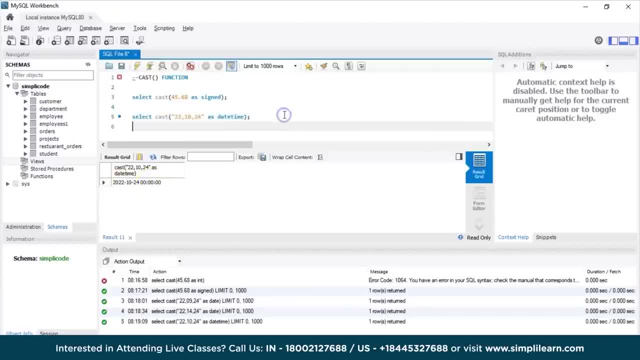 As well as the time format here. So let us now understand another example. Now, as discussed earlier, A cast function not only changes the data type Of an expression, It can also change the data type of the column values in the table as well. 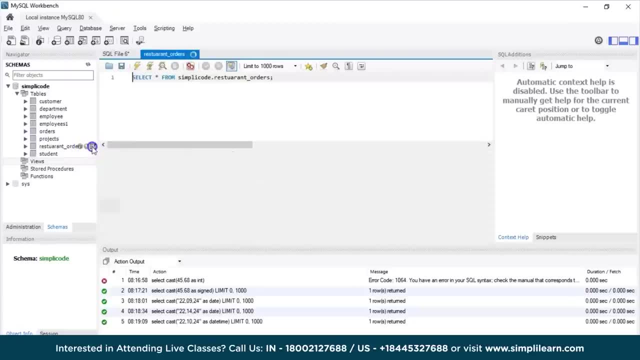 So for that, let us take an example for this, Let me consider the restaurant orders table here. Now I have this price column Which is in decimal values. Now let's say, if I want to round off these values into integer values, Then the following query would be: 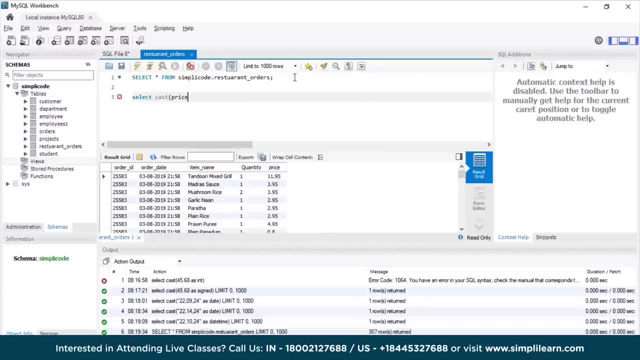 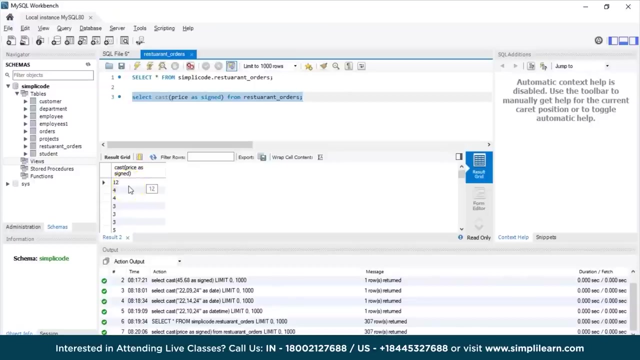 Select cast Mention the parameter which is price As Sign From The table name, that is, restaurant orders. So let us execute and see the output. So, as you can see, the prices have been changed Into the integer values now And the decimal values have been rounded off. 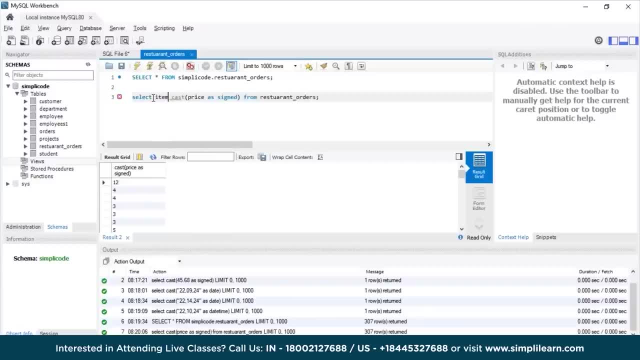 So, similarly, if I want to mention the columns, I can mention them as well. So I will take the item name, The previous price And the change price. So I am giving this change price as the new price, As a new column. 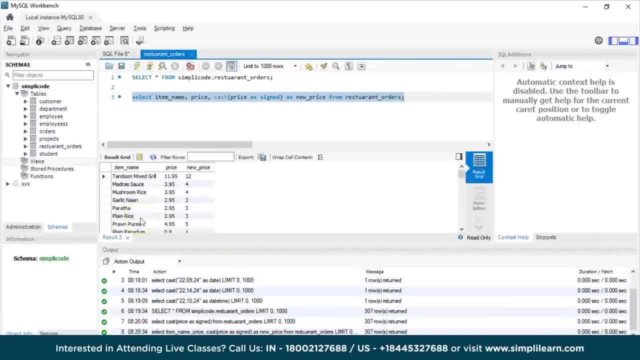 So let us now execute this statement And see the output. So, as you can see, it will display The item name, The price And the new price of these items. Now, as you can see, the price of the tandoori mix grill. 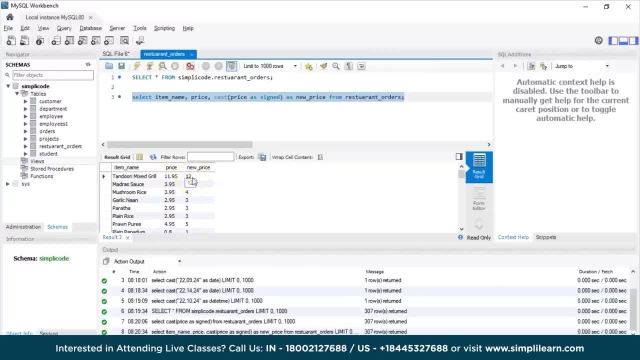 Which is 11.95, has been rounded off To an integer value that is 12.. And similarly all the other values as well. Now, if you scroll down a bit, As you can see, We have a price which is 0.5.. 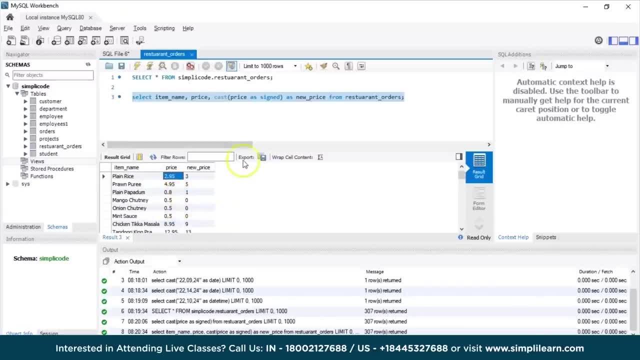 And the new price is changed into 0. Which is not acceptable. right Now, the price has should be of a value Now instead of sign. If you can take the decimal data type Where in you can mention this And it will change the value. 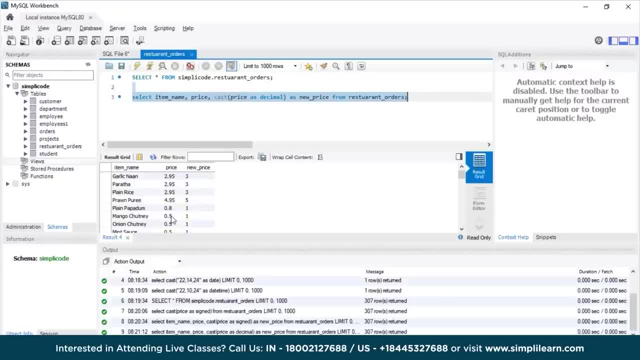 Into the nearest value of the decimal value. Now, as you can see here, The 0.5 has been rounded off to 1 here, And similarly 0.8.. Which is more than 0.5 is also rounded to 1.. 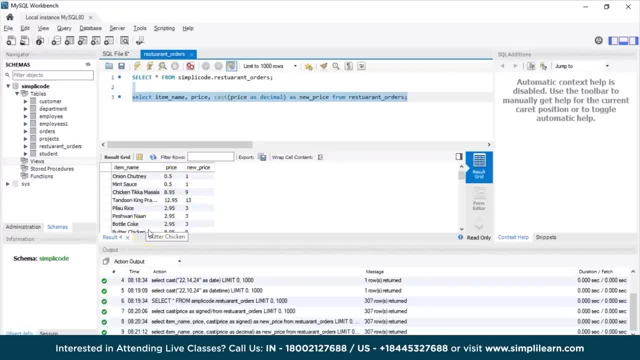 So in this way, you can use the cast function To change the data type accordingly. So now that we have covered the cast functions, Let us now see a few data type conversions here, Which will help you understand the usage Of the convert function as well. 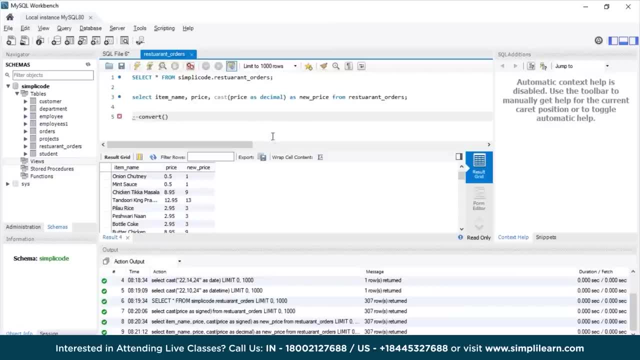 Now, firstly, let us start with the decimal data type. Now, as the name suggests, Decimal produces a decimal value And has two optional parameters, Which is basically m and d, Where m is the maximum number of digits That you want to show in the resultant table. 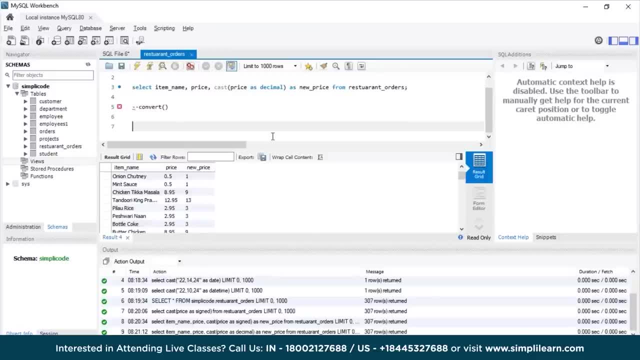 Which is also known as precision, And d is the number of digits After the decimal points from the scale You understand with an example here. So the following query would be: Select, convert And inside the convert, Mention the expression. So I am taking the value as: 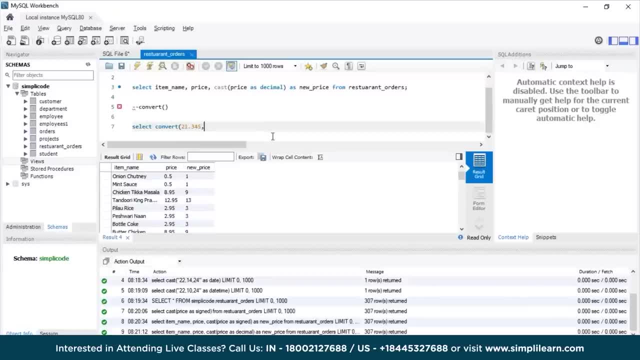 Let us say 21.345.. And I want to change this value Into decimal data type And inside the decimal I am mentioning the parameters. So I am taking as- Let us say 7. As the total number of digits. 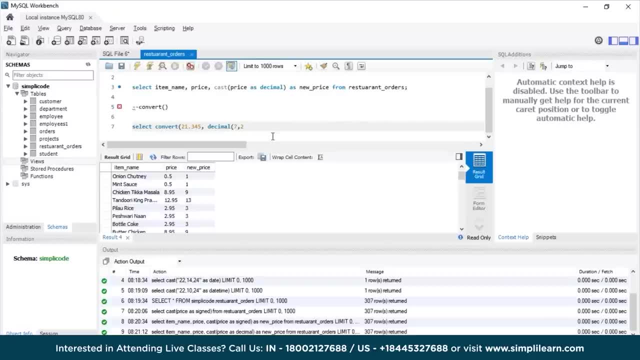 That I will display, And I am taking only two decimal values That I want to display After the decimal point. So let us just execute this statement And we will see the output. So, as you can see, It will show me only the two values. 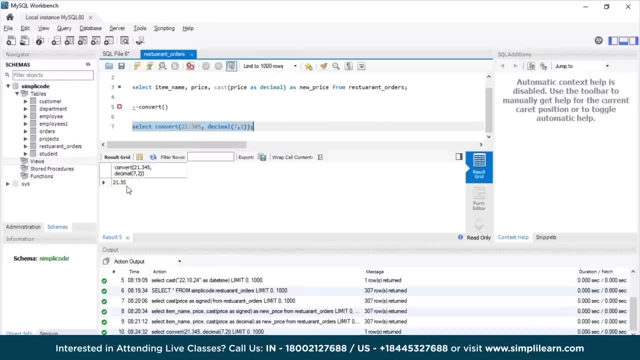 That is 35. After the decimal point. So the output is 21.35.. Now the value that we have taken is 21.345.. Which is converted into decimal Data type format, which is 21.35.. Basically it will round off. 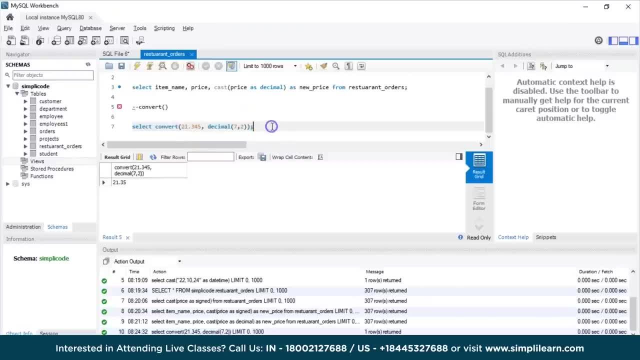 The value of 345 into 35.. Now, similarly, You can convert the values Into date and time data types As well in using the convert function. So let us consider the example For that as well. So select, convert, Let us say now: 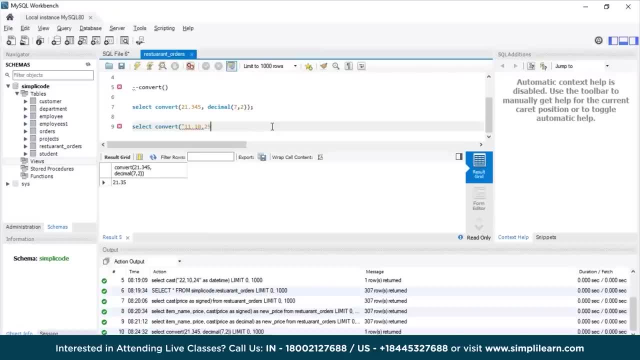 I have a value 10, comma 25.. As date time Data type, So we will convert this into date time Data type. So let us see the output. So, as you can see the value, The string value which was specified here, 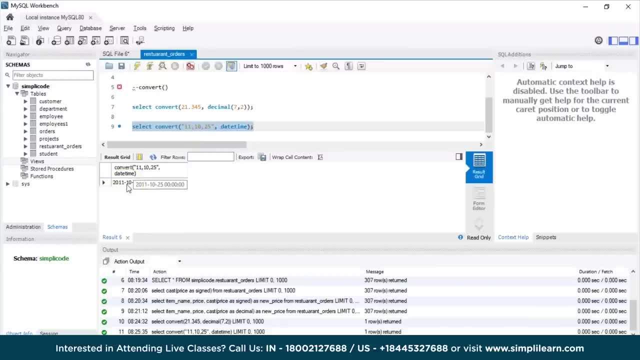 As 11.10.25.. It will be changed into the date time data type, That is, 2011.10.25.. And the time as well, And similarly You can use the convert function To change a number or a string value. 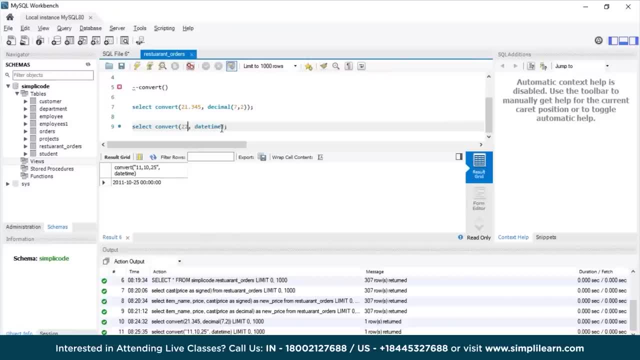 Into year data type as well. So let us say I am taking a value 22. And I want to change this string value Into year data type. So the following query would be: Select, convert 22 as year. So as you can see the output, 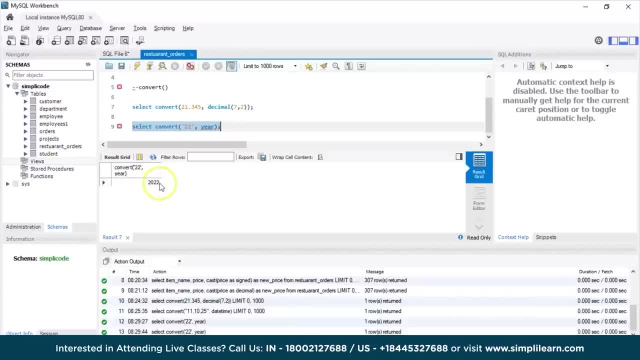 The value- the string value That we have taken as 22. Has been now converted into 2022., Which is in the format of year data type. Now, similarly, you can convert A string value into the time as well. So let us say: 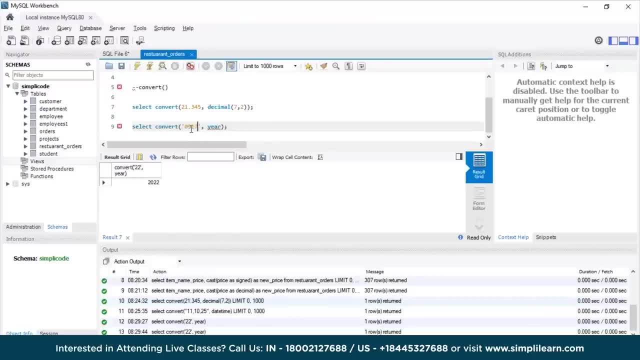 I am taking a value like, let us say, 09.17.26.. And I am specifying the data type As time. So let us see the output For this as well. So as you can see the string value That we have taken as 09.17.26.. 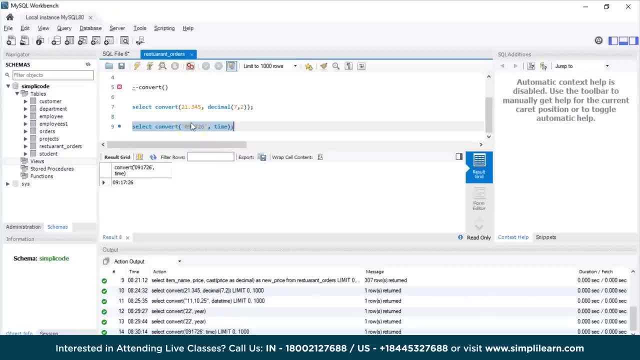 Which is basically a number, And we want to convert that number Into time data type, So it will display the value as 9.17.26. In the format of hours, minutes and seconds. And that brings us to the End of today's session, guys. 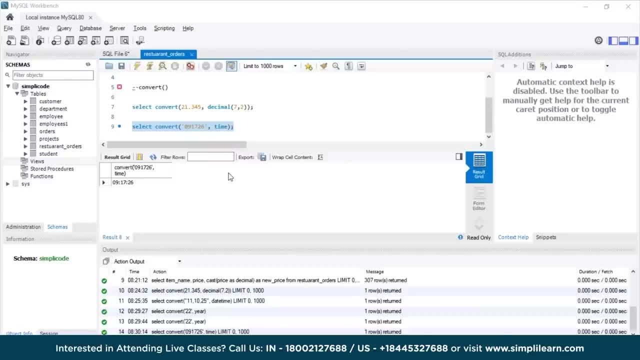 That was all about the MySQL conversion functions. We have studied and understood What convert and cast function does, How exactly it works, Its parameters, with some examples Now you can try converting The value in every valid data type Using these two functions. 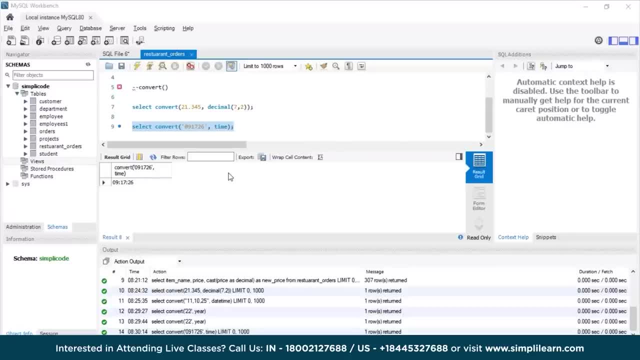 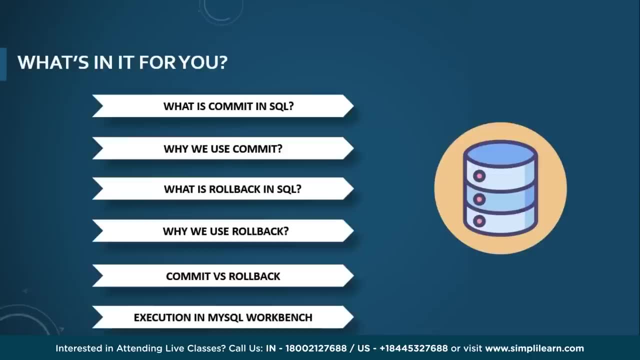 That is, convert and cast. So I hope you found this tutorial Helpful and informative. We will start the tutorial by understanding What is commit in SQL And discuss why we use commit, And then we will understand What is rollback in SQL. 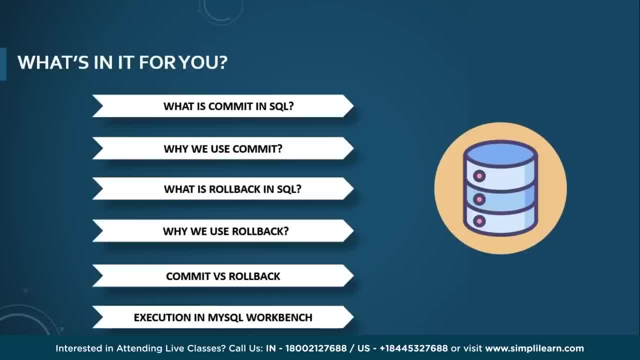 And discuss why we use the rollback command in SQL, And then we will have a detailed comparison Between commit and rollback And see how they are different from each other, And finally We will execute both these commands In MySQL Workbench. So what is commit? 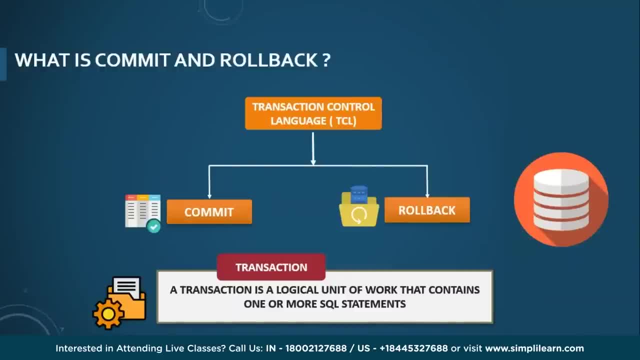 And rollback in SQL. Commit and rollback Are the commonly used Transaction control language commands, Or TCL commands, used in SQL. These TCL commands, Or transaction control language commands, Are basically used for managing And controlling the transactions in a database To maintain consistency. 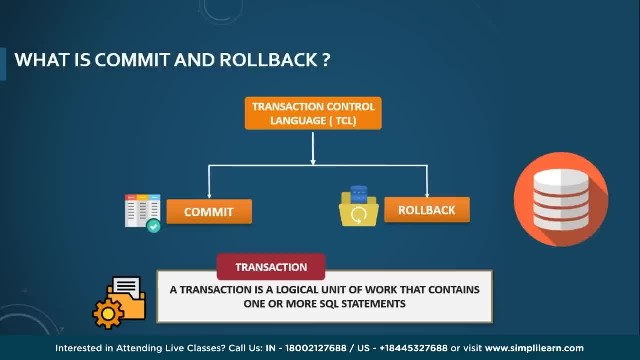 And it also helps a user manage All the changes made by the DML commands For maintaining its transactions, TCL lets the statements Get grouped into a logical transaction. Now, to understand More about commit and rollback, We need to understand what exactly are transactions. 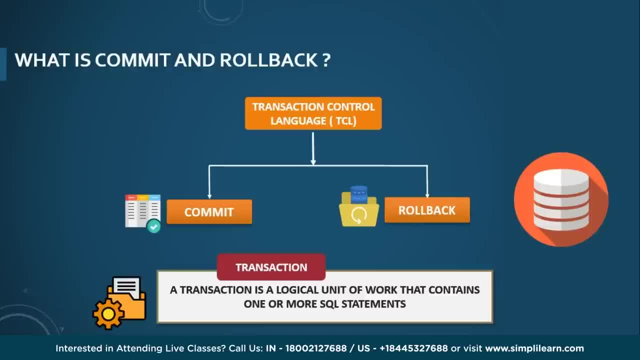 Now a transaction is basically A block of SQL query Or set of SQL statements Executed on the information And data stored in the database management system. So any transaction, When made, happens temporarily Or permanently in database. Now a user needs. 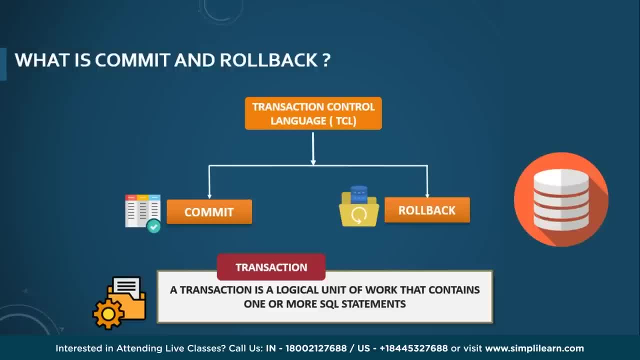 TCL commands to make these changes Permanent or temporary. For example, If you are creating a record Or updating a record From a table, Then you are performing a transaction on that table. So it is important to control these transactions To ensure that the data integrity. 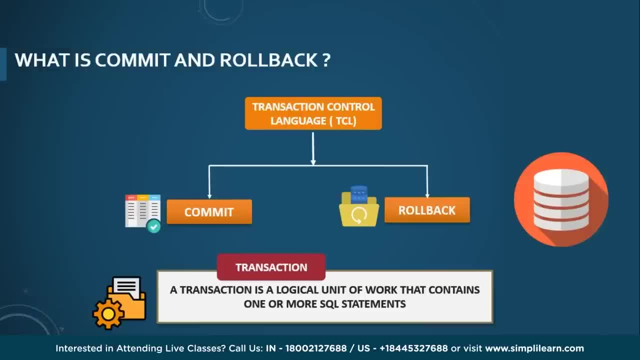 Is maintained, And it also handles the database errors effectively. So generally, you will incorporate Many SQL queries into a group And you will execute all of them together As a part of a transaction. Next, let us discuss About the commit command in SQL. 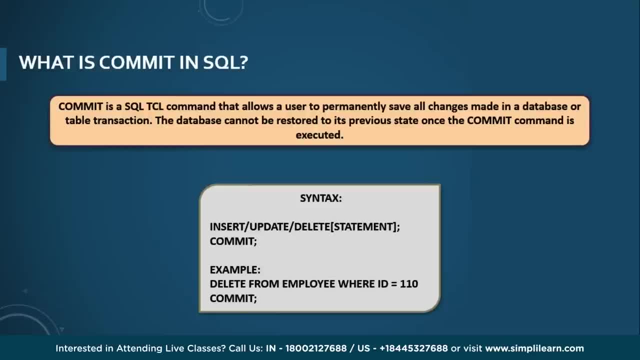 The commit command in SQL Is a transaction command That is used to save Any changes made by a particular transaction In RDBMS Since the last commit Or rollback command is used. It signifies the end of a successful transaction In an SQL database. 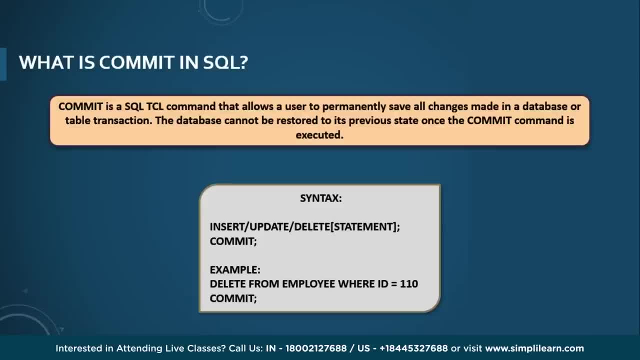 Now, generally, the commit command Is used after a data manipulation Language or DML operations Like insert, delete and update transactions. Now, when you perform a DML operation Without a commit statement, The changes are only visible to you. Now you can use a select statement. 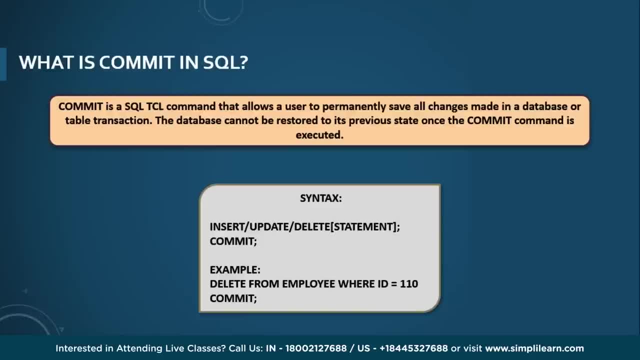 And check the updated records For a data, But once you use a commit command After a transaction, The changes in the table or database Are visible to other database users as well. Now, another thing to keep in mind Is that the database cannot be restored. 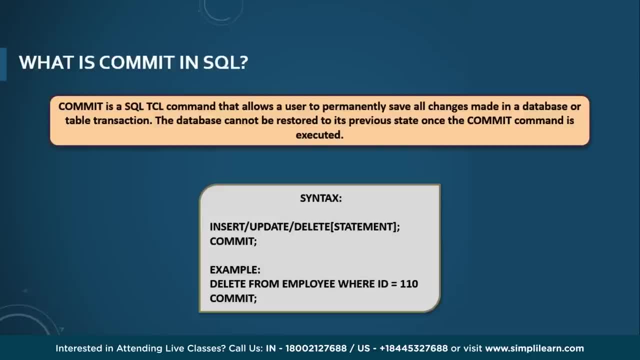 To its previous state. Once the commit command is executed, All the transaction commands Obeys The basic principles of asset properties In SQL, And the syntax for commit in SQL Is followed as. So the syntax is basically: Is uses just one keyword. 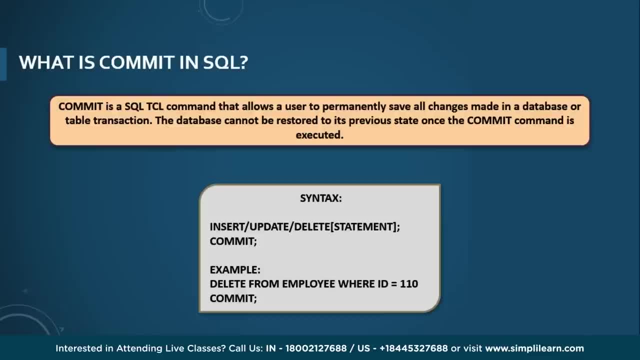 That is commit, And you can use this commit Using various DML operators Like insert, update, delete statements as well. Now let us say, for example, I have an employee table And from that I want to delete An employee record. 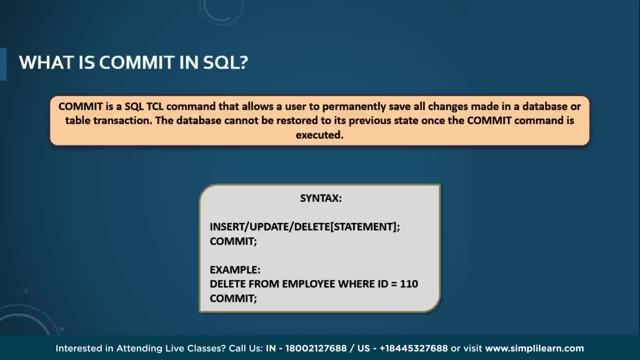 Whose ID is 110.. Now, when I perform this query, It will delete the employee ID 110. And then if I perform a commit operation, Then it will permanently save The transaction, That is, it will completely delete the record from the table. 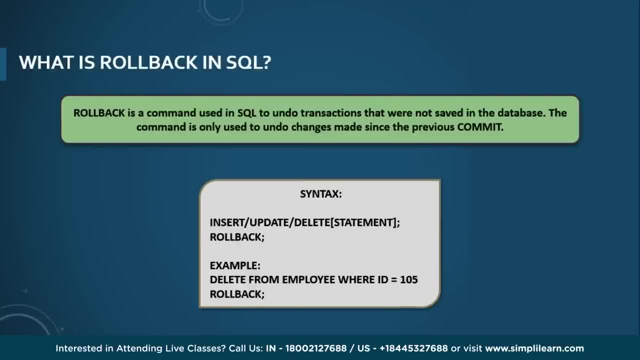 Next, let us discuss about The rollback in SQL. The rollback in SQL is a command That is used to revert changes Performed by a transaction. Now, whenever a rollback command is used, It reverts all the changes Since the last commit or rollback. 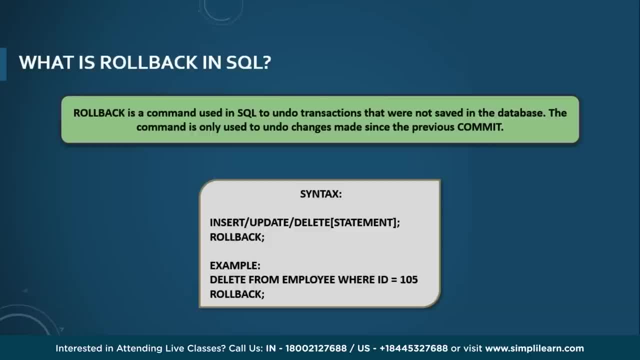 That we have made in our SQL table. The syntax is similar to that. It is includes just one keyword, That is, rollback. Similarly used with the insert, update, delete statement. And let us say, for example, I am deleting a record. 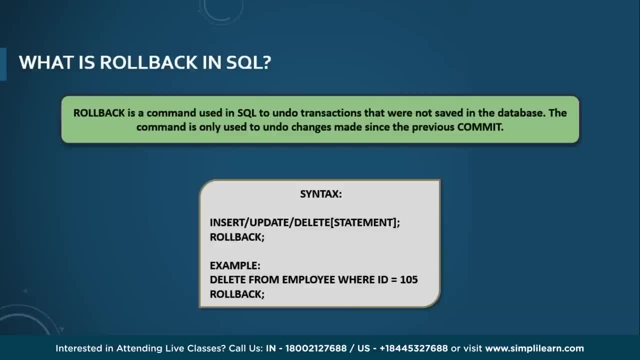 Whose ID is 105.. And for some reasons, if I want That record back in my table, Then I will use the rollback command here, Which will restore The deleted record, That is, the ID of the employee Who is having as 105.. 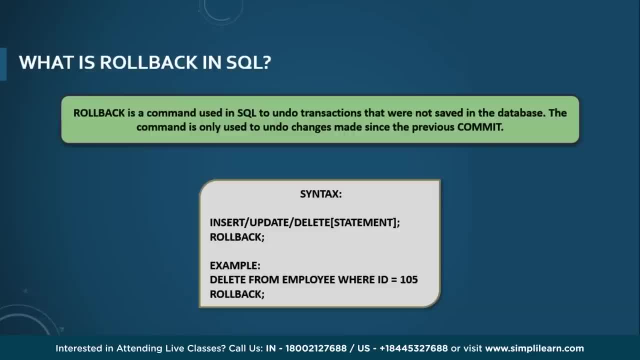 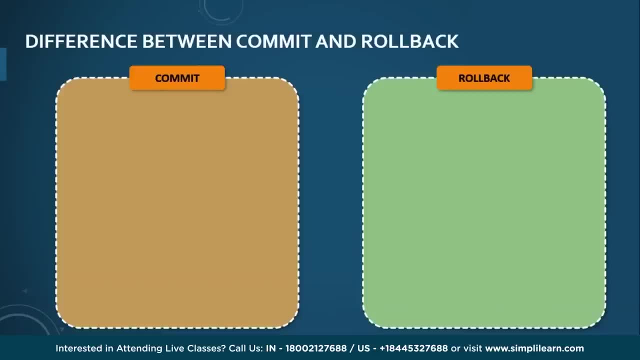 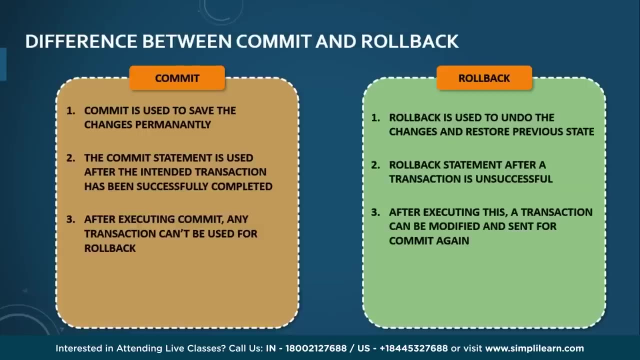 So it will revert back The changes that were made in the database By bringing back the original state. So it will revert back. Let us now understand Some differences between commit And rollback. The commit is used to save the changes Permanently in the database. 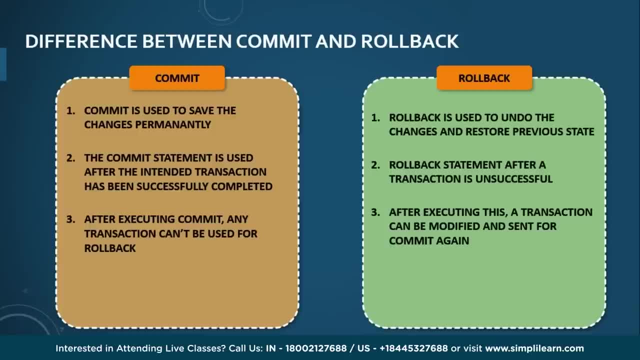 Whereas the rollback is used to undo the changes And restore its previous states, The commit statement Is basically used after An intended transaction Which has been successfully completed, That is, if you are performing any SQL operations Or transaction in SQL And if you are sure that. 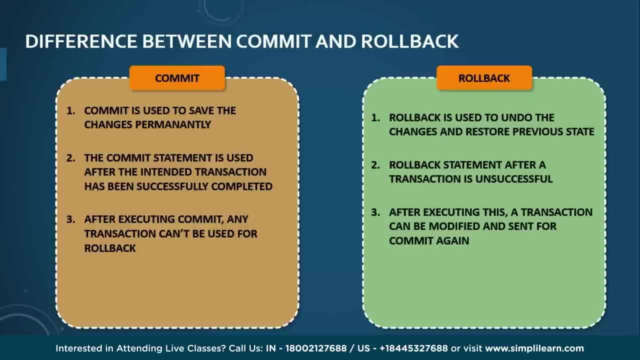 If there is no changes to be made In the transaction Only, then you have to use the commit statement, Whereas rollback statement Is used after a transaction is unsuccessful Due to any circumstances, Like system failure, etc. After executing Commit command. 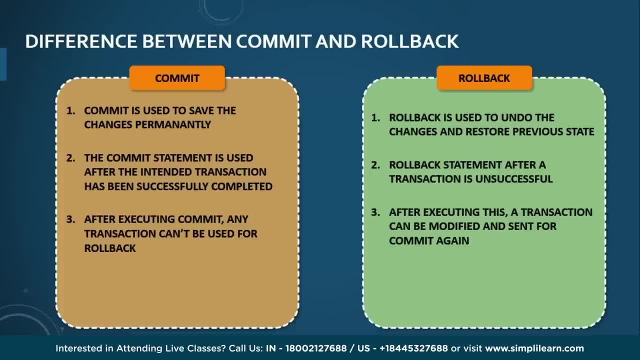 Any transaction can't be used for rollback, Which we have discussed earlier, And on the other hand, After executing the rollback command, A transaction can be still modified And sent for commit again. So now that we have understood The changes and rollback are, 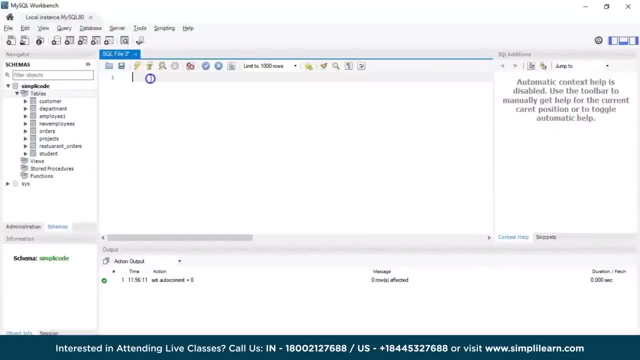 Let us jump into MySQL workbench for execution part. As you can see, MySQL workbench has started And now, by default, MySQL automatically commits the changes Permanently to the database. So in order to force MySQL Not to commit changes automatically, 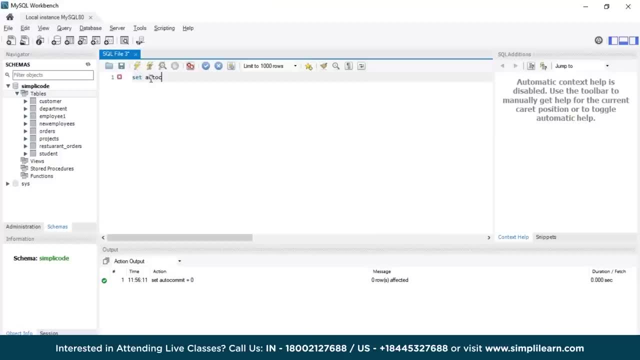 We use a following statement here, Which is followed as: Set auto commit to 0.. So let me just display this. Okay, It is successfully executed. Now what this basically does is It changes permanently That were done prior to the database earlier. 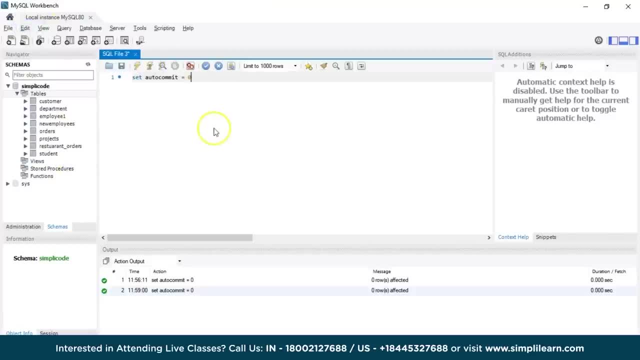 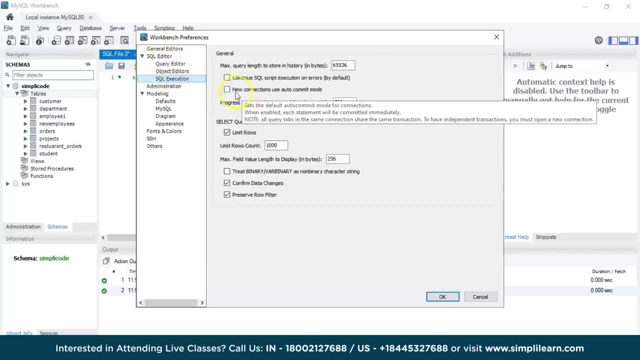 Or else you can click on edit option here And choose preferences And in preferences You will find SQL execution Under the SQL editor section. So you will find an option Which says new connections use auto commit mode. So if you find a tick here in this checkbox, 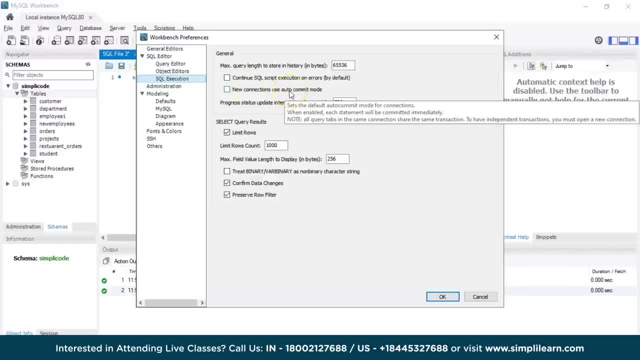 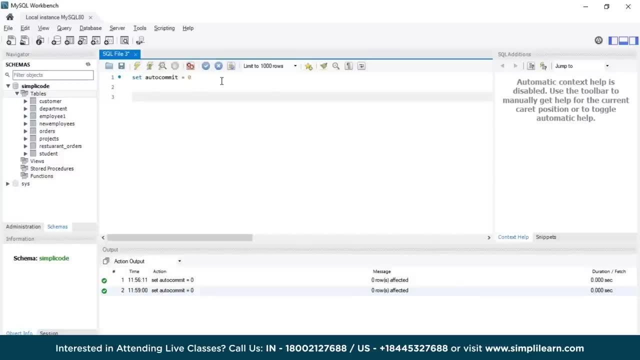 Make sure you untick Before you proceed to commit And rollback commands. So click on okay So that you are good to go now And you will see A table here to perform the commit And rollback commands here. So for that I am taking the employee1 table as a reference. 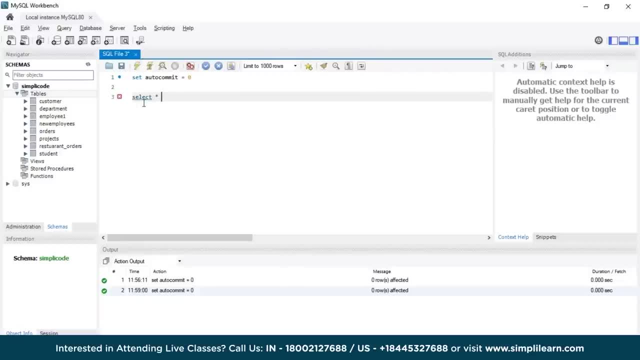 So let me just display the records From that table And I will use the select statement for that Select star from employee1.. So let me execute this statement. So in our employee1. We have various columns, Such as employee id. 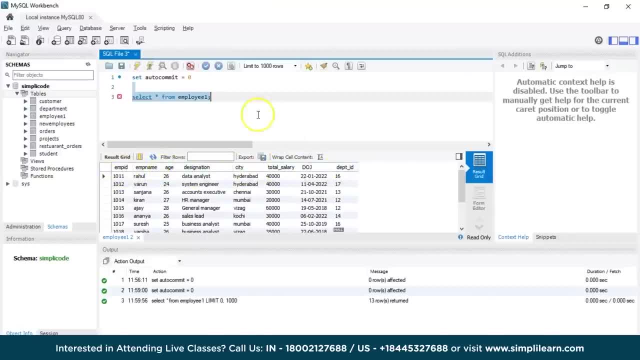 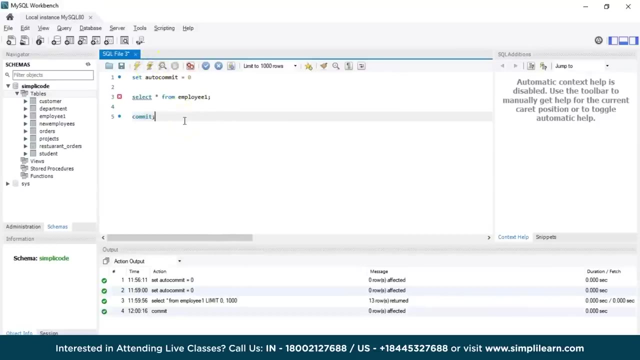 Employee name, Age, designation, City. We want to commit the current transaction And make its changes permanent. We use the commit statement, So I will use the commit command here And I will execute this. So now, basically, what this does is: 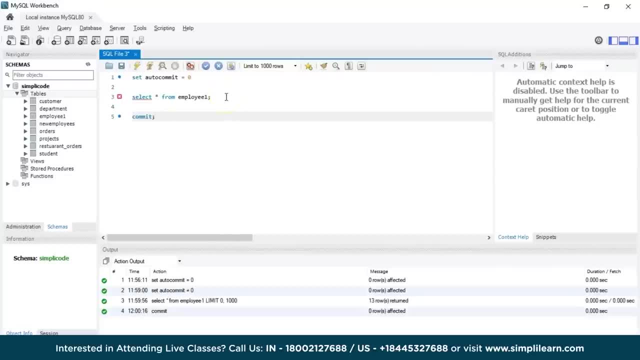 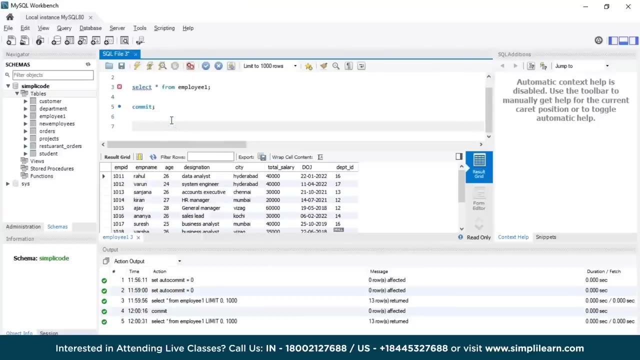 It will permanently Or save the changes That were done prior to this Database. That is database table. That is the employee1 table. So let me just display the values now. So now let us perform some transactions On this table. 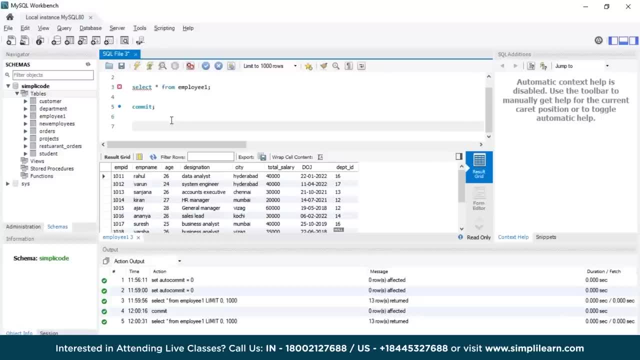 As we discussed earlier, We can use any DML operators Like insert, update or delete, To perform operations using the commit and rollback command. So I am going to use the update Command here. So I am basically updating The salary of an employee. 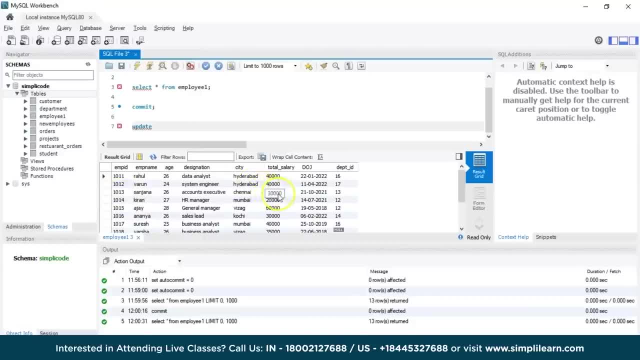 Let's say Sanjana, whose employee id is 1013.. Whose total salary is 30000.. Now I want to update that salary As 35000.. So for that I am using the update statement. Update the table name. 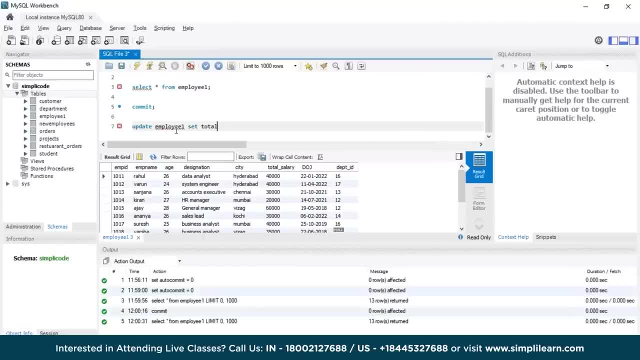 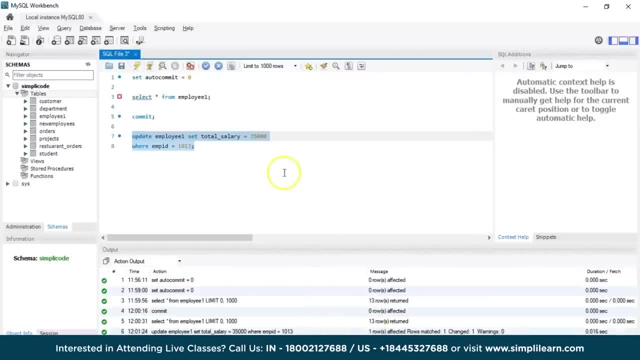 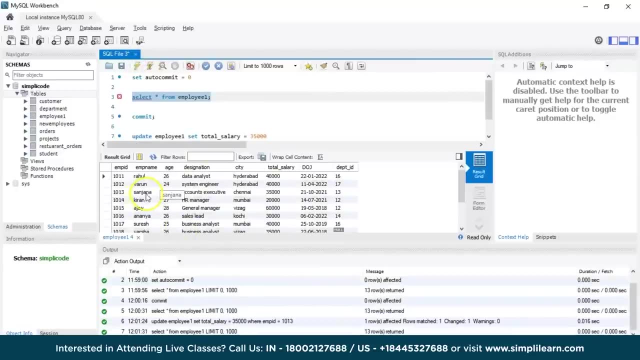 So, as you can see, One row has been affected And our query has been executed successfully. Let me just display the records again. So, as you can see, Employee Sanjana, whose employee id is 1013.. Her total salary has been changed to 35000.. 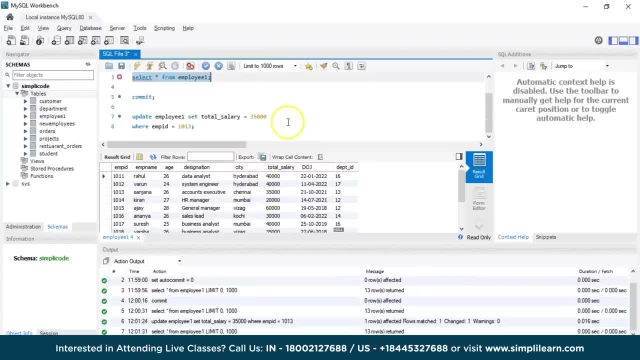 Her total salary has been changed to 35000.. Which was earlier 30000.. Now let's say, in future I have this requirement Where I want to have the original salary, Where I want to have the original salary Now, for that I can use the rollback here. 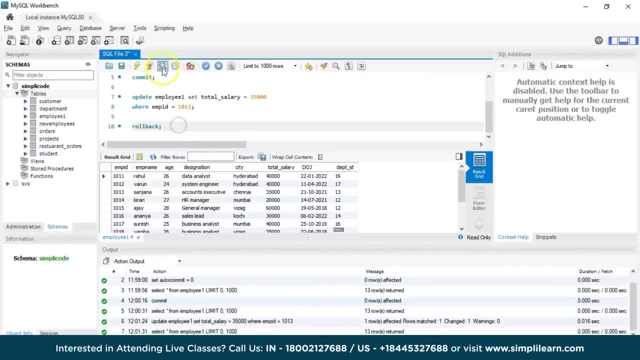 Now for that, I can use the rollback here. So when I execute the rollback, So when I execute the rollback Statement here And select this table again, And select this table again, The total salary has been changed to 30000 again. 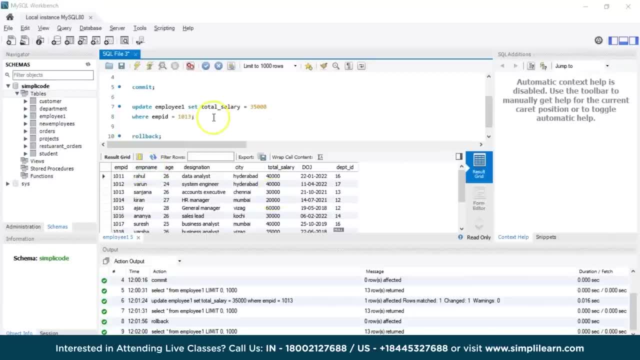 The total salary has been changed to 30000 again. So basically we have done a transaction. So basically we have done a transaction Where we have updated the total salary of the employee Sanjana to 35000.. Where we have updated the total salary of the employee Sanjana to 35000. 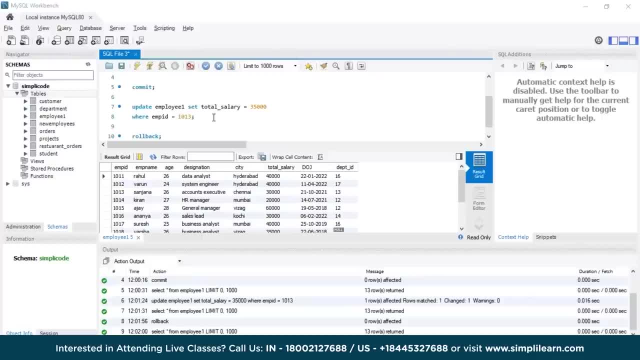 And after that we are again rolling back to its previous state, And after that we are again rolling back to its previous state, That is, again to 30000.. Now, similarly, you can perform another transaction. Now, similarly, you can perform another transaction, Let's say, using the delete operation. 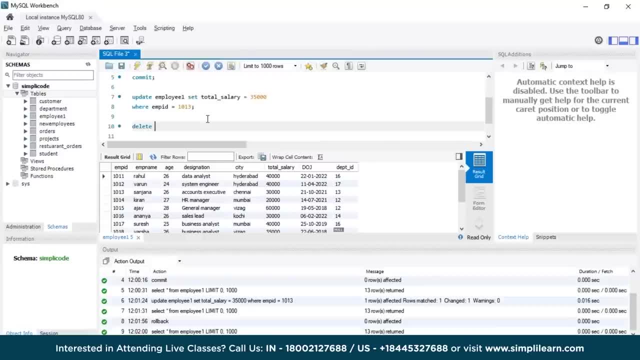 Now I want to delete all the records from this employee. one table. Now I want to delete all the records from this employee. one table. Whose designation is, let's say, business ID. Whose designation is, let's say, business ID. Now we have a total of business analyst 123.. 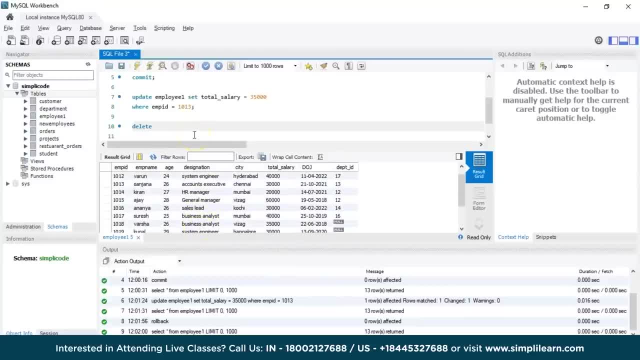 Now we have a total of business analyst 123.. We have total 3 records. So we will be deleting all these records from the table. So delete from employee one where designation equals to business analyst. So delete from employee one where designation equals to business analyst. 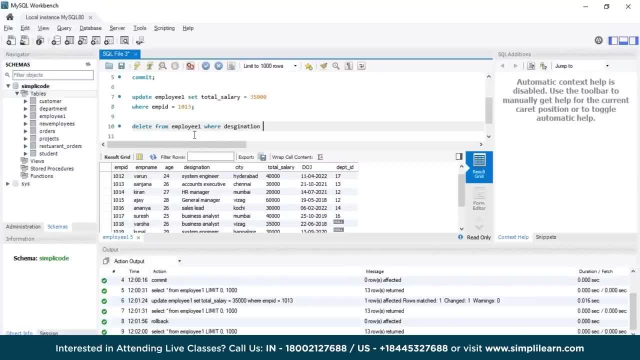 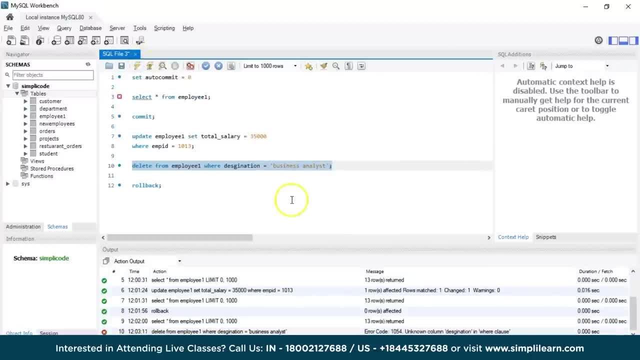 So let me just execute this statement. So let me just execute this statement: Okay, Okay, Sorry, the column name has been written wrong. Sorry, the column name has been written wrong, So that is why it is showing as error. So, as you can see, our query has been successfully executed and it shows 3 rows are affected. 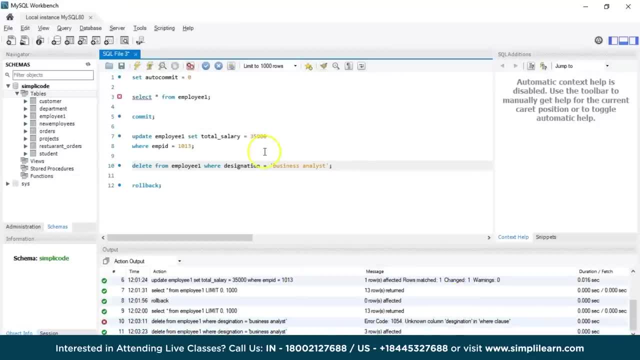 So, as you can see, our query has been successfully executed and it shows 3 rows are affected. So, as you can see, our query has been successfully executed and it shows 3 rows are affected. That means all the records of the employees whose designation is business analyst have been deleted. 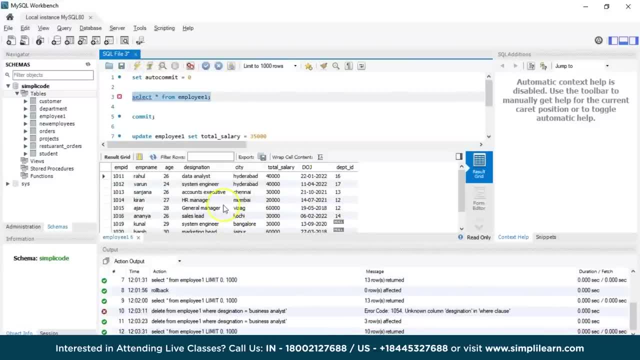 That means all the records of the employees whose designation is business analyst have been deleted. That means all the records of the employees whose designation is business analyst have been deleted. See, as you can clearly see, there are no records of business analyst records. See, as you can clearly see, there are no records of business analyst records. 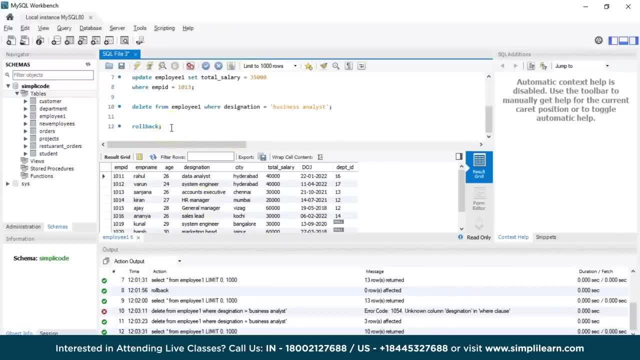 See, as you can clearly see, there are no records of business analyst records. So again, I have this requirement where I want to get back the results or the records of the employees who are working as business analysts from this employee one table. So for that I can simply use the rollback here. 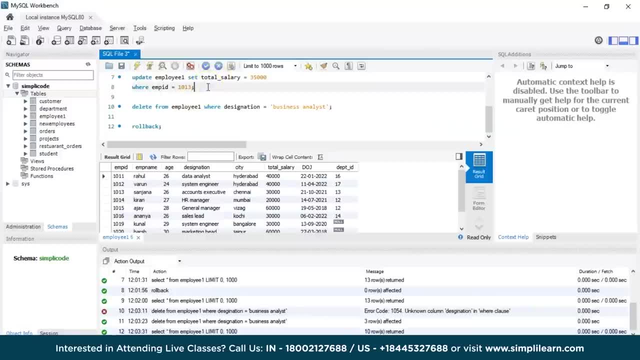 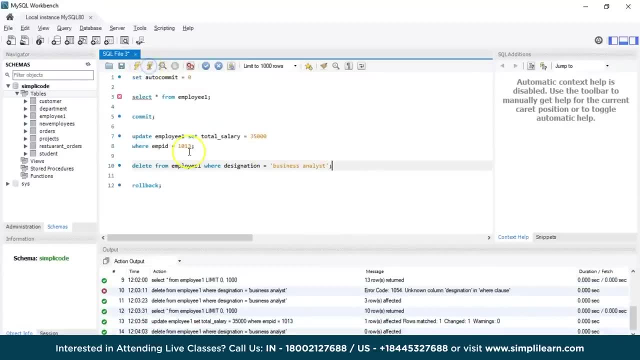 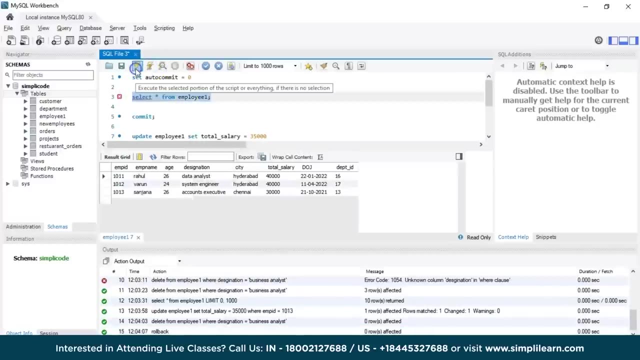 So we'll simultaneously perform to our transaction here. Firstly, we'll update this table again and then we'll delete, which was already done. So now let me just roll back the statement again. So when I roll back this statement and display the records from the table as you, 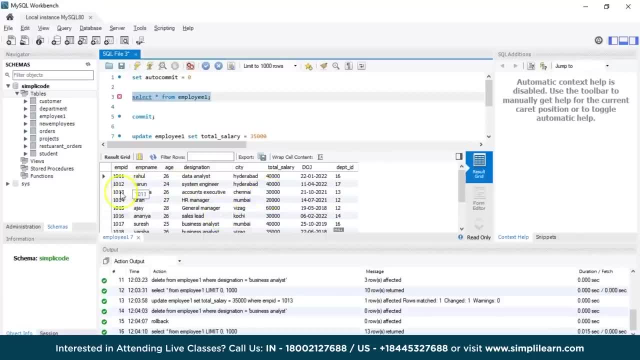 can clearly see the employee Sanjana, whose employee ID is 1,013. her salary, which we have set as 35,000, has been reverted back to 30,000, to its previous or original state, and similarly we have deleted the records of employees whose designation. 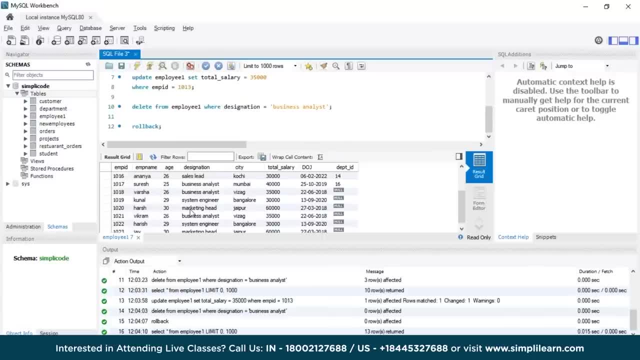 as business analysts, and similarly, their records also have been reverted back. So in this way, you can use the rollback command to get back to the current transaction and cancel. it changes Now. let us take another scenario here. Now, what if I perform a transaction before the commit command? 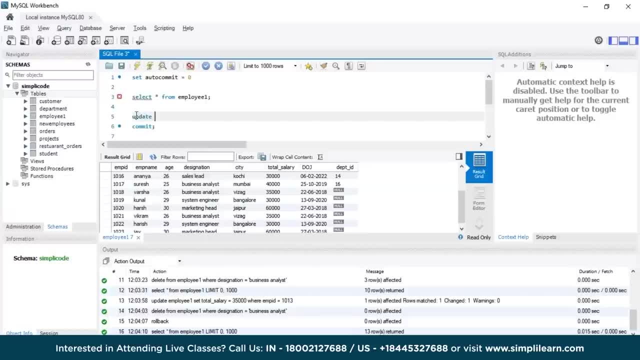 So for that I'll take another, another example where I'll update the age of an employee. Let's say, Rahul is employed, is 1,013 and his age is 26.. I want to change it to 27, so I'll use another update statement here. 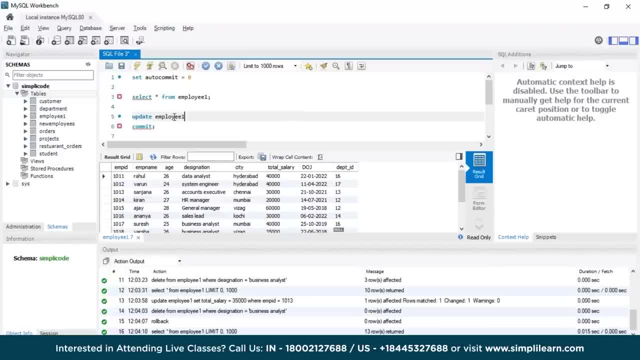 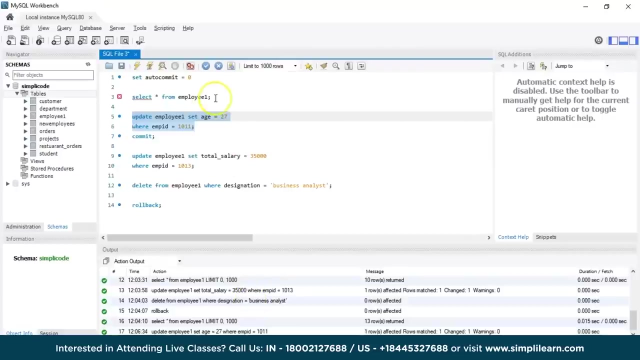 Update employee 1. table set age equals to 27, so his previous age was 26. now I'm changing it to 27, where employee ID is 1,011.. All right, so let me just execute the statement. So it is successfully executed and we'll select the records. 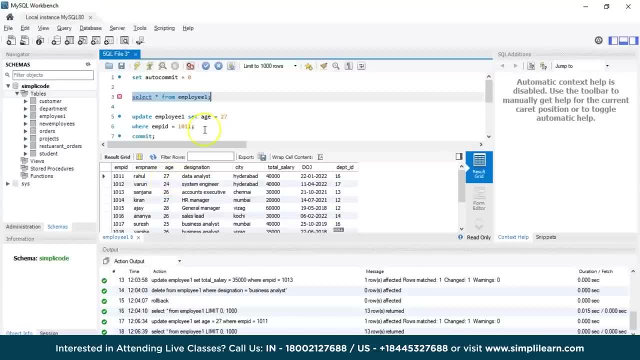 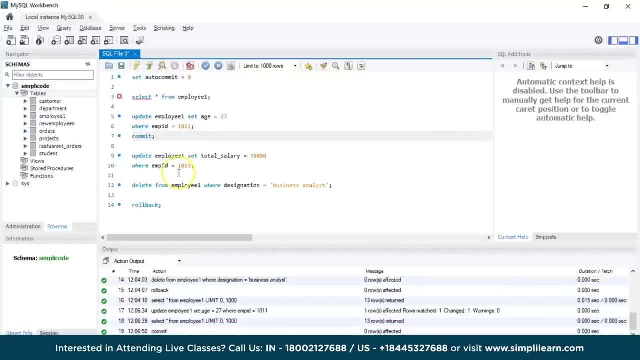 So, as you can see, Rahul's age has been changed to 27 from 26.. Now let's say: if I commit this transaction, All right, so I'll just commit this transaction. So, basically, you cannot make any further changes to this record, since we have 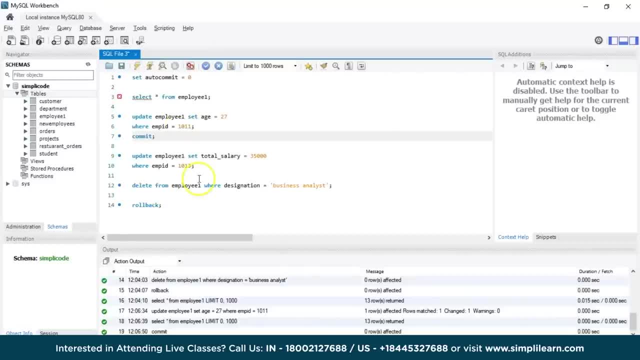 committed the transaction already, So I'll perform the two transactions again here, which is basically updating the employees total salary to 35,000 and deleting all the records of employees whose designation is business analyst. So let me just execute this So, as you can clearly see, all our SQL queries has been successfully executed. so let me just 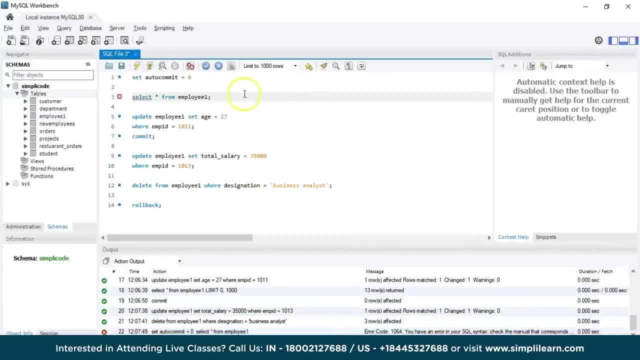 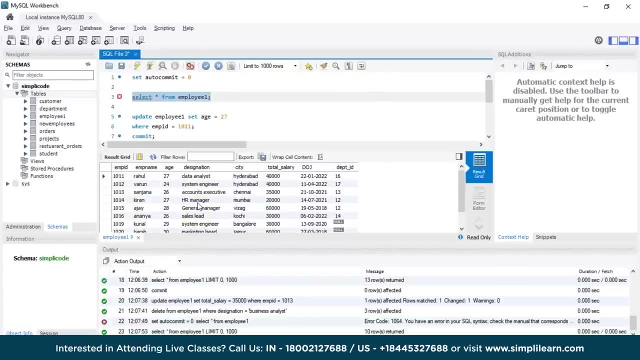 display the table here now. So, as you can clearly see that we employ Sanjana, who is having one employee ID as 1,013.. Her salary has been changed to 35,000 and we also have no records of those employees whose designation is business analyst and similarly the first. 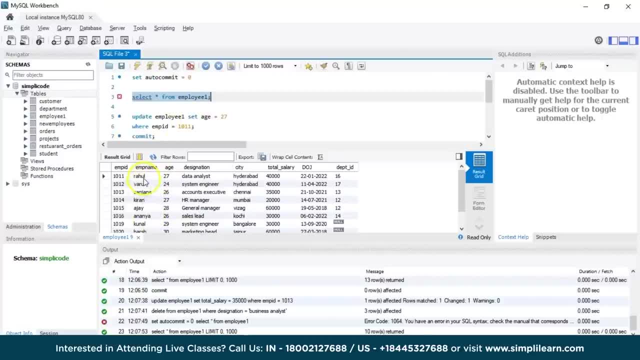 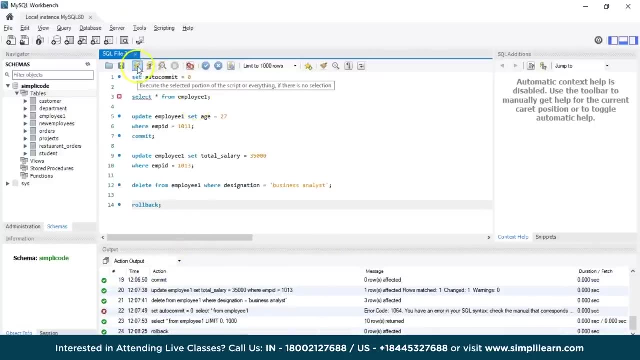 transaction which you have done, which is updating the salary of employee rahul, whose id is 1011 to 27. now let's say, if i want to roll back this trans, all these transactions, so let me just roll back here and we'll see what happens. so our rollback has been successfully executed and let me just 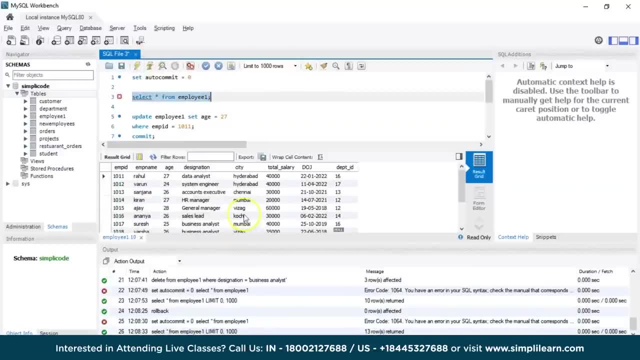 display the records again now. all the changes done past the last commit will be reverted if we roll back a transaction, since we have uh performed two operations or transactions after commit statement, which is basically updating uh the employee salary to 35 000 and delete the records. 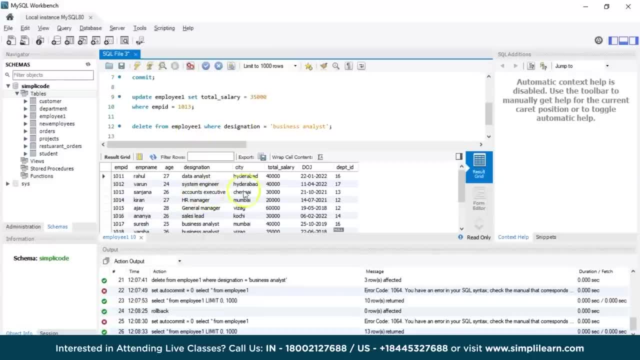 of employees whose designation is business analyst. now, clearly, we can see that their records have been reverted back to their original state. so so, like you can see that the records have been reverted back to their original state, so so, like we can, we have this employee named sanjana, whose salary was 30 000, which is we have changed to 35 000, and 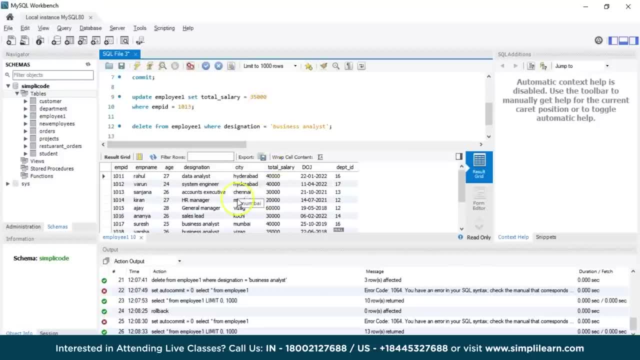 since we have rolled back again to its previous state. it is 30 000 and similarly we all. we have all the records of the business analyst as well. but if you look at here, we have changed the employees age here, like we have taken rahul's age as 27, which was earlier 26, and we have changed. 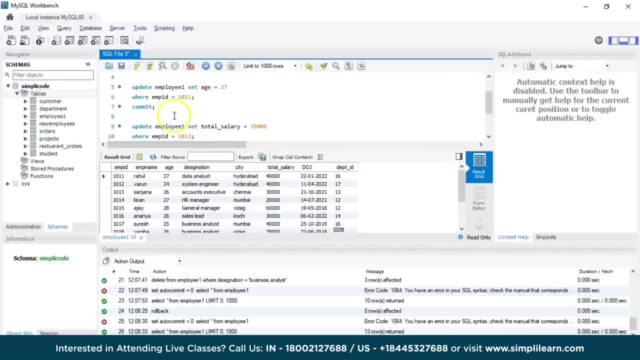 that to 27. but even after rolling back, we have changed the age of the employee. so we have changed that to 27, but even after rolling back this, we haven't uh got the original record that is his age as 26. that's because we have already committed this transaction, so it will basically uh not 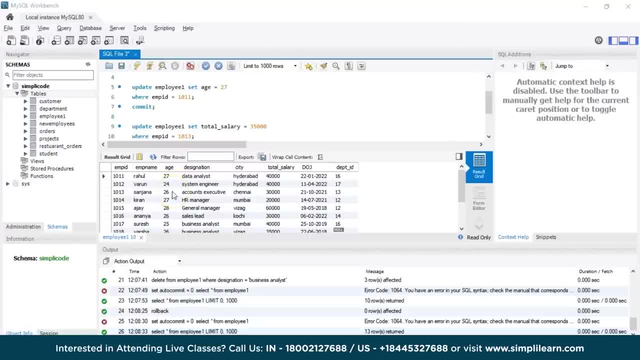 revert back to its previous state. so once the commit statement has executed the modification made by the transaction, it cannot be rolled back again. however, once the rollback statement is executed, the database reaches its previous state. so that brings us to the end of today's session. guys, now that was all about the commit and rollback commands in sql. so basically, to ensure 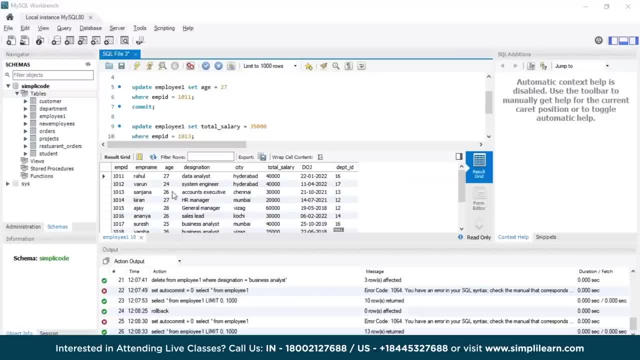 that the changes made by the transactions are permanently saved in the database. we use the commit after the transaction successful completion. in case the transaction faces any error while execution, then to undo or revert the changes done by the transaction, a rollback command is used. now you might uh get a doubt that where we have to use this and where this is applicable now, if you are. 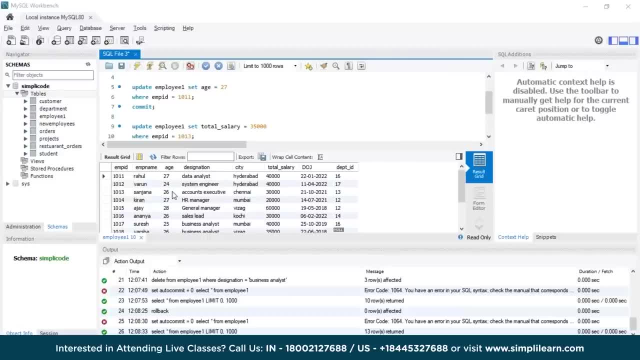 an sql developer or even a beginner who is working on a database. let's say you're working on a database which has thousands of records and you're modifying, let's say, 100 records in that. now, due to some errors, you want to revert back all the changes that you have made, right? 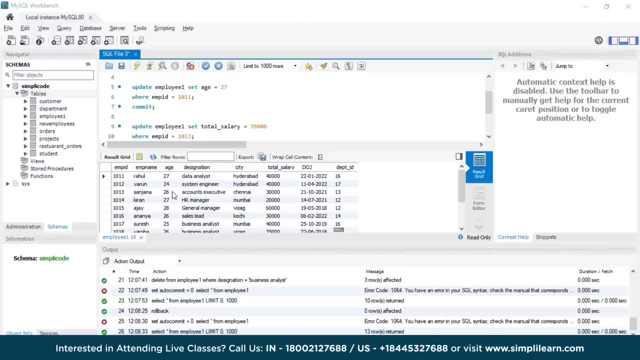 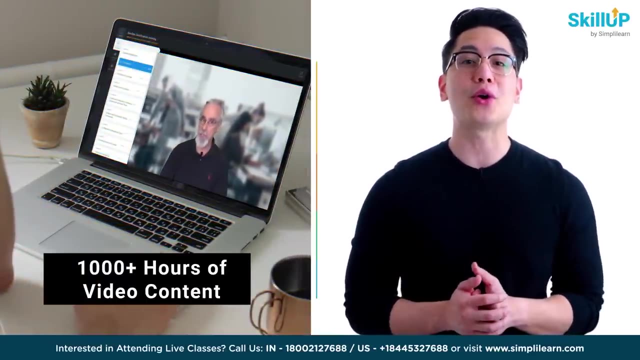 so for that you basically use the rollback function for that. so in this way it will be helpful for getting the records again back to its original state. choose from over 300 records and revert back all the changes that you have made so that you can revert back all the. 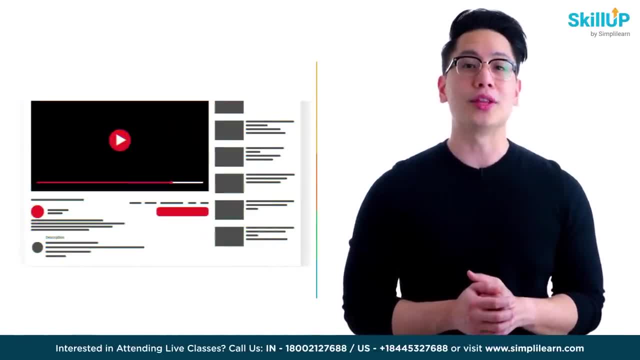 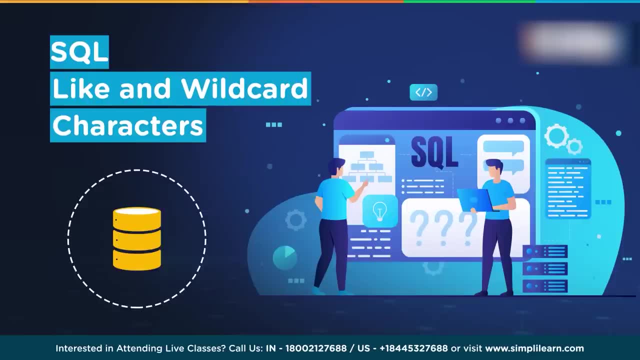 changes that you have made, so in this way, you can revert back all the changes that you have made. sql developers who frequently work with large data sets and analyze enormous amounts of data, find that they often need to query specific types. now, sql provides us with many such tools to 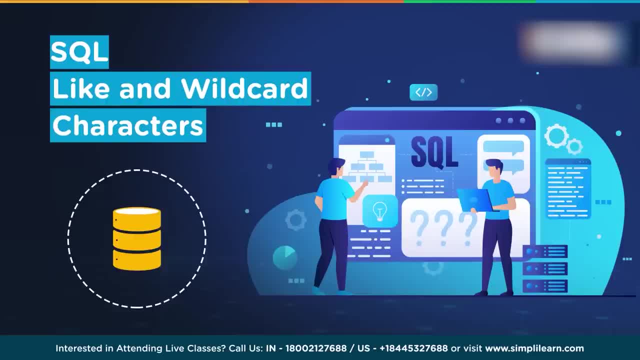 accomplish this, and one such operator is sql, like, which helps us to look at specific data types instead of the entire database. this reduces the time it takes to query specific types of data, so it makes it easier for sql developers to work efficiently in the database. so in this tutorial, 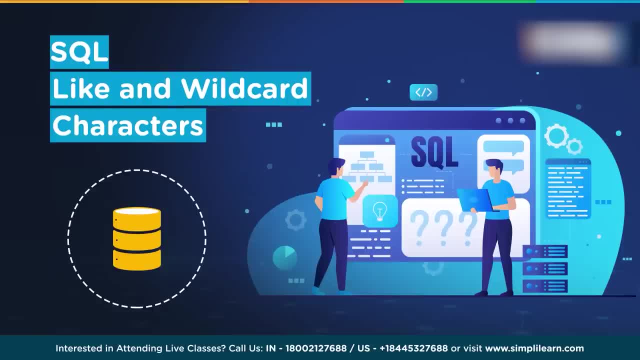 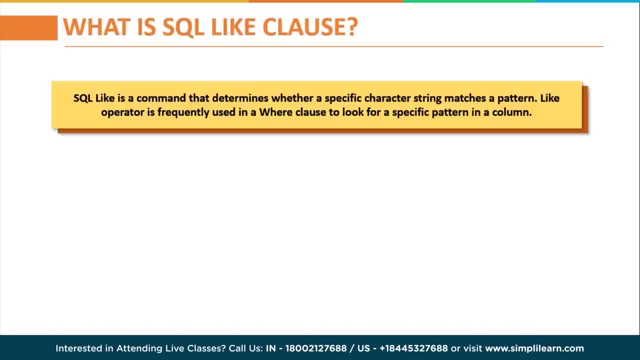 on sql like operator. we'll be learning how to query data to find specific patterns using the like operator in sql. firstly, let us understand what is sql like clause? the like operator is used to find specific characters in a tables column. it is also used to compare columns with the specified. 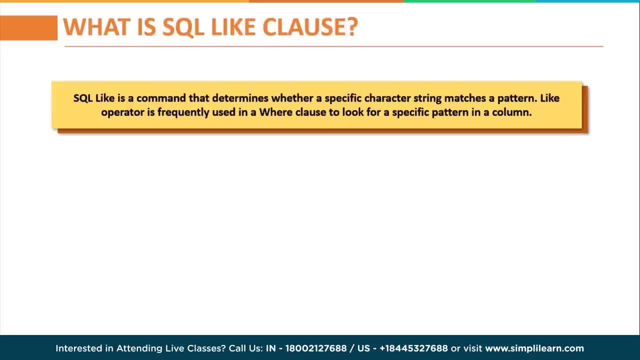 values. together with the where clause, it determines if a pattern matches specific values in a table, and if it matches specific values in the table, it is used to compare values table. It uses wildcard characters, which are characters used to replace one or more characters in a string. to fulfill this purpose, We can also use like when only a portion of the value in that. 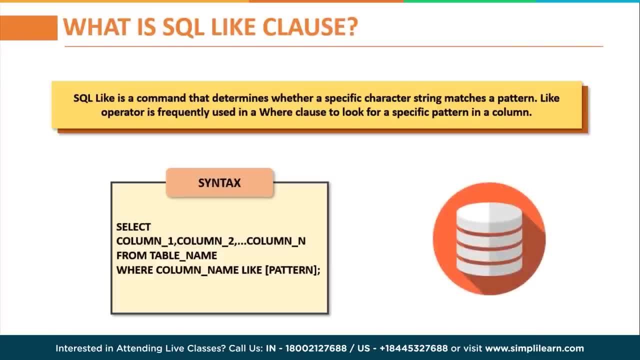 table is known. Let us now understand the syntax. The syntax is simple. It is usually used with the select command and the syntax of this is followed as select: column 1,, column 2, so on up to column n from table name, where column name like and pattern. Now basically the columns to be shown in. 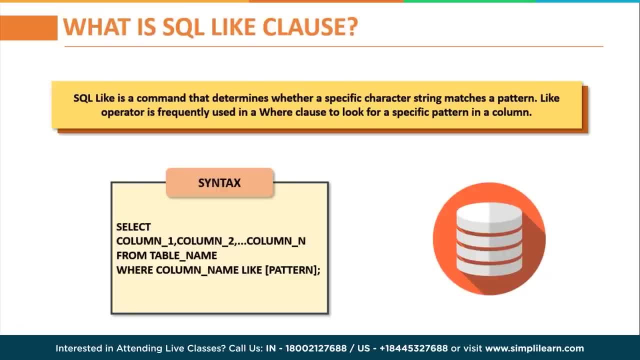 the result table are specified after the select statement. The column that is designed for pattern matching is specified in the where clause and the pattern forms from the specific row selection, which is defined in the pattern parameter of the like operator. Now the like operator is case. 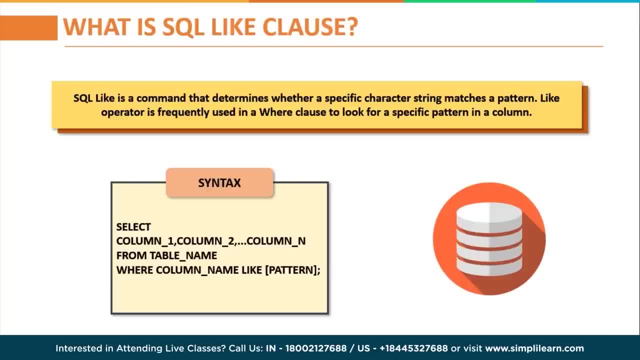 insensitive. that means you can either give capital or small letters as well. Now, multiple patterns can be used to define the like operator. Now the like operator is case insensitive. that means you specify with this operator using the and or or keywords as well, And wildcard characters are the. 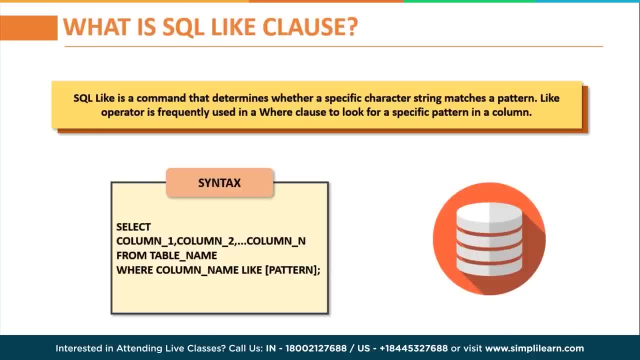 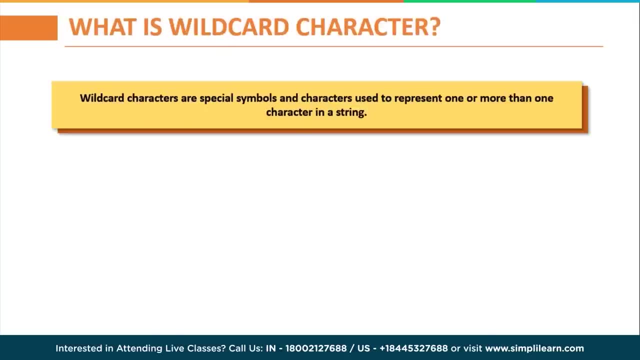 most vital tools of this operator. So let us go over what these are and how they are used with the like operator. So what is wildcard character? Now, wildcard characters are special symbols and characters used to represent one or more than one character in a string. These are imperative to 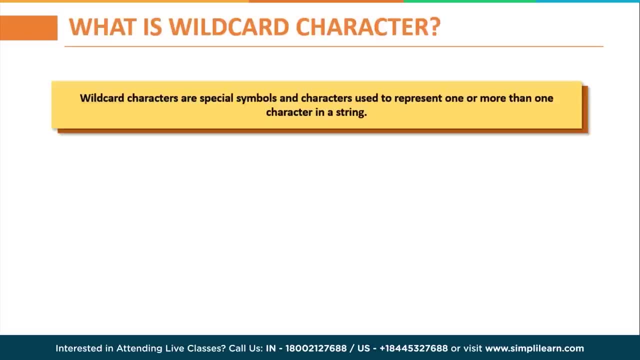 the like operator, as these enable patterns to be specified, That is, it filters the data using certain patterns to identify a value of a string in the database. Now the two wildcards used with the like operator are generally percent and the underscore. Now the percent sign is used to. 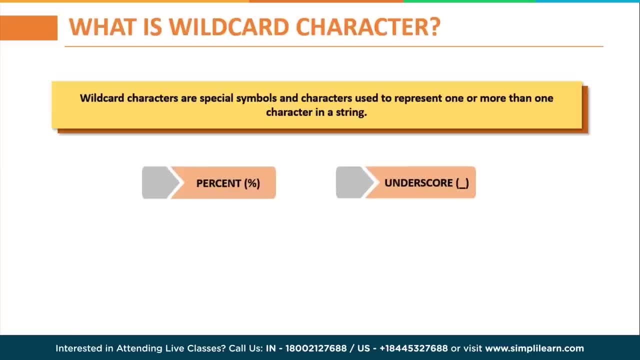 represent zero or one or more characters, whereas the underscore is used to represent exactly one character. Now, to get a clear picture of both these characters, let us look at an example in our SQL statement and see how they are used. Now consider this following example, which is: select employee ID, employee name from employees. 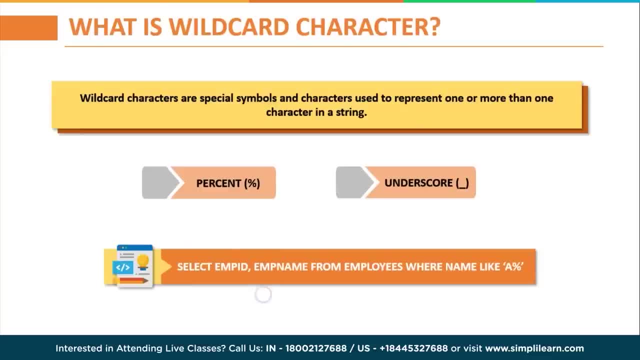 where name like a percent Now from this table employee. if you want to know the employee ID of all the employees whose name start with a letter or character a, you should use this following query: which is the character or the pattern we are using? here is a percentage Now, as we discussed earlier. 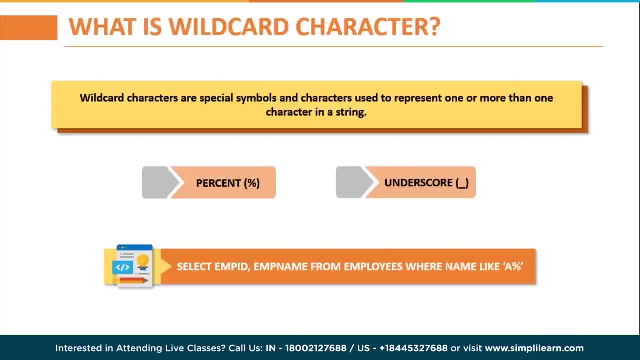 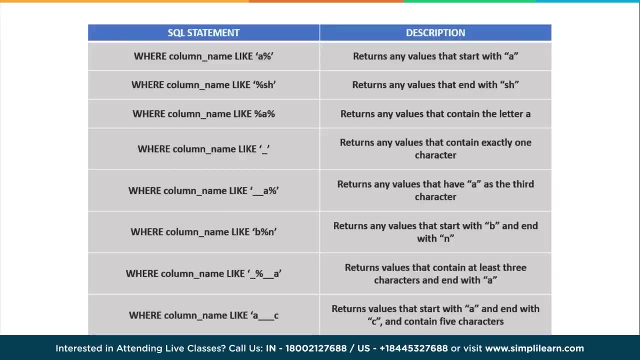 you can also use a small letter a instead of capital a. So let us look at the example in our SQL statement where we are using the letter a because the like operator is not case sensitive. Now there are many operations that can you that you can perform using 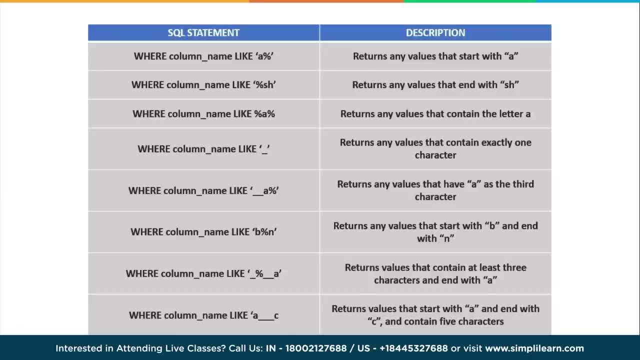 by specifying different patterns using the like operators. Now, for example, if you have to find a value that starts with a, then the following query would be: where column name like a pattern? So basically, we are mentioning the pattern here as a percentage which will retrieve all those. 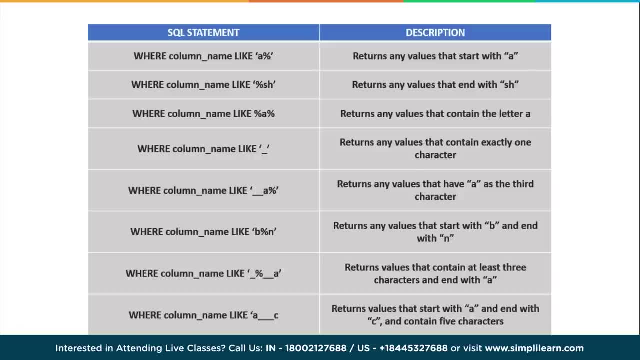 string values which starts with the character a. Now, similarly, if you want to find values that end with, let us say, sh, then you have to use percentage sh. Now, similarly, if you want to find values that can have a character a in any position, then you: 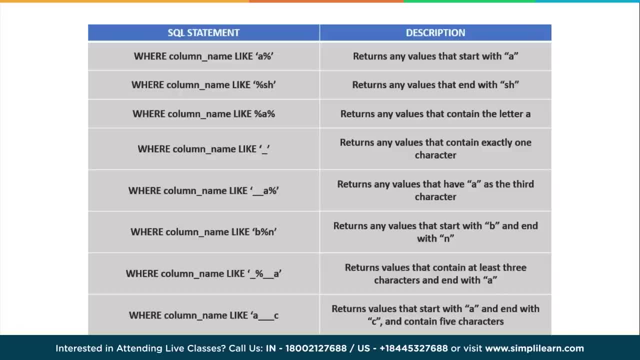 have to mention the pattern, as where column name like percentage, a percentage which basically returns any values that contain the letter a in any position, And similarly you can use the underscore operator as well. Let us say: if you want to return only exact, return exactly one. 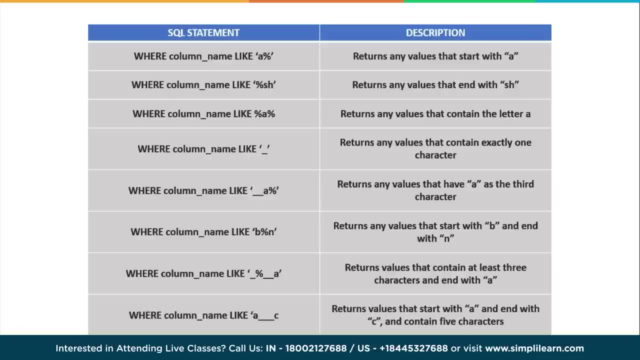 character, then you have to mention a single underscore sign. Now let us say, if you want to find values that have a character a in third position, then the following query would be: where column name like and within the single quotes, you have to mention three underscores, that is three. 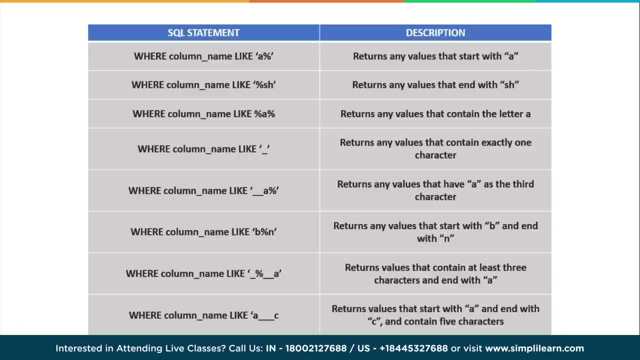 times you have to specify the underscore that would be present before the character a, and then you have to mention the percentage, And, similarly, you have these different types of operations, which you can take a screenshot of this by pausing this video now. So, now that we have understood how exactly SQLite works, let us jump into MySQL Workbench to 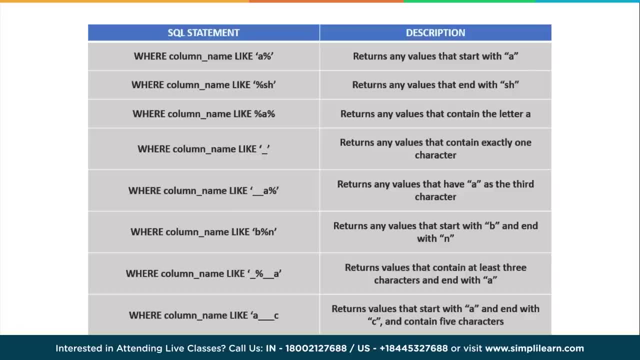 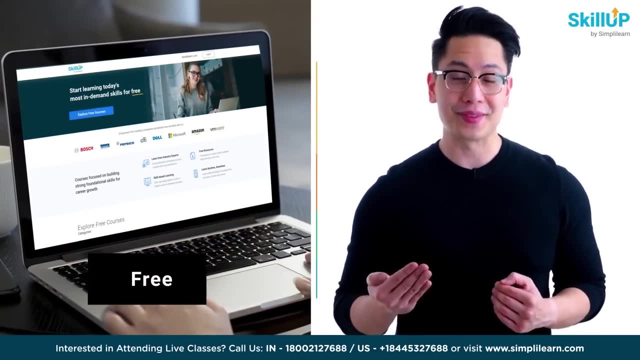 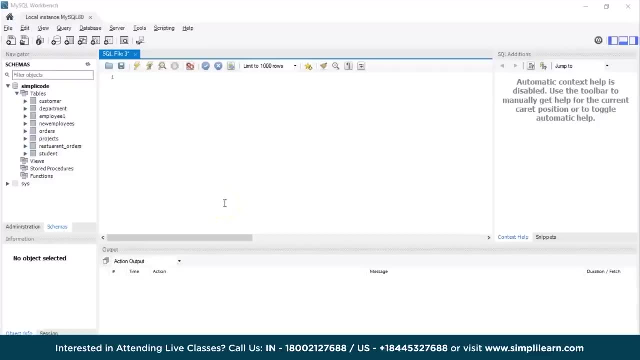 understand in depth on how these exactly work by using their different examples. If getting your learning started is half the battle, what if you could do that for free? Visit SkillUp by SimplyLearn. Click on the link in the description below. As you can see, MySQL Workbench just started and in order to execute the SQLite operator, let us 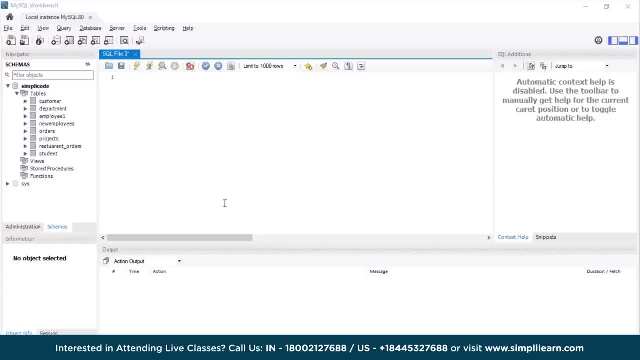 consider a following table in our database, let's say new employees, on which will apply various operations using the like operator. So let me first display the records that are present in the new employees table, and for that I'm using the select operator and the query select star from. 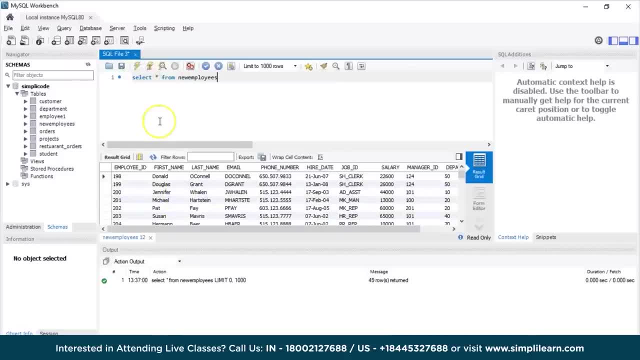 new employees. So let me just execute this. and the new employees table has various columns such as employee id, first name, last name, email phone number, hiring date, job id, salary, manager id and department. So firstly, let us discuss some examples using the percent wildcard. 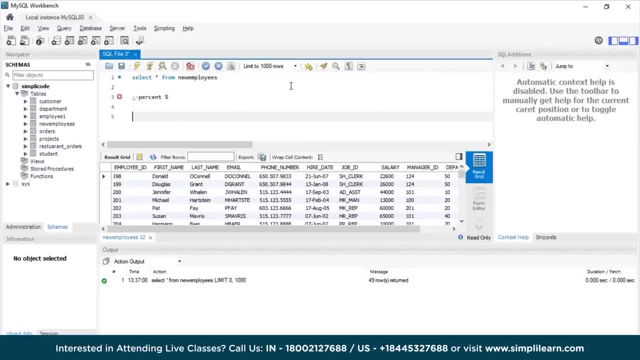 which basically uses the percentage sign. So let's say, if I want to fetch the details of all those employees whose first name starts with a or, let's say, s, then the following query would be: SELECT star from the table name, that is, new employees, employees. where is the conditional clause? 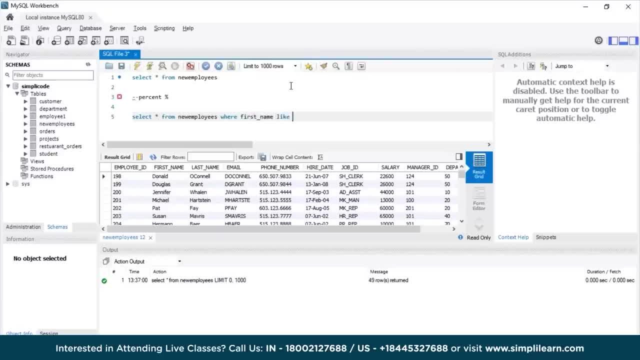 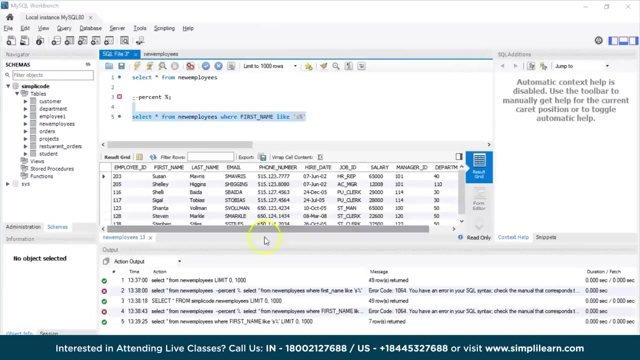 first name, like is the keyword and, within the single quotes, mention s percentage. now it is important to enclose all the patterns that you have specified in a single inverted comma, otherwise the query will return a syntax error. so let me just display this and execute this. so when you execute this query, it has returned me seven rows. 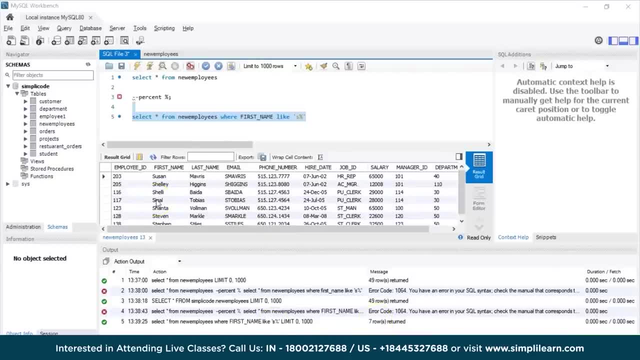 as you can see in the output, which basically returns all those employees name whose first name starts with the character, that is s. so we have, like different employees like susan maverice, shelley higgins, shelley baida, sigal tobias and etc. now, similarly, let's say: if we want to, 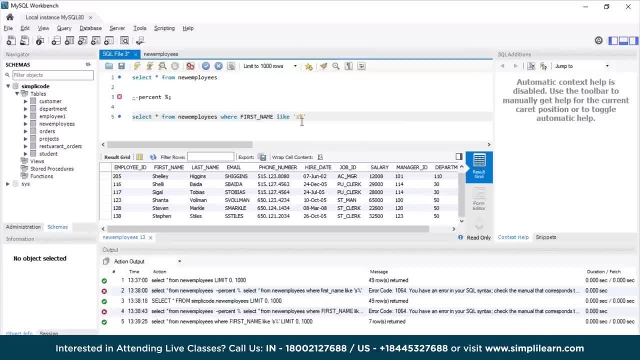 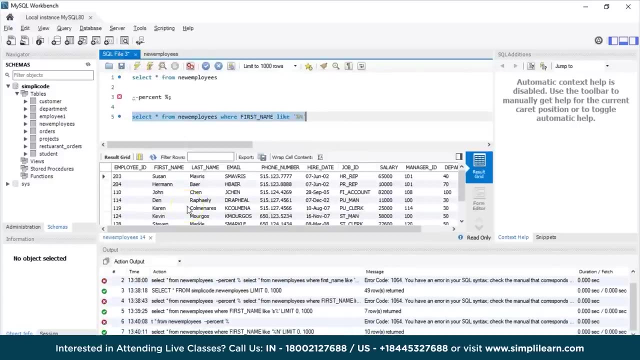 fix the details of all those employees whose uh, last name, or like first name, ends with uh. let us take a character, let's say n, so let me just display and execute the query. so when you execute this query, it basically returns all those employees uh details whose first name ends with n, like, for example, if you consider here: 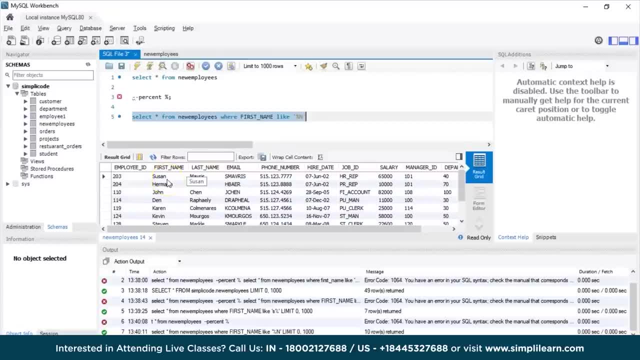 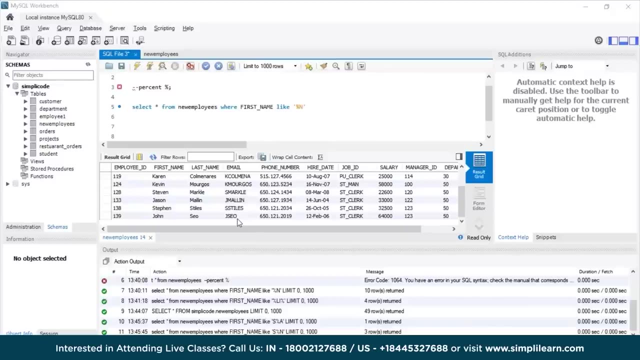 susan maveris, whose first name has uh n, in the last position. and similarly we have herman bayer, john chen, den raffley and etc. next, let us take another example. let's say, if i want to select all the employees whose first name starts with uh, let's say s and ends with 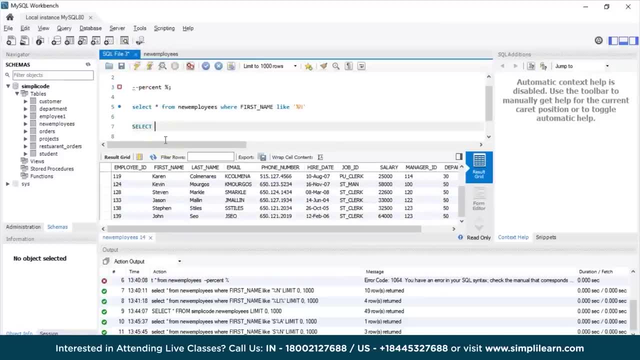 let's say n. so then the following query would be: select star from new employee, where first name, like now, the first character would be s and you have to mention the percentage symbol and the next last character would be n. so let me just display, execute this statement. 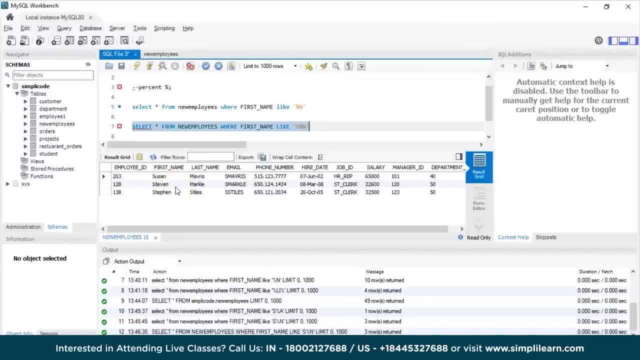 so, as you can see, we have a records of three employees whose first name have the letter or the character s in the first place and the character n in the second place. so let's say in the last place, for example, suzanne maverice. in the first name, we have s in the first place and 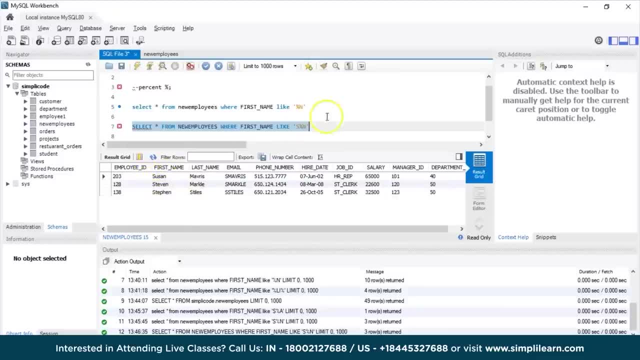 n in the last place. similarly, we have stephen markle and stephen styles. now let us take another example. let's say i want to find the details of the particular employee. now the thing is, i don't know the exact name of that employee, but i know that, uh, his salary is somewhere between 30 000. 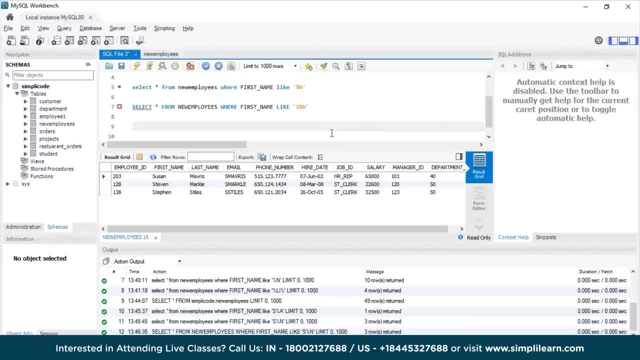 and 50 000, so for that i can use the and or operator here. so the following query would be: select star from new employee where first name like let's say i know the employee name starts with uh k. okay, then we'll mention the percentage symbol. 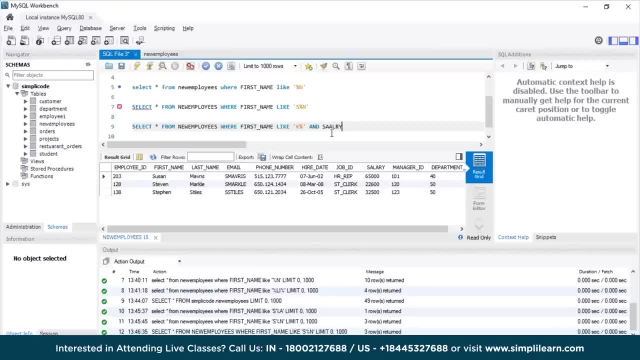 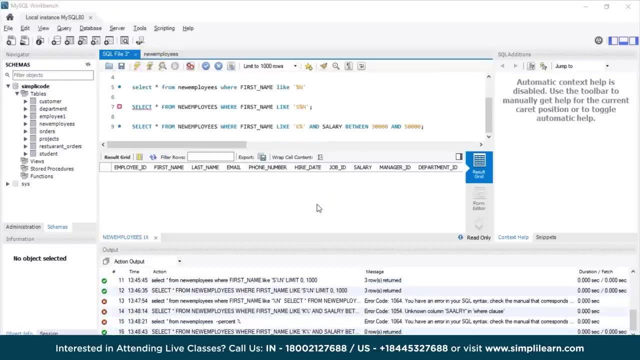 and we'll mention uh, the and operator here, and salary between thirty thousand and thirty thousand, 1900. so let us execute this statement and we'll see the output. so when we execute this, we can see that there are no records in the table. that means there is. 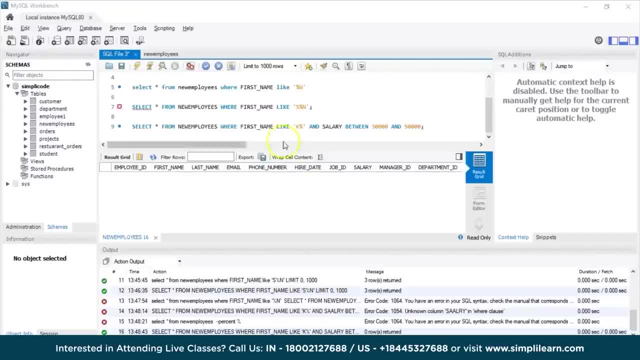 no employee whose name starts with k and the salary is between thirty thousand and fifty thousand. so let us take another example. let's say the employer's name starts with j, so, and his salary is somewhere between thirty thousand and fifteen thousand. so let me just execute this statement now. 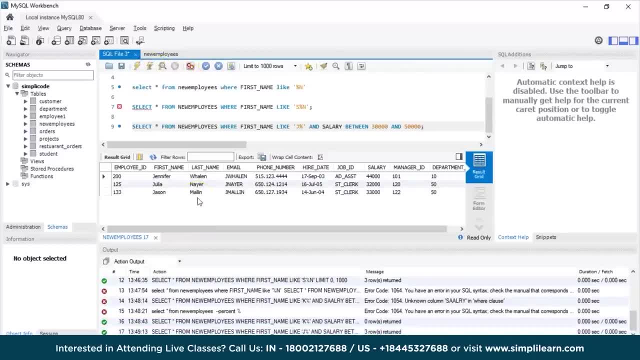 as you can see in a result set, we have three different employees: Jennifer Valen, Julia Nair and Jasson Malin, whose salary is between thirty thousand and fifty thousand respectively, like we have forty four thousand, thirty two thousand and thirty three thousand. so in this way you can find the details of employee. 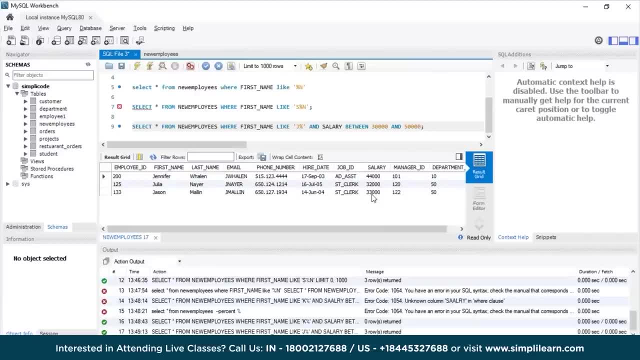 even if you do not know the complete details. but just by specifying the pattern of their name or the character that we have in their name, you can fetch their details now if you want to. if you further know their department ID, let's say Jennifer Valen, department ID is 10 and she belongs to that department and I 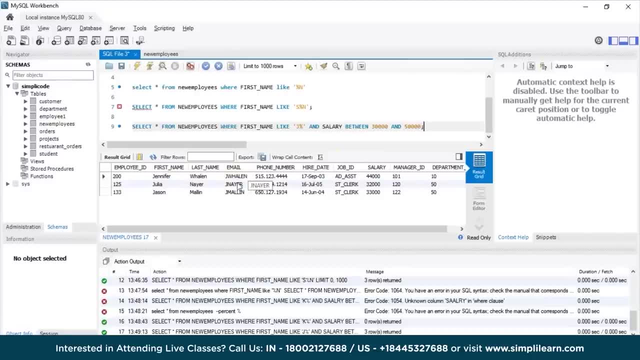 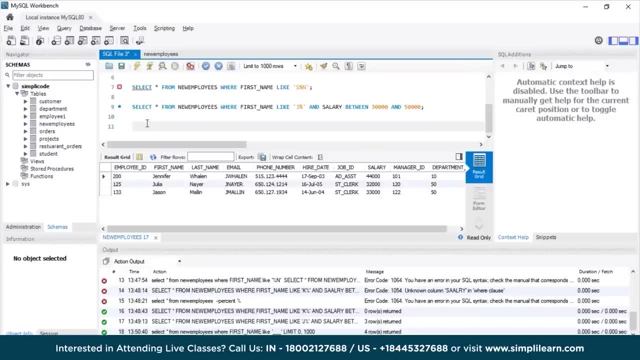 want to get the details of that employee. only then I can retrieve their details in this way. so I hope you've understood how to use the percentage sign to find the different patterns in order to find the complete string value from the table. let us now discuss some examples using the underscore. 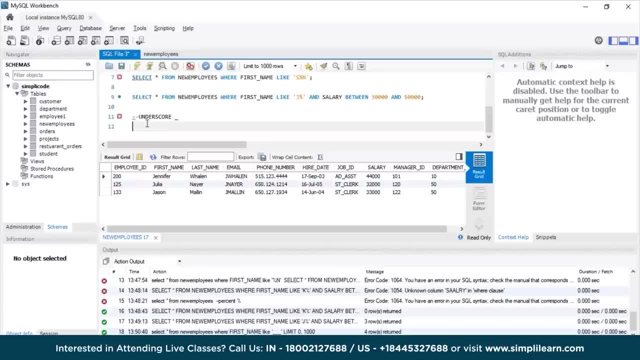 you while character using the under underscore symbol. so let me take an example here. let's say, if you want to fix the details of all those employees who have exactly three characters in their first name. so in that case the following query would be: select star from new employees where first name like 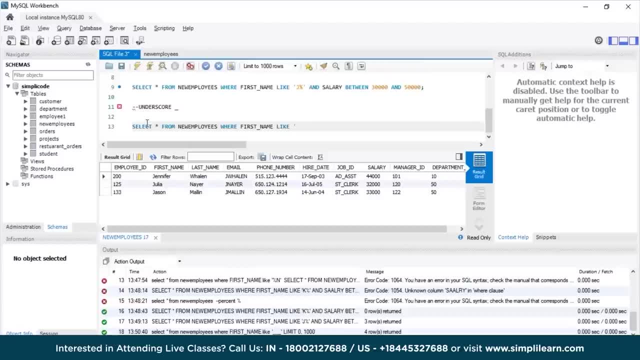 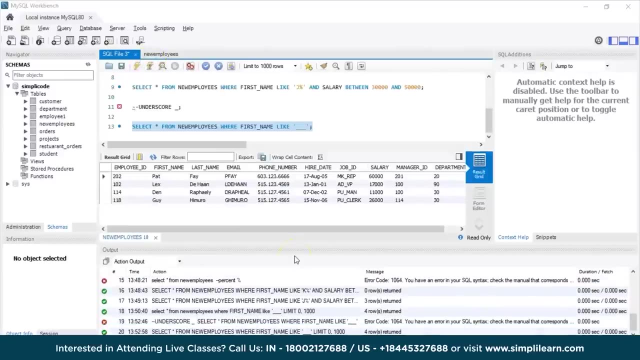 and within the codes. now we will discuss. there should be only three examples. exactly three characters in their name, right? so we'll mention the underscore three times: one, two, three, close the single brackets and let us execute this statement. so, as you can see, it has fetched a total of four records for. 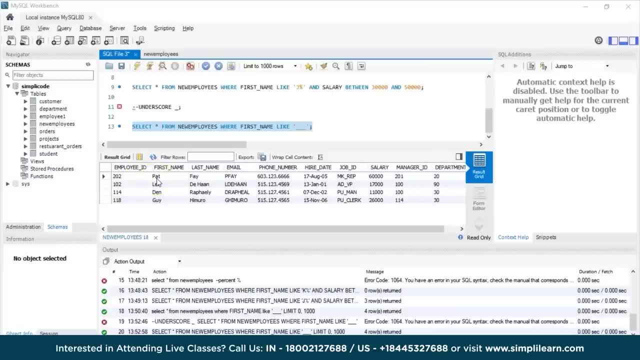 example, Pat Faye. we have only three characters. that is pat in his first name, and similarly we have Lex Dayhan Den Rapidly Guy Himro. all these employees have only exactly three characters in their first name. Let us take another example. 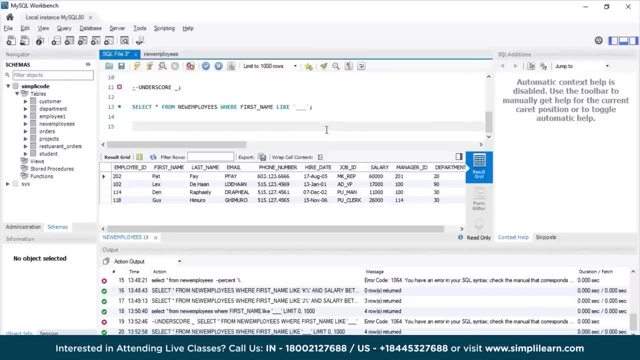 Let's say, if you want to select all the employees with the first name that starts with S and are at least five characters in length, Then in that case the following query would be: select star from new employees where first name, like single quotes, Now the first character would be S. So I'm mentioning S. 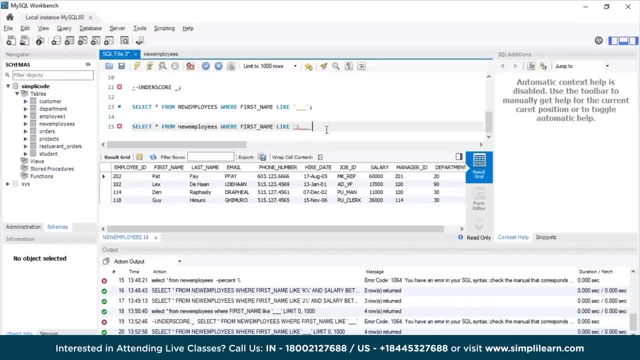 And after S we have to mention the underscore four times. That basically means it will return an exactly of at least five characters in our employees table. who's having the first name having five characters? So let me just execute this statement and we'll see the output. 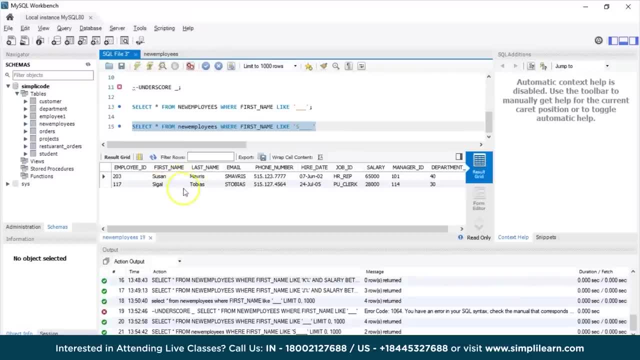 So, as you can see, we have two records of employees: Susan Maverice and Seagal Tobias. Now, if you look carefully, Susan, whose first name, has a total of five characters, That is S-U-S-A and that is five, And similarly we have Seagal. 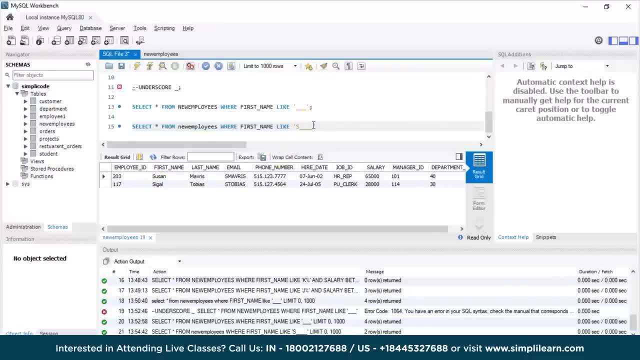 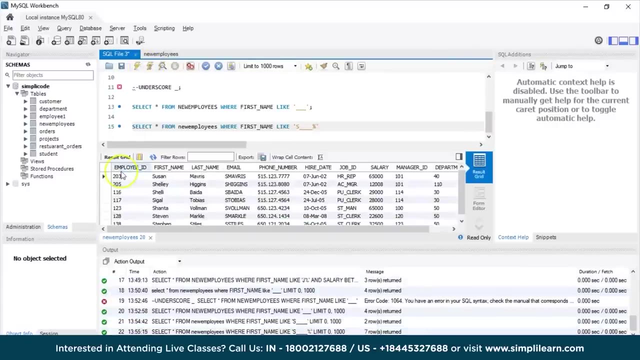 Now, if you want at least, let's say, five characters in length, then you have to mention the percentage sign. So it basically means the employee's name will start with S and it will have at least five characters in length. So let me just execute the statement. 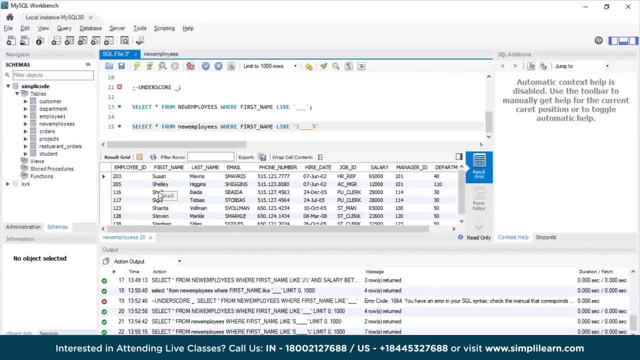 So it will display all those records whose first name is starts with the character S and have at least five characters in length. So it will display all those records whose first name is starts with the character S and have at least five characters in length. So they first name, for instance, Susan Maverice. 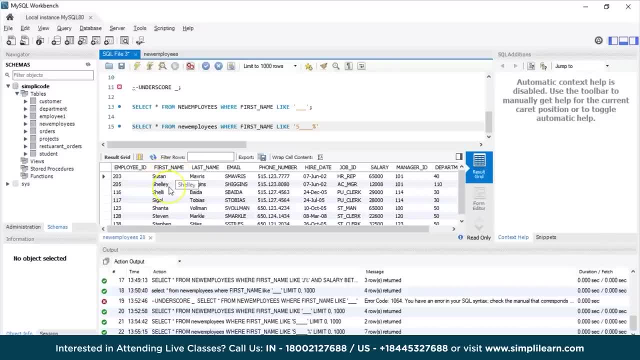 So we have Susan Maverice, like we have also Shelly, who's who's having a, let's say, 1234567 characters in total in there in her first name. So in this way we will retrieve all those values whose first names start with S and 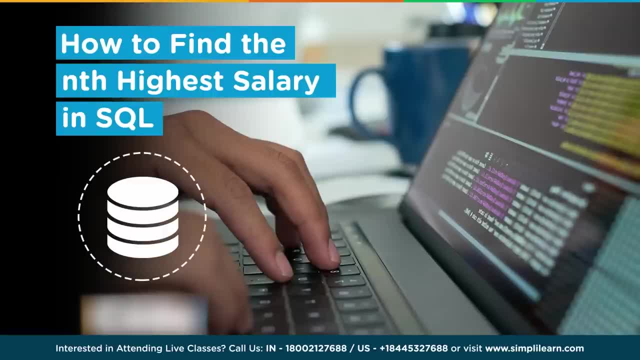 basically have at least five characters in length and description. we are going to discuss one of the most commonly asked SQL query during job interviews as well as campus placements, that is, how to find the end highest salvation SQL. So now we will look at the SQL query. 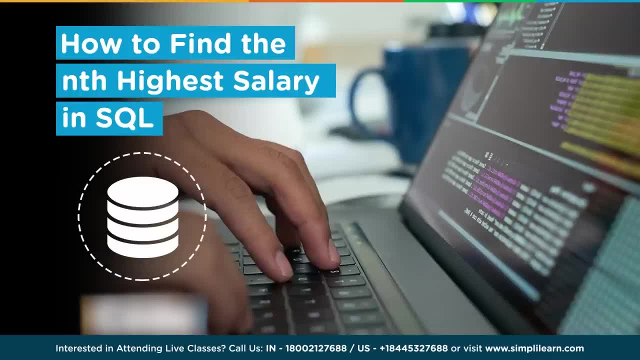 SQL. Now, there are many ways to find the answer to this query, but in today's session we are going to discuss the easiest and the most simplest way to find the nth highest salary in SQL. Let us jump into MySQL Workbench for execution and understand how to find the nth highest salary in SQL. 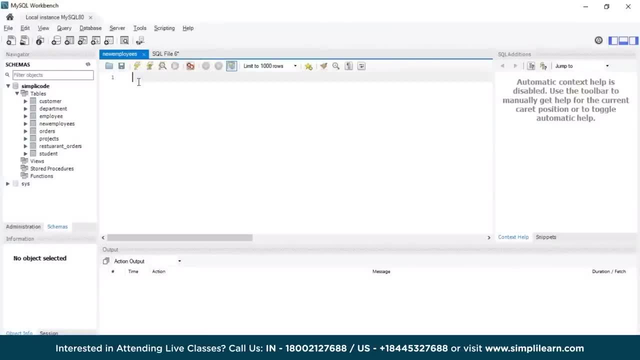 As you can see, MySQL Workbench has started. Now, in order to find the nth highest salary, we need an employee table, and for that I'm going to consider the new employees table here. So let me just display the records that are present in the table, and for that I'll use the select. 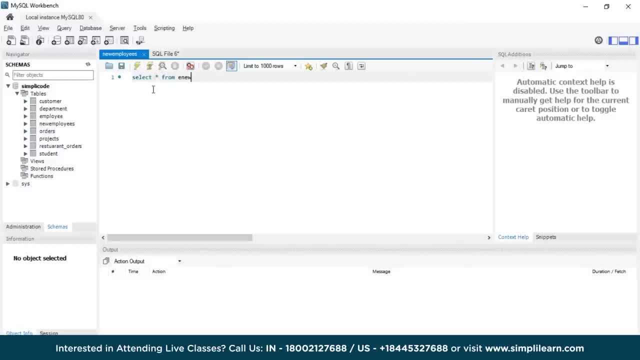 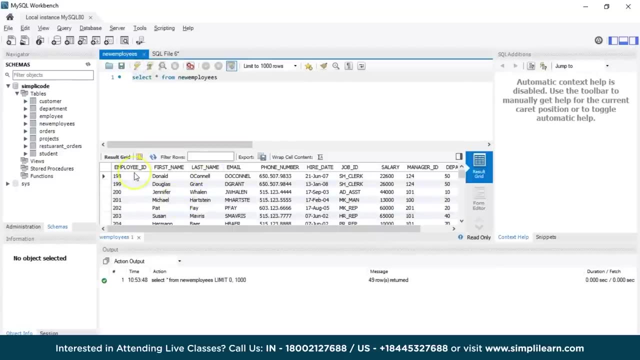 statement and the query is followed as select star from new employees. So let me just display the results. So, as you can see, the new employees table has various columns, such as employee ID: first name, last name, email, phone number, hiring date, salary, manager ID and department. 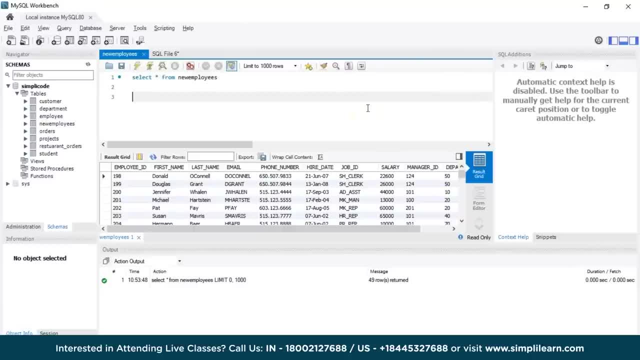 So firstly, before discussing how to find the nth highest salary, let us see how to find the nth highest salary in SQL. So let's first see how to find the nth highest salary in SQL. Now, to find the maximum salary in SQL, you can simply use the aggregate function max to find. 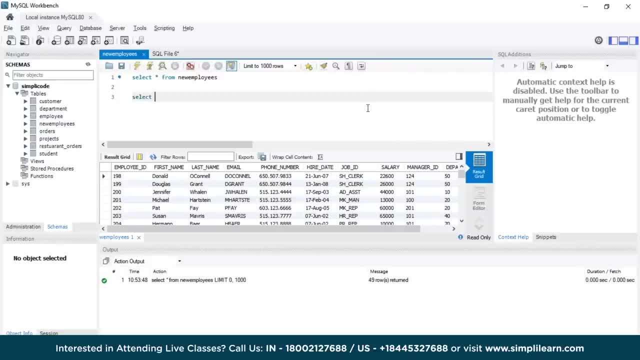 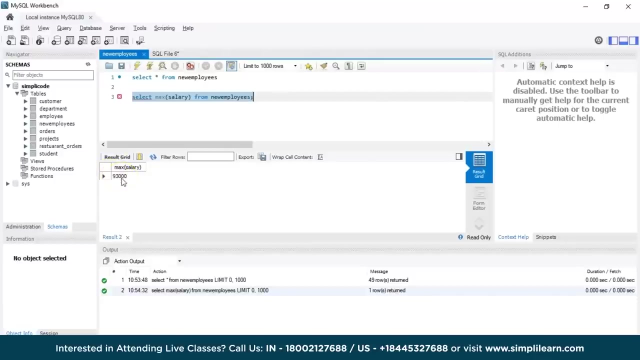 the highest salary in SQL. So the following query would be: select max salary from the table, that is new employees. So let me just display the results. So, as you can see, it is showing as 93,000, which is the highest salary in our table. Now next to find the second highest salary in the 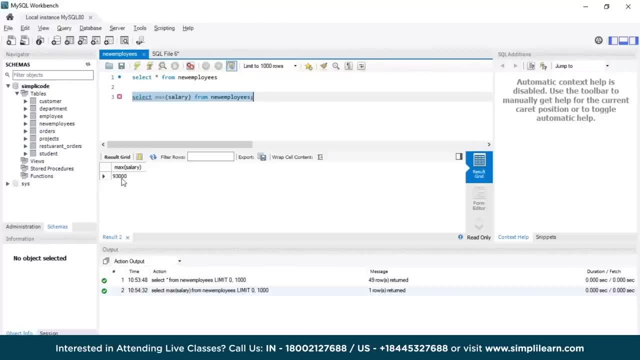 above table. we'll use the concept of subquery, which means that firstly we'll find the highest salary in the table and then we'll nest that query to a subquery to find the second highest salary in SQL. So the query would basically be as now. I'll put this as a subquery here. 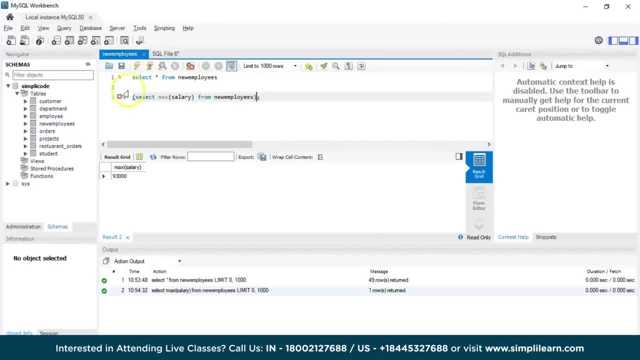 and I'll write the outermost query now, that is, select salary from the table, that is, new employees, where salary is less than this inner query or the subquery. So let us just execute this query and see the output. Now it will display all the salaries that 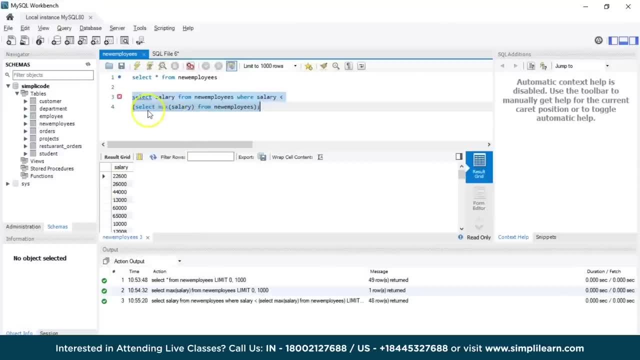 are greater, that is, less than the subquery that we have written here. that is the maximum salary, which is 93,000.. Now that is not the answer that we want or the result set we want. Now we want the maximum salary, which is less than the 93,000.. So I'm going to take the max function again here. 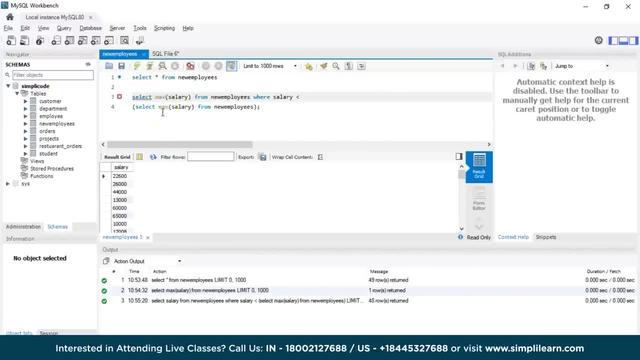 So basically, how this query works is the: firstly, the inner query gets executed, which is the maximum salary, that is, 93,000.. Next, the outer query executes, that is, it will select the maximum salary from the new employee table, which is less than the 93,000.. So let me just display the results. 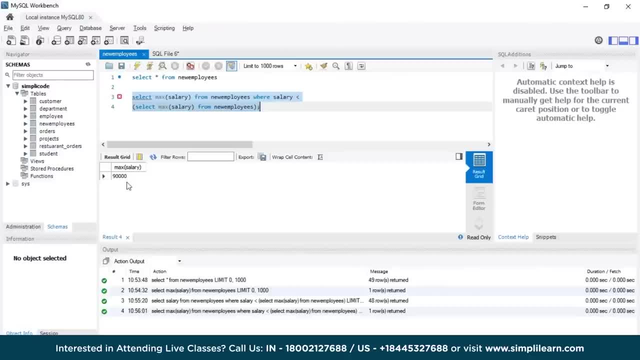 So, as you can see, it is showing as 90,000 and as the second highest salary. So let us just verify whether it is correct or not. I'll use the select statement again: select star from new employees. We'll use the order by order by function, order by salary, and I'll display the values in descending. 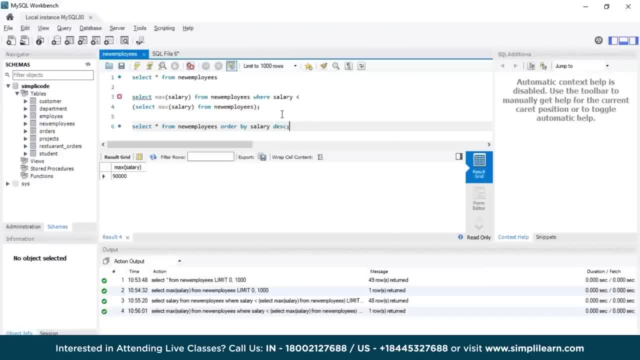 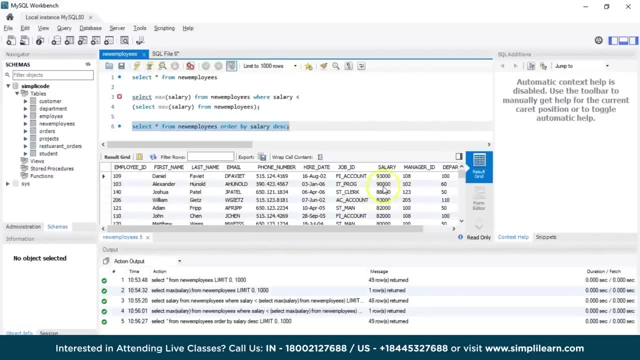 order. that means from highest to lowest. So in this way we can find the highest salary and the corresponding salaries that are less than the highest salary. So, as you can clearly see that we have 93,000 as our highest salary and the next salary as 90,000 as our next second highest salary. 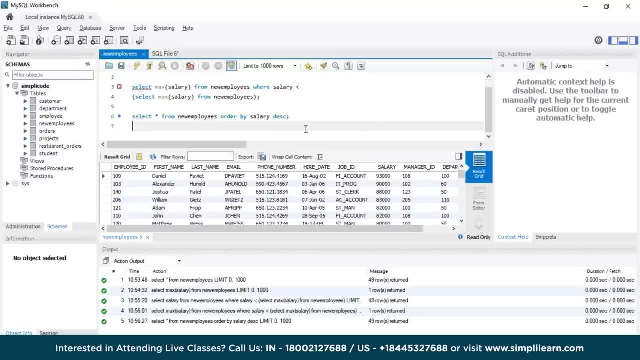 Now, till now, it is fine. Now, let's say, if you are asked to find the fifth highest salary, or let's say, 20th highest salary, or basically nth highest salary from this table, Now you can't keep on adding sub queries to this already. a return query right? It will become time consuming. 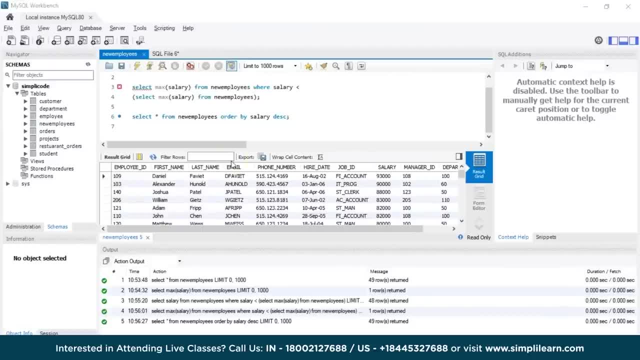 and it becomes complex as well. Now, in general, there are two ways to find the nth highest salary. The first one is using the limit clause and the second one is using the dense rank function, which is an inbuilt function provided by SQL, which we are going to discuss about in a while. So, firstly, 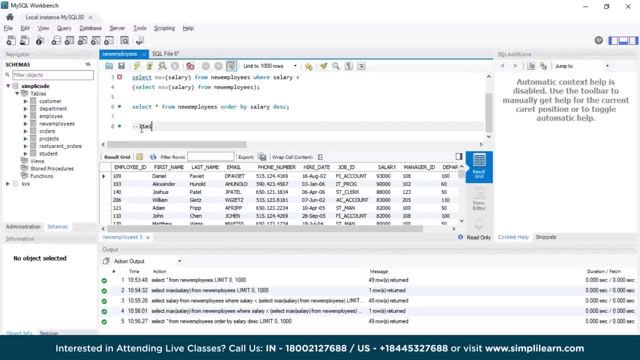 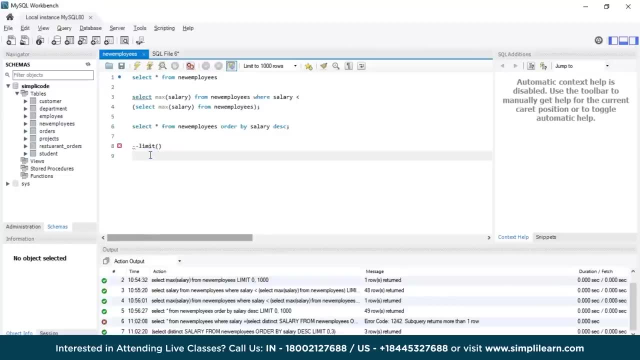 let us discuss about the limit clause and how we'll use the limit clause to find the nth highest salary here. So firstly let us understand the syntax here. Now the syntax is followed as select column list from table name, order by expression. Now in initialization, limit n minus one comma one. So let me just explain the syntax here. 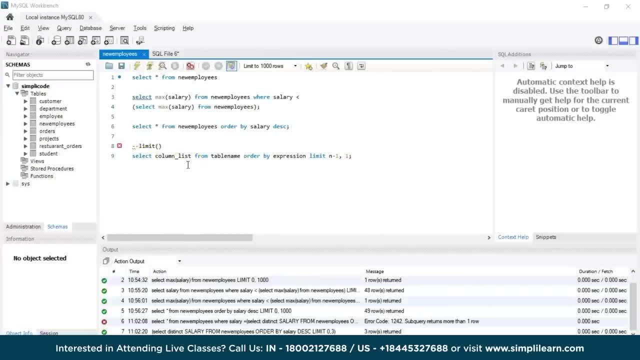 Now, after the select starts, you will have to mention all the columns that you want to fetch in your resulting table from the table name order by expression, which is basically the column name you have to specify here, And you are using the limit keyword, and after that we have two parameters here. 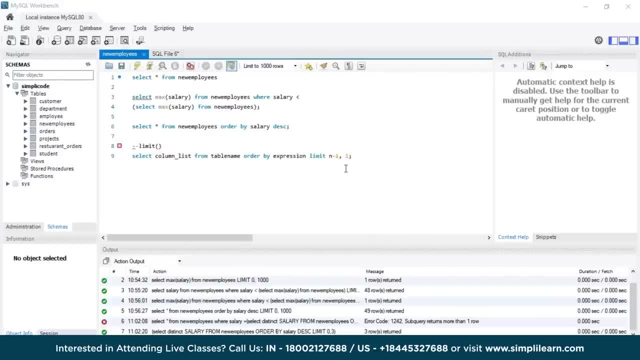 that is n minus one comma one. Now in the syntax, the limit n minus one comma one clause returns one row that starts after the row end. Now, in other words, if I have to define this, the first parameter, that is n minus 1, defines after how many rows it will start fetching the records in. 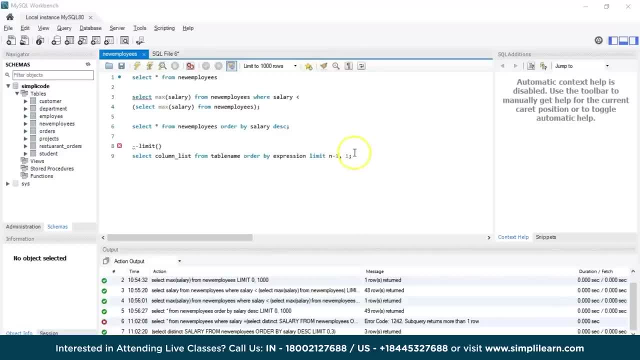 our resultant set And the second parameter will basically return the number of rows in that table. So let me just explain this with an example. So select. Now I'll use the distinct keyword here, which will basically remove all the anomalies or the repeated values in our table. So distinct salary from table name. 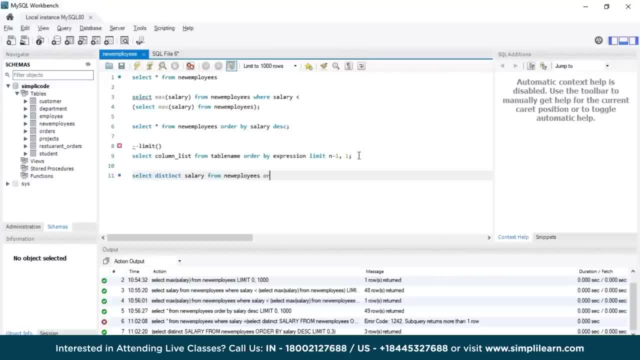 that is, new employees order by salary limit. Now let's say, if I want to find the 10th highest salary in our table, So now our n becomes 10.. So the value here it will be n minus 1.. So 10 minus 1 is basically 9 comma 1.. Now what this? 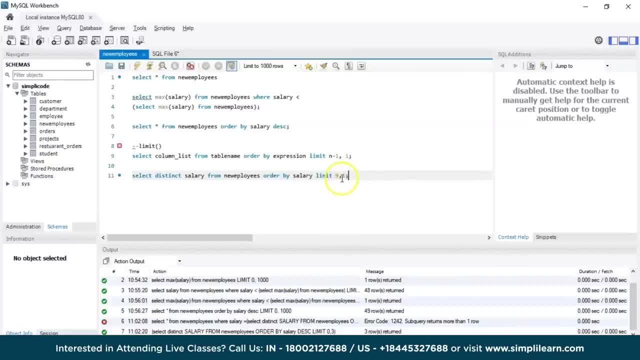 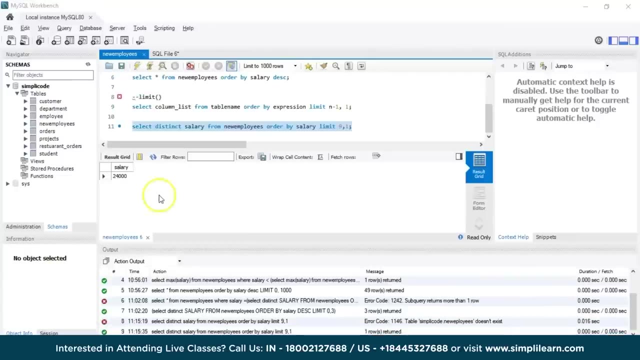 query basically does is it will return one record after the first nine rows. that is basically the 10th row, which is the query that we want, that is, to find the 10th highest salary. So let me just execute this statement. Okay, there is an error. So, yes, the query is: 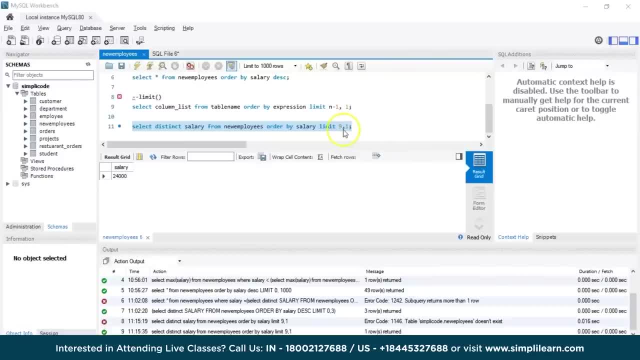 returning me as 24,000, which is the 10th highest salary here Now. similarly, if you want to find the, let's say, 24th highest salary, I'll just change the value into 24.. So sorry also. basically, if you wanted to find the 24th highest salary, you will have to mention: 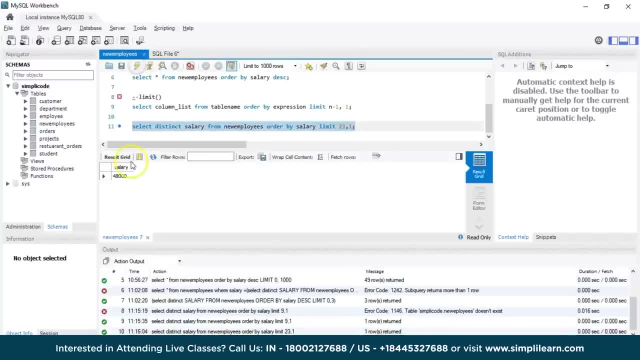 23 here. That is n minus 1, right? So let us find the output. So the next highest salary is 48,000.. So I forgot to mention the descending keyword here. That is why it is showing me the highest value. So if I run this query again, So the 24th highest salary here is 29,900. 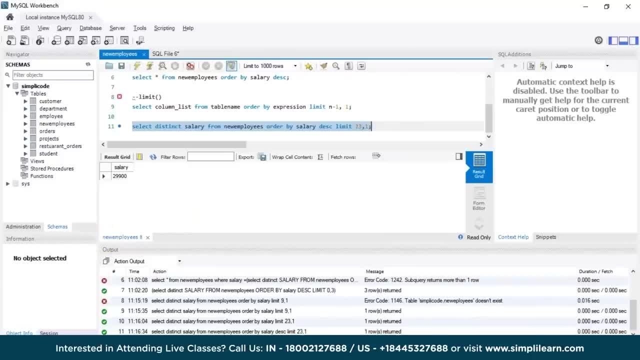 So in this way, you can basically use the limit clause to find the nth highest. Now, let's say, if I want to fetch the complete details of that employee who is having the 24th highest salary, I'll simply use a subquery here. So I'll put this query as a subquery and I'll write another outer query using the SELECT. 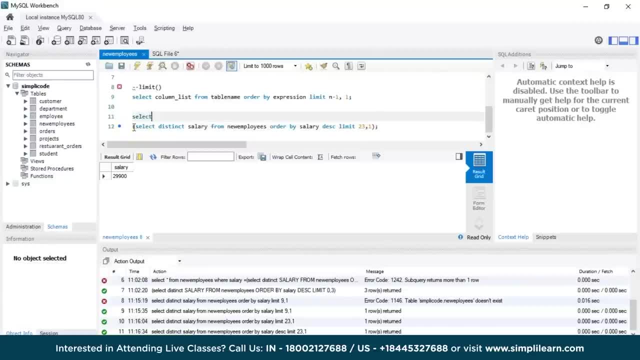 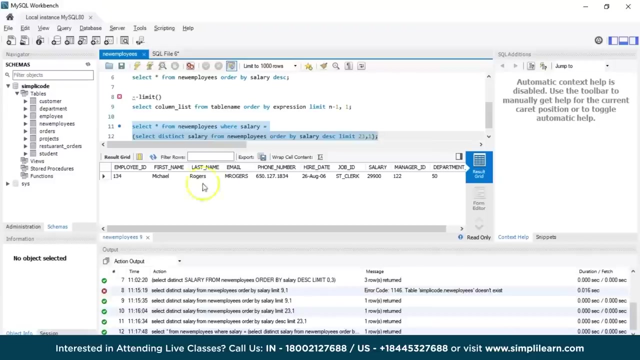 statement: SELECT star from new employees where salary is equals to the inner query. So let me just execute this query and we'll see the output. So now it will display the complete details of the employee: their employee ID, first name, last name, email phone number, their salary manager ID department. 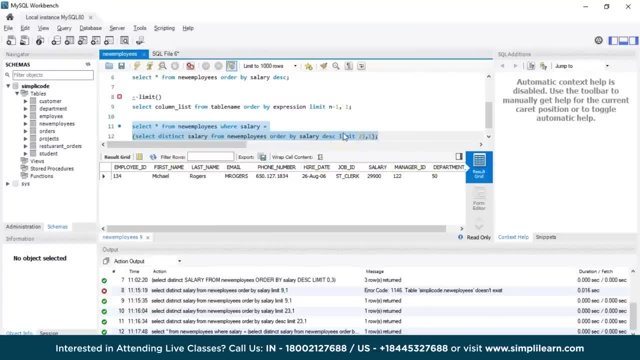 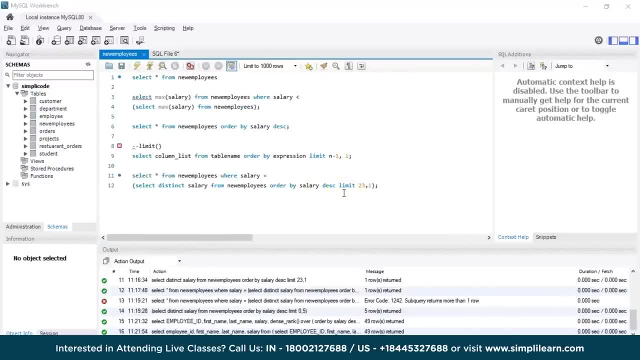 So in this way, if you want to fetch the complete details as well, you can use this subquery here. Now, let's say, if you're asked to find the first five highest salaries in the table, then the parameter here will be changed. 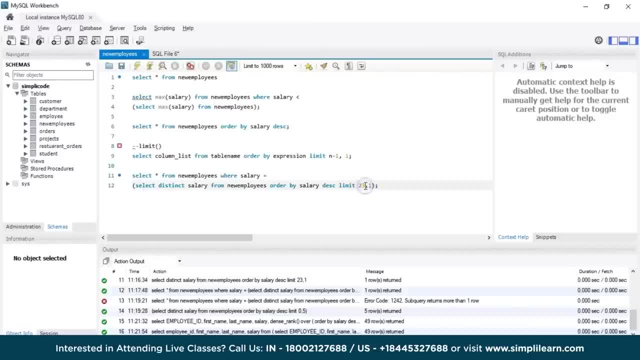 Now here our N value becomes one, So the M minus one becomes zero. Now and we want to fetch the first five records from the table, So we'll mention five as our second parameter, which will basically display the first five records. So let me just display. 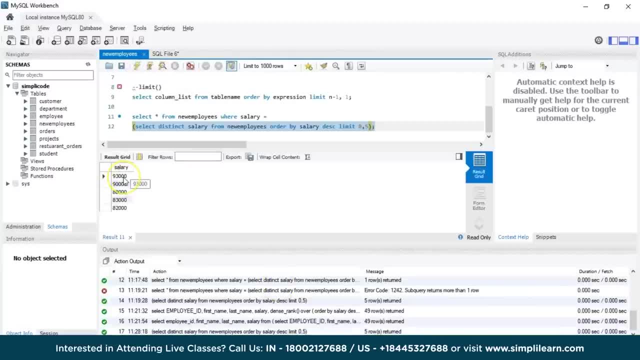 Okay And execute this statement. So, as you can see, it will display the first five highest salaries, starting from 93,000, 90,000, next 88,000, 83,000 and next 82,000.. Now, if you observe this query carefully, it is somewhat similar to that of the top function. 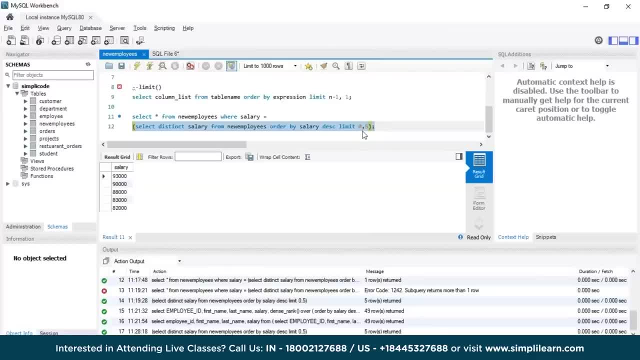 we use Now. since top function is not applicable in MySQL, we are using the limit clause here. Now, if you're working on different other databases like SQL Server or MongoDB or Oracle, you can use the top function Now. the format will remain the same. 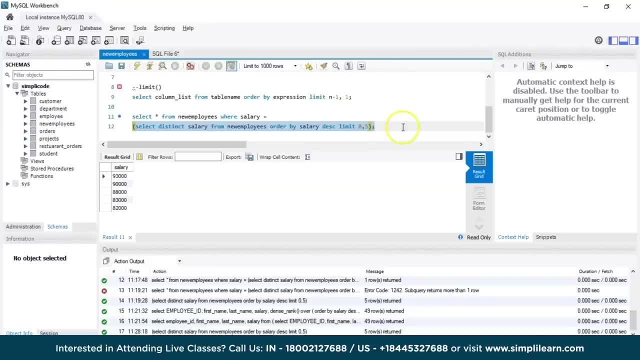 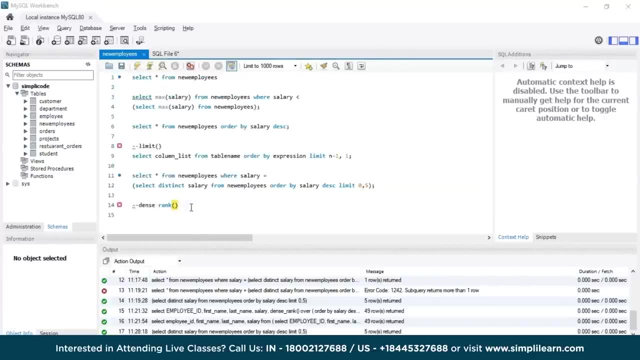 Only the syntax will change with the use of top keyword. So in this way you can use the limit clause to find the nth highest salary. Let us now discuss the second way, that is, using the dense rank function. Now MySQL. dense rank function is an ilbin function which is used to return sequential 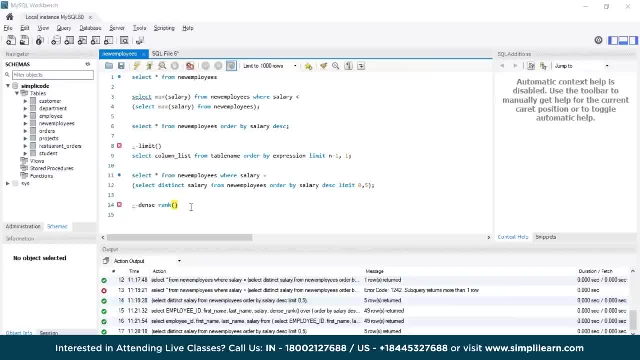 numbers starting from one, based on the ordering of rows. It is imposed by the order by clause. Now, when you have two records with the same data set, then it will give the same rank to the both rows. So firstly let us understand the syntax here. 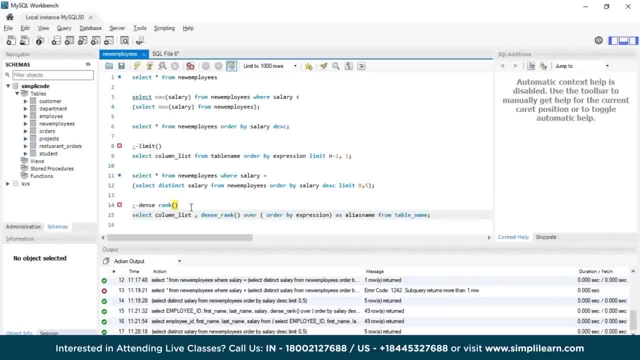 The syntax is followed as: select column list. These are basically all the columns that you want to fetch in your resultant table. comma dense rank is the keyword we use here. over and inside the parenthesis we are writing the order by clause and we'll mention the expression as and we'll give an alias name. 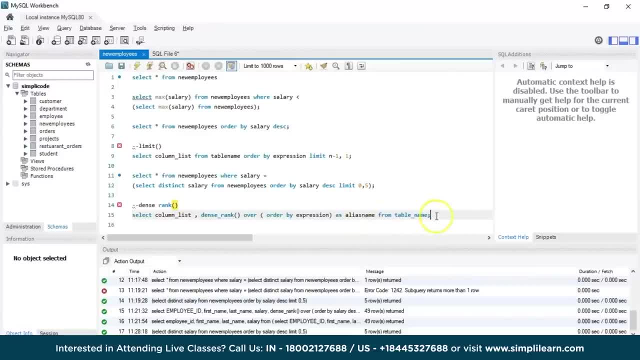 to this. Okay, A dense rank function from the table name. So now, basically, the function is always used with over clause here, which will always assign rank on basis of the order by clause, and the rank is also assigned to the rows in a sequential. 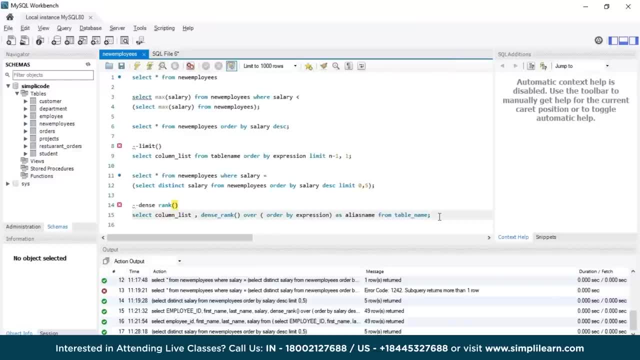 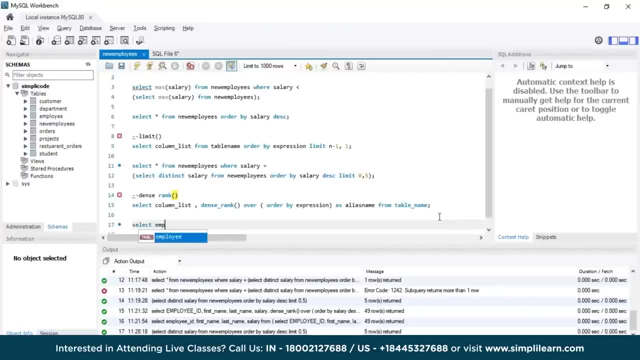 manner. That is, the rank. the assignment of rank to these rows will always start from one, and the next value will be one greater than the previous rank aside. So let us understand this with an example. Now let's say I'm, I'll use the select clause here and I want to display the employee ID, the first name. 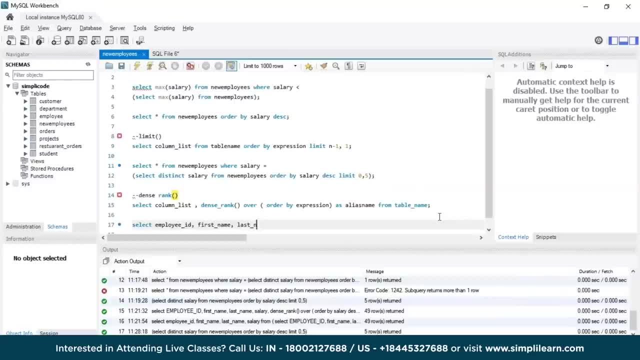 of the employee: last name, comma, salary, And next I'll mention the dense rank keyword. over and inside the brackets, use the order by clause and mention the expression. Now we want to specify the condition here, which is basically on the salary right. 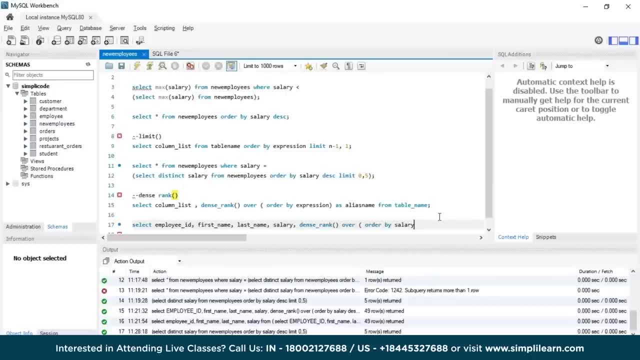 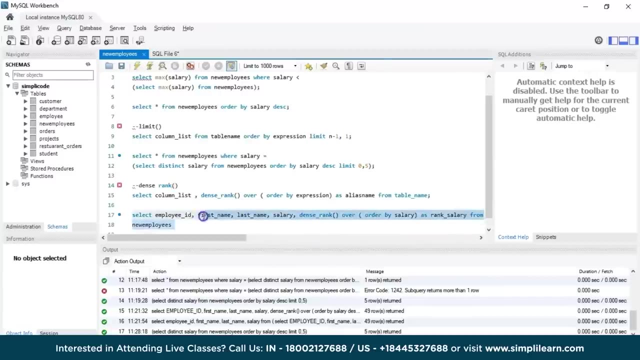 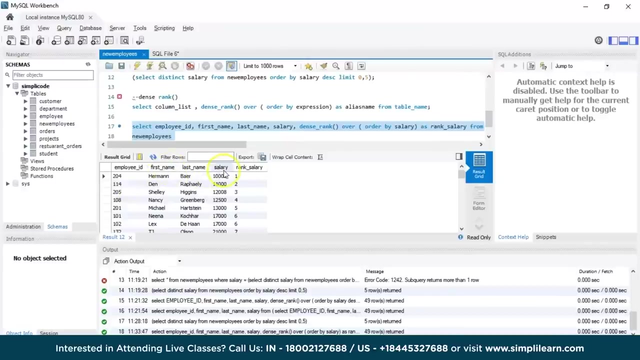 We want to find the entire salary here, So we'll specify the salary here, as let's give an alias name, let's say rank salary from the table that is new employee. So let us execute the statement and we'll see the output. So, as you can see, it will display the employee ID: the first name, last name, salary and 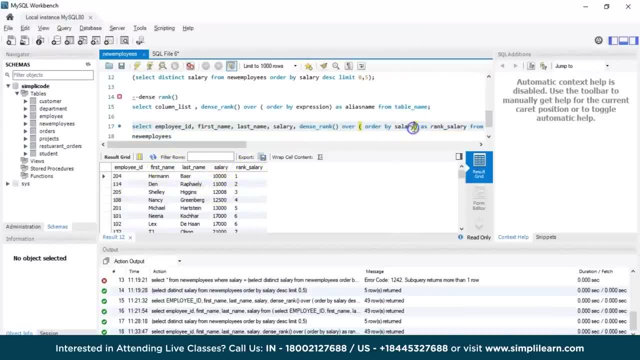 the rank of the salary. Now, since we haven't given any a keyword here for descending and ascending, it is showing in the ascending order by default. So let me just write the descending keyword by using the DESC. So let us now display this. as you can clearly see, it will display the records from highest. 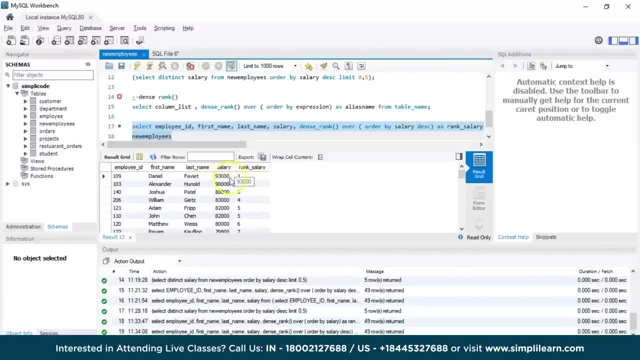 to the lowest value and the rank is assigned accordingly. Now for the salary: 93,000, it is giving rank as one, And for 90,002, for 88,003 and so on. Now, if you look here like the employee Adam Fripp, who's having 82,000 as salary and similarly, 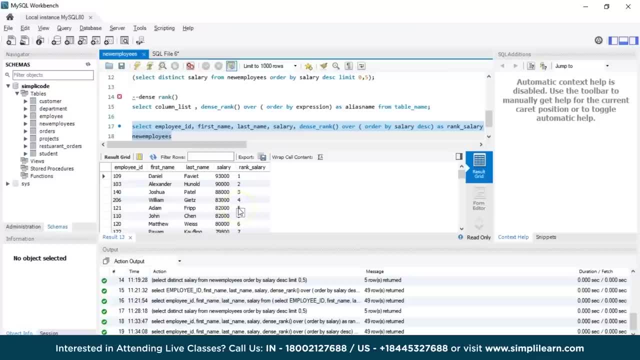 John Chen, who's also having 82,000 salary, and the rank is assigned as five, which is same. Now, if you carefully look here, it will assign rank based on the value and not on the number. So even if the values are repeated, it will assign the same rank to that value. 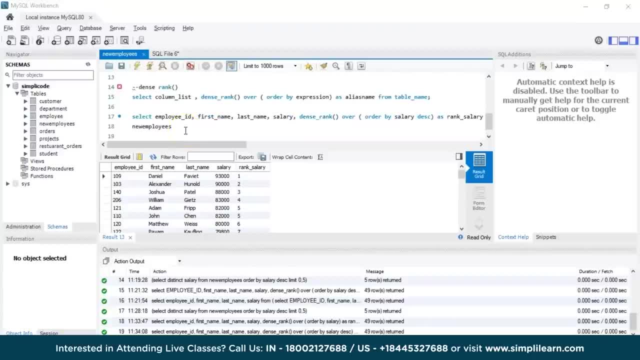 So I hope you understood how to use the dense rank function here Now. let's say, to find the nth highest salary, we'll have to use a sub query here. Now, basically, I'll keep this as a sub query here and I'll use another select statement. 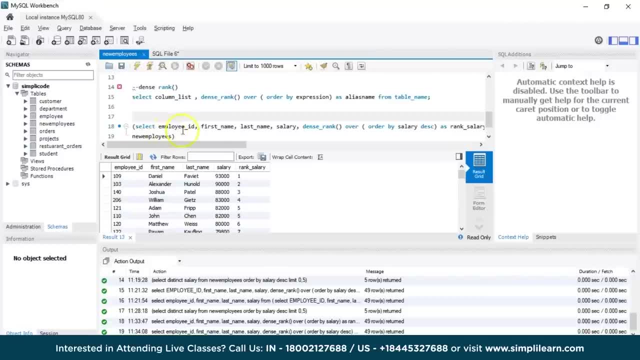 So basically, I want to again display the employee ID- first name, last name and salary in a resultant table. So I'll just copy this and keep it as an outer query From this table, right? So, and I'll mention a where condition where rank salary is equals to now, you can mention: 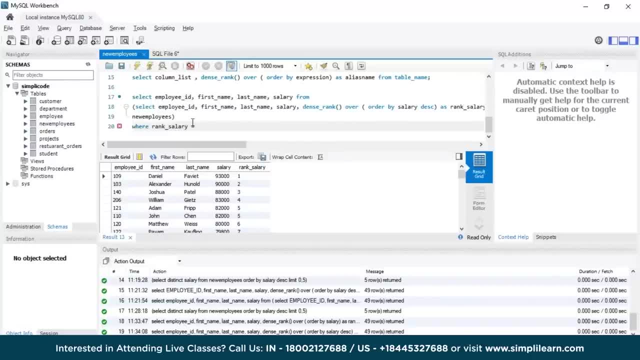 the nth highest salary. Now, whatever you want to display, you can mention this here. Now let's say: if I want to find the 32nd highest salary, I'll just mention the rank: salary equals to 32.. So let us now execute this statement and we'll see the output. 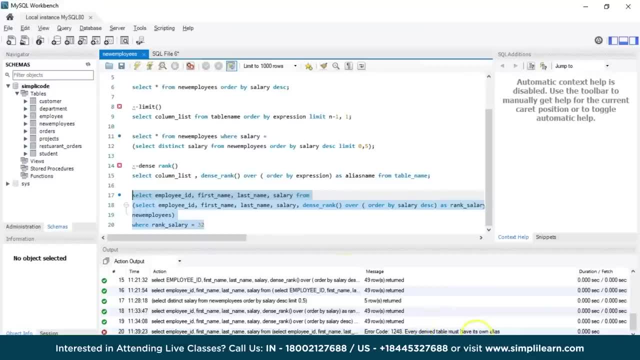 Now it will show me an error. This table here which says every derived table must have its own alias name. So we have not given any specific alias name to our table here. So let us just give alias name. let's say as E, or you can take EMP or anything as per. 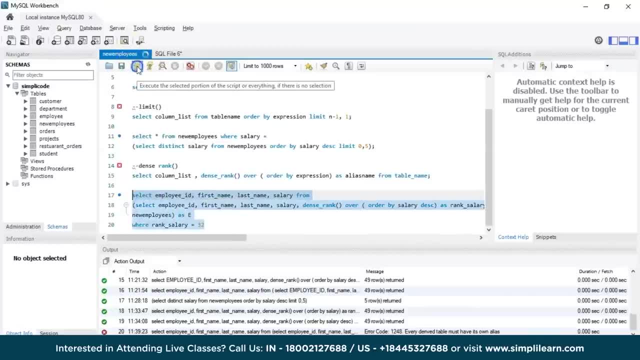 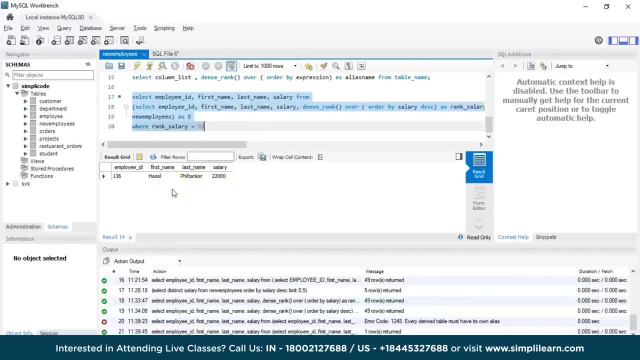 your choice, Right? So let me just display this and we'll see the output. So, as you can see the 30,, what is that? 32nd highest salary has been assigned to the employee Hazel Filtanker, whose salary is 22,000. 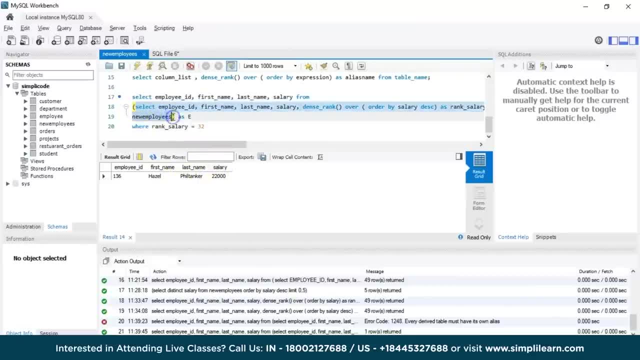 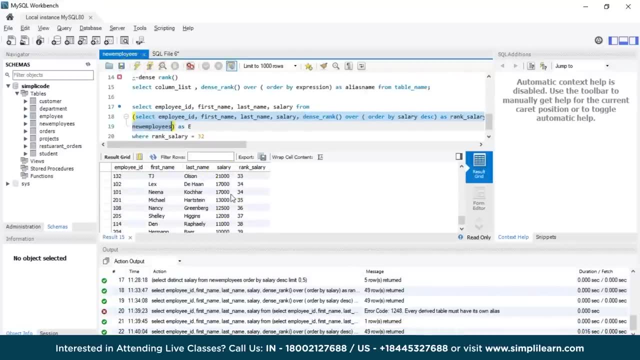 So let's just check whether it is correct or not. I'll just copy this dense rank select statement again. So let's just scroll down and, as you can see, 32, which is the rank here, has been assigned to the employee Hazel Filtanker, whose salary is 22,000. 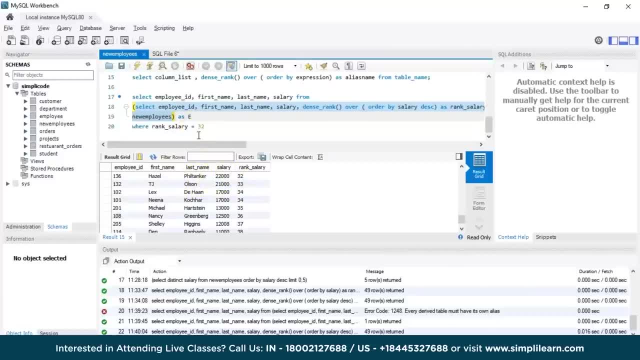 So, which is correct, and you have successfully executed query in this case. Now, similarly, if you want to find another, Okay, If you want to find employee salary, let's say, if you want to find 18,, 16th highest salary. 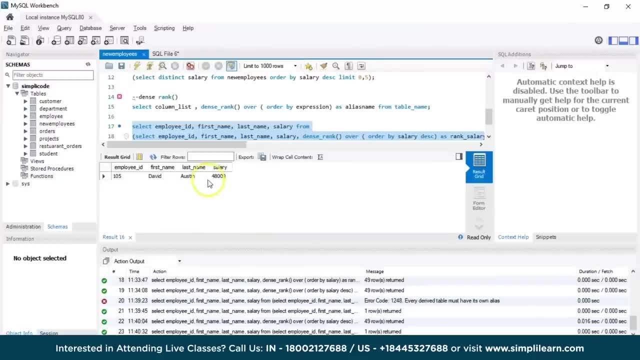 where it take this and will execute the statement. and it is showing me as the 48,000, which is the 16th highest salary, and the employee ID is 105.. The employee name is David Austin and in today's session we are going to learn about views. 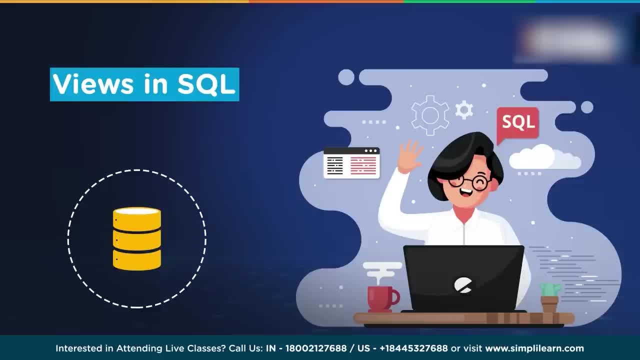 in SQL. SQL views are very powerful in its usage. when used properly, They allow the user to store SQL queries into virtualized containers, Or in other words, virtualized containers. Okay, So in today's tutorial, we are going to learn how to create a view in SQL and understand. 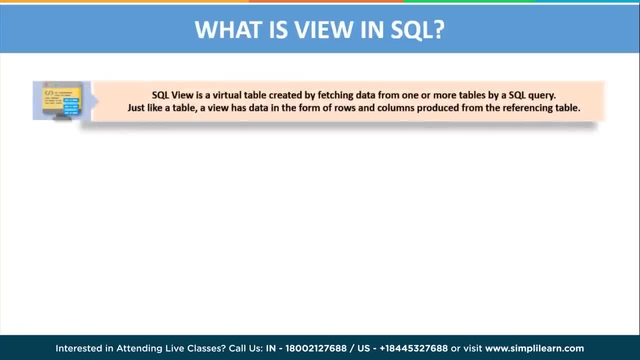 how exactly they work. What is view in SQL? A database? view in SQL is like having virtual tables containing a single query and its result. The result is usually a virtual table with rows and columns, just like the actual table in a database. We can either pass a query to store all the rows and columns of a table or only a part. 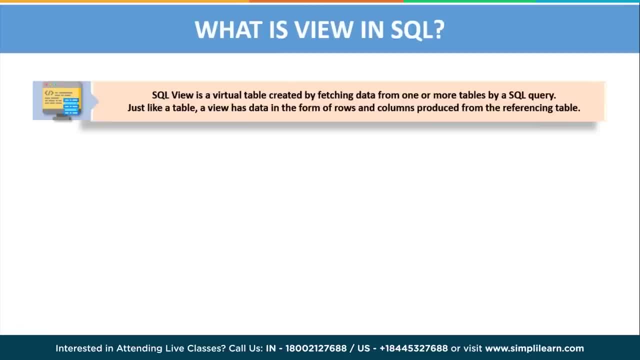 of it. But the most significant advantage of a view in SQL is that it stores the query and hence we don't have to write it again and again from scratch Now. but then then a question arises: why not use the stored procedure instead? Even a stored procedure can hold a query and execute whenever called. 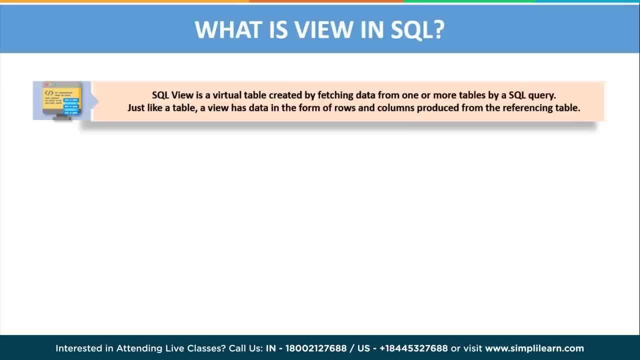 However, the advantage with view is that they are easier and more straightforward compared to procedures. While procedures can have multiple statements with them, views can have only one. Also, views do not accept any password. Views can be considered as one of the database objects which is created over an SQL query. 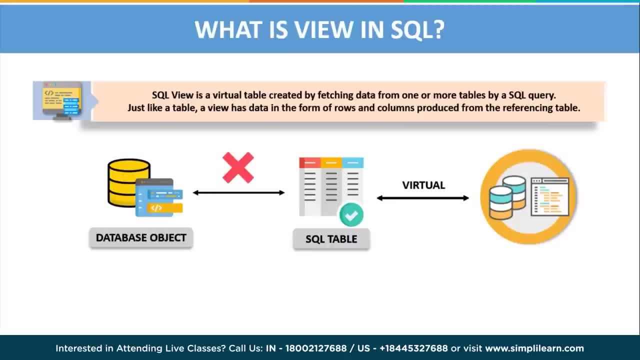 It simply represents the data returned by an SQL query. So a view does not actually store the data in the tables. but every time we call a view in the database it returns the result set of the query in which it is defined. So in a nutshell, we can say that a view is similar to that of a relational database table. 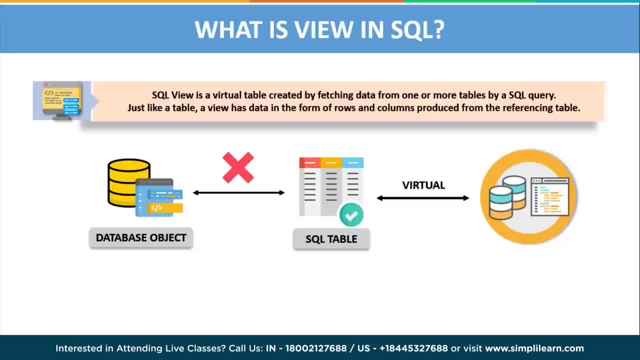 which can be treated as a virtual table, And it is just a mere representative of an underlying SQL query. It always fetches the data from base tables that are used to create the view using the view creation query. Let us now understand the syntax. 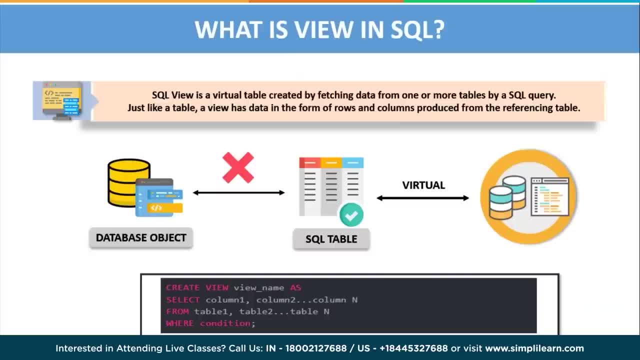 The views in SQL are created with the create view syntax and creating views in SQL is very simple. Following is the basic syntax to create a view in SQL and it is followed as create view view. name as select column one, column two, up to: 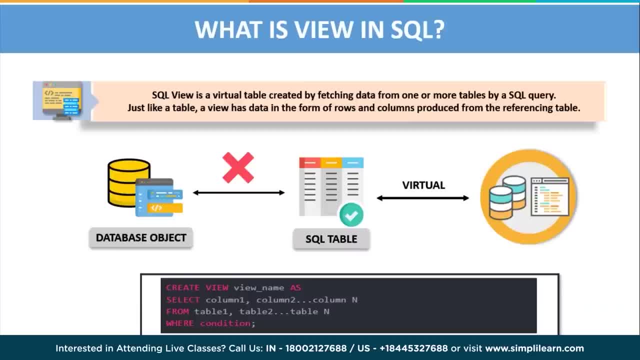 So on column N from table one, table two, table N, where condition Now to see the data in the view. we can query the view using the following select statement: Now create view is used at the start of the code to initiate the view and then select. 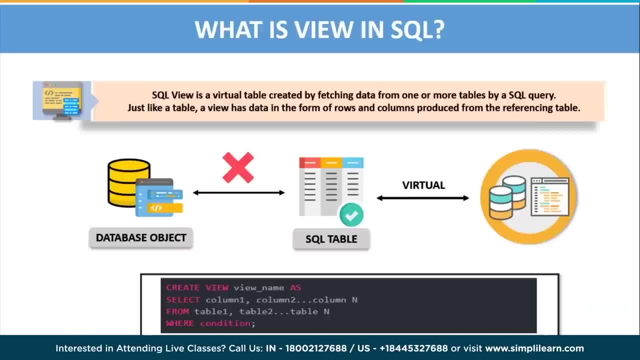 is used to decide which columns to pick from the tables. Now table one, table up to so on table and denotes the names of the table. However, you can work on a single table as well. Now, where is used to define the condition Which is used to select only a particular number of rows? 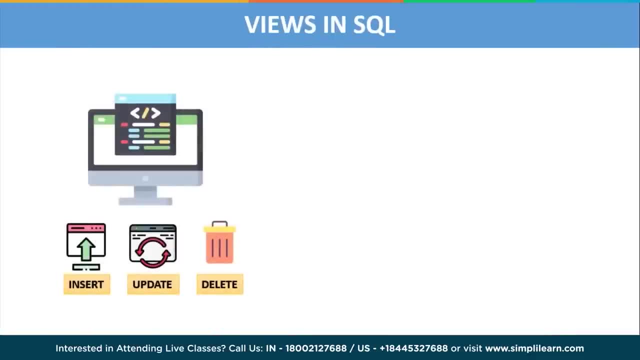 Now, another significant advantage of views is that it allows certain operations like insert, update, delete, just like you perform in a normal SQL table. Now, other than this, we have other operations which can be performed using the view. Now, view is used to filter records using where clause. 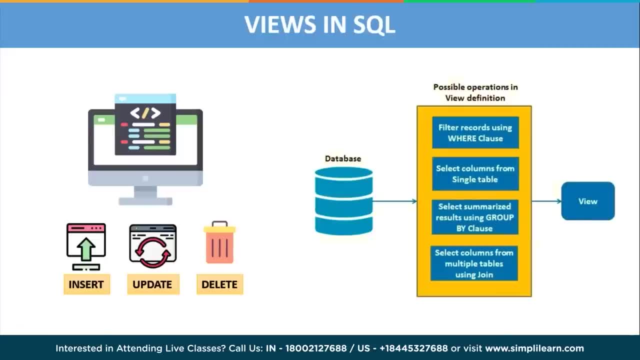 Now we know that there is a lot of chunks of data in our database, And if we want only a part of it, we can filter the data using the where clause. Similarly, we can select columns from a single table as per our need. 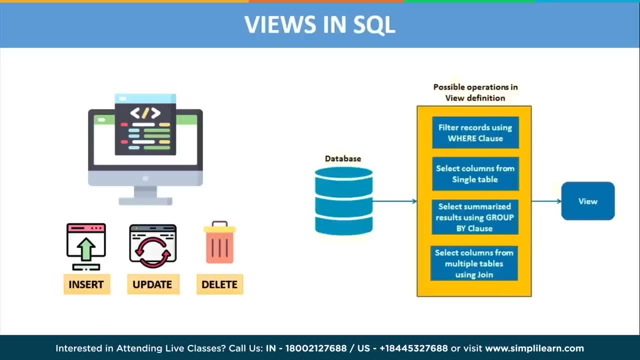 And in the same way, we can use the group by clause to select only a particular or a summarized result of a resultant set. And finally, we can also select columns from multiple tables using the join condition as well. So now that we've understood what exactly views are, let us jump into MySQL workbench. 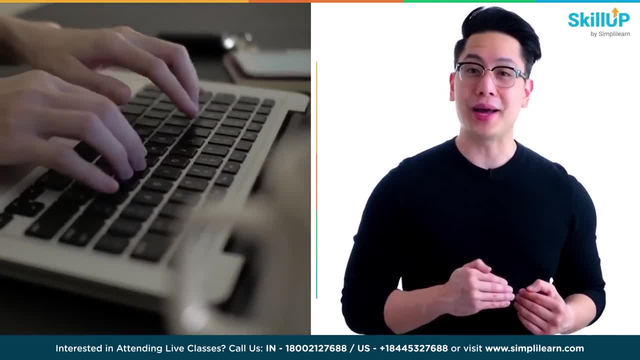 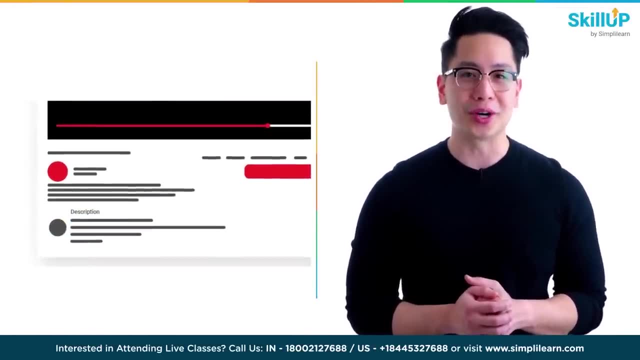 for execution part. If getting your learning started Is half the battle, what if you could do that for free? Visit SkillUp by SimplyLearn. Click on the link in the description to know more. So, as you can see, MySQL workbench has started, and before we proceed into the execution part, 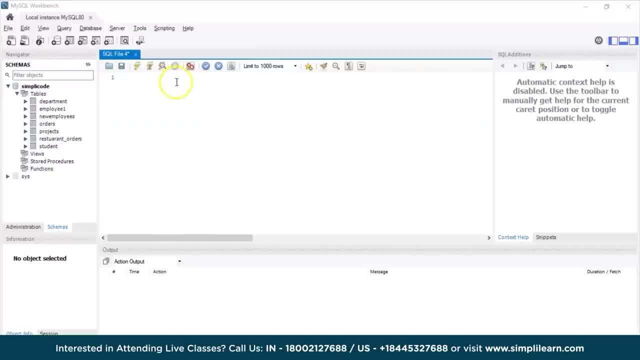 and see how to create a view in SQL using various examples. let us first quickly understand why we use views in SQL, so that we'll have a clear picture before we get into the execution part. Now there are various reasons for using views in SQL. 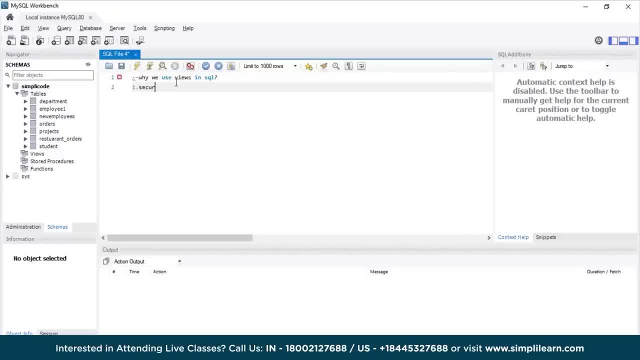 The first one, Views provide security to the data, acting as a security mechanism, and views can actually enhance security by restricting data access to users. For instance, we can limit a user from accessing the actual table that contains sensitive data, but provide access to the view that has only insensitive data. 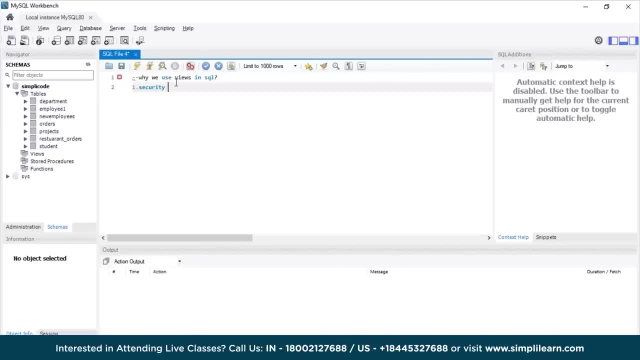 Let's take an example to understand this now. in a company there is an employee, HR and a manager who might be working on On A same database table. to fetch some information Now, because they are from different departments, there must be some data that might be irrelevant. 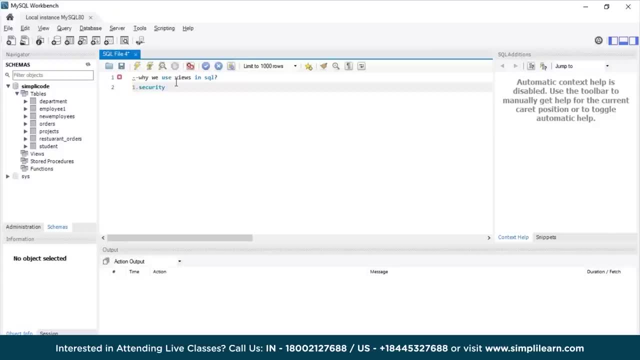 to HR but it might be relevant to the manager, and in other case that data might be relevant to manager but it might be irrelevant to the employee. So in that case there should be a security mechanism that would hide irrelevant information of the table from certain usage. 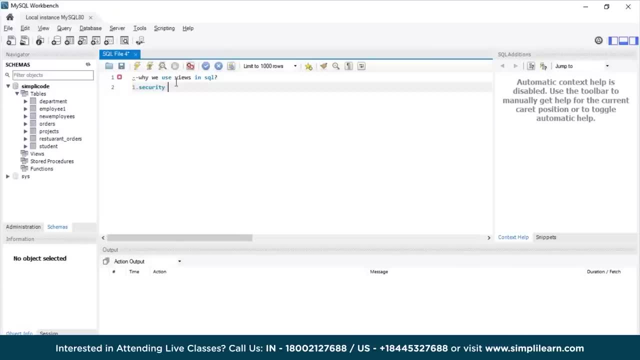 Now views allows us to hide or show some data. Now. the second reason is because of to reduce the complexity. Now views are introduced, or whatever actually introduced, to reduce the complexity of the multiple tables and deliver data in a simple manner. views hide the complexity of the data. 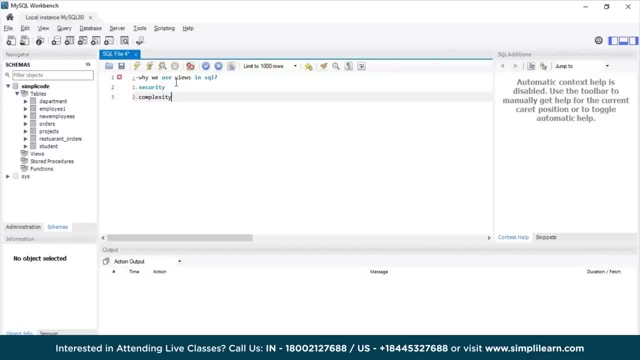 in the database, as they join and simplify multiple tables into a single virtual table, which is easier for user to understand. And finally, because of consistency reasons. now views also maintain the data integrity, as it presents a consistent and accurate data from the database. You can easily make changes to the views according to the user requirement and the effect of. 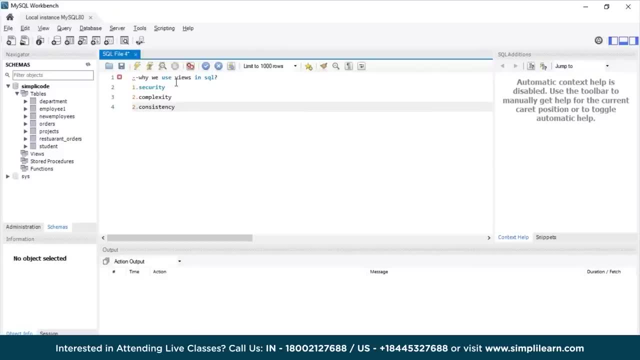 the same will be seen quickly in a quick manner. So now that we've understood why we use views in SQL, let us just quickly go get into the execution part now. Now we can easily create a view SQL from a single table, or even multiple tables, using the create view statement. 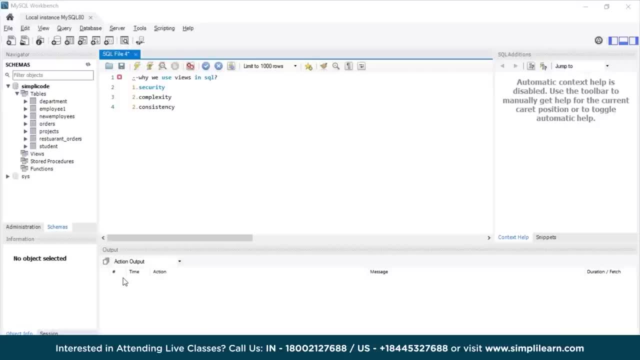 Now, but before we create a view, we'll create a table named customers that we will use throughout this session now. So let us just create a table first, which is a customer table, and the syntax is create table, customer and in the customer table, I'm going to create various columns or fields. 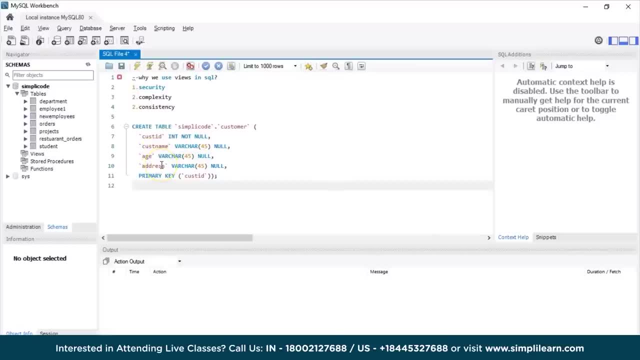 such as customer ID, customer name, age, address- and I'm giving customer ID as a primary key because it uniquely identifies each and every record in the table. So let us just execute the statement and we'll see the output. So our query has been successfully executed. 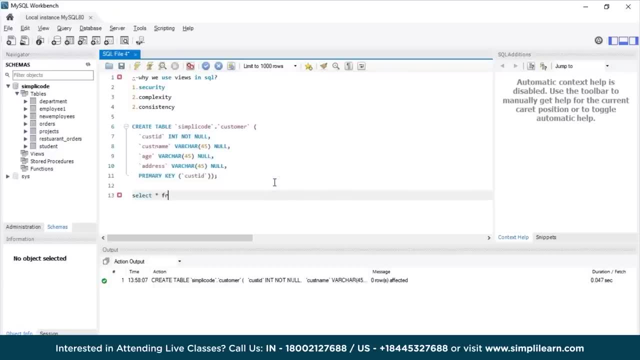 So let me just use the select statement to display the result. So let's start from customer right. So our table has been created and the fields our customer ID, customer name, age and address are being displayed. Now let us quickly insert some values into the API. 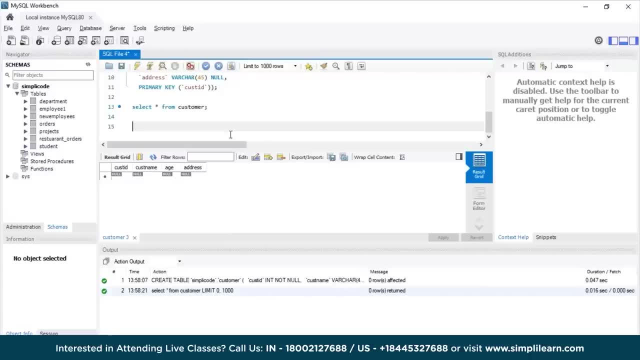 So let's create a table, So let's create a table, So let's create a table in this table. Now I'll use the insert statement for that. Insert into table name, which is customer values, and within the brackets Now, customer ID. let us take as 101.. 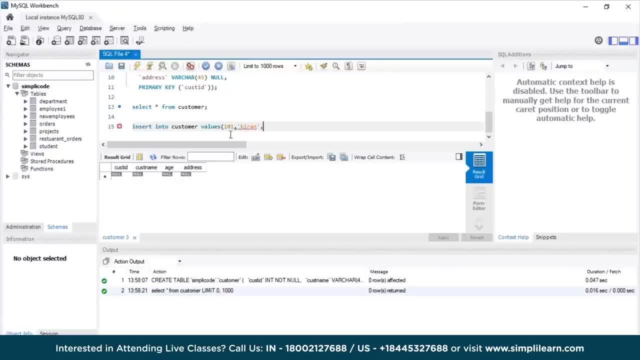 Name: let us take as Kiran, and age: I'm taking as 25, and address: I'm taking as Hyderabad Right. So let us execute the statement and we'll see the output. So our query has been successfully executed and the information has been inserted into. 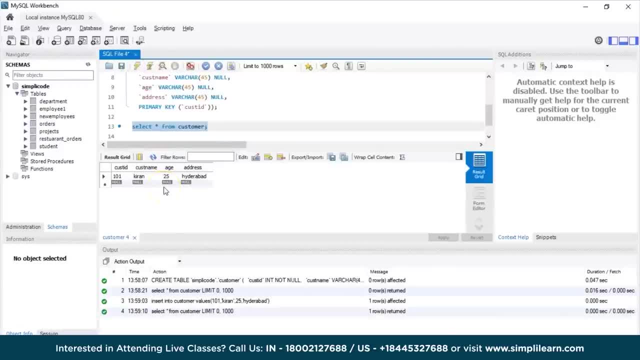 our table. So, as you can see, the details of Kiran has been successfully executed and displayed in our table. Now, similarly, I'll insert some more records into the table. So let me just copy this insert statement: Okay, Okay. 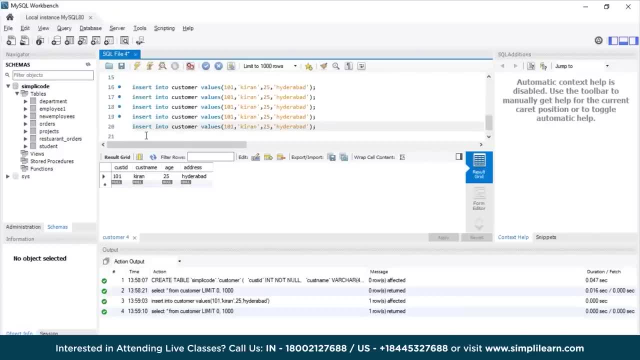 Okay, Okay, Okay, Thank you. Okay. So let us change the values here- 102,, 103,, 104 and 105, and name also let us change. I'm taking another customer name as Priya Kushal Vaibhav and let's say Gayathri, and 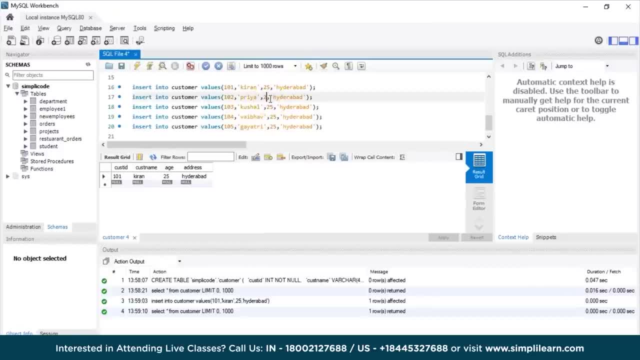 let us change the their ages. vaiabhav and ayatriya their age as well. i'm taking as 26, 24, 28 and 23.. now you can change their address as well. so i'm taking the address of priya as bangalore. for kushal i'm taking as mumbai. let us just uh, remain. 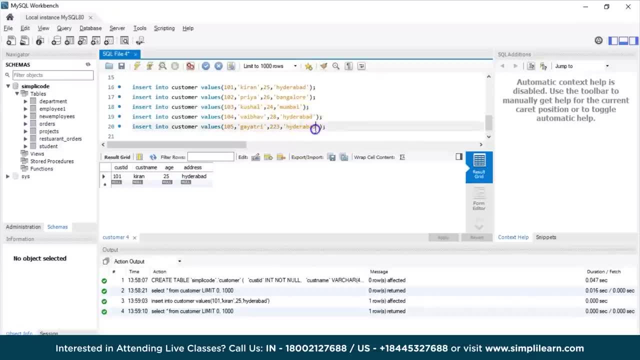 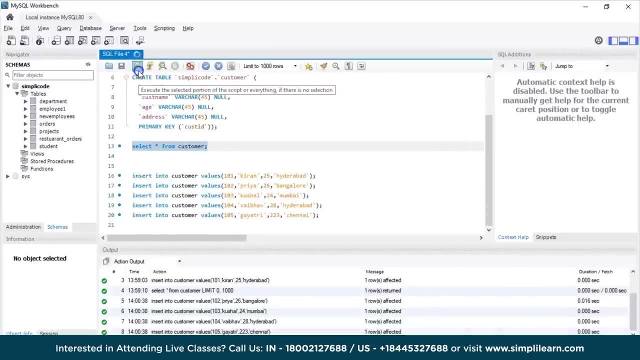 in hyderabad for weiber itself and let us take as chennai for guy 3.. so let us just execute this statement and we'll see the output. so our query has been successfully executed. let me just display the values now. so, as you can see, a total of five records have been inserted into our table. 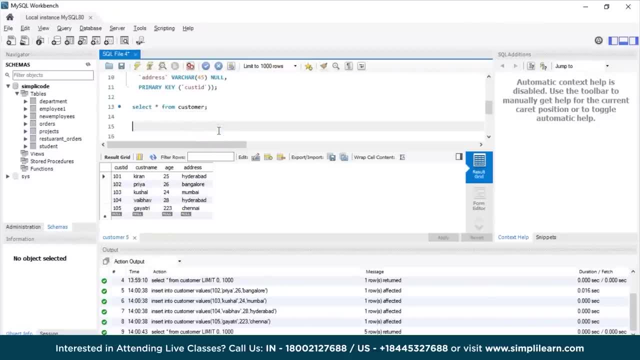 now we can proceed, uh, into creating a view for our table customer. now, to begin with, uh, we'll create a simple view from our customer table, which is an existing table which we've created just now. so the following syntax would be: create view, which is the keyword we use. 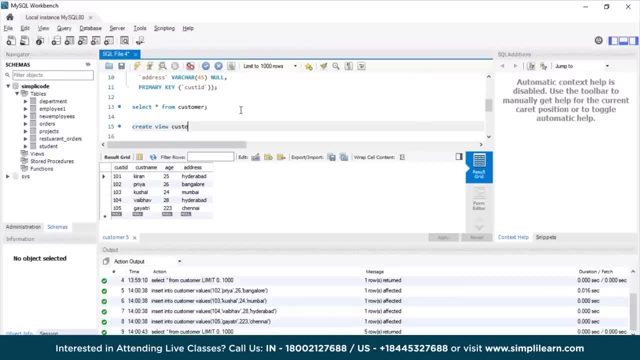 you can give any name to your view, let's say customer view, as select the columns that you want to display in your resultant view table, which is a virtual table, right? so i want to display all the fields in my resultant view table, so i'll use the select star. 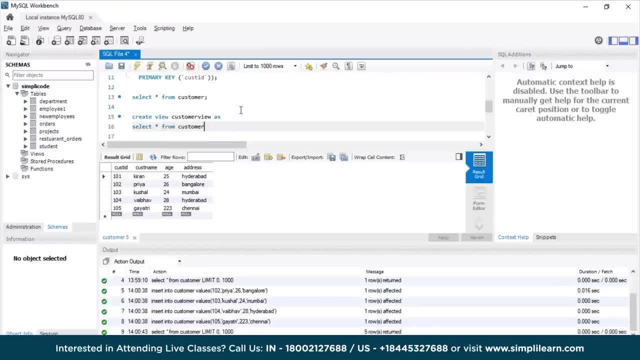 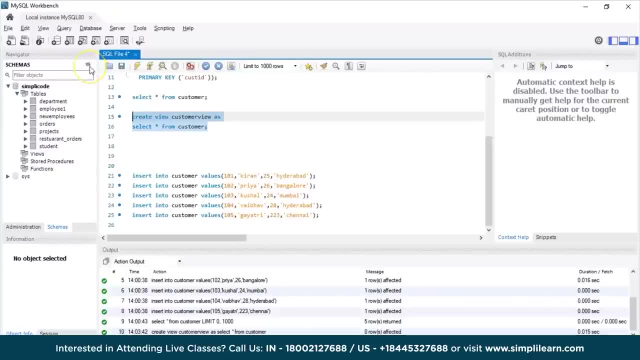 from customer. so let us execute the statement and we'll see the output. so our query has been successfully executed and now, when you refresh the schema section, you can see in views you can find a new one which is created as a customer view. so let me just display the results in the view. 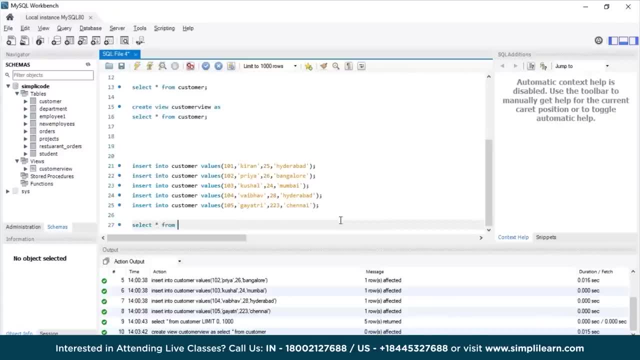 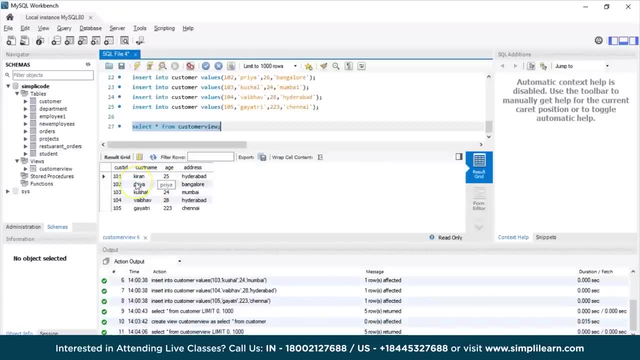 for that i'll use the select query again- select star from customer view- so as you can see the exact details of the customers that we have already inserted in our previous table. customers has been inserted in the customer view as well, so that means in this way, this view will store all the columns that were uh in the customer table and it will simply copy paste. 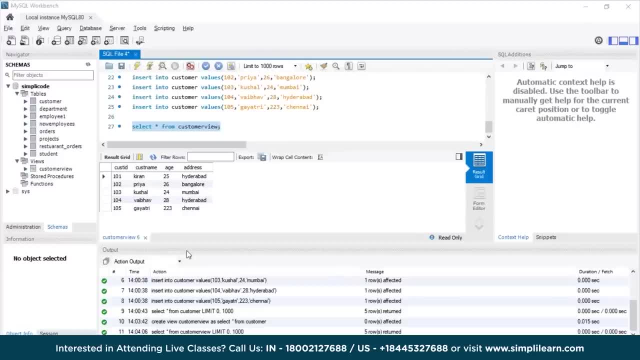 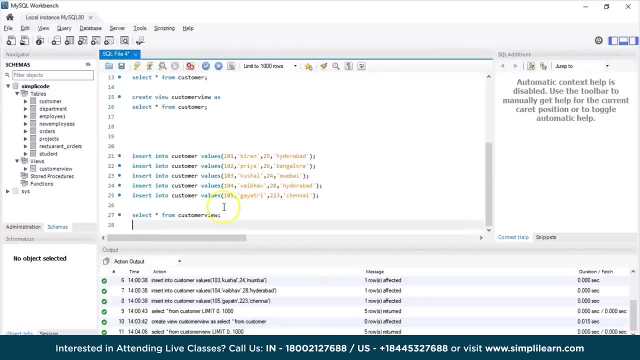 all the records from customer table into the customer view which we have created now. so let's go now. similarly, you can also, uh, create a view from the existing table as well. so for that, let us take an example. let's say, if i want to create a view of projects table here, 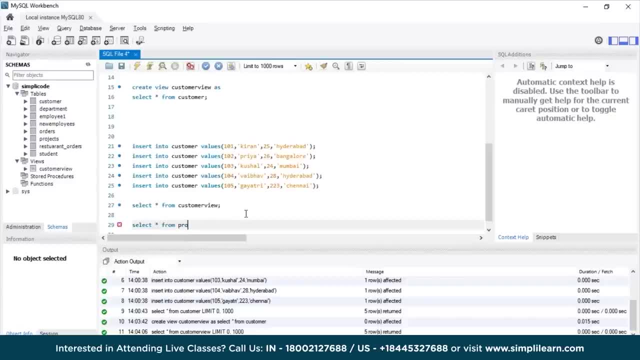 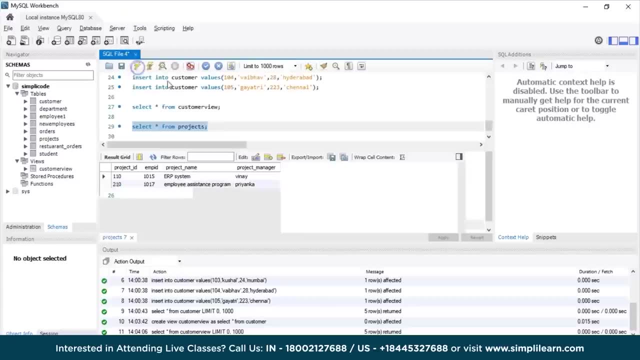 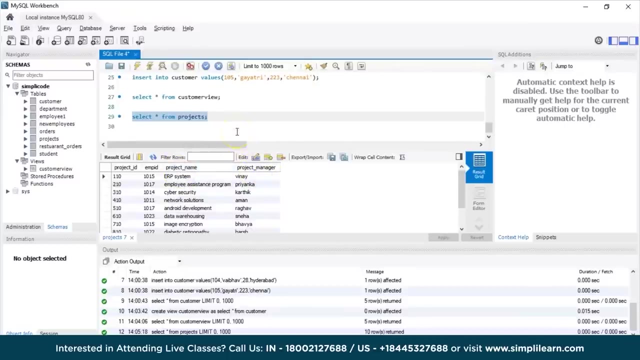 so let me just display the records from the projects table and we'll see the output. so, as you can see, the project table has various fields, such as project id, employee id, project name, project manager. now, let's say i have, i've had a new requirement wherein, uh, there is a new employee who is joining as a fresher into the company and 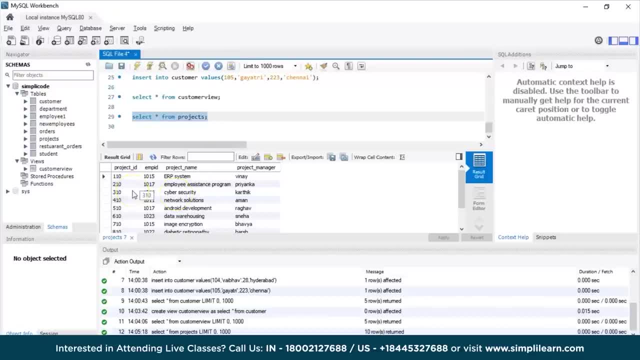 as a manager, i want to uh show the details of all the project names uh that the company is currently working on. now i want to hide the employee id details because i don't want the fresher to uh have exact idea on which project the current employees are working. so for that. 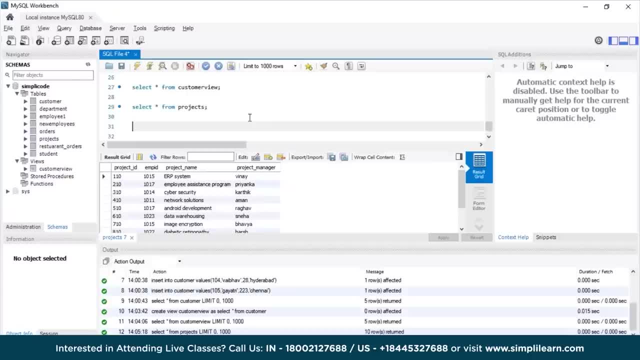 i'll create a view, a simple view here, which will basically uh give all access to the uh fresher or the the employee who have recently joined. he can only view the project name and project uh manager's name. that's it. so let me just create a view here. 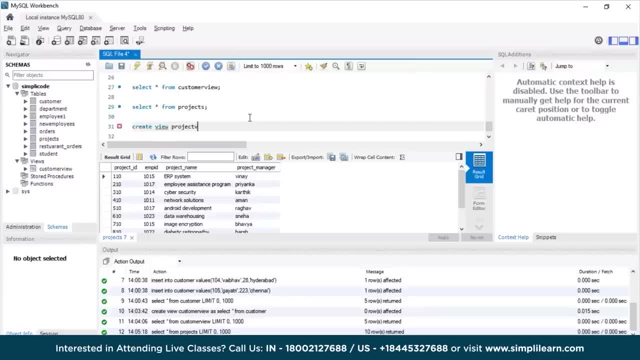 create view. let us take the view name as project view again as select the columns. now i'll just select the project id, the project name and the project manager's name here click managers from the table. that is projects. so let us execute this statement and we'll see the output. 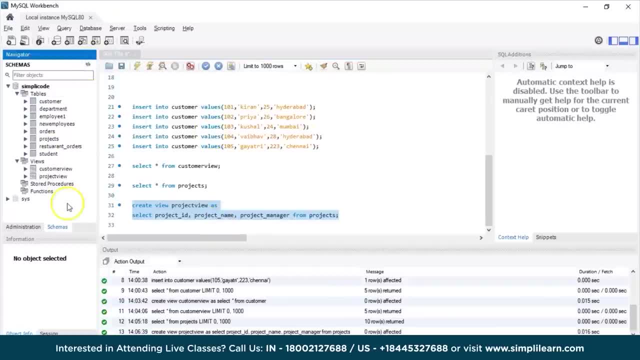 so our query has been successfully executed. now, when you refresh this again, you can see another view is formed in the view section, which is the project view. so let me just display the records that are present in this view. i'll use the select statement again. select star from projects. 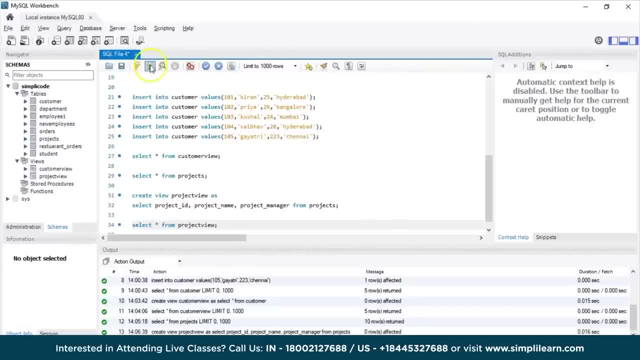 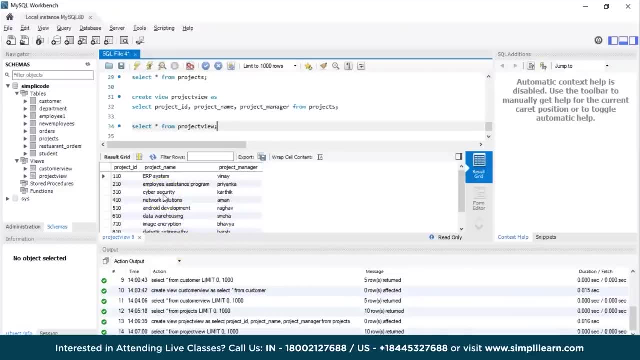 so, as you can see, now only the project id, the project name and the name of the project manager are being displayed, without uh displaying the employee ids in this view table. so it will basically encapsulate or hide the unwanted details for the new employee so that he can only view the 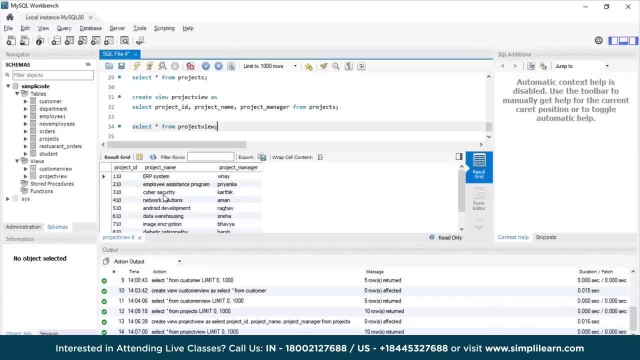 project name and the project manager's name itself. that's it right. so that brings us to the next segment, wherein we'll look at the project name and the project manager's name itself. that's it right. we'll understand how to perform various operations in a view in sql, that is, how to insert, update and. 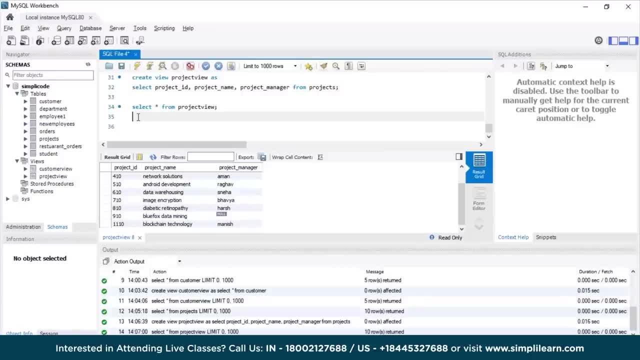 delete records in a view. now, just like actual tables, we can easily insert, update and delete rows in a view. that is not allowed in stored procedures. now, firstly, let us discuss how to insert a row in a view. for an inserting a row in a view, we'll use the project view. 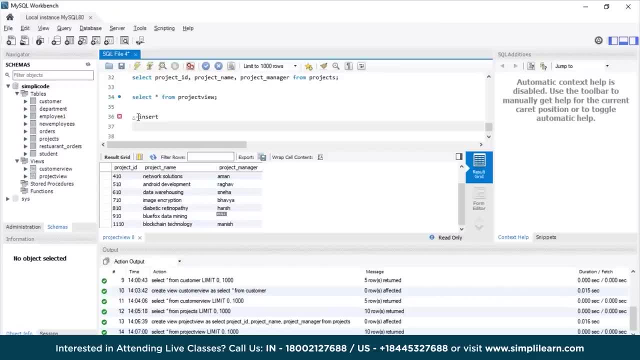 as an example that we have created earlier now, the view already had, let's say, i think, 10 rows and we'll insert another row using the insert into command. so the following syntax is: insert into name of the view, that is, project views, project view values, and inside that, let's say i'm taking a project id as 1, 1, 2, 0 comma. project name, let us say artificial. 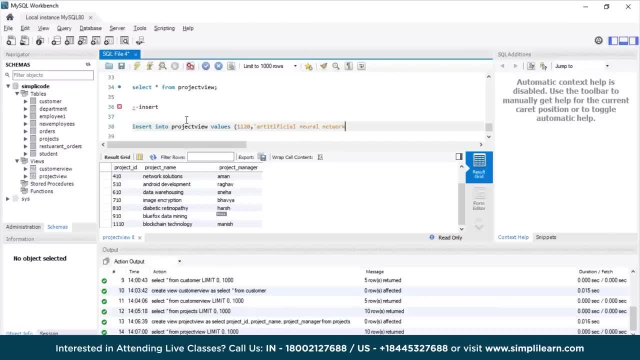 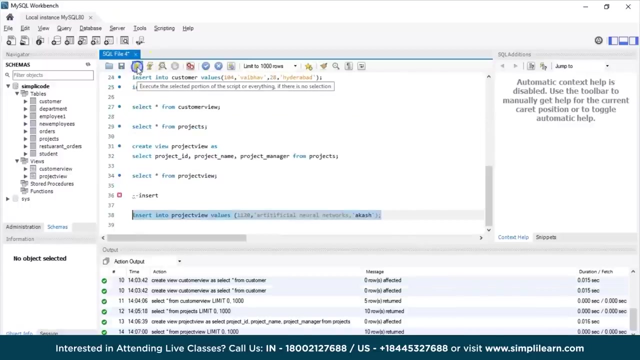 neural network comma. and let us say, the project manager name is akash, so let us execute the statement and we'll see the output. so our query has been successful. so that's it for this segment. so this is the end of our video today. i hope you've enjoyed or found useful this video to be a help for others. if you're interested in this kind of project, you can also give a thumbs up. let us know in the comments if you have any question or would like to proceed with the next steps. please don't forget to share this video with your friends and family. so thanks for that. 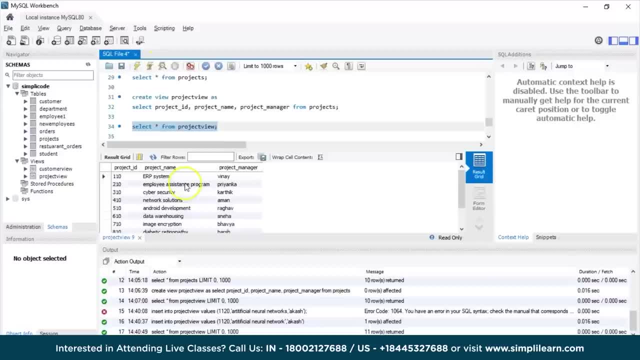 executed. so let me just use the select statement again to display the records. So, as you can see, there is a new record with the project ID 1120 and the project name is artificial neural networks and the project manager name is Akash. So, as you can see in the output, in this way we can create another row by 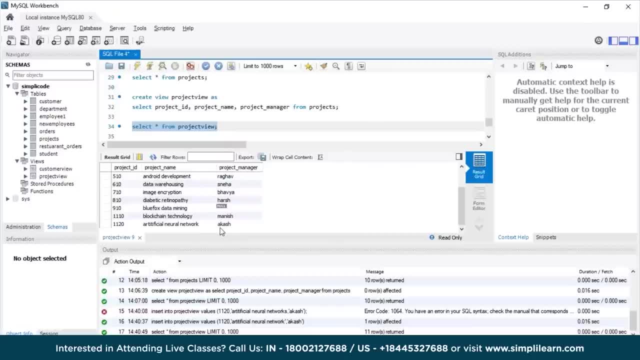 inserting in the view, which confirms that the insert statement has been successfully executed. Right, so next, let us discuss how to update a record in a view. Now, like just like inserting, we can also update a row in a view. If you notice the previous example, we have inserted a new row, that is, with the: 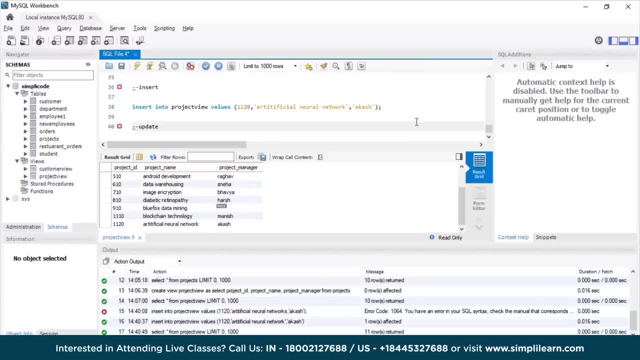 project ID as 1120.. Let us update one of the record in this. Let's say, if I want to update the project details of blockchain technology as something else, I'll use the update statement here. So the syntax for the update would be: update. mention the view name. that is, project view. 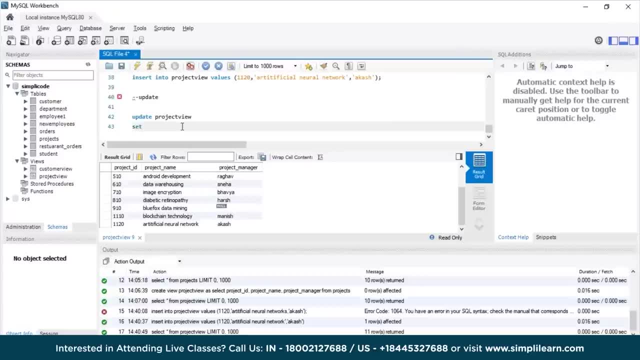 update. mention the view name, that is, project view set. now, since you are changing the project name, I'll mention the field: project name set. project name equals to Now. let's say, if I want to change the project ID 110 as, let's say, SEO optimization or let's say, SEO analytics. 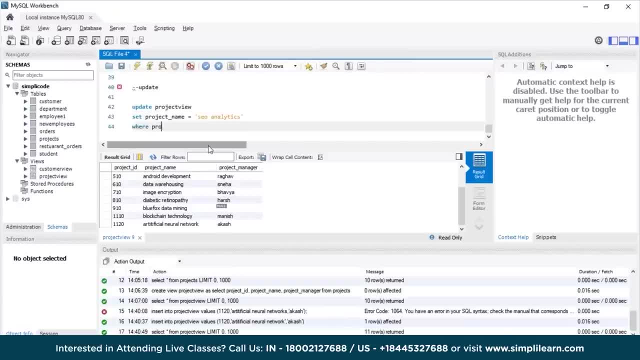 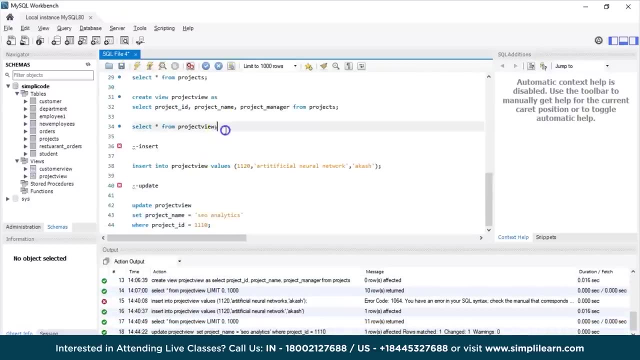 where project ID equals to 1110.. Right, so let us execute this statement and we'll see the output. Our query has been successfully executed, so let me run the select statement again to display the records, So as you can clearly see that the project ID which was 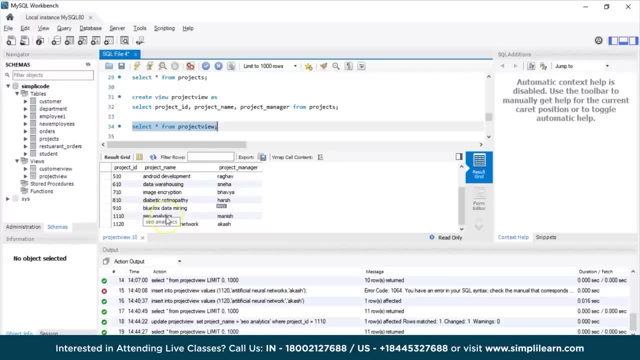 1110, which was earlier blockchain technology, has been changed into SEO analytics, So the updated the version of the column name, which was blockchain technology, has been changed into SEO analytics successfully. Thus, it is confirmed that the update statement has been executed successfully as well Now. 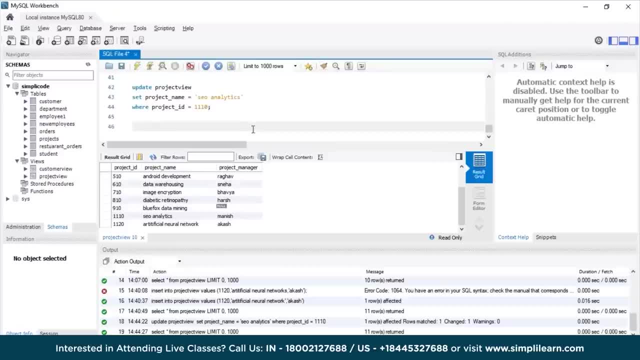 finally, let us see how to delete a record in a view. Now, just like how we inserted and updated a row, we can also delete a row using the delete statement. for example, we will delete the row which is having project ID, let's say 810, which is project name as diabetic retinopathy, and the project manager name. 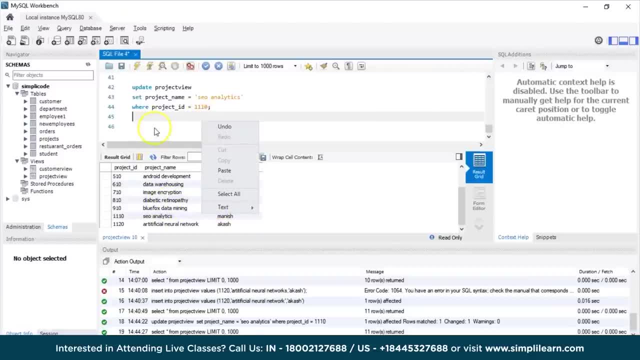 is Harsh, so let me just delete this record. so I'll use the delete statement here: delete from project view. where is the condition we use here where project ID equals to 8, 10, right? so let me just execute this again. so our query has been: 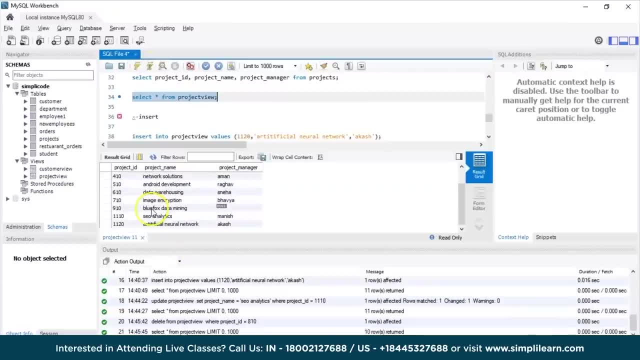 executed successfully. let me just display the records so as you can see the record. the project ID which is having 8: 10, which is one of the record in this table, has been successfully deleted. so in this way you can perform various such operations which we actually generally perform in the normal. 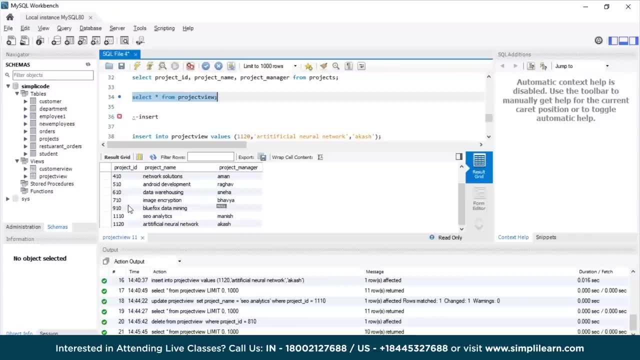 SQL tables. you can similarly perform them in SQL views as well. now, first, for some reasons, if you want to delete the whole view, that is the view that we have already created. now, for some reasons, if you want to delete it, you can delete it as well as you can delete it as well as you can delete it. 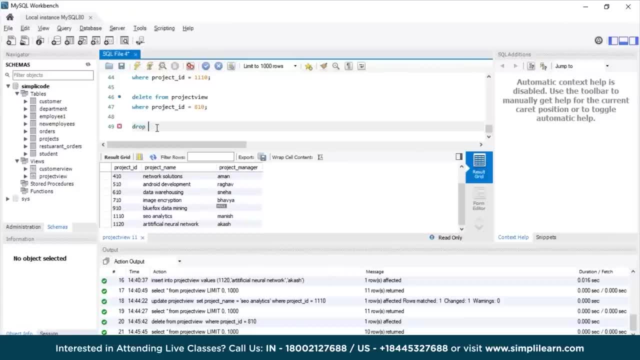 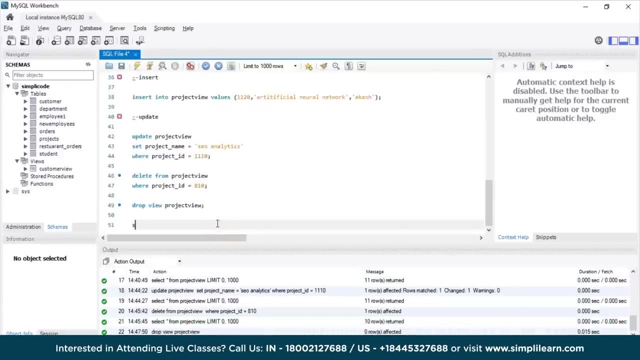 you can simply use the drop command here, which will completely delete the view that you have created. so the query would be drop. mention the view name, which is project view, right? so let us just execute this. so our query has been successfully executed. so let me just use the select statement to display the 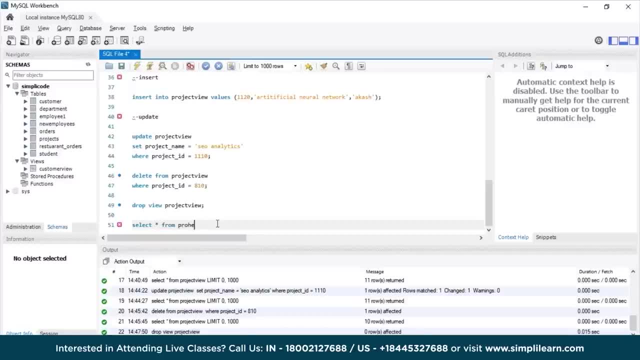 record, select star, from which is project view. right, so let us execute this now. when we execute this, it will simply say that project view does not exist, which means that our view, which we've created, has been successfully deleted from the database and the schema as well. and then 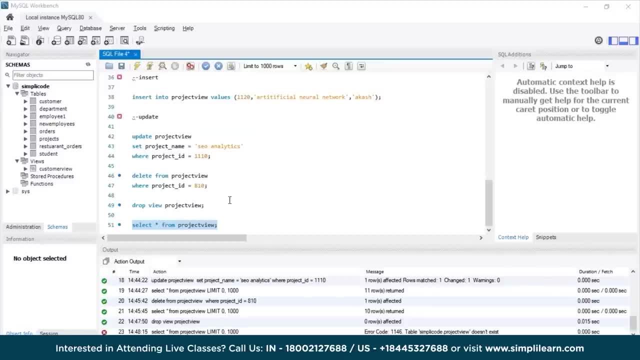 Printes to the end of right session. guys, I hope you understood how to create of you in SQL. now you might have a doubt that when to use of using SQL now, since views have both advantages and disadvantages, the question arises when to use them right now, for instance, if you remove an attribute or if you actually delete a table. 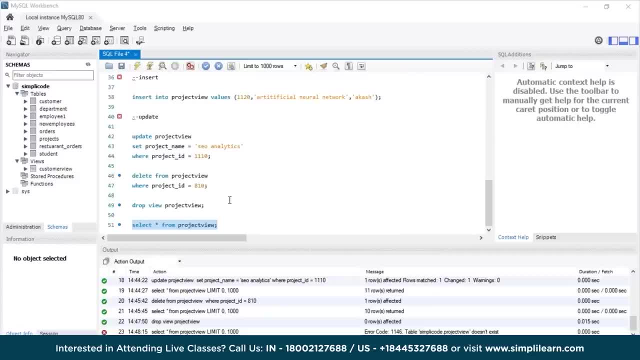 it can impact the functionality of a view as well, just like in a related table. for instance, if a view is using the email column of a table and you drop that column or even a single data of it that isn't used by the view, the output of the view will be impacted. now the short answer. 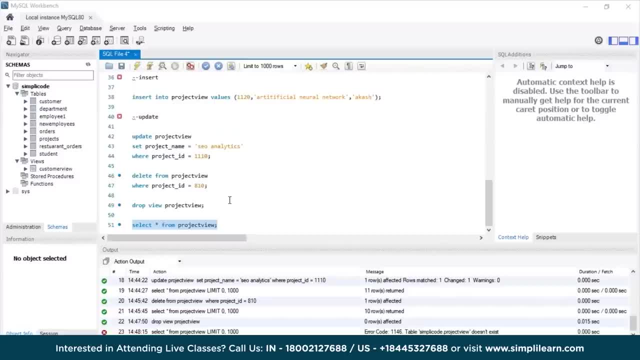 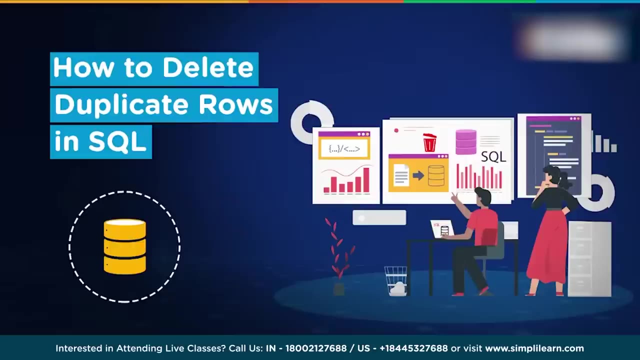 to when to use views in sql is when you want to write complex select queries that require gathering data from multiple tables. in that case, you can use sql views. in order to understand how to delete this duplicate records in sql, let us jump straight into mysql workbench for execution part. 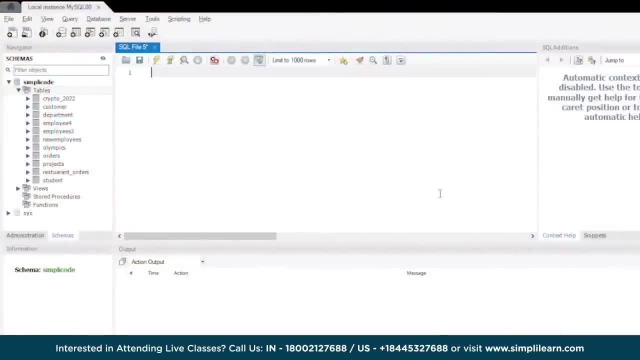 so i hope you are able to see the mysql workbench window and, as you can see, the mysql workbench has started- and on the left side, you can see the simplicode database, where we have different tables, such as crypto 2022, customer department, employee 4, employee 3, and so on. right now, before we get into the execution part, wherein 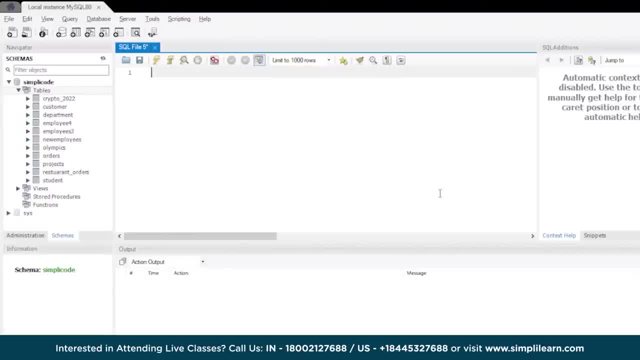 we'll discuss how to delete the duplicates in sql. let us understand why there are actually duplicate records in sql. now, as you know, sometimes you might see more than one copy of the same record appearing in your mysql database table. now, this usually happens after importing data from external sources, such as spreadsheet applications like excel, or from external 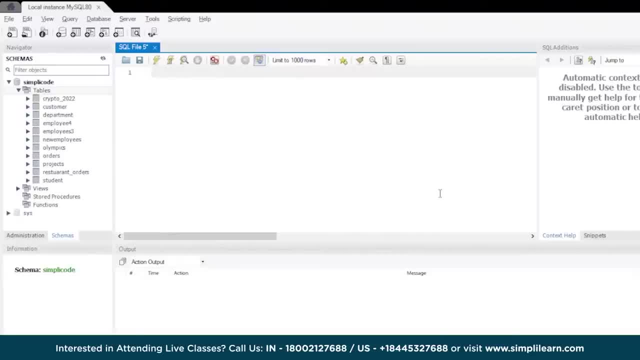 websites like kaggle and etc. which do not have the features of relational databases right. so having this identical copies of the same record may negatively affect your application and your business logic. so to overcome these challenges, you must need to delete the duplicate records from your table now only. 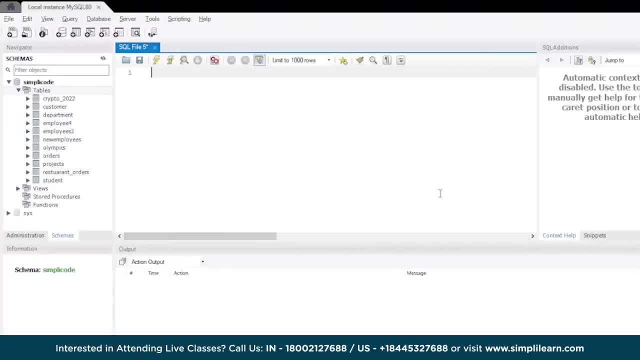 rarely you will find to remove duplicate entries from a table, because the tables in these databases generally have this constraint, such as primary key or unique constraint, for instance. so if we add all of the to prevent these duplicate entries occurring in the first place, but due to some mistakes or the 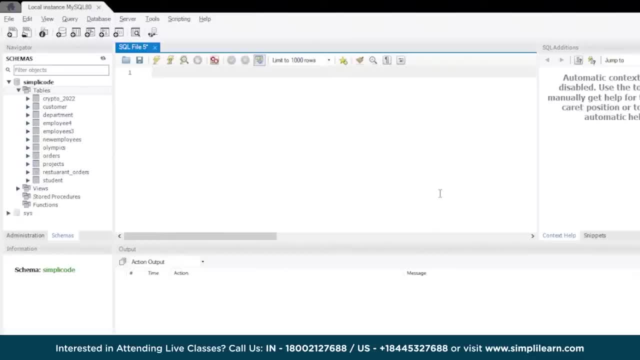 duplicates can get into properly a design table wherein this is due to changes in the business side, where, after merging of two or more different systems or data from two or more different tables will have this duplicate data in our tables. so in this session, uh, we'll look at some of the ways to 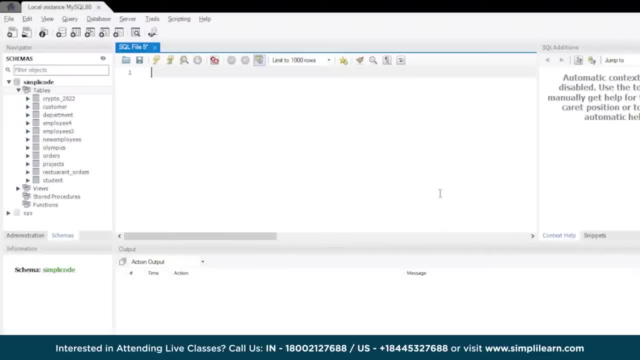 remove duplicate records from the table in sql. right? so i've already created uh tables and inserted some values in it, as well as some duplicate values also. so let us consider uh. firstly the employee 4 table. here let me just display the records, so use the select statement which is select star from employee 4. 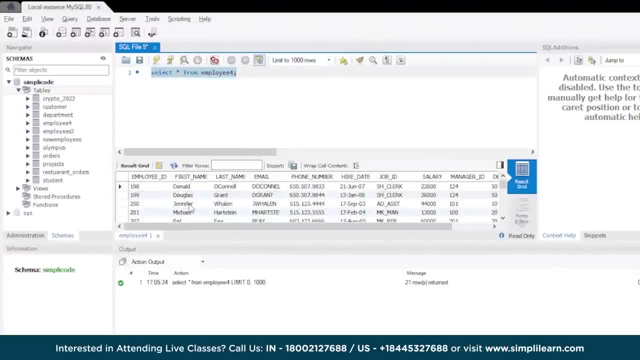 so let us execute this statement and we'll see the output right now. employee 4 table has various columns, such as employee id, first name, last name, email phone number, hiring date, job id, salary manager id and, finally, department id. now there are different ways to delete the duplicate records, so we'll 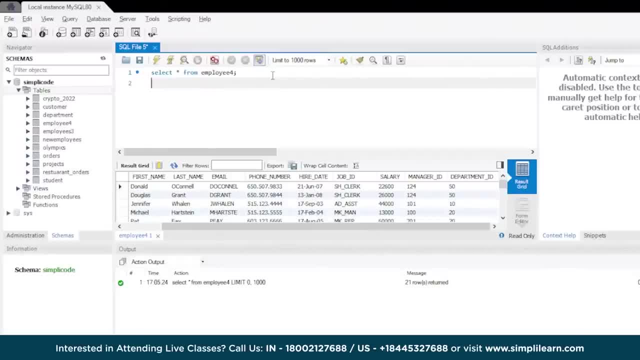 discuss uh one by one each. so firstly, we can delete the duplicate records using the group by and having function. so let us understand the syntax first. now, before we get into the execution part, you'll have to understand how to uh fetch the duplicate records from the database table right. so for that we'll use the following query as select: 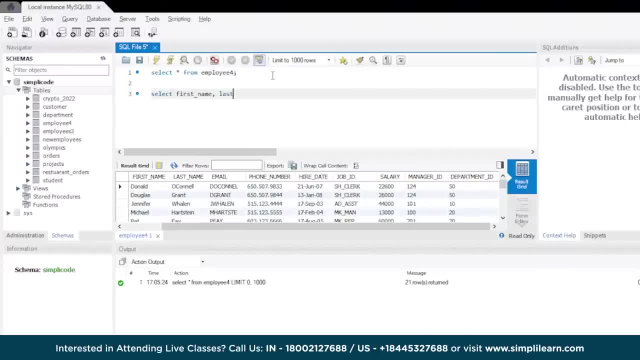 first name, comma, last name, which are basically the columns, and i'll use the count function which will basically count all the duplicate values that are present in our employee4 table. mention the table name and we'll use the group by function, group by mention the column names. 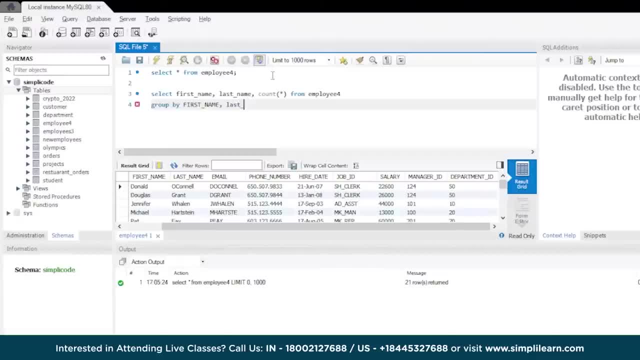 you want to group, which is good, which is basically the first name and the last name. right having count. mention the star operator greater than one: right. let us now execute the statement and we'll see the output. so, as you can clearly see, in our resultant set we have a total of five. 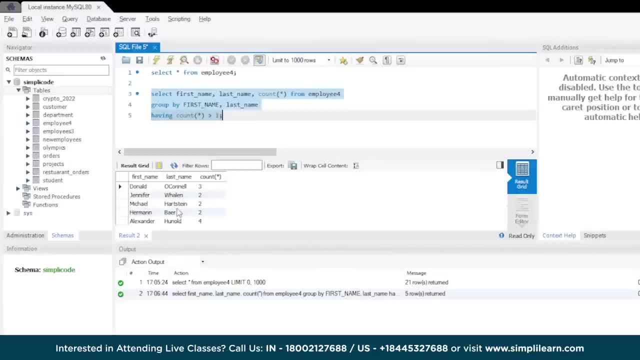 records such as donald o'collan, jennifer vallen, michael hastein, herman behr and finally alexander hundt-holt, where the records in the employee table have been repeated. For example, Donald O'Colin records have been repeated three times here. 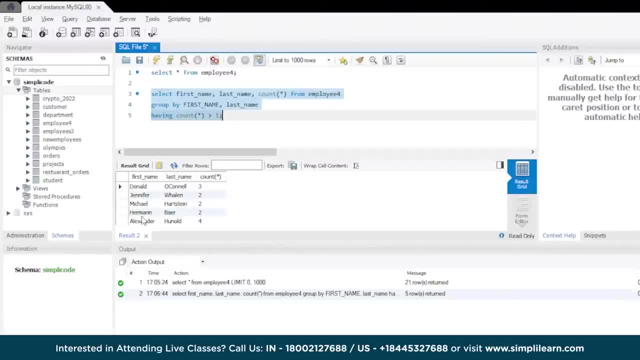 And similarly we have Jennifer Valens two, Michael Hatton's two times again, Hermann's Bayer's also two times and finally Alexander Horner's also four times. Now that we have understood how to find the duplicate records that are present in our 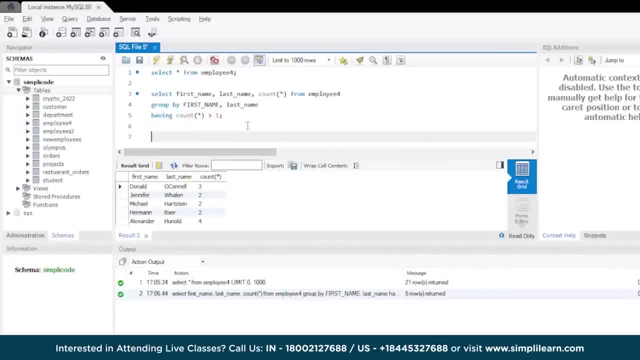 table. let us now understand how to delete Now the query, for that would be delete from mention the table name, which is employee four, where employee ID not in. So let us first understand the syntax, then I'll clearly explain how it actually works. 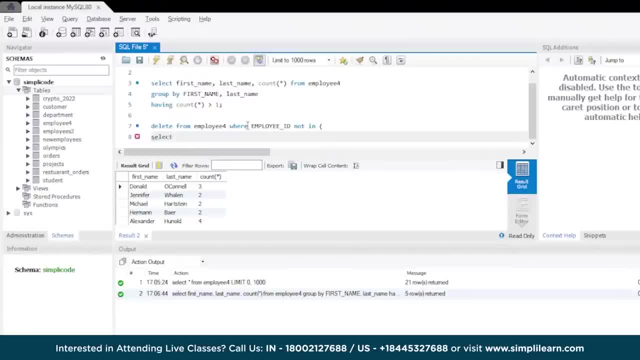 So select which is a subquery. now Use the max function. Okay, Mention the employee ID column name, Close the parenthesis from employee four and you can use the group by function as well. So we'll group by the first name and the last name here and close the brackets right there. 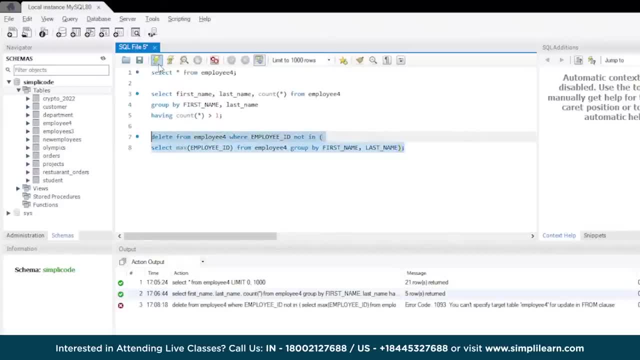 So let us now execute this statement and we'll see the output. There is an error in the code. It says you can't specify the target table- employee four- for update in from clause. Well guys, I think there is an issue in the backend. 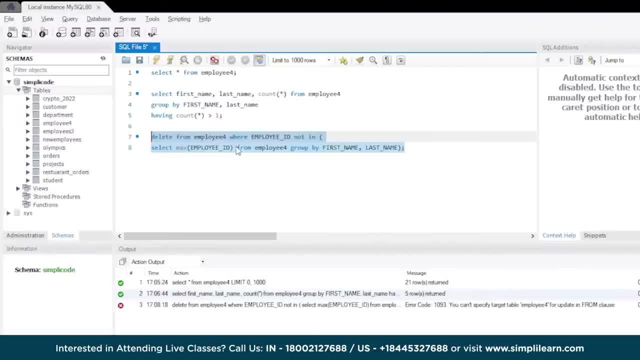 Maybe there's a error in the code, but I think the logic is correct here. So what this query actually does is it basically executes the inner query first, which is it selects maximum employee ID from the employee table right And it will display all those records. 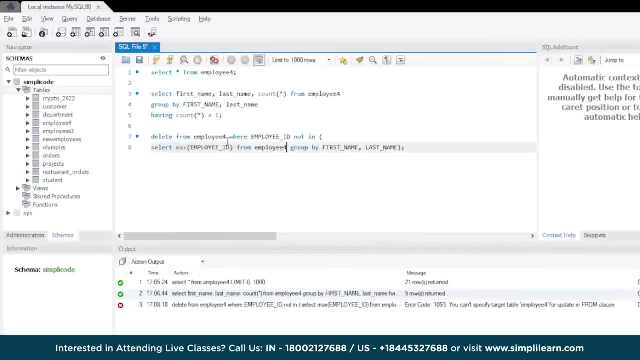 Now it will delete all the records in the employee four table whose employed is not in the maximum value, such as if I have, let's say, one or four is the maximum value, And if I have one or one, one or two or one or three, which are basically the duplicate. 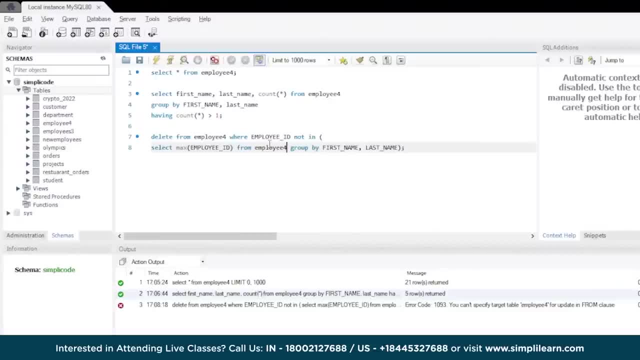 records. So it will basically delete all those records, right? So this is how it will delete the duplicate records in the SQL. I don't know why it is showing error, but we'll get back to you again with the right code. So this is one of the way to actually delete the duplicate rows from SQL using the group. 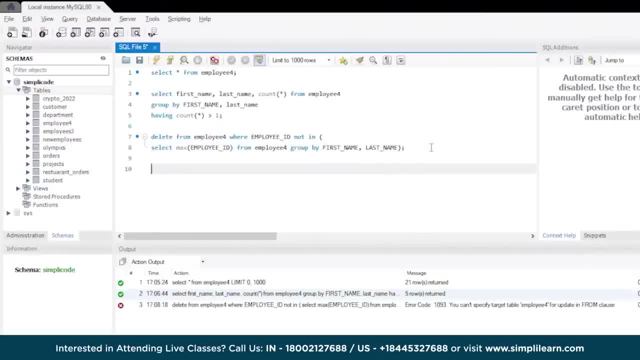 by and having function. So let us now understand A different scenario where you'd use another method. here. We can also delete the duplicate records using the delete joint statement. Okay, So for that the query would be delete. Now I'll first first let me write the query and then we'll understand how the syntax works. 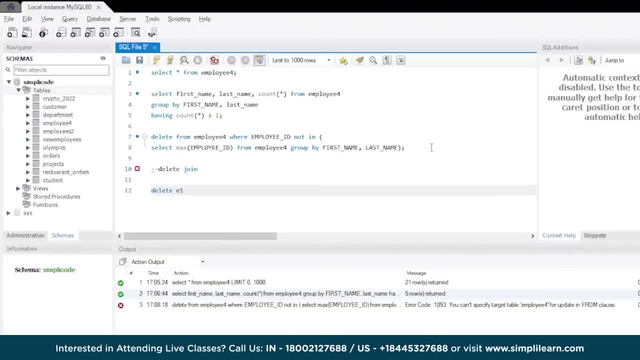 So delete. I'm taking an alias name for a table employee, So I'm taking us even from employee four. Let's see. Okay, So I'm taking an alias name Which is the table right As E1 and I'm joining the table employee four as E2, where even dot employee ID is less. 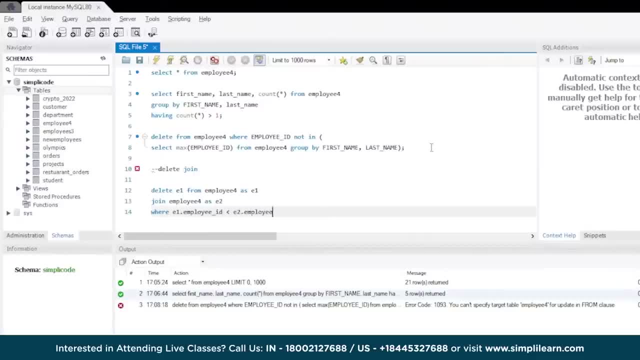 than E2 dot employee ID. Okay, Okay, Okay, Okay, So we are taking this. Even dot First name is equals to P2 dot first name, right? So this is our query now. So let us understand how this actually works here, right? 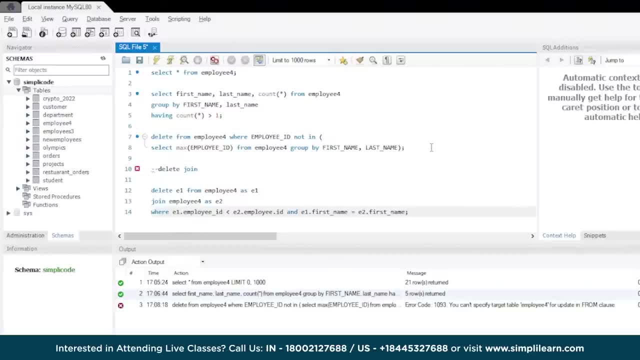 So now, basically, we are, this query is referencing this to employ for table twice and therefore we are using. we'll use the stable LAS as E1 and E2. and E2, and after these, executing the statement will get the following output as so, let us see the output and we'll understand it's showing error, which is: 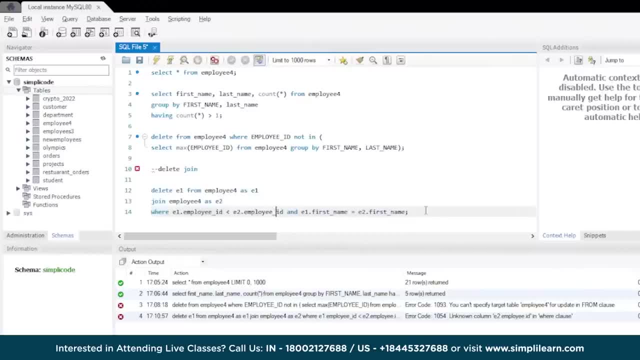 okay. employee underscore ID. it is so. as you can see in our output, our total eight rows have been affected. now let us understand how this query is working right now. I've taken two similar tables here. that is basically one table. I am referencing it twice here, so basically it will delete all the rows which are 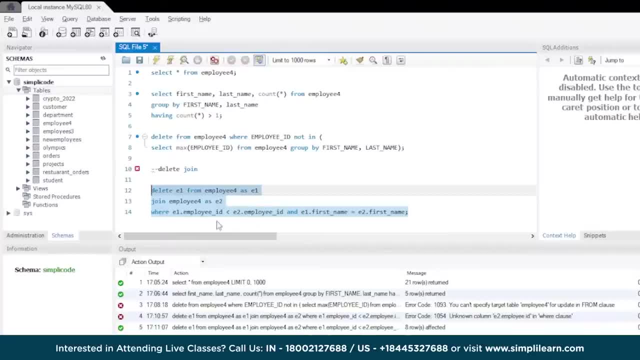 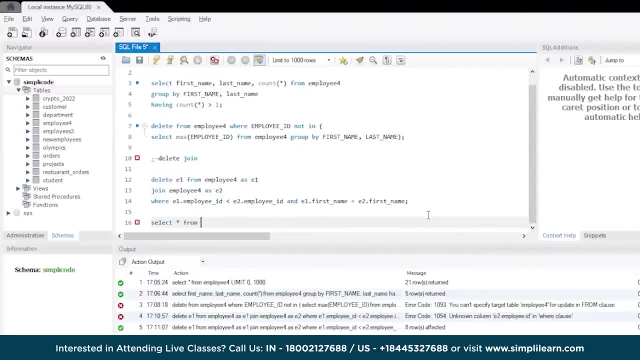 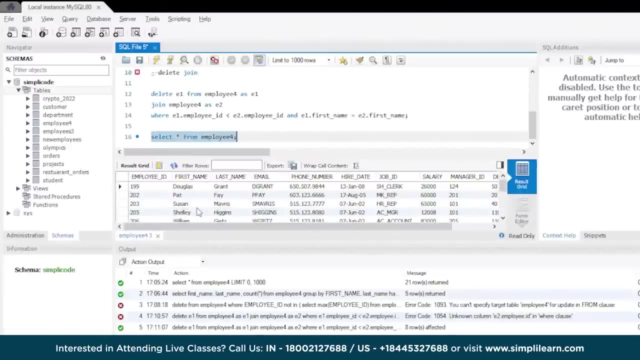 less than the values that are present in the employee to table here. so let me just display the values again so that we'll have a clear idea. select star from employee for table. so as you can see now, previously we had the repetition of certain records, for example Douglas grant. 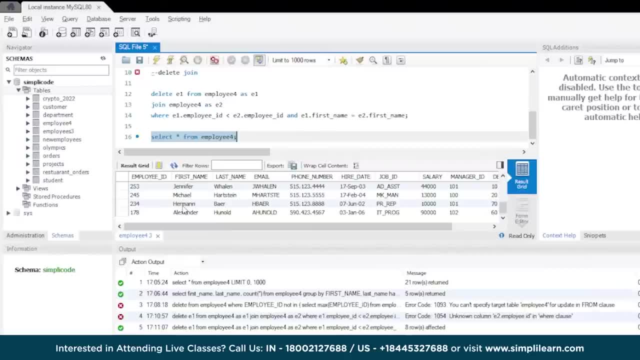 we had and similarly we had, Alexander, who knolled, and for, similarly, Herman Banos. after execute the statement, we have only a single record where all the existing duplicate records have been successfully deleted. so in this way, you can use the delete join statement as well to delete the duplicate records. 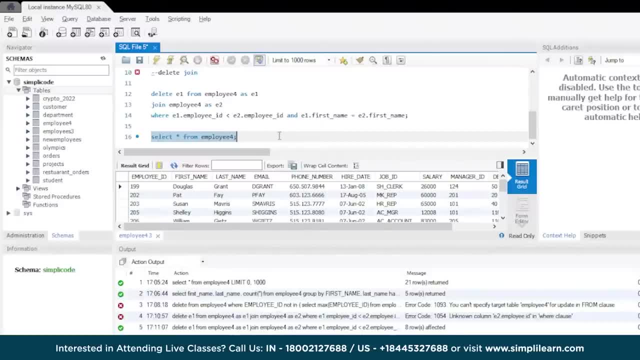 from your table. now let's know. the next method to delete these duplicate records is using the row number function. now, row number function is basically a SQL ranking function, guys, that will assign a sequential rank number to each record in a partition. now, when this SQL row number 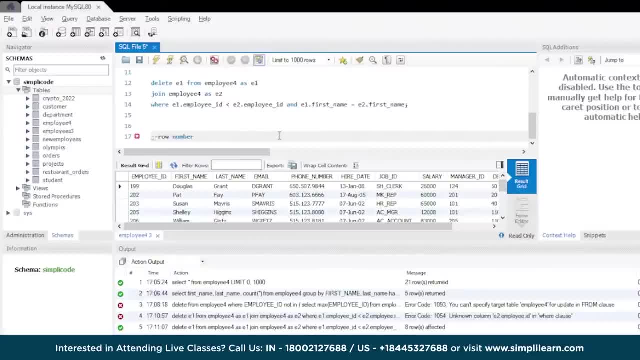 function detects any two identical values, or let's say duplicate values, in the same partition. it assigns different rank numbers to both, and this rank number will be determined by the sequence in which they are being displayed. I know this might sound a bit confusing, so let us understand the query and see how it. 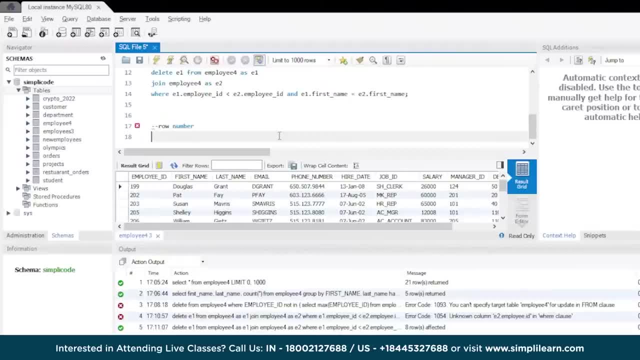 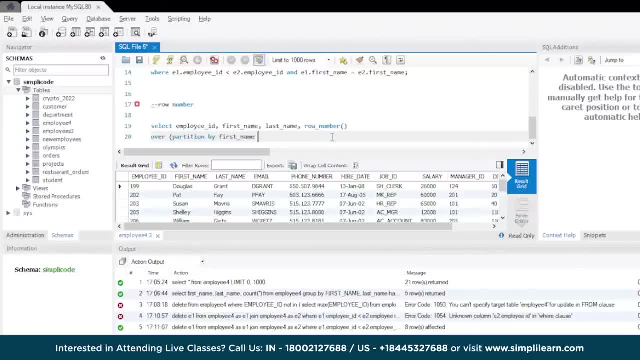 the first name here, right so mention the column name as first name, and similarly we'll also mention the order by clause. mention the first name again, as now, let us give an alias name for this. let's say we'll take it as row underscore num. mention the table name. 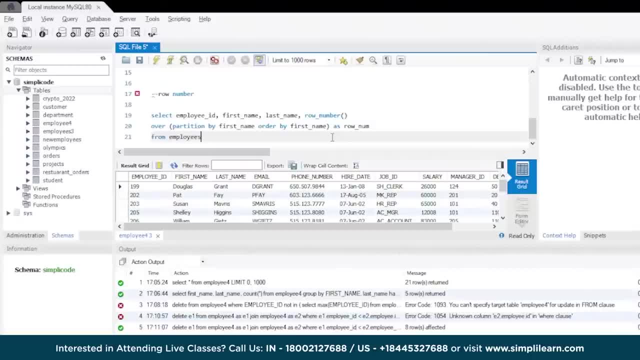 that is, employee employees. so let us consider another table here, which is employees 3, right? so this is our query. so let us understand what exactly the syntax is all about. now we are using the over keyword here, which basically is a clause which specifies the windows or set of rows that the window function. 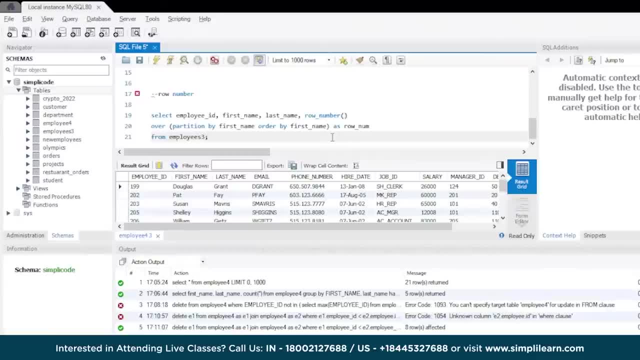 operates, and the partition by an order by are the two possible clauses of the over clause, and next we have the partition by keyword, which is an optional clause in the row number function. it is basically a clause that divides the result set into partitions. now, the row number method is then applied to each partition, which. 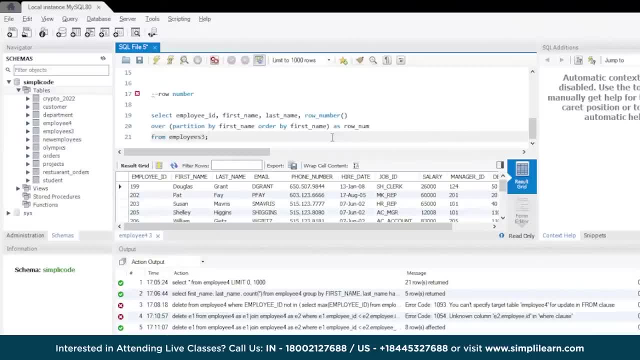 assigns a separate rank number to each partition and if the partition by a clause is not specified, the row number function will treat the entire result as a single partition and rank it from top to bottom. and finally, we also have order by clause we are using here, which is the clause 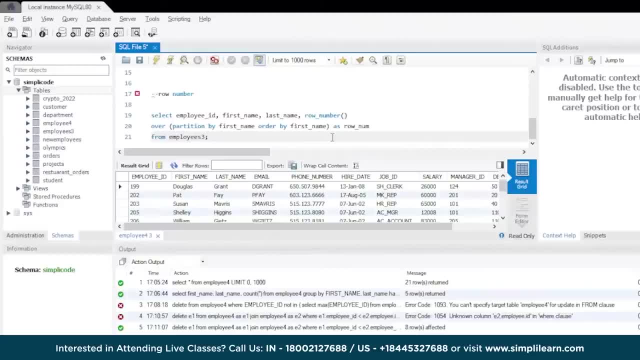 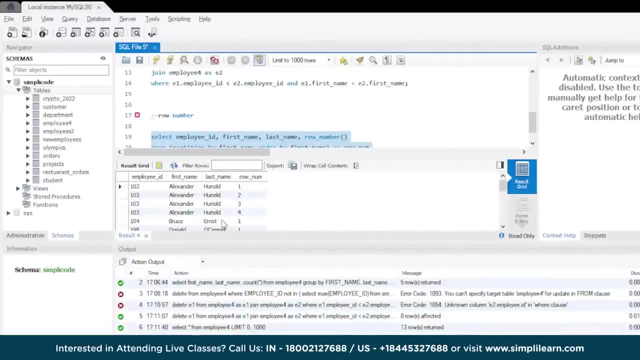 it allows the allows the user to order the rows in the result and set, So I hope you've understood this. So let us now execute this statement and we'll see the output Right Now. as you can see, in a result and set we have. 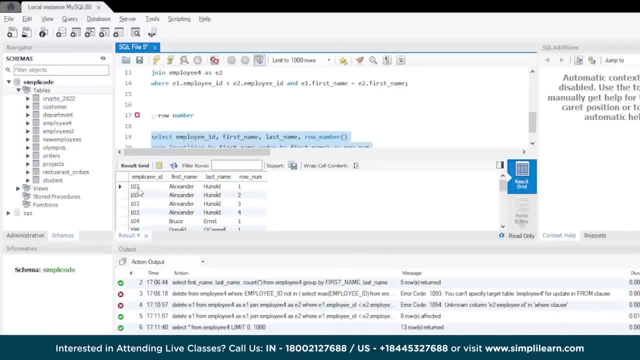 details of an employee, Alexander Hunold, whose employee ID is 103 here, which has been repeated for four times here. Right? So in this way, the row number function will assign values in a sequential manner, starting from one, That is one, two, three, four, That is basically four different. 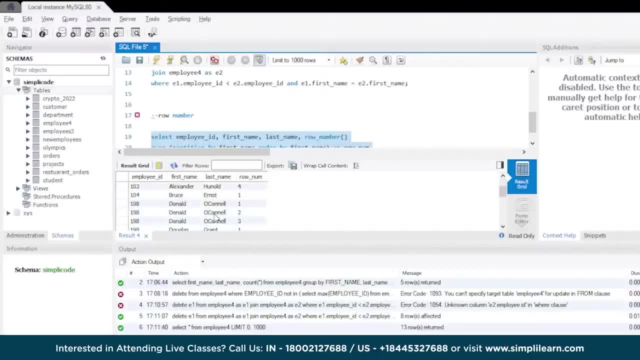 values. Now again, we do not have a repetition of this value, So again it is mentioning or it is assigning one as value for the next record. Now, similarly, we have Bruce Ernest as only one record, So we have row number as one. Now, next we have Donald O'Connell, whose records are again: 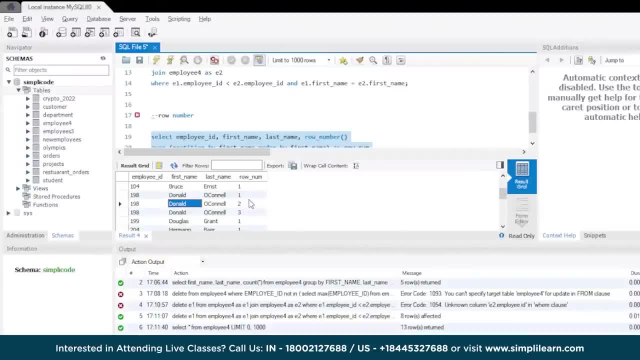 repeated thrice here. Right You can see here. So the row number function assigns the values as one, two, three. So similarly, for all the rest of the records that are present in the table, it assigns the value in a sequential order. 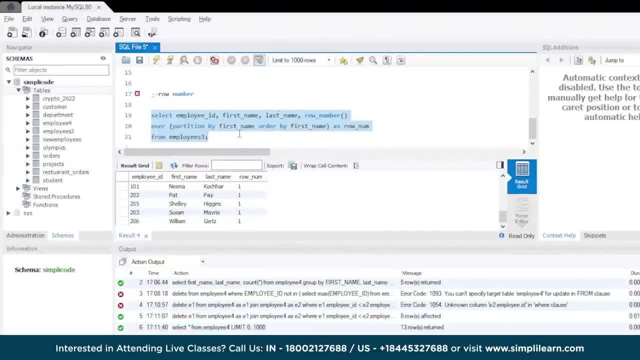 On the number of times it has been repeated. So, now that we've added the partitions and the row numbers to the result and set, let us now understand how to delete these duplicate records Now. the syntax for that would be: delete from Sorry, delete from employee three. 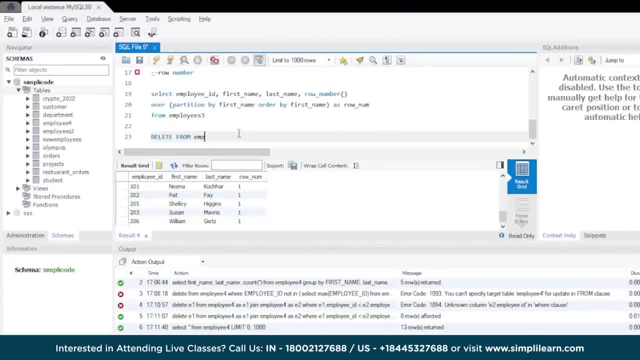 which is the table name. Employee three where employee ID in. Now, within the parenthesis, we'll write a subquery here which is basically select all the employee IDs From mention another subquery here, which is basically the previous query that we have. 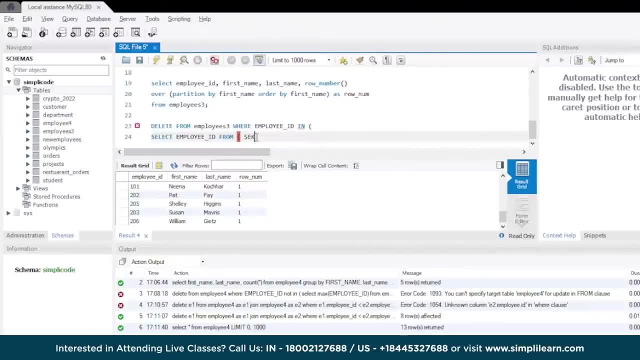 written here, So we'll just write it again. Select employee ID: first name, last name and mention the row number function over Partition by is the keyword First name. Again, we'll use the order by clause for the first name again And we'll give an alias name for this sub table, which is Ronam From. 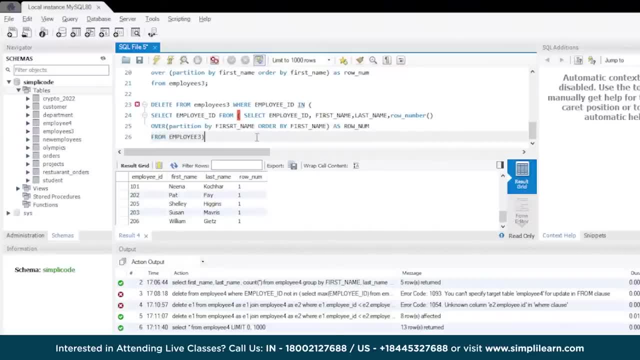 here we'll write employee three table And for this outer part of the query we'll give another temporary name, Let's say temp table, where row number is basically greater than one. So what this query does is is basically it will check all the values and it will see. 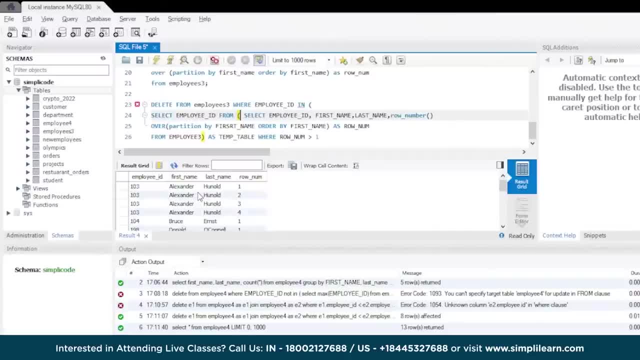 that for all the values, which is having row number greater than 1.. For example, we have for Alexander Hunold, we have row numbers has 1,, 2,, 3, 4, right. So it will remain this the first record as it is. 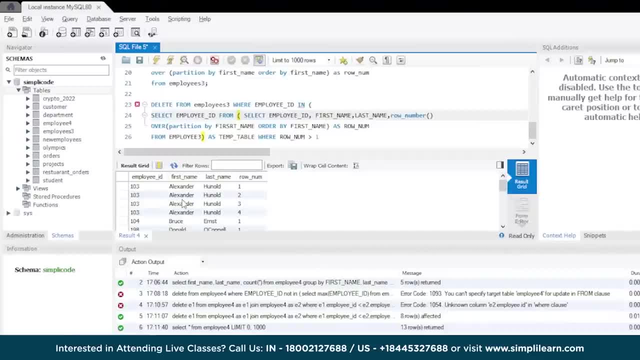 and it will delete the remaining records. For example, the records having Alexander Hunold as row number, function 2,, 3, 4 will be deleted, and similarly for Donald O'Connell- 2, 3- the row numbers will be deleted. So let us now execute the statement and we'll see the output. It is. 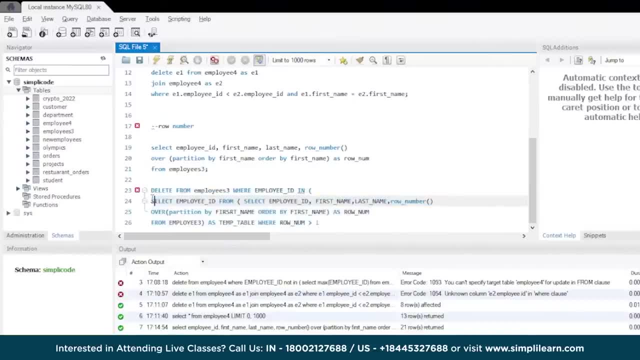 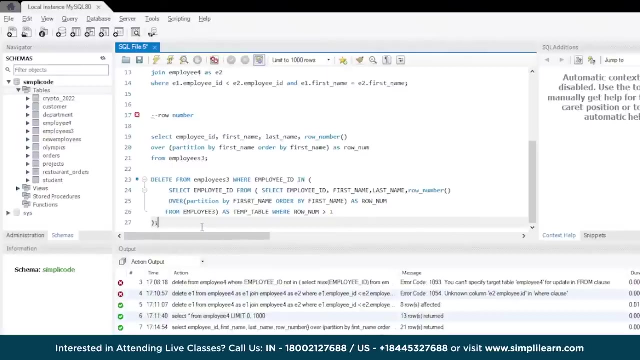 showing an error again, so let me just make some changes. Well, the query is actually correct, guys. I don't know why it is showing the error here. Okay, I forgot to close the parenthesis here, right? so that was my mistake, sorry. So let us now execute this statement and we'll see the output. 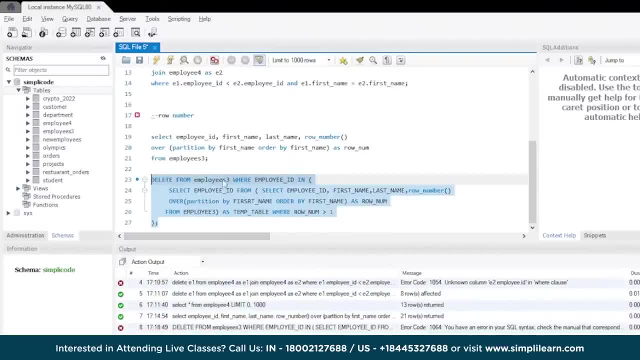 i3. I think the initial table name has been higher, meaning that the return has been wrong, right? So let us execute this statement and we'll see the output. So our query has been successfully executed, guys, and we can see that 13 rows have been have been affected, so let us now use the 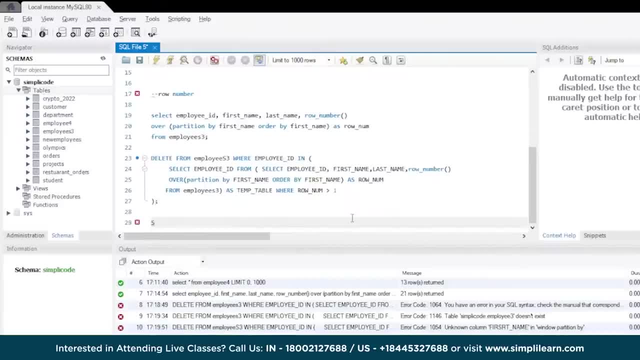 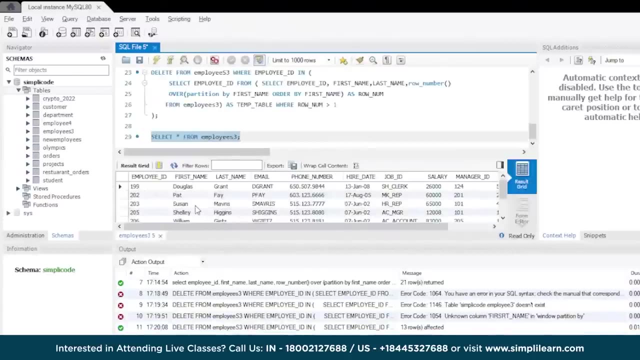 select statement again and we'll see the records where, whether they are not, whether the duplicate records have been not deleted or not. so select star from employee three, table right. so clearly you can see that in a resultant set we have all the duplicate values that have been successfully deleted permanently. so 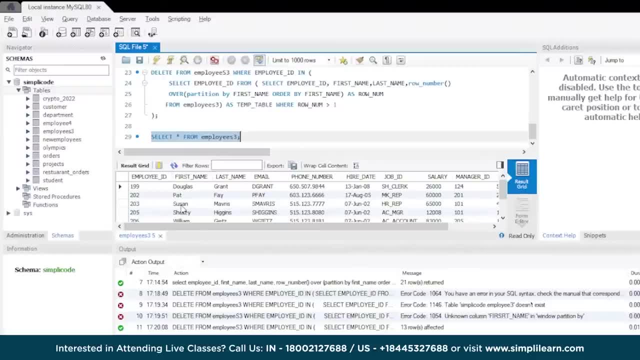 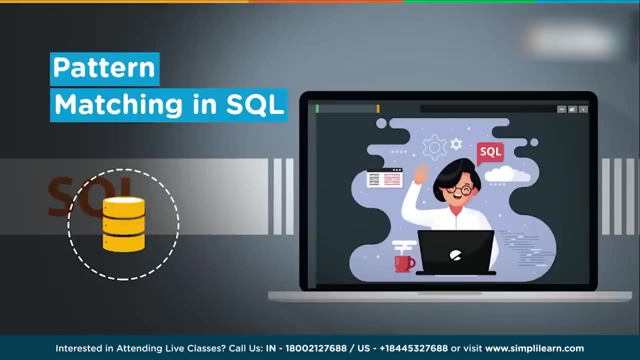 in this way, you can use the row number function as well to delete the duplicate records in your SQL table. so that brings us to the end of today's session. guys, that was all about how to delete the duplicate records or rows from the SQL tables. I hope you understood how to implement this. discussing what is. 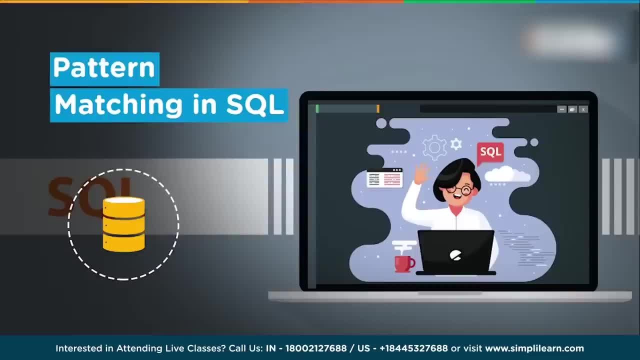 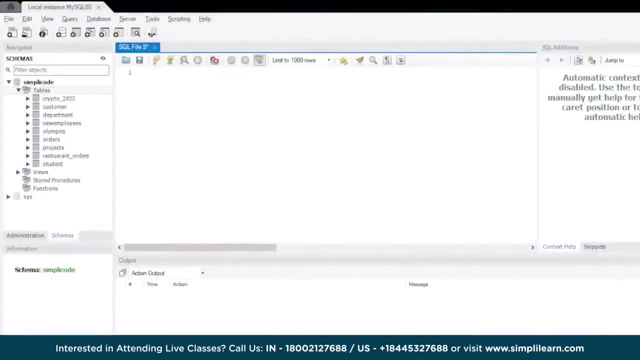 pattern matching in SQL and we'll see how to find certain values in the table using so using some patterns, with the help of some special characters. so, without any further delay, let's get started now. in order for the execution part, let us jump into MySQL workbench. so, as you can see, MySQL workbench has started and, on the left, 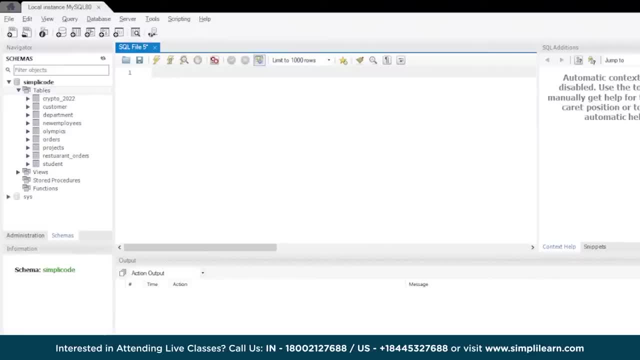 side, you can see the simply code database, which has various tables like crypto 2022, customer department, new employees, Olympics and etc. so before getting into the execution part, guys, let us understand how exactly the pattern matching works. now, remember when you start typing something into Google search bar and it: 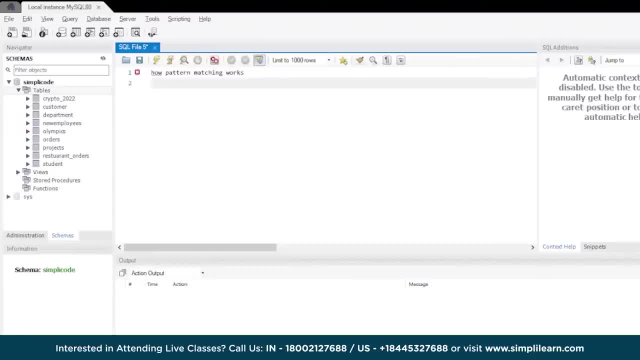 auto completes feature already completes your sentence, right. so what exactly is happening there? so Google is basically trying to accomplish is: what is pattern matching? pattern matching is basically checking whether a specific sequence of characters or token, or a data or the other information that you are looking is existing in the database or not. so let's get started now. let's see how to. 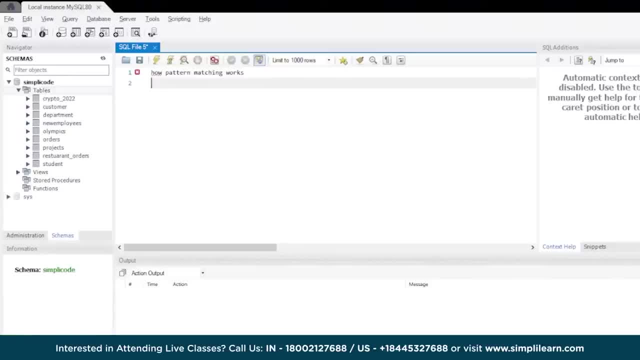 do that, so for that we use pattern matching in SQL. now, SQL pattern matching allows you to search for patterns in data if you don't know how the exact word or phrase your finding is there or not. so this kind of SQL query uses wild card characters to match up. 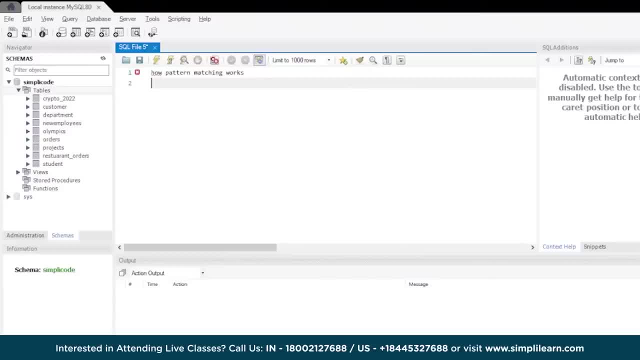 pattern. now the like operator is basically used to find the specific pattern in the tables column. it is also used to compare columns within the specified values. now, together with the where clause, it determines if a pattern matches pattern matching or not. but it will take time and time to gepr. 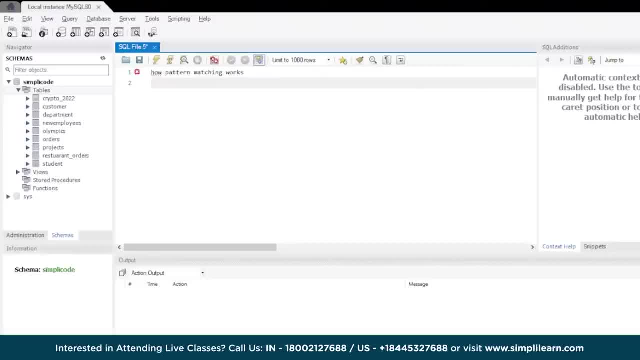 specific values in a table. It also uses some special wildcard characters, such as the like percentage, as well as the like underscore operator to find the specific pattern. So basically, the like percentage sign is used to represent zero or more characters and the underscore sign is used to represent exactly one character Right. To get a clear picture. 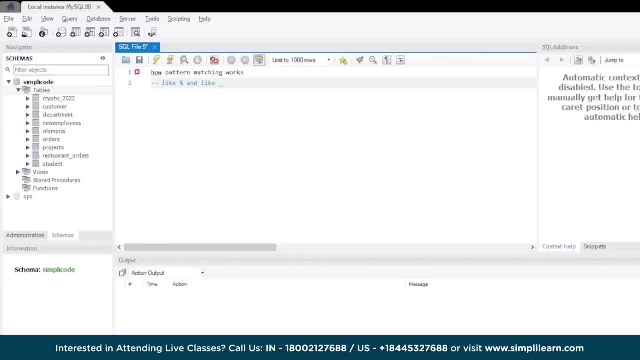 of both these operators using the special wildcard symbols. let us look at some examples and see how they are executed and how it will return the values. So for that, let me just switch to another tab and let us consider the Olympics table. to perform operations using 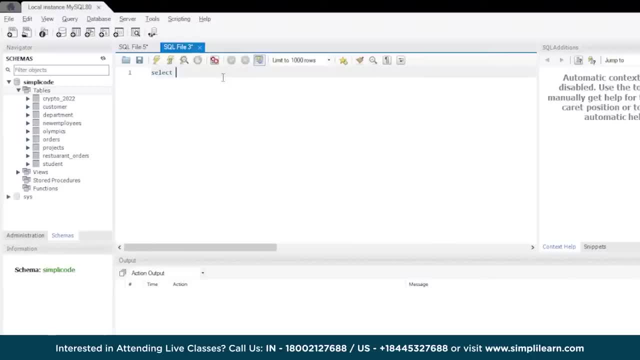 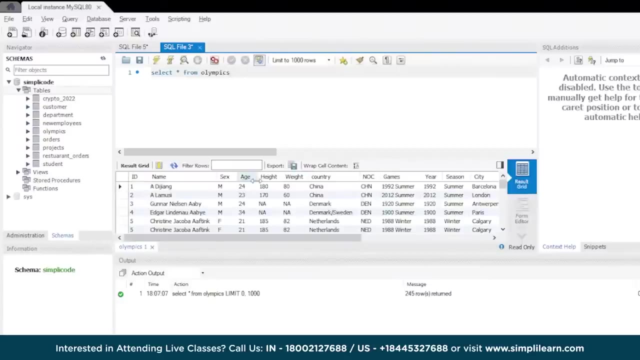 the pattern matching in SQL. So let me just display the results from the Olympics table. So I'm using the select star from the Olympics table. Okay, Right. So the Olympics table has various columns or fields, such as ID name, sex, age. 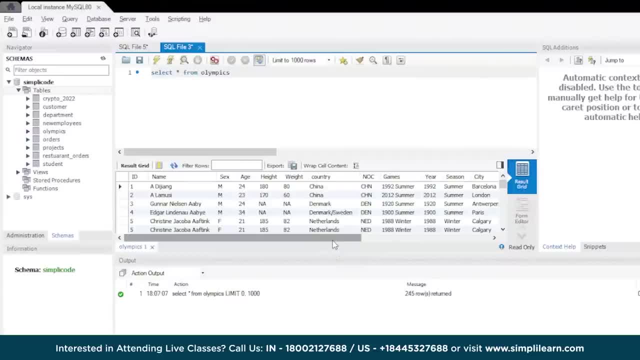 height, weight, country, NOC games, year, season, city, sport and event And also the medal that they have won. So firstly, let us discuss some examples using the like percentage operator guys. So, as we discussed earlier, like percentage operator basically returns. 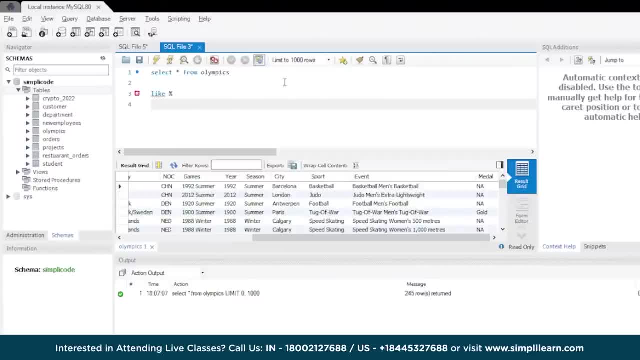 one or more characters having certain patterns that we want to see. We have mentioned in the condition in our query. So let me just take a first example here and we'll see how it gets executed. Now, let's say, if I want to fetch details of all, 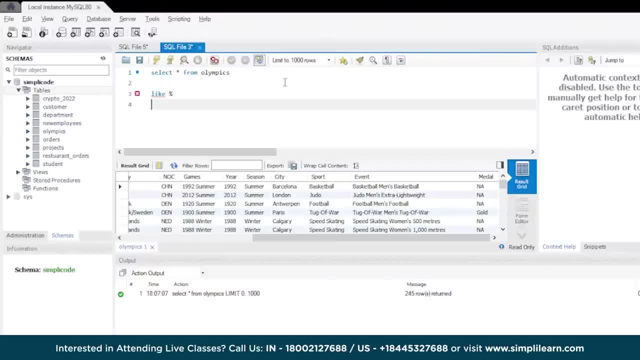 of the athletes who have participated in the Olympic games whose name starts with S. So in that case, the following query would be: select star from Olympics where name like and within the single quotes you have to mention the character that you're. 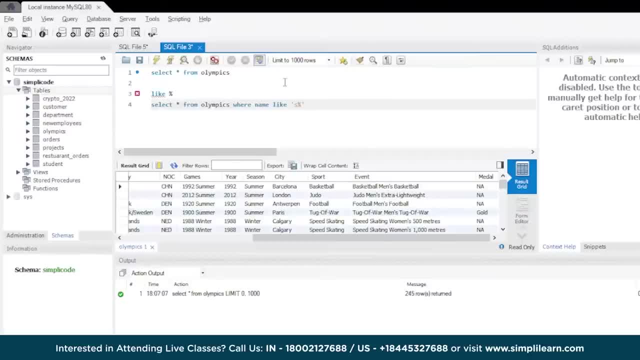 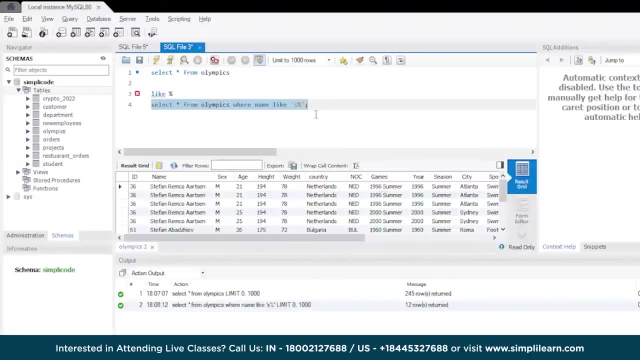 searching for which is s and mention the percentage symbol. so let us just execute this statement and we'll say the output. so it will basically display the results of all those uh athletes who have participated in the olympics whose name starts with s. so if you want to further uh, write a. 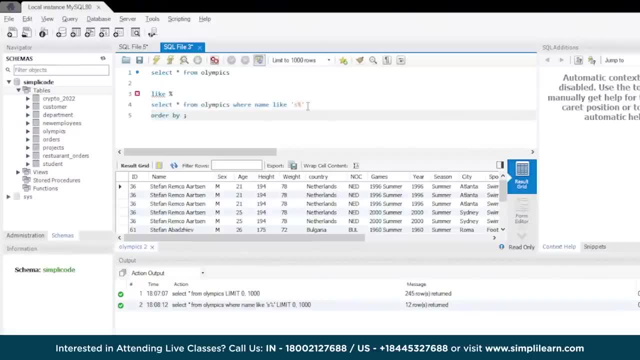 query in order to display in ascending order. you can use the order by function as well, so i'll use the order by name. so this will basically uh represent all the names starting from s and also the second character, uh, which will maintain the ascending order, like, if you see, salim abinosh and. 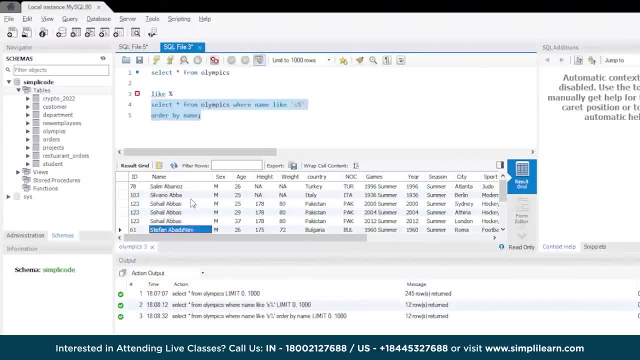 next we have silvano abba and so on till stephen anthony base, right? so in this way, if you want to display only the results using the first character, you can use this. next, let us just uh discuss another example. now you can use multiple characters also to find the patterns, uh, in order to fetch the data. let's say: 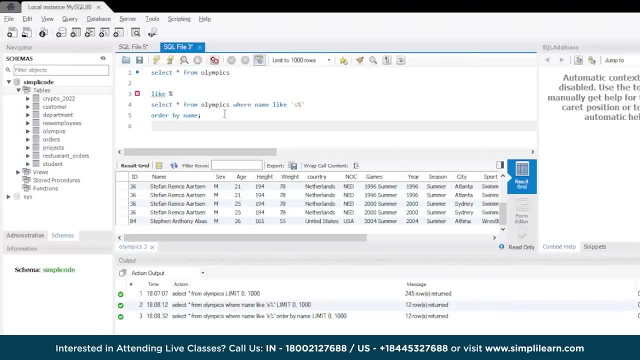 if you want to retrieve the details of all the events. uh, in the olympic games whose name starts with, let's say, s a. so in that case we'll be using the query as select star from olympics where event like s a person. so let us execute this and we'll see the output. 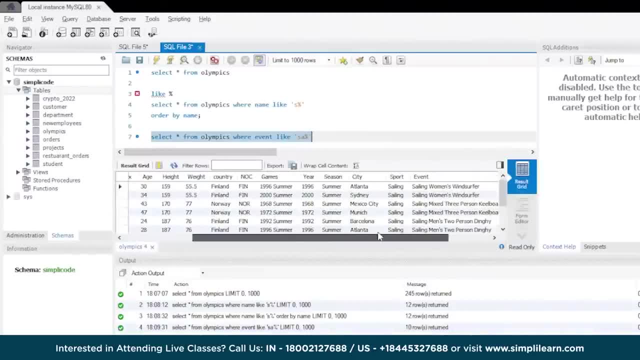 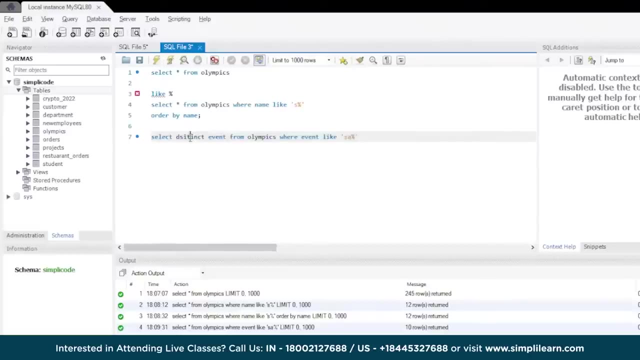 so we were talking about events, right? so we have events here, like various events. so let me just uh use the distinct so that we'll have only the events name, select distinct event and we'll see the output. so, as you can see, we have a total of 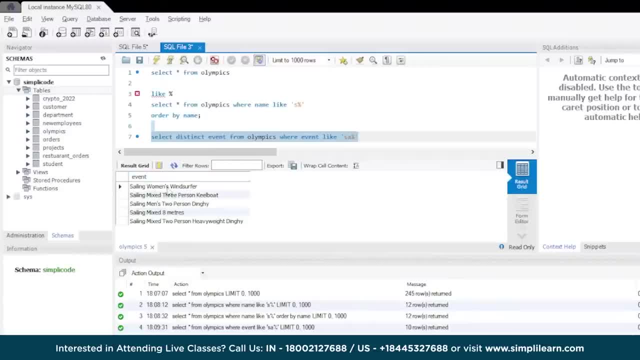 four events. so let's do this. so we're going to do the output. so let's do the output, so let's do the five records. that starts with the characters SA, like sailings, women's windsurfer, sailing makes three percent, keyboard, and so on. so in this way, if you know the first two characters of the value, 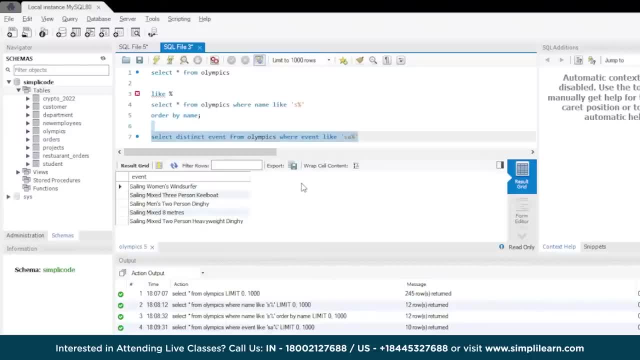 that you want to search, then you can use the percentage operator with by mentioning the first two characters here. that is, we have taken SA here, right, so let us move to the next query. uh, let's say, if you want to display the names of all those employees- sorry, all those are athletes in the 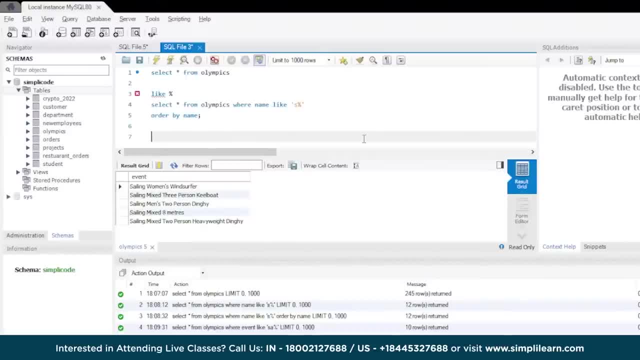 olympics table whose name ends with letter or the character in. so in that case you use the query as select star from olympics where name, like now. in order to get the details of all those athletes whose name ends with them, you have to first mention the percentage. 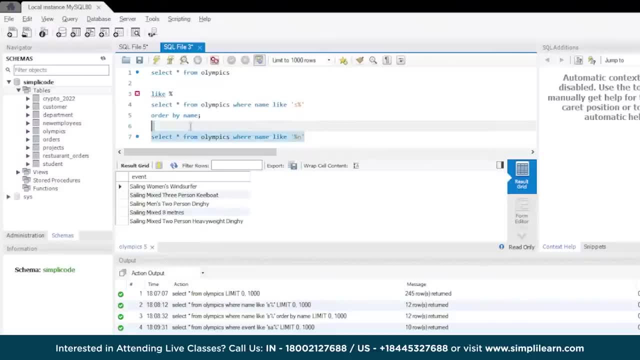 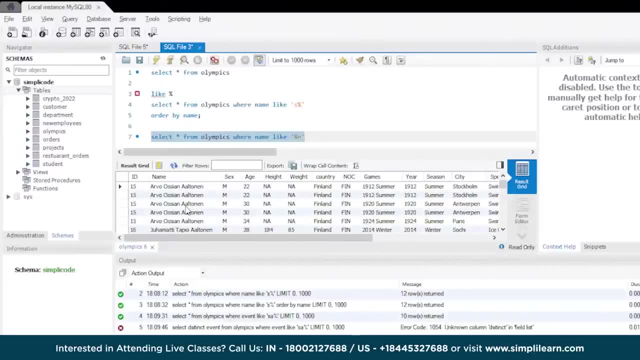 and then mention the character that you're searching for, which is basically in right. so we'll execute this query and we'll see the output. so in our resultant set you can see list of all those uh athletes whose name ends with a like, if you consider arvo, ocean, oilton and similarly, we 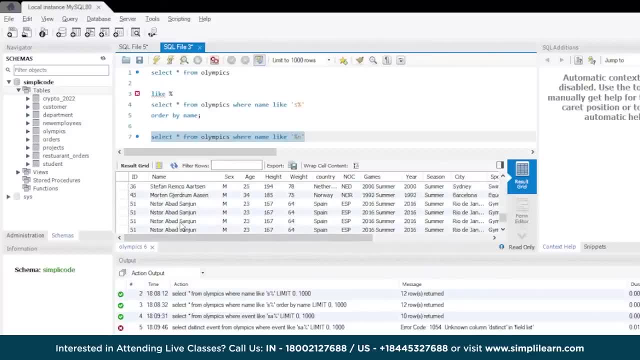 have jumati, tapio altonen. and if you scroll down a bit you'll find all those names of the athletes whose name ends with n. so you can use this uh percentage operator to find the uh names of all those uh athletes in the olympics table that ends with n as well. right moving ahead. 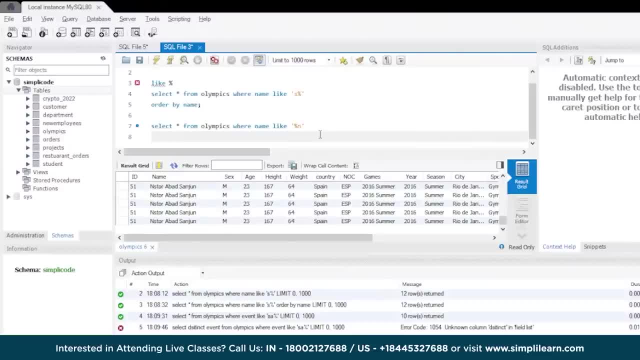 uh. similarly, you can also uh find the names of the m name of the athletes in the olympics table that ends with multiple characters. so now, other than names, let us take another example. let's say, if i want to display distinct uh records of the sports whose sports name ends with ing. so in that case, 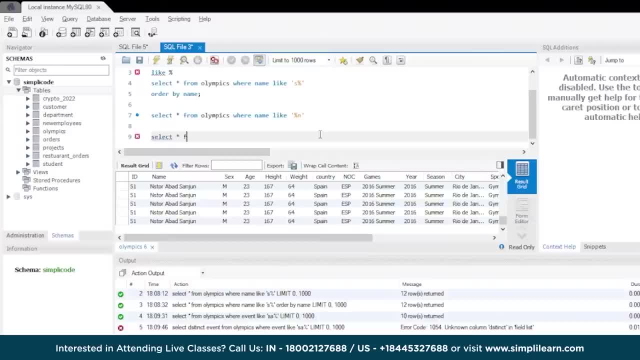 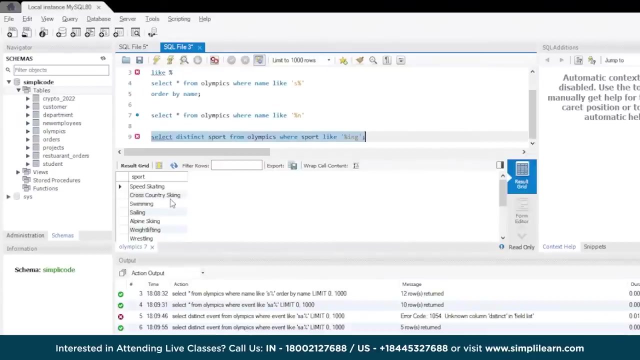 i'll use select star, sorry, select distinct sport from olympics, where sport, like percentage, ing. so let us execute this statement and we'll see the output. so it will basically display the records of all those sports played in the olympic games, which ends with the characters ing. so no matter what it has in the starting places, it should end: 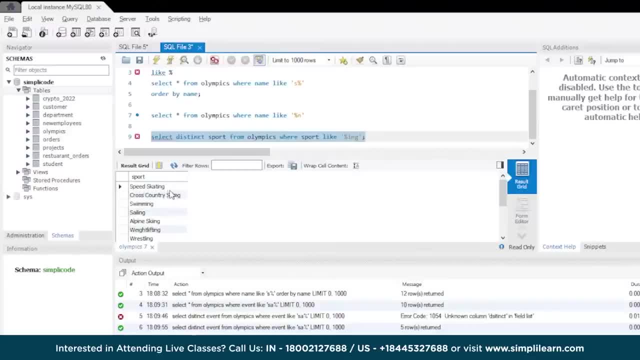 with the ing characters. so we have various sports like speed skating, cross country skiing, swimming, sailing, alpine skiing, weightlifting and finally, wrestling. oh sorry, we have more than uh that. so basically it displays all those uh sports which have ing in the last place. so i hope you've. 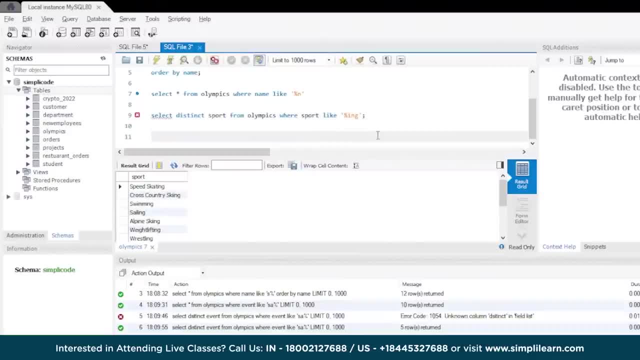 understood this uh. so let us now understand another scenario where we'll use this percentage. now, if you want to uh display the records of all those uh athletes, who's who have i or k, let's say ik- in any particular order in their names, so in that case you'll use the following query as select star: 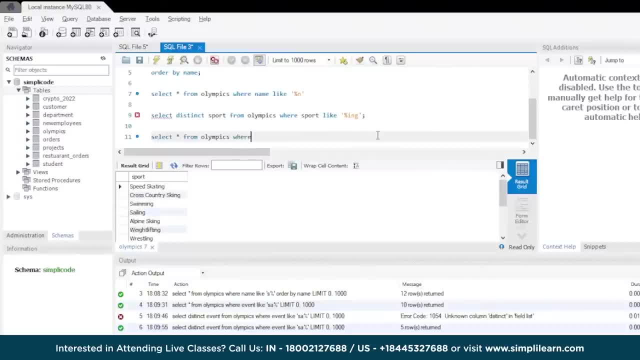 from olympics, a stable name where name like, so the name can start with any character. so i'm using the percentage. now it should have only ik in between their name. so at any positions and Finally I'll enclose in with the percentage so it can be in a second, third or you can say fifth six. 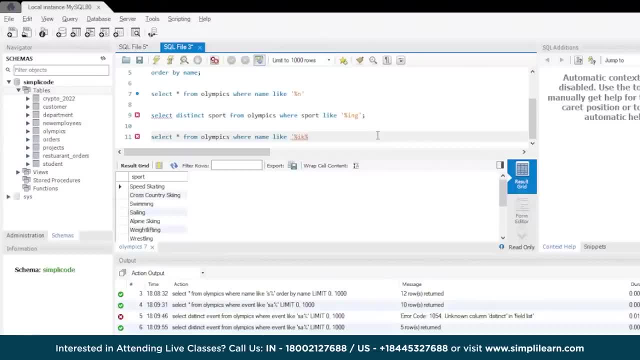 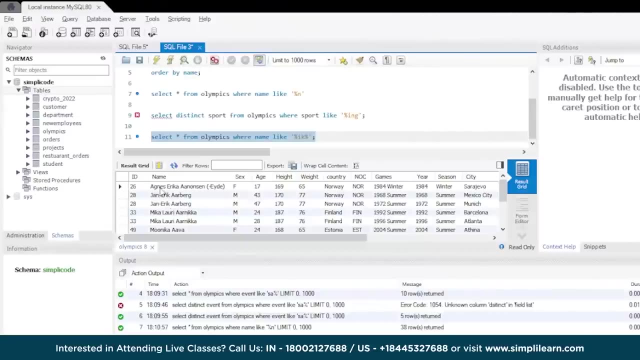 But basically it should have IK characters in the name. So let us just, For what to mention a single code. So let us execute this statement and then we'll see the output Right. so, as you can see, we have the resultant set which has, for example, you, if you consider Agnes Erica Anacin. 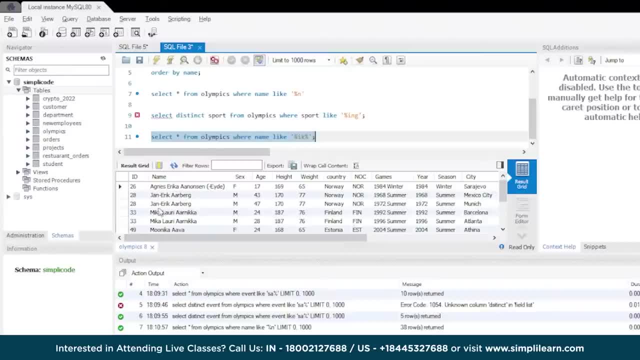 She. she has IK in between her name and similarly Jan Eric. Similarly, he has IK characters in the middle of his name, and similarly we have Mika, Lowry, Aaron, Eka, RV, Alec, Monica, Ava and so on. So even in this way, you can use a different scenario where you can understand and use the percentage operator. 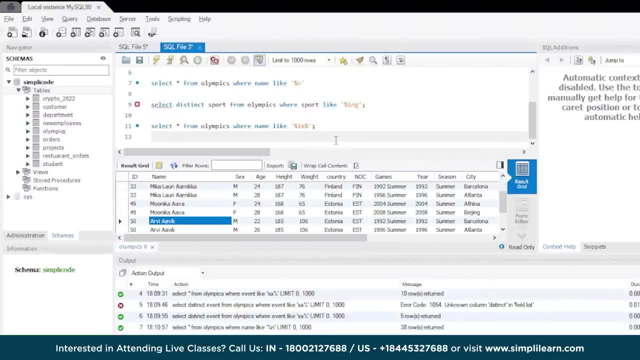 Well, let us now consider another example, guys. Let's say, if you want to display all those countries where the Olympics are, Say so, sorry, are the countries of all the athletes who have participated in the Olympics whose country name starts with C and Ends with a. so in that case, the following query would be: select star from Olympics. 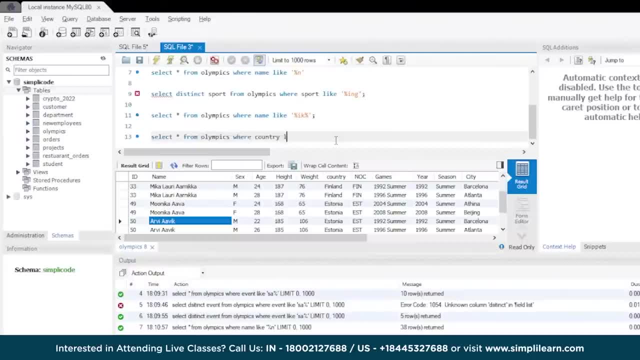 Where Country like, See percentage a. so what is basically does is it will retrieve all the of the countries which has the letter C as its by the first position and A as in the last position, and it can have any number of characters in between. so for that we are using percentage sign. 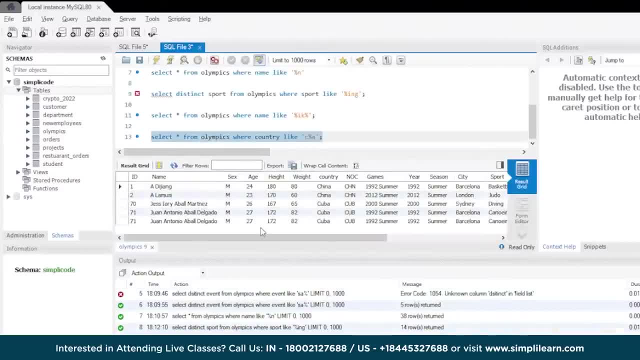 So let me just execute this and we'll see the output. So, if you can see, in our output we have Different countries that start with C and ends with a, so let me just use this thing so that we can have a clear picture. So, as you can see, we have China and Cuba, which are only two countries. 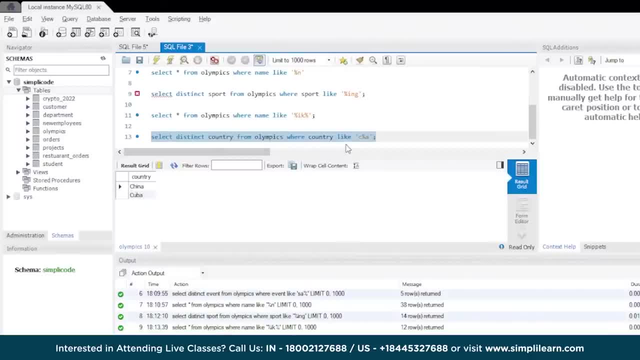 Which have the letter C as it's in the first position and a in the last position as well. So this is another case where you can use the percentage Operator sign as well. So and finally, let us look another example of like before moving ahead with the underscore operator. 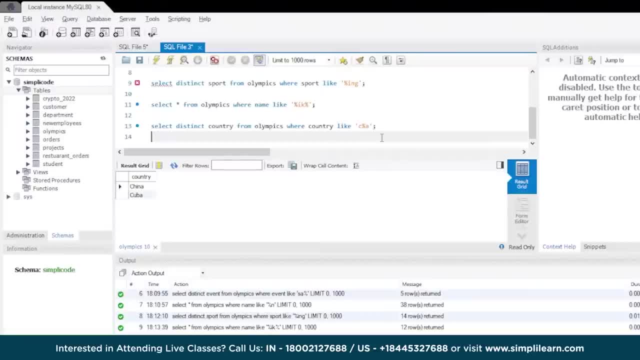 now, let's say, if you want to find the details of all the athletes who have participated in the Games in the 20th century, that is, from 1900 to 2000. So not only the character values, you can even work on the numerical values as well while you are performing like, like operations. 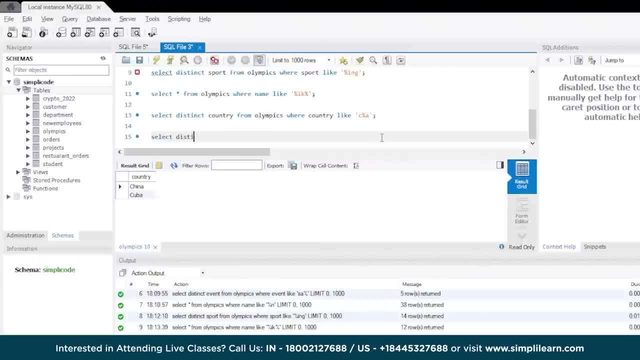 So let me just write a query, So select- I'll use the distinct names because we have repeated values of athletes, so- and also mention the year From Olympics and where Game like 19 percentage. so it will basically display all the records whose The games that were played in the year 19, 9 or 20th century, that is, between 1900 and 2000. 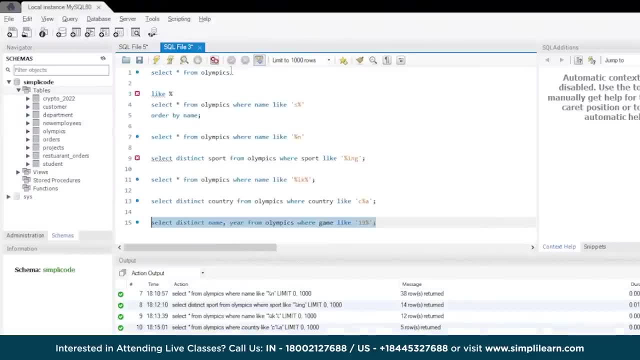 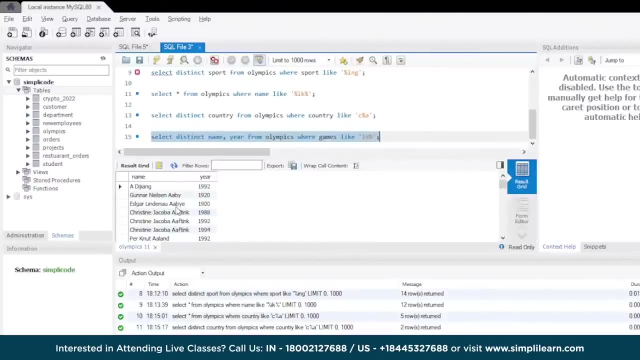 So let us just execute this and we'll see the output. Sorry, I think it's games. the column name is games, So, as you can see, it will display the records of all the athletes who have played various games in this year, starting from 1900s to 2000. so if you want a more, 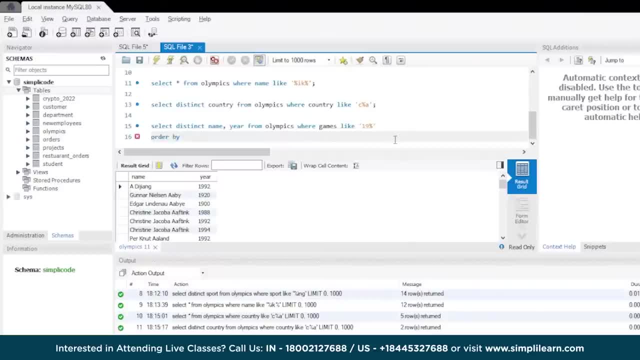 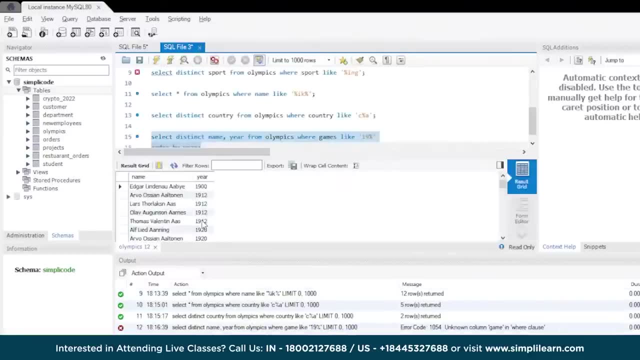 Good-looking query. you can use the order by so that it will sort the result in Ascending order. So let us just execute this. so, as you can see in a resultant set, it is displaying the record starting from 1900 and so on up to 1998. so in this way you 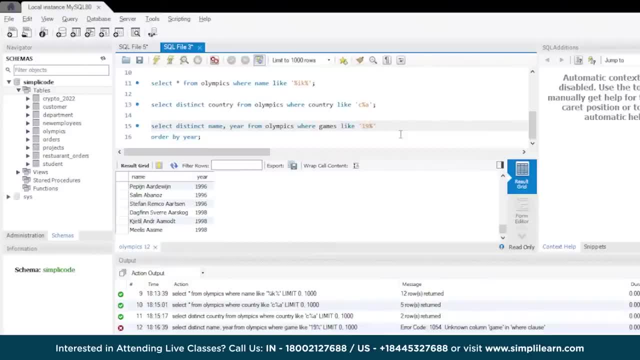 can use the numerical values also to find certain patterns as well, and you can also use the and or operator, and or or operator as well. so let us consider an another example there now. let's say, if you want to face the details of all these athletes who have taken part in various olympic 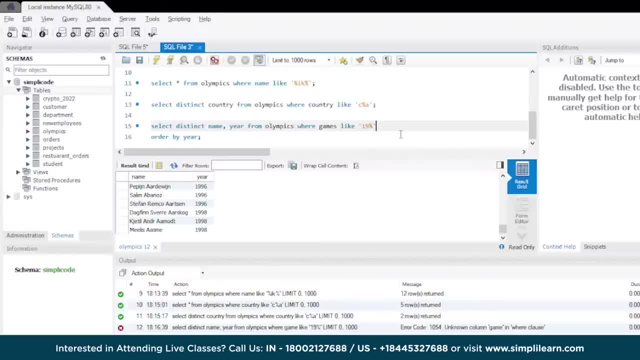 games, be it summer olympic games or winter olympic games, and the sport that they have participated is basically starts with the letter b. so in that case, what we'll do is we'll add game section as well, which is a column mention the and operator and sport like percentage b. so what it? 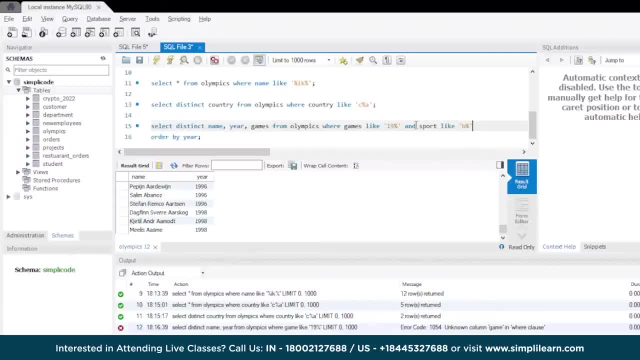 does is basically displays all the records of the athletes who have taken part in all the olympic games, be it summer or winter olympic games in the 19th, 20th century, that is, from 1900 to 2000, and also it will filter the records wherein it will only display the sport which starts with. 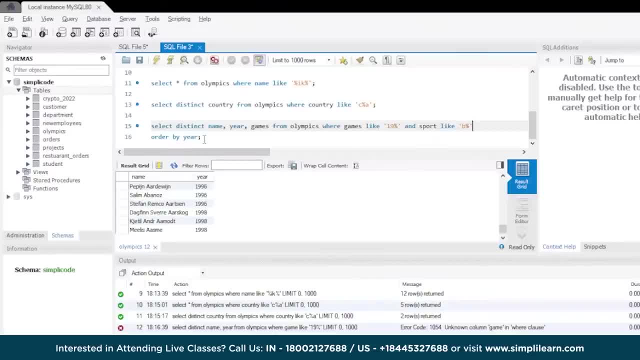 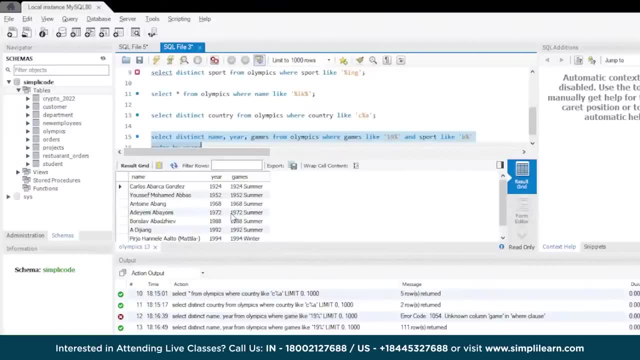 the letter b and similarly we'll do the order by year. so let us just execute the statement and we'll see the output. so, as you can see, it is displaying me the record of all those athletes who have taken part in various games, starting in the 19th, from 1900s, from we have 1924, 1952 and so 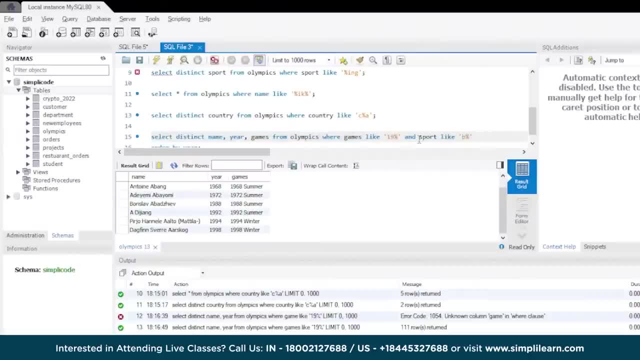 in this way you can use also use the and operator, basically to fetch the records using the percentage operator. so i hope you've understood till now how we use the like percentage, uh, in order to find certain pattern in our values that are present in our tables, to fetch those records. 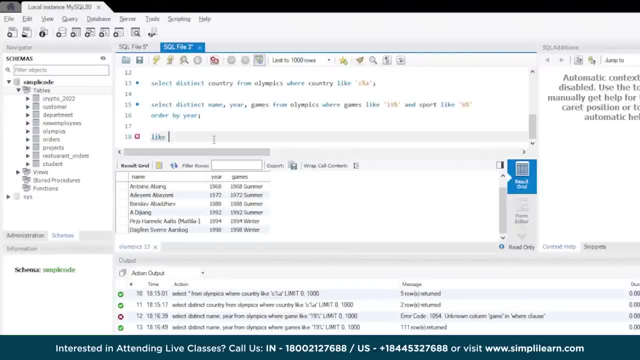 let us move ahead and discuss some examples. uh, by using the like underscore operator, right, as we discussed, like underscore operator basically returns only exactly one character that we specified. so let us just understand with an example here so that you'll have a clear idea. so let's say, if i want to fetch the details of all the names of athletes in the 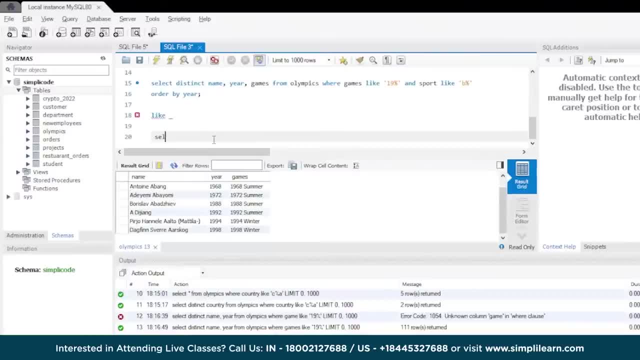 olympics table whose name starts with j and have a total of, let's say, five characters. so in that case, the following query would be: select star from olympics is the table name? where name like mention the single brackets and we know that their name starts with j and they have a total. 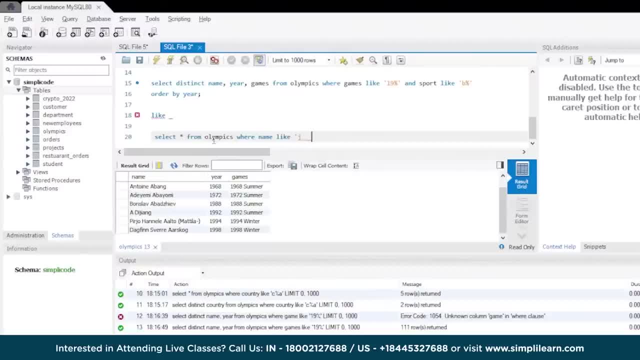 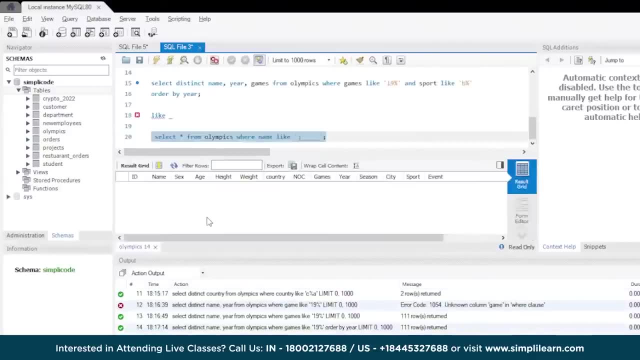 of six characters. so we'll write underscore five times: one, two, three, four and five. so let us see the output. so, as you can see in a result, and said, we have no records of the athletes whose name starts with j and has a total of six characters. so let us take another example. let's say 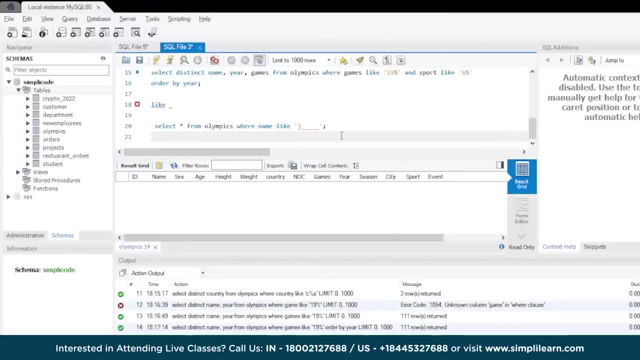 we want to, uh, find the details of the cities where the olympic games have played, which basically starts with the letter b and has a total of six characters, right? so in that case, what we'll do is select star from olympics where city like b and mention five underscores because it has a total of 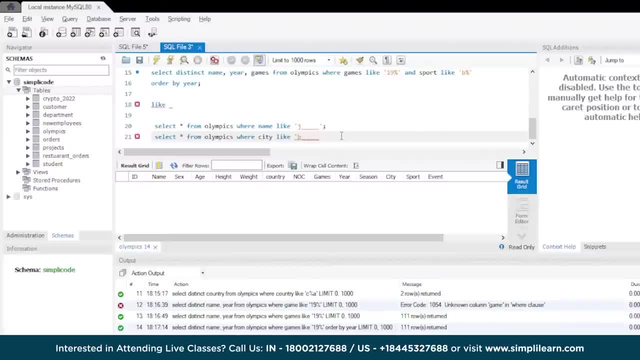 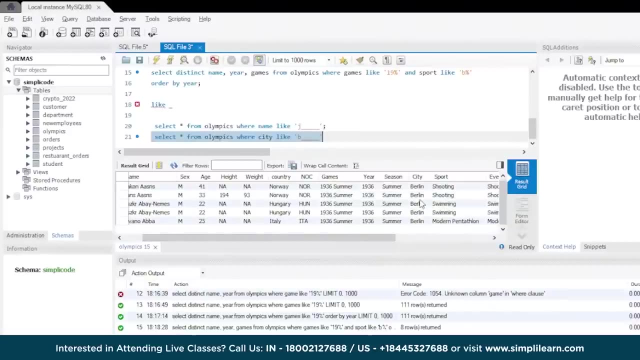 six characters. we also- we already mentioned the character b in the first place. so we'll have five uh underscores. so let us just execute this and we'll see the output. so, in a result, and said, we can see berlin is basically the city. i think it is only one and only the city that they have. 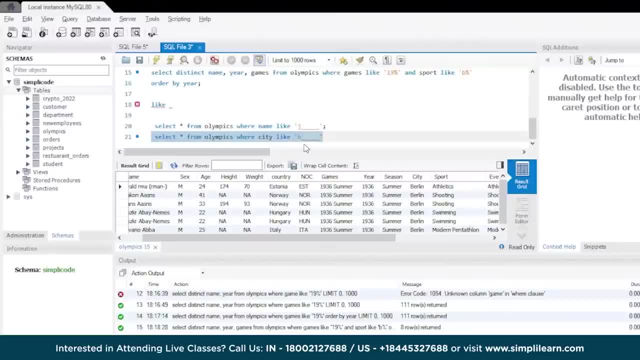 played in, which has the letter b in the first position, and it has a total of six characters. now, since you don't know, uh, the exact characters that are present in what positions, you're basically using the underscore characters to send that right. i hope you understood this, guys. uh, let us take another scenario, uh, so that we have 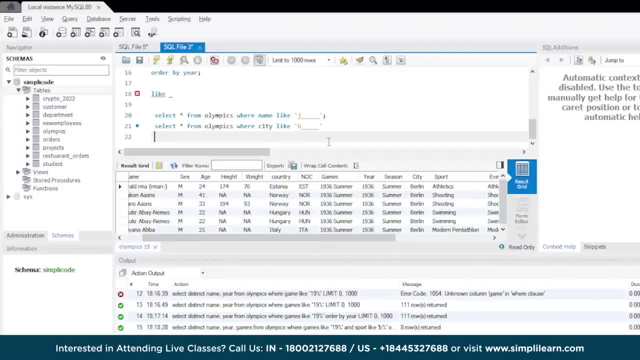 a more clear picture of how the underscore works now. we'll use this uh underscore in the last position, wherein we'll display the records of all the countries of the athletes that they have taken part in the olympic games, whose country name ends with n and has a basically uh six characters in. 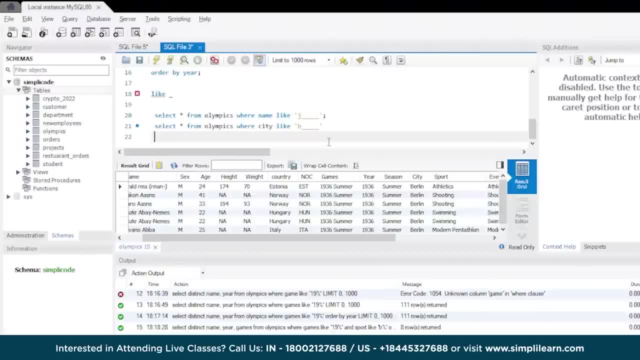 total that is five characters. so here the ass is actually a five percent hit. when the year falls we have to use that as the prime word for country. i'm going to use a particular idea to show you that one of these characters we have to mention as underscore and we 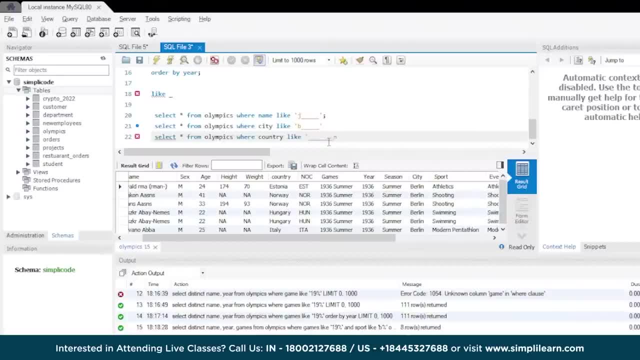 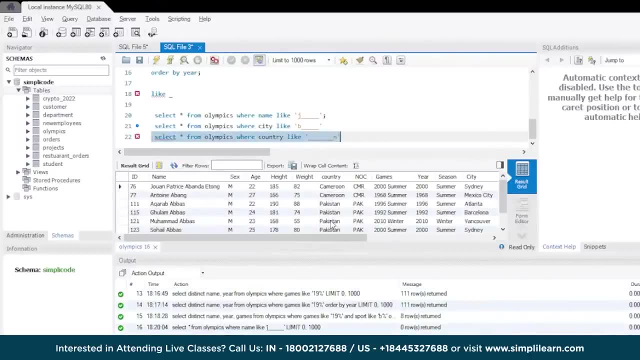 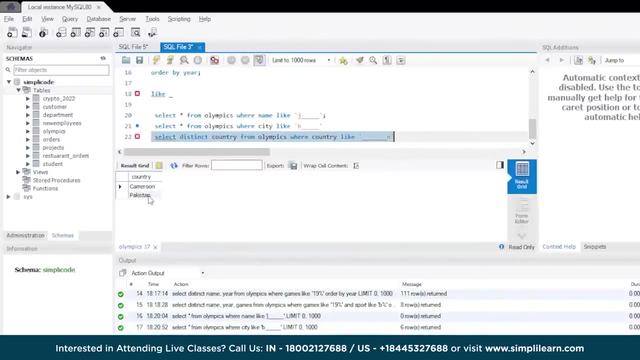 will have the n as the last letter. so select star from olympics where country like, so mention a total of six and mention the last letter which ends with a. we will have only the country names in our result table. So basically, Cameroon and Pakistan are basically the two countries that the athletes belong. 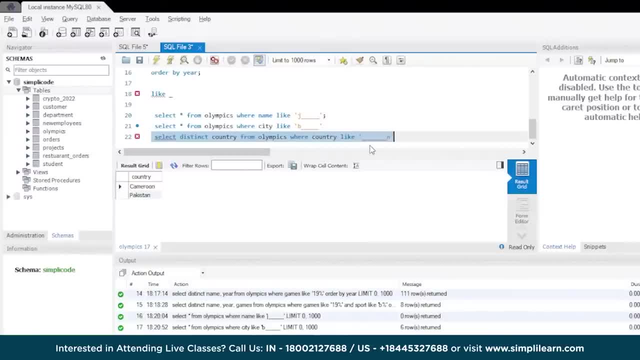 to which have a total of seven characters, and has n in the last position. So, as you can see, Cameroon and Pakistan are both those countries. So let us discuss another example, a final example, before we move on to our next scenario. So, finally, let's say, if you do not know the name of the, let's say the sport that you want. 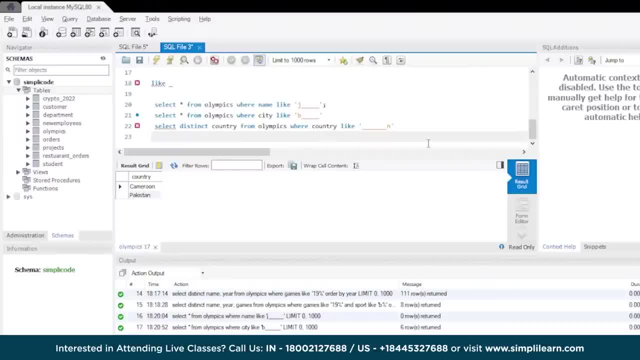 to retrieve, but you know it has a total of only six characters. You don't know the starting letter, You don't know the ending letter, but you know that it has at least, or let's say, a six characters in total. So in that case we'll use select distinct. 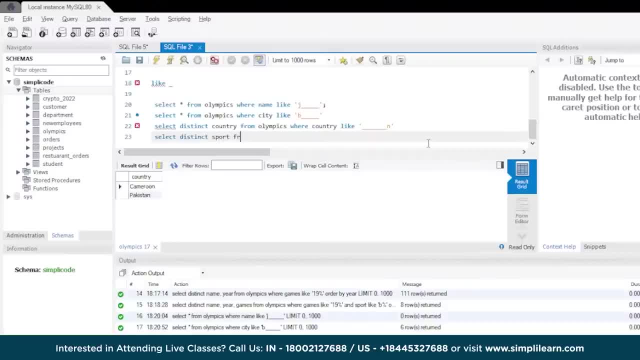 So we'll display this. So I'm taking the sport column from Olympic Games. Olympics, where sport, like So, mention six underscore values: one, two, three, four, five, six. So let us execute the statement and we'll see the output. So basically, we have five records of these sports that are played in the Olympic Games. 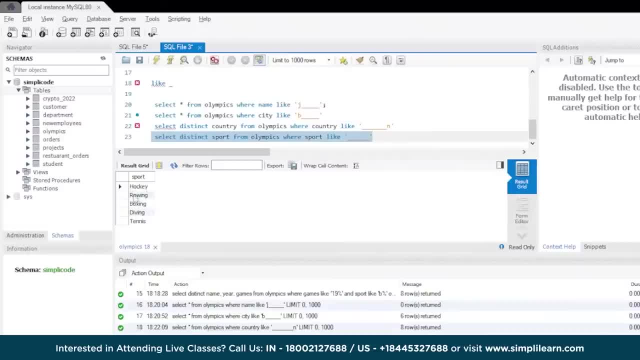 which have a total of six characters, Which is hockey, Bowing, boeing, diving and tennis. So in this way, you can use the underscore operator, without mentioning any characters or values at all, to find the actual or the value that you're searching for in your table. 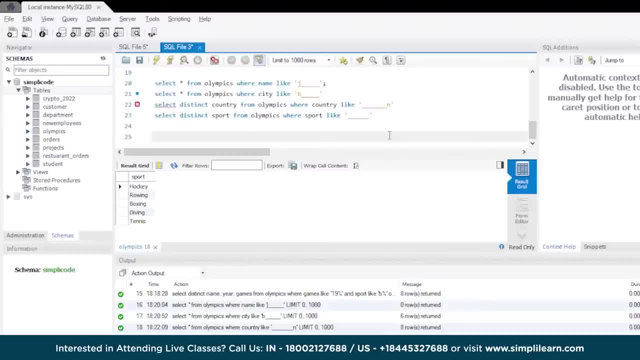 So that is how you use the like underscore operator guys. Now we have another case wherein we'll use both the like percent as well as the underscore values all together in order to retrieve the data from our table by specifying certain patterns, patterns. So So let's try to understand this with an example. 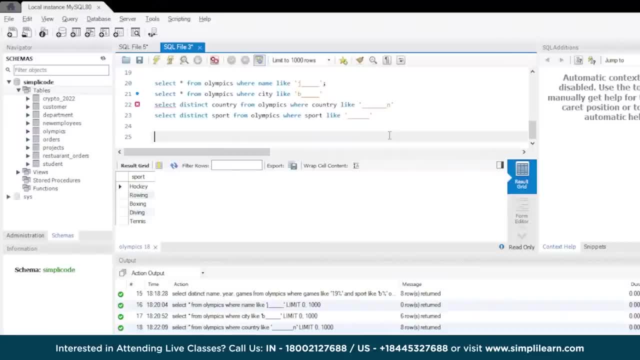 So let's say, if you're trying to fetch the details of all the countries of the athletes which whose country name starts with S and has at least three characters- I'm using the word at least, because it can have any number of values after the first character. 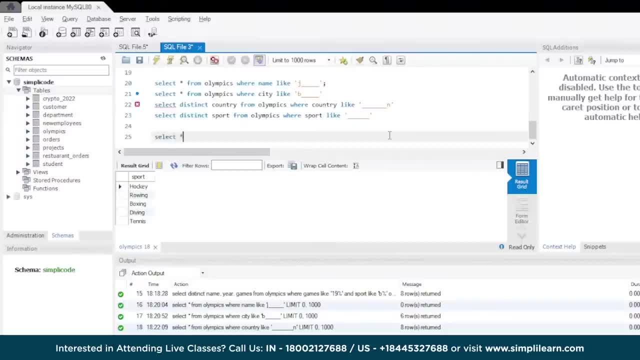 So let me just explain this with a query here: Select star from Olympics, Okay, Okay, Okay, Okay. Now I need this call around: admit piece of where country, like. Now the country name should start with this and it can have basically three characters: 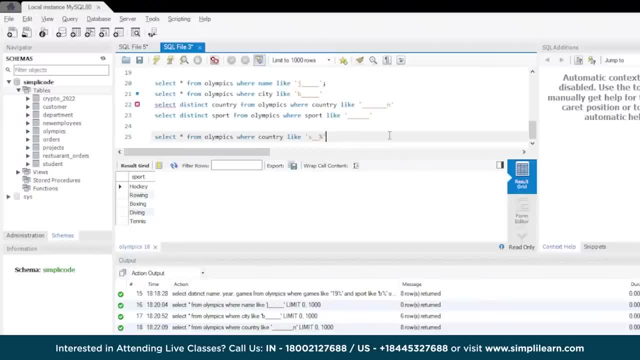 So I'm using the person to sign as well. No, I'm not telling it should have exactly three characters. It can have at least three characters. that is, it can have 45 or even six. So let us just execute the statement and we'll see the output. 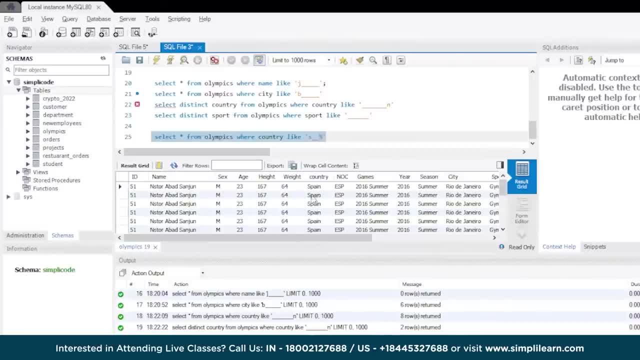 So when is this country Right? We can see in a resultant set. Spain is a country which starts with S and have at least three characters in total, And similarly we have Soviet Union as well. So in this way you can use both underscore as well as the percentage operator. 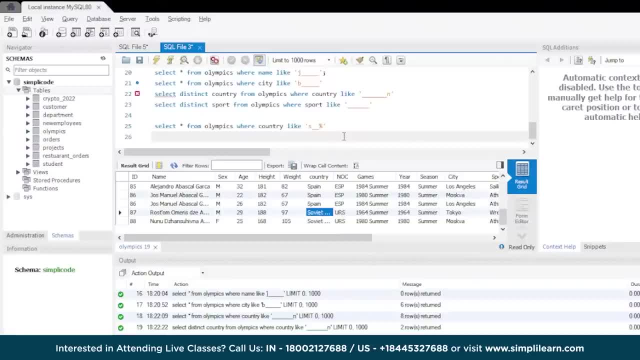 So let us just understand with another example here, guys. Let's say, if you're trying to fetch the details of all the events from the Olympic Games that were played, which basically has M in its third position and can have any number of characters, 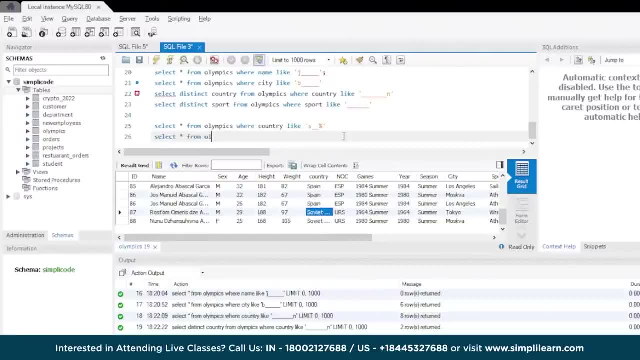 So in that case, the following query would be: select star from Olympics. Sorry, we're just selecting the event, right, So I'll mention the event. Select event from Olympics where event, like Now I said, the Character M is present at the third position. 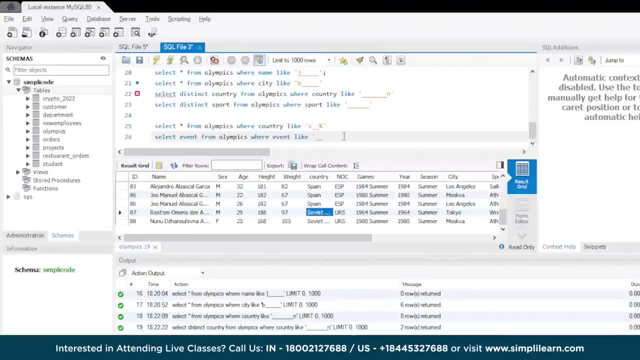 So first I'll mention two underscores, Next I'll mention the M character And then, finally, I'll mention the percentage, so that it can have any number of values after the character M. So let us just execute the statement and we'll see the output. 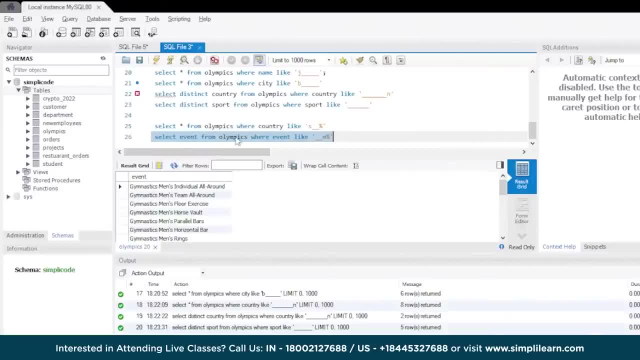 So it will basically retrieve all the events that are played in Olympic Games, which has M in the third position. So as you can see, gymnastics men's individual all round. Similarly, gymnastics men's team all round Floor exercise. 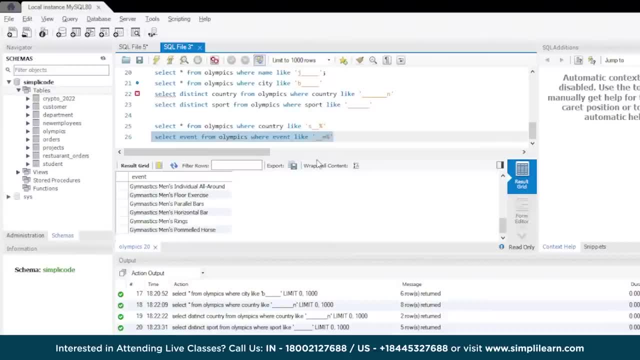 Exercises, horse vault, and all these have M in the third position And basically it has any number of characters. That is a total number of characters. So I hope you're following with me and you're understanding this. So let us consider another example. 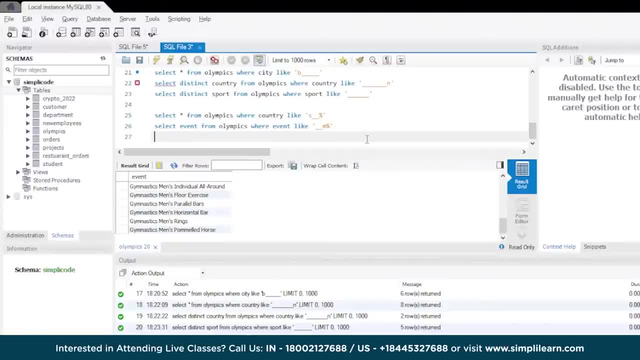 So let's say: if you want to, if you're trying to retrieve the countries that the athletes are belonging to, where the country name has A in the second letter And it ends with N, So in that case what we'll do is I'll write another query, which is: select star from Olympics, where country like 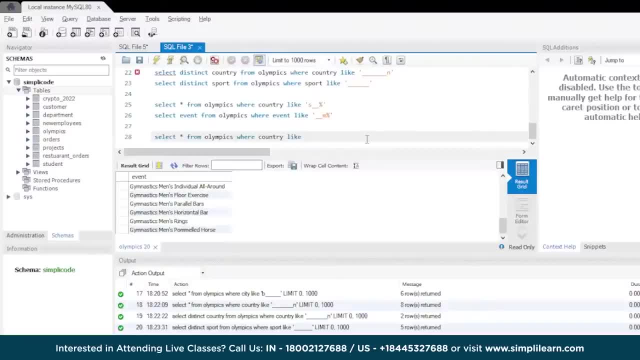 So I said we have A in the second position, so we do not know what is present in the first place. So I'm just mentioning an underscore and then I'm mentioning A and then I'm using percentage, because we have no restriction here. It can have any number of values. 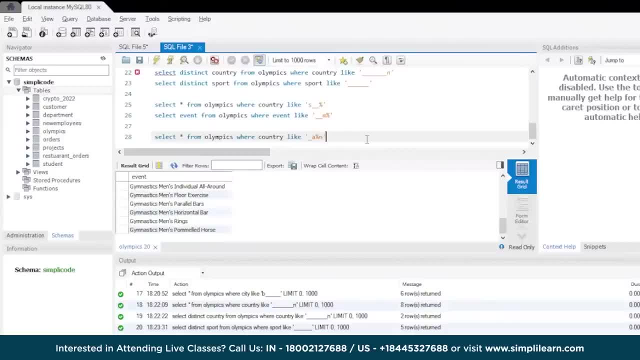 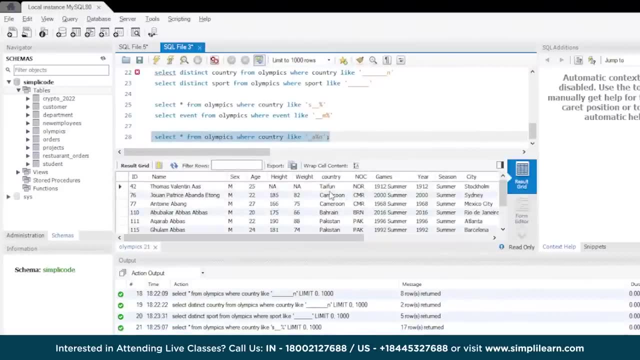 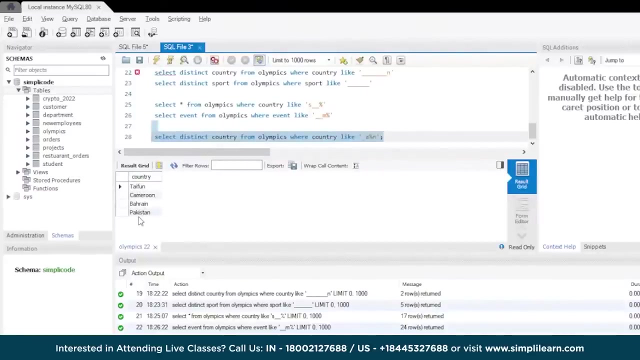 Now the only criteria is that it should end with N, right, So we'll just execute this and we'll see the output. Okay, it is displaying all the records, right, So let's just use the country. So, as you can see, we have a total of four records, which are basically Typhoon, Cameroon, Bahrain and Pakistan. 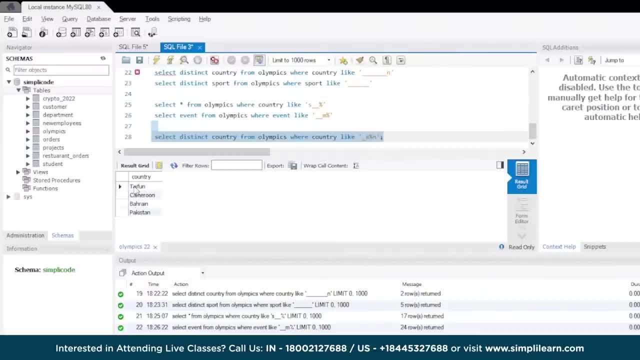 Now, if you clearly look into this resultant set, We have A in the second position. you can see right. So we have A in the second position and it is having N number of characters, which is which is of no limit, And the only condition we have specified is it should end with N. 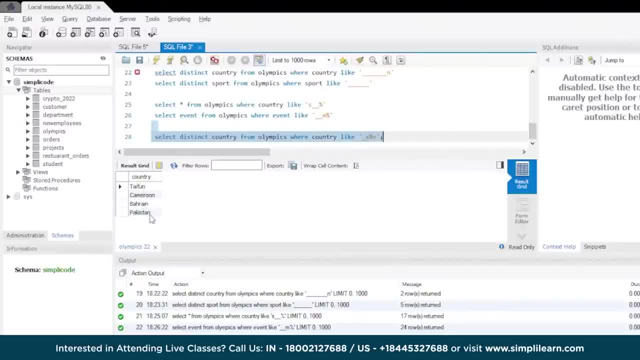 So in all these records the country names are ending with N, So in this way you can use the percentage and alias- sorry, percentage- and the underscore to specify this kind of pattern as well. So I hope you have Understood this, guys. 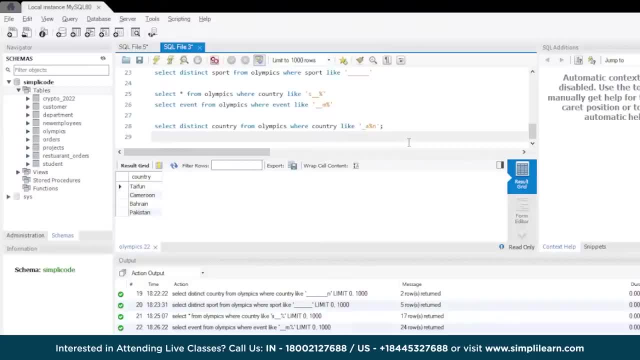 So, finally, let us look at another example so that we can wrap this session finally. So let's say, if you want to display records of various sports that are played, which can have any number of characters, But the last but one character should be in, that is, it should contain letter N, or basically, the penultimate character should end with them. 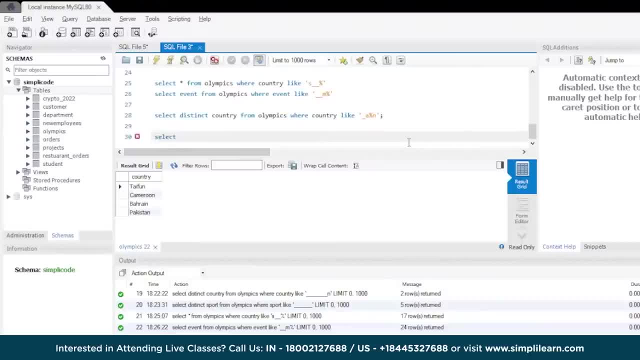 So in that case, the following query would be: select distinct sport. it could stay anything from Olympics where sports like What is an sport, but with this order. So I hope you understood the question, though the question is: The sport can have any number of characters, but the only condition is the last but one character should be N. 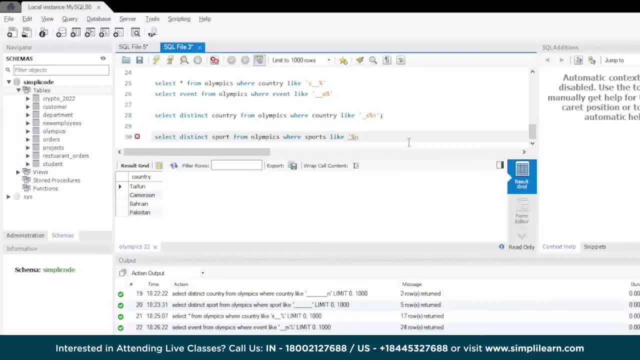 So I'll first mention the percentage, That is, it can have any number of characters Before but one character- and i'm mentioning an underscore- that is, it can have any number of any value in the last place, that is, any it can fill any character in that place. so let's just execute this statement. 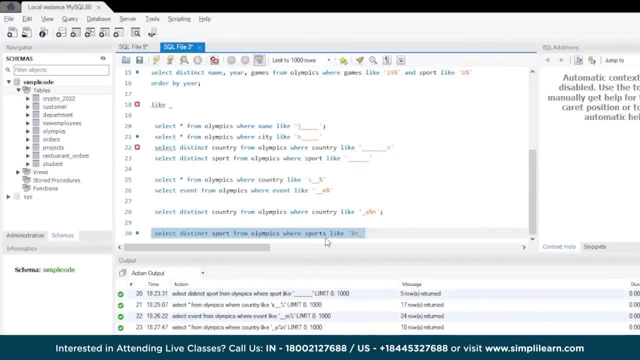 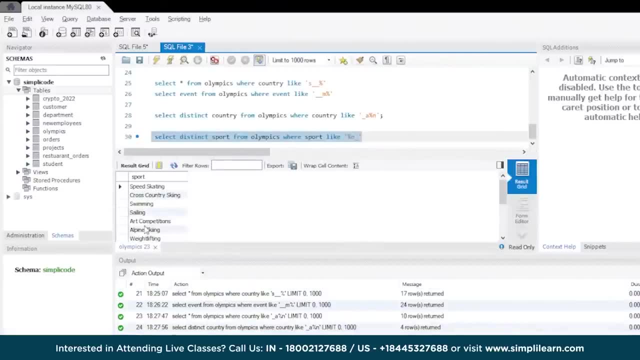 and we'll see the output. okay, sport, sorry, it is just sport, not sports. so in a result and set, you can see that we have various ports which basically has n in this second last position. so you can see in speed skating, in cross country, skiing, swimming, sailing. 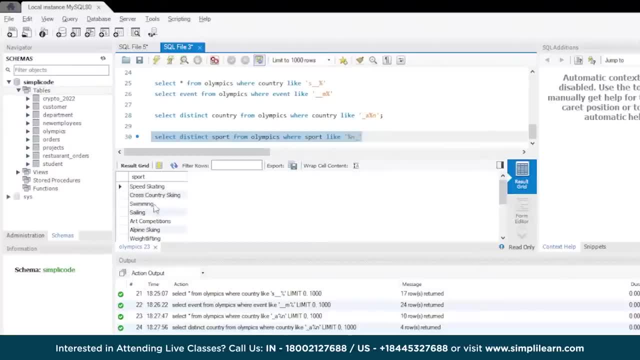 and so on. in all these are values. we have n at the last position. so in this way you can use the. you can use both percentage as well as underscore to find patterns in your data table as well. so, and similarly, guys, we have the not like uh operator to find the pattern matching as well. so let me just 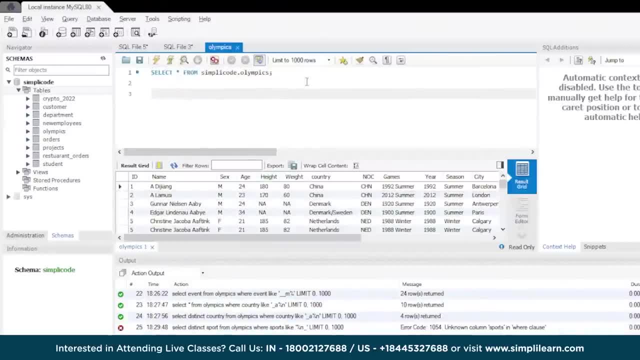 help you with this example. so let's say, if you want to find the age of all the athletes, uh who's who are not in the age of, who are in the not in the age group of 20, right? so in that case, what i'll do is select star from olympics. where age use the not like keyword. 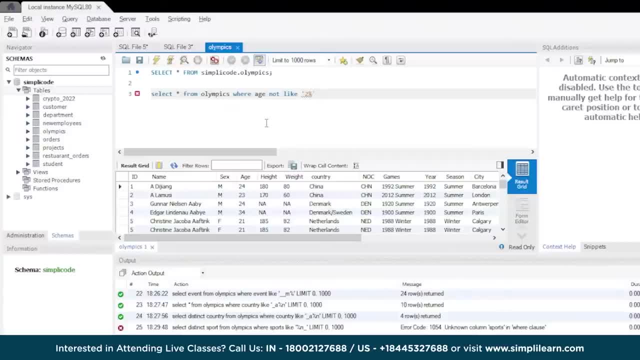 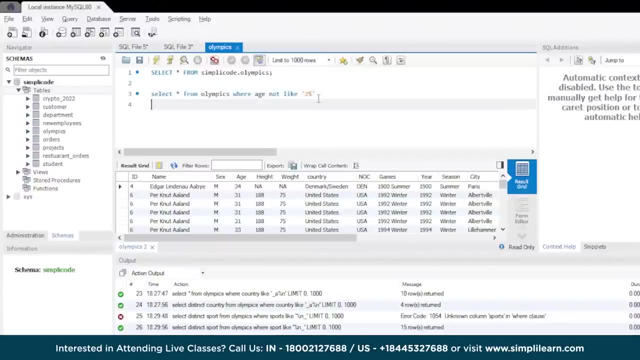 and mention two percent. so it will basically uh omit all the values, or the values of all the athletes. who's a who's arranging in the age group of 20 to 30.. so let us just execute this statement and we'll see the output. uh, we'll also uh use the order by, so that we'll have in the 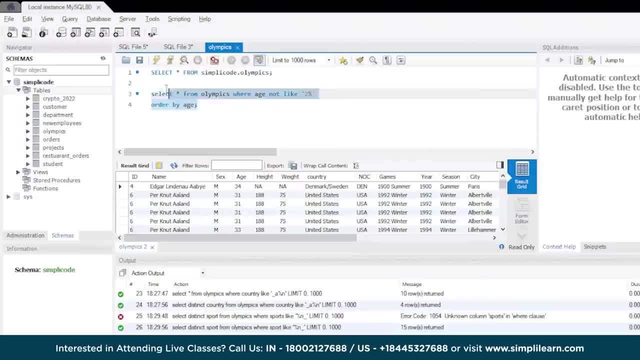 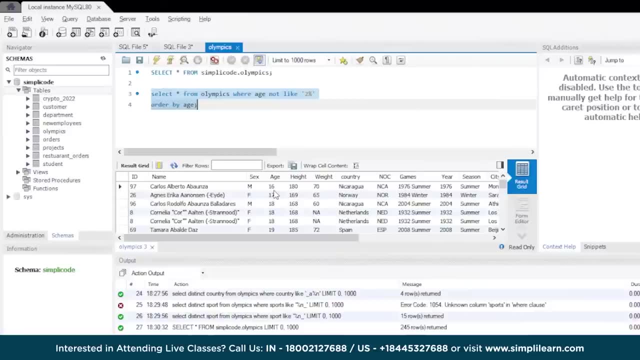 ascending order. order by h. right, as you can see, the resultant set has all the ages of the athletes, uh, starting from 16, 17, 18 and 19, and, if you clearly observe here, after the age of the athletes, after 19, we have 30. so basically, it is omitting all the values that has. 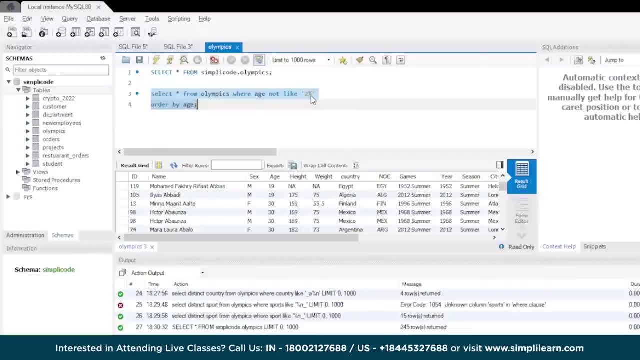 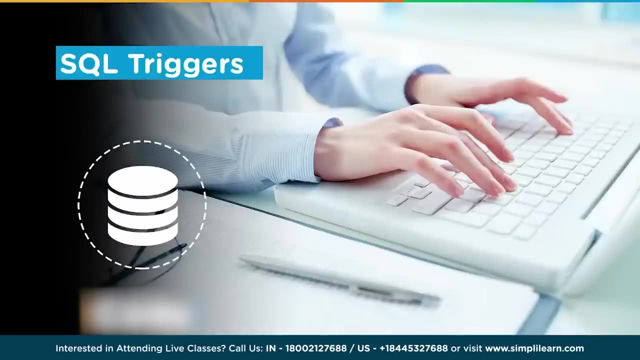 uh two, or that is the uh. athlete's uh age is lying in the range of between 20 and 30. so in this way you can also use the not like uh values not like operator to omit the values that in the pattern matching we will be discussing about triggers in sql, so in this tutorial we'll 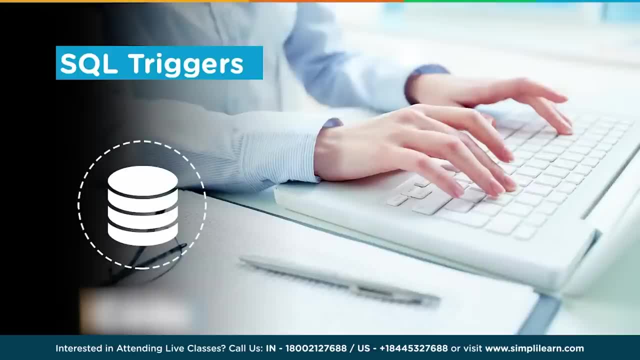 be going through various concepts of triggers, understand its significance and see how it exactly works in sql. now, have you ever watched a line of dominoes fall when you knock the first one down? now, in that case, you have just invoked a trigger which has created an event there. your 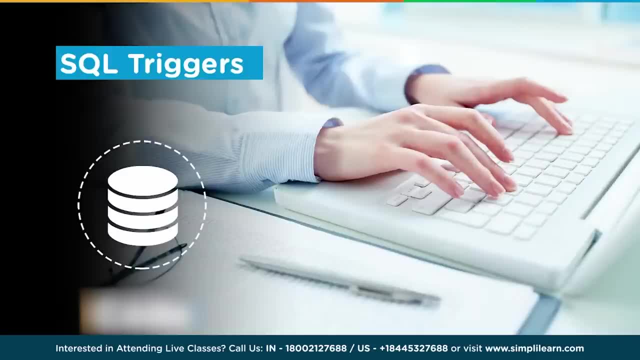 touch of first style triggered the chain reaction that has knocked down the rest of the dominoes as well now this is the same principle applied to database triggers as well. now a trigger in database terms is set of instructions that is activated, or we say it has fired by some specific 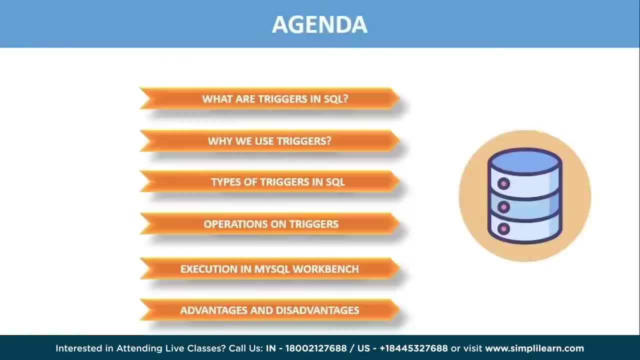 event. normally, a command issued to the trigger is triggered in the same way that a trigger is triggered through a sql code. firstly, let us discuss the agenda for today's session. we'll start the tutorial by understanding what are triggers in sql, and then we'll go through why we use. 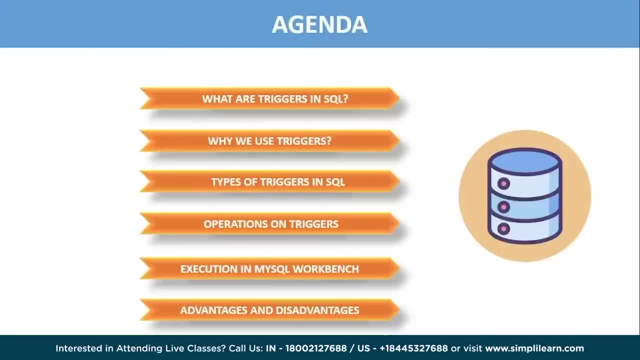 triggers, and after that we'll see different types of triggers used in sql, and after that we'll be discussing various operations used with triggers. and then we'll get into the execution part in mysql workbench using various examples. and finally we'll wrap the session by discussing some 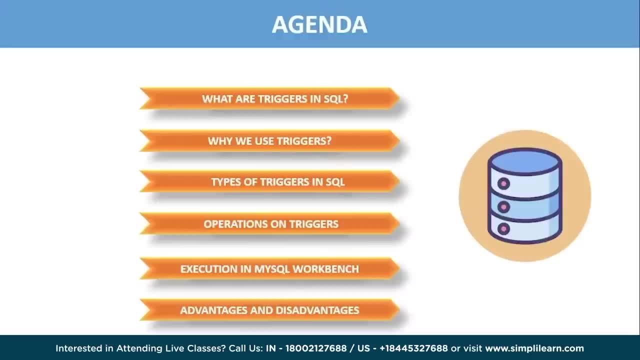 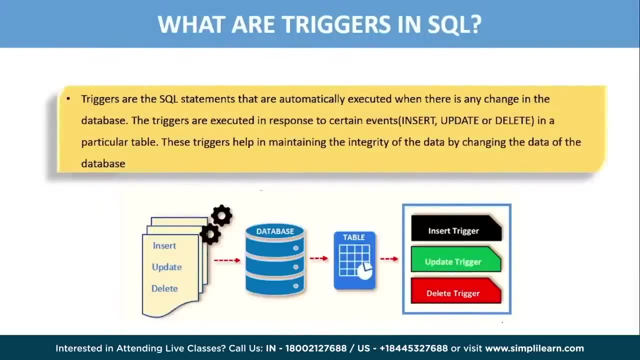 of the advantages and disadvantages of triggers. so, without any further ado, let us jump straight into today's topic. so, firstly, what are triggers in sql? now? triggers is a database object which fires when an event occurs in a database. or you can say: a trigger is a piece of code executed. 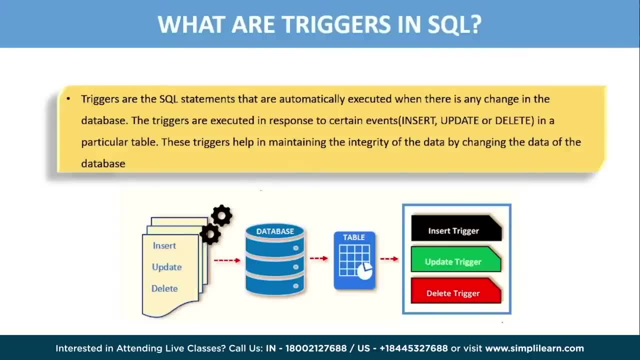 automatically in response to a specific event occurred on a table in the database. now, triggers, as the name suggests, are stored procedures. are stored procedures means procedures are basically functions which contain sql statements which are stored in database and can return some output which are executed or fired when some event 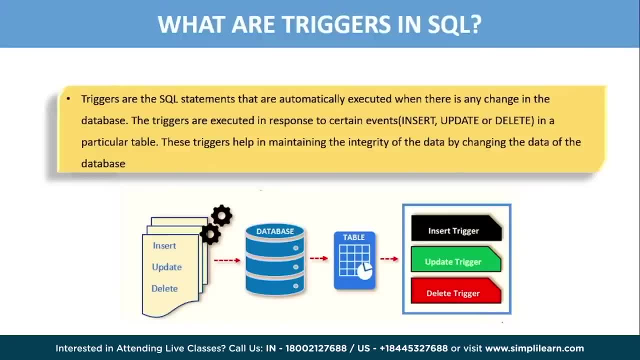 occurs. now a trigger is always associated with a particular table and if the table is deleted, all the associated triggers are also deleted automatically. now the triggers are executed in response to certain events like insert, update or delete in a particular table. now a trigger is worked either before or after the following events of: from the dml commands, like through: 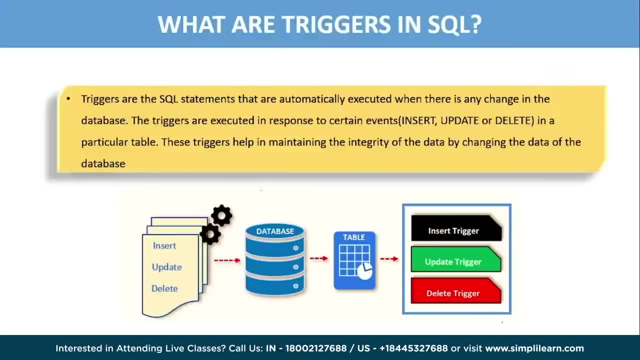 insert when a new row is inserted, or through an update command when an existing row is updated, or through a delete command when a row is deleted. so when you issue an insert, update or delete statement, the relational database management system fires the corresponding trigger and also these triggers, helps in maintaining the integrity of the data by changing the date of the database. 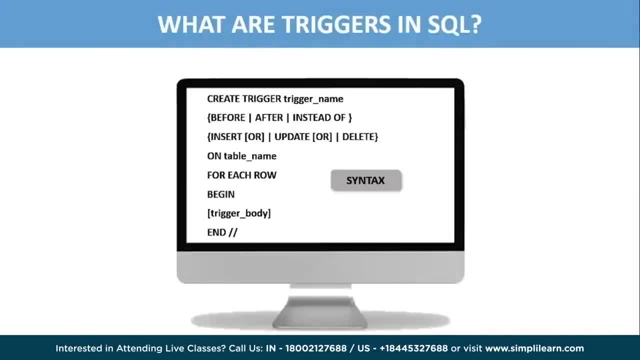 let us now understand the syntax of triggers. now we can create triggers for various types of operations, as discussed above, and we'll mostly focus on dml triggers, as these are the most commonly and extensively used triggers and also, at the same time, most important. so a dml trigger can be created. 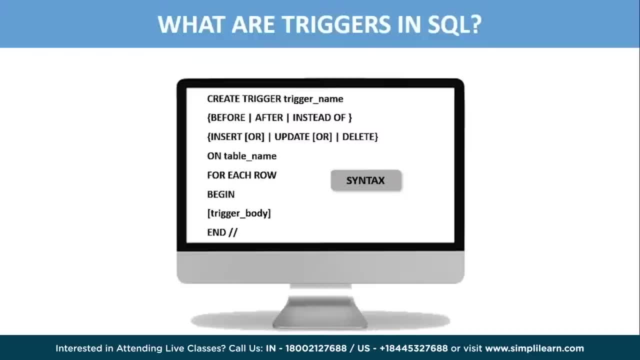 using the following syntax, which is followed as: create trigger trigger name before, after: instead of insert or update or delete on table name for each row: begin trigger body, end, double slash. so let's just discuss the different parts of the syntax clearly. now we have the create or replace trigger trigger name in the first line, where we give the name of: 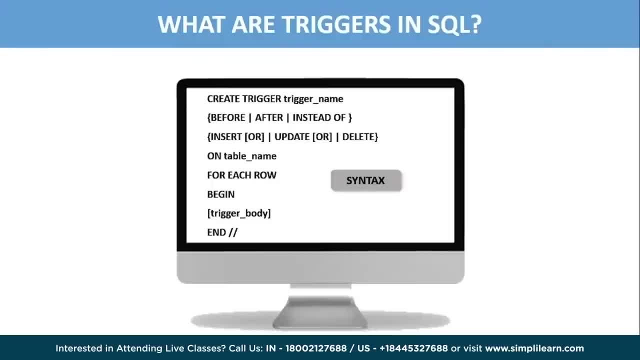 the trigger we are creating or updating here. trigger name is to be replaced by the name you want to have for your trigger in your database. now it can be of any name as per your choice. next we have the before- after instead of keywords. here we define when the trigger would run, that is, before or. 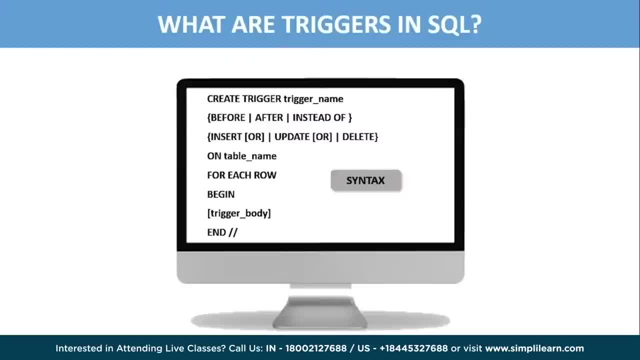 after the trigger would run. that is before or after the trigger would run. that is, before or after the dml operation. for example, if you want a trigger to be executed after insertion to a table, we will consider after insert here next we have various dml commands like insert or update or delete this. 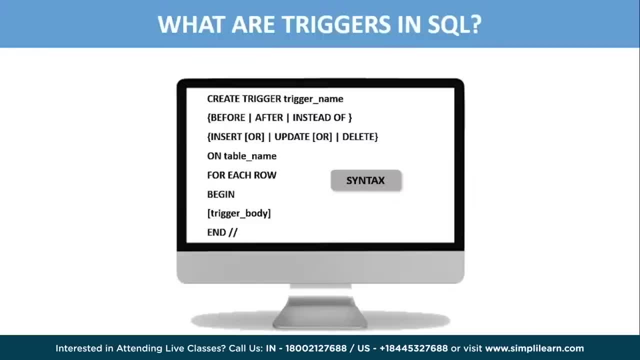 is the operation or event we have to define which will trigger a procedure to be executed. if we want a procedure to run after a deletion happens on the table, then we'll consider writing delete there. next we have on table name. here we have to specify the name of the table on which we are. 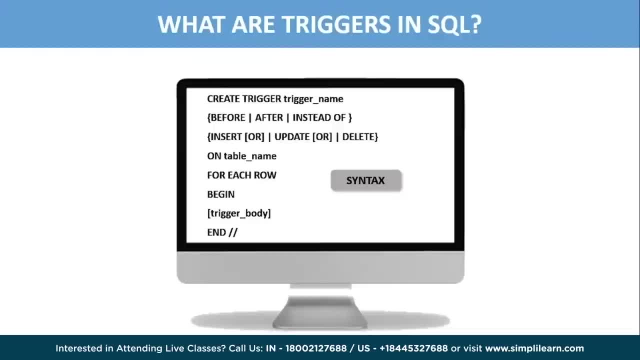 attacking the trigger, we have to specify the name of the table on which we are attacking the trigger. we have to specify the name of the table on which we are attacking the trigger and next we have, for each row, keyword where this line specifies that the procedure will be executed for each one of the 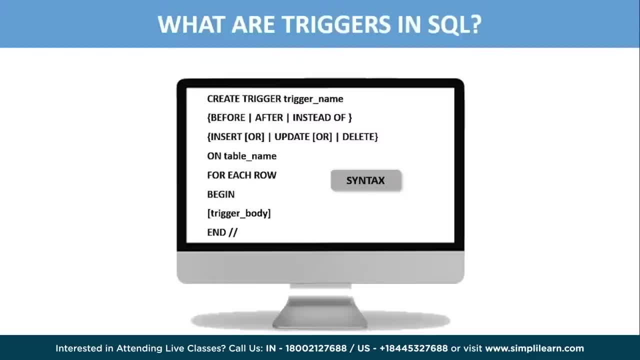 rows present. here we can set a condition for which rows to be impacted. this part is optional, though. in case we don't use this, the trigger shall convert to a statement level trigger rather than being a row level one, so we'll discuss about that later. so next we have the when condition. 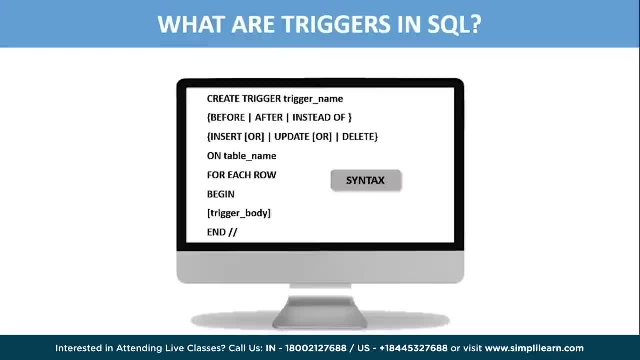 where, which mentions some condition basis of which the trigger will run. in absence of when- condition which is again optional, you can expect it to run for all the eligible rows. so this is very important, as this will control which rows the trigger must run. and, finally, we have the trigger body, which is the main logic of what to perform once the trigger is fired. 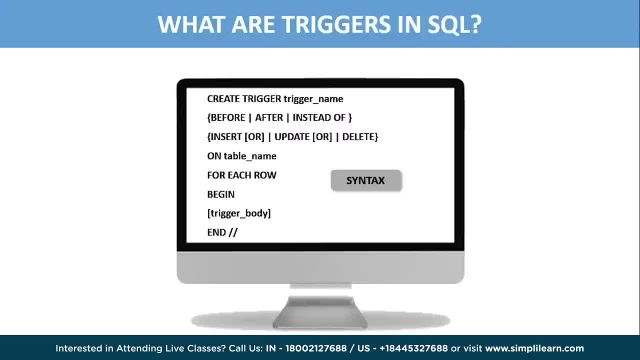 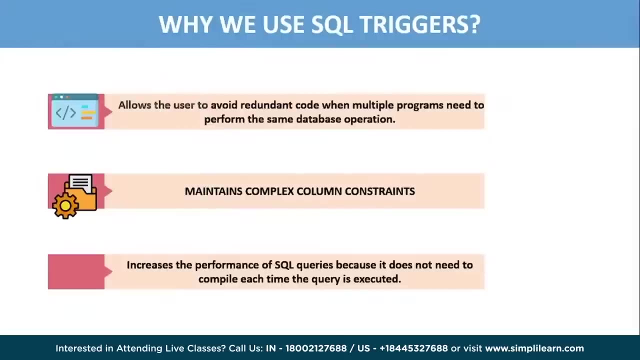 in the previous statements, all we define is when this trigger will be fired, but here we have to define what to do after the trigger is fired. so this is the main execution part of the sql code and we end the syntax with n double slash, right moving ahead. why we use sql triggers now, since a trigger resides, 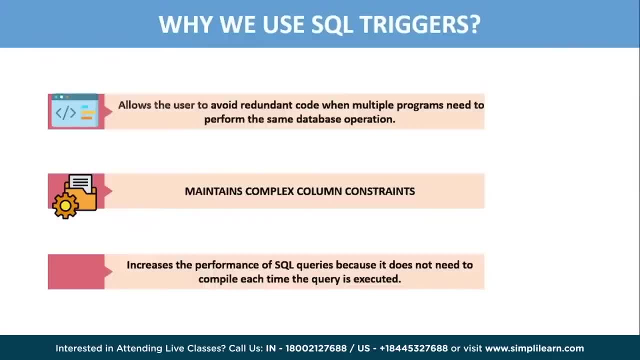 in the database and anyone who has the required privilege can use it. or trigger lets you to write a set of sql statements that multiple applications can use, so it allows the user to avoid redundant code when multiple programs need to perform the same database operations. sql triggers also maintains: 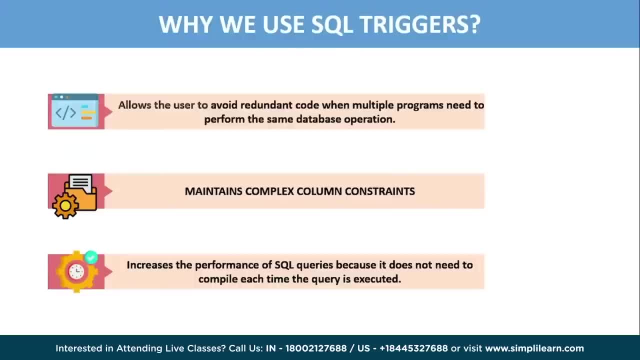 the integrity constraints in the database tables, especially when the primary key and foreign key constraints are not defined, and it also helps in maintaining the track of all the changes, like updation, deletion and insertion, that occur in the database table. triggers also increase the performance of sql queries, because it does not- it does not need to compile each time the query is. 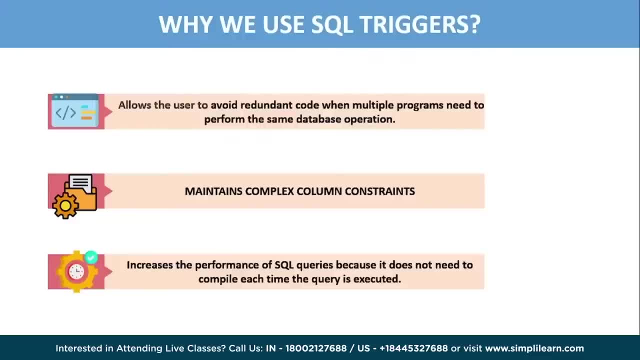 executed. all right. moving ahead, let us now discuss the type of sql code and the other features of sql that we are going to talk about in this video. so first of all, let's talk about the type of sql code that we are going to talk about in this video. so, first of all, let's talk about the type of sql code. 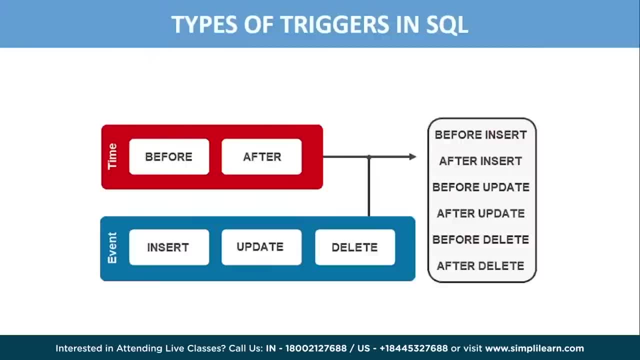 of triggers in sql. now, triggers are of two types in general, according to the sql standard language, which is row level trigger and statement level trigger. now, row level trigger, which is activated for each row by a triggering statement such as insert, update or delete. now, for example, if a 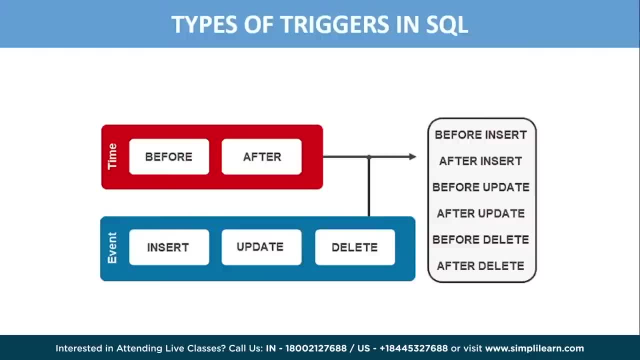 table has inserted, updated or deleted multiple rows, the row trigger is fired automatically for each row affected by this insert or update or delete statement. next, we have the statement level trigger, which is uh, fired once for each event that occurs on a table, regardless of how many rows are inserted, updated or triggered. now further, we have uh. 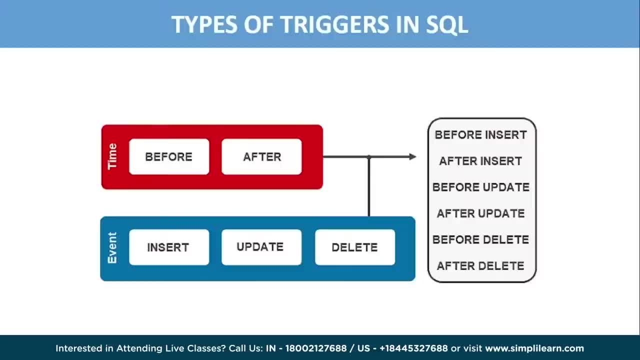 six types of triggers based on the uh events of occurrence of the triggers uh through the dml commands that are invoked and at the time of when they are uh executed. so we can define the maximum of six types of actions or events in the form of triggers, which is 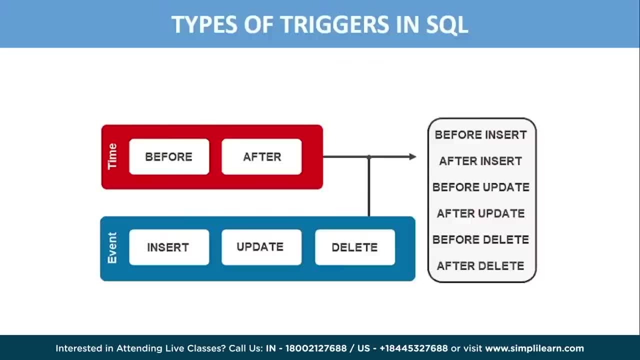 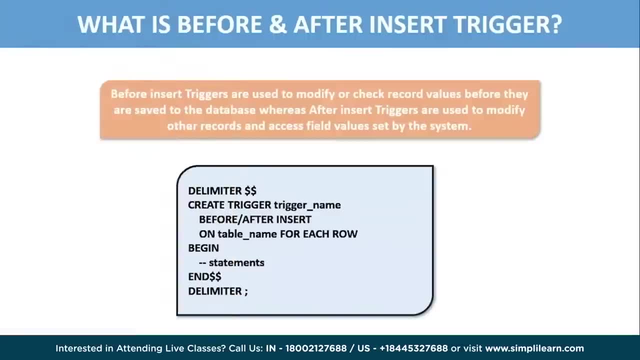 before insert, after insert, before update, after update, before delete and after delete. let us now discuss about them in detail. now. first, we have uh, the before and after insert trigger. the before insert triggers are used to modify or check record values before they are saved to the database. 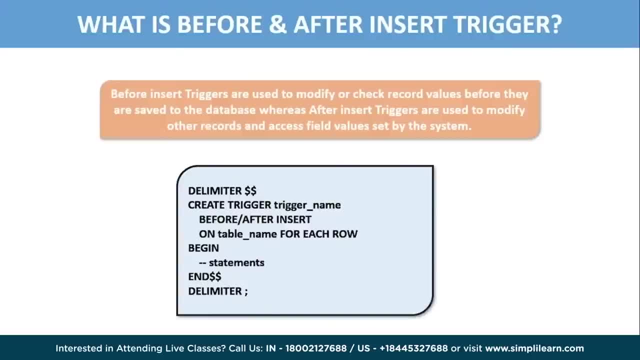 whereas the after insert triggers are used to modify other records and access field values set by the system and the syntax for before and after insert trigger is followed as delimiter. create trigger. trigger name: before or after is the keyword we have to mention uh prior to the insert uh name. 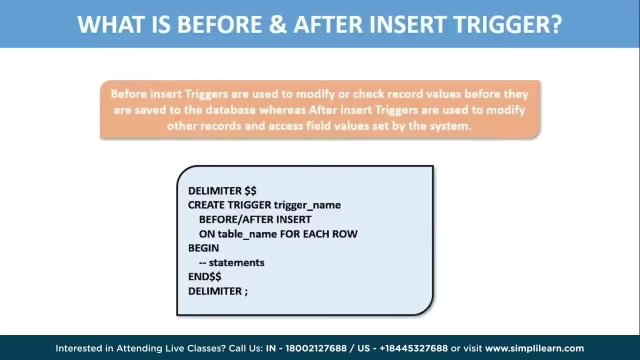 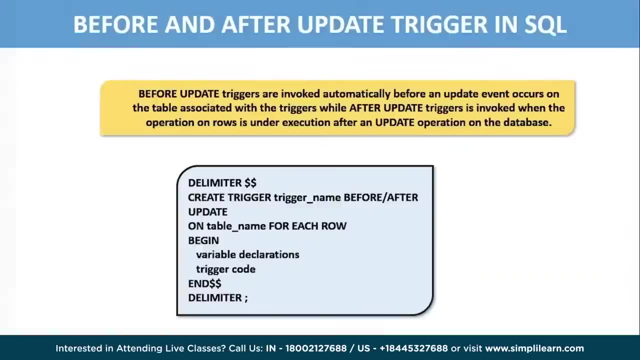 on table name for each row, begin, mention the uh body of the trigger and mention the end keyword and end with the delimiter. next we have the before and after update trigger in sql. now the before update triggers are invoked automatically before an update event occurs on the table. 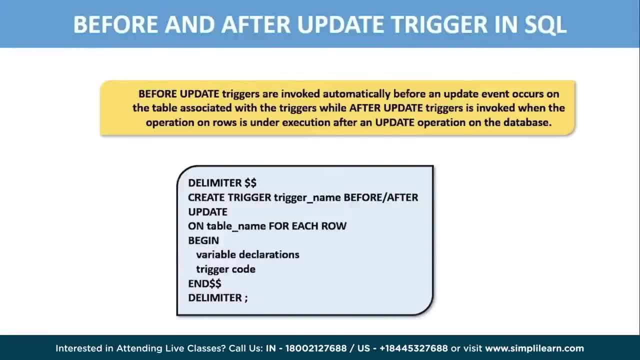 associated with the triggers, while after update trigger is invoked when the operations on row is under execution after an update operation on the database. now the syntax is also same. instead of the insert, you have to just replay, replace it with the update keyword, uh, with the before and. 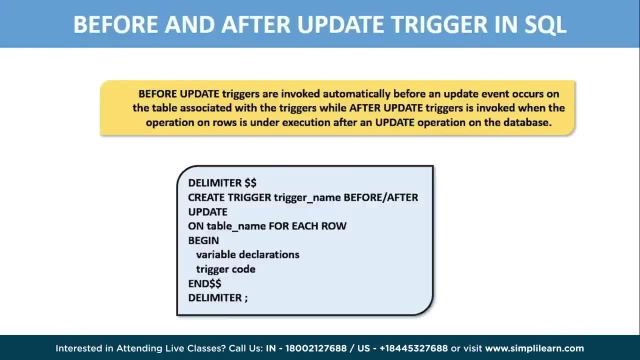 after keywords as well. now, firstly, we will specify the trigger name that we want to create, and then specify the trigger action time, which should be before update or after update, so this trigger will be invoked before each row of alterations occurs on the table, if you use before, and similarly with the after keyword as well. and third, we will specify the name of the. 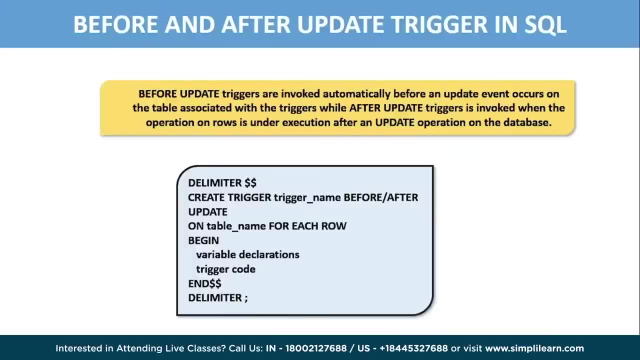 table to which the trigger is associated, so it must be written after the on keyword and if you do not specify the table name, a trigger would not exist. finally, we'll specify the trigger body that contains a statement of execution: uh, when the trigger is activated, where you can mention: 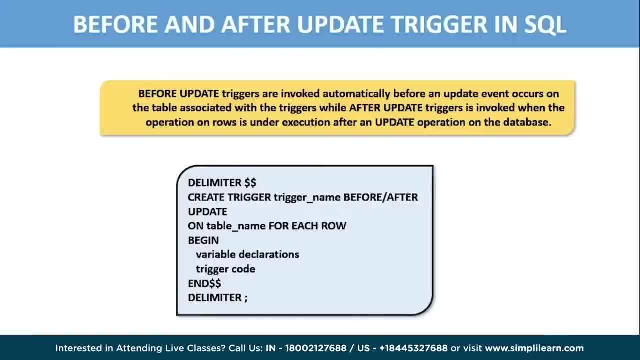 different condition using the when keyword as well. now we cannot update the old values in a before update trigger where and we can change the new values as well, which we'll discuss while we are executing the code in mysql workbench, so that you'll have a clear idea. 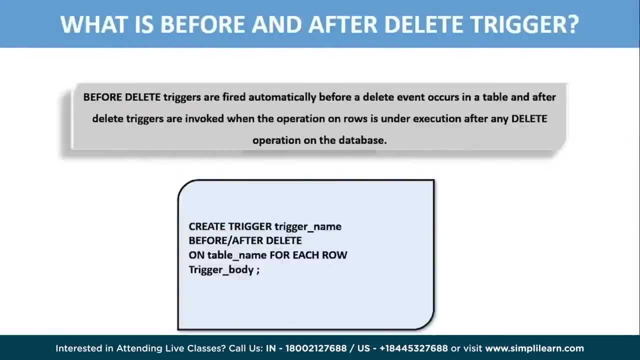 and finally, we have the before and after delay trigger as well: before delay triggers are fired automatically before a delete event occurs in a table and after delete triggers are invoked when the operations on the rows is under execution- after any delete operation on the database as well. now the syntax is also: 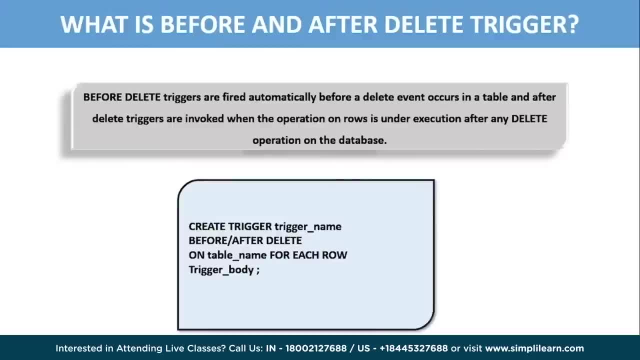 similar to that of uh previously, to that of insert and update, which is, create trigger trigger name before, after delete on table name for each row and then mention the trigger body. so in this way you can apply various uh triggers on your database. so to understand this in a more better way, uh let. 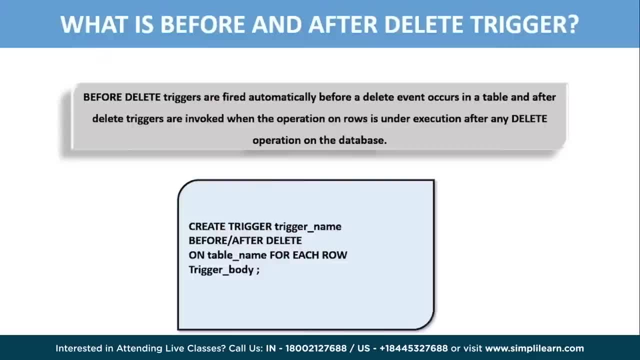 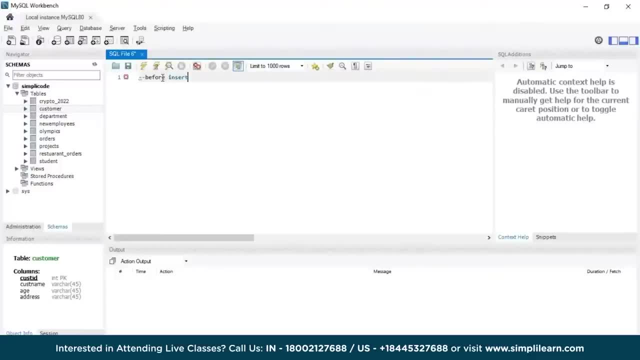 us jump into mysql workbench for further execution part. so, as you can see, mysql workbench has started and first let us uh discuss how to create a before insert trigger. now. now, as discussed earlier, uh, before insert trigger in sql is invoked automatically whenever an insert operation is. 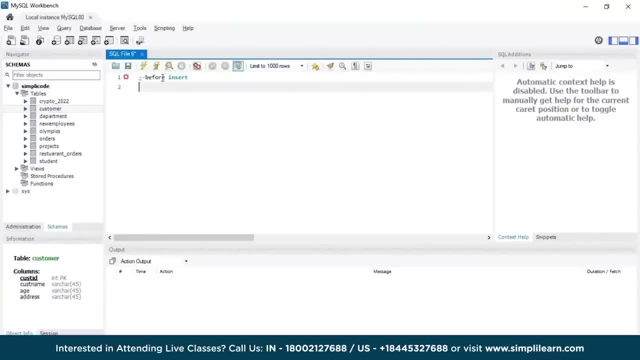 executed. so let us discuss how to create a before insert trigger with its syntax and an example. now, in order to create a trigger, you have to first create a new table and then insert values into it to perform a trigger operation. but we already know how to create a table and 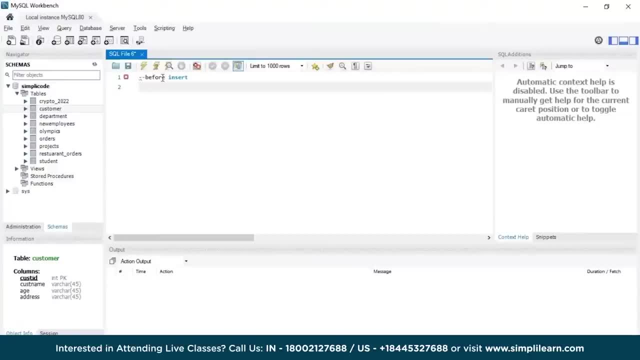 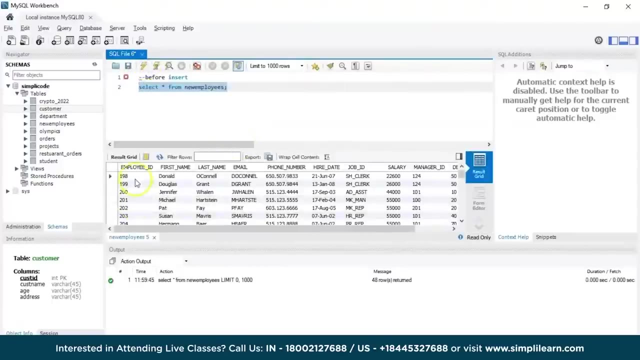 insert values into it. so let us just consider an already existing table, let's say new employees. so i'll just display the values, select star from new employees. so the new employees table has various attributes such as employee id, first name, last name, email, phone number, hiring date, job id, salary, manager id and department id. 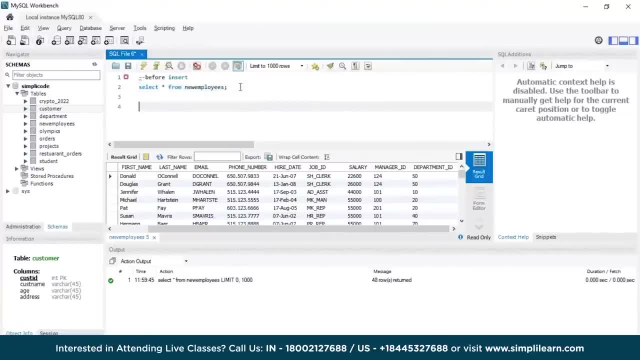 right, so let us now run the before insert uh syntax. so first we have the delimiter here. now, when we are writing our sql statements, we generally use the semicolon right to separate two statements. now, since uh a trigger is a stored procedure which consists of multiple statements. 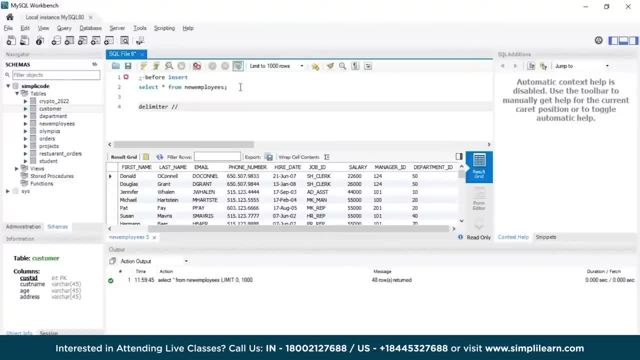 operated by a column. so if you are using mysql to define a stored procedure like trigger that contains semicolon characters, it will not trade the whole like the stored procedure as a single statement, but many statements. therefore you have to define the delimiter temporarily so that you can pass the whole. 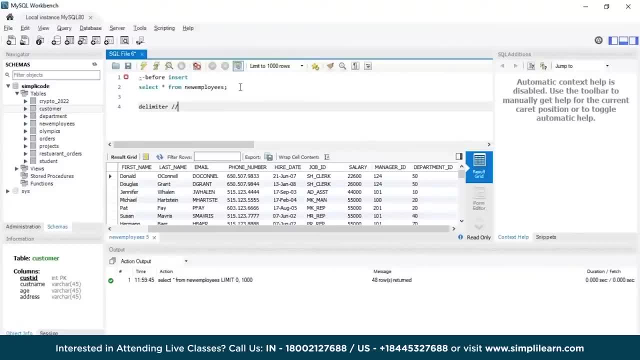 uh, the body of the trigger as a single statement. so typically we are just uh separating uh these statements using the uh double slash here, so delimiter. now we have to write the actual syntax for the before insert trigger, which is create trigger, which is the keyword i'm using, and let 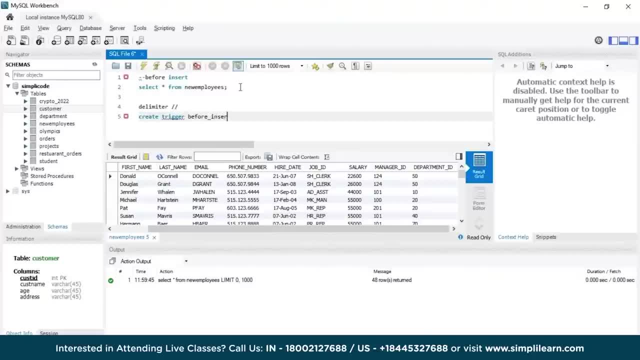 us take the trigger name as, let's say before, insert. you can take it as per your own choice: insert, insert is the keyword on the table, that is, new employees. now i'm applying trigger for each row, so i'm specifying for each row. now here, uh, comes the main part where you have to mention the condition. 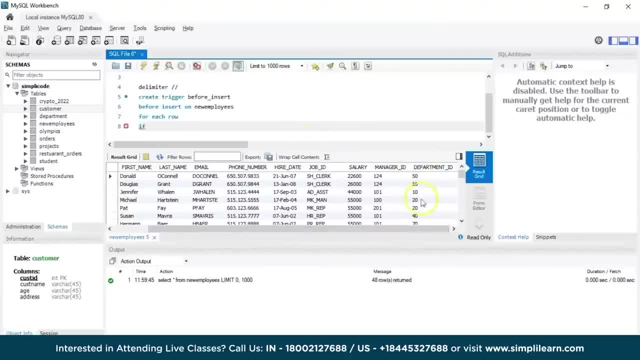 now, the trigger that i'll be invoking is: uh, let's say, now we have department ids here, right, which are uh, having values like 10, 20, 50, 100, 60s and 100. so if you notice here, uh, we have the department ids in the name, in the multiples of values of 10.. so i'll be creating. 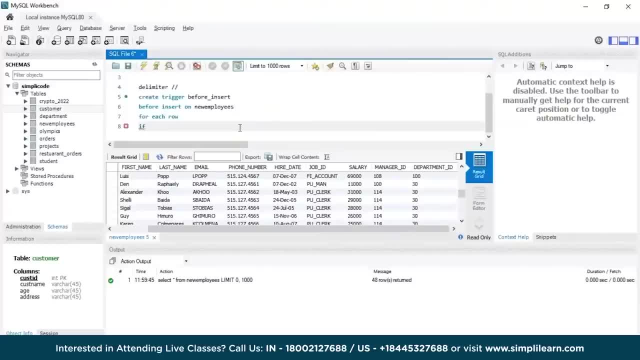 a trigger whenever a new user is trying to insert values into the table as department id which is less than 10.. so in that case i'll set the new department id as 0.. so the query would be if new dot department id is less than 10. 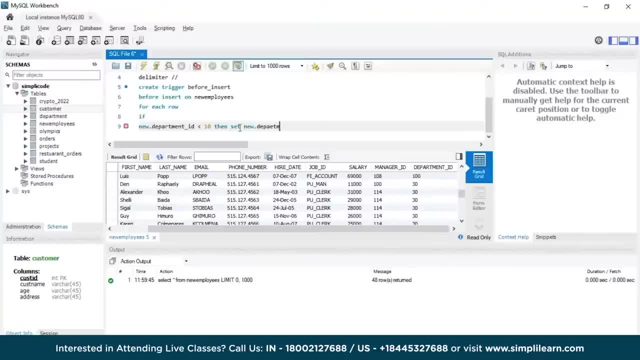 then set new dot department id equals to zero. so mention the end if and in double slash, depend on the trigger event which you're performing now, since you're checking or modifying a value when you're trying to insert data using the new dot column modifier, which is available, whereas if you are trying to insert old values, that 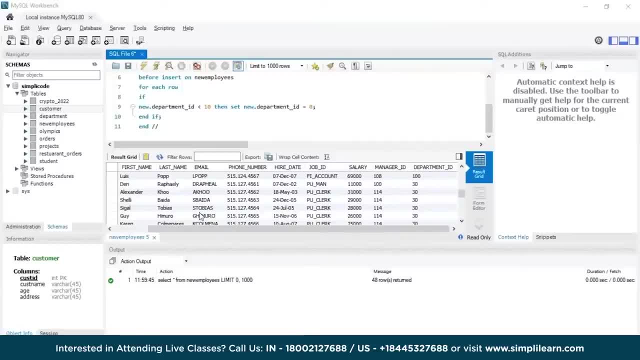 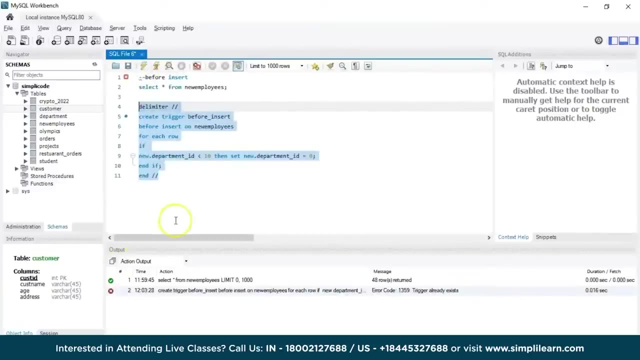 is using the old dot column. name value does not exist for an insert statement because there is no information exists in in its place beforehand. so that is the reason I'm taking the new keyword here. so we have created our trigger, so let's just execute the statement and we'll see the output. okay, there is an. 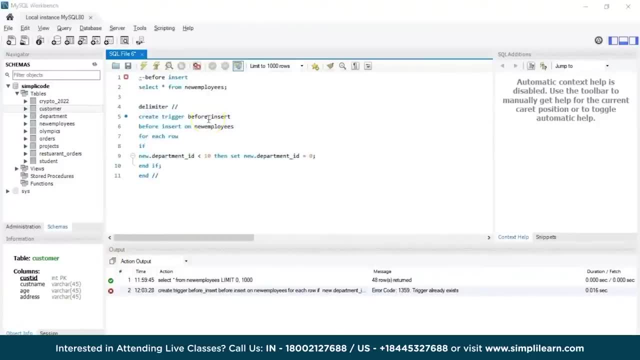 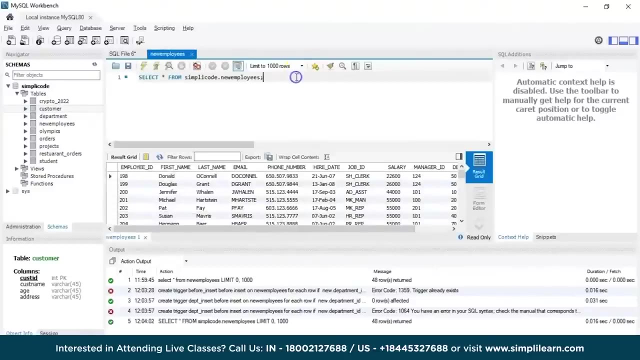 error, so let me just so it says that trigger already exists. might be have taken it already, so let me just change it and keep it as department insert. so, as you can see, a trigger has been successfully created. now let us consider the new employee table again and let us insert some values to understand how. 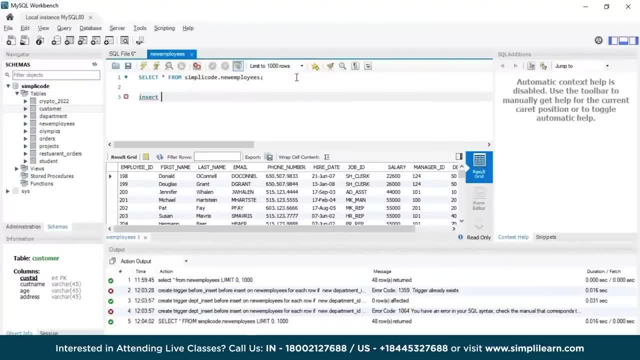 this works. so I'll be inserting some values here. so I'll be inserting some values here into the table, so I'm using insert into new employees values. so mention the employee ID, let's say 288 comma. mention the name of the employee: first name, let's say Carl, and the last name as Haddon. next we have email, so let's take. 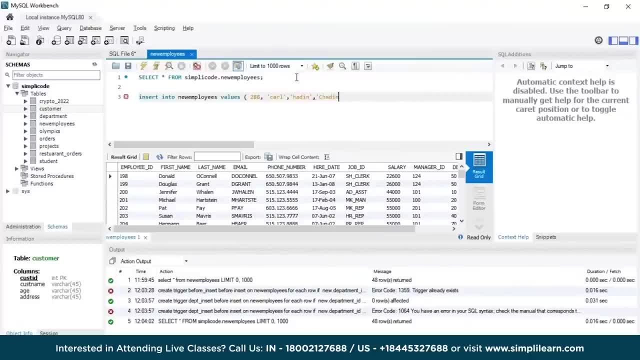 see Haddon. next we have phone number this type, a random number. next we have hiring date, so let us take as 15th June 2009. next we have job ID: let's take shclerk as our job ID. next we have salary: let's take 35,000. next manager ID: let's take one. 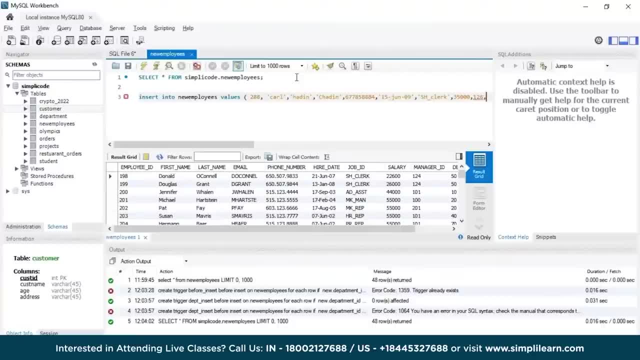 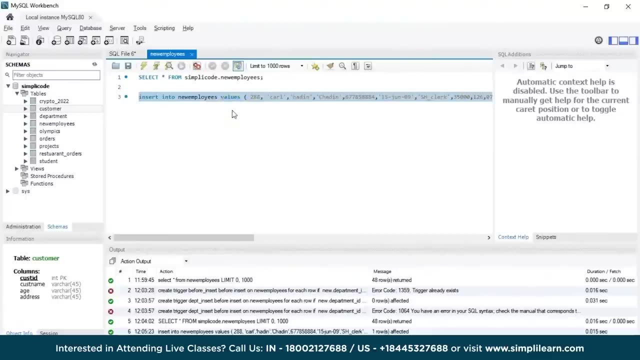 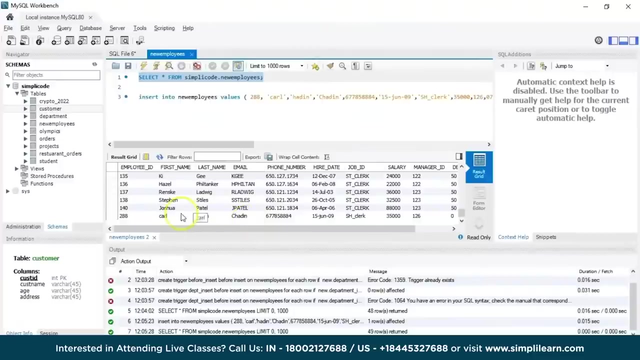 20, five or manage six. next, we have the department id. so we are I'm taking the department IDiyoruz seven, right? so let us just execute this statement and we'll see the output. so our record has been inserted, so let me just retrieve the values again. so if you scroll down a bit, we have our new leaders of our employee. 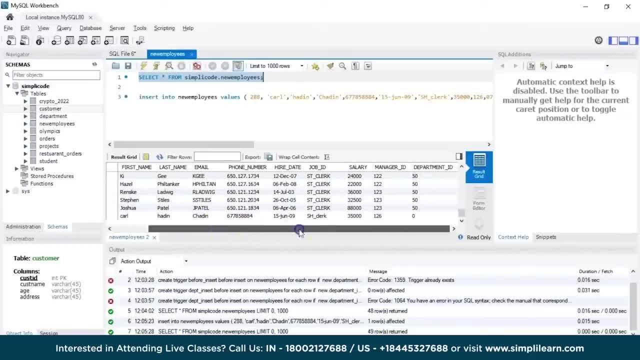 having employee ideas 288, whose name is Carl Haddon, and if you scroll down a bit we have our new Criminal Da boom, we added our first employee as her name is Carl Haddon and if you slide a bit and you can see that, since we have inserted the department id value as 7 and the 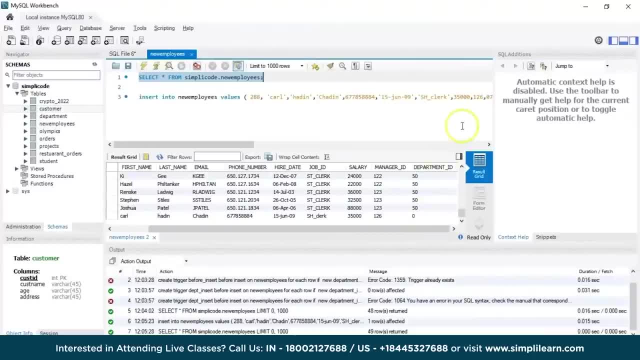 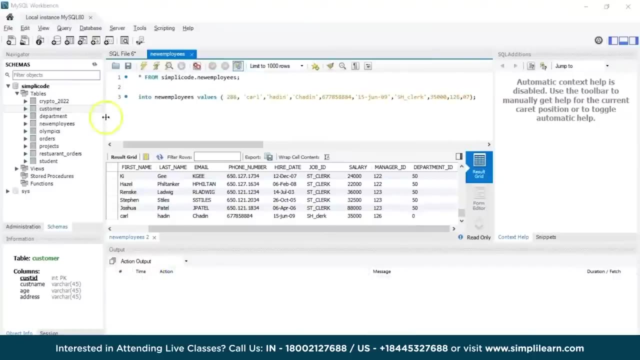 trigger will automatically be created here, which is: department id is less than 10, right? so automatically it has changed the value into 0. So in this way you can use the before insert to create a trigger in your table, Right? so I hope you have understood how to create a before insert. 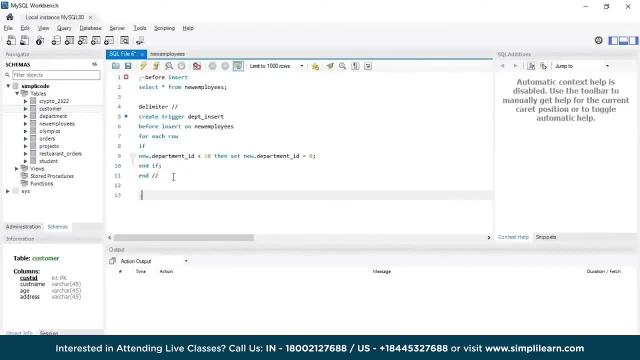 trigger. Let's move ahead. Let us now discuss how to create an after insert trigger. Now, after insert trigger in SQL is basically invoked automatically whenever an insert has already occurred on the table. So let us just understand this with an example. So let us consider the. 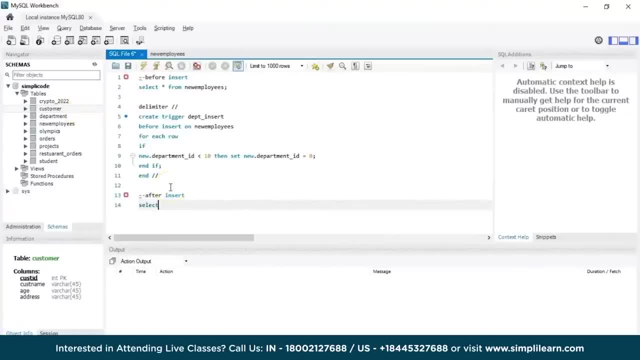 customer tables here. So let us just display the values in the customer table. So so a customer table has four attributes, which is customer id, customer name, age, address, and we have a total of five records. So let us understand how this after insert trigger works. Now we have 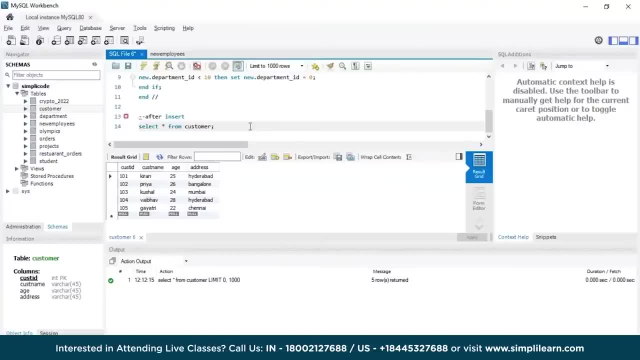 customer id, starting from 101 and 105.. Now, basically, I am going to create a trigger, like whenever a customer's details has been inserted, which is having customer id more than 200. So in that case, I will be inserting this into an other table instead of this customer table. So for that. 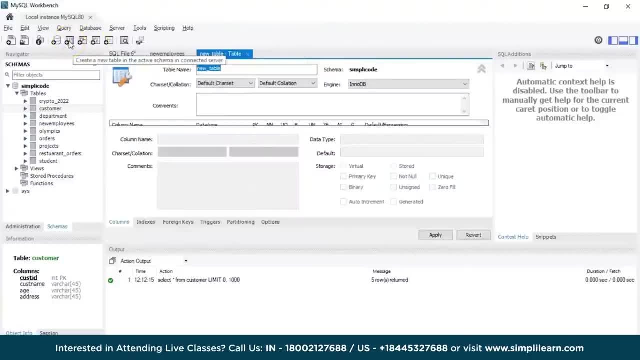 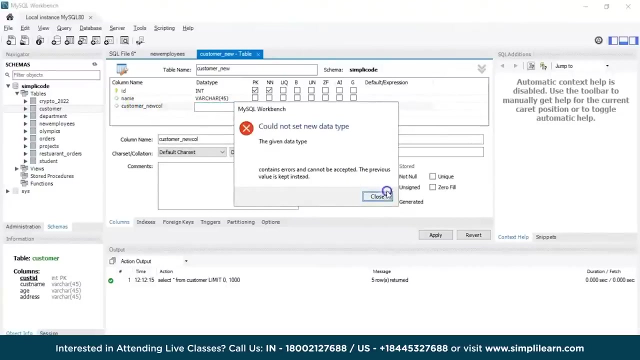 You can tell using the Have peace into adjustment. All right, let me create a new table, So I will then select the system header and then go to have next tab, we, and then we have the age and finally we have the address right. so let us just 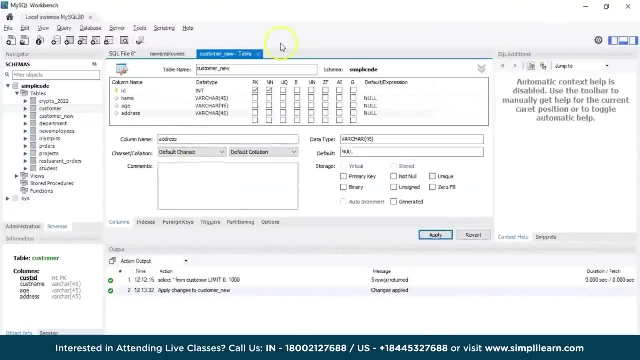 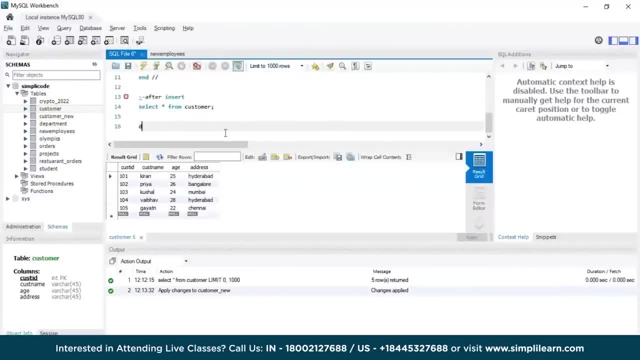 apply and we'll create a new table. all right, so we have created a new table, which is customer new here. so let us now write the syntax for after insert. so I'm again using the delimiter and let us create a trigger now. create trigger. so I'm taking the trigger name as again after insert. you can take it as for your. 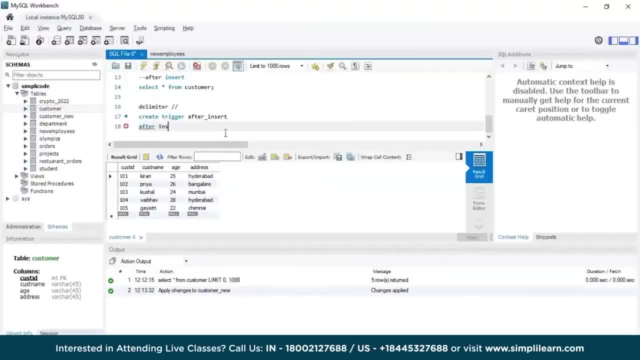 own choice. so, since we are creating after insert, mention the after insert on the customer table for each row now begin. so let us now created trigger here. so the condition that we have taken is if new dot cust id is greater than, let's say, 200. so in that case, insert into. 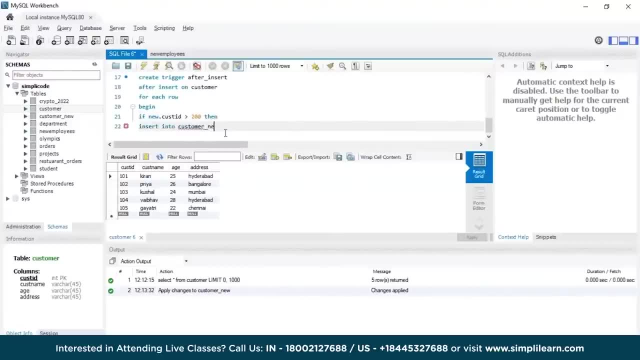 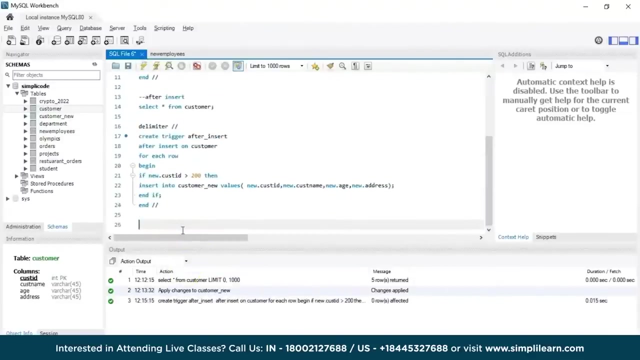 customer, new values, new dot cust id comma, new dot customer name, and then we have newage comma, newaddress, right. so let us just close this and we have the end if double slash. so let us just execute this query and we'll see the output. so our query has been successfully executed. let us now try to. 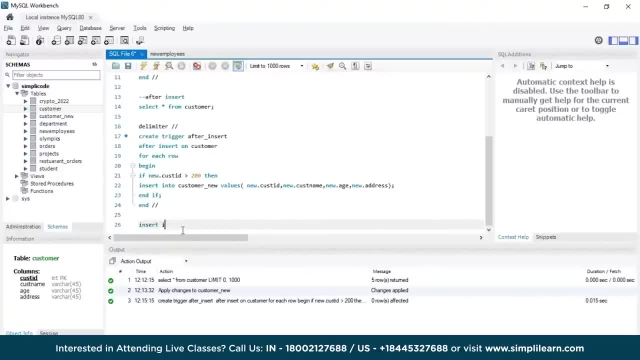 insert some values into the customer table. so I'm using the insert into again, insert into customer values, so customer ID. let's say I'm taking 108 name of the customer, let us say Trier, let us take the age as 24 and address asgee and 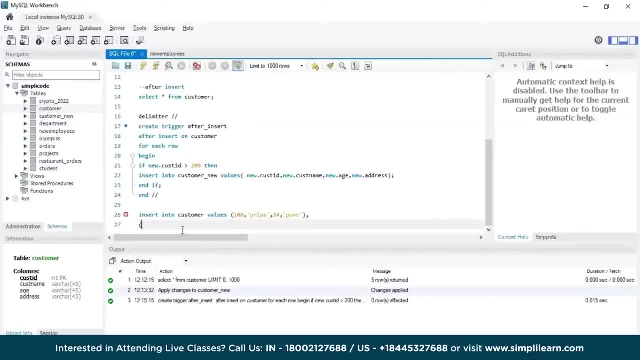 similarly, let us insert some more value. let us now take: do not address the customer ID name as harsh and the age is 27 and address as you should like. let us fragments by final record, which is, let's say, 180109 comma. name as Sam, age, 24, city. let us. 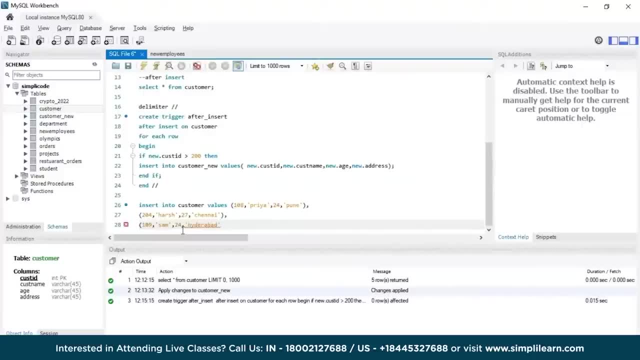 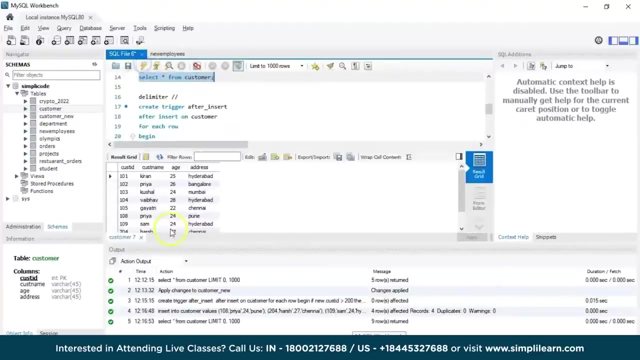 take Hyderabad, close the brackets and let us insert one more final record. let us take 214 as the customer ID, and the name will be John, age 25 and city will be Mumbai. right, so we have inserted the values into our customer table. so, as you can see, four rows have been inserted, so let us just display the records again. so 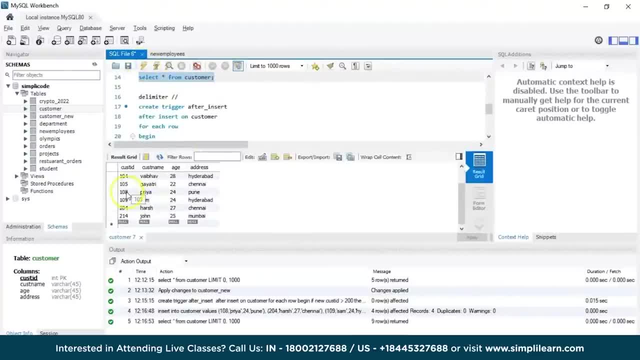 as you can see, we have four new records of the customers having customer ID 108, 109, 204 and 214. now let us see whether our trigger has been created or not. so let us display the values from the customer. new table now select star from. 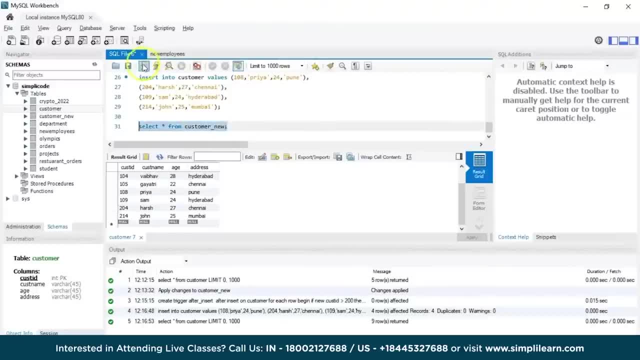 customer new. so, as you can clearly see that, the trigger that we have applied to our table is whenever the customer ID exceeds 200. now, in this case, we have two IDs of the customers, which is 204 and 214. in that case, the trigger will automatically insert new values into the 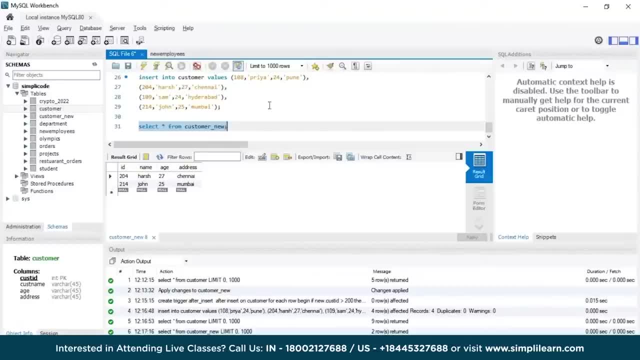 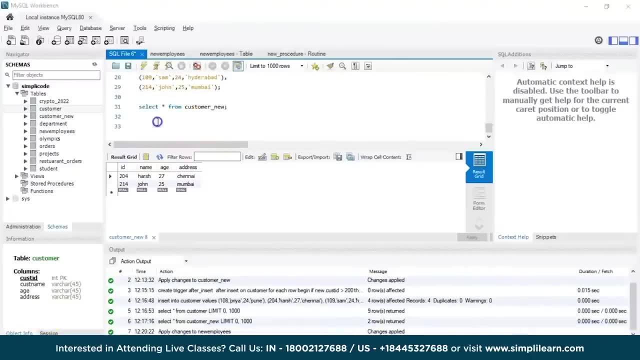 new table instead of the previous table, which is customer. so in this way the after insert trigger works all right. moving ahead, let us now discuss about the before update in our trigger. now, before update. a trigger in SQL is invoked automatically whenever an update operation is performed or fired on the. 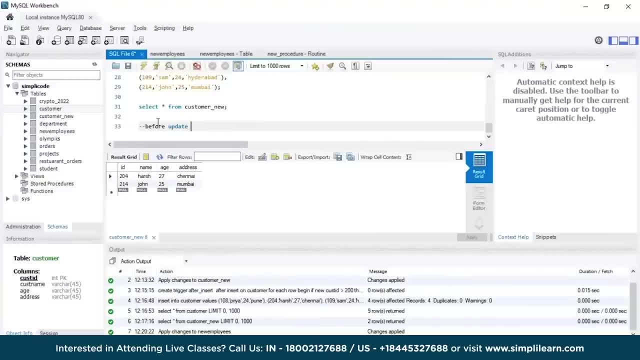 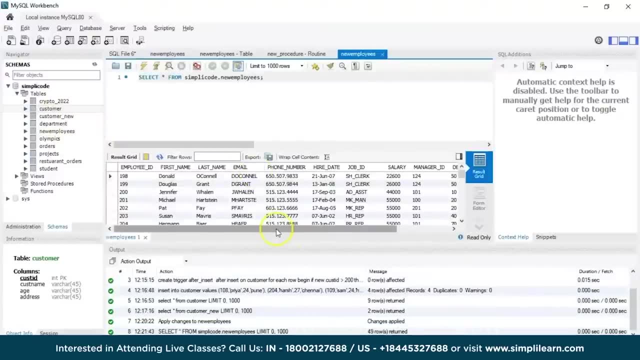 table associated with that trigger. so let us just understand this with an example here. so let us just consider again the new employees table here, for our reference, added another attribute which is bonus in our table. now, basically, the trigger which are going to create will be of this sort: wherein, if you're 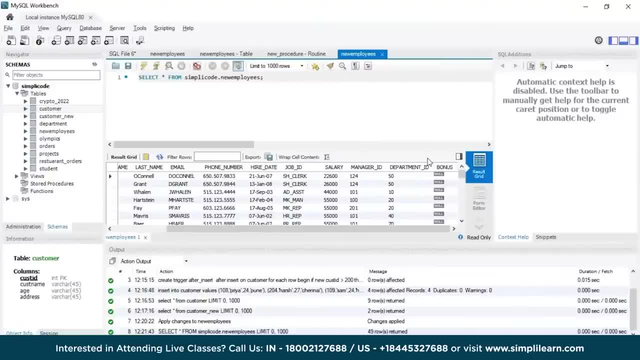 updating the salary of the employees. let's say, if you're updating the salary of employees whose salary is greater than 40,000 or 50,000 or 40,000, then we will set the bonus value as 5,000, and if the 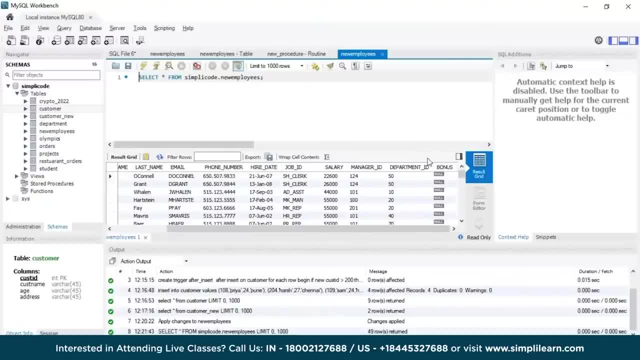 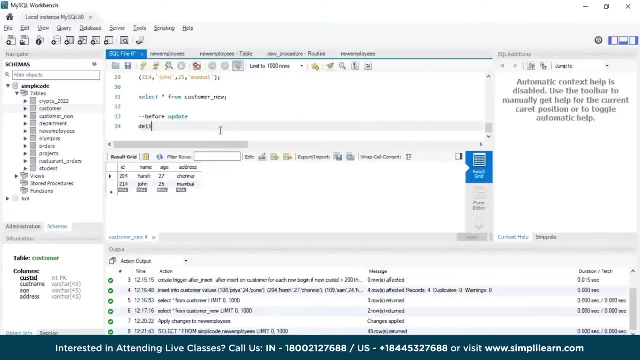 salary is less than 40,000. in that case, their bonus will be 3,000. so let me just write this entire so that will have a clear understanding of it. so we'll use the delimiter again. let us create a trigger update bonus. so we are creating 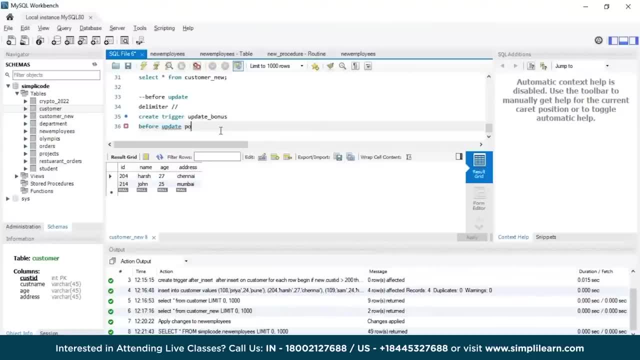 before update trigger. so I'm writing the before update keyword- new employees- for each row. since we're performing on all the rows, mention the begin statement and mention the condition now. so the condition is basically is new dot salary is greater than 40,000. so in that case the 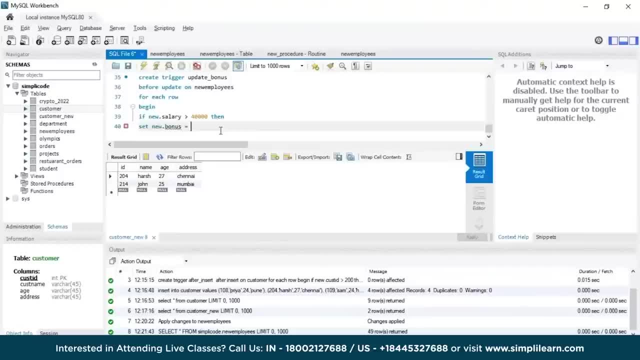 new bonus value will be equals to 5,000. so else if, if the salary- new dot salary- is less than 40,000, so in that case we'll set the bonus value as 3,000. set new bonus equals to 3,000. so mention that. 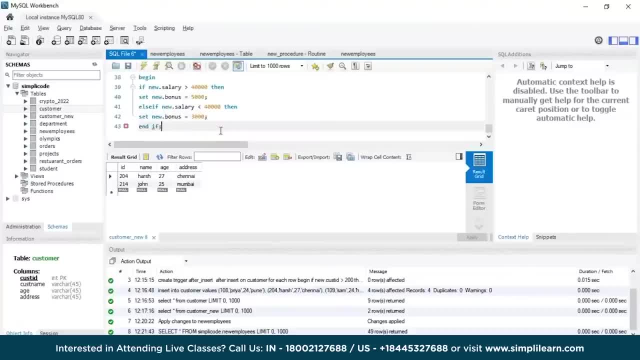 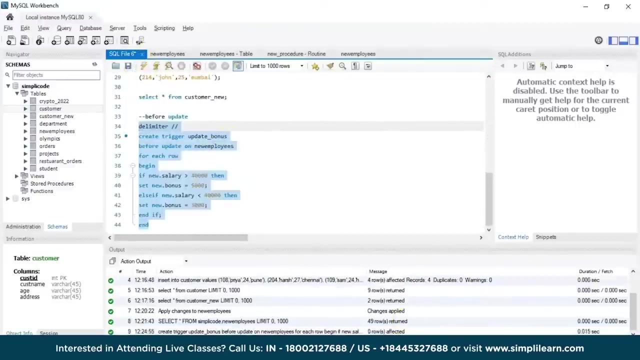 the semicolon and mention the end if, since we have used to end if statements, if statements. so we'll mention and if two times before we close our statement here. so let us now execute this statement and we'll see the output. so our query has been successfully created here, guys. let us now update the. 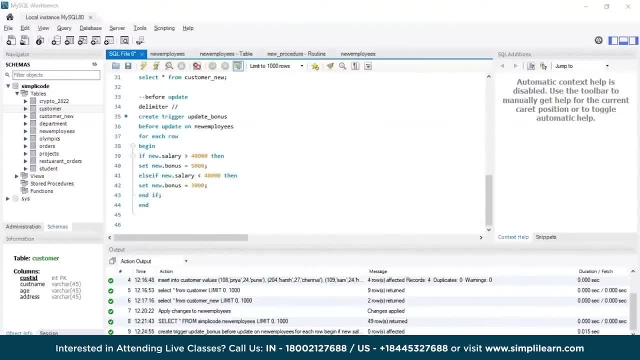 values in our new employee table. so let us write the update statement here. so I'm updating the new employees table, so update new employees. set salary equals to, let's say, 45,000 for only limited employees, let's say, whose employee ID is more than 200. so I'm just taking our reference. 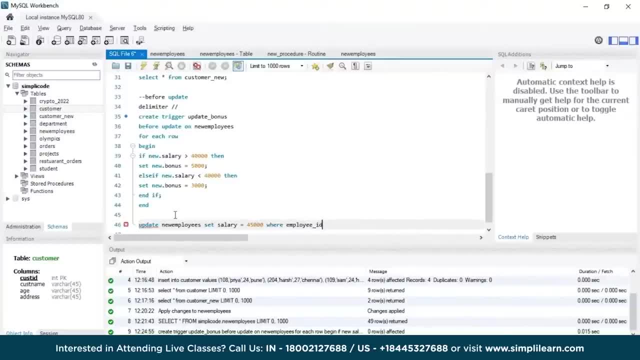 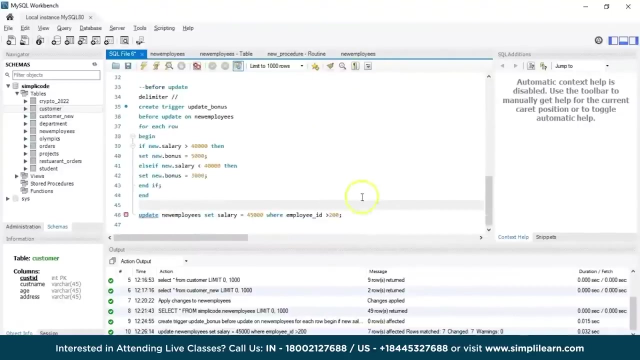 here, or just an example or a scenario, so that we'll have an understanding on how this before update trigger works whose employee ID is greater than 200. so right, let us just execute the statement. so, as you can see, seven rows have been affected. so let us now display the new employees table again. so I'm using the 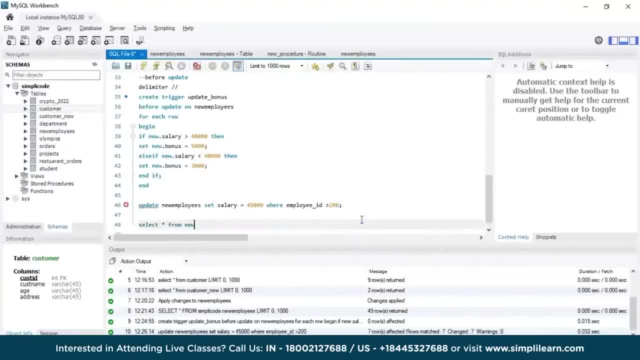 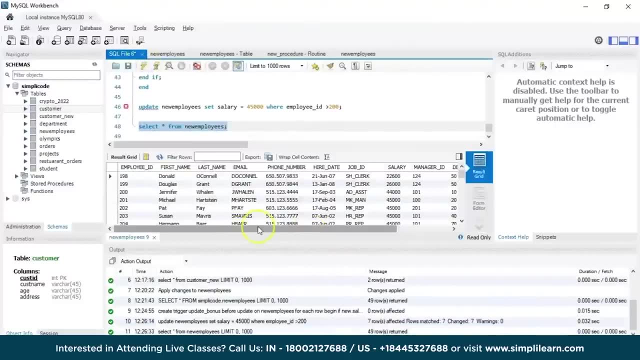 select star from new employees. all right, so let us move aside and see now, as you can clearly see, that now employees who are having employees ID more than 200 which you have taken in our query now, if you can see, employee ID of Michael Haston is 201 and Pat Faye. 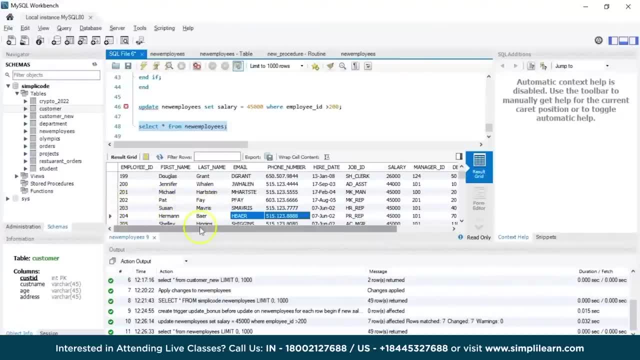 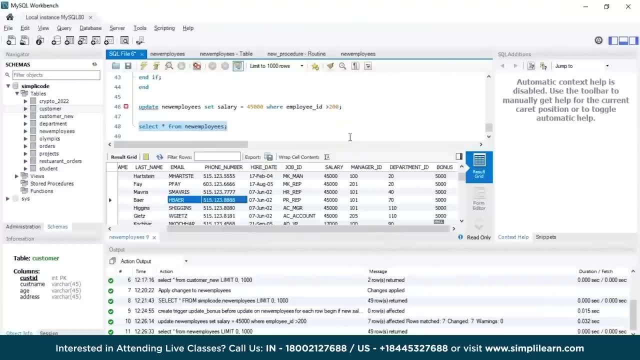 which is 5000, which is basically the tree trigger that we have created, that is, if the salary is more than 40,000, in that case will invoke a trigger where it will add bonus of 5000 to all those employees. so in this way, before update, 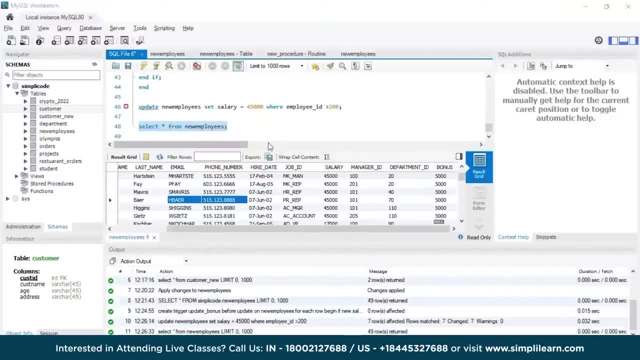 trigger works in SQL, so in the same way you can also create the before and after delete trigger as well. so in this way, before update trigger works in SQL, so in the same way you can also create the before and after delete trigger as well. so now that you've understood how to implement this, and now try to. 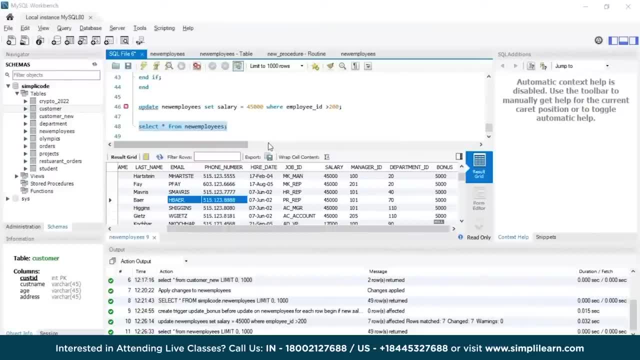 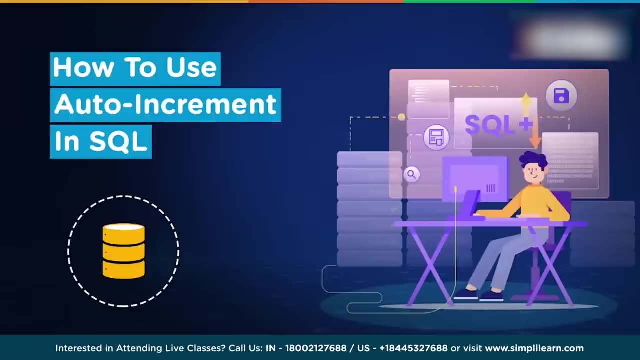 implement this before an insert delete in your system. if you are facing any issues, do let us know in the comment section below will help you out. if you still face further issues, let us know that if you if you want us to create a separate video on those you all know while working with vast databases in SQL. 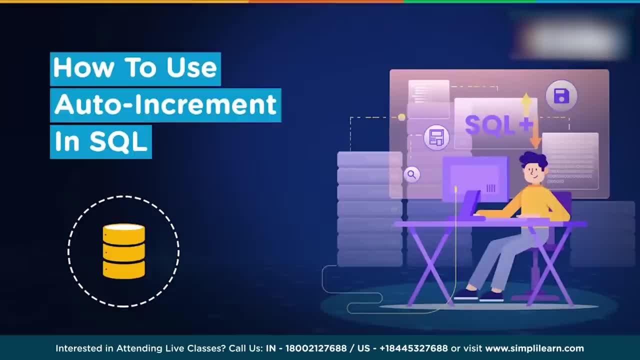 several tables and data fields will require unique numbers. now, for instance, a column of the table with a primary key or a unique constraint will always require a new number. that means in that field you always need to enter a new number and it's not have any duplicate values, so you might be able to do it. 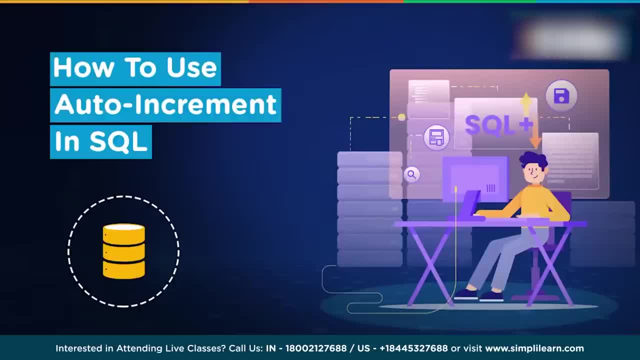 manually to a limited extent, but when it comes to enormous or large or huge databases, you might forget the last unique number you have entered or nearly include the same number twice, as it isn't easy to remember everything right. besides it, providing a unique number to all the records is also a tedious task. 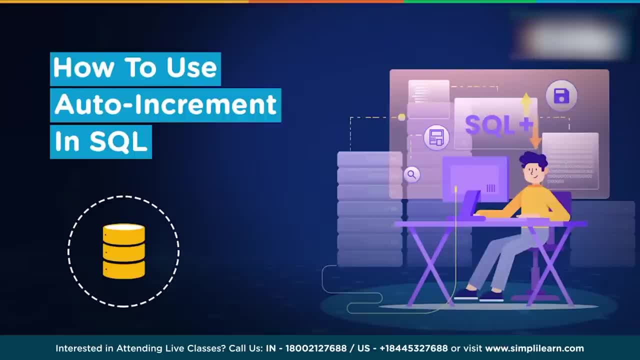 and that's where auto increment in SQL comes to play. so in this tutorial, we are going to discuss what exactly is auto increment in SQL and how to use it. so without any further delay, let's get started. let us now jump head into my SQL workbench for execution part. 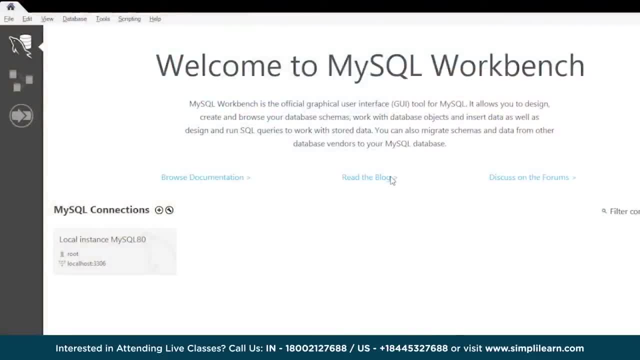 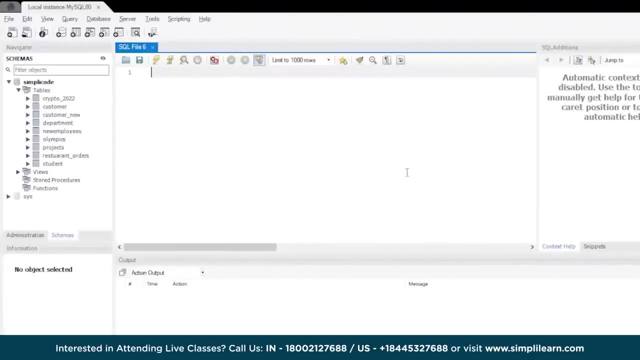 so, as you can see, my SQL workbench has started. let me just enter the password to enter into it. all right, we have logged in into our my SQL workbench. so before getting into the execution part, let us just quickly understand what is auto increment. now, the auto increment in SQL is basically a. 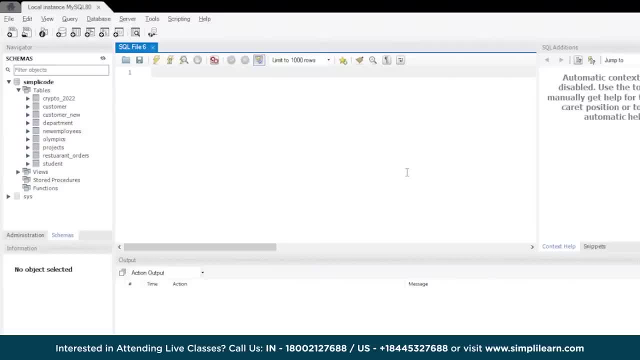 feature that is applied to a field so that it can automatically generate and provide a unique value to every record that you enter in an SQL table. now, this field is often used as the primary key column, where you need to provide a unique value for every record you add. however, 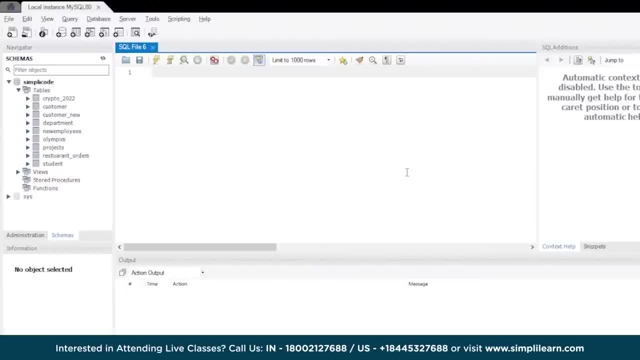 it can also be used for unique constraint columns as well. So let us now understand this with an example here. So let me just create a new table so that we can implement it. So let us create a new table here which is, let's say, orders. 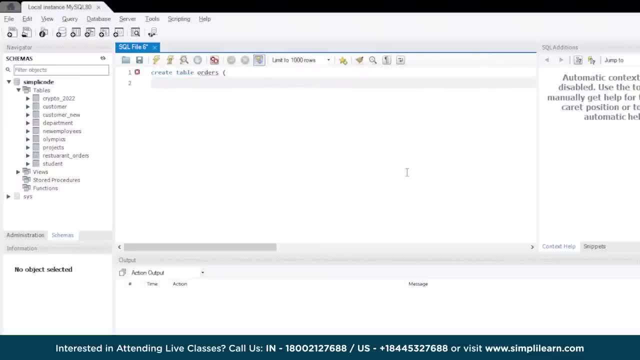 Open the parenthesis and let us now mention the columns that you want to create. So let us take the first column as product id, and product id will be of int and we'll make sure that it is not null, and then, if you're working on SQL, it applies an auto increment field with 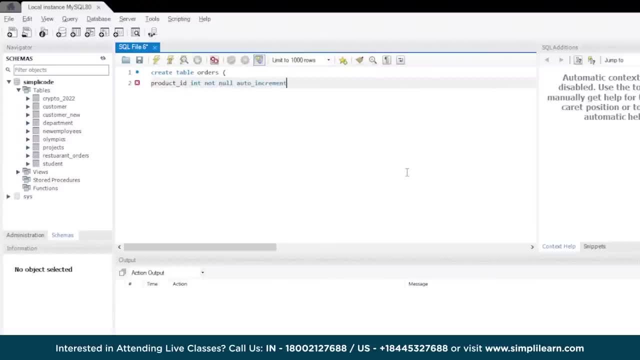 the keyword as auto increment, So we'll write it as auto increment and then comma mention the next. let's say: let us take as customer id in our orders table and I'm again giving int as the data type for this, and again we cannot have customer id as null. so I'm mentioning the constraint, not null. 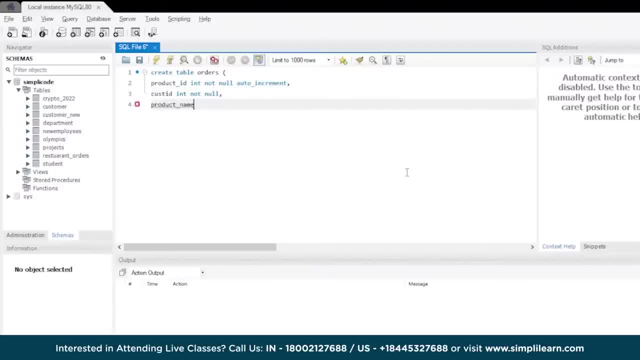 Next, I'm mentioning the product name, that is, the list of orders that the customer has placed and the name of that product, and here I'm taking the data type as varchar and I'm taking its size of up to 20.. Next, let us take, let's say, quantity. 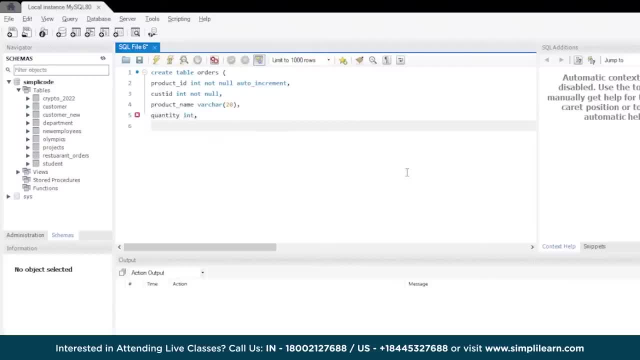 and let us now take it as int data type. and next and finally, we'll take price, which would be again of varchar of 20 size. So that's it: mention the comma and let us close it. So let us just execute the statement. there is an error. 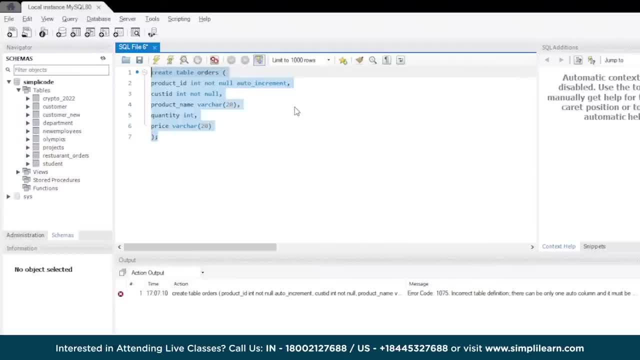 So let's do that. So I'm going to be ready for my show. Okay, so I'm going to be ready for my show. So I'm going to be ready for my show. So I'm going to be ready for my show. 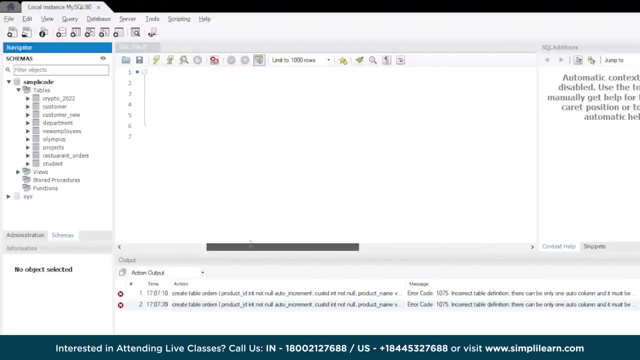 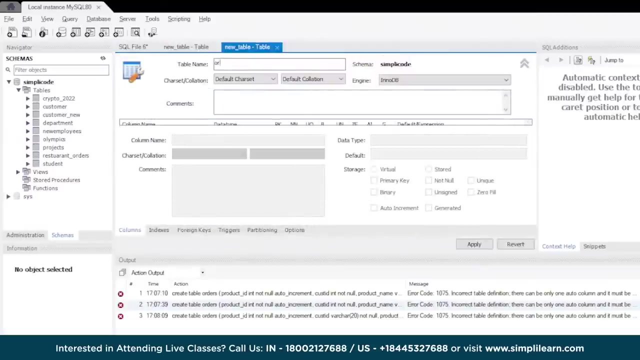 I don't know, guys, why it is showing as error. let me just check it once. so I think there is an error. so let us just create a table using this icon here, so orders, and let us mention the column names here, which is customer ID. sorry, first one will be product ID. 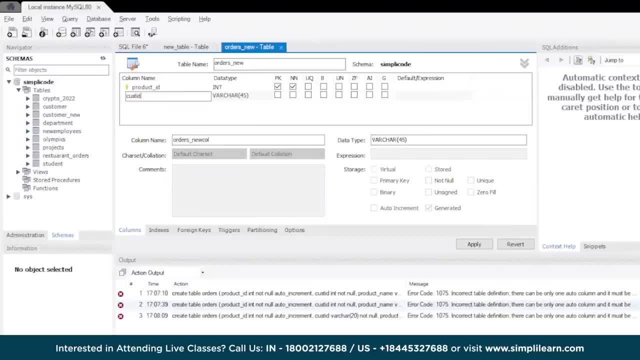 we have customer ID and then we have product name, quantity, and finally we will take the price, alright. so let us give a. we have customer ID, and then we have the product name and then quantity, and finally we will take the price here, alright. so let us give a. 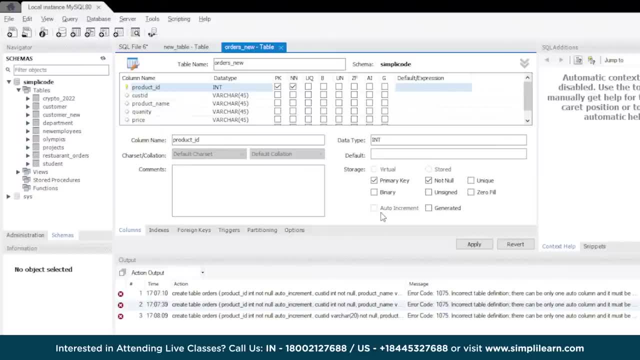 the product ID as the auto increment. So click on this auto increment value, where you can find it as AI, and let us now execute. click on apply and our table will be created. So, as you can see, our table has now created, so let us now just insert some values into. 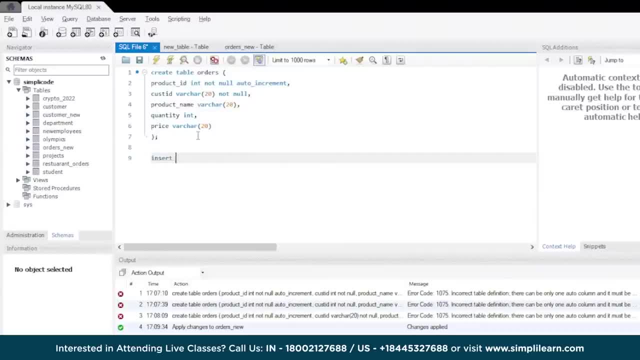 it and we will see the output. So mention the insert into mention the table name, that is, orders. Now, in order to insert the values into it, you need not write the product ID column here, So we will just directly write the customer ID and we will see how the auto increment. 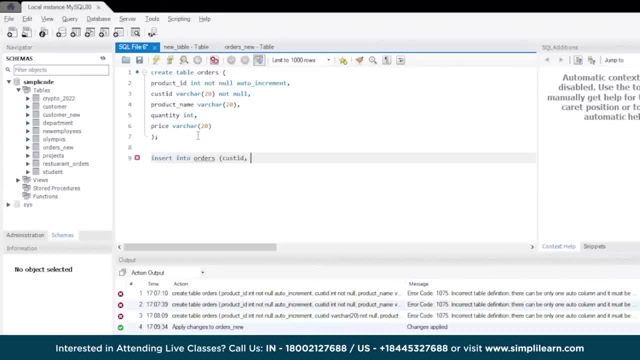 directly works. So customer ID. next we have product name. Next we have quantity, Next we have price and mention values and insert some values. So customer ID, I will just take it as 101.. Next product name: let us take as AC for quantity let us say 2 and price will be 60,000. alright, 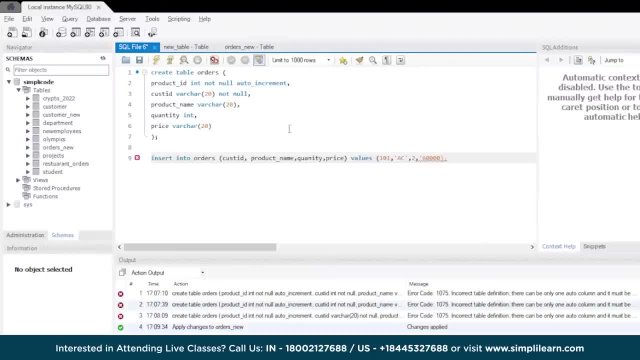 And similarly, let us insert another value here. Next we have quantity. I am taking the next order, customer ID as 102 and we will take the next product as cooker And close in my single brackets. next we will take quantity 1 and price will be 25,000. sorry, 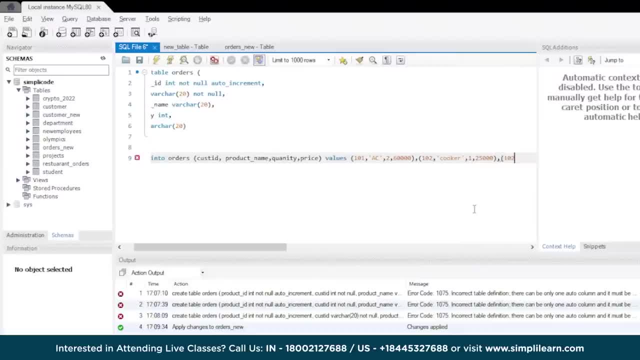 And finally, let us take another example. let us say 102,, 103. Comma, let us say phone as our next product name, and we will take the quantity as 3 and the price will be 90,000. alright, We are good to go now. 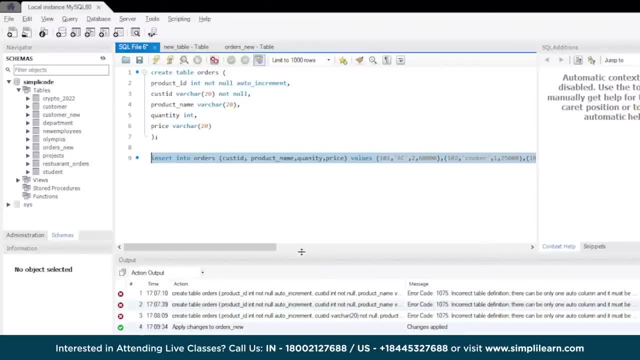 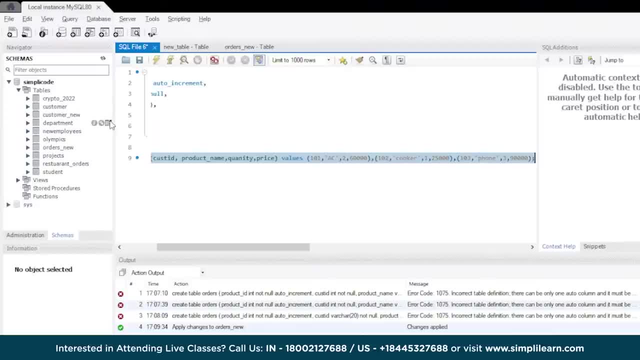 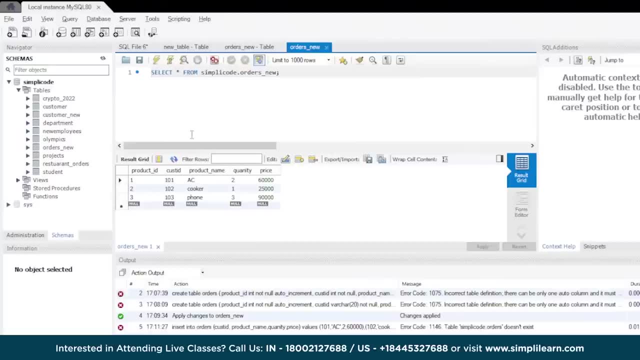 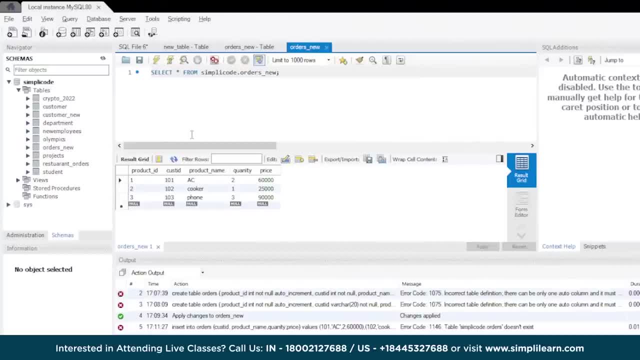 statement and it is automatically generating the values like sequential, starting from one, two and three. Now you can also make an auto increment in SQL to start from other value with a following syntax as well: guys, now let's say if you're working on an employee table. or let's say if you are working: 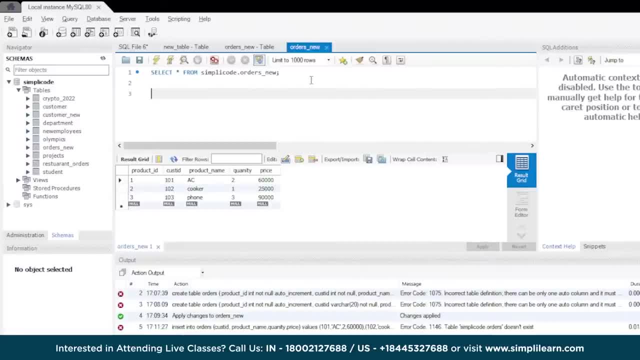 on any other student table, for example, in that it might be of different digits, like the employee id can be of five digits or six digits. so in that case you have to change the order in which you want to create and increase the employee ids, right? so in that case, what we'll do is we'll write. 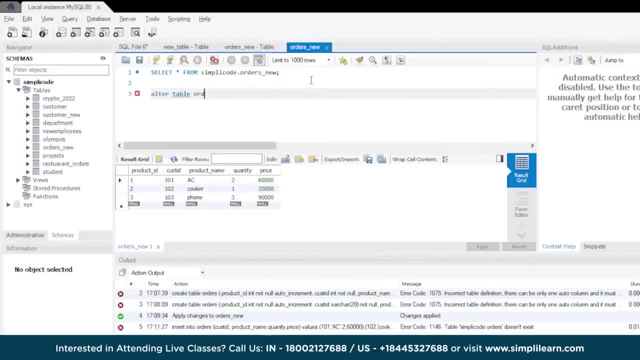 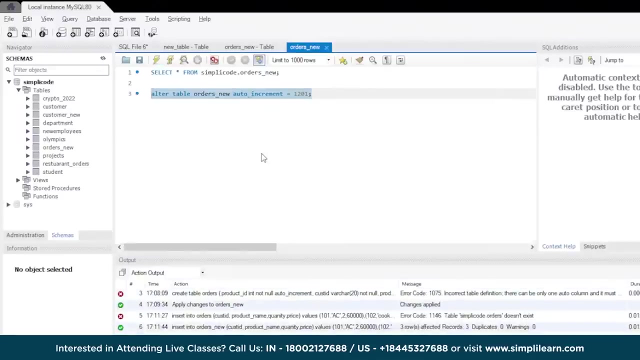 alter table and then mention the table name. so we are taking orders- new table here- and mention the auto increment keyword and set from where you want to start it. so let's say, if I want to start it from twelve thousand and one, right, so let us just execute and we'll see the output. 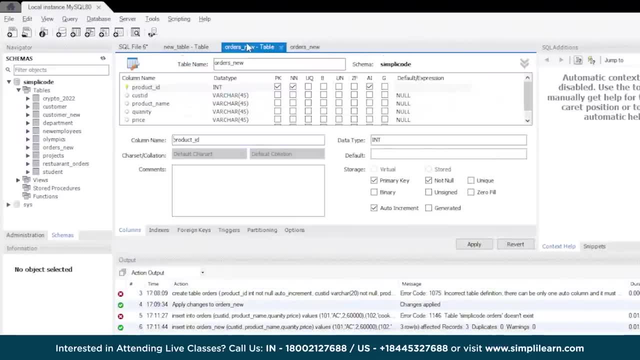 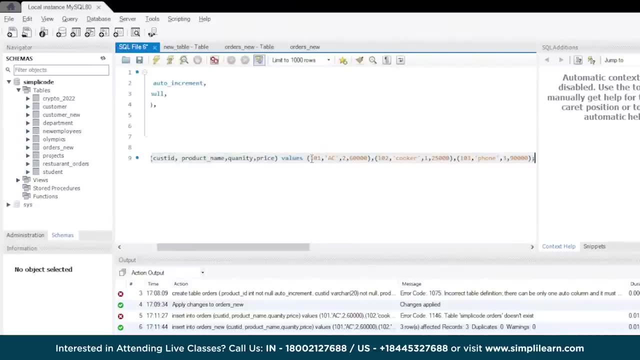 so our query has been executed. so let us now insert some more values into our table and we'll see how it goes. so let me just now I'll add some more values like 107 comma, the product name as cooker, let's say the quantity 2 and the price. 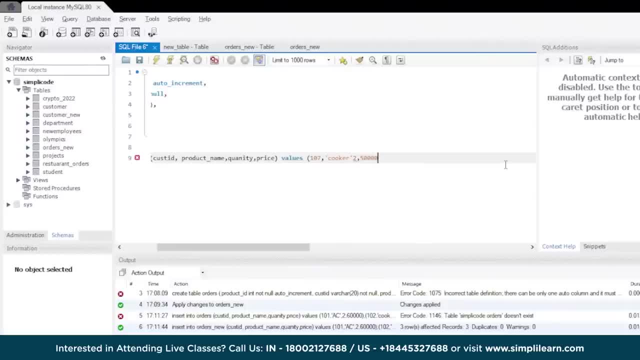 will be 50,000. similarly, let us take another record. let's say 109 comma. let us take as tablet as our product name, and then we'll mention the number of quantity as 4 and price will be 1 lakh 50,000. all right, so let's just. 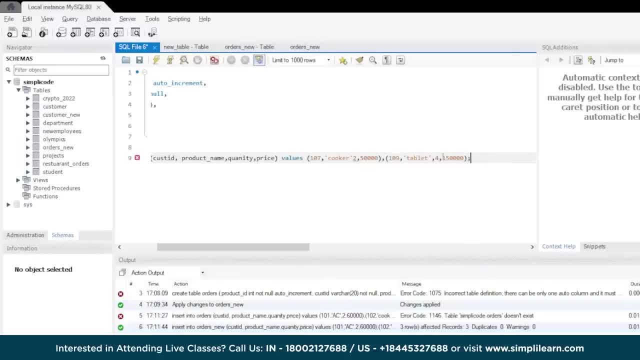 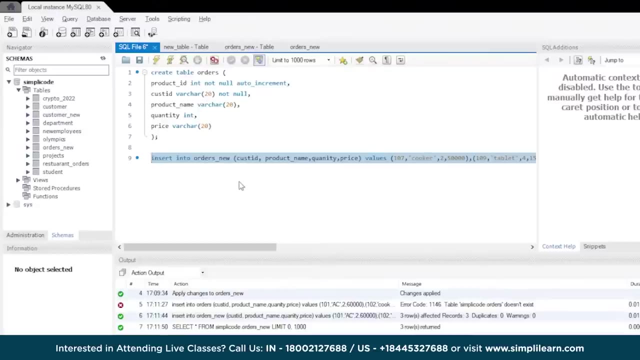 execute the statement and we'll see the output. so two rows have been inserted into a table successfully, so let us just call the orders new table again. so let me just use the select statement, select star from orders- orders. so, as you can see there now there are two records that we have inserted, which. 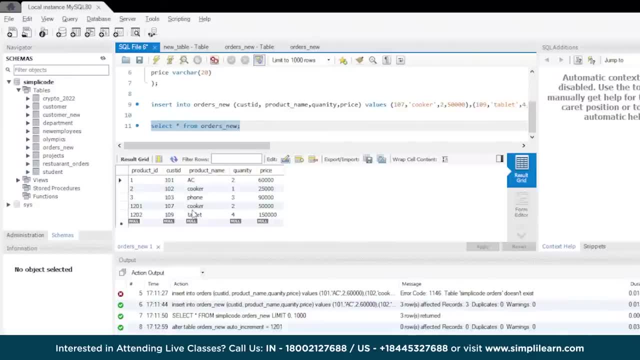 is of customer at ID 107 and 109 and the orders they have placed is cooker and tab. Now, if you look at the product ID, we have started their product ID from 12001 and sequentially it will increase the value by one. that is, now we have 12001 and next we have the 12002.. 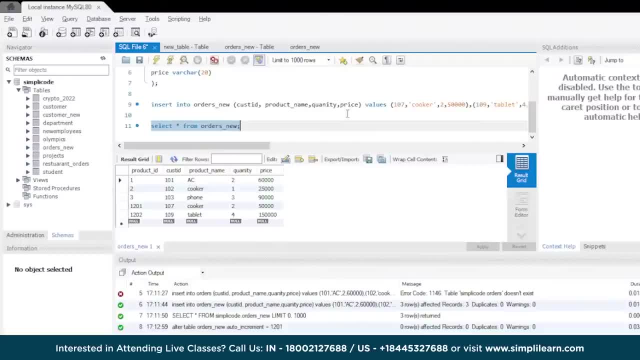 So in this way, you can use the auto increment in SQL to set up values in order to make them automatically update for your database. Now, instead of writing every time, you can just simply mention the auto increment and it will do the job. And if you are working on various other databases like SQL Server or even Oracle, in that case, 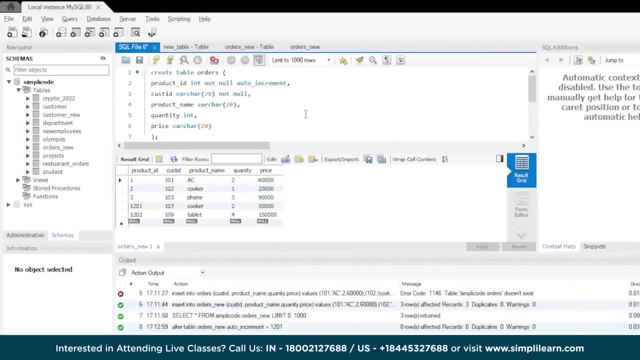 the syntax will change. In that case, what you have to do is, in the create statement, you have to take the keyword as identity and mention the values from which your column values will start. Let's say, I am taking as 100 comma And how much values you want to increment, like let's say, if I mention one, it will increase. 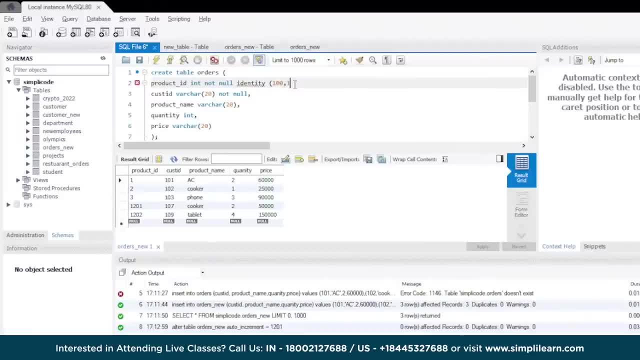 the value by one, like 100, 101, 102 and so on. But if I take it as, let's say, five, then it will start from 100.. Next the value will be 105, 110 and so on. So in this way, if you are working on various other databases, you can use this as well. 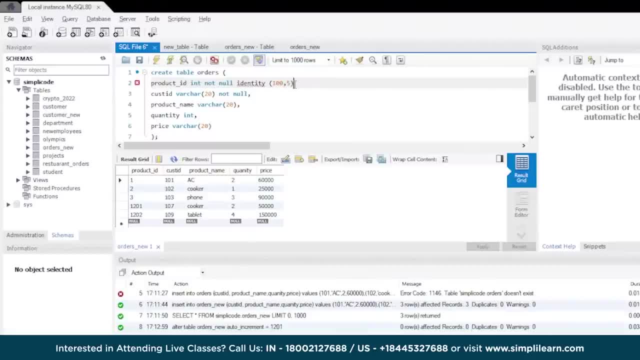 So that brings us to the end of today's session. guys, I hope you understood how to use the auto increment in SQL. So now that you have learned everything about auto increment in SQL and you have gotten the information, Let's move on to the use of auto increment in SQL and to set up in different DBMS servers. 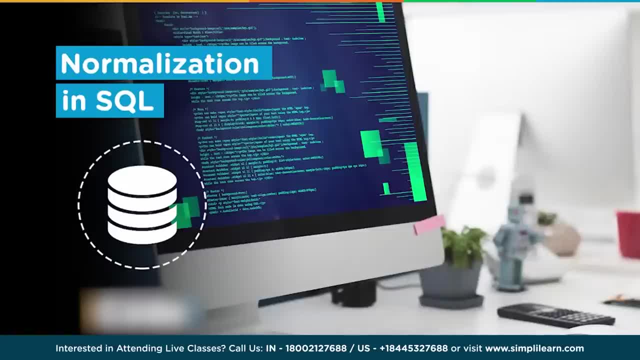 So I hope you can execute in your. as you all know, as a SQL developer, you often work with enormous amounts of data stored in different tables, right So that are present inside the multiple databases. Now, it often becomes difficult to extract the data if it is not organized correctly. 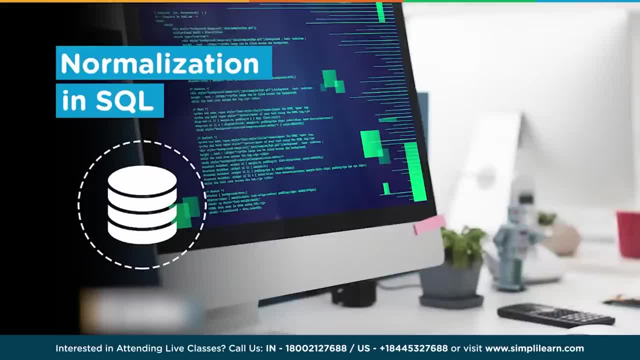 So, using normalization, you can solve the problem of data redundancy and organize the data using different forms. So this tutorial will help you to get, Or know, the concepts of normalization in SQL in detail. So, without any further ado, let us dive into today's topic. 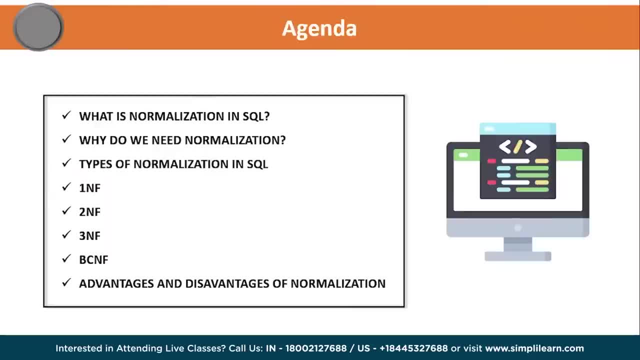 So let me just present you my screen. Firstly, let us go through the agenda for today's session. guys will start the tutorial by understanding what is normalization in SQL, and then we'll understand why do we need normalization, And after that we'll discuss various types of normalization used in SQL, which are basically: 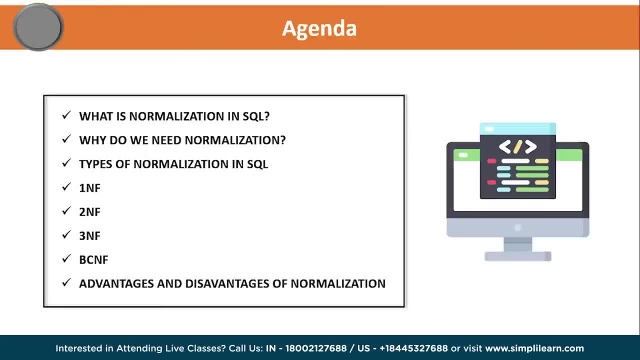 different normal forms, such as first normal form, second normal form, third normal form And finally, we'll wrap up the session by discussing some advantages and disadvantages of normalization. So, without any further ado, let us just dive into today's topic. All right, So what is normalization in SQL? 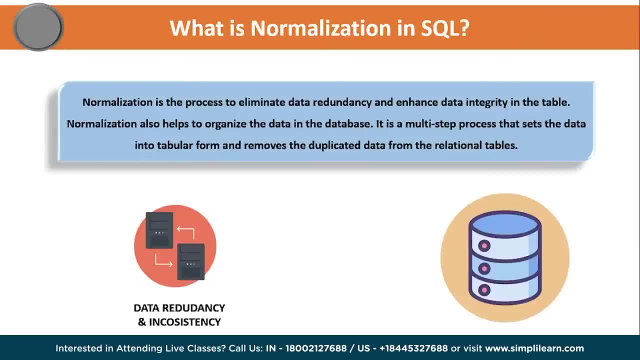 Normalization is the process to eliminate data redundancy and enhance data integrity in the table. Normalization also helps to organize the data in the database and it is a multi step process that sets the data Data into tabular form and removes all the duplicated data, that is, the repeated data. 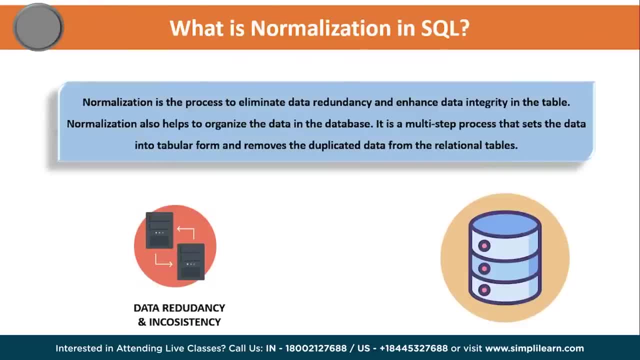 in the relational database tables. Normalization organizes the columns and tables of a database to ensure the database integrity constraints properly execute their dependencies. So it is a systematic technique of decomposing tables to eliminate data redundancy and various other undesirable characteristics. Now to better understand this concept, it simply means to bring something to its normal state. 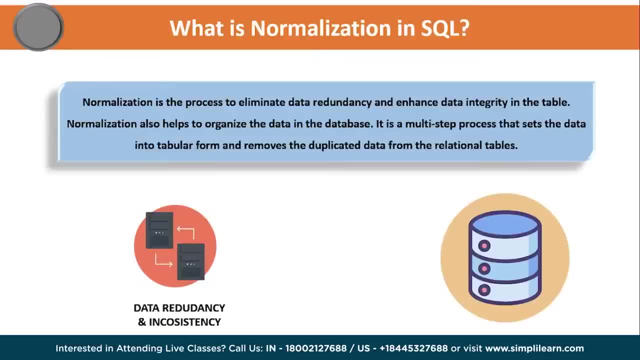 Now, from that what I mean is that columns and tables are organized to ensure that the data integrity constraints are appropriately executed, with their dependencies in normalization. So normalization in SQL is mainly used to reduce the redundancy of the data. SQL is a language that interacts with the database. to start any interactions with the 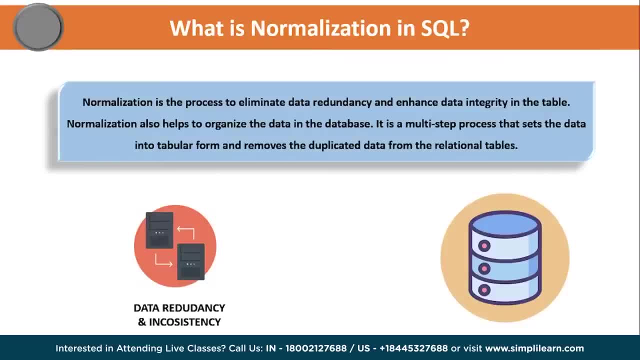 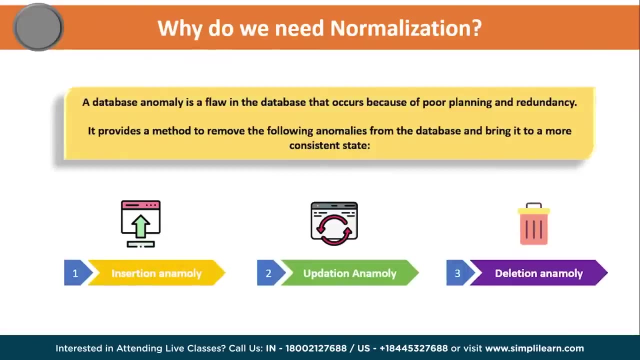 data in the database. The data which is present in this database should be the normalized form before it is processed further. So that's why normalization in SQL improves the data distribution in the database across. Next, why do we need normalization Now, as discussed, 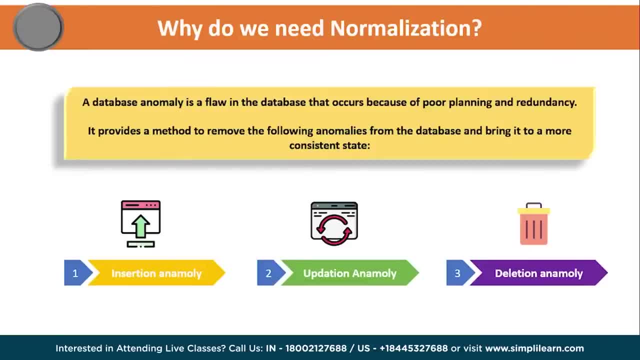 earlier. normalization is used to reduce data redundancy, which is the most important thing, so it provides a method to remove the falling anomalies from the database and bring it to a more consistent state. Now, a database anomaly is a flaw in a database that occurs because of various reasons, such 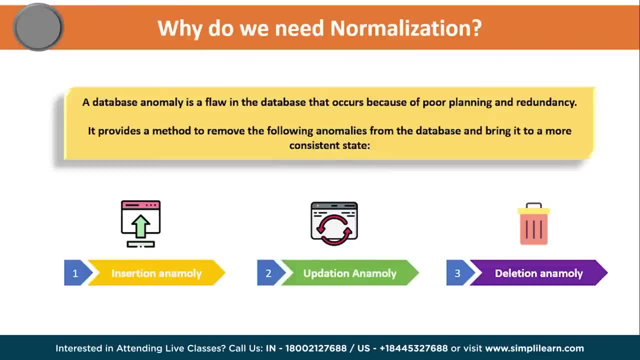 as poor planning and redundancy. Now there are various reasons, such as insertion anomalies, which occurs when we are not able to insert data into a database because some attributes may be missing at the time of insertion. Next, we have updation anomaly as well, which occurs when the same data items 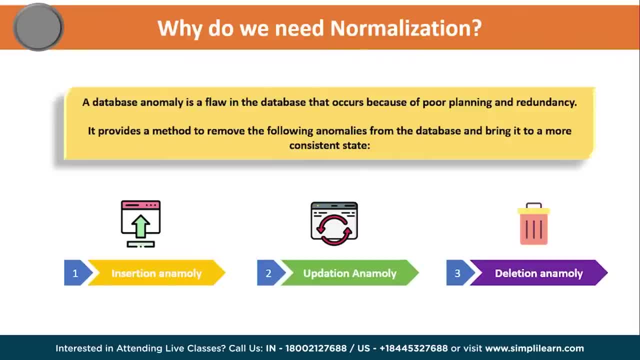 are repeated with the same values and are not linked to each other. and finally, we have deletion anomaly, which occurs when deleting one part of the data deletes the other unnecessary or necessary information from the database. So that is the reason we need normalization. So, if I put them, 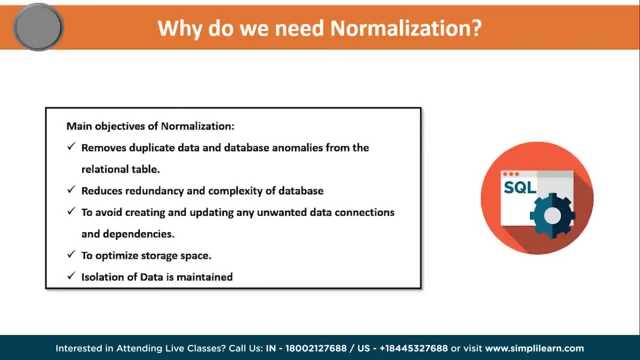 into a nutshell. these are the main objectives of normalization, guys. So the normalization removes duplicate data and database anomalies from the relational database. It also reduces redundancy and complexity of database by clearing unwanted records or values in the database. It is also used to avoid creating and updating any unwanted data connections and dependencies. Now if 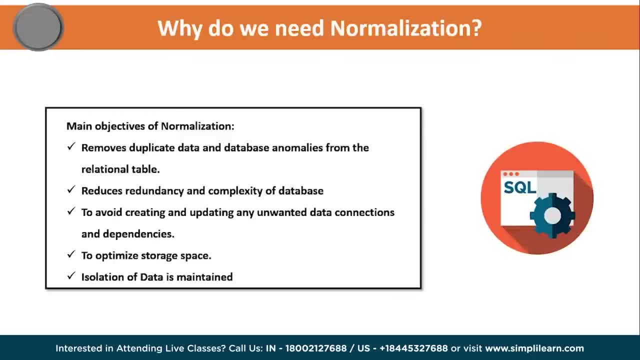 you are working on a multiple tables, there may be a chance of unwanted connections, So normalization prevents that. It is also used to optimize storage space as well. guys, Now you don't want unnecessary or repeated values in your database or tables, right? So to organize and optimize the 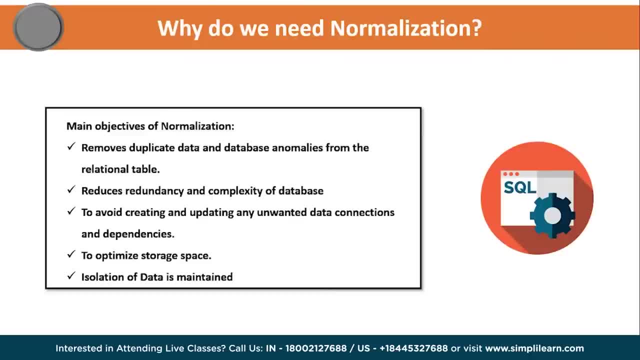 storage space. we need normalization. And finally, isolation of data is also maintained. Now, a good design database states that the changes in one table or field should not affect each other, So this can be achieved through normalization. So these were some of the important characteristics of normalizations and 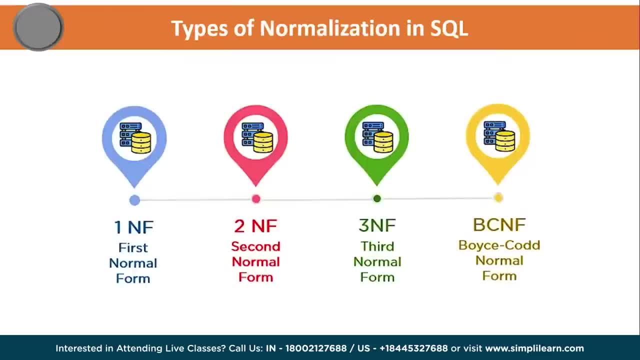 why we need it. Alright, moving ahead, let us now discuss some different types of normalization in SQL. Now there are four types of normal forms that are usually used in relational database, as you can see in the following figure. The first one is first normal form, or 1f. Next we have second normal form, or 2nf. Next we have 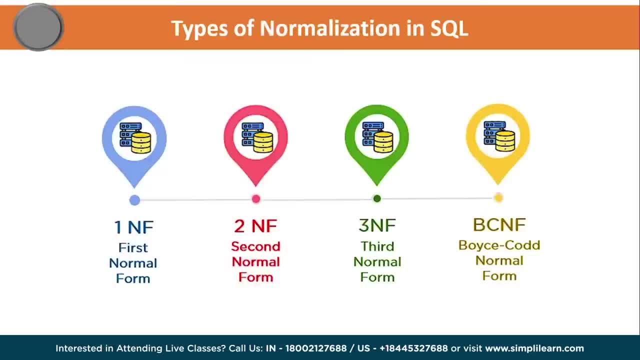 third, normal form, or 3nf, and finally we have Boyce-Codd normal form. Now, actually, we divide the normalization process into a set of normal forms. so a normal form is nothing but a form of a table that follows some rules or regulations that prevent the above anomalies that we have discussed earlier. 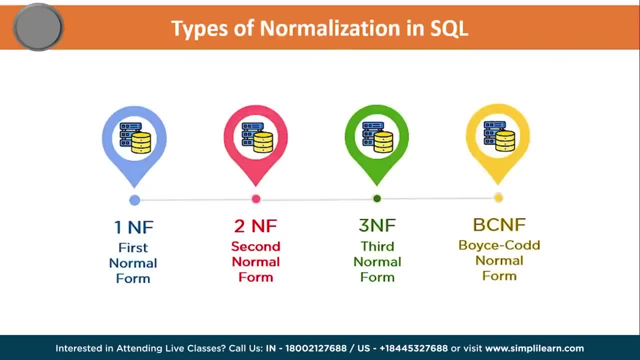 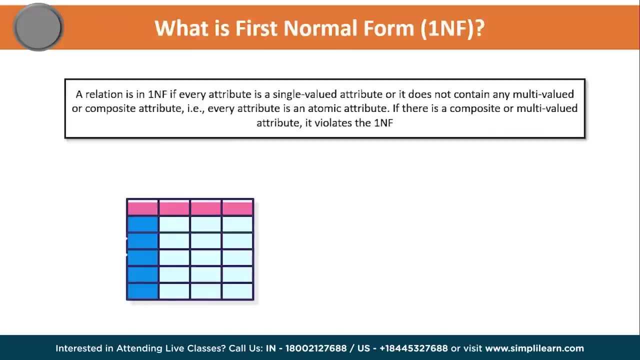 to some extent. So let us discuss about them in detail and see how they are different from each other and understand why they are important. So first, what is first normal form or 1nf? Now a table is referred to as being in its first normal. 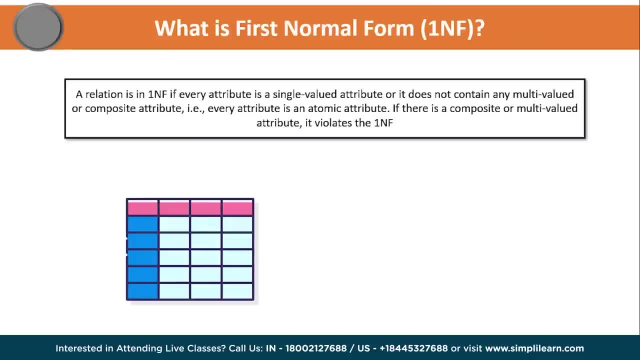 form if atomicity of the table is 1.. Here atomicity states that a single cell cannot hold multiple values. It must hold only a single valued attribute. The first normal form disallows the multivalued attribute, composite attributes and their combinations. 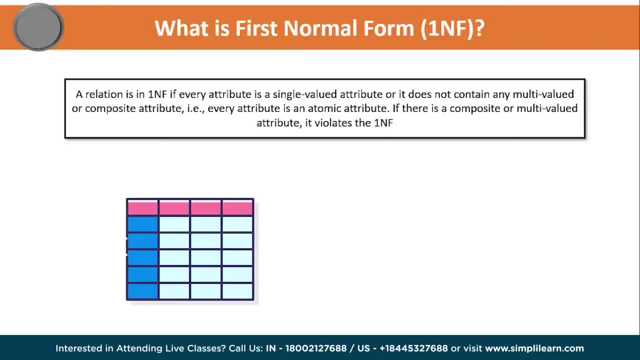 I hope this is quite a bit confusing, So let us just understand the first normal form with the help of an example. So these are the two conditions which I have already discussed, that the conditions for a table to be in first normal form is that every table cell should. 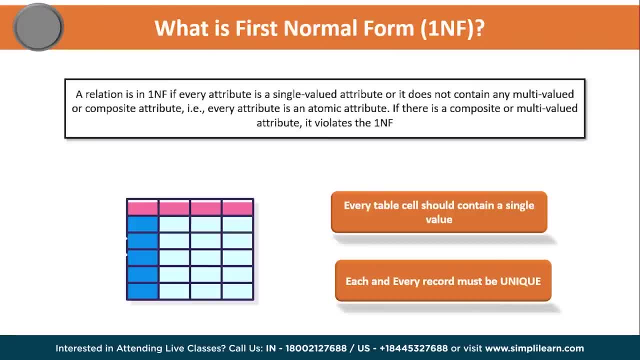 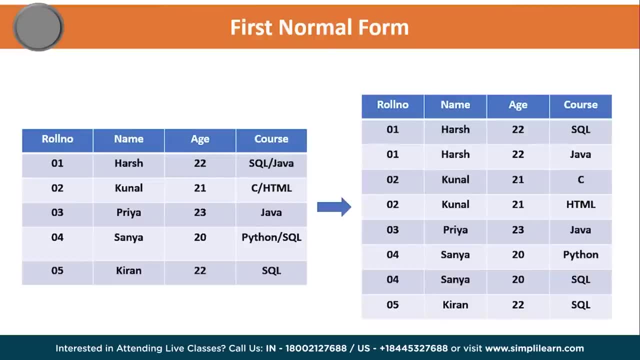 contain a single value and each and every record must be unique. Alright, let us understand with an example. Now, in the student table, let us say you can see, the course column has certain values. So if you look at some of the courses assigned to each student, we have 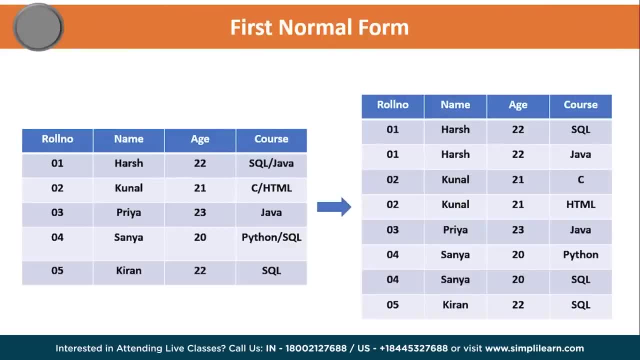 more than one column. that is the course. column has two values, thus it does not follow the first normal form. Now, if you use the first normal form to the above table, you can get the below table as a result. If you look at the side, the second table, in that we have basically divided the 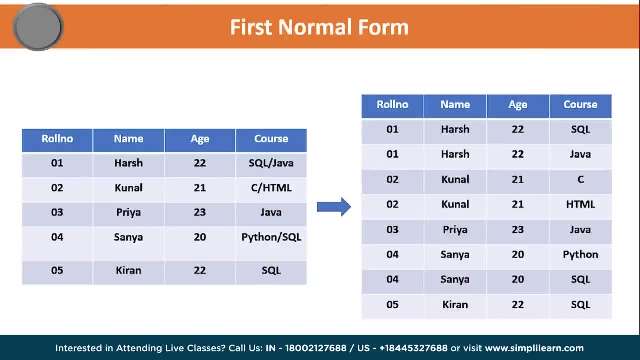 record into two parts. that is Harsh, whose roll number is 1, who has enrolled in courses SQL and Java, which we are basically dividing into two records separately. that is Harsh 22 SQL course and similarly Harsh 22 into Java, And similarly we have for Kunal as well. 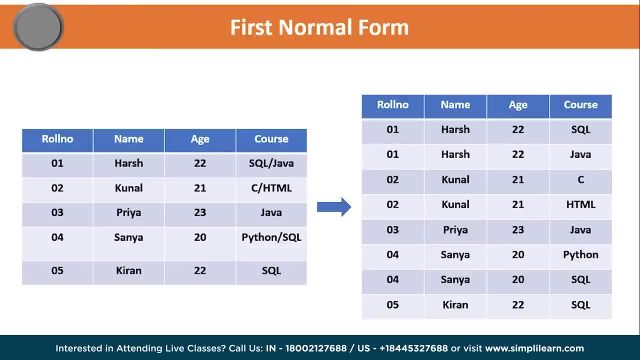 who has enrolled for courses C and HTML, And also we have Sanya who has enrolled for Python and SQL, which we have basically separated into two different records. So by applying the first normal form you can achieve atomicity and also every column has unique values. So that was first normal form, guys. Let us now move. 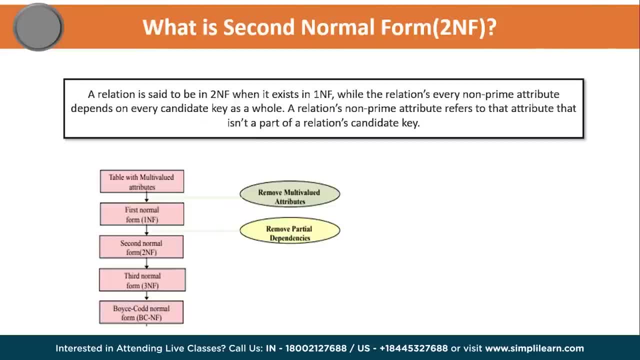 into the next normal form, which is second normal form. So the second step in a normalization is basically 2NF or the second normal form, which is basically an additional layer added to the 1NF. So a table or a relation isn't 2NF only if the relation, the table should. 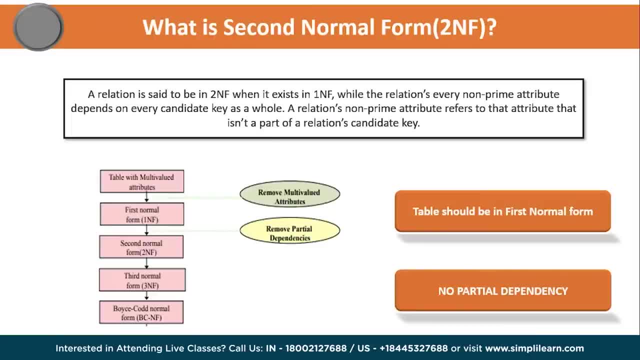 be in first normal form, that is, it should satisfy all the properties of the first normal form. while the relations, every non-prime attribute depends on every candidate key as a whole, So it should meet all the rules and every non-key attribute is fully dependent on the. 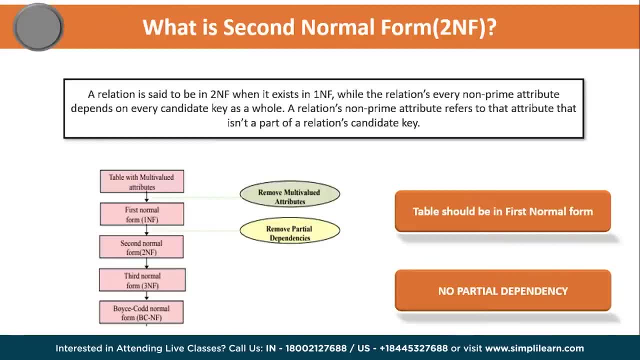 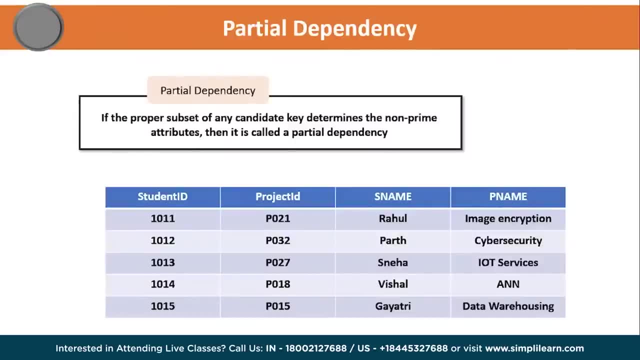 primary key. So I hope this is a bit challenging and confusing. So let us again understand this. Let us start with an example here. All right Now. the second normal form states that there shouldn't be any partial dependency. You know, partial dependency is nothing, but if a proper subset of a candidate key determines. 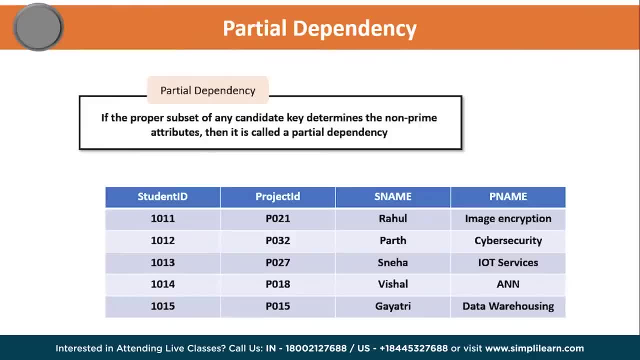 the non-prime attribute, then it is called a partial dependency. So let me just explain you with an example here. Consider this student table here which has student ID, project ID, student name and project name. here Now in the above table, if you look at clearly, we 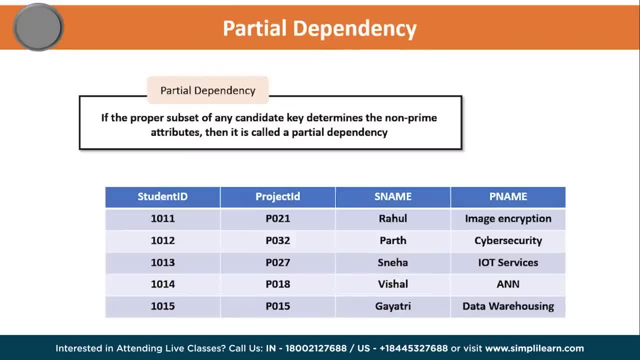 have partial dependency. Let us understand how Now the prime key attributes here are student ID and project ID And, as stated, the non-prime attributes, that is, student name and project name, should be functionally dependent on part of a candidate key to be partially. 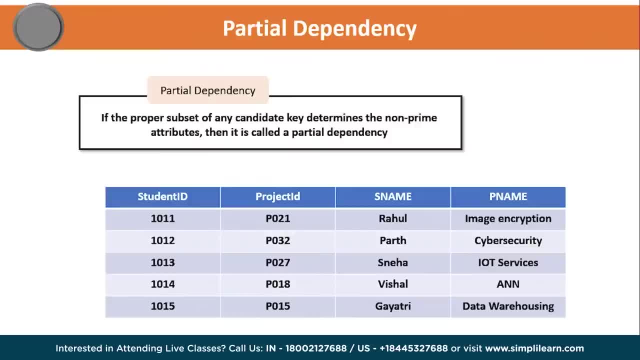 dependent. I hope you are confusing between the keys guys. So if you want to learn more about SQL keys, we have a dedicated and a separate video on our channel, So make sure you check that out. So, coming back to the second normal form, So the student name can be dedicated to the. 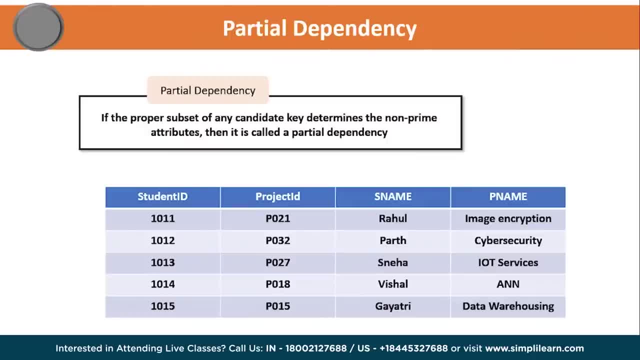 candidate key. So if you want to learn more about SQL keys, we have a dedicated and a separate video on our channel, So make sure you check that out. So, coming back to the second normal form, here partial dependency can be determined If tail is removed from this. 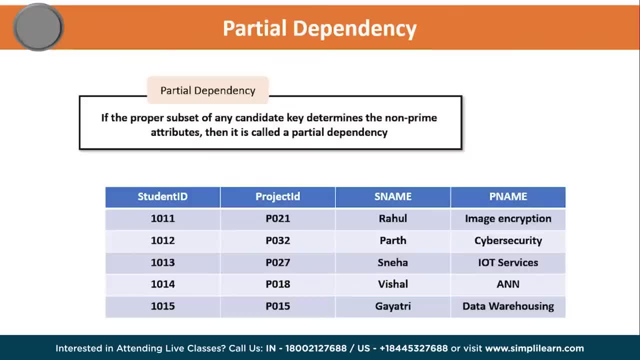 table, it has to have two new RT values. So to remove this partial dependency and the violation of the new RT, we have to further decompose this table in order to satisfy the property of second normal form. So right, let us now understand. how can we do that? 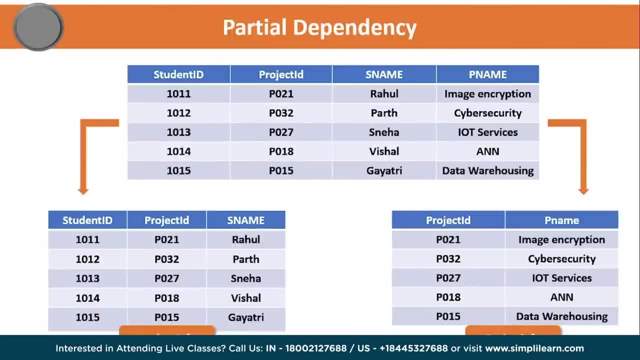 Now, basically I have been converting this student table into 2NT envulsions. So along the origin one may generally do the settlement by using Ref sql schorr stack statement. otherwise separate tables, which is student info and project info. Now the student info. 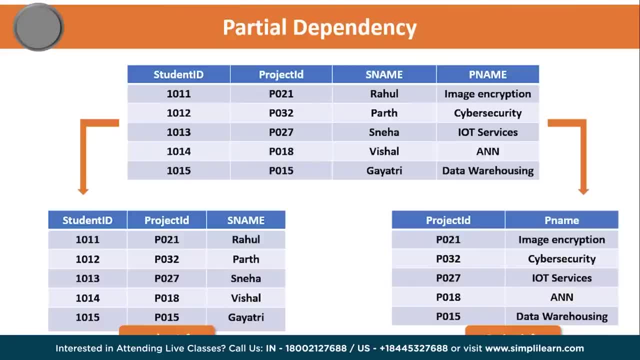 table has the student ID, project ID and the student name, whereas the project info has project ID and project name. Now a student name can be identified separately with the help of student ID, so it is uniquely identifying every record of the student name using the student ID. Hence the 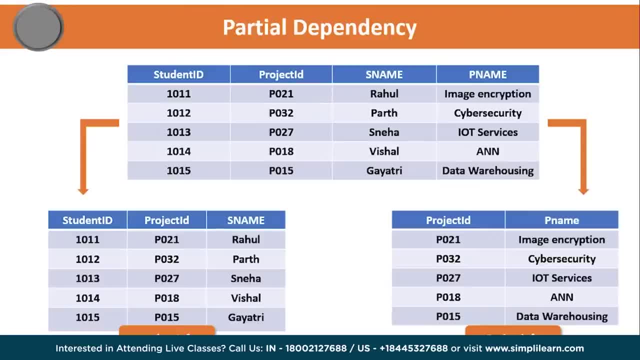 condition has been satisfied here and similarly we have the project info. with the help of project ID we can get the name of different projects that are allotted to students. So now the relation is in second normal form, in the form of a database normalization using the second normal form. I hope you understood. 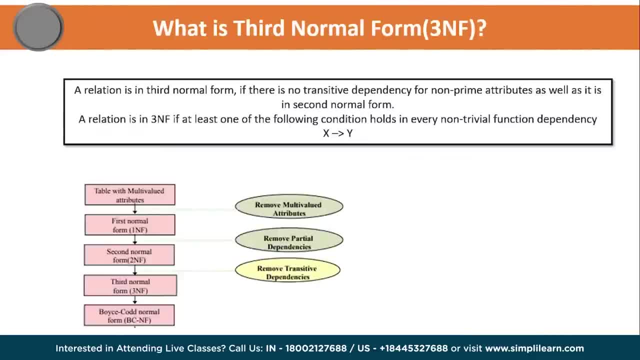 that, guys. So moving ahead, let us now understand what is third normal form. Now. it is a normalization level in DBMS similar to that of 1NF and similarly 2NF. So a relation is said to be in third normal form in SQL when it is in the second. 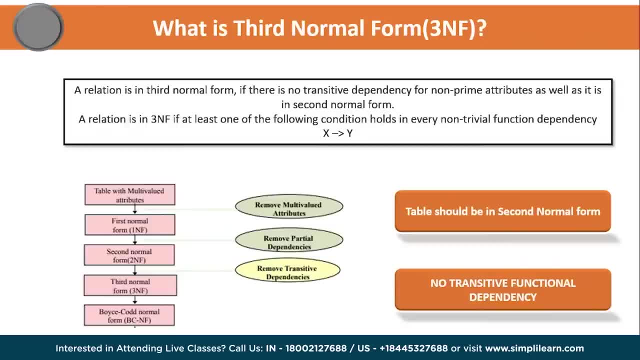 normal form, but no transitive dependency exists for a non-prime attribute. So let me just clearly explain you again Now. a given relation is said to be in its third normal form when it is in 2NF, that is, it should satisfy second normal form. 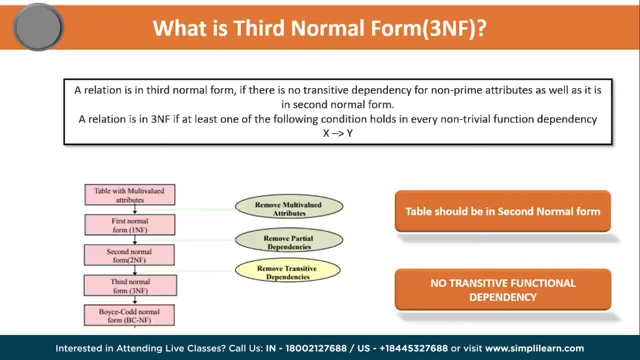 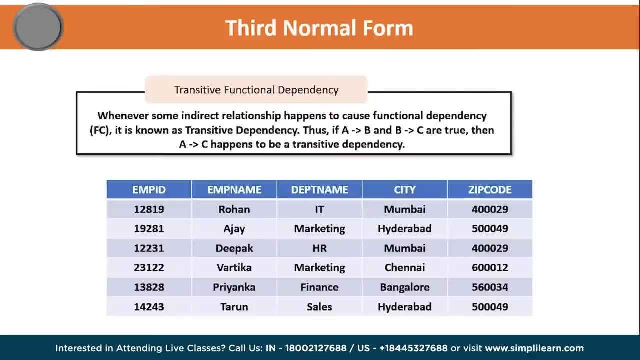 properties, that is ultimately indirectly- should satisfy first normal form as well, but has no transitive partial dependency, meaning when no transitive dependency exists for the attribute. So we can say that relation is in third normal form when it holds any of the given condition. in case of functional dependency, that is non-trivial. 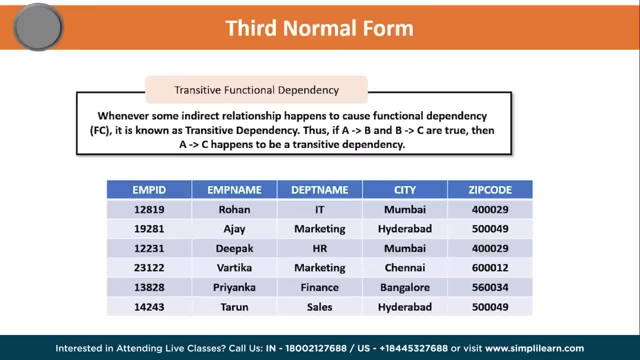 P. Let us say X relates to Y, where X as a super key and Y acts as a non-prime attribute, meaning every element of Y forms a part of a candidate key. So let us understand this with a simple example so that you will have a clear understanding of that. so for that, and taking another table, 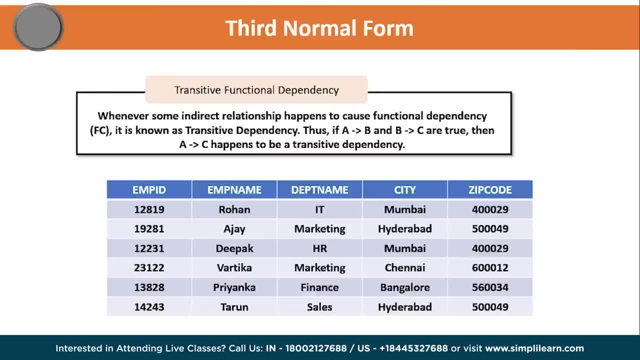 which is employee ID, employee name, department name, city, zip code as its attributes. Now the super key in the table mentioned above can be candidate id, candidate id plus candidate name, or else candidate id, candidate name and candidate- uh, let's say zip code, and so on. now the candidate key here is basically the. 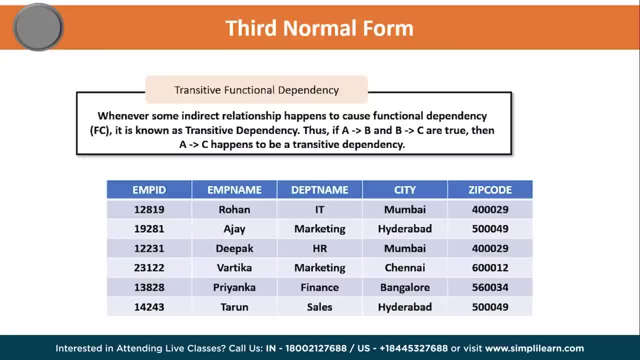 employee id because it is uniquely identifying each and every record. so if you look at the non-prime attributes, all the attributes in the table mentioned above are non-prime. instead, only instead of the employee id, right? so notice that employee id and the employee city that the employee 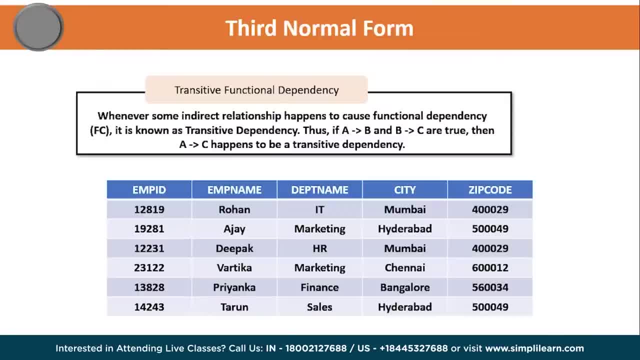 belongs to are dependent on candidate zip code and the employees zip code. and employee zip code is dependent on the employee id. here all the non-prime attributes, like the city of the employee and employees state, are dependently transitively on the super key, which is employee id. 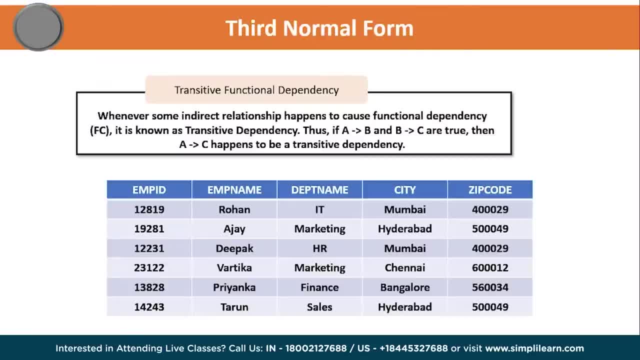 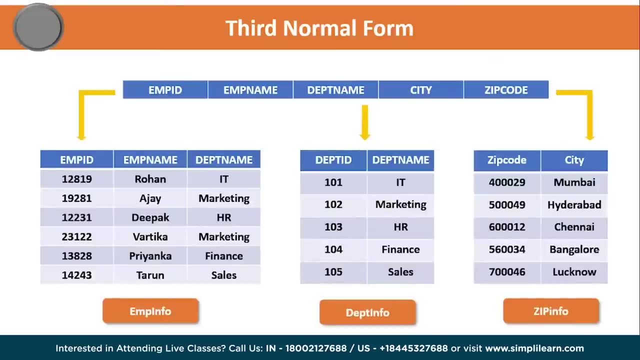 so the transitive dependency here would violate the rule of the third normal form. thus we must move the employee city and the employees uh zip code to a new table of uh, let's say into another table which is zip info. so if you look at this uh resultant table where i have segregated the 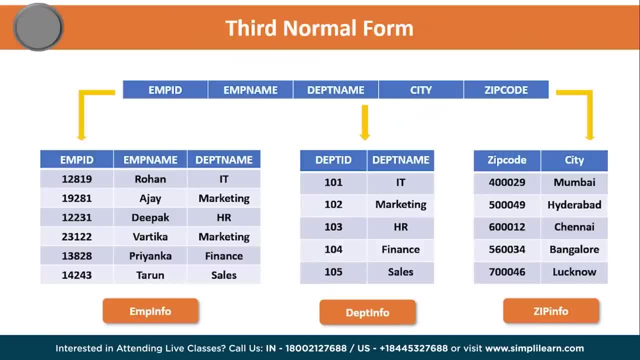 original table, which is the employee table, into three different tables here, which has: the first one is employee info, which holds the employee id, employee name, department as the attributes and its information. and in the second table we have department id and department name separately. and finally i'm categorizing, uh, the 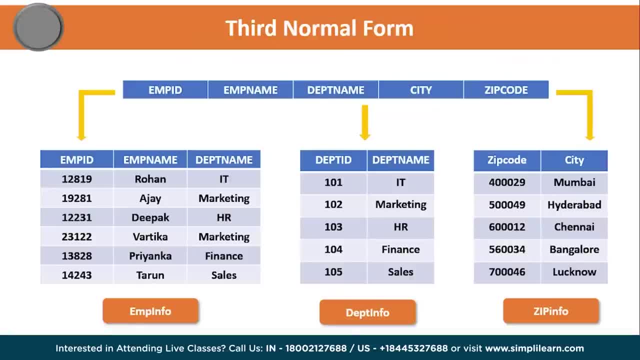 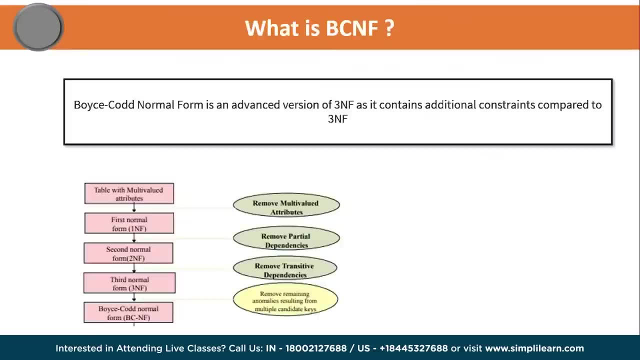 cities based on their zip codes, that is, into zip info table. so in this way you can use the third normal form, uh, to perform the normalization using the three nf characteristics. all right, let us now move into the final uh normalization, which is bcnf. now applications of uh general definitions of 2nf and 3nf may identify additional redundancy. 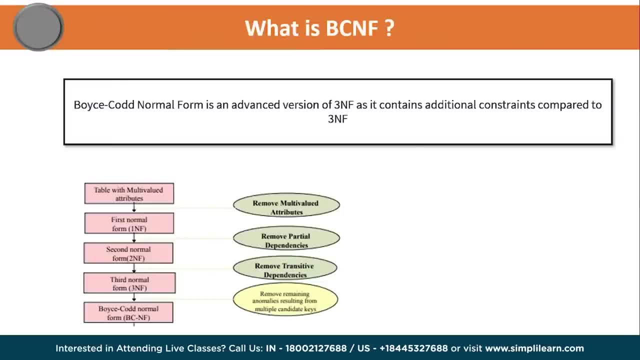 caused by the dependencies that can violate one or more candidates key in a table. so, however, despite these additional cringe constraints, dependencies can still exist that will cause redundancy to be present in three mf relations. so this weakness in three nf resulted in the presentation of a much stronger normal form called boy's call, normal form or simply 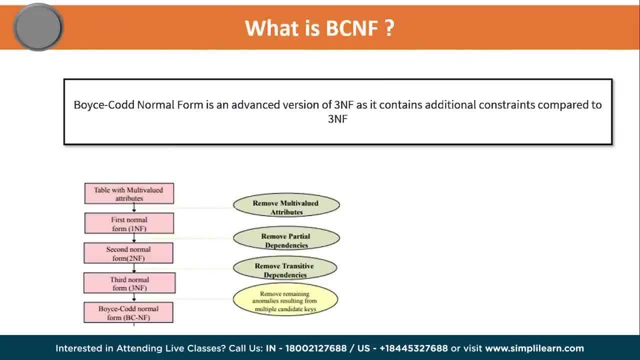 BC NF. So it was initially started. it was coined by Dr H Codd in 1974. So we will understand how this works. So it basically adds a more layer to our first normal form, second normal form as well as the third normal form. So a Boyce-Codd normal form is also. 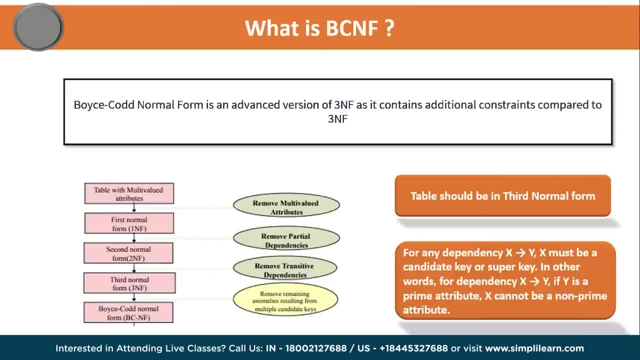 known as a 3.5 NF, which is a superior or advanced version of 3 NF and was developed by Raymond F Boyce, as discussed, which could tackle certain types of anomalies which were not resolved with the help of the third normal form. So the first condition of the table, 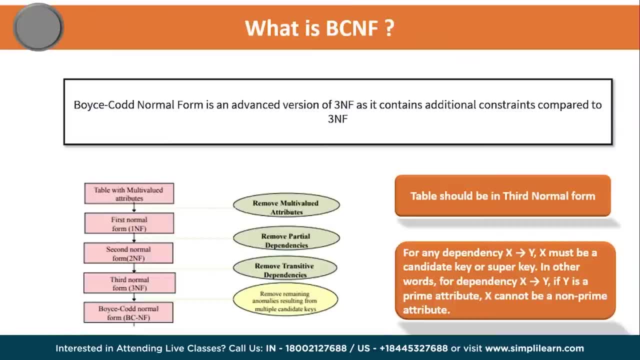 to be in Boyce-Codd normal form is that the table should be in the third normal form and secondly, every right hand side attribute of the functional dependency should depend on the super key of that particular table. So for example, for A, any dependency, let's say a relation X to Y, X must be a candidate key or a super key. 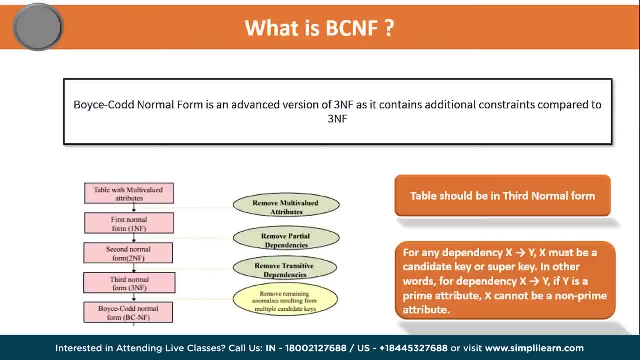 In other words, for dependency, X relates to Y if Y is any prime attribute, So X cannot be a non-prime attribute. So now, in general, if a table is in third normal form, it would possibly be in BC NF, and similarly, like 4 NF and 5 NF as well. So we do not need much. 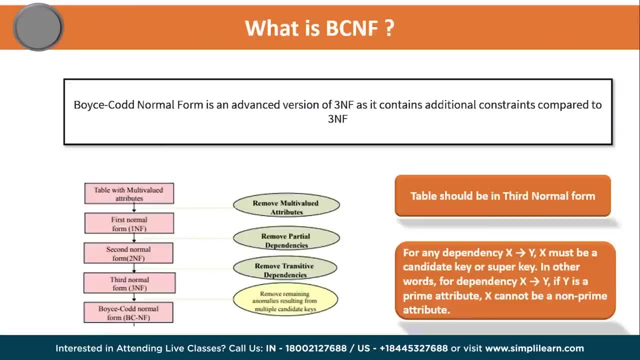 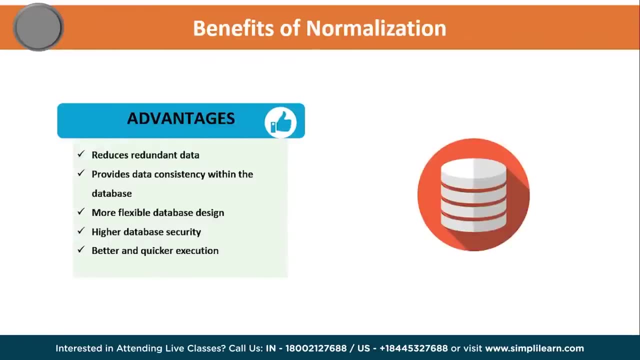 of BC NF. if we know what is exactly 1 NF, 2 NF and 3 NF, We are good to go and which is more than sufficient for a beginner level. So that was all about the BC NF guys, and that brings us to the end of today's session, and 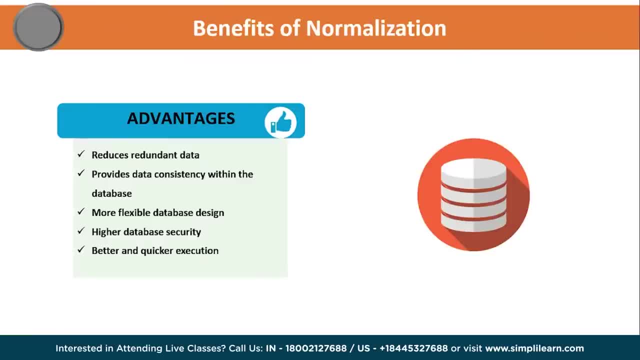 let us now finally understand some of the benefits of normalization by understanding some advantages of normalization Now. the first obvious reason is it reduces redundant data. Now we might have multiple data or multiple values in our database Because of human errors, or we do not know what we are entering, So we might add additional. 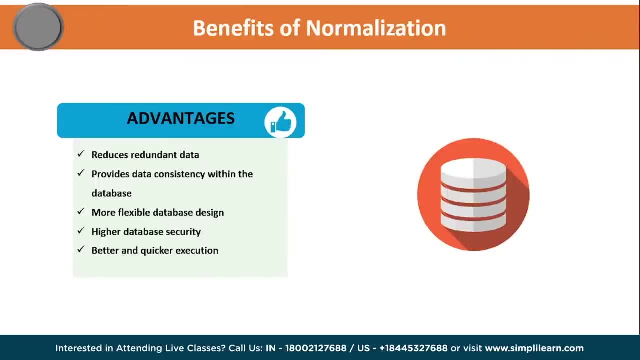 files without our knowledge. So in order to reduce that, you know repeated values or unnecessary records, we need normalization. Normalization also provides data consistency within the database and it is also more flexible and it gives more flexible data design, which in turn gives a higher database security and 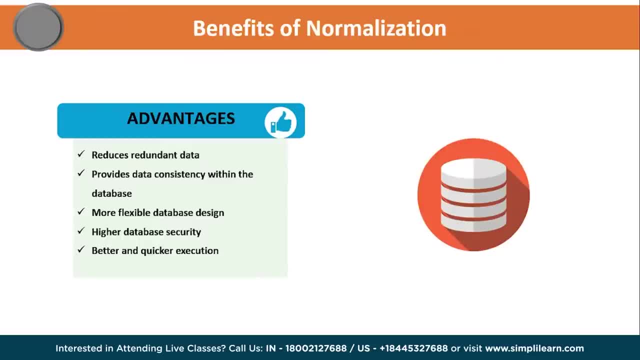 it is also better And quicker in execution as well. So that was some main. you see, advantages of normalization and talking about disadvantages. there are not. there aren't much disadvantages to talk about, like, since the data is not duplicated. we need table joins. you know more numbers, which would make queries more complicated. 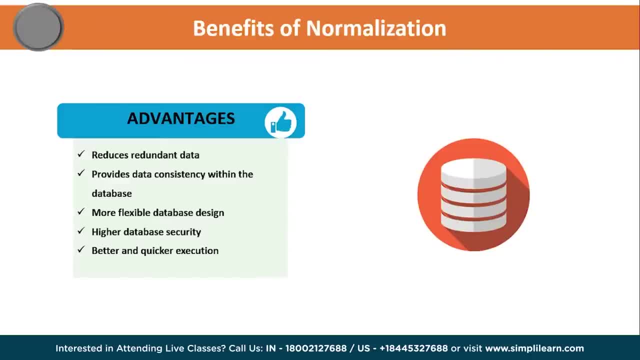 and thus read times are also slower. Since joins are required, the indexing of the tables also does not Work as efficiently. Again, this makes read time slower because the joins don't typically work well with the indexing. So that brings us to the end of today's tutorial. guys, I hope you've understood the tutorial. 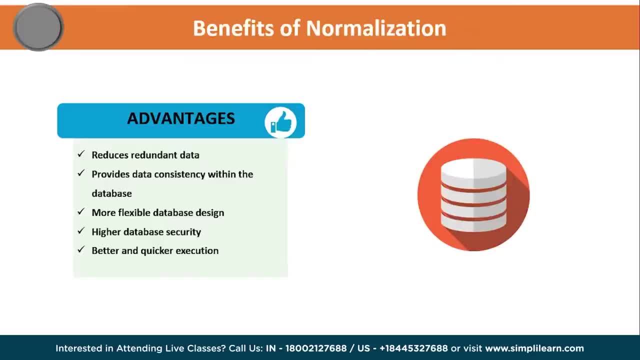 So let us just wrap up what we have discussed. We have discussed about various normal forms such as 1NF, 2NF and 3NF in our tutorial. So in this tutorial you have seen normalization in SQL in a glance And understood how the different normal forms of normalization. Now you can organize the 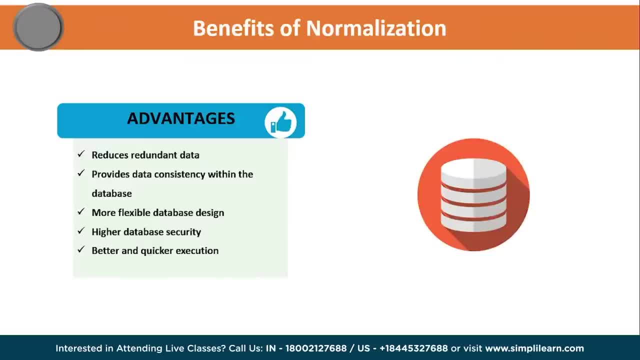 data in the database and remove the data redundancy and promote and achieve data integrity. So, in terms of if you're working on SQL databases, this isn't much an important concept, but this tutorial also helps for you if you are preparing for any interviews, which is a basic 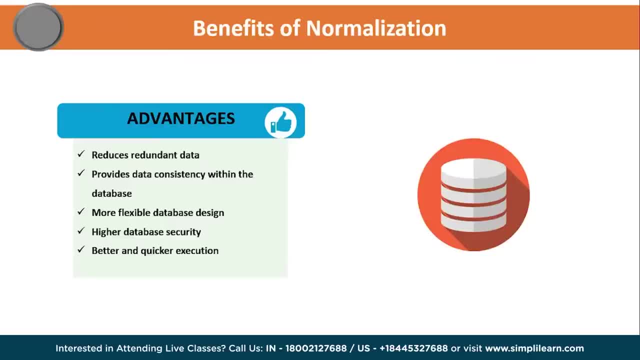 question which is asked in many of the interviews in various companies. So it is important to understand the concept of normalization in SQL. So I hope you've understood this. Good indexes are the key to good performance in SQL and the key to creating good indexes. 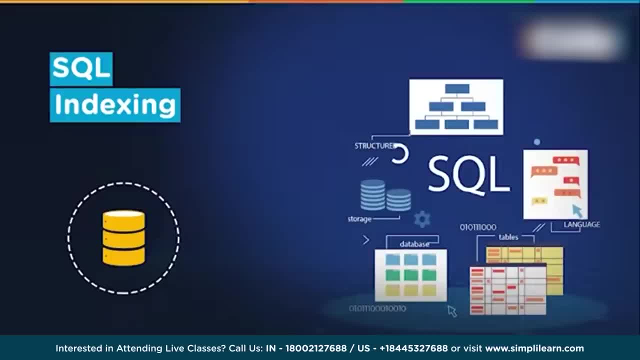 is to understand what indexes are and how SQL uses them to evaluate queries. Now, an SQL index is a structure within SQL which is used to quickly locate specific rows within a table. More on that soon, But before we get started, if you're new to the channel, 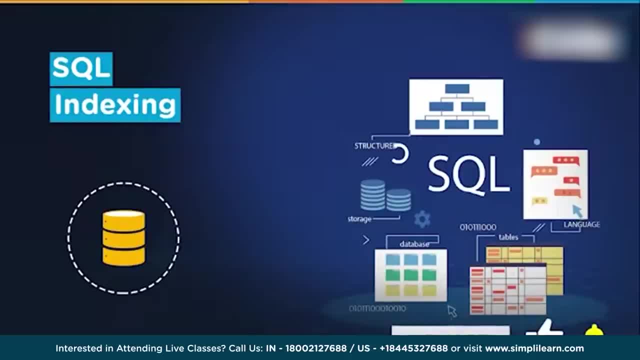 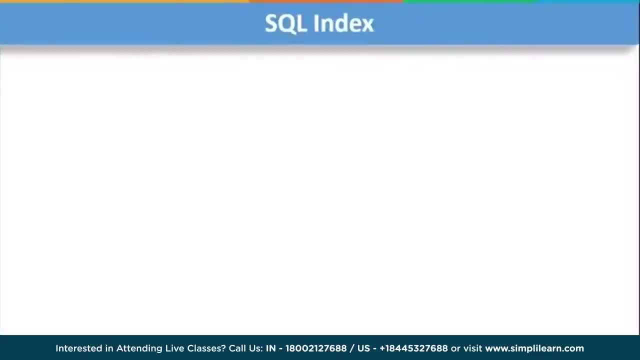 and haven't subscribed already. consider getting subscribed to our channel simply to stay updated with all the latest technologies, And we'll see you in the next video. Bye, And hit that bell icon to never miss an update from us. So, without any further ado, let's. 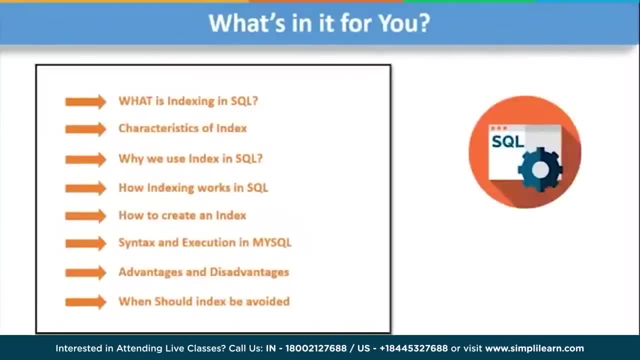 get started with today's topic. Firstly, let us go through the agenda for today's session. We'll start the tutorial by understanding what is indexing in SQL, and then we'll go through different characteristics of indexing in SQL. After that we'll understand why we exactly use indexing in SQL. Up next, 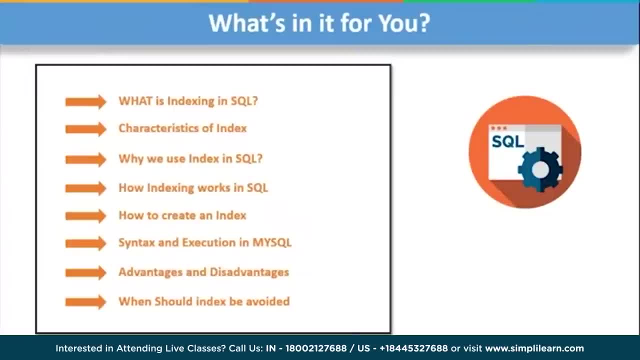 we'll discuss how exactly indexing works in SQL, and then we'll discuss how to create an index using its syntax, And after that we'll be going through the syntax and execution of the indexing part in MySQL workbench using certain examples. After that, let us discuss advantages and 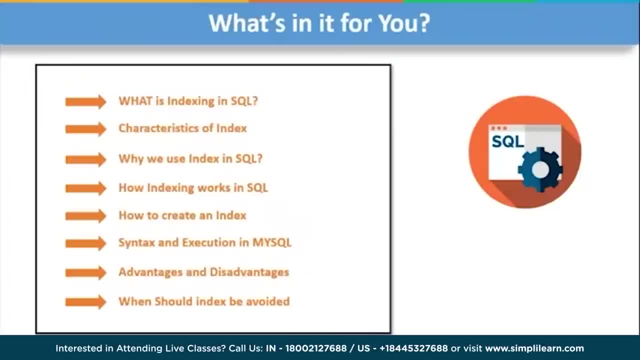 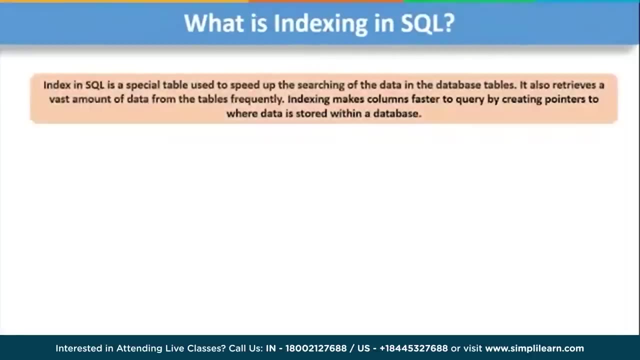 disadvantages of using indexing. And finally, we'll wrap up the session by understanding when you should be using and when you should not be using indexing in SQL. I hope the agenda is clear, So let us just dive straight into today's topic. All right, So what is indexing in SQL? 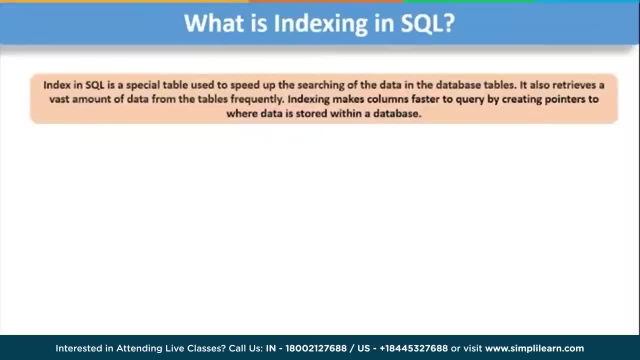 Indexing in SQL is a tool that allows you to use indexing in multiple languages. For example, if a table is moving by itself or you have a database that is working on a database, you can use an indexing indexing, which is a very simple format to do The indexing of. 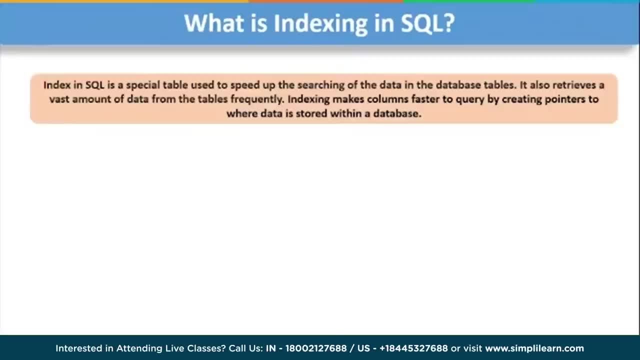 data is actually a simple expression that can be used by a database search engine to speed up the data retrieval process. So an index is simply a reference to data in a table, and a database index is similar to that to the index in a back of a book. Now it also. 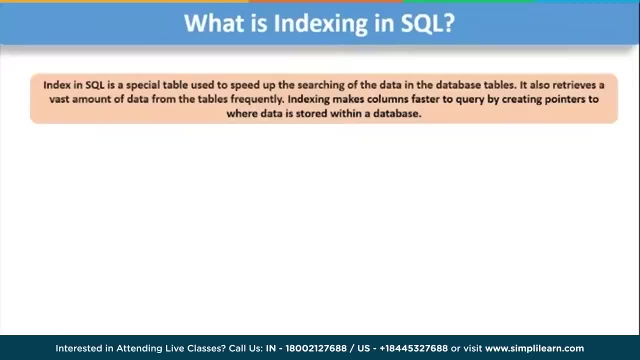 retrieves vast amounts of data from the tables quickly. So if you're working on large databases, creating pointers to where data is stored within a database, We'll understand when we'll discuss how exactly indexing work. So now, for example, in order to reference all pages in a book that address a particular subject, 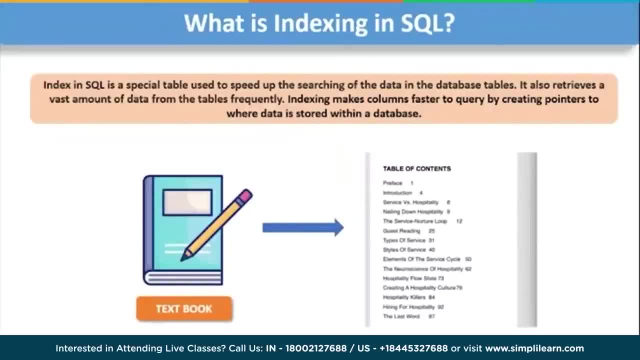 you go to the index first, which lists all the topics alphabetically right. So if you consider a textbook, it has various topics which scatters to a particular subject. So if you want to find a particular topic you go to one or more specific page numbers. 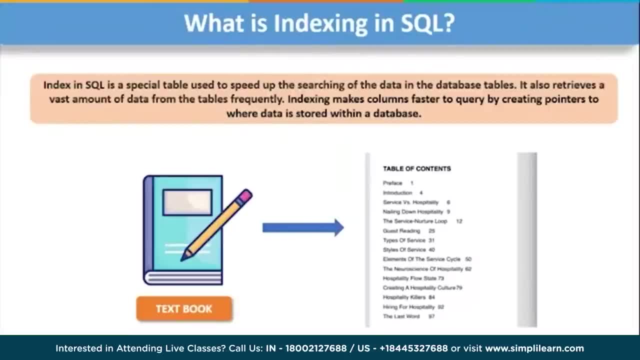 Now, indexes in a database are similar to that of indexes that you find in a book, guys. So if a book has an index and if I ask you to find a chapter in that book, you can quickly find that with the help of the index. 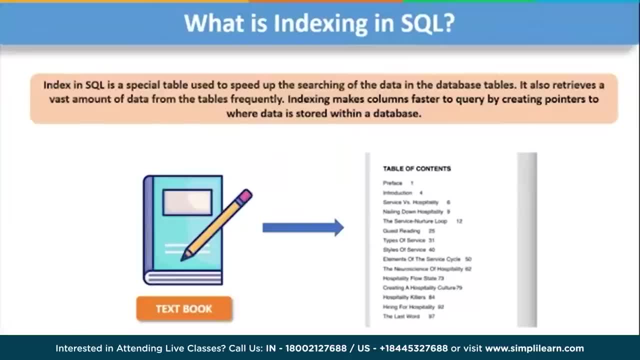 On the other hand, if the book does not have any index, you'll have to spend more time looking for the chapter by looking at each and every page from the start to the end of the book. So it is time-taking and tedious as well. 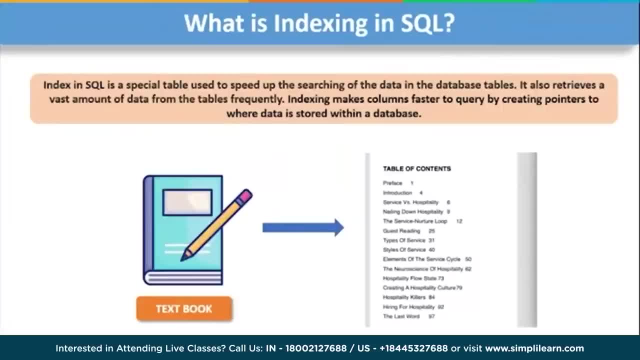 So simply, you can use the index and you can directly go to that page. So basically, indexes prevent duplicate entries in the columns or combination of columns on which it is created. So you can say that MySQL indexes are quickly used to find rows within a specific column values. 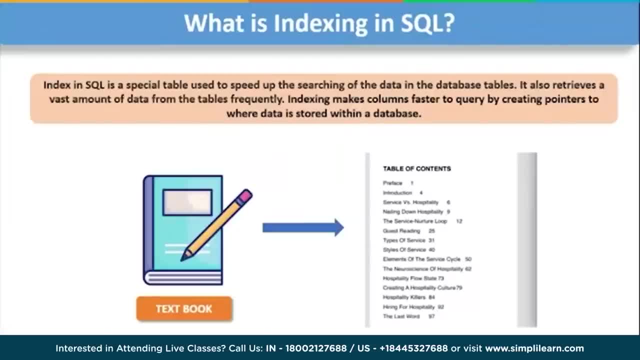 and without an index, MySQL or any SQL database, must scan the whole table to locate the relevant rows. So now, the larger the table becomes, the slower it searches. So I hope you understood what exactly is indexing in SQL. Let us now understand why we use indexing in SQL. 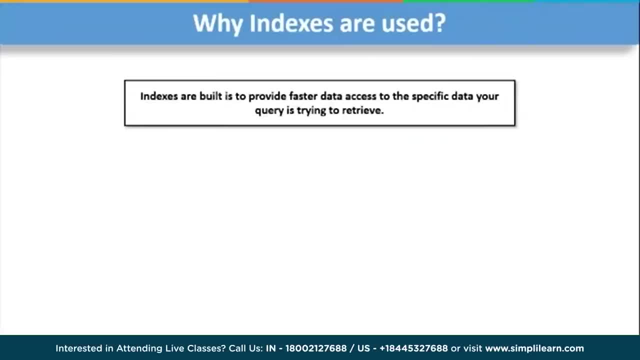 Now indexes are built to provide faster data access to the user to the specific data your query is trying to retrieve Now. indexing in DBMS is a technique that uses data structures to optimize the searching time of a database query and makes the overall database performs better. 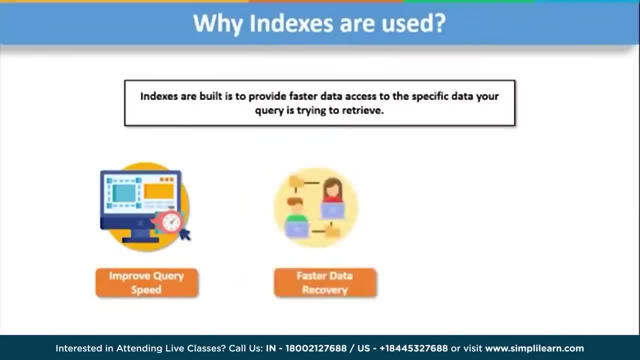 Now indexes are used for faster data recovery guys. Indexes are used to quickly locate data without having to search every row in a database table every time a database table is accessed. Indexes can be created using one or more columns of a database. 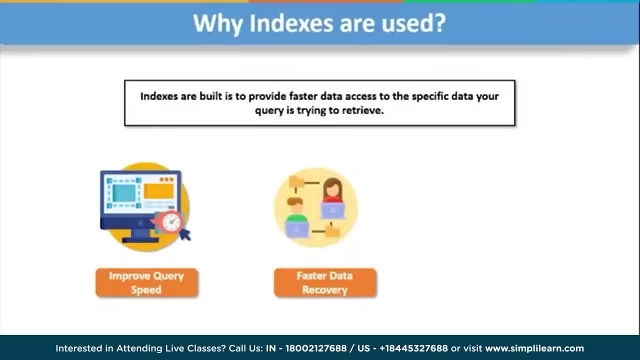 providing the basis for both random lookups and efficient access of ordered records. And finally, indexes provide search efficiency. An index can be used to efficiently find all rows matching some columns in your query and then walk through only that subset of the table to find exact matches. 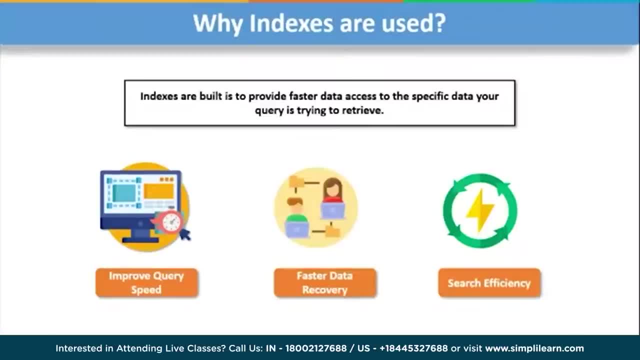 So if you don't have indexes on any column in the WHERE clause or the SELECT clause, the SQL engine has to walk through the whole table to find the exact matches. And if you don't have indexes on any column in the WHERE clause or the SELECT clause, 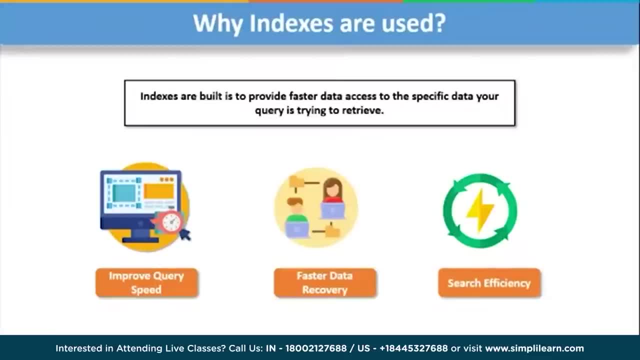 the SQL engine has to walk through the whole table to find the exact matches. And if you don't have indexes on any column in the WHERE clause or the SELECT clause, the SQL engine has to walk through the whole table to find the exact matches. 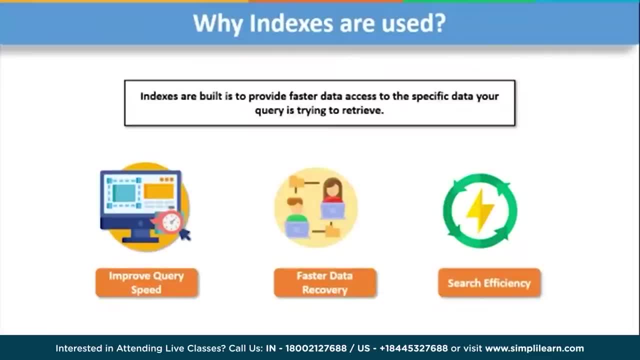 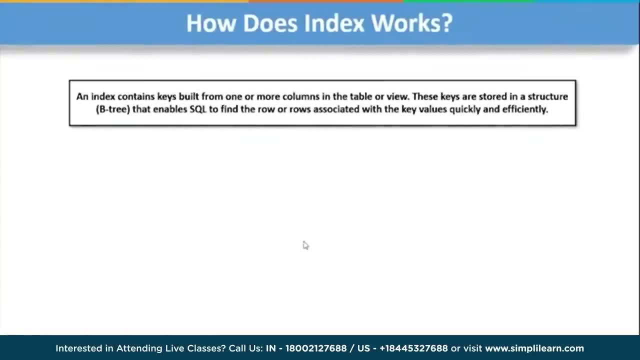 So these are the main reasons why we exactly use indexes in SQL. Alright, let us now understand how exactly indexing works. Now, generally, the database takes the columns provided with the CREATE INDEX command and sorts the column values using a special data structure called as B-trees. 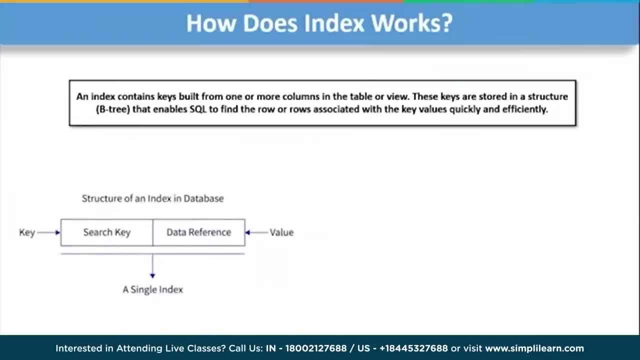 Now, a B-tree is a type of tree data structure that contains two things, which is basically the index and the index key and the corresponding disk address. Now, index key refers to a certain disk address, and that disk further contains rows or tuples of data. 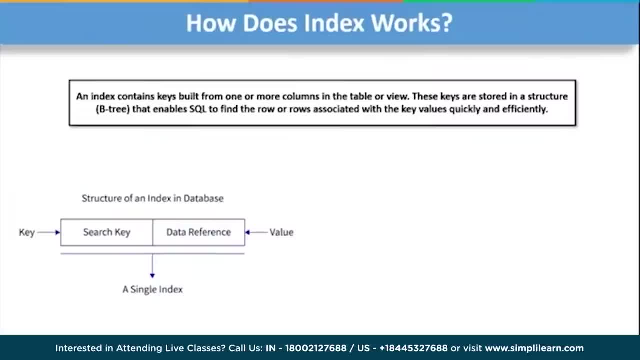 Now, using B-tree, we can achieve faster searches and faster retrievals of data, And since the data structure of B-tree is sorted in order, it makes a search more efficient. So this is how, in general, index works in SQL. So let us understand this with an example here, guys. 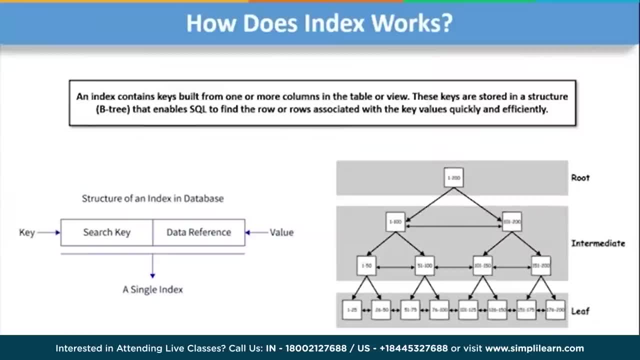 Now let us consider we have an employee table which has, let's say, 200 reports in it. Now, employee ID in that table, let us consider it as a primary key. So by default an index on the employee ID column is created. This means employee data is sorted by employee ID column and physically stored in series of data pages. here 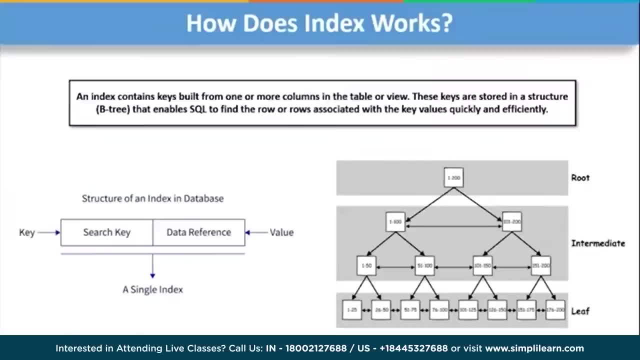 in a tree like structure that look like the following, which is like the visible on the screen, as you can see. So let's say, the notes at the bottom of the tree are basically called as data pages or leaf notes, and contains the actual data rows. 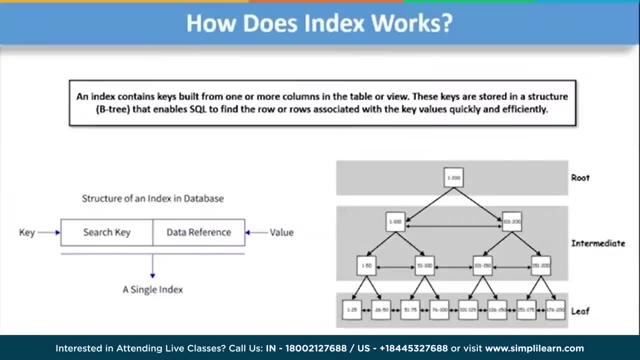 In our case, the employee data's information. So these employee rows are sorted by employee ID column, because employee ID is the primary key and by default, an index on this column is already created. Now, for example, let's say in our employee table we have 200 rows and let us assume in each data page we have, let's say, 25 rows. 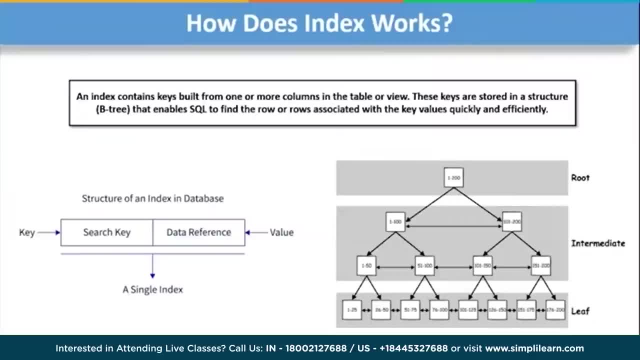 in each of them. So the first data page we have is from 1 to 25. in the second we have from 26 to 50, and then 51 to 75, and so on and so forth, and the node at the top of the tree, as you can see, is called as the root node. guys. 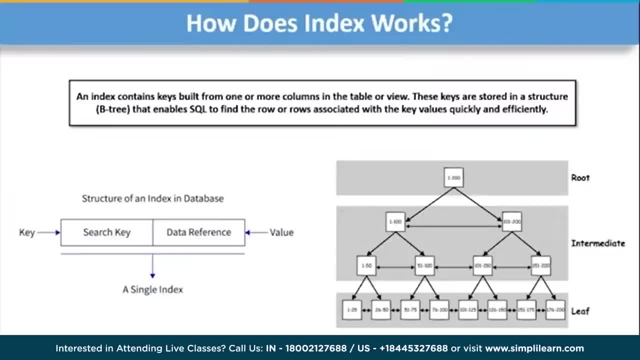 and the node between the root node and the leaf node are called as intermediate level nodes. So the root and the intermediate level nodes contain index rows. As you can see, the 1 to 200 rows has been further subjugated into 1 to 100 and into 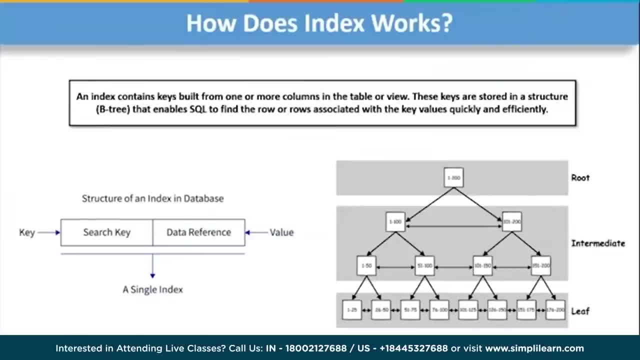 101 to 200 and so on. So each index row contains a key value, which is, in our case, as the employee ID and a pointer to either an intermediate intermediate level page in the B tree or a data row in the leaf node is been given. 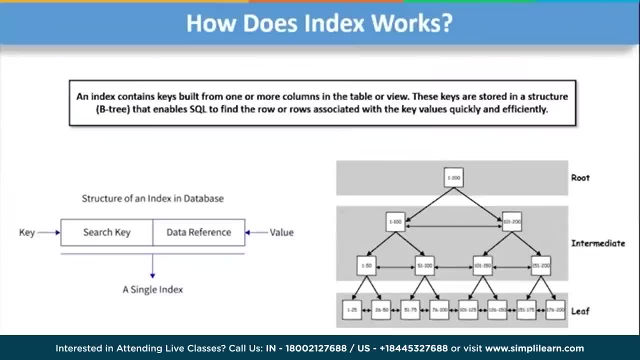 So this tree, like structure, has a series of pointer that helps the query engine find data quickly. Now let us understand how SQL finds the particular row by ID that we want to search. For example, let's say we want to find employee row which is having employee ID. 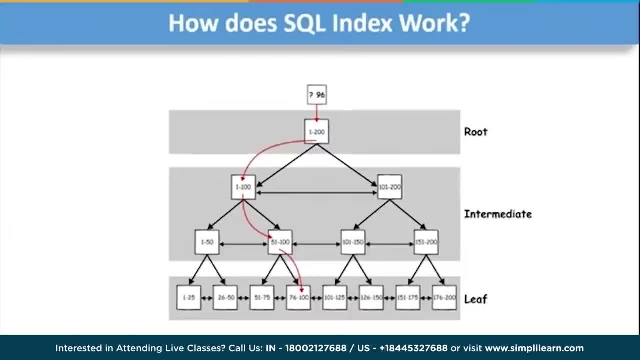 as 96.. So in that case how the SQL engine performs indexing on this data? So basically the database engine starts at the root node and it picks the index node, which is the root node, that is, from 1 to 200, and it basically searches on the left side. 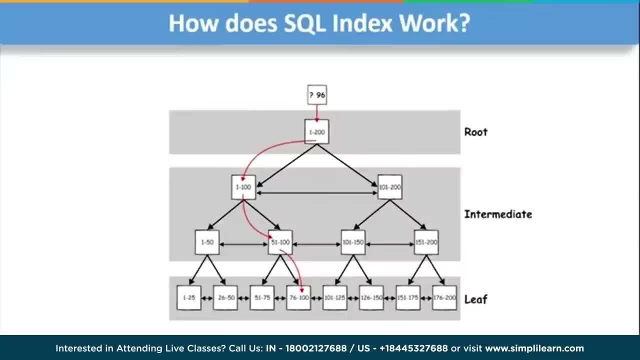 because the 1 to 200 data has been further divided into 1 to 100 on the left side right. So because the data engine knows it is this node that contains employee ID from 1 to 100, it will basically look for all the records starting from 1 to 100 from there. 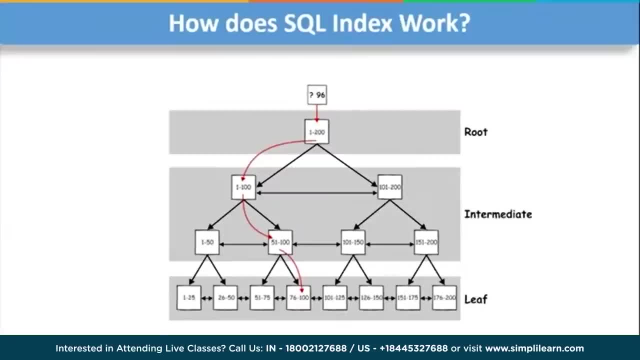 It picks the leaf node that is present on the extreme left because employee data rows from 1 to 100 again and are present in this leaf node, and then the data rows in the leaf node are sorted by employee ID. So it is easy for the database engine to find the employee row with ID 96 here. 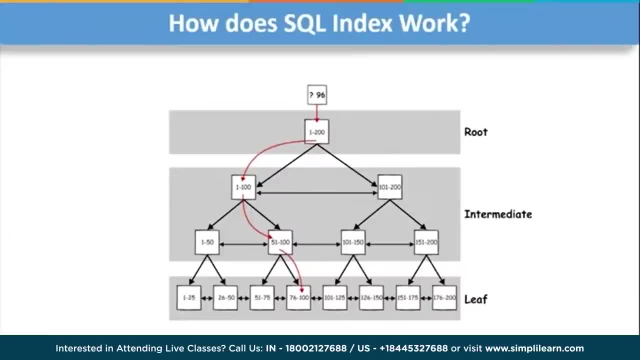 So, as you can see, in just three operations or SQL is able to find the data we are looking for. So it's making use of the index We have on the table and performing the operation in the most simplest way. So this is how exactly SQL indexing works. 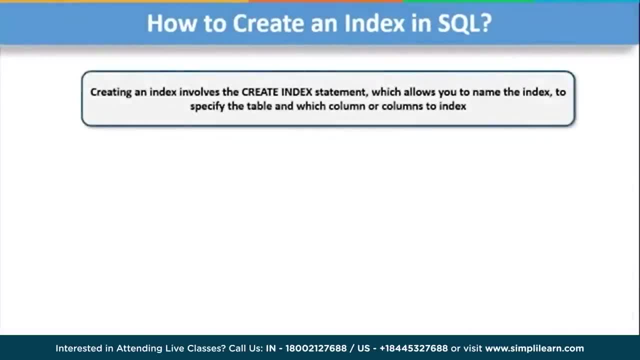 All right, moving ahead, Let us now discuss how to create an index in SQL. Now creating an index involves create index statement, which allows you to name the index name to the specify the table and which column or columns that you want to create index. 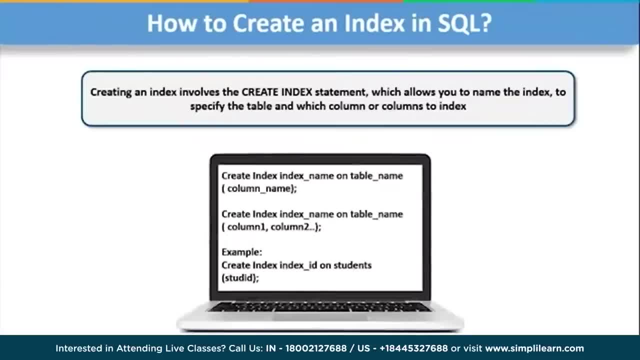 So this command is used to basically generating the table index in SQL using the built index app Expression. So let us now go through the syntax. The syntax is followed as: create index, which is the keyword index name on table name and in within the brackets: 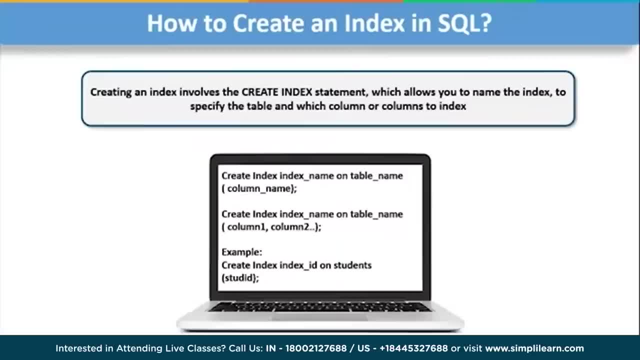 You have to mention the column name. So if you want to create indexes from more than one column, in that case you have to mention the different column names and the query is followed as create index, index name on table name: column 1, column 2 and so on. 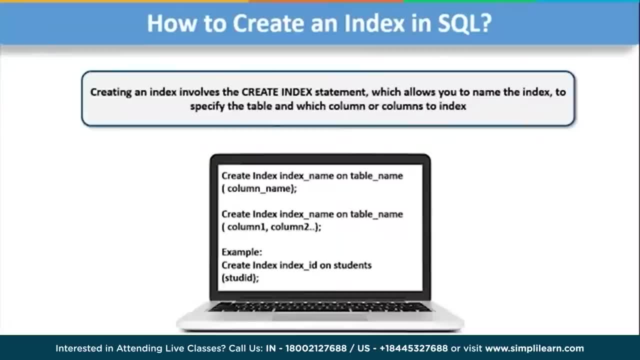 So basically, we can generate sorted list using indexes in SQL instead of having to create New sorted table, which would take up a lot of storage space, right? So, for example, if I want to create an index, let's say index underscore ID, on a tables called students and on the column student ID, 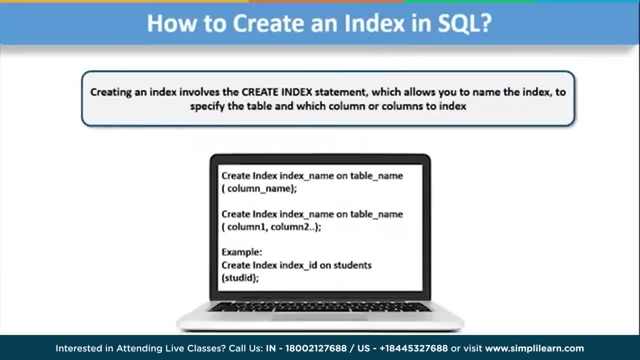 then in that case the query would be followed as: create index index ID on students student ID. So, basically, if you are working on the student ID column and if you want to fetch details which has a relation to that attribute, in that case you can use this example. 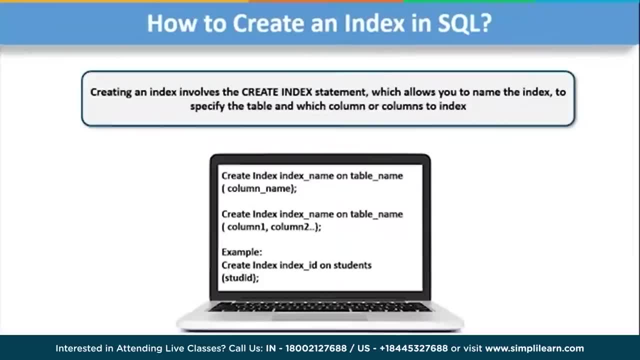 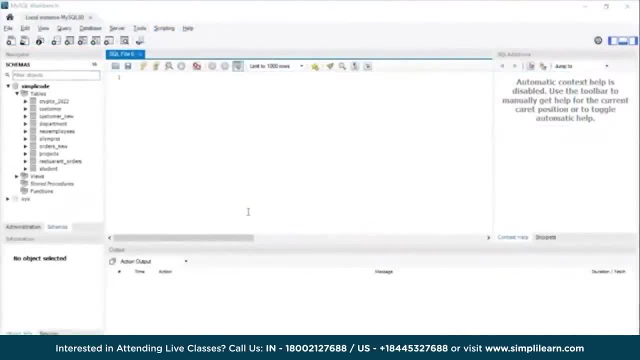 I hope the syntax is clear. So let us now jump straight into MySQL workbench for the execution part. So, as you can see, MySQL workbench has started and we are good to go now. So, as discussed earlier, in order to perform indexing in SQL, 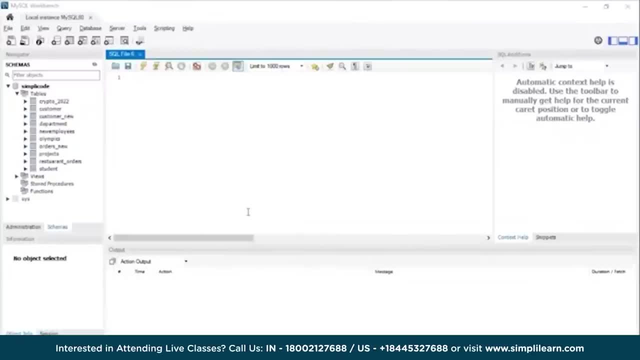 you need a data set or a table that has a large number of records. Now when I talk about record number of records, it shouldn't be like a hundred or two hundred. It should have more than hundred, like in thousands. So I have downloaded a data set. 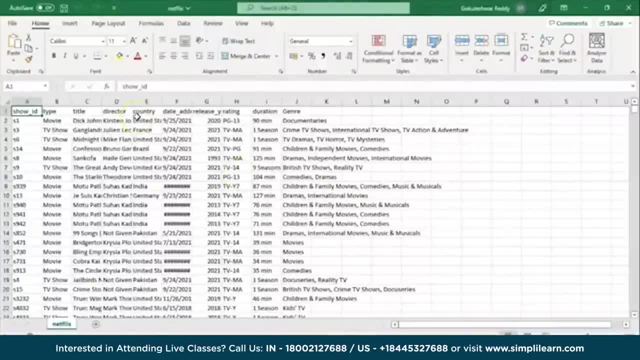 It's from Kaggle, which is of Netflix information which is, as you can see, in this excel sheet, which has been show ID, the type, title, director, country, date, added release year, rating, duration and the genre of that particular movie or show. So if you look at this table, 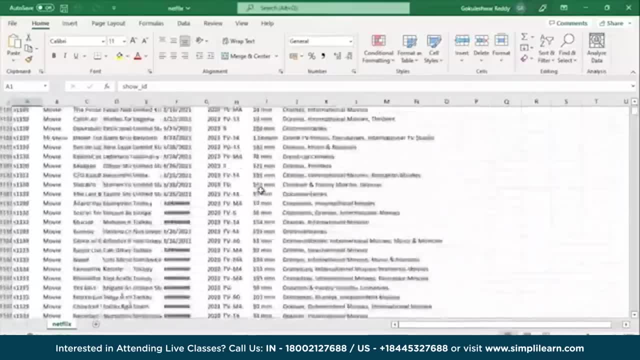 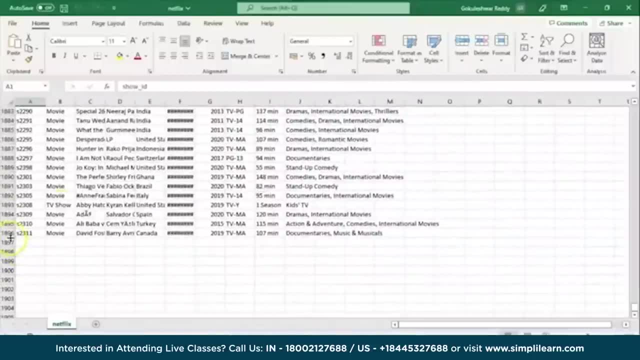 we have like thousands of records, I guess. let me just scroll down and show you guys. So, as you can see, we have a chunk of records. As you can see, we have a total of 1896 records. So I think we can perform indexing on this table and we'll see how it works. 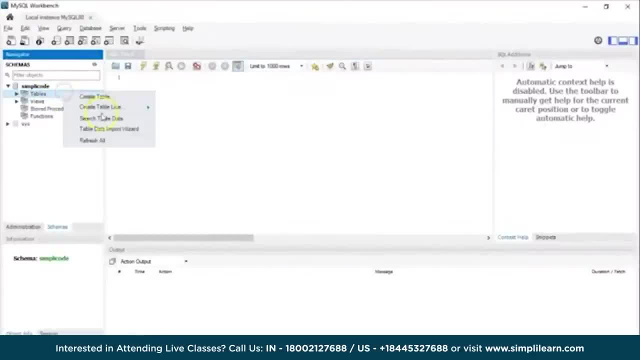 So let us just import the data set first. So right click on the table section, click on browse and the table name is Netflix. Open the table next. click on, next, Again, click on next and we are good to go and we can import the data now. 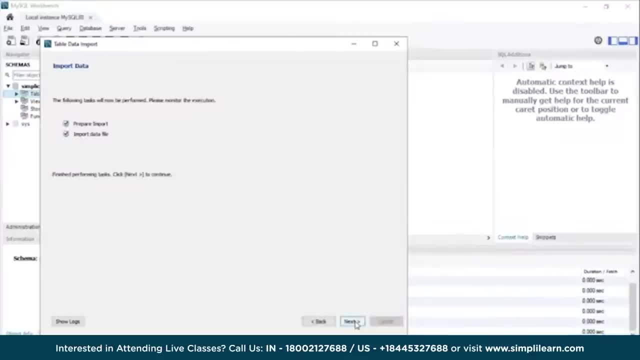 So click on next again. So wait some time. depending upon your net speed or your RAM functions, It will take some time. So just hold back for some time and let it finish. So, as you can see, the data has been successfully imported. click on next. 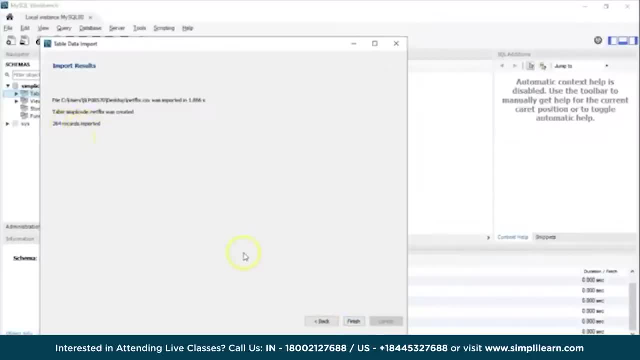 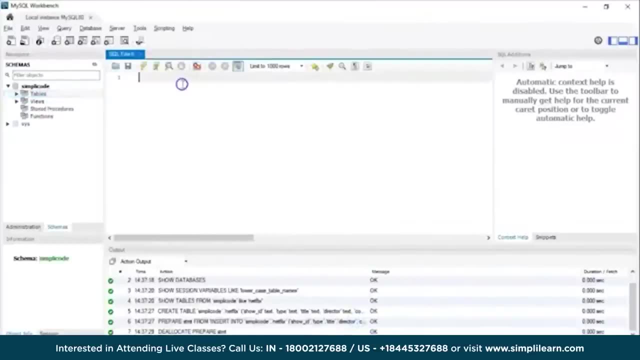 I think only 264 records have been imported. I don't know why exactly, but it's okay, I'll let us go ahead and let us understand how it works anyway. So let us just double click here and we'll refresh the schema part. 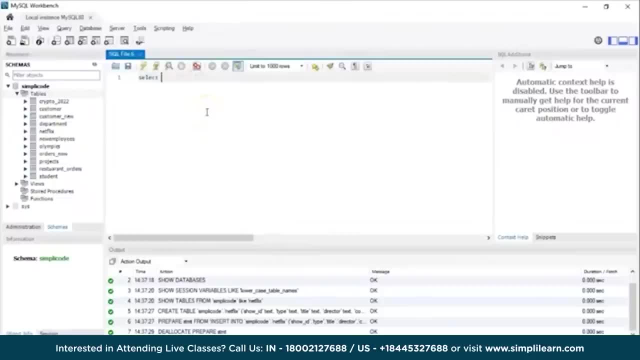 As you can see, Netflix table has been added, So let me just display the values from the table. So I'm using the select operator, select star from Netflix. So let's execute this query and we'll see the output. as you can see, various attributes: 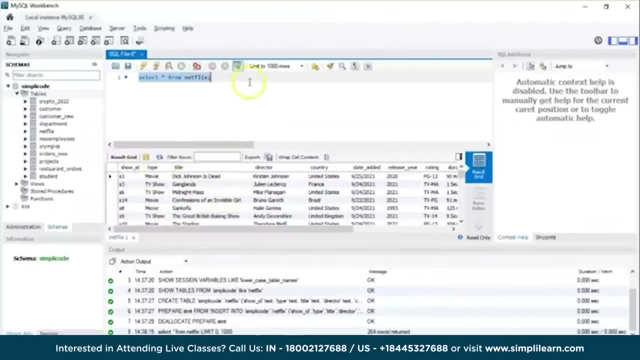 that we have discussed earlier has been displaying in our resultant table. So let us now go ahead and we'll. let us write a simple query first. Let's say, if I want to select all the titles Or the shows that are related to movie type and that have the release year, 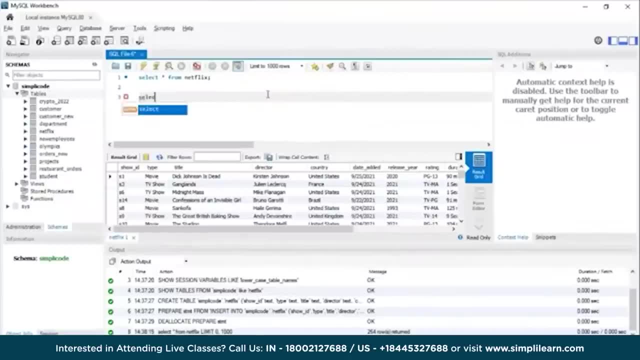 Let's say after 2000.. So in that case I'll take as select title Comma type, Comma release- Okay, as title type from table Netflix where release year is greater Than 2000.. So let me just execute this query. 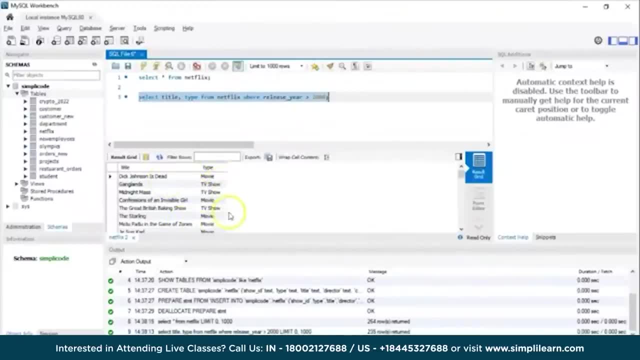 So, as you can see, it will display the records of all those titles and the type of that show or the movie name which is released after 2000.. Now, if you look at the duration part, I am not sure why it is showing 0.00 seconds. 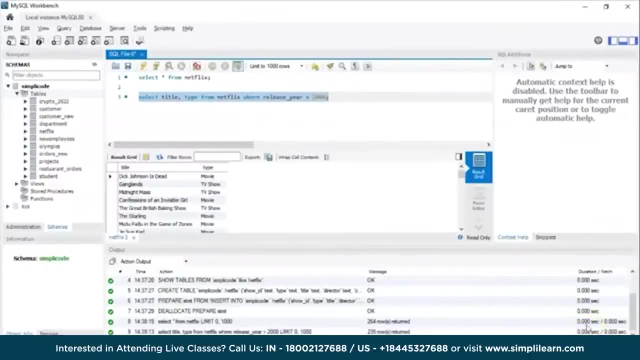 but it should like. it should specify like more than like half a second or something. but I'm not sure why it is, but it is showing like that. So maybe since we have imported only limited number of rows, that is like almost around 300.. 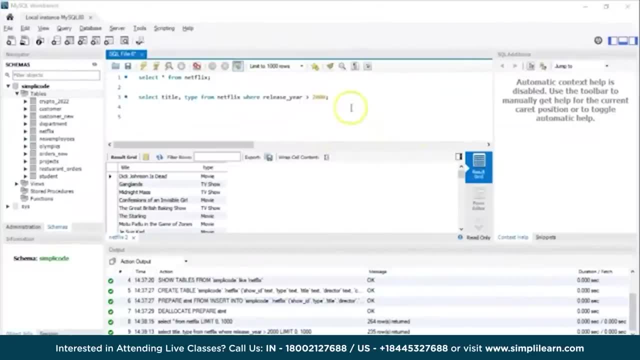 That is the reason why it is showing in 0.00 seconds, But in generally. if you're working on large data sets which have thousands of records, it will generally take like 0.05 or 0.36 seconds like that. 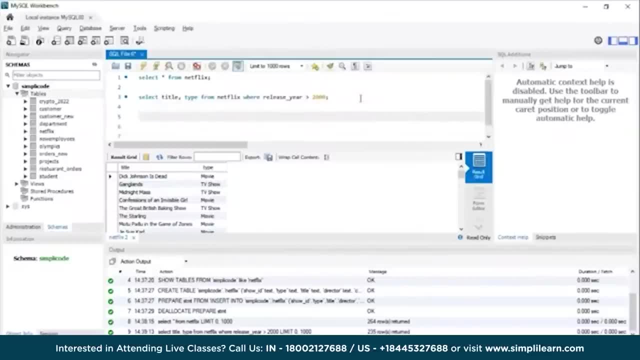 So let us go ahead and let us just create a, you know, a simple index for this table Netflix. So the query is followed as create index. Let us take index. I'm taking indexing on title, So I'll just specify index. Okay, Netflix will mention the table name here. on table name, that is Netflix and mention all the columns. 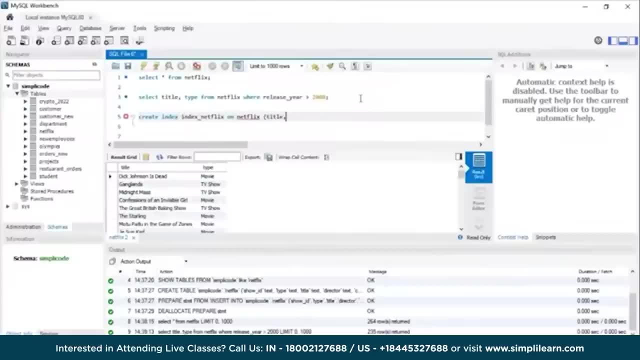 that you want to create an index on, So I'll basically specify the title and the type. Okay, first we'll discuss on one column and we'll see the output, So let us execute this. So there was an error in the data type that we have mentioned since the. 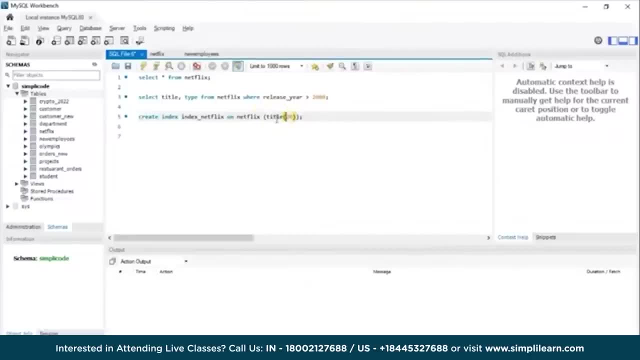 title, which is the column name, has a data type of text, So we have to mention the number of bytes that it takes. So I'm basically mentioning 20 here. So let us just execute the statement and we'll see the output. So, as you can see, our index. 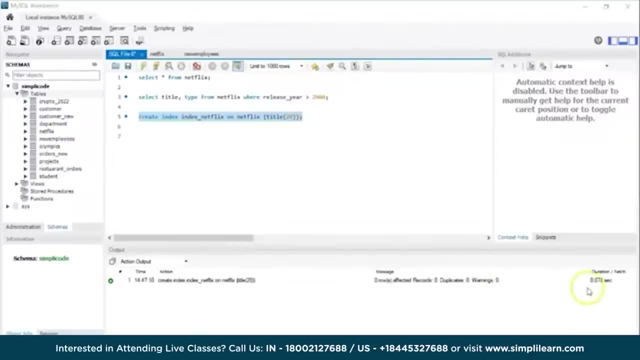 which is index underscore. Netflix has been successfully created And if you look at the duration here, it has taken 0.078 seconds in order to execute this query Now. similarly, if you're working on large data sets- and we are- when you are querying data, 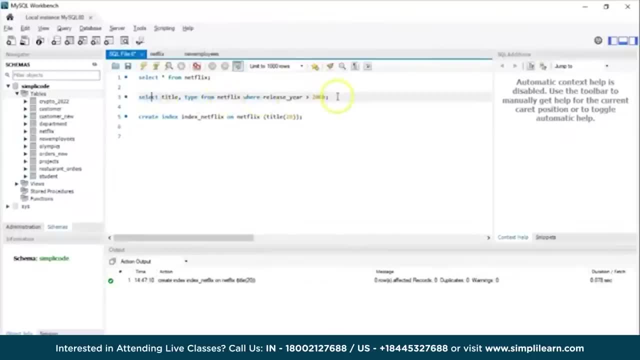 for example, select title type from Netflix where release year is greater than 2000.. It generally takes more than like half a second, but I don't know why it is showing, since we have taken only certain number of reports. So again, when you retrieve the query where you want to select title type from the 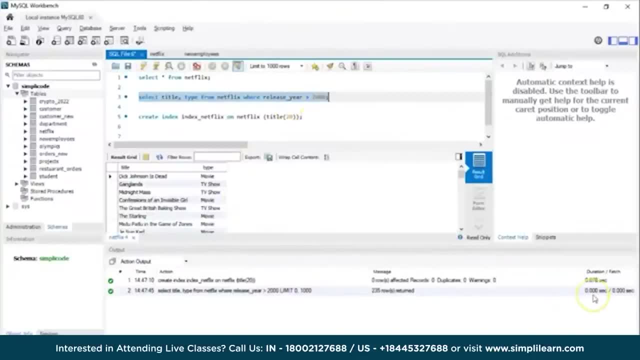 Netflix where the release year is greater than 2000,. it will basically take duration almost like in milliseconds, Like it is showing 0.00 seconds, but it will take a max to max up to one or two milliseconds only. So in this way you can use 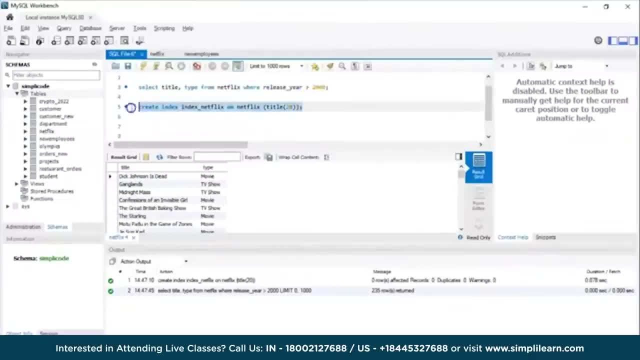 or index on certain columns. Now, if you want to create multiple indexes on different various columns, you can specify the different column names as well. So I'll just pop with this and I'll show you how it actually works. So title and similarly. 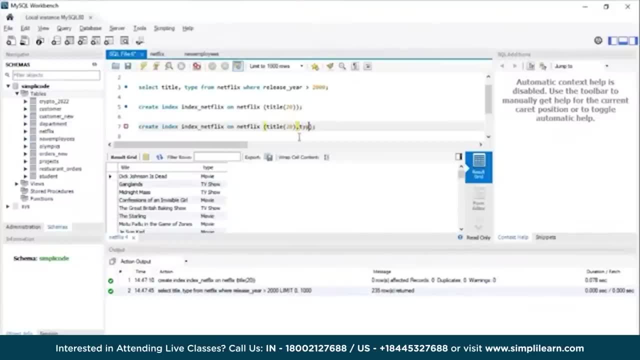 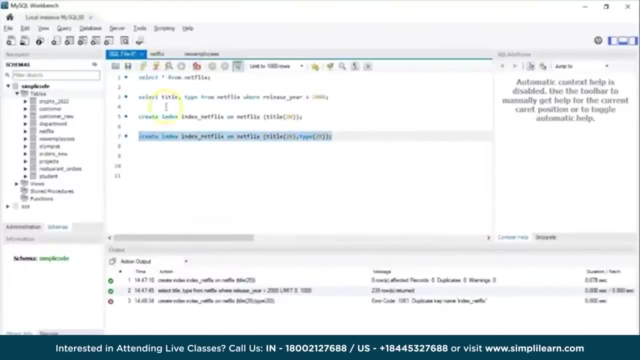 I want to create an index for the type as well, So let me just execute this statement. So I think we have to take another keyword here, So let me just take index new on Netflix. So, as you can see, a new index has been created successfully. 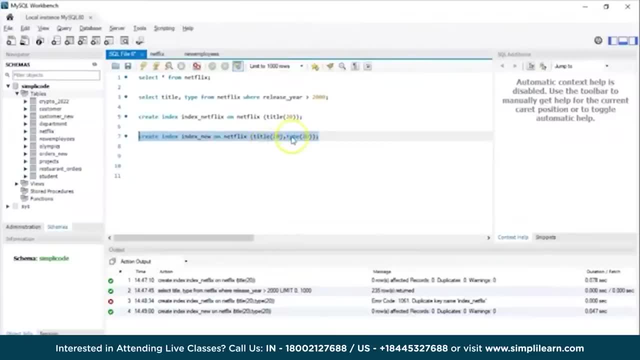 wherein it will create a new index for title and type. So whenever you are performing a certain query in order to retrieve the data from these two columns, that is, title and type, it will basically speed up the query process and it will retrieve the results. 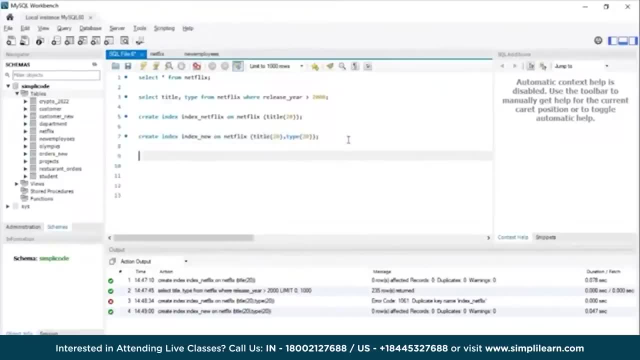 quickly. So let's say, if you want to know all the indexes that you have applied on the table, So in that case you have to write as show index from table name, which is Netflix, So it will basically show all the index details. 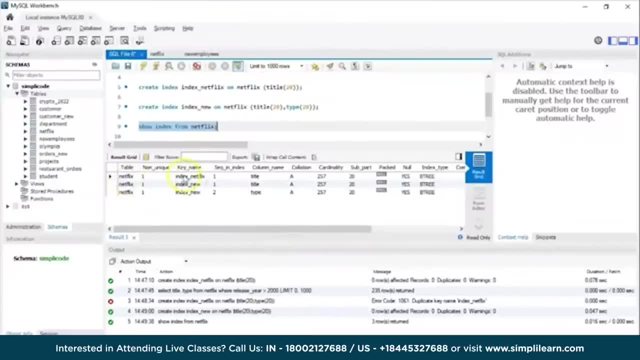 As you can see, we have created three indexes till now on the Netflix table, For example, index Netflix index, new index, new two times. We have created indexes on column names, like title type And similarly you can see, the index type is of B tree. 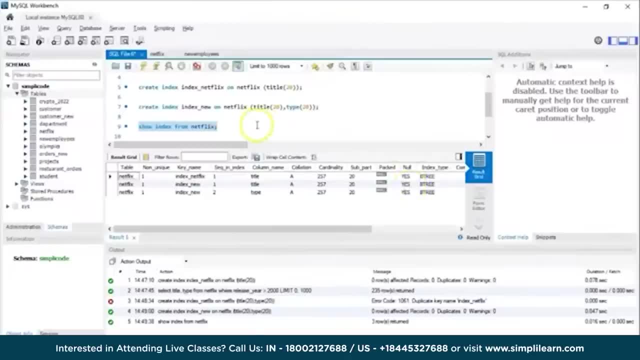 which we have discussed earlier, And it, of course, has null values. Now, finally, if you want to delete the indexes that you have created on your table, in that case you have to mention drop index, So the index that we have created. 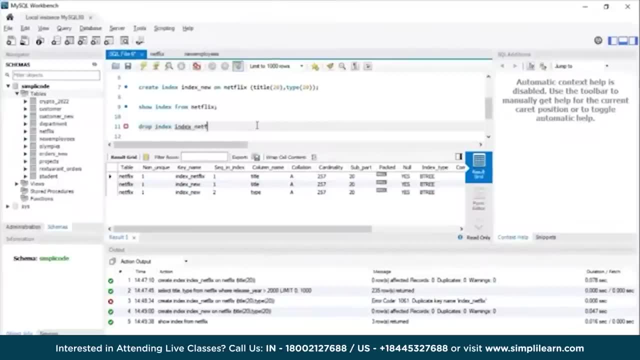 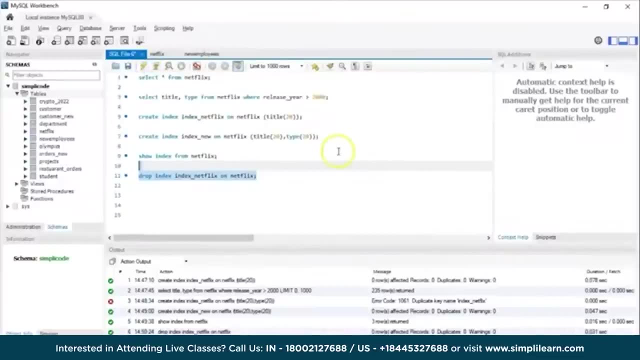 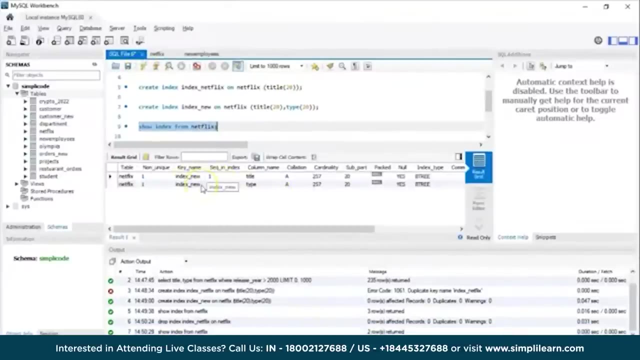 for example, let's say index Netflix On Netflix table, So it would basically drop the index. So, as you can see, it was successfully deleted. So let me just show the indexes. as you can clearly see, index Netflix has been successfully created. 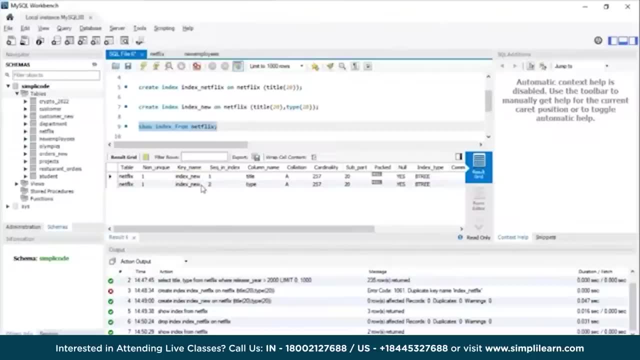 So in this way, you can use the indexes, as I discussed earlier, in order to make sure that your results are being processed fast and the data that you have in your tables are being retrieved quickly. So in that case, you will basically use the indexes. 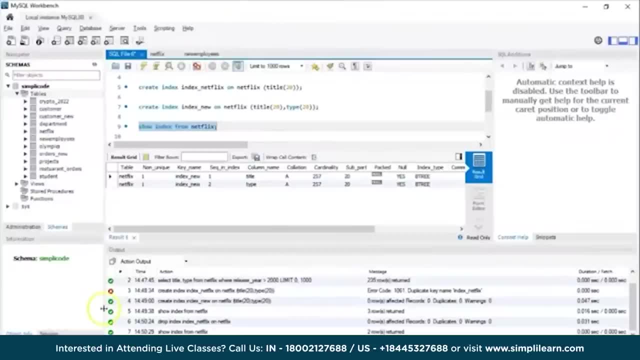 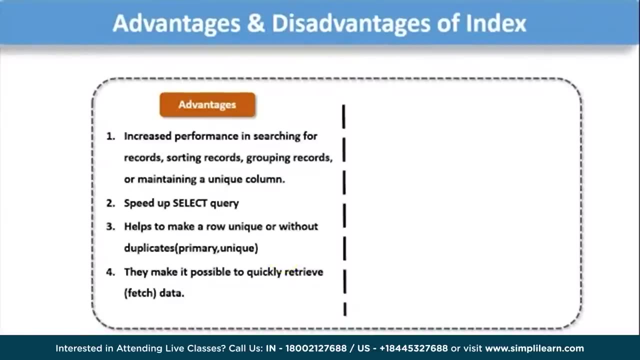 I hope you understood with this. So let us now move ahead and let us discuss some advantages and disadvantages of indexes. So firstly, let us discuss some of the advantages of index. Index basically gives the query optimization, which basically gives increased performance in searching for records or even sorting records. 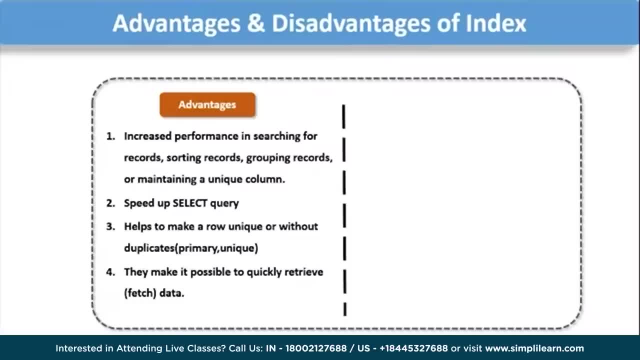 grouping different records or maintaining a unique columns, And it will also speed up the select query. And similarly, you can also speed up the process of the queries using the select as well as the where clause as well. Index also gives you uniqueness, guys. 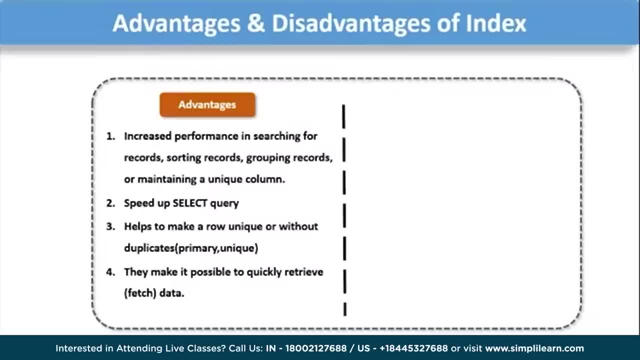 indexes, like primary key index and unique index, helps to avoid duplicate rows data. And, finally, indexes make it possible to quickly retrieve data, which is obviously one of the main characteristics of indexes. Now, there are a certain number of disadvantages as well. The first one is the indexes takes up. 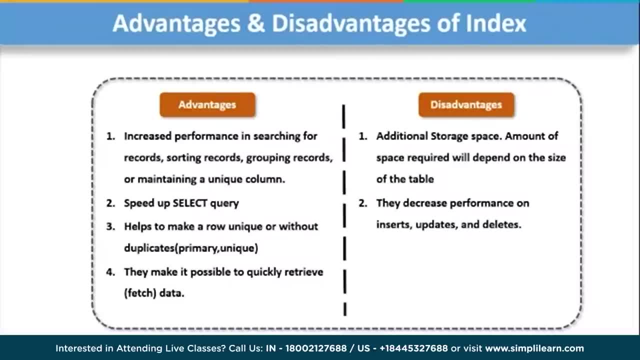 More or additional disk space. Usually the space usage usage isn't significant but because of creating index on every column in every possible combination, the index file would grow much more quickly from the data file. So in the case when a table is of larger table size or the data set you are performing is of larger size, 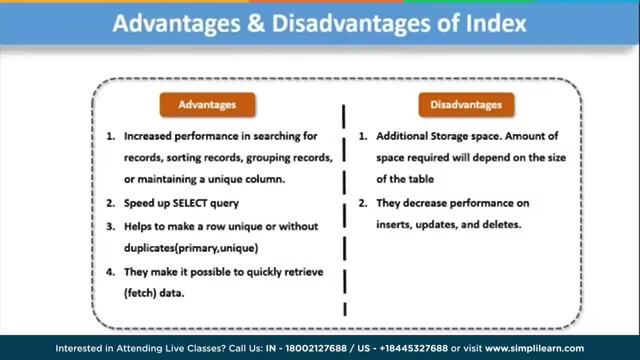 the index file could reach the operating systems maximum file size, and it can take a lot of size as well. Now, secondly, the indexes slow down the speed of writing queries such as insert, update and delete, because in MySQL, MySQL has to internally maintain the pointers to the inserted rows in the actual data file. 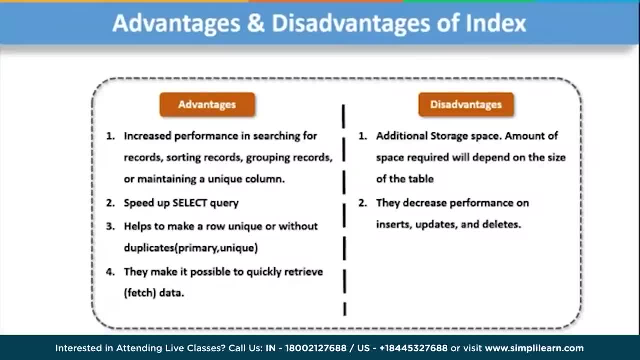 So there is a performance deficit, in order to pay in case of above said, the writing queries like insert operations, update operations and delete operations, because every time a record is updated or changed or manipulated, the indexes must also be updated. So, however, you might be able to write your. 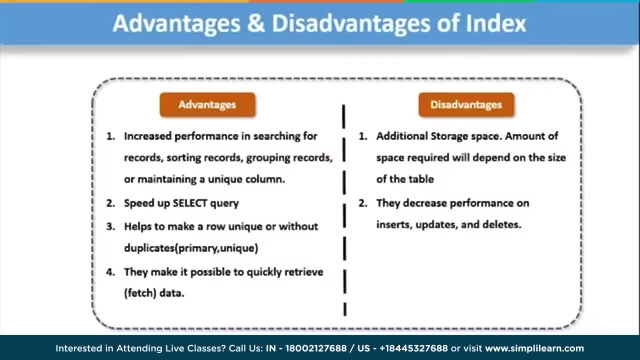 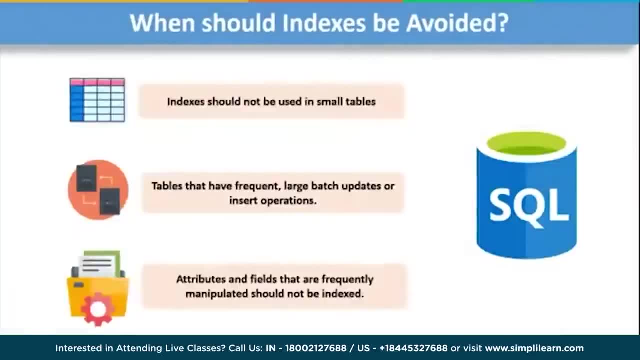 queries in a way that do not cause that very notable, noticeable performance degradation. right, So these were some advantages and disadvantages of indexing. So, finally, we'll move to our segment, which is: when should you avoid using indexes in SQL? Now, indexes should not be used in small tables. 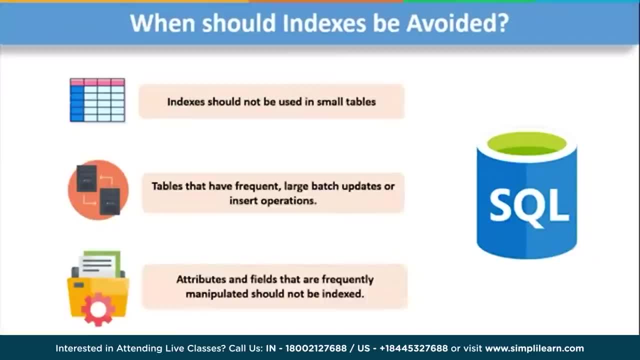 Like as I said earlier, indexes are only confined to large data sets or large tables that you want to retrieve the information from. So if a table has, let's say, less than thousands of records, I think it's better to avoid using indexes, and it will be of no use as well. 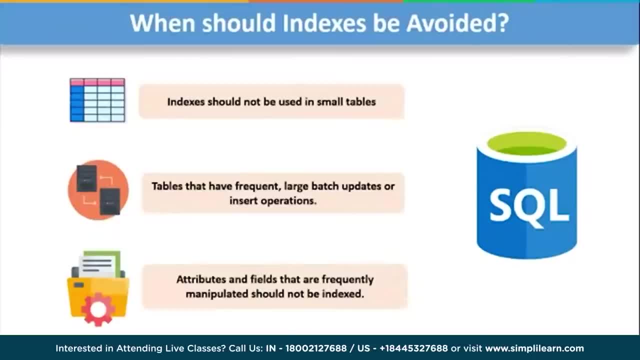 Next, tables that have frequent or large batch updates or insert operations. Now you can use indexes on huge chunks of data sets that have, like, frequent changes to its inner values, For example, if you're performing various search or insert operations on your tables. in that case, 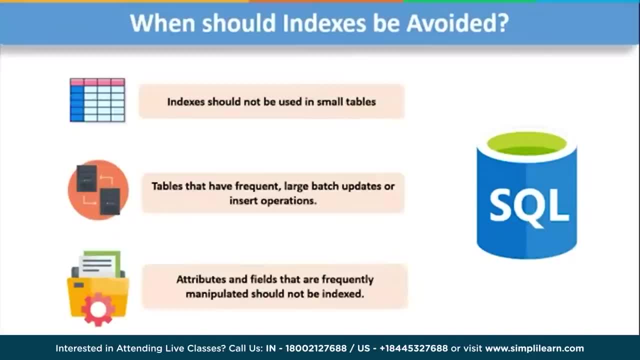 you can take the index. And finally, attributes and fields that are frequently manipulated should not be indexed. So if you're working on certain columns and the values that are frequently manipulated or updated, in that case you have to not use indexes. So that were some exemptions in the cases where 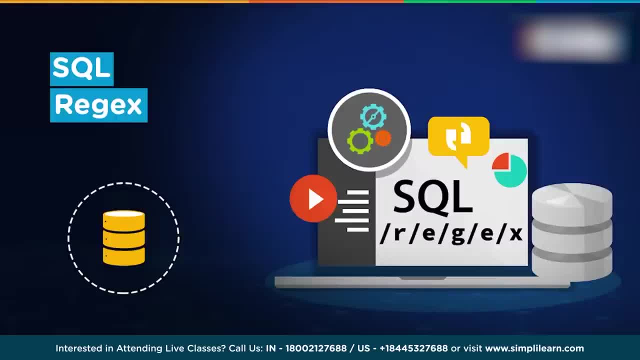 so, as discussed earlier, we'll be discussing about SQL Regex, which is a regular expressions. Now, as we all know, databases are enormous, enormous collections of data that are stored into organized data sets, But frequently we encounter circumstances in which we need to get some particular data. 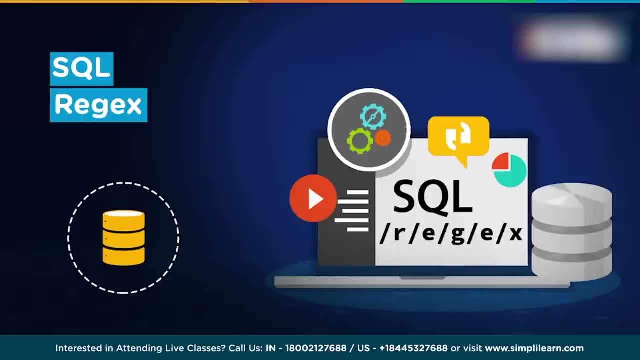 but lack the information necessary to filter it out. Regular expressions, which is a fantastic feature of SQL, comes in handy in this situation. So in this tutorial, I'll provide you with entire explanation of SQL Regex and we'll see how to use them to these mediums of various syntaxes and etc. 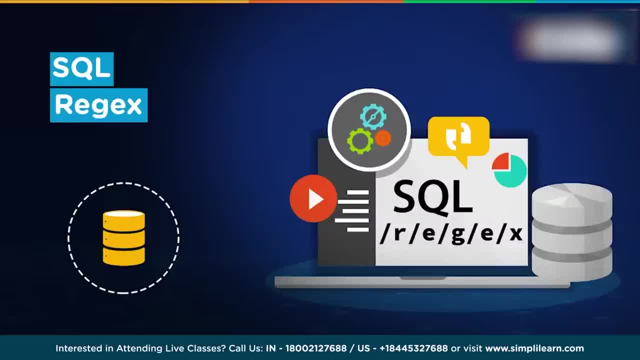 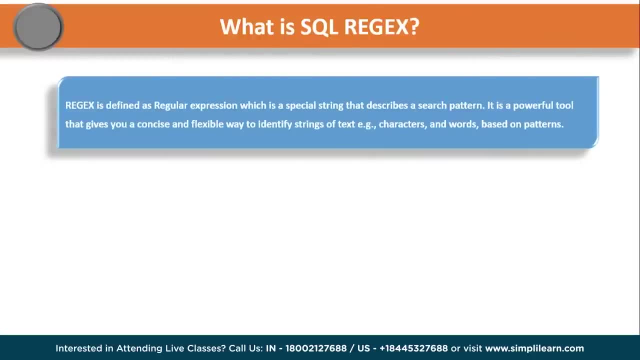 So let me just present my screen so that we'll go to the presentation Presentation part. All right, I hope my screen is clearly visible, guys. So let us first understand what is SQL Regex. Now, SQL Regex is defined as regular expression. 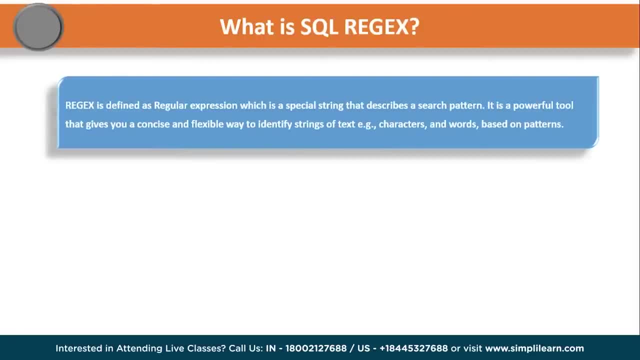 which contains a sequence of characters that are used to search and find a particular sequence of characters that matches a pattern. It is a rule that defines the way characters should appear on an expression. Search pattern is determined by the sequence of character or set text. 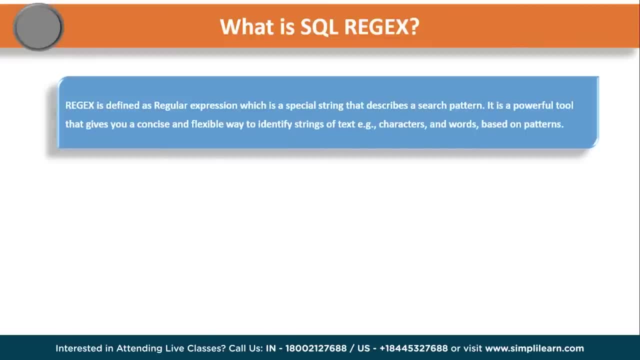 Say, for example: if you want to identify the data that contains a combination like a student's name, contact number, email ID, we can use a regular expression. It is also used in cases where you need to identify a particular text pattern or you need to apply a filter over numbers. 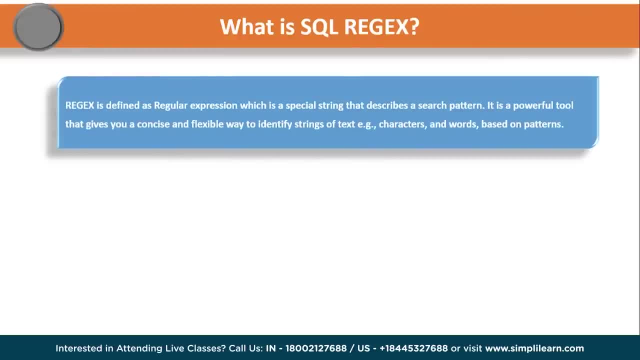 text or special characters data. Now you might be wondering: we have SQL like operation, So why is it? How is it different from the like operation? So basically, guys, if you're working on complex data set and if your search pattern is quite difficult, in that case, 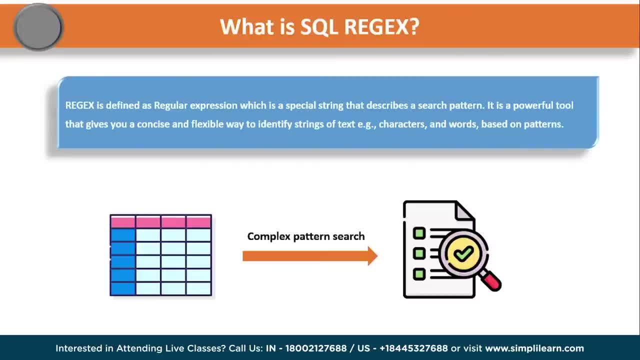 you have to use the SQL Regex. So, basically, regular expression provide a powerful means of identifying a pattern within a body of text. So a pattern describes what the text to identify looks like, and it could be something quite simple, such as that which describes any, let's say, a three letter word or four letter word. to something quite complex like that. 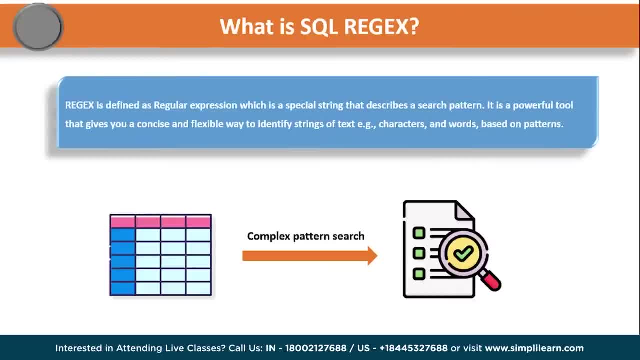 which can describe as an email Address. So it is a tool that gives you a concise and flexible way to identify strings of test for a text- example like characters, words based on patterns and etc. So let us now understand why we use SQL Regex. 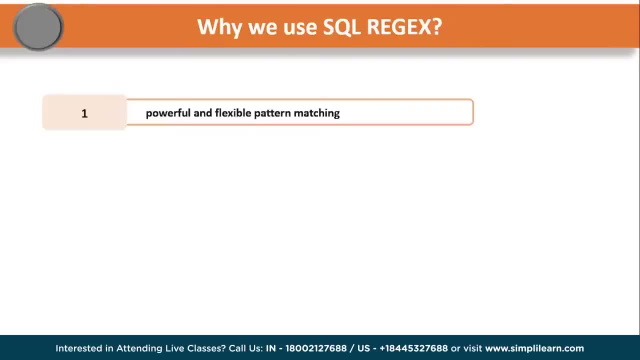 Now, regular expressions provide a powerful and flexible pattern matching that can help us implement power search utilities for our database systems. and it are also- and it is also not case sensitive, that is, it can work on both uppercase and the database. And it is also not case sensitive, that is, it can work on both uppercase and the database. 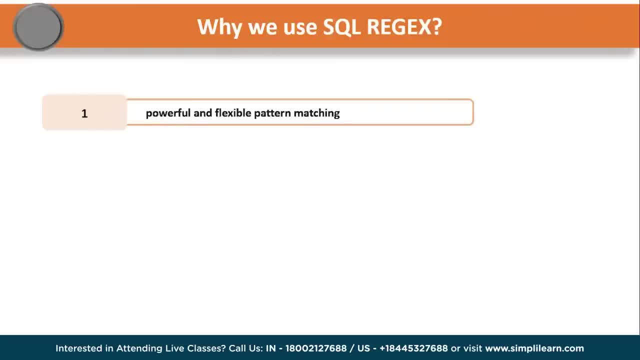 And the lower case as well. So if you want a particular case, you can mention them and you can proceed with your database set. So, basically, it provides a simple yet powerful mechanism for rapidly describe describing patterns and greatly simplifies the way in which you search, extract, format and manipulate the data in your database. 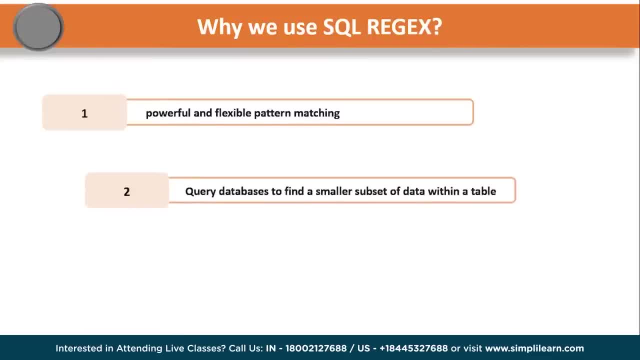 The second reason is it queries database to find a smaller subset of data within a table. Now we, as we all know that a simple form of pattern matching has been a part of SQL through the likes of the SQL like operator condition. that provides two variants of wildcards: with the zero or more than one characters. 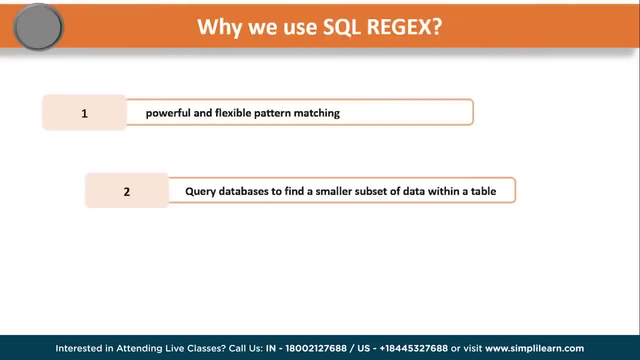 That is the percentage and the underscore. So such characters are termed as meta characters as they describe the pattern rather than the partake in it. So a simple example could be like: you know, if you want to find a name that starts with ABC in that case, 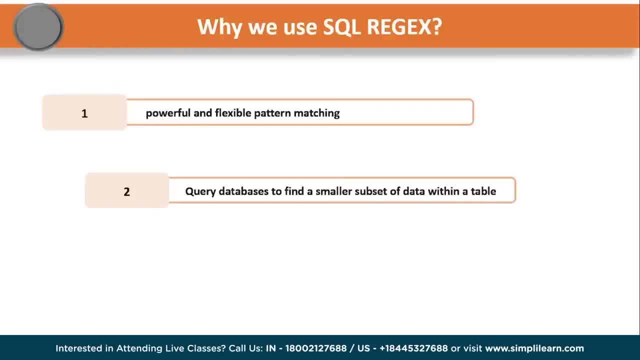 we use ABC percentage That matches any row that begins with the characters ABC right. So in many cases like is limiting and other solutions have been sought as mean to perform more complexes queries. So that is the reason we started using SQL reg X. 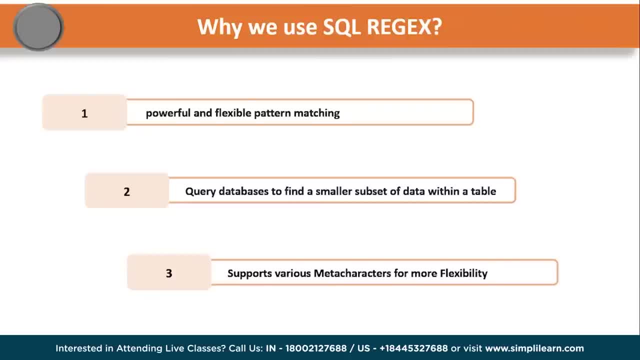 And finally, as discussed, it suppose we supports various meta characters for more flexibility. Now, unlike SQL, like, which provides only two wild characters, that is, percentage and underscore, We have a lot of meta characters when we use regular expressions, which will be will be discussing in a while. 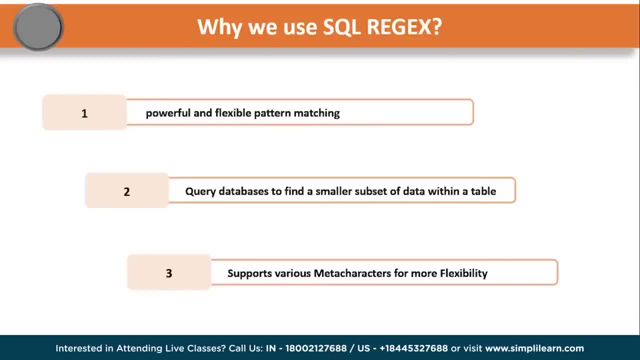 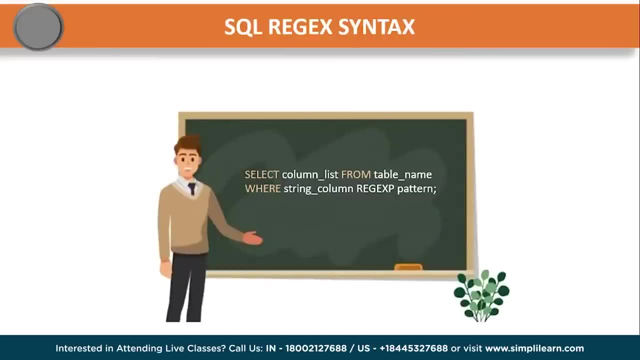 So those are some of the reasons why we need to use SQL reg X And finally, we'll discuss how it is different from SQL like operation as well when we jump into MySQL for execution part. So let us now understand the syntax of reg X. that is regular expression. 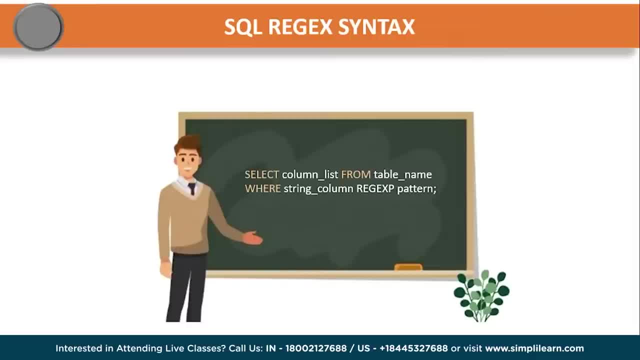 The syntax is followed as: select column list from table name. where string column: regular expression pattern. So basically the statement performs a pattern match of a string column against a pattern. So if a value in the string column matches the pattern, the expression in the where clause returns true. 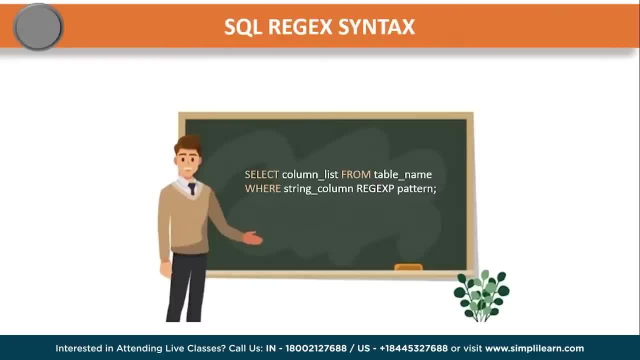 otherwise it returns false. So if either a string column or the pattern is null, the result rent set is also null. So again we have the select statement, which is the standard SQL keyword to retrieve the data, and we have the column list, which basically specify the rows that are to be retrieved, and we have where clause, which is used to 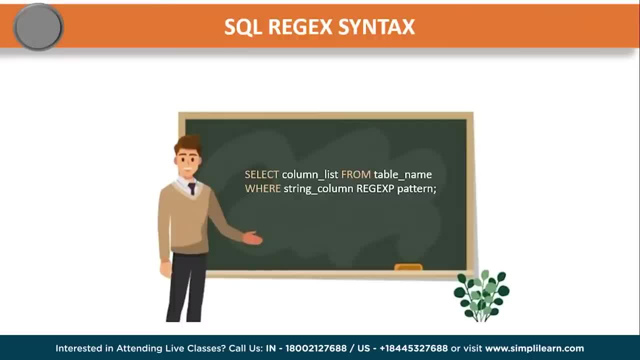 specify a condition while fetching the data. And then we have the field names, which represents the name of the column on which the regular expression needs to be applied on, And then we also have the reg X, P, which is the keyword that is used to find the pattern. 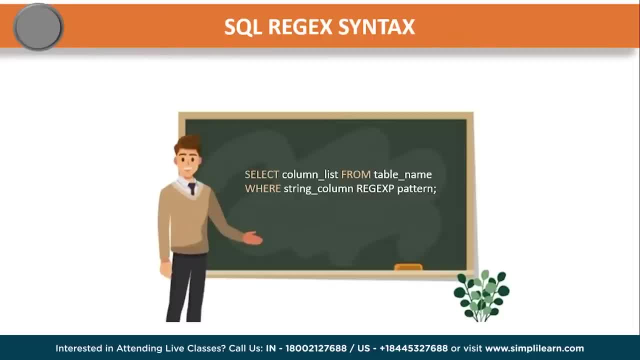 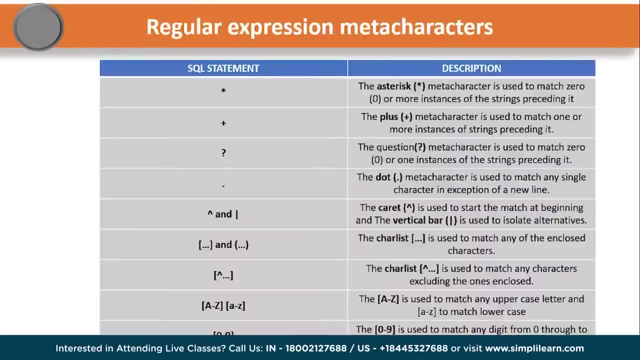 And finally, you have to mention the pattern, which is basically a user defined reg X pattern using certain meta characters to search the data. All right, So let us now discuss some regular expression meta characters that are used in SQL Now. the first one is the asterisk operator. 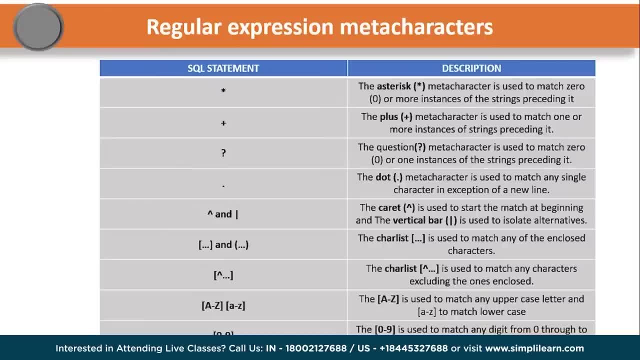 So the asterisk meta character, basically, is used to match zero or more instances of the strings preceding it. Now we'll understand this when we are executing in the MySQL workbench, So I'll just explain the description of how this meta characters work. 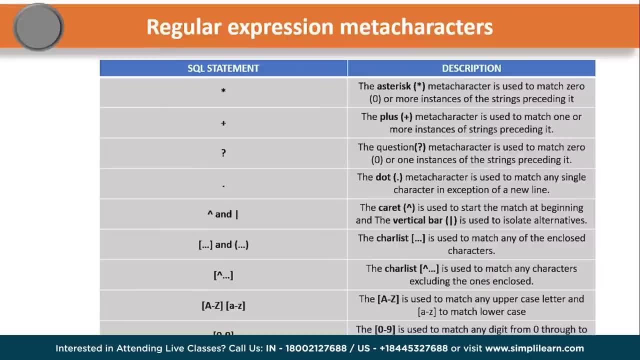 So next we have the plus meta character, which is used to match one or more instances of a string, And next we have the question meta character, which is used to match zero or only one instance of a string. And then we have the dot character. 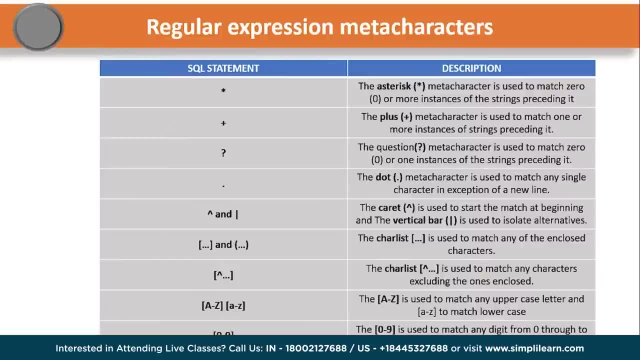 which is used to match any single character, in exception of any new line. And then we have the caret, which is the symbol which you can see, And we have the vertical bar or the pipe symbol, which is used to start the matching at beginning and which is used to find the characters, alternatively, respectively: 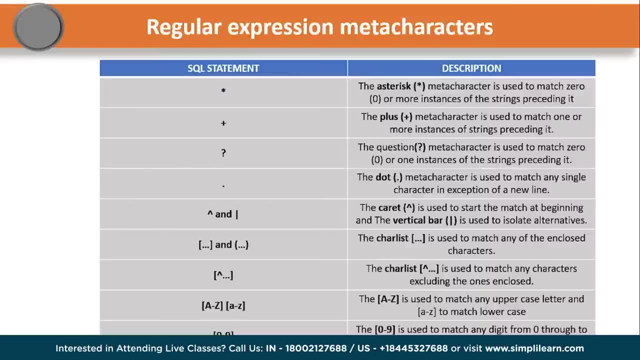 Next, we have the square brackets and the closed brackets, which are used to match any of the characters in the enclosed characters, which basically matches all the characters that are mentioned within the brackets And if you want to find exact, so exact name or the characters name, 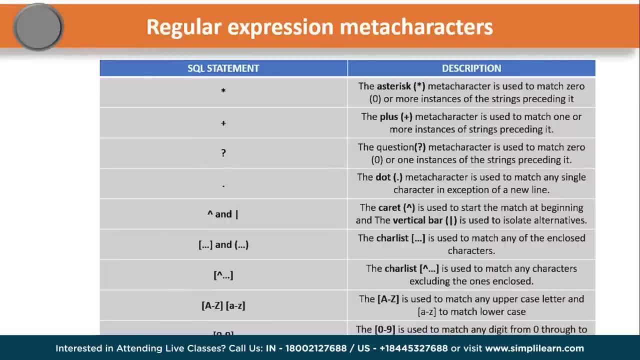 you have to take the closed brackets. And then we have the closed brackets And we have the caret meta character, which is used to match only those characters, excluding the ones that are enclosed within the square brackets. And finally and next, we have the uppercase and lowercase characters. 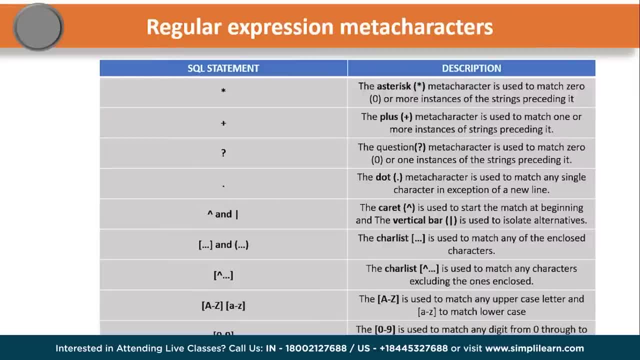 as well. If you want to specify only, if you want to retrieve only certain data which is in like, if you want, in uppercase letters, you can use from A to Z, which in upper cases and similarly in lower cases, that is, from A to Z. 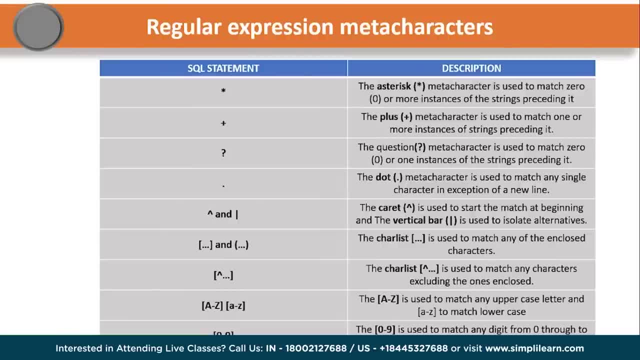 And finally, you can also perform operations on the numerical values as well. So, within these square brackets, you can mention any numbers starting from ranging from 0 to 9, which basically matches any digits from 0 through 9.. So these are the most commonly used regular expression meta characters. 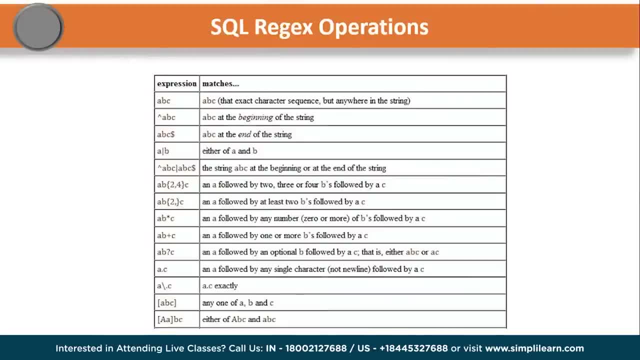 So let us now discuss some SQL regex operation and see how they exactly work. So you can also take a snapshot of this so that you can it can be handy in future as well. So, for example, if I have an expression where I'm stating as ABC: 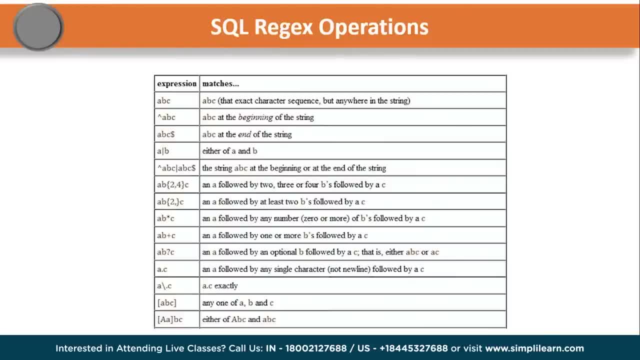 that means the query is basically searching the exact character sequence. that is ABC, that it should be in a proper sequence but it can be in any way. that can be in any position of the string. And next we have the caret ABC. 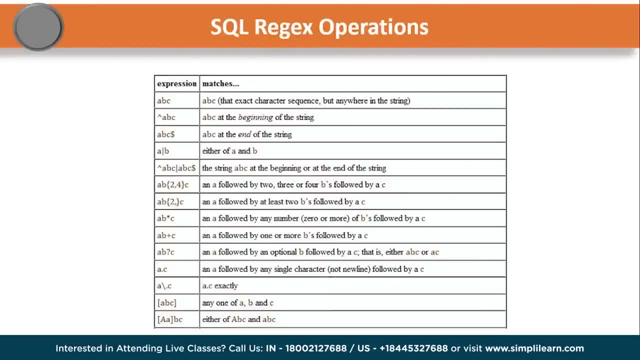 that is, ABC should start at the beginning of the string And similarly we have ABC dollar sign, which will basically search for ABC pattern at the end of the string. And we have A pi B, which will retrieve the values which has either a character A or B. 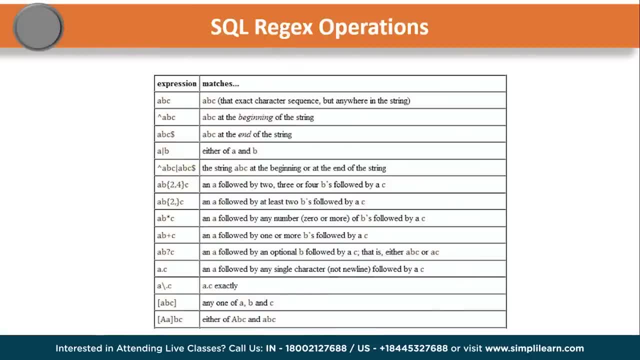 Now we can also perform multiple operations using various meta characters simultaneously. Now, if you look at here, I have- I've taken the caret- I've taken the pipe symbol as well as the dollar symbol. So which basically states that it will look for the string ABC at the beginning or at the end of the string. 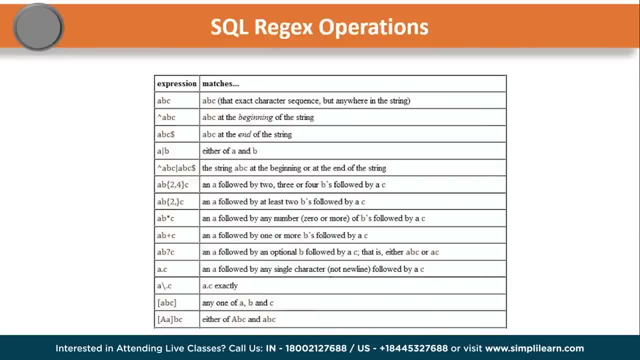 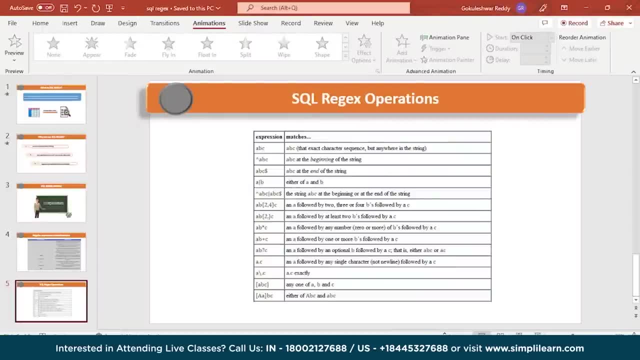 So and so on. you can look at different operations which we'll now discuss as we jump into the MySQL workbench for execution part. So let us just jump into MySQL workbench. So, as you can see, MySQL workbench has started. 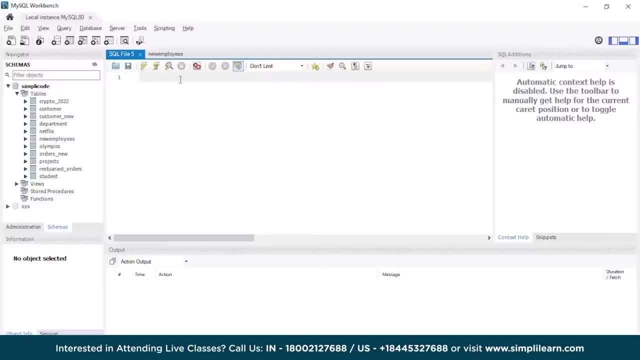 Let us now consider a simple table to perform MySQL regular operations. So let us just consider the Netflix table which is in our database. So let me just retrieve the values I'm using select star from Netflix. So the Netflix table has various attributes. here, guys, 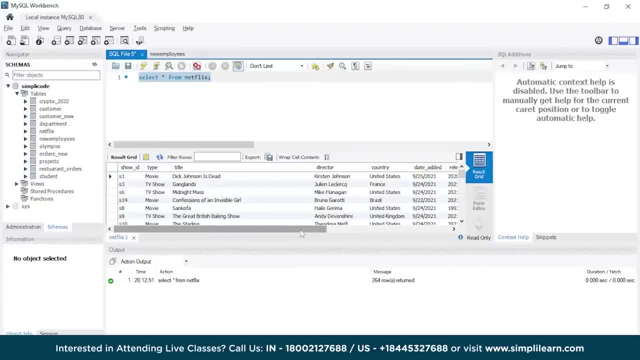 which has show ID, type, title, director, country, date which is added, release year, rating, duration and journal. So let us perform some basic to advanced. you know SQL regular queries, So let us start with a simple one. 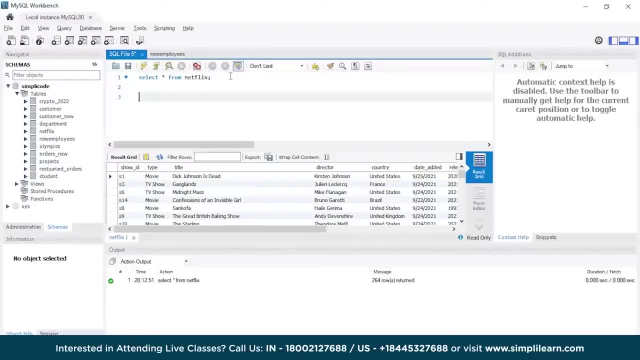 which matches literally the complete sequence of a string that we've discussed earlier. So let's say, if I want to find the title from the Netflix table where the title starts with, let's say, let us take any sequence like ran, Okay. 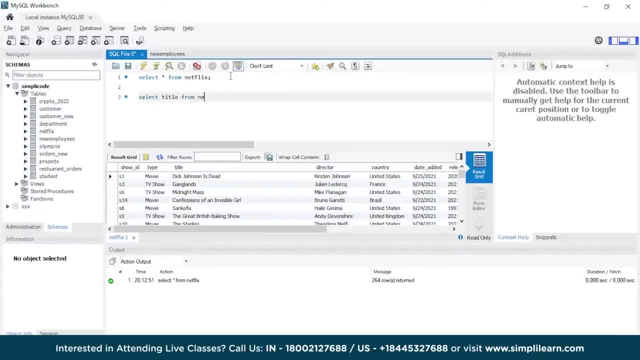 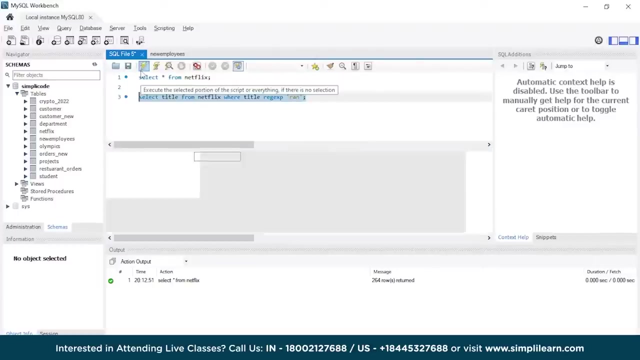 In that case, the following query would be: select title from Netflix, Where title reg XP is the keyword And within a single quotes mentioned the characters that you want to see. So let us take a ran, as I've said earlier. Let us just execute this query and we'll see the output. 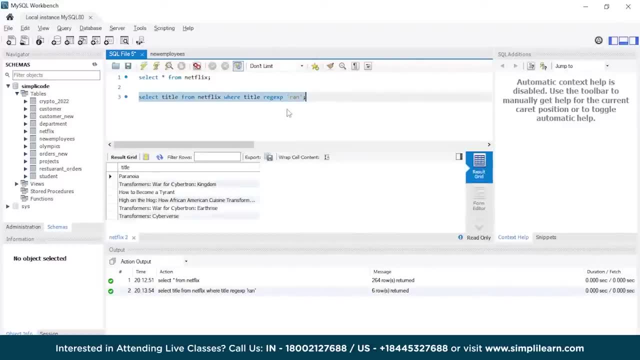 So it will basically search for all those titles which has RA and that is ran in the same order or the same sequence. So if you look at your paranoia, which has a ran in the same or the car in the same order And similarly, 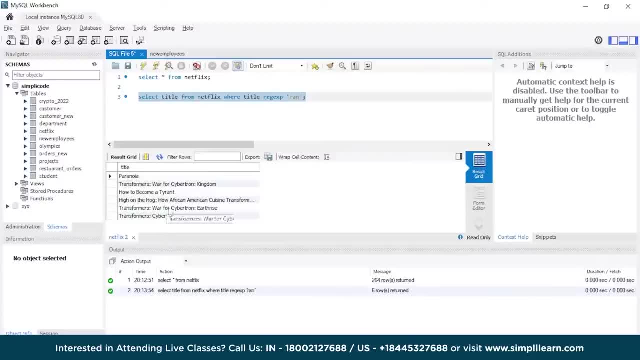 we have Transformers again, which it has ran, And if you look at the next title, which is how to become a tyrant, Similarly in tyrant we have ran and so on. So in this case you can- you can take the multiple characters to find a complete sequence that is in its original sequence. 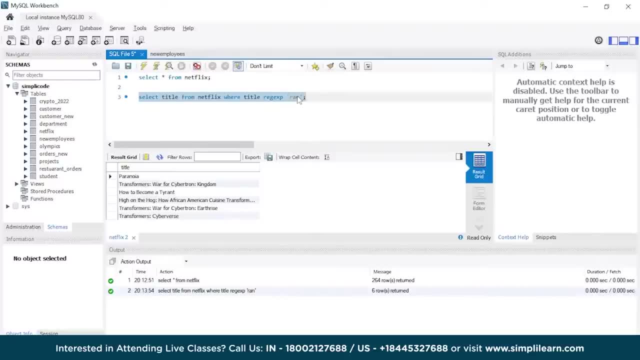 All right, moving ahead. not just only characters, guys, you can also find for for a particular word, which is basically a substance. So let's say: if I want to find, let's consider love. So if you want love in our title, 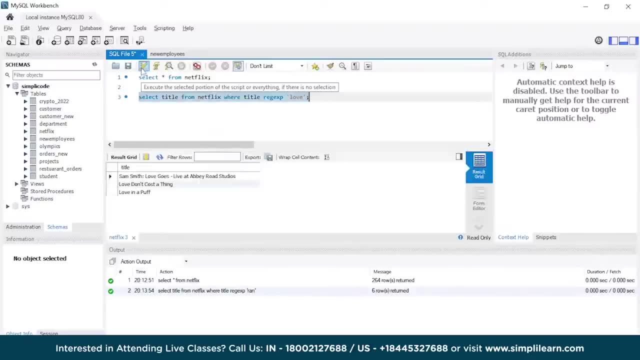 let us just mention love in the single brackets and we'll see the output. So, as you can see, there are a total of three titles that has a love substring in the complete title. For example, Sam Smith: love goes live at Abbey Road Studios. 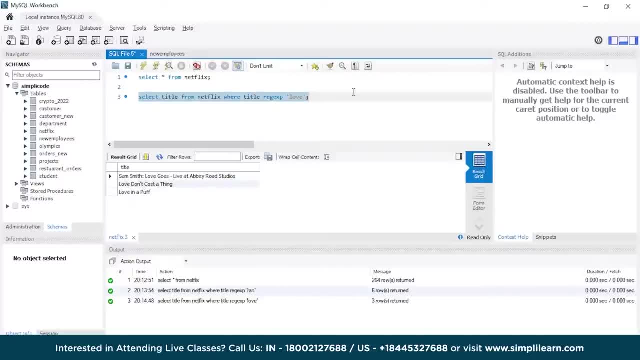 And next we have love don't cost a thing. and finally love in a bus. All right, moving ahead. Let us now discuss another example where we'll use the asterisk, the plus sign and the question mark. So let's say, if I want to find the title from the Netflix table again. 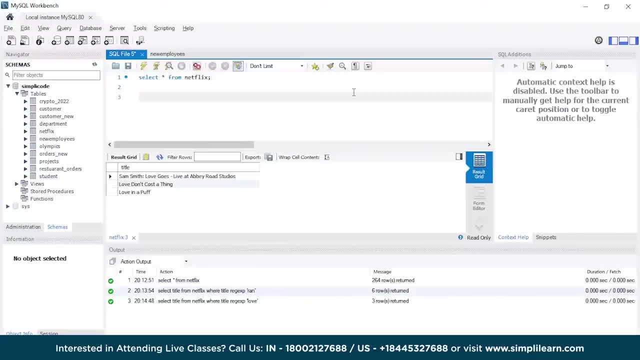 where in the pattern is. it starts with a and n and it should at least have a one instance that it occurs and finally should have an key. So what? and it's bit confusing, So let me just write the query so that you guys will understand. 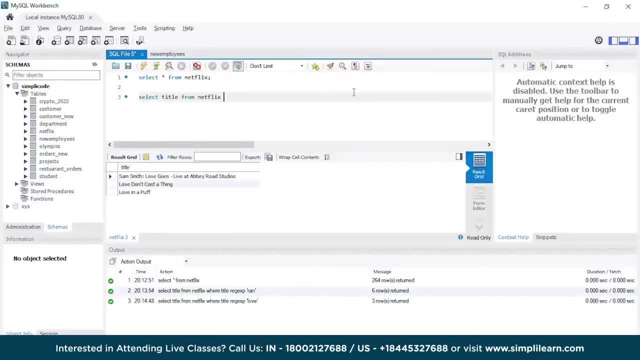 So select title from Netflix Where title reg xp, a, n, star, operator and mention k. So what this query does is it will find all the titles from the Netflix table which has a, which has, and that is now, as we discussed. the asterisk operator finds: 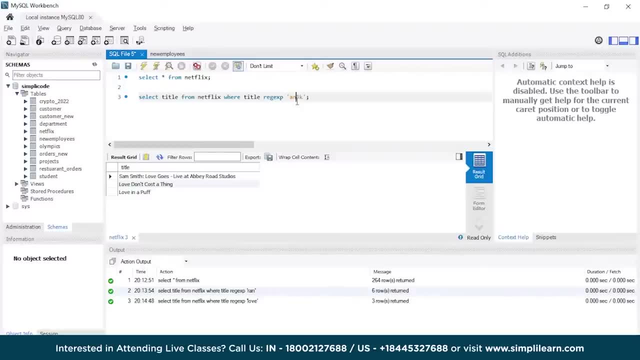 you know characters which have zero or more instances. that occurs In a table right, So in that case the asterisk operators work. So let us now execute and we'll see the output. So, as you can see, these are all the titles. that has a and k as a sequence. 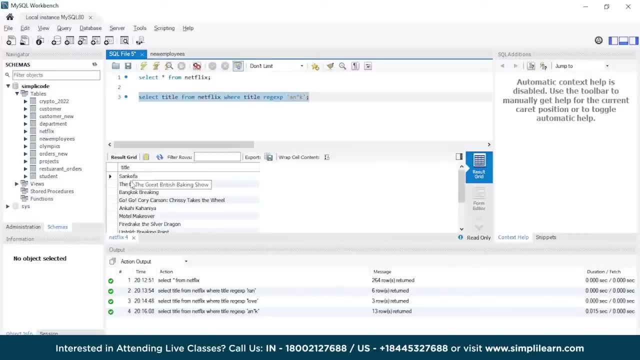 wherein it can have zero or more than one in. So if you look at Sankofa, it has a and k, which has one in, and similarly, if you look at the Bangkok breaking, it does not have any in between. that is because it can have zero or more. 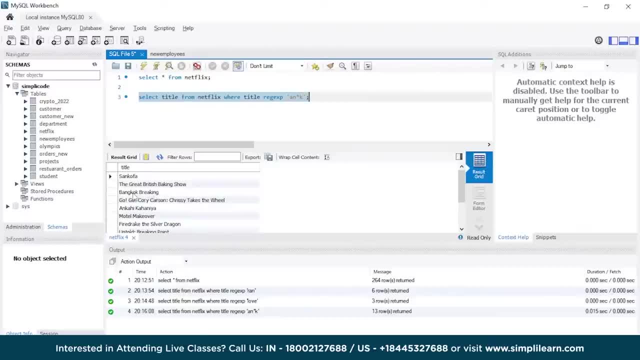 More than one in. So in that case we are taking the Bangkok breaking as well in our title and similarly the others as well. So in this way, if you want to use this asterisk operator wherein the first one has a character and then the next one has zero or more than one instance of appearing in the sequences that you have mentioned, in that case 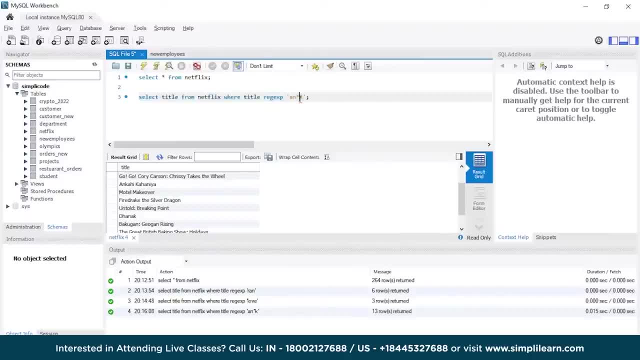 you'll use the asterisk operator. So let us now take another example where we'll understand how to use the pipe meta character. Let's say, if you want to find the genre of all the details of the titles, you know where it can be crime or it can be either thriller or it can be fantasy. 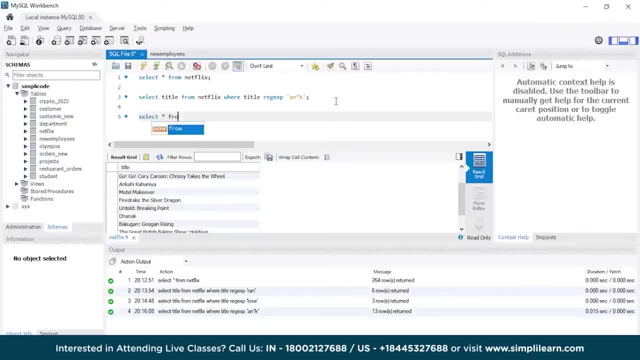 So in that case, the following query would be: select star from Netflix Where Genre Reg Xp Within single quotes? Now I want the genre to be either crime- and I'll mention the pipe symbol, So do not mention the space here. guys directly mention it and why it can be thriller and finally it can be a fantasy as well. 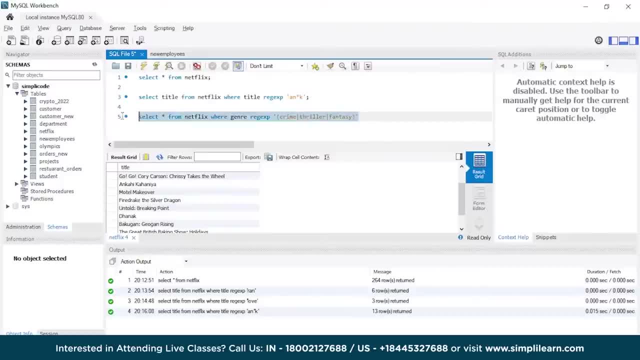 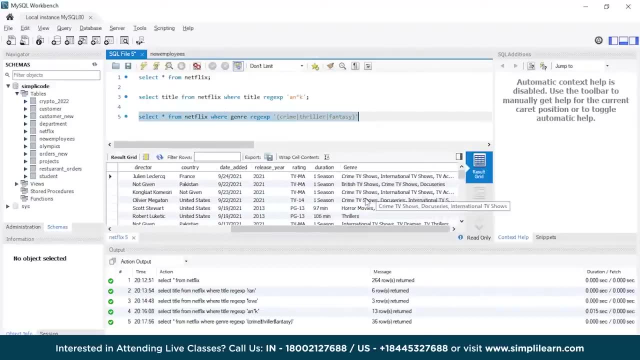 So let us just execute this statement and we'll see the output. So, as you can see, if I scroll this a bit, so it will display the uh records of all the titles that were added to Netflix, which has genre of either crime. 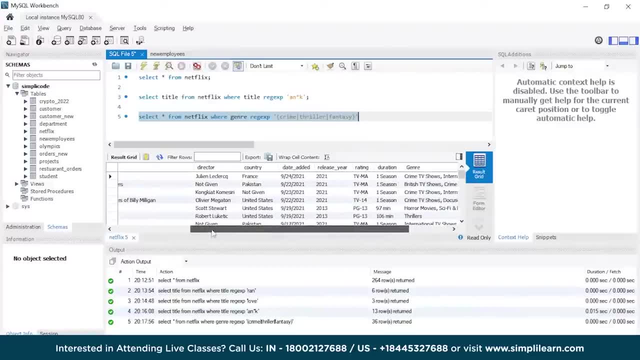 thriller or fantasy. So if you look at this, uh, for example, title Ganglands, which is crime, TV shows Similarly. second one: we have crime again. And if you look at, we have a thriller here which is basically movie paranoia. 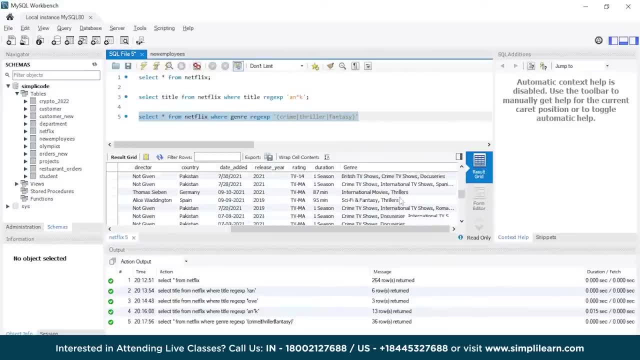 And similarly we have fantasy as well. I guess if you scroll down a bit we can find it. So, as you can see, we have action, adventure, sci fi and fantasy, So it will basically search for all the substance. 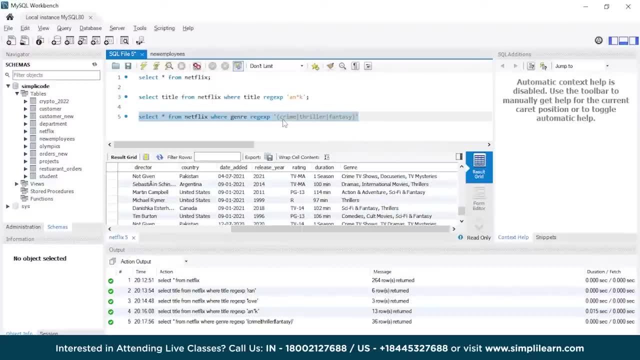 which has basically has a crime or thriller of fantasy, stop substring in the genre names. So this is how you can use uh, the pipe operator, instead of now, when we, if you remember, if we use the SQL like operator, which we use the percentage sign. 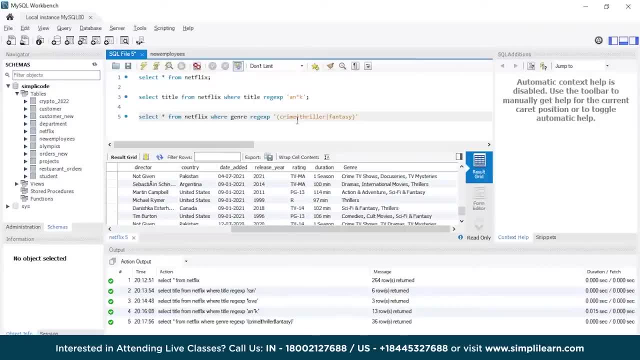 right. So in that we have to use multiple or uh operator in order to find the result. So in this case we are just mentioning the pipe operator, which will automatically search for all the uh characters or the strings that you have mentioned. 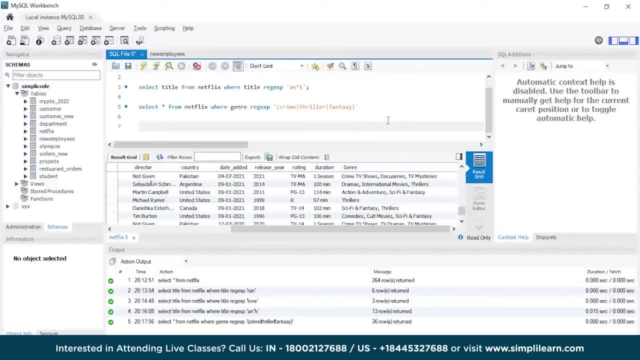 All right, let us now move to another example, where and discuss another scenario wherein we'll uh match multiple, multiple characters with a single characters. So what I mean from that is, uh, let's say, if I want to find the details of all the titles- 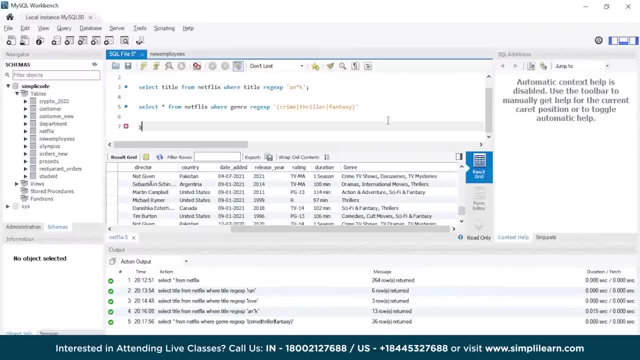 which has a combination of characters B, C and R. So in that case, the following query would be: select star from Netflix where title reg XP. Now, within the close brackets, I'll mention two words, That is, B. 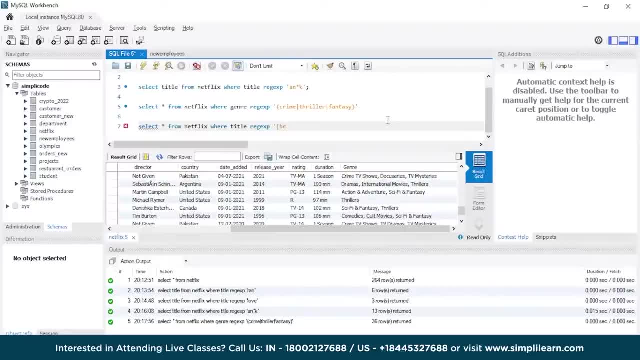 R, sorry, B C. let us take as a B C and I'll close the brackets and I'll mention our next. So it will basically search for all the patterns which has either B? R or C? R in the title name. 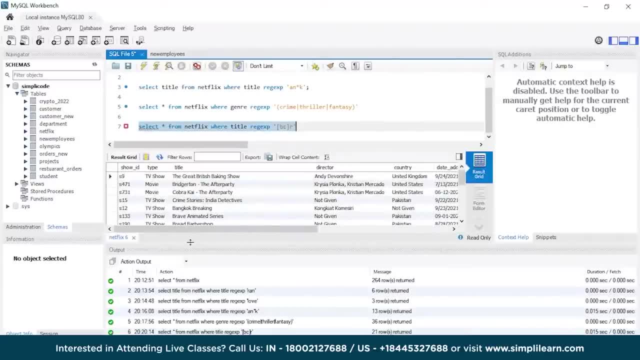 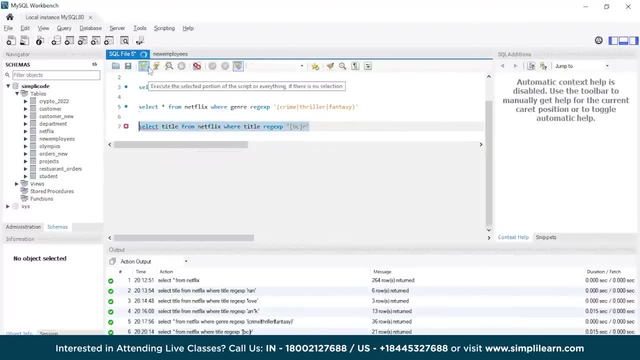 So let us just execute this and we'll see the output. Okay, Let us just only mention the title so that we have a clear idea. All right, So as you can see, uh, if you look at the pattern B R, 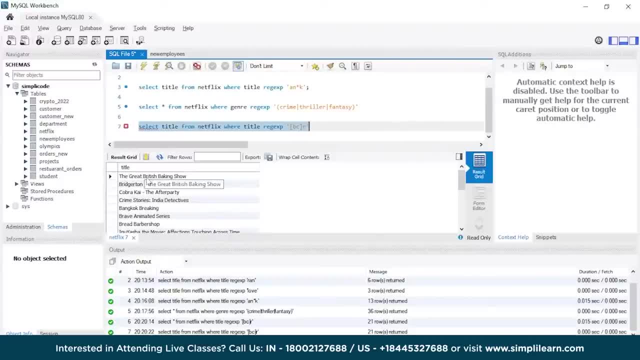 right. So in the first one we have the great British, which has B R continuously, So it. it does not mean that it can have it any random position. It should be in a sequential order. that is continuous position, So B. 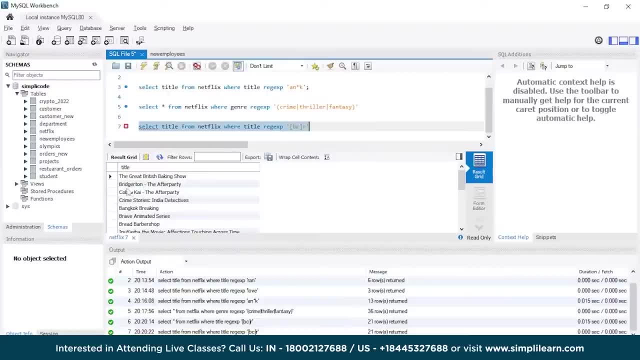 R, we have British right. Next, if you look at the Bridgerton, again we have B? R. And similarly, if you look at the Cobra Kai, we have B? R again. So that was one instance Now. 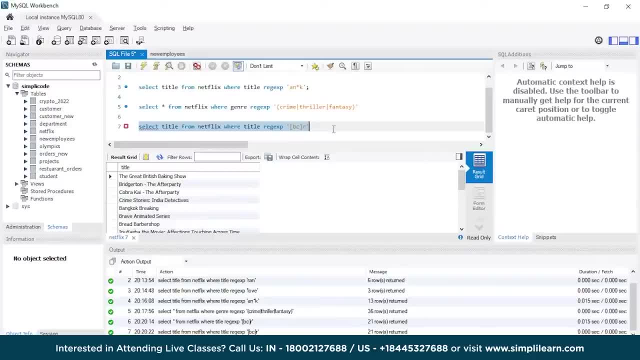 if you look at the CR combination, right, If you come back to the CR combination, we have crime stories which has CR, And similarly, if you scroll down a bit as well, you can find some more examples Of CR as well. 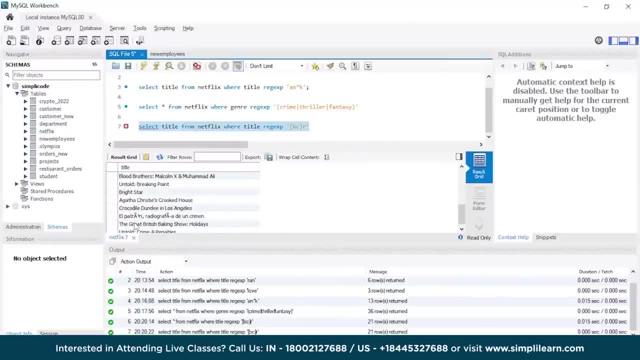 So again, you can find Crocodile Dundee in Los Angeles, which again starts with CR pattern. So in this way, you can find multiple characters while mentioning them in the square brackets and with a single character as well. All right, let us now move to another example where we'll use the close brackets. 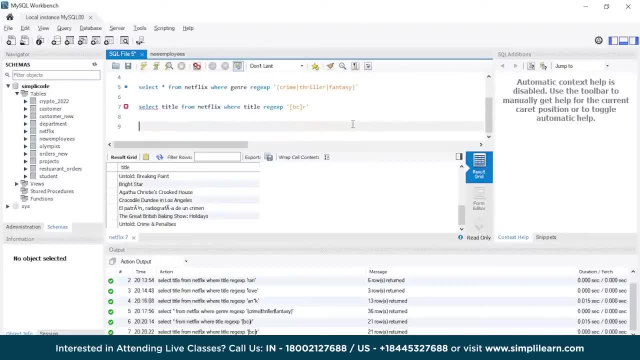 Now the close brackets is complete opposite of the square brackets, which will find the exact word that you are trying to find. So let's say, if I'm finding, if I want to retrieve the director details of the shows that they have directed, and the director's name should be either: 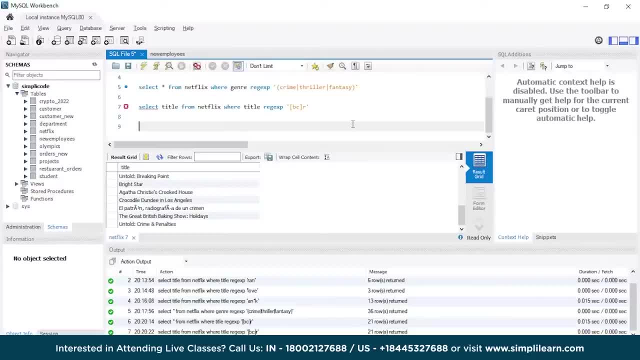 Let's say Anthony on it. should, you can either have its name has, that can start with B or or a character C. So in that case, what I'll do is select director from Netflix there. Director reg XB. Mention the single quotes and we'll use: 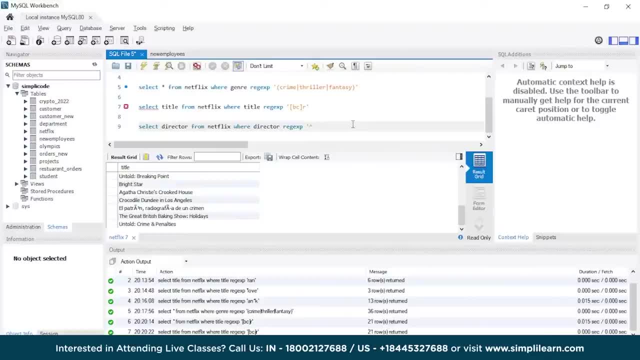 This operator, Which is basically the carrot symbol, And within the close brackets I'm mentioning and doing that is, the director names should start with Antony, Or his name can start with B or his name Can start with C. So this is one of the pattern that we are looking into now. 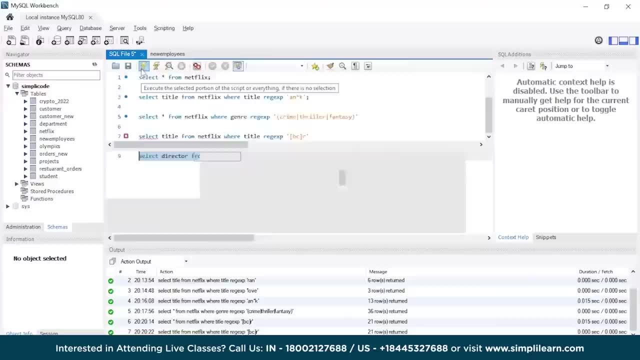 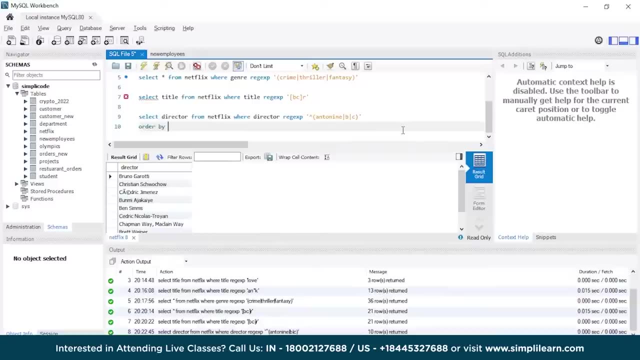 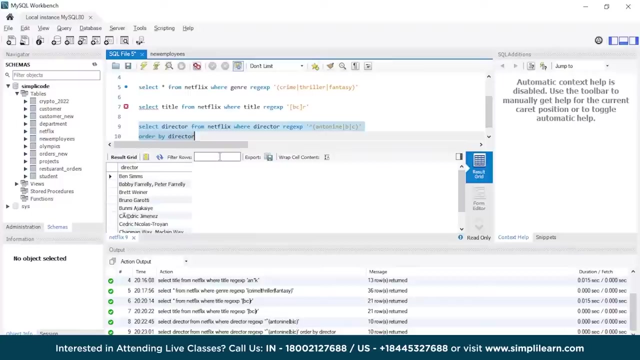 So let us see how it executes. So let me just display the results. All right, Also, we will use the order by, so that we'll have in, Yes, any descending or ascending order as per our wish. All right, as you can see in the result and said, the director's name has started with B. 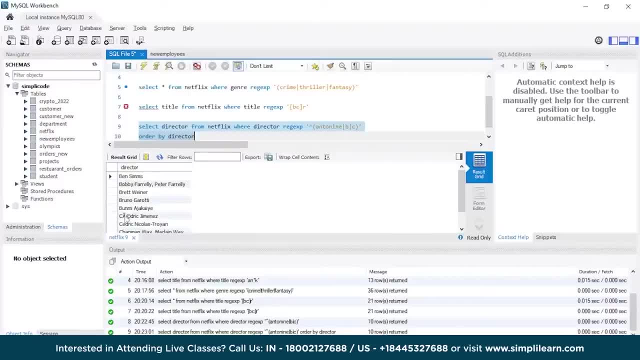 So which is satisfying a condition which you have taken, B and similar. if you scroll down, we have the director's name starting with C, which is again satisfying the condition that we have taken, and also it will look for the director name whether it is starting with Antony or not. 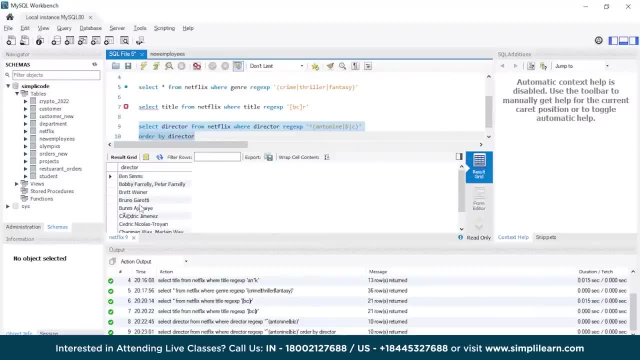 So I don't think we have Antony here in this, So it will omit. so you can basically take Any other character as well. So let's say, if I want the director names to start with M, So in that case it will search for it as well. 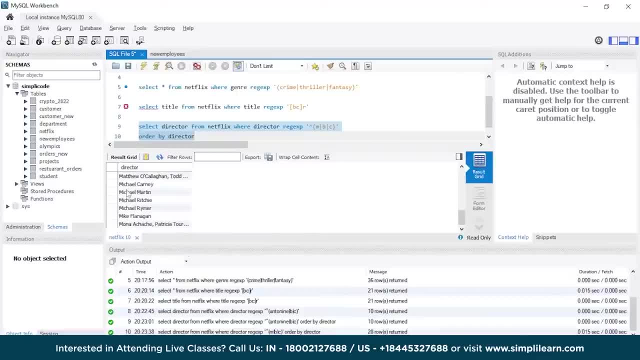 So if you scroll down, it will display the reports of all the directors. who has M as the starting letter? So we have like Mark Romson, Mark Thornton and Martin Campbell and similarly, etc. So in this way you can use the close brackets with the carrot symbol as well as the pipe symbol to find another pattern in this way as well. 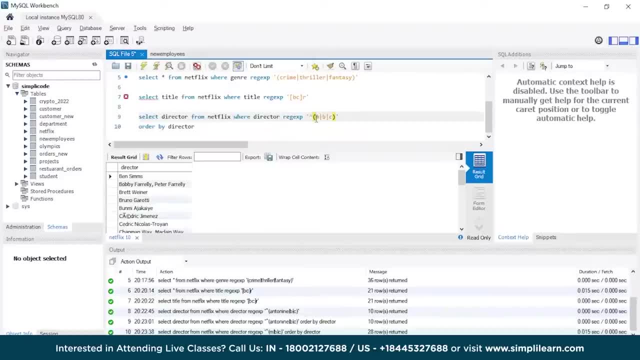 So now, if you want to find the director's name other than M, B or C, in that case you have to use the negation operator, which is basically another carrot which should be embedded inside the close brackets. So when you execute this query, 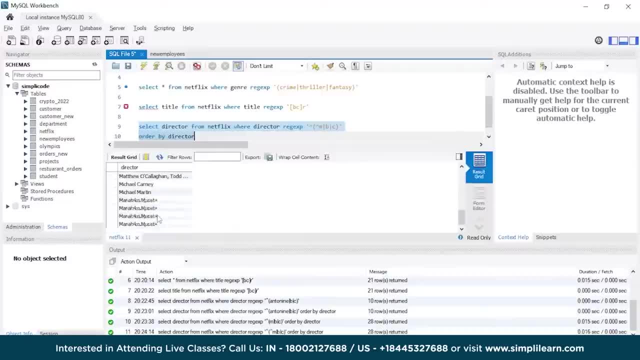 All right. so we have to use the square brackets here in order to retrieve all the details of director's name whose name doesn't start with the characters M, B or C. So if you look at the result and said, it is displaying the director's names like starting with. 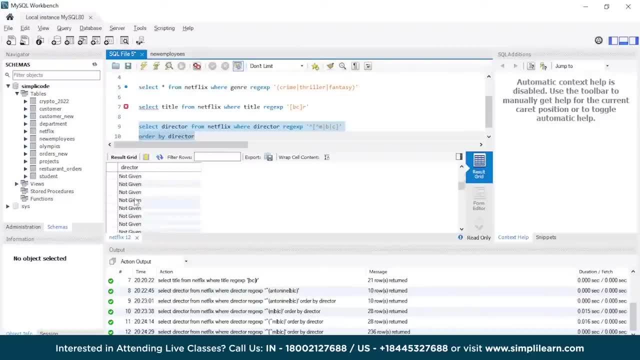 A, D, F, G, H, J and so on, S, T, W and Y. that is basically except M, B and C characters. It will display the records of all the directors, So in this way, you can also use this kind of pattern in order to find the data as well. 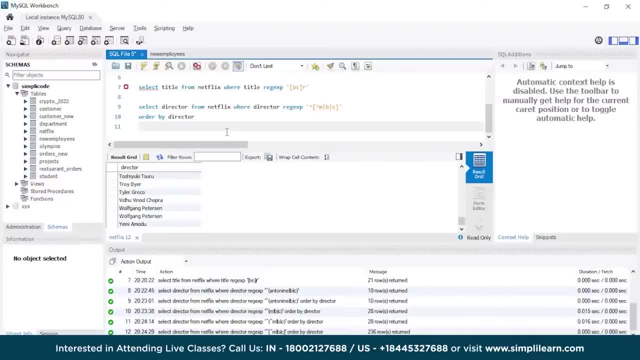 So let us look into our final, you know- example wherein will perform a complex, you know, regular expression Search, wherein will find the title, the directors and the release here and the type, that is, the genre from the table where the title name will be within a range. 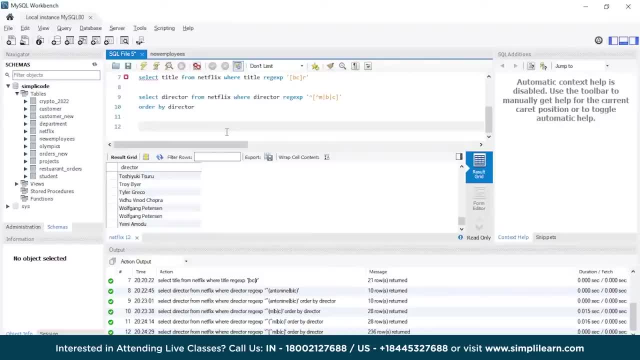 So let us consider a range here. That is the all. these are the target title, that where the title name starts with a character C and it can be in between C to K, and it should have a type from Netflix. From Netflix, where title Reg, EXP is a keyword. 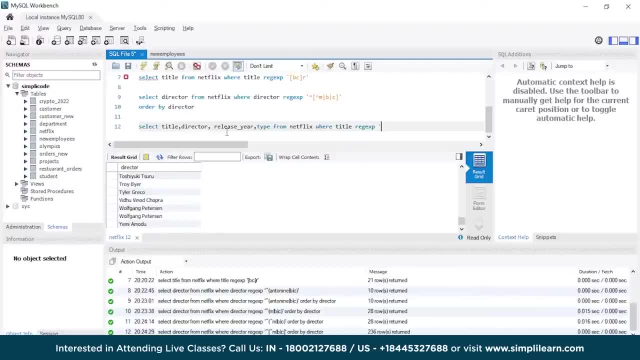 Open the single brackets. I'll mention the carrots in well, and let us mention the range now. So I want the titles name in the range of the characters C to K. So let us mention them and we'll close the brackets and then mention the dot symbol because it will. 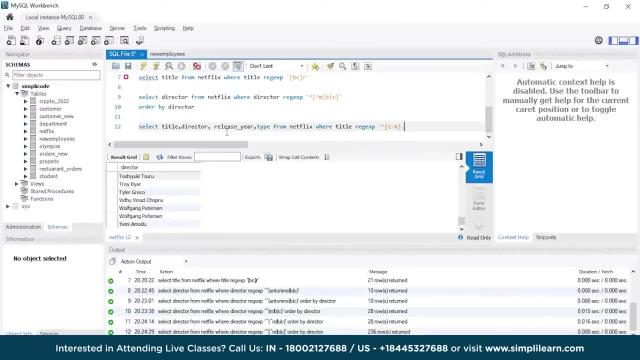 allow you to find a single character in between, and we'll have a total of 12 characters. So the title name should be of total 12 characters and we have to mention the dollar symbol. So let us just execute the statement and we'll see the output. 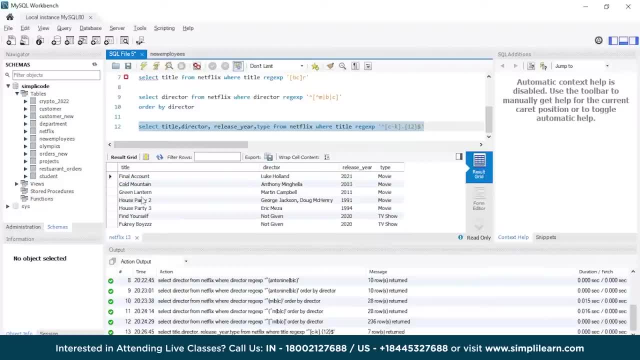 So if you look at the result and set in the, we have the title names, which has a total of 12 letters. So if you count the first title, which is final, account 1,, 2,, 3,, 4,, 5,, 6,, 7,, 8,, 9,, 10,, 11,, 12.. So 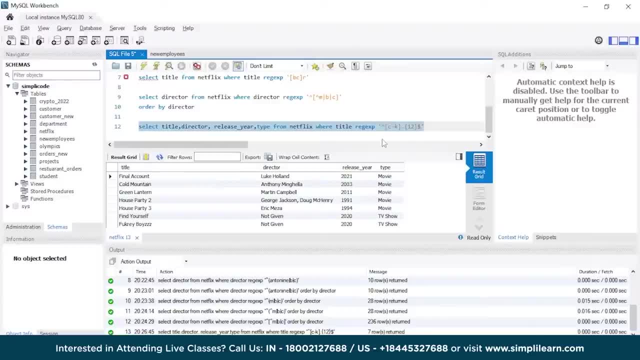 it has exactly 12 characters in it and it is also satisfying the condition within the range, that is, it is starting with the character f, which is lying in the range of c to k, and similarly all the others as well. So in this way, you can also mention the range in the pattern that you want to search for. 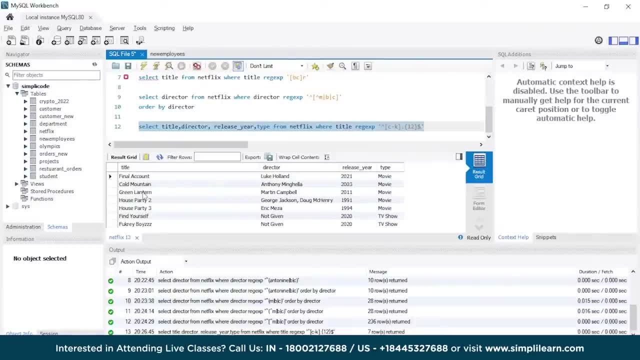 as well, and you can also use the numerical values. Now we don't have asset of numerical values to retrieve, so I'm not taking any examples, So I hope you understood this various scenario, guys. So that brings us to the end of today's session. that was all about. 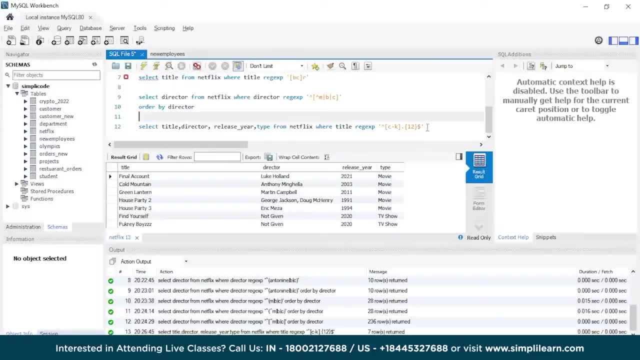 the SQL RegEx operator. Now the now as we know that the advantage of using a regular expression is that you're not limited to search for a string based on a fixed pattern with the percentage sign or an underscore. So the regular expression has more meta characters to construct. flexible as well as the complex. 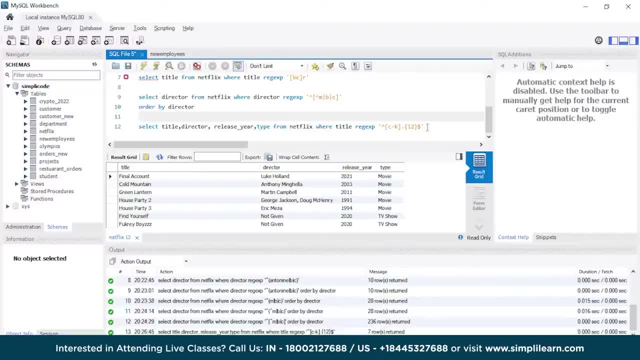 patterns. So that is the reason why we are using the SQL RegEx operation and coming to. the disadvantages of using regular expression is that it is quite, you know, difficult to understand and maintain a complicated pattern. So if you're an SQL beginner you might struggle with, you know. 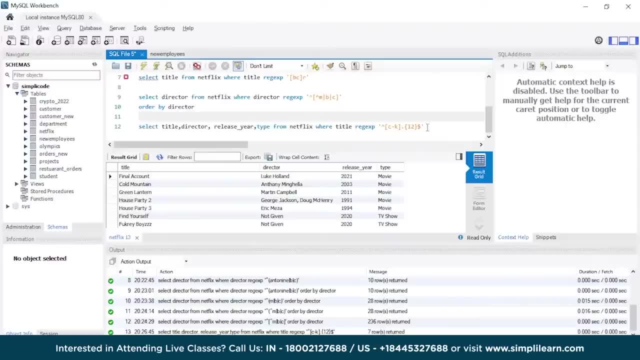 all these patterns. So with the question given you have to change the patterns accordingly. So if you're working on first time with this regular expression, so you might find it a bit difficult. So therefore you should describe the meaning of the regular expression in the comment of the SQL statement so that you can understand clearly. In addition, the speed of 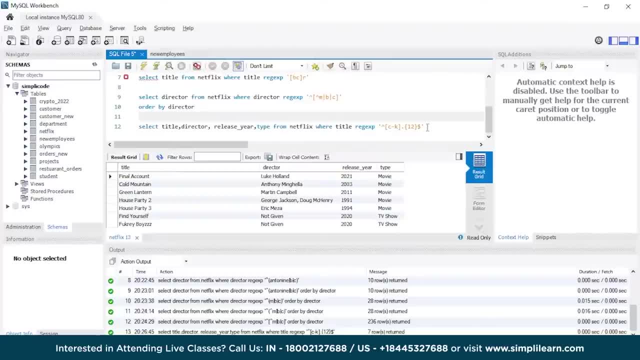 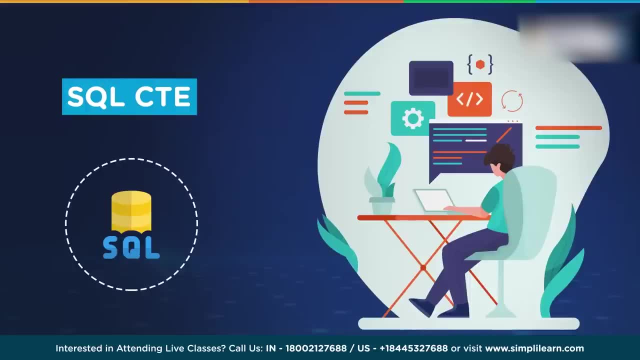 the data retrieval in some cases is also decreased. if you know, use complex pattern in regular expression. Now, as you all know, working on long queries with complex logic is common for any SQL developer, So this can include using various joins, various levels of aggregation, data aggregations and 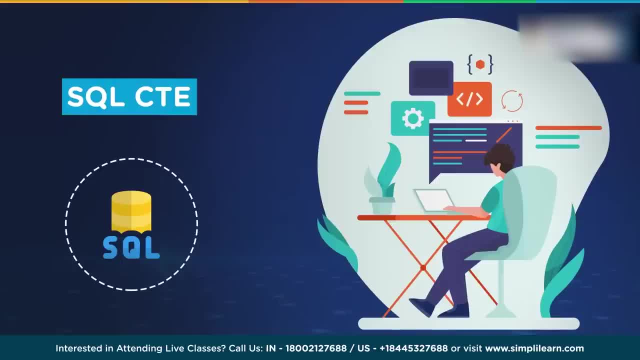 filtering across any number of tables. Now, in some cases, a result resultant set can be- cannot be obtained with a single query, using a select statement or using a where condition: It requires a series of queries to be put together. Now, furthermore, for complex queries, the best way. 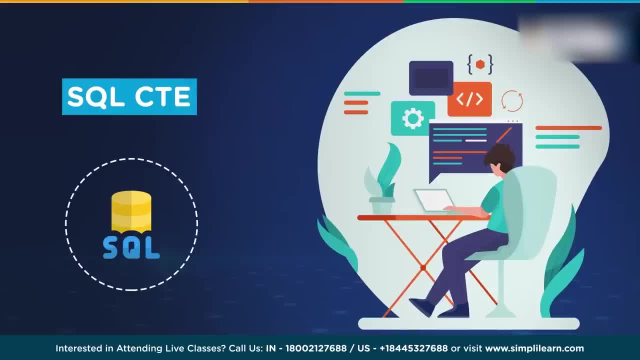 to write a query is to break it down into a logical steps and build it piece by piece. Now, sub queries are typically one way to consolidate functionality into a single SQL statement that can be later be incorporated back to the main query. Now this has the potential to be useful. 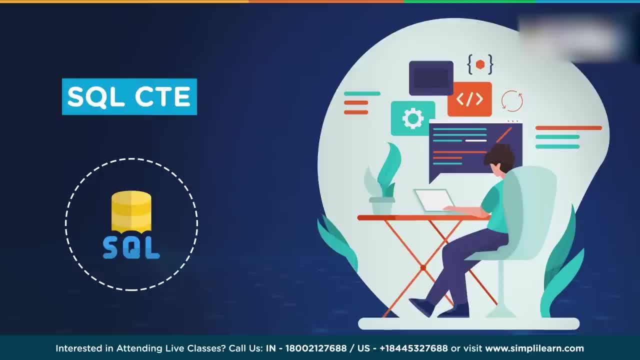 but it is also challenging for a beginner who has just started with you know a new level to read and comprehend and understand it well. So this is where and it is possible to simplify difficult queries into a sequence of logical steps using CTE or common table expression. 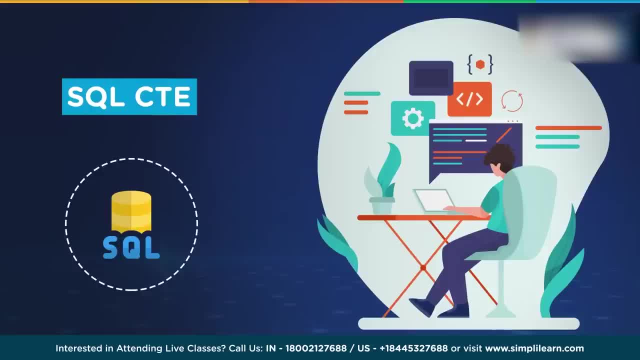 Which also helps to make your queries more readable and allow you to produce more complex resultant set. So in this session we'll be discussing all about common table expressions, or CTEs, in SQL, how they are used and implement them using certain examples in MySQL Workbench. 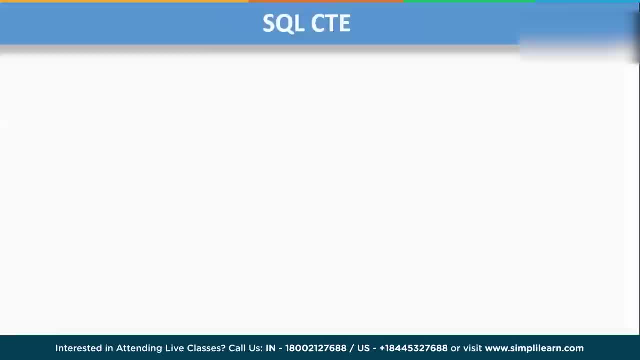 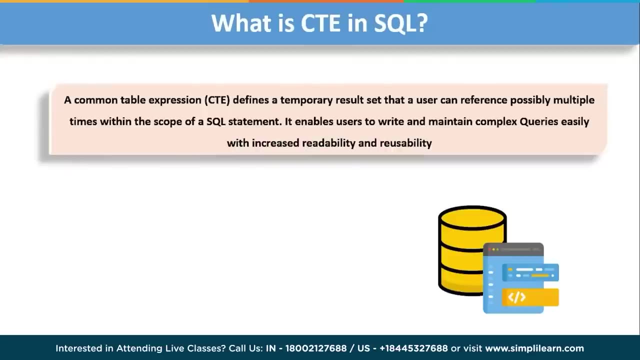 So, without any further ado, let's get started. So firstly, let us understand what is SQL CTE? Now, CTE stands for common table expressions and in SQL it is a temporary resultant set that has a range within a single SQL statement. Now a CTE can be referenced at any place within that statement multiple times. 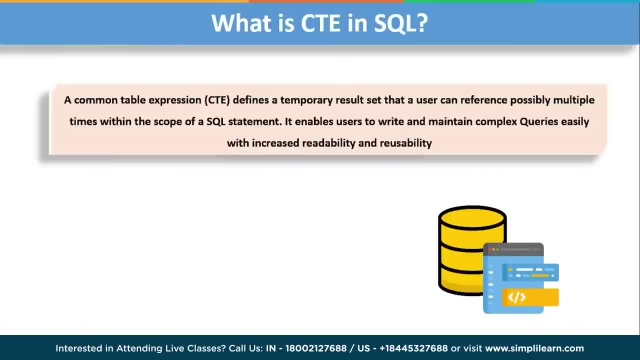 Now, generally, the with clause is used to define a CTE- A common table expression, do not exist as a separate statement. instead, it is always used along with a select insert, update or delete statement, which immediately follows the CTE. So it is generally used. 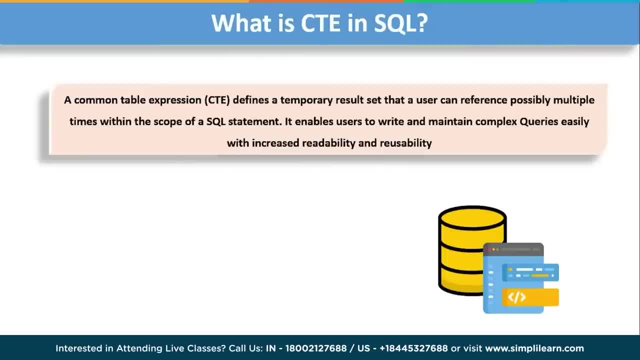 and it enables users to write and maintain complex queries easily, with increased readability and usability. So you can basically define multiple expressions within a single query So, once defined, these expressions can be referenced repeatedly throughout the rest of your queries. Now, common table expressions was relatively a new SQL feature which was lately introduced in 1999. 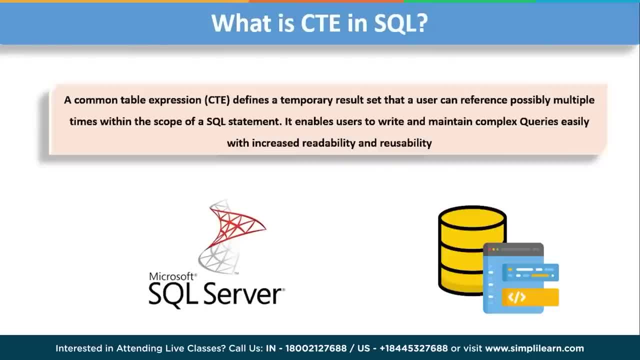 by Microsoft SQL Studio. Now, CTE was first introduced in SQL Server in the year 2005, and then PostgreSQL made them available, starting in 2009, and which was further used by MySQL, which which has waited a bit longer, and made them available in the year 2018, starting with the version of 8.0.. So again, simply put it together. 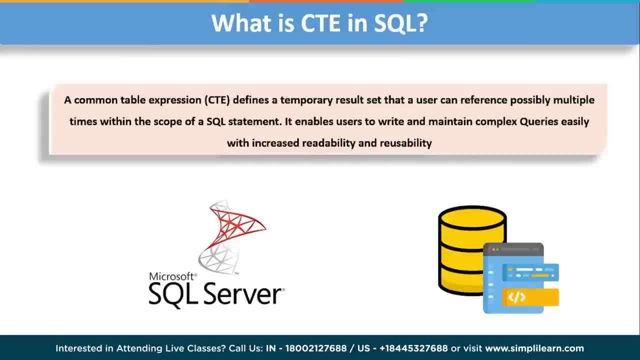 it is a temporary data set, guys, which returns, you know, a query which is then used by another query. So, in order to reduce the complexity of a query, we use CTE. So it is temporary because the result is not stored anywhere, so it exists only when the query is being run. So that is what CTE is all about. 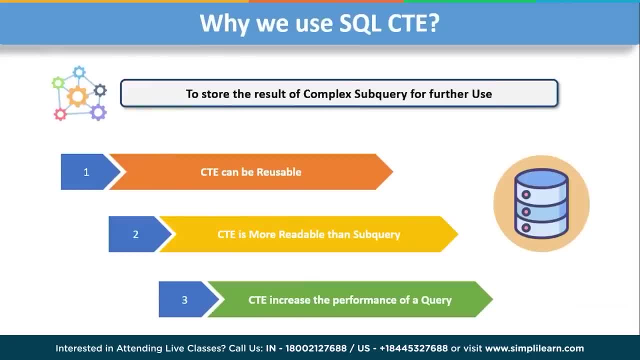 So let us now move ahead and let us understand why we use SQL CTE Now. the main reason is to start the result of a complex subquery for further use. Now in SQL, we will use subqueries to join the records or filter the records from a subquery. 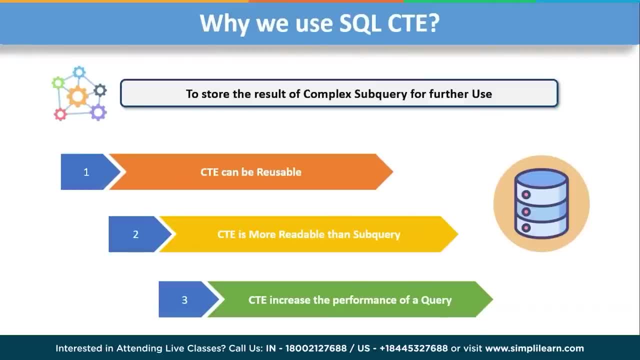 So whenever we refer the same data or join the same set of records using a subquery, the code maintainability will be difficult. So a CTE makes improved readability and maintenance easier for the user. And another reason being is CTE can be reusable guys. Now the reason why I am. 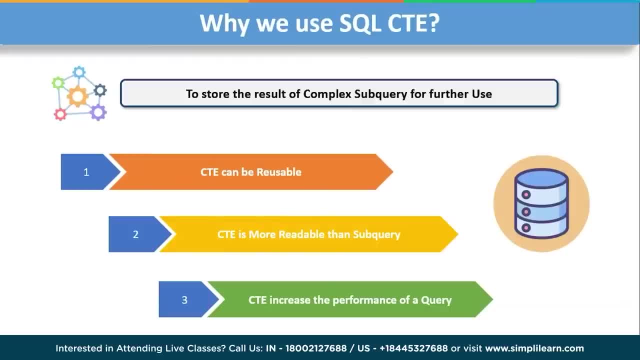 telling it is reusable means you know a CTE is reusable by design instead of having to declare the same subquery in every place you need to use it. So you can simply use a CTE to define a temporary table once, then refer to it whenever you need it. 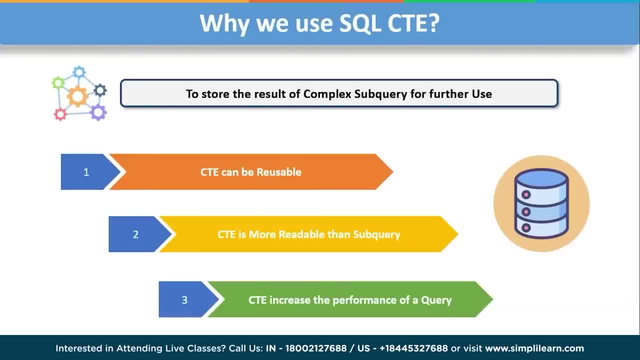 So you can call upon the specified CTE whenever you want in your query. Also, CTE is more readable than a subquery. Now, another reason why we use CTE is they are more readable than subquery. Since CTE can be reusable, you can write less code using CTE than using 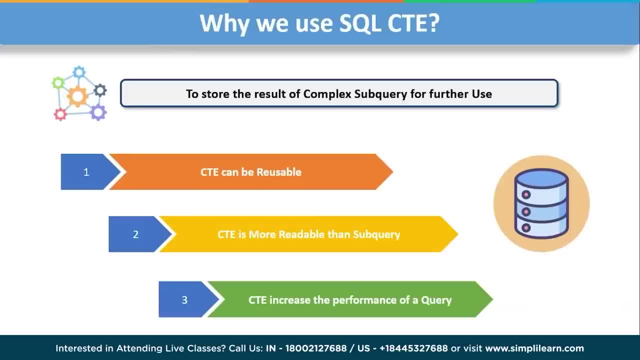 subquery. Also, people tend to follow the logic that we put behind CTE in an easier way than in a nested query fashion. So whenever you write a query, it is easier to break down a complex query into smaller pieces using CTE. And finally, CTE increases the 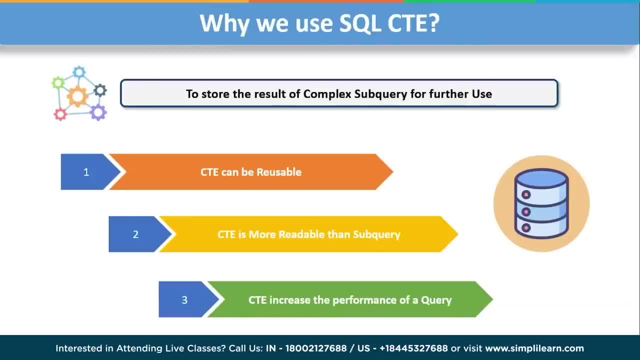 performance of a query. Now, if you are working on a complex data, performance is paramount, right? So, using subqueries, using multiple joins and joining various tables put together, can you know increase can decrease the performance of a query. Now, CTE can be defined in various scenarios, like in procedures, views, triggers and many more, So it can be used. 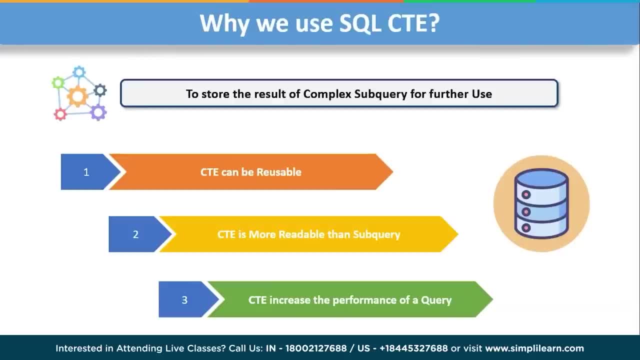 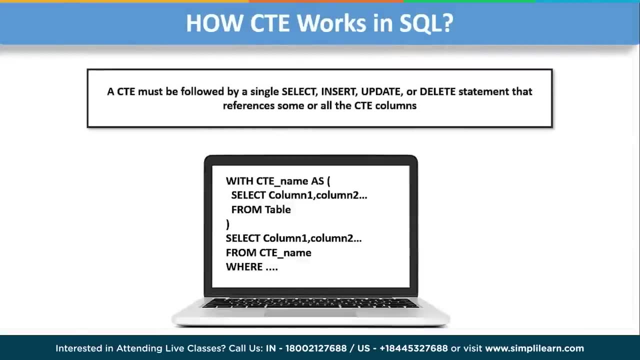 recursively with a subquery, not, which can ultimately increase the performance of a query. All right, let us now understand how CTE works. Now, a CTE must be followed by a single select, insert, update or a delete statement that references some or all the CTE columns. 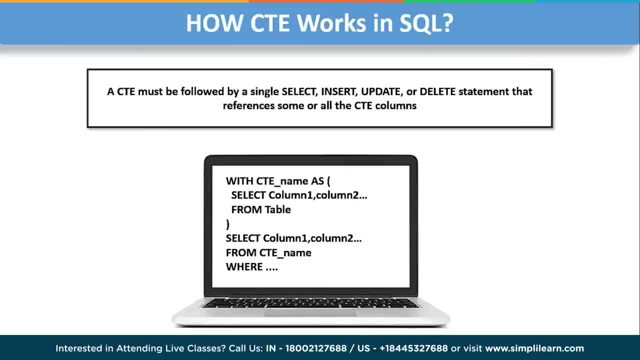 So let us now understand the syntax. So let us now understand the syntax of common table expression. The syntax is followed as with: is the keyword we use: CTE name. Now you can specify the name of your choice for the CTE as, and within the parenthesis, mention the select statement with all the columns you want to. 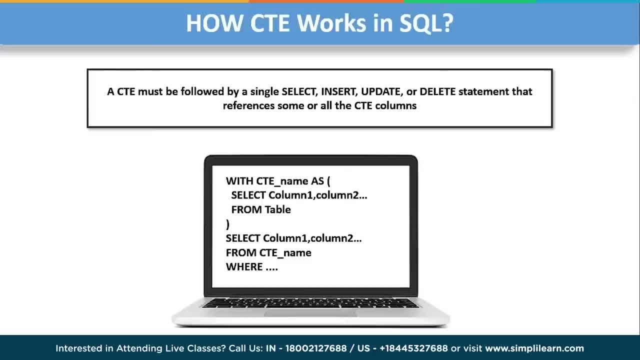 get in your resultant table and from the table name And close the parenthesis and after that we'll be basically again selecting the columns from the CTE name instead of the table and you can specify the where condition as per your requirement. I hope you understood the syntax and how CTE works. 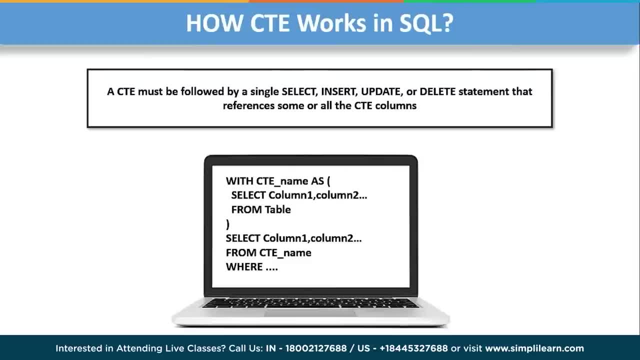 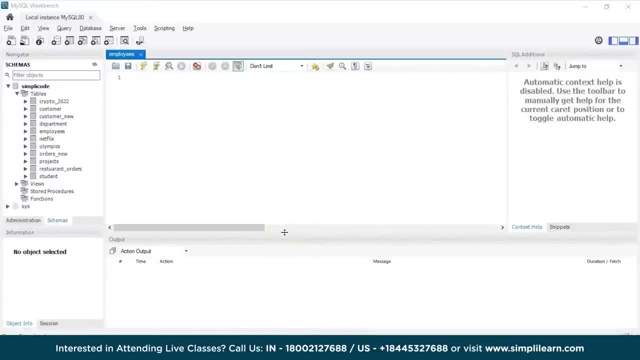 Now it will be clear when we get into the execution part. So let us directly jump into MySQL Workbench for execution. All right, as you can see, MySQL Workbench has started and let us now run some queries using CTE. So let us just take an example for that. Let us consider the employee table. 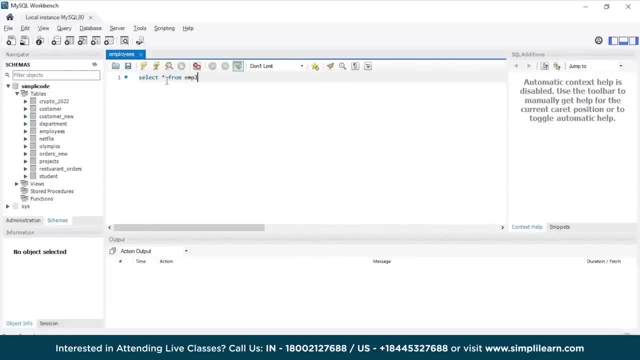 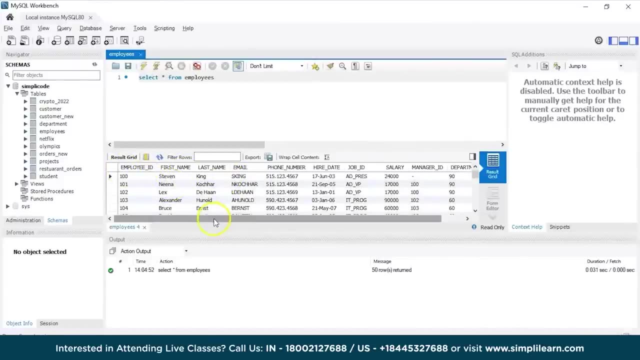 for understanding how CTE works, So let me just display the value from the employees table. All right, so the employees table has various attributes, such as employee id, first name, last name, email phone number, hiring date, job id, salary manager id and their department id. 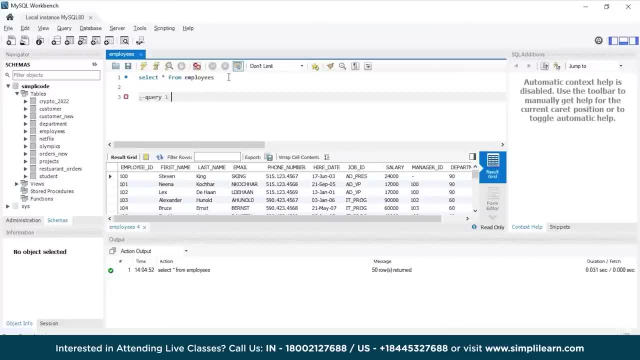 So let us now run a first query wherein we'll find the highest salary of an employee working in different departments, or you can say each department. So in that case we'll use a CTE here and, as we discussed earlier, in the syntax it starts with the with keyword and after that you: 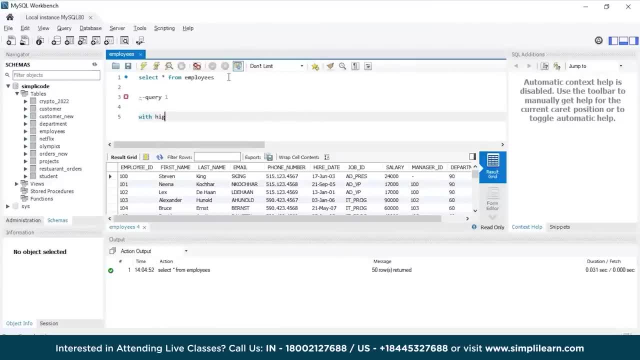 can give the CTE name as per your choice. So let us give it as highest salary, since we're finding the highest salary of employees in different departments. So highest salary. and after that use the as keyword and within the parenthesis, use the select statement and display. 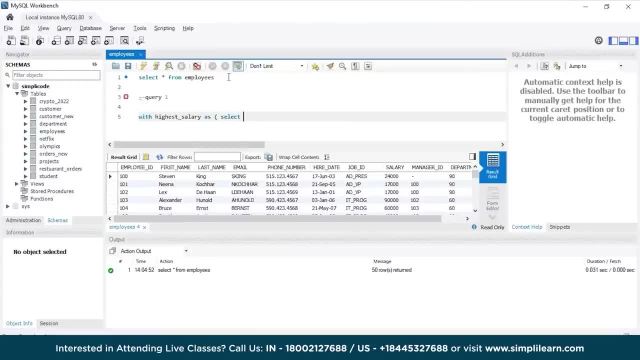 all the records that you want to fetch in a resultant table, So select. I want my first name of the employee. last name, comma department id comma salary: Now, since we are finding the highest salary of each employee from different departments, we'll be using the rank over function. Now we have discussed about the rank over function. 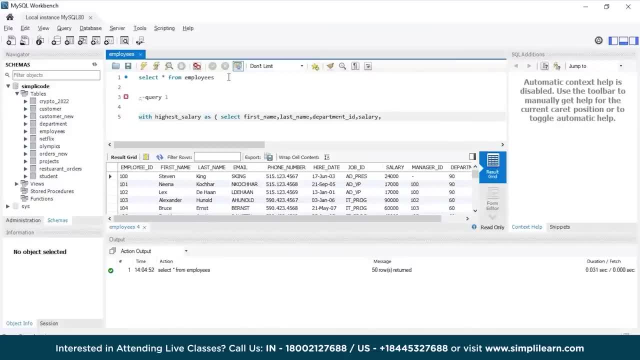 in how in our previous video, which is how to find the nth highest salary. So if you want to know it in a more detailed way, make sure you check that out. So I'm using a rank over function and which is followed by the partition keyword, which is partition by. 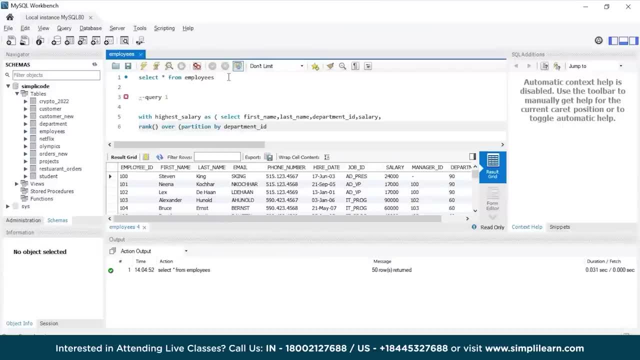 we are partitioning based on the department id here, order by salary, and we'll use the descending keyword here because we we are only concerned with the highest salary, so it will be basically from highest to the lowest point. So close the parenthesis and you need to give a temporary name for the. 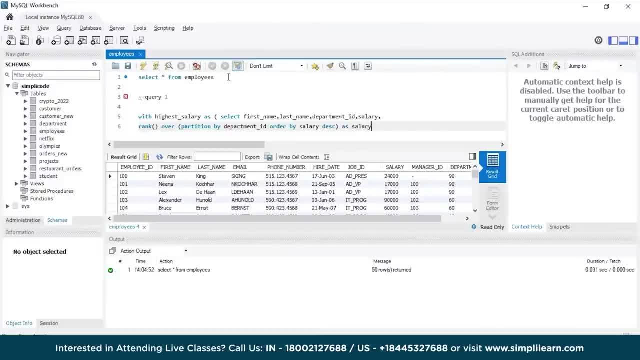 rank over function. so let us just, let's say, give it as salary rank from employee table: employees table right, all right. and after that we have to mention the select statement again, where we'll display all the columns that we have mentioned in our CTE again. 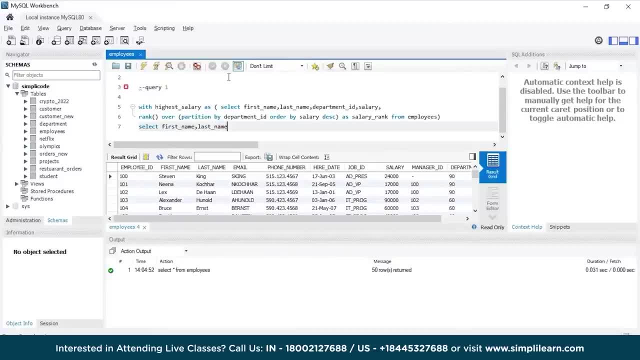 So let me just mention the first name. last name, salary department id. from now we have to mention the CTE that we have chosen here. now. highest salary is basically the name of our CTE, so I'll mention the highest salary here instead of the table name. 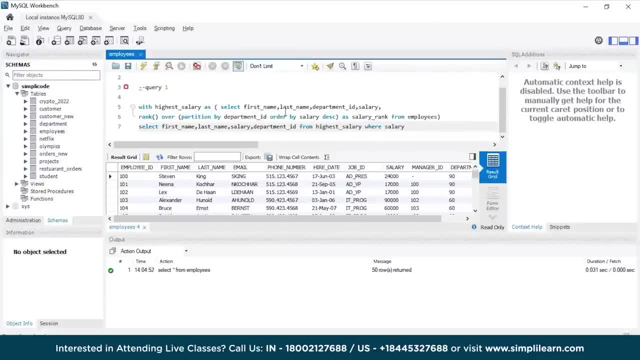 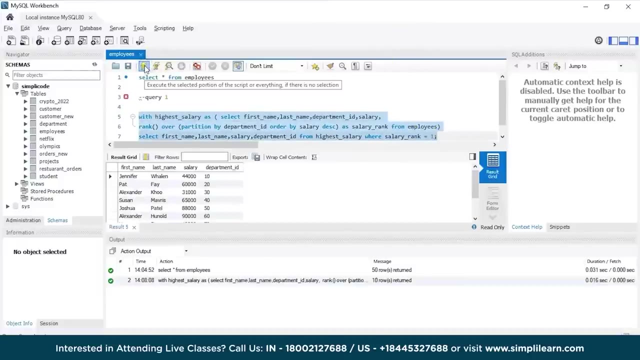 where salary, salary rank, is equals to one. now, why I am choosing one is it will segregate all the salaries and it will only choose the highest salary from that. so, all right, I think we can. we are good to go, so let us just execute the statement, then we'll see the output. all right, as you can see, 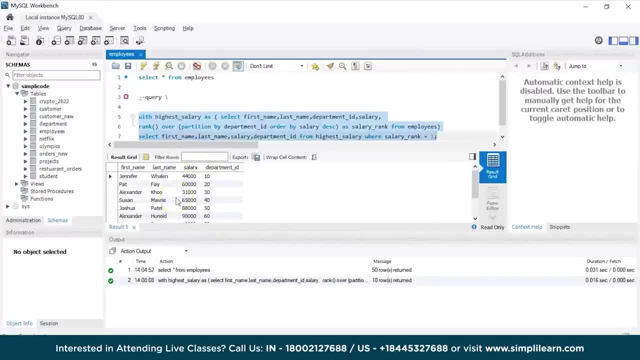 in a resultant set. it is displaying all the data of the employees. that is, their first name, last name and their highest salary. that is, the employees working in different departments. So let me just explain how the query is working here now. the CTE is named here as highest salary. 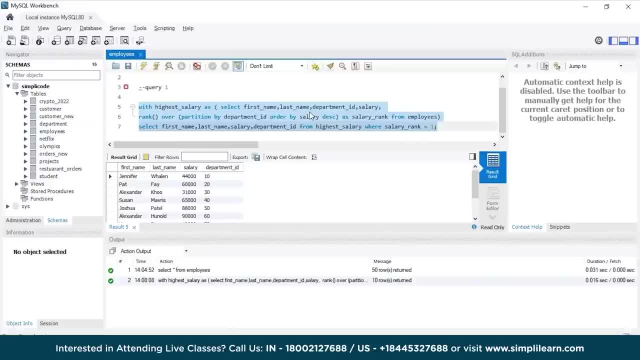 we use it to rank employees within each department by salary by using the window function rank over. now we partition that data by the column which is department id. this means we rank the salaries only within each department, not across all the table. right, so the data is sorted according to. 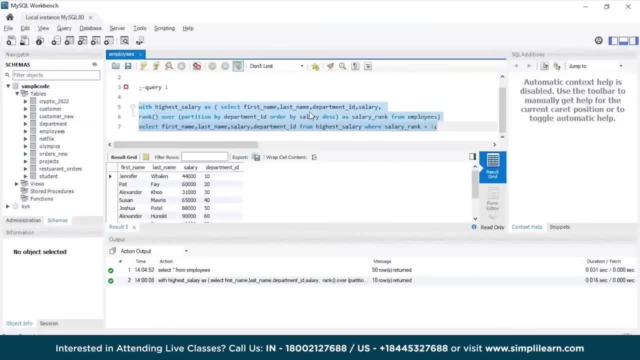 the column salary and the department id is the highest salary so we can rank employees within each department. So we want the highest salary in descending order because we want the highest salary, as I said earlier, in the department, to have the highest rank, which is one. also. we also have selected several 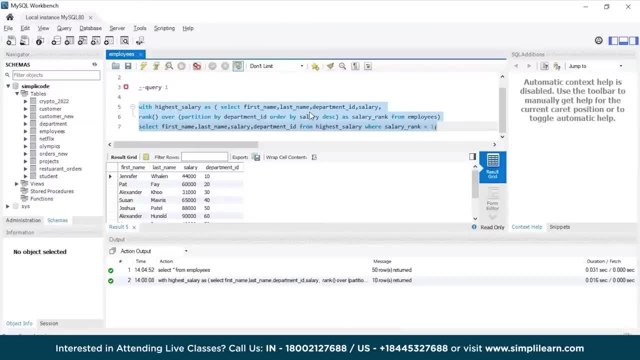 columns from the table employees in the same CTE and we need data from the CTE in the next select statement in order to fetch in our resultant set. and in the select statement we are basically selecting the columns needed to have in a resultant set, that is the first name, last name, salary and 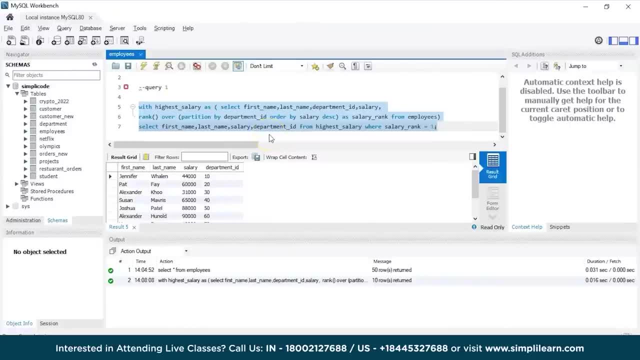 id. so in this way you can use the CTE to find the highest salary of each employee from different departments. now I know you might be wondered. you know why CTE is being used, where you can simply write a sub query to find the highest salary. now I get it. I'll explain it in a bit where we'll 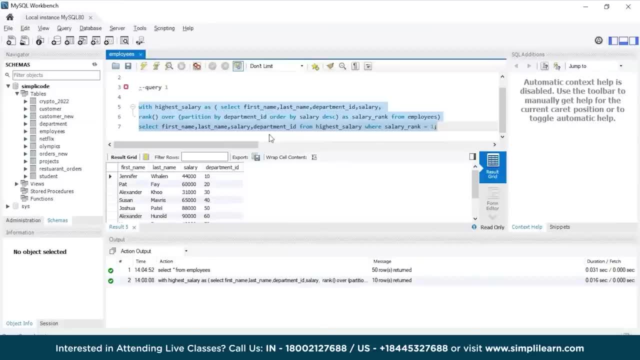 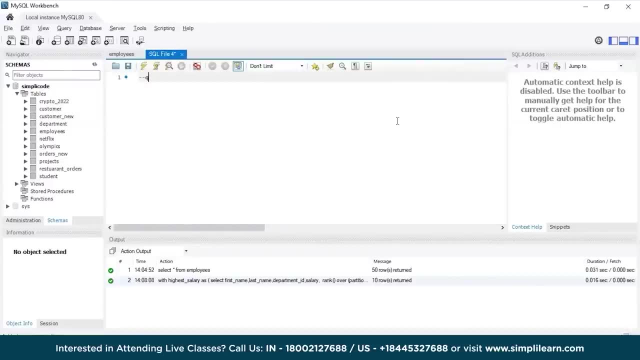 discuss in in the end why we are using CTE here. so let us just again take another example here, guys, so that we can have a clear-cut idea On more how the CTE can work. so in the second query we will be basically finding the: 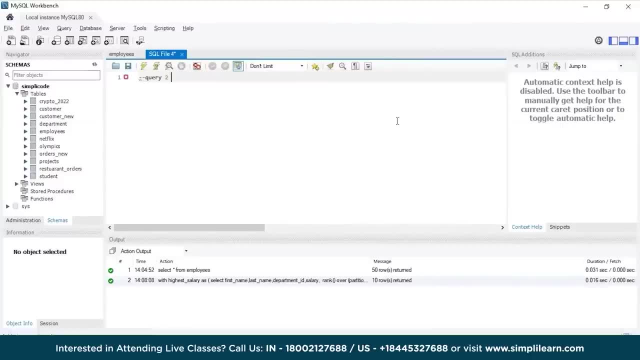 average salary of each employee working in different employee. now, previously we have found the highest salary of the employee. In this case we'll be using the. we'll be finding the average salary by each department of the employee, so let us just write the query here first. 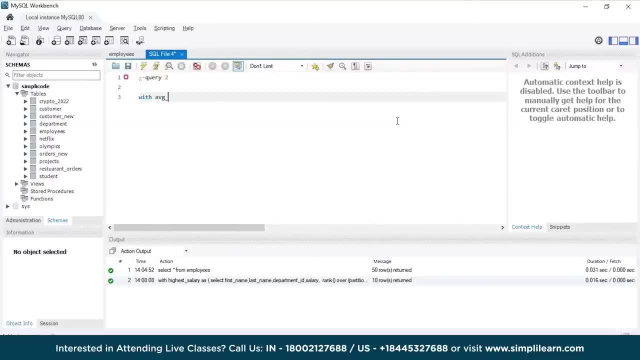 so again, I'm taking with- so let us name our ct name as average salary here, since we are finding the average salary, and within the parenthesis mention all the column names and the operation that you are performing. so since we are performing the average operation on the salary, i'm taking as average salary. 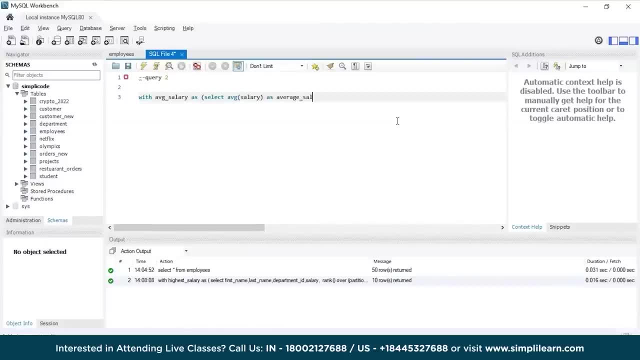 as i am taking it as average salary. just give it a alias name and then we are mentioning the department id from the table, that is, employees, and we'll be basically grouping all the details of the employees by their department id so that we can have the average salary in. 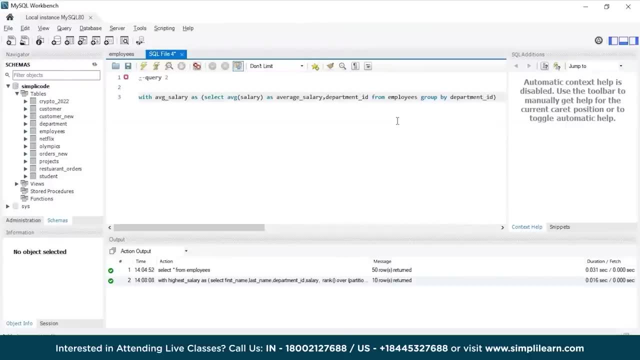 each department. so close the parenthesis. now, again, we have to mention the select statement, which is the outer statement after the ct. so we are going to mention the outer statement after the ct. so we are going to mention the outer statement after the ct. Now select: first name, last name, department ID, salary from employee table- employees table right. 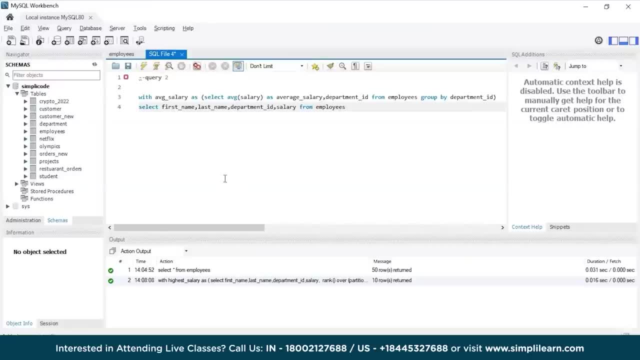 Now, basically, the criteria, which is to find the average salary, is basically we have to join the two tables, which is basically the same table, that is, employees, and we'll be comparing the salary of employees from these two tables simultaneously. right, So we have to join these two tables, that is, the CTE table and the employees table here. So that is the reason I'll be joining the table now. 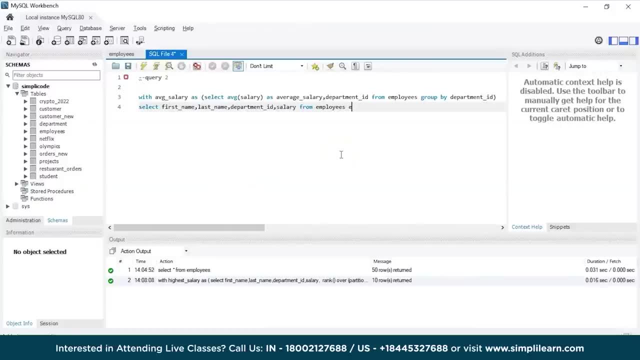 So let me just take the employees table alias name as E so that we can find it easily. So Efirst name I'm taking Elast name, Edepartment ID and Esalary from employees E and basically I'll be joining this with the CTE. that is average salary that we have taken, all right. 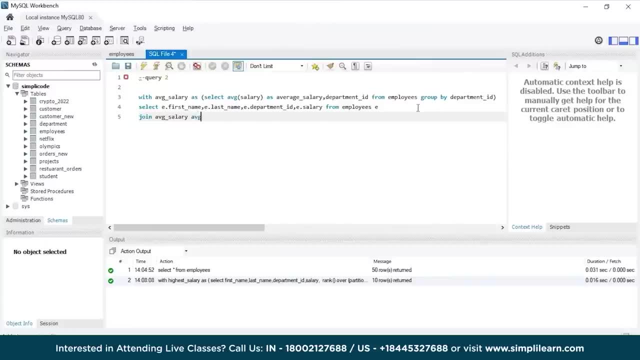 So I hope you have understood this till now. So let us just give a name to this. Let's say AVC, AVG, and we are joining the table based on the department ID from both these reference tables, right? So I'm taking, Edepartment ID is equals to AVG, which is the name of our CTE table. that is the temporary table which we have taken. 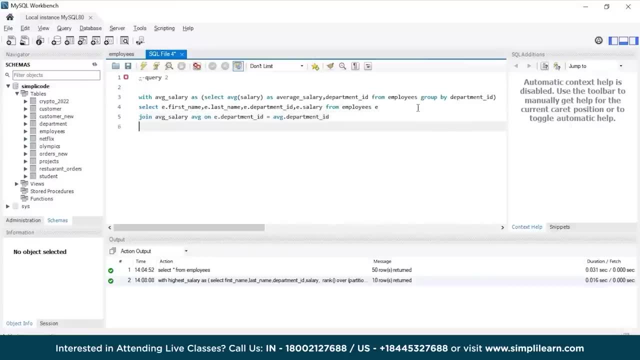 So department ID and we'll order. Then we use the order by statement So that will have a more clear resultant set order by department ID and we are good to go. So let us just execute this statement and we'll see the output. 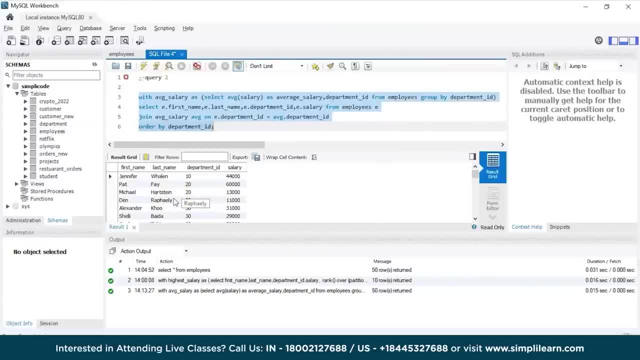 All right. as you can see, in our resultant table it is displaying all the average salaries of the employees, So let us just quickly go through the explanation. So this query is using a CTE named average salary. guys calculate the average salary in each department. Now the select statement in the CTE groups: the 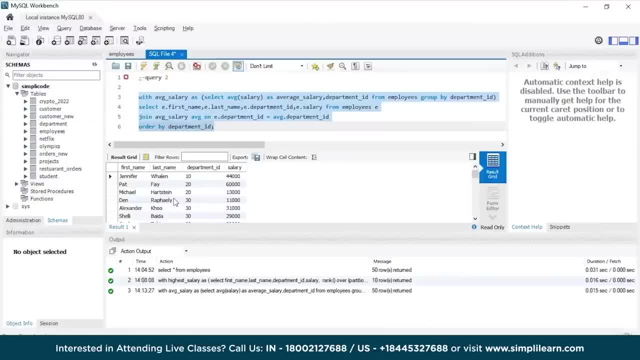 rows by department and uses the average aggregate function to calculate the average for each department. Now, once we have that, we combine it with other columns from the table employees- to complete the resultant answer. Now, to do so, we are basically joining the employees with the CTE. 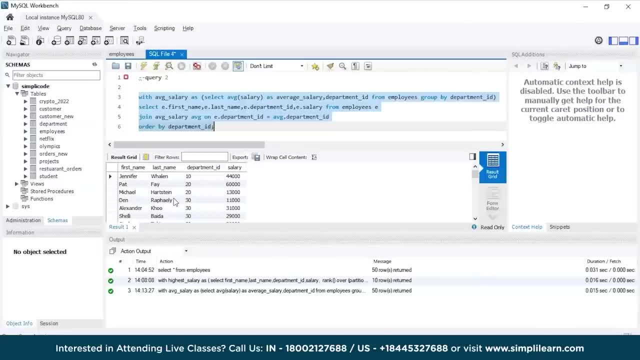 name, as we would do with any two tables, to join them. So we select the columns, the required columns as we have taken here, which is the first name, last name, department and salary from the employee table and the column average salary from the CTE. So in this way you can use the CTE to 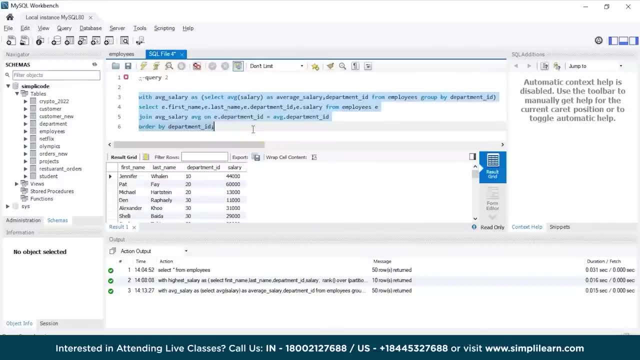 find the average salary in each department of different employees. So there's a little error, guys. I forgot to mention the average salary column. so I was just wondering why we didn't have the average salary. So let us just mention that now. average dot, average salary which we have taken earlier. all right, so 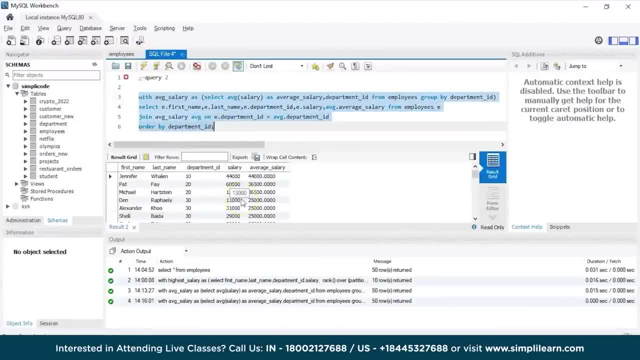 let us execute the statement. All right now you can see the salary of the employees working in different departments and also the average salary of that particular department. Now, if you look at the department 10 now, the salary is 44,000 and the average salary is 44,000.. So let us just mention. 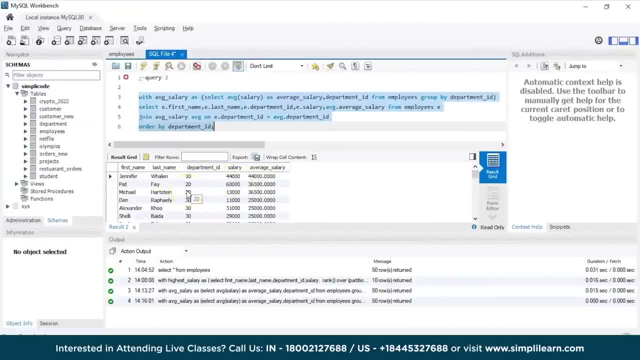 that the average salary is also 44,000.. Now, if you look at the department ID, which is 20, now we have two different employees, Pat Frey and Michael Hatchton, whose salaries are different, that is, 60,000 and 13,000, but the average salary in that department is 36,500, and similarly you can see for the rest of 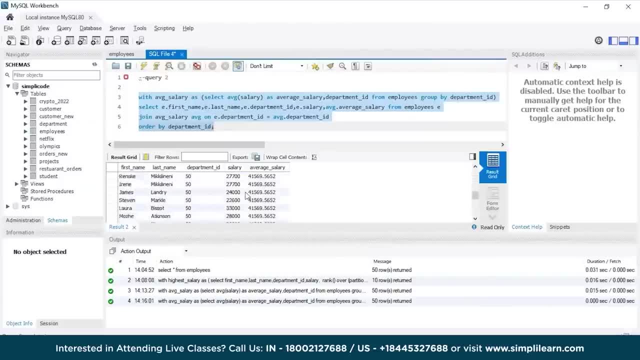 the different departments as well. So I hope this is clear. Now it brings us to the main question that why are we using and when we are using? you know CTE Now. traditionally, you've probably noticed that CTEs are a lot like subqueries. Maybe you're. 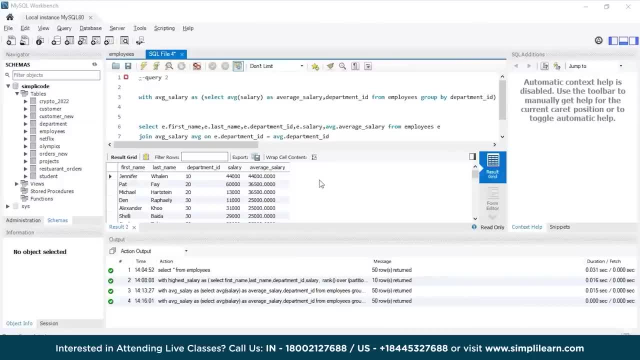 wondering why I'm using CTEs when everything I did could have been done with a simple subquery. you know That's true. aside from being more readable, CTEs have one big advantage of subqueries, that is, the resultant set or the results from a CTE can be used more than once in a query. So 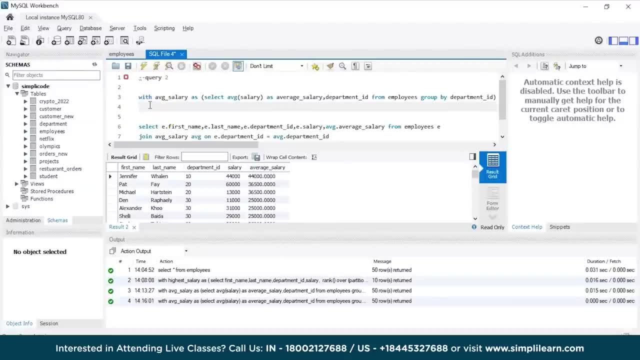 let's say if you're working on a complex database where you have to join multiple tables from the database and you have to perform various operations, So in that case you have to keep on writing the subqueries. Now let's say, if I want to find the maximum of average salary from the 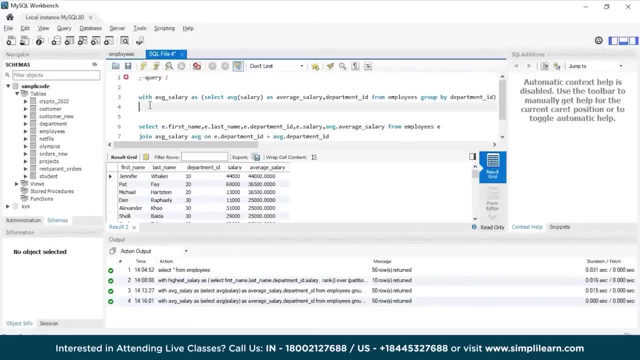 employees table. So in that case, now that I've created a CTE, I can directly write a select statement which says select max and inside that I'll be writing the average salary Which is the name of the CTE. from the CTE name, that is, we have taken as AVG underscore salary. 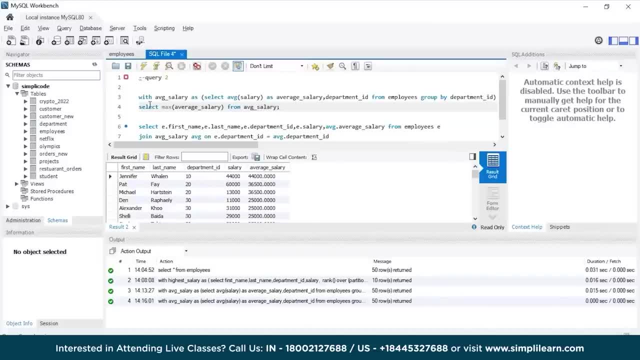 So now, instead of calculating the average salary of each employee from different department using subqueries- which is a whole, complete, whole process- right, it takes a bit of time. So instead of that, I'm writing a simple CTE for that, and later I'm using the same to calculate the maximum average. 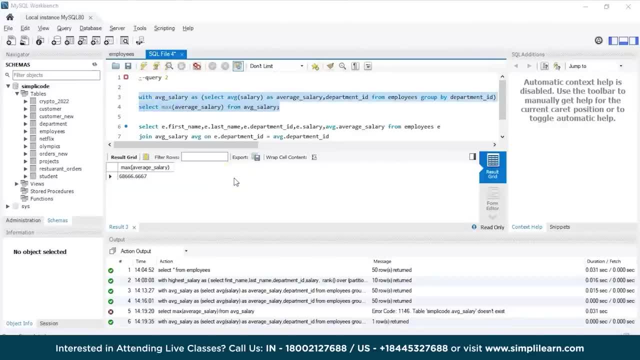 salary. So when I execute this, it will directly give me the average salary. So I'm going to display the maximum of average salary of all the employees in a different department. So it becomes quite easier, you know, instead of writing subqueries each and every time. Now, if the code with the 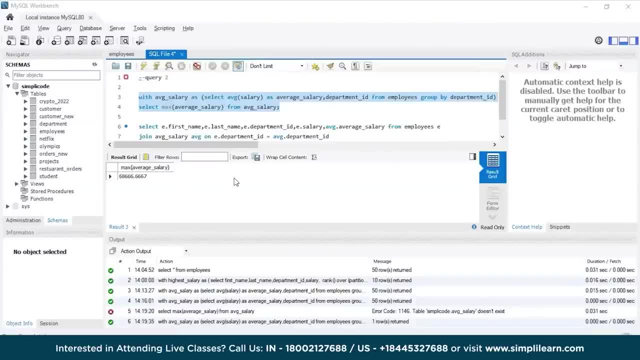 subquery is less readable and it is harder to understand the code with a CTE in simple way, right. So you would be trying really hard just to understand what every part of the code does when you're writing subqueries. Now, having difficulties understanding a code can be. 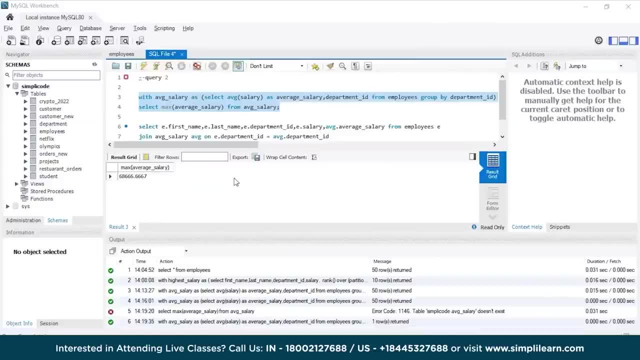 frustrating. So that is where CTE is going to help you. So let's say, if I want to write a subquery of one of my subquery first, Then CTEs can help you guys, It is one of the most powerful tools to. 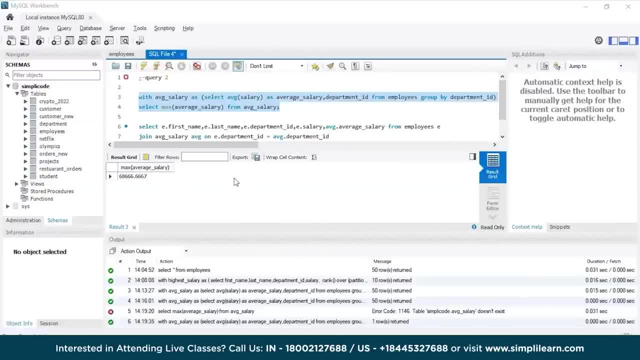 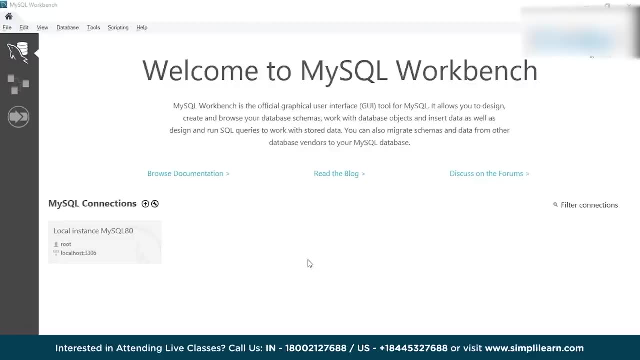 process hierarchical, complex data into a simple manner where you can use it multiple times. So that brings us to the end of today's session. guys, that was all about CTEs and SQL. I hope you, as you all know, learning how to answer the SQL interview questions is a powerful skill which can 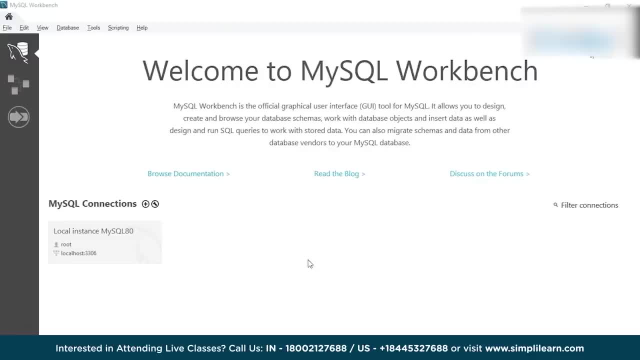 make the difference between getting hired for the job or not- And nowadays the competition for one job is quite high- are applying for the same position. so if you want to get hired, you cannot afford for not being prepared to present yourself as the best fit candidate for. 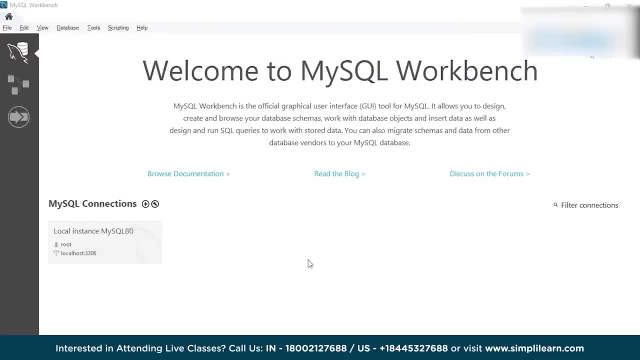 that particular job role. so, in order to answer the interview questions, one of the main area where you can prepare the best is especially when it comes to the most common SQL interview questions, because these questions are asked during all the interview, all the job interview questions, right? so in this session we will be discussing some SQL queries. 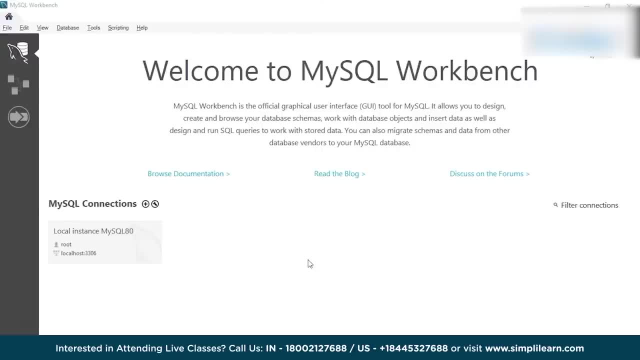 where you can practice them and which will also help you during your interviews as well. more on that soon, but before we get started, if you are new to the channel and haven't subscribed already, consider getting subscribed to our channel. simply quote to stay updated with all the latest technologies and hit. 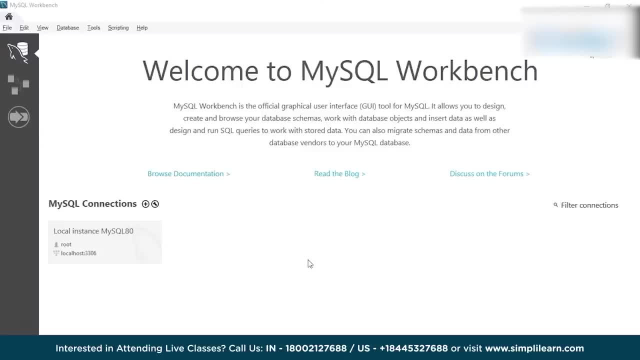 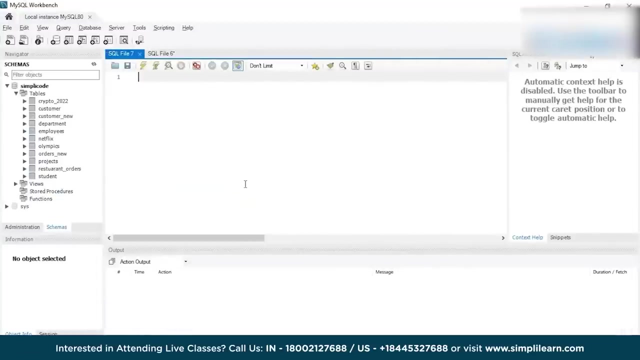 that bell icon to never miss an update from us. so, without any further ado, let's get started. so let us jump into MySQL workbench in order to execute this top 5 3k SQL queries. so let's get started. all right, as you can see, MySQL workbench has started. so firstly, let us look at 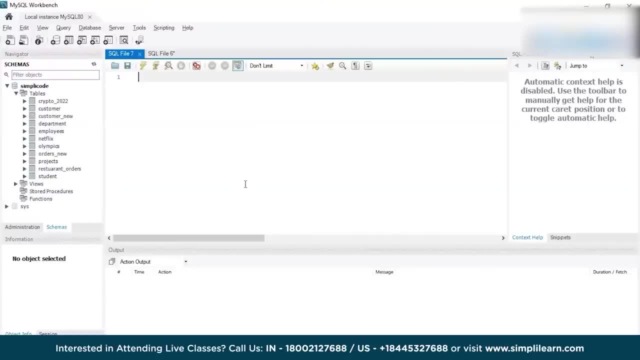 some of the key things that you need to keep in mind while you know preparing or answering the interview questions. now the general questions will revolve around key concepts, like you know, asking the different type of commands in SQL, different constraints, indexes, views, joins, different functions and etc. and at the same time, not just this theoretical and the you. 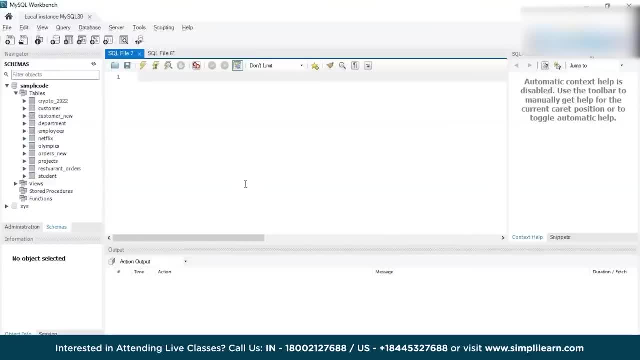 know scenario based questions rather than the objective questions wherein you can be asked to write a query. you know a proper SQL query wherein the interviewer wants to test your knowledge in deep. you know whether you are understanding the SQL queries or not. now this level of interview questions also entirely depend. 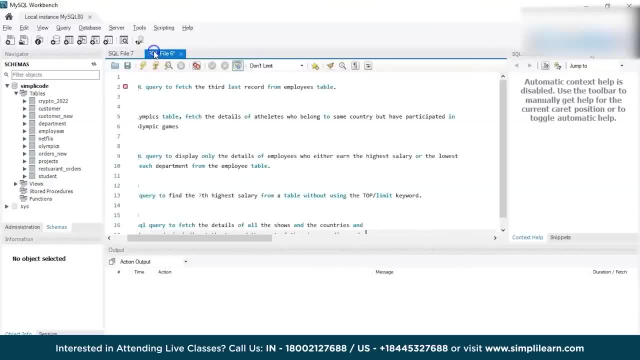 on the position that you are applying. so, keeping in mind, I have already created five SQL questions that you might find tricky, so this might be useful for a beginner as well, which is the difficulty of the queries is from, you know, from beginner level to moderate level so you can easily answer this queries. but there 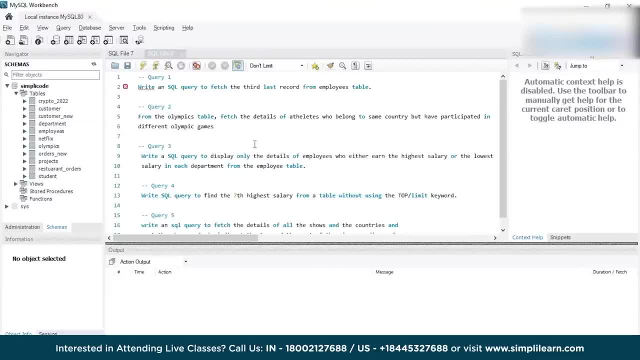 is a bit of, you know, a tricky part in them as well, which we'll discuss as the session progresses. so before answering the queries, you have to be thorough with all the concepts of SQL. so we have a dedicated playlist on SQL wherein we have covered various topics on topics. 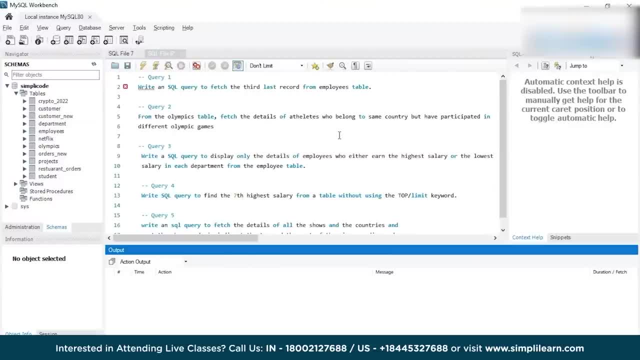 and concepts regarding SQL, so make sure you check that out before you know you start perform the queries. so let us discuss the queries one by one. so the first query is write an SQL query to fetch the third last record from employees table. so let me just open this new tab. 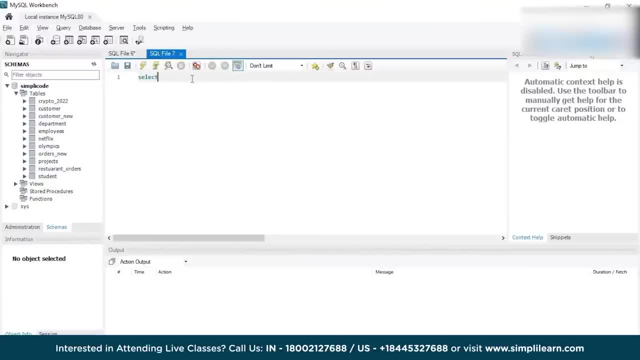 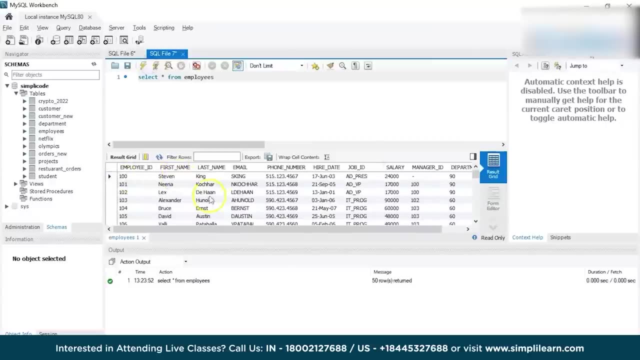 all right, let us know. first display the records from the employee table, that is, select star from employees. so, as you can see, the employee table has various columns, such as you know: employee ID, first name, last name, email phone number, hiring date, job ID, salary manager ID and department ID. so the 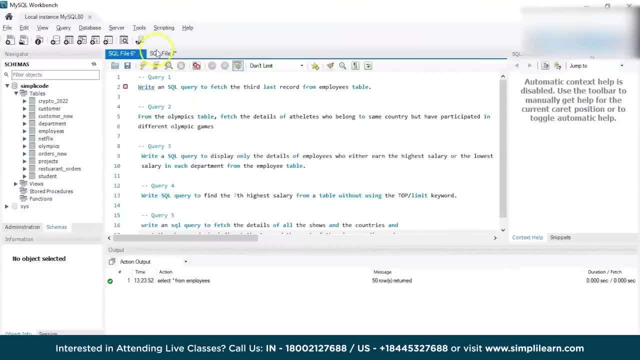 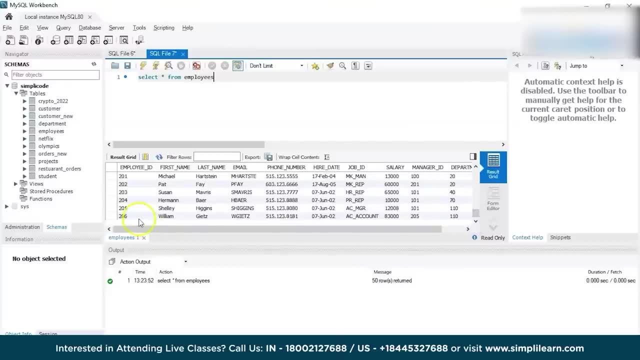 queries. that was asked is write an SQL query to fetch the third last record from this employee table. so if you scroll down a bit and you can see, the last record is William and the third last record is Herman Bayer. so basically we need to get the record of this employee who's having employee ideas, 204, whose 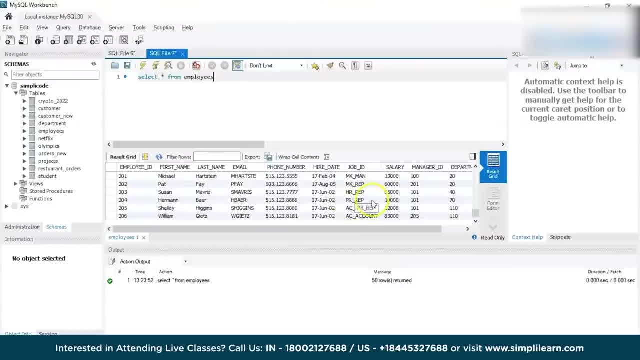 name is Herman Bayer and he works as a PR or some PR, as a specialist on PR, so right. so basically you can solve this. you know in different ways. so basically the logical approach is using any window function, which we'll be discussing now, and sort the data. 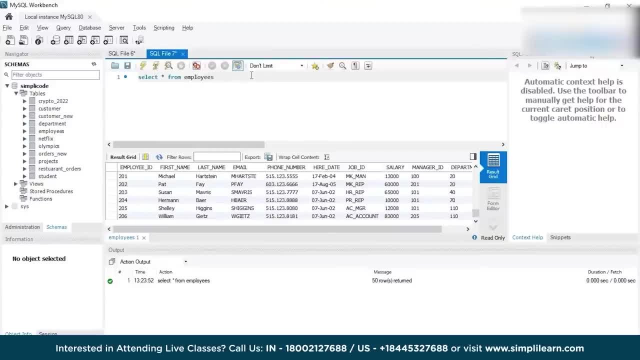 sending order, you know based on the employee ID, and then provide a row number to each of the record and fetch the record having row number as three. I know it is a bit of confusing so let us just directly write the query first so you guys can have a clear-cut understanding. select mention. 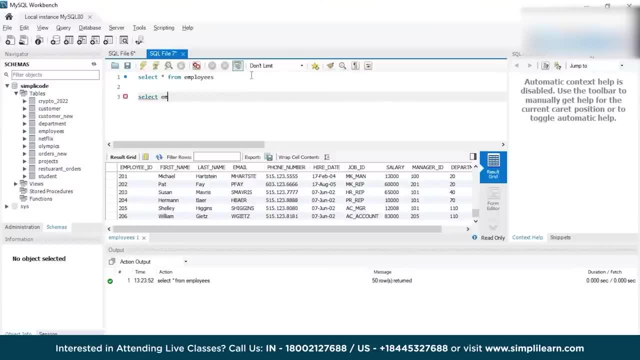 the all the rows you want in your resultant table. so I am taking employee ID, their first name, their last name, department ID as well, salary from now. we have to write a subquery in this wherein we'll use a select operator: select star comma. now we have to use a window function here. now the 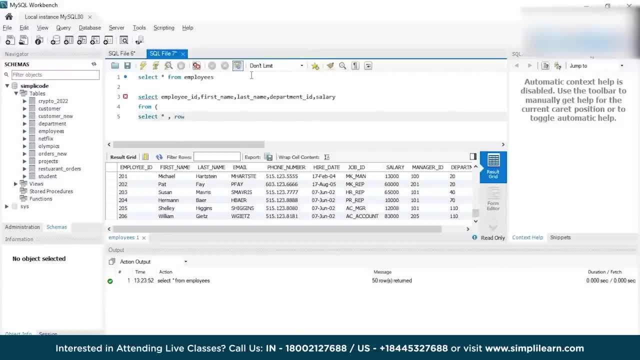 window function which I'm going to use here is row number function. so the row number function is basically- uh, you know, SQL ranking function that assigns a sequential ranking number to each new record in a partition. now, when the SQL row number function detects two identical values in the same position, it will assign different rank numbers to both. so the 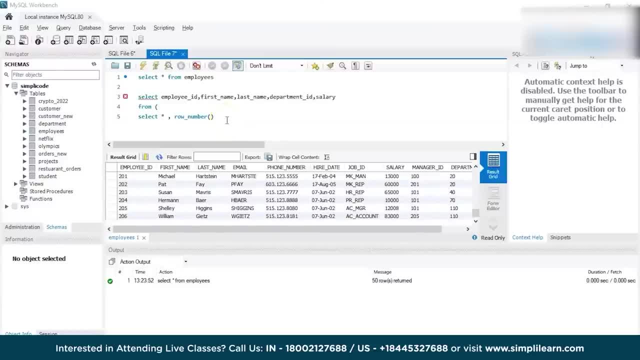 logic behind is that we'll be assigning row number to each of the records, based on the employee ID, and then we'll find the third, last, you know record from this table. all right, so row number, and I'll be using the over, which is the syntax, and we'll order. we'll sort the data in descending order, so order. 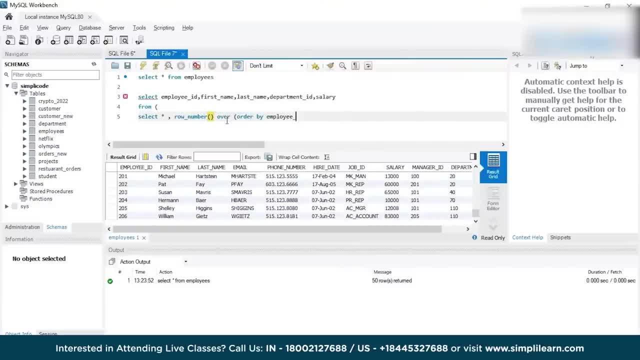 by employee ID in descending order from the employee table, that is, employees, where you have to mention the row number as well, so row number. so let us take the row number here as row number. this is basically a sub table, right? so you need to mention the row number as well where row number is equals to. 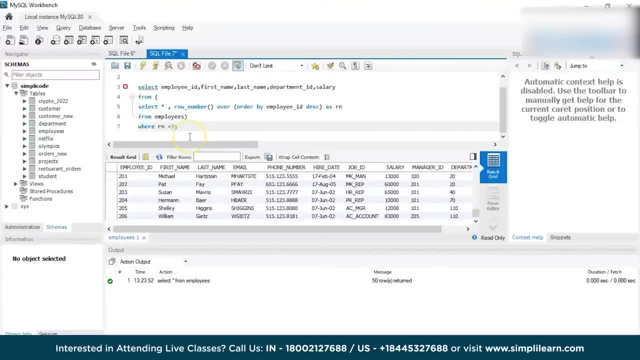 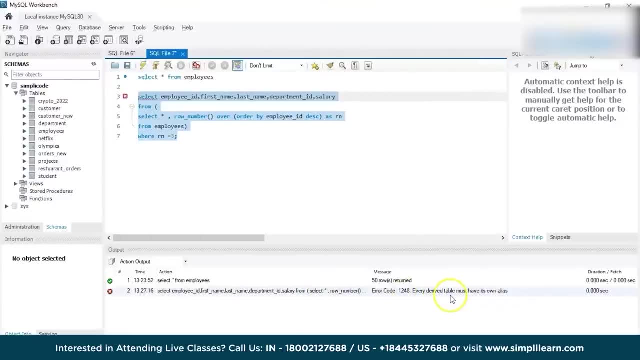 three, since we are finding the third, last record from a table. so let us execute this and we'll see the output. so there is an error which says every derived table must have its own alias, so I think we forgot to mention the alias name for the table. 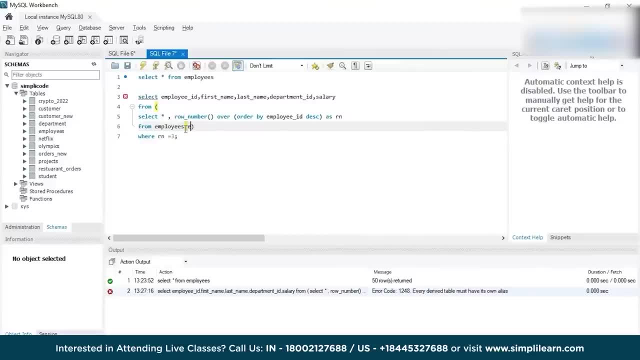 so during theannée last recording we have looking at the table here. so let us take the alias name as employees E here and let us take it as X, so it will basically be X dot Rn. so I think it is correct now. so as you can, 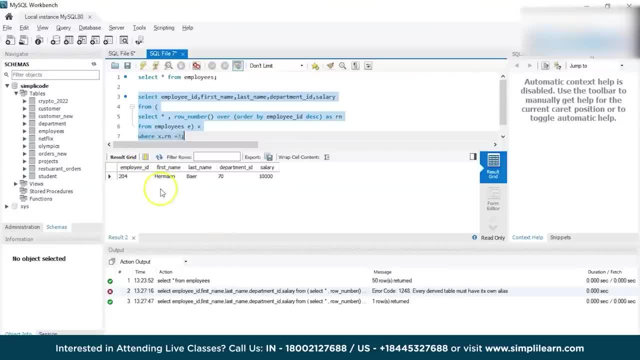 see in our resulting set we have got the resultant table which is of hermann's by a record, hermann, just by a record. then the resultant table is represented from the list and this table over here, dedi, whose employee id is 204, just as we discussed previously, which is the third last record in 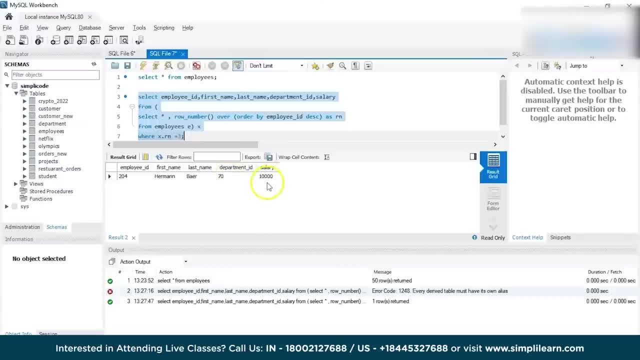 the table who belongs to department id 70 and his salary is ten thousand dollars. so in this way you can simply use the window function row number to find the third last record from the table. so similarly, you might be asked to find the you know second last or fifth last in different. 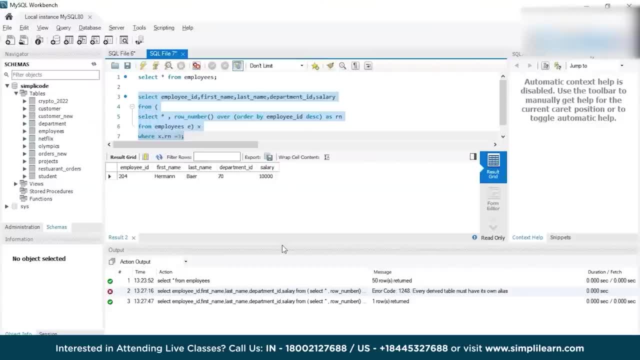 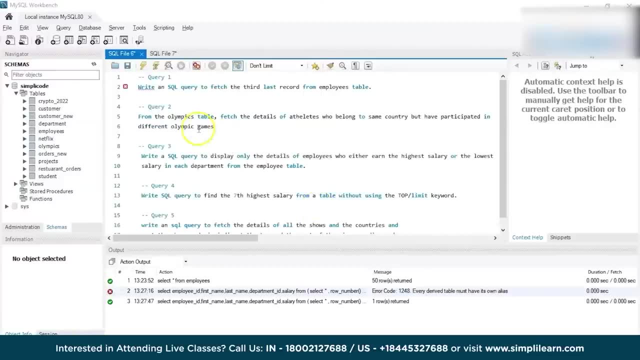 contexts, so the scenario might be different, but the order and the approach to solve this query is the same. all right, moving ahead, let us now discuss the second query. now, the secondary states that from the Olympics table, fetch the details of all athletes who belong to the same country but have 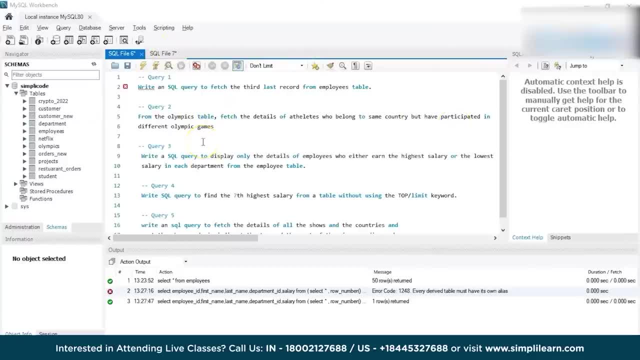 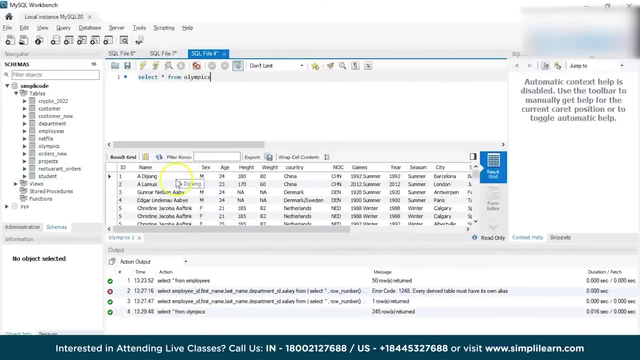 participated in different Olympic Games. alright, so let me just open another tab. so firstly, let us retrieve the details from the Olympics table, which is select star from Olympics. so the Olympic table, which is select star from Olympics, so the Olympic table, which is select star from Olympics, has various attributes like ID name, sex, age, height, weight, country, NOC games, year, season, city, sports and 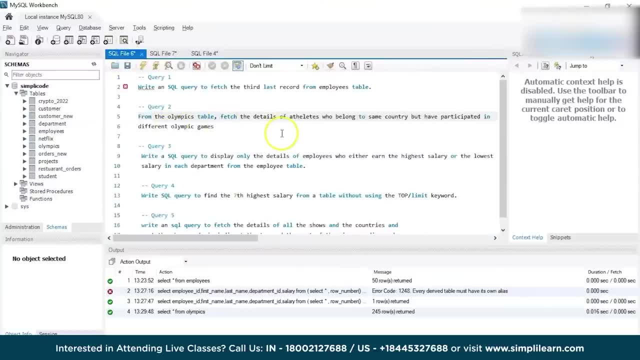 even so, what the query states is: from the Olympics table fetch the details of all the athletes. so we are concerned with these column, which is name, which is the details of all the athletes who belong to the same country but have participated in different Olympic Games. now, in the resultant 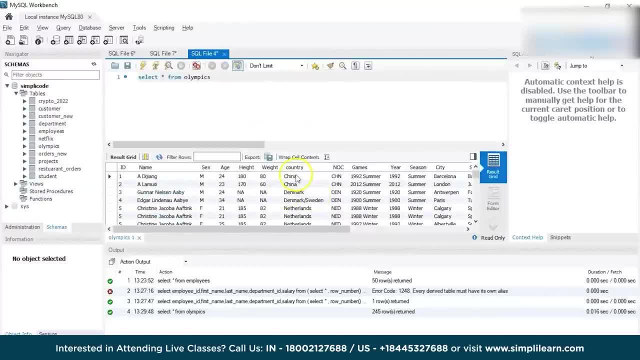 set. we need to have the resultant table which has the details of all the athletes who have who are from the same country but have participated in different Olympic Games here, like the 1992 summer, uh, 2012 summer. so basically they have to be from the same country but different games. now, the logical approach, uh, to write this query is: 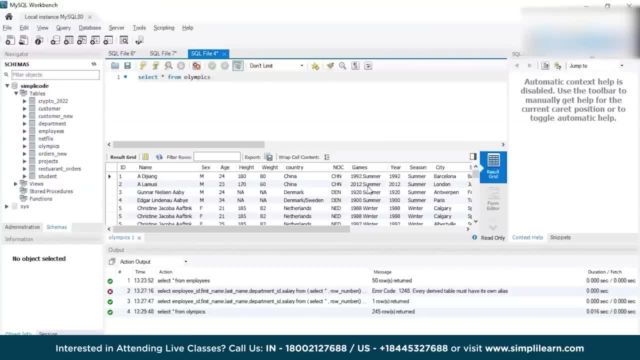 basically, by using the self join to solve this problem, which is, uh, used to join a table to itself to compare the values within the same table. all right, so let us discuss the query now. so again, though, in order to solve this query, you have to be- uh thoroughly you know, knowing the 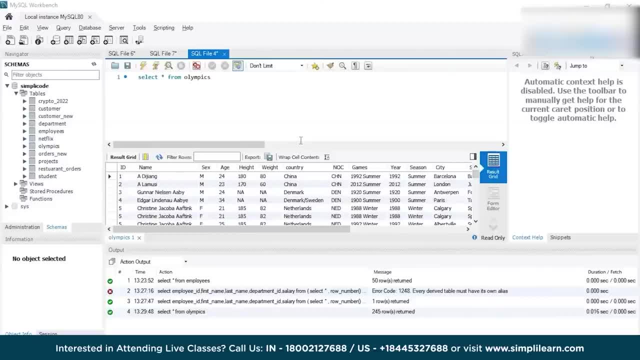 joints concept. so we also have a dedicated video on that as well, where you've discussed the various different kinds of joints, so make sure you check that out as well. so let me just write the query: select. now. there might be, uh, you know, multiple- uh, you know- athletes participating in same or 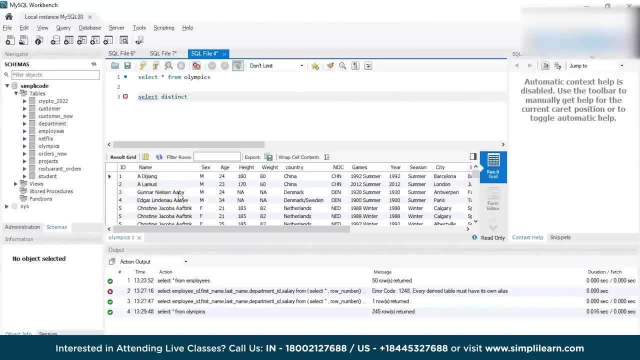 different games, right, so I'll be using distant clauses here, distinct, and since we are joining the two tables, we need to have a temporary name for two different tables. so the for the first table I am taking it as D1 dot name, which is the athletes uh details. next, I am taking D1 dot country comma. D1 dot- games from Olympics. 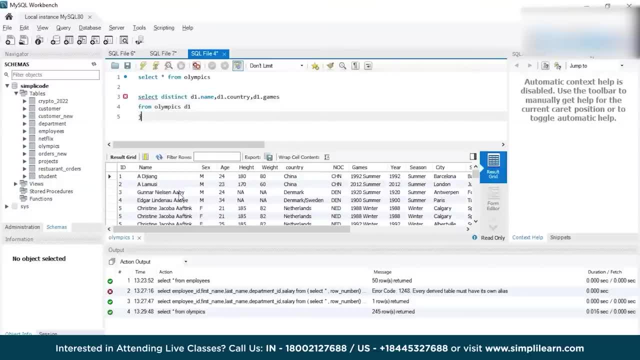 which is the first table, D1, and then I'll use the join keyword, which will basically self join the same table, which is Olympics again, but we have to mention a different temporary name, which will be D2 here. I hope you are understanding this. on: D1 dot country equals to D2 dot country. 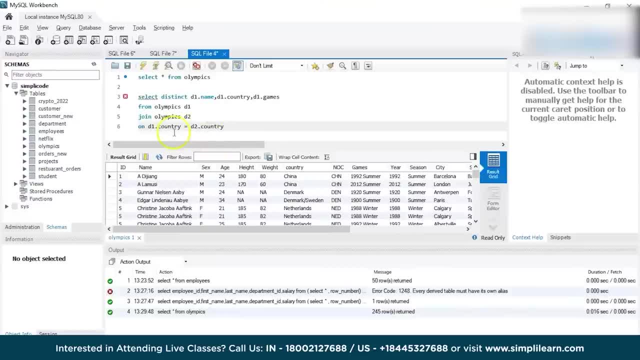 so the condition that I'm specifying here. specifying here is that we need to have these in country here, that is, the athletes participating in different Olympic games should be from the same country. but he should be, it should have, he should have played different Olympic games. so in that sense, I'm using another condition, which is and operator where D1 games. 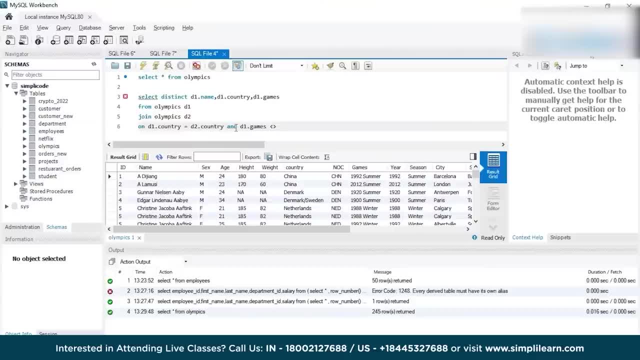 I'm using not equals to operator here, which will compare two operators if they are same or not. if they are not same, it will retrieve all the values. so D2 dot games and I'll similarly use an order by message so we can have in uh sorted order, which is order by name as well as, let's say, a country as well. 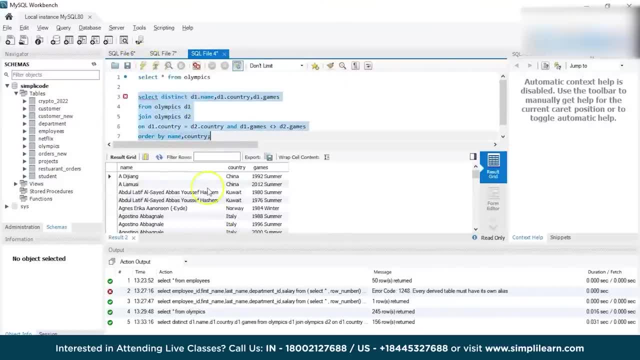 all right. so let us now execute the statement and we'll see the output. all right, we have the resultant set. uh, as you can see, in a resultant set, we have the details of athletics who have participated in various different games but belong to the same country. now, if you look at uh, a djang, who's belong to China, has participated in 1992 summer games, whereas a lamusi, who home part of mahfaye on 2016, said negated two length of ». 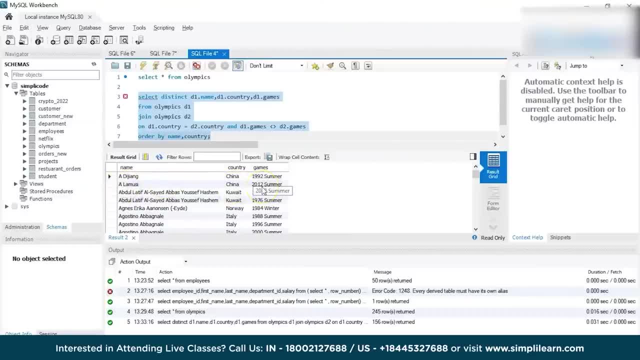 who is from the same country again, China, but has participated in 2012 Summer Games. Now, similarly, we have this Abdul Latif. It's a big name. Let us just take another one. We have Augustino Abangel. 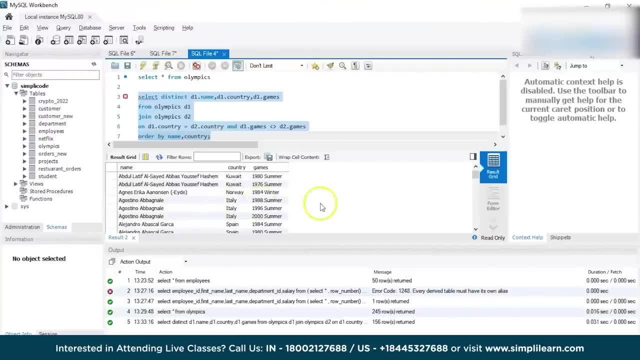 who's from the country, Italy, who has participated in 1988 Summer Games. Similarly, we have, you know, Alejandro Abascal Garza, who's from Spain, who has participated in various different games ranging from 1984,, 1980, and 1976 Summer Games. 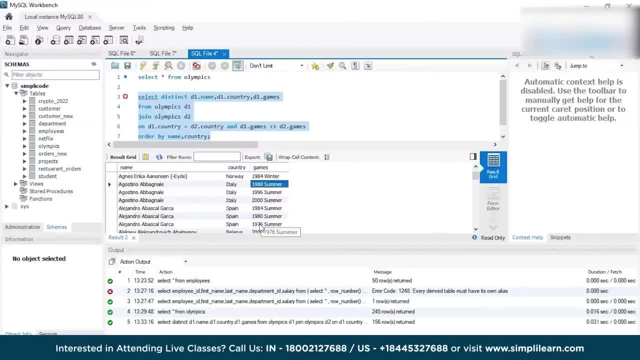 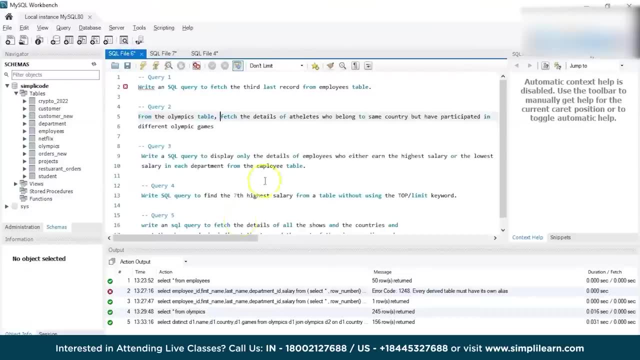 So in this way, you can find the details of all the athletes who's from the same country but have participated in different games. Alright, let us now move on to the next query, which is write a SQL query to display only the details of employees. 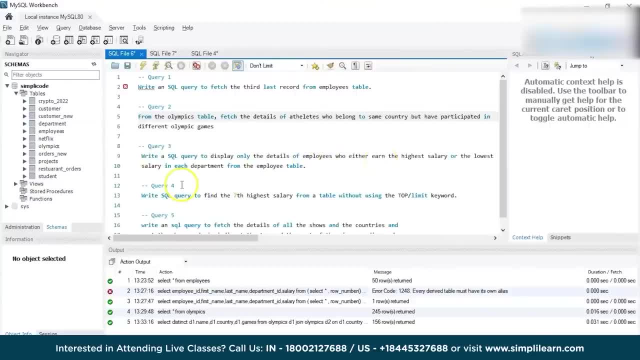 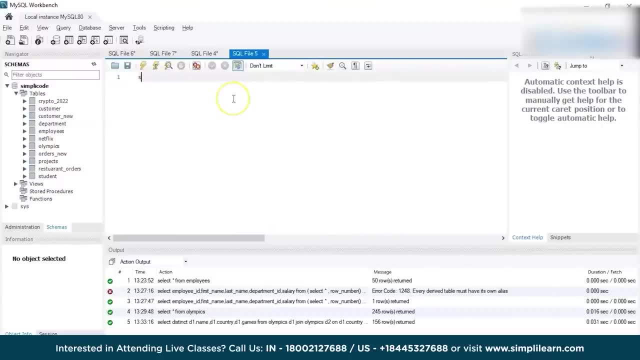 who either earn the highest salary or the lowest salary in each department from the employee table. Alright, so let me just open another tab and we'll retrieve the details from the employee table again. So we'll start from Employees. Alright, we have the Employees table. 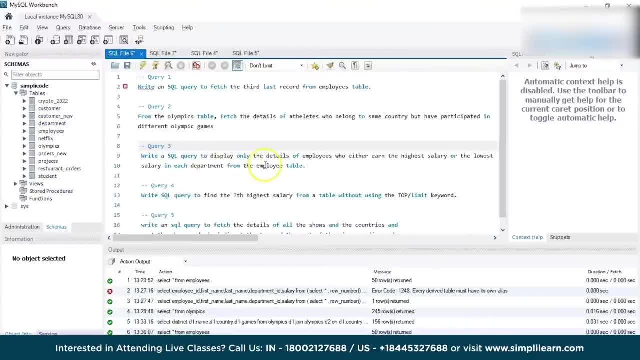 So the question, let us go through the question again, which says: write an SQL query to display only the details of employees who either earn the highest salary or the lowest salary in each department from the employee table. So we need to provide in the resultant set: 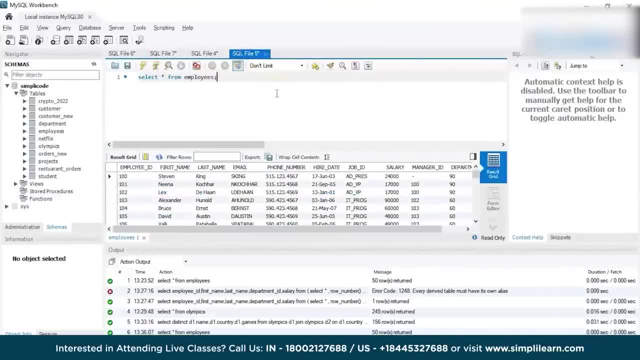 the details of all those employees who are either having the highest salary or the lowest salary from each department. Now the logical approach to this question can be is like we can write a sub-query which will partition the data based on each department ID. 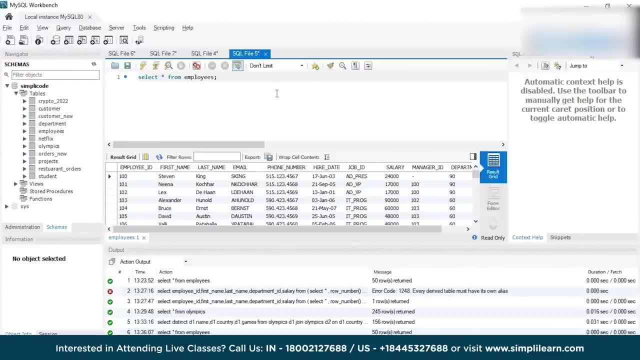 and then identify the record with the maximum and the minimum salary for each of the partition department. And you know you can. finally, from the main query you can fetch only the data which matches the maximum and the minimum salary returned from the sub-query. 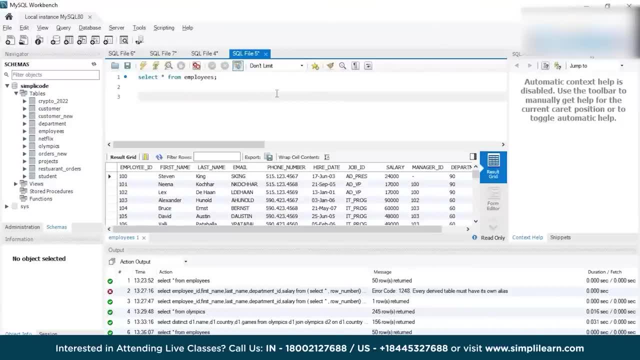 I know it is a bit confusing, so let us write the query so that we'll have a clear understanding again. So select, I'll just display all the records, So I'll use the select star operator. Select star from employee employees. 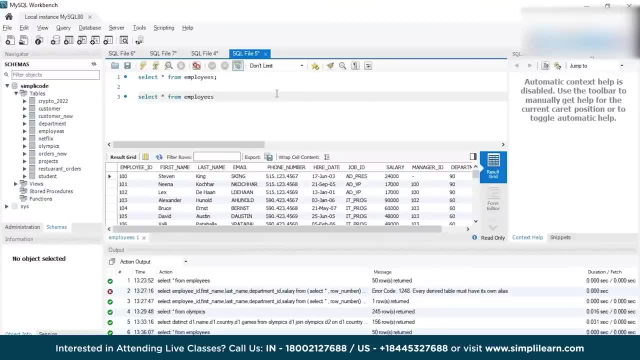 So we'll give an alias name, since it will take a lot of time writing employees each and every time, So I'm just taking it as E. Now we have to basically self-join, where it will compare the records from the same table. 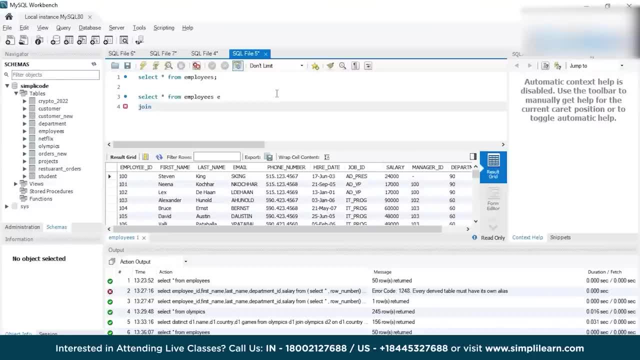 So I'm using the join table, So join statement again, and I'm using a sub-query and within the sub-query I'm basically selecting the records again, which is select star, and now we have to create, you know, the partition for maximum salary and minimum salary in our employee table. 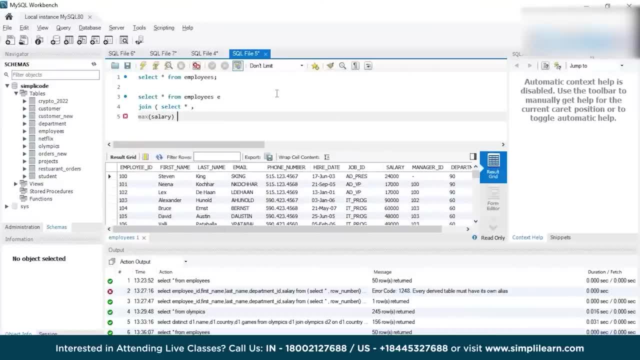 So create a partition which is maximum salary over partition by department ID Now, since we want the highest and lowest salary from each department, so I'm considering the department ID here. Now, since we are using the partition, we need to give a name for this. 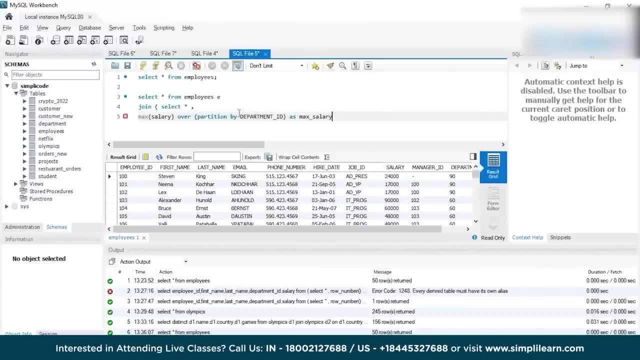 So we'll take it as max salary. And similarly you have to create, you know, minimum salary partition as well. The syntax remains same, guys Just mention it. So partition by again department ID: This will be minimum salary, all right. 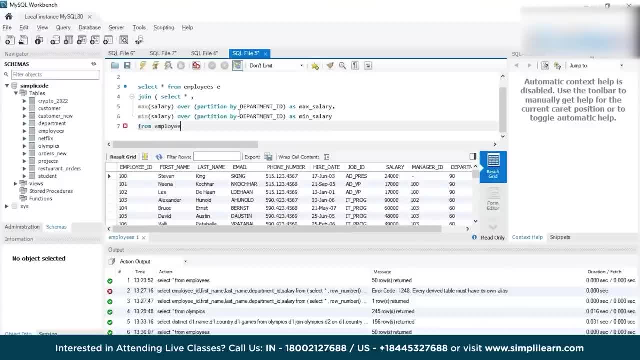 From the table, which is employees. Now, since this is a sub-query and it is a derived table, we need to give a layer's name for this table as well. So we'll just take it as X And since we have used the join, we have to mention the join on which. 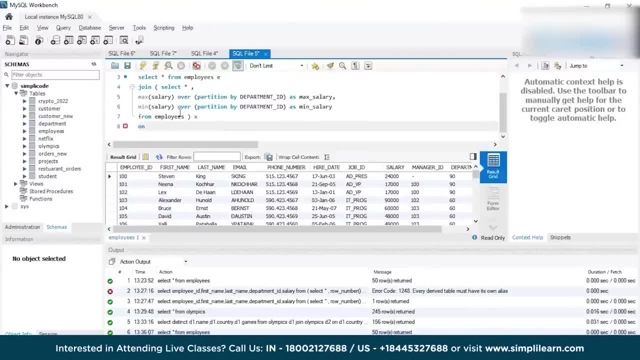 table we have performed, which is basically a self-join on the employee table itself. So E dot, employee ID, which is basically the primary key which has, which will uniquely, you know, identify all the records. So that's why I'm taking employee ID here. 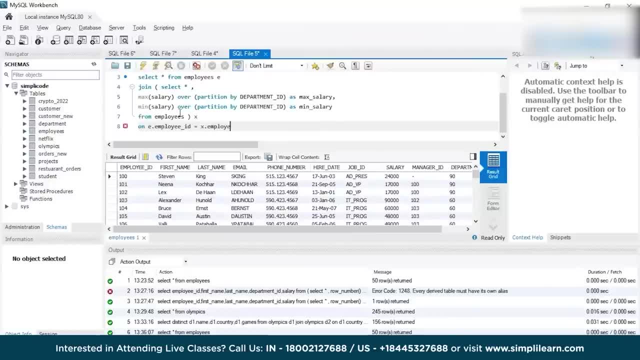 is equals to X dot employee ID. All right, And now mention the condition here. So the condition is basically it should match the salary with the maximum salary from the table that is employee, or it should match the salary with the minimum salary from the same table that is employee. 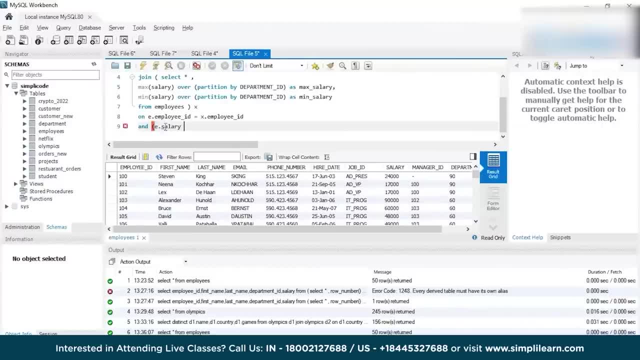 So I'll be taking E dot salary is equals to X dot maximum salary, All right. Or the condition can be: E dot salary equals to X dot maximum salary, All right, X dot minimum salary. So it would basically find all the you know details. 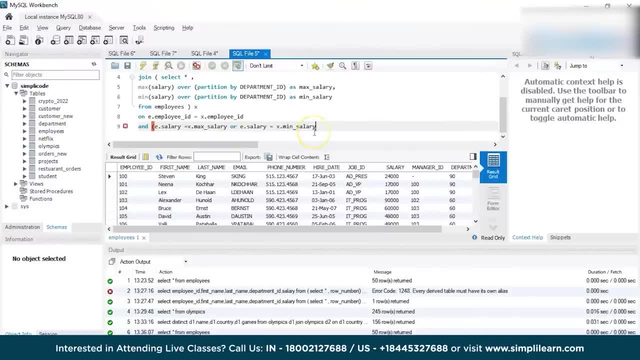 which has the salary which is either maximum or minimum. Right, That is it, And you can also use order by if you want to get in a, you know, particular order. So order by X dot, department ID, comma, X dot, let's say salary. 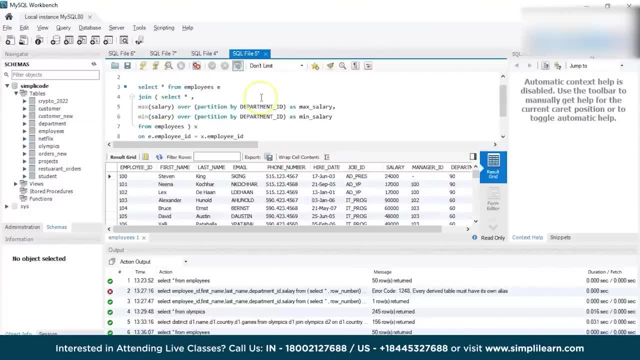 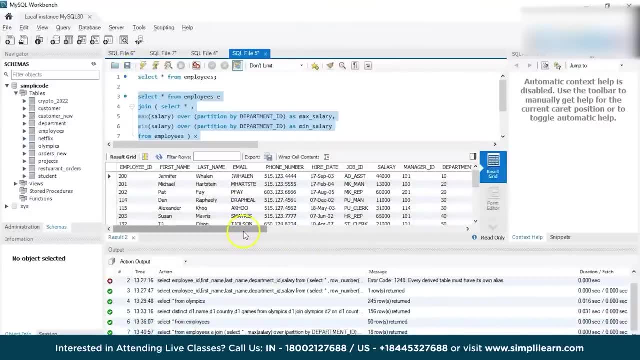 As well. All right, I think we do not have any error. We can just directly run the query and we will see the output. All right, Our query has been successfully executed and we have a total of 18 records, So let us just understand how the query has worked here. 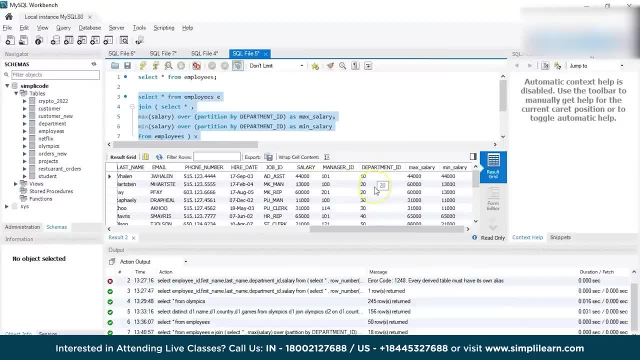 All right. Now we have various departments IDs that are being displayed in our resultant table. Now, if you look at the first department ID, which is 10,, the maximum salary is 44,000.. And the minimum salary is also 44,000 in this department. 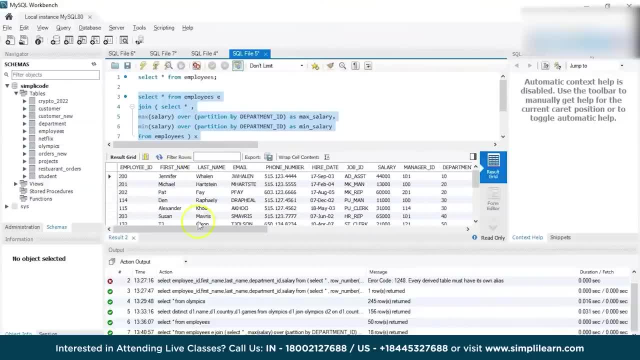 And the employee ID or the employee details, is Jennifer Valen. So let us just discuss another example here. So next let us move on to the department ID 20,, which has the maximum salary as 60,000 and minimum salary as 30,000.. 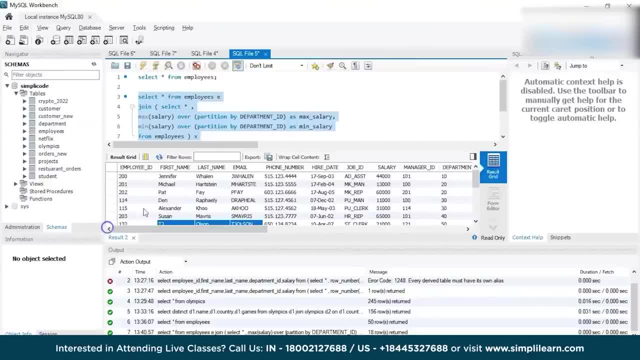 Now we have a total of two records here, That is basically Mike and Hashton, who is basically having the lowest salary in the department, who belongs to the department 20.. And we have Pat Fay whose salary is the highest, which is 60,000 in the department 20,. 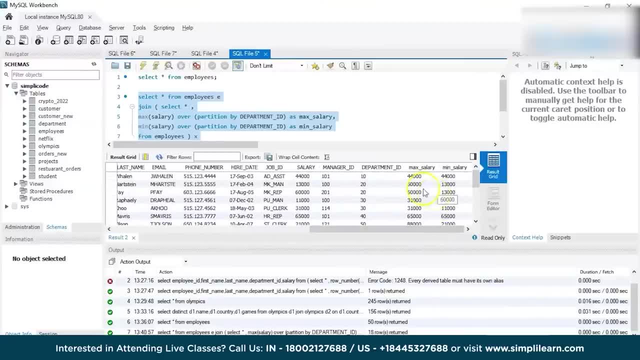 which is being displayed here in the separate section as maximum salary and minimum salary And so on. for the rest of the department IDs also, It will basically segregate all the details of the employees: who is having the maximum salary and the minimum salary? So I hope you have understood. 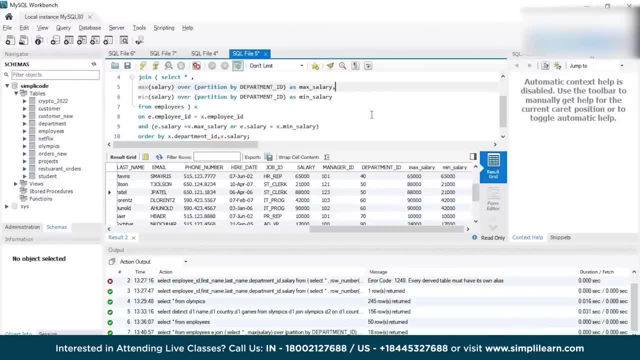 how to solve this query. This isn't, you know, rocket science, or you know having a lot of difficulty to solve the question. We have just basically used, you know, a self-join and a partition by statement. Now, partition by is basically an optional clause. 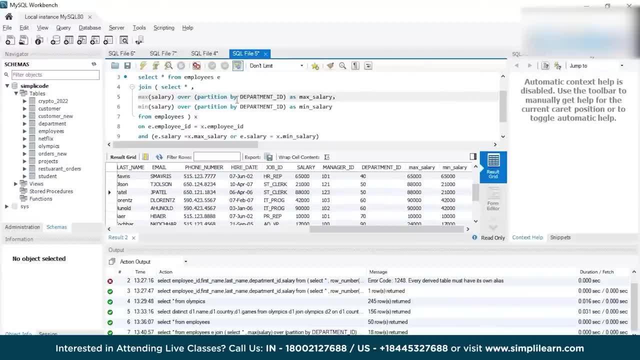 used in the row number function, basically, which is a clause that divides the resultant set into partitions, like you know, group of rows. Now, the partition which we have created is basically the maximum salary and the minimum salary Now, when this row number is applied to each partition. 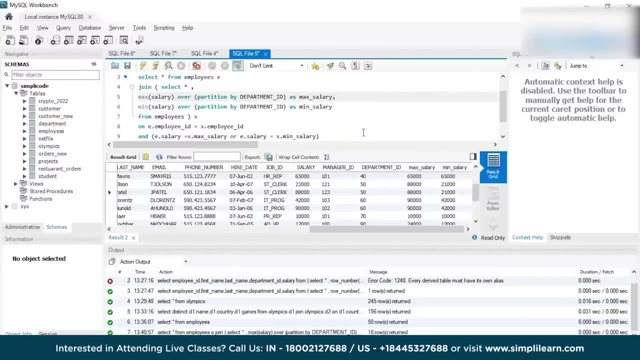 which assigns a separate rank number to each partition right. So in the same way, we can see that you know, different salaries are being assigned to the maximum salary partition that we have created. All right, let us now move on to our next query. 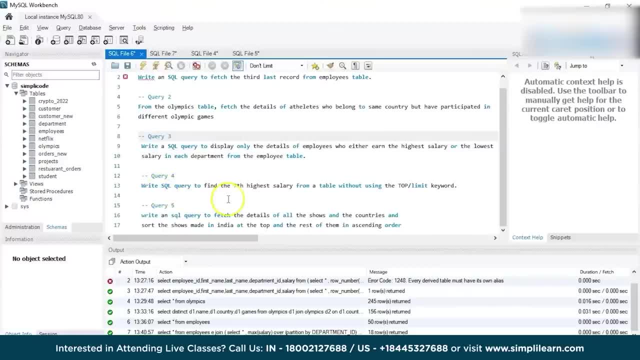 which is our query. four, which says write SQL query to find the seventh highest salary from a table without using the top or limit keyword. Now, this is one of the most common SQL. you know interview questions is to find the nth highest salary of employees. 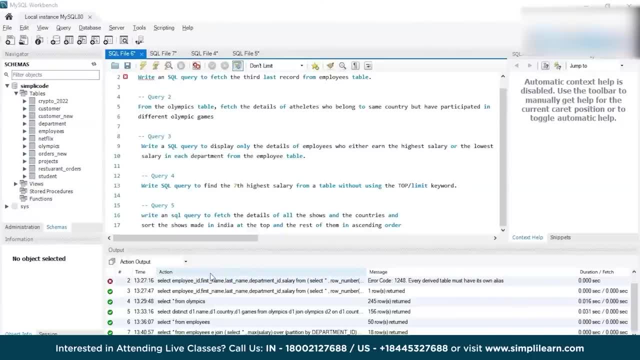 where n could be anything like 3,, 4,, 7,, 13,, anything you know, based on number of records that the interviewer wants to know, Like in order to find the, let us say, 13th highest salary in SQL. 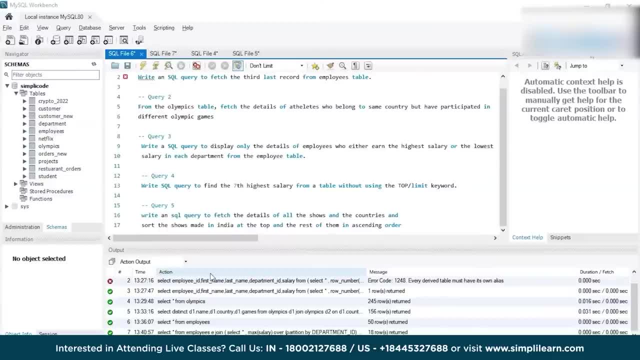 sometimes this question is also twisted to find the nth minimum or nth highest maximum salary in SQL. Now, since many programmers only know, the easiest way to solve the problem is using the top or the limit keyword, which will directly fetch the maximum salary, that is the records. 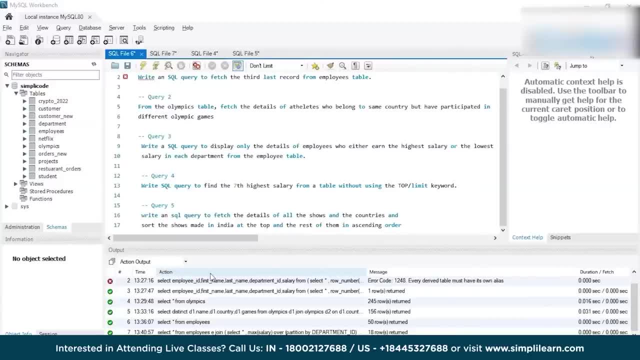 Now what if the interviewer wants to know another? you know case to solve this problem. So in that situation, what you will do? You cannot use the top or limit keyword for that, So basically we use the row number function. 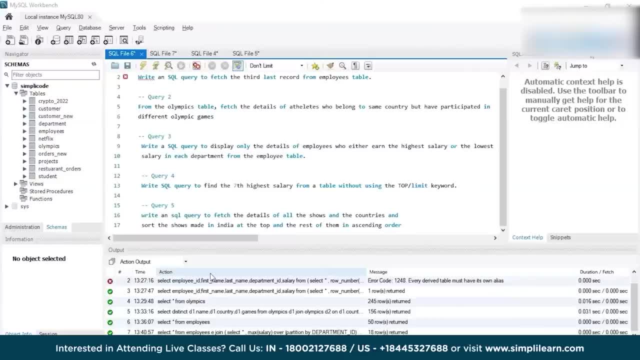 or the rank or dense rank function to find the nth highest salary, to find the highest salary from the table. But in this case we shouldn't use all those and even the top and limit keyword. So let us now see how to you know. 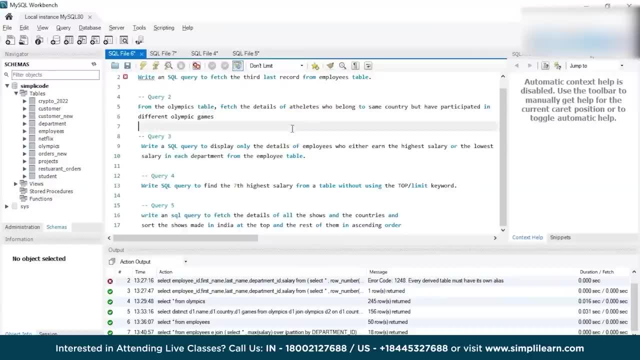 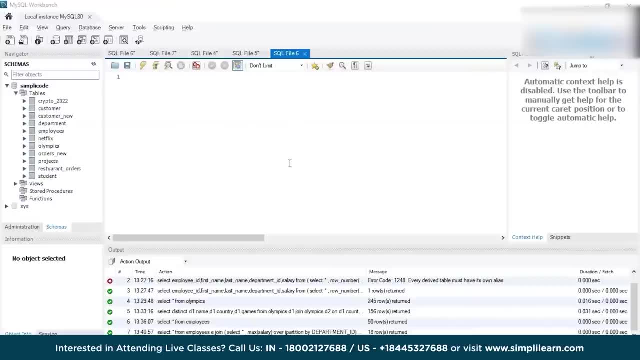 write this query, So let me again use a new tab. Now, in order to find the nth maximum salary from the employee table, we have to use a correlated subquery. Now the question that is asked is to find the 7th highest salary from the employee table. 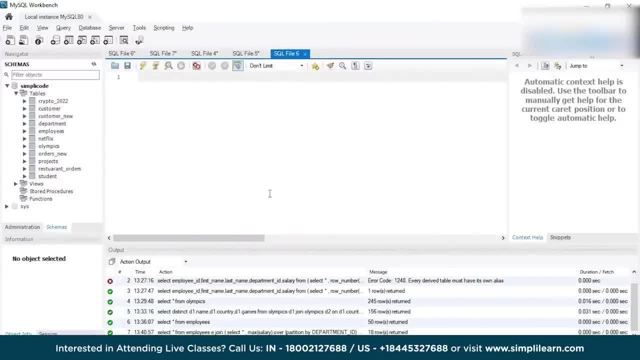 So, basically, a correlated subquery is a special type of subquery where the subquery depends upon the main query and executes for each and every row returned by the main query. Now, the only drawback of this is that it is a bit slow, but it can solve the problems. 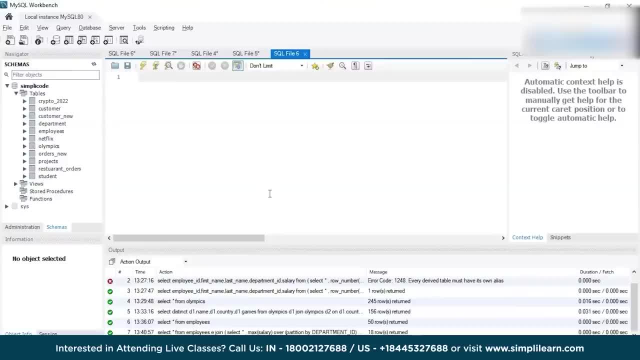 which are difficult to solve. For example, like to find the 15th, 20th, 100th, like in 1000th, you know, highest salary from the employee table. So let us now write the query so that we'll have a clear understanding again. 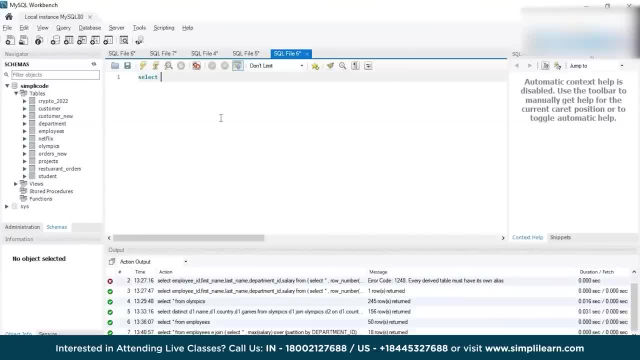 So the query is followed as select. So basically, first let us, you know, find the 7th highest salary. for that I'll be using the maximum Select max salary from the employees table. Sorry guys, there was a mistake. 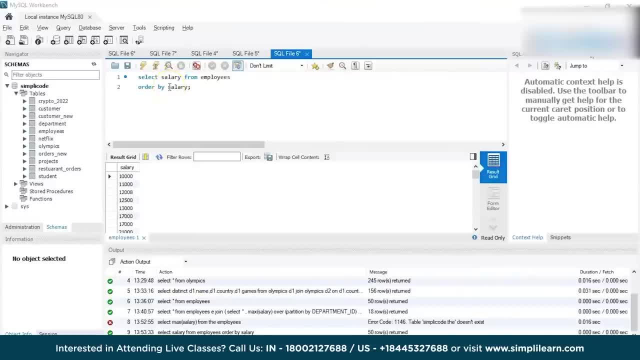 We shouldn't need the maximum salary, We just need the salaries, and in the order of which they are separated. So order by salary, in descending order, that is, from highest to lowest, We'll be sorting them right. So let me just execute this query. 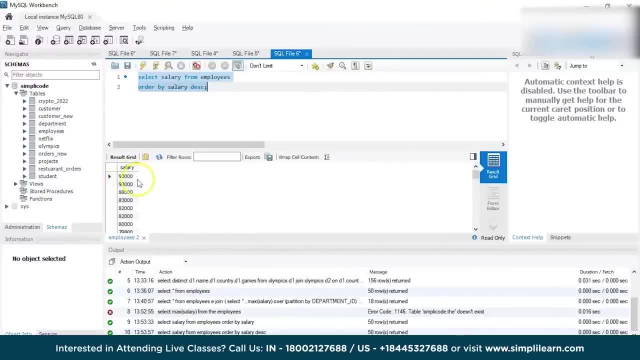 So the highest salary in our table is 93,000 and the second highest salary is 90,000.. So the query that was asked for is to find the 7th highest salary, That is, 1,, 2,, 3,, 4,, 5,, 6 and 7.. 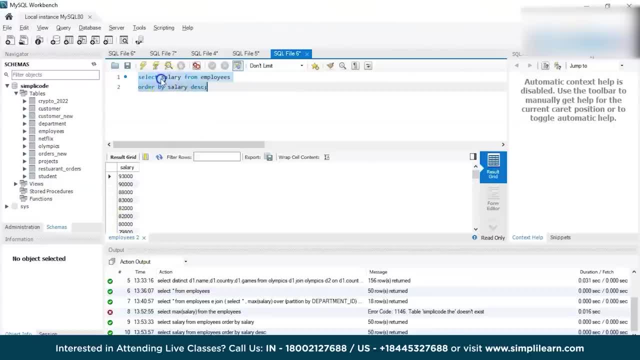 So 80,000.. Okay, we have repeated values, So we'll just use the distinct keyword as well, So that we'll have unique records. All right, So 1, 2, 3, 4, 5, 6, 7.. 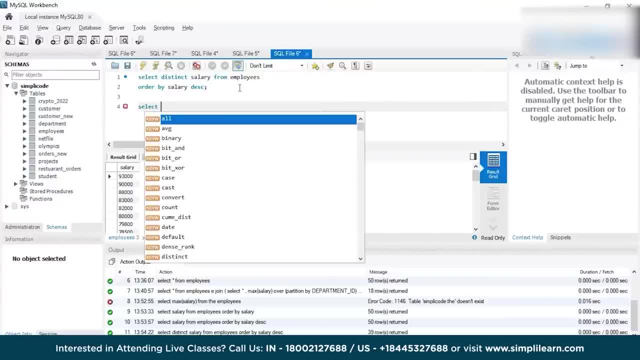 as select, you know, star from employee employees. Let us take it as even- since we will be, you know, comparing the same table where n minus 1. I'll explain in the, at the last, why we are using n minus 1 here, guys. 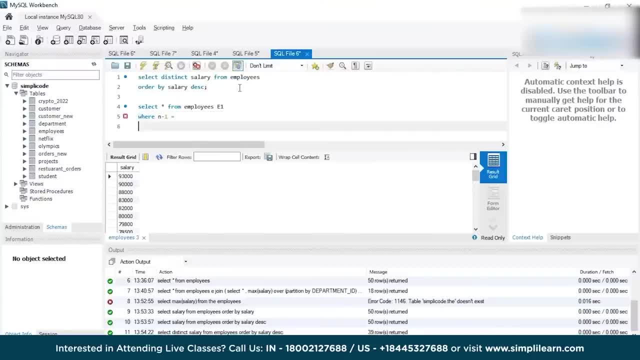 So let's just continue with the query. Now we have to write a correlated sub query- just we've discussed earlier- which is basically select count, distinct salary. So I'm using distinct E2 dot salary. Basically we are comparing the same table. 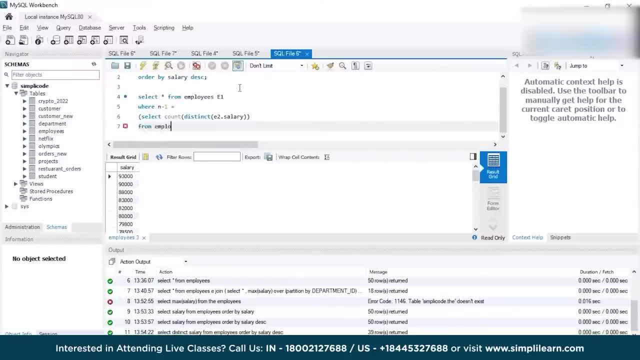 once again from employees E2 where mention the condition on which you want to perform. you know the separation. Now we need to find the highest salary right. So the salary in second table, that is, E2 dot salary, should be greater than. 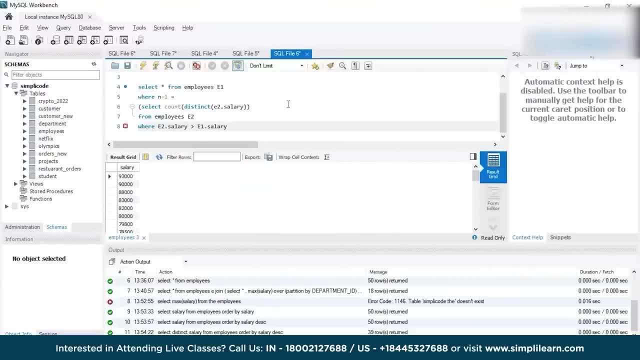 E1 dot salary. So this is what the query exactly is, guys. So let us just understand how you know how this query is working here. So, as I said, the distinct keyword is there in order to deal with any duplicate records. 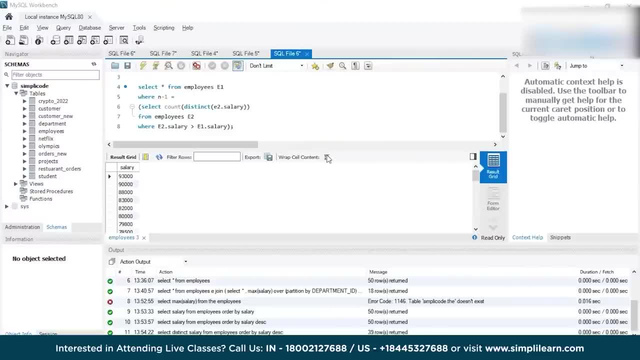 or the salaries that are present in the table. So in order to find the nth highest salary, which is basically, we need to find the seventh highest salary. right, We are only considering the unique salaries here, and the highest salary means no salary should be higher than it. 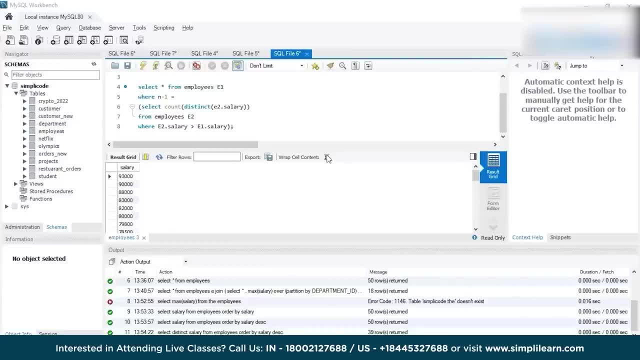 For example, if the second highest salary means only one salary is higher than it, that is the first salary. Similarly, the third highest means no two salaries are higher than the first two salaries. Similarly, for the seventh highest salaries you can say there are n minus one salaries. 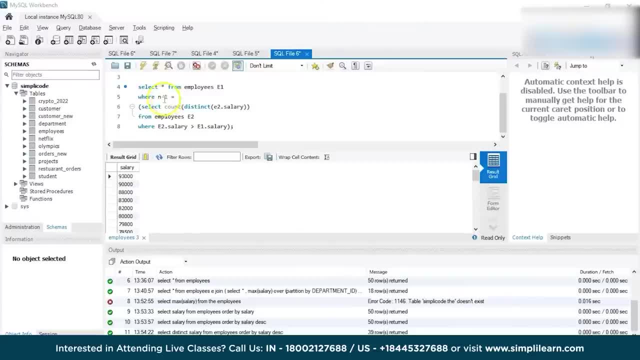 that are higher than it. So, for example, if I am taking seventh salary, so n basically becomes seven. So seven minus one is basically six, Right, So which is finding the seventh highest salary from the table. So let us just execute this and we will see the output. 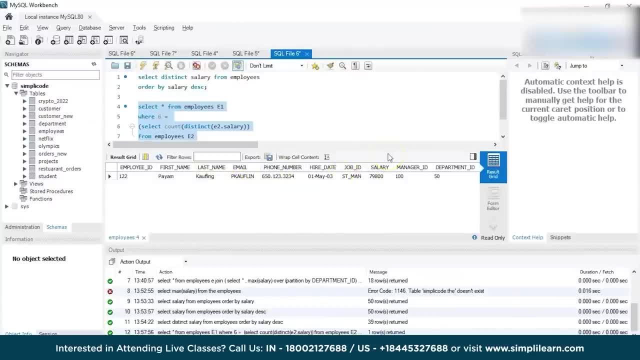 So, as you can see the seventh highest salary, that we have already seen the output table, which should have 79,800, as a resultant table and it is showcasing all the details of the employees. who is having the seventh highest salary? who is Payam Coughlin, whose. 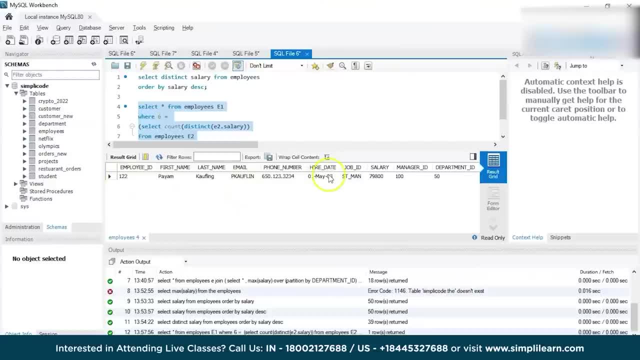 employee ID is 122, whose email is P Coughlin. his hiring date, his job ID and the rest of the details are being displayed. So in this way you can find the seventh highest salary from the employees table. So this is basically a generic solution. 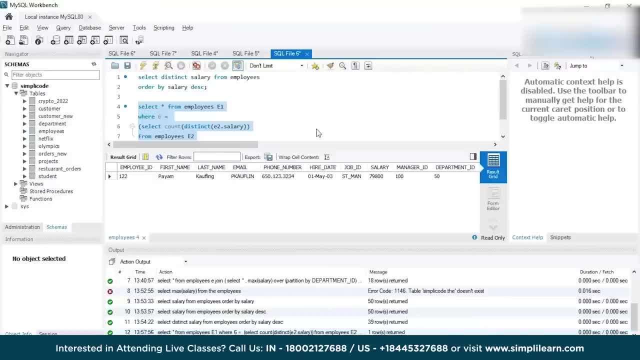 which works in all databases, including MySQL, Oracle database, SQL, PostgreSQL, and the only drawback, as I said earlier, is it is slow because the inner query will run for every row possessed by the outer query. So do let us know in the comment section below what all different methods 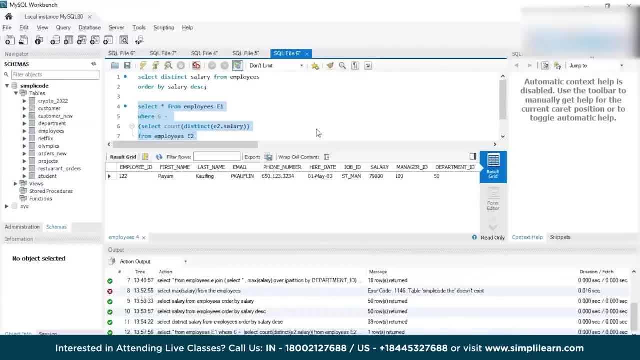 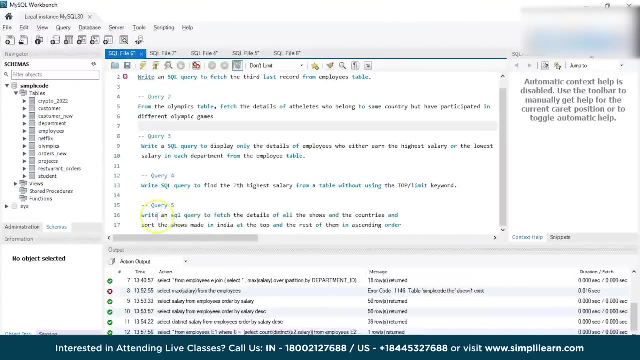 we can use for this same query, and we also have a dedicated video on how to find the nth highest salary using various keywords, like the top limit, using dense rank functions, So you can check that out as well. So, moving on to the final question, guys. 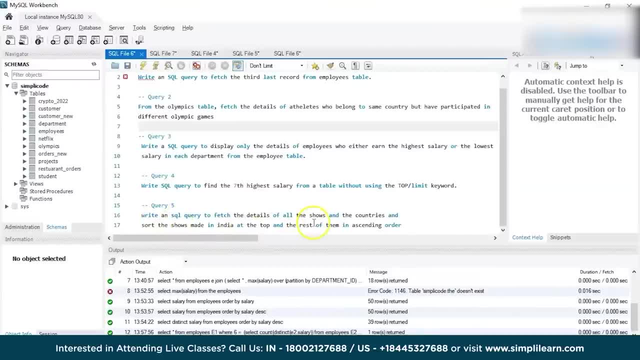 So the final question is write an SQL query to fetch the details of all the shows and the countries and sort the shows made in India at the top and the rest of them in ascending order. I think this is from Netflix table, So from the Netflix table. So let us just 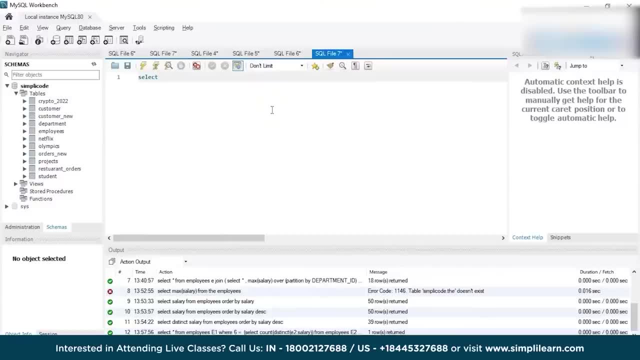 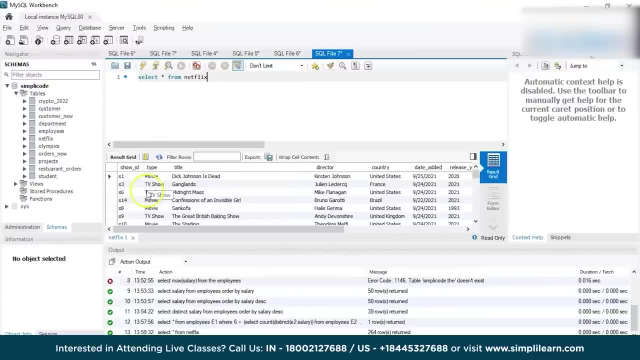 retrieve the details first and we will see how the query works. Select star from Netflix. Alright, So the Netflix table has the show: id, title, director, country, date added release year, rating duration, genre. So let us. 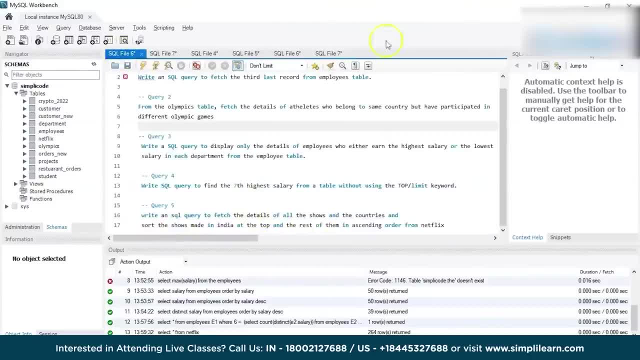 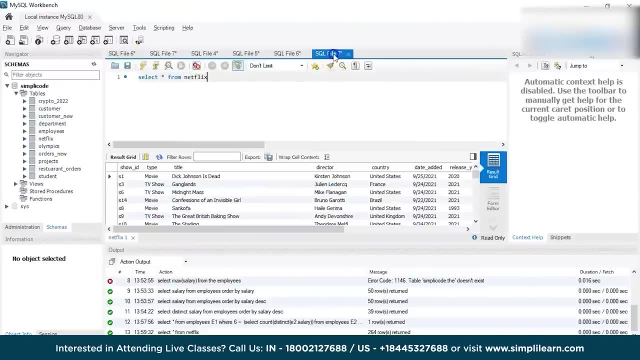 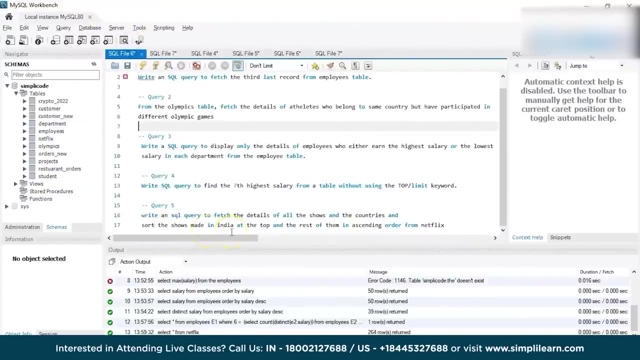 go through the query again. It says that we need to fetch the details of all the shows. That is basically the title. These are the show names and the countries. We have the countries also which they are made in and sort the shows that are made in India. 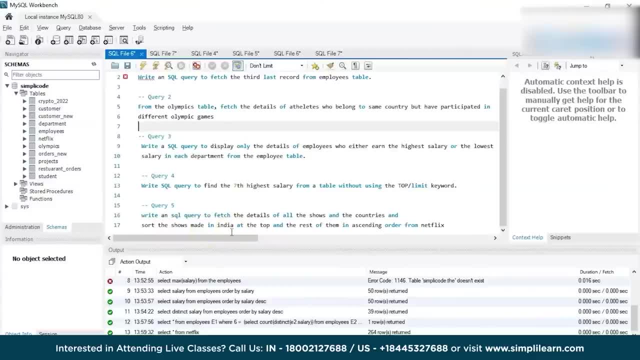 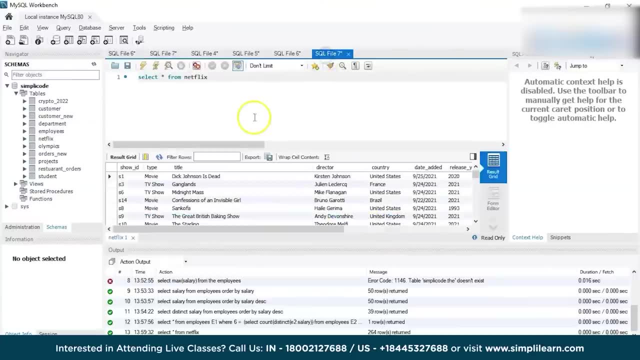 at the top. That is, we need to display all the shows that were made in India at the top level and the rest of them in ascending order from the Netflix table. So I hope the question is clear, guys. So let us now write the query. 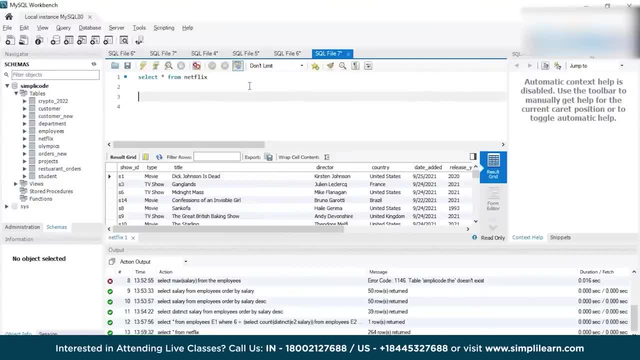 Alright, Since we are only concerned with the show name, that is, the title and the country, we will just select those. Now we may have the titles repeated, So I am just taking the distinct values. Distinct title, comma, country from Netflix. 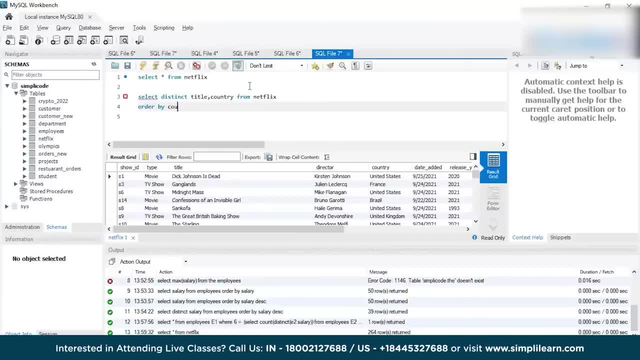 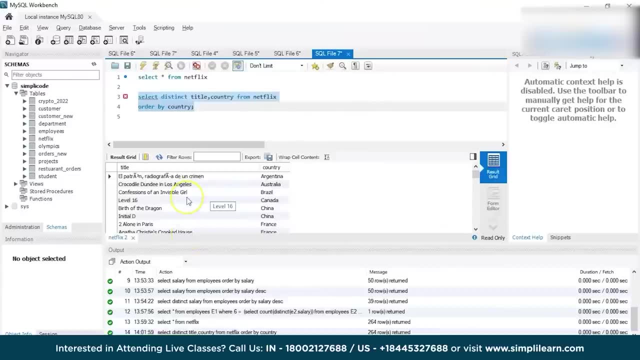 And we will basically order by country first and we will see how the output is Alright. So it basically displays all the details of all the shows that were made by different countries. For example, you can see El Patron Radrigo de Uncrimen. 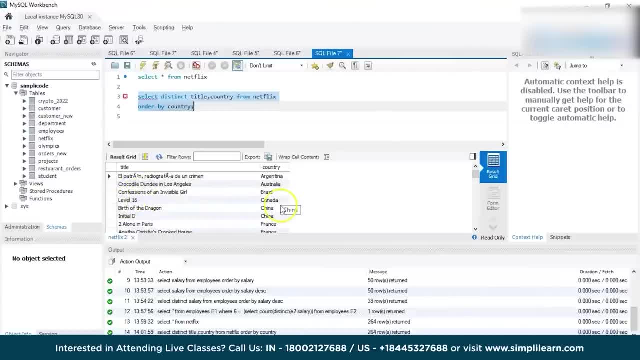 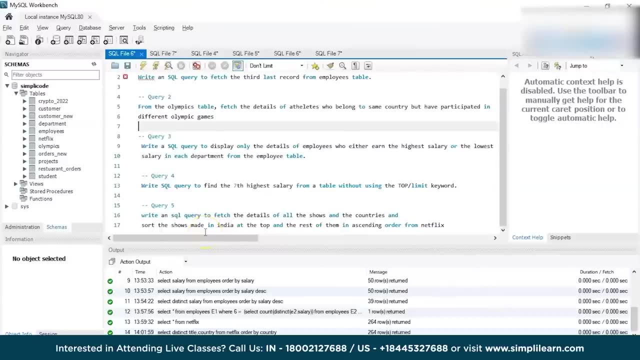 has been made from Argentina. We have level 16 from Canada. So the query that was asked is: we need to sort the shows made in India at the top and rest of all the shows in ascending order. So basically we need to have 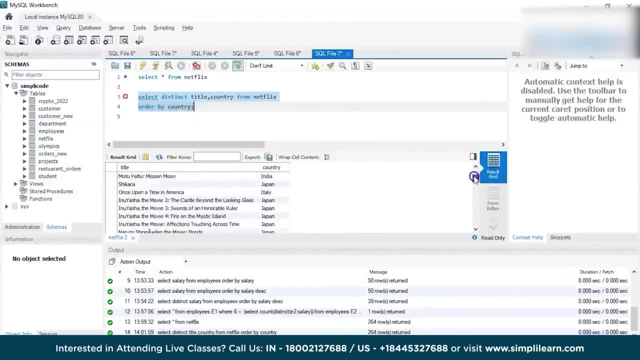 the show names that are in India. So let me just check, We have. So yeah, right, We have certain shows that were made in India as well. So you can see there are list of so many records of all the shows For. 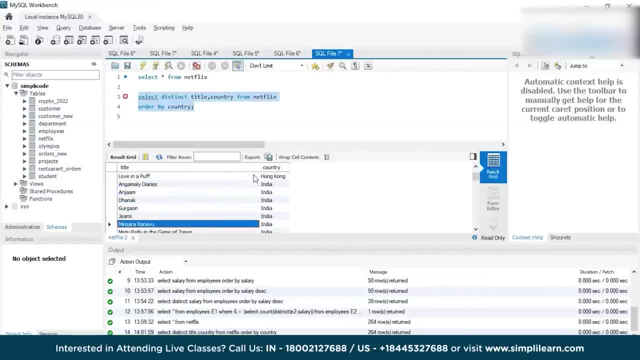 example, Angamaly Diaries, Anjam Dhanak, Gurgaon Jeans, Minasara, Kanavu and so many others. So basically, in a resultant set, we want all the details of all the shows to be at the top and 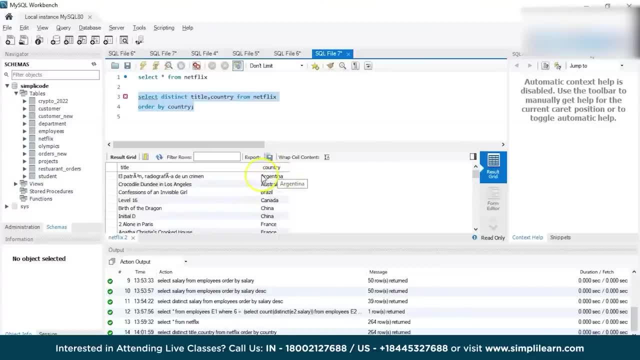 the rest of them in the ascending order, like, for example, Australia, and then we need Brazil and then Canada and similarly France, So basically in the alphabetical order. So the logical approach for this is using the case expression. guys, Now that is the. 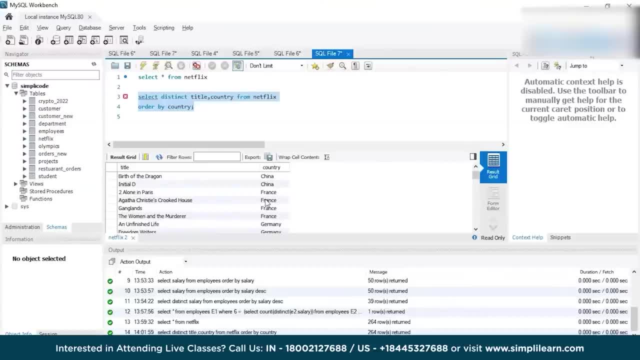 tricky part, where you know the interviewer wants to know whether you are familiar with this concept of case expressions. So basically, the case expression goes through the conditions and return a value when the first condition is met, Just like an if and else statement you use for other programming. 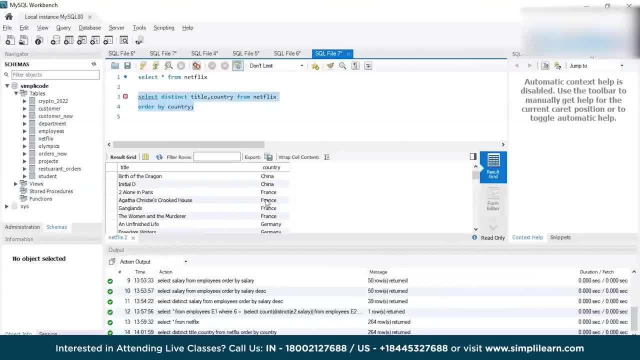 languages like C, C++. So once the condition is true, it will stop reading and return the result, And if no conditions are true, it returns the values in the else clause. So basically we need to mention the case condition here. 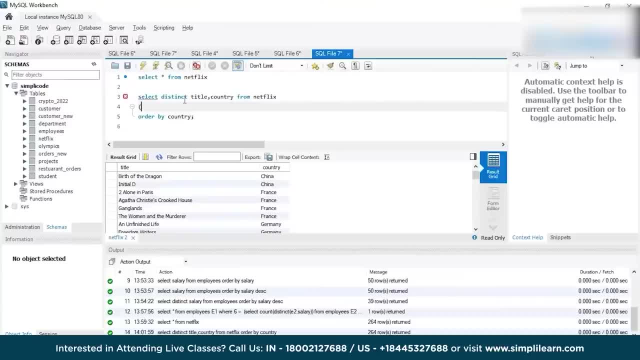 Alright, So the query is followed as So mention the case keyword. The syntax is followed in this way, which is case when country is equals to India, then return 0. That is basically return the true values. if there is any record or the 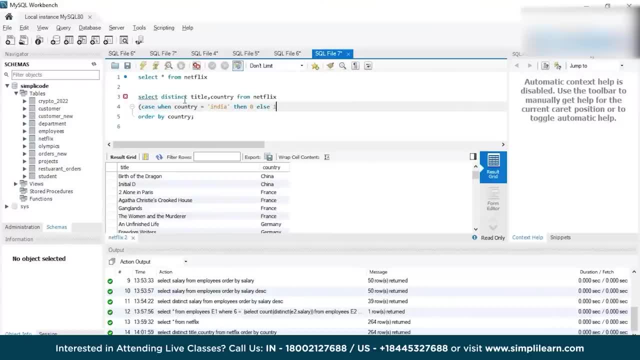 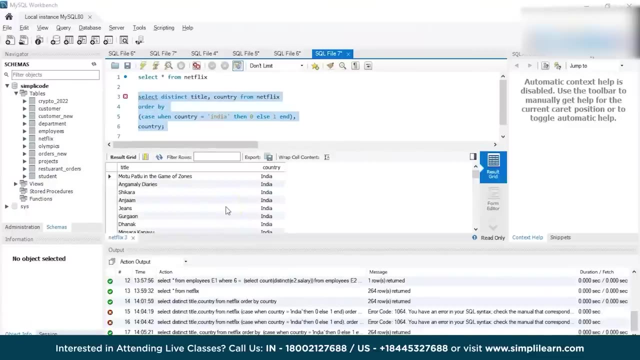 title name having India, else we will mention it as 1.. And finally, we will end this statement, which is again the keyword we have to use for case expression. Alright, So let us now just implement this and we will see the output. So there was a. 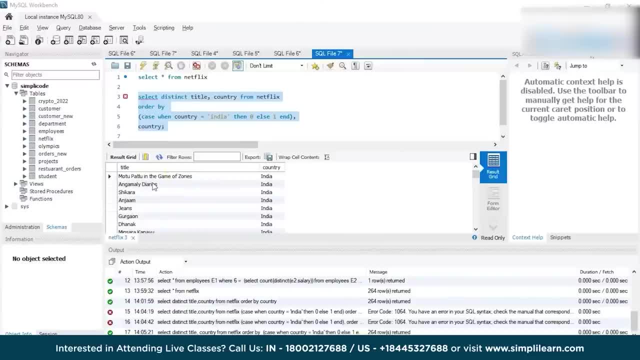 minor error, guys. So, as you can see, in the resultant set we have the details of all the shows that were made in India. that is being displayed at the top. As you can see, we have all the list of all the shows of India and 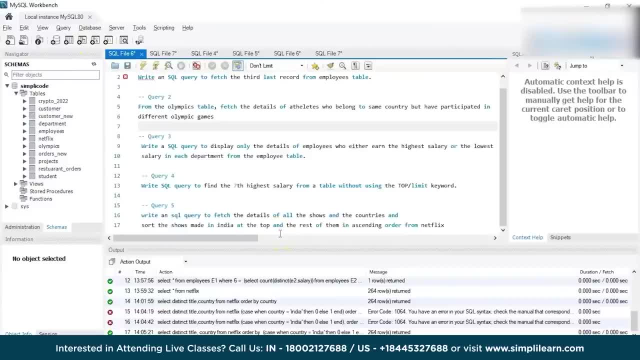 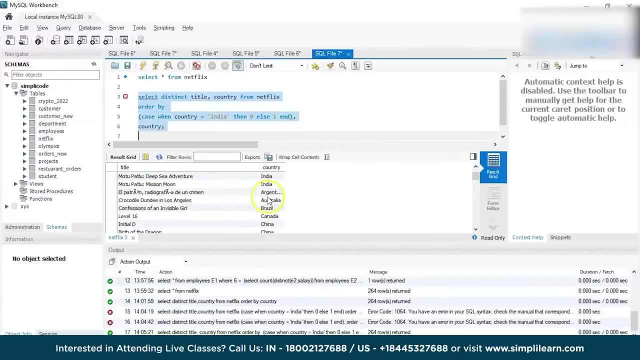 then after that, the query states that we need to sort the rest of the or the remaining shows that were made from different countries in ascending order. As you can see, just like we have discussed earlier, the country names have been sorted in ascending order, like Argentina. 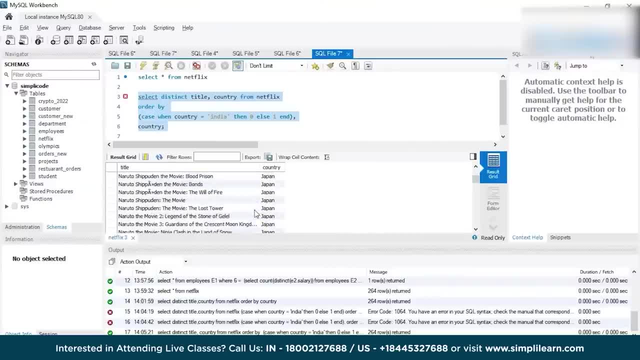 Austria, Brazil, Canada, China, Italy, Japan, Nigeria and so on. Pakistan, United States, Right, So United States is the last country which is being sorted in the alphabetical order. Now the same question can be asked, you know, when we have multiple. 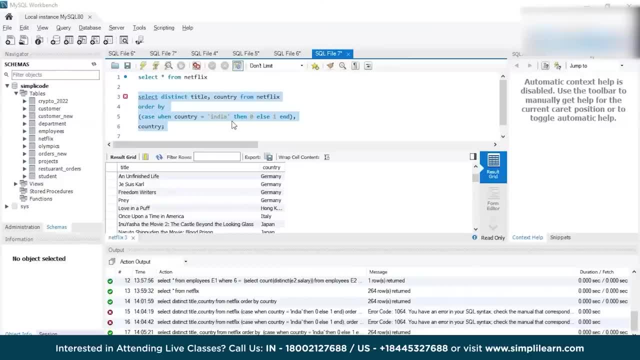 conditions to specify Now, for example, if I want all the shows that were made in India, as well as Germany, to be at the top and the rest of the remaining shows from different countries to be sorted in the ascending order, after the shows that were made in. 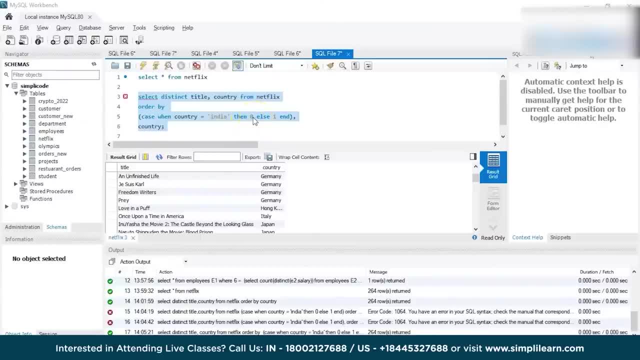 India and Germany. So in that case, the query just remains the same. you just need to add another condition Now. first, which is case, and country is equals to India, then 0. Next, the condition will be case. I don't think we need to write the case. 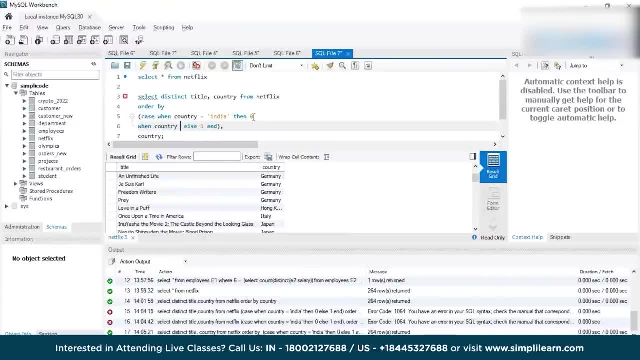 again and again, when country equals to Germany, Germany, then we will specify it as 1.. So if there is no country that is having shows other than India and Germany, so we will be basically we will mention it as 2 and we are ending the statement. 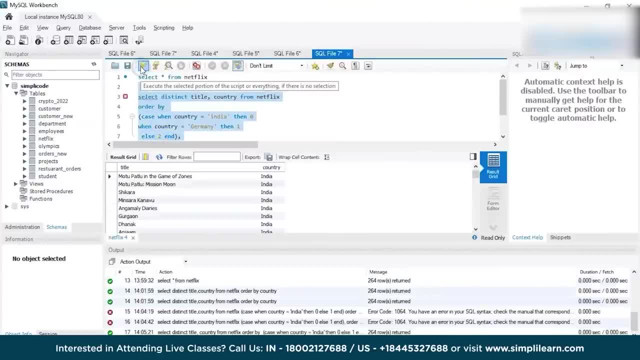 So let us just execute this query and we will see the output. So, as you can see in a resultants query, the firstly we have the case condition, which will retrieve all the details of the shows that were made in India. as you can see in a 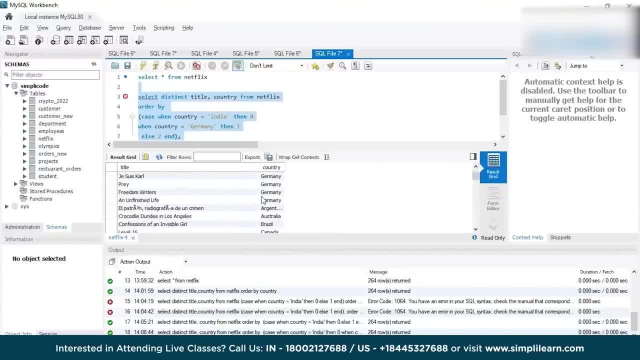 resultant set and after that we need to have the shows that were made in Germany. So, since we have mentioned the country as Germany, it is being displayed as Germany. that is, the titles or the shows that were made in Germany, and the rest of the remaining 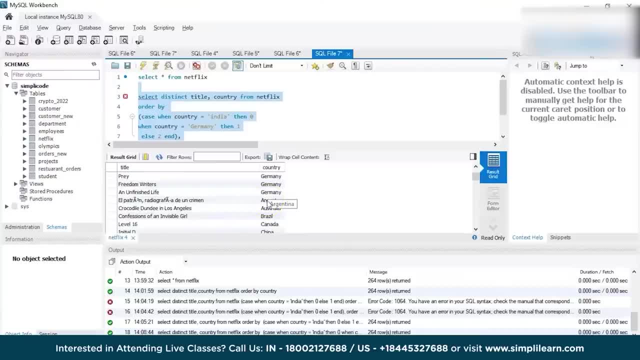 shows that were that belongs to other countries and we need to sort them in ascending order, in the form of the alphabetical orders, like Argentina, Australia, Brazil and so on. So this query is asked in general, you know when you want to give certain records a priority. 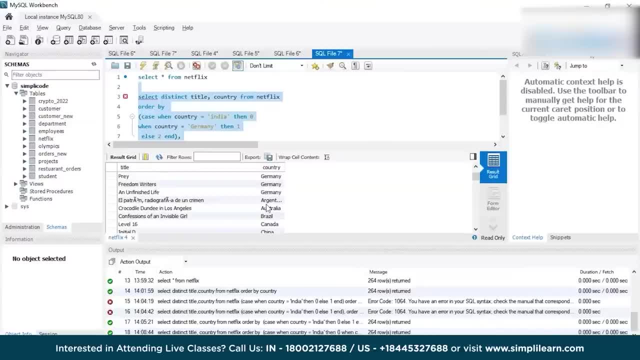 that is you want to mention. you know you want to display certain records at the top and the remaining at the bottom, So in that case this query will be useful, which can be done using a case expression. And with that we have come to the end of today's session. 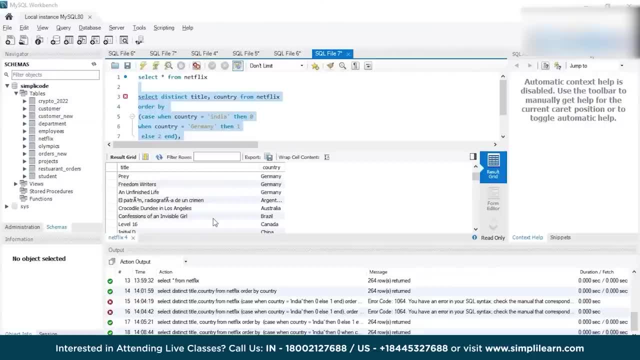 guys. These were some of the top 5. you know SQL interview question and answers. that would have given you an insight into what kind of questions could be asked in your next interview and you need to be prepared for it as well. As discussed earlier, not just the theoretical questions- 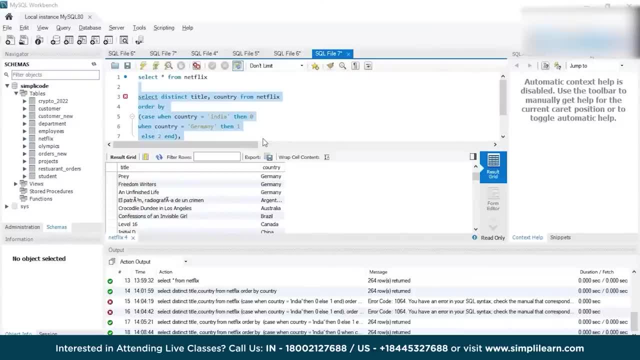 you need to be prepared for the real time SQL queries where you have to write the queries. you know exact queries, so in that case you have to be prepared for that as well. So in this session we only covered- you know- the difficulty level, from easy to moderate level. So